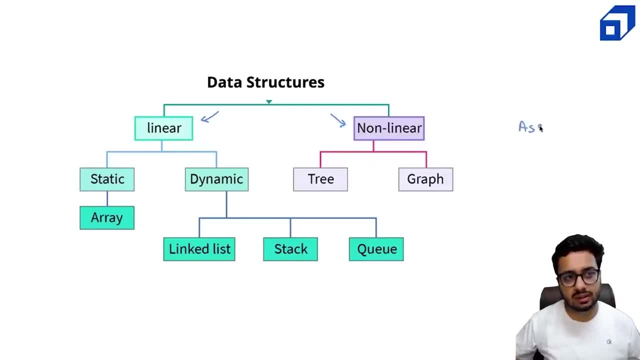 data structures. There is one more category I would say. we have associative data structures in which we store data in the form of Key value pairs, for example your hash maps- We will talk about hash maps later in this course- Those linear data structures. they can be a fixed size, like a fixed size array. 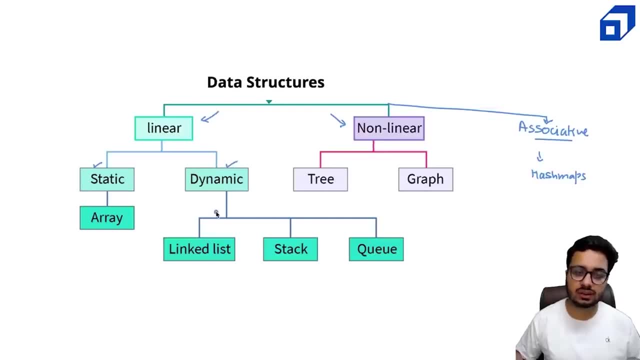 or they can be dynamic. That means they can grow and shrink in size, For example, your array list, your linked list, your stack, your queue. In non-linear data structures, we might have data structures which have a hierarchical structure, For example, your. 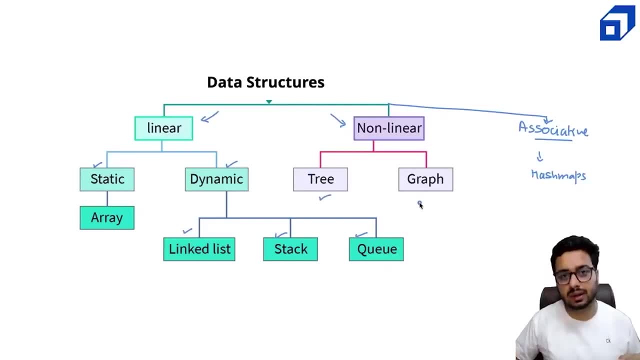 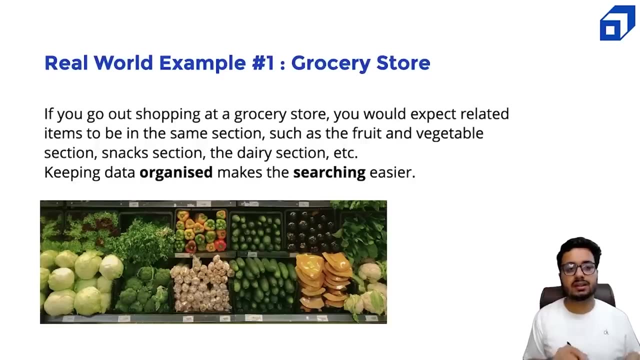 trees Also have data structures, which have network data structure, For example. this is a very high level overview of how data structures are classified. But let us start by revisiting the importance of data structures in our real life. So suppose you go to a grocery store and you find everything is disorganized. then 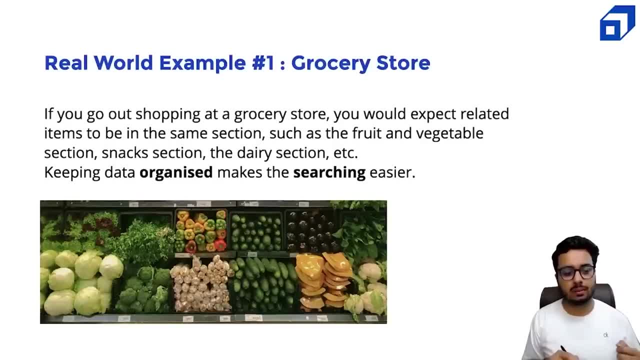 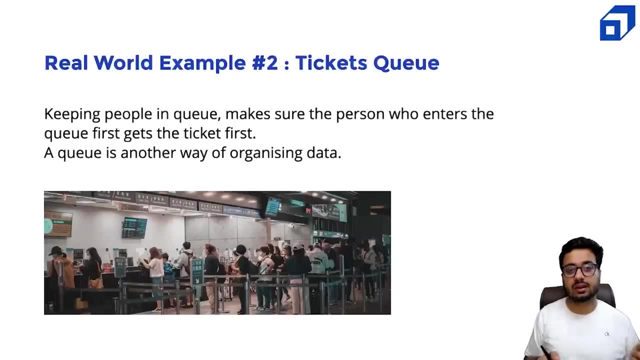 it would become very difficult for you to search for a given item, But if your items are organized across racks and categories, you will easily find a particular item that you're looking for right. Similarly, if you go to tickets and if there is no queue, then it would be very unfair. 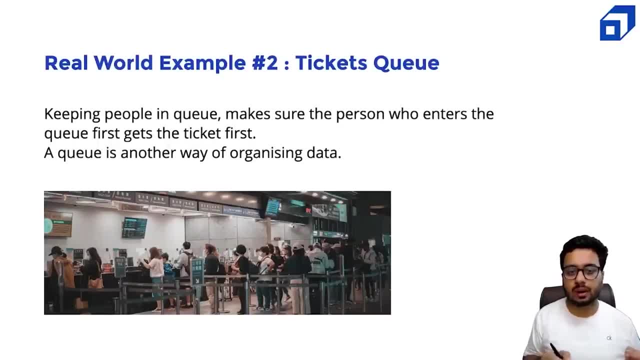 for the people to wait randomly. But if people are organized on the basis of their priority, the person who is coming first and he is getting the queue ticket first, then it is called as FIFO ordering. Similarly, in data we might require FIFO ordering, So queue is a data. 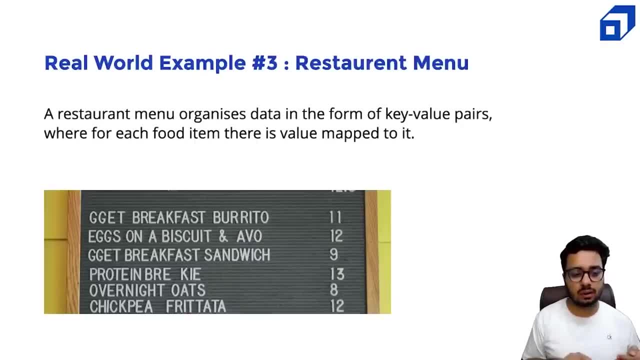 structure that provides us with this kind of ordering. And let us look at one more example. Sometimes I go to a restaurant and I say: okay, I want to order a burger. Then I quickly get an answer that the burger cost is rupees hundred. What? 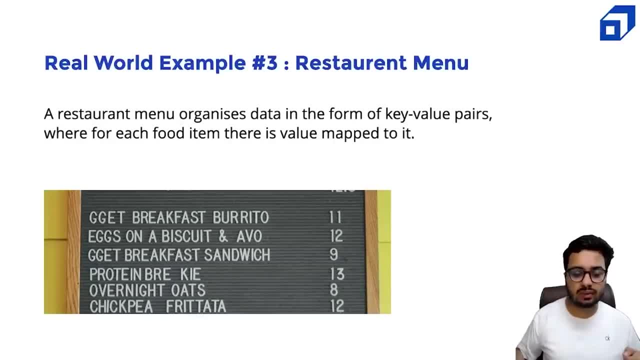 is happening. For every item, there is a value attached to it, right, So for every key, there is a value, right So the data can might be stored in the form of key value pairs, And this is where some other data searches, like hash maps, come into the picture, right Another. 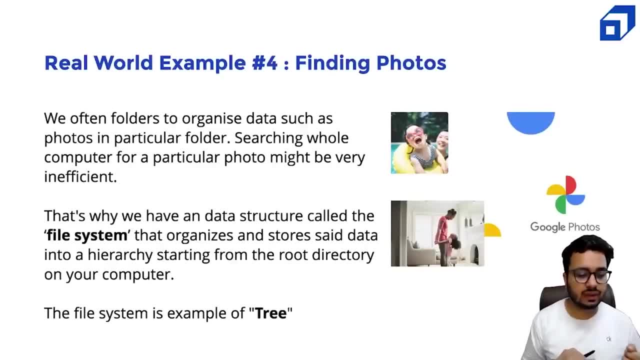 example could be that if I'm on my system and I'm locating certain files right, I know that, okay, in this folder. I have kept this kind of a data in this folder. I have kept my PDFs in this folder, in this drive. I've kept my pictures, right. What is your file? 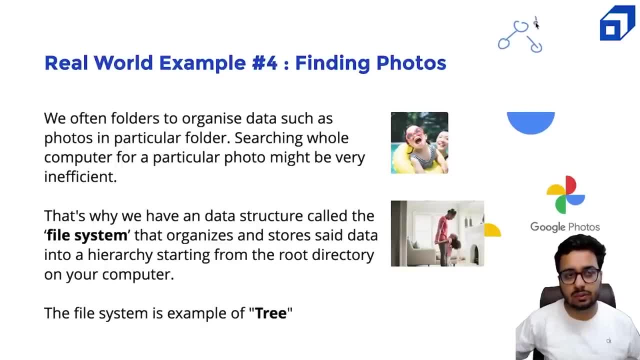 system. The file system is a tree-like structure. You start with your my computer, you go to your drive, then you go to certain folders and you find the files that you're looking for, right? You do not organize this data in the form of hierarchy, And if so, I'll search. 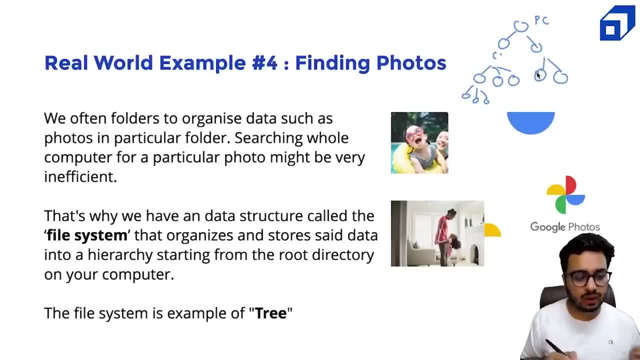 the whole computer. it would be very inefficient for you And you will spend a lot of time searching for a given file Right. The file system is also an example of a tree-like data structure. That means we use data structures a lot in our daily life in building software applications. So 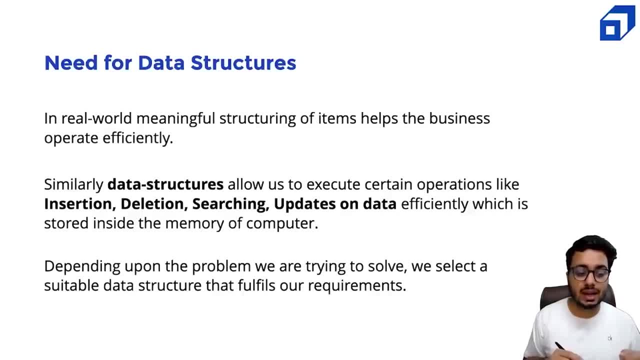 in real world also, the meaningful structuring of items helps businesses operate efficiently. We saw the example of grocery store, So, similarly, data structures allow us to execute certain operations like insertion, deletion, searching, updates on the data very efficiently, And this data is stored inside the memory of the computer. 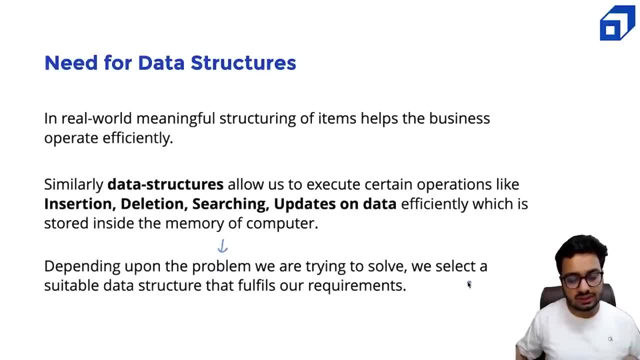 Okay, So, depending on the problem that we are trying to solve, we select a suitable data structure that fulfills our requirements. This is the goal of this video. In this lecture, we are going to understand how, according to different requirements, what data structure we will. 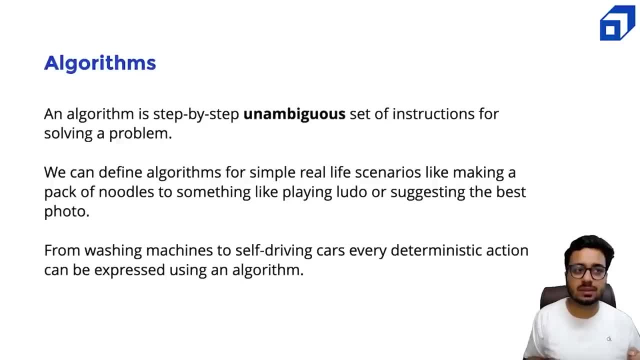 use and we will look at its implementation using Java collections framework. right, You might ask, okay, that's data structure. What is an algorithm then? Algorithm is the main logic. It is the step-by-step, unambiguous set of instructions for solving a problem. 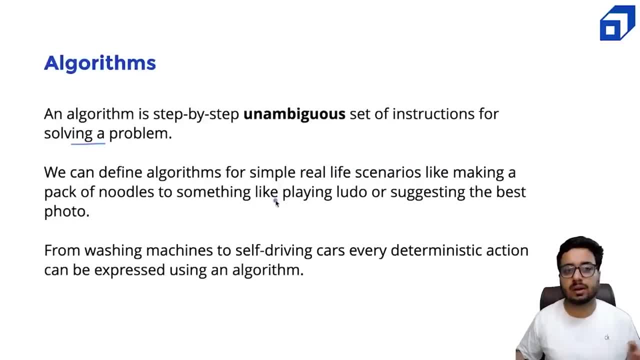 We can define algorithms for real life scenarios like making a pack of noodles. You might say, okay, take a pan, put two cups of water inside it, boil something. something That list of instructions is an algorithm to make a pack of noodles. or maybe something complex Like 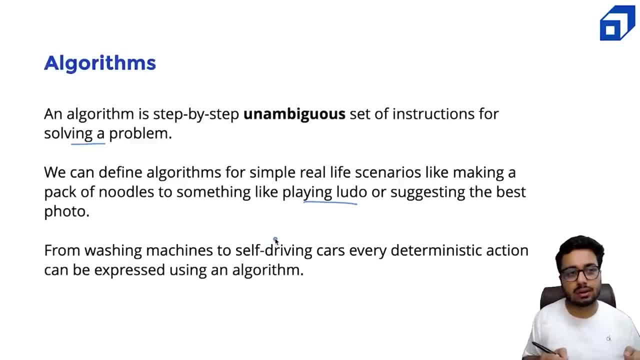 if we want to play a Ludo game or if I want to make an algorithm that suggests the best photo out of a set of photos, we can devise an algorithm for that. So in real world, from every, every deterministic action, for example, your washing machine, your washing machine. 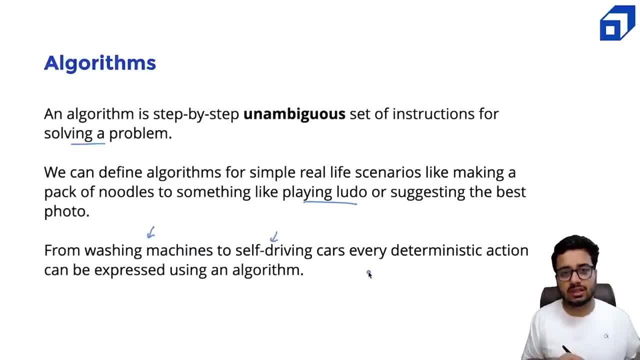 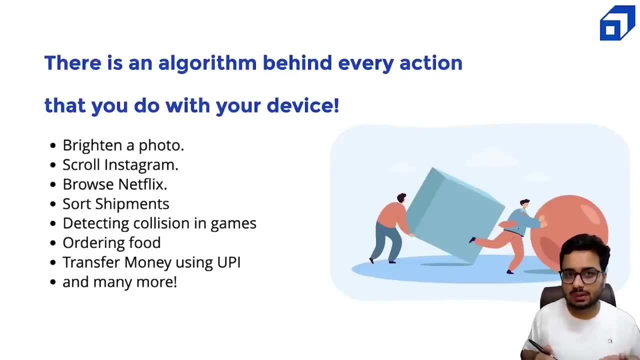 a self driving car. all the actions your machines are taking that can also be expressed using an algorithm In the software world. all the apps that you're using: photo editing, app scrolling, Instagram, browsing, Netflix in a cargo hub, sorting of shipments, detecting. 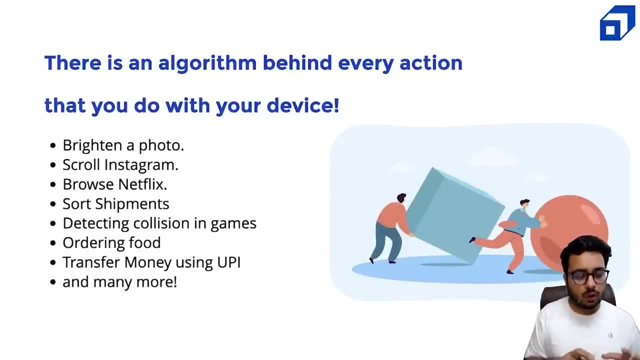 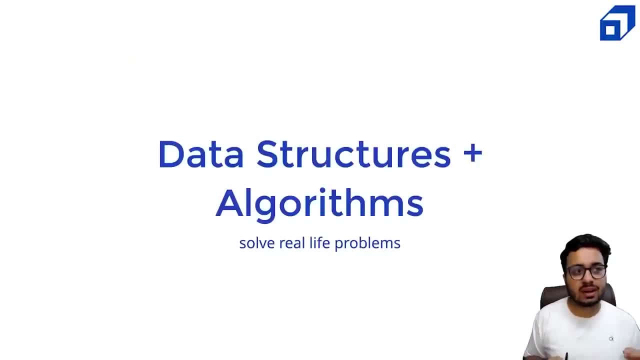 collisions in games, transferring money through UAPI, ordering food. There is an algorithm behind every action that we perform, So that is why it is very important for us to learn data structures and algorithms right, And when we combine data structures along with algorithms, we build products that can. 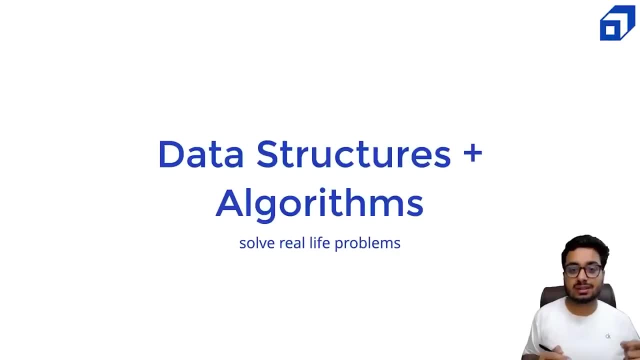 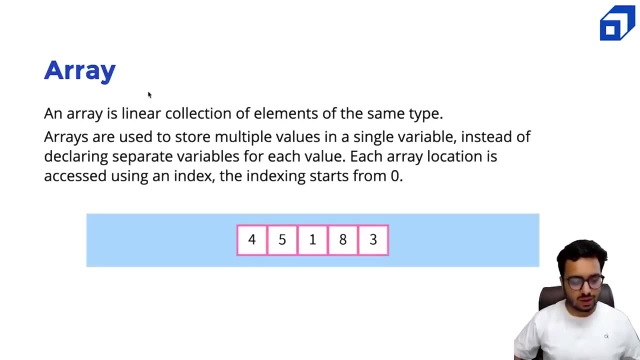 solve real life problems. That is an importance of data structures and algorithms. I will start with arrays. Let us start with the array, which is the simplest and the most widely used data structure. I'm hoping most of you have must have worked with an array. What? 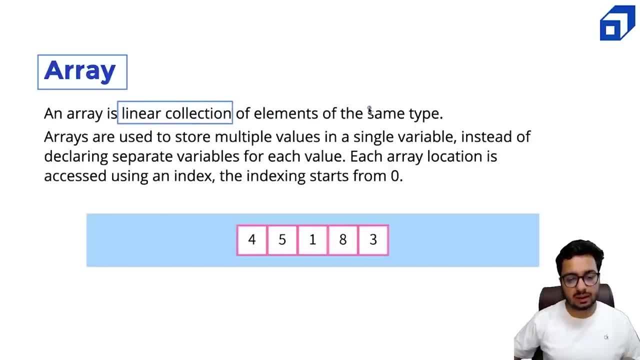 is an array. Array is a linear collection of elements of the same type. So this is true for Java- Other languages like Python. they also support heterogeneous arrays. That means you can put different arrays of different types of data, So you can put different arrays. 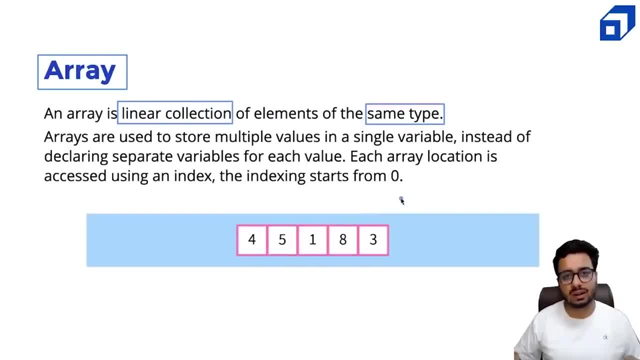 you can put different arrays of different types of data, So you can put different arrays. you can put different arrays of different types of data, So you can put different arrays of different types of data, For example, integer string float inside one array Arrays. 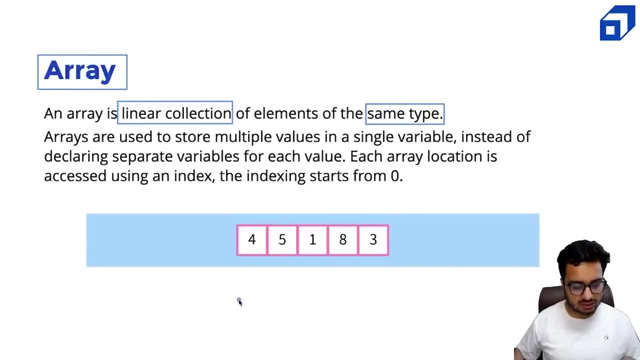 are used to store multiple values in a single variable. So let's say this is a container which is linear. That means it will occupy linear block of memory. For example, if this address is 104 and this bucket takes four bytes, the next address will be 108.. Next. 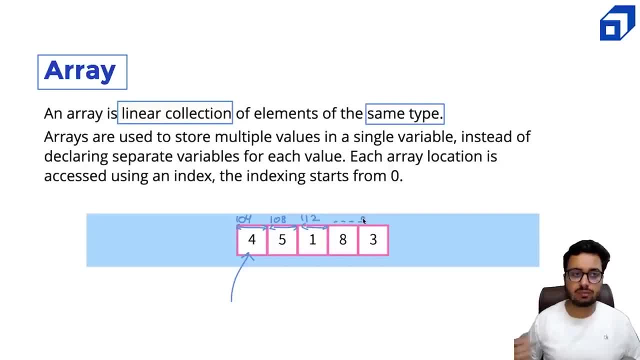 address will be 112,, right, So it is a linear block of memory And this whole block of memory has a single name, right? And each element if I want to access it can be accessed using an index. The indexing starts with zero, So I can say, okay, I want to put something at array of zero, Then I 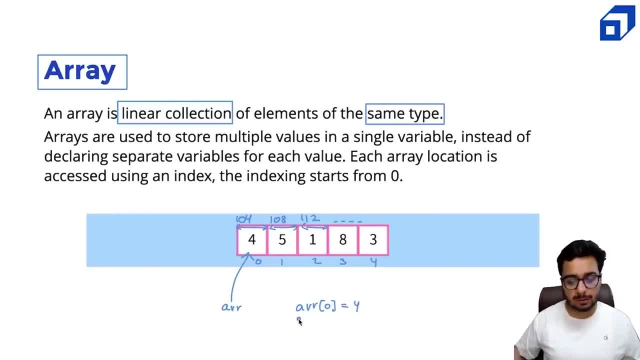 will say: array of zero, it is four. If I want to overwrite it, I will say: okay, array of t, it's going to be 20.. So I can just overwrite this data and it will keep 20, right Each. 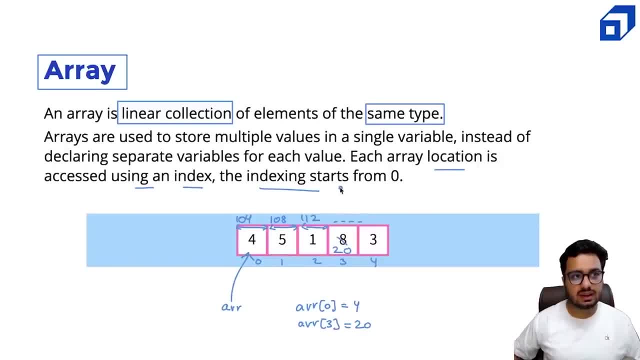 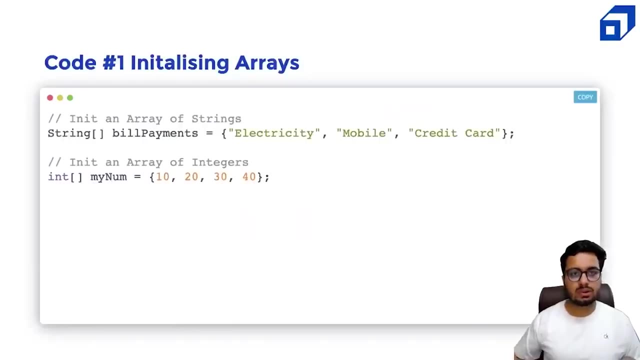 array location is accessed using an index, The indexing starts from zero. That is what we have just seen, So we have the array name followed by the index. This is how you access the ith location inside an array. Now let us look at some examples of an arrays. For example, if I want to create 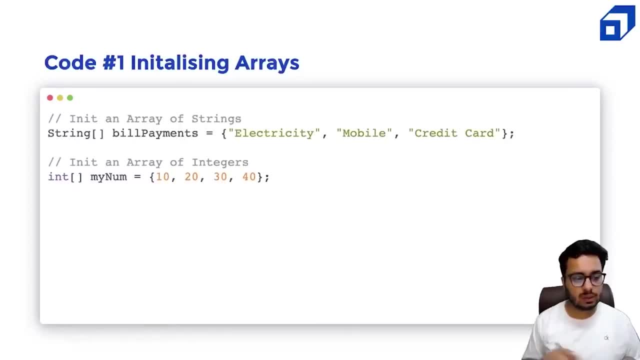 an array of things in which I'm calling the variable as bill payments. I have defined three strings- electricity, mobile and credit card right- And I have an array of numbers. I have defined four numbers here. I have int followed by string. 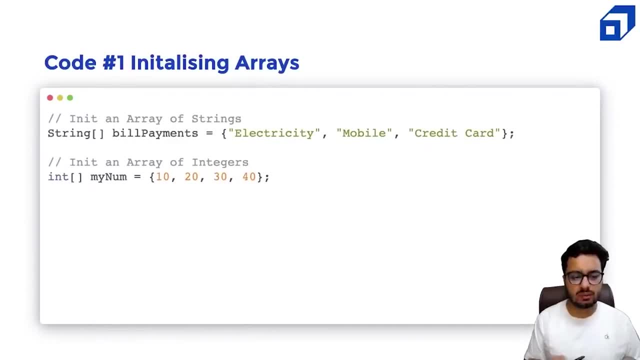 Square brackets followed by name of the array. This is a very simple way of creating an array, but you can also create an array of fixed size where you have not given your data right. In the previous scenario, we have not defined the size. Size will depend upon how many items. 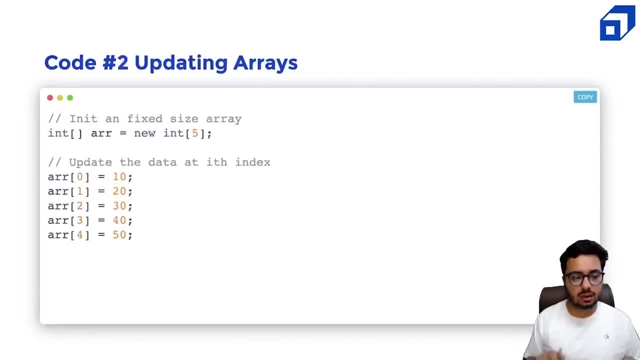 we have initialized in this list. So you can directly initialize or you can first create a fixed size block. You can say: okay, I want an array that is able to hold five integers. We'll use the new keyword, followed by the data type. 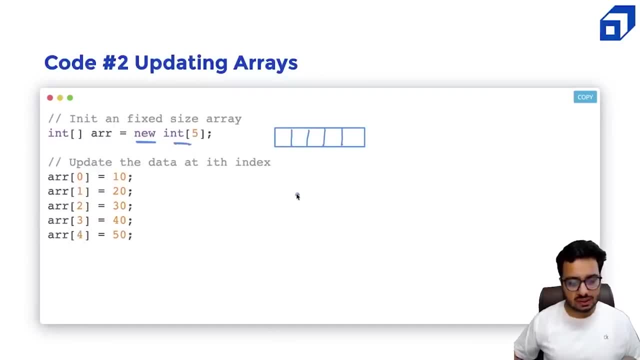 It will be the district and followed by the size. What happens? It creates an array. So if I talk about Java, the variable ARR, It most likely it goes into your stack memory and the actual array that we have. This. this is created in the memory. Now ARR we call. 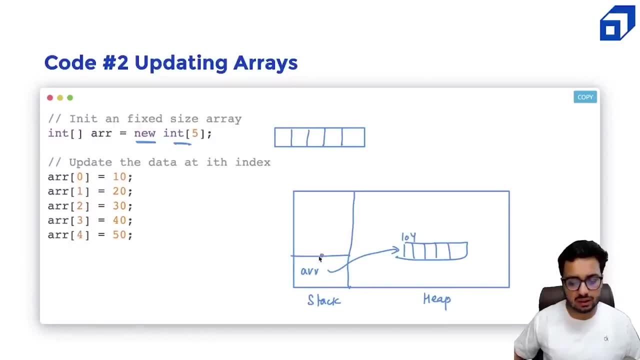 as a object reference. ARR is holding the address of this array. ARR is going to hold one zero four. ARR is in the stack, whereas this object reference- we are looking at one actual object. it is in the deep memory. now we are updating the data at the is index. 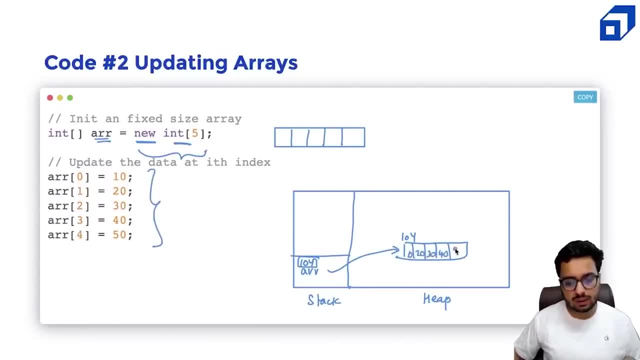 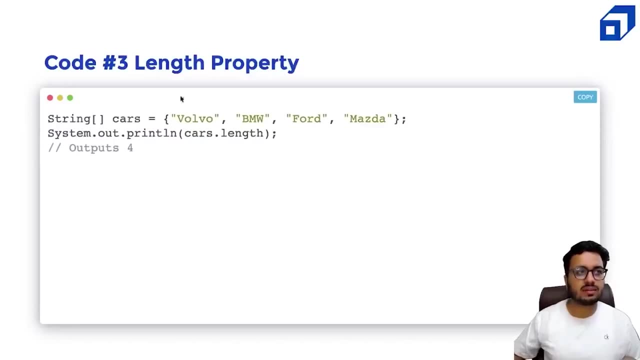 we are actually storing 10, 20, 30, 40 and 50 here. this is how you create an array and all the array objects. they have length property added to it. so if you say, okay, this is a cars area and i want to say cars dot length, this will give me, okay, how many objects are stored. 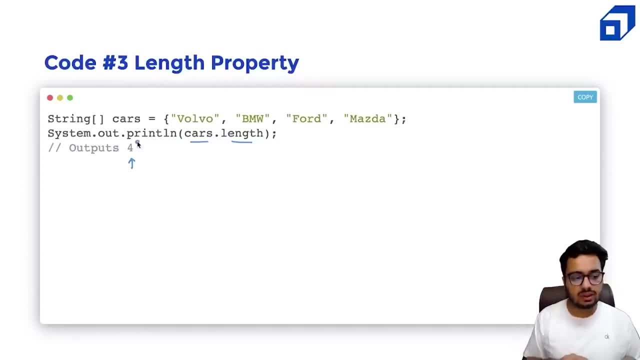 in this array, or what is the size of this array? this will give me four: right, the size of this array. and using the length property, i can also iterate over the arrays, right? so i can say, okay, let me go over every index from zero till cars dot length. that means i'm iterating from zero one. 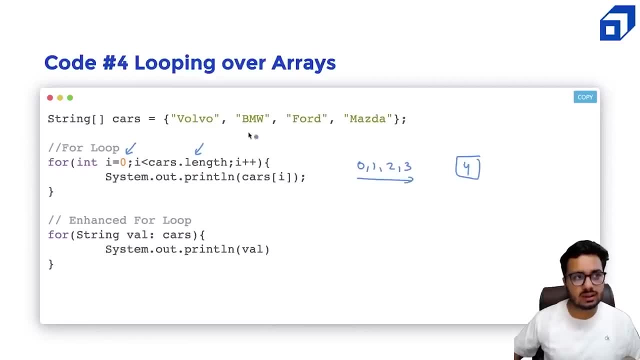 two, three. the length is four. so i'm iterating over these indices. and else, okay, let me print every car. i will print the ith object. right, that is one way of iterating. using the length property you can get the size. other ways you can use for each loop, or also called as enhanced for loop, you can joke for every string value that is there inside. 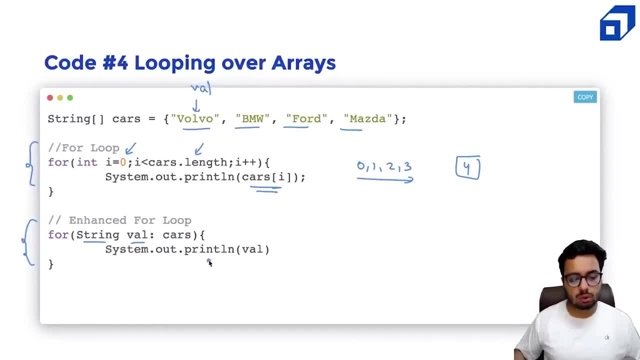 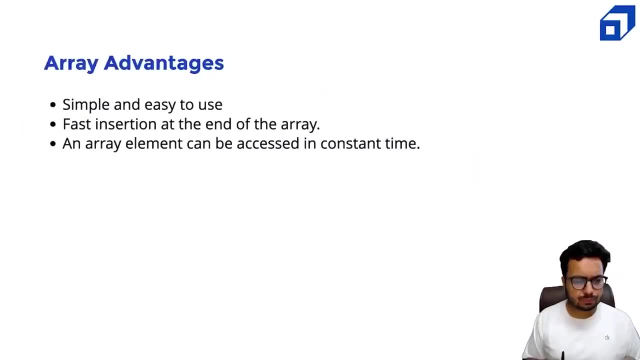 my um cars array. i want to go over that value and i want to print it. that is another way of iterating over the complete array object. then let's talk about the advantages of arrays. they are very simple and they are very easy to use. the insertion is really fast at. 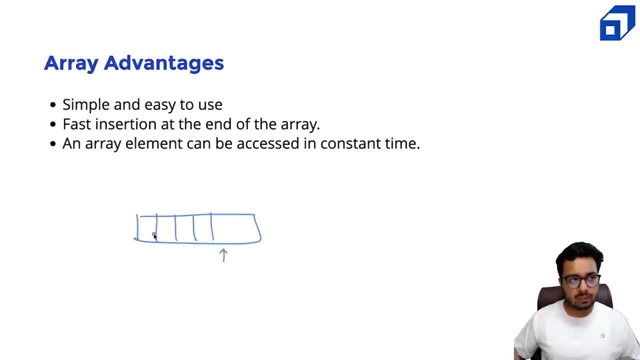 the end of the array because if you keep a variable, that okay, these positions are filled. i want to put something here. you can simply say: array of i equal to value, so that value will get stored here. so you can insert at the end of the array very fast and array element can be accessed. 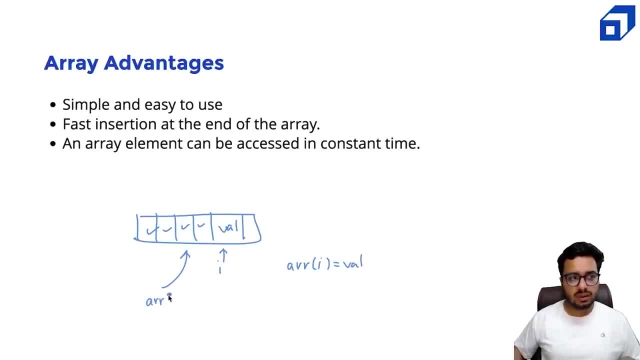 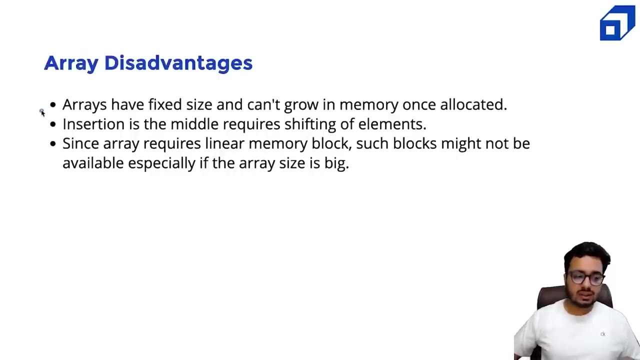 in a constant time. so if you want to get this element, you can simply say: okay, give me the jth element so you can access any random element, any random index and just order one time. that is an advantage of an array, but they also have certain disadvantages. the thing is, arrays have fixed size. 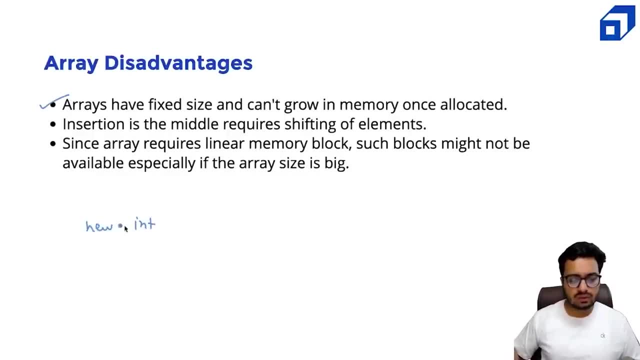 so once you create an array- okay, new int of some size 10, you cannot say i will make it 15 or i will make it 20.. they have a fixed size. they cannot grow in memory once they are allocated. insertion in the middle requires shifting of the elements. if you have inserted something, let's say one, two. 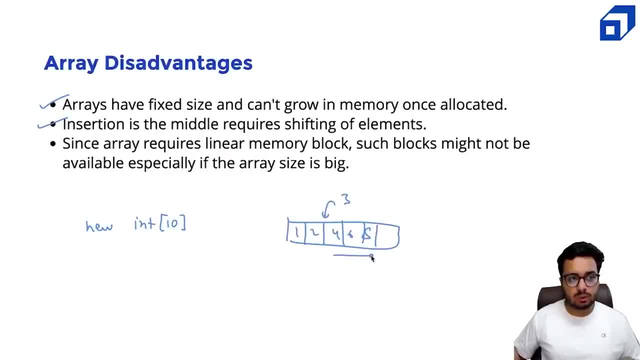 four, six, eight, and you say, okay, i want to insert three. what you will have to do? you will have to shift these elements to the right. you can insert three in the middle. it's going to take order of end time for doing the insertion. and second thing is, since array requires a linear memory block, such blocks might not be available. 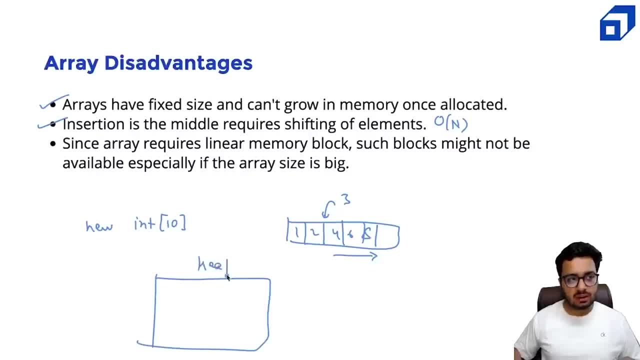 if the array size is big. suppose this is your heap memory and suppose certain portions of the heap memory- they are already used up, right, and suppose you want to create a very big array which might go like this: now it is possible that such a linear block of memory is not available. 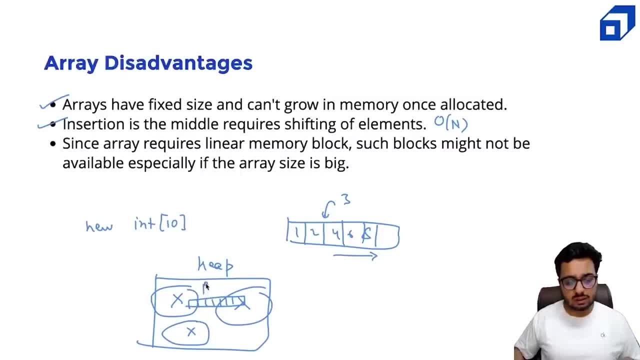 but this amount of memory is available in the heap in chunks, right. so you might say, okay, some memory is available here, some memory is available here, some memory is available here. that is where linked list might perform better, because linked list does not need big linear chunk of the memory, whereas array requires a big linear chunk of the memory. right, so for big. 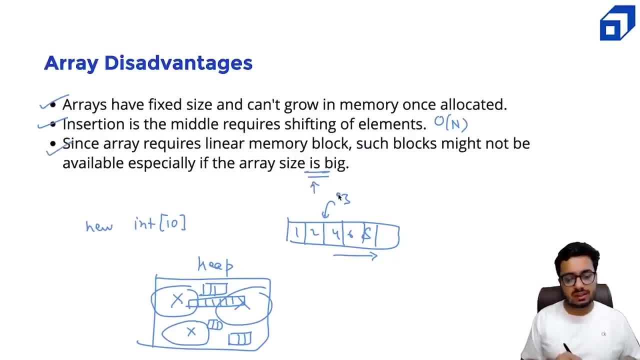 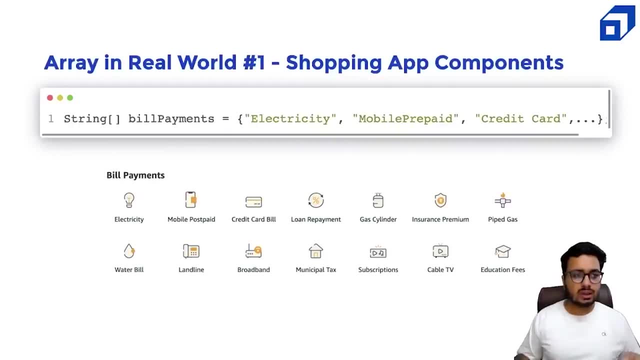 arrays. it could be a disadvantage that such a linear block could not be present in the memory. now, arrays are used a lot in the real world. for example, this is a ui from a shopping website. i have to display these components right, the type of bill payments. i can say okay. 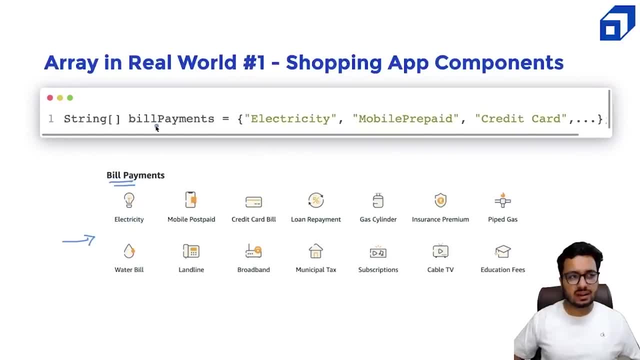 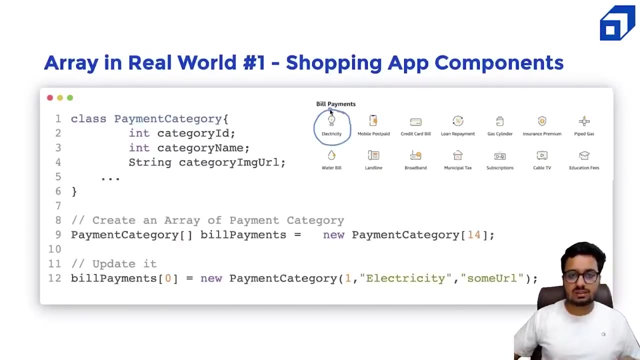 each bill payment is a string, so i have a fixed size array of bill payments in which i have defined all the categories. right now you might say, okay, this looks very simple. in actual world it might be a bit more complicated. yes, it can be. what may happen is that each item is not just a 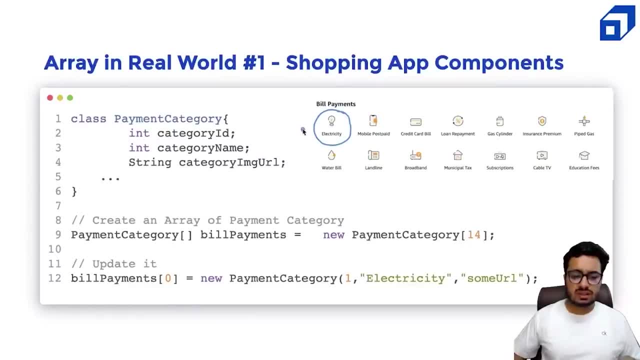 string, but it is a um something more complex. let me call this as a payment category. what i can do? i can define a class called as payment category, which hold three things: maybe the category id, which is not displayed, the category name and the image of the category right, the url of the image. 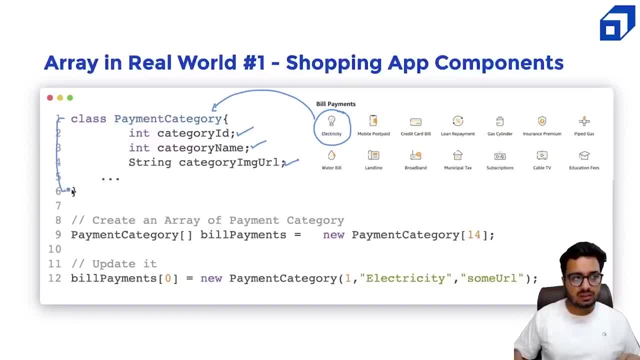 of the category. so i can hold all these things inside a class and then i can create an array of the following class. i can say, okay, i'm creating an array where each item is of the type payment category right. so i'm creating an array of objects of the type payment category right. 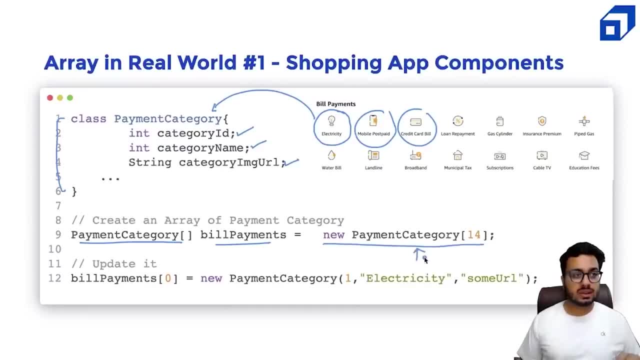 i have initialized this array that is going to contain 14 items and i i need to create these objects as well. i need to say, okay, the bill payments of zero. it is going to hold new payment category and, using the contractor, i've initialized these values. okay, the payment category is one. 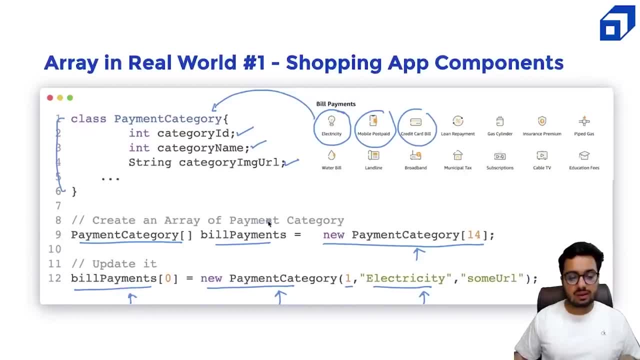 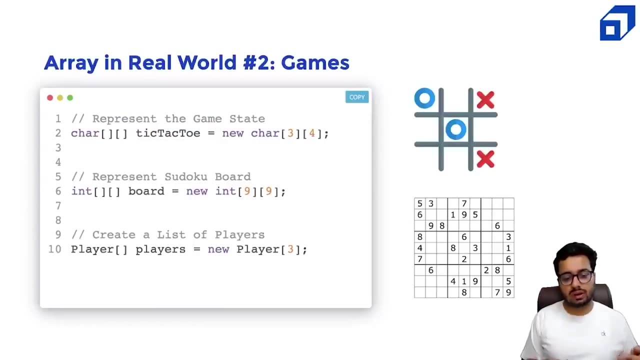 the name is electricity and some url. so instead of creating an array of primitive data types such as integer or float, we can also create an array of complex data types, such as payment categories in this example. Secondly, there are two-dimensional arrays as well, which are also used a lot, especially. 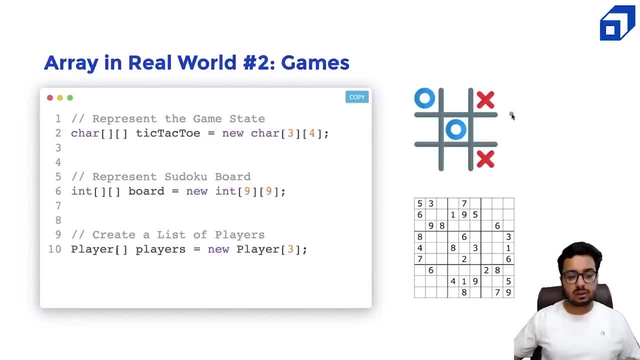 in games and puzzles right. Here is an example of tic-tac-toe, where we might need a board, or here is an example of a duduco game, where we might need a two-dimensional array to represent the state of the game. 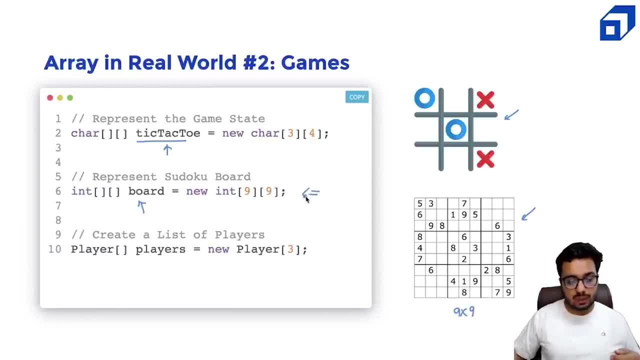 right. So it's a 9 x 9 array. So I've created this array right And I can also create a list of players. It's going to be a 1D array, but the data type is now a player, right. 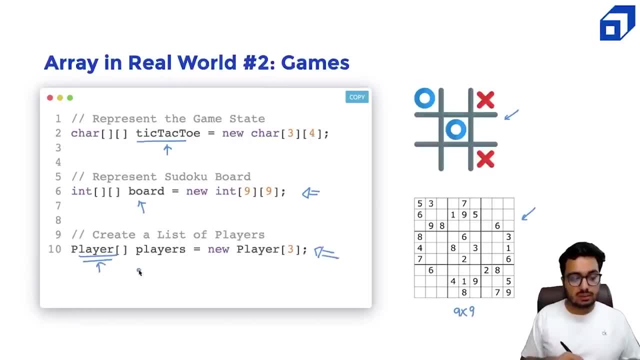 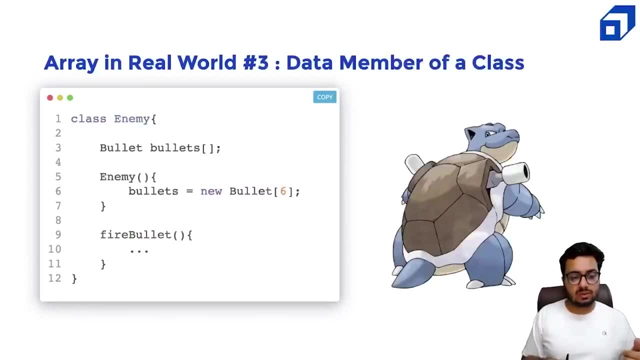 Each player might have a name, It might have a score, might have certain methods associated with it. right, It's an array of players, right? That is also how arrays can be used. Another use case could be that array can also be part of a data, member of a class. 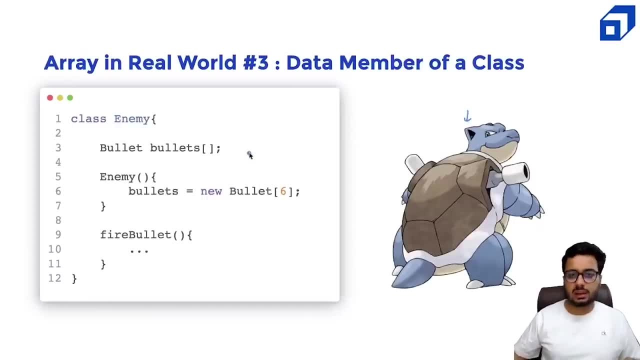 For example, you have an enemy object. The enemy has certain bullets inside it, like a certain number of bullets. The enemy has a number of bullets inside it. The enemy can fire. I can create an array of bullets where each bullet is of the type bullet and I have created. 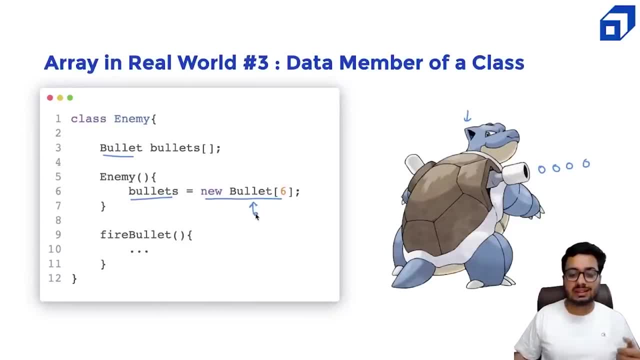 it when the enemy is created. For example, I want this enemy to have exactly six bullets. when this enemy is created, I can do something like this, And when you're firing the bullet, maybe a particular bullet might get deactivated. Something like this can also be possible where your array is a data member. 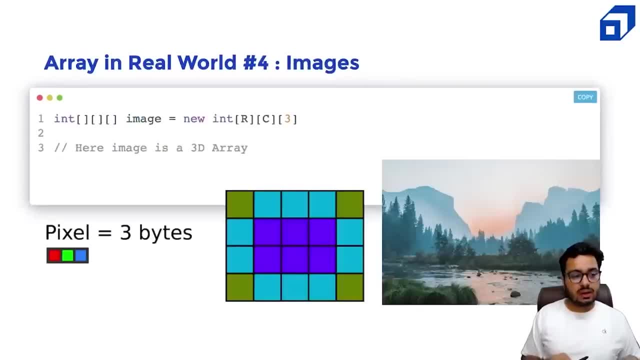 Of a particular class. This can also happen. Another example could be the your images. When you deal with images, you know each image is made up of a matrix of pixels- okay, of the size rows into columns. So you might have heard about an HD image. 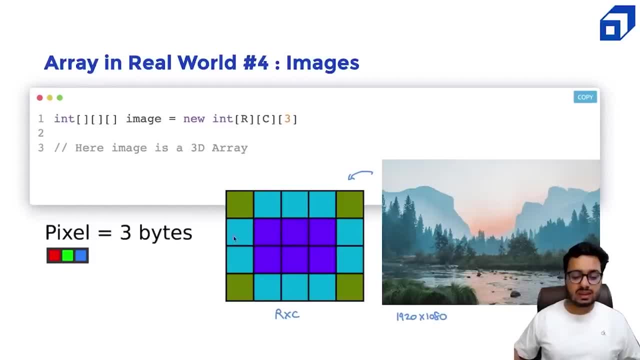 So that is 1920 by 1080.. That simply means that we have these many pixels in this image And each pixel is actually made up of three numbers: a component of red, component of green and a component of blue. So that means each pixel itself is an array of three numbers, right? 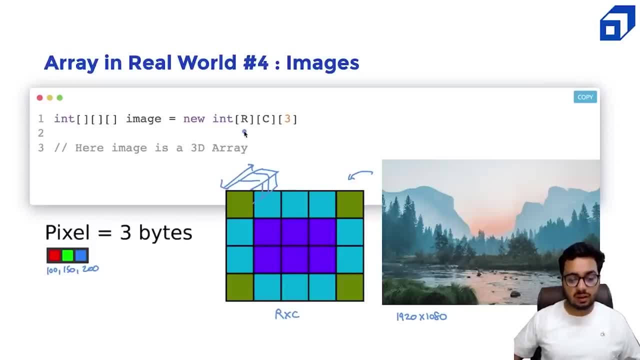 If I look at an image, the image is actually a three dimensional array of rows, comma columns into three Right, Where each pixel is actually going to store three numbers. When we do with work with images in Python, you often see the areas are three dimensional. 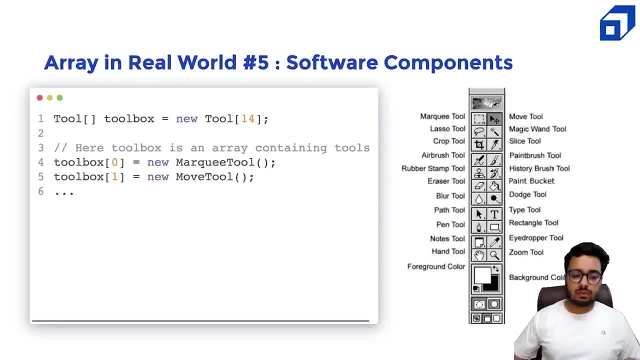 Okay. Another example: When you're building a software components, for example, a tool like Photoshop, right, You will say: okay, there is this grid where every item is a tool. I can say: okay, tool toolbox. This is new tool. 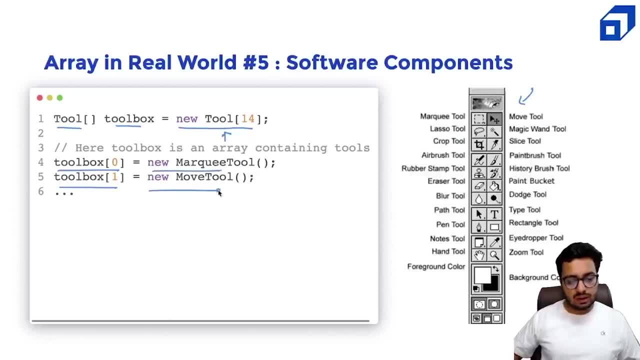 And in every index I'm creating a new tool. right Marquee tool is a type of a tool. Move tool is a type of a tool. I can also do something like this. They are used a lot in building real life software. 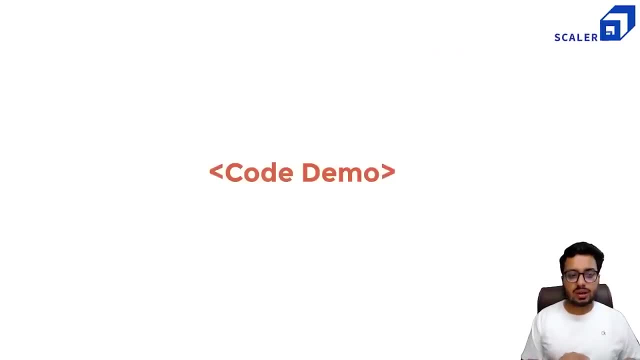 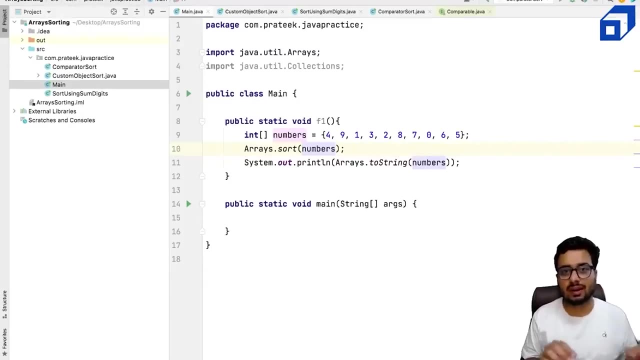 And that is the importance of ArrayFlight. We'll look at Some code demo to work with. that is now. we are going to look at some code of an areas, especially how do we perform an operation like sorting on areas, which comes very handy. 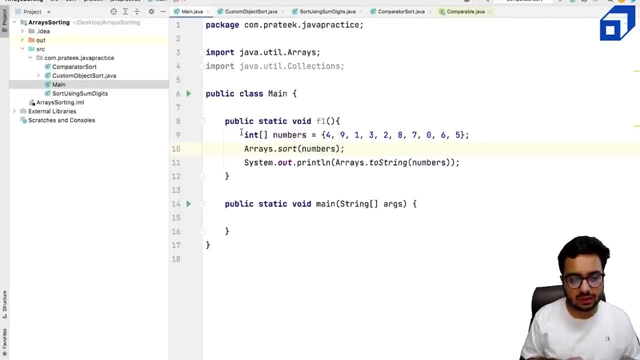 in solving lot of problems. Okay, So I have an area of numbers and I want to use a method called as sort. right In Java dot util package there is a class called arrays. This class contains methods that will work on a area that we have created right. 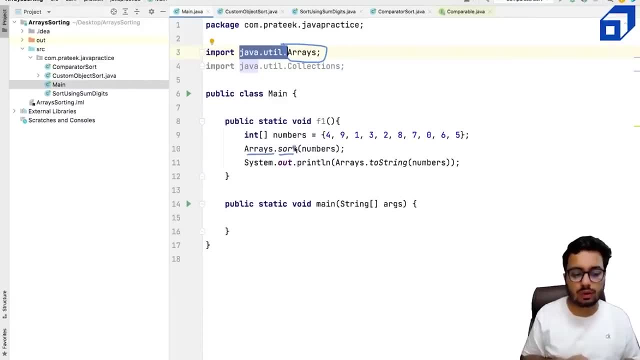 It is. So what is one such method? We want to use this method to sort our numbers that it let's see if I go and run this code. So I just need to call this function F1.. My array is created, The array will get sorted and we are going to output this array. 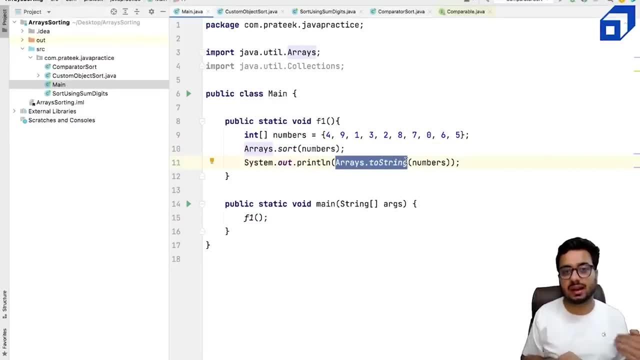 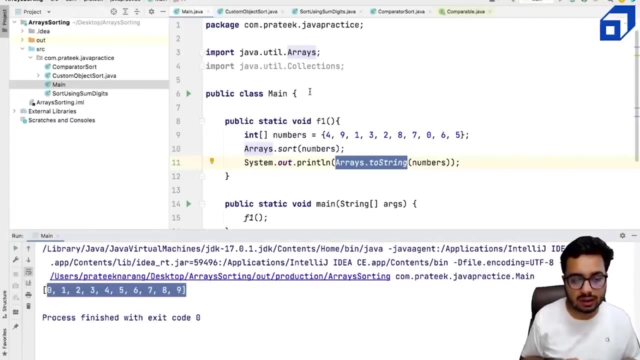 Another such method is arrays dot to string. I can convert this array into a string, like representation, that I can print directly, So let us just go and run this method. So now you see, the data that you're getting is in a sorted order. 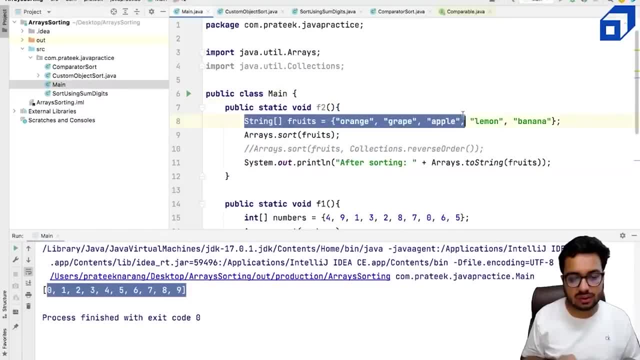 Let us look at one more example. Let's say I have an array of strings and I want to sort these strings again. What I can do, I can use arrays dot sort method, which is again an inbuilt method inside Java, dot util, and I just need to pass the array object to this method. 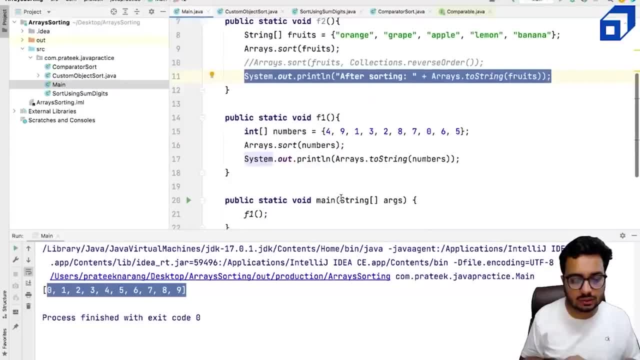 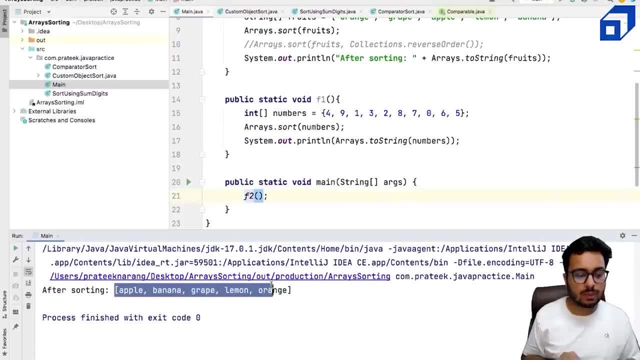 It's going to sort these objects and let us call our function F2.. Okay, And let us run this code. Now, what do I see? I see output: apple, banana, grape, lemon, orange. right, How do strings are compared? 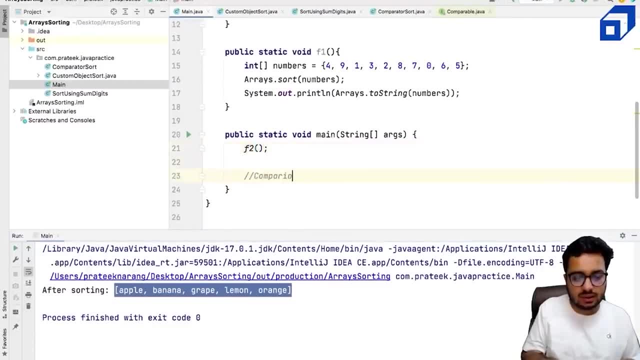 Let us talk a little bit about comparisons as well. Now, comparing numbers is easy. I can compare as five less than 13. answer is yes. But if I have a string called as, let's say S1, that is ABC, and I have string S2, let's. 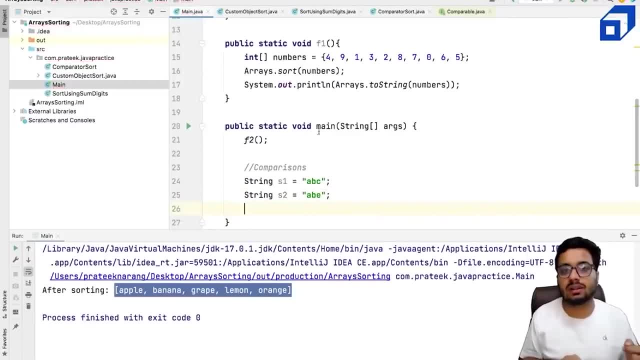 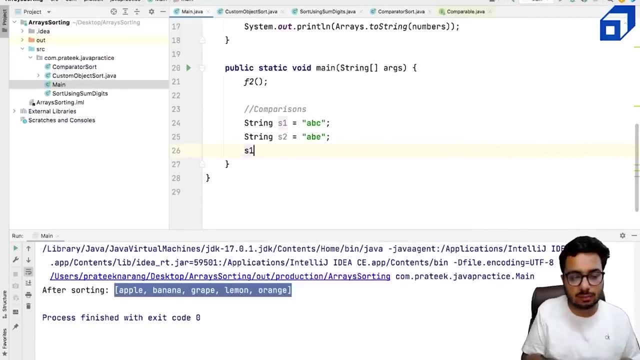 say I call it as ABE Right? Are they comfortable or are they naughty? How do we compare? by default, inside the string class, it is a method called as compared to. if I say S1 dot compared to. you see, there is a suggestion coming out and I say okay. 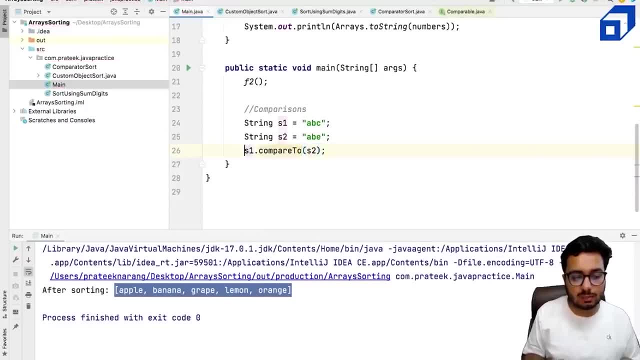 let me compare it with the string S2 and let me, uh, show you the output of what this comparison function is going to return. Now, why I'm teaching you is: this is very important because we also want to write custom comparisons for our object and getting an output that is mine. 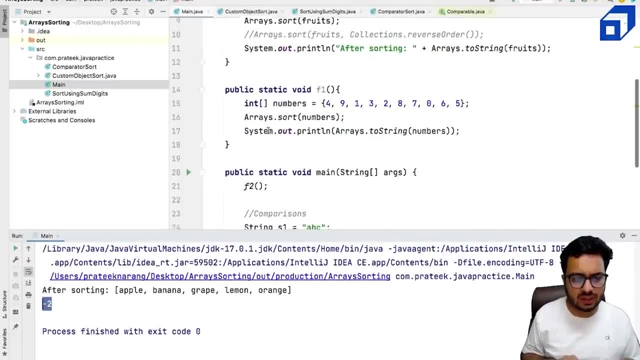 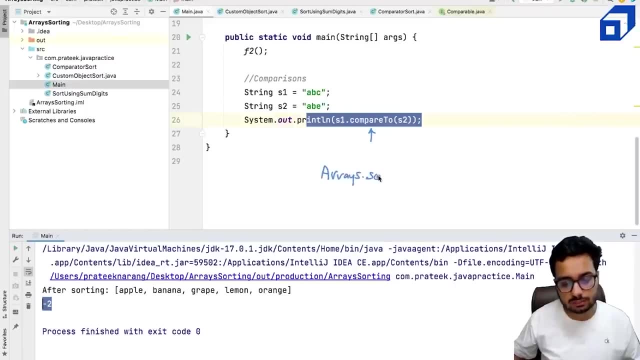 Basically how sorting function works is internally calls the compared to method. When you use it is a dot sort. can you give um some area of objects to sort right? So what it does, it calls the compared to method of that object to string. 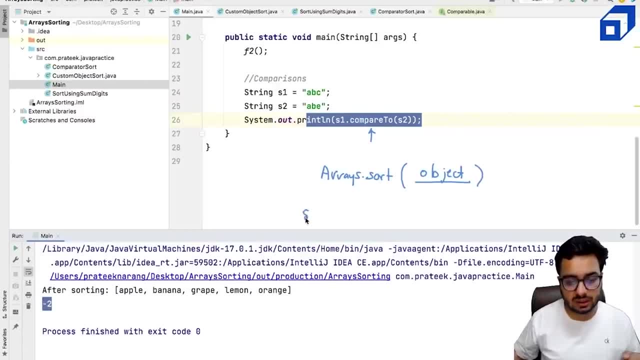 Basically, it is calling the compared to method of this object Right, Which is ABC. I want to compare it with another string, ABE, or this compared to method. It's going to produce the types of outputs: One is a negative output, One is zero and that there is positive. 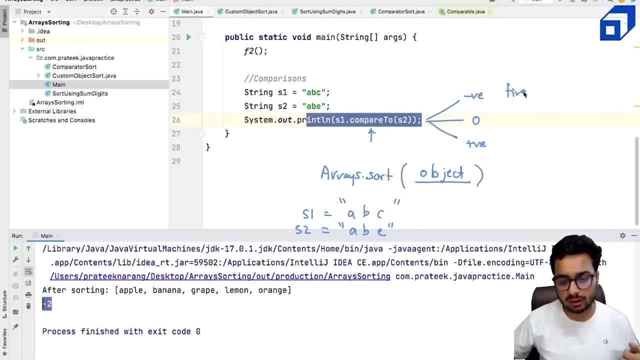 The negative output simply means that my first number is smaller. First object is smaller, That means it will come first in the list. Positive number means my second object Is smaller, That means it will come first in the list, and zero means the two objects they are actually. 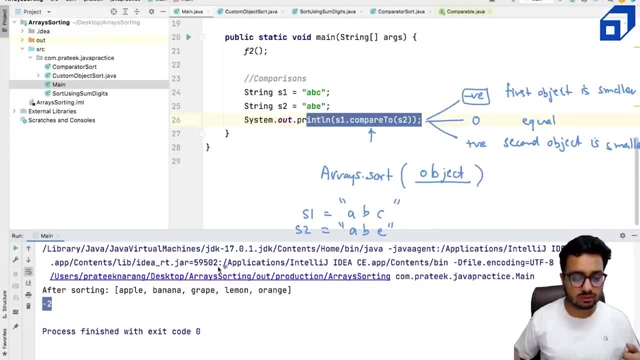 equal If, if I get a negative output, which I'm getting in this case, that means ABC is smaller than ABE. Let us also see how this minus two is actually coming Right. So when you compare, uh, ABC with ABE, right. 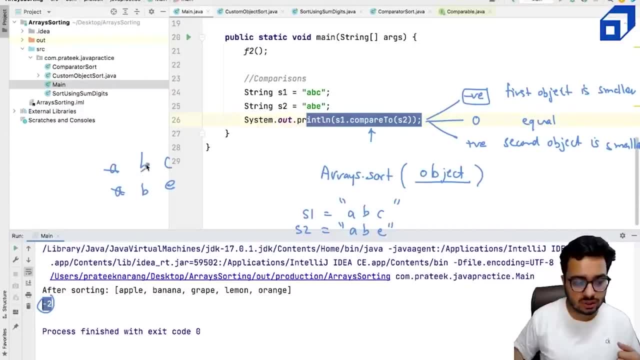 So you compare A with A. they are equal. So you move to the next position. you go with B. B and B, they are equal. You move to the next position. Now you compare C and D. right now, suppose C has some ASCII value, right? 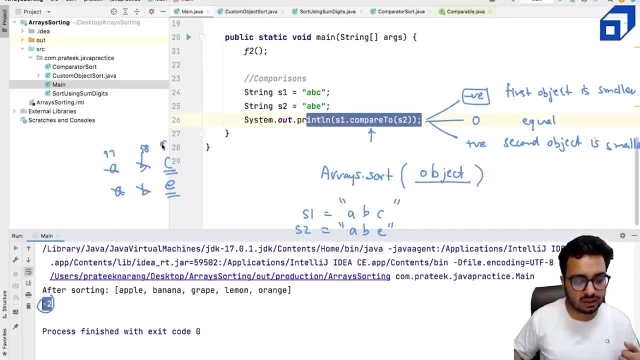 So maybe this is: uh, this was 97,, 98,, 99, right And this is 97, 98, 99, 100, 1 0, 1, right. The ASCII value of E could be 1 0, 1.. 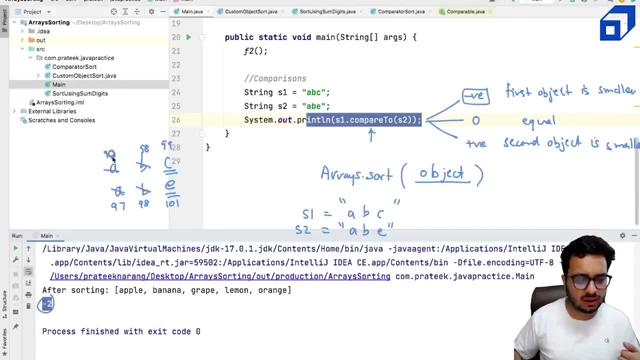 So when you take this difference, I think A is actually 90, not 97. Whatever the ASCII value is, you will take the difference. If you subtract C from E, you will get a difference of mine. That basically tells the sorting function that I will place ABC first. 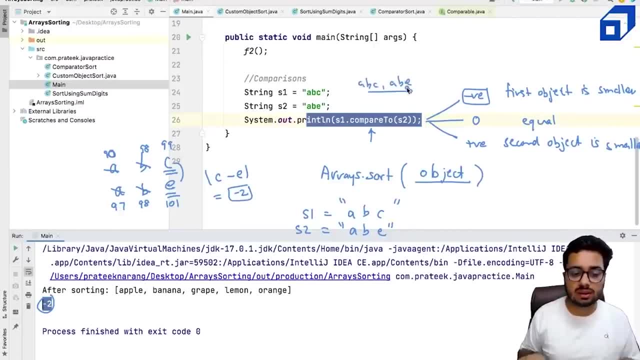 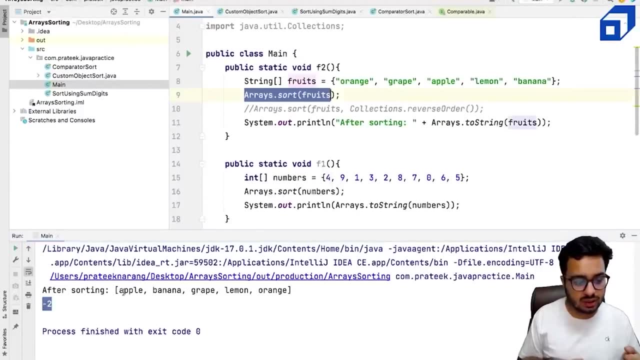 And then I will place ABE, the sorted order. So compare to function is responsible for defining the sorting order. When I'm sorting these fruits, you see apple, banana, grape, lemon and orange. They're coming in their dictionary order right. 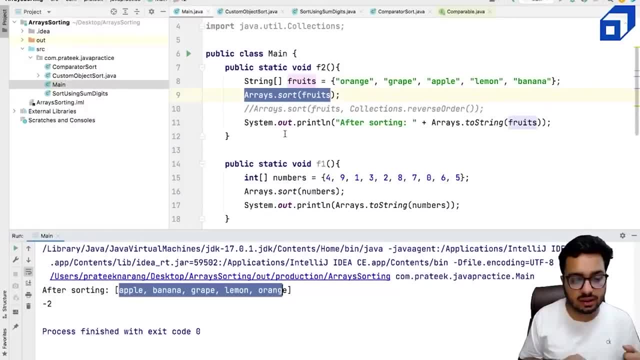 Because a string knows a compare to function is present inside it, right? Then I say: okay, I want to. I want to reverse this order, right? What you can do is one simple way of doing it is that you apply a custom comparator called 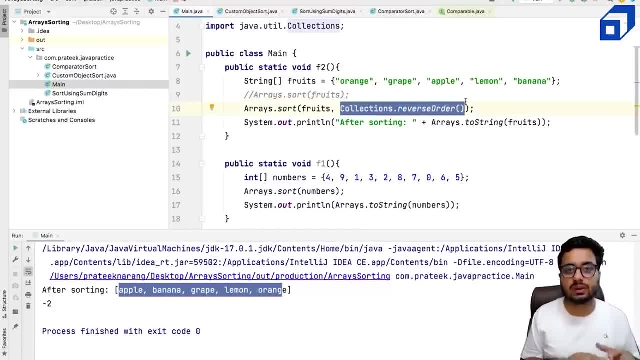 as collections or reverse order. That is exactly going to reverse the default output. Okay, By default you're getting this output. If you specify this, it's going to reverse the default output. I run this code Now we'll see. I will get orange first, followed by lemon, grape, banana and apple. 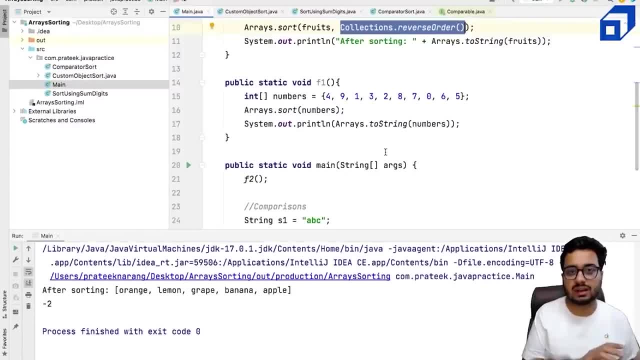 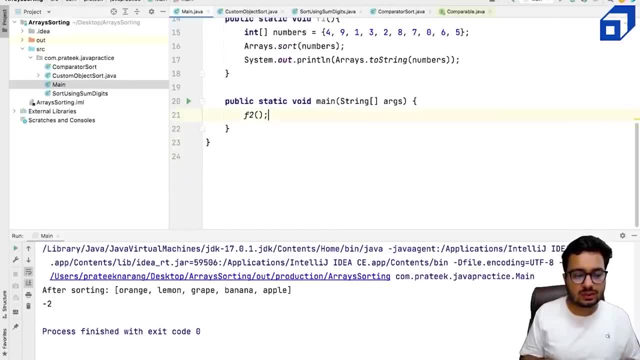 That is one thing that you can use to Convert your ascending array into a descending. That is one way of doing it. So now you might ask why we are studying this compared to method, or where do we need it. Let us try to understand that as well. 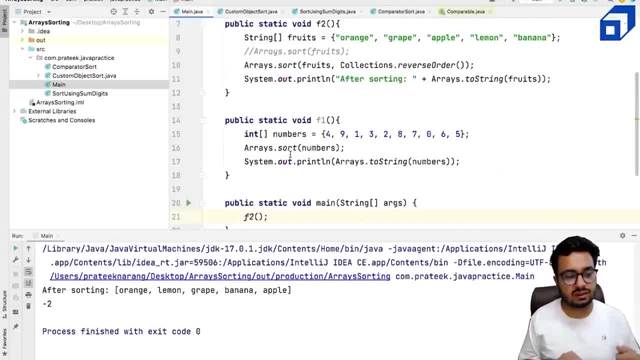 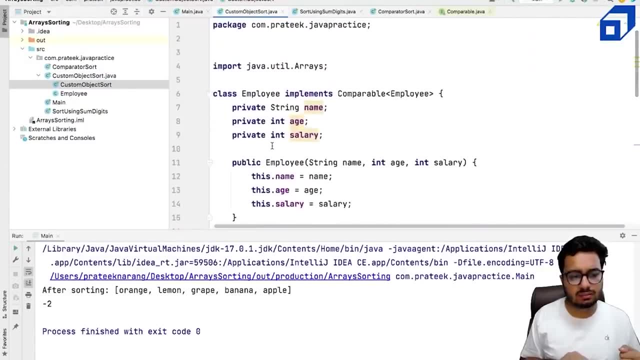 This was very simple. This was an array of integers or an array of strings, right, You might say that I have a custom object. I have, let's say, a class called as employee, Where My employee has a name: Agents. 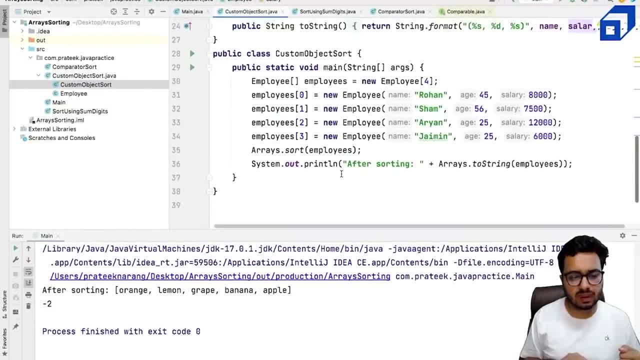 All right, And I want to create an array of employees. I have an array of employees, an array of custom objects, and I want to sort them. If you sort them right And if you do not tell Java that, okay, I do not know. how do we, how do I compare to? 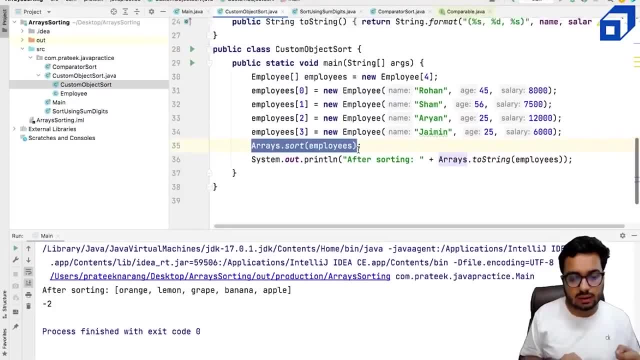 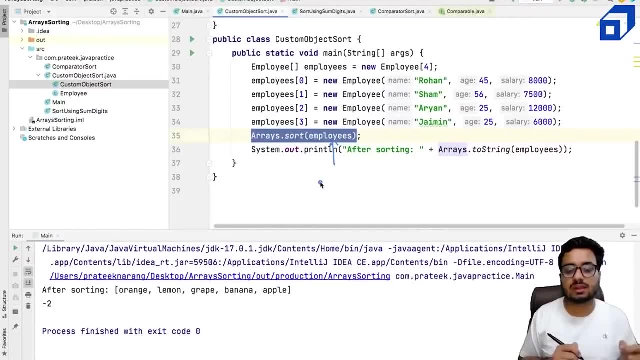 employees, Most likely you're going to get an error right Now. errorssort can also accept employees, but given that you define a method called as compare to inside the employee, If in the string class it is an inbuilt method, but in the employee class, which we 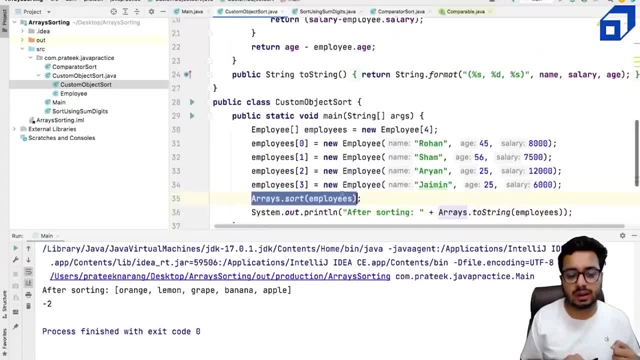 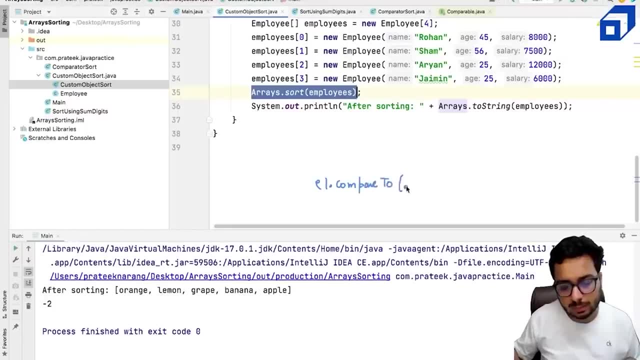 have written. we have to define: how do I compare to employees? For example, I have an employee- even I want to call the compare to method- and supplied some another employee to write. So when you say, okay, I'm sorting a list of employees, right. 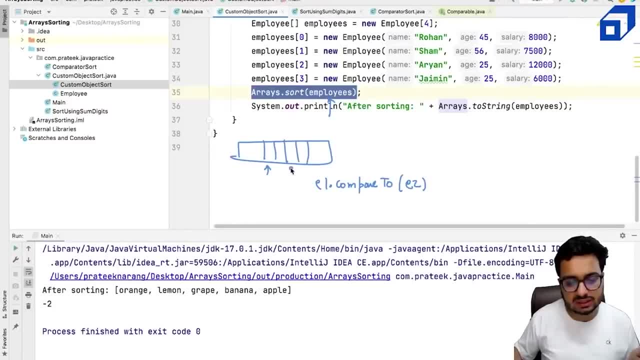 This is an area of employees, It will. Okay, I'm going to compare this employee with some other employees, So I will say employee. I thought compared to some other employee, that is employee J. The sort function is internally going to call this method, called compared to right. 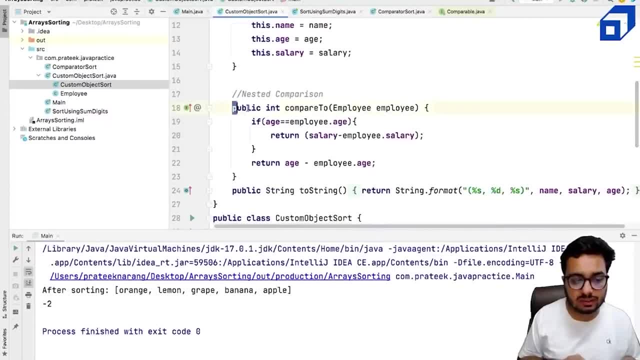 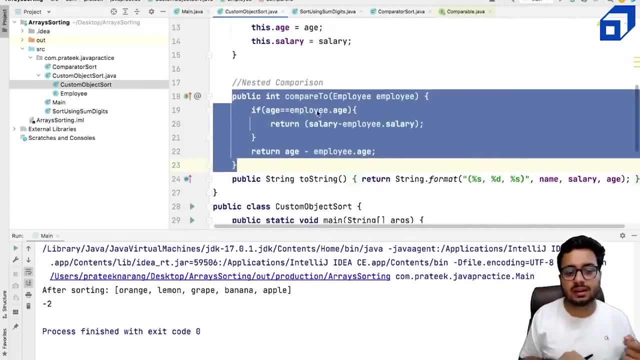 This method is not there. What we have to do? We have to define this method inside our employee. I have my employee class and here I'm going to define my compared to method. how it will get caught. It will get caught internally. 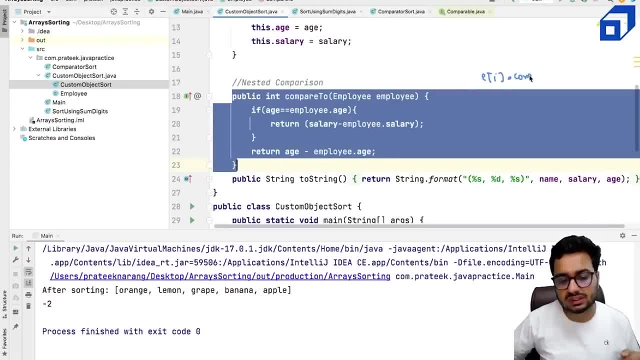 Employee I getting compared to with some other employee: J right now. It is up to you. How do you compare to employees Right Some other employee? Okay, Right, EMP. Now look at this: How do I write this method? 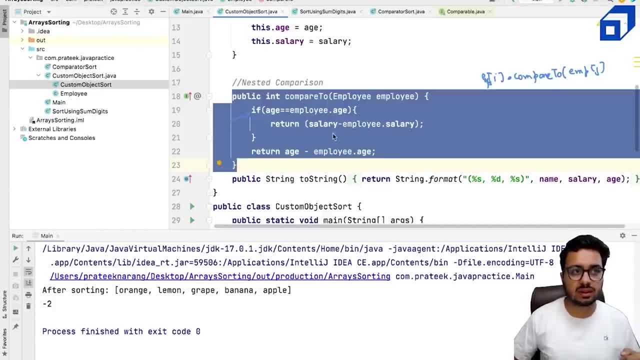 Basically what I'm doing. I'm saying: if the two employees have the same age, I will compare them according to their salary. I'm saying salary one minus salary Two. So the first employee salary is 100 and second employee salary is, let's say, 60, a hundred. 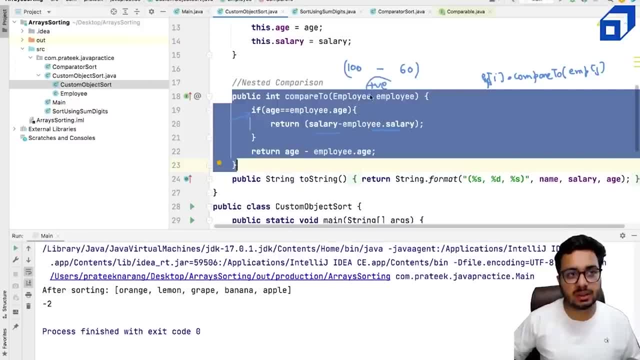 minus 60. It's going to produce a positive number. That means the second employee will come first, The person with the lesser salary will come first. or if the age is not equal- I'm saying age minus employee, dot age- This is the age of the first employee and this is the age of the second employee. 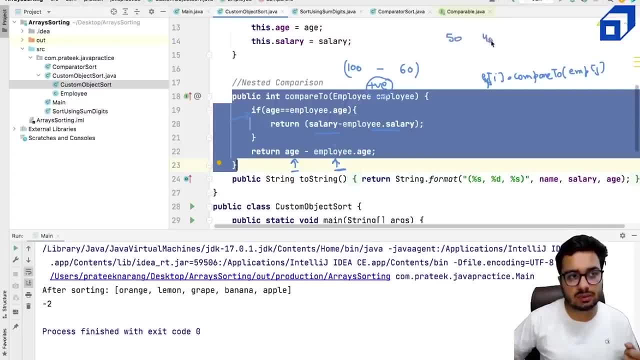 For example, if the first employee is 50 years old, The second employee is 40 years old, 50 minus 40. It's also going to produce a positive number. That means the second employee. it is smaller in age right. 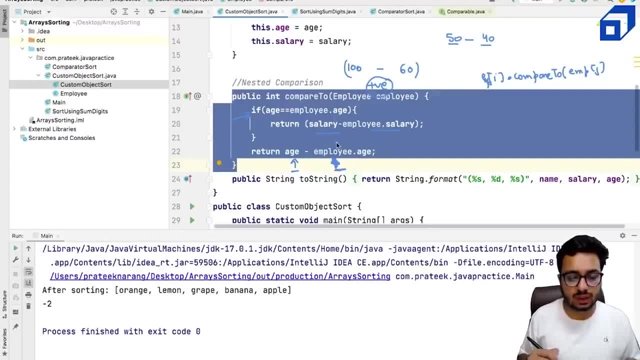 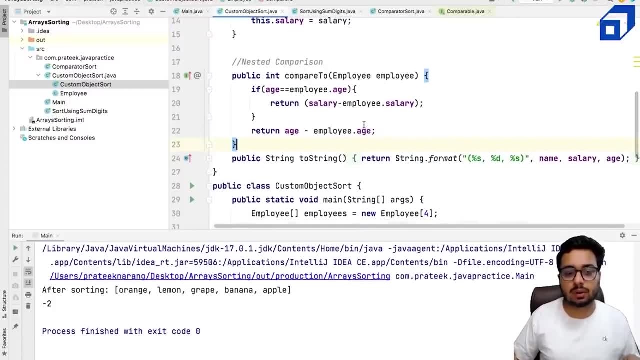 What this sort function is going to do. what this compare function is going to do: It's simply going to compare the two employees based on their age. If their ages are equal, it's going to compare according to their salary- People with the less age and less salary. they are given priority. 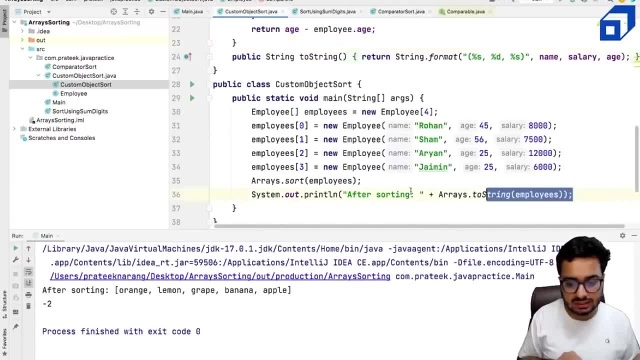 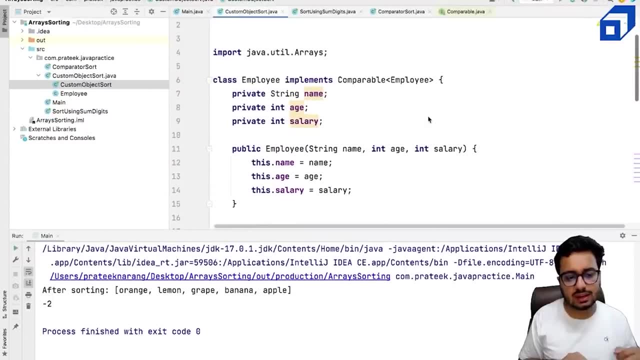 They will come first in the output. So let us, Let us run this code and see what do we really get right? Okay? One more thing is that, uh, we have to. so whenever you're creating this class, you have. 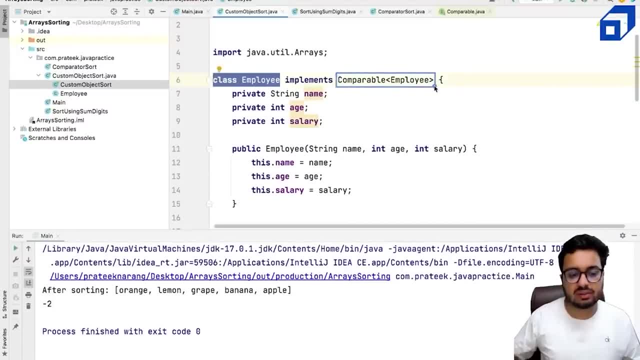 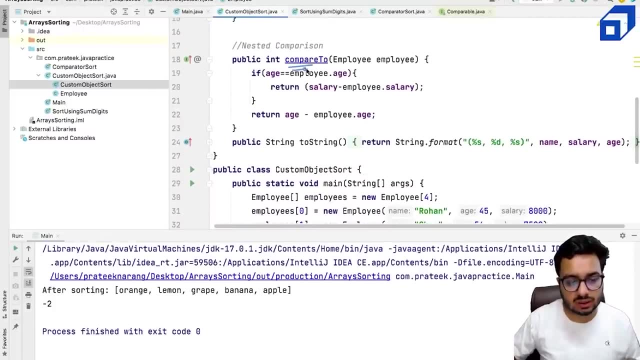 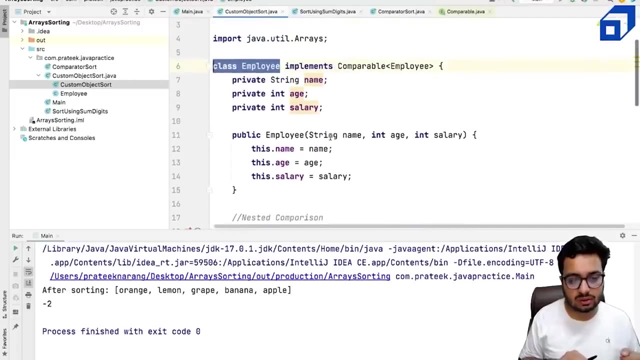 to tell that it implements the comparable interface. right, Why? Because the sort function expects that you will implement a compare to method. This compare to method is coming from the comparable interface. Right, We will talk about the concept of interface very shortly, but you should know that, uh. 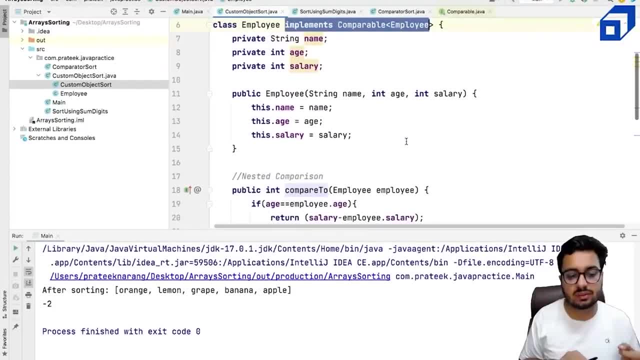 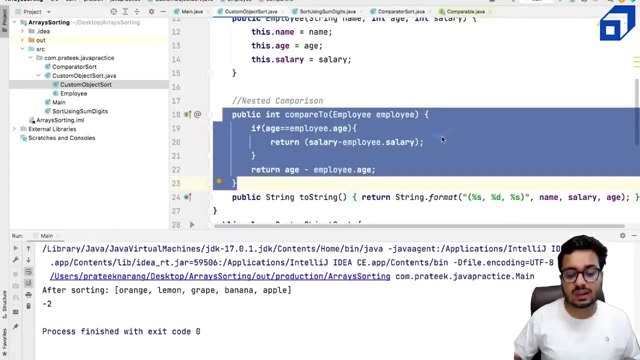 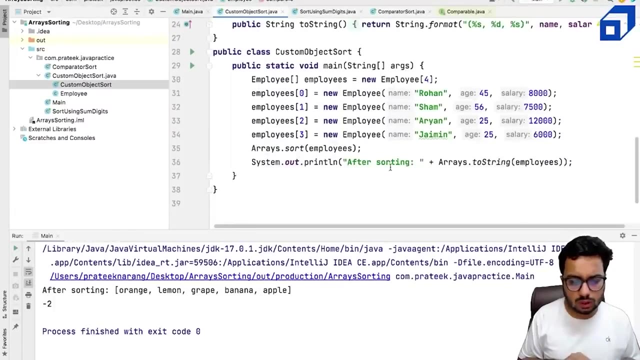 you have to say, this class implements the comparable interface for the employee, in which we have an abstract method compared to, and we have defined this method in the current employee class right. The body must be given here. So what? what is happening now? 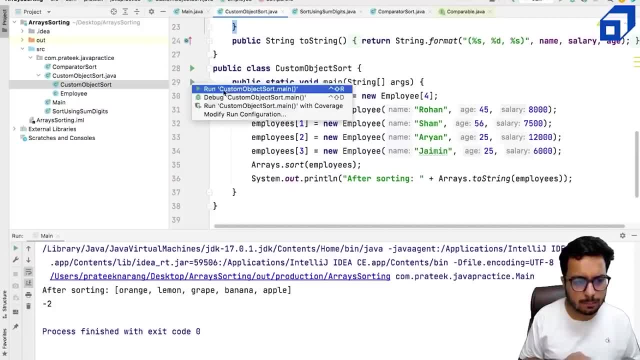 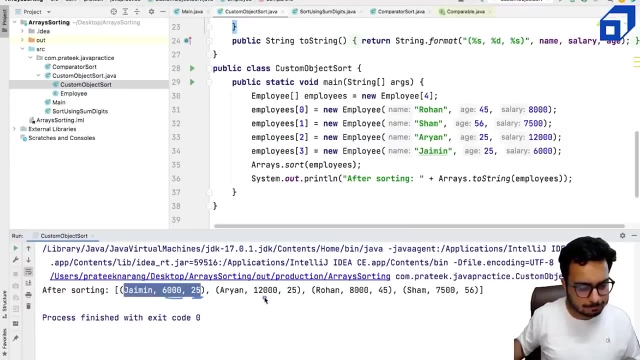 Uh, let me show you the output. Let's run this one. Yeah, Yeah, Yeah, Let me show you the array of objects, right? So I'm saying let me print employees. So now I'm getting 6025. if this is salary and age, uh, I'm getting 12,025.. 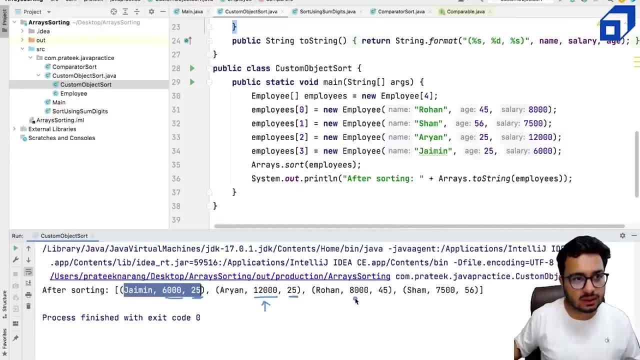 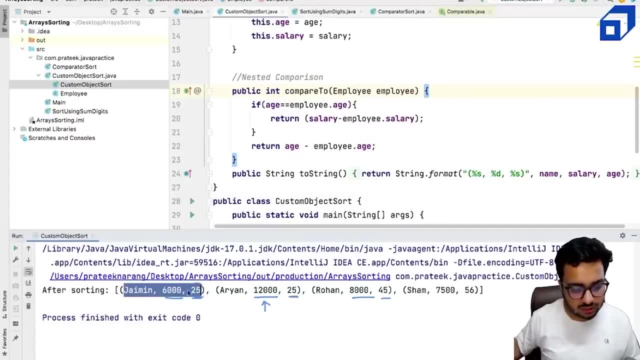 That means higher salary, same age, and I'm getting uh, 8,045.. According to my logic, the first preference is on age. employees are sorted first on their age: 25, 25,, 45 and 56.. 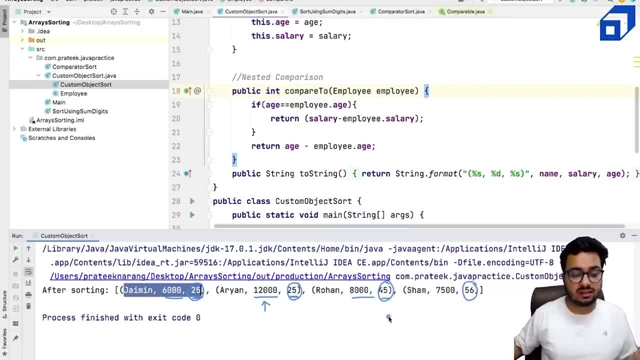 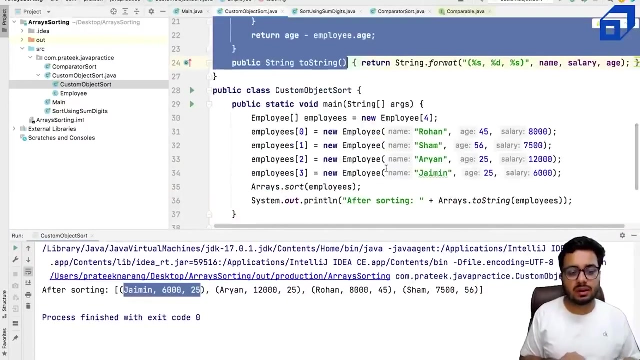 Yeah, Yeah, celery if the age is same. so jam, jam in and rn. they have the same age. so the person with less celery it's going to come first. so you can do, you can make any logic like depending upon the situation, and this compare to method will tell the sort function. how do i actually sort? so i'm 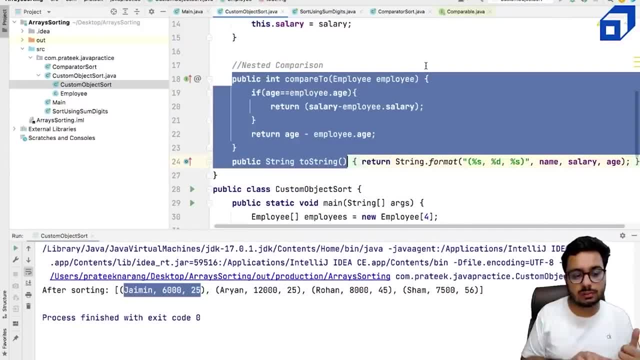 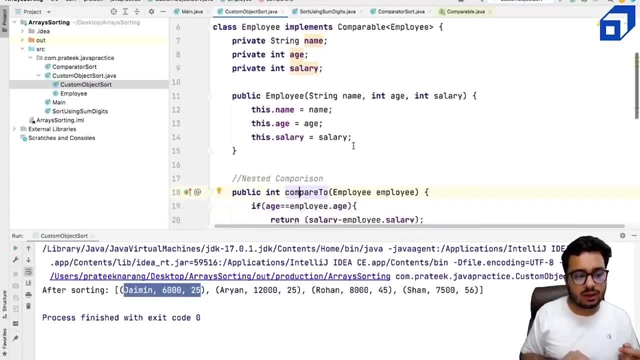 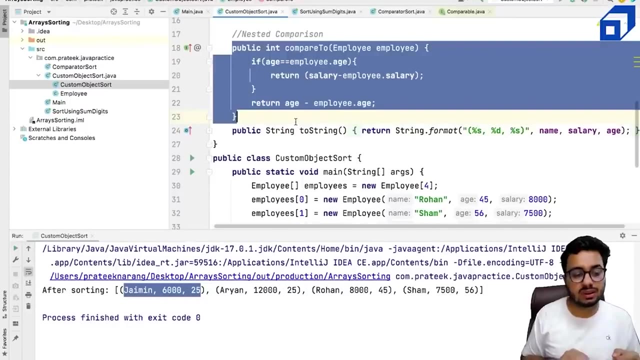 hoping that this is clear. so one way is use the default sort function, but it does not work for the custom objects. right then, what you can do, you can write the compare to method. and now there is one more scenario in which might not want to go this way, you might want to go go with the comparator. 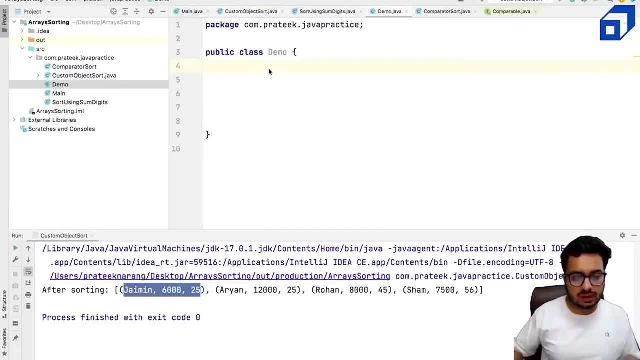 way. right, let me discuss that as well. so let us discuss one one more way of sorting using comparator. now i'm going to tell you why it could be important. now suppose you have maybe a list of strings. if let's say abcd, or let's say some fruits- apple, mango, guava and orange- and you want to say, okay, i want to sort my 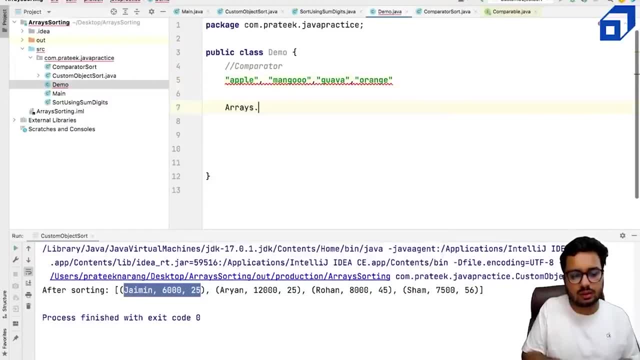 fruits. i want to say, okay, um, there is dot, sort, i want to sort fruits. but i want to sort fruits, maybe, according to the dictionary order. i want to use the default comparison. or maybe i want to sort fruits, uh, according to their length. i'm not writing writing the proper code, but what i'm trying to tell you is that 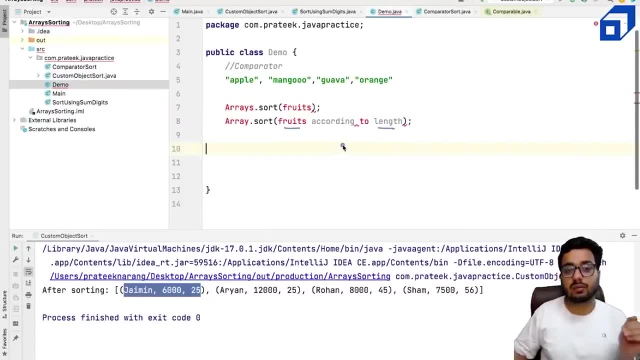 if i want to sort fruits according to their length, i will have to go inside the string class, and inside the string class i will have to change the compare to method. do you think changing the compare to method inside the string class, which is implemented in the java library, will be a good thing? answer is no. we cannot go and make. 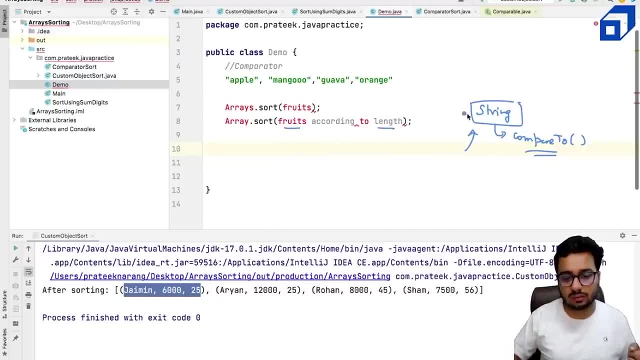 changes in the library right. that is one reason we will not use the default compare to method or we need some other way to do the sorting so that we have the flexibility right. another option could. another reason could be that, uh, i might have a if else, like this, if the condition is this: 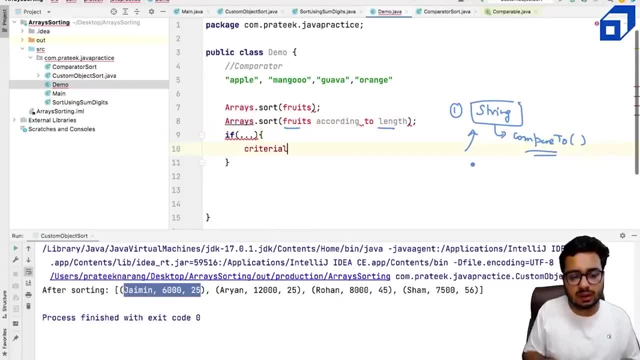 i want to sort according to some criteria. if there is some other condition, then i have to use some other criteria for sorting. right, i might have something like this. then also, i will have to say that okay, go with the first way if your if condition is true, go with the second way if. 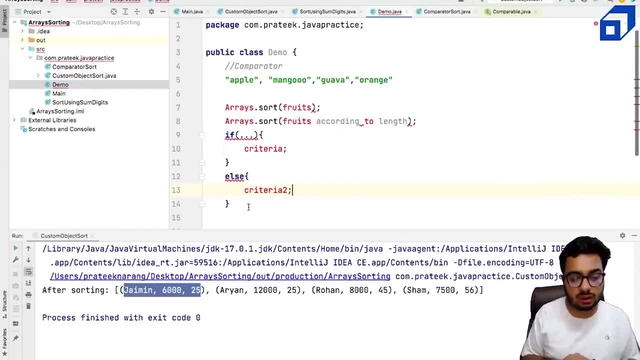 your second condition is something of this sort. what i'm going to tell you is that in such scenarios, where either you have conditional sorting or you will have to use your, you cannot go and change the library. compare to method for for that particular class. there is third way of. 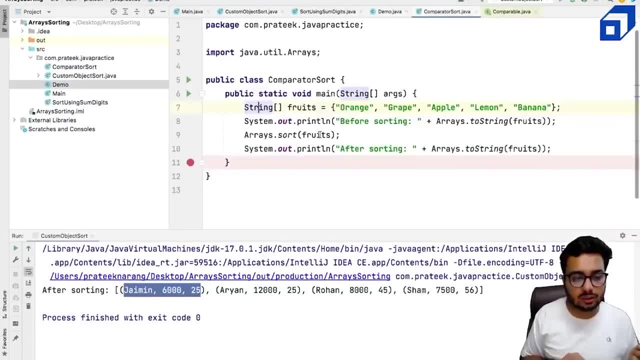 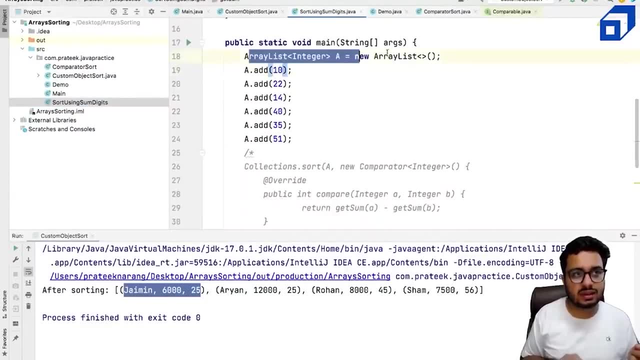 doing the sorting. so that way is called as comparator. i'll show you an example of using a comparator right. in this case i am creating an array list of integers. so array list we will study very shortly. it's just like a array but it's dynamic inside. it can grow and shrink, so it 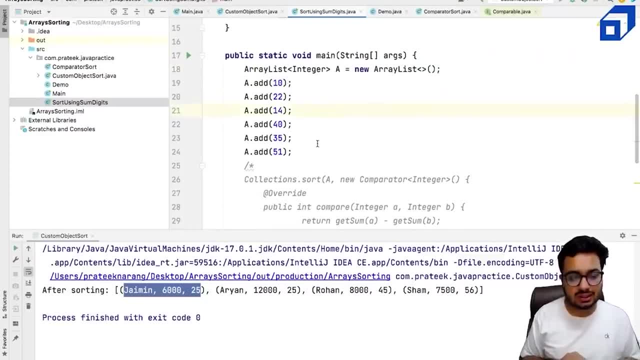 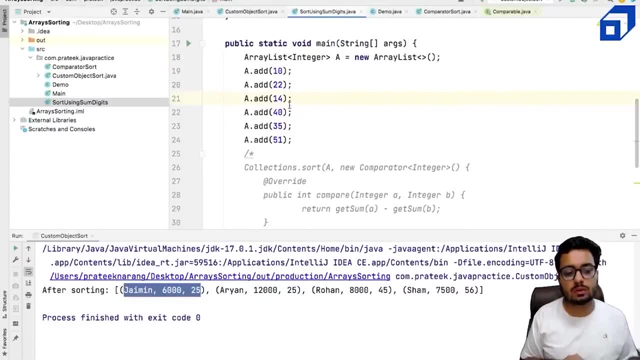 is part of collections framework. we will study, so the teach the, the demo that i'm going to do here, is also up to you. what we have done is we have created a dynamic array in which i have added few numbers. what i want to do is, instead of sorting these numbers directly. right, i know, 10 is less than 22, that's. 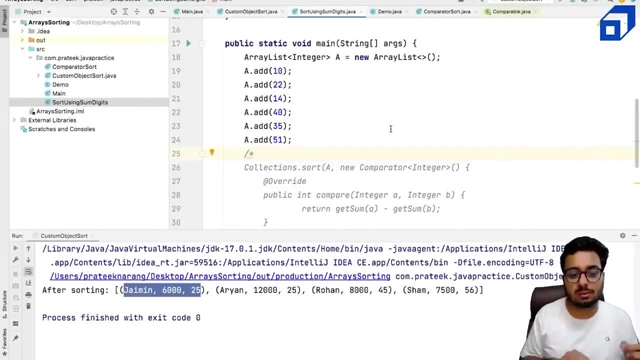 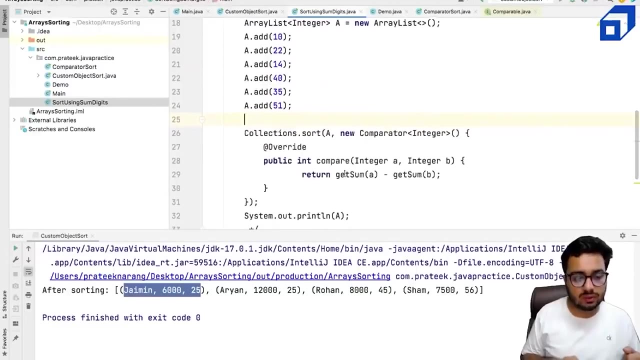 okay, but what i want to do? i want to sort these numbers based on their sum of their digits. you might say: okay, how do i override such a comparison? in such scenario, there is this third way that i'm going to teach you. it is called as sorting using comparator. right, what we can do, we can. we still need to call the sort method. 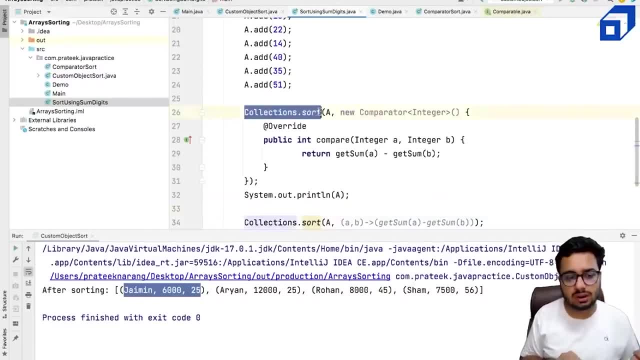 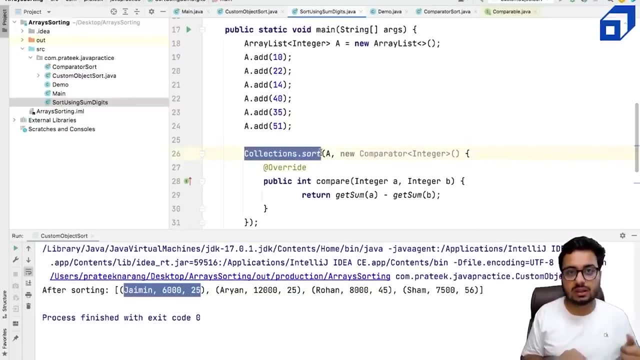 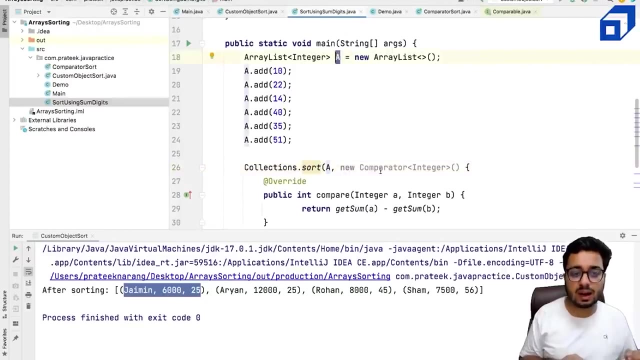 if it is an array object, you will use arrays dot sort, but if it is an array list which is part of your collections framework, you will use collections dot sort. in this sort method, you need to give your array list object. that is a, that that we have given, and now you have to say that. okay, i'm. 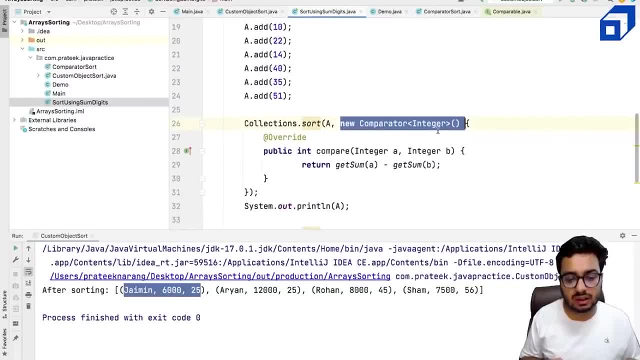 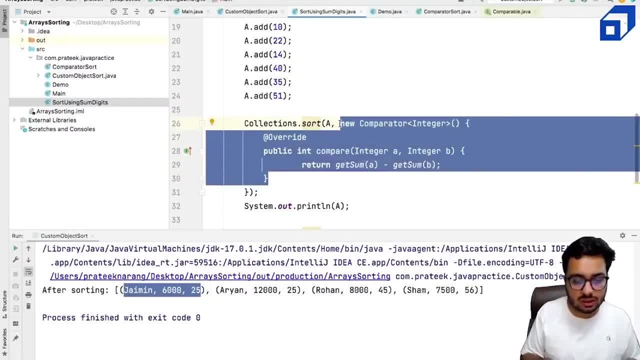 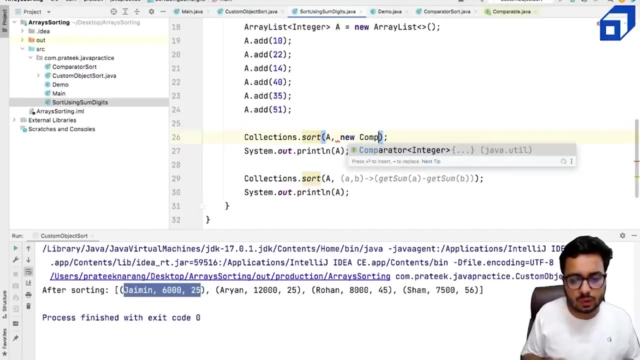 creating a new comparator object. it's an anonymous object. we are not giving you an array list object, we are not giving it any, and in this object we have to override the compare method right. so i'll just write this part again. once you will see, if you're using intellij, it will come using the auto. 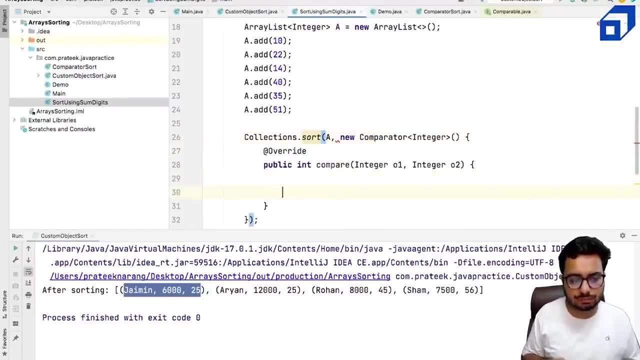 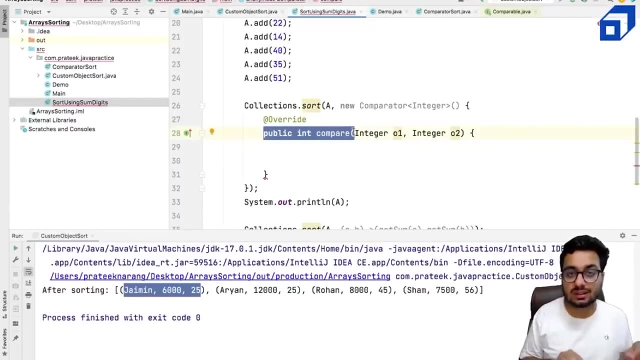 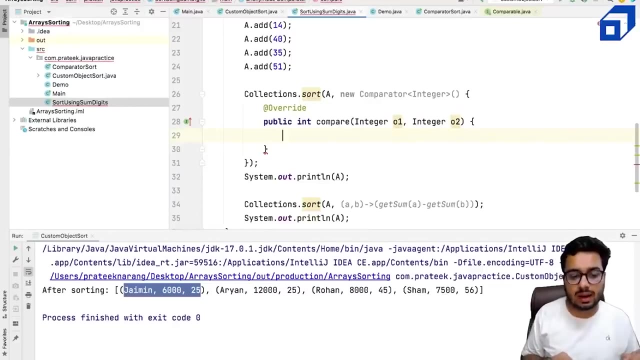 complete feature. i create a new comparator object and in this it automatically creates method called as public int compare. note that it is not compared to this method. it's going to accept two objects that you want to compare and you want to tell how do i compare these two objects? okay, if there are. 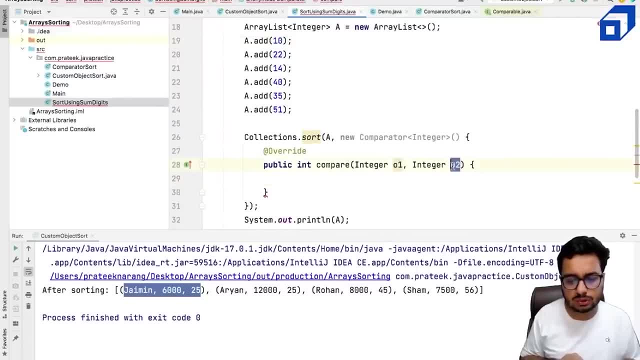 simple strings, so integer o1, integer o2. let's say first object a is 10, b is 20.. if you simply return a minus b, that will simply compare these strings based on their values. that means okay 10 minus 20. sorry, o1 minus o2. first object minus second object. i can do that right. 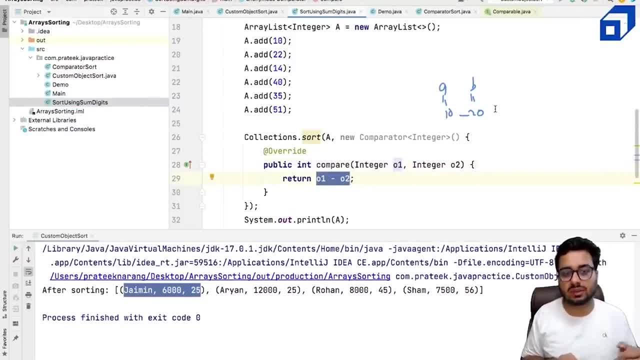 that will say, okay, 10 minus 20, it's a negative number. that means 10 will come first. but if i do it other way, if i say i will negate this entire comparison, that means i'm doing o2 minus o1. that means this list will be sorted in the descending order. but suppose, if i want to do, 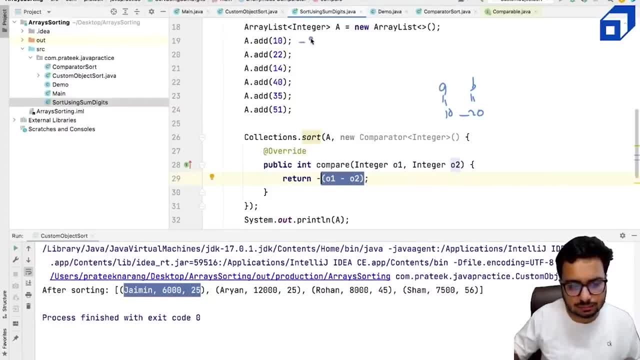 based upon the sum of their digits. okay, for example, this is 10.. the sum is 1 plus 0, that is 1. 2 plus 2, that is 4, 4 plus 1, 5, 4 plus 0, that is 4- 35. 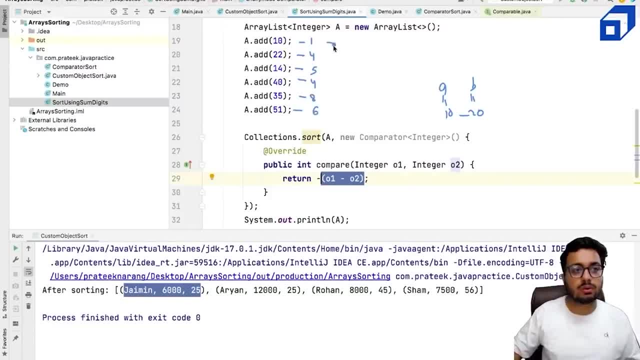 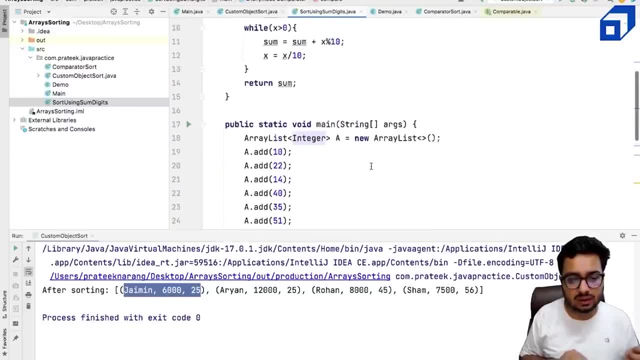 3 plus 5, 8, 5 plus 1, that is 6.. i want to sort according to this what i can do. i can convert an integer into its sum, right, what i have done? i've written a function called as get sum given. 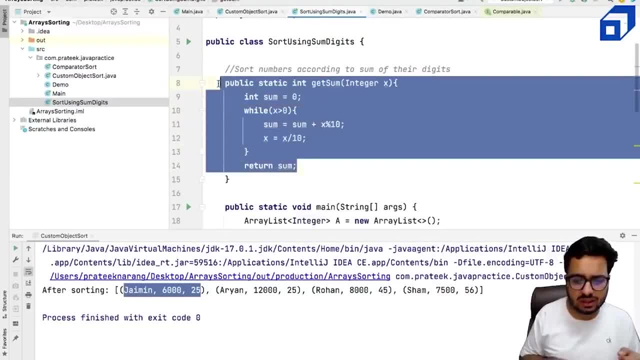 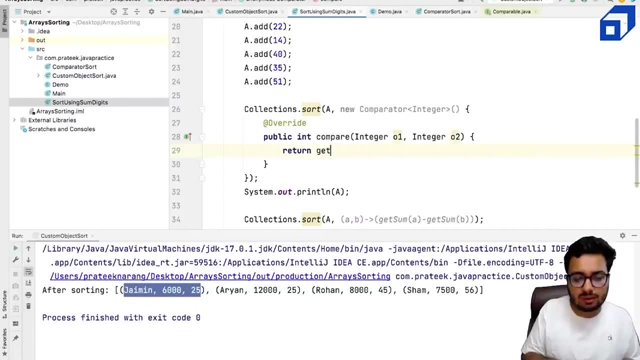 an integer x. i want to get the sum right. so this is very easy. you know how to find the sum of an entity when i'm making a comparison. what i will do else. okay, i'll get the sum of first integer object. i'll say: get sum of a. 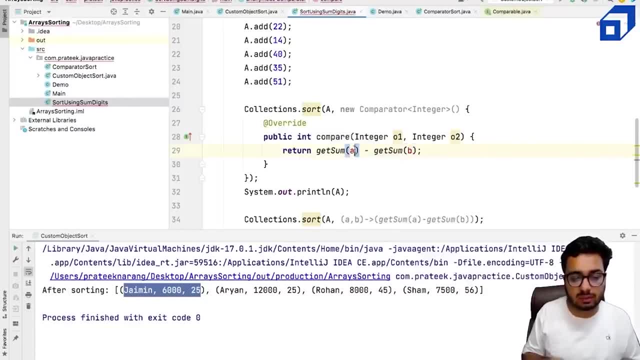 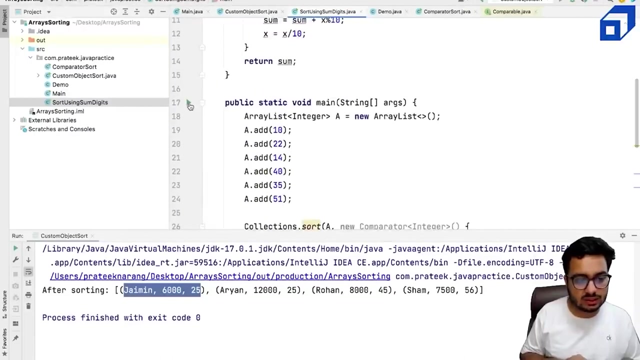 and i will subtract, get sum of a is my object o1 and b is my object o2. if i do this, what's going to happen? so numbers whose sum is lesser, right? i'll just comment this code out. i'll show you the output. i'll show you the output. let us then this code once, right? 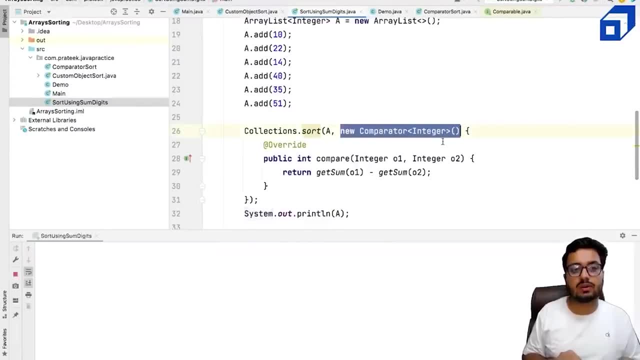 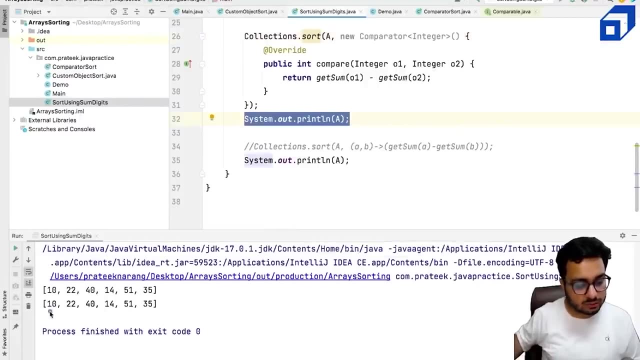 this comparator is telling the code function that now you have to compare the objects using the following criteria: okay, so i've printed it twice. now, if you look carefully, one plus zero is one, this is four, this is four, this five, this is six and this is eight. now you look carefully at these numbers. they are sorted. 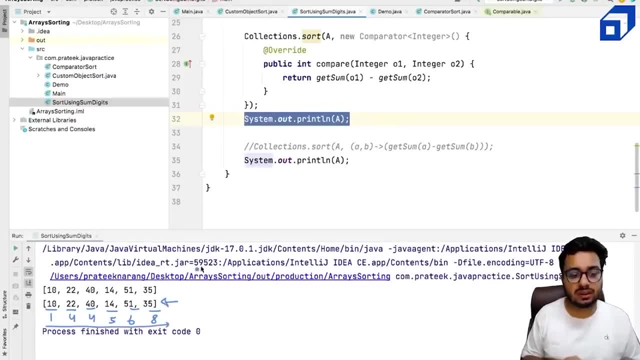 according to their sum. that is something that you can do, right? you can do the same thing with strings as well. you can do the same thing with employee as well. you do not want to implement the compare to method inside the employee class. you can use a comparator, or you. 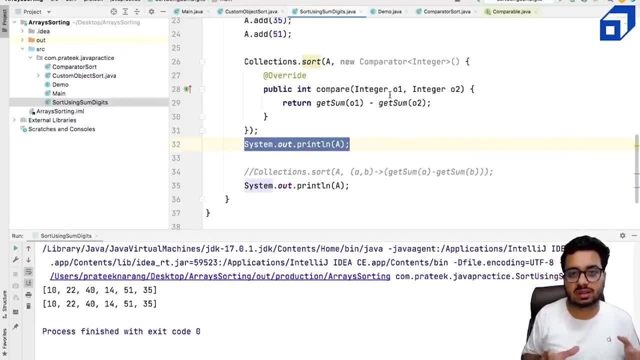 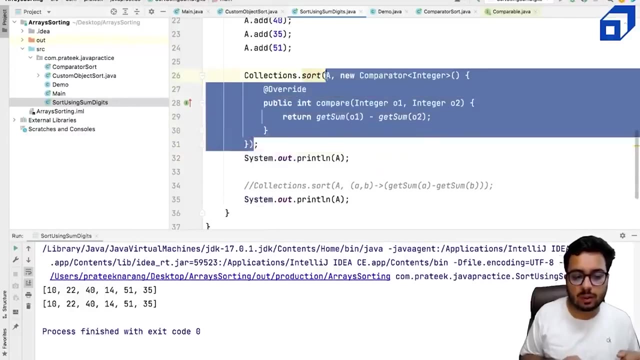 want that. on the top of it, i need another comparison based upon certain condition. right, if employees are uh near their performance period, i want to compare according to their salaries, not according to their age, so you can have that comparator. gives you another option to do the sorting right. you might say, okay, this looks uh little tricky, is there a shorter is? 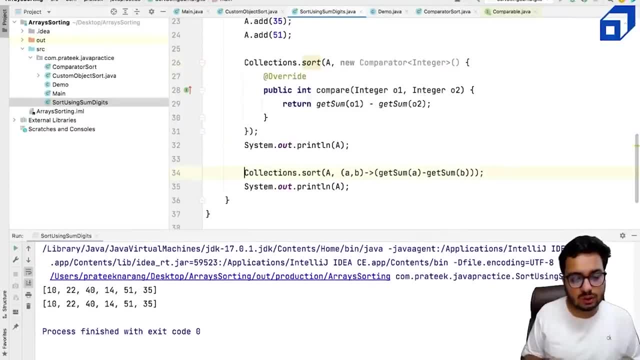 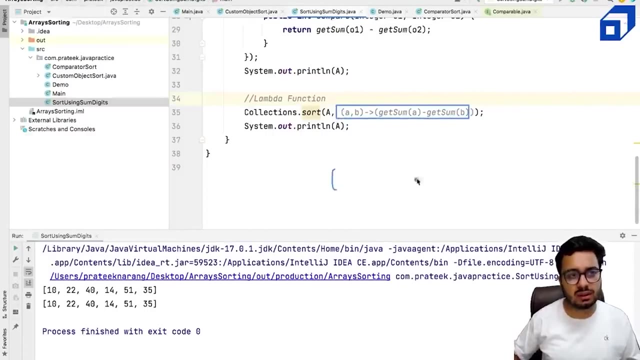 the easier way to do it? the answer is yes. so what we can do, we can use something called as a lambda function as well. i'll just tell you in a very short way what is a lambda function. it's a one line function, it's an anonymous function. so in java, what you have to do, you have to. 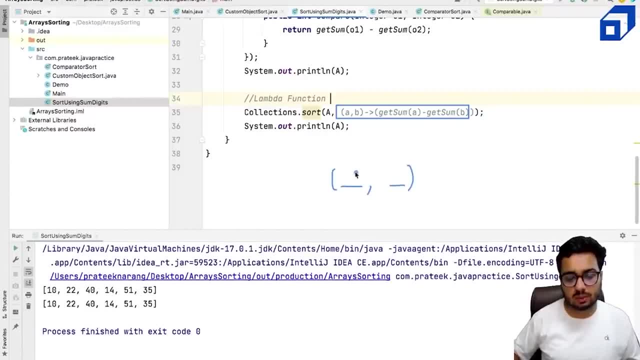 write the inputs that you need to compare in these round brackets. for example, if i'm comparing two objects, a and b, right and with an arrow, you have to write the output of the comparison. now, if you want to compare a and b in this case, what is the output? i'm saying, okay, get sum of a. 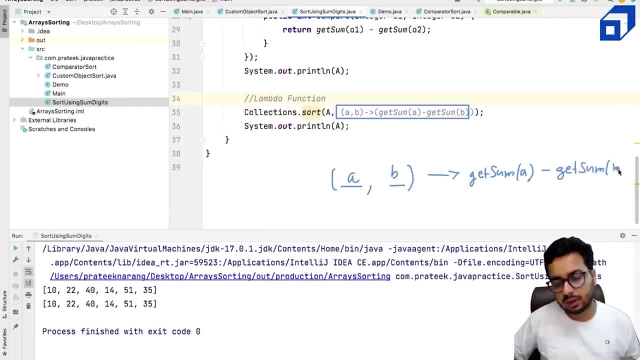 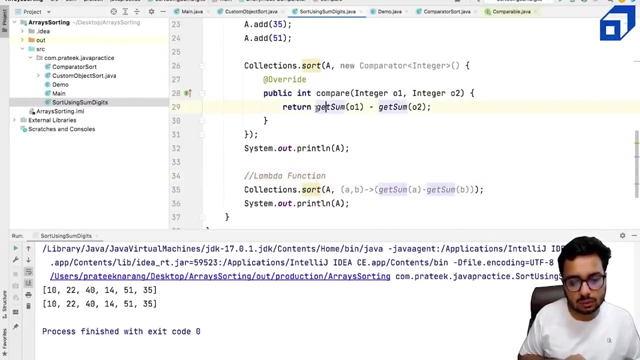 minus get some of. that is what we are doing in the compare function as well. that thing, you put it here and this becomes a lambda function and it will do the trick for you, right? so you can just say that, okay, i don't want to write the compare method, i just want to use this value that is output, and use these numbers that are my. 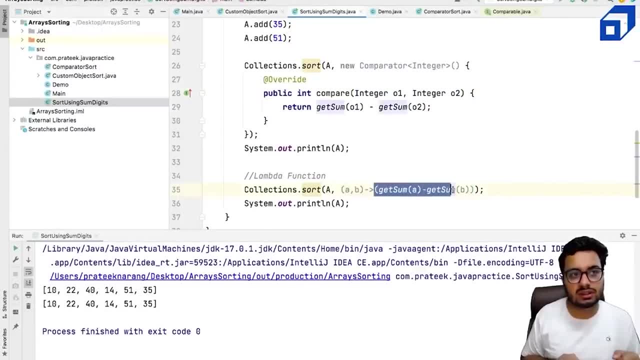 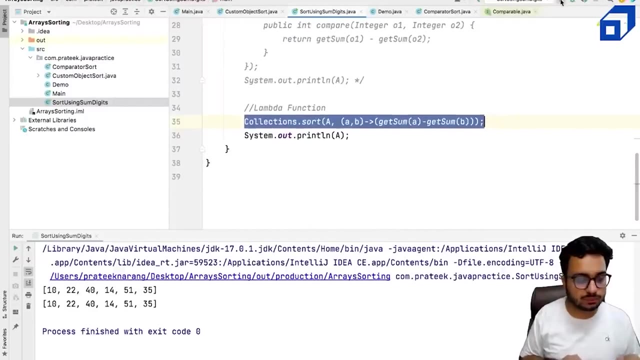 inputs. given these two inputs, i want to return this output from the comparison. this will also work, and if i show you, if i comment this code out, this lambda function will also do the same sorting thing that we want to do. let us start them and let's see what do we get. 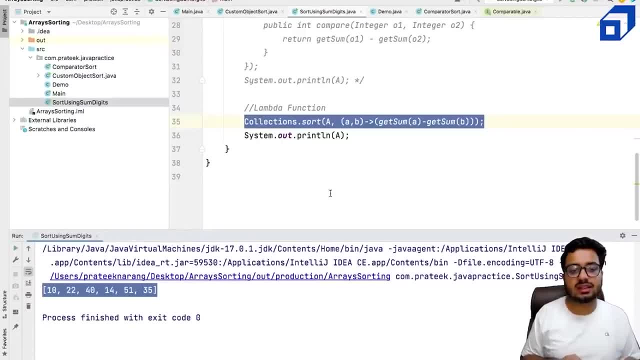 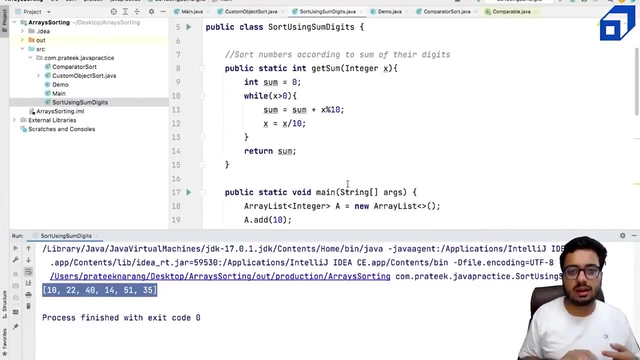 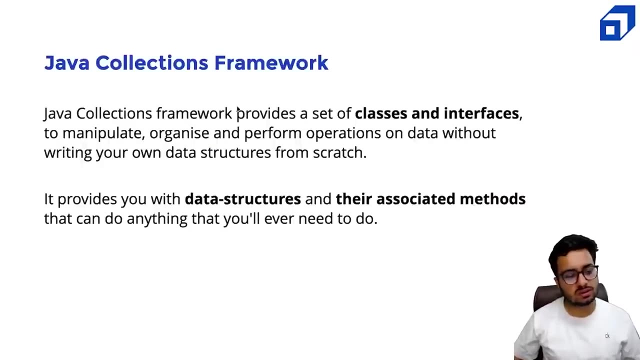 we are still getting the same output. that is another way of doing this one. so hopefully now you have stood the three different ways of doing sort and that's all for sorting and we'll start with the collections framework. next, let's talk about java collections framework now. so java collections. 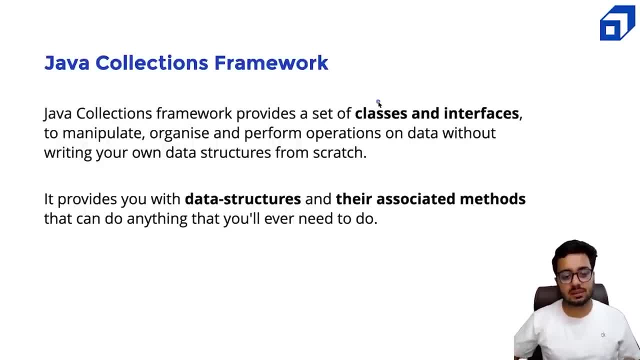 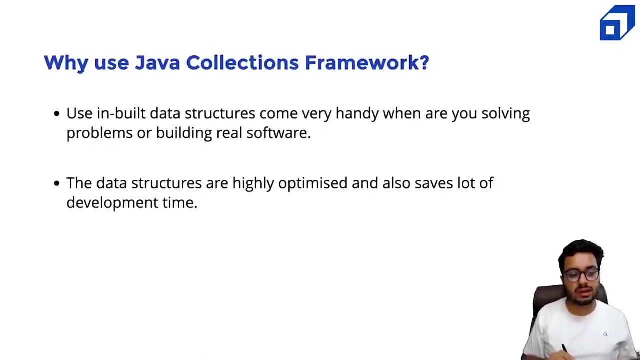 framework is a framework in java that provides us with set of classes, interfaces to manipulate, organize and perform operations on data without writing your own data structures. from scrum. it provides you with library implementation of data structures and their associated methods that can do anything that you will ever need to do right. that means you will be using inbuilt data. 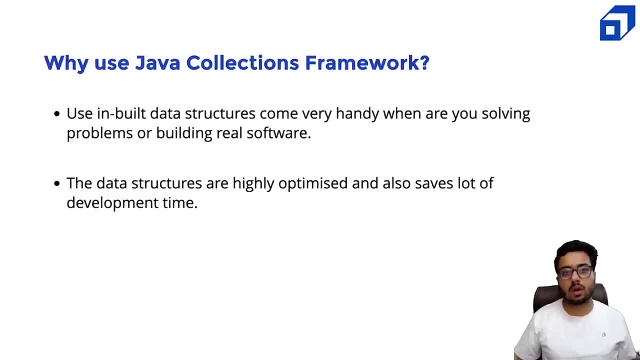 structures because they come very handy when you are solving problems or you are building real life software. these data structures are also highly optimized and they will, of course, save a lot of development. so you don't need to write your own hash table. you don't need to write your own link. 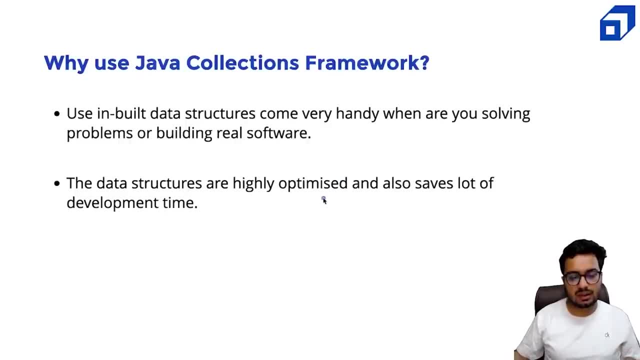 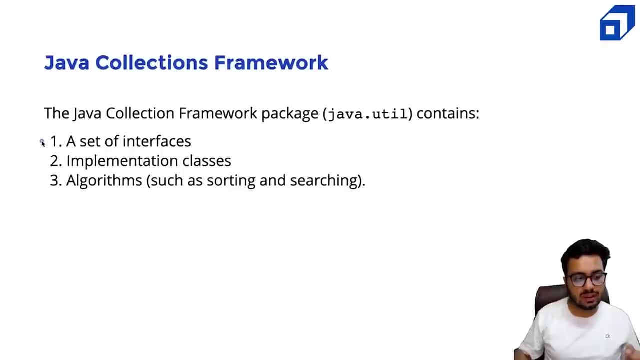 list right. so this is what is a standard practice we will most of the times we would be using the library implement. just to summarize once again, what do we have? we have set of interfaces- we'll see. we have implementation classes, the classes that actually implement those interfaces. 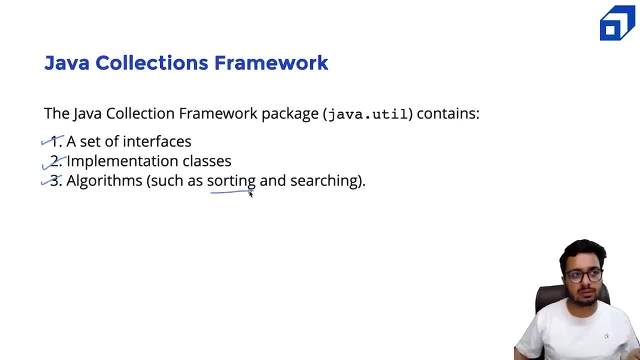 and we have also algorithms, okay, so i showed you the examples of erase- dot sort method, collection dot sort method. similarly, we have methods for searching, like binary search, available in the java collections, so you can just go and look at what all those methods are. but for now, what i will be doing i will be doing is i will be doing a little bit of a. 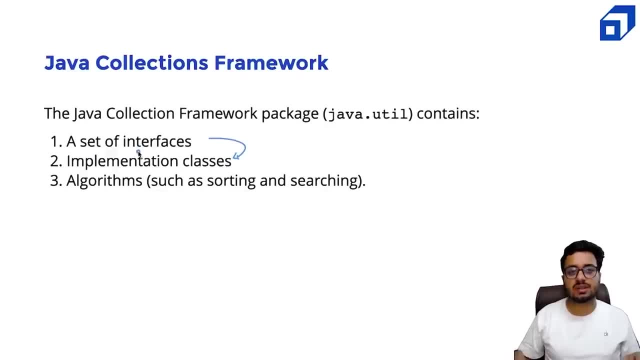 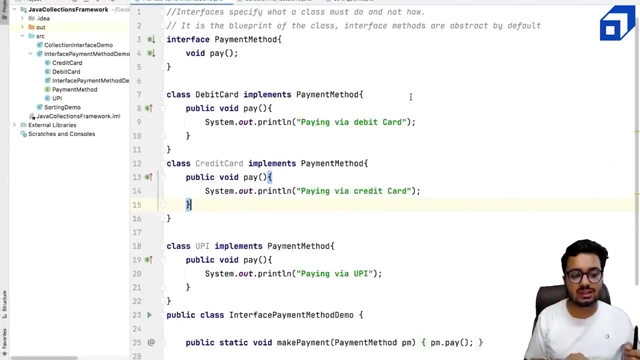 quick demo of interface versus a class so that you can really understand how these interfaces and classes are being organized inside the java collections. right, let us jump into a small code demo to understand the concept of interface versus a class in this example. what i have done, i have 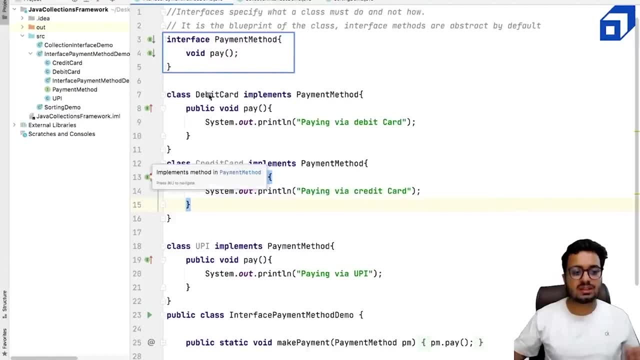 defined an interface called as a payment method. so what is an interface? an interface specifies what a class must do and not how. that means we do not have the implementation of the pay method. we do not know how to make the payment, but we are saying there must be something called as a pay. 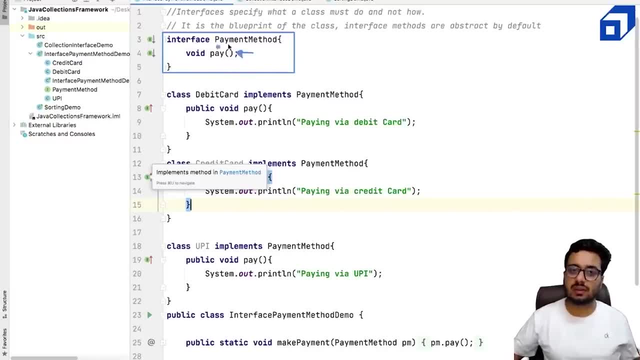 if it is a payment method. any payment method that we have must implement a pay method inside it. so it is a blueprint for for the class interface methods are abstract by default, so they they don't have any code inside. now suppose i have, i'm going to create payment. 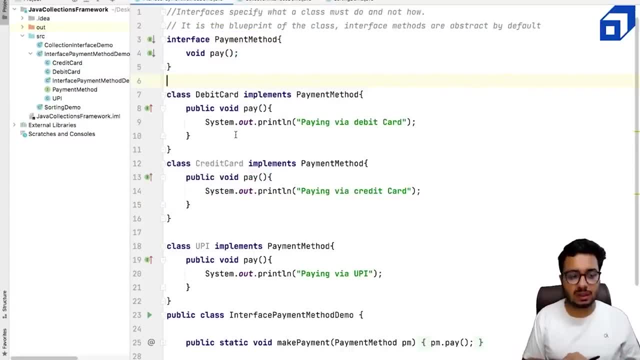 method inside youtube. so today they don't have any code inside. now suppose i have. i'm going to create method called as debit card. so debit card is a class which implements payment method. that means now debit card must define a pay method. it's so for now I'm just saying that debit card pay method. 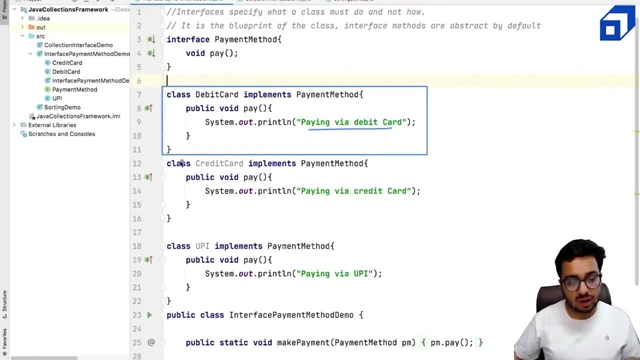 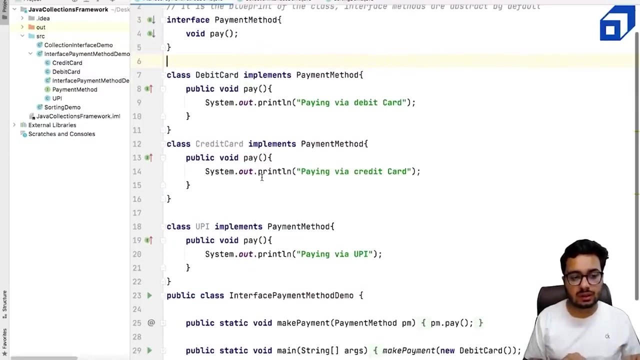 prints paying via debit card. similarly, I have one more class called credit card, which also implements the payment method. I have one more class called UPI, which also implements the payment. all these classes, they have the pay method and they're implementing the payment method. there are different ways of creating the payment method. execution of each payment method would be: 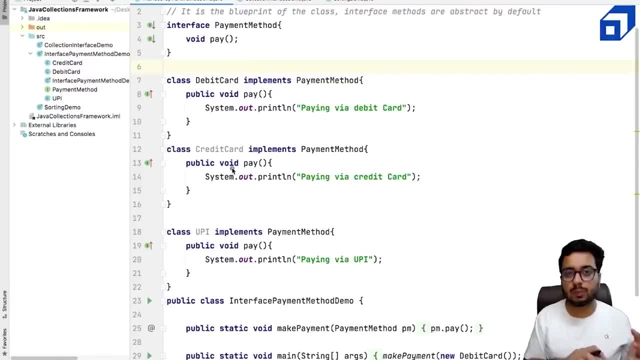 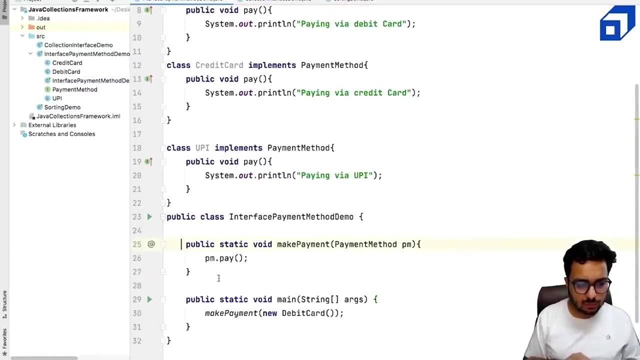 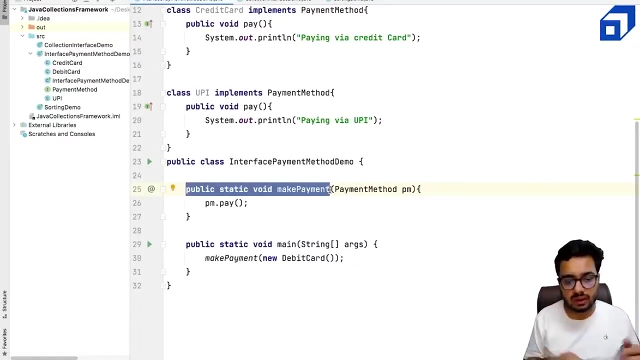 different. if a credit card might have a different mechanism, UPI might have a different mechanism of making the payment. debit card will have a different mechanism of making the payment. why we are doing this? let us try to understand now. suppose we have you method called as make payment and this method can accept any payment method. right, I'm not. 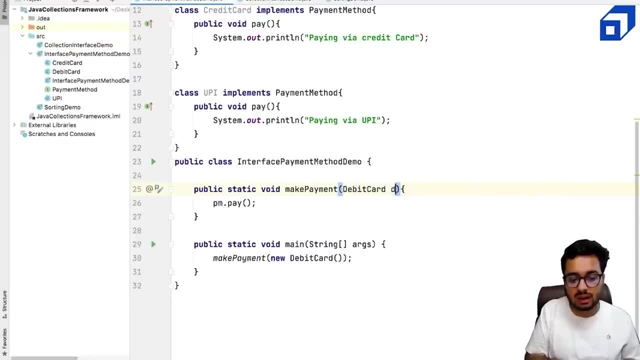 hard coding here. I'm not saying that I will only accept debit card DC. I will not accept debit card. I can accept any payment method. one thing is: we need a general structure. we need a general data type that can hold all payment method, if- and here I'm going to call pmpay. so now, why this? 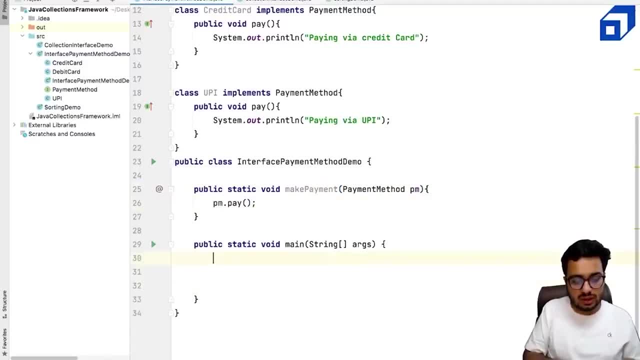 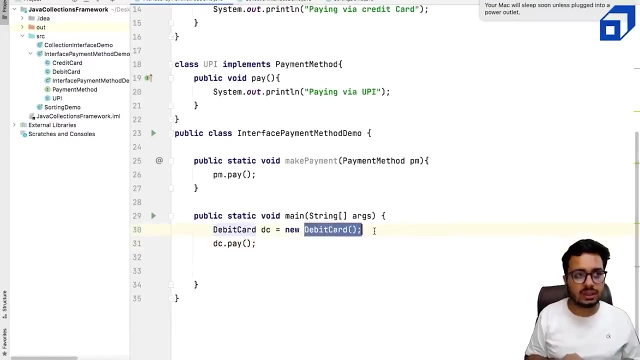 method will work. let me show you how do you create objects of it so I can say, okay, debit card DC, this is equal to new debit card. and I say, okay, I'm creating a debit card. then I can call dcpay, so this will work. I'm creating a debit card object. dcpay will actually work. right, I'm not calling. 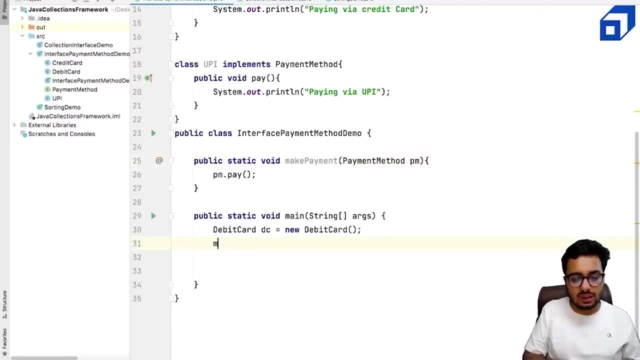 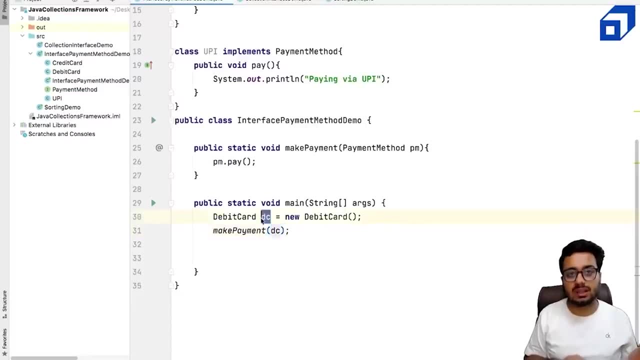 this method as of now. but what I can do is I can call the make payment method and I can pass it the debit card object. so I can call the make payment method and I can pass it the debit card object. why? because debit card object demands the payment method interface. a better way to do it is suppose. 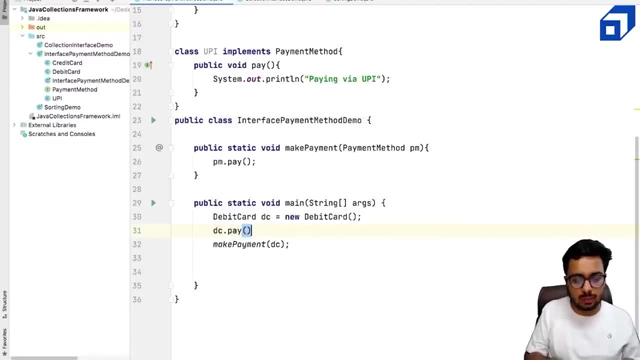 you have like some code here, you say dcpay. suppose your debit card is not working or the debit card service is down or there is some issue and you want to make it change it to the credit card. okay, you want to say, okay, no, I want to try credit card now. if you do this, this is going to 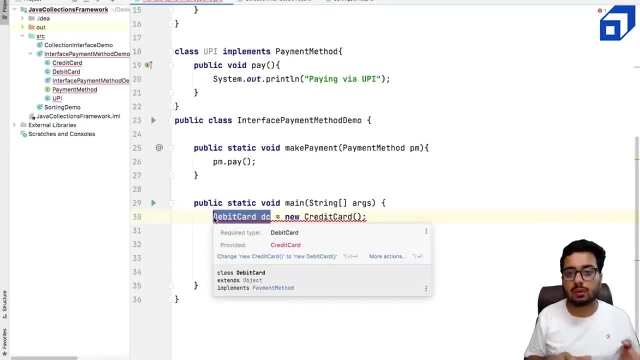 give you a problem because if you do this, this is going to give you a problem because if you do this, a debit card data type cannot hold a credit card right. but what we can do is we can use a more general data type, that is payment. payment method is pm. I can say: okay, on the left side I'll have a. 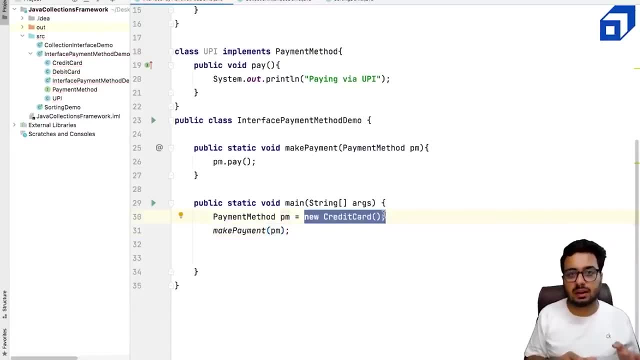 payment method, which is implemented by a credit card right. so payment method is a more general data type. so this is a good design practice as well. so this data type will keep it more generic and this is a specific class that provides implementation of methods defined in this class. this is a specific class. 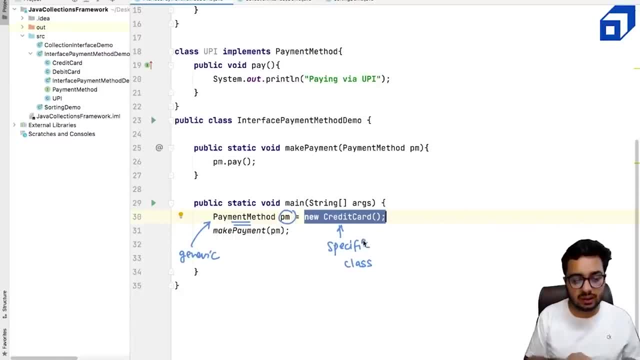 now. this could be credit card, this could be debit card, this could be upi. right, and I can pass the. this object: pm to any method: make payment right now. it does not care whether it I'm going to call the pay method of debit card, credit card, upi, whatever is the object. 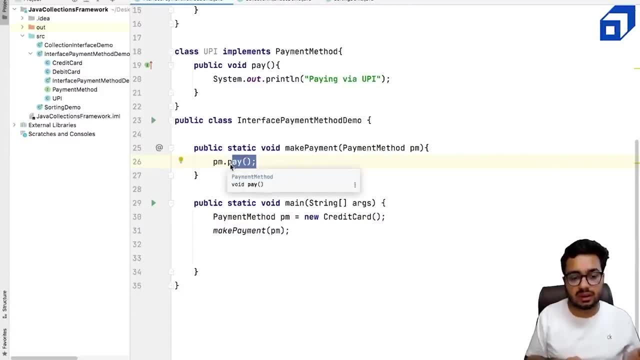 passed, it will call the pay method of that object. so that means with minimum change in code we can keep this general, general behavior right. so any payment method object will work inside the make payment method. if I go and run this code I will show you what's going to happen. 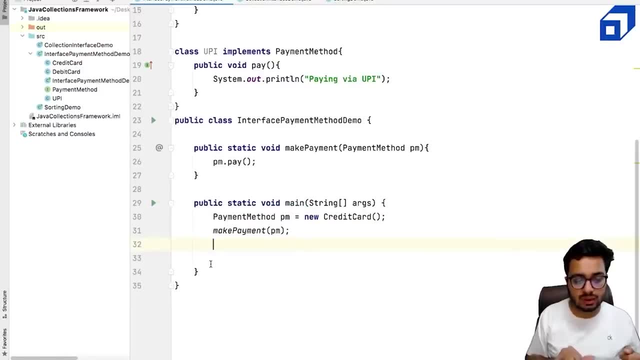 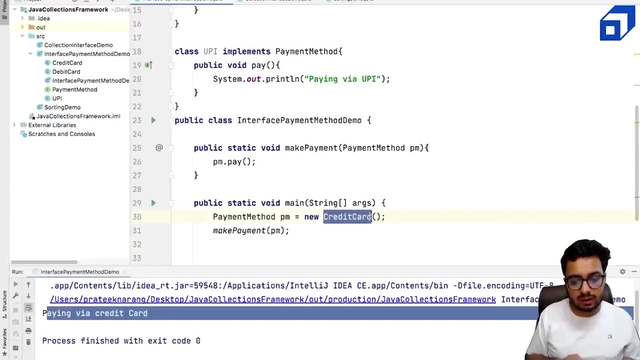 it will say: okay, I'm going to make a payment using a credit card, paying via credit card. but if I say okay, no, I will make it upi without changing your make payment method. you have just changed this object. it will pay via upi. right, going to run this code now paying via you. that means this: 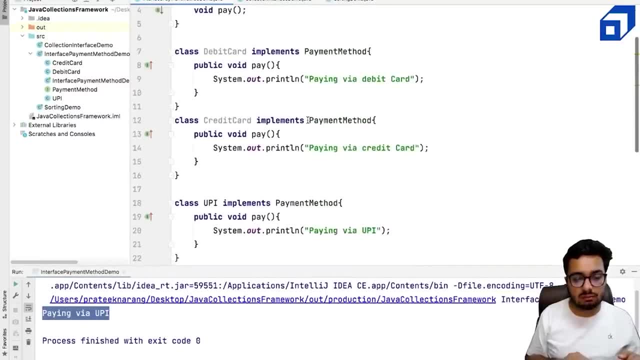 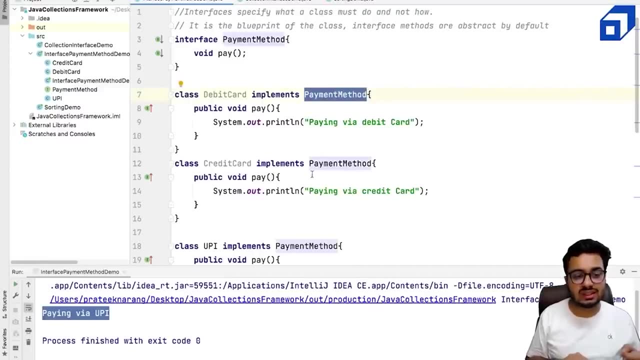 object reference can hold any object like any object which implements the payment method interface. that is a quick revision about interfaces and classes in java and collections framework heavily uses this concept of interfaces and classes a lot. let us look at this is implemented in the collection framework as well. there are so many components inside. 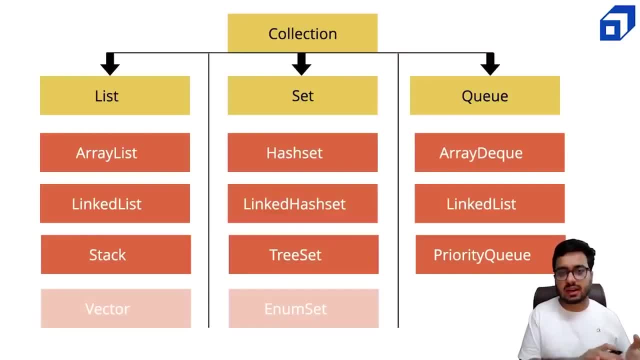 collection framework. there are interfaces, there are classes, there are child interfaces, there are child classes, and the hierarchy is a bit complex. so what i've done is i've drawn a simplified diagram so that you can understand how these components are related. on the top, we have something called as a collection interface. okay, collection is a interface inside collections. 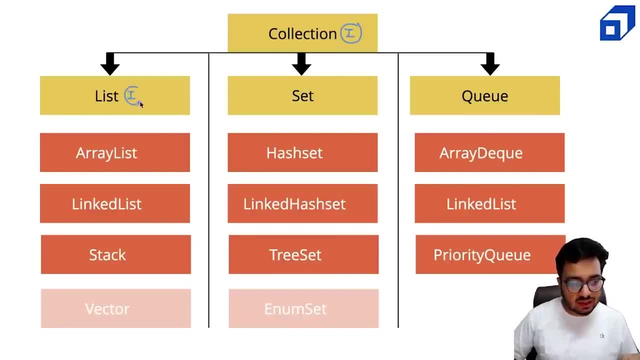 framework. there are three more interfaces which are child interfaces of the collection interface, so they are list, set and queue. they all extend the collection interface. okay, you extends collection, set extends collection and list also extends collection. that means some methods are there in collection and list adds some additional methods which are specific to the list. that adds. 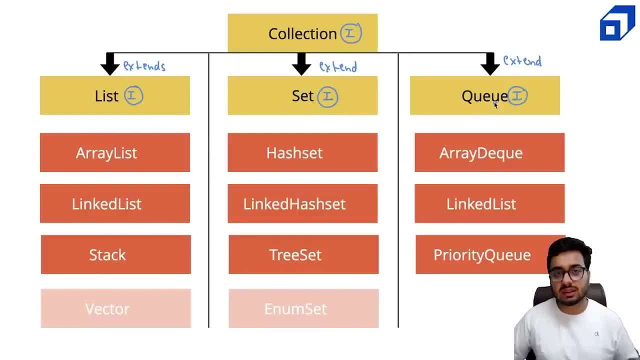 more methods which are specific to the set. queue adds more methods which are specific for the queue, like behavior. and then there are implementation classes which actually implement a list. so array list implements a list. the other way, the array list is going to implement a list. link list is also going to implement a list. 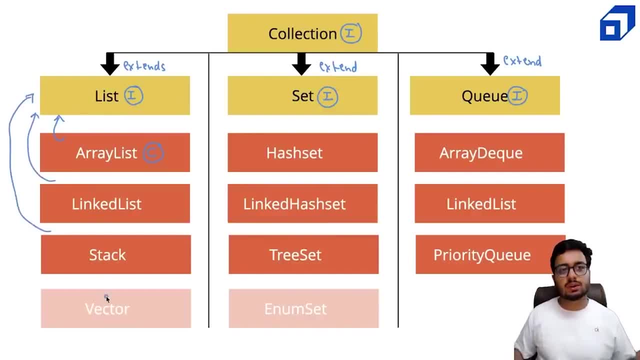 stack is also going to implement a list. vector is also going to implement a list. so a vector is a concurrent list data structure. that means: um, if there, if you need to work, if you need, you need to share this data structure across multiple threads, then vector is the synchronized data structure. okay, so we are. 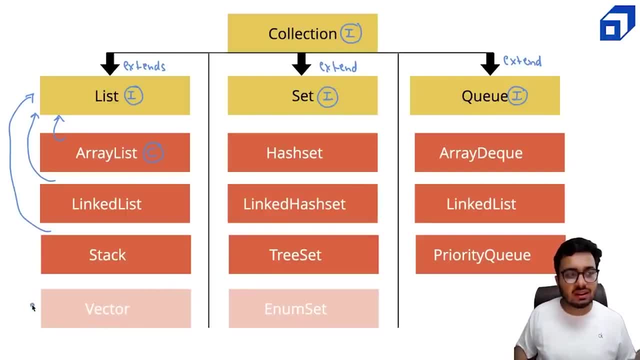 not going to do concurrent data structures in this tutorial, so i will leave vector at the moment. similarly, hash set implements the methods of the set. linked list implements linked hash set implements methods of the set and tree set also implements methods of the set. now what is the? 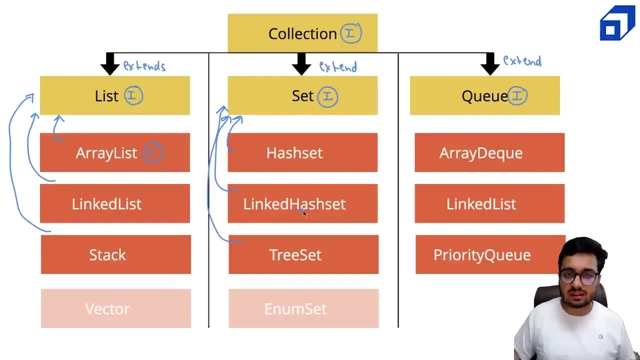 difference, the way these methods internally work, is that if you are applying this methods in a set work, that is different. okay, a tree set might use something like a self balancing binary search tree, whereas hash set might use the concept of a hash table to store the data, right. so the implementation of methods is different. 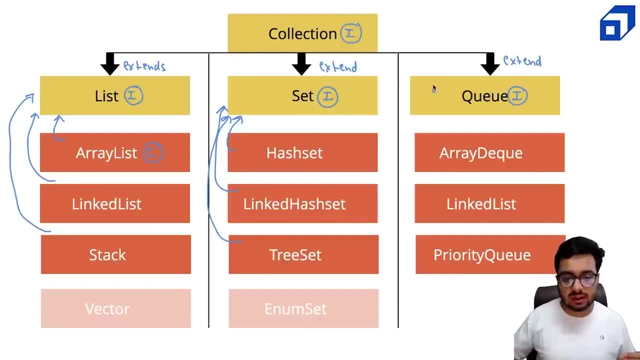 and their time complexities. they are also different. so for queue we have three implementations. we have array deck, which is a double ended queue. we have a link list which is like your, which serves as your FIFO link list, and there is a priority queue which again internally uses a heap like data structure to give. 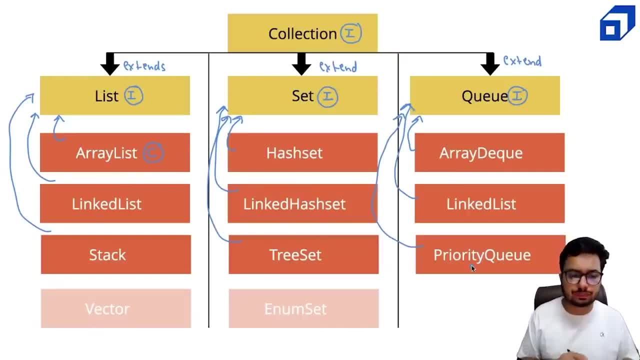 priority to the elements which should come first, right? so we have interfaces and we have classes that implement those interfaces. the ones that are in the orange, they are the classes. the ones which are in yellow, they are the interfaces. right? I hope you understood this simple hierarchy. now you might be. 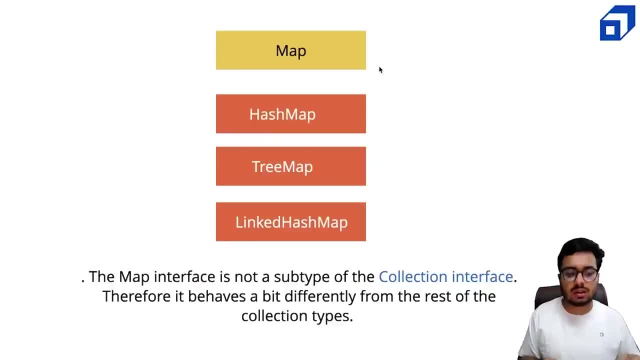 wondering: where is a hash map? hash map is not part of collection interface. it is not a subtype of a collection interface. it has been kept separately and it behaves differently from the rest of the collection types. so that means the map will be treated differently. so map is a. 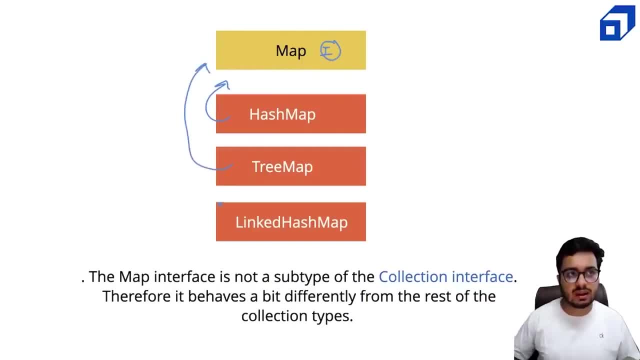 interface that we will look and hash map, tree map and linked hash map. they are the implementations for the map interface. right, we will use one of these implementations if you want to build up something like a map which can store key. we'll understand the differences between these implementations as we go. 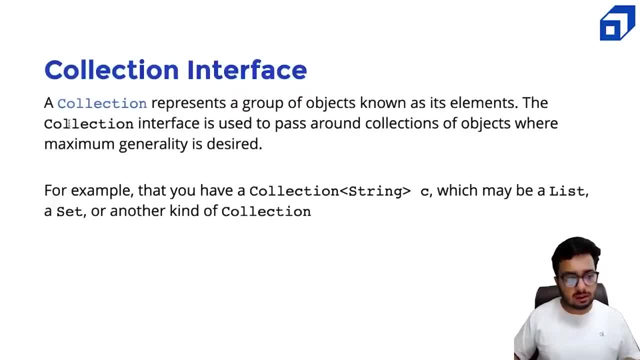 through this tutorial, right? so let me tell you little more about collection interface. the collection interface, it's a general interface. it represents a group of objects which are known as elements, right? so it's simply grouping different objects, and it is used to pass around collections of objects where maximum generality is required. okay, you just want a group of. 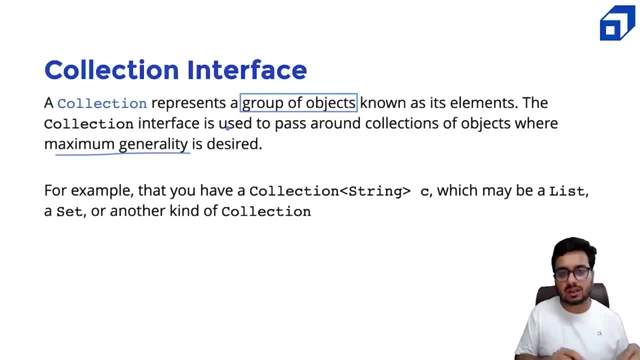 objects. you don't want to use specific priority queue method or specific queue method, or you don't want to use specific hash map method, right? so you just want some general methods that i should be able to add into the collection. i should be able to remove from the collection. i should be able to delete from the collection, right? for example, 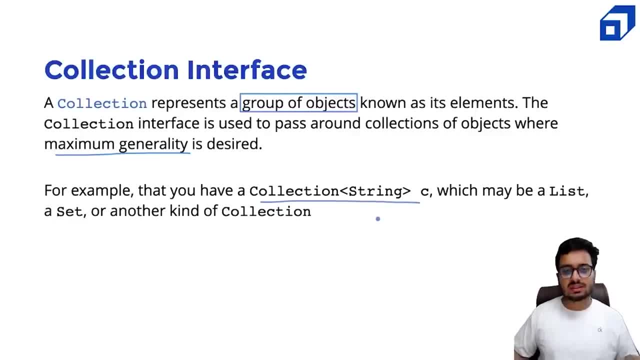 you have a collection of string. of this collection, again, it might be implemented using a link list. it might be implemented using a set. it might be implemented using a error list, we don't know. right, we have to provide one way: implement or represent this group of strings, right? so let me show you a 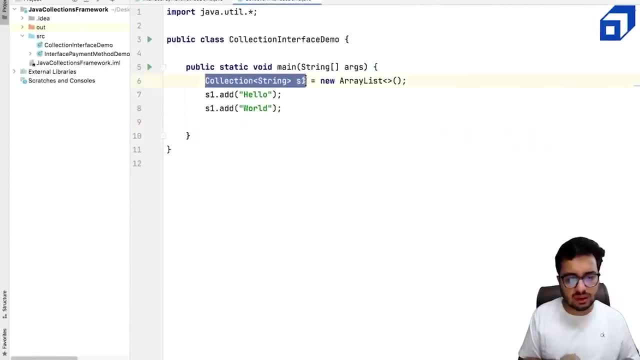 code demo here. so i have collection of string s1. this interface collection is an interface, so i need a class to implement it. files- okay, this collection will be stored using the error list. so i'm adding something into the error list, right? i'm saying s1 dot add. hello, s1 dot add. 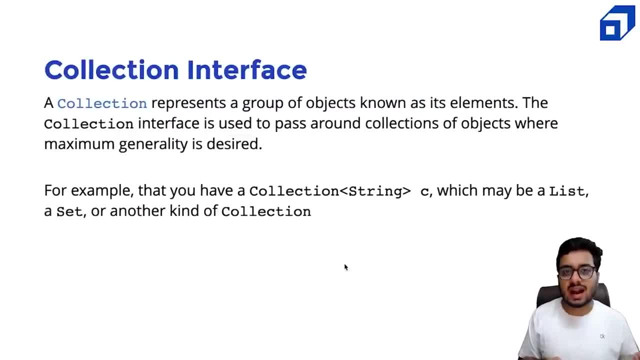 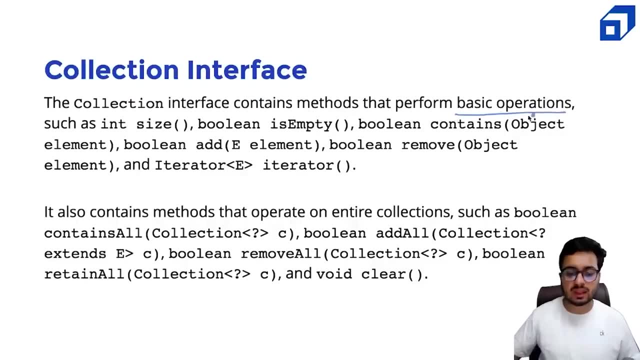 world right now. you might ask. you might ask: where is this add method defined? so i will tell you. the collection interface contains method that performs basic operation. okay, so, such as size, every data structure you need to get its size. every data structure should know whether it is empty or not. every data structure should know. 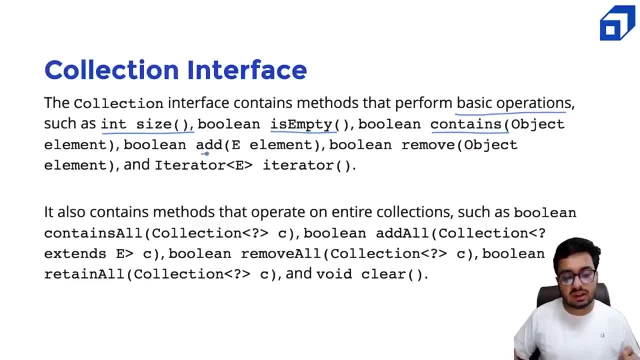 whether a particular object is present inside it or not. every data structure should support that. i want to add some element. i want to remove some element. i need a iterator right. it also contains methods that operate on anything, entire collections, such as add all. given another collection. can i add all the elements of this? 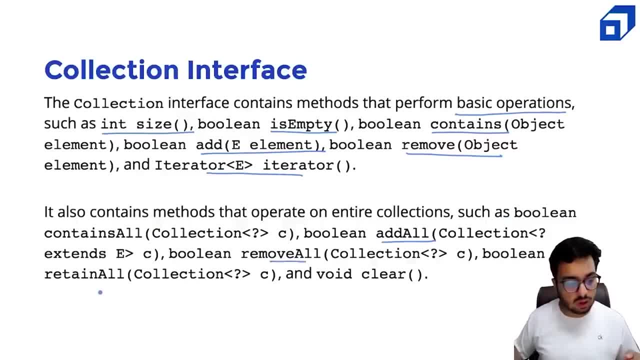 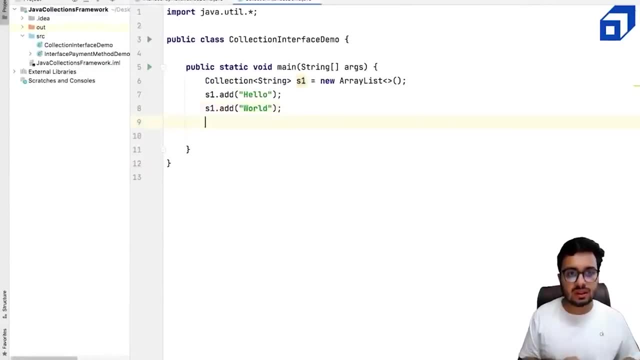 collection into the current collection. yes, i can right, remove all, retain all clear, right, these are general methods that are defined in the collection interface. that means all the implementation classes will have to define these methods. let me show you, uh, something here. so let us say i create one more. 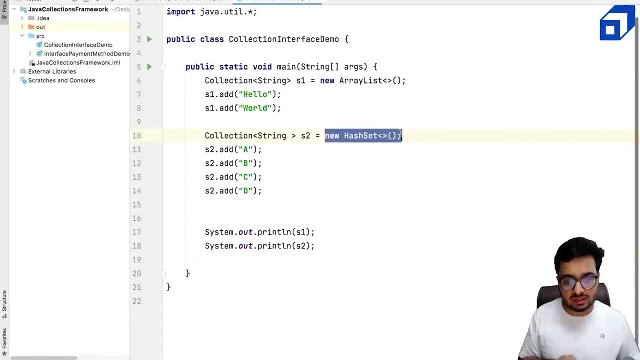 collection and this collection is implemented using a collection interface and i can add all the a hash set. now in this asset. i am adding q of strings a, b, c and d. right now. this add function is going to behave differently from this add function because this add function is implemented. 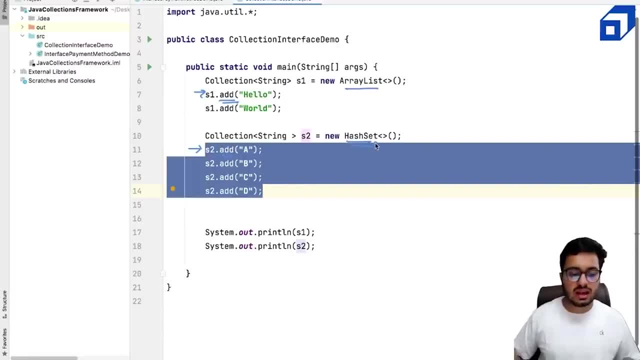 by the array list. but this add function is implemented by the asset. so if i print s1 and s2, i would be able to see: okay, there are two group of elements. okay, if i just run this code, i'll say, okay, i have a collection s1 and i have a collection s2. now suppose i want to add all. 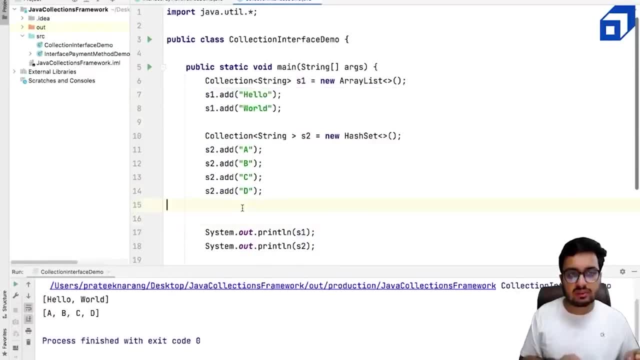 elements of s1 into s2. can we do that? of course i can do that, because the collection interface gives me methods like add all. so s1, dot add. i can give any collection here. i can give list, i can give array list, i can give q right, i can say okay, uh, in my hash set. 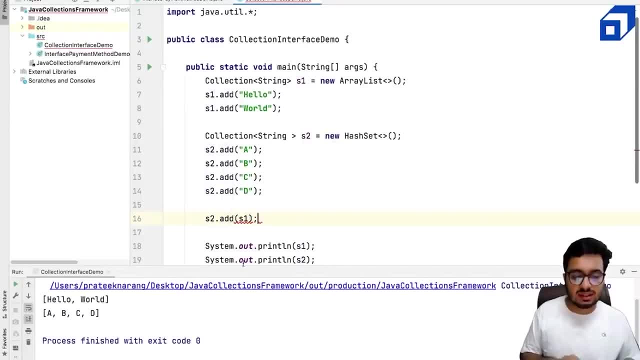 i can say: okay, i have a collection s1 and i have a collection s2, and i have a collection s2. i want to add all elements of array list that is s1, so i can pass another collection into my add all method. method is add all, right, so it's a general method. any collection can be passed. 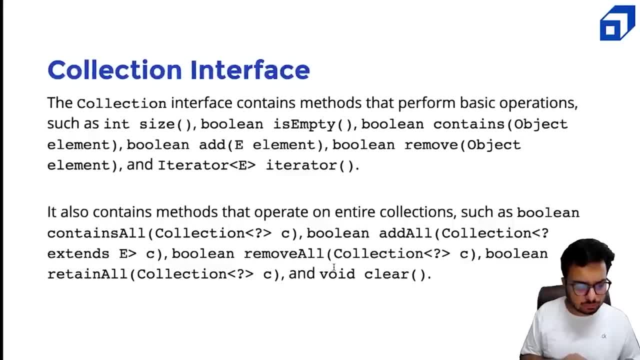 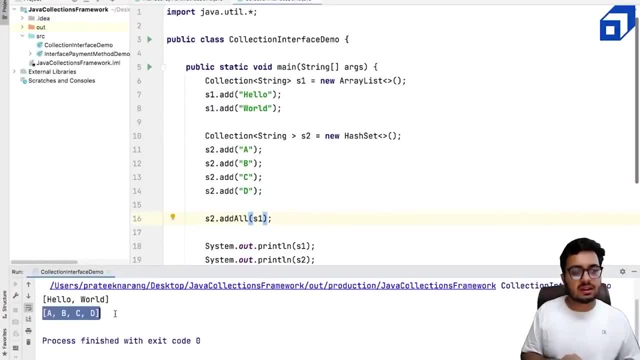 this is what it means. right method is add. all that's correct, so let's go and run this code now. if i see a, b, c, d it's here, i will also see hello world is also there, so you can see all elements of s1. they got added into it so i can say, okay, i have a collection s1 and i have a collection s2. 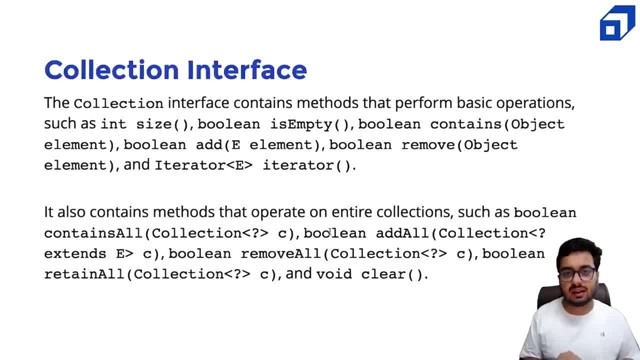 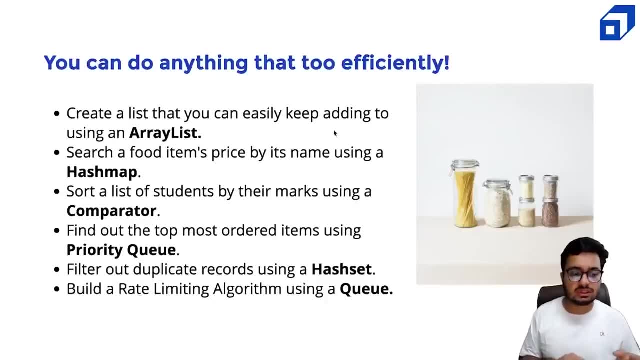 right, all these general methods. they are defined in the collection interval. okay, i hope you are understanding it. so that is at the top right now. why we are learning this? because we want to use this data, such as to solve problems efficiently. it is so powerful that we can do a lot of things. 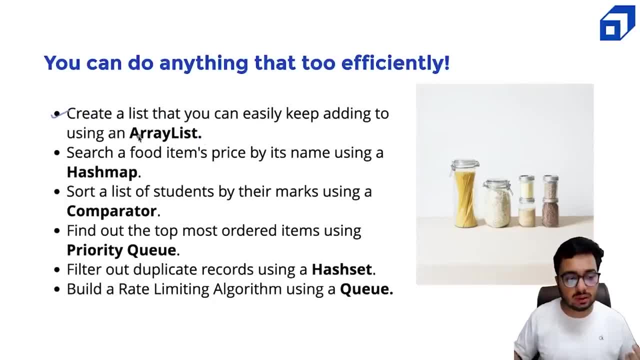 for example, we can create a list in which we can keep adding to. we just saw an example of array list. we can search items very quickly inside a hash map. we can sort a list of students by using a comparator. right, we have just seen comparators. you can also find top most ordered items using a priority queue. 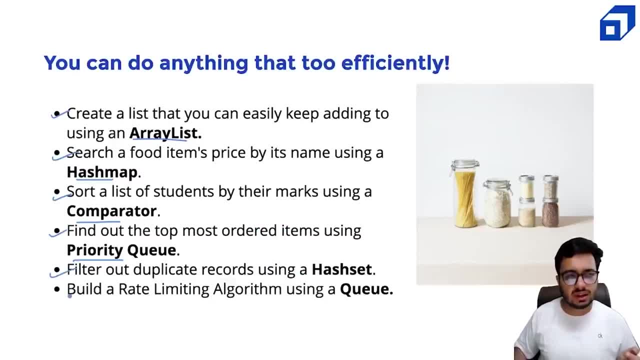 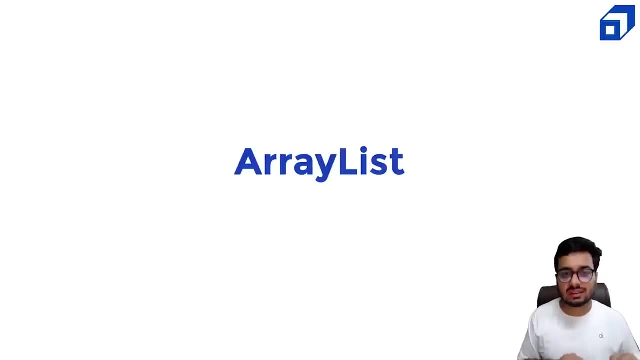 we can filter out duplicate elements using a hash set. we can build a rate limiting algorithm using a queue. we can do a lot of stuff using the collection framework, and that is why we are learning it now. next we will dive into specific classes, and the first class that we will start is: 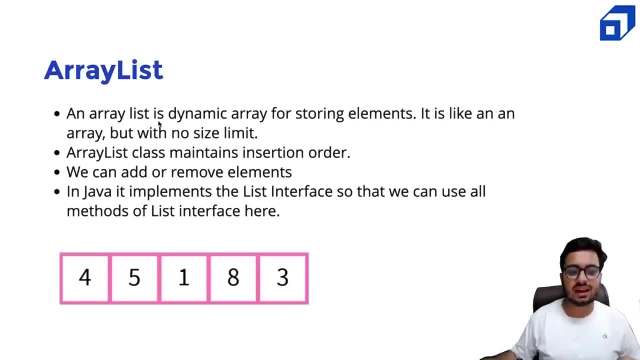 array list. let us talk about array list. so array list is like a dynamic array for storing elements. it's an array list. it's a dynamic array for storing elements. it's an array list. it's a dynamic array but with no size limit. that means if an array gets full, it will grow in size and it can accommodate. 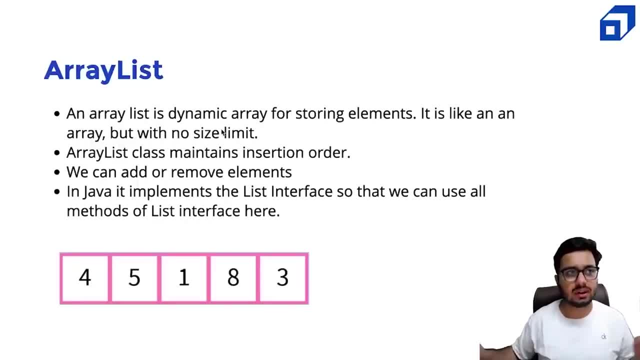 more elements till you have memory available inside your heap right. so array list class: it's a dynamic array. it maintains the relative insertion order, so if you add element it will always get added at the end. so that means we'll get the same order as insertion. we can add or remove elements. even we 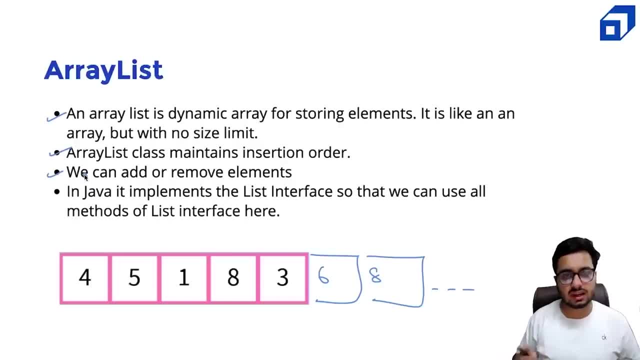 can search for elements and it implements linear search. that means it will take linear time to search it. in java it implements the list interface. so we saw that list is a interface and array list is a implementation of list interface. all the methods that are available in the list interface are: 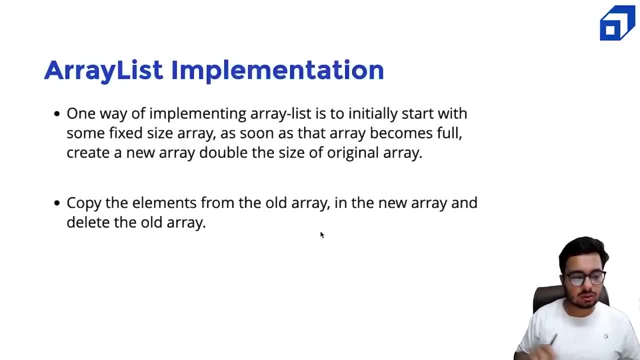 implemented by error list. now how it is going to work internally, so i'll give you a quick idea. so internally it uses a fixed size array. only right? so it starts with some fixed size array. so in java the default size is 10, so by default it will create a new array of size 10. 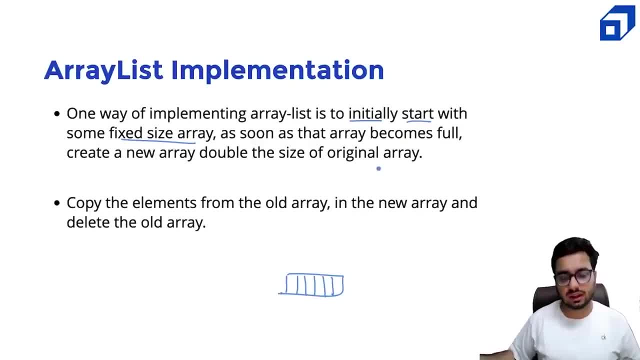 as soon as the array gets full, it will double the size of the original. now that doubling cannot happen in the same place. suppose this array was full. right, what it will do? it will create a new linear array. suppose this size was 10. it will create a new array of size 20 and it will copy. 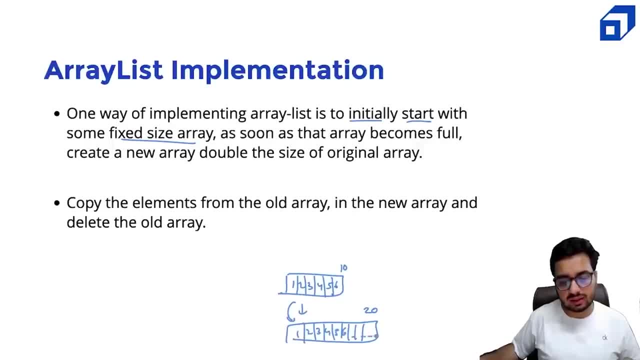 all these elements into the new array and then you will have some extra buckets for new elements. once this gets full, it will again delete the previous array. it will create an new array of double the size copy elements here and delete this area as well. this is how it happens. 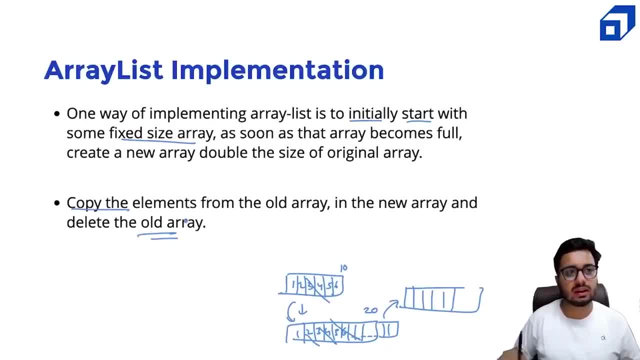 copy the elements from the old array in the new array and delete the old. this is how this array actually works. that means the doubling of the array list is a expensive operation and we should reduce the frequency of this doubling. how do we do that if you know you're going to store? 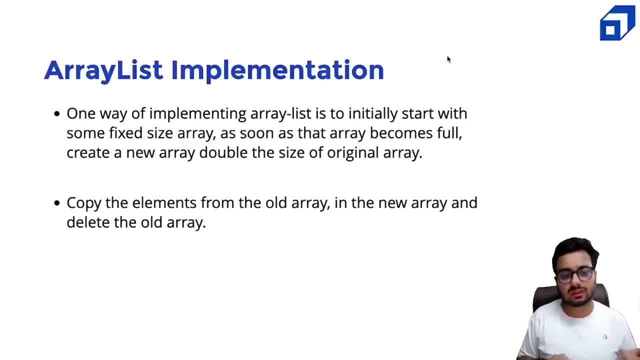 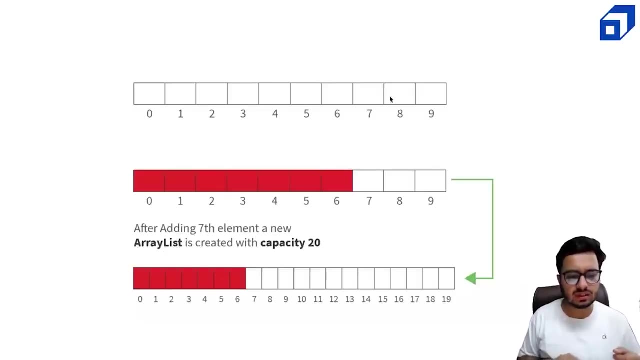 1000 elements. create an array list of initial size 1000.. if, if you by chance exceed one thousand, the doubling will happen. the array size will become 2000, right, so it's good idea to start with the sum initial size that is equal to your requirements in java. this doubling procedure is: 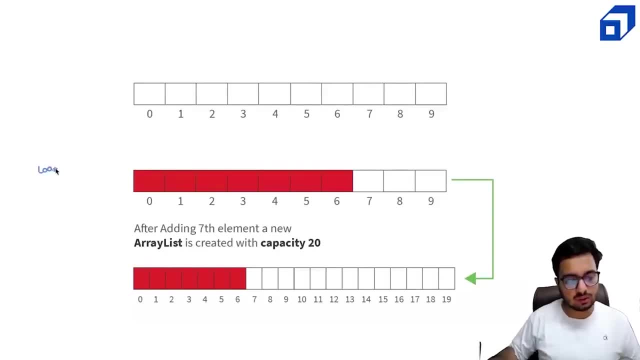 little different. it says: okay, i'll maintain something called as a load factor. this load factor is, i think, around 0.7. that means if 70 percent of your array is full, the doubling will get triggered. so we will not wait till- uh, filling of hundred. 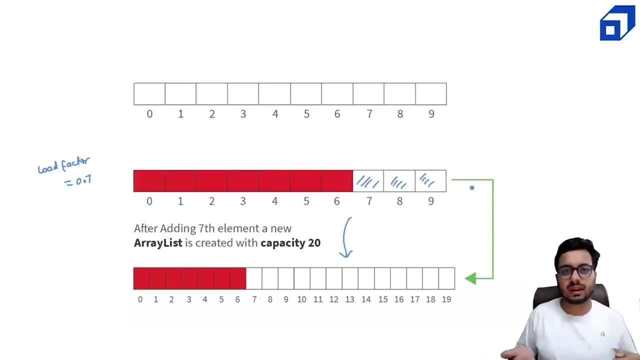 percent of the array. if seventy percent of the array gets full, the doubling gets the doubling function. it's. it's triggered. okay, so after adding the seventh element, if the initial size was 10, new array is created with the capacity of 20.. so there are two things when you talk about size of 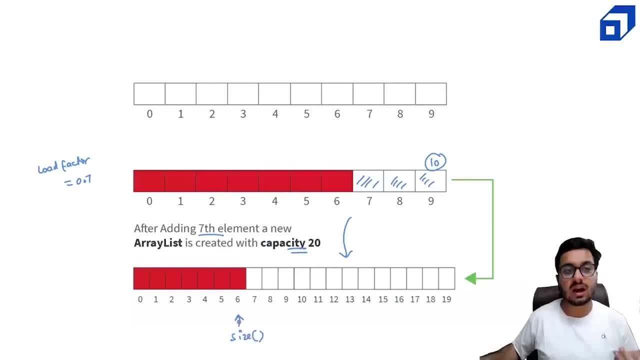 the array list. it tells you how many elements are currently stored in the array list. if you use the size method, it's not the capacity. capacity is generally more than the size. right, the capacity is how how much space has been allocated internally, whereas size is the number of elements that we 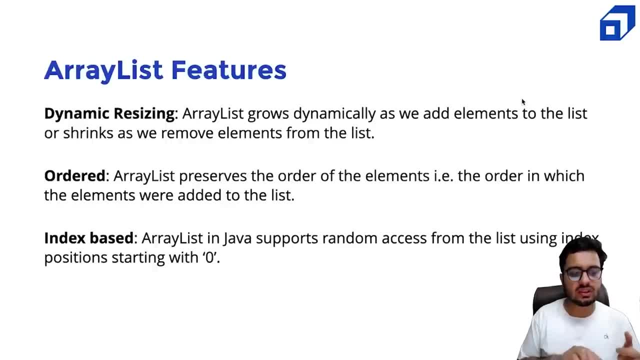 have stored in the array list, right? so what are the features? it is dynamic in size. it can grow and shrink in size. secondly, it is ordered. it preserves the order of elements. third, it has index space, just like an array. you have indices. array list also have indices if you want to access. 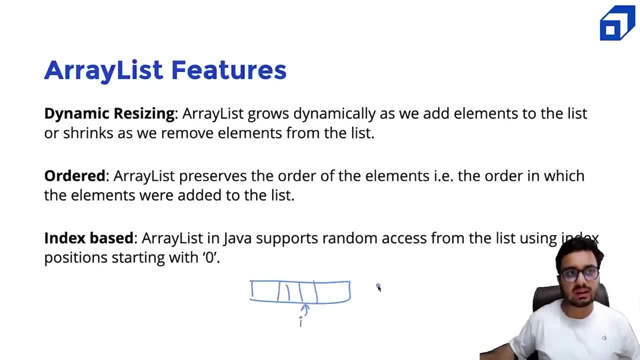 a particular element. okay, i want to get this ith element. you do not write array of i. instead you write arraylist dot get. i give me the ith element. get is a method that you will use to access any ith element, so this also works in order. one time. right indexing is zero based, so another property. 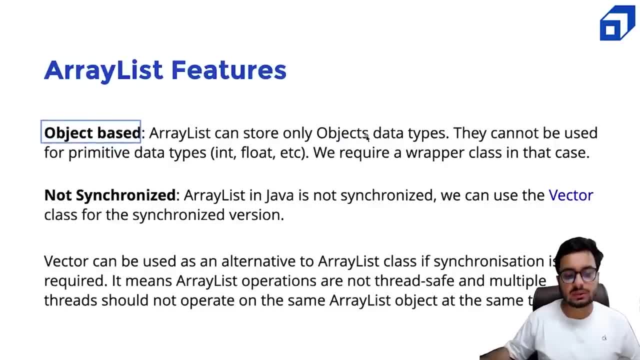 you need to know is it is object based. arrow list can only store object data types. that means it cannot be used with primitive data types. you cannot create an array list of int, float, etc. then you might be wondering: how do we create an array list of integers? for that you have to use the wrapper classes in java, the wrapper. 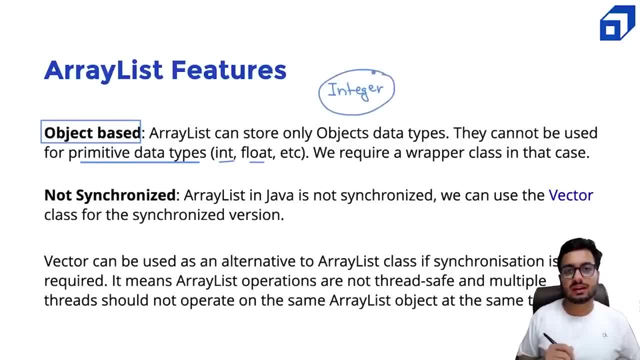 class for int is called as integer, so you will always create an array list of the data type integer, not as int. and secondly, it is not synchronized. that means it's not a concurrent data structure. if you need, if concurrence is important for your application, you have to use vector, which. 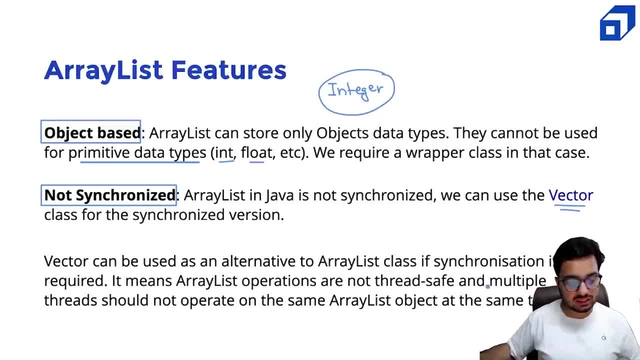 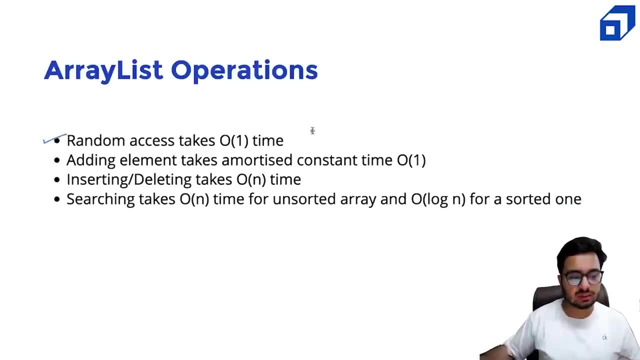 is the synchronized version of arrow list, right? so arrow list operations are not thread safe and multiple threads should not operate on the same arrow list. so this is a basic data success tutorial. you want to learn about advanced concepts? we will cover it in some other video, right? so what are the operations? we can get any element using the get function. 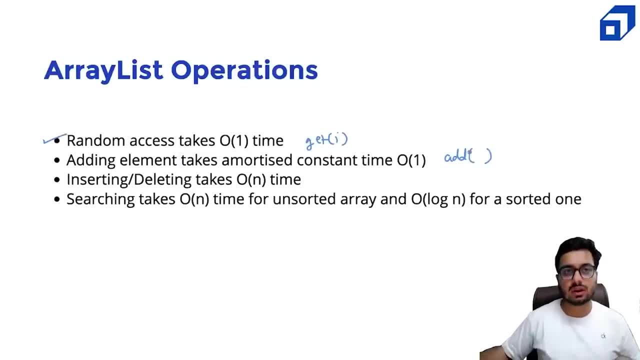 we can add any element using the add function. we can also add more elements using the add all function. so i give you a list. i want to add it. i can use add all. right, i can give some element x that can be added. insertion and deletion in the middle. it's going to take order of end. 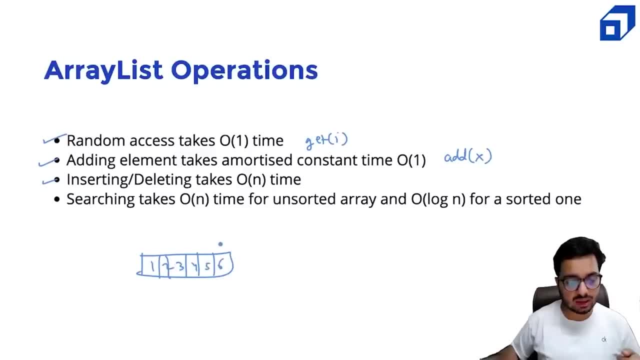 time. so if you insert something in the middle- right, so it is okay, i want to add something in between- it will require shifting of remaining elements. that means that will take order of end time. searching takes order end time. so by default, if you use the contains method, it's going to do linear search, right? 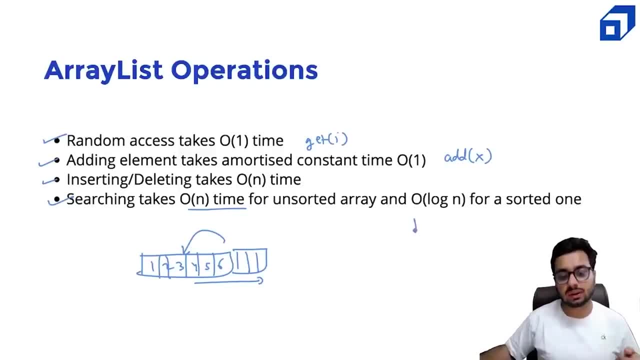 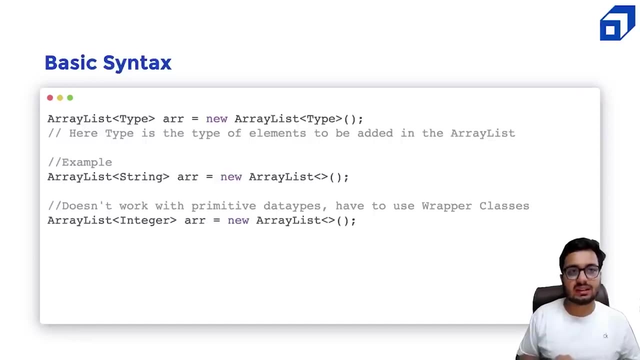 but if you know the array list is sorted, then you can use your own binary search method or the binary search provided by the library function. you can use that as well. that searching will take login time if your array list is already sorted. right now let us look at basic syntax: how? 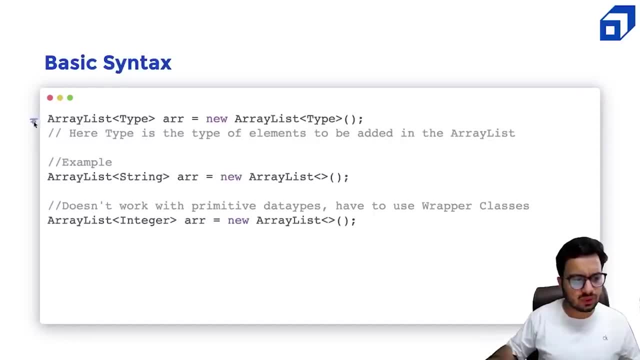 we can create an array list. array list- this is, you have to define what kind of objects you want to store here, right, and then use: okay, i want to create a new array list object, right. so this is how we do it. for example, you can create an array list of strings and you say it's a new. 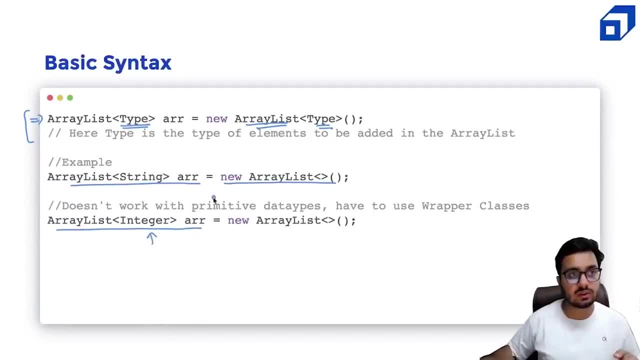 array list. you can create an array list of integer right. i told you it does not work with primitive data type. you have to use other upper classes. okay, in general, i would make this left data type to be of the list type, because array list is a type of a list right. 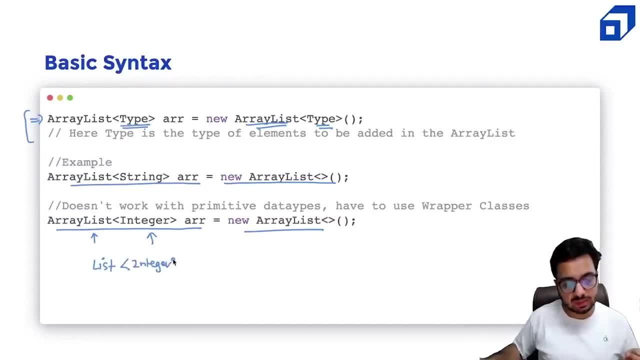 and as a good design principle, it is preferred that we make this data type more general as possible so we can say, okay, the list we are creating an object of the type list implementation is given by new array list. this is a more recommended thing to do, right then, doing array list right. this you will learn in the design. 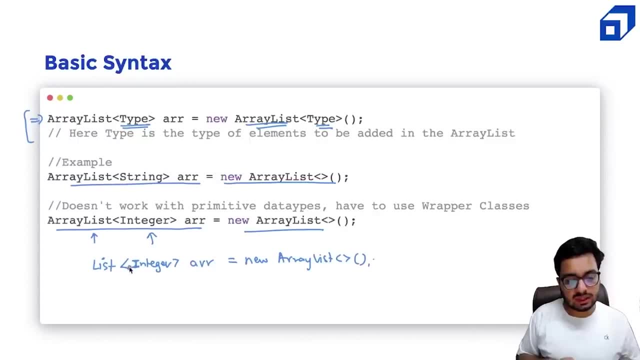 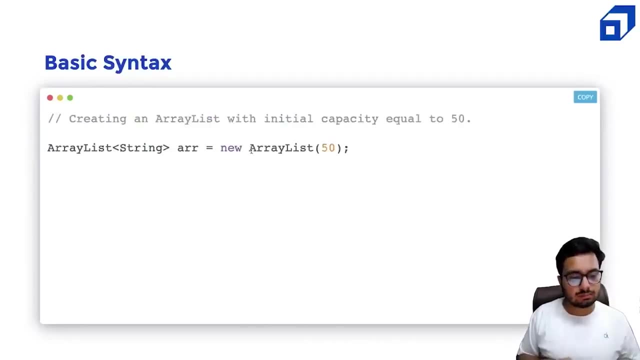 principles. right, so we'll create an object of the type list, which, which is implemented using the array list class. right, this is what we will do, right? uh, so we can also use the constructor to give an initial capacity. right, so you can pass a number here that will tell me, okay. 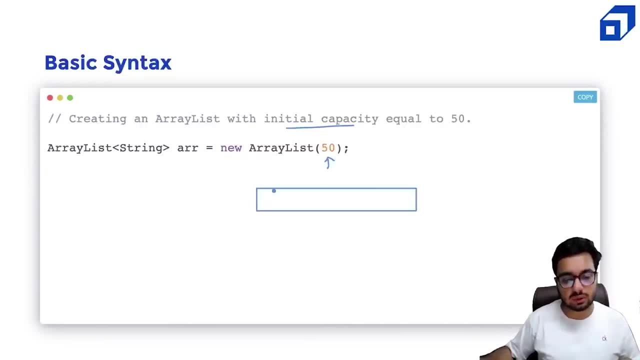 i want an array list whose initial size is 50. it is not going to be 10, so by default the initial capacity of the array list would be. that means, until this array list is not full or it's not 70 percent full, the doubling will not execute. if you know that you are. 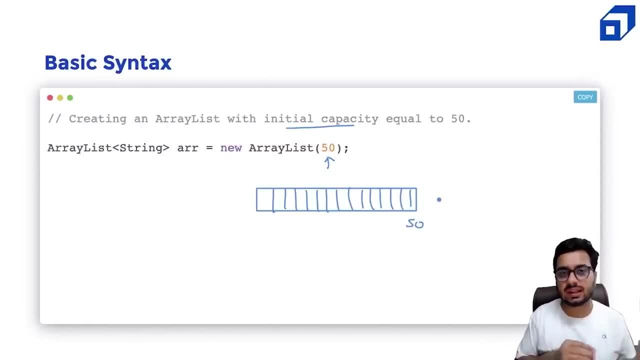 going to work with 10 000 elements. create an array list of size 10 000 or 11 000 so that your doubling does not happen again and again because it's a expensive operation. we can also initialize array list using an another list. okay, so you can give another list for. 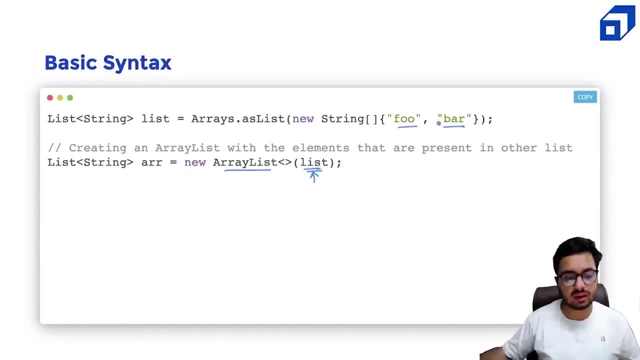 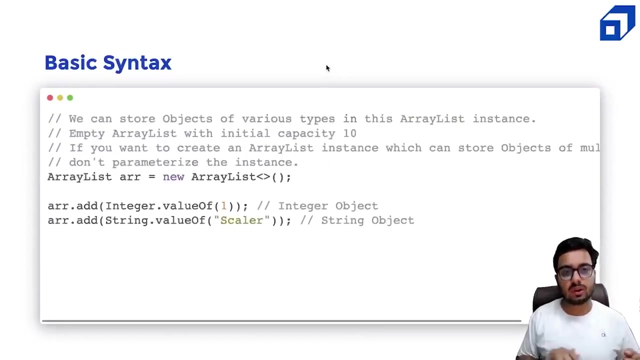 example, here we have a list of strings which is storing wind bar, and I'm going to initialize an error list with another list that is also possible. so we have seen three ways: the default constructor, a constructor with the initial capacity and a constructor that accepts another list collection to initialize this error list. right now, one more. 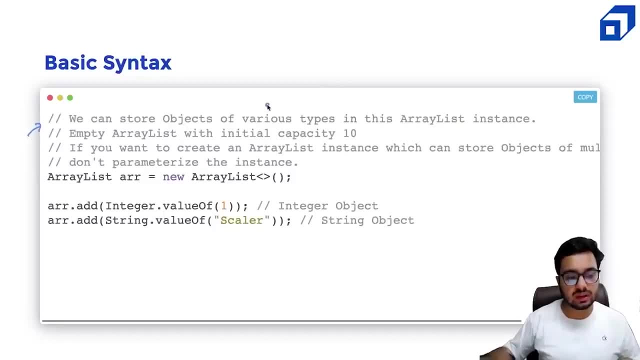 cool thing about error list is you can also store objects of various types in this error list. why so? if you want to create an error list which can store objects of multiple different data types, then don't parameterize the instance. so you, if you see, here I have not specified any specific. 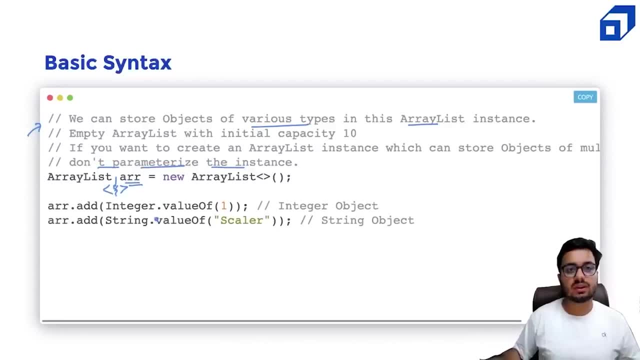 data type. here that means this error list can store different object data types so I can add an integer right. so I'm saying: error list dot add integer dot value of one. now you might ask why I cannot do this: error list dot add one because it is of the type int, right. so I need 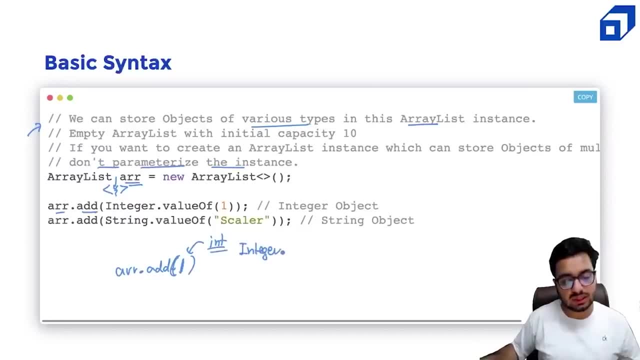 to type: cast this into integer data type. integer dot value of is a method that creates a integer object out of this one right string dot value of scalar. so this is optional. we can simply say aralist dot add scalar. so it's, it's going to add a string object inside my aralist right. if i show you in the demo i have 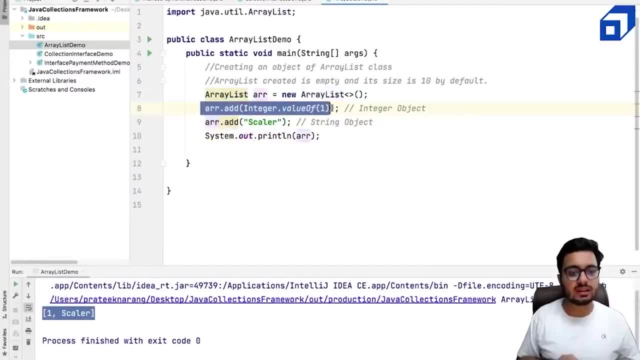 created a aralist here. i say, okay, aralist dot add integer dot- value of one- this is going to add an integer. and then aralist dot add scalar. so i'm storing an integer object and a string object inside the same aralist, right? so this is also possible, right? so you see the output here, right? 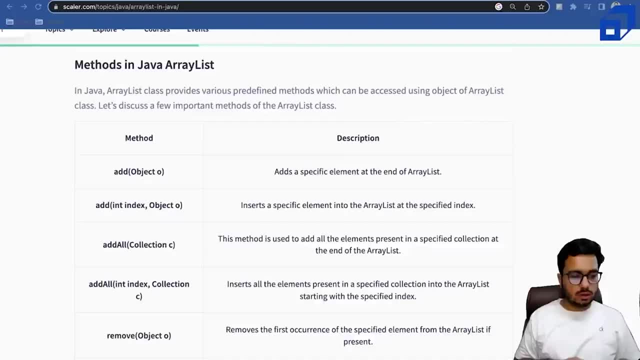 let us talk about some more methods of aralist. so predefined methods include a lot of methods. so there are methods for adding objects. if i simply call the add method, it will add. at the end of the list there is a add method which also accepts an index and an object. it will insert. 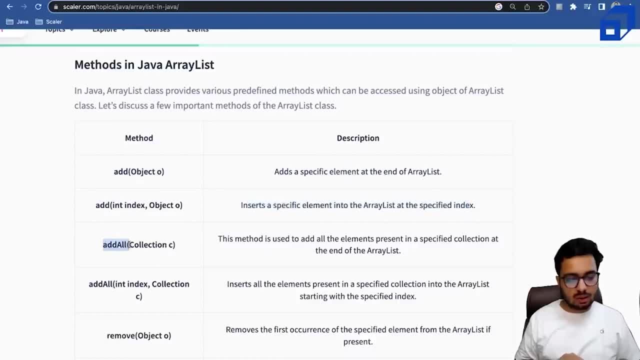 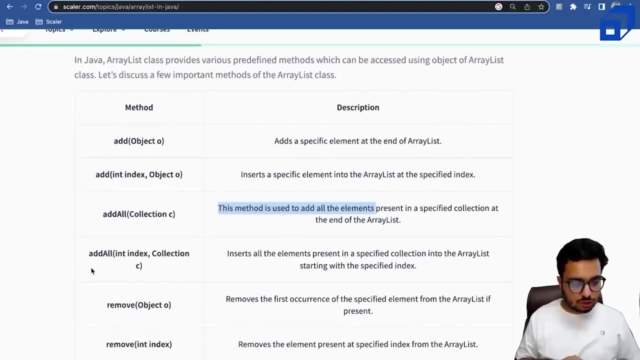 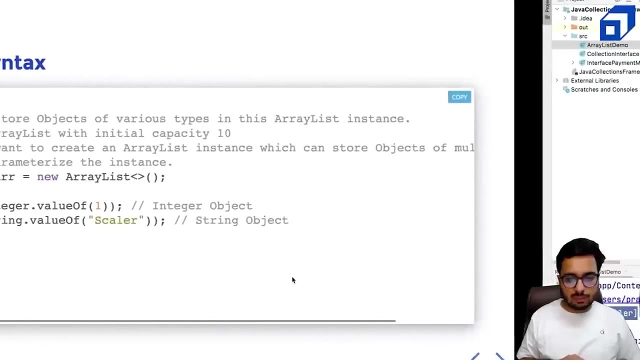 into a specific index of the list, right? there is a add all method. it will add another list in another collection into this list, right? so we can also add another collection at a particular index in this list. let us look at the add methods first. i can say i want to create an aralist. 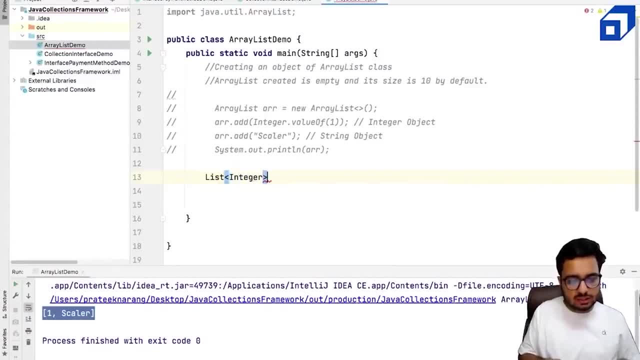 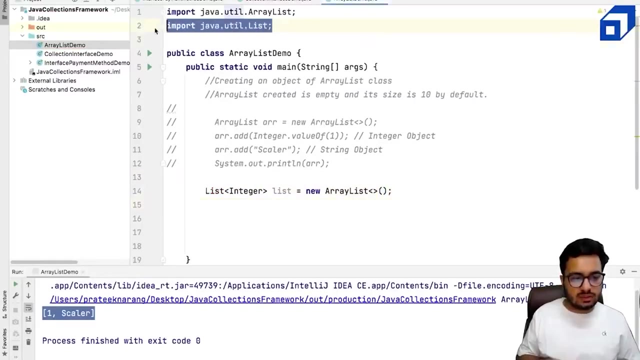 so list of its integers. i call it as list and this is equal to. you can see we have imported the list interface and we have imported the aralist class. inside this list i need to add some numbers. i can say: add one, add two, add four. so let me show you. 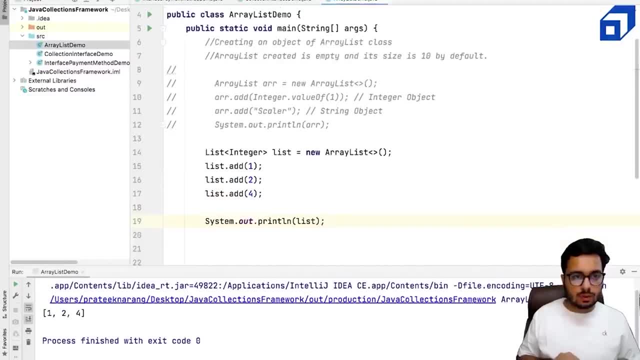 and if i print this list i see i get one to four. i have added these numbers. okay, now what i can do. i can add a number to this list and i can say: i want to add a number to this list, add at a particular index as well. i can say, okay, i want to add at a certain index. so either i give, 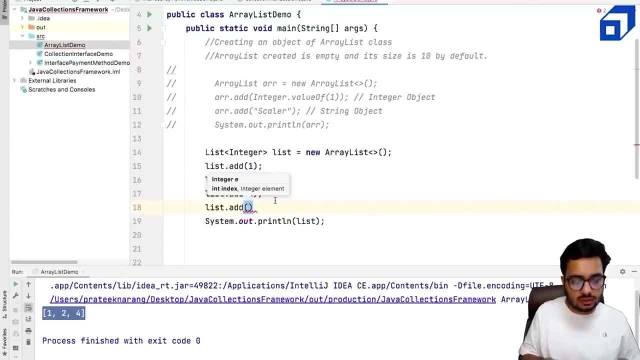 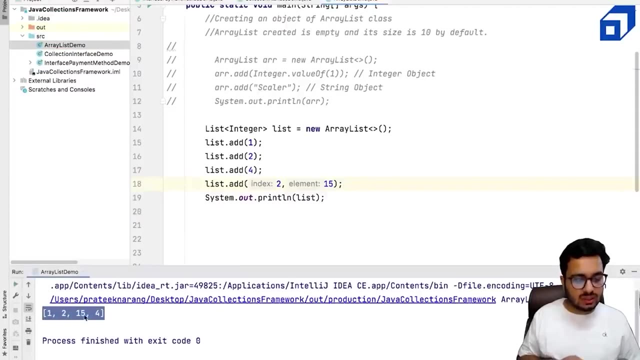 an integer or i give a int followed by an integer, i can say, okay, add at index two, the element is 15. if i do it, it will do insertion in the middle of the list. that is also possible. so you can see, i get 15, which is now present at index two. so by default it is like the first parameter is is the. 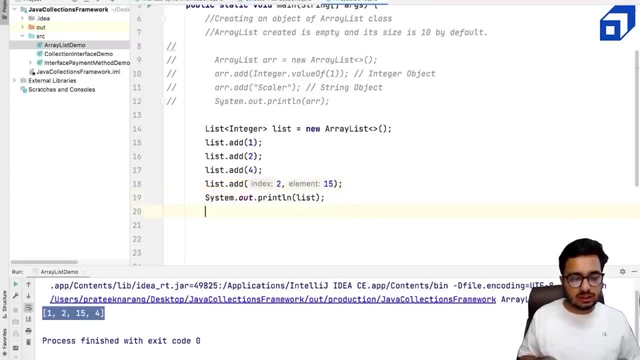 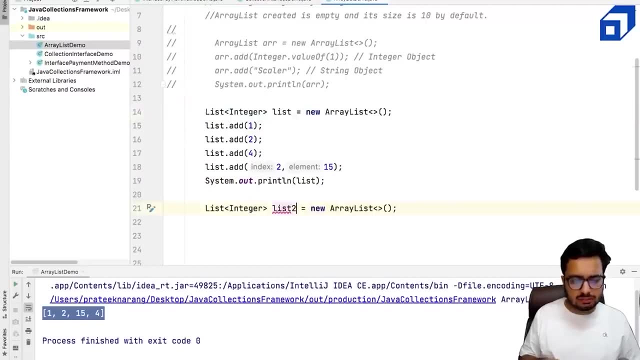 second parameter is the value that i am going to insert. right, that is the add function. i can create another list as well. i can say, okay, um, i need another list, list two, and i can say list two, dot, add 15, and i can, or let's say, this is 25. i can also add all elements of list one in list two. i. 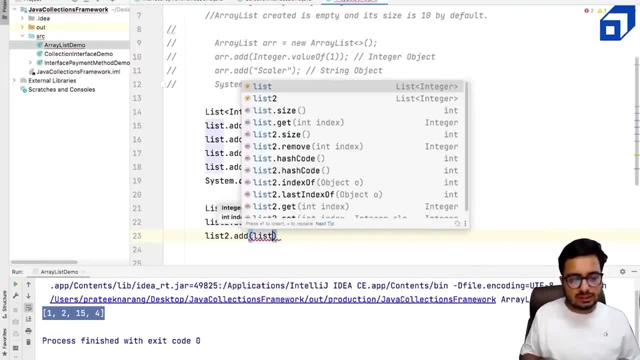 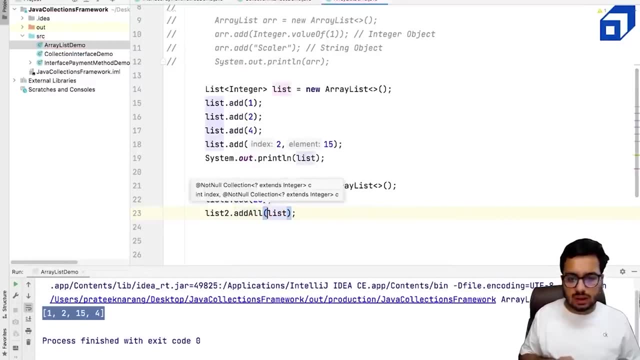 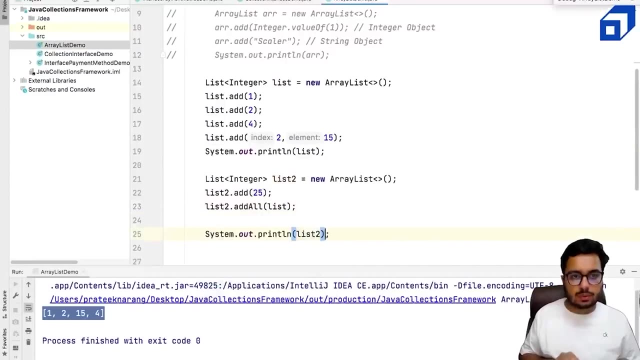 can say list two, dot, add uh, list. so i can pass another collection here. so add all. i need to call method and this will also work, and i can print list two as well. you can see i'm having 25 here followed by all elements of list one. that is how do we use the add method. next we will look at 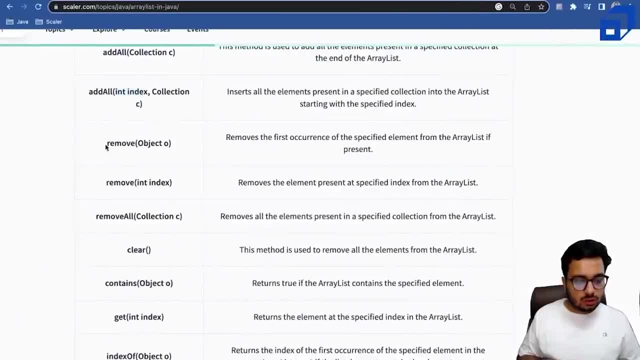 look at the remove method. so now, remove method is it's actually a overloaded method? if you look at: we have, we can pass an object, we can also pass an object, we can also pass an object, we can also pass an index. now this becomes tricky, especially if you are working with integers. right, if i say: 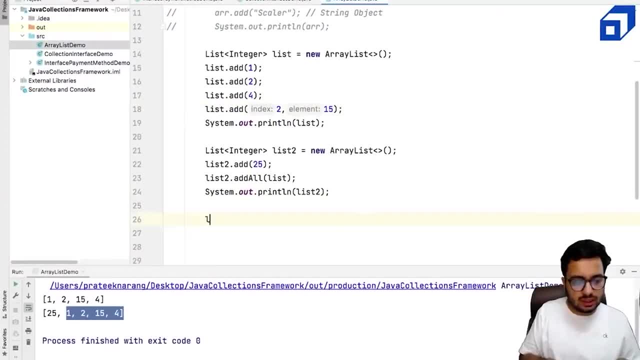 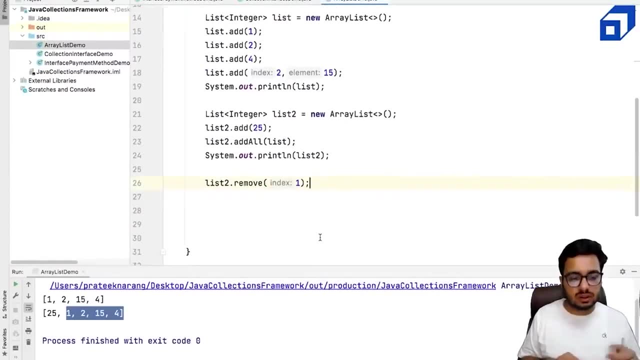 okay, i want to remove something. i want to say, uh, list two, dot, remove one. what does it mean? am i removing the index, or am i removing the value one, right? so? or let me just say, list, dot, remove one. so if i talk about first list and i want to remove one from it, so let me show you it will actually. 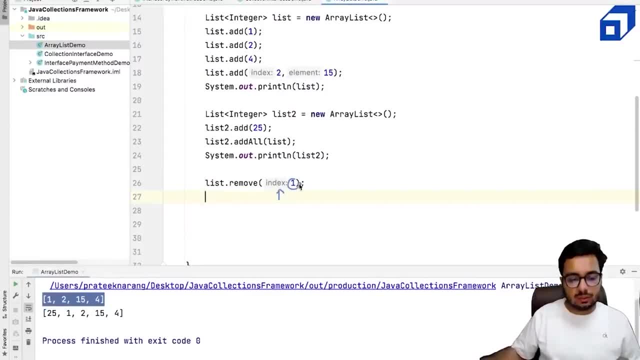 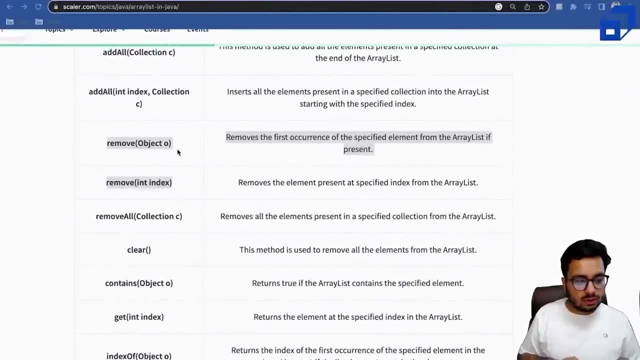 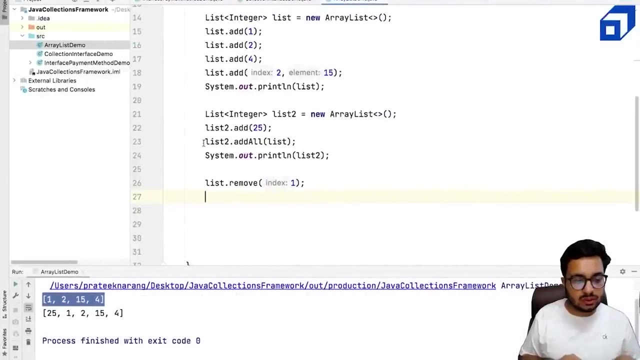 remove the index. because when you're passing one simply like this, it's going to assume it is of the data type int, right? so if you look here, so when i pass int data type it removes the index at the. at the following index it will remove. so that means it will remove the element two from list one. but if i want to remove 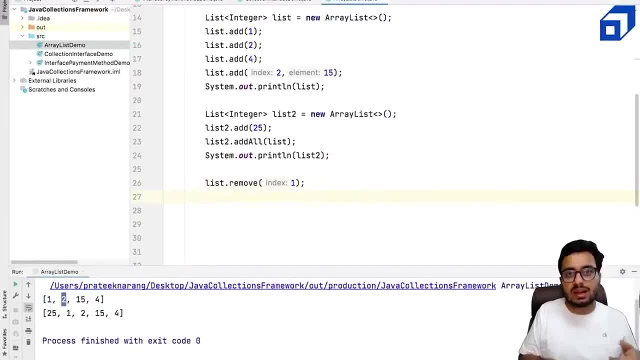 the value, that is one. what will i have to do? i have to convert that into a integer object, right, so that means remove one as a uh object. so if i remove both, let's say so, that means one and two. both will get removed. let me show you the output. i'll print system s out list. show me what you're. 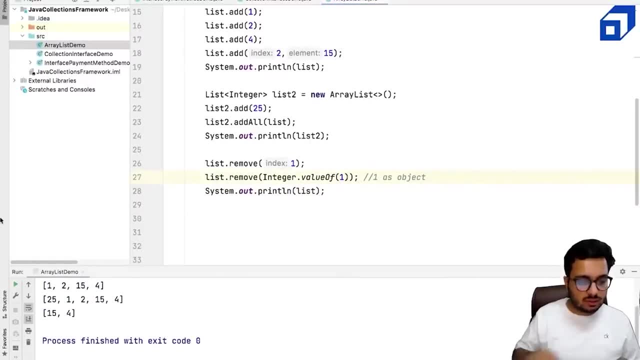 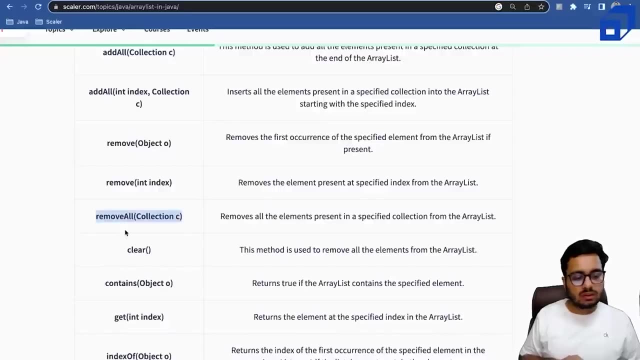 going to remove, like now. you can see the output that both one and two they got removed and we got 15 and four. similarly, you have a removal method which will accept another collection. it will remove all elements from that collection, from the given collection. clear will remove all elements from the list. 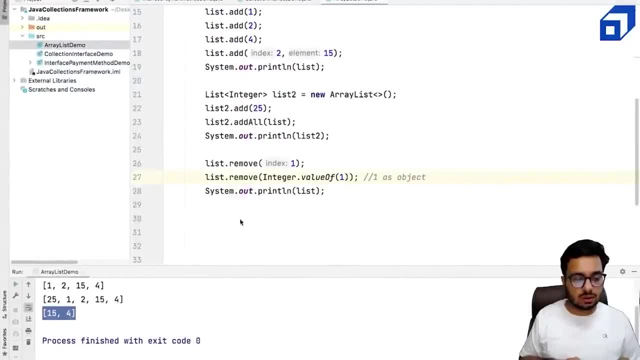 contains will tell me whether a particular element is present or not, so i can check that. okay, if list contains 15, do something right. contains is is your linear search, so s out: uh, yes, 15 is present, something like this. so you can use the contains method with almost every. 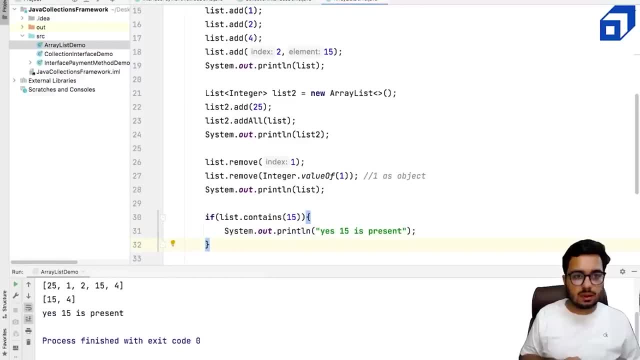 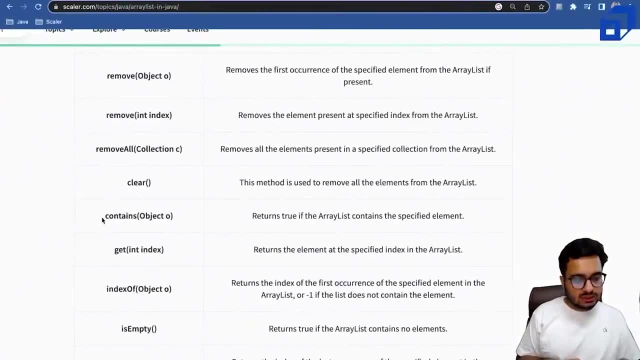 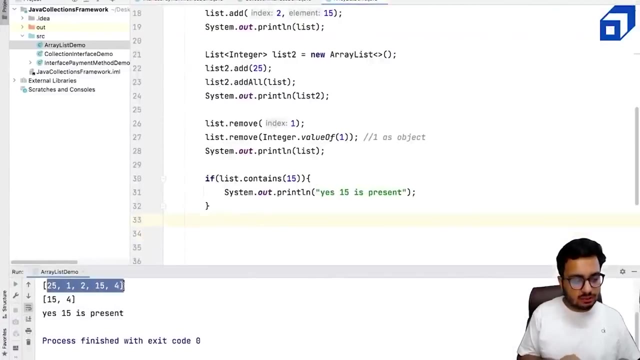 collection. let me run this and you can see that we are getting. 15 is present. okay, so there are more methods. uh, there is a get method. so if you want to read a particular index, you want to say, okay, show me what is present at, uh, the zeroth. 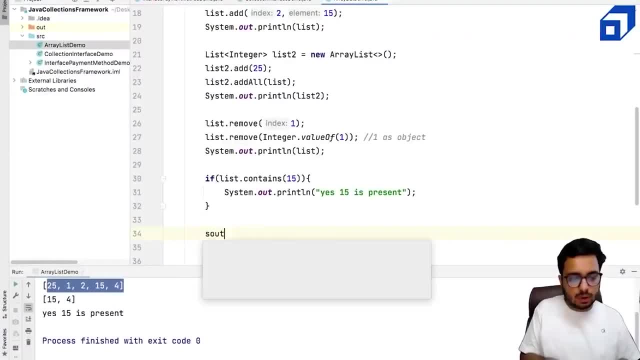 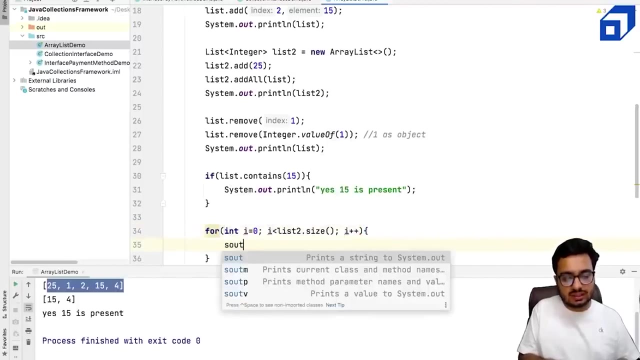 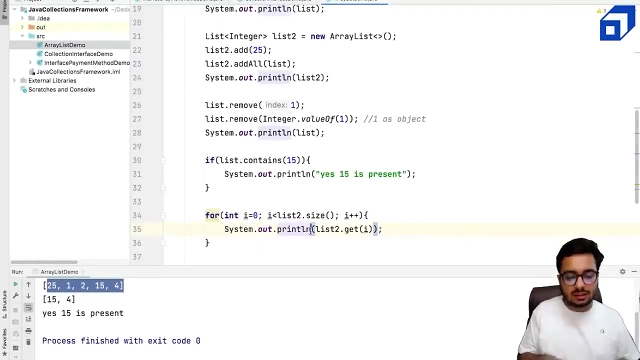 index. you can say s out or you can maybe you want to iterate over the entire array list. you can say for int i equal to zero, i less than list dot size, or list to dot size, i plus plus. i want to get the elements at each index inside s out. list to dot, get i. this will give you the elements at given is. 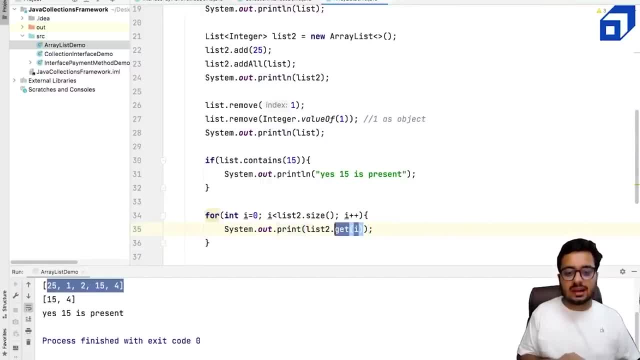 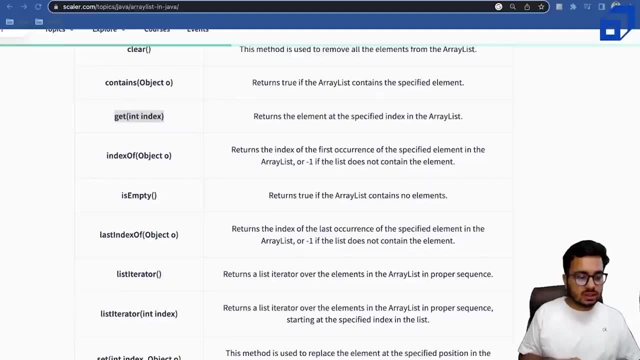 index. so get function is used to access the i'th element. so let me run this and you can see we are able to iterate over all the elements in this list. so just like get. there is another method that is called set. so if you want to update a particular 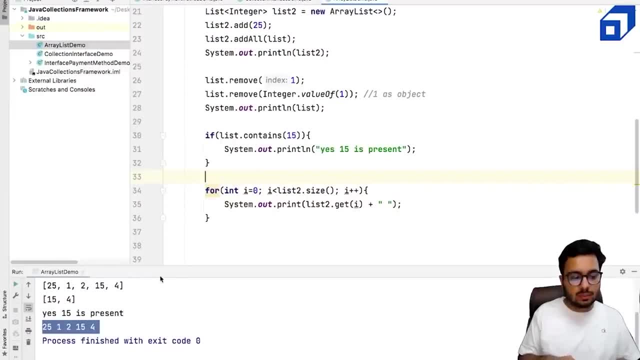 index. you want to say, okay, i want to make this zeroth element as 50. so you can say, okay, list to dot set: zeroth element, make it 50.. this will work and now your zeroth element will be 50.. you need to give the index and the object that is that you need to store here. this is the set. 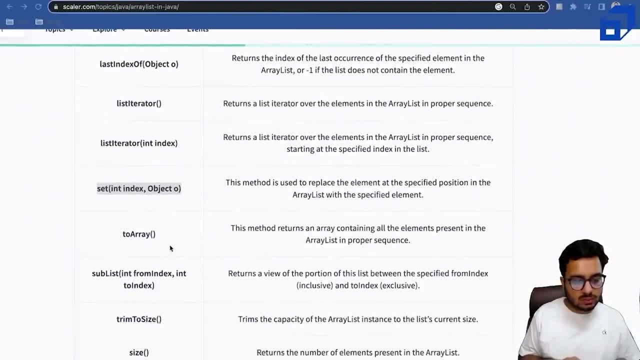 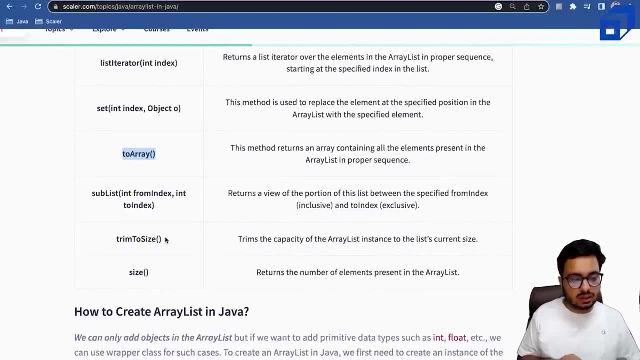 function. there are more methods. i won't be able to cover all the methods, but we have covered, like most of the important methods. there is a method called to array- if you want to get an array from an array list, you can use this- and there is a method called as size, which we have just seen. 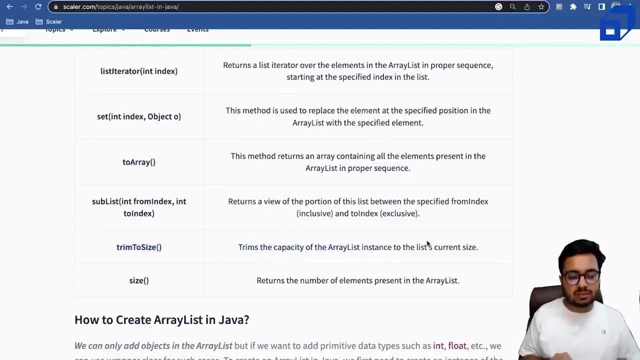 there is also a method called trim to size. that means if we have, if we want to reduce the current size right, like if we want to reduce the capacity to the current size, we can use this method: trim to size right. these are some of the important methods that we have covered in this. 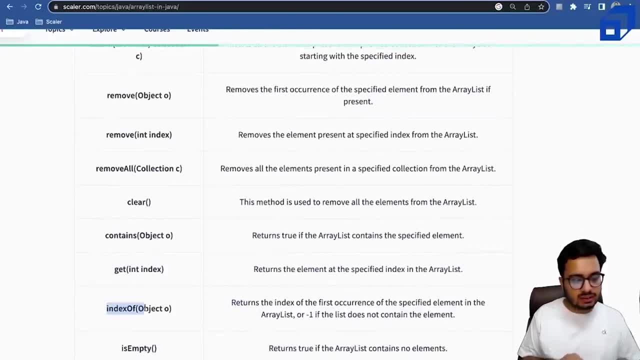 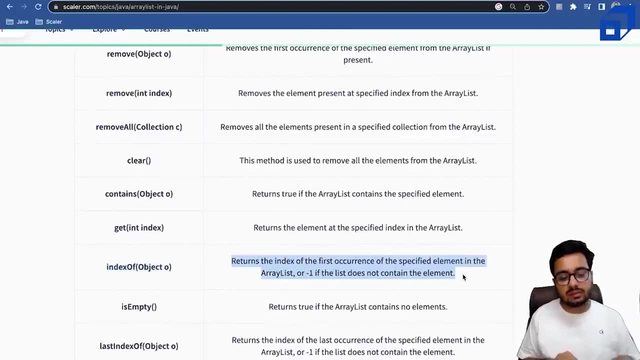 method trim to size right. these are some of the important methods. uh associated with uh array list there is also index of returns, the index of the first occurrence of the specified element in the array list, or minus one if it does not contain. the element so contains is going to give you boolean. 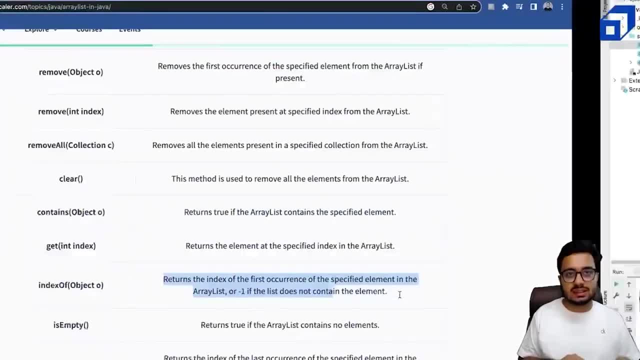 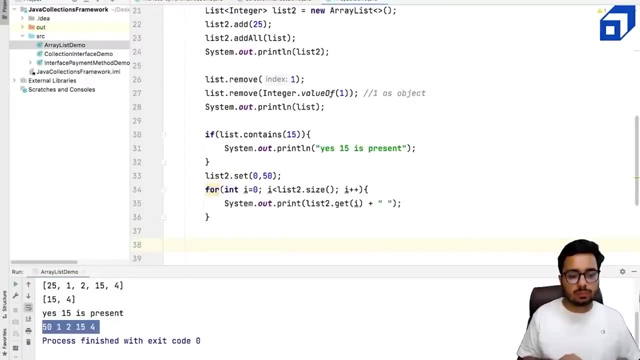 present or not. index of is going to give you at what index it is present or not. right now. we'll look at some more ways to iterate on the array list. let's do a quick demo. so we have seen uh for loop. we can also use a for each loop, so i can. 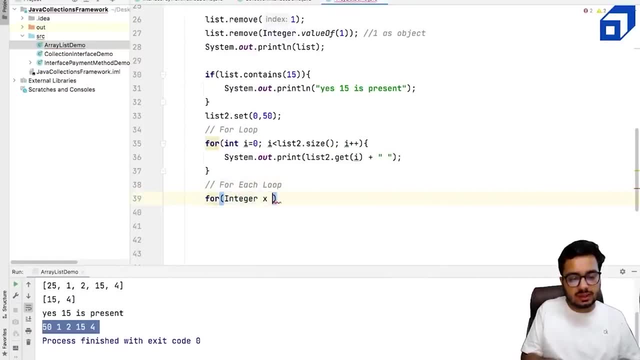 say, for every uh, integer x in my list 2, i want to access it and i want to print it so i can say, okay s out, list 2 dot get i. that is my another way of iterating and printing. so sorry, i will not do this. 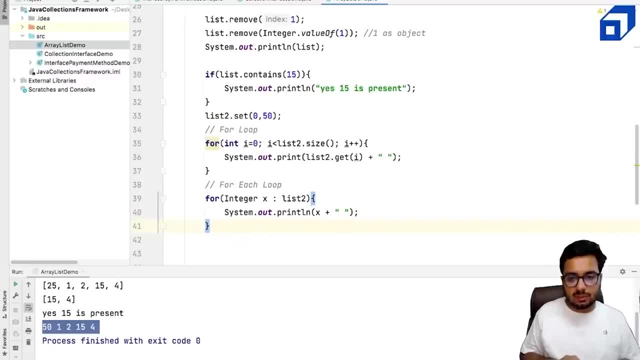 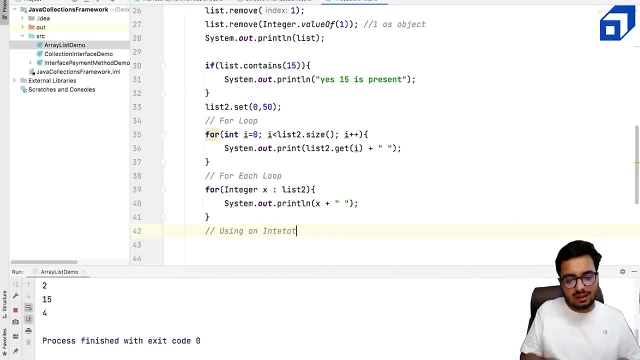 as. okay, let me print this number x, let me run this code. there is one more way that i can also iterate on the list using an iterator, right, so you can see we are getting, uh, all the elements, that is, 1, 2, 15, 4 and 50 is also there, right? so we are starting from 50 here. 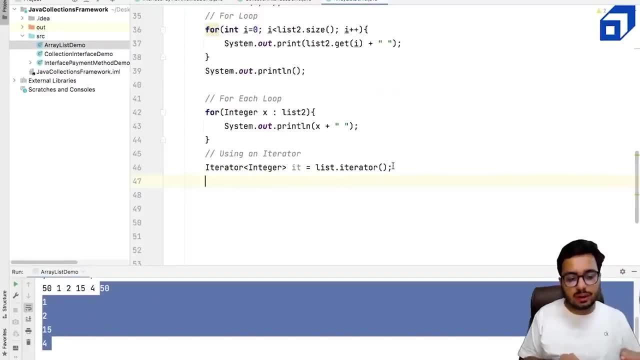 we are getting all these elements okay. so iterator is one more way to traverse on on on a java collection, all java collections. they they support iterators. so what you can do, you can create a iterator object by calling list dot iterator. this iterator has a method called has next, which tells me whether i can access the next element in the collection, not or not. 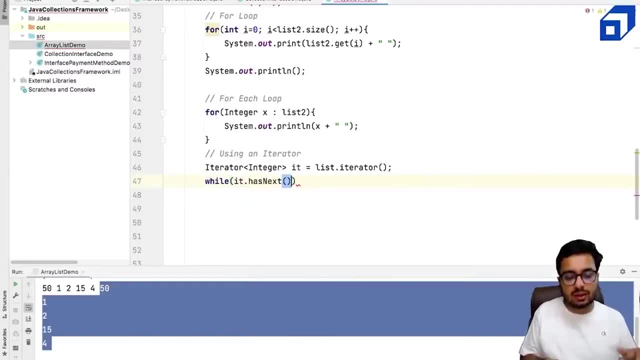 if your collection has finished, your has next will give you okay, there is no other element, right, so i can say: while it dot has. next, if there is an element present, i can access it. so i can say: okay, s out it dot next. this will give me the next element in the collection. this is another way. 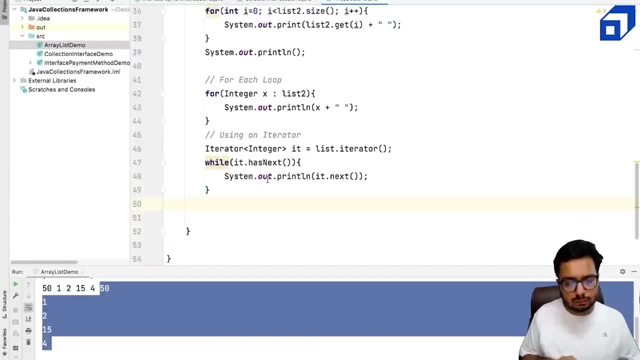 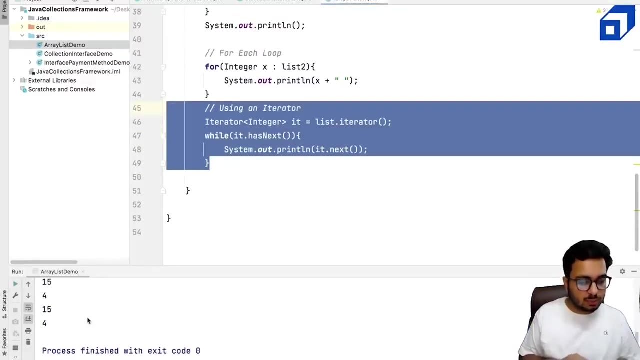 using which i can iterate on given collection. right, so iterator is coming from the javautil package only, right? so this will also print all the elements present in this. at least let us quickly run the code and see we are getting the same output. uh, using iterator as well, so we, i iterated. 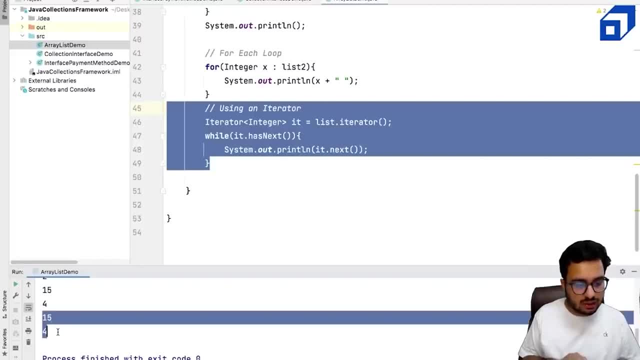 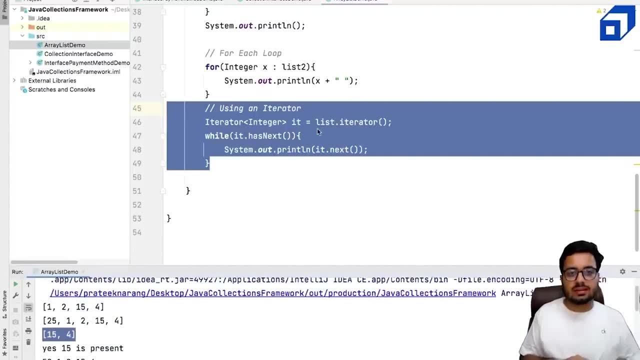 on list one so, which is 15 and 4. again, i iterated using iterator, which is 15 comma 4.. that is what i am getting by iterating on my list. that's all for error list. i hope you understood the methods of error list. 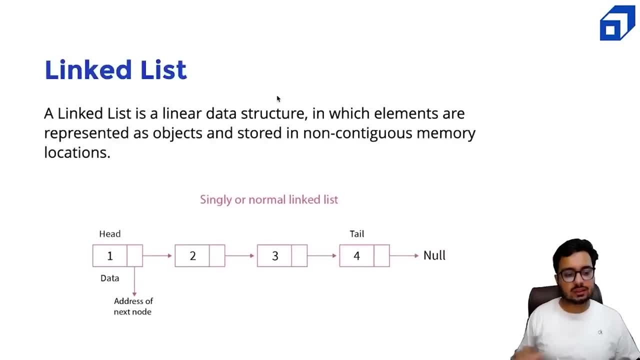 and how it works. now let us jump into linked list. so linked list is also a linear data structure in which elements are represented as objects stored in non-continuous memory. for example, if this is your heap memory and you have some data, maybe one is stored here, two is stored here, three stored here. 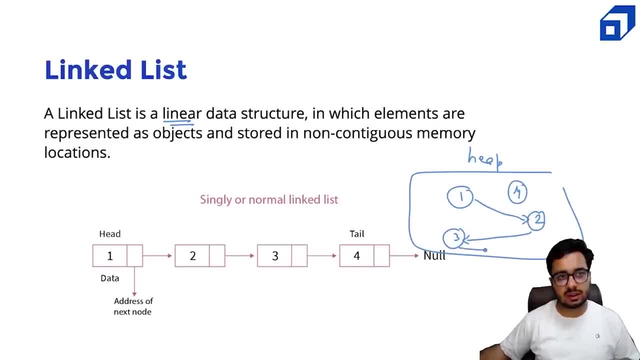 four is stored here. they might form a chain like structure, and where each object is referring to the is holding the address of the next object in the chain. this is called as a singly linked list, where each object knows the address of the next node but it does not know anything about the previous nodes. if you arrive, 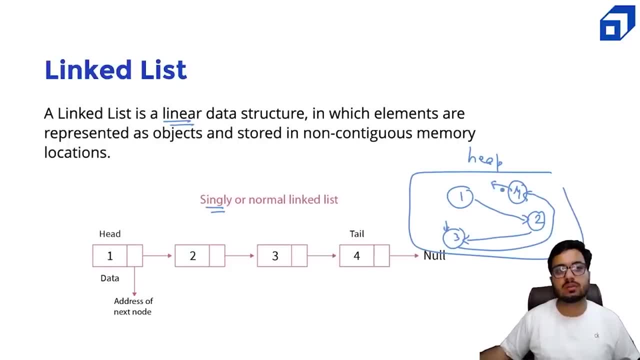 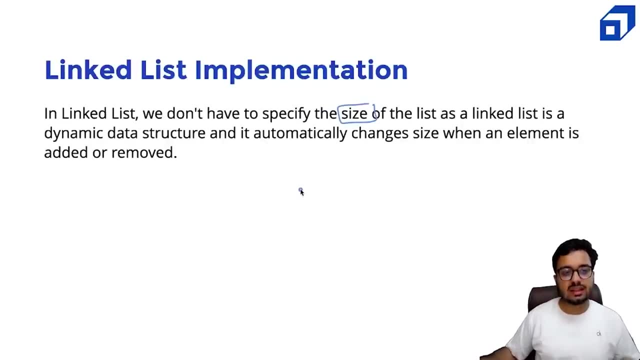 at three, you can only go to four. if you arrive at four, you can only go in the forward direction. let us talk about linked list, little more so we don't have to specify the size of the linked list. it's a dynamic data sector. as you add more data, more objects get created in the 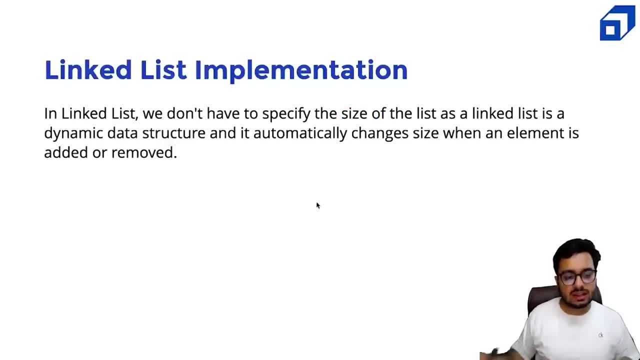 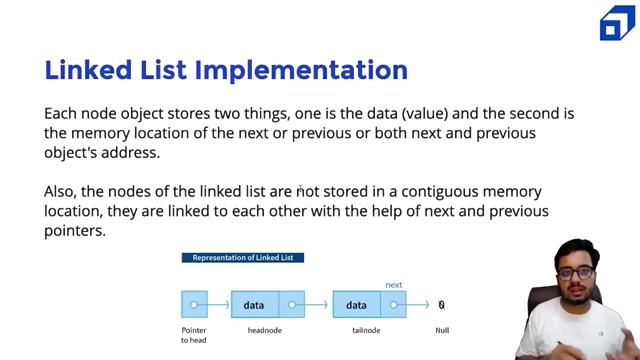 memory and they become part of the chain, and size is changing automatically as the data is added or removed, so you don't need any fixed size array to initialize it. right now. let's talk about the implementation, as i just talked about each node in a linked list, it's: 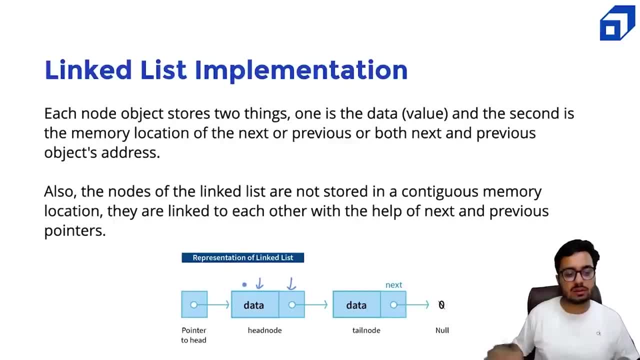 it's going to hold data. it is also going to hold the address of the next node and if it is a doubly linked list, it is also going to hold the address of the previous node. nodes are not stored in a continuous memory location. they are linked to each other with the help of next and previous pointers. 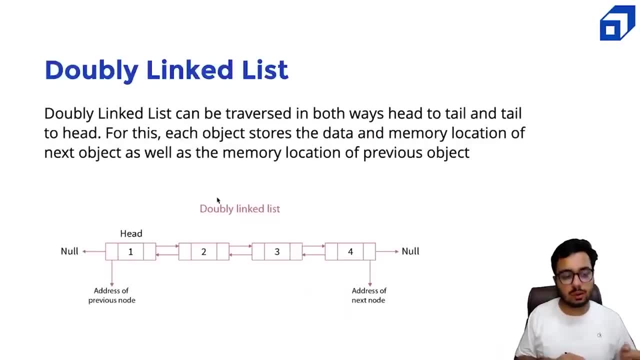 okay. so this is it, something we'll go into detail when we talk about, uh, when we do a tutorial on linked list, but for now, we just want to see how to use the inbuilt linked list class and understand its advantages and when to use it. right? so in java, the default implementation provides us with a double linked. 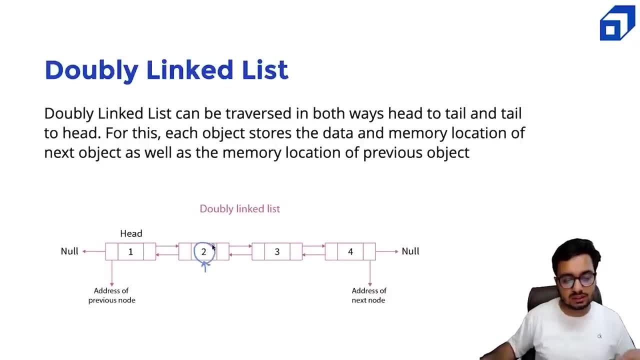 list, so a double linked list. each node stores three things: the object or the data, the next node's address and the previous node's address. so at two, you know where is the next node located and where is the previous node located. at three, you know where is the next node located and where. 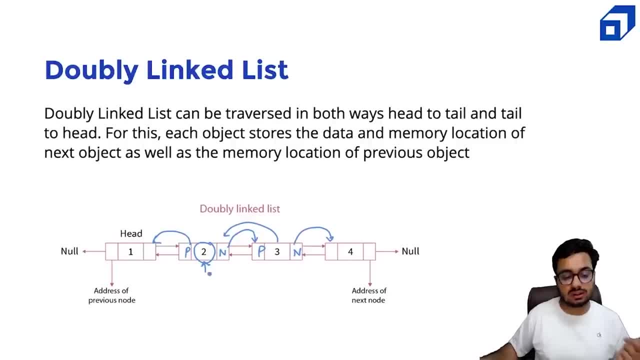 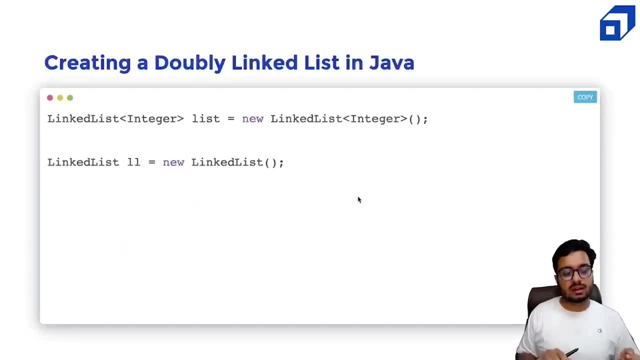 is the previous node located, so you know all the three things at each node inside the linked list. that is what a double linked list is right, and creating a double linked list is fairly simple, so you just need to use the linked list class provided by the javautil package. 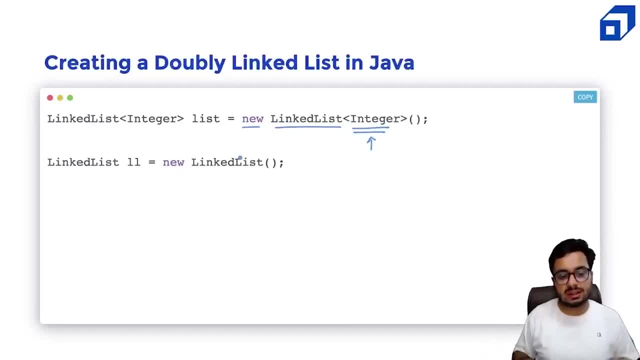 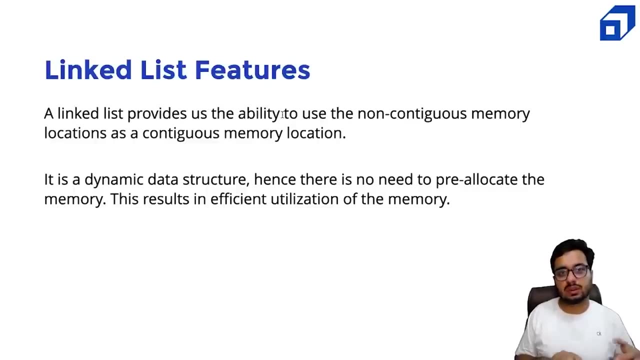 and the data type, what kind of data you want to store in this linked list, and it will create a linked list for you. right now let's talk about the features of the linked list. the biggest feature is we can use the non-continuous memory, so if you don't have 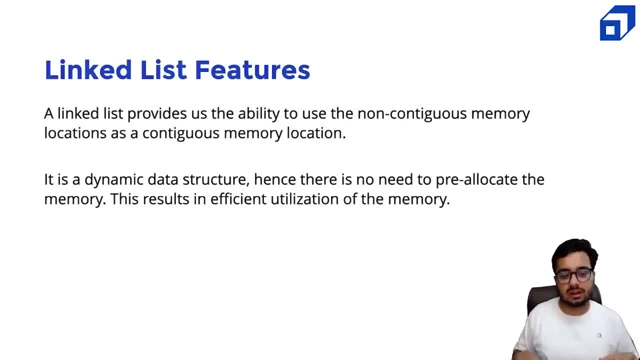 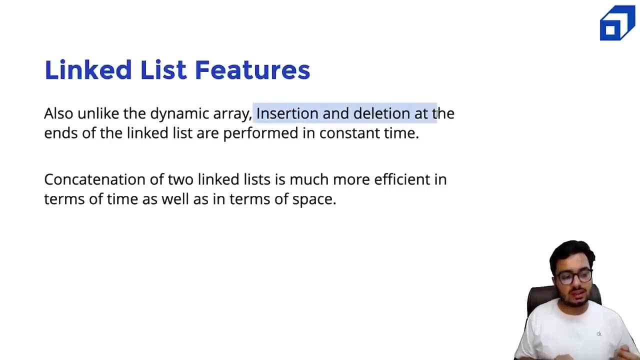 a linear block available, we can still create a big chain by utilizing the non-continuous blocks of the memory. it is a dynamic data structure. there is no need to pre-allocate the memory and hence it results in efficient utilization of the memory as well. right and insertion and deletion. 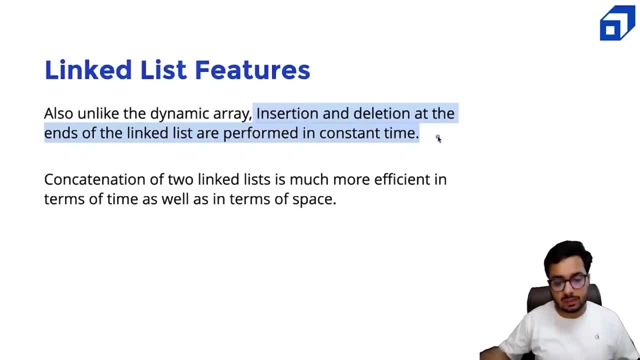 at the ends of the linked list are performed in constant time. now, this is a very big advantage. so if you have an array and you want to insert something at the beginning, you would see that i will have to shift the entire array. then i can insert a zero here, right? 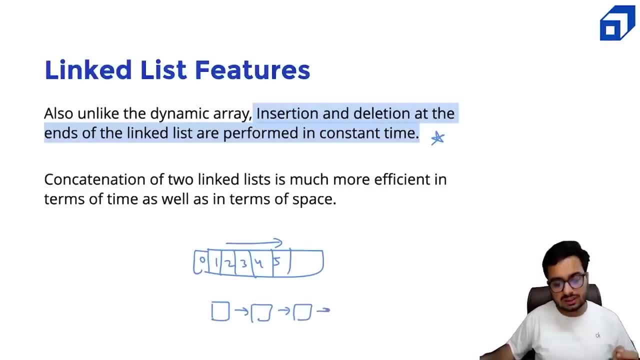 but in case of a linked list, this time, which is order n in an array, inserting at the beginning, it's going to be very fast. suppose you have one, two, three, four, five. you already know this node, okay. and you say i want to insert a zero here, so you create a new node and it's okay. head should point. 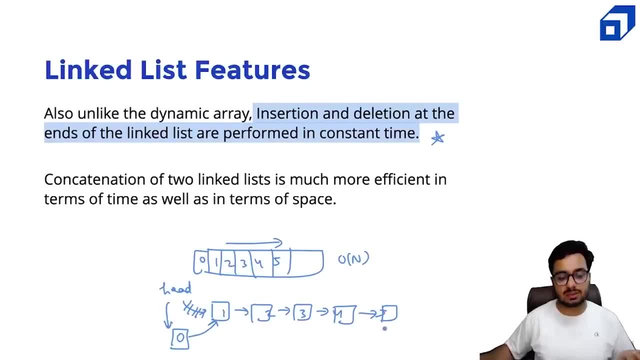 here and zero should point here. this can be done in order one time. similarly, the last node is, uh, referred by a tail pointer. if you want to create something at tail, you can simply add six here and your tail will move here, right? so if it is a doubly linked list, 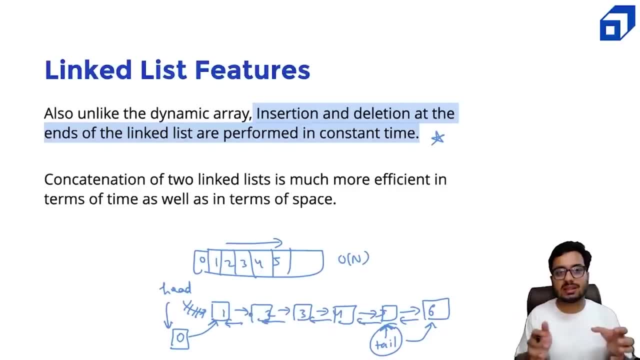 insertion and deletion, both at the both ends, can be just done in order one time. this is a very, very big advantage of linked list and concatenation of two linked list is much more efficient in terms of pace and time. so if you want to merge two array lists, you will have to copy all the data right. but 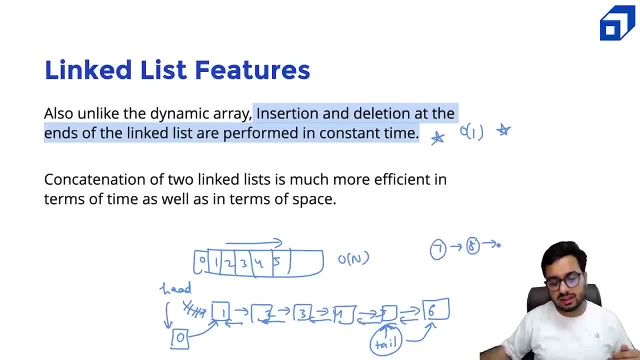 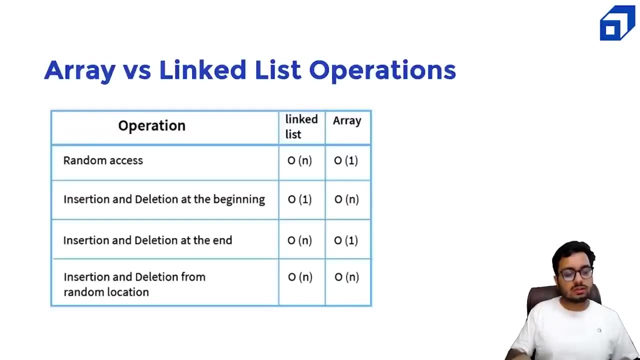 if you want to merge two lists, let's say i have another list- seven, eight and nine. in that case, merging is also very easy. you just need to connect this node with this one, which is again going to take order one time. concatenation is also very fast in case of a linked list, right, so let's talk. 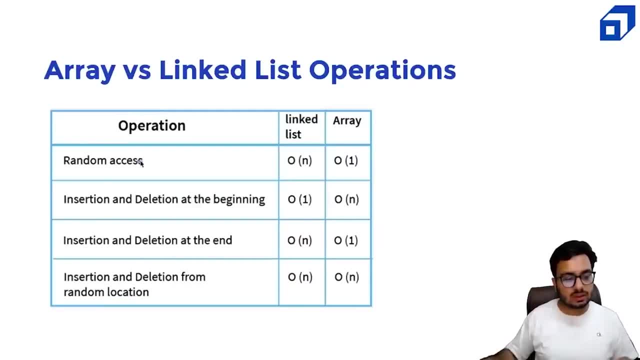 about, uh, the differences between the operations, right. so random access. now that means if i want to get any ith element, this is very fast in array, right? so i know i can get uh, i can do array dot, get i. this works in order one. but if you want to get some ith element inside the linked list, there is. 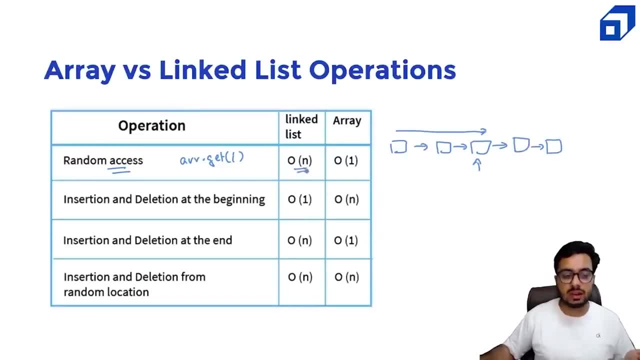 no direct way. you have to iterate it. it's in the worst case. it will be order of n- insertion and deletion- at the beginning. in case of linked list, as i told you, it's order one in an array. it's going to be order n because you have to do the shifting- insertion and deletion- at the end. so 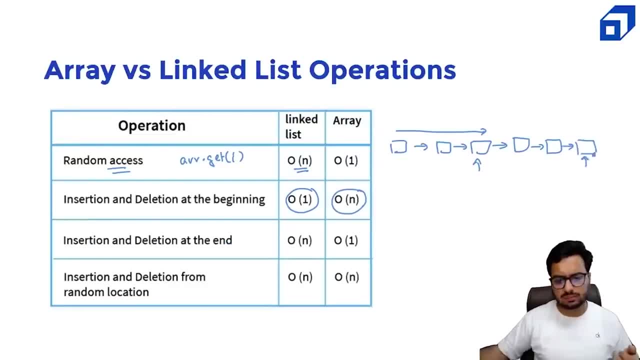 if it is a doubly linked list, uh, and we are maintaining the tail pointer, you can do it in order one time as well, and uh, in array it is also order one. so this this can be made order one. right depends upon the implement. insertion and deletion from the random location. 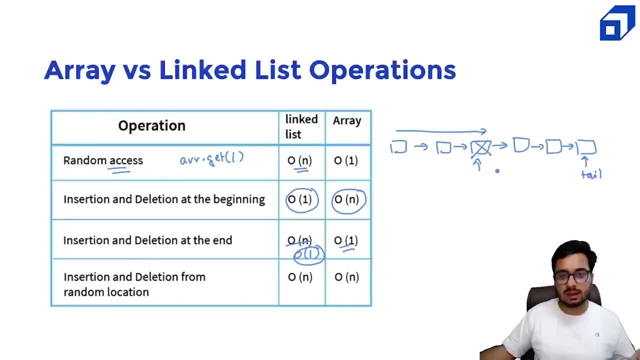 so, of course, this inserting, deleting something from the middle, both in array and the linked list, will take order of n time. so i hope you understood the basics of a linked list. now let's look at the implementation. so i have this code in which we said: okay, we are creating a list which is using a. 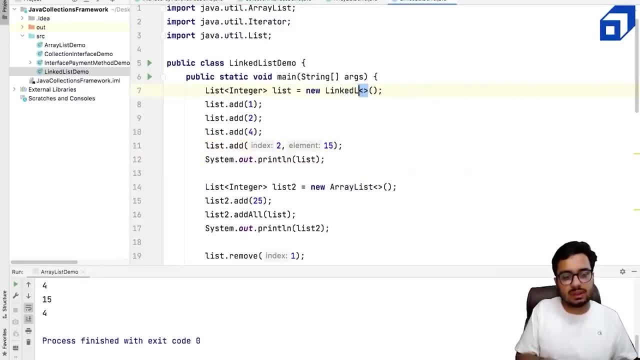 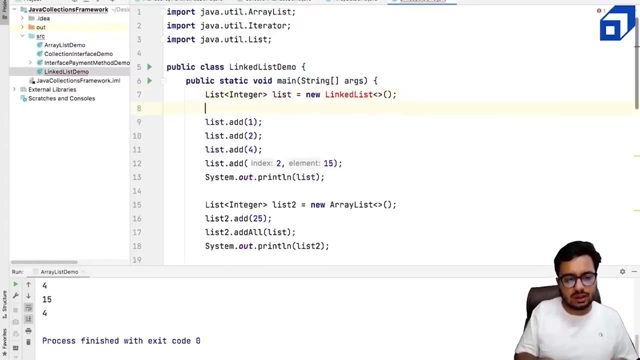 new arraylist object. so instead of now using arraylist, i can simply replace it with with linked list, and since both arraylist and linked list implement the list interface, all the methods that we saw, uh, with this list, they will also work with linked list as well. right, if i need? 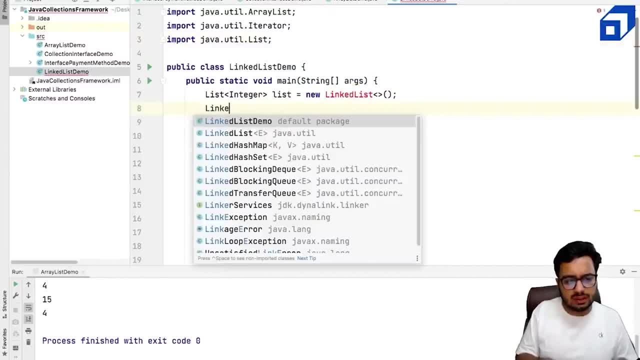 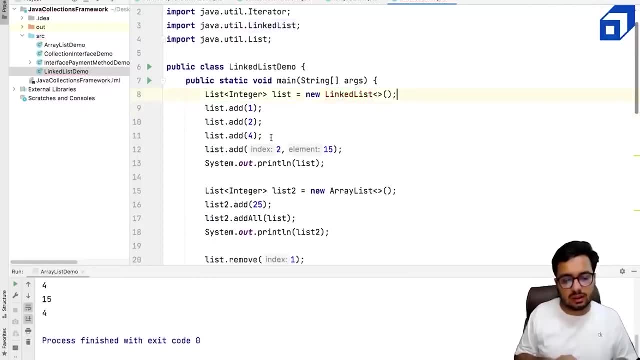 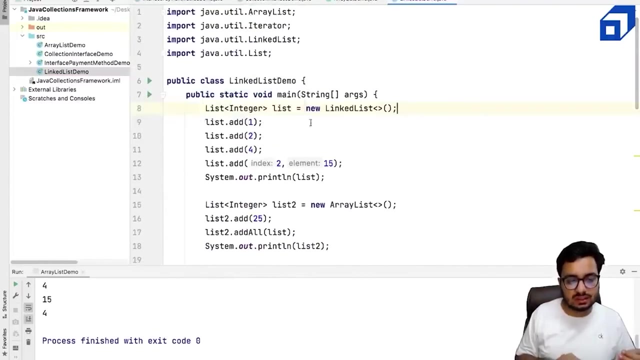 to import this class. let me just type linked list and this will get imported. so port javautillink. so this is also there. if i run this code, as it is the same arraylist code, it will work. all the methods that we used on arraylist will also work. 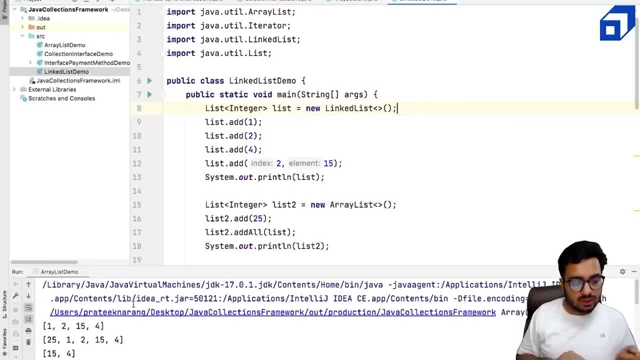 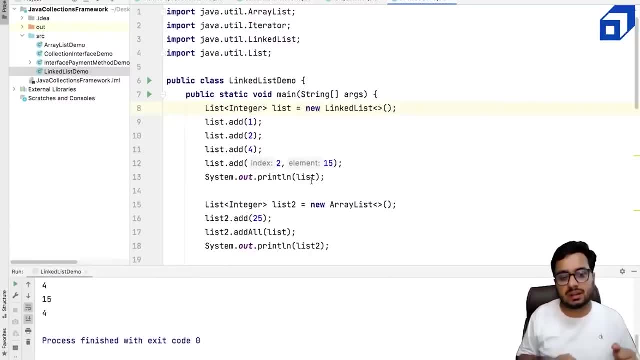 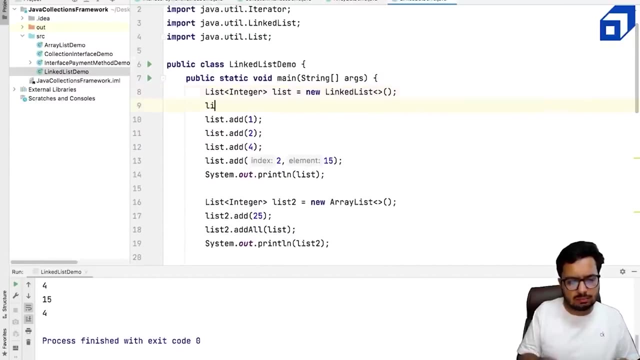 on linked list as well. now, apart from it, there are some additional methods as well which are provided by linked list, for example, adding something at the beginning of the list so that method is not there in arraylist. we can use that method. for example, i can say, uh, this dot add first. i can say okay, in 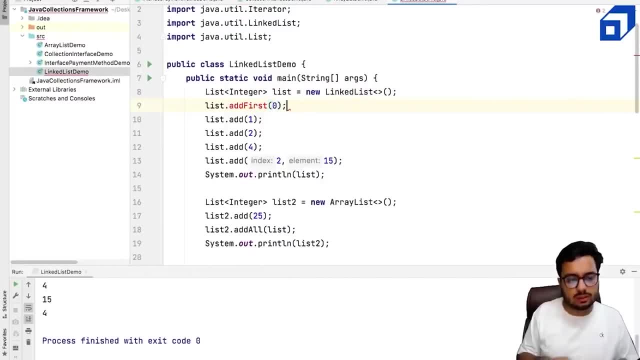 the beginning, you add an element that is zero. you might be saying, okay, we are getting an error here. at first, it is nothing like this. now why? why we are getting this error? because add first is not a method inside the list, okay. so what happens is your list says that, okay, you must implement an add method. 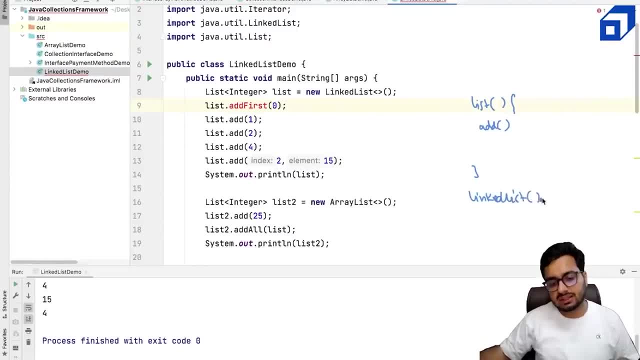 whereas your linked list class, which implements your list interface, right it says: okay, i will implement the add method, i will also implement the add first method. that means you cannot call add first method on on a list kind of a variable, right it is of the type list. what i need to do? i 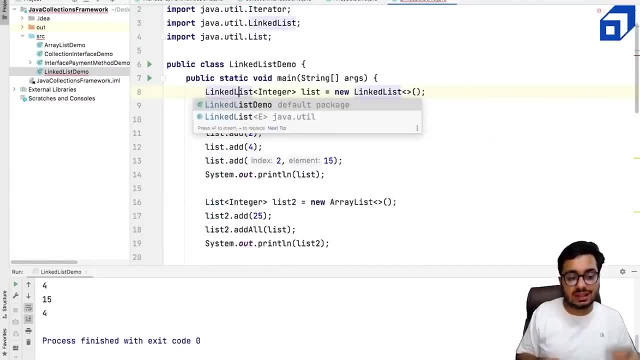 need to say okay, the object that i am now creating is exactly a linked list. if i make it linked list, you can see, add first will work, because you can easily add in the beginning of a linked list. i can say, okay, maybe add uh minus 20 here and show me this list. 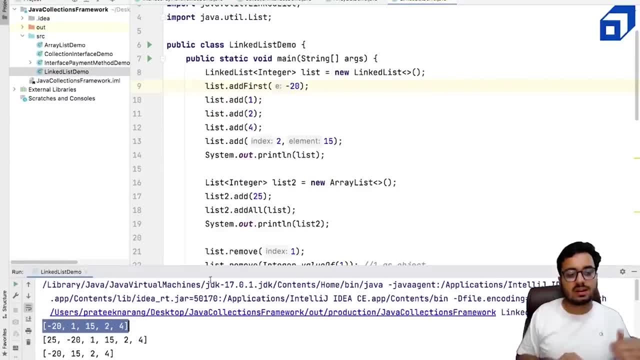 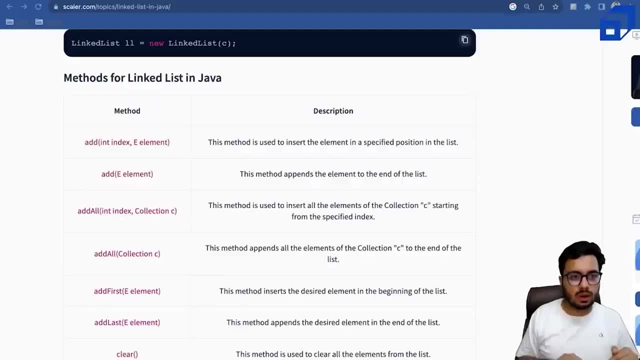 i'm running the code and you can see minus 20 is there. it's added in the beginning of the list. so we have more methods. let's look at some more methods. all right, so just to save time, i'll quickly go through all of these methods. so there is a add method which we saw on the list. this is: 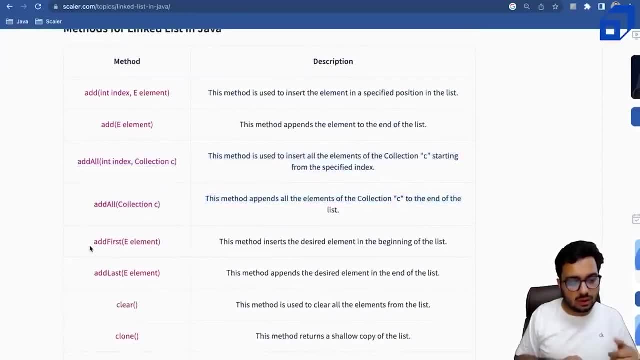 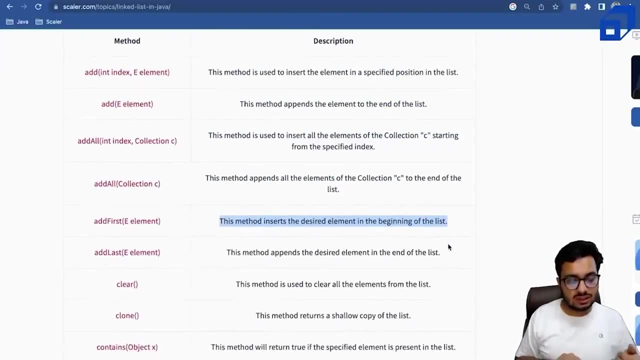 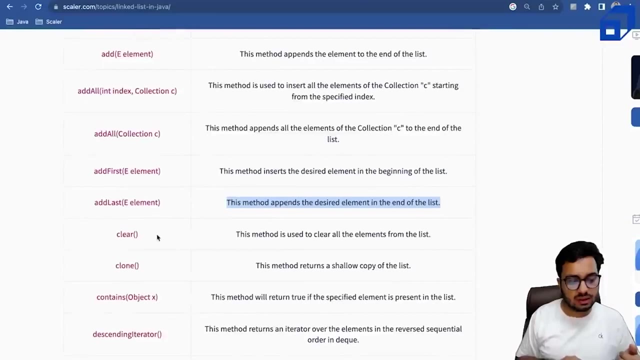 also there. add all is also there. add all we have seen right now. add first. i just show you, showed you the demo. it adds the desired element in the beginning of the list. similarly, there is a add last method. it will add at the end of the list. so it will work same as your add method. there is a clear. 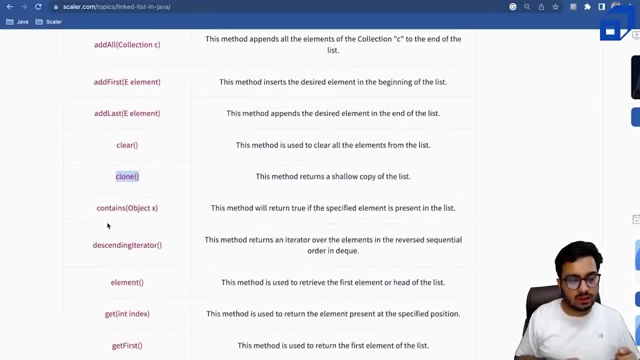 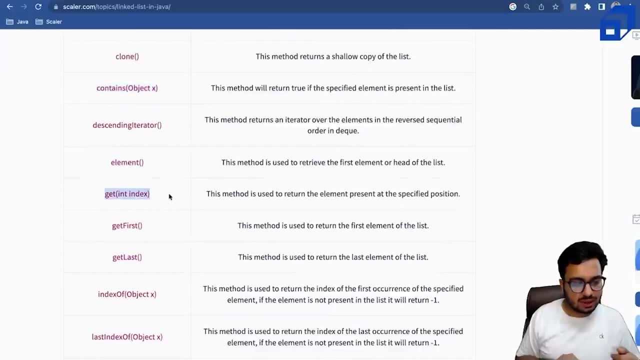 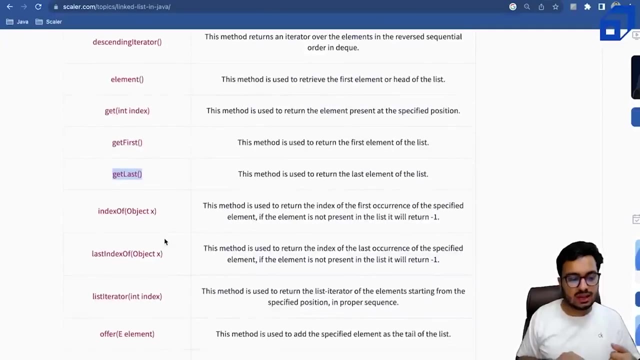 method, which is fine. there is a clone method: creates a shallow copy. there is a contains method element present or not, then popular methods are: get. i want to get particular element works in a linear time: get first, get the first element. get last, get the last element. index off. you can use. 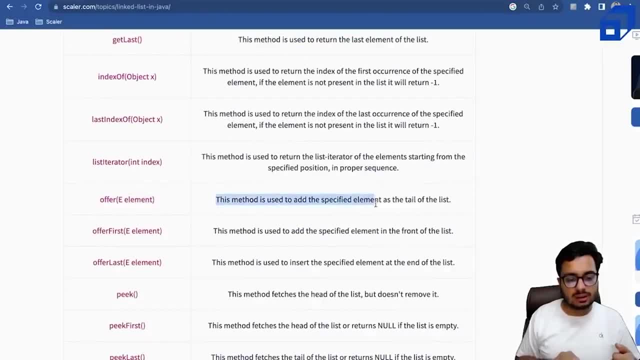 the add method and then the add method. so this method is used to add at a specified element at the tail of the list. now you might be asking: what is the difference between add versus offer? let us discuss this as well. for that you need to go to the java linked list class, right? so i'm look. 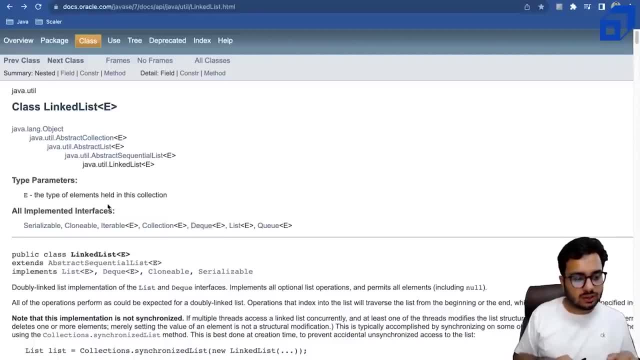 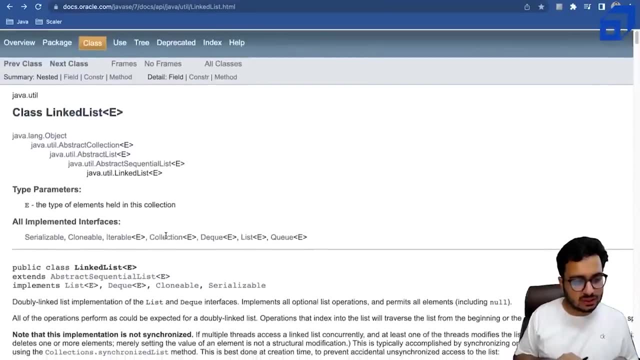 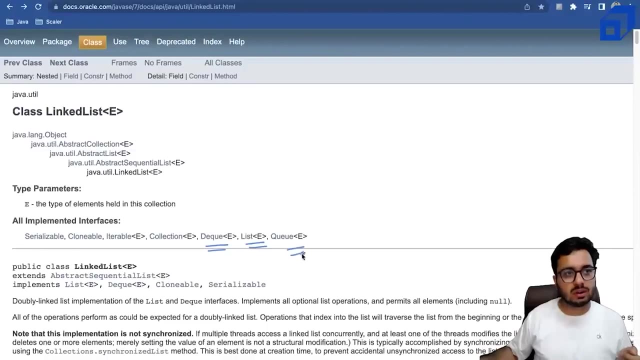 uh, java linked list. the oracle docs right. so if i look, look here what is happening? uh, the linked list class it. it actually implements, uh, not just your uh list in of your interface, it also implements your deck interface. it also implements your you interface. that means all the methods of the queue, all the methods of deck. they should be. 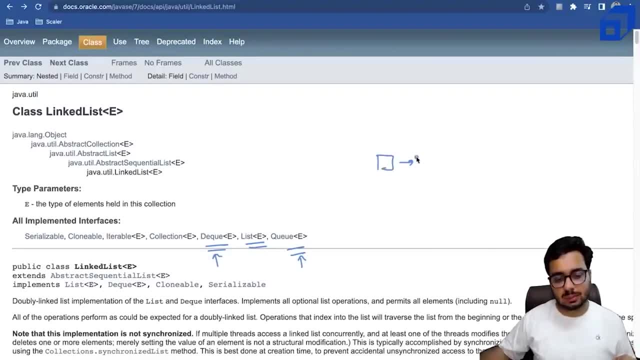 available as a part of linked list. so what is tech deck is a doubly ended link. uh, it's a doubly ended uh queue. that means you can do push and pop. that means you can add from the rear end, add, remove from the rear end. and you can also do push and pop. that means you can add from the front right. 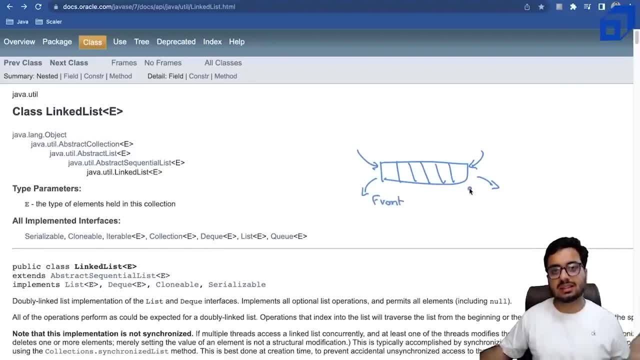 removed from the front side of the queue. That means insertion and deletion can happen at the both ends of the queue. Now, in order to implement this deck interface or the queue interface, let us look at what all methods are there in the deck interface. 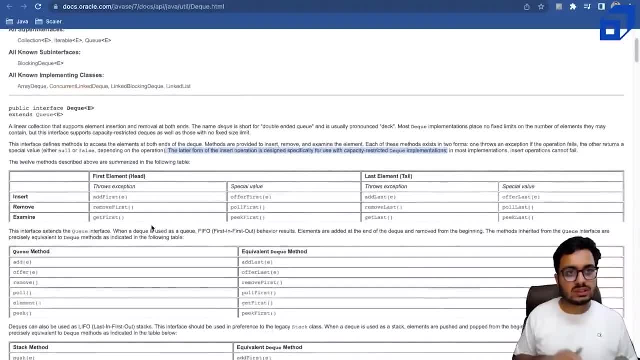 Inside the deck interface you see there are methods. you want to insert something: at the beginning there is an addFirst method that should be implemented by that class. You want to remove something? the removeFirst should be there. You want to get something? getFirst should be there. 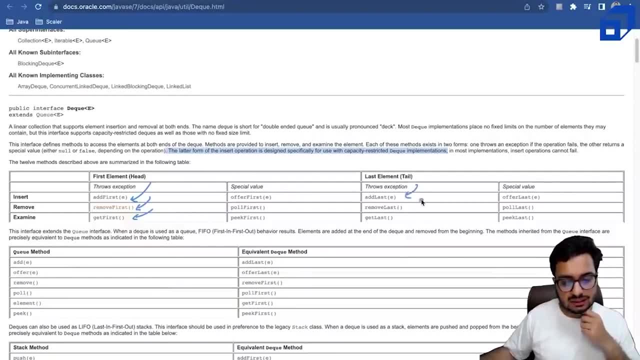 Similarly for the last element. addLast, removeLast and getLast should be there. Now there are two versions of the same method. One is addFirst, one is offerFirst. What is the difference between addFirst and offerFirst? The difference is written here. 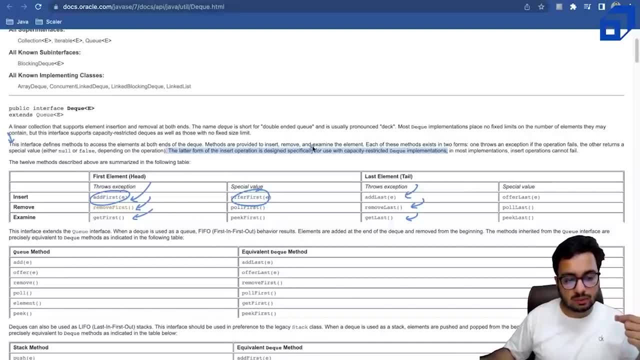 What they are saying is that both methods are provided to insert, remove and examine the element. Each of these methods exist in two forms. One throws an exception if the operation fails. the other returns a special value, Basically your offer method. it returns like true or false or null if your operation fails. 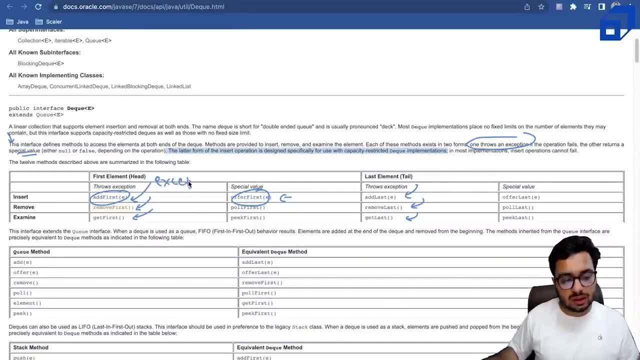 Whereas addFirst will throw an exception. It again depends upon your use case: how you want to use this method. If you are working in an environment where your capacity of the data structure is restricted and you are trying to insert something And your data structure is already full. 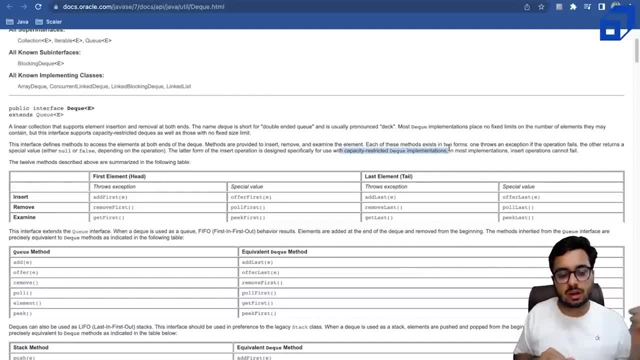 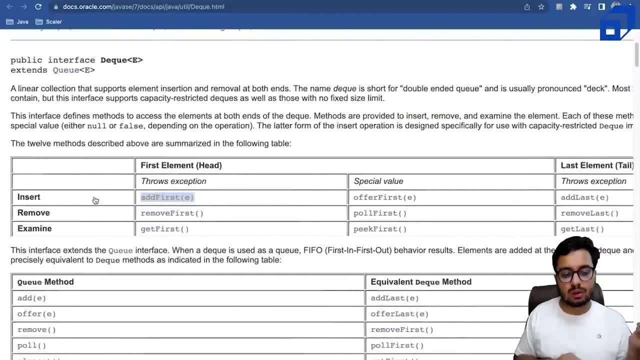 What do you want? Should I, should it return false, that I cannot execute this operation, or should it throw an exception? If you want to throw an exception, go with the addFirst method. You want to handle it using a value like true, false or null, you will have to go with the. 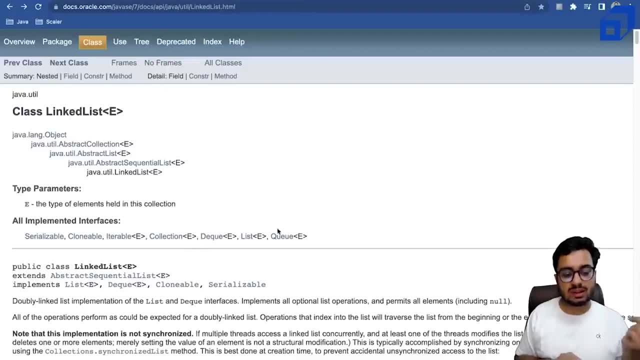 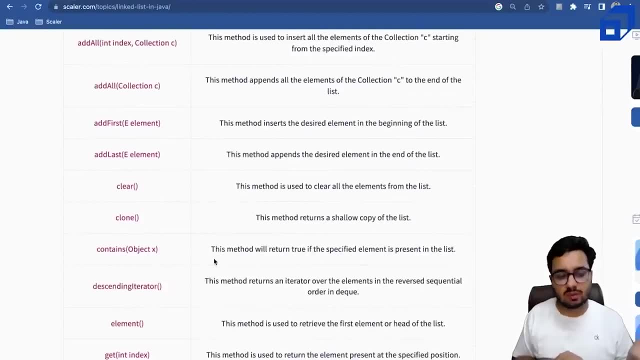 offerFirst method Because linkless implements the queue and the deck interface which needs these methods. Hence you will see there are many methods which are doing this almost same work, right Between addFirst and offerFirst. Between add and offer, there is a difference of the return type. 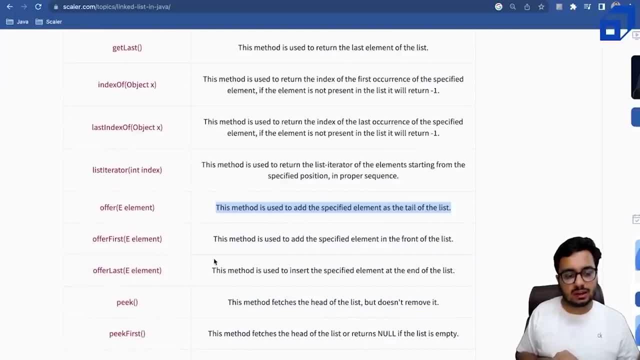 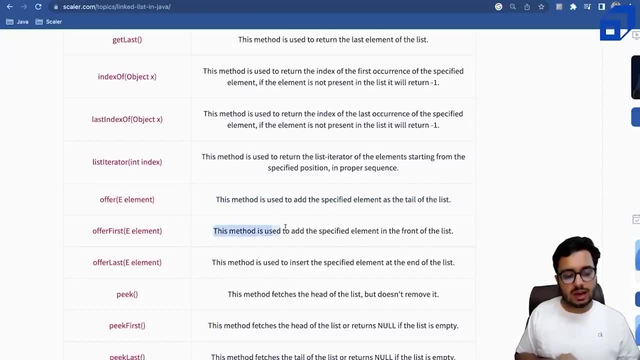 Should you not the return type, but how do you handle the failure case? right? So you are going to return something like true, false, or should I throw an exception? right? So that is offer And we have offerFirst, we have offerLast right. 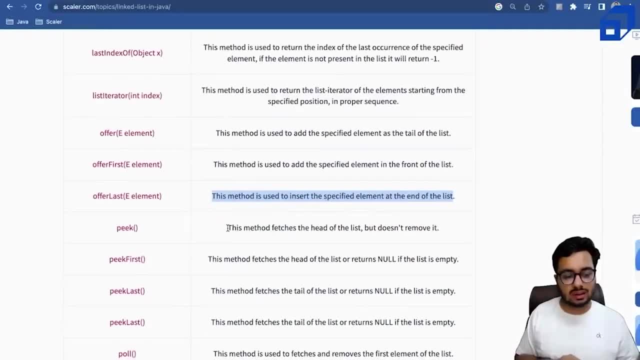 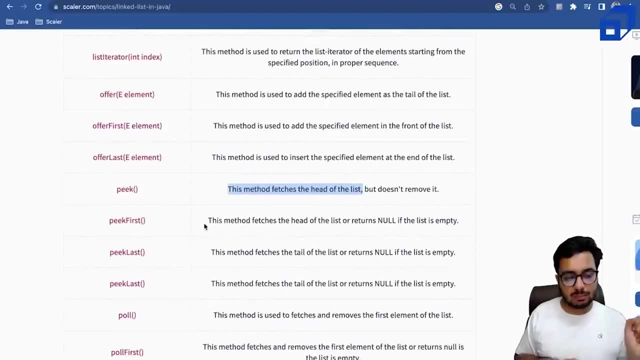 Then there is a method, peek. So peek means look. I want to look at the element. So if you simply call peek, it will show you the first element of the link list, the head of the link list. Peek. first Fetch is the head of the link list. 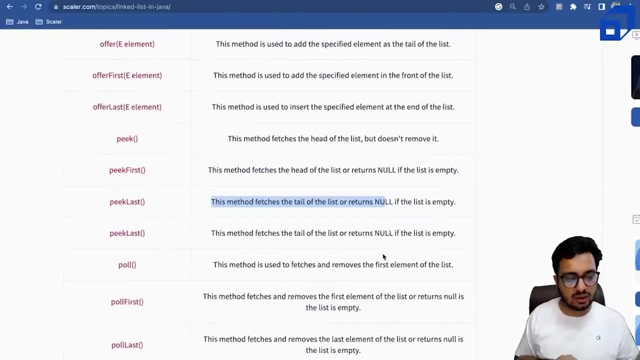 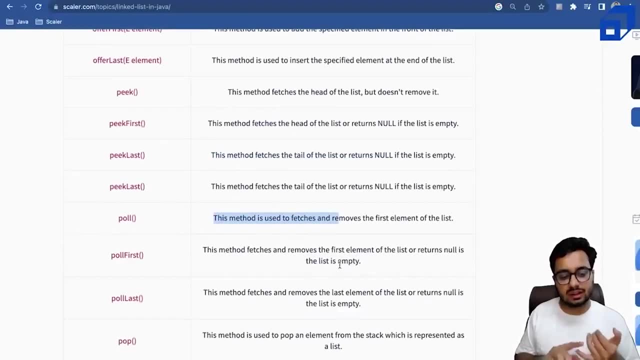 Peek and peek first. they are same, Peek last. show me the last element, right. Then there is a method: poll. Poll means I want to fetch the first element of the link list. It will return the first element and remove it, right. 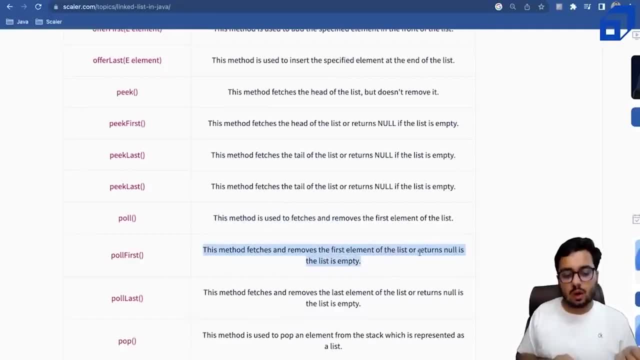 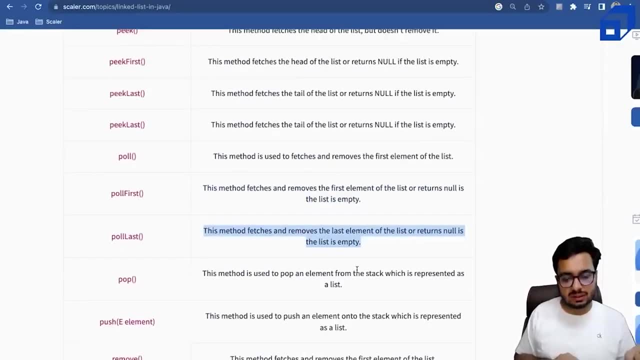 Poll first is also same: Remove the first element, or it's going to return null if the list is empty. Then there is poll last: It will remove and give you the last element of the link list, or it will give you null if the link list is empty. right, 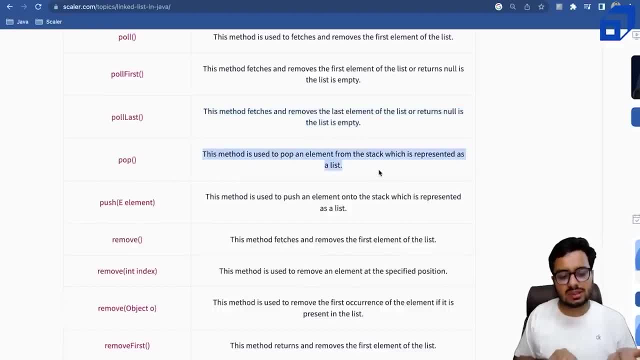 There is a method called pop as well. Link list can also be used as a stack. So in stack we generally call removing the last element as pop right And push is also there. If you want to push something in the stack, I can say, okay, I'm pushing something. 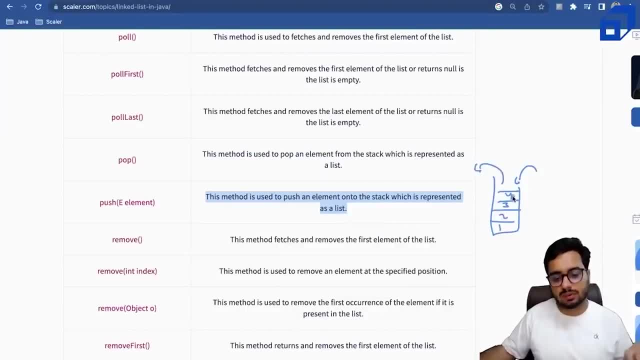 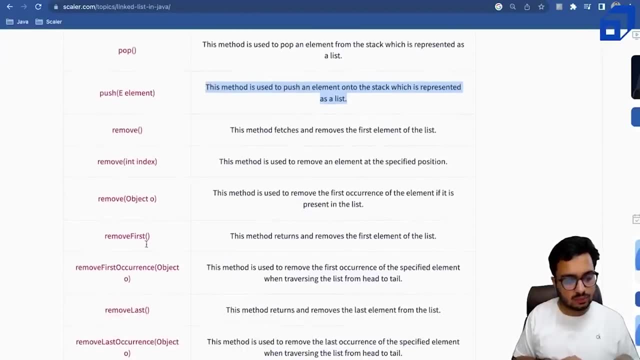 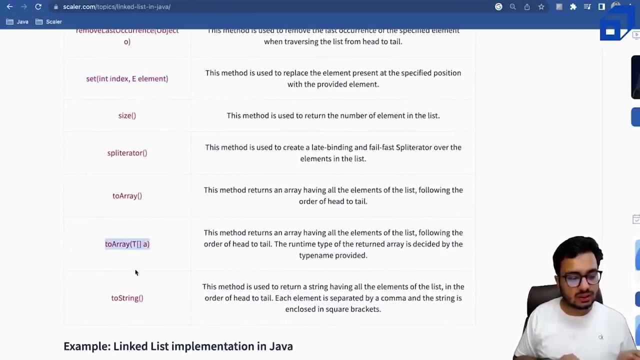 So it will push something into the link list. If I say pop, it will remove last inserted element from the link list. Similarly, the remove method is there. Remove first is there. Remove last is there. Set is there. You want to update a particular element and to string: is there? 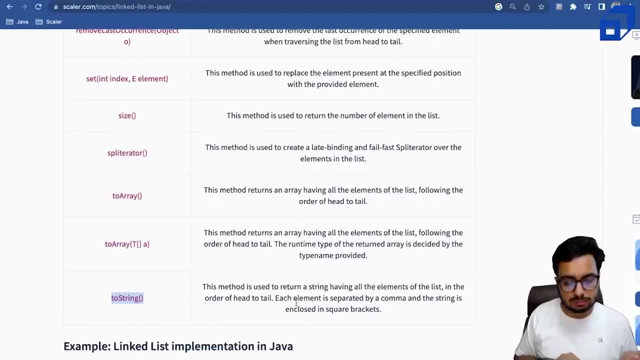 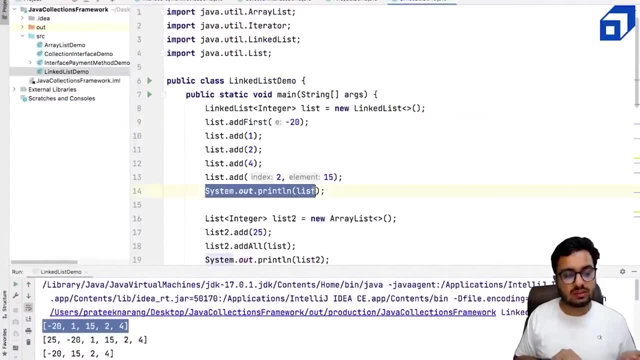 That means if I want to print a link list, it will call the two string method and each element is separated by a comma and it is enclosed in square bracket. When, whenever we are printing this and whenever we are using system dot out, dot print list. 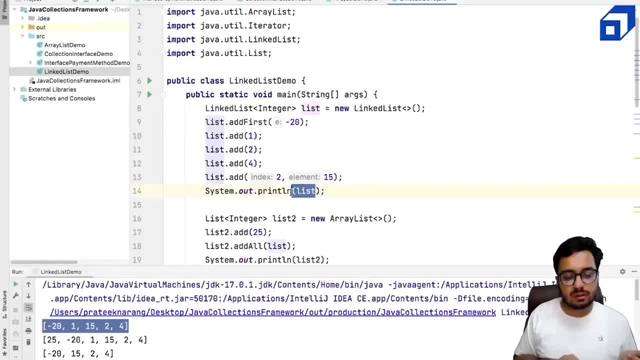 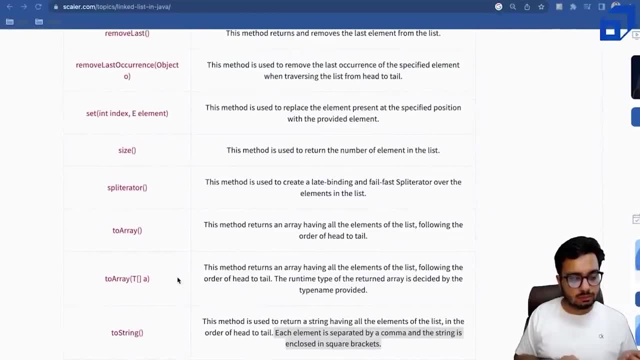 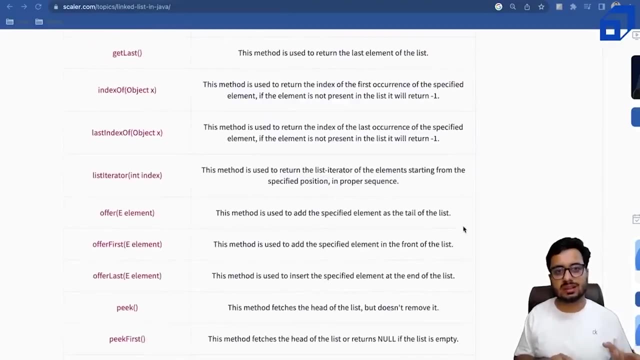 what is happening internally. It is using the two string method of the list object to give us list which looks like this: Okay, So I hope you really got an idea on what all methods you can use on a link list. So many methods are there. 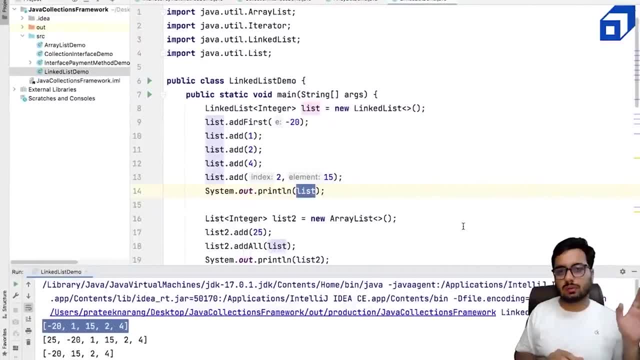 So mainly you need to remember that you can work on both ends. You can work on the front side, you can work on the rear end and you can also insert in the middle, search in the middle, but insertion and deletion at the ends it is fast in the 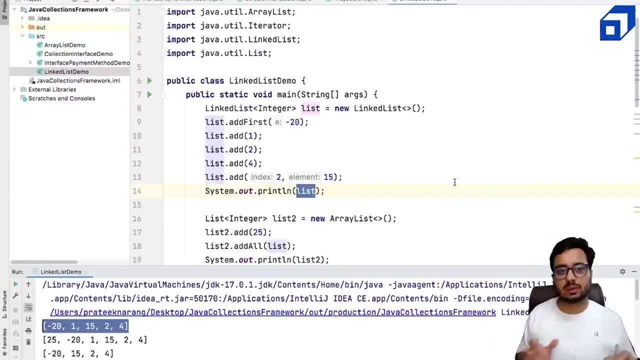 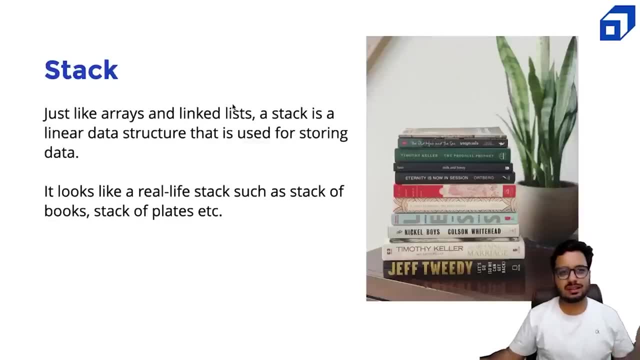 middle: It's difficult. Random access: It's difficult. It's going to take order of end time compared to an array. So that's all. I will see you in the next data structure. Let's talk about stock. Stock is a very simple and easy to use data structure. 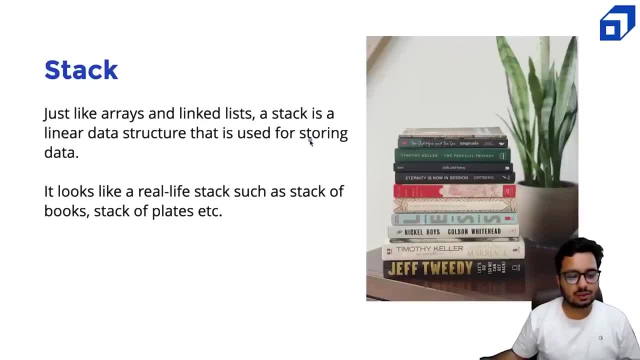 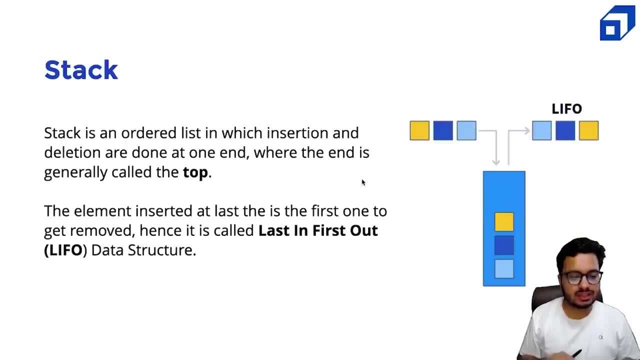 So, just like errors and link list, it is also a linear data structure that is used for storing data and it looks very much like a real life stock, such as a stock of books, a stock of plates And uh, let's see. so it's kind of an ordered list in which insertion and deletion are done. 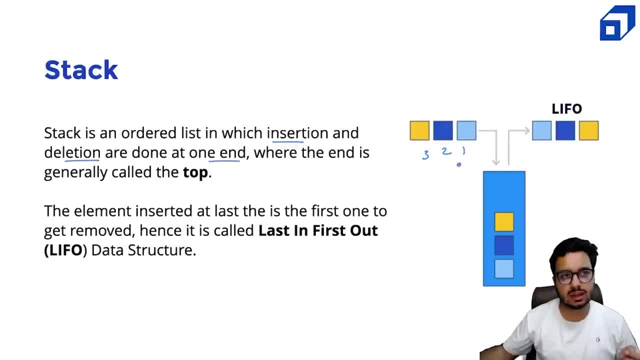 only at one end. For example, if you have items coming in, one, two, three and you push them items into a stock, So one will go, then on the top of it two, two will go and three will go. And if you start popping items, three will come first, then two will come and then one. 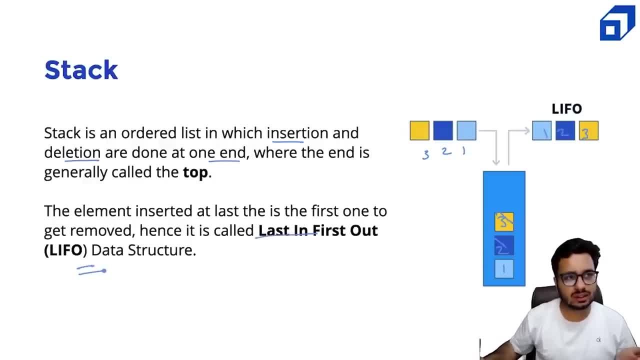 will come. So it's also called as last in, first out data structure. The element which is inserted at the last is the first one to get removed. For example, if you keep a stack of books, you put a C++ book and you put a Java book. 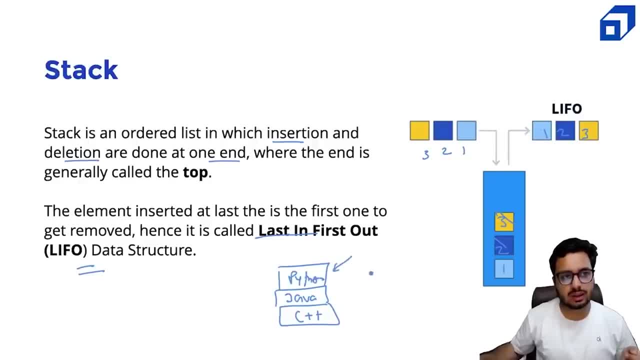 and then you buy: put a Python book- Python book is the one that you can pick first, followed by Java book, followed by C++ book, last in, first out, property stackhacker. Okay, So internally, if you want to see how it is implemented, you can use a fixed size array. 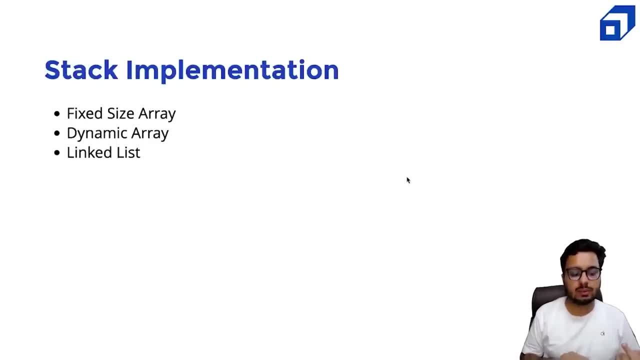 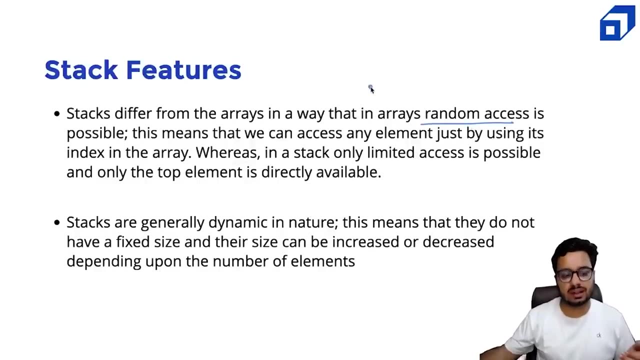 You can also use a dynamic array. You can also use a linked list to implement a stack And how it is different from arrays. arrays allows random access. You can get any ith element, but in case of stack of books, you can only access the top. 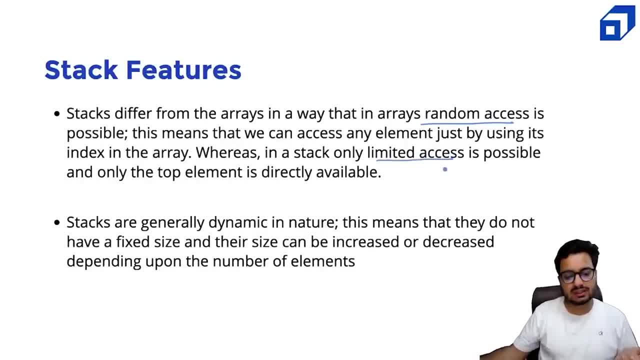 most element. So in a way there is a limited access possible and only top most element is directly available in case of a stack, Stacks are generally dynamic in nature. That means you don't have a fixed size And size can be increased or decreased depending upon the push and the pop operations that 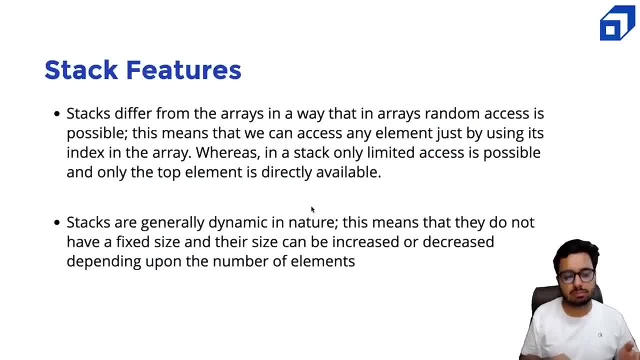 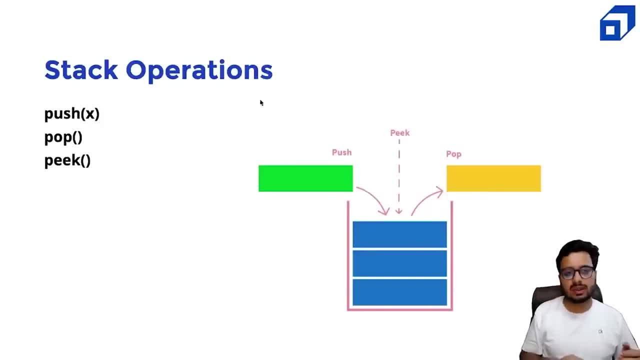 we are doing Right. So the container that you are using can be a fixed size array as well, But in general it would be dynamic, such as a dynamic array or a linked list. So the operations on stack: they are very simple. 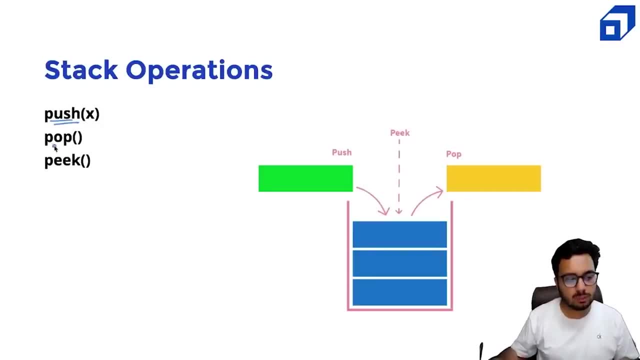 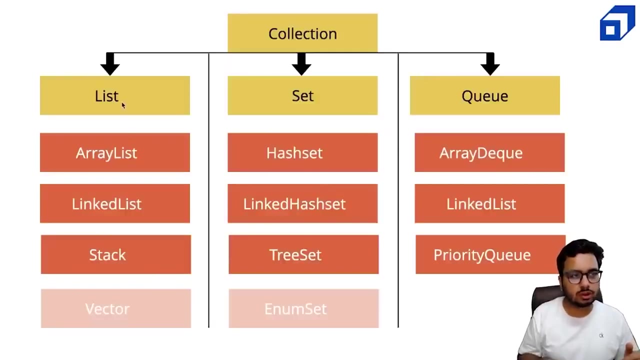 You can push an element into the stack and pop something from the stack and you can peak. peak means you can look at the top most. Let us look at a code demo to understand these operations. Okay, So in Java we have a stack class which is uh, which also implements your uh list interface. 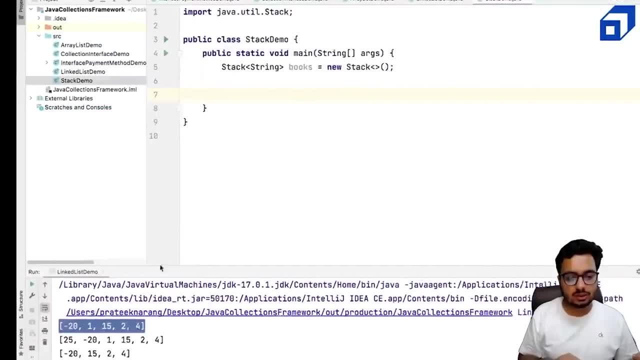 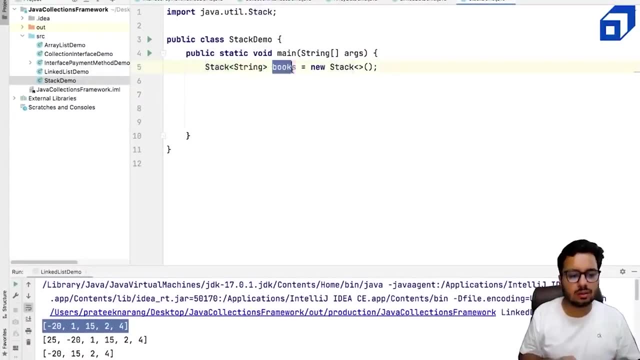 but on the top of it stack has its own methods as well. So let's look at a demo, right? So I have created a stock object stack of string or books, and in this I can push something. So I can say: books, dot push right. 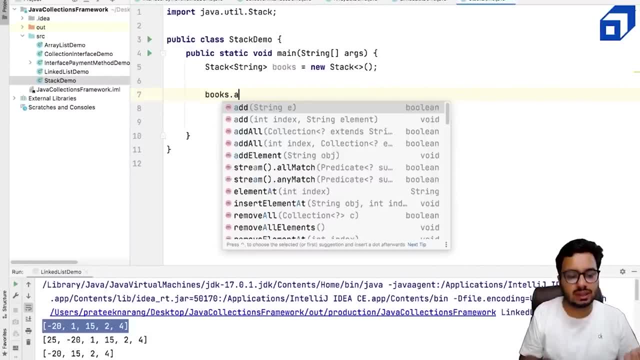 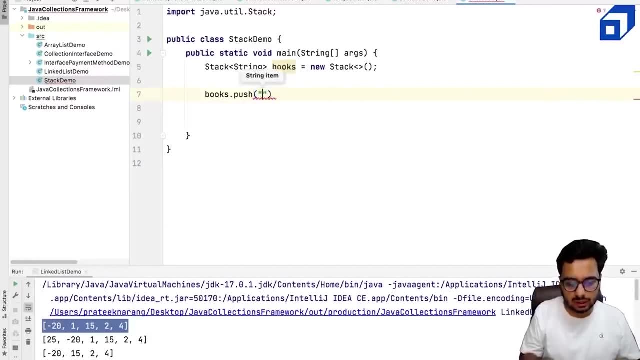 Now you see, there is an art method as well. The art method is coming from the list interface. Oh, So I can simply call push method, which is specifically implemented by the stock class. So I can do. Okay, Let me push C plus plus. 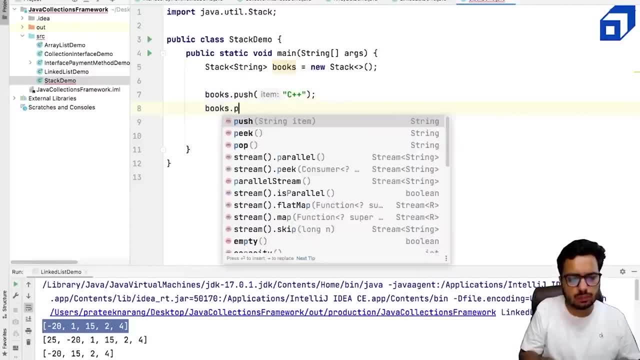 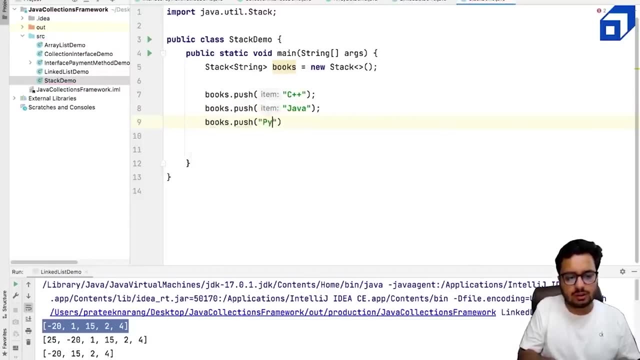 Let me push Java And let me push Python. Let me just create three books and push it as, okay, Python. Oh, if I print the stock, it can. Okay, Show me, what elements do we have? I call it as books. 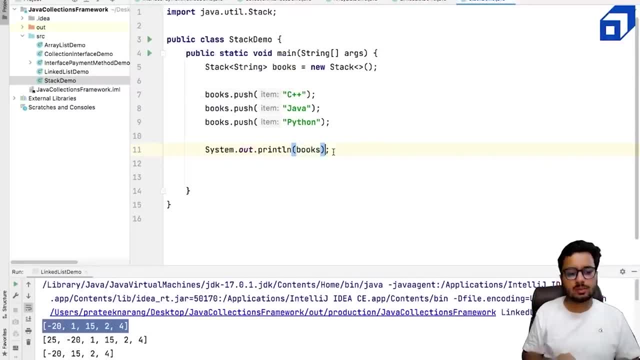 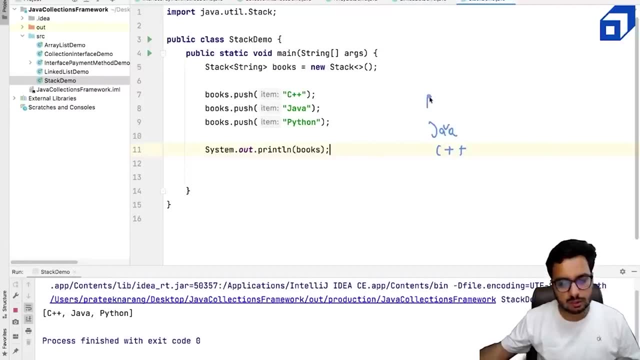 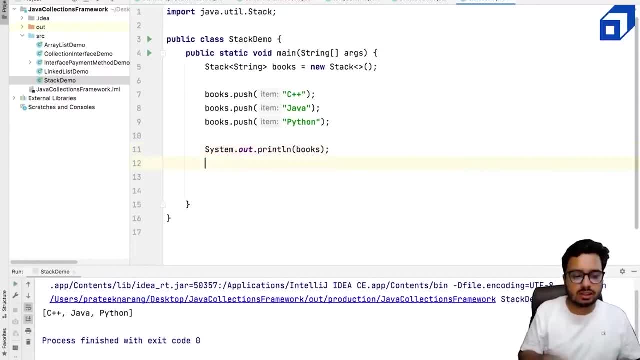 I want to look at the top most element, so I can simply call peak, right. So I can say, okay, Uh S out books start peak, that will give me by 10. And if I want to remove it I can call the pop method. 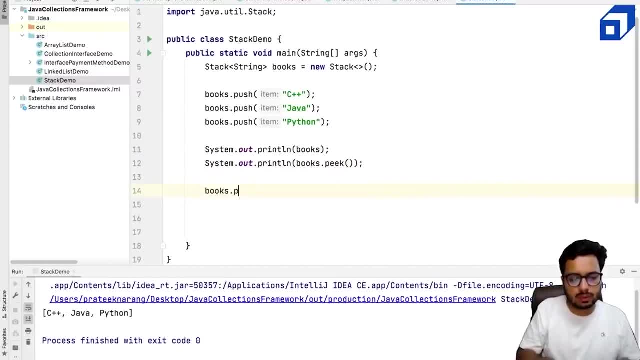 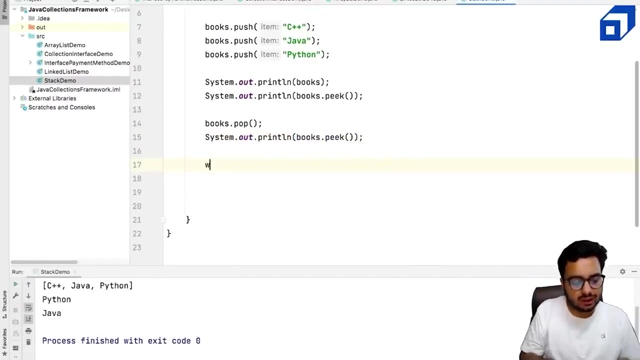 I can say: book start, pop, That is going to remove topmost element. and now, if i do peek, i will see java next s out books dot. and apart from these methods, we also we can run a loop, like we can say: okay, uh, while the stack is not empty, i want to uh. 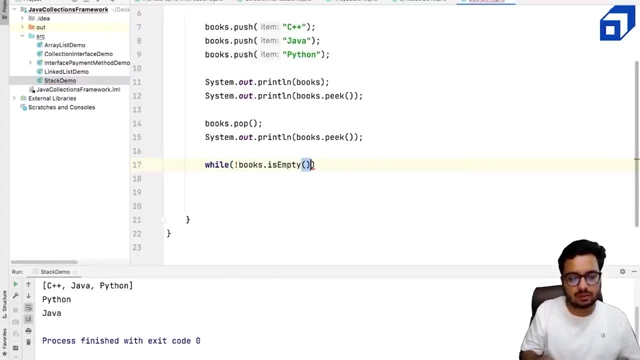 stack dot. sorry, books dot is empty. while this is not empty, i want to keep on copying elements. i want to remove them so i can say s out um, books dot peak and i want to pop everything books dot. this is one way to iterate on the stack. you have to remove all the elements and 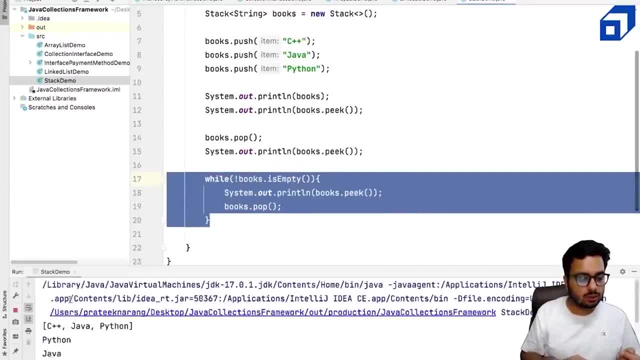 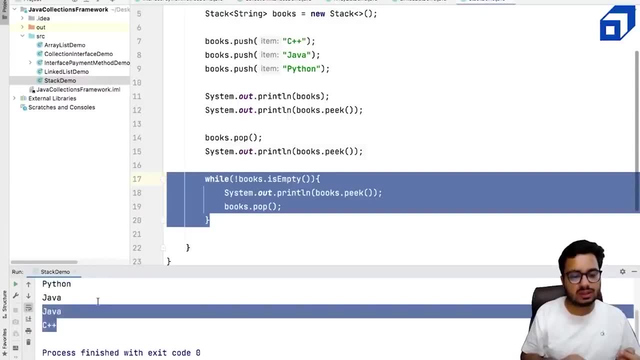 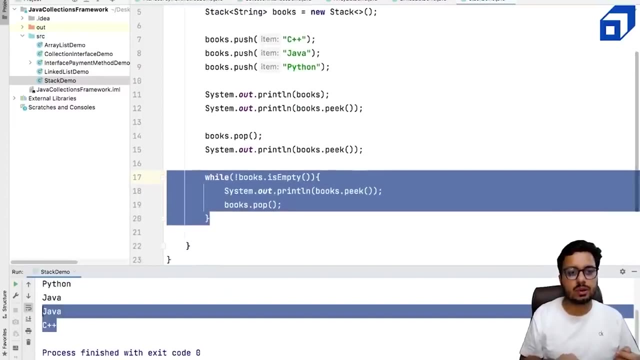 yeah, so i hope you are able to understand this example. so we are able to remove all elements. we first removed python, then we removed java and then we removed s plus as well. that's all about stack. uh, very simple data structure, right, and hopefully you will be able to use it. let us talk about queue. 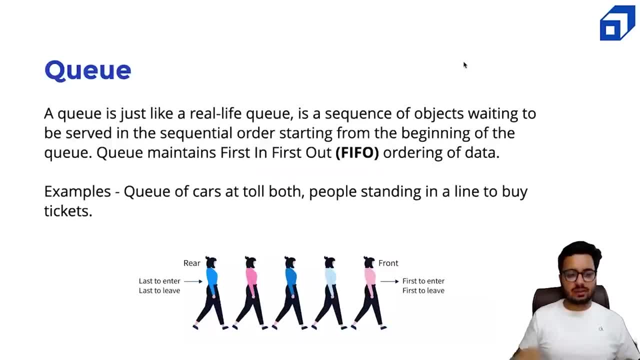 a queue again is a very simple data structure. it's just like a real life queue: the sequence of object waiting to be served in the sequential order, starting from the beginning of the queue. so in general queue maintains a fifo kind of ordering, but we also have something called as: 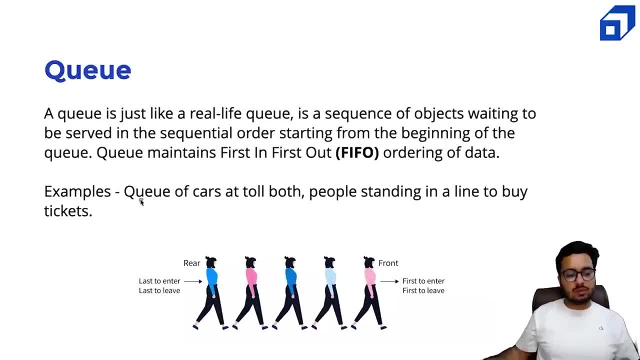 a priority queue, which is little different. for example, a fifa cube would mean a queue of cars at a toll booth. cars are coming in to get their ticket, or people are standing in a line to buy their ticket. what happens in general? people enter from the rear end of the queue and they leave from the. 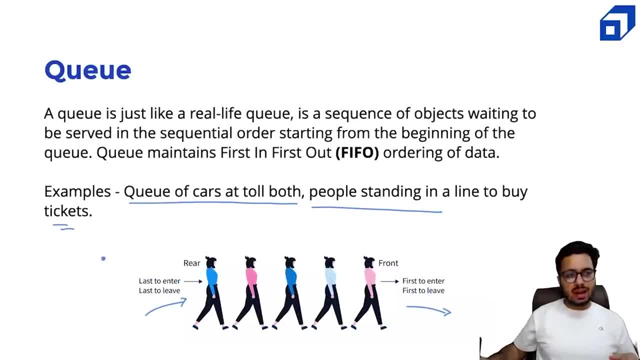 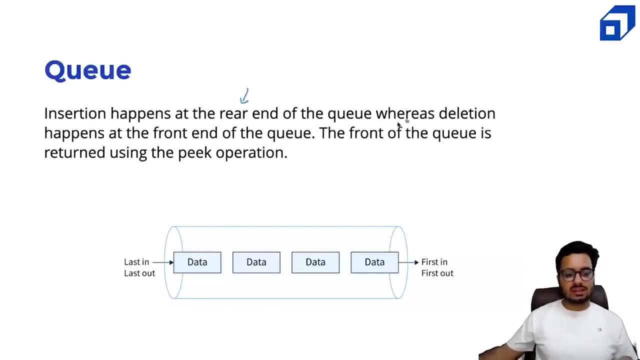 front side of the queue once they get the ticket. so adding something in into the queue, it's called as nq. removing something from the queue is called as dq. someone has been removed from the queue. so insertion, as i discussed, it happens at the rear end of the queue, whereas deletion 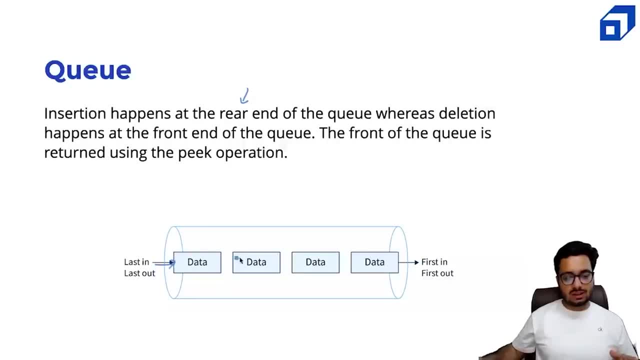 happens at the front end of the queue. last in, uh, last out. the person who is entering in the last is the last one to come out, or you can say it's a fifo: first in, first out. the person who is coming first is the first one to come out right the front. 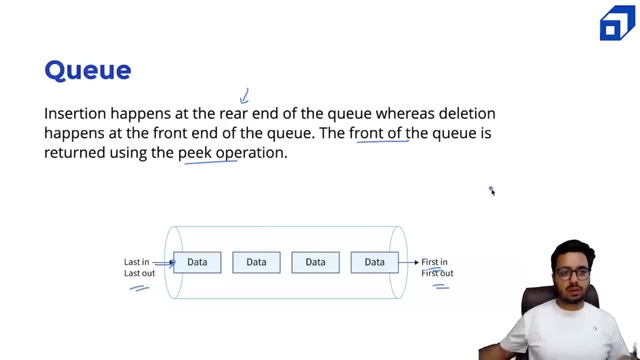 of the queue is returned using a peak operation. so if you want to say okay, i want to see who is at the front, the most libraries. they have a peak method like in java. we have a peak method to see what element is at the front of the queue right, and similarly there are methods like offer to add. 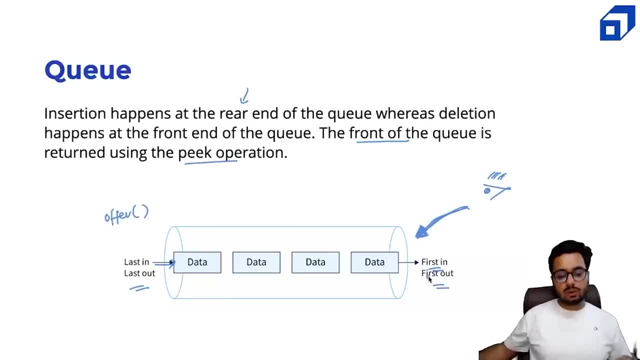 something at the end of the queue and if you want to remove something from the front side, it's called as pole right. we'll look at three methods: offer adding something at the rear end, polling, removing something from the front side. and peaking means looking what is at the front. okay, so 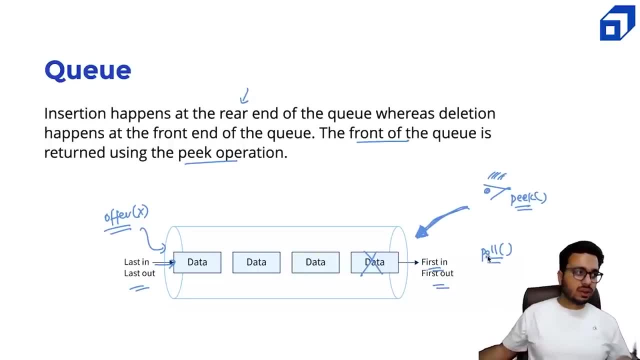 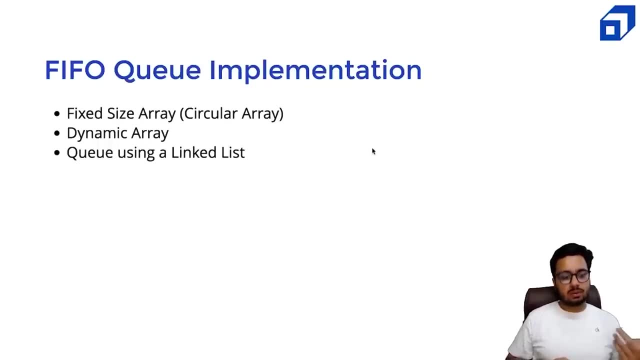 peak only gives you the element, whereas pole removes an element from the queue type. so these are three methods that we will discuss. if you want to implement a cube at your own end, you can use a fixed size array, also known as a circular array, to implement the. 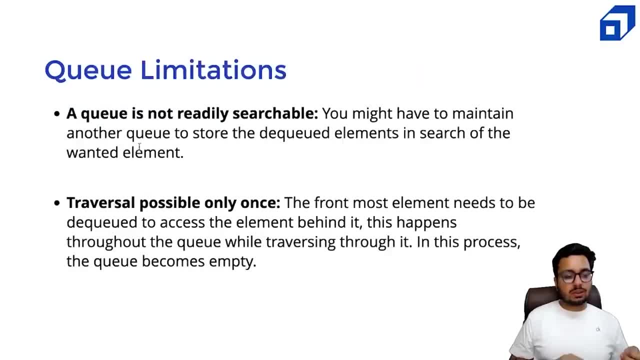 queue. you can also use a dynamic area or also you can use a linked list. so there are limitations of queue data structures. a queue is not readily searchable. you cannot go inside the queue and search, so you might have to maintain another queue to store the dqd elements. okay, so you have to empty. 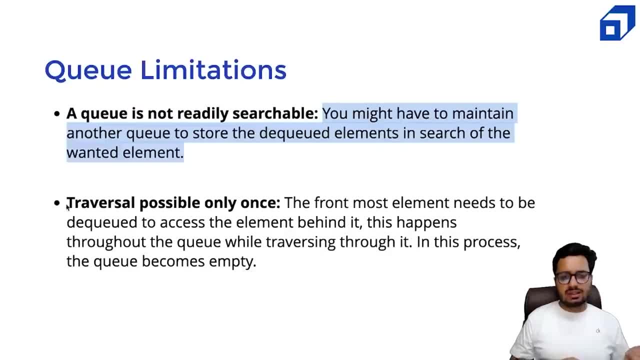 the entire queue. if you want to search for something and traverse cell, of course we cannot traverse, that is the same thing. so you have to again remove the element from the queue type and move all the elements to do that reversal and in this process q becomes empty. so these are: 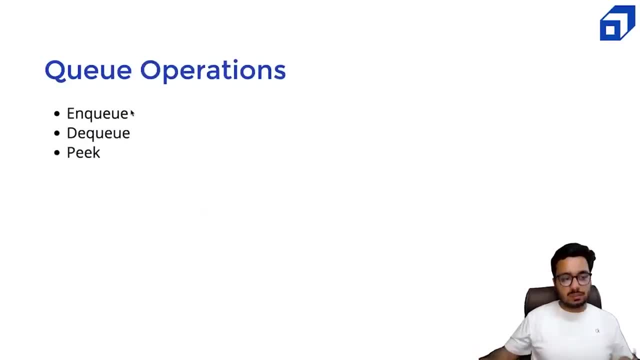 limitations of the queue, so operations. you want to add something? so the equivalent java method. it is called as offer. i want to add something into the queue, want to remove something? the java method. it is called as pole. and if you want to look, who is there standing at the front? 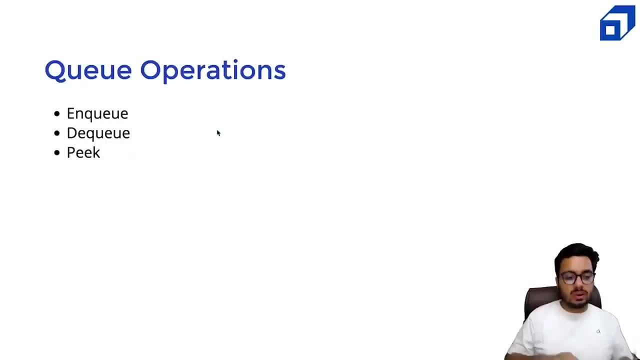 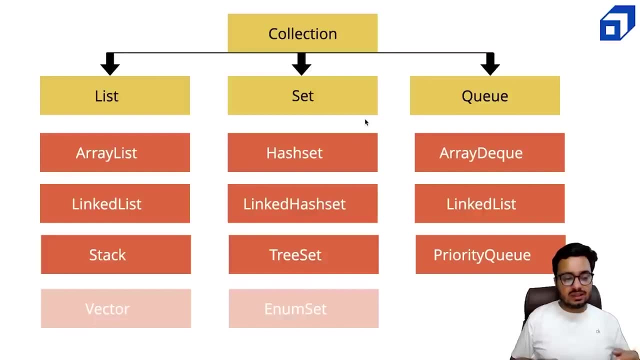 the method is called as p. let us look at the q methods in our code demo. and if i talk about what are the methods there in java, right? so if i told you that q is an interface in java, right? so this interface is implemented by three different classes. one is called aerodeck. 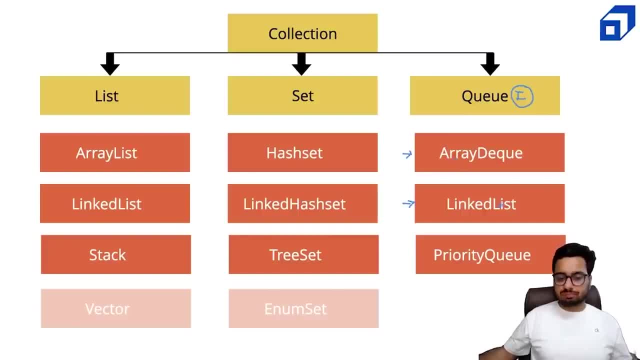 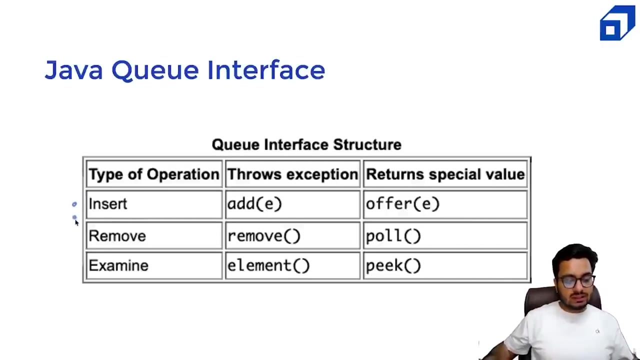 which stands for w ended queue. we can use linked list, which we will be using to implement our before queue, and there is also something called as priority queue which we will also study very soon. we'll go with the linked list while implementation right the methods that i told you. they are insert. 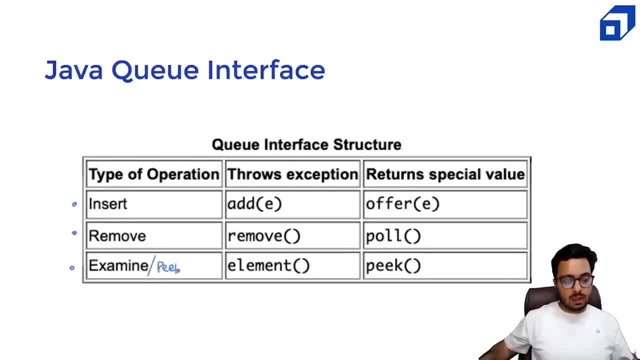 remove and examining. examine is like peak right now. again, i told you there are two, two versions that java provides one set of methods that throws exception. so if you use- okay, i want to add something into the queue, there is a add method. or if you want to do the same functionality, you can also use the offer. 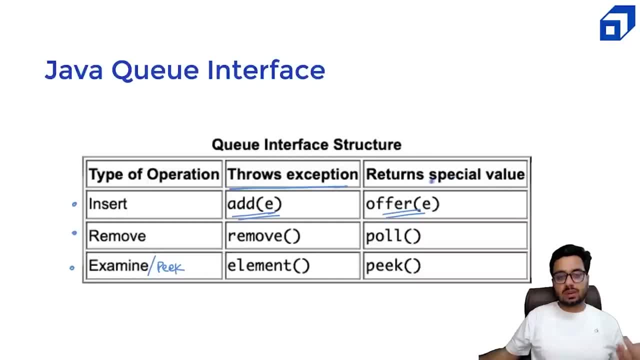 method. offer method returns a special value, whether your operation was successful or not. add method might throw an exception if your add operation fails because of some reason. okay, similarly, remove throws an exception if your operation fails. pole will not throw an exception element. you're looking for an? 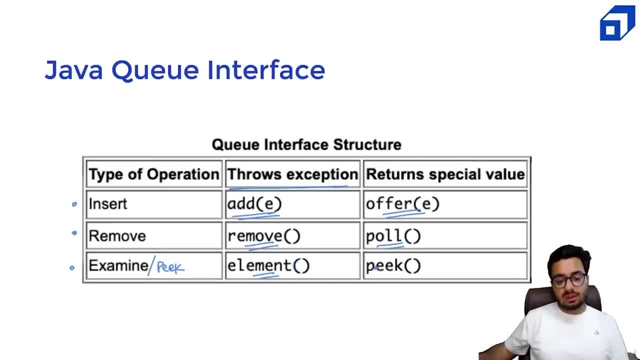 element, maybe at the empty queue right, it can throw an exception. peak will not throw in. this is how these methods are designed, so i will be going with these methods. okay, in the implementation, let me jump into the code and let's quickly create a queue, right? well, it's okay, i want to create a queue of. 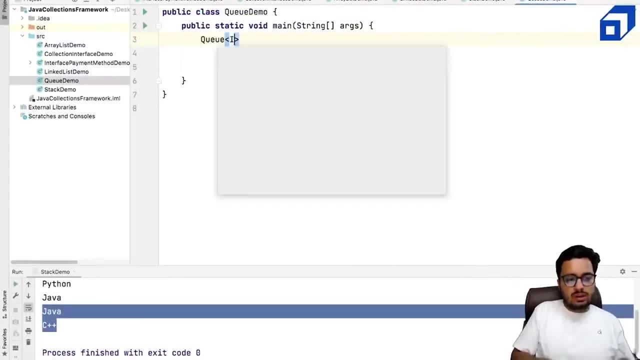 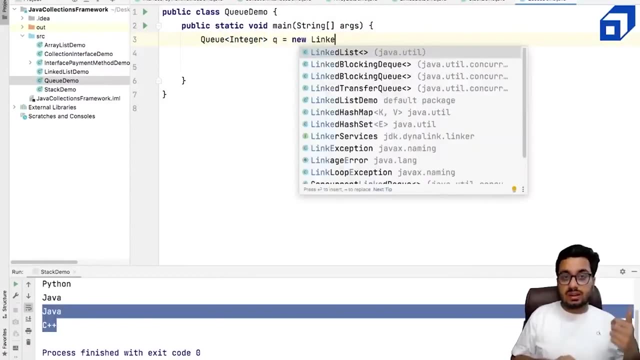 let me jump into the code and let's quickly create a queue, right? well, it's okay. i want to create a integers. i call it as q and is okay. the q implementation. so q is an interface. the implementation is provided by the linked list. so we'll be using linked list for this queue, right? 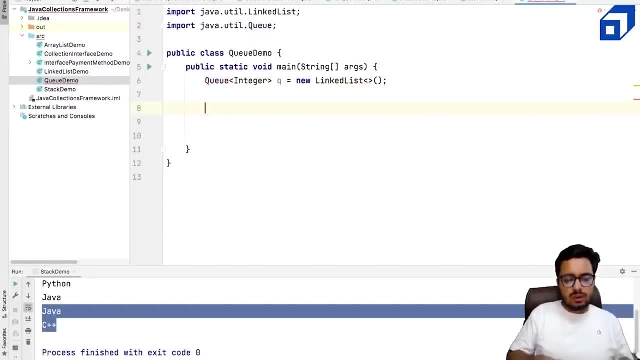 so we also need to import it. now how do i do it? i can say q, dot, add some numbers. let's say one, two, three and four. let me just copy this now if i say, okay, i want to see who is at the front of the queue. or let's just print: 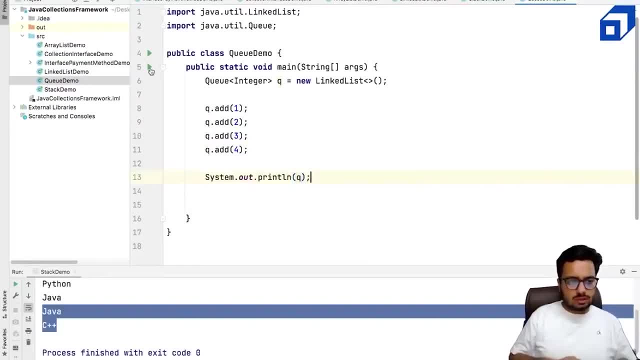 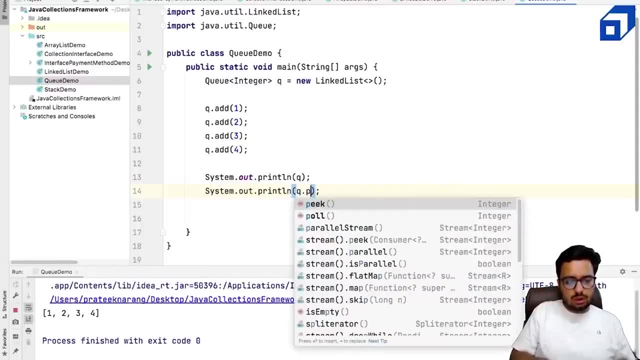 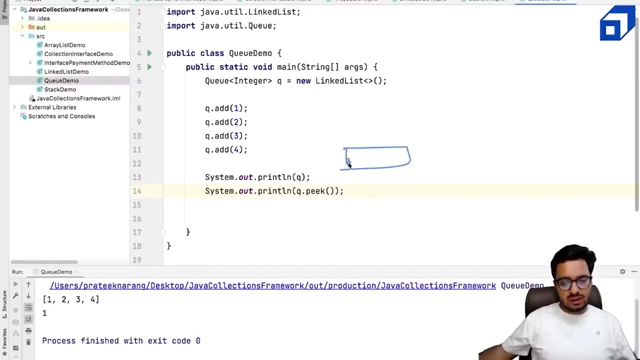 the entire queue. let's uh run this code and simultaneously let's see who is at the front of the queue so i can say: s out q dot p. show me who is standing at the front, i will see. one is standing at the front, so one came first. right now, if i remove this, it's okay. i want to remove one. i. 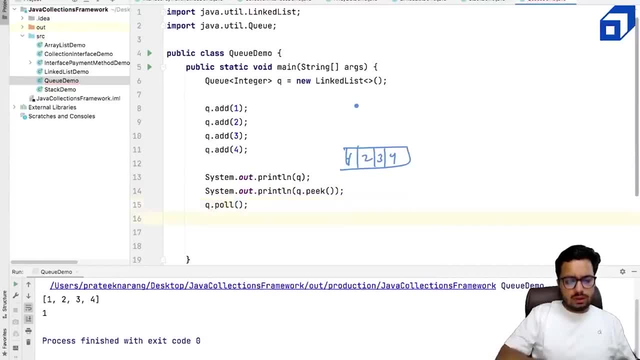 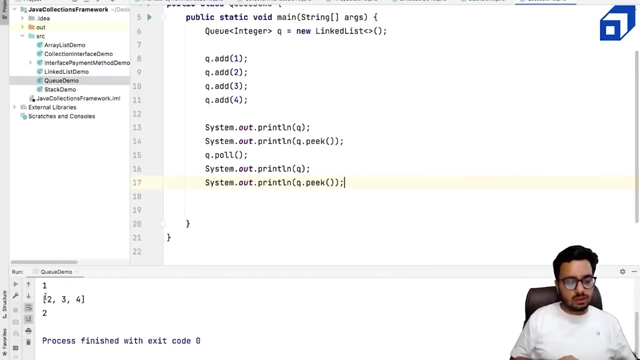 can say q dot, um whole. and then i can say: show me the entire queue and also show me the front element. i can say q dot, just like stack. you can also use a while loop to empty all the elements of the queue. so after removing one, the queue is two, three, four. and if i look at the front element, the front element is now. 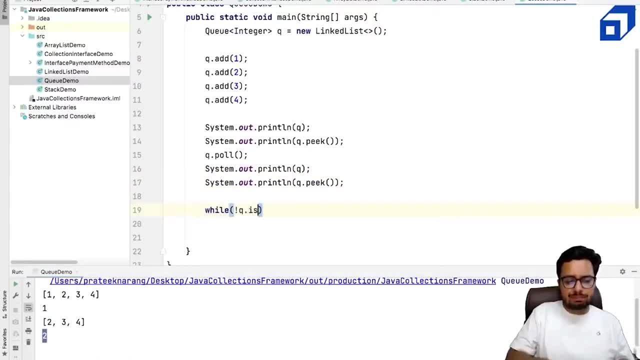 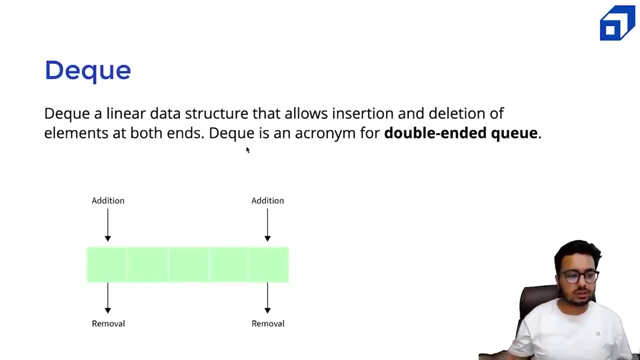 so you can put a loop like this: while your queue is not empty, you can keep on removing the elements from the queue. that is all about q. i hope you really understood how to use q in java. so next in line is the dec data structure. so it stands for doubly ended queue and it's pronounced as dec. 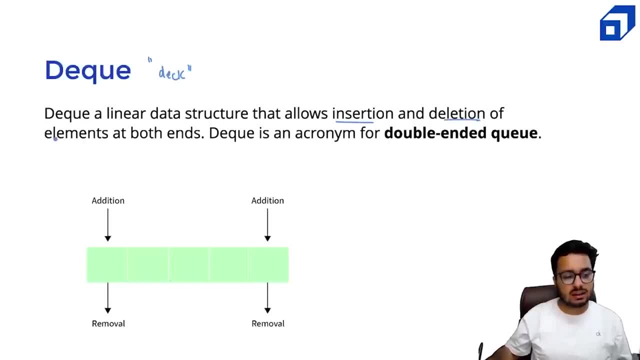 so it is again a linear data structure that allows insertion and deletion at the both ends. okay, so you, you can do insert here, you can. okay, i can expand in this side, or i can also expand in this side. maybe i insert 5, maybe i insert 12.. 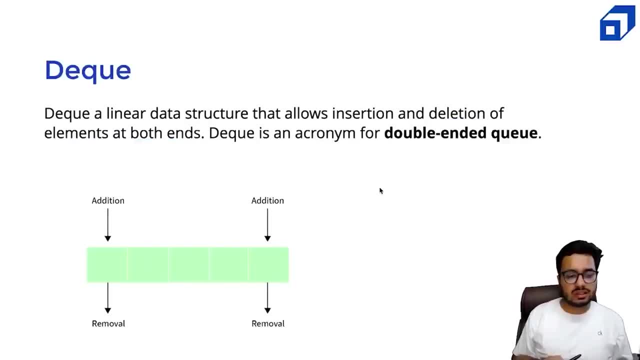 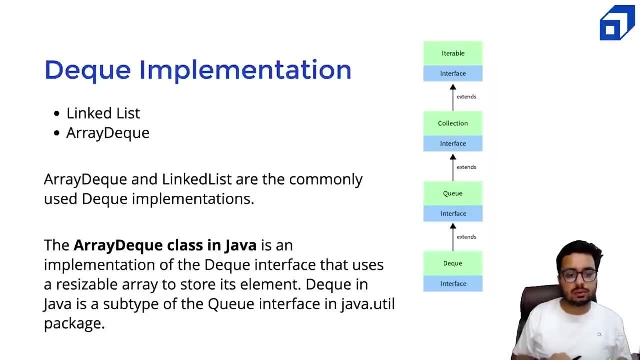 question as well. with q dot add, you just need to check your performance and other businesses with q dot remove from both ends of the queue. it's a queue that supports insertion and deletion at both ends. basically, internally, we can use a linked list to implement it, and java also provides a special 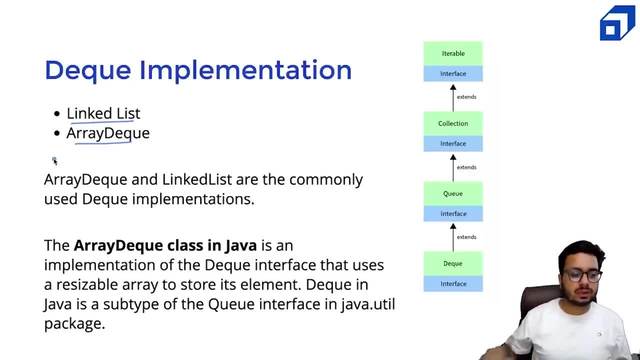 class called as array deck, which implements the deck right. so if i look at the hierarchy, so we start with the collection interface. we have seen the queue interface extends the collection interface. it adds some more methods into the collection. then there is also a deck interface which i have not shown earlier in the diagram, and the array deck is a implementation of. 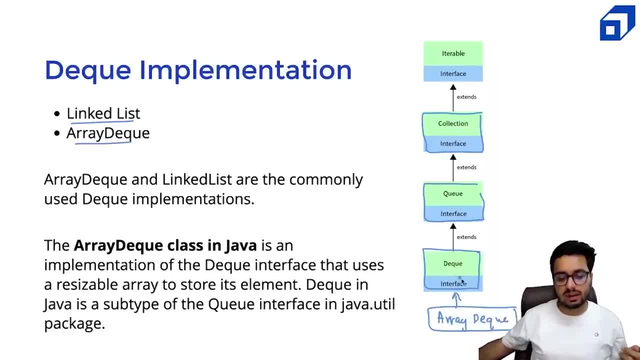 the deck interface. array deck is implementing the class that implements the deck interface, which is extending the queue interface. okay, so this is what you- it's a good to know thing, not mandatory. right, array, deck and linked list are commonly used deck implementation if it is a w linked list, you can see it is very easy to expand something on both the ends right. 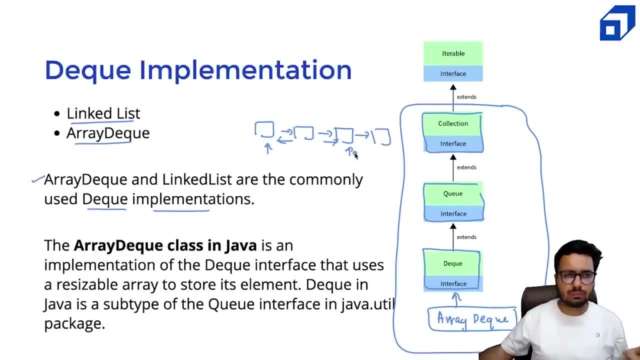 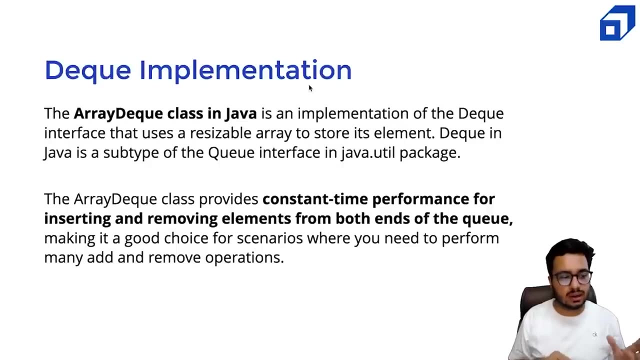 so you can simply add something here as well, and your tail will move right. and add something here as well, your head will move right. so it's pretty easy to use linked list. but array deck internal implementation is little more complicated. i'll discuss few more points about array deck. it is 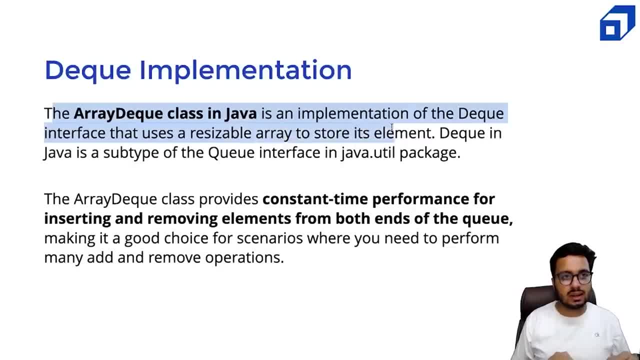 implementation of the deck interface. that uses a resizable array to store its element, and deck is a subtype of queue interface that we have just discussed. best thing about array deck classes: it provides constant time performance for inserting and removing elements from both the ends of the queue. now this is very tricky. right in an array we cannot do constant time insertion and deletion. 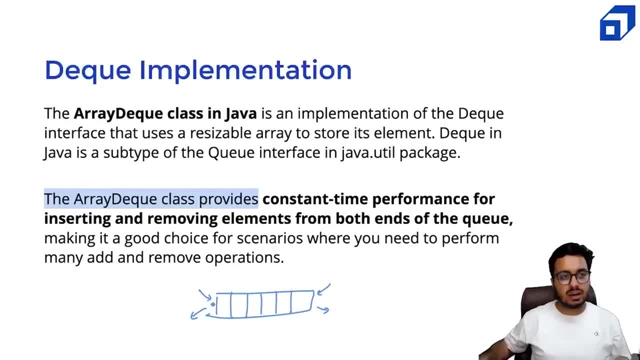 at both the ends. we can do only at one end, right, but in deck, in array deck. it uses internally some complicated mechanism so that we can remove and insert from both the ends of the queue and these operations can be done in order one time from both the ends. this is a very powerful feature of 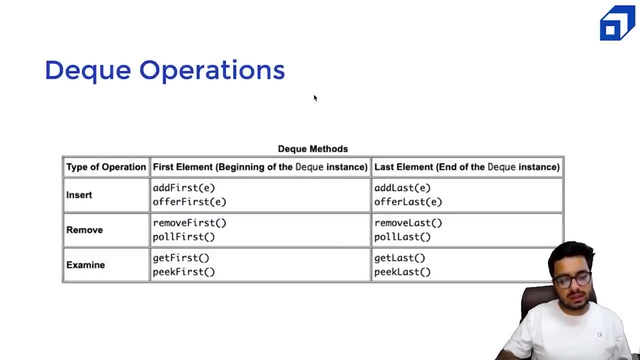 array deck that we must know. talking about the operations, right? if you want to add something at the beginning, you can say add first, okay, or you can use a method called as offer first. these are two methods which are doing the same work. there is a minute difference if due to, let's say, capacity. 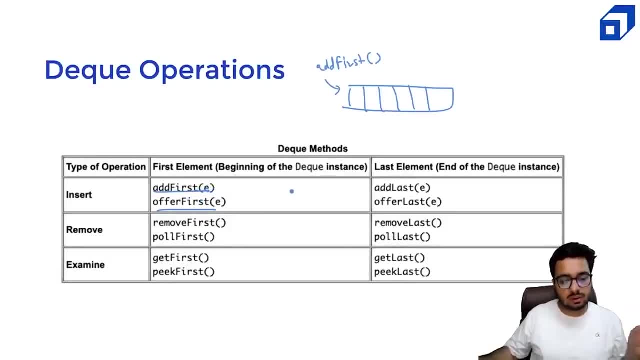 limitation- you don't have many memory- or restricting the size of the queue and you're trying to add some element, then add first. we'll throw an exception. we'll throw an exception, just like other ad methods. we have discount. the offer method will return false. that okay. I could not return this element. I could not add. 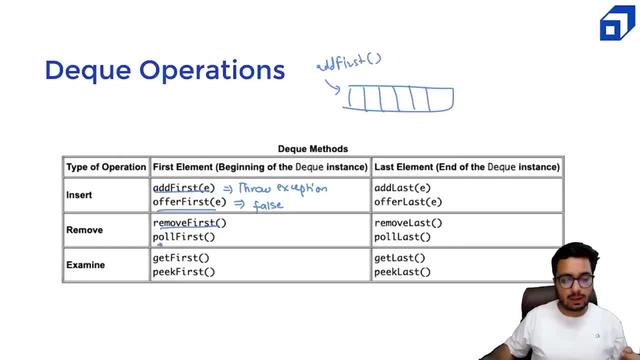 this element. similarly, we have remove first and pole first methods. so remove will throw an exception, pole will return true or false. get first will throw an exception. peak will tell me whether the element like. if I could not get that element, it will throw an exception. peak will tell. 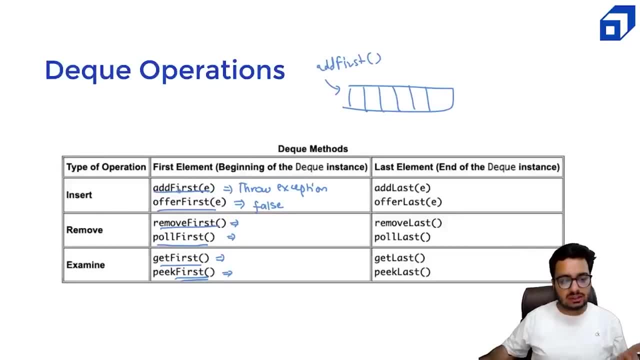 me null. I could not remove that element. that might happen. right, there is add first, there is add last, offer last, remove last whole last, get last peak. if you ask me what method I would be using, I would be using offer first, whole first, peak first. so if you want to do operations at this end, you want to 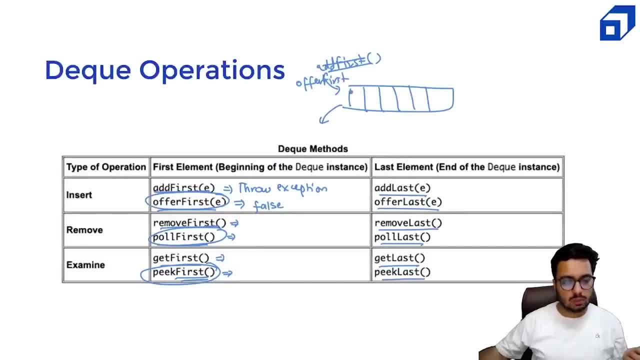 you want to remove something from the front, use pole first. and if you want to look at what is this element you can use, speak first, right same operations. if you want to do at this end what you will do, you will say: offer last. I want to add something here, I want to remove something from. 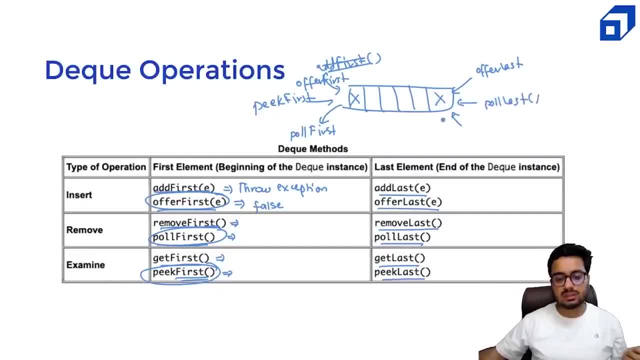 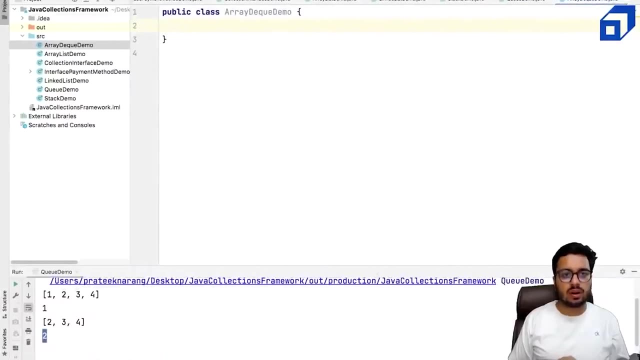 here I will say pole last, and I want to see something. what is this last element? so I can say: peak, show me the last element, this tech. so that is about the operations of tech. now let us look at a code demo or for deck. let us create a array deck object in say array deck of. let's integer: 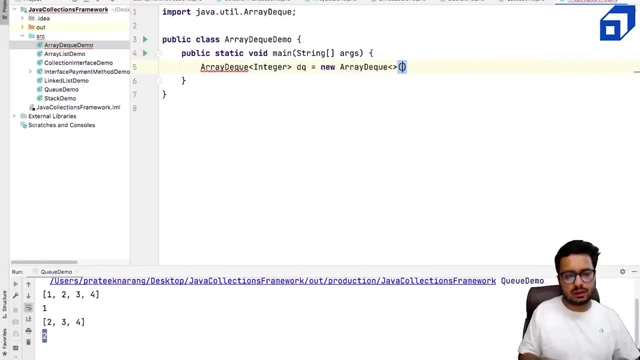 heck. and in this deck I can add elements. I can say, uh, offer. so there is an offer method as well. offer first is there, offer last is seconds. okay, let me show you. offer first, let's say 12, tag dot. offer first, let's say 15. 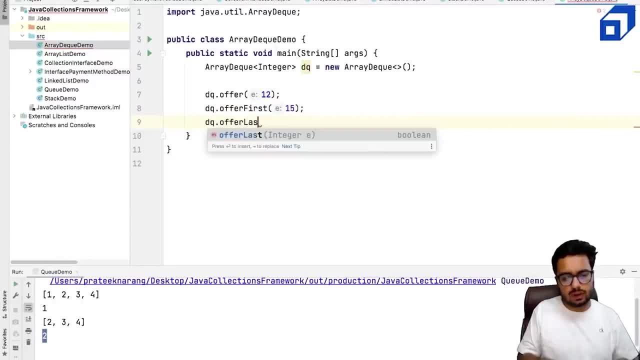 egg dot offer. offer last: it's a 20 egg dot offer. let's say 30.. let me show you what, in what order, the elements will look like. let me show you what, in what order the elements will look like. let us say 30. let me. 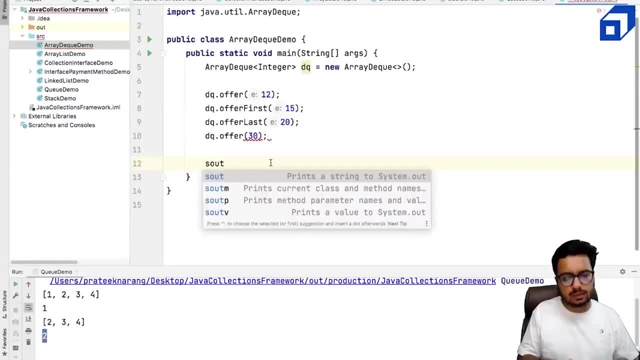 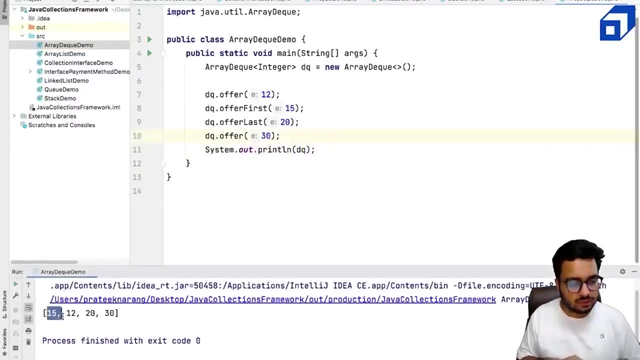 me show you what, in what order, the elements have been inserted. s out, I will say deck and let's run this code. I'm getting 15, 12, 20 and 30. so first I had 12 offer. first I said in the beginning I want 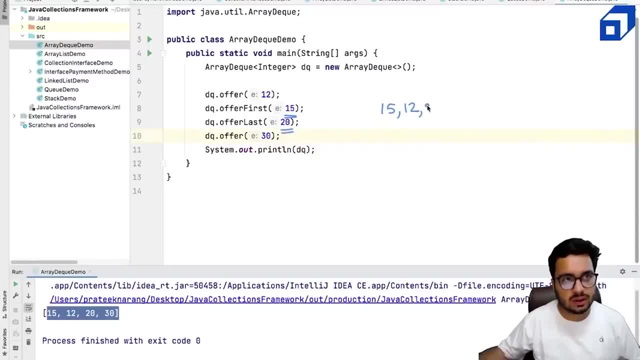 to add something. 15 gets added here and I say offer last 20, so 20 gets added here, then I said offer 30. offer is actually behaving like offer last offer and offer last. they are doing the same work. this is how your deck is getting created. similarly, if you want to remove something and 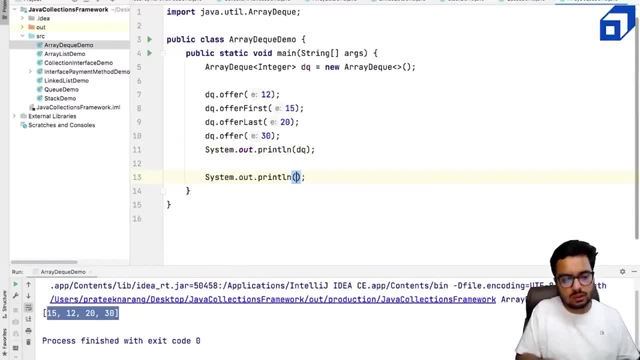 call the poll method. you can say: s out deck dot last, give me the last element. s out deck dot pole first, give me the first element. and if you want to see now what is the new first element, you can just call peak. so when s out deck dot peak first, come with a new first element. 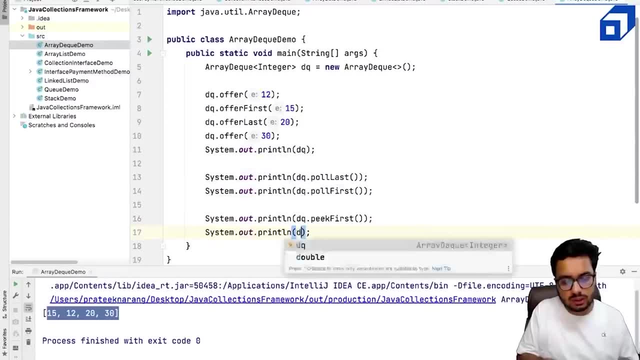 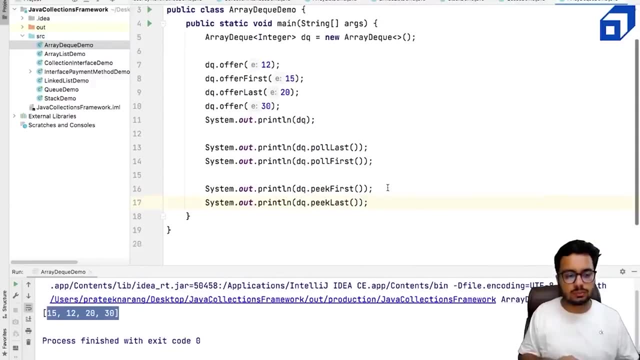 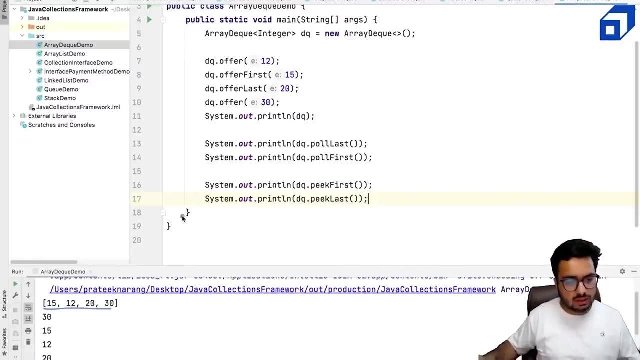 you can just call pick so and say s out deck dot peak. first, show me the new first element element and s out some is a new last element, peak last. let us run the code and see. so this is our deck. now i say, uh, give me the last element, so it removes 30, it's gone. 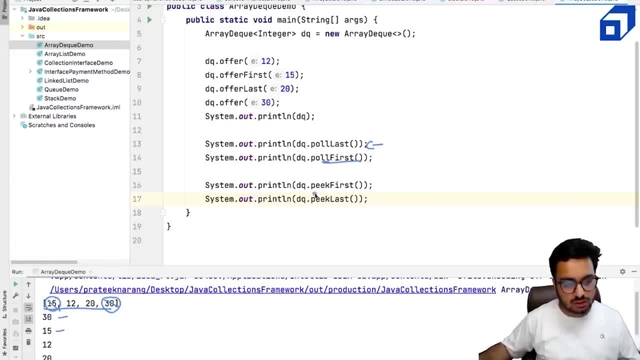 give me the first element. it removes 15. it is gone. show me the first element. the first element is 12. show me the last element, the last element. that is how easy it is to work with tech and i hope you understood the concept. let us talk about priority use. priority queue is a special 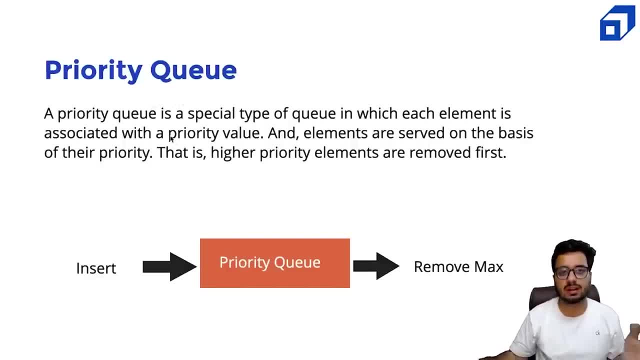 type of queue in which each element is associated with the priority value. for example, if people are standing in a queue and you might want to give priority to the senior citizens, maybe age is a criteria in which people will get their tickets. a senior people will get their ticket first. young- 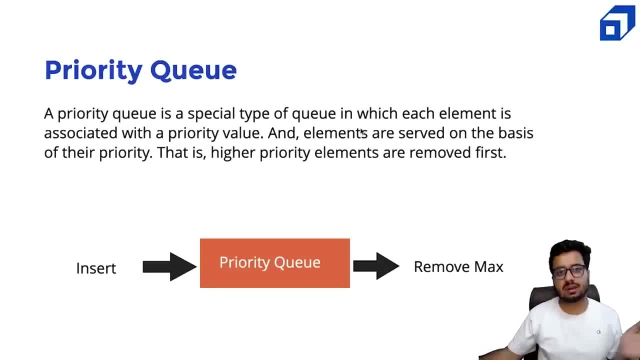 people will get their ticket first and they will get their ticket first and they will get their tickets later. so, basically, elements that we are going to serve in the queue, they will be served according to a certain priority. higher priority elements are going to be removed and it is up to. 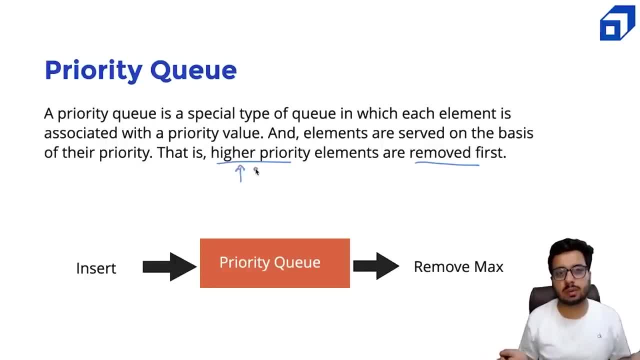 you, how do you define the priority? okay, maybe a big number has a more priority or maybe a lower number has a more priority. you can have a max priority queue. we have a min priority queue. we can insert like: people can join the queue, right, but maybe this is 16 years, this is 20 years and 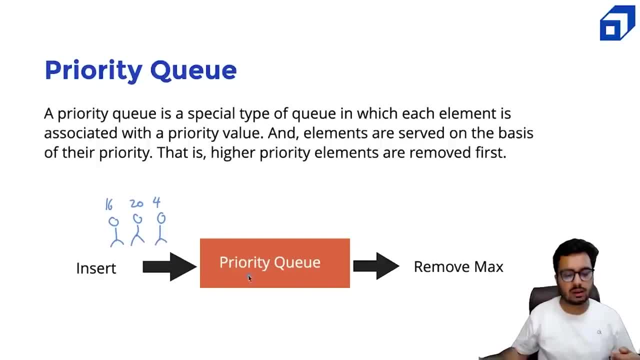 this is maybe uh, four years, this is 16 years, this is 20 years and this is maybe uh, four years. right now, if i say, okay, i want to remove someone, i'll remove the person. with the maximum i will remove person 20, right? so this will get removed so people can join the queue. but when i'm going 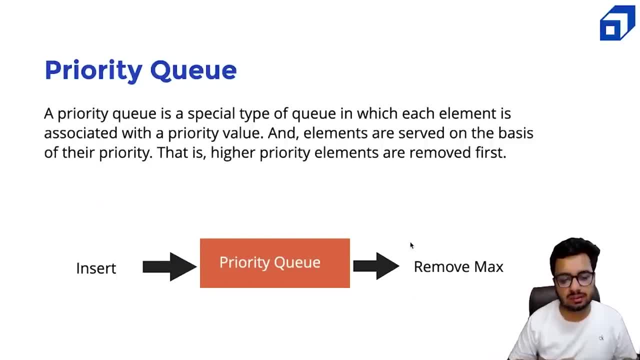 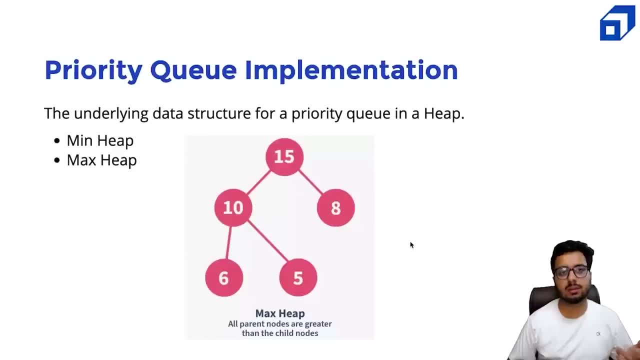 to remove people. the people with the higher priority will get third first, right. so the underlying data structure for a priority queue. it's a heap. we can have a mini for a maxi. i will not be able to dive into the details of heap at the moment. we'll be looking at how do we use the. 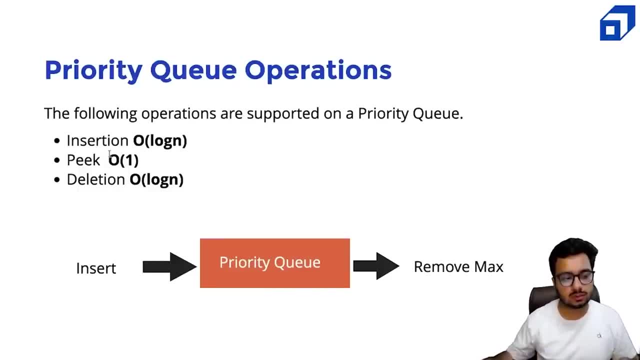 java priority, so the operations that are supported. we can insert something. inserting in a queue it's called as a offer. i can offer some data inside a queue. i can look at if i want to see who is standing at the front of the queue that is called as peak and if i want to perform deletion. i want to remove someone. 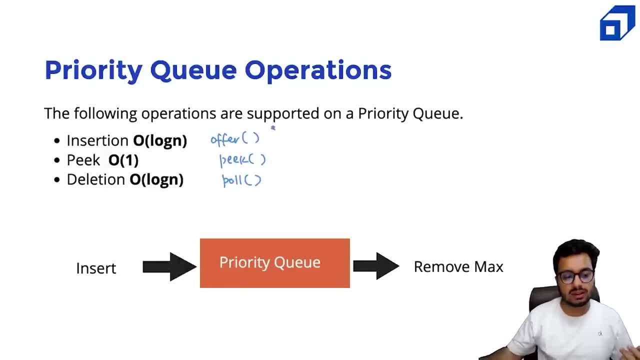 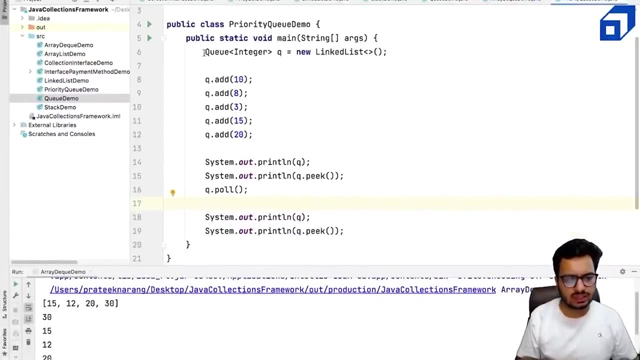 from the queue that that is called as poll. we'll be looking at these methods and insertion and deletion. they are login methods, looking who is at the front, the order, one method, right, so let us do a quick code code demo as well. so we have seen how to work with the queue. this is the code for a queue, a priority queue. 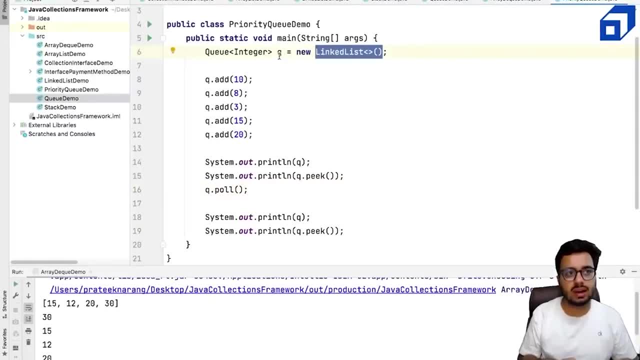 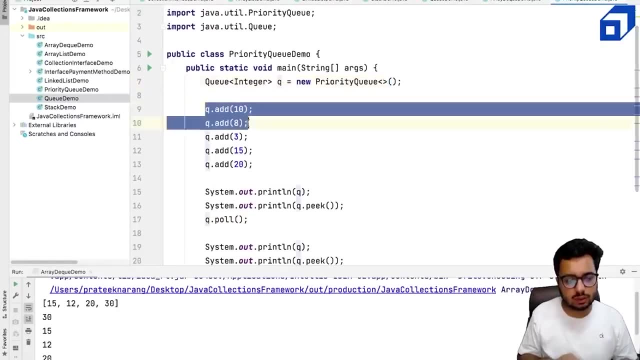 also is a class that implements the queue interface. okay, so right now it was a feed focus. now i'm going to change it to a priority queue, right, so rest, everything will change. if you want to add, add method will also work, but if you want to use the offer method, 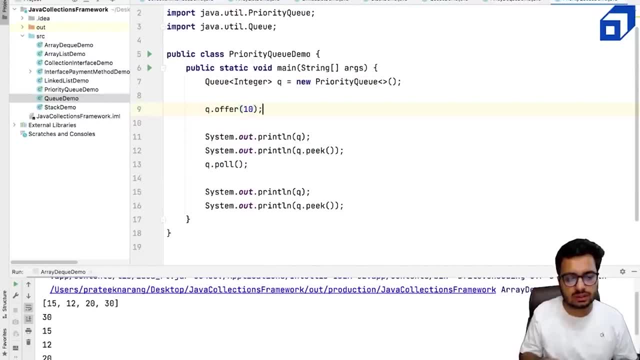 i can use offer method. i can do without offer some numbers. uh 10 will change the data later. i have 10, 0, 8, maybe 7 and let's say uh 9. right now, if i say okay, i want to print the entire queue. 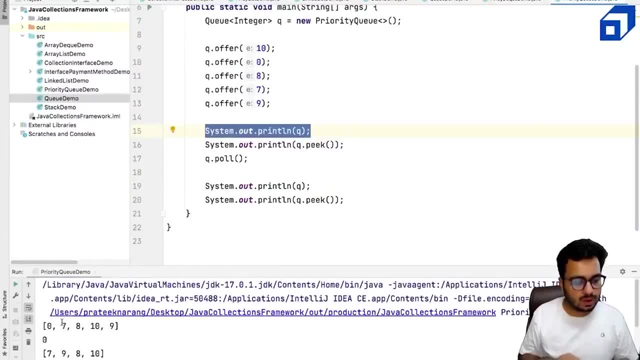 let's see what output do we really get. okay, so i'm getting this output: 0, 7, 8, 10 and 9.. i want to print the entire queue. let's see what output do we really get. okay, so i'm getting this output: 0, 7, 8, 10 and 9.. 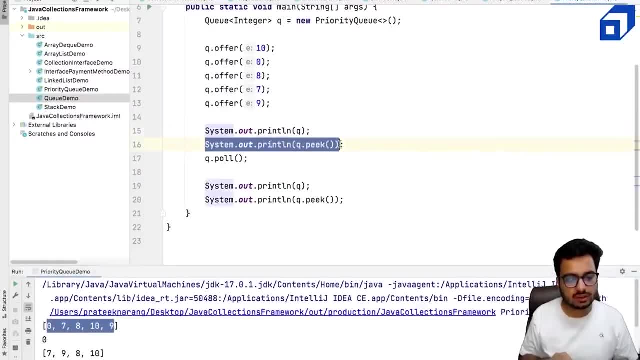 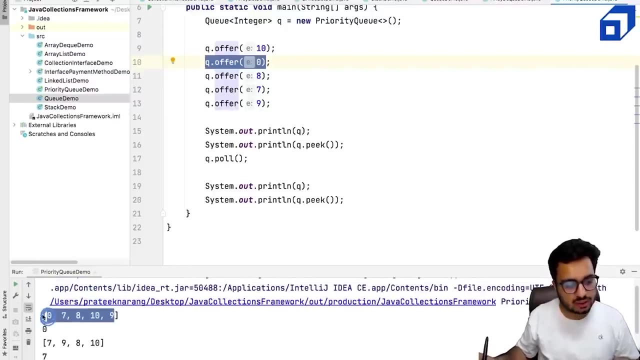 nine. i want to look at what is the first element. i'm in this case the lowest element. it's getting priority right. so you see, zero is coming at the front of the queue. rest of the queue is not actually sorted, only the priority element. it comes to the front of the queue right. 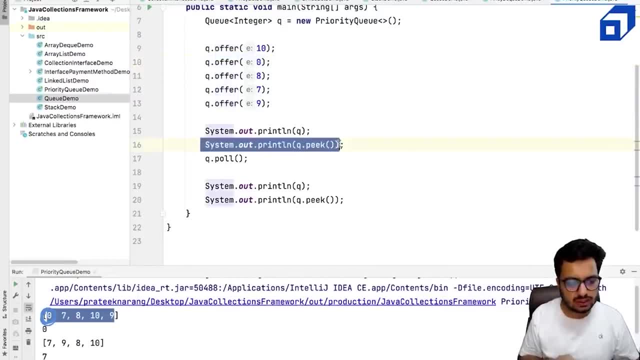 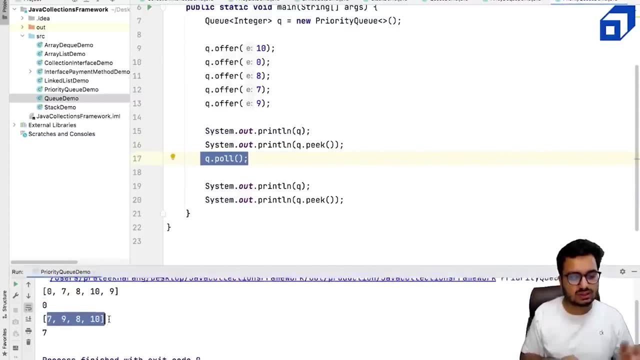 so zero is there. if i say, okay, i want to look at this element, so this element is zero and i want to remove this element, so it removes zero. and now what is the next lowest element in the queue? that is seven. so seven comes to the front of queue. if i make it 17, then the next lowest would be. 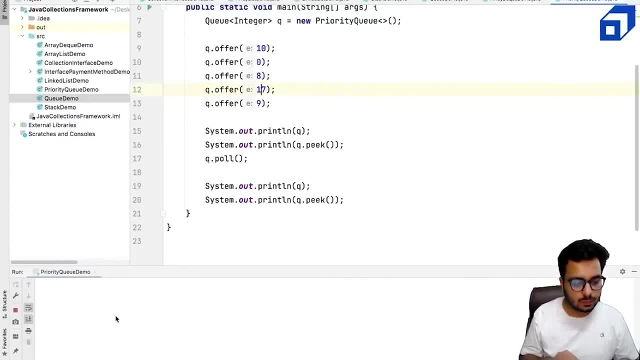 eight, right, so let's let me run it once again. now i have zero, nine, eight, seventeen and ten. the lowest element it is at the front right. then if i remove zero, the next lowest is actually eight, so that comes to the front. so if i remove that element, or if i look at what is the 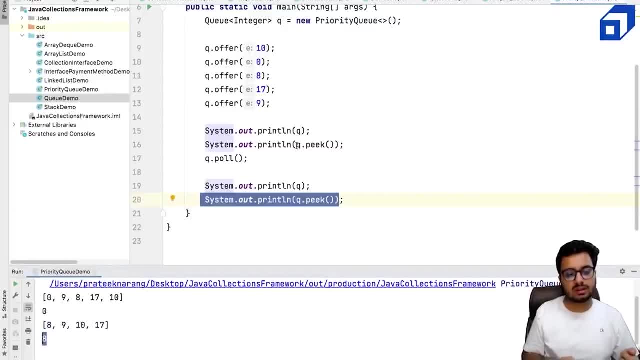 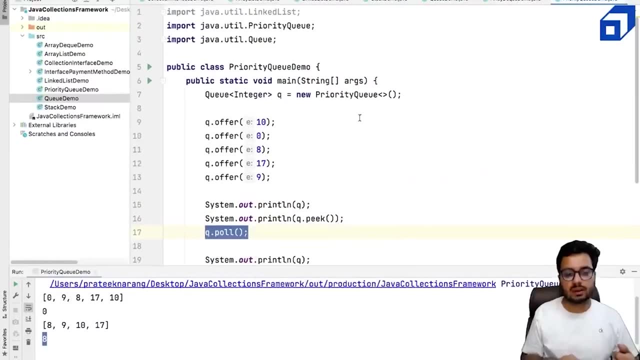 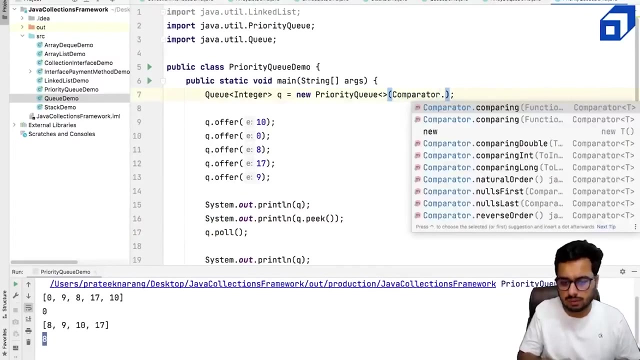 element. i get that element eight using the peak operation. you can see the element. using the pole operation you can remove the priority element. now you might ask if i want to reverse the order. okay, so in that case you can pass one more comparator. so i can say, okay, comparator dot reverse order. 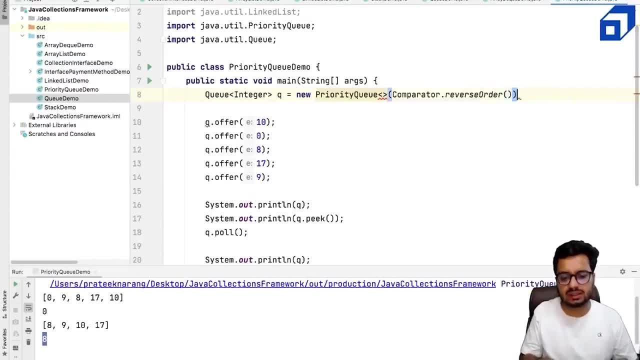 this is exactly going to reverse the comparison. a min priority queue becomes a max priority queue. in this case, the highest element, it's going to get a priority right. so now you look at, 17 is standing at the front. if we remove 17, 10 is standing at the front and there is no specific order for rest of the. 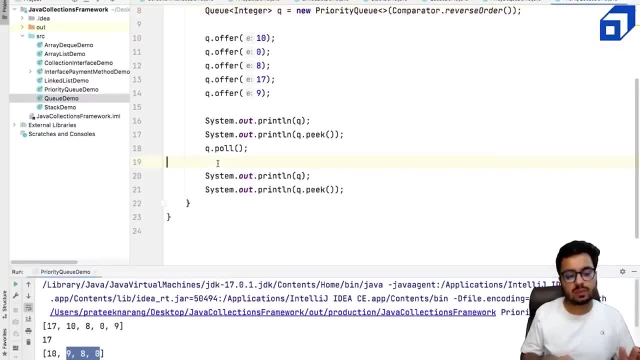 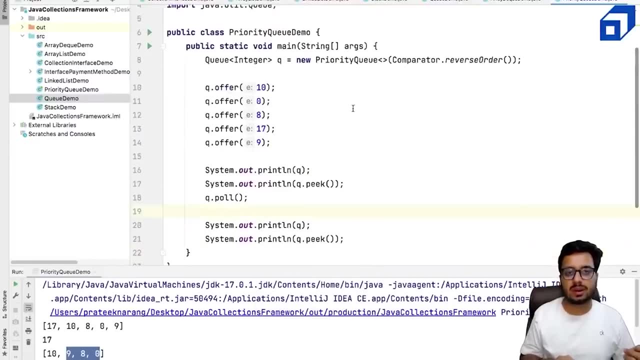 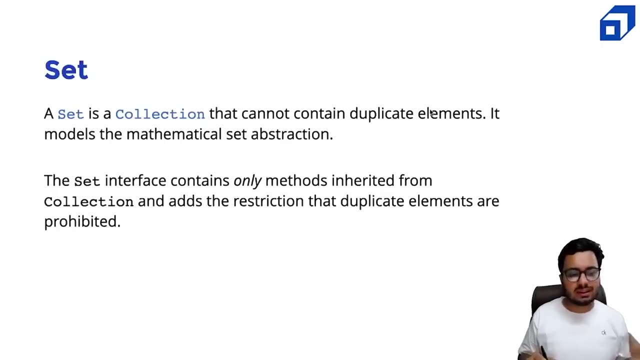 elements. that is unpredictable. we are only worried about the element at the front should be either the min element or the max element. this is about priority queue in java. let us talk about set interface now. so what is a set mathematically? it has a collection of. 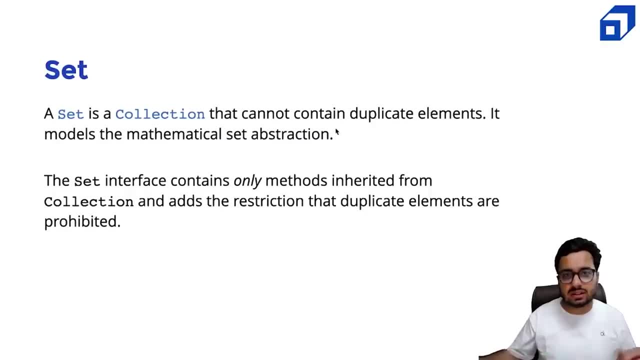 elements that cannot contain duplicate elements. okay, so set in java it models the mathematical set abstraction. now the set interface that we have seen. it contains only the methods inherited from the collection. that means there are no additional methods inside the set interface. all the methods are inherited from the collection. but it adds the restriction that the duplicate elements are. 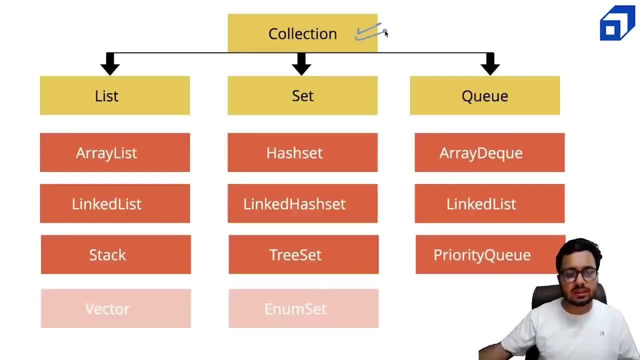 prohibited everything. all the methods which are there in collection right. the same methods are there in set, except the condition that duplicate elements cannot be pressed. there are three classes in java that provide the implementation of set. there is a has set. there is link set, linked hash set. 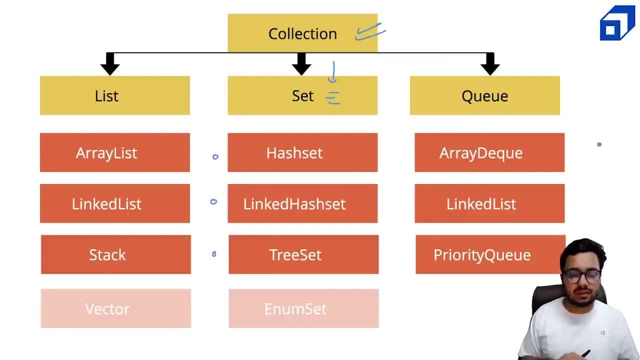 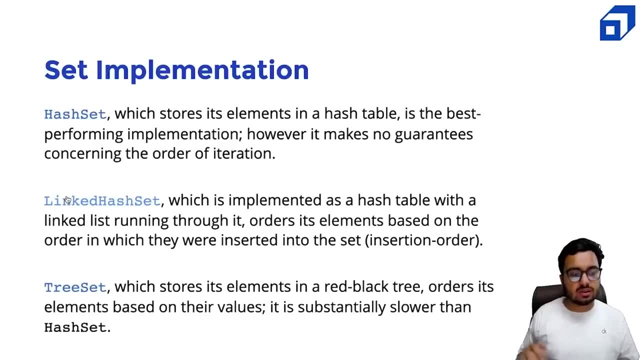 and there is preset. so let us try to understand the differences between the three implement. so, as i discussed, there is hash set, preset and linked asset. so hash set stores the elements inside a hash table. it is the best performing implementation. however, it makes no good performance. however, it makes no good performance. however, it makes no good performance. however, it makes no good. 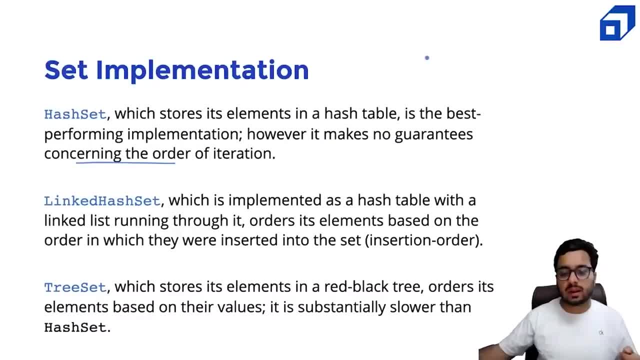 no guarantees regarding the order of iteration. you say, okay, i inserted 10, 20, 15, 18 inside the set and if you start, uh, iterating over the elements, you are not guaranteed to get any order. you might get 20, 18, 10 and 15.. so the elements will come out in any random order it so it does not ensure 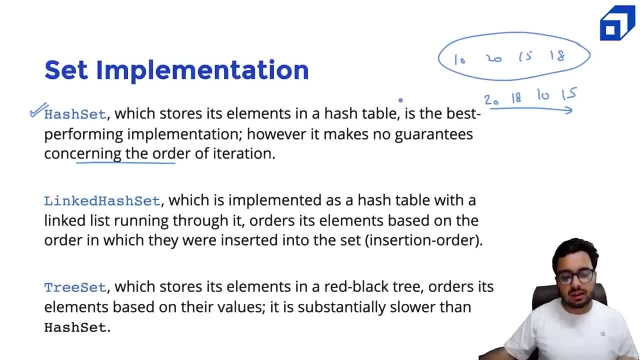 any kind of ordering on the high set. the internal data structure is a hash table. then there is a linked asset, so it is implemented again as a hash table and along with the hash table we maintain a linked list. so that means these elements are going inside the hash table, but also we 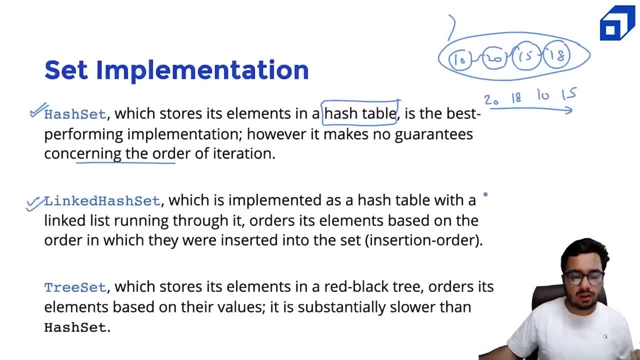 exchange them together so that we are able to maintain the order of insertion. so it has implemented a hash table with a linked list running through it. it combines the features of hash table and a linked list and orders its elements based upon the order in which they were inserted. so, basically, 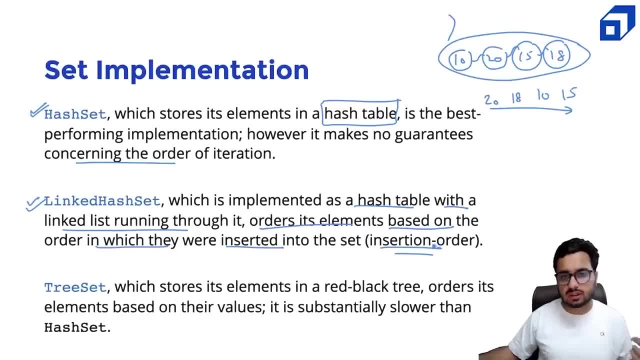 it maintains the insertion order. okay, so it's going to give you the features of the high set, along with the ordering that is maintained. there is one more thing that is called tree set. it stores the elements in a red black tree. so red black tree is a self balancing binary search tree. 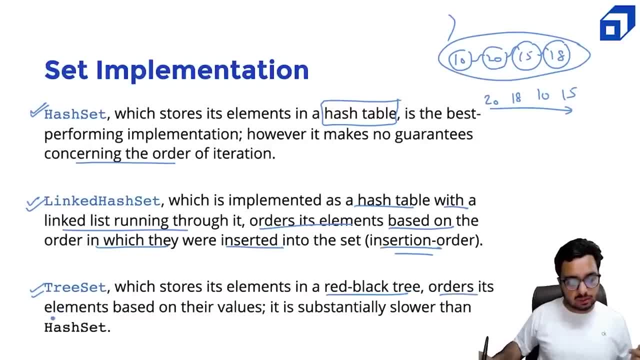 which is a height balanced tree and it orders its elements based upon their values and it is subsequently slower than the high set. basically, whenever we talk about bst, right and it is a height balance bst. so if you have to do an insertion, searching inside in such a tree where the tree height is log in, so it's going to. 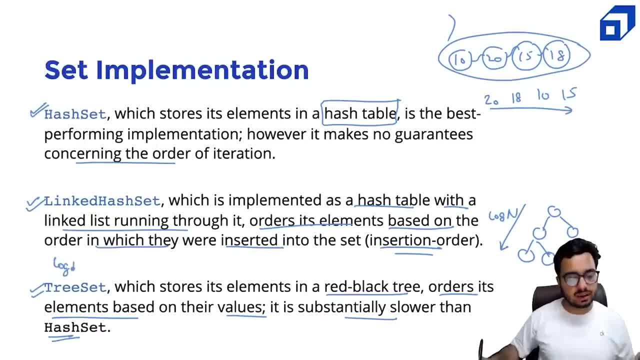 take all the methods like inserting data, finding data, they are going to take order of login time inside a preset, whereas on hash set and linked asset the time complexity is going to be order one on average right. basically, the advantage of tree set is it keeps your data sorted. 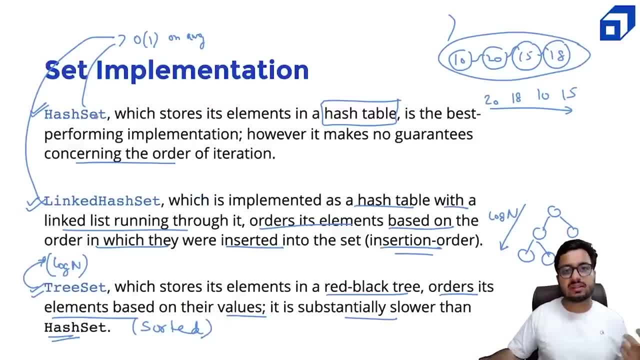 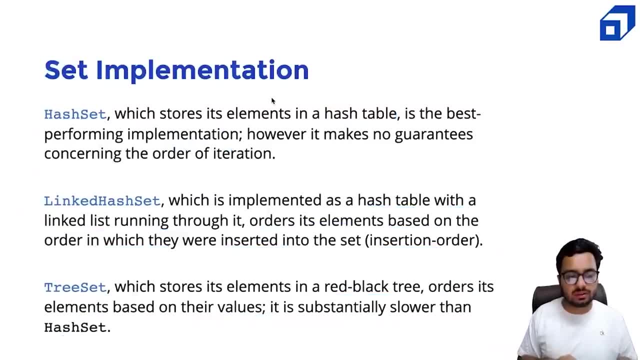 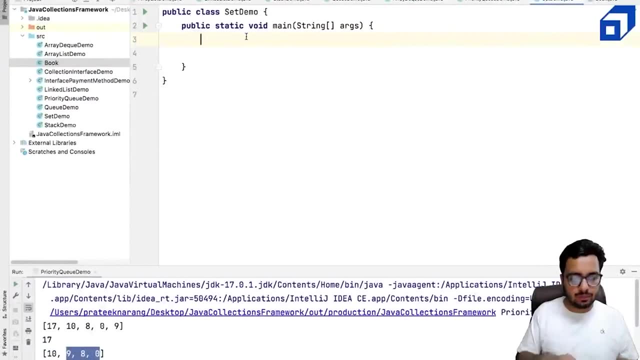 linked hash set keeps the same order as input asset. it is the fastest and it is the, but it does not give us any guarantees on the order. so these are three different implementations of set in java. let us look at the code demo for uh hash set. okay, if i want to create a set, that's a set of integers. 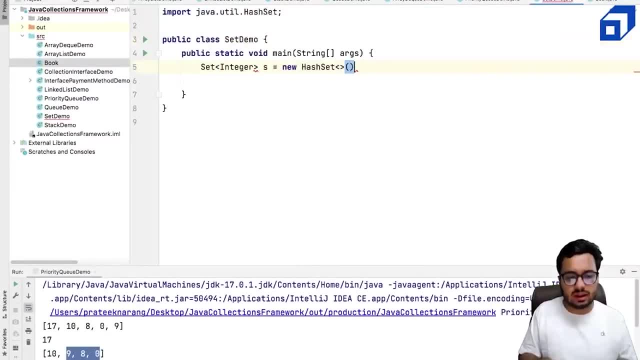 yes, this is equal to new hash set. right now i want to do something on this. let us import as well javautilset. import has been done. let us import some numbers into it. it's a set dot add- uh, sorry s dot add some numbers. let's say 10. 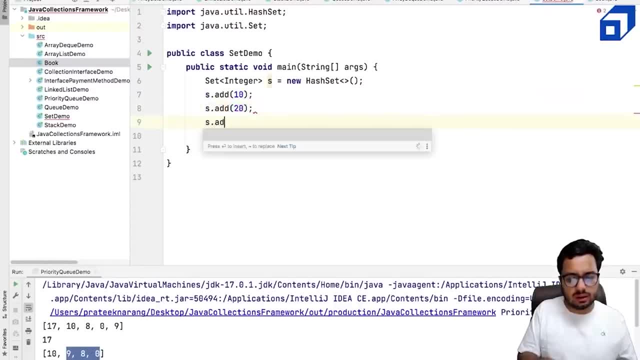 s dot add 20, s dot add 18 and s dot add, let's say, 15, right, and s dot add port. i've added few numbers, so let me display s s out the set. let us run this code and see what do we get. i'm getting 18, 20, 40, 10. 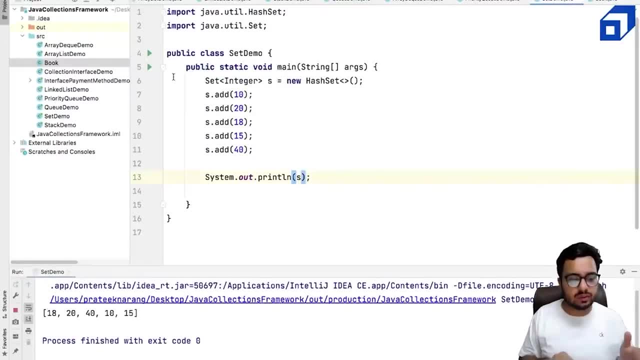 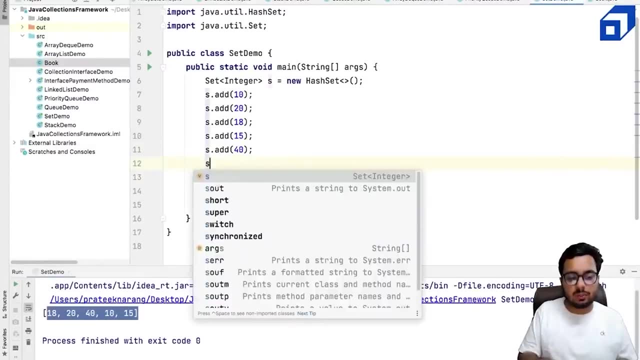 and 15.. you see, the order is random. there is no fixed order: 18, 20, 40, 10, 15.. it's, it's kind of a random order, right, if i want to add, like, if i add a duplicate element once again, if that's okay. 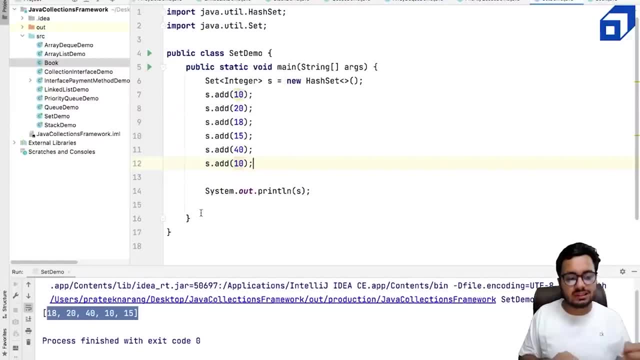 add 10 once again and if i run this code you will see this. it will not store the duplicate elements. only one, 10, is stored. even if i add it once again, the duplicates get filtered out. no duplicates are allowed in the set right. suppose i want to remove an element so i can say s. 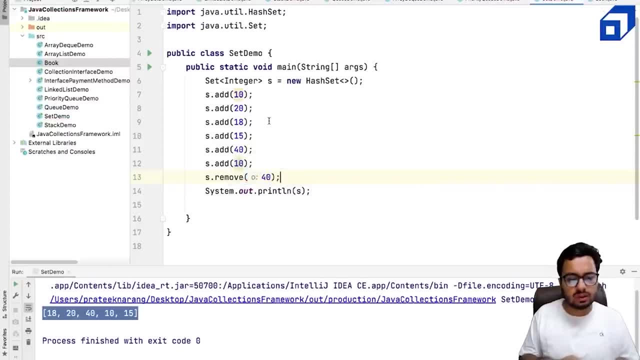 dot remove 40 it, this will remove 40 from the set. and, uh, what is not there, right? and suppose, if i want to check if a particular element is present or not, so if i can say, s dot contains, uh, some number 20, so you can say, yes, it is present. 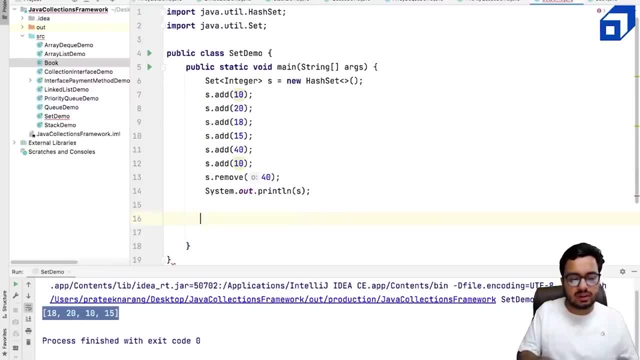 or i can simply say: uh, just do s out whether 20 is present or not, s out s dot contains. so it will give me true or false whether this element is present or not, so i will get a true here, right. so 20 is present. these are the three fundamental methods: add, remove and contains. and 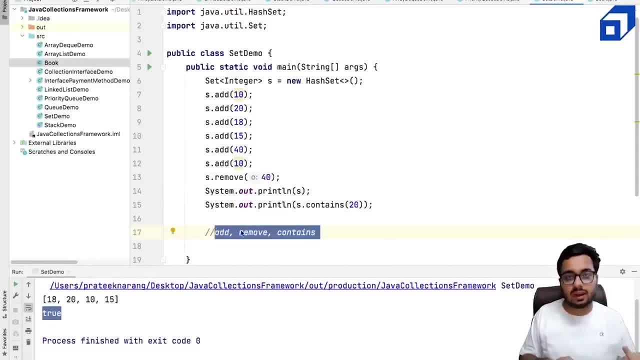 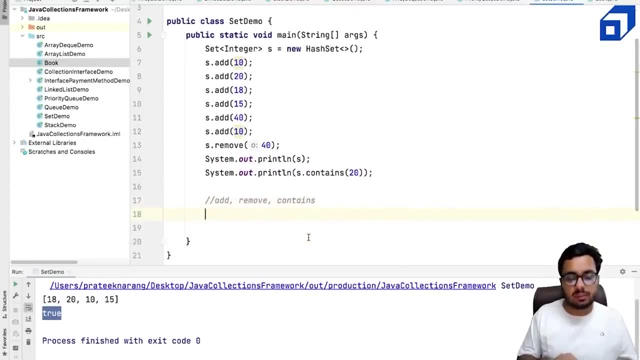 if you remember, these are the methods. they were part of collection interface as well. we can use these methods on any- uh, any data structure that we have seen so far. right, and all of them they inherit from the collection interface. uh, there are few more methods which we have with the collection interface. 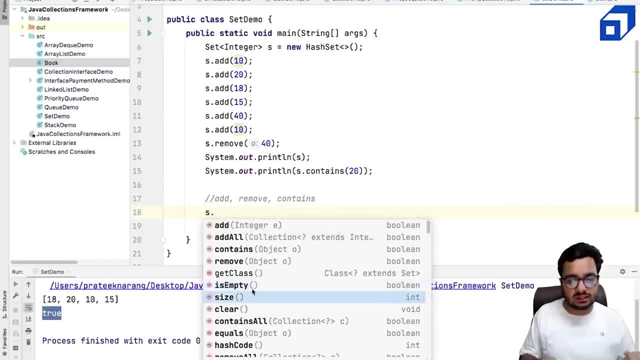 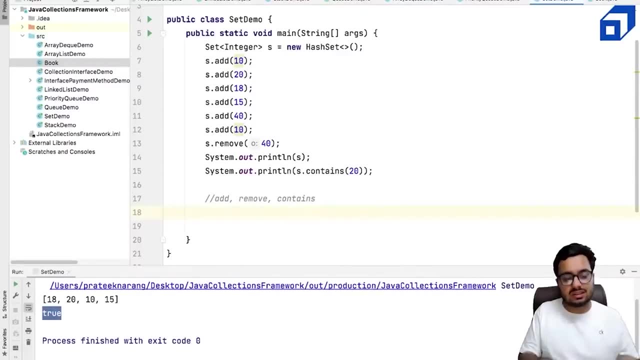 is empty. we can check size. how many elements are there in the set? clear, remove all elements from the set and we'll also see how do we use set with custom objects. so let me first first show you the size method. how many elements are there in this set? so currently we have four elements, so this: 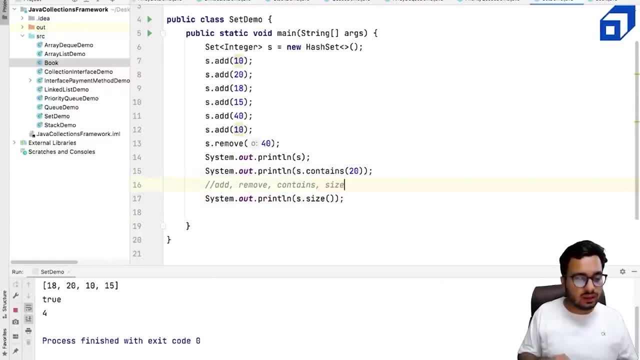 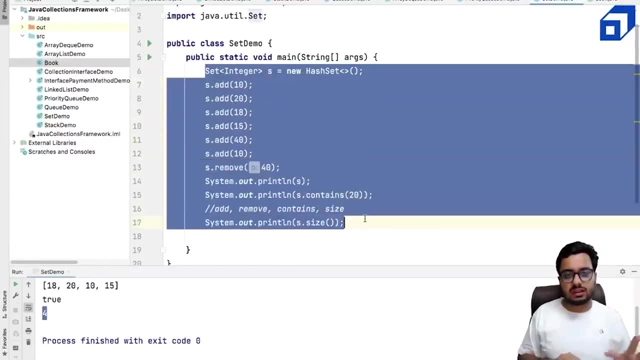 method will um tell me. okay, there are four methods. there are four elements inside it. now we have worked with a set of integers. now sometimes we might have to work with a set of a complex class, maybe a set of books, set of students, a set of- uh- payment ids or set of debit cards. right, anything, anything can come here. so 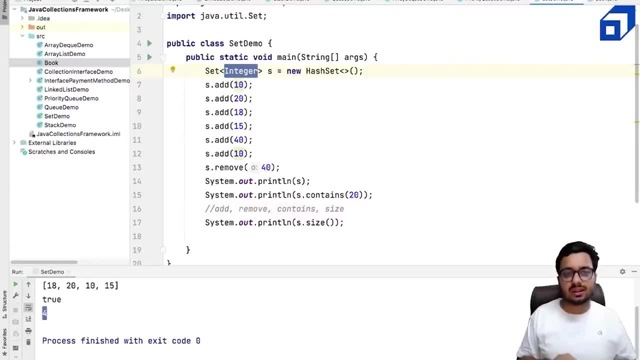 data type can be anything. so let us see how do we implement set with a custom data type and what will change. okay, before we uh, discuss the custom set, there is one more thing. so we just discussed that, okay, we can use a hash set class in java, but we can also use linked asset and we can also use 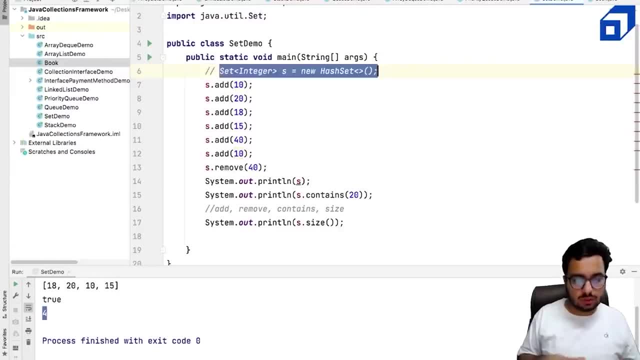 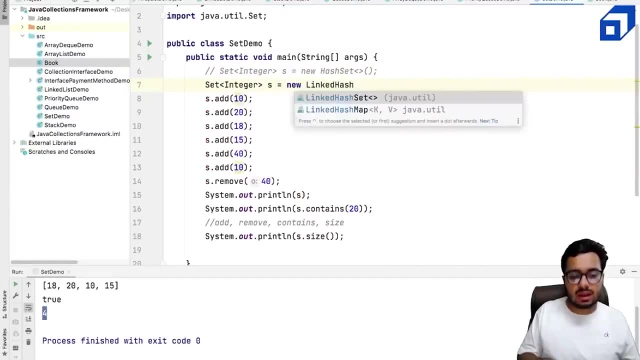 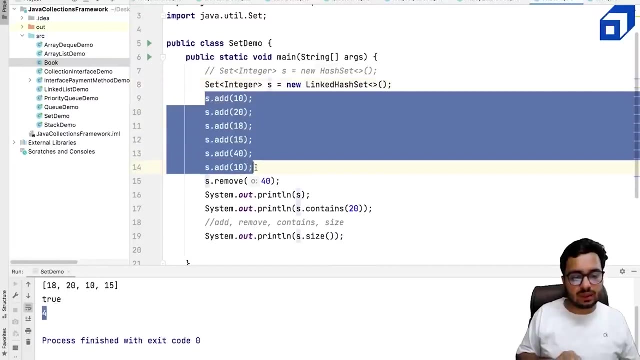 preset. so i'll comment this out and i'll show you two more examples. instead of creating a asset, i can create linked hash set in java and if i use this, you will see i will be able to maintain the same order as insertion in this set. if i remove 40, i will get 10, 20, 18 and 50.. 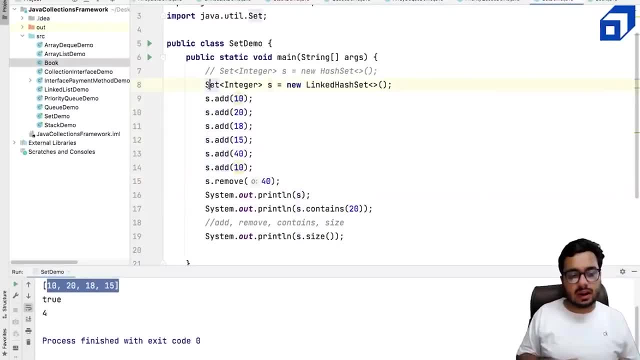 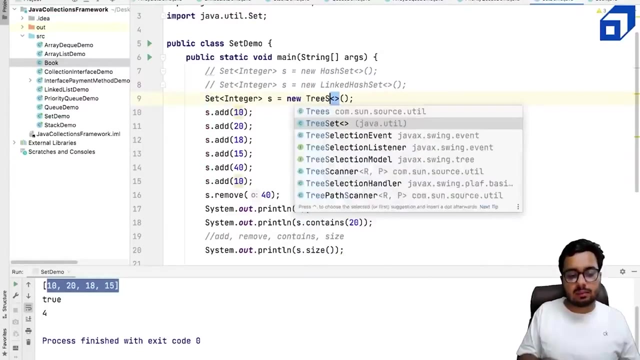 this, for this follows the order of insertion and if i use something like a tree set that is slower, uses uh self-balancing binary search trees doing add and remove. it's going to take login time on a tree set but it's going to maintain elements in a sorted order, so let's see that as well. 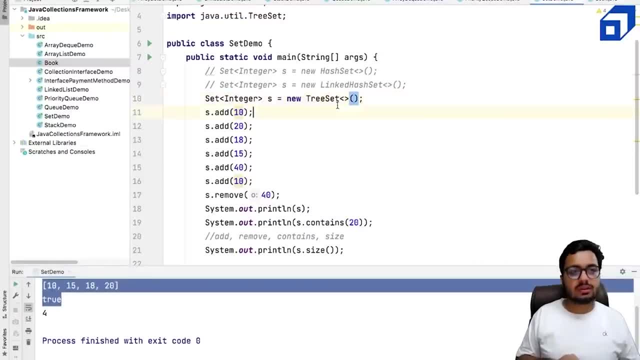 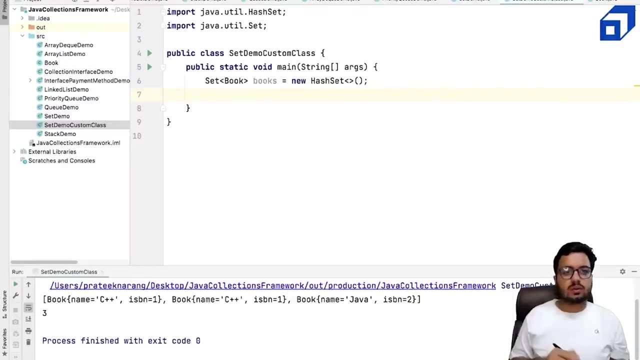 now the elements are sorted in the set because we are using a tree. so i hope you are able to understand the differences between has set, link set and tree set. now we will move into a set with the custom class set of custom objects. let's see that. now let us discuss how do we use set with a? 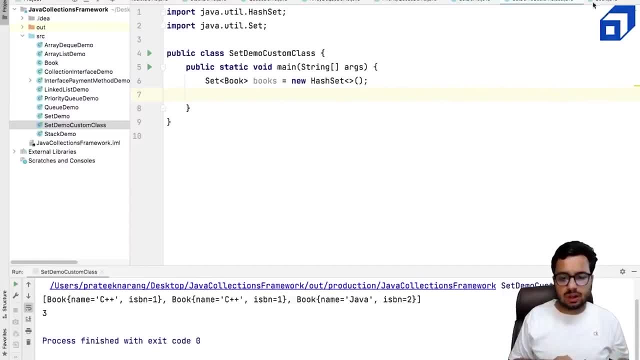 custom class. now suppose you want to create a set of books. what i have done: i have defined a book class in which book has three properties- isbn, name and price- as the attributes of a book. what i'm doing, i want to create a set in which every item is of the type book. now let us insert few. 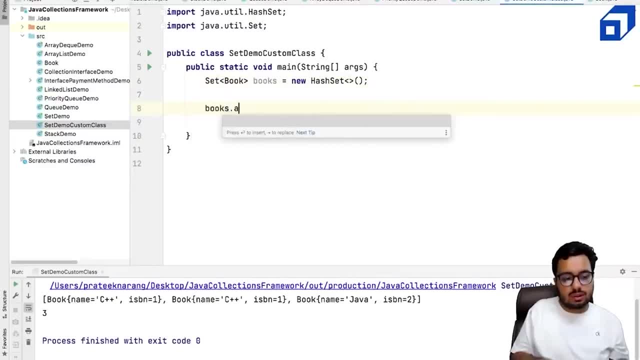 books into this hash set. i can say booksadd. let's say i want to create a new book. each book should have a name, isbin, which is a unique code, and let's say the price of the book, and let me say, okay, i'm going to add few more books. 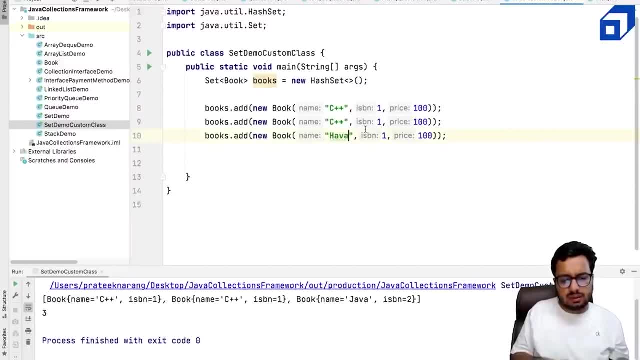 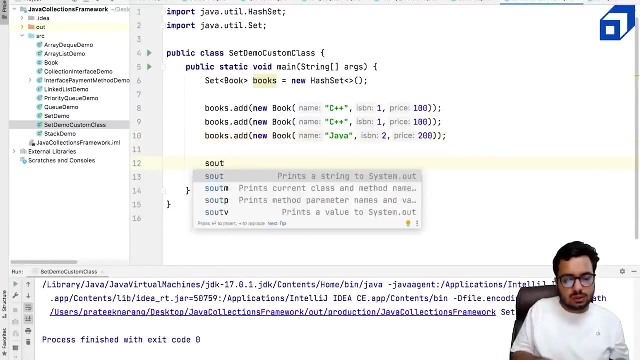 and here i make the name as, let's say, java isbin is two. and let's say i change the price right now if i let's say, go and run this code, let us see how many books we will have. so let's say s out books, dot size, and let's say s out books. i also want to see what are the books. 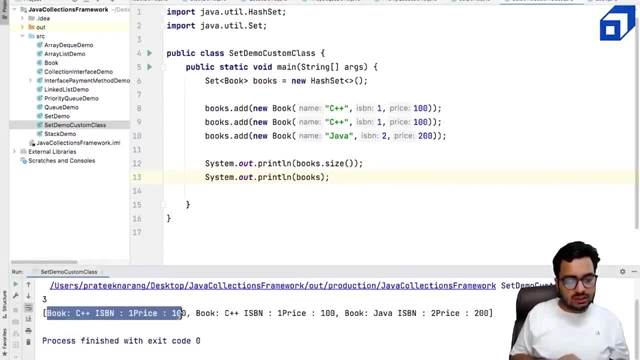 that the set is stored. so i'm storing three books and you can see c++ book is getting stored twice and java book is coming once. now why is this happening? why it is not able to filter out that these two books are really same. the reason is we are creating this object using new right, so for 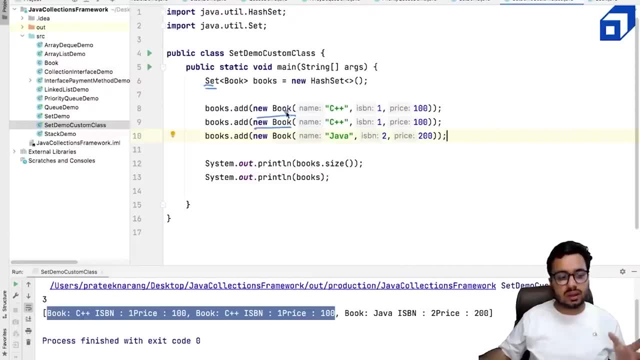 the set to know whether these two objects are same or no. there is no way right, so we are creating a new object that will treat that these. these are two different objects created at two different memory locations. maybe this is one zero five six, this two zero eight. 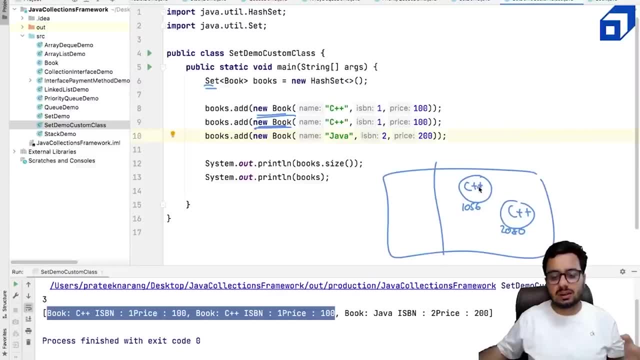 zero. so, for set, these two books are different because they are two different objects in the memory. right, we need a way to tell this set that, okay, you should consider these two objects as same. in order to do that, one thing we need to do is we need to define internally. it is using the concept. 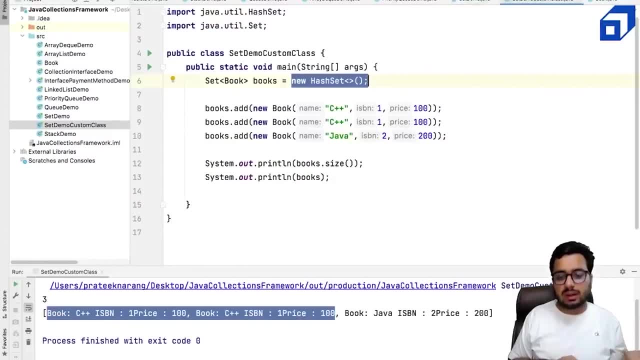 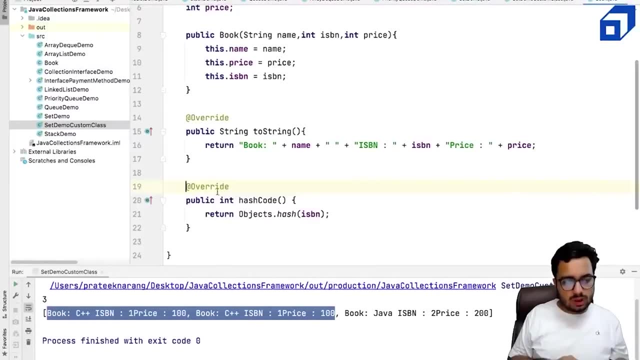 it's going to compute the hash code for an object. you have to tell me how do i compute the hash code. so for that, i need to uh overwrite a method which is called as a hash code. what i'm going to do, i'm going to overwrite a method called as a hash code. in this case, if i want to compute the hash code of 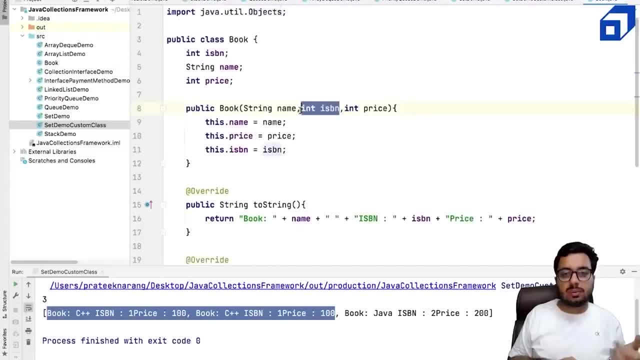 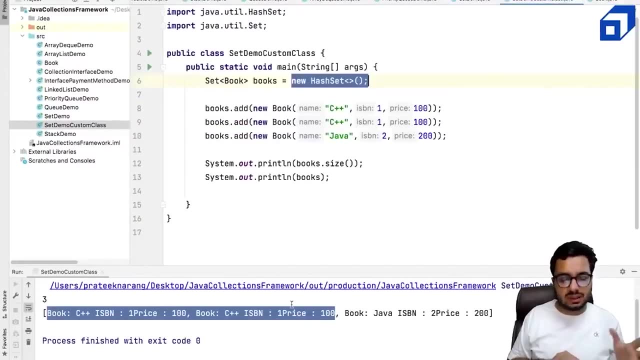 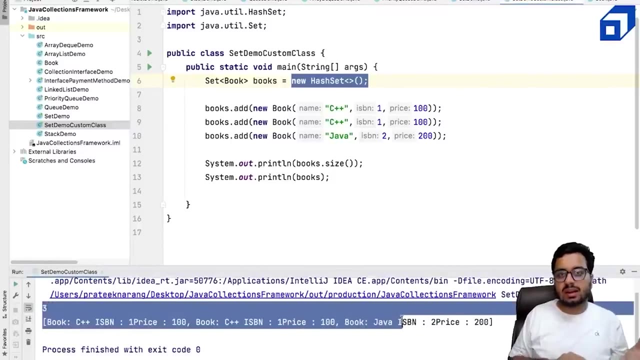 a book maybe i want to say okay, compute it only on the basis of: is been is been is a unique number. so let me do it once again now. let's see if something changes or not. it is not changing so when i'm hashing the books, although the books are getting hashed on the basis, 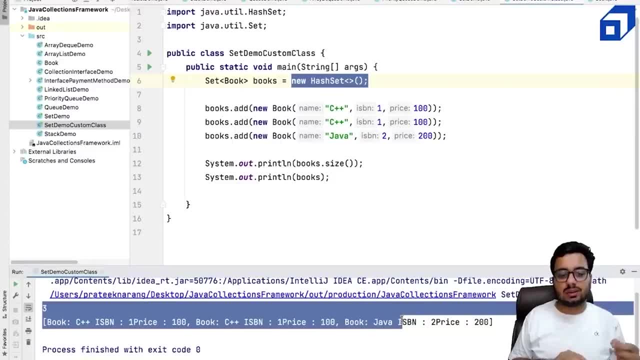 of isbn. still, the set does not know whether the two books are equal or not. so what happened? we, uh, computed the hash code for this book, inserted it into the set. this book went into the set. he again computed a hash code for this book. it also went into the set. two objects: they can. 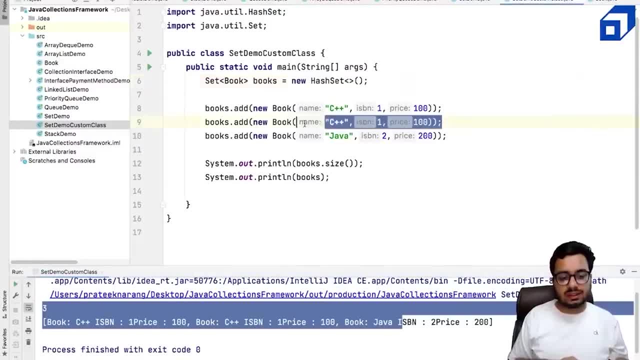 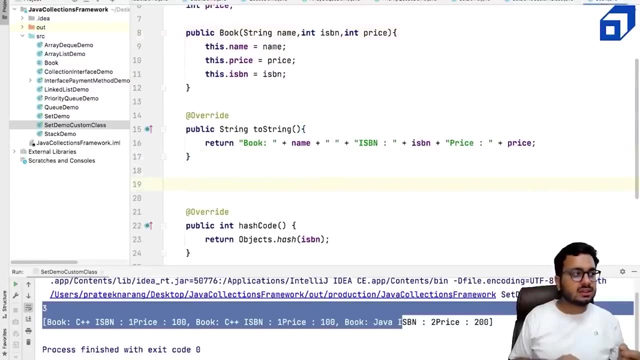 have the same hash code. that is okay, and uh, the thing is, i need a way to tell the set: consider: these two objects are equal. so maybe i want to say that, uh, so i need to uh provide a method that is called as equals method. okay, so let's see how do we write. 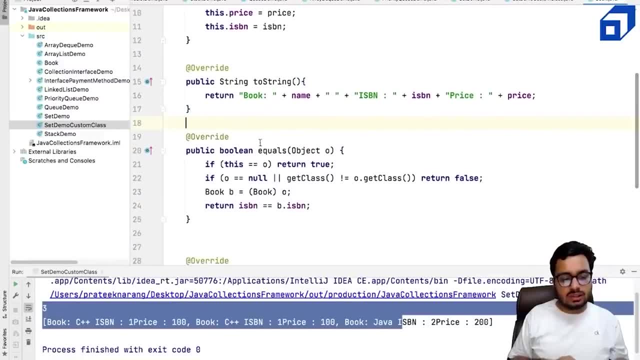 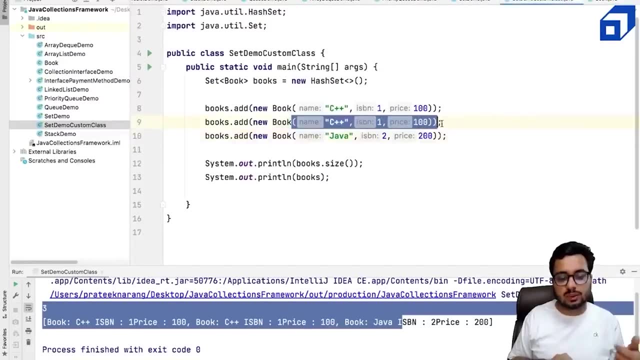 this method, so there is a pretty standard template to do it. so whether two objects are equal or not. so whenever you are inserting a new object- let's say you are inserting this object into your headset- it's going to compare that, whether such an object is present or not. so why, at what location? 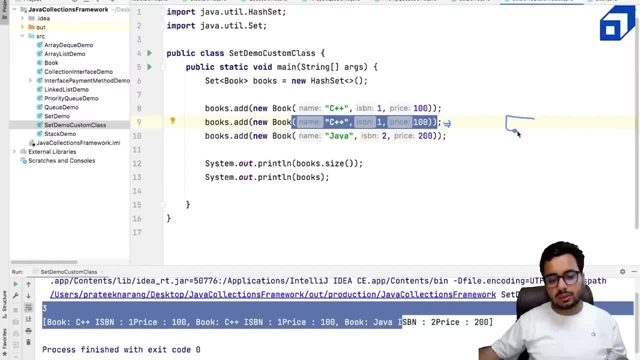 it's going to compare, it's going to compute the hash code and it's going to check whether we have uh something at that location or not. so suppose c plus plus was there some other book python was there? suppose they do to have the same hash code. so it's going to compare whether these two are. 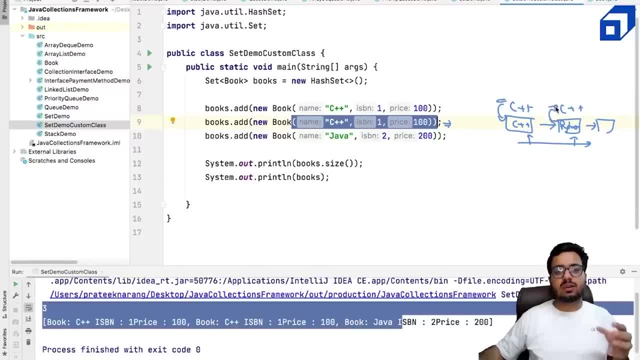 equal or not. whether these two are equal or not, this concept will be little more clear if you understand the technique of separate chaining right different objects. they can have a same hash code if they have the same is been, or the hash function is producing the same value for two different numbers as well. it can happen, right, but what we need to do is we. 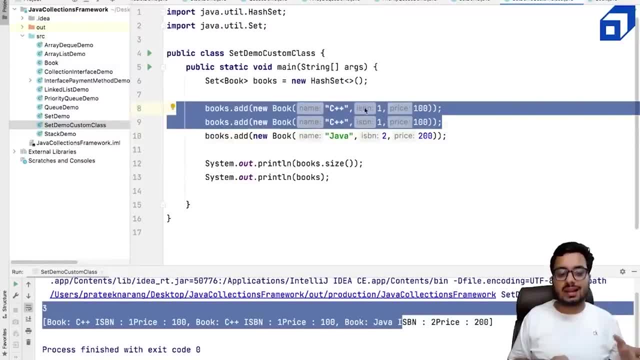 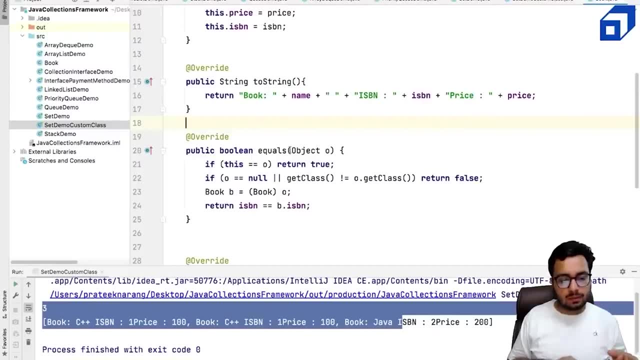 need to tell that, okay, the two objects are equal if their isbn is same. so what i will do is: uh, what i have done here is i'm saying that, okay, um, i'm giving you an object, so i say, okay, book b1, compare this object, equal to b2. there they do. these two objects are equal in like two, three. 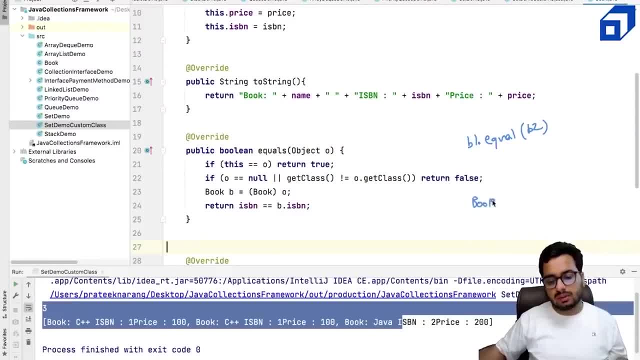 scenarios. i'll discuss what are those scenarios. suppose i create a book b1 which is equal to new book and i say, okay, b2 is a book which is equal to b1. so in this case what is happening? i have just one book object, both b1 and b2. they are pointing to same right if b i, if i make any. 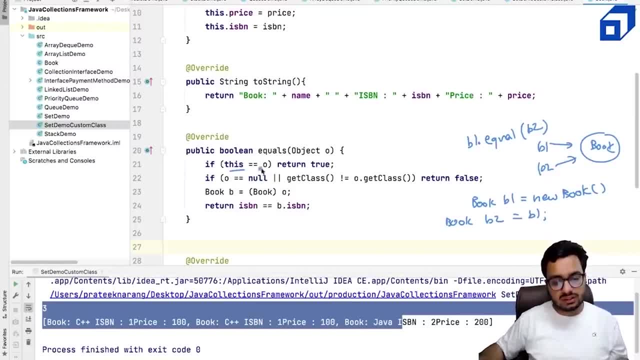 change in b1 it will also affect in b2. so what i'm doing? that if this is equal to o, that means if the current object and the other objects they are referring to the same book, b1 and b2- they are pointing to the same book, b1 and b2 they are pointing to. 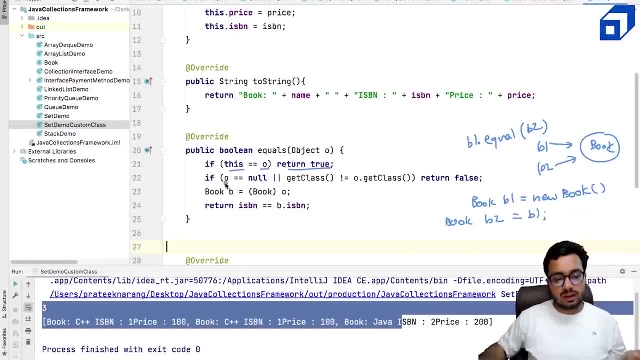 the same memory. that means they are equal right if o is null, if one of the object is null, they cannot be equal, or if the two objects they belong to the different class. so suppose if i compare a book with a student, they can never be equal. i am returning false, otherwise any given object. 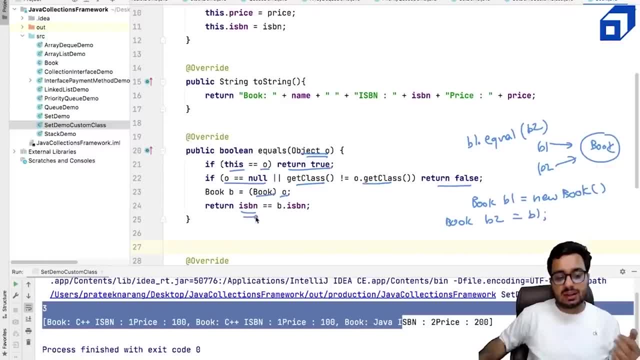 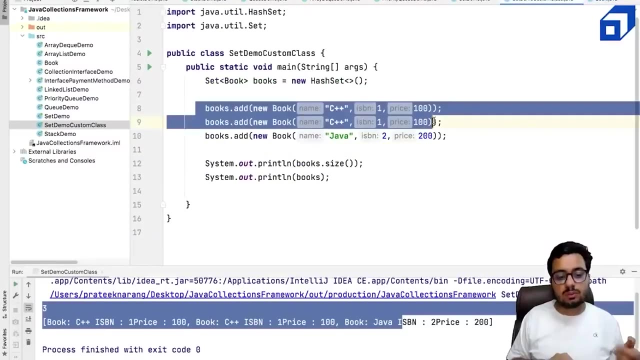 i typecast this into book loss and then i compare. that is, the is bin of my book is equal to the is bin of other book. if this is the case, consider the two book objects to be equal. if i have this equals method, my hash set will come to know that, okay, these two books. they have the same isbn. 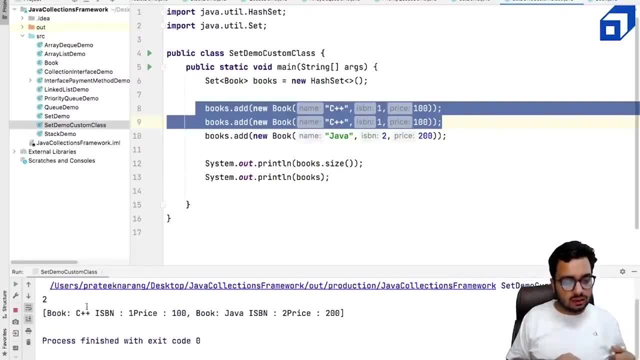 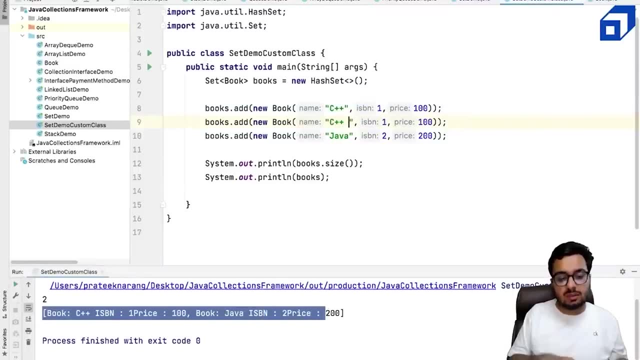 i will not insert them again, even if i now now look i have only two books, okay, and c plus plus is stored. only once now, even if i change the name of this book, i say, okay, this is c plus plus version two and the price has been increased to 120, will hash, let's store this book. 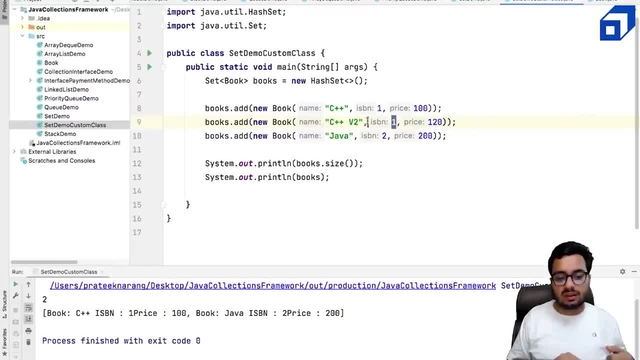 the answer is no, because it is only going to compare on the basis of isbn. if isbn is same, i will not again store this book, right. but if you want, okay, the two books are equal if their name is same, if their price is same, if their is been is same, then in the equals method. 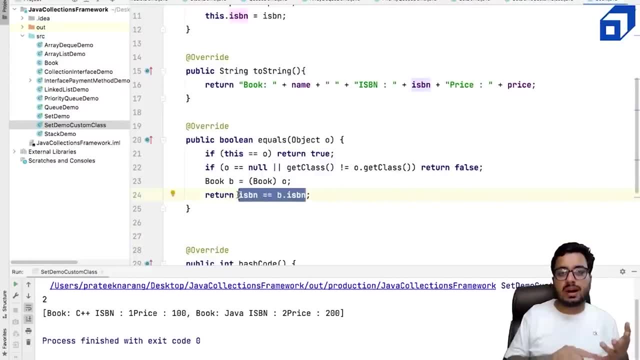 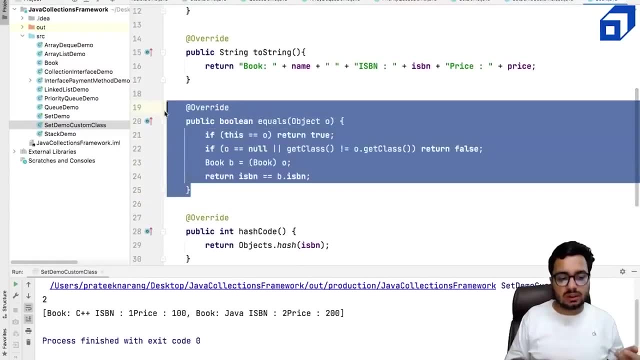 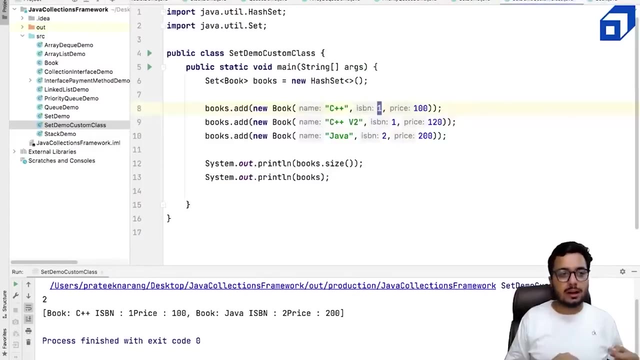 you can have two more conditions along with the is bin that i should match all the three parameters for the comparison. the equals method is important, so you need to override this method to tell the set in what scenario you should consider two objects as equal. i hope you are getting it and 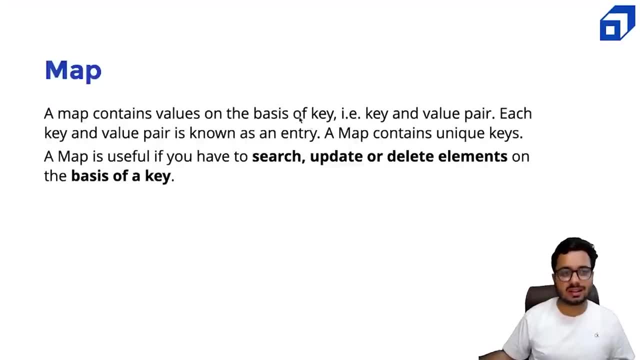 that's all for this implement. let us talk about the final data structure. that is a map. a map contains values on the basis of a key. that means it contains information in the form of key value pairs, just like a restaurant menu. whenever you go to a restaurant, you say, okay, i want to have a burger. 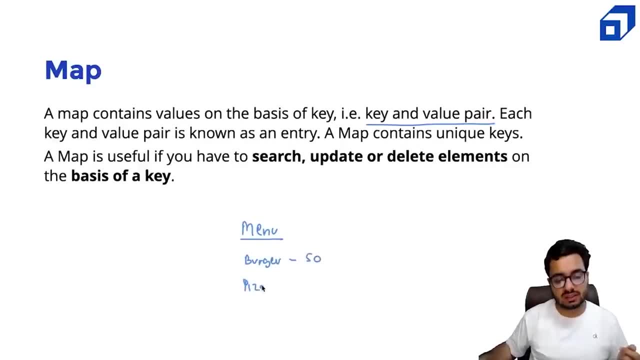 and you immediately get to know: the burger is 50.. i want to have a pizza. the pizza is 200. i want to have a coke. the coke is, let's say, 70.. there is a key, there is a value associated. a map contains. 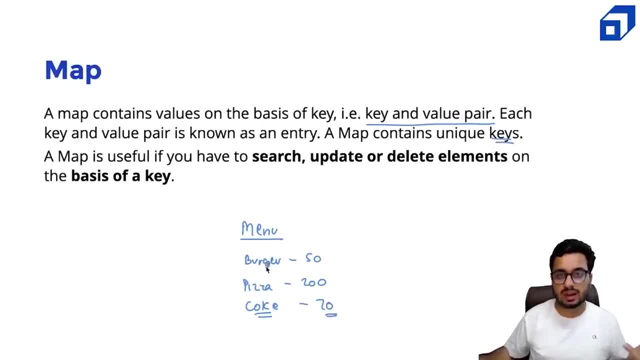 unique keys. that means i cannot have a burger twice in my menu. okay, a map is useful if you have to search, update or delete elements on the basis of key. so we do not ask: okay, what item is after burger or what item is coming before pizza. the ordering is not that important to us. what is important? that, given 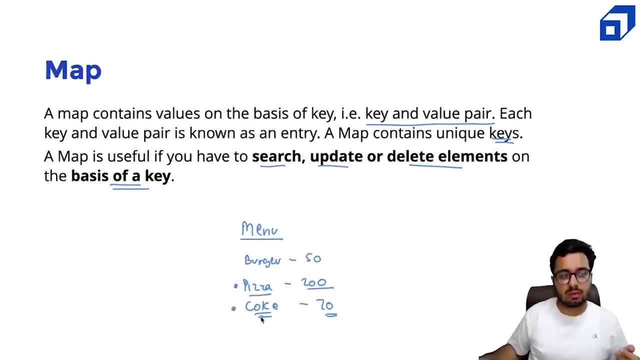 a key, what is the value associated with that item? and i want to. okay, coke is out of stock, so i want to delete this key value pair or something new has come up? i want to insert that key value pair so we can see that we have a map, and a map is a very good, useful, powerful data structure. and 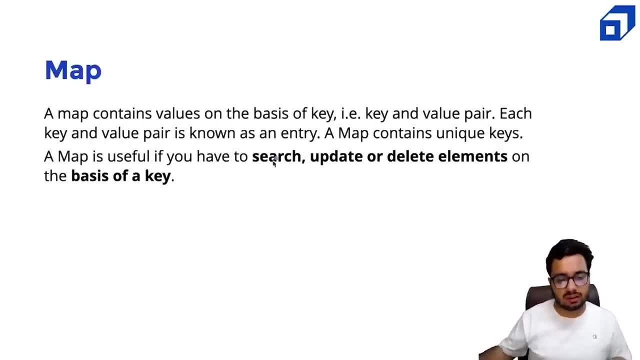 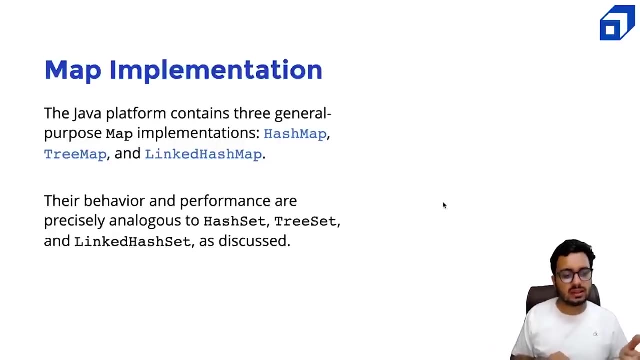 most of these operations they run in order one on average. so search is order one on average, update is order one on average, delete is order one on average. so very powerful data structure. now let us talk a bit more about map. java platform contains three general purpose implementations. 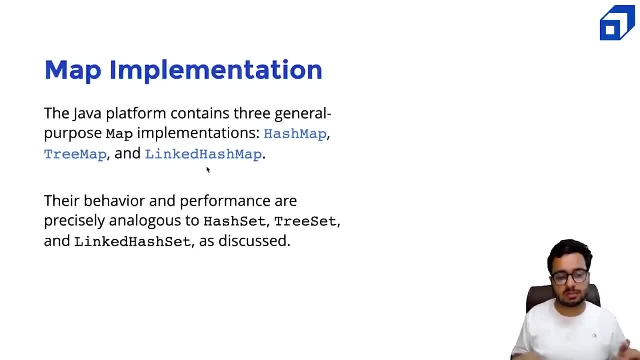 one is your harsh map, another is your tree map, another is your linked hash map. so the behavior and the performance is same as the way hash set, preset and linkset work right. so hash map internally uses a hash table. it's the technique called separate chaining that is used to implement a 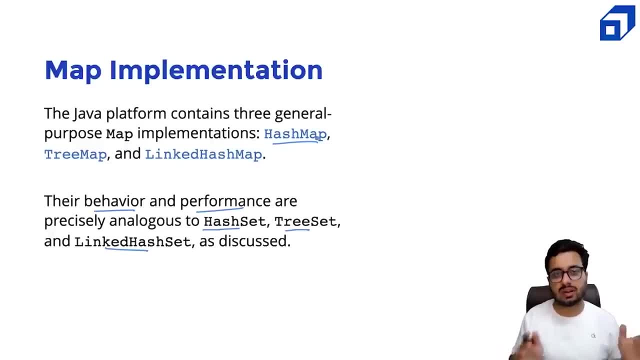 hash map. so to understand hash map, we'll do a separate video where we'll dive into the internals of a hash map. free map is like a self balancing binary search tree and linked hash map or hash table. sash table and linked hash map is your hash table and it also maintains a linked list of the hash table and is also maintains a linked list of her. 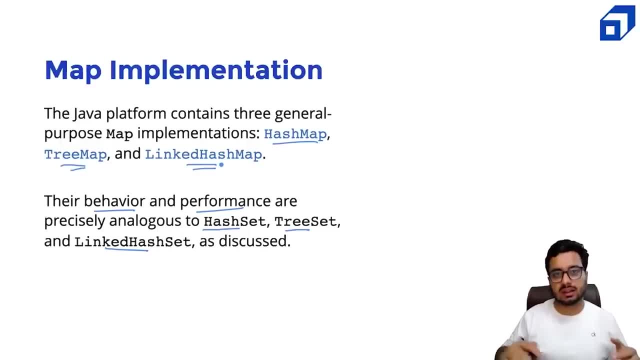 string and linked hash map is your hash table and it also maintains a linked list of the tree set of the three trees. the tree layer belongs to the tree and then sits in the array and, if that case, also nós, And it also maintains a linked list of the elements in which, like, it changes the elements. 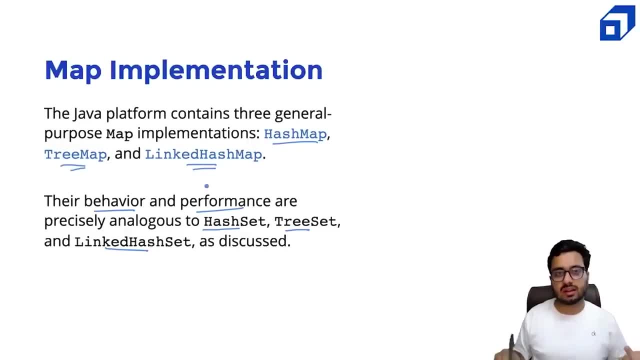 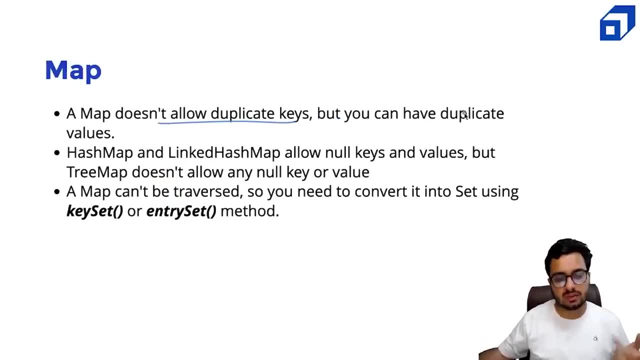 through the linked list as well, in the order in which they were inserted. It's more complex than a hash map. Map does not allow duplicate keys, Just like a hash set. we do not have duplicate elements, but we can have duplicate values. 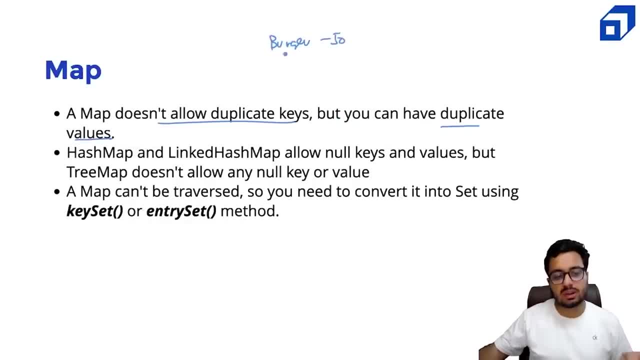 For example, burger can cost 50, noodles can also cost 50. The value can be duplicated, but the key must be different, right? So hash map and linked hash map. they allow null keys and values, but tree map does not. 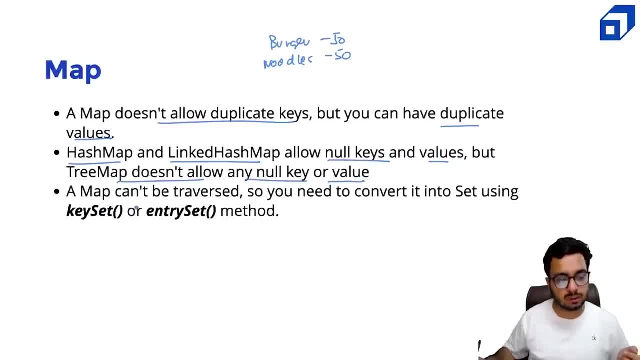 allow null key or a value right Tree map. you cannot store a null key. A map cannot be traversed so you cannot directly iterate on the map. So you need to convert it into set using key set or entry. This we will look into the code demo. 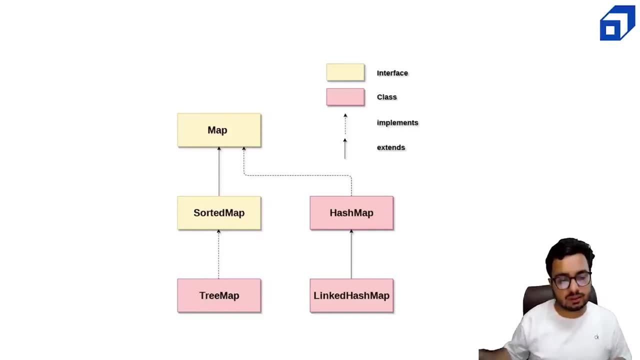 Talking a bit more about the hierarchy in Java, there is a map interface- okay, And hash map is an implementation for the map interface. There is a linked hash map which builds on the top of your hash map class right. Hash map is a class. 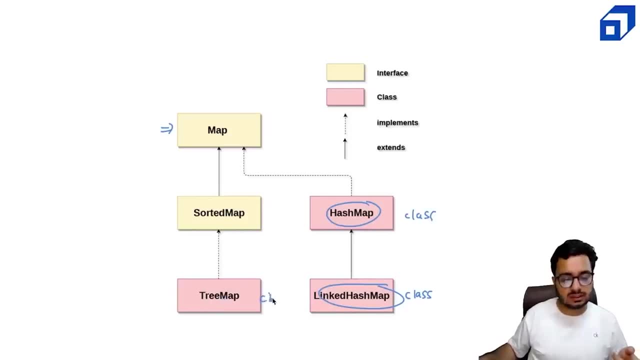 Linked. hash map is also a class. Tree map is a class that implements your sorted map interface. Sorted map interface is again a child interface of map, right? It kind of extends that map. Here. ordering is important, right. You get the keys in a sorted order. 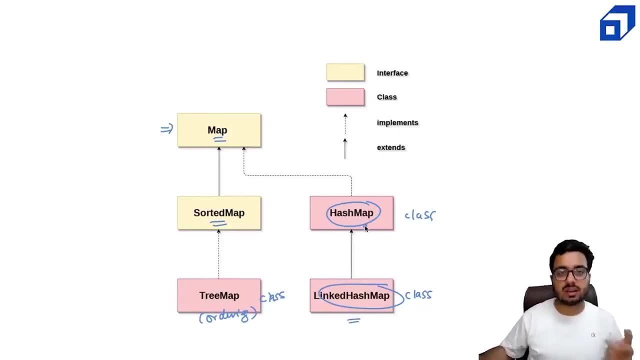 Here you get keys in the order in which they were inserted And hash map. it is the. Here you don't get any ordering on the key. This is the difference between the implementation. Also, the operations are order 1 here on average. 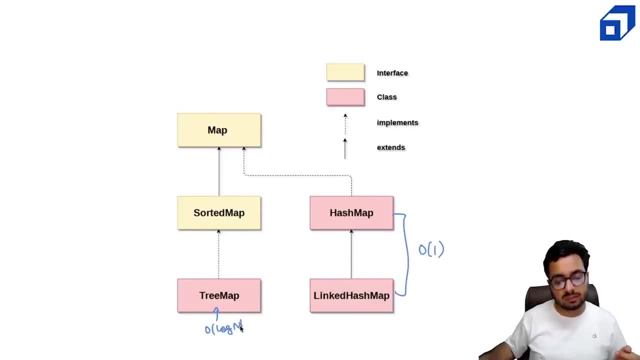 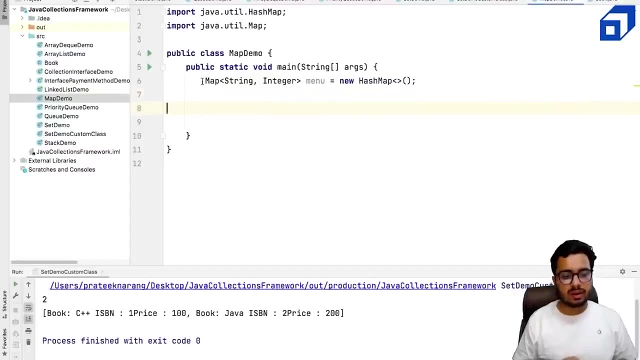 Operations on tree map. they are order of log n on average. Why? Because it is using a self-balancing binary search tree. okay, So here I have implemented a map object by using the hash map class, right? So I've created a map called as menu and I'm going to add certain items in. 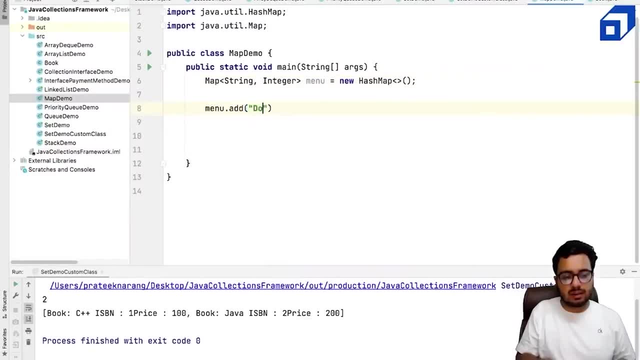 So I can say: menuadd, Let's say the item is dosa and the price is 200.. Menuadd, Let's say the item is burger, The price is 50.. We are getting an error here, So the method is called as put. 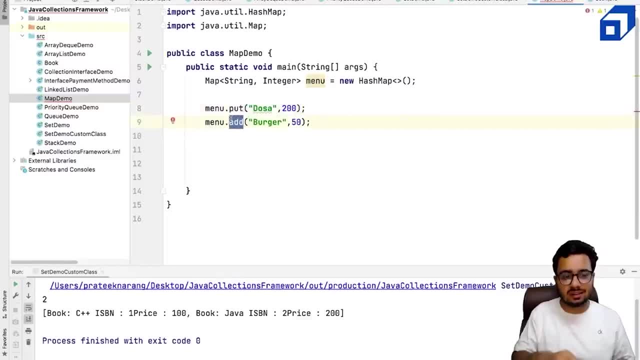 Hash map. we don't have the add method because it does not inherit the collection interface. okay, I told you, map is separate from Map. interface is not a child interface of collections interface. Okay, So it has method. It does not have a method called put. 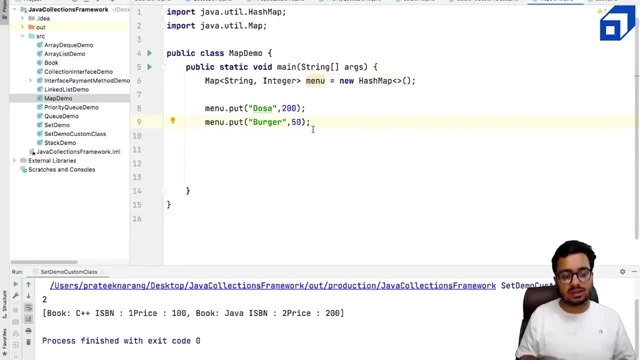 It does not have a method called add. I can put key value pairs like this. I can say menuput Noodles and maybe some price. And here I can say, sout, Show me the menu, Let's see if we get something here. 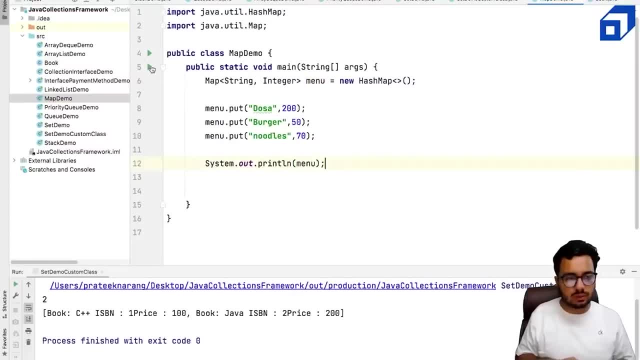 So let's see what do we get if I run this code. In the meanwhile I will write down some more methods. I can see there are. I can see the list of key value pairs That are stored inside this map. I can also remove something. 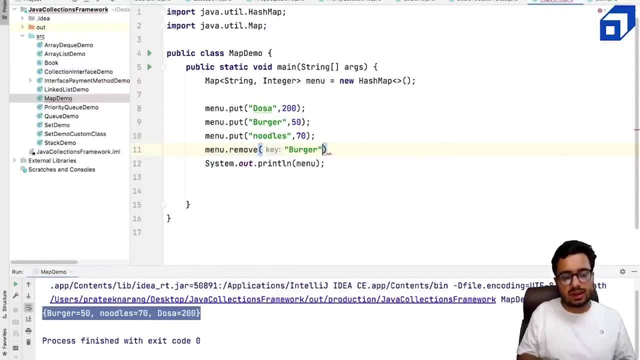 I can say menuremove. I give burger, I just need to give the key. Burger will get removed from the map. I can also search that if my menu contains some item like dosa, I can say contains key. This is the method. 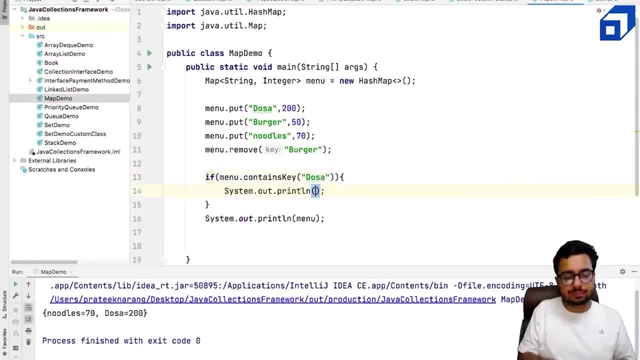 And I can check whether it is present, So you can say yes, Sout dosa found, So you can do this as well. Burger: After removing burger, we have two items- noodles and dosa- in our map, So dosa is there. 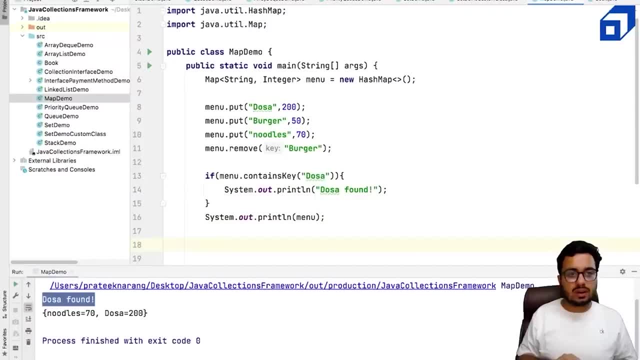 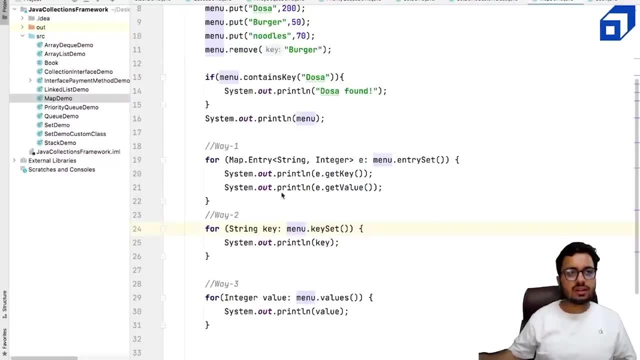 So dosa found It gets printed. Now let us also talk about how we can iterate on the map. There are multiple ways, So what we can do is: Okay, I just written the three ways to iterate so that we can save some time. 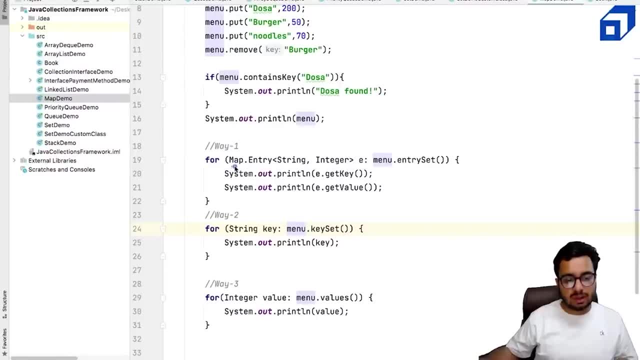 So the way one is, I can create an object of the type mapentry And this object is iterating over all, So menuentry. So menuentryset is a method that gives me the list of key-value pairs, where each key-value pair is considered as an entry right. 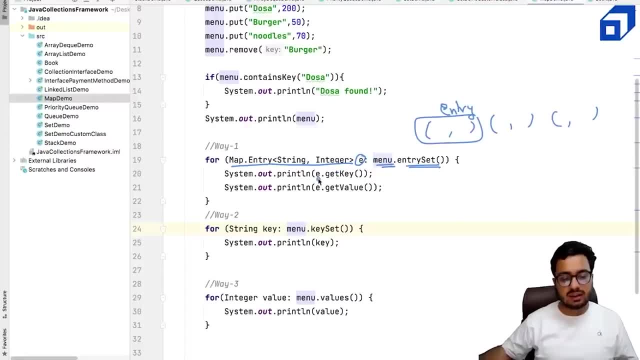 I am saying, okay, give me all the entries and given any entry, I want to get the key and I want to get the value. So that is one way. So you are printing the first entry, the second entry and then the third entry. 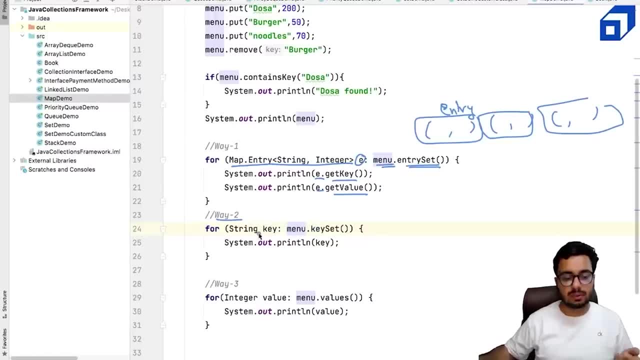 That is one way. Another way is, if you want to just get the keys of the map, you can say menukeyset, So it will give me all the keys, like dosa, burger noodles and you are iterating over these keys. 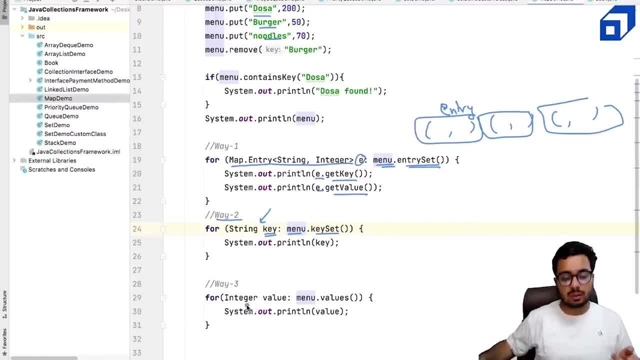 Those keys will give me all the keys, like dosa, burger noodles, and you are iterating over these keys. These are strings. Then you can say: okay, I want to iterate over the values that are 250, 70.. 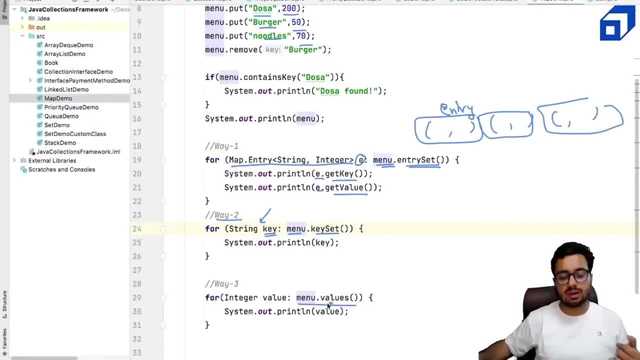 I just want to iterate over these values. So you can call the method called menuvalues and it will give you a set of values and you can iterate over this set using a for each loop And for every value you can print. I will just run this code and show you the output. 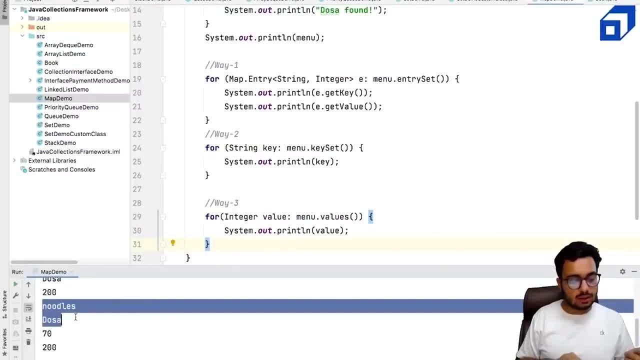 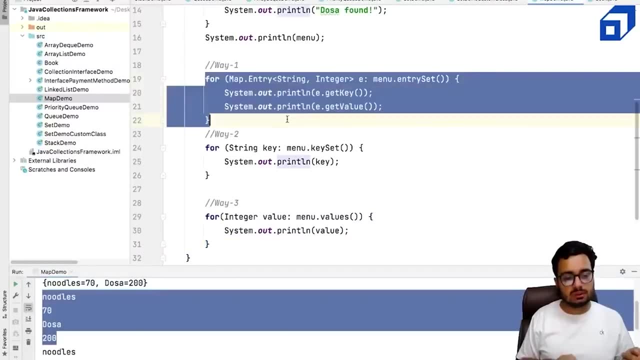 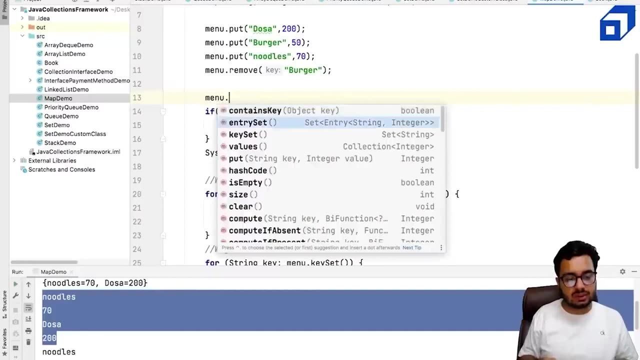 You can see, I am able to iterate over the keys, I am able to iterate over the values and I am also able to iterate over key value pairs. right, so this is coming from this loop and apart from it there are some more functions which can come handy. so you can, i would suggest and try those methods is empty, whether the 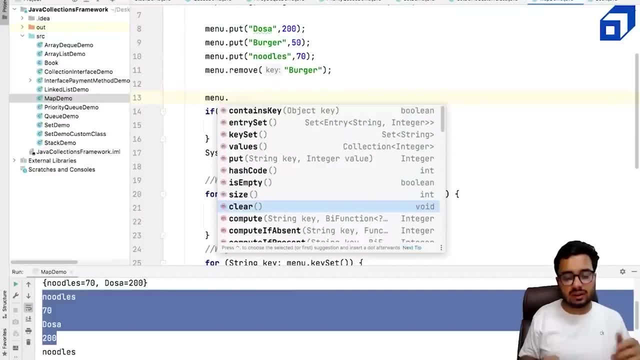 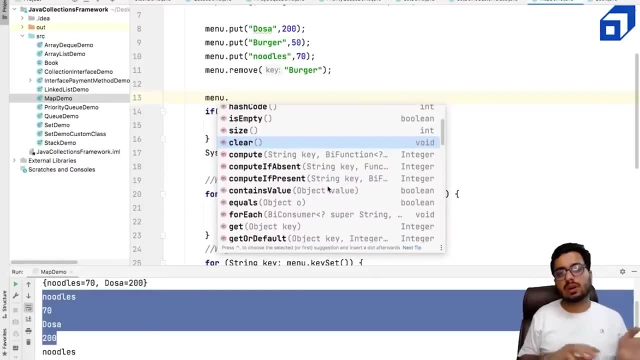 map is empty or not. size how many elements we have here. clear out everything in the map, right, this is clear. method is helpful if you are working with multiple test cases. every time you have to load new items and discard the previous items from the hash maps instead of destroying the object and 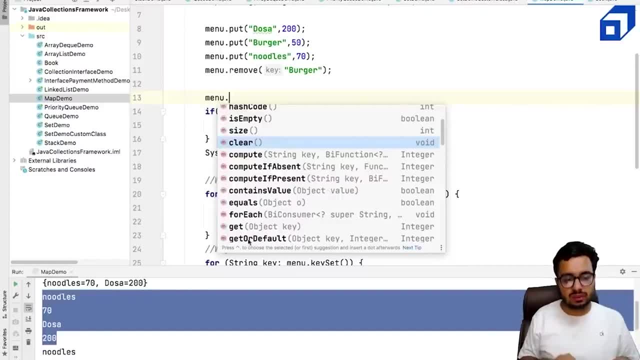 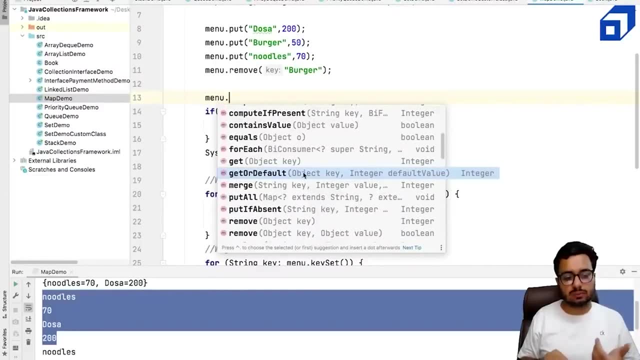 creating a new object, it's better to clear out everything from the previous map. so then there is: get our default. if the key is found, you want to return some value, you want to return the value, or if the key is not present, you want to return some default value. this is something you can use. 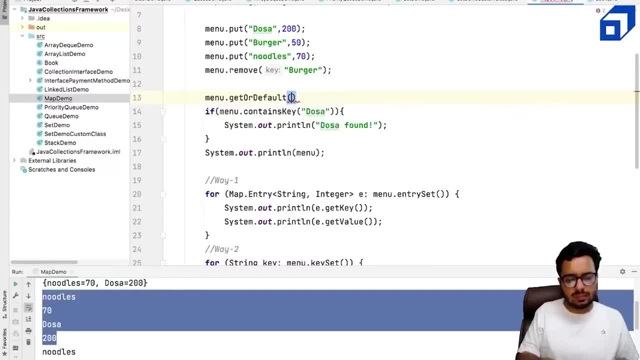 so, for example, i can say menu dot get uh. let's say uh, pizza, so pizza i have not inserted. if the pizza is not there, i can say the default value is, let's say, zero. that means um. in this case i will get an answer that is zero s out. 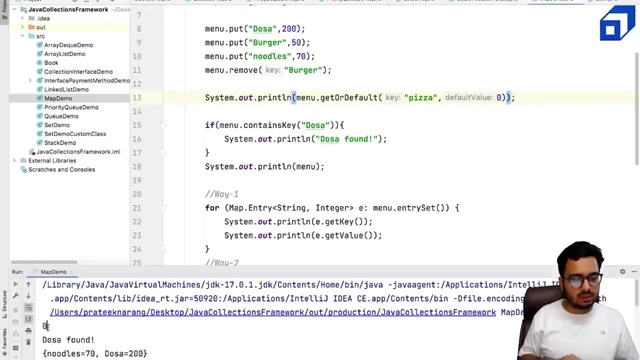 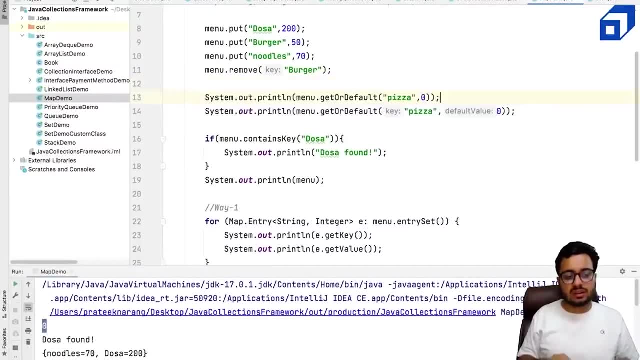 this value, right, what i'm getting? i'm getting zero. that means visa is not present, the default value. if the item is not present, i think the default value for that item is zero. i can also say: uh, i want to put pizza if it is not there, so menu dot put. if absent, i can say, okay, it will first check. 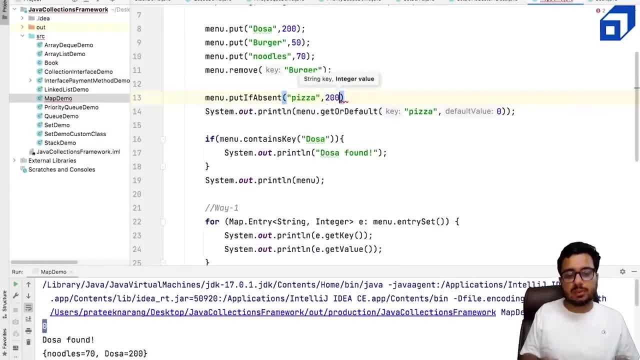 if the item is not there there, if pizza is not there, put pizza inside the map and put the value of pizza as 200. if i go and run this now, it will first insert pizza because it's not there. so it's basically using the put method with the condition and now, if, if i inquire about, give me the price of pizza now, the pizza is. 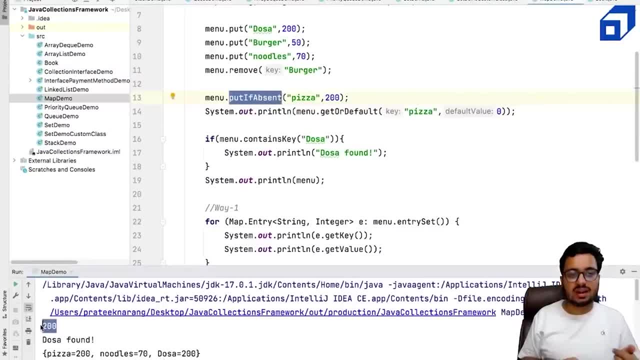 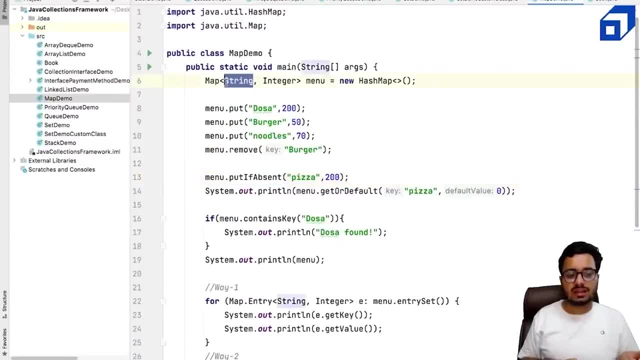 present because we have added it and i'm getting the piece of price, as that's all for map. right and now. what you can do is you can also have a custom. you can also have something more complex here. for example, list of integers, list of books. he can be of any type, value can be of any type, but if you're using a custom key, again you will. 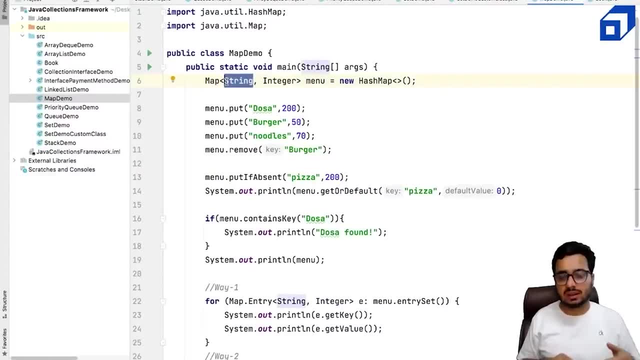 have to overwrite your hash code method and the equals method, as we did in the case of hash set as well. one more thing we can do is, if you want to replace this with a linked hash map, you can do that. everything will remain same and your ordering will also be maintained, and you can. 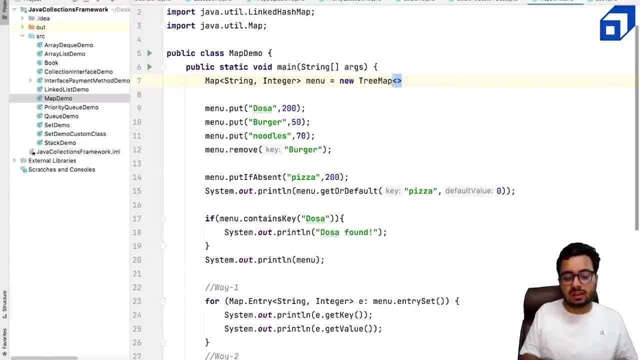 replace it with a tree map, if you want. everything will remain same, except the internal structure will be. now it will be using a self balancing- uh, bsd right, so you can also do a tree map and a first up here. we need to import it- a tree map, map, is it? the code will work fine. 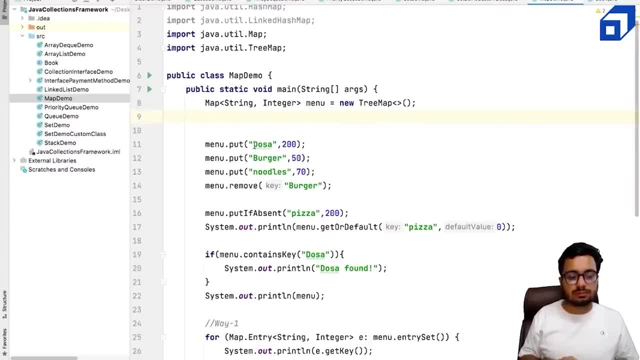 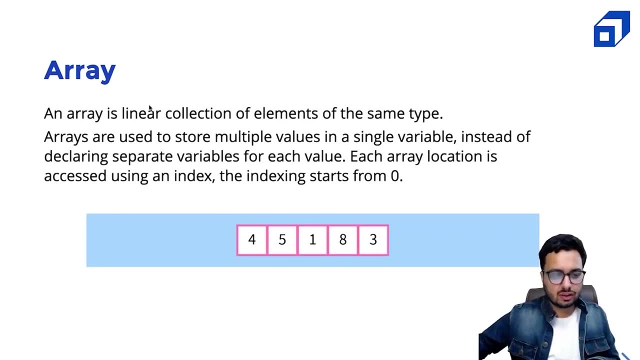 yep, now the elements will be sorted according to their keys搔 is right, so let us do this here. so now let us manage our tree map. let us begin by revisiting the concept of an array. array is a very simple data structure that represents a linear collection of elements of the same type. right, so the concept of array is? 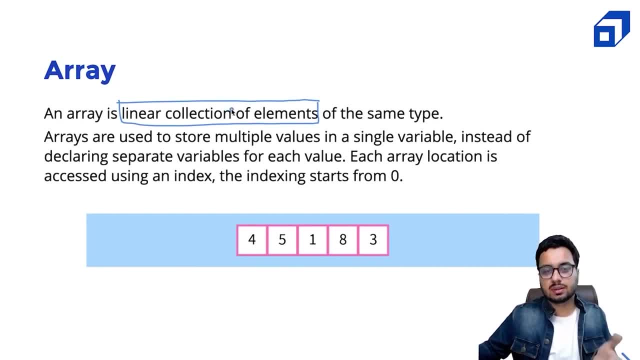 here in across all languages. in python it is called as list, in p plus plus and java it is called as an array right, and most of the time it is of the same type, but in python the arrays can also store elements of the different type, so arrays are used to store multiple values inside. 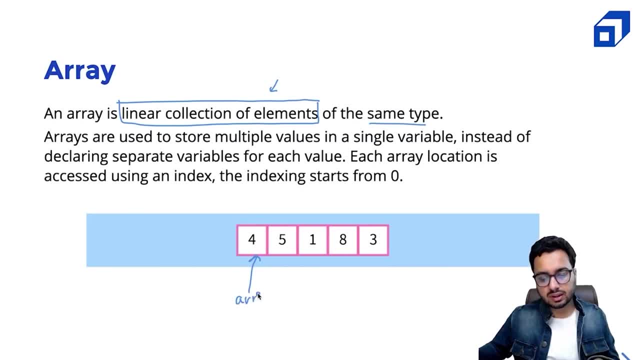 a single variable. i say, okay, this is a container, the name of the container is just one variable, but it is going to hold multiple values, right? instead of declaring separate variables for each value, we just create one variable. now this helps us because suppose you want to store. 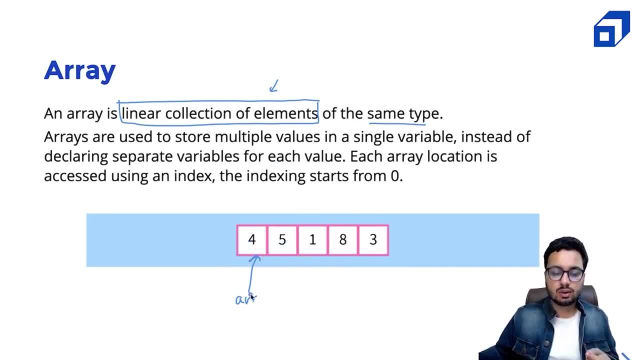 hundred integers will not create hundred variables. instead, you will create one array and in this array you will have multiple buckets. each bucket is referenced by an index. okay, if you want to store something at this position, indexing always starts from zero. right, you will take a array of zero. i want to store the number four at this position. if i want to store 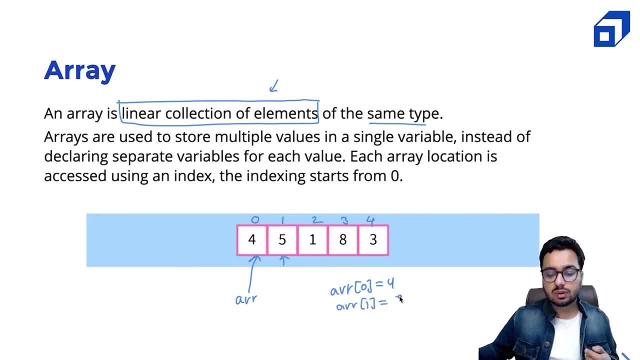 something, or i want to update something. i will take an array of, one should store five, or it should be 15.. so i can update the value anytime i want, right? so this is the syntax, right? so the variable name is array, and how do i create it? so if i want to create an array of, indeed, i will. 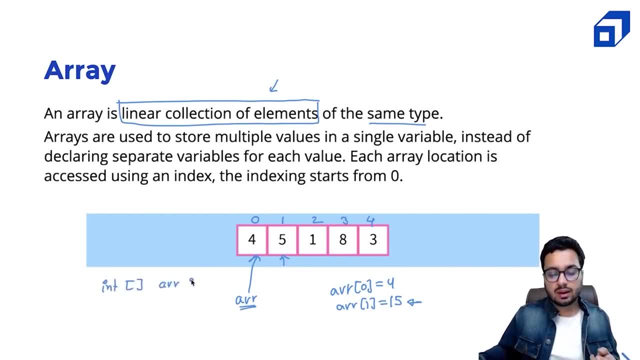 say int, followed by square brackets, followed by arr, followed by. here we will see. there are a few ways to create an array, and one is we can use new keyword to allocate some memory, or we can directly give the values which which we want to initialize the array with right. let us jump directly into. 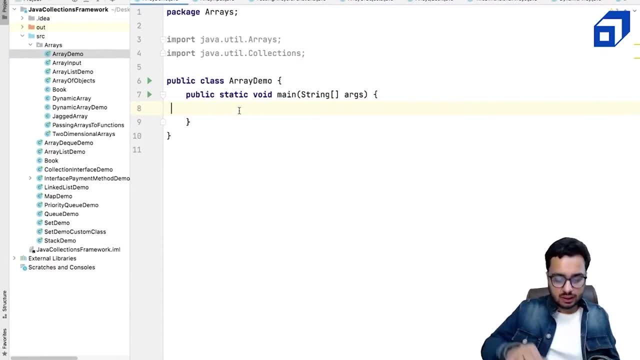 the code and see various ways to create an array and work with them. so first of all i'll say: okay, i want to create an array. so this time i'm just initializing it with some random numbers. i'm not using the new syntax, we will do that as well. this creates an array if you do s out. 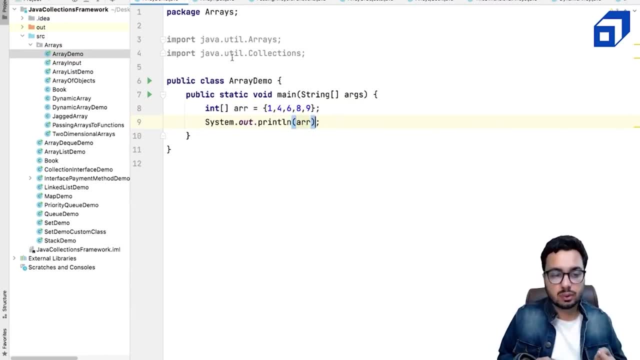 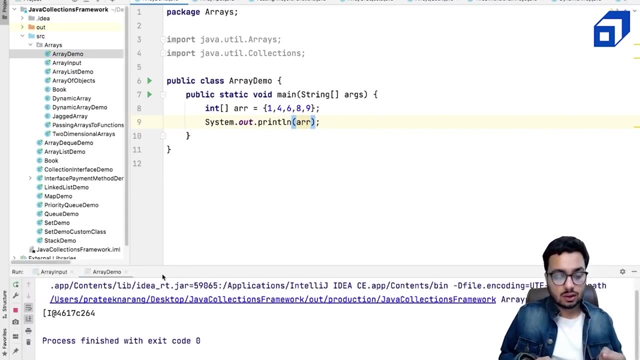 let us understand what happens behind the scenes in the memory. if you do this right, so let me go and run this code. i will see some, some kind of address. in java it is called as object reference, so i see this number. now. what is happening if you uh dive little bit into? uh, what is happening in? 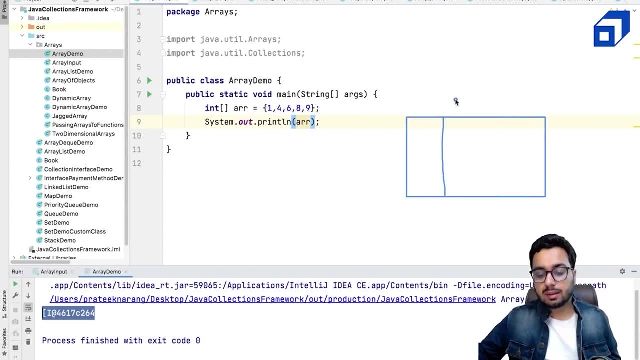 the memory. right when your program is executing, your ram memory is divided into two parts. one is your stack memory and one is your heap memory. both of these memories have their different any function that you're calling. it goes into stock and it creates a stack frame out of it, right? 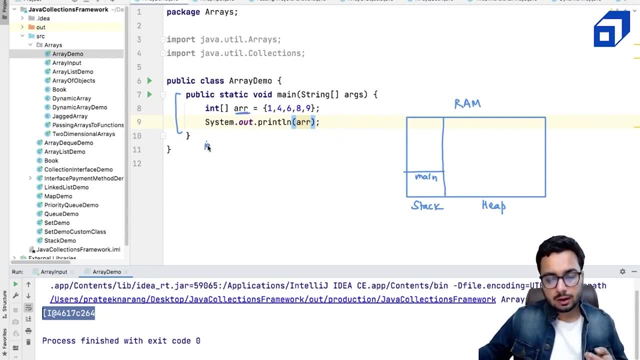 and when you're creating this, something like this, you say, okay, i'm doing index this, that is equal to 20.. when you create a primitive variable like this: x is a bucket, it is created here and it is storing 20.. but when you create an object, java is object, the actual object it. 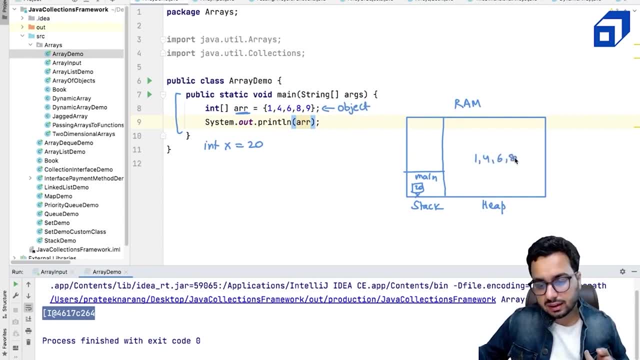 is created in the heap. so your one, four, six, eight, nine, it is created in the heap and the address of this object, whatever is this address? 264, right? so 264 is stored in a variable which is there in the stack, and this is storing 264, that means the variable in the stack. 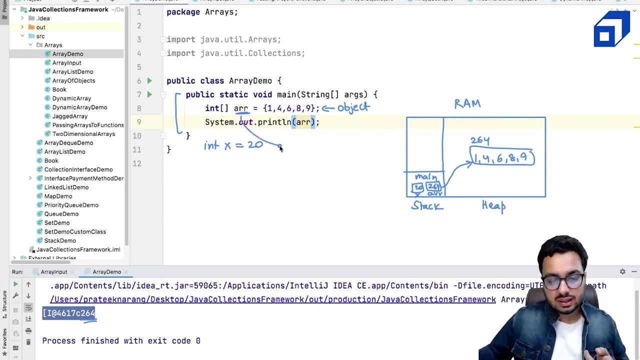 frame is pointing to the array object, so we call this arr as a. this is a object reference. this arr is not the array itself. it is referring to the array. this is how it is created a behind the memory. right now, when you are going to print arr, it's not going to print the contents. 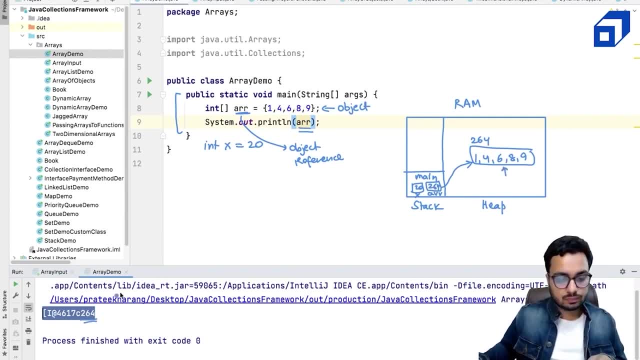 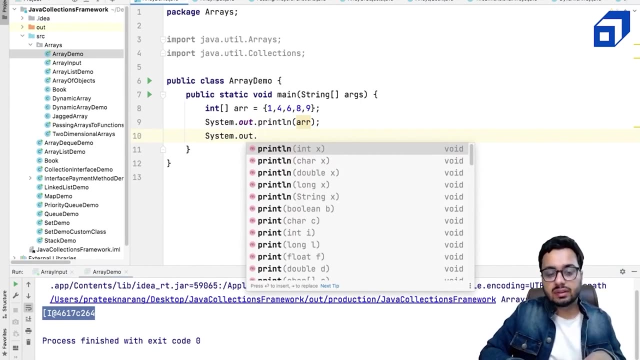 of the array. instead, it is going to print what is stored in arr, right, if you want. okay, i want to print the contents of this array. right, what i will do. i will say: okay, i need a way to iterate on this array and convert everything and print everything right there. 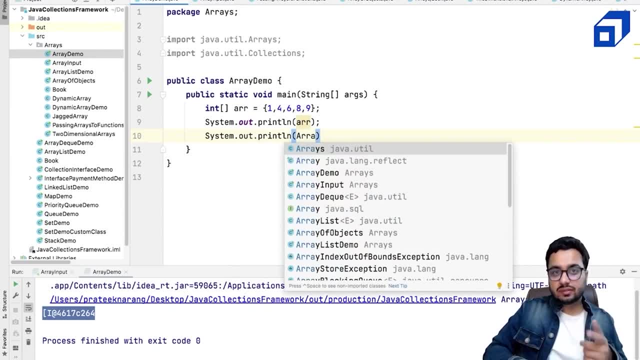 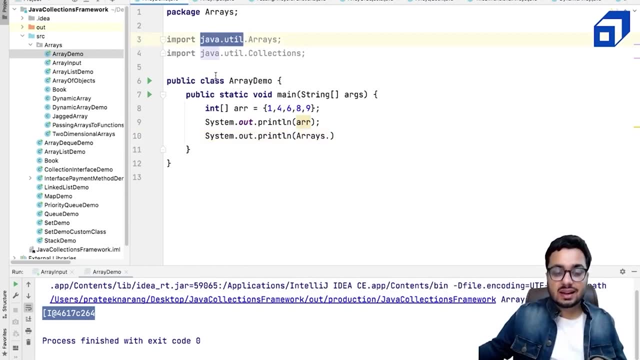 is a inbuilt function that we can use, so there is a different class. okay, it's. there is a class called as arrays and it is part of javautil, so arrays class has certain helper methods to work with these kinds of arrays. in this these methods, we have to pass the array object and get a- get our. 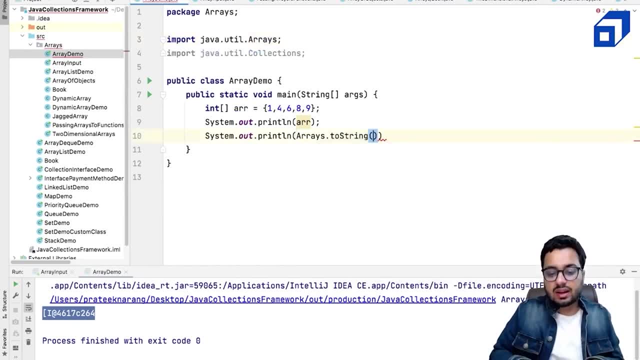 work done. so one such method is to string. i will give you some kind of array and you want, i want you to convert this into a string, like representation, that can be printed using system dot out dot println. so let me give this array and now, if i show you what i am, 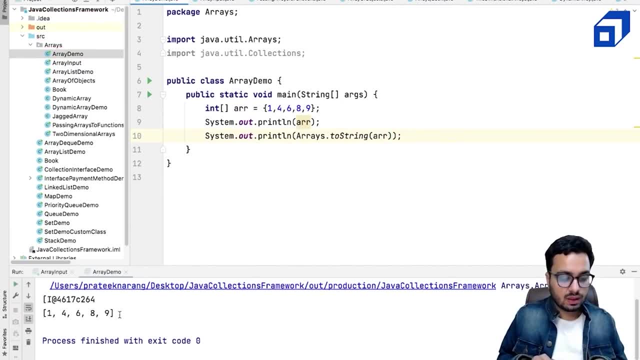 doing? what is the output? let's see. now i am getting this array, so i am hoping that you are able to understand why this is working right. what could be the logic behind this two string? it is doing nothing, but it is doing a traversal on the array using a for loop. 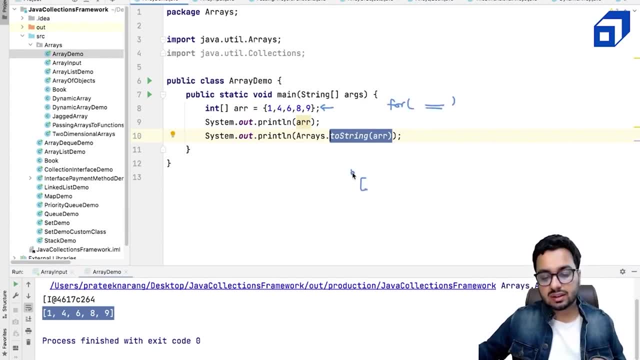 and it is adding everything into a string. so it says, okay, i'll start the string with the square brackets, then i will add the zeroth element, then i will append the first element, and so on. something like this it is doing. but what is happening? it is simply iterating. 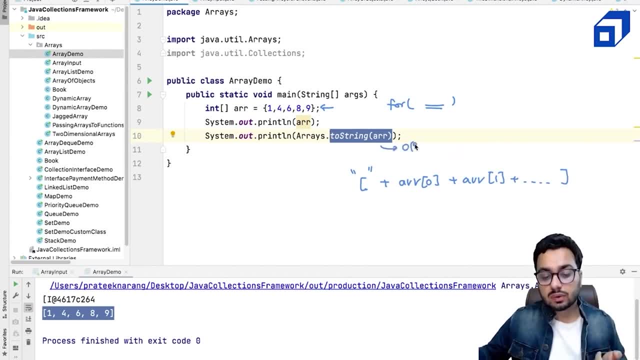 over the array. Now let's talk about how much time it will take. it will first take order of end time to iterate over all the elements of the array. Let us look at one more method in this array. so let me create one more array. let me call: 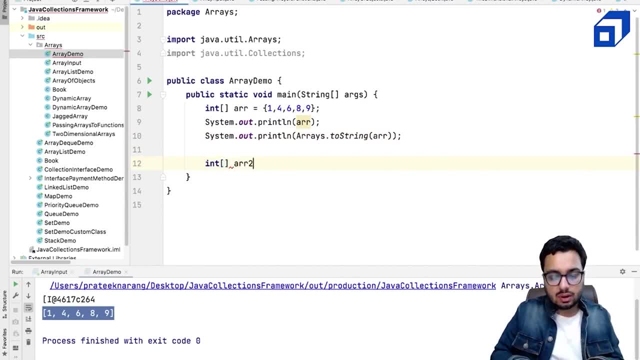 that. call it as some array, let me call it as array2. this is equal to new int. i am saying, okay, let me create an array. this time i am not going to define you the, give you the data, but i am simply giving you size of the array. that okay. 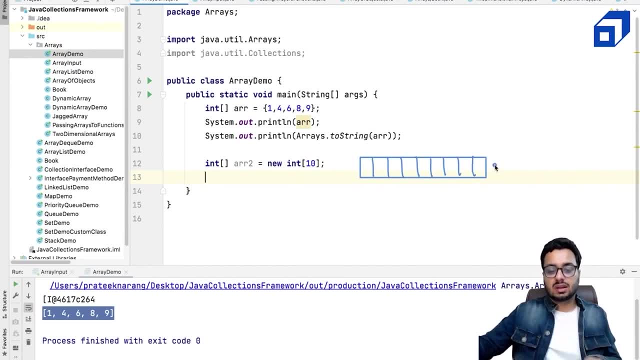 I want an array. I want an array that should be able to hold 10 numbers. one thing you can do is you can manually initialize every index. you can say array of 0 should be 8, or let's say, i want to fill 5 in every position. right, one way is you put a loop and update every index, or 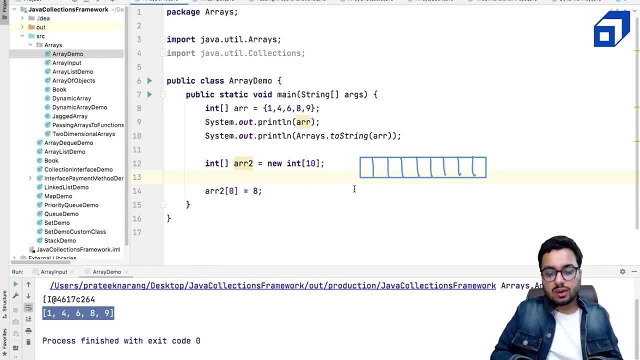 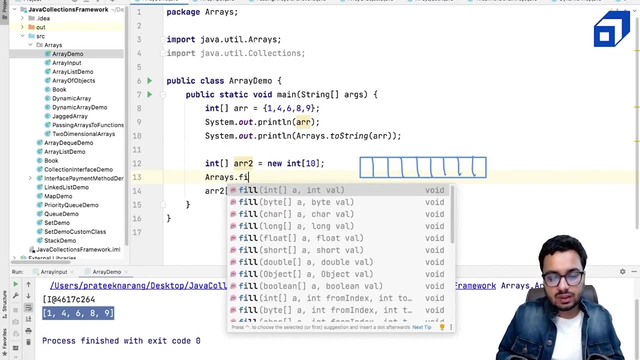 you read input that we will see very soon. but there is one more method. if you want to initialize an array with a particular number, so that method is called as arraysfill, look at this, there is a fill method and you can say: okay, i want to fill this array with number. 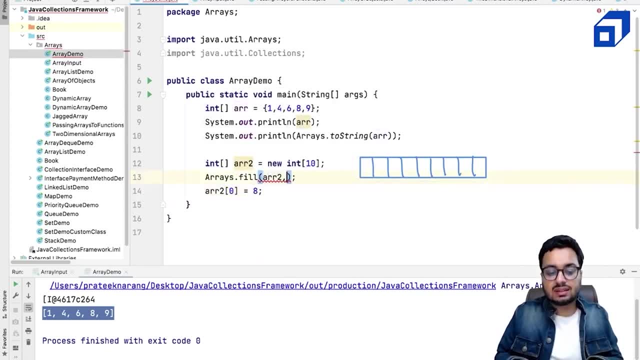 that is 12, so you need to pass the array object, that is array2, and maybe the value that you want to fill. maybe i want to fill with the number 13. now, if i show you the output, i can say: sout, array2. but i have to first convert it into a string so that i can print it: arraystoString. 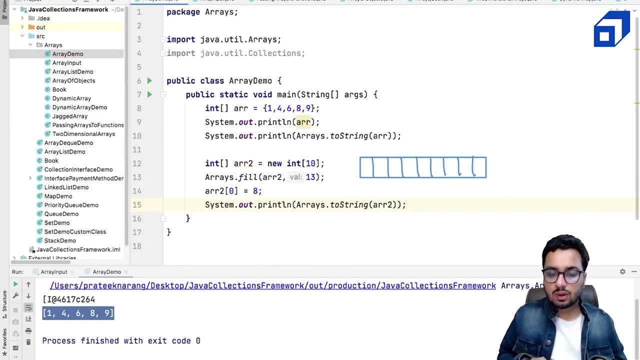 that is array2.. okay, let me print the second array. can you guess what the output would be? the first element would be 8, which i have overwritten. okay, so this is updating the zeroth element, and rest all the elements will be 13. this is what we are getting right. the fill method is going. 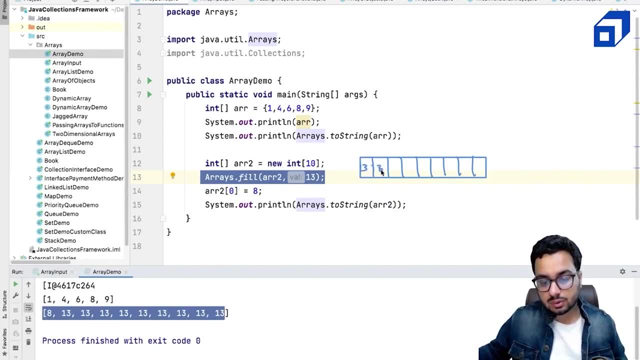 to fill this array with 13 at each position and so on, and first zeroth index i am updating as 8, so i get 8 followed by all 13s. that is another method present in arrays class. okay, if arraystoString arraysfill- one more method that is coming into my mind. it is very popular. 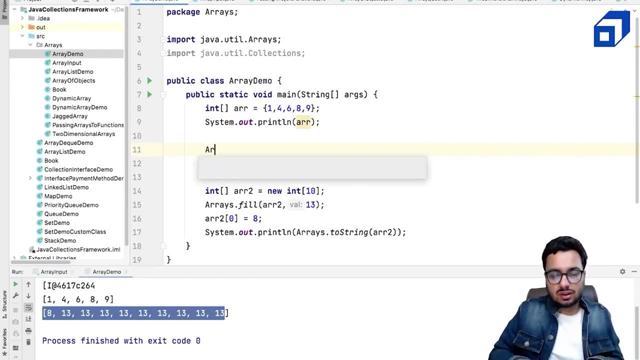 we need it often. this method is called as arrayssort. that is also present in this arrays class seconds. okay, let me sort this array. i want to put all these numbers into ascending order. so i say 1, 14 um 81. just randomize the numbers so that after sorting i can see they're actually. 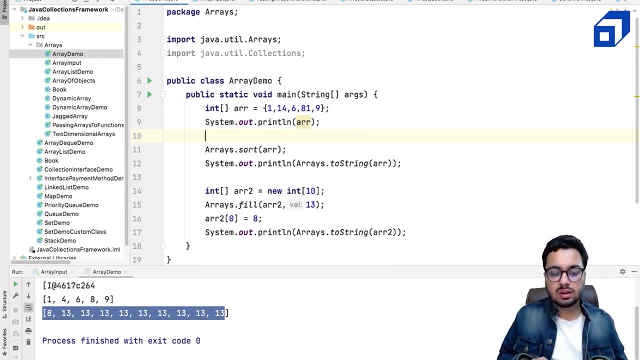 in the sorted order. right, let me run this code now. you will see this array. it's going to be in the sorted order. see, the array is getting sorted. so internally it uses something like a quick sort kind of an algorithm and the running time complexity of the sort method it is. order of nlogin. okay. 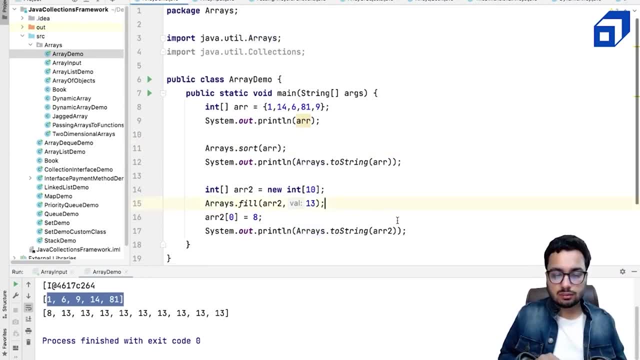 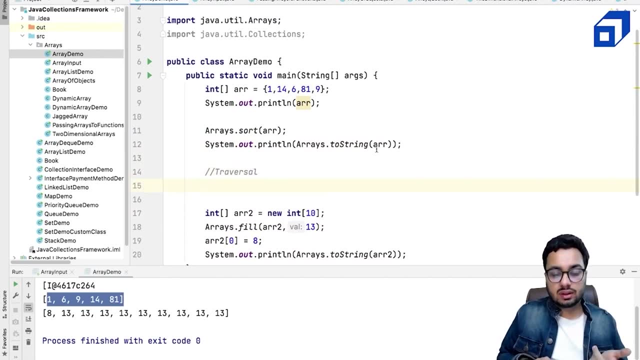 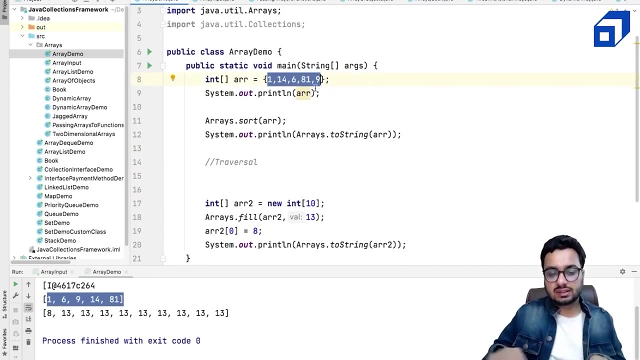 this is something that you should, okay, so let us look at one more fundamental thing in arrays, that is reversal. so there are three ways to, two ways to traverse the array. one is that i can find out the length of the array and then i can go over every index. if i talk about this array, i know there are five. 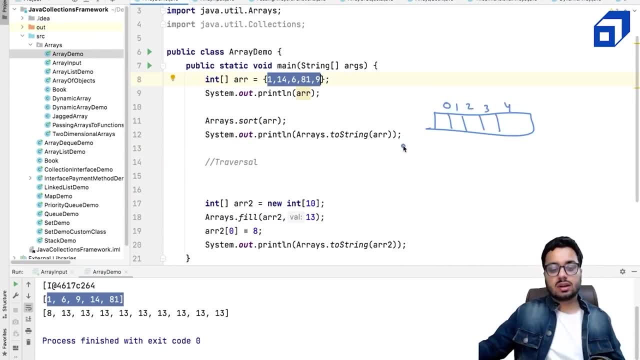 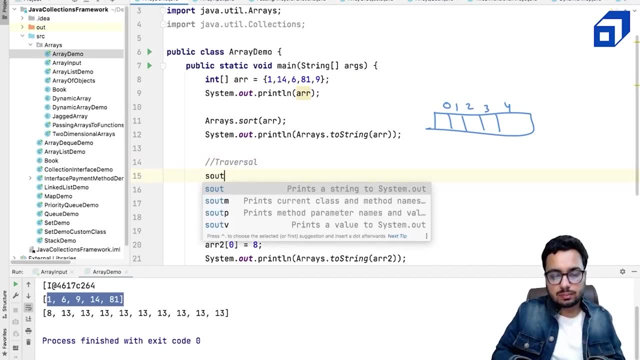 elements. so the indices are zero, one, two, three. so uh array object has a property called as length. so if i say okay, i want to see the length of the array. so s out, uh array length. i can say: this is given by length attribute of the array objects. i can say: array dot. 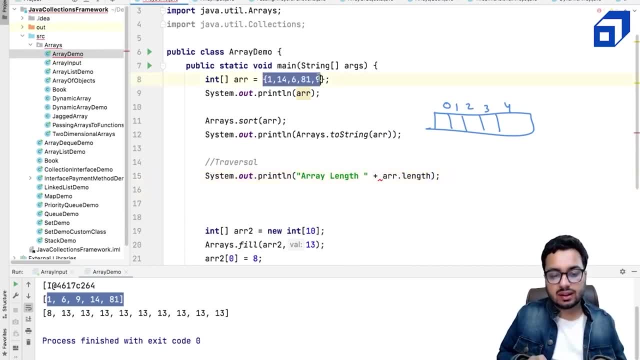 length. this will give me okay. this particular array has five elements, so, and if i have to iterate, i can say: okay, for i equal to 0, the index starting from zero, i less than array length, i plus plus, and what i will do, i will say s out. 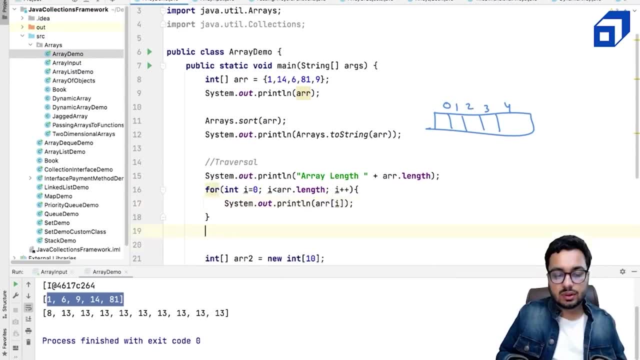 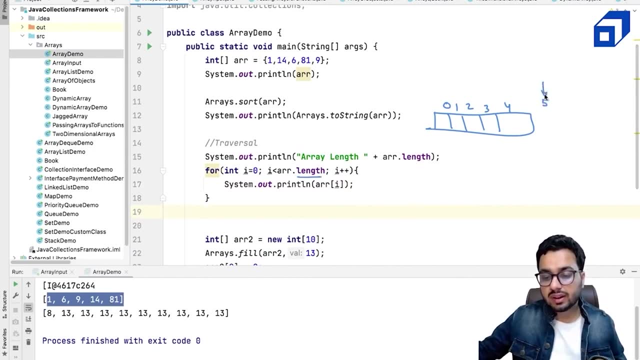 array of i, i plus plus. this is essential for running a Homně gerangaine project. it's the way you close, going to print the ith element of the array and we are doing it for all indices less than five. we do not go till five, but we go till less than five because the indices start from zero and they 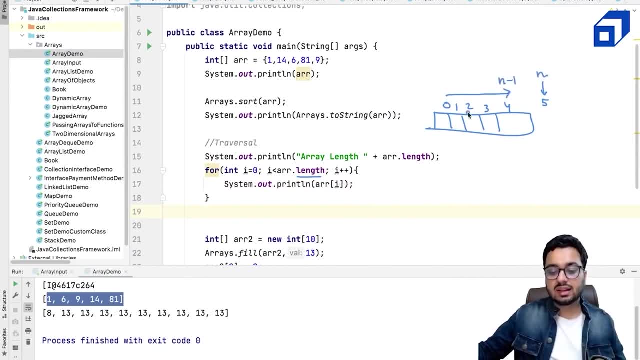 go till n minus one. this is n. the last index will be n minus. the other way is: you can also use uh enhanced for loop, also known as for each loop right, so you can take a for every integer x that is present in this array. i want to print that x, in this case x, is not your. 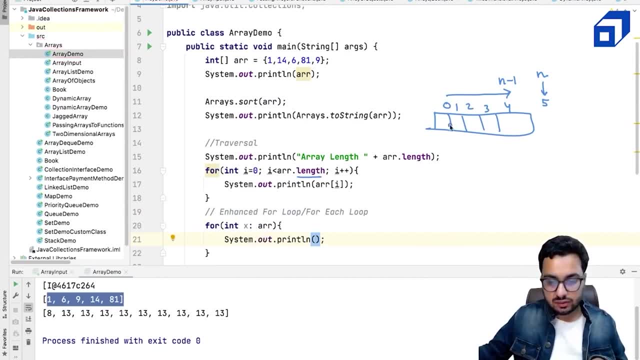 index, but x is the value that that is contained in this area, if it is like 1, 6, 9, 14 and 81. so in the first iteration x will take the value 1, the next iteration it will take the value 6 and it will take the value 9, then it will take 14 and then it will take 81.. if i simply print: 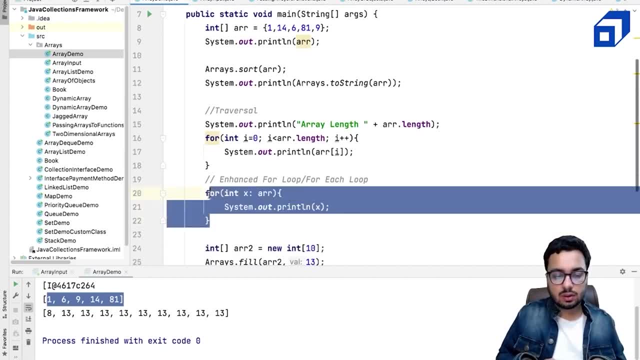 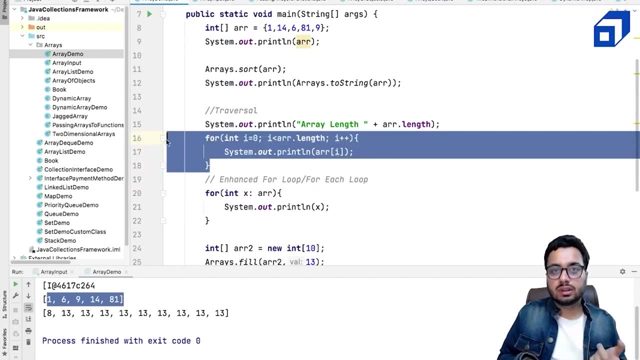 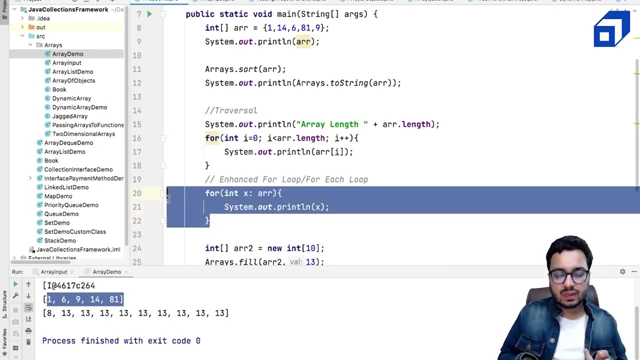 the value of x. it will again give me the contents of these are two ways to iterate on the array. if you want to iterate on some part of the array, better go with the for loop, if you know that. okay, i want to iterate over all the values, then the for each loop is a more simpler syntax. okay, but the first loop is more powerful. 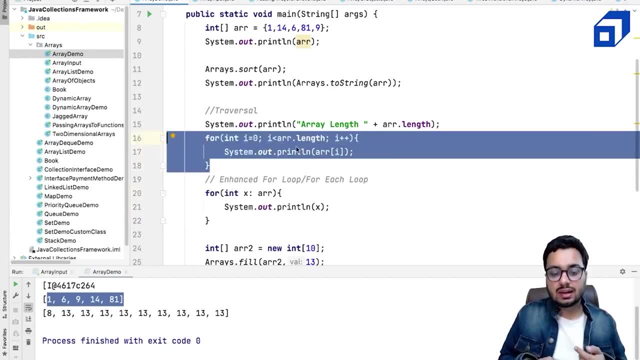 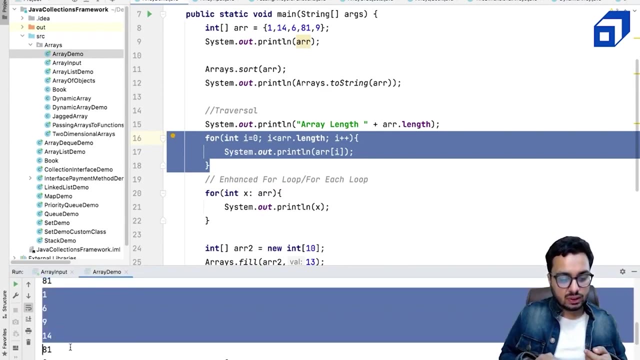 because you can start at any point, start at any index and you can stop at any index. so let's run this code and see that we are able to iterate on this. okay, so we can see we are able to iterate 1, 6, 9, 14 and 81- this is coming from the for loop- and 1, 6, 9, 14 and 81- this 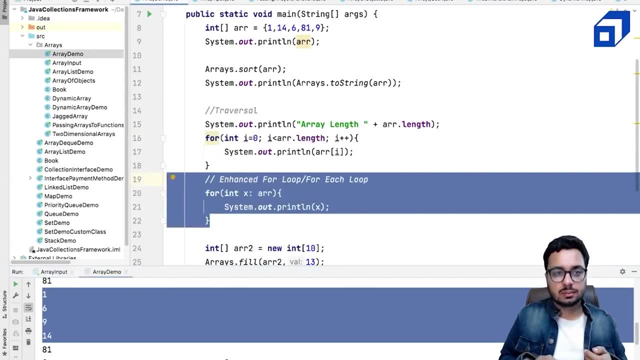 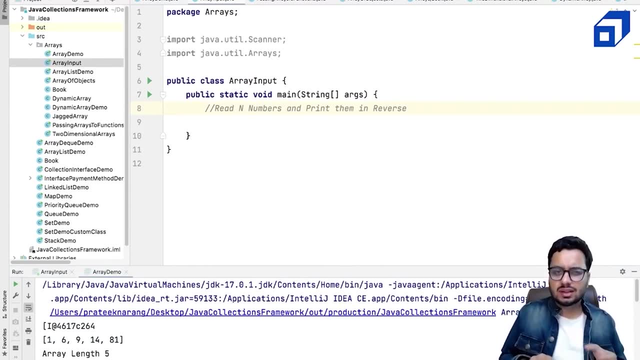 is coming from the for each loop that we have written. let us look at another way of building an array. many problems will require you to reading n numbers and storing them and working with them. so, for example, a very simple use case is we have to read n numbers and we want to print them in. 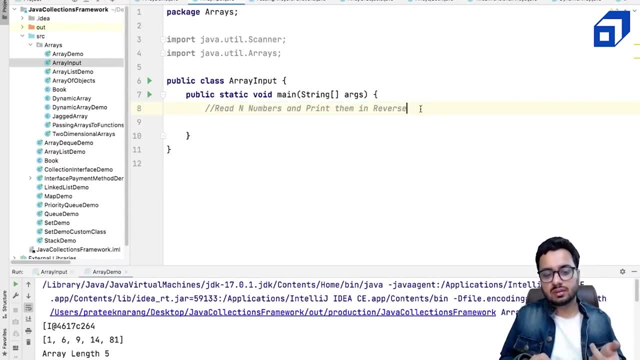 reverse. without storing them. we cannot print them in reverse. that means we will need an array to do it. how do we read n numbers? so it's very simple. first of all we need a scanner java. so scanner is used to uh. scanner object is used to read something from the command. okay. 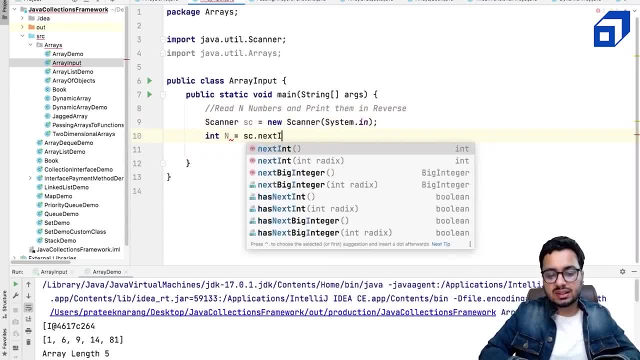 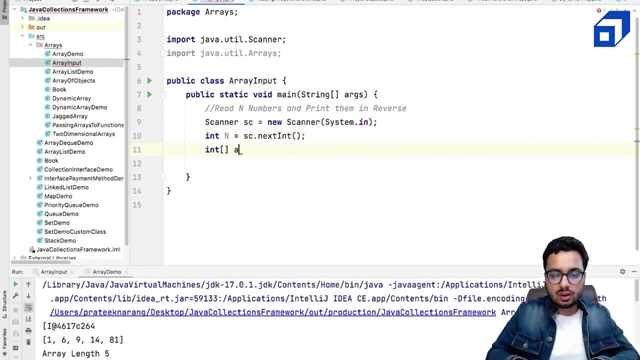 i can, okay, first tell me how many numbers are there. the method is called as: next. once you know n, then okay, i'm going to create an array. how do we create an array? let's say i want an integer array and i can say- this is new here. i define: uh, what is the size of this? 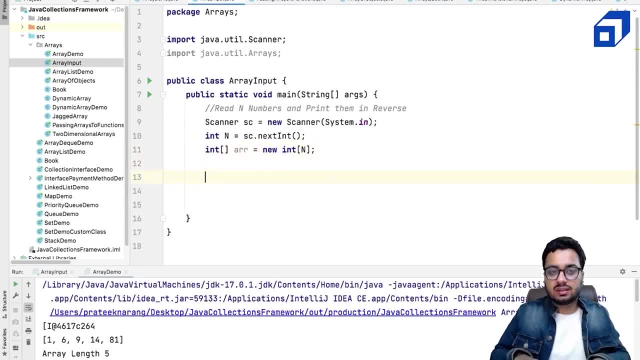 this will create an array of size n. now i want to read this array again. it is pretty simple. i will read the youth index, first index, second index, up to n minus one at the end it's okay, i less than n, i plus, and in every iteration i can do, array of i is going to hold. 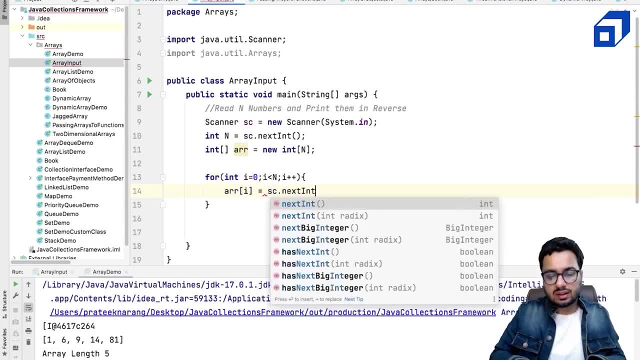 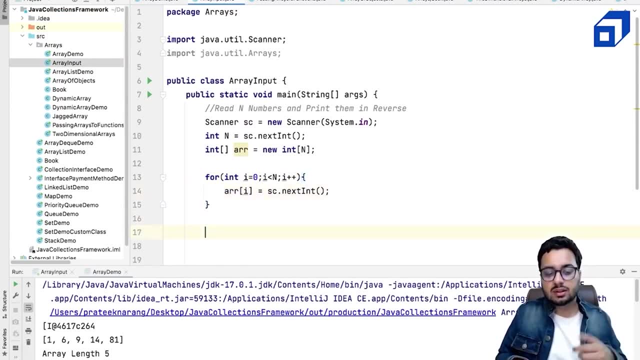 n value will read from the user. i can say: scanner dot next, scanner dot next, and will pick one number from the command, put it in the ith bucket and once i am done i want to print them in. print is easy, so how do we print it? i can say: okay, i can start from the last index, that is n. 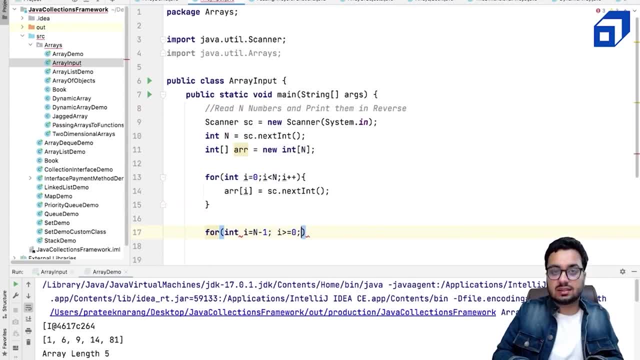 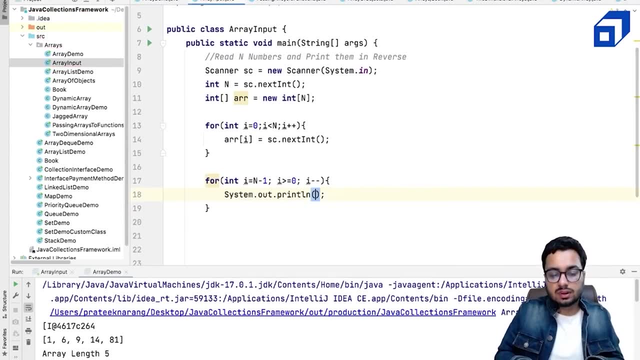 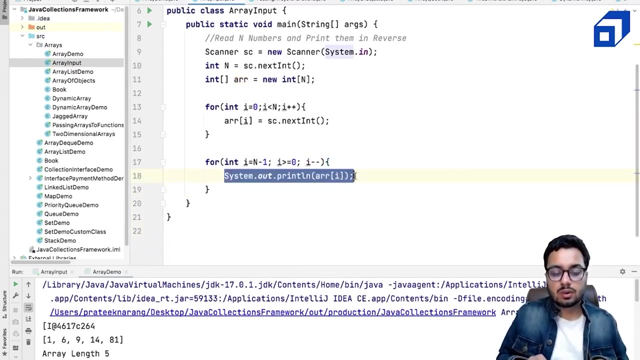 minus. i can go till the first index that is zero, i minus. so i just need to reverse the loop that i'm using to iterate over the array and i can simply uh iterate in the reverse direction. so system dot out dot print ln array of i. let us go and run this code and: 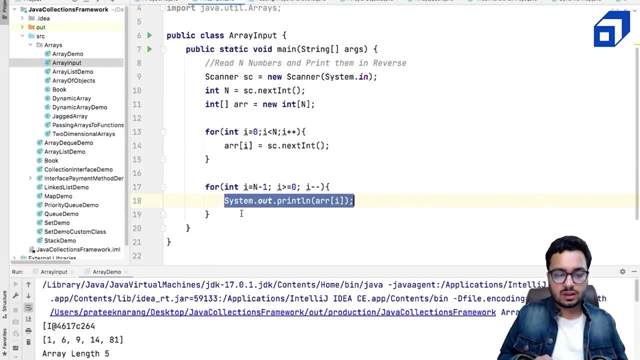 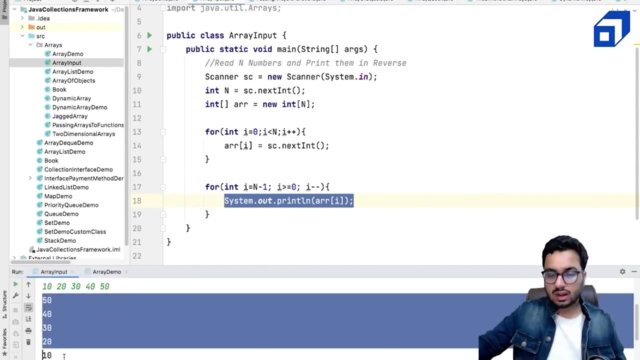 see, suppose i want to uh read five numbers and print them. so let's say the numbers are 10, 20, 30, 40. so you can see, i'm able to print 50, 40, 30, 20, 10.. so what happened? i created an array of. 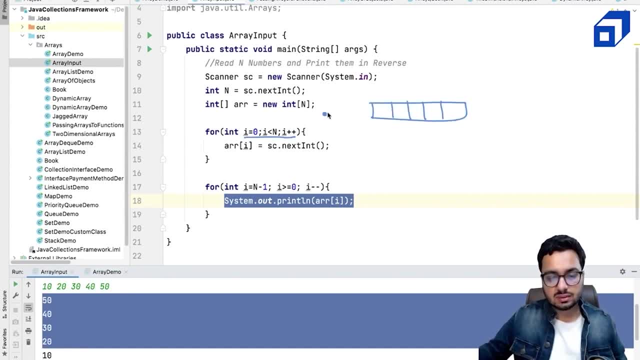 size n. then i stored numbers. i said, okay, go over index 0 and read one number from the command line. then i becomes one. it is reading one number again, scanner dot. next in the next integer in the line it is reading, it is storing here and so on. so 30, 40, 50. then what i did? i iterated from the last. 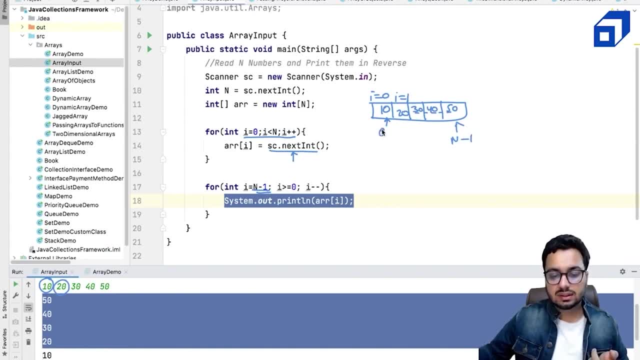 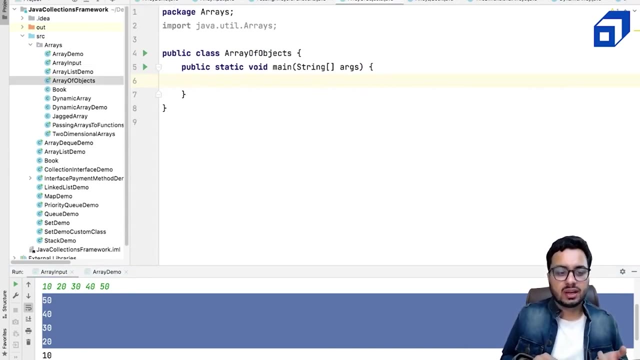 index which is n minus one till zero. in this direction i iterated and i printed array of i. this will print my array in the reverse order. the next thing i want to talk about arrays is array of objects. okay, we have seen how do we create an array of primitive. 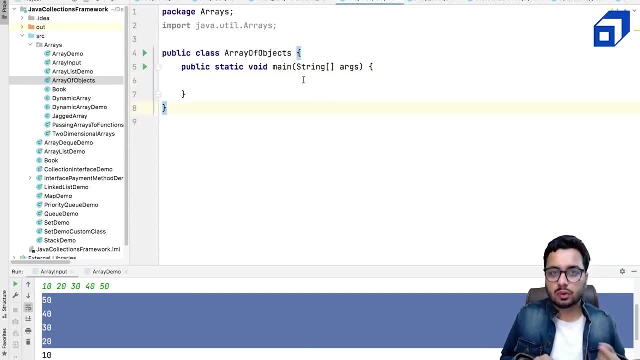 data types like integer. similarly, you can make up an array of float area, of boolean, like primitive data types you can work with. but what is an object? so complex data type like strings? string is an object. okay, you can also have a user defined class and you want to store objects of. 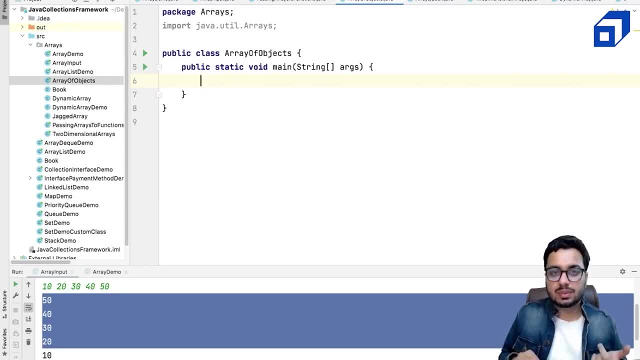 that class in your array. let us see how that actually happens at the memory level and also at the syntax level, right? so suppose i have. i have a book class. i'll just delete this method. in this book class i have defined three attributes of the book. one is isbn, which is your unique book code, a name and a price. 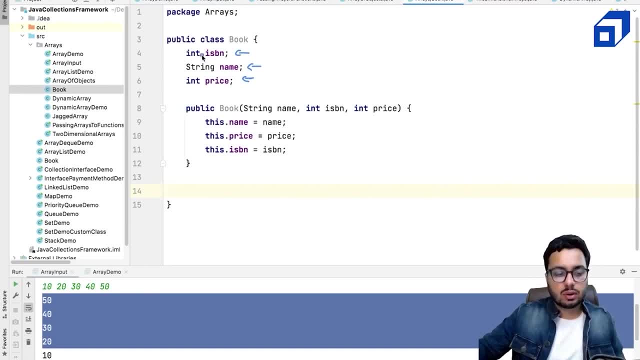 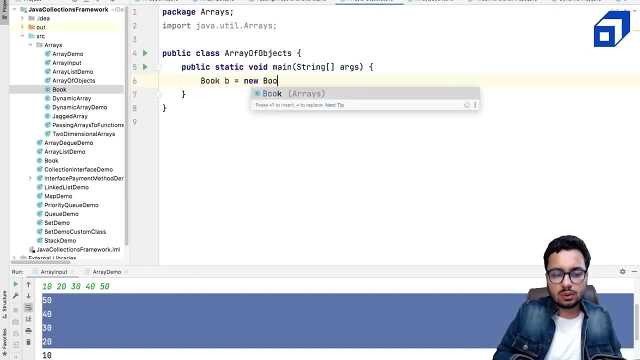 and i also have a constructor to create a book object. right, if i want to simply create one book object, how i will do it? i will say, okay, i want a book b. this is equal to new book. in this new book i want to pass the name of the book and isbn and the price. i say okay. 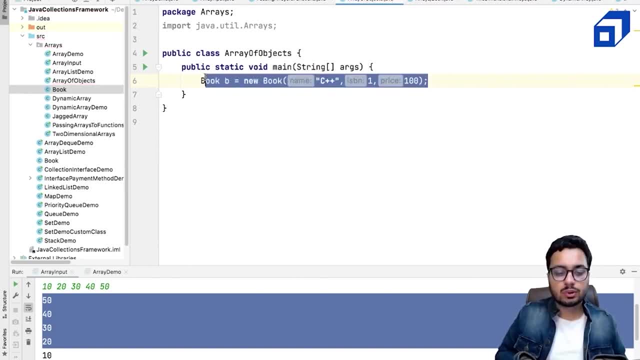 these are the three attribute, or three values that i'm going to initialize this book with. this just creates one book object. but what we really want? we want to create an array of book. how do we do it, please? okay, book, followed by square brackets. that is the data type of the array. 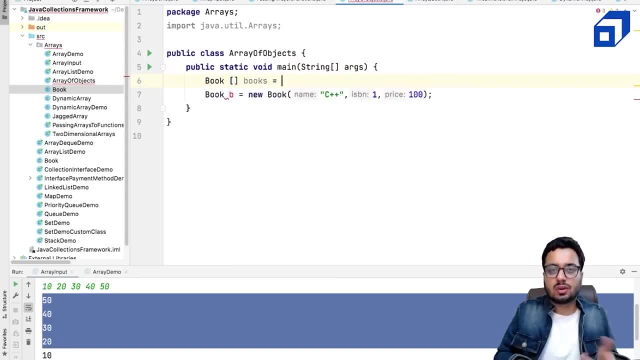 then you have to give a variable name. i say, okay, the name of the array is called as books, let's keep it intuitive. and followed by new book. suppose i want to store three books in an array, right, this is going to be three. now what it's going to do, right? so, as i 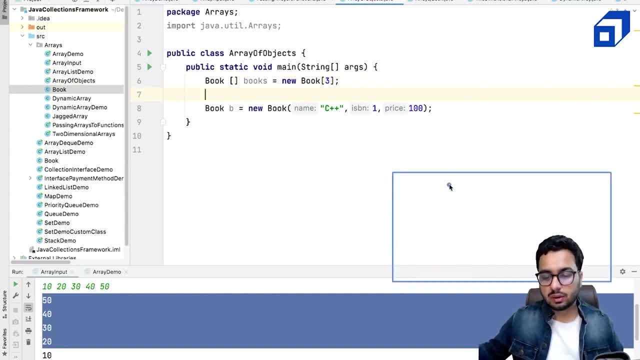 discussed in an integer. your memory is going to get divided into two parts. one is your stack memory, which your main is getting called, and we have a variable called as books, which is going to refer to an array that is capable of holding three. now, this is this position: is books of zero. 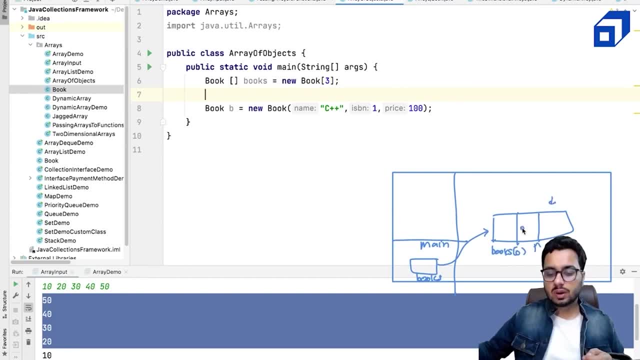 this is books of one and this is books of. how do i put a book here? one option is that: okay, i have created a book, object b, already. b is a book, so b is also created here. b is pointing to book. that is a c plus plus book. c plus plus book has 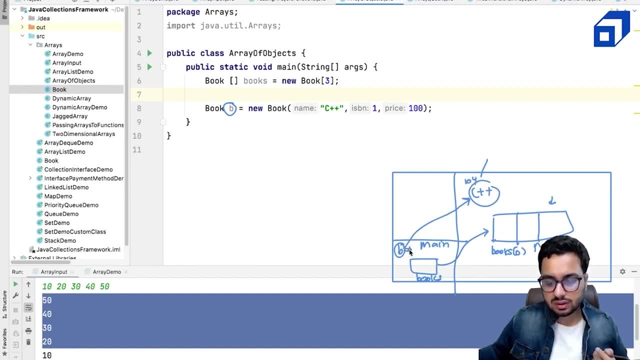 some address. let's say 1 0, 4.. b is storing this value 1 0, 4.. now i want to put this book inside this array. i cannot like physically, i i cannot say, okay, this object will go inside this box in the heap. no, this is now not how it happens. the way to do it is you will have to say that books of 0. 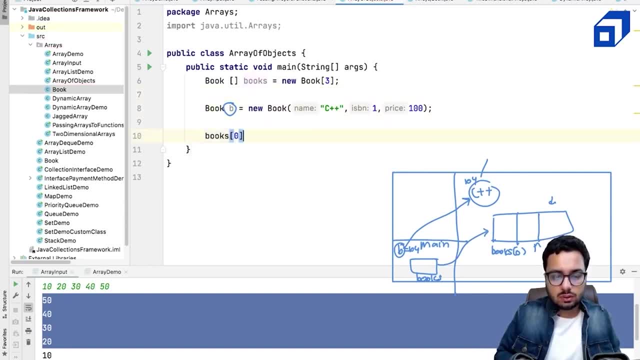 it is going to hold b. books of 0 is going to hold b. that simply means that whatever is the value in stored in b, it is also stored in here. this value is 1: 0.. what does it mean? so it simply means that books of 0 is referring to the e plus plus object, c plus plus book object that is present in the heap. 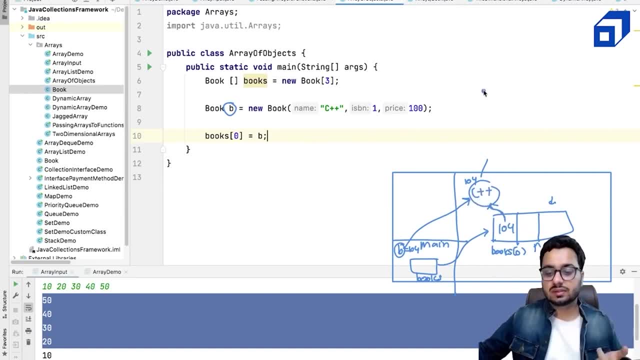 this is how it is getting stored. in case of array of integers, it is different. case of array of integers, you say, okay, uh, array of 0, this is equal to 5.. the number is directly stored here, right. but when you say books of 0, this is equal to b. uh, books of 0 is holding the address of this book of you might say, okay. 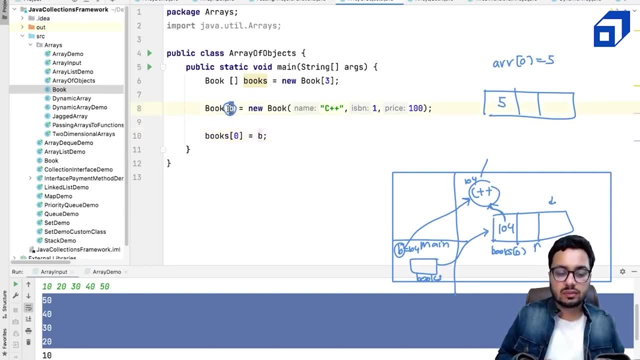 this. this might be the reason, um, because we have created a b reference variable and then we are copying that value. even if you do something like this, you say, okay, uh, books of one should be equal to new book, and let's say: this is a java book, uh, with code. 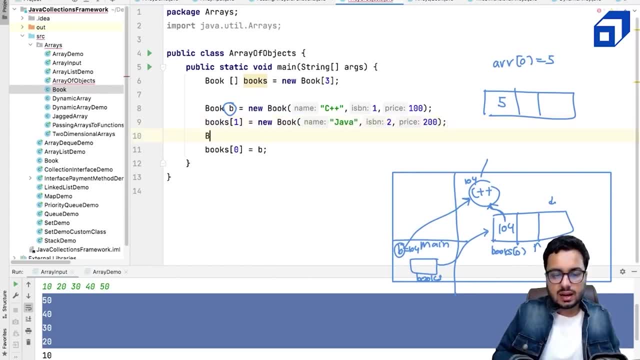 two and price is, let's say, uh 200, and let's say: books of two is a new book which is, let's say, a python book, and uh code is, let's say, three prices. let's say one. something like this: let's say: we have now books of zero, books of one, books of two. 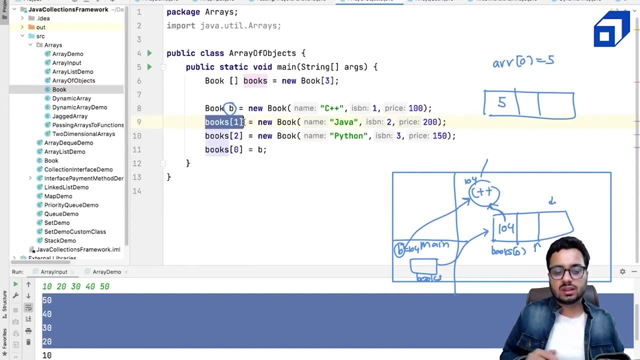 what is happening when you're doing this statement. this is even doing the same work, just that this new book object is getting directly stored inside books of one. so that simply means whenever you use new book, it creates a book object in the heap memory, right? it's not going to create inside the array. the java book is created somewhere in the 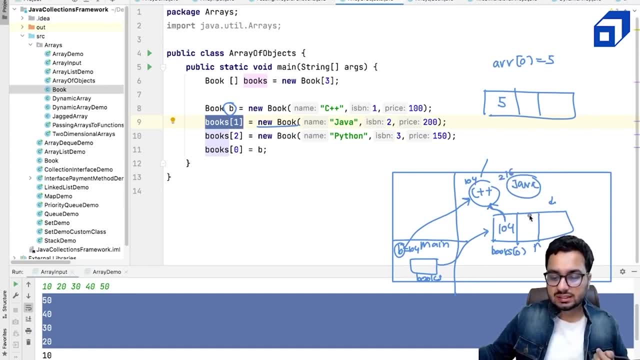 heap. maybe this location is 216 and this address is getting copied here, so this is going to be 216. that means books of one is going to refer to this java object, and when i say books of two, this is equal to new book. so again, a new book object will be created in the heap. let's say this is python. 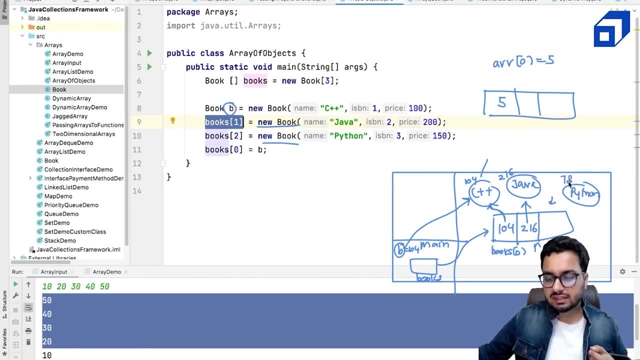 and it has some address, let's say 780, so 780 will get copied here. now you want to say okay, i want to really verify. this is how it is stored. let me show you, um, by doing an s out. right if i say s out, uh? 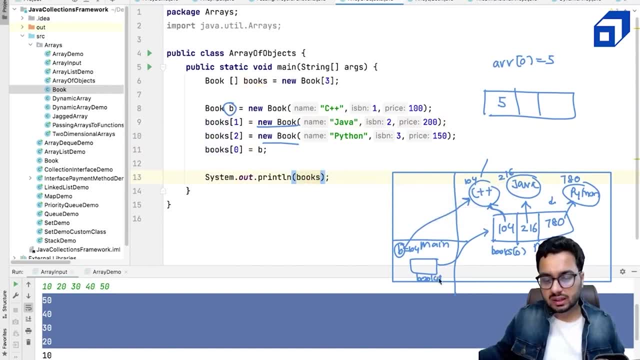 books. what i'm going to get. i'm going to get the address of the whole array. maybe this uh books array is created at a location that is 200. i'm going to get this 200, but now you might say, okay, no, i don't want to print this, i want to print this entire. 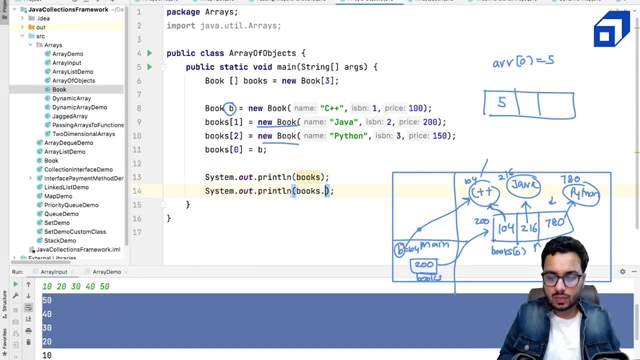 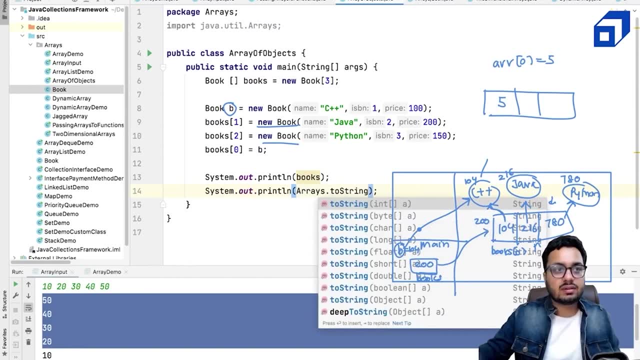 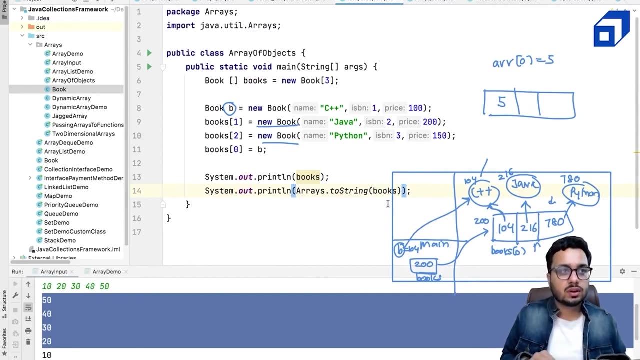 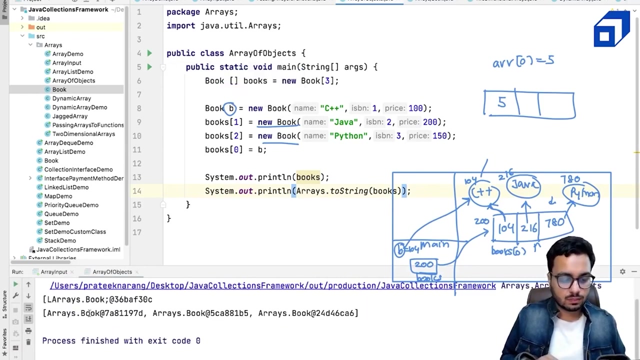 array. if i say s out: uh, arrays, dot to string. basically, i want to, i traverse on this books array and i want to print it. let me show you this output. what output and do we really get? let me run this one now you see what we are getting. here is the address. 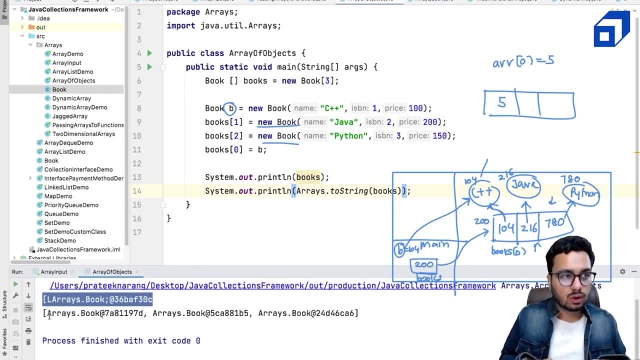 is the value that is stored in this books variable and what we are getting here. these are the three addresses stored in this array which are referring to the three books that we have. this: this is c plus plus java and python: three objects. their addresses are stored in the books array and this: 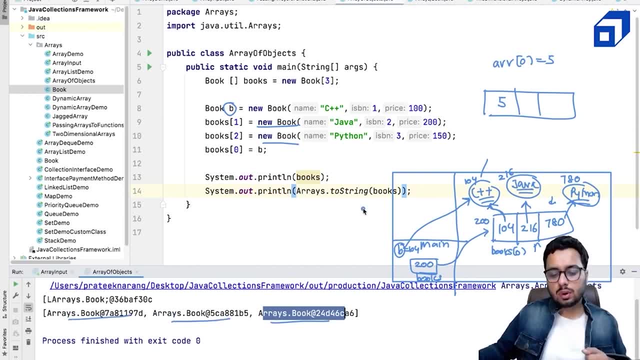 is what we are getting right now. you might say: i want to print the content. i actually want to print the object, i don't want to print the print an address. how do i do that? right, the reason is: java does not know how do we print this book. okay, how do we actually go to a location and print that? 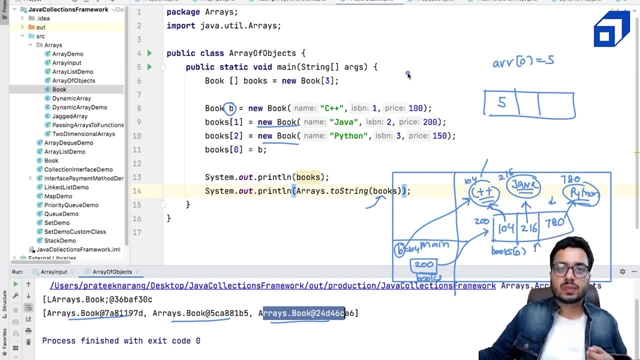 object. so in order to do this, there is a method called as to string that is present in inbuilt classes. okay, for example, when you print strings, string has a to string. or if you print like some object, right, so many objects have their own to string method. 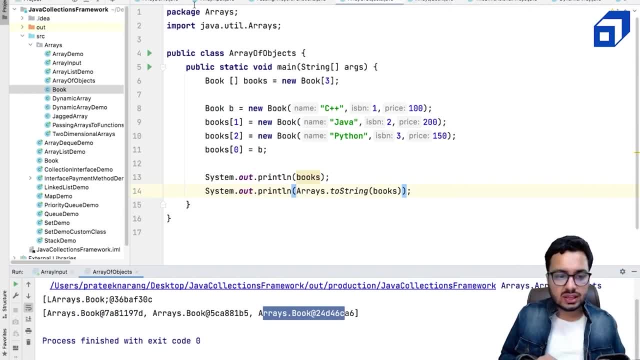 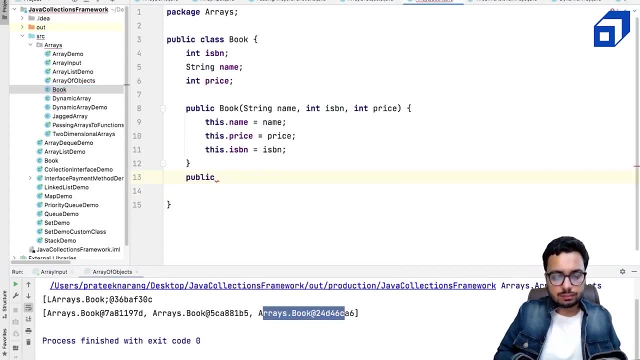 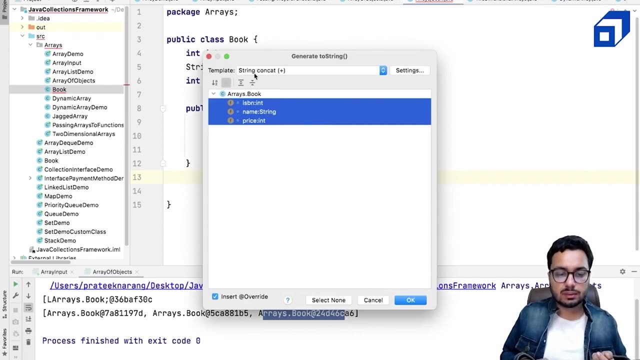 what we have to do. uh, we have to go inside the book class, which is this, and we have to say: okay, i want a two string method, right, public string, two string. so this method should return a string. it is automatically giving me a recommendation that there is a default template in which i will. 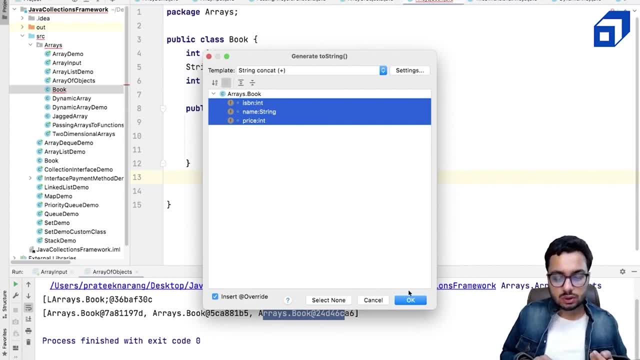 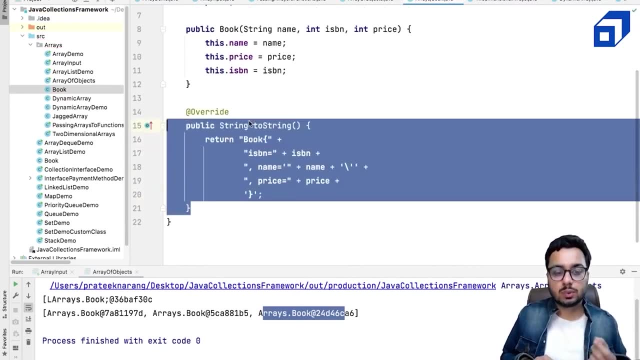 concatenate these three properties of the book, which looks good to me, so i will just click ok and it will create a method for me, right, when i want to say, Okay, I want to convert this book into a string Internally, it is going to call the toString method of book, right? 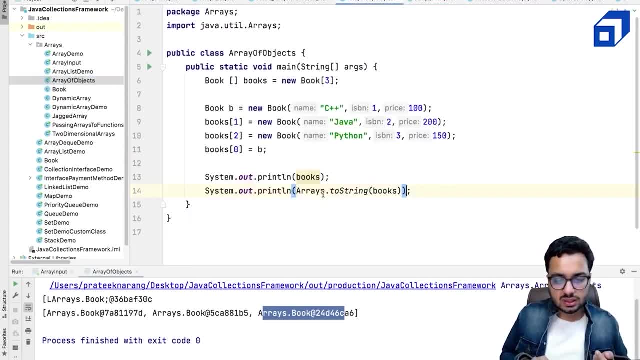 Which method I will tell you. Let us go to array of objects. When are you saying arraystoString? It is going to iterate on each book And it is going to convert that book object into the string-like representation If the toString method is overwritten, right? 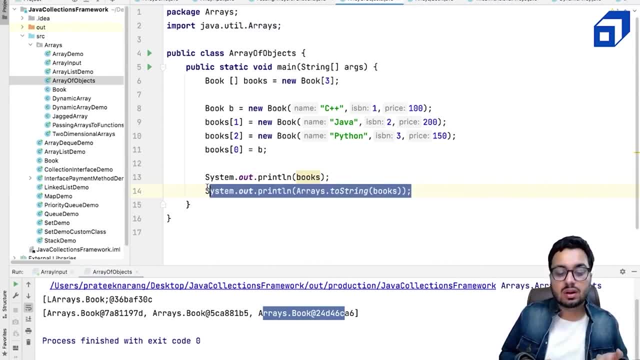 We have overwritten that method. So what we will get, We will get the contents of the book. Let us run this code now once again And see what do we get now. Now you can see I am getting a book. That is the C++ book. 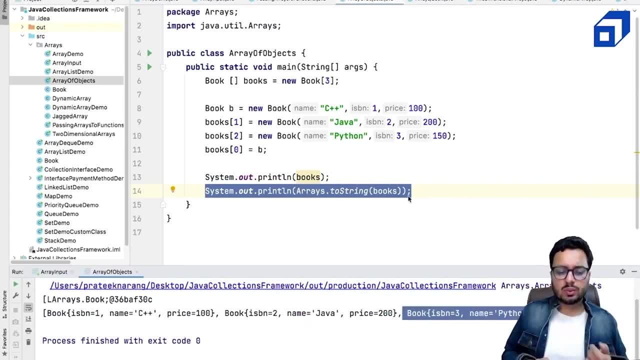 Then the Java book And then the Python book. You might ask: okay, can we do something more on this object? The answer is yes. Maybe you want to sort this array of books right? Do you think arrayssort will work? 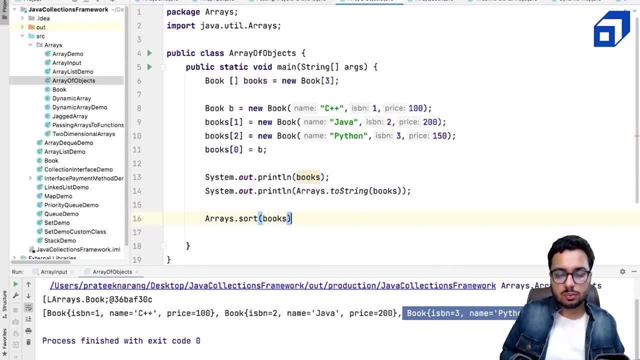 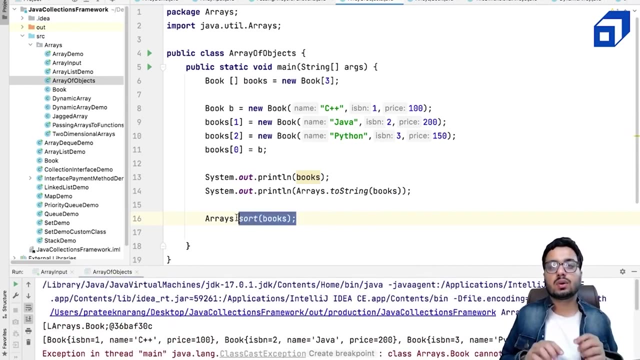 I want to sort this array of books. Will it work? I might get an error. Okay, I am really getting an error here. Why? Because the sort function does not know how do I compare two book objects. Okay, how do I do it? 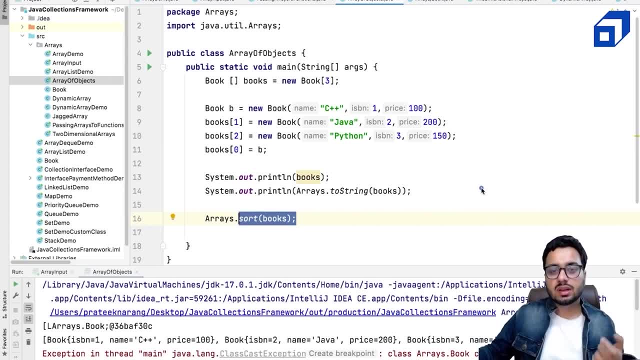 There are three ways that I have discussed in my previous video in which I have discussed Java collections. One is using compareTo method, One is using comparator and one is using lambda function. I will give you a quick Way to do it, which is using the lambda function in this video. by what I need to do. 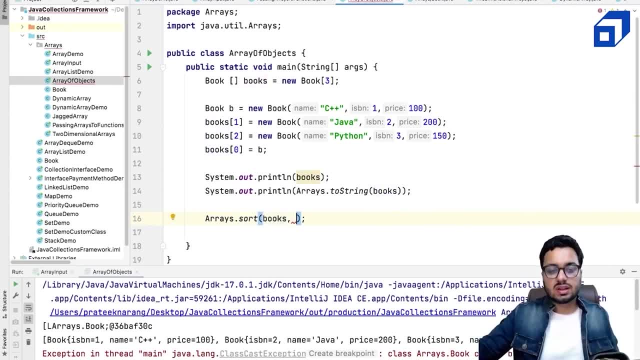 I need to define one line function in which I will say: okay, how do I compare two book objects, The two inputs, let's say book B1 and B2.. So they can be any two books. The sorting algorithm is going to pass book objects to this function, followed by an arrow. 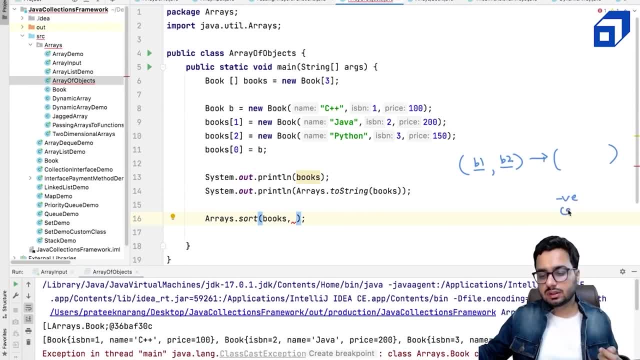 followed by: I should return a number which is negative, zero or positive. If I return a number That is negative, It simply means that my first book is smaller. Okay. and if I return a number that is positive, that means my first book is bigger, right. 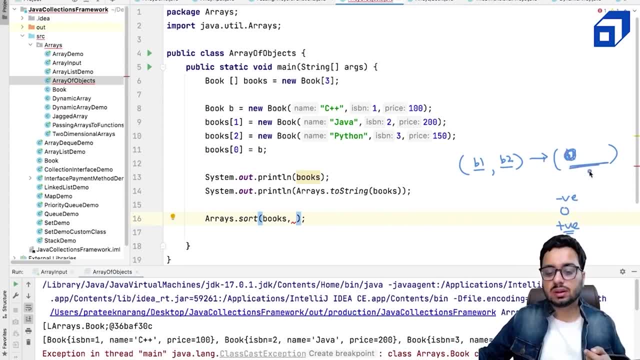 I need some way to convert these two books into the numeric values, For example. I want to sort these books according to their price. Let's say I'm comparing C++ and Java. If I return 100 minus 150.. What does it return? 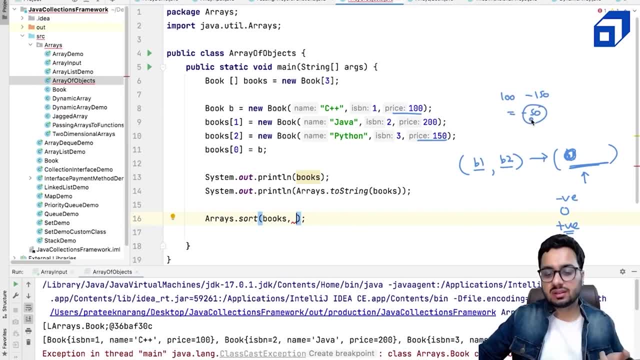 It returns a negative number. That means the C++ book is smaller than the Python book, something like that. Let me show you: if I say I want to compare two book objects, B1 and B2, and in return I will say that compare on the basis of their price, I will return a number: B1.price minus B2.price. 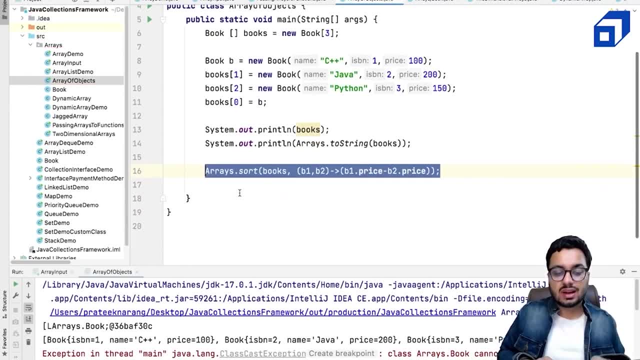 This is a shortcut way of writing a comparator right Using a lambda function. I'm comparing two books. If the first book prices, let's say, 50 and second book prices 100. This expression will return a negative number. That means the first book is smaller and hence it will be placed first in the list. 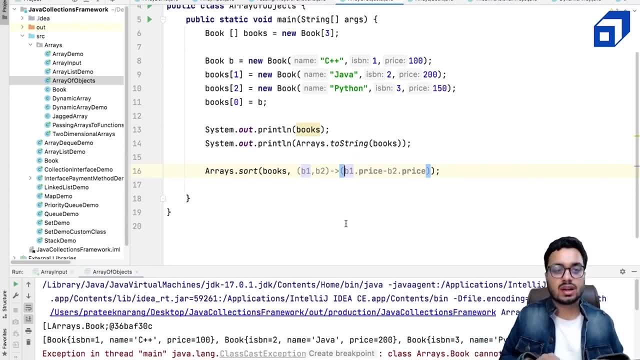 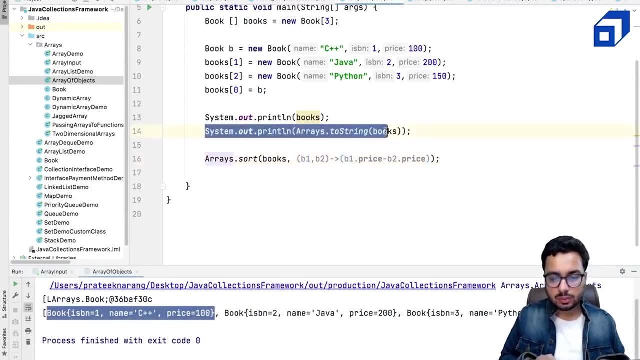 Let me go and run this and we will see what happens. I'm getting now the C++ book, followed by: Okay, I forgot to print this after sorting. before sorting, It is C++, Java and Python. Let us see what happens after doing the sorting, right. 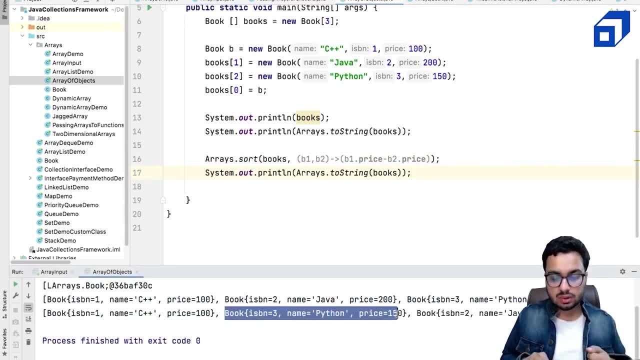 I'm getting C++- the least price, and I'm getting the Python book which is 150 price, And then I'm getting the Java book which is having a price of 200.. Okay, So I hope you're really understanding how we are doing the comparison and we can tell the sort function. 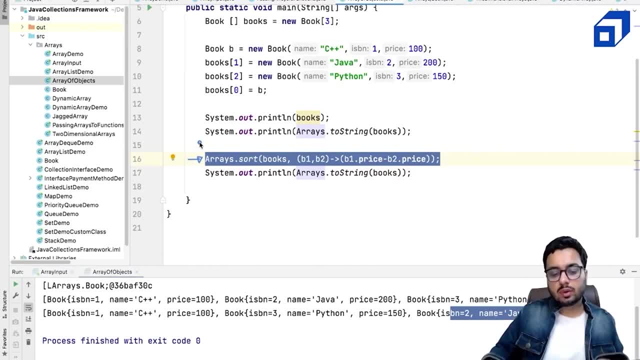 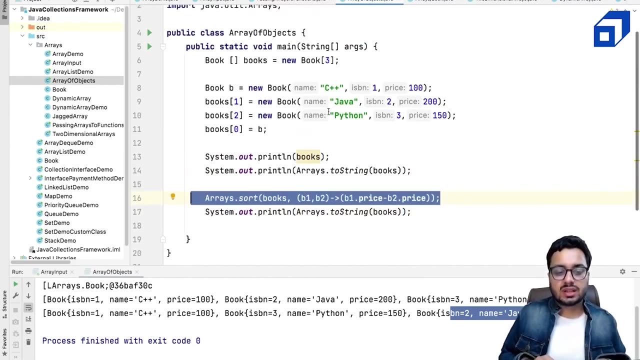 This is the parameter on which I want to do the sorting right. If you want to Write more complex comparisons, like multiple, if else conditions, then you have to go with the comparator way of uh comparing the two books. So that is how you work with array of objects. 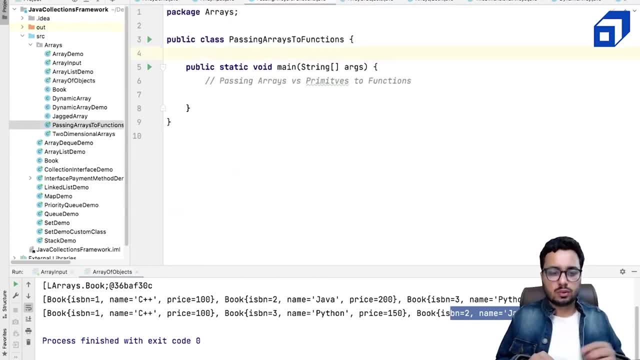 And, uh, I hope these concepts are clear. Let us move on to the next concept, That is, how do we pass errors to functions? What happens internally in the memory? So let us discuss this concept. For example, uh, let's say I have a variable called as uh, money, which is, let's say, I have a 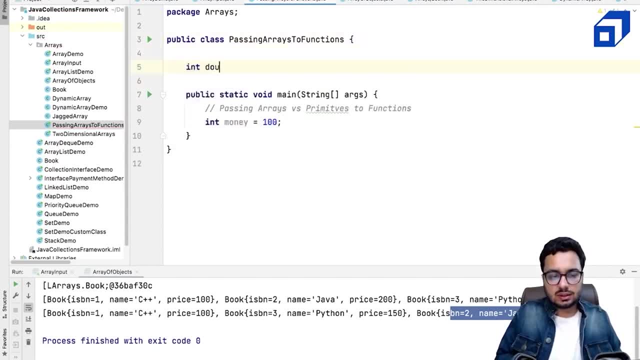 A hundred rupees. And let's say I have a function called as, uh, double money. So I said, okay, I will get some money and I want to double it So I can joke: money equals to price of money And uh, that's it. 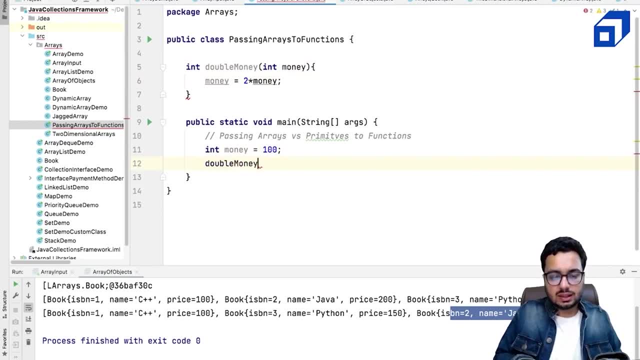 Now I call this method, I call the method called as double money, and I give it money And now I can say, okay, let me go, Let me call it as public void, I'm not going to return anything. Public, static void, double money. 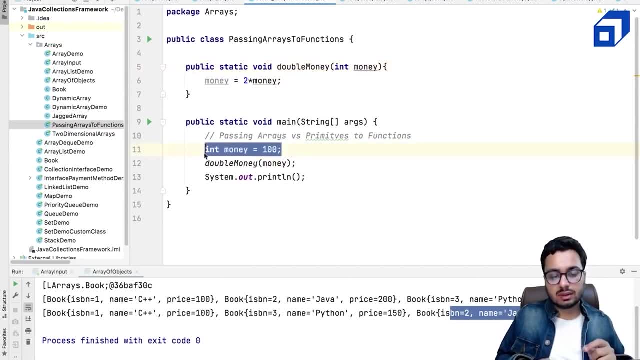 I've just, I have, I have a single variable right. So basically, what I'm trying to tell you is: I have this money variable. I pass it to a method called as double money, which should which people might think that it's going to double it. but let's see. what do we really get? 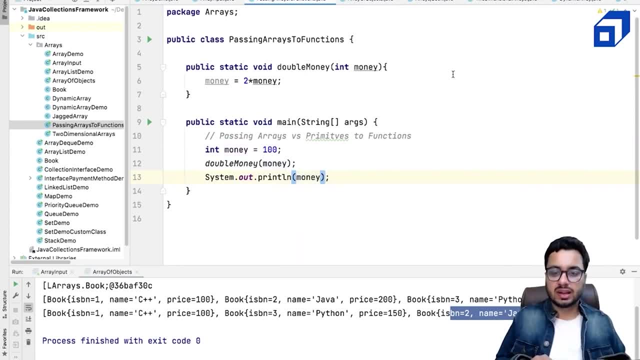 If I print money here, what do you think What output you can expect here? Let me go and run this code. The output will be still a hundred. The money is not going to change, I'm still getting a hundred. So let us understand what is happening behind the scenes. 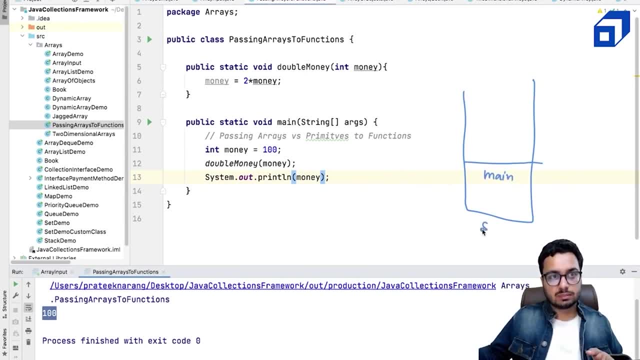 This main function created in your stock memory is your stock memory And there is a variable called as money And when you make a function call, another function is called that is your double money And in this function you have another variable called as money. 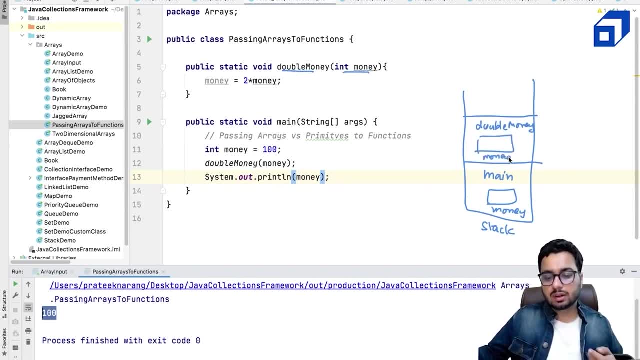 It exists in a different scope, It in a different part of the memory. this money was a hundred. So when you call this function, this money is getting copied here right. Copy right. Pass by value the value that is here. it is getting passed here. 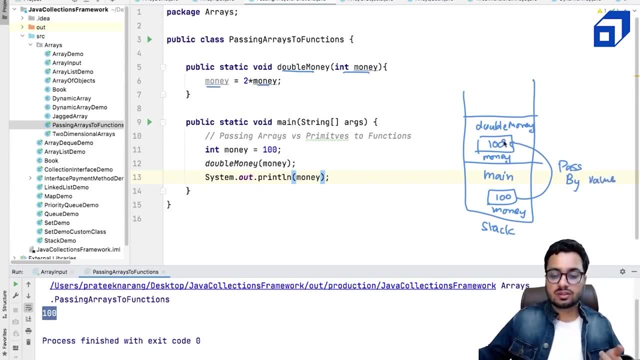 We are passing this value a hundred, and here you say money equal to twice of money. You say, okay, I'll make it double, I will make it 200.. Now this function call is over. It does not return anything, This stack frame is destroyed and you are back here. 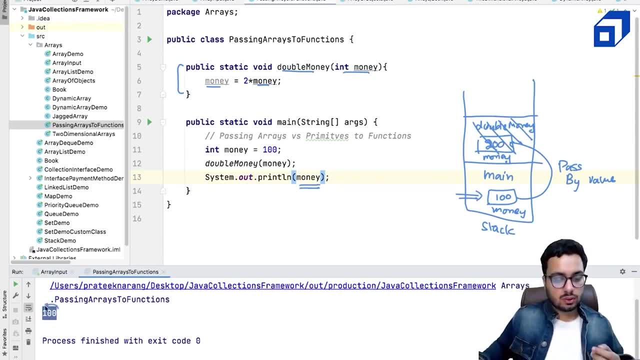 Oh, when you print this money, What you're going to get? you're going to get the stand. Let us repeat this experiment in in in a case. instead of having one variable, let's have a array object. So I said, okay, I have multiple friends and they have some money. 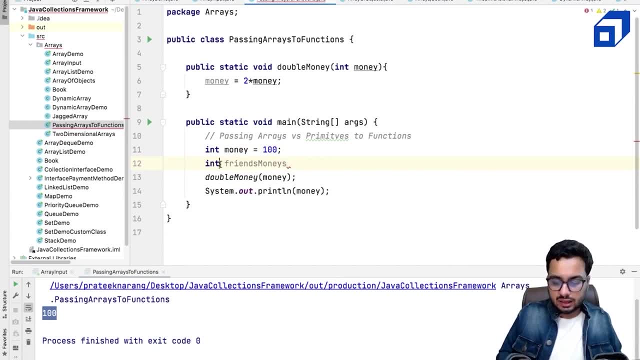 It's why I say friends money. It's a integer array And let's say, a friend has 200 and 300.. And I ate One more function called double money, which is going to accept money or friends money, whatever you want to call it. 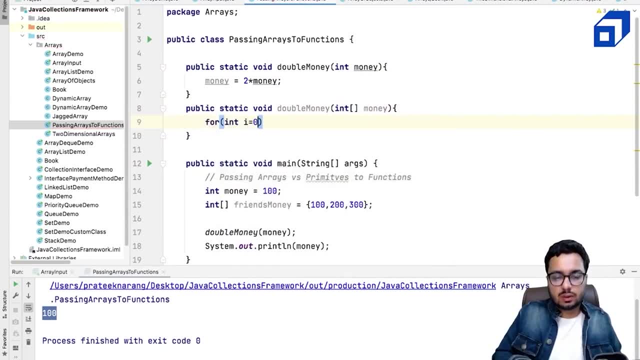 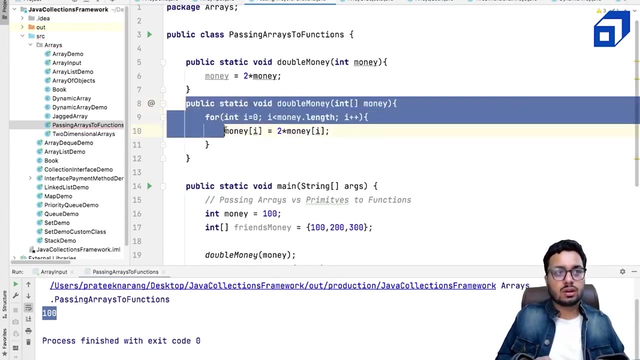 In this case I, I treat over this area or anti equal to zero. I list and money dot length, I plus, plus And I say money of I would be twice of money off, And again I do not do anything. 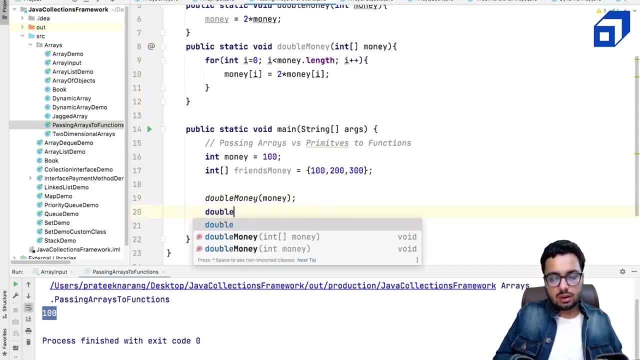 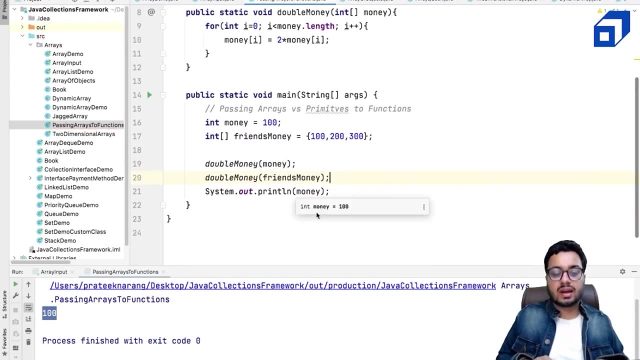 I do not return anything. Now I again call this function, I call double money and I give friends money, which is an array. Oh, what do you think? Well, my aggregate doubled. Will my money in this area? will it get doubled? 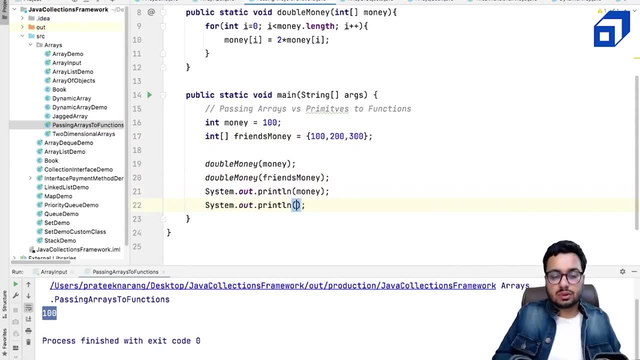 The answer is yes, it will. Let us see how and why it's going to happen. So if I print friends money and if I show you the output now, okay, I have to use the method Arrays dot two string So that I can actually 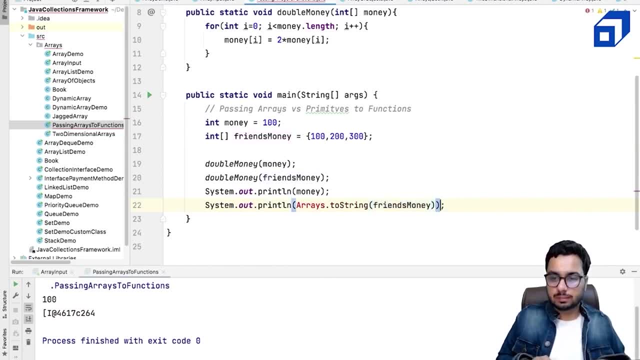 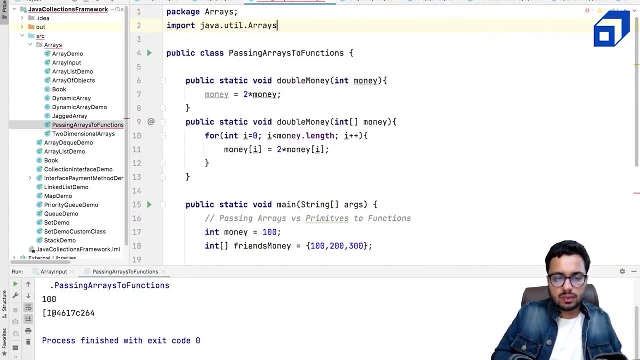 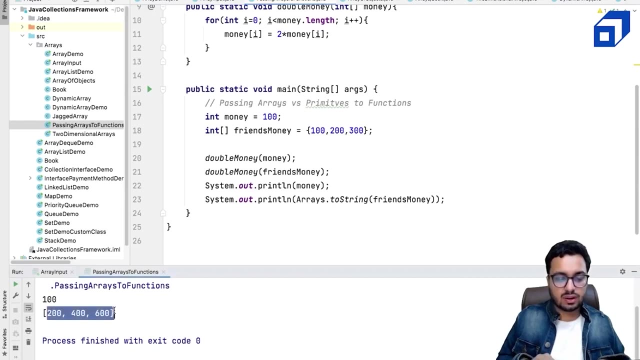 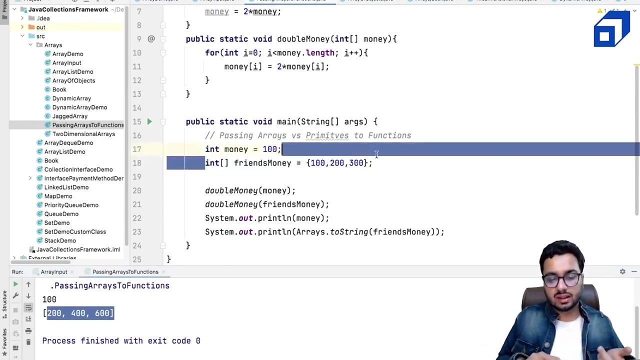 Print the contents of the array. Oh, oh, Dawa dot You did. Now this money is actually getting 200, 400.. You might think it is not doubling for the primitive data type, but it is doubling for the array primitive behind the scenes. 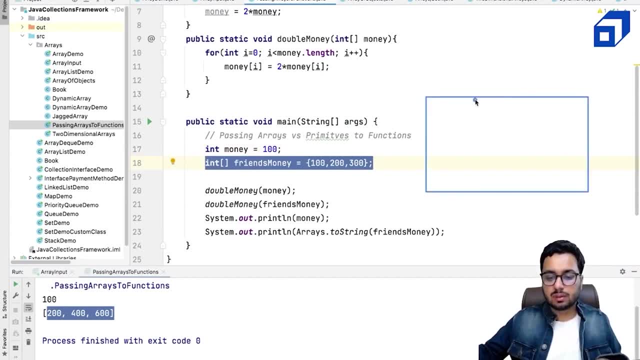 What is happening We have already seen. Let us see what is happening when you are Passing an array, So you have your stock memory. I told you the array is created in the heap memory: your hundred, 200 and 300. 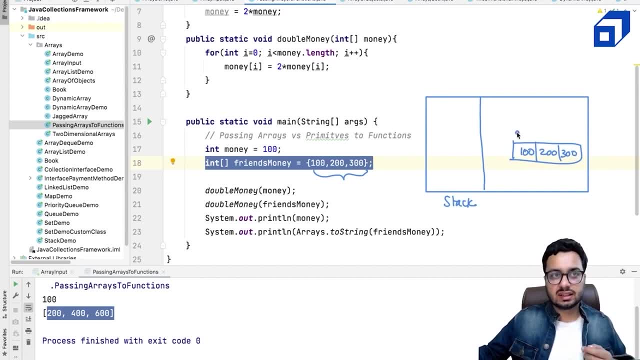 They are created here and they have some address. Let's say, the address is uh five, 56.. This is the location at which the array is created. When you called your main function, it got created in the stock. your variable friends, money. 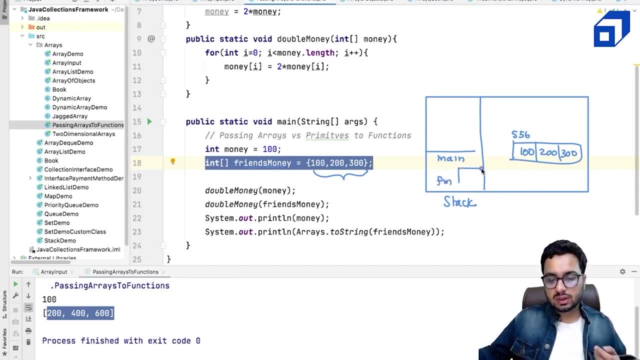 It is also created here. What does this variable holding? It is holding the address of the array. It is holding Five, five, six. Now when you call this function double money, you're passing the variable, the object reference, friends, money- to it. 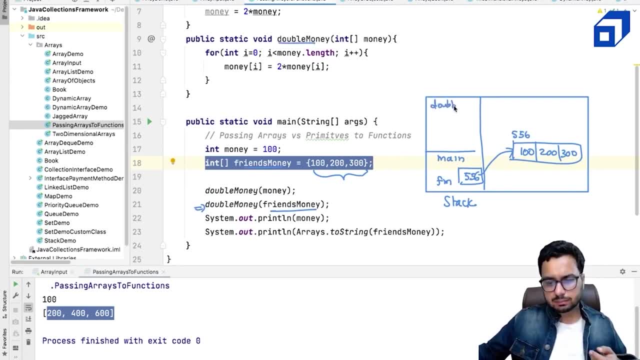 Okay, So we are calling this function double money and it has a variable called as money, in which what is the value that is getting copied? It is not the area that is getting corporate, It is the value inside this function: variable friends, money. 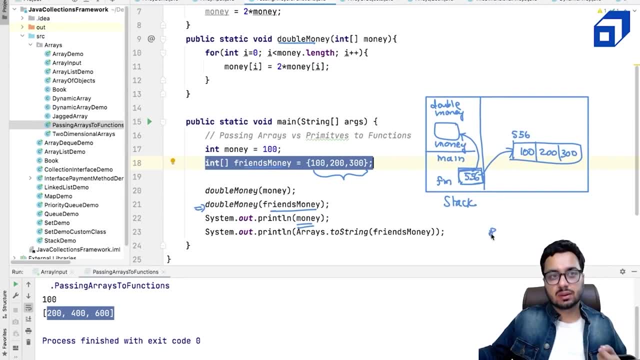 It is getting corporate right. In Java, Everything Is passed by value. Okay, But in case of area, what is the value that is getting passed? It is not the area object, It is the address that is getting passed. You have five, five, six getting copied here. 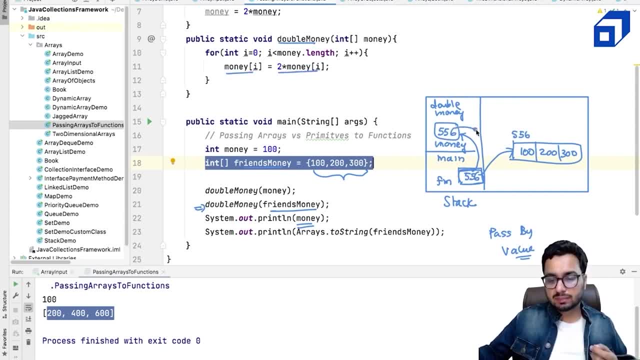 When you say okay money, I equal to twice of money, So this money is also referring to the same area. When you access the location using this address, you eventually end up here. It's okay Money of. I should be twice of money. 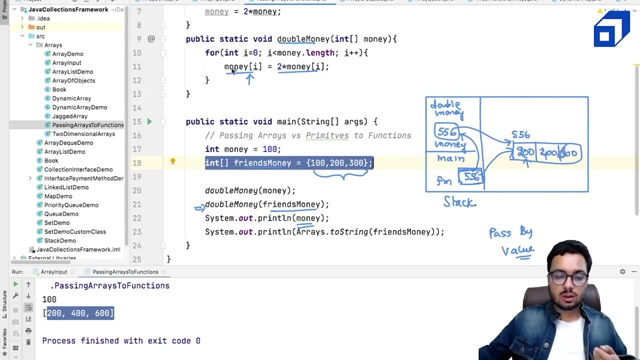 You make it double, make it 400.. You make it 600. Now this function is over. This is uh. this call is gone. This link is also gone, And when you come back again here and you try to access the friend's money array, the actual array has been changed, right. 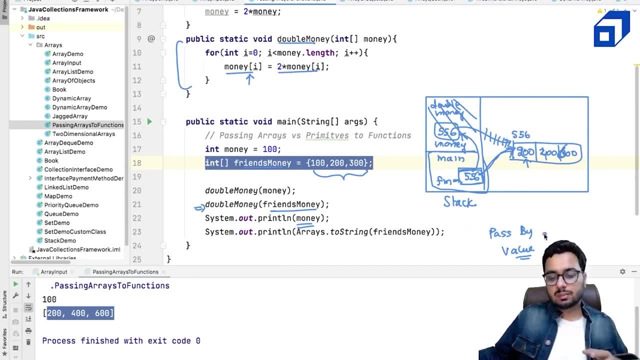 Okay, So although it appears like a pass by reference, but the concept is still called as pass by value in Java. Okay, But for the objects that are stored in the heap, okay, Objects in the heap. when you pass them to a function, their address is being passed. 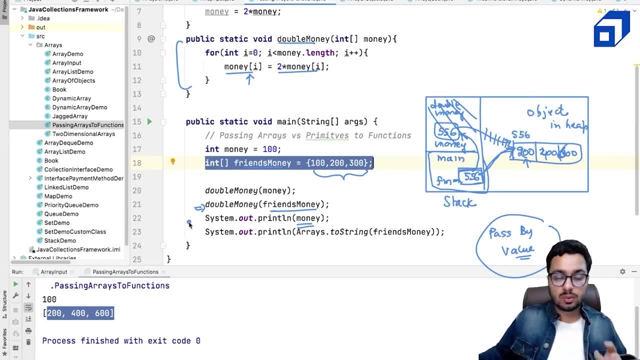 Okay, That is something that you should know, And now I hope you're able to understand what happens. when you pass an area to a function, you change the array. the actual array will get changed If, if you want to create a copy of the array, you have to use some methods like loan or what right. 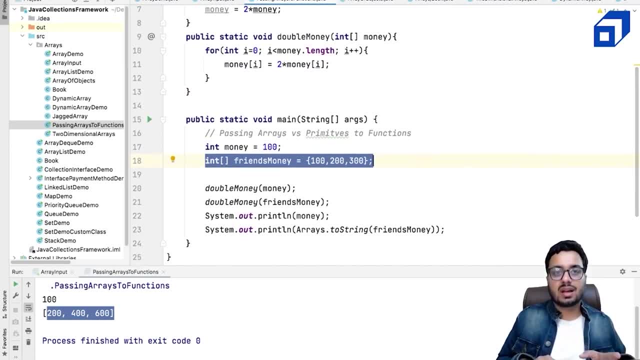 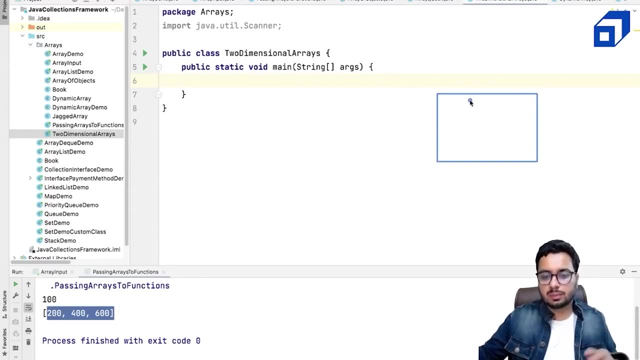 So that is how it is that passed to a function. Now let us move on to two dimensional areas. Okay, So many real life problems, for example, games and puzzles like tic-tac-toe. Yeah, My trick. I will require you to store data in the form form of a 2d matrix. 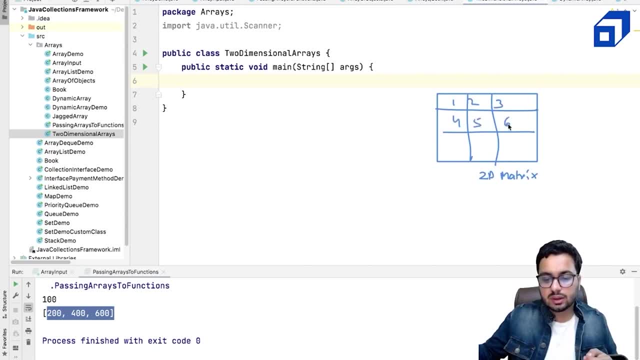 Now, if you want to store data in the form of a 2d matrix, you need a two dimensional array, right? You can also have a three dimensional, four dimensional and dimensional array, right? How do we create such an area? 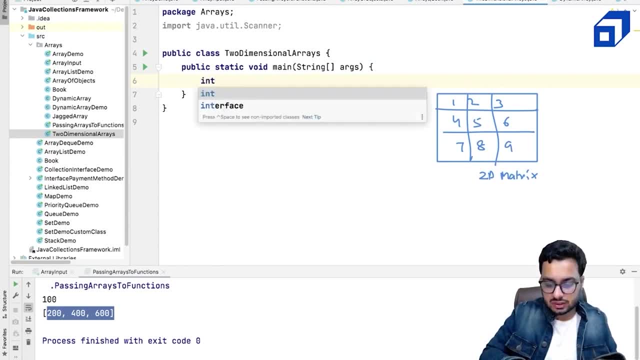 I'll show you a few ways to create these kinds of areas. The first: I need to define the data type, And in this case it's a 2d area, So I will have to use these square brackets two times. I'll tell you the reason why. 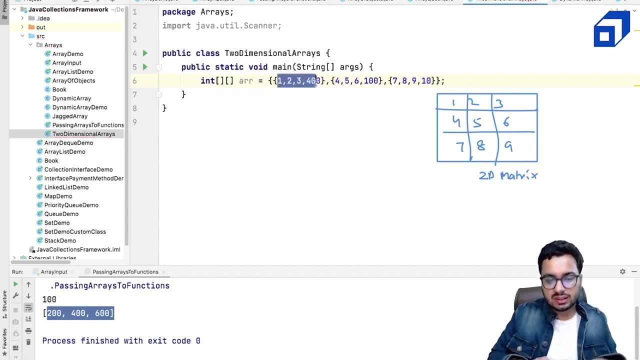 Then one way is I can directly give that Data right Now. if you look at this area, it has three rows and four columns. It is like one, two, three and 400.. This is like one object and I have four, five, six and a hundred. 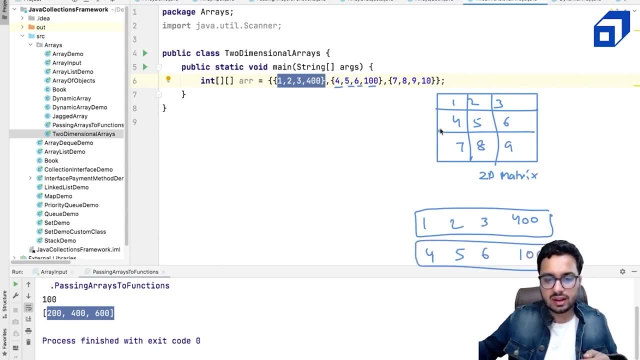 This is like another object. And then I have seven, eight, nine and a hundred. seven, eight, nine and a hundred, This is like another one. Now how they are stored internally. The memory, let us just put: Java 2d array is nothing, but it's a one day. 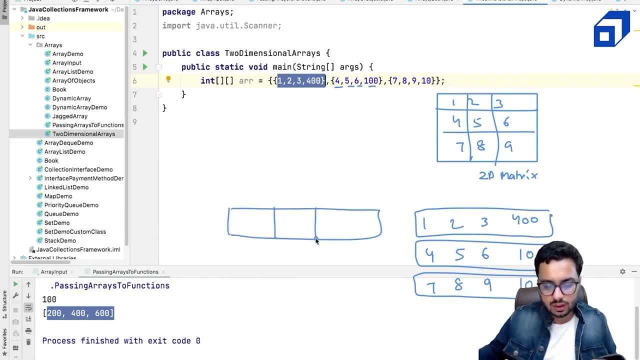 And in which each, each row or each, uh, each row is like one object, right? So can I say it's a one day of objects, where each object itself is a one dimension in the memory. There is no 2d Eric rated internally. 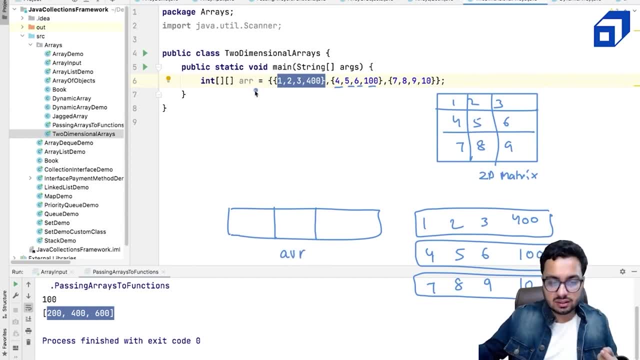 It's going to use a one day where I can say the zero: throw this. this element is my area of zero. area of zero itself is an area. That is what I'm trying to tell here. Array of zero is of the type int- square brackets. 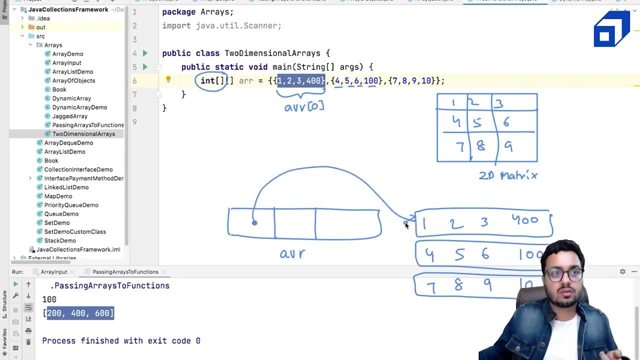 That means array of zero represents one day array. Array of zero is going to hold the address of another one day. Let's say this address is some, something. that address will be present here. I say area of one that is also going to hold the address of another area and area of two. 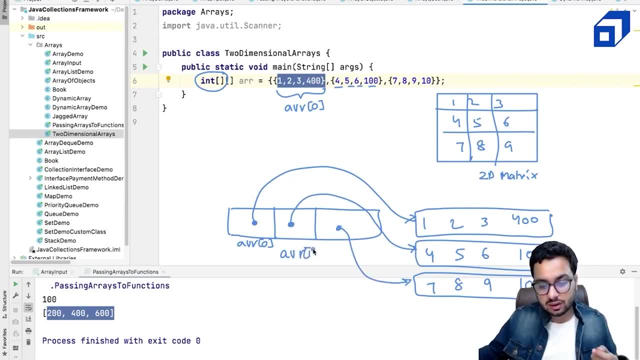 It's also going to hold the address of another. This is area of fun And this is exactly how It is stored right. And where is your era? era is here, this variable? it is in the stack memory and these areas, these four areas here in the okay, this, I'm saying this is an object, a 2d array is nothing, but it's a one day of object, one day array of objects, where each object is also an area. 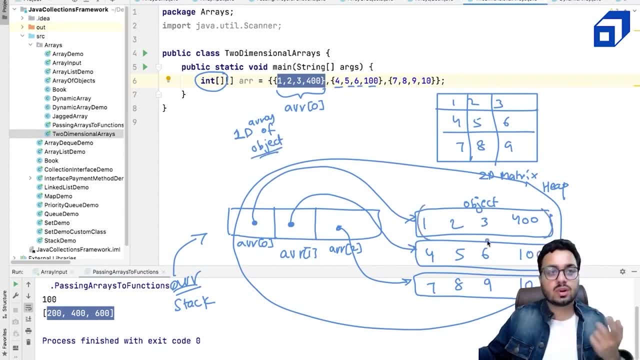 This treated like this way, right. So treated like this is one book. This is another book. This is another book, right? Each row is one object. Now you might say, okay, prove me, This is how it is. So let us go and do a south. 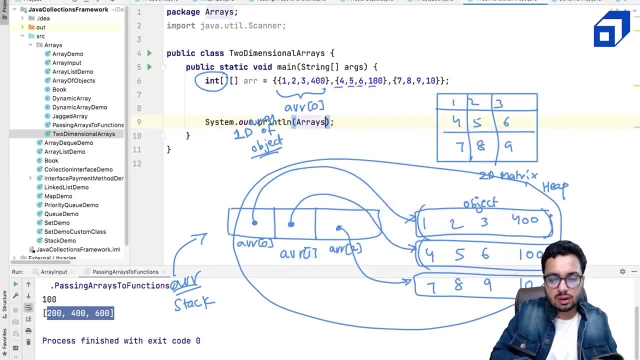 Let me show you. I can say it is taught to string. I want to print this array. I give era And again I will import Java Utah Dill dot. If I make this import and I call this method, it is taught to string. 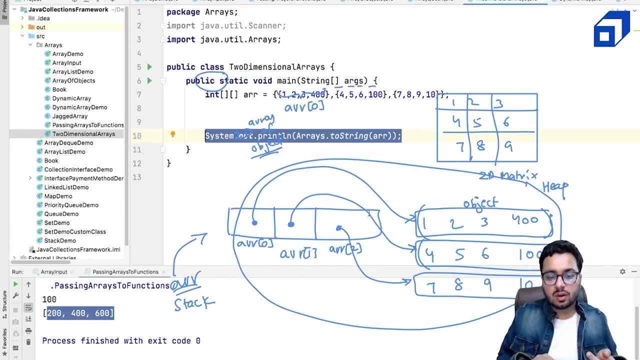 Now what I'm hoping to get. will I get the contents of the array or will I get these addresses? Let us see What do we really get. I need to run this. Look at this. I'm getting three addresses. What are these three addresses? 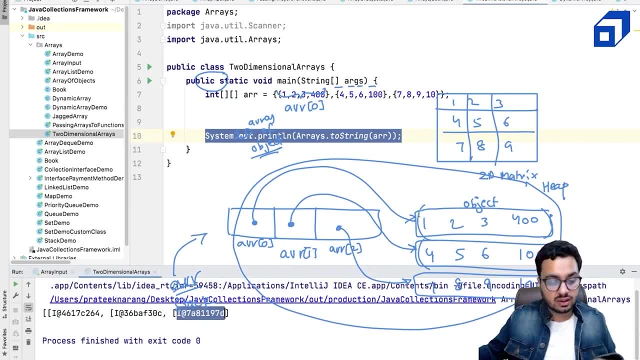 These are the three addresses of these three row objects that we have created. This is 264.. This is stored here. This is a TC. This is this is the address 30 C and this is one nine seven. one one nine seven. 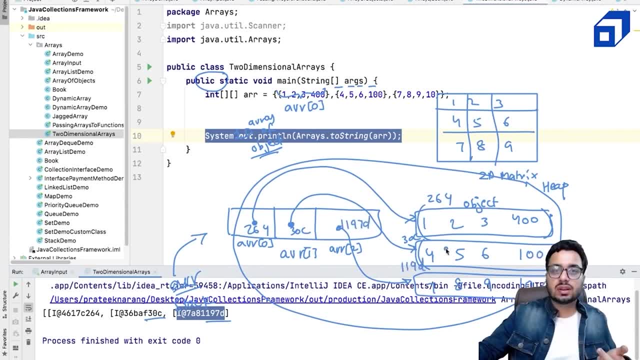 This is the address of enough. And you might ask: okay, if I want to print a 2d array using a true two string method, can I do that, Or should I iterate over this area? I will tell you you can do both. 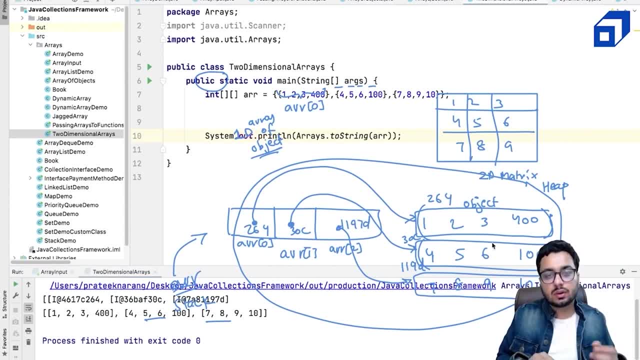 You can use an inbuilt method to print this entire array. You can also iterate over this area. Let us first look at an inbuilt method. If, if you have a structure like this, So you have to, you just don't need to iterate over these values, but instead you need to. 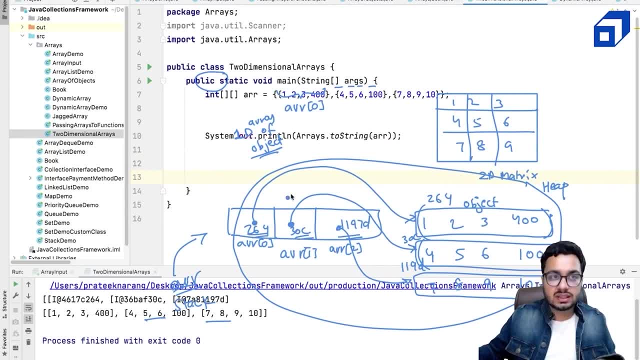 say okay, I also need to iterate the objects they're referring to it. So basically it's kind of a recursive structure, right? So this is referring to some object. This might also be referring to some some other object, right? 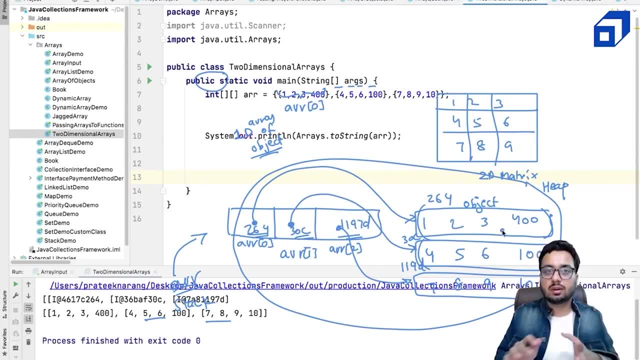 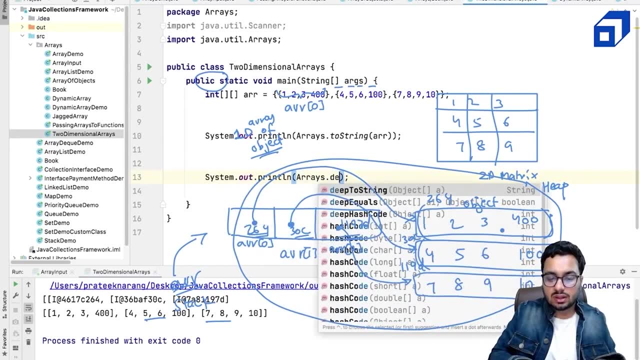 I want to go deep inside this structure and iterate over all the values, right? In order to do an iteration like this, what I have to do? I have to use a method called arrays dot deep two string. I iterate deeply inside these structures and then print this array. 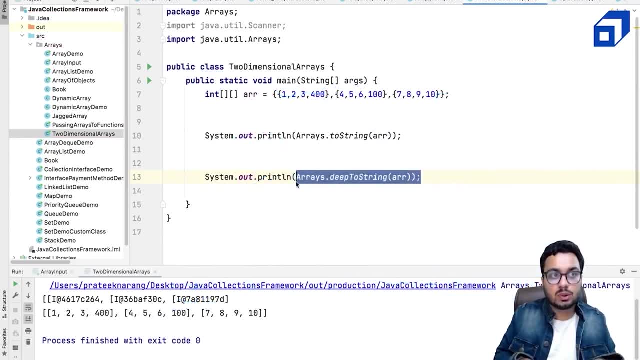 I call this method right: Arrays dot deep two string. What will happen? It will go inside those arrays, those rows as well, and it will print them right. If I go and run this code, you can see this is the output that I'm getting right. 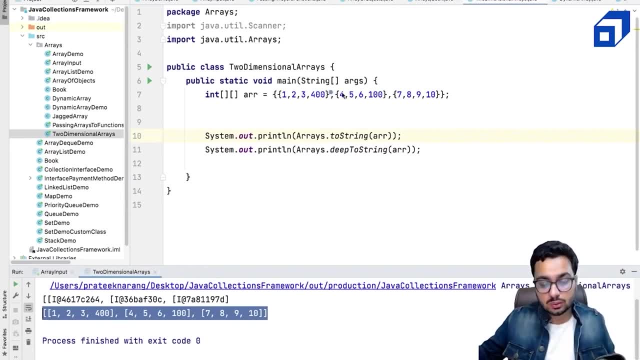 I hope you are able to understand the difference. You know how this 2d array is stored. Just a quick recap: This array- This error- is a 1d array which is holding three rows in it, Three rows Each row is a 1d array object containing four numbers. 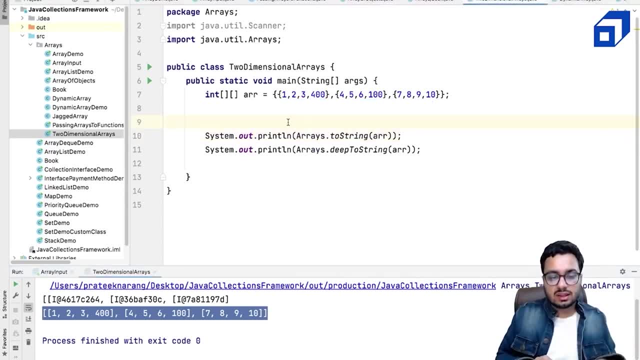 So now let us do one more thing. Let us write a method called as print that is going to iterate on this 2d array. Sometimes we have to manually use a for loop to iterate over a 2d array. Let's see how we can do it. 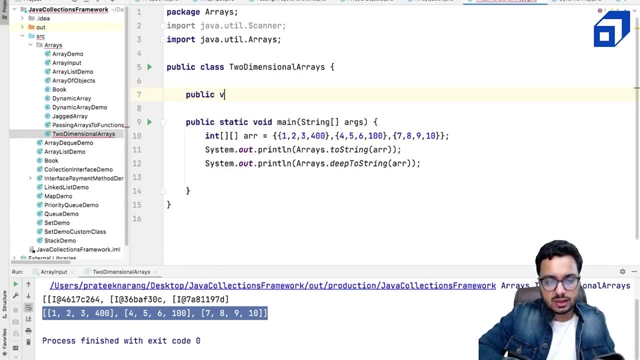 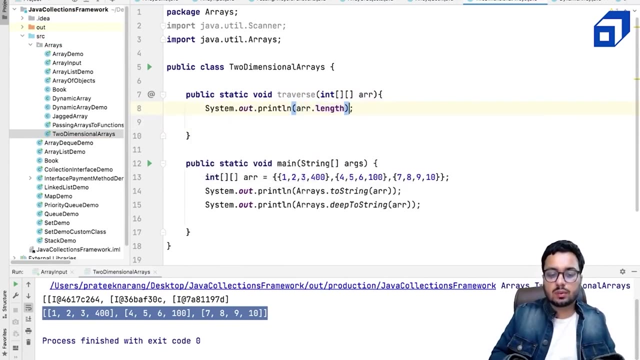 So public Public void, Public static void. It's a traverse, Input is a 2d array, So I'll create a reference variable, ARR. How do I iterate? If I simply say sout error dot length, Can you guess what is this length going to be? 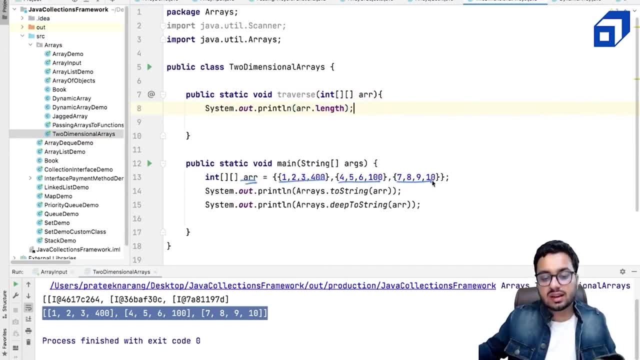 What is the length of this array? This array is holding three items. This length is giving me the number of rows I have. If you want to figure out how many rows I have in this array, these are the number of rows, How many columns I have in this. 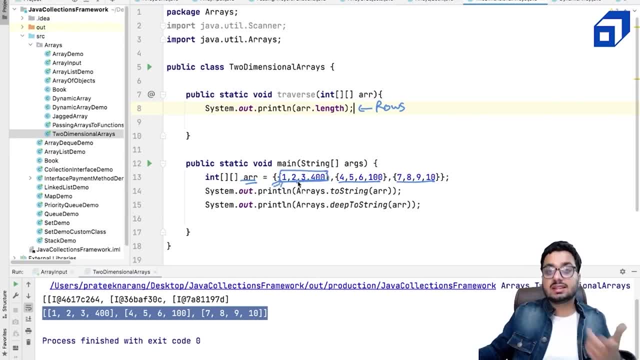 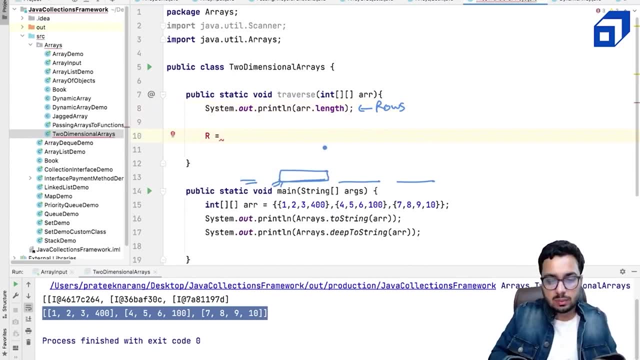 That is nothing but the number of elements in each array is the number of columns. So I can say: if it is a fixed size array, rows cross columns. Rows will be nothing but array dot length. How many columns I will have? That is nothing but array of 0 dot length. 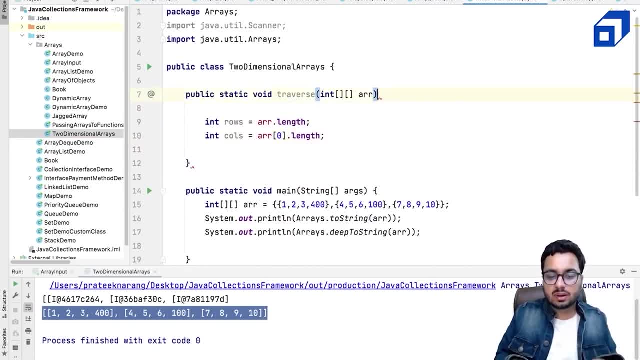 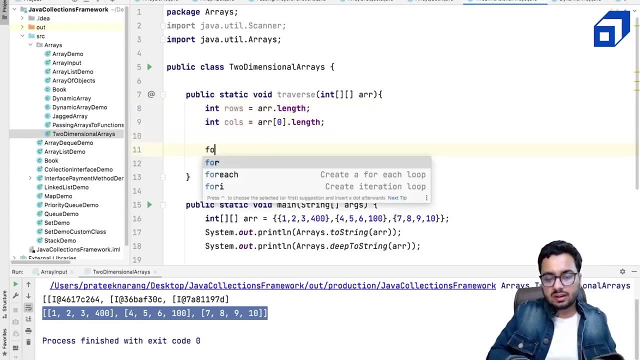 The number of elements in the first array. If this is same across all the arrays, The number of columns I don't write. How do I iterate? Iteration is pretty easy. I can say: I equal to 0.. I less than the number of rows. 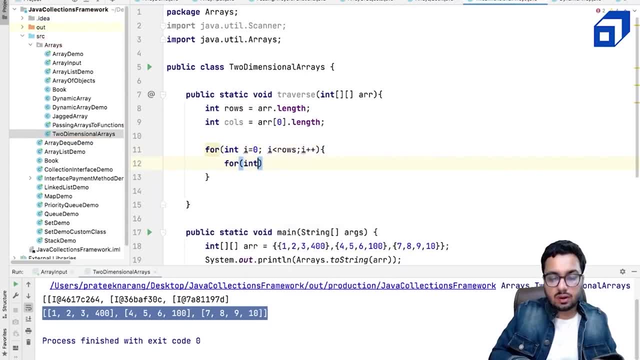 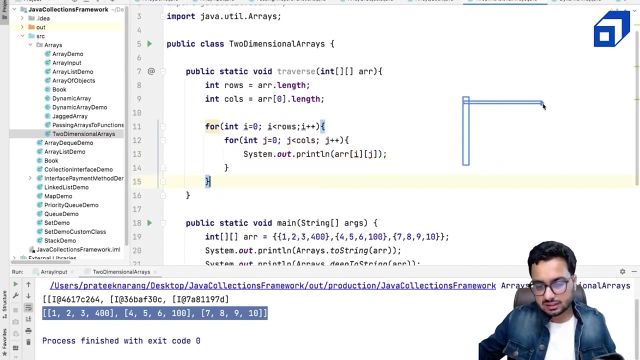 I plus plus, And then I can say, okay for j equal to 0.. j less than the number of columns, j plus plus sout array of ij. So let's see what does it really mean? So if I have an array like this, 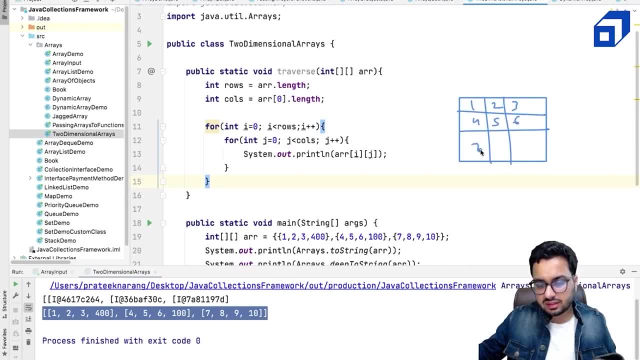 Let's say 1,, 2,, 3,, 4,, 5,, 6,, 7,, 8, 9.. This is one object. Another object. This is another object. Array of 0.. If I iterate over rows, 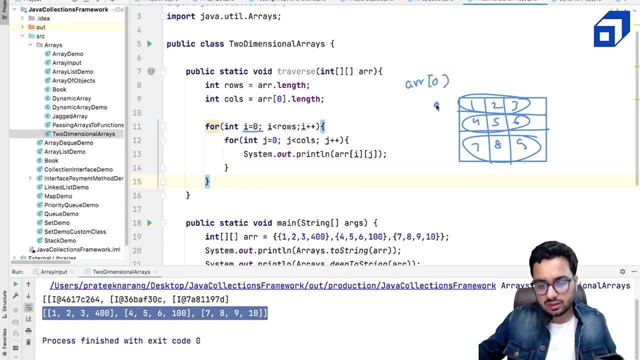 i is 0.. So array of 0 is fixed If I go over 0,, 1,, 2.. These are the row numbers. For each row number I say okay. I iterate over the columns. Array of i gives me this: 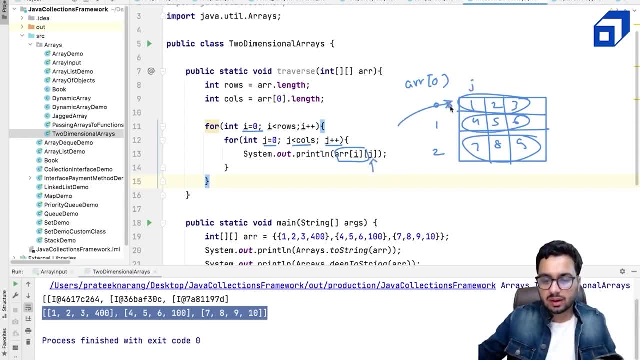 Then, using this, j gives me the column. So array of 0, 0 gives me 1.. Array of 0, 1 gives me 2.. Array of 0, 2 gives me this number. So j is going along this direction. 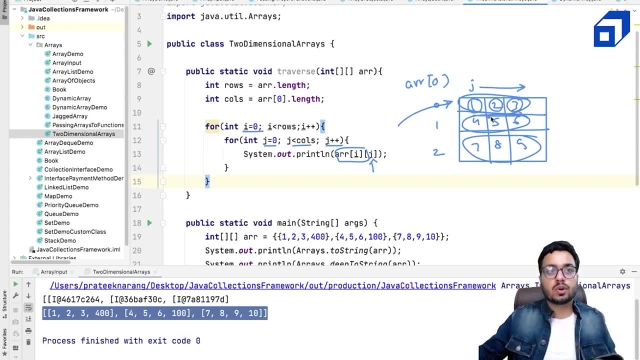 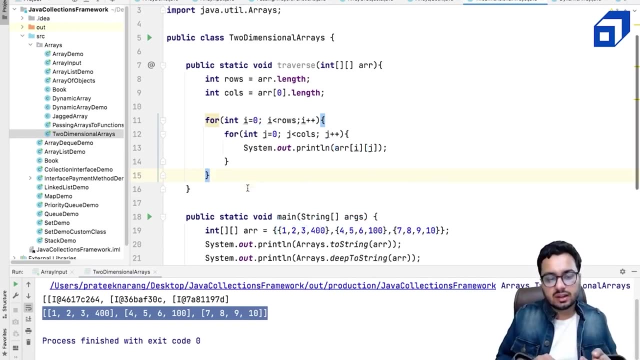 i is changing across rows. So what I am doing, I am going over each ith object And then I am using a j to traverse the elements of that particular row. This is how we generally do the traversal. You can also do it other way round. 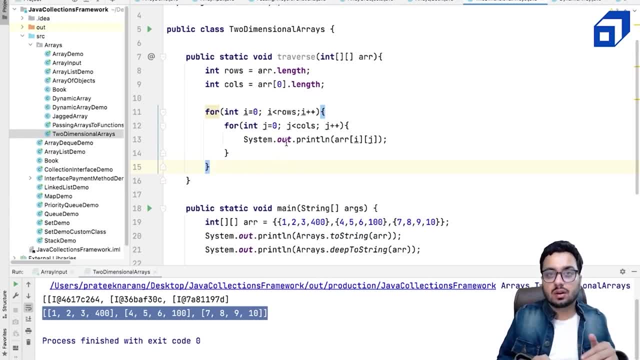 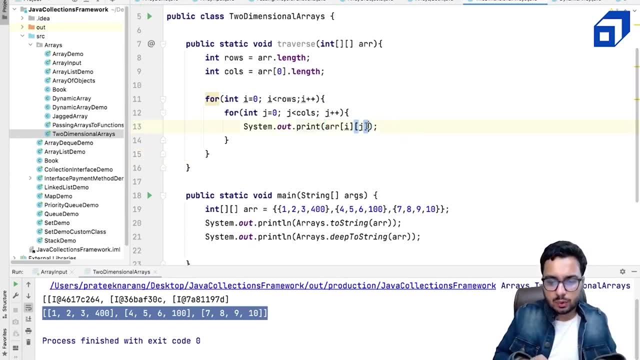 So I am iterating across the rows. You can also iterate across the columns By changing the order of these. If I show you the output, I am going to print them in the same line And after my row is finished, I am going to give a new line. 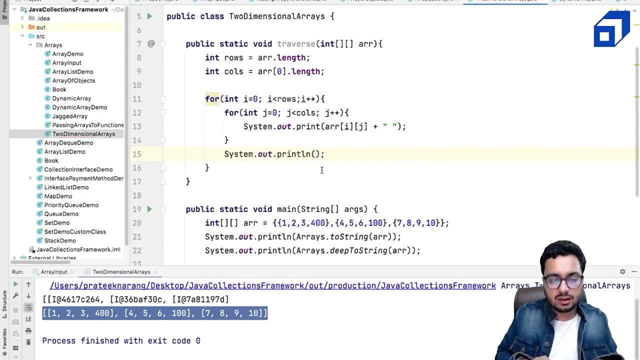 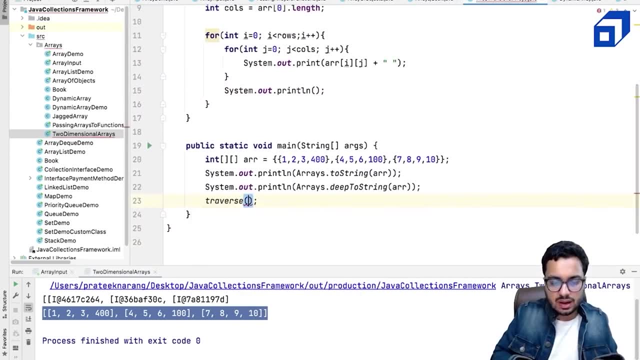 So I can say sout println. So now, if I call this method That is going to be traverse, And I give this array, I will see an output Which looks like a 2D array. Let us go and run this code. 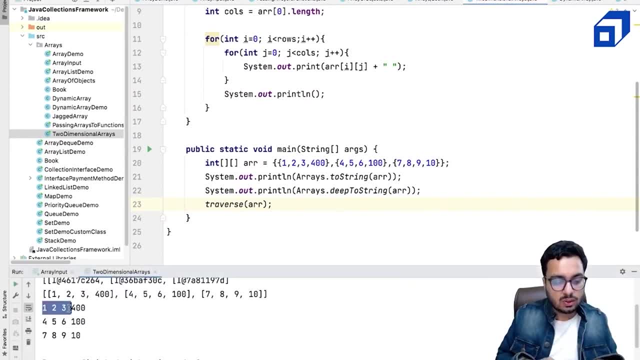 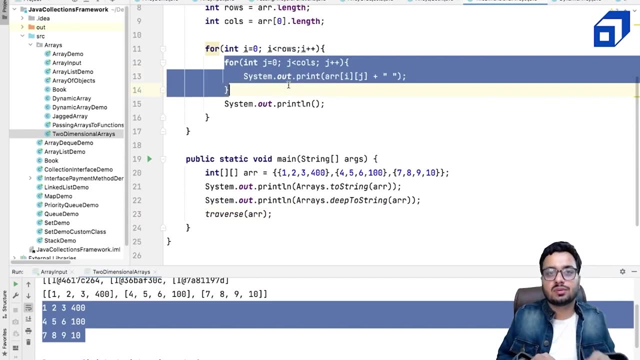 And you can see. So I am able to iterate over all the rows And for each row I am able to iterate over all the columns of that particular row Or all the numbers in that particular row. So I hope traversal is clear to you. 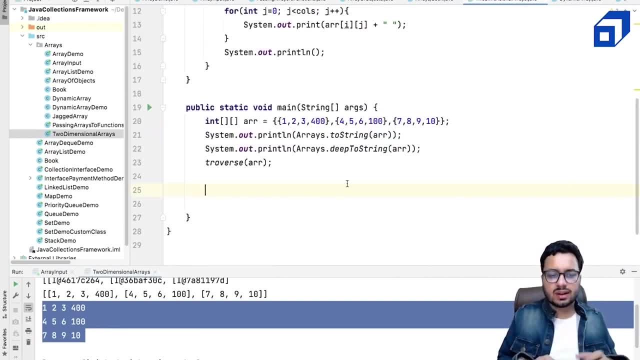 Now some of you might ask: Can we do some kind of sorting on this 2D array Maybe? I want to compare each row with some other row, So I want to do sorting across the rows. I want to sort rows And you might have a different criteria. 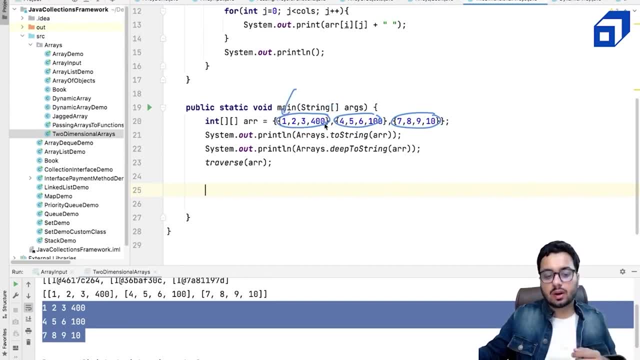 You might say I want to sort on the basis of first element, Or I might want to consider the sum of all elements. So how do I do that? So it is very easy. Consider each row as one object And I want to compare this with other objects. 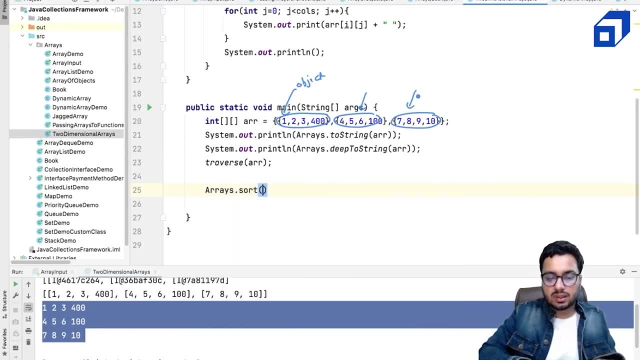 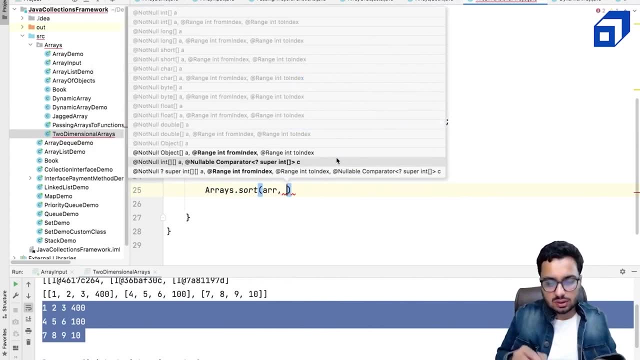 What I can do. I can use arrayssort method. It will assume that I am going to give you a 1D array. That is okay. So it is going to, And this is actually a 1D array. Okay, Although the syntax is 2D array. 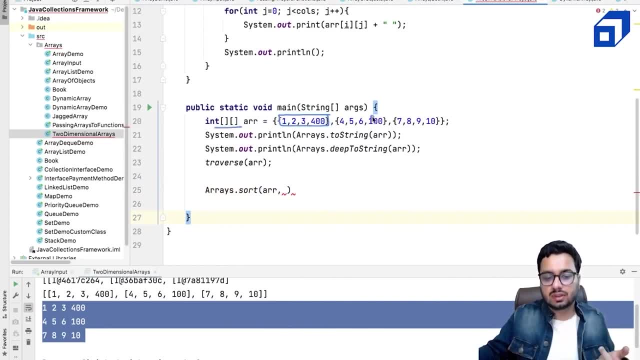 But java considers This as one element of the array, This as another element of the array And this as another element of the array. Suppose, if I want to sort according to their sum, What I have to do, I will give you two objects. 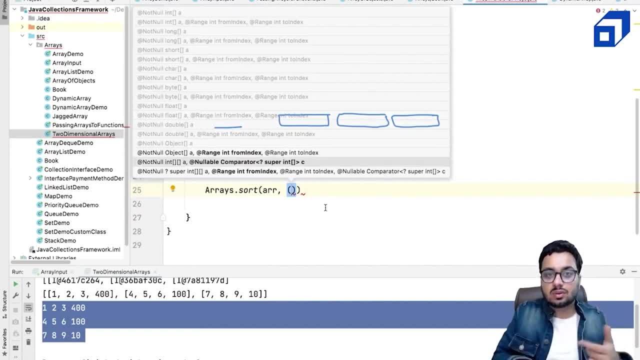 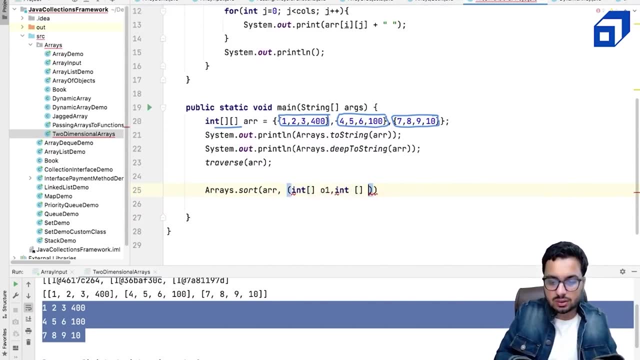 What are the data types of these two objects? These two objects are arrays. I have int. square brackets, object 1.. Int. square brackets, object 2.. And in return I want to Get their sum. So I can create some method called as getSum. 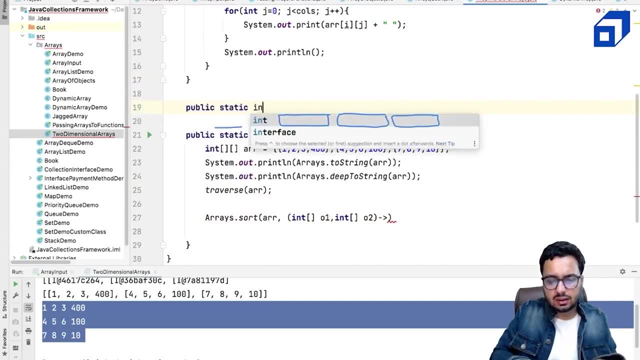 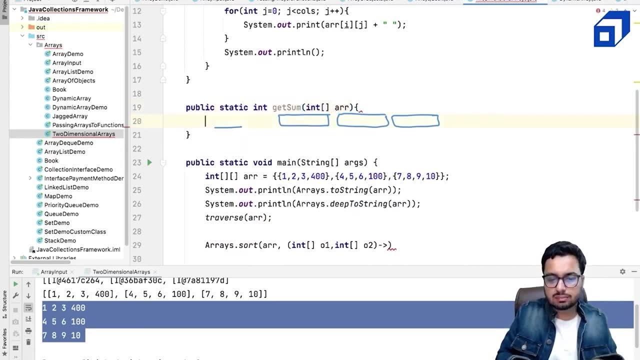 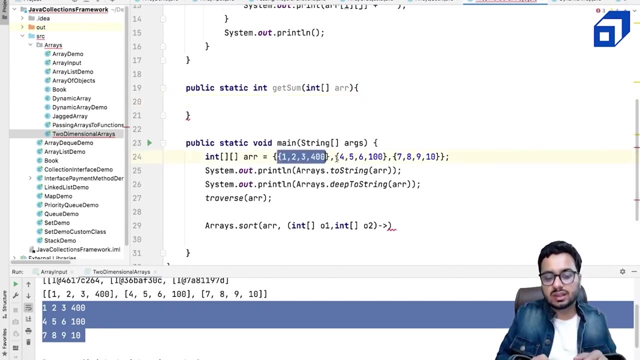 Int- public- static. int getSum. Given a 1D array, I want to find the sum of that array. I give sum array. I want to find the sum of that. I want to sort these rows according to their sum. So basically. 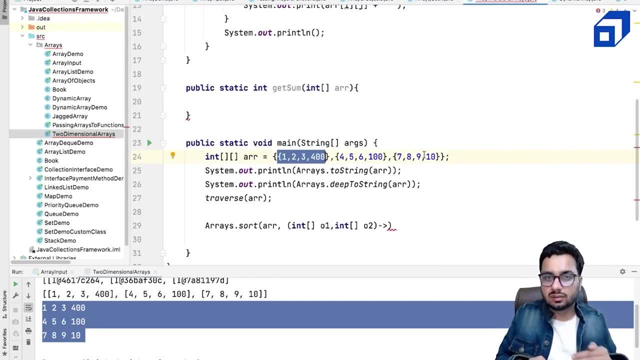 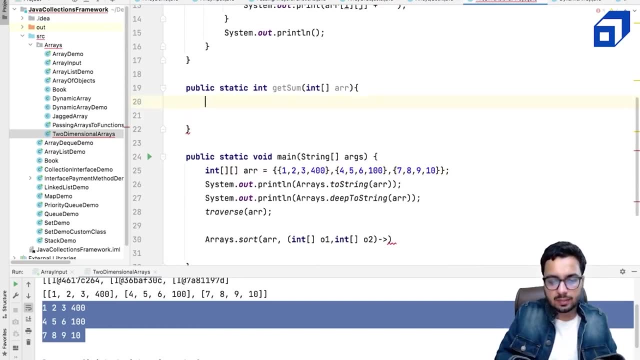 The row which has a higher sum should come at the end of this array. How do I do it? First, let's write a helper function To get the sum. For now I can say: Int sum equals to 0.. For Int value inside this array. 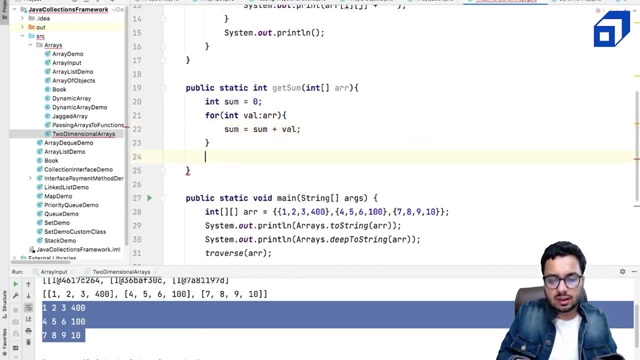 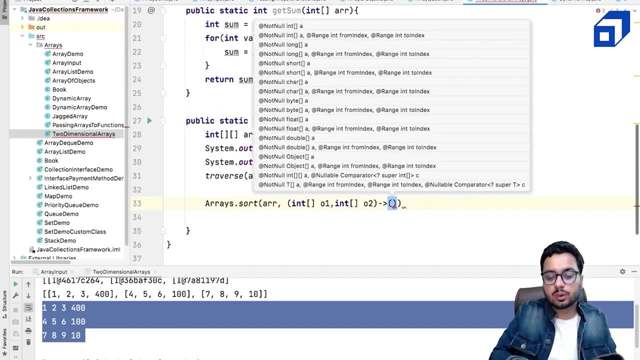 Making the sum equal to sum plus value, And I can return this. Finding the sum is pretty easy. Now, Here, in my lambda expression, I can say: okay, I am going to compare on the basis of Sum of These arrays. 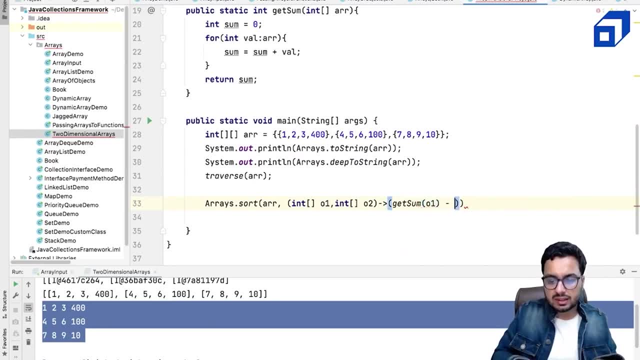 So array 1., Which is my object, 1. Minus Get sum of Array 2., Which is my Object, 2.. That's it. And if I do this- And now I want to show you the output- 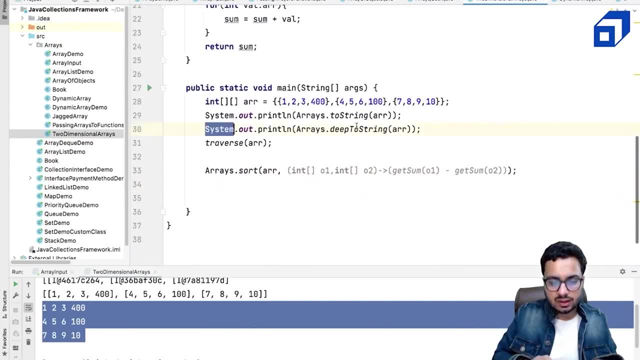 I can again Print this array After doing the sorting And let us see what do we Really get Now? if you look carefully, I am getting this array first, Which has the least sum. This array has A higher sum. 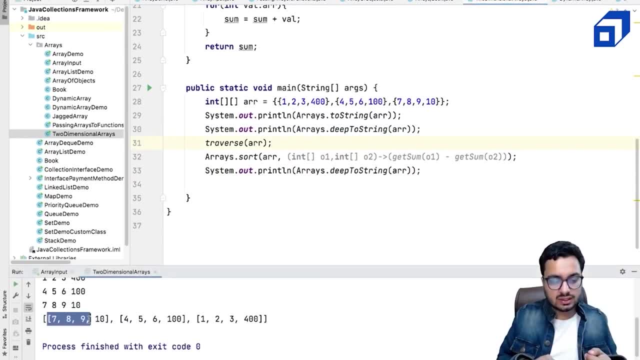 And this Array has Even the highest sum. Why? Because I am. I have a very big element, So I am getting This array first Which has the least sum. This array has A higher sum. I have a very big element. 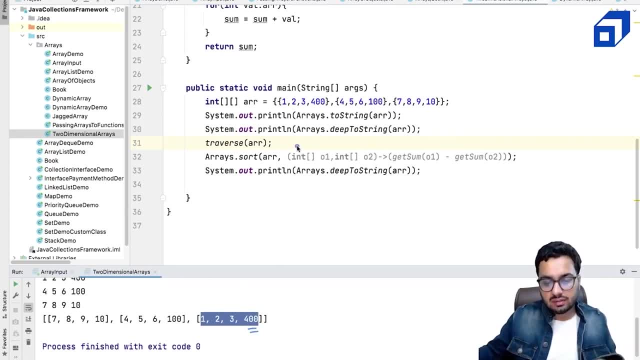 400.. You can verify So What I have done. I have written a Lambda function That is Comparing Two rows Any Like Internally. It will call Some logic To compare Two rows. 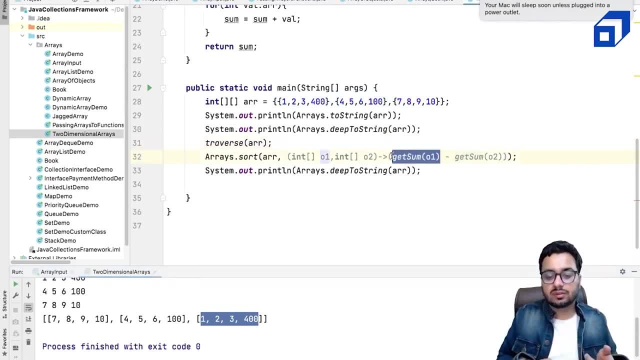 Okay, So it is comparing Two rows According to their sum. If you want to compare On the basis of First element Or the last element, That That. That can also be done If I Do this Okay. 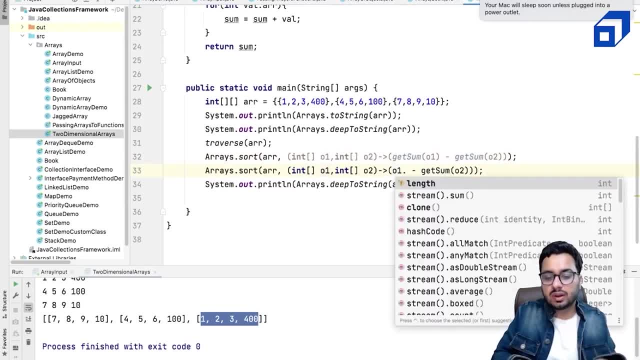 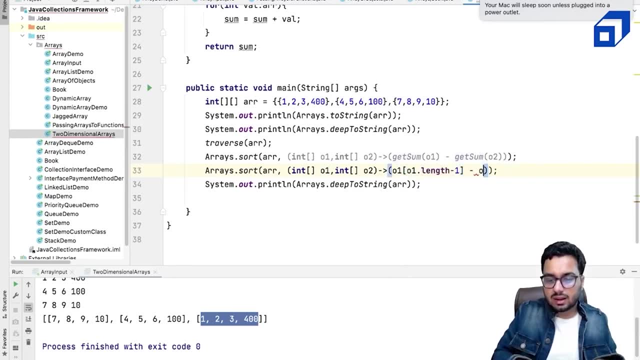 Oh, One Dot, Get Last element. How do I get it Into? Okay, Oh, One Dot And Minus One, That Is Giving Me The Last Element, And Or: 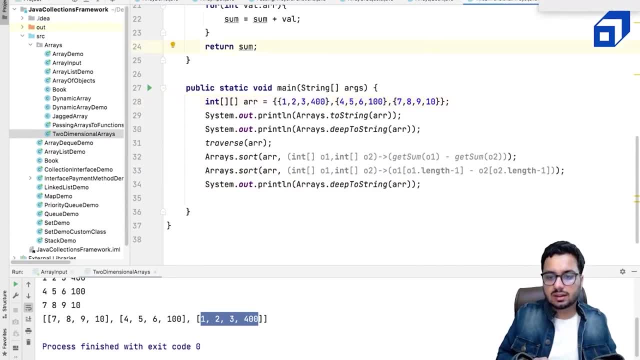 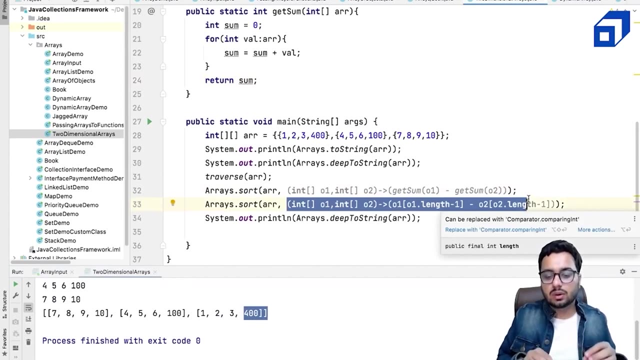 Two Of Or Two Dot. Okay, So I am Getting Ten, Hundred And Four Hundred. That Is How Powerful These Lambda Functions Are. They Can Also. 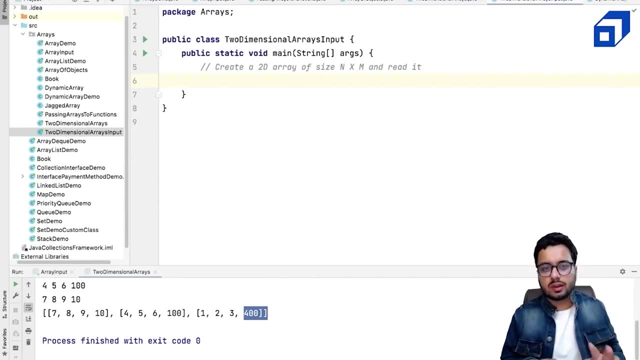 Work With 2D Arrays, But Now You Are Not Going To Do That As Well. First Of All, I'll Create A Scanner, So That. 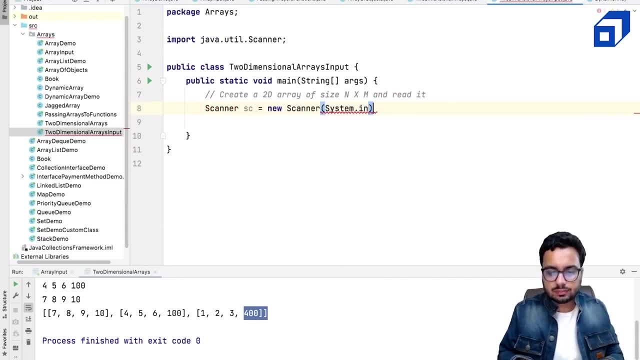 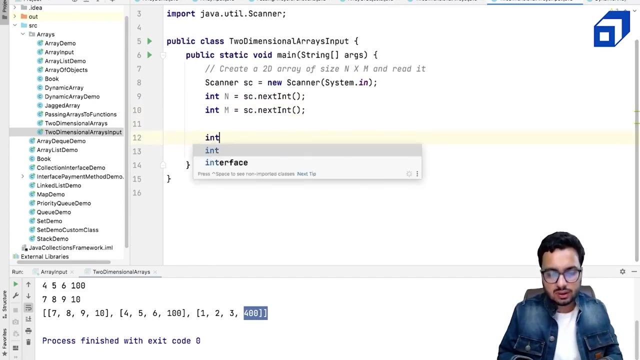 We Can Read Numbers From The User. So Scanner Sc. This Is Equal To Create A 2D Array Of Size And Cross M. How Do? 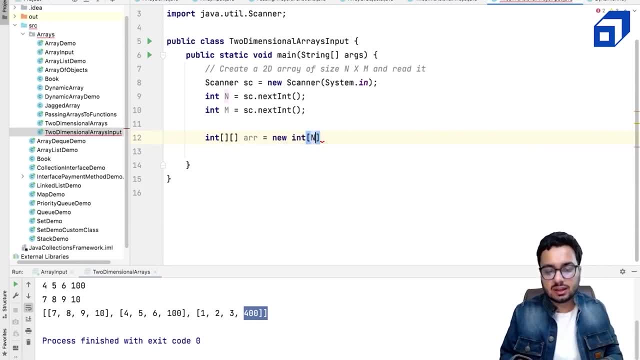 It Pretty Simple. I Define Variable Error Is Of The Type In: Square Bracket: Square Bracket. This Is How They Will Get Created. Now What I 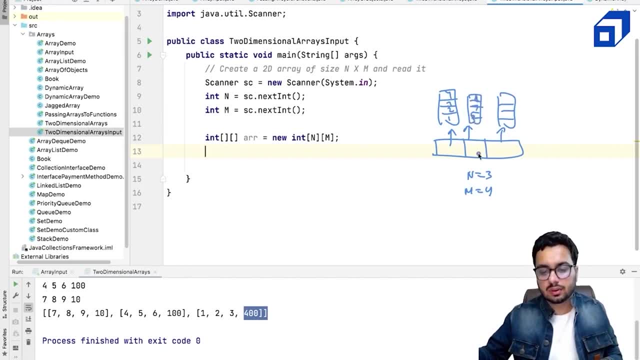 Want To Do? I Want To Read Numbers And Put Them Here. One, Two, Three Is The First Row, Five, Six, I Can Say For Int. 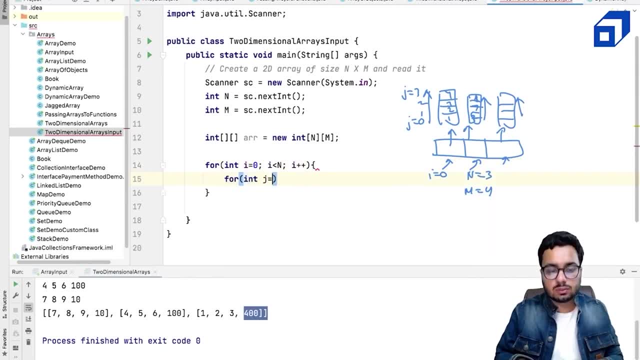 I Equal To Zero. I Less Than N. I Plus Plus. Then For Each Row I Need To Read The Elements Equal To Zero. This Is: 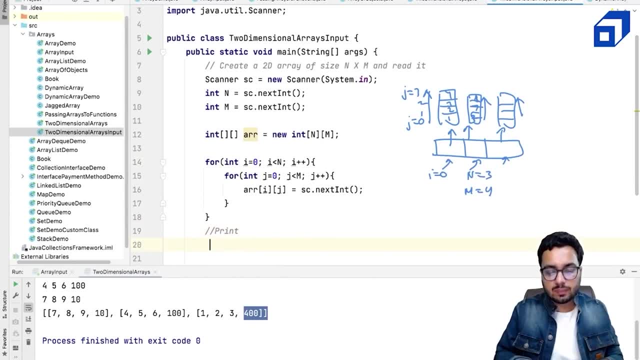 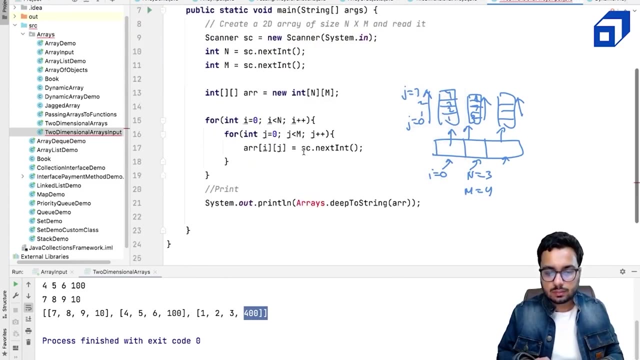 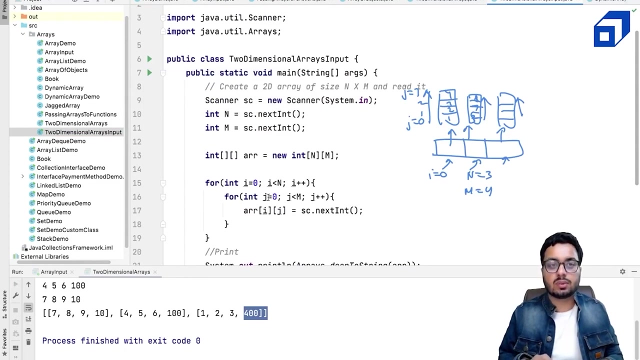 Done. I Have Read All The Elements And What I Need To Do. I Need To Print So I Can Say: Okay S Out, There Is. 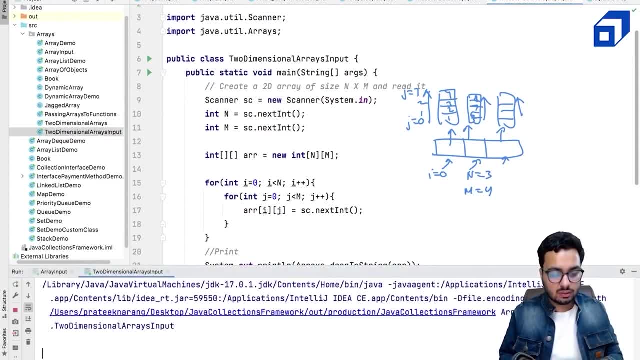 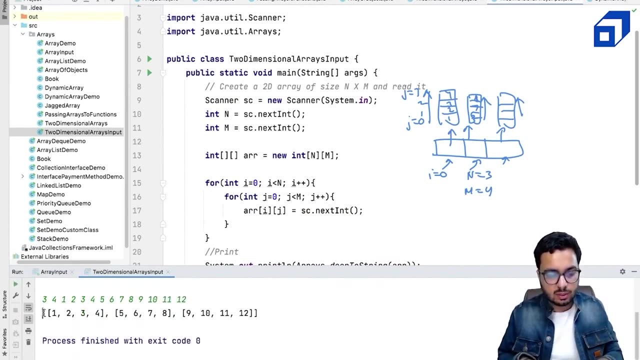 Dot. Let's Say I Want To Have Three Rows And Four Columns. I Need To Give Data. Let's Say I'll Give Twelve Elements One. 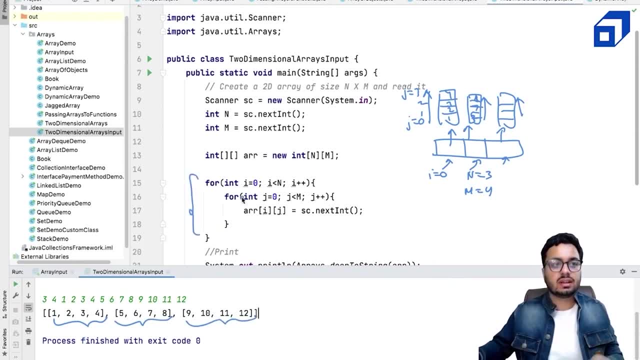 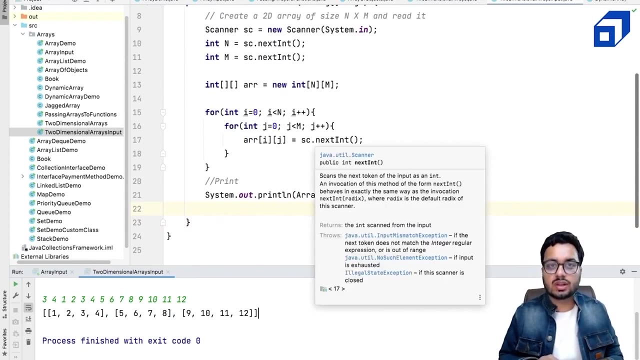 Two, Three, Four, Five, Six, Seven, Seven, Eight, Seven och And contents. So A Part Of This, All This All Has a ructa. Input D. 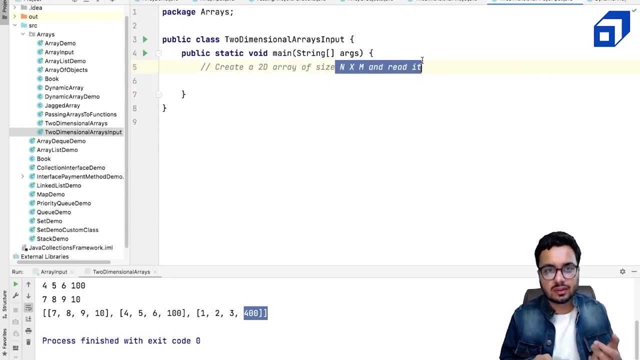 And Client, Because So I Need To Write One Man Initiative user, So scanner SC. this is equal to use scanner And let's read how many rows we want to create. number of rows is scanner, dot next end And number of columns is also going to. 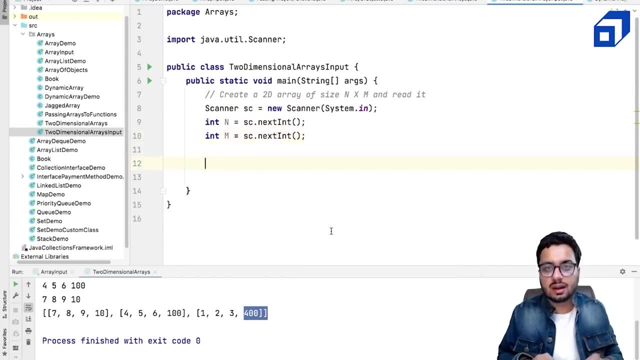 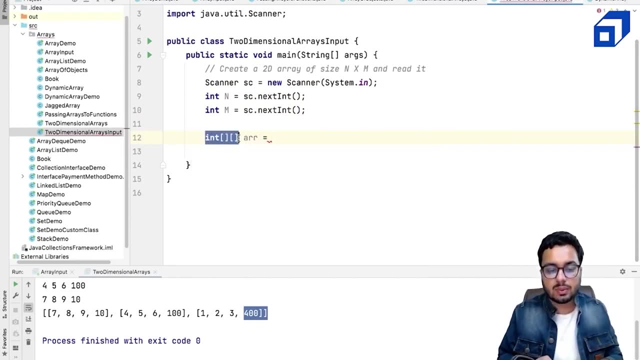 be standard. So I'm going to create a 2d array of size n cross m. how do I do it? Pretty simple, I define variable. ARR is of the type int- square bracket- square bracket. this is equal to new int, And here I define the number of rows is n and the number of columns which. 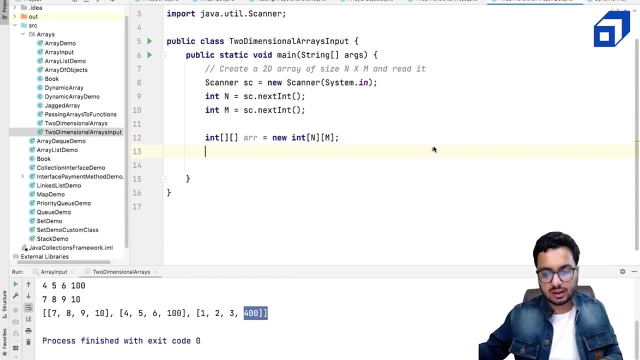 is m. Once I do this, Java will create an array in which I have, let's say, n equal to three and m is four. it's going to link these like that Internally. this is how they will get created. Now, what I want to do? I want to. 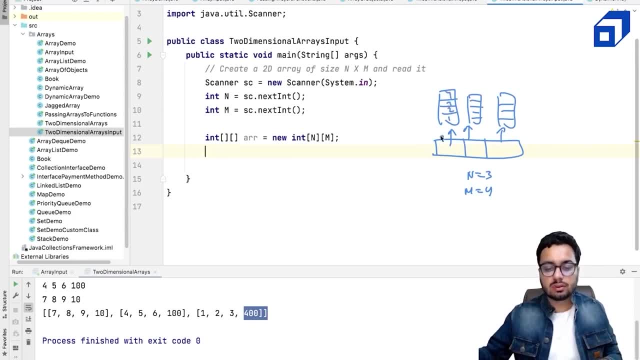 read numbers and put put them here I want to show. the 123 is the first row, 5678 is the another row. How do I do it? I have to go to the zeros index. then I have to iterate over from j equal to zero till j equal to 3012.. Then I have to go to this index. read. 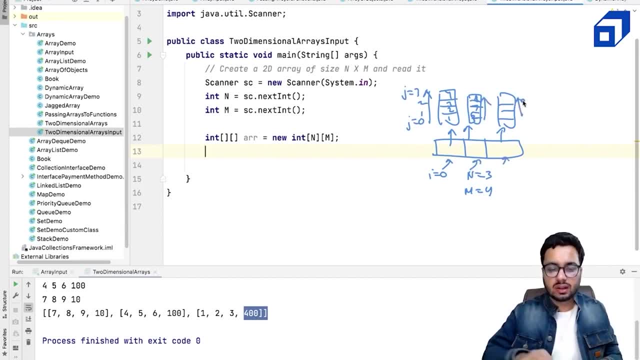 this array. I have to go to this index. read this array. Let's see how we can do it. I can say for int: i equal to zero. i less than n, i plus plus. Then for each row I need to read the elements: j equal to zero. j less than m, a plus plus. 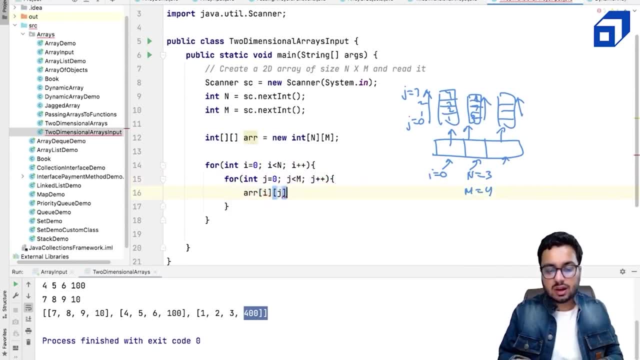 and array of i comma j, In the ith row, the jth cell, I want to read a number and a dot extent. Fine, This is it. It's once this is done. I have read all the elements And what I need to do. I need to print so I can say: okay s out. 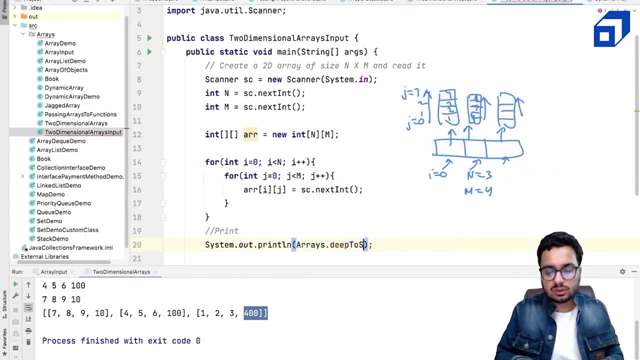 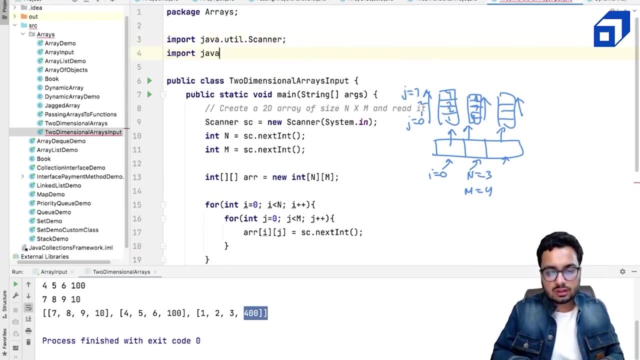 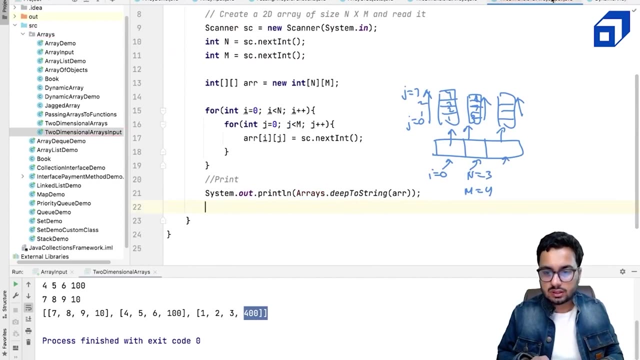 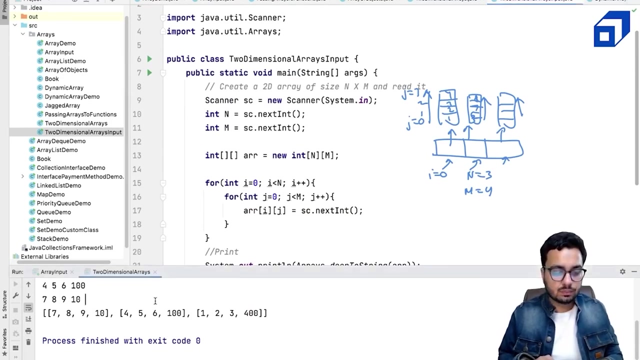 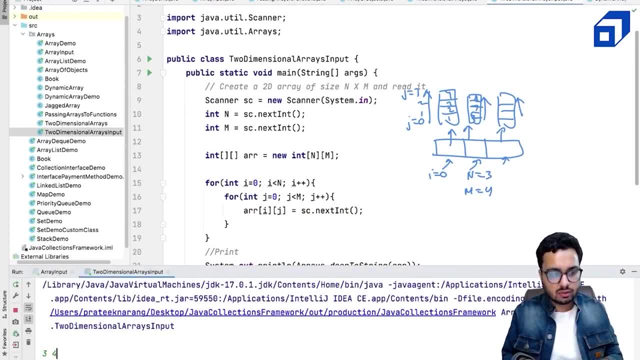 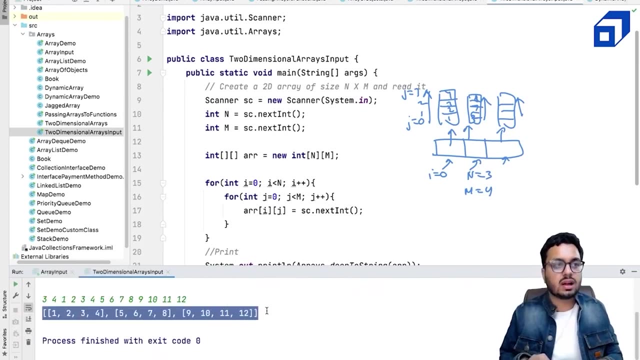 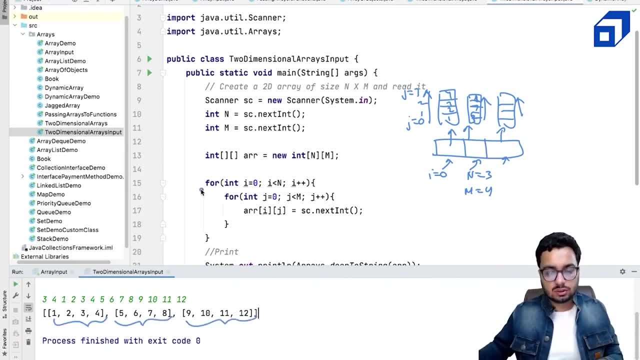 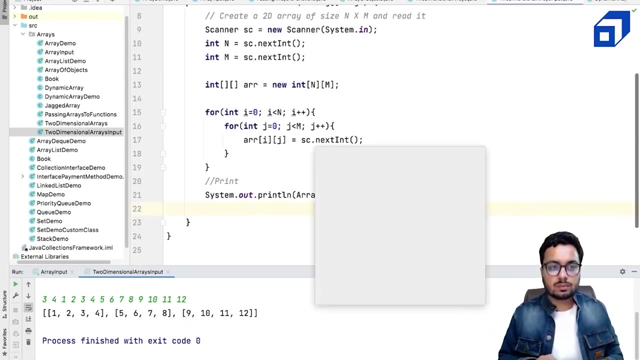 row, second row and the third. So this is how exactly we get a two dimensional array And this is how the memory represents the array. The memory representation of 2d array looks like this is my variable era. Okay, so let's. 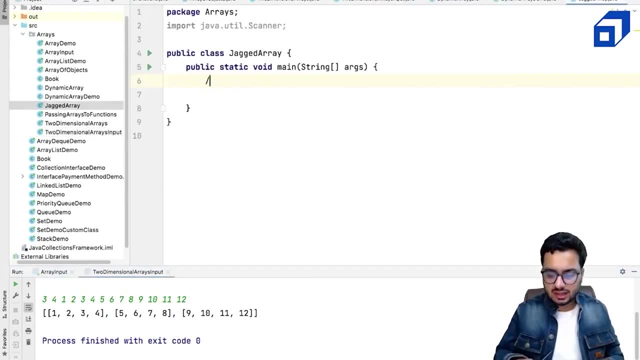 move on to jagged array. Next let us discuss what is a jagged array. A jagged array is an array with variable number of columns. variable number of columns. How this is possible, Let's see. It's an example. Let's say I have three columns in one row. In another row, 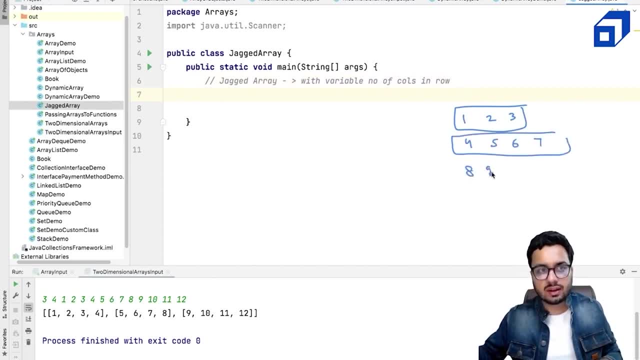 I have, let's say, four columns And in another row I have, let's say, four columns And in another row I have just two columns, And we create such an array. The answer is yes. Why? because when you create a 2d array in Java, each bucket is referring to an array. 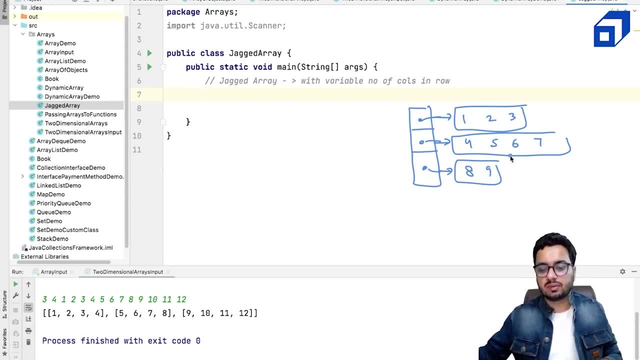 object. Now, each array object is independent of the previous object that we have created. What I'm saying is, we are creating three different objects for three different rows And each object can have its different length. For example, this length is two. this length is: 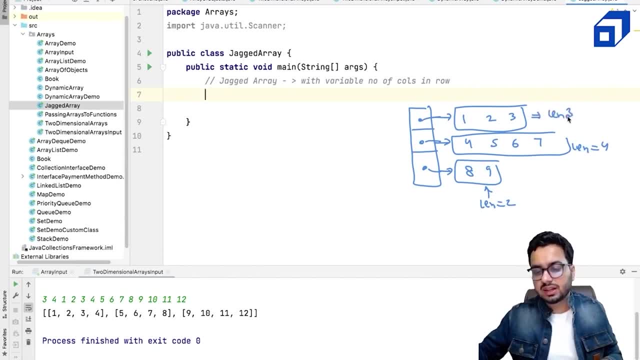 four, Let's see how we can create an array like this. Now it's again a 2d array which looks like this: 123456789.. In this case we don't have fixed number of columns. we need to. number of columns are variable in each row. How do I do it? So let's see, I'll start by creating: 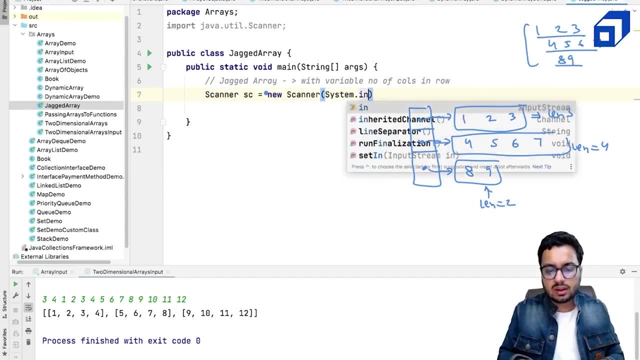 a scanner equal to new and as it's gotten. I'm just going to read the number of rows from the user: is a scanner dot. next, Once I know the number of rows, I can initialize my array. I can say int, square, bracket, square. 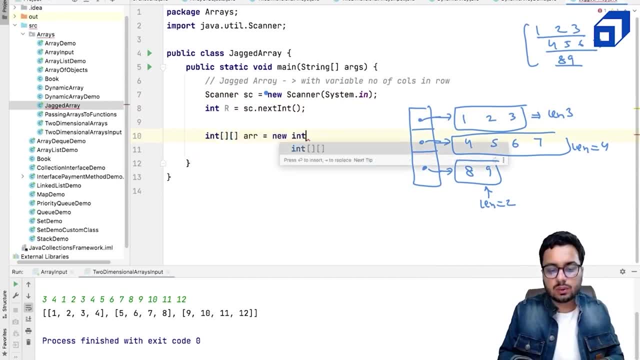 bracket ARR. this is equal to new, and- and here I just define the number of rows- is okay, I need our number of rows. how many columns are there? I will tell you later. What does this code do? It creates an ARR that points to an array that is going. that will hold that. 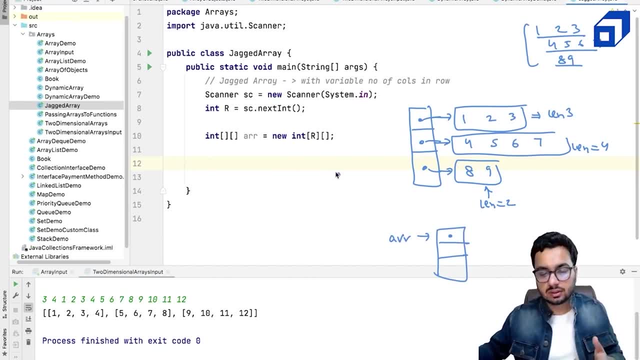 will hold These array objects, but they will be created later. it's only going to create an array with our number of buckets inside These. these will be created later. this part we will do next, right Now, what I need to do, I need to iterate over each bucket I equal. 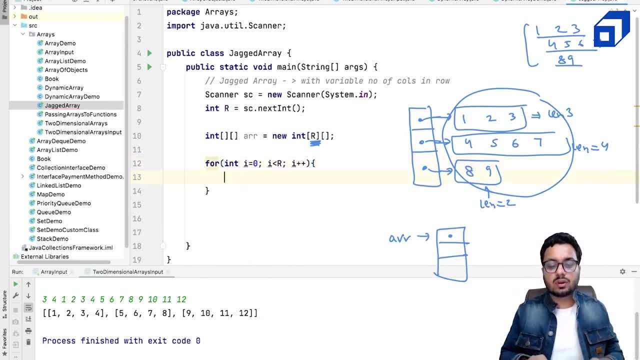 to zero, I less than R, I plus plus. Now I'm going to ask: okay, tell me how many columns you're going to have in this row. I will ask the user I can accept a columns in this row. I will ask the user: I can accept a columns in this row. I will ask the user I can accept. 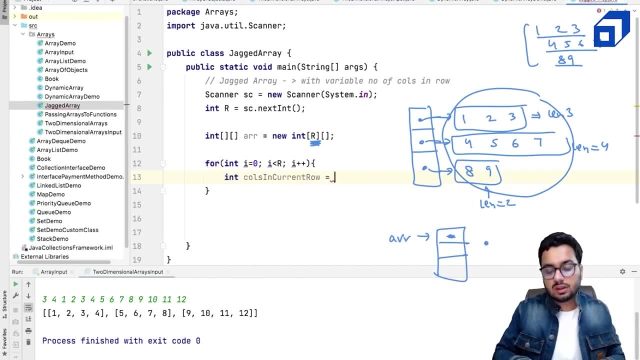 a columns in this row In the current row, how many columns. I'll ask the user to tell me number of columns in the current row. can also output here s out columns in the current row. tell me how many columns will have in the current row And then you can say s out data in the current. 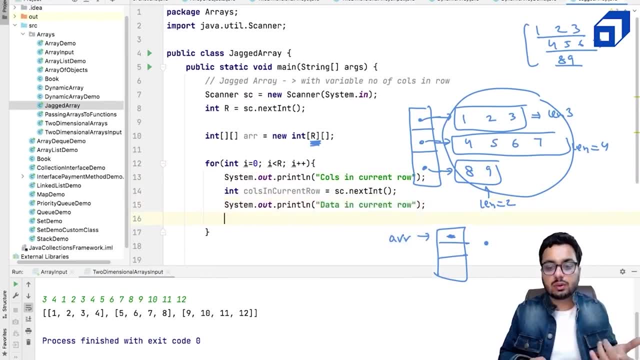 row. Maybe if I said I have two or three columns, then I will run a loop three times to read those numbers. So it's okay, for int i equal or int j equal to zero, It's fine. Now the thing is, where should I store this data? This array object is not yet created. 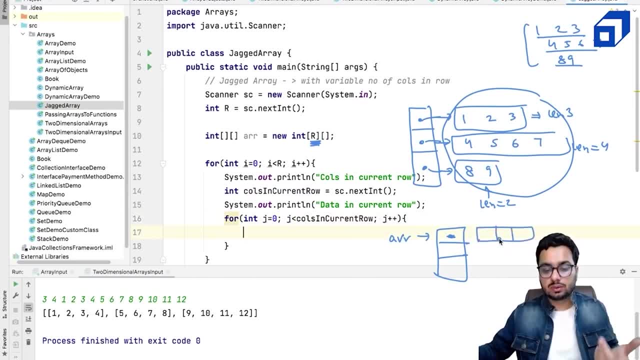 First, I have to create an array object here in which I should be able to store data. How do I do it? I said, Fine, this array is this bucket. it should point to a new bundle I'll in which I can hold these, many of these many numbers. that is equal to columns in. 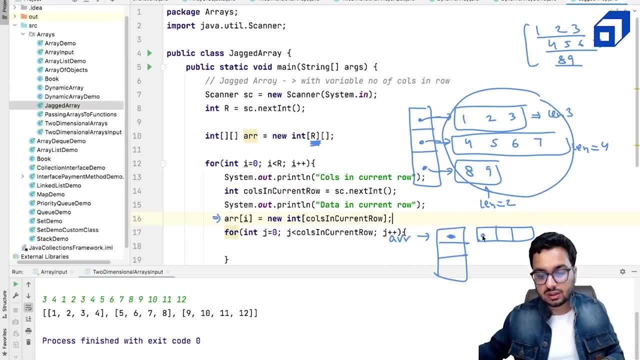 the current. this line of code will actually create this array. and suppose this address is now 7 0, 2, this is stored here: 7 and this link is established. now I can read data and I can store it in this thing. we will repeat for every row. 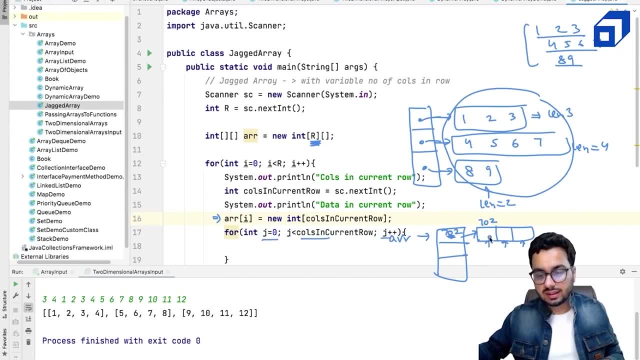 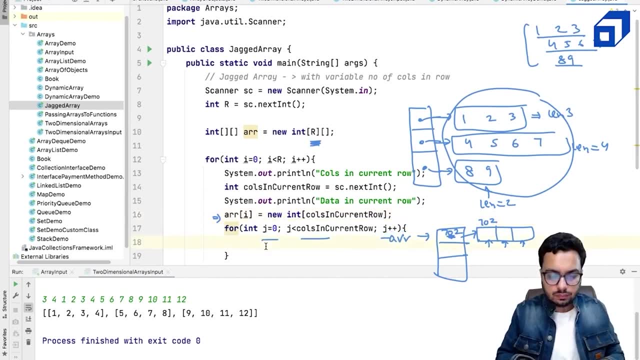 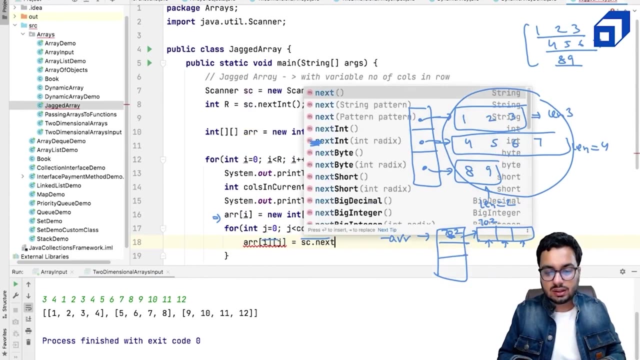 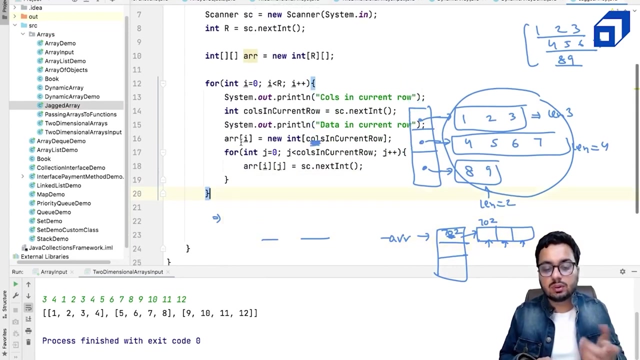 and I trading over these buckets now and I'm going to say, ok, read the next number and store it here. I can say: array of I am on J, this is equal to and Idol. that's it. and in the next iteration we move on to the next row and we do the 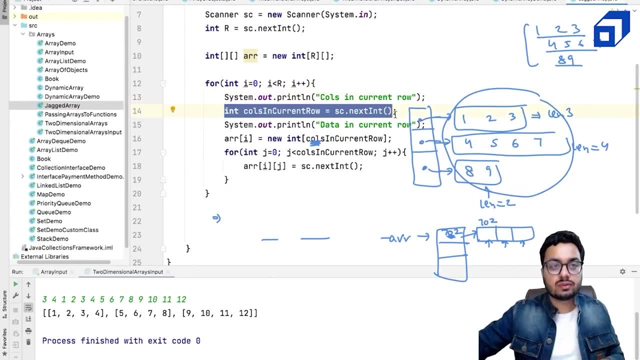 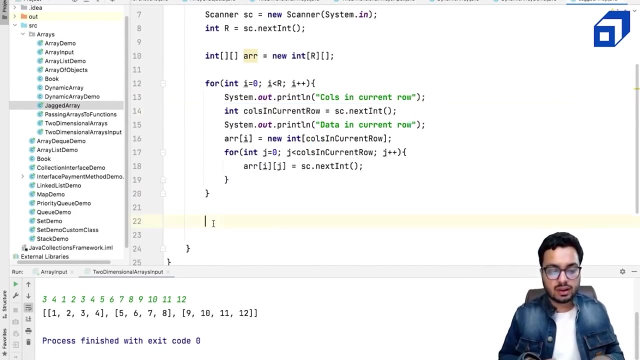 same begin. we ask how many columns you have. in the next row, it says, okay, I have four columns. I create a ô, an array of size 4, and i link it here using this line, and then i again read it. i read these: let me show you, uh, by running this code, that we can actually create a jagged array s out there is. 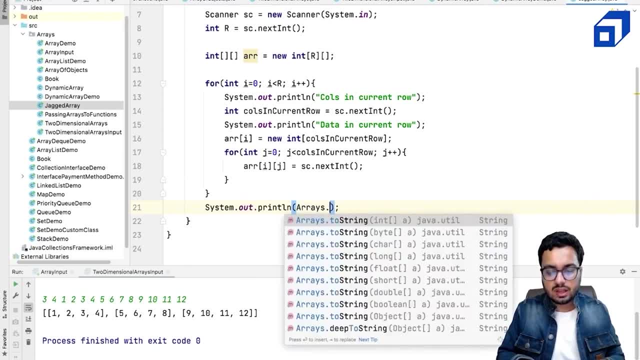 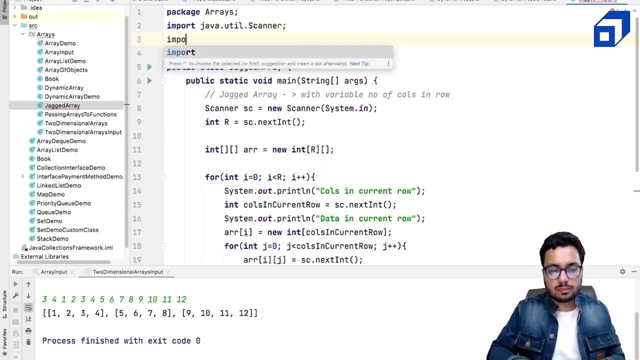 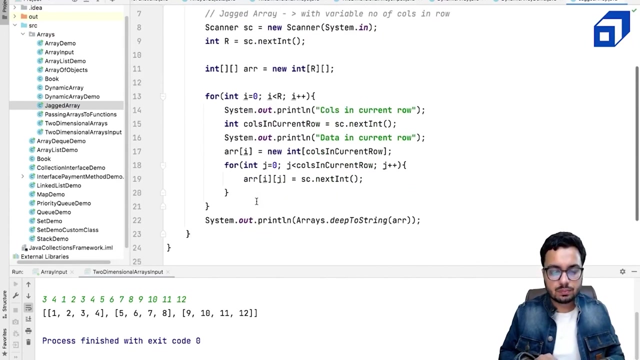 dot uh deep to string and i can give a here and again. i have to import java dot youtube, so let's go and turn this. okay. i want to create an array with three rows. now i have to tell me how many columns in the current row is okay- four columns- And then I have to tell me what are the four. 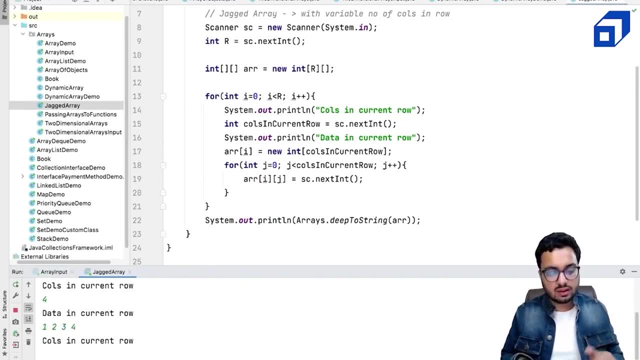 numbers in that. So it's a one, two, four. then the next row: how many columns? maybe just the columns, and the numbers are 789.. And in the next row, let's say two columns, the numbers are, let's say, 10 and 20.. What do I see? I see a jagged array: four columns. 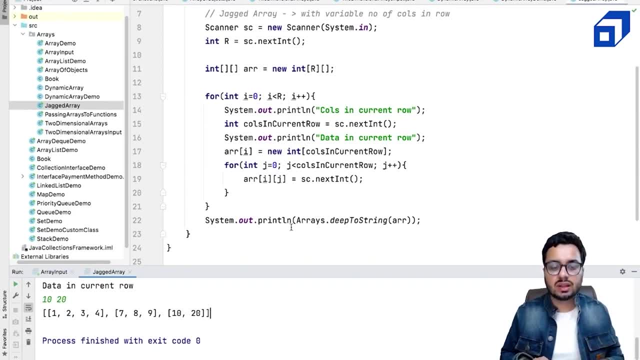 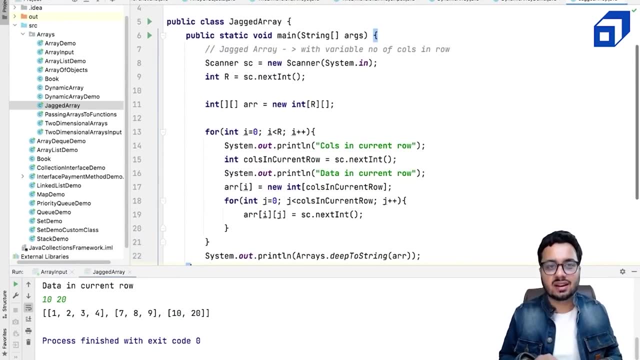 three columns and two columns. This is how we can create an array in which every row has variable number of elements, And this is called as a jagged array. Now we are going to look at dynamic arrays. So far, the arrays we have created, they had a fixed size Once. 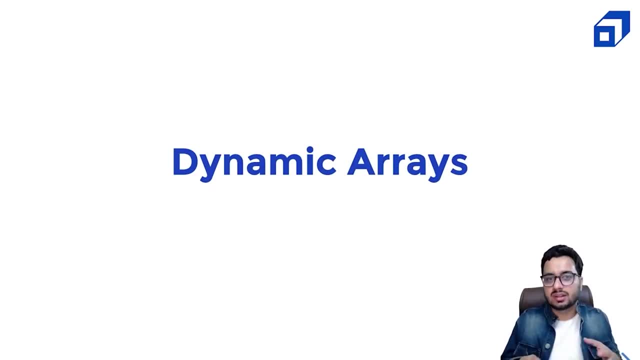 you create an array of size n, you cannot add more than n elements into it. That is where dynamic arrays come into picture. For example, you're building a to do list where you can keep on adding tasks every day And you might be removing a number of elements. 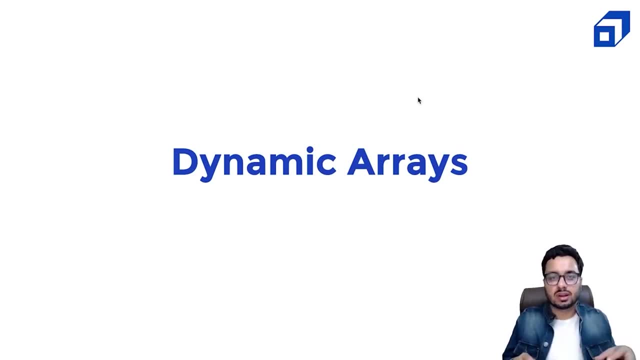 doing some old task as well, So you do not know how many elements you would be storing in your list, So you need something like a dynamic array in that case. In Java, dynamic array is provided by the library As a part of Java collections framework. the class is: 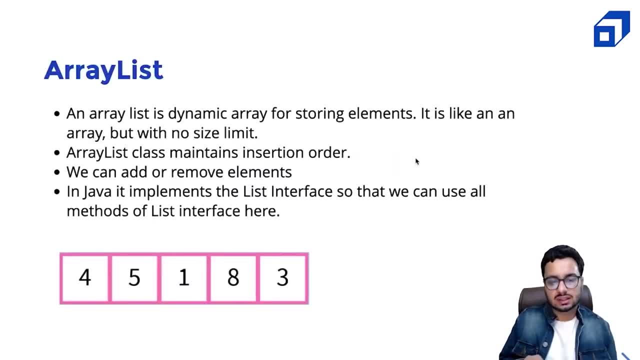 called as ArrayList. You will also see how this class internally works. But before that we will look at a demo of using ArrayList. An ArrayList is a dynamic array for storing elements. It's like an array, but with no size limit. It also maintains the insertion. 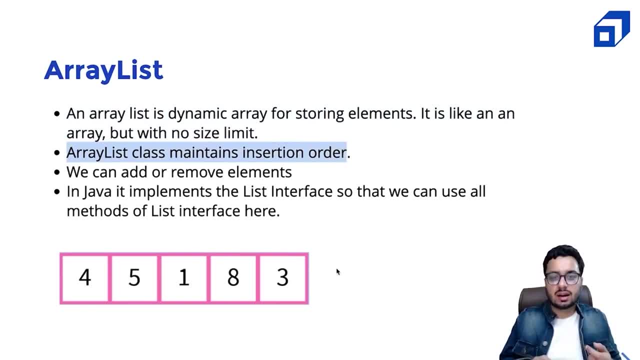 order. That means keep on adding elements and they will get added at the end of this array, right? So if I say, okay, I want to add six, I want to add seven, I want to add 12, they will keep on adding in this. at the end of the array we can add elements. we. 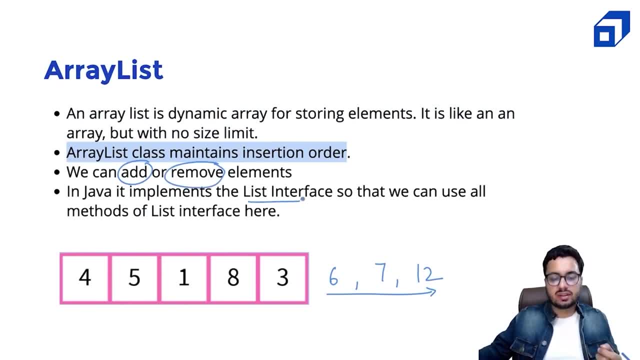 can also remove elements And it implements the list interface in Java So we can use all the methods of the list interface here. So list interface is part of collection framework And I've done a detailed video on collections framework link you can find in the description. 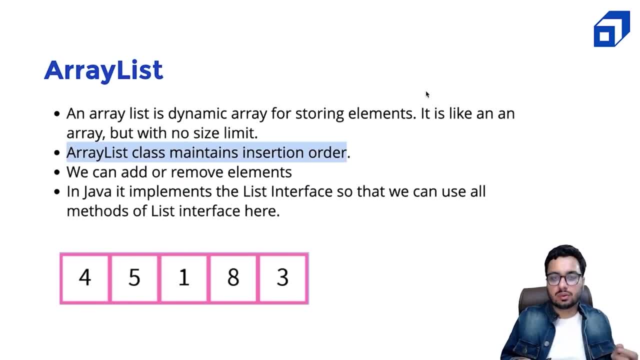 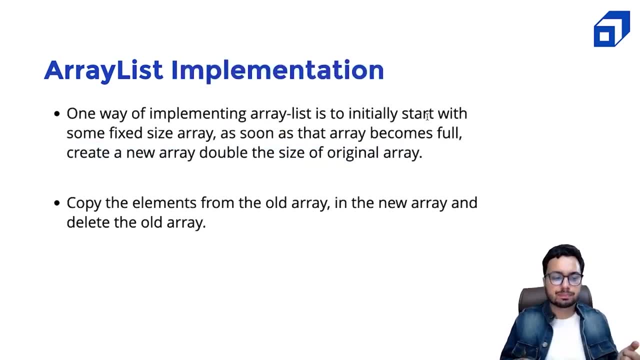 You can watch that video if you want to learn about. what about the collections framework and various data structures present inside the Java collections framework. Now, how this ArrayList is implemented. Let us talk about how this array is actually dynamic. How does it grow and shrink? One way of implementing the ArrayList is start with some fixed size. 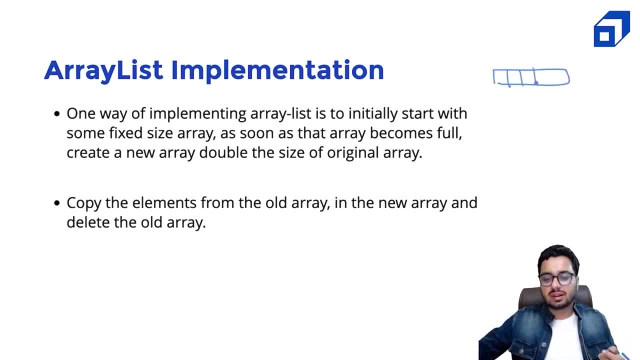 array. So I guess in Java this fixed size array is having a default size of 10.. So whenever it's okay, You create an ArrayList, it will give you a base for 10 elements. But as soon as this gets full, it is okay, I've used all the elements. like what it will do, it will double itself. 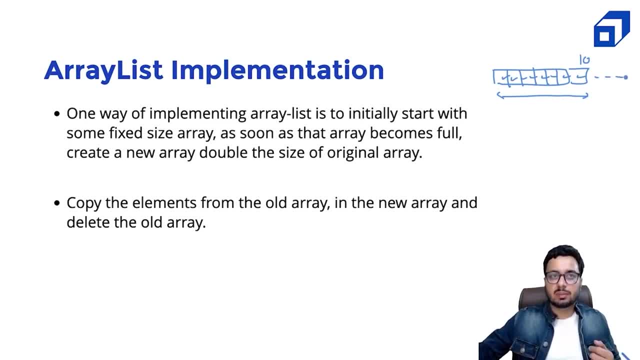 Now, you cannot double in the same memory, because this memory might be occupied by some other data sector or some other part of the program. what it does, it looks for new memory in the heap, where it creates an array of the double size And it's going to copy the old data. 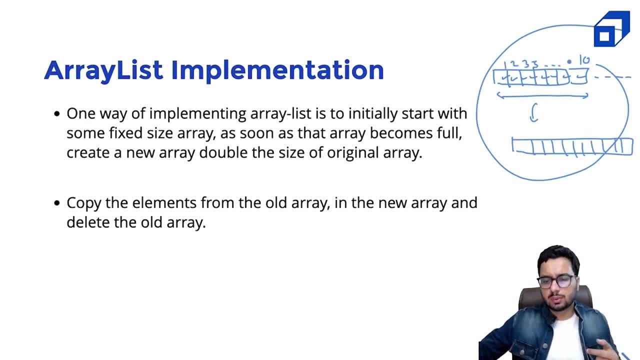 into the new array. So it's going to copy all this data in the new array And then the remaining elements. the remaining 10 boxes are available for putting some new data right. Once this gets full again, you have to do the same thing again: double the old array by creating a new array. 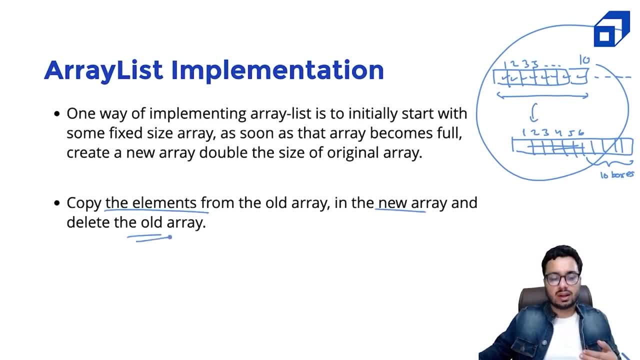 copy the data from the old array And you have to delete the old array. So in Java the deletion is done by the garbage collector. For example, if this is my old array and I say old ARR equal to null, what does it mean? No one is referring to this array. this 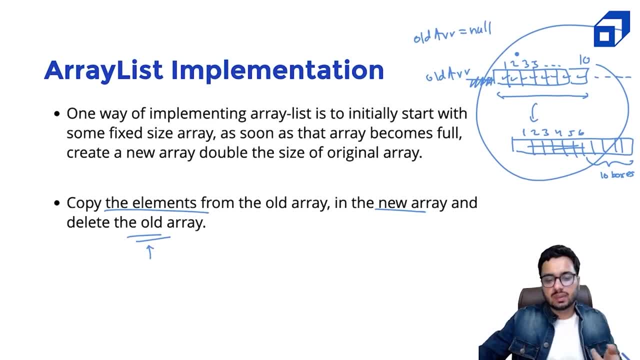 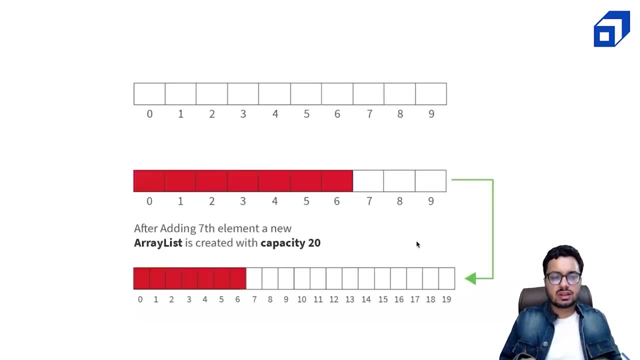 object becomes eligible for garbage collection. Okay, so in other languages, like C++, you have to use the delete keyword, But in Java the garbage collector takes care of objects that no one is referring to. So first, let us first look at the demo, right, So to be. 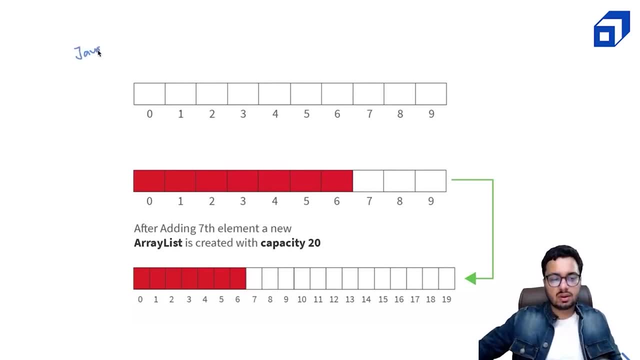 precise in Java. Java maintains something, Something called as a load factor. Load factor is what percentage of your array is currently filled, right? So if I say okay, if my load factor goes more than point seven, that means if I have space for 10 elements and I put eight elements in this array, right That? 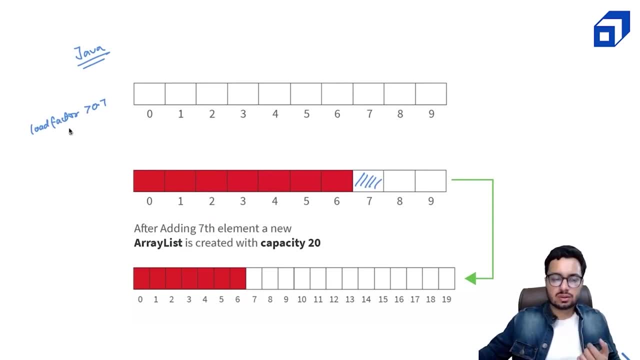 means it is the time to double the array, right. So right now I was doing it full capacity, but you can also do it early If you're 70% of the array is full. So that is your current size upon your capacity. 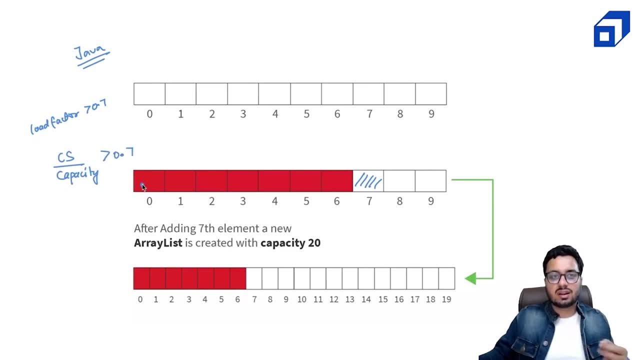 If this percentage exceeds point seven, the Java triggers this function that doubles this array. So it gets a new array, copies the data here And you have more space available for storing new elements. Okay, So ideally, if you know that, okay, I'm building the application. in which I will require space for around 1000 elements. it is better to initialize your ArrayList with the initial capacity of 1000.. Again and again, And if you okay, I need maybe 1100 elements to take a safer limit. 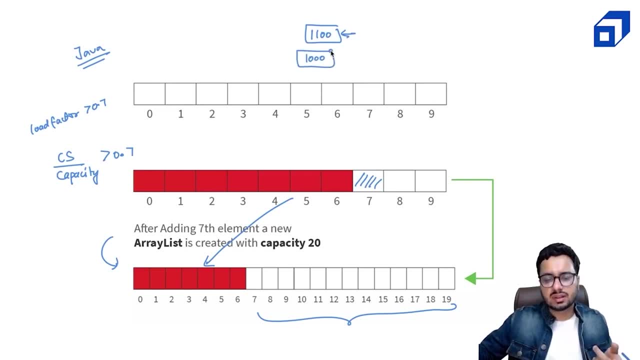 okay and you took okay. I created an array with 1000 elements. that is fine. it will double one time, So from 1000, it will become 2000.. Right In 2000,. you can easily store. 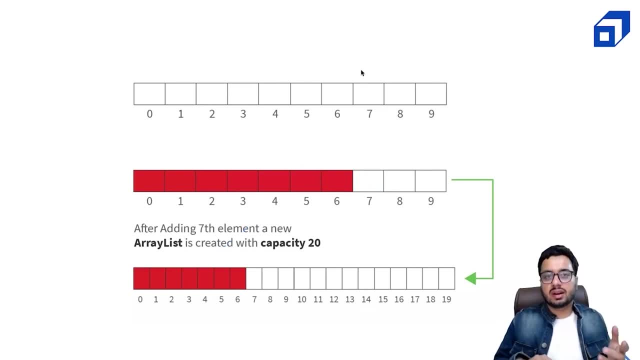 1100 elements. Basically, you should have a rough idea of the range, how many elements you would be needed, And accordingly you can initialize the ArrayList so that your repeated doubling operations will be completed. So that's it. Thank you for watching this. 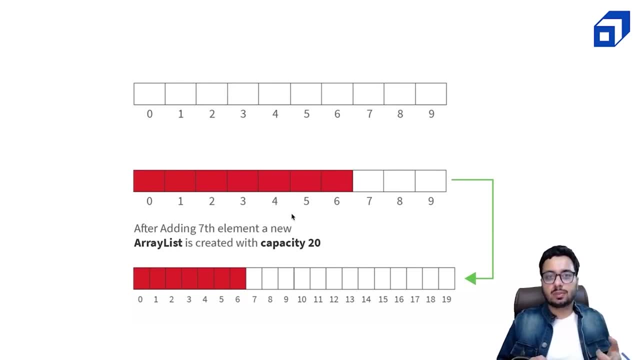 video customization can be minimized. And doubling is an expensive operation. Why? Because it copies all your data into the new array, which is going to take linear timeline. That is how the internals of the ArrayList work Right. So let us also talk about features- ArrayList. 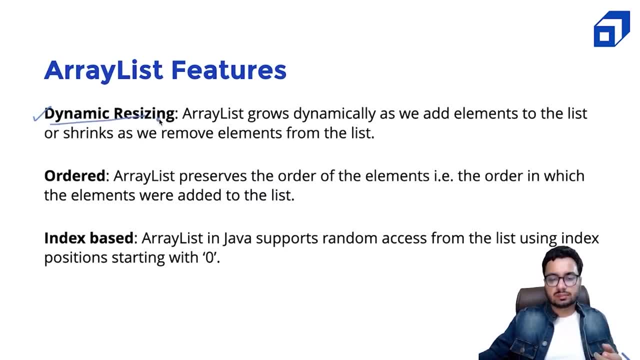 is a dynamic data structure And it can grow dynamically. it can also shrink as we remove elements from this. So again, there is certain criteria. Okay, When 20% of the list is occupied, I might shrink it to the half, something like this. we can have a conditional condition. 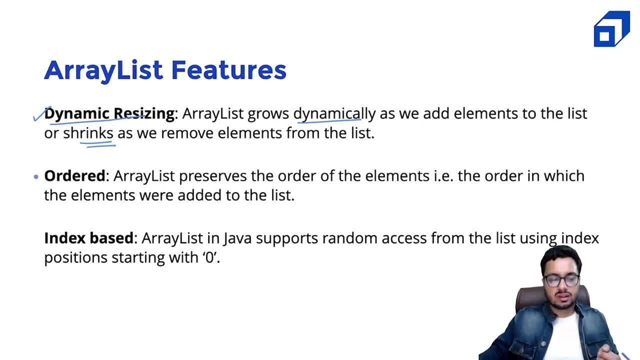 on shrinking as well, just like we have a condition on growing. Second thing is: it is ordered. it preserves the order in which the elements were added to the list. It is index base, does it's? it's an error internally right, So it also has indexing. So if you want to get this, 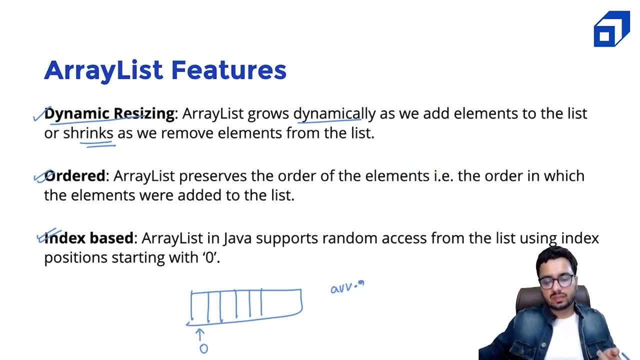 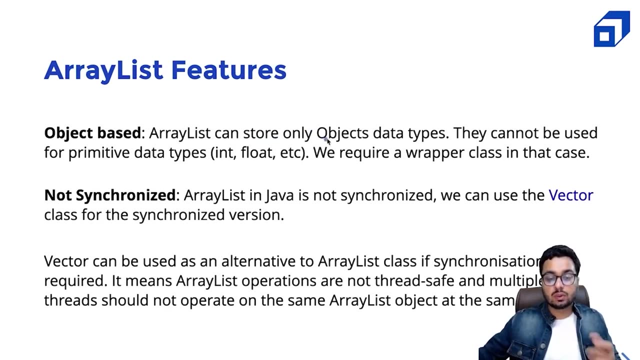 element. we will say: okay, array dot, get zero. it provides us with a get method And I need to allocate. this is the index I need to access. right And okay. and ArrayList can also store. It can only store object data types. That means it cannot store primitive data types. 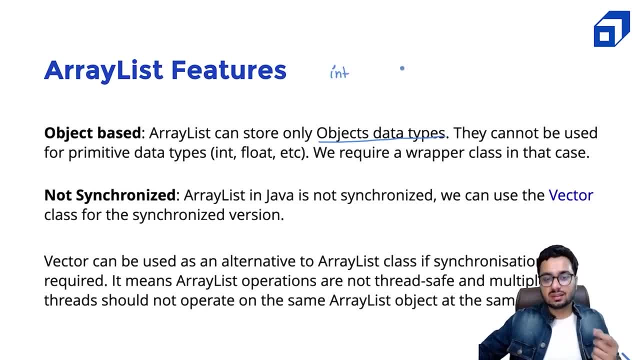 like int. If you want to create an ArrayList of ints, you will have to use the corresponding wrapper classes. So you have to have some idea about wrapper classes. I can create an ArrayList of integer where integer is a wrapper class For int data type. it cannot be used for primitive data types require a wrapper class. 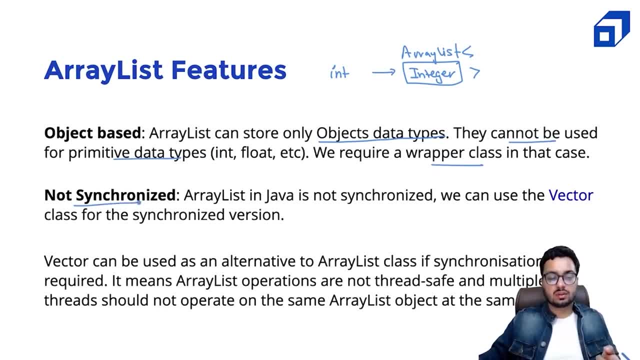 in that, And another thing is it is not organized, So you need a concurrent data structure. then there is a something called as vector, which is a synchronized implementation of ArrayList. Okay, This concept is pretty advanced If you're working with multiple threads and stuff. 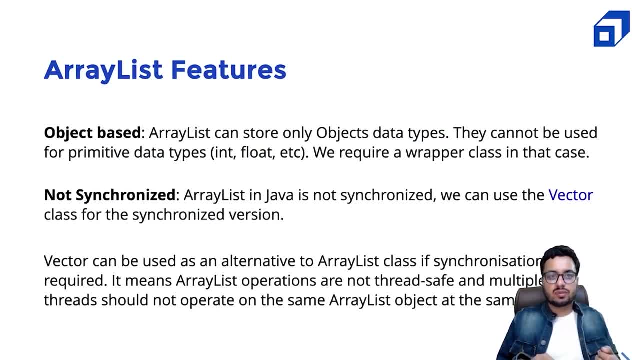 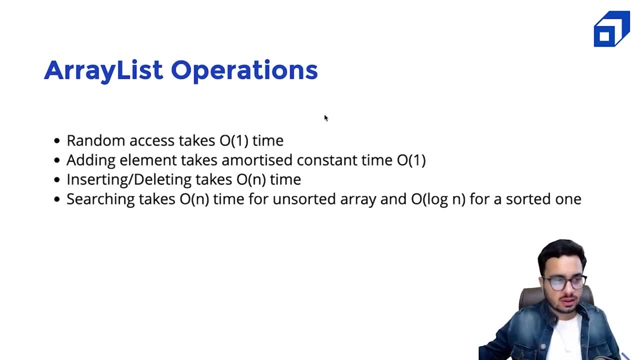 then you might be using vector. So let us look at a demo of using ArrayList. Before we jump into the code, let us talk a little bit about the kind of operations we can do on an ArrayList. So one common operation that we do is we want to access an element. 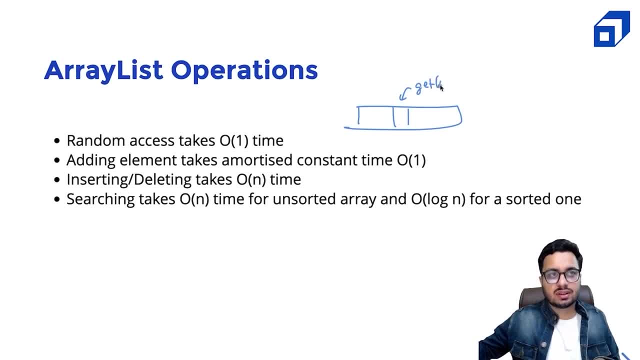 so it is called as random access. That is done using the get function. I can get any random element in order of one time, which is pretty obvious because internally it is accessing the array. Then I can add elements. I can add elements at the end of the ArrayList. 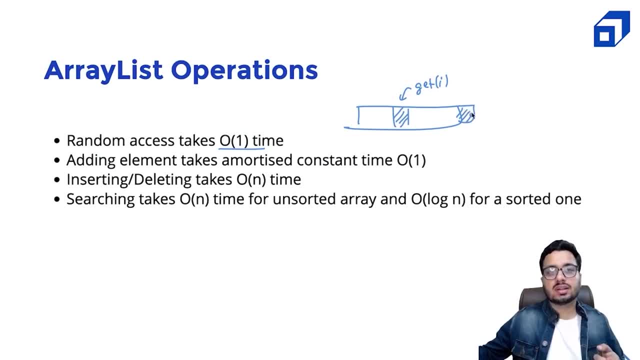 which will take order of one time. You can also add elements in the middle of ArrayList, which will require shifting of elements. Okay, inserting elements in the middle, it's going to take order of n time. Similarly, deleting something from the middle is also going to take order of n time, because 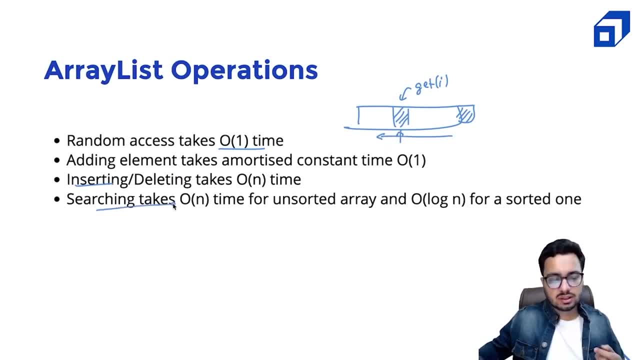 remaining elements will have to get shifted. Searching in general it takes order of n time because it's going to use a linear search type, But if you have a sorted ArrayList you can use your own binary search method Or you can use collections dot binary search. 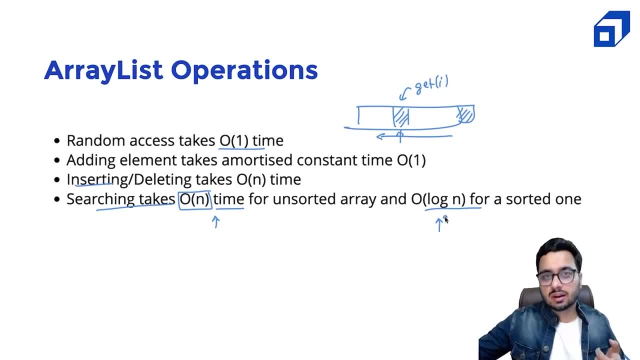 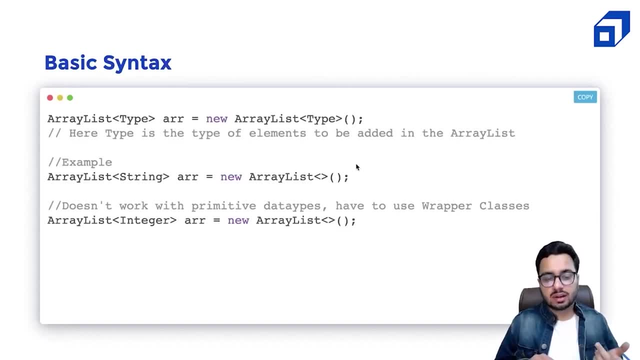 method To search in order of log n, in order of log n time, if your ArrayList is sorted, Okay. So how do we create an ArrayList? It's a predefined class in Java collections. I can say: okay, ArrayList of a following type, followed by name of the variable, followed by new ArrayList. 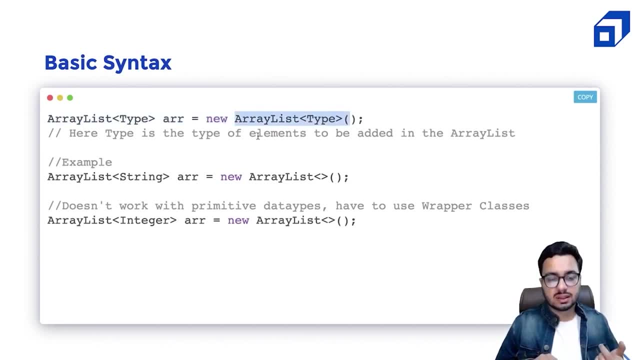 And this will create an ArrayList with a default size. default size in Java, it is 10.. For example, an ArrayList of strings can be created like this, And it does not work with primitive data types. Okay, so I told you that we have to use wrapper. 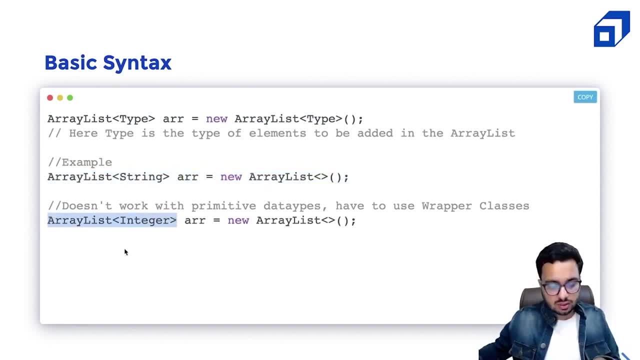 classes, we will have to say ArrayList of integer. if you say ArrayList of int, it will not work, So you will have to say ArrayList of integer. right, This is equal to new ArrayList. That is how you will create an ArrayList object in Java. 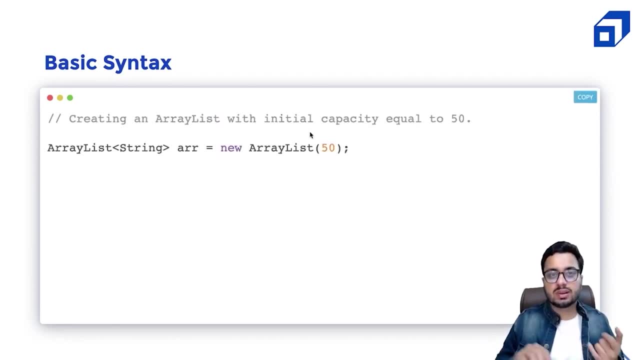 Next thing is you can also give some default size. So basically the ArrayList class has three constructors In. Okay, In one constructor you can, you don't give anything, So it uses a default size of 10.. In another constructor it accepts, you give me the default size and I will create an. 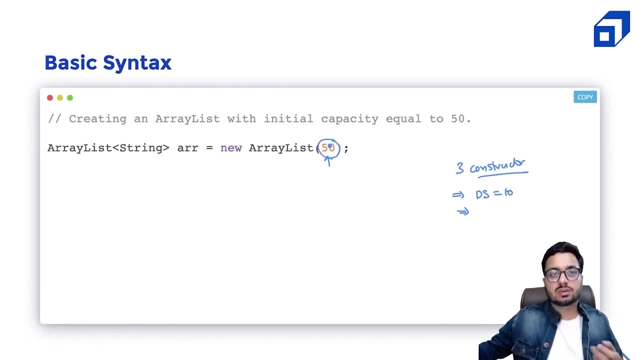 ArrayList of that capacity. So I'm saying 50. That means it is able to hold 50 objects in this ArrayList, And once you reach 50 capacity it will double itself. right. And there is a third constructor as well in which you can initialize an ArrayList from some other list. 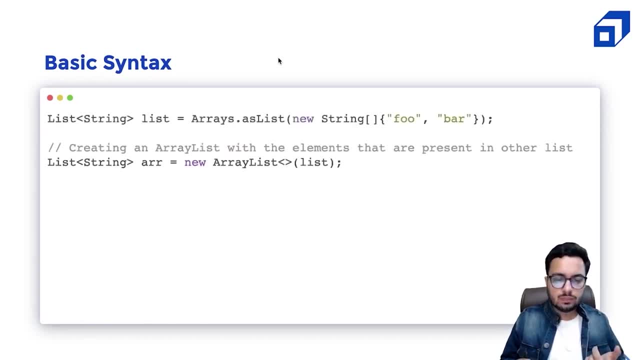 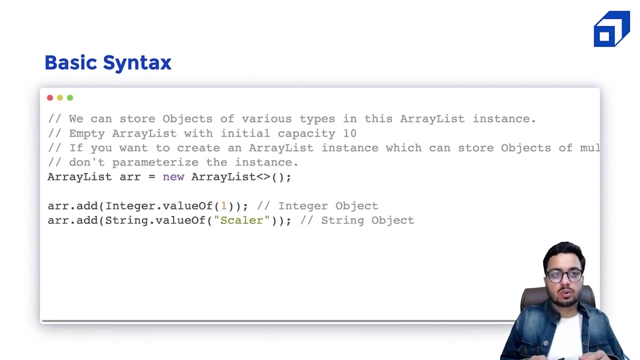 or from from some other collection as well. That can also be done. For example, in this case we have a list of strings And we are initializing the ArrayList using this list. That is the third constructor call. that is being done Right. So one more point to note about ArrayList is it allows us to store heterogeneous elements. 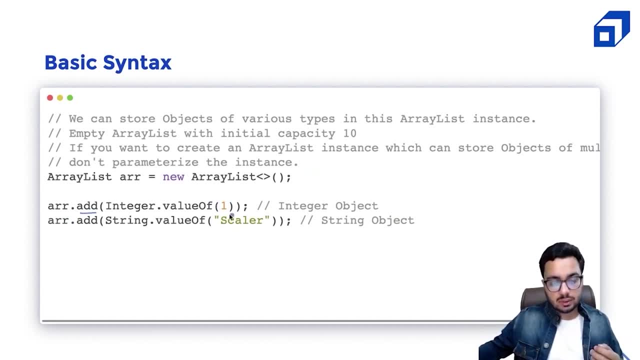 as well. For example, I can add an integer into it. I can also add a string object into it. Right, We can store objects with various types in an ArrayList instance. Also, we can store objects with various types in an ArrayList instance as well. 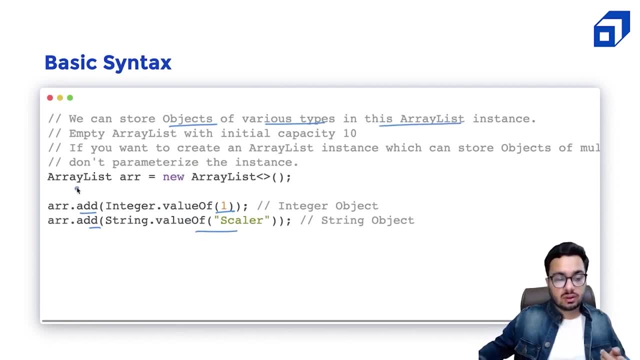 Okay, Okay. So in this case, when you're creating this ArrayList object, you don't need to parameterize the instance, you don't need to define what kind of data it is going to hold. it will hold all types of objects in it, right? So you can put a string, you can put a book. 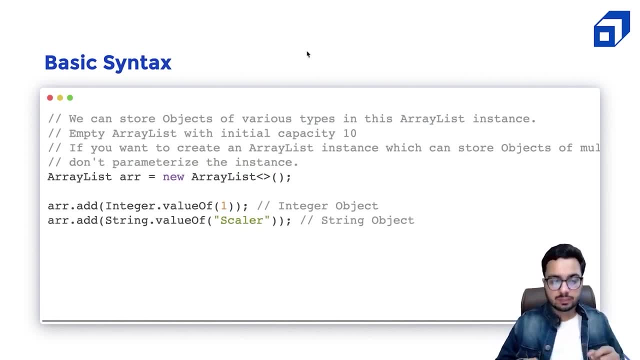 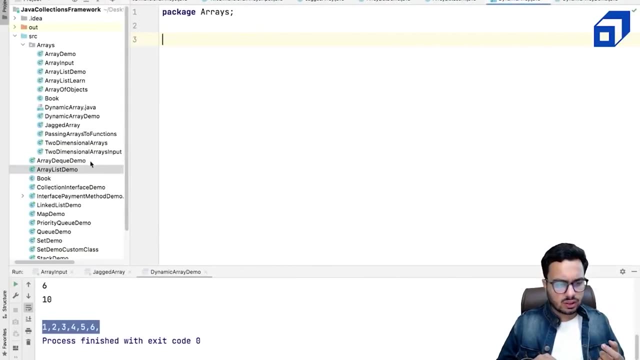 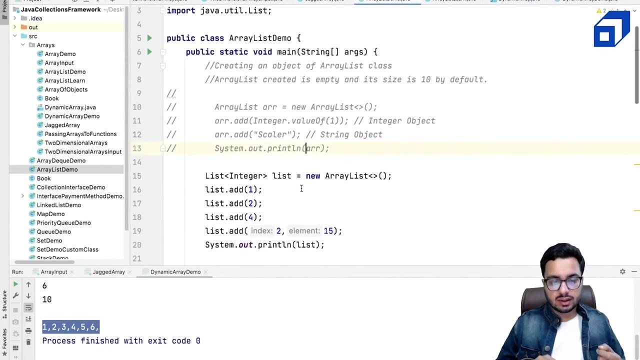 you can put a dog. anything will work in the same ArrayList. So that is about how do we create an ArrayList. Now I will show you a quick demo as well. So I did this demo in Java collections. In this video that I have already done, I have shown you that you can create an ArrayList. 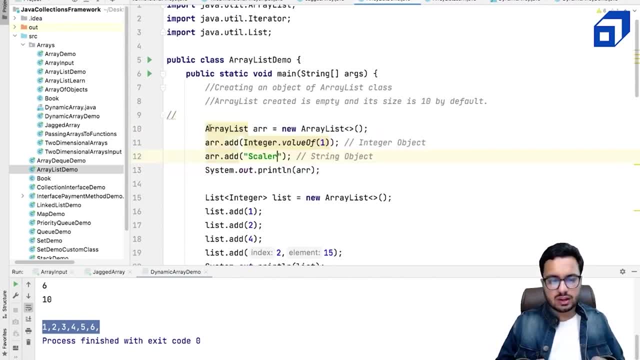 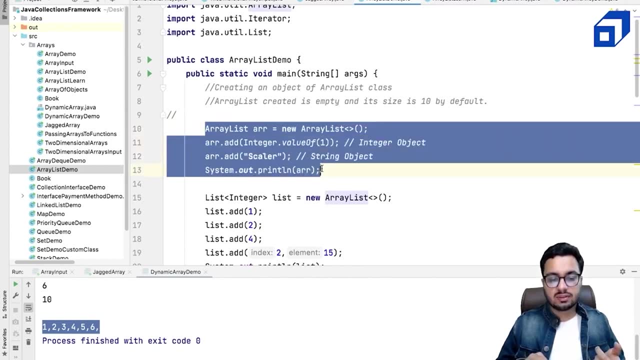 So the first four lines I show you. we are creating an ArrayList in which we have not defined the data type, then we are pushing an integer, then we are adding a string and then we are going to print it. let me just run this code And let me show you the output. 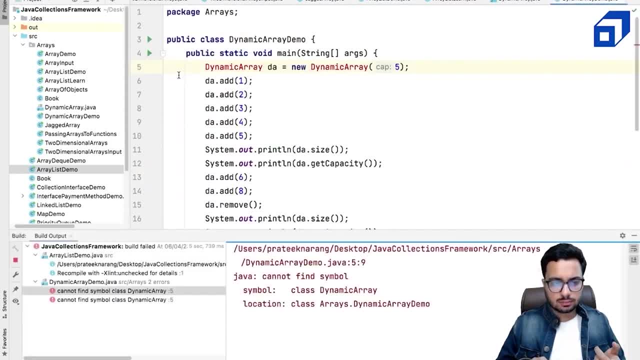 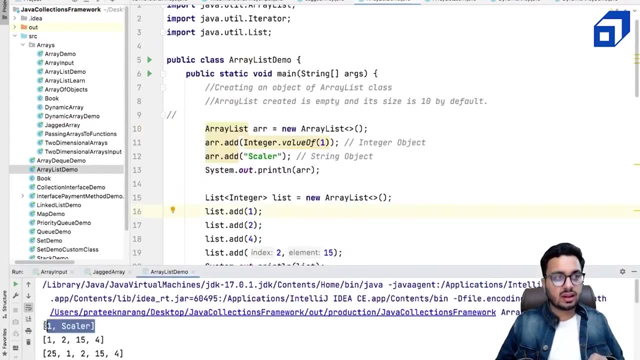 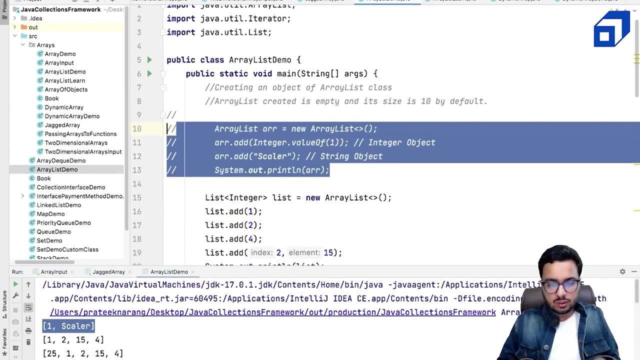 I need to run this, Yeah Yeah. So if you see, here I'm getting an ArrayList in which one item is an integer object, the other item is a string object. So we can definitely do this. I'll comment it out, then I can say: 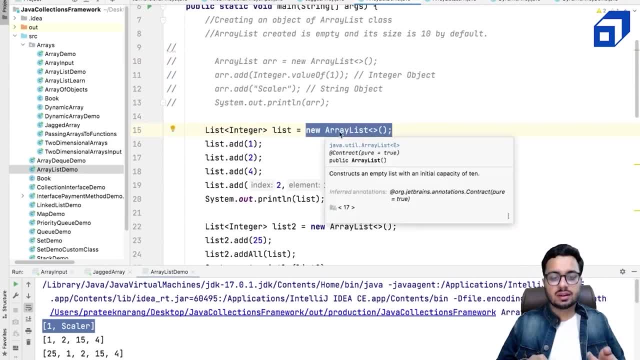 okay, create an ArrayList, Because ArrayList implements an interface. So I can say this: left and right data type can be more generic, it can be. it can have list as the data type. that is perfectly fine, because an ArrayList is an implementation of a list, So I can call. 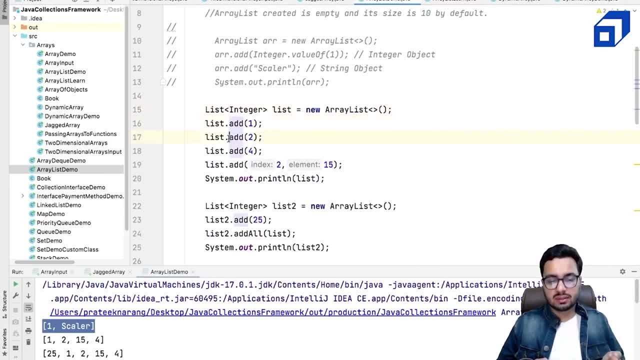 the add method add something at the end. I'm saying, add one, add two, add four. then I can also use this add method by specifying the index. So the add method is overloaded. There are two add methods: one which adds at the end and one which adds at a particular. 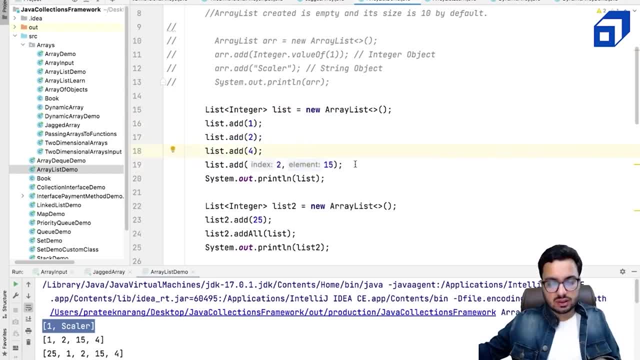 index. I'm saying, okay, at the second index you should add 15.. So it becomes like this: one, two, four. then add the second index, which is zero, one, two. I want to add 15 here. It will be increasing the number, So I can add two, two, three, four, And then 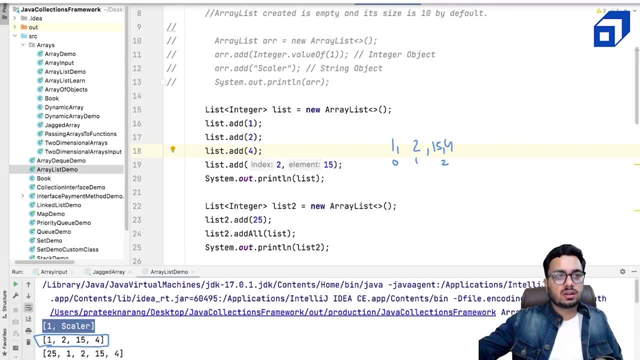 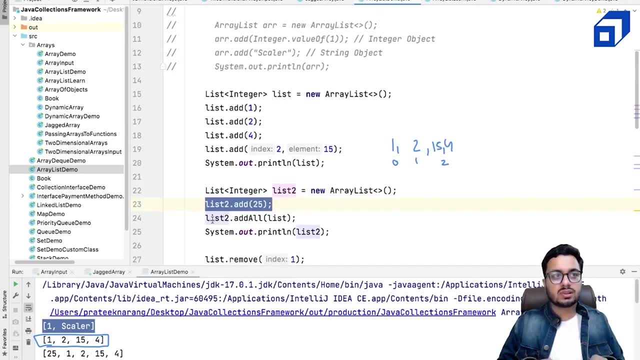 become 1,, 2,, 15 and 4.. This is the output that we get. Then I've created another list in which I have added 25, and then I'm using a method called as add all. Add all is used if you want to add all items present in one list into another list. Add all will iterate. 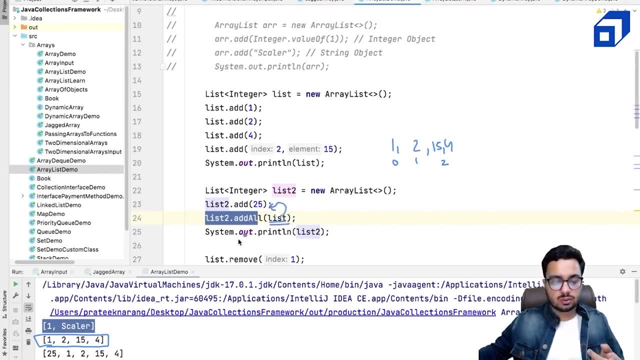 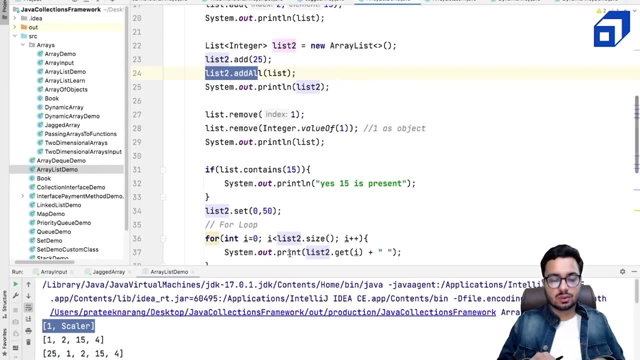 over all items in list one and it will add them into list two. So you will see 25, followed by all items that are present in list one are now present in list two. So just like add, we have a remove method. Remove method is also. there are two remove methods: The. 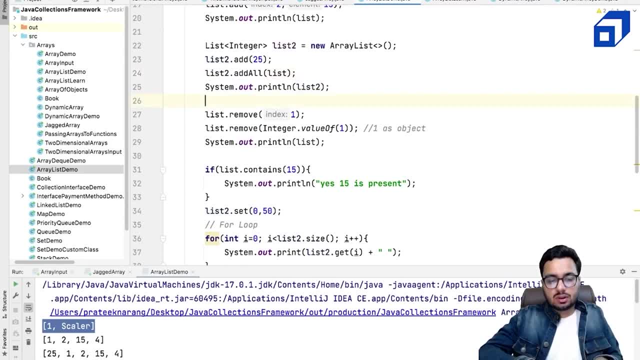 one remove method which accepts an integer. So if I show you something like this list dot remove, So you can see one remove method accepts the index and second remove method accepts the object. If you have to give the object of the type integer, you have to type: 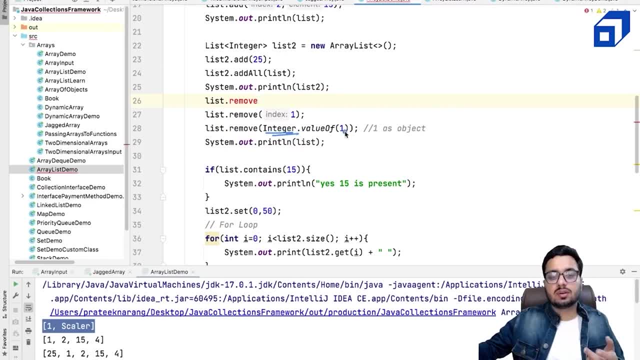 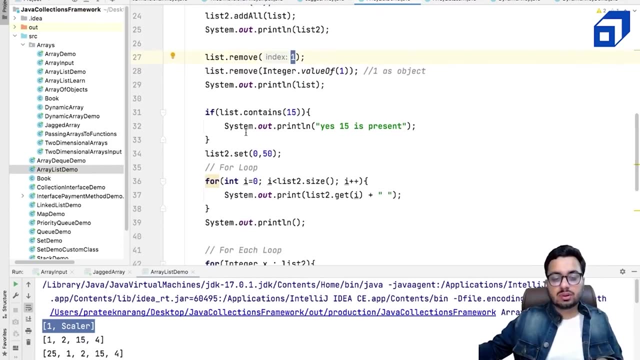 cast integer, So I can say integer, dot value of one. It will mean that I'm I want to remove one from this list, But if I simply pass one, it would mean that I want to remove the element at index one. right, That is how the remove method works, right, And if you want to search something, 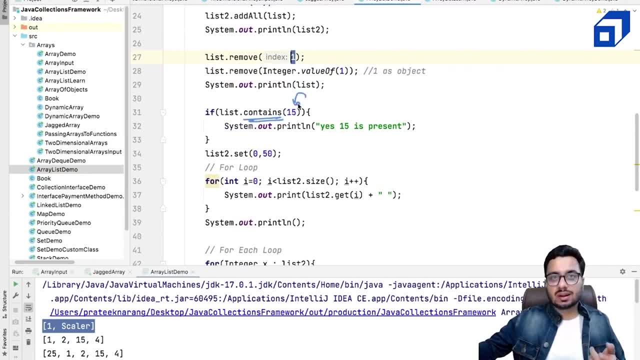 then there is a contains method. We'll tell you, okay, whether the following integer or following object is present inside this list or not. That is your searching method. Now there is one more method that is called as set, So that means I want to update something. 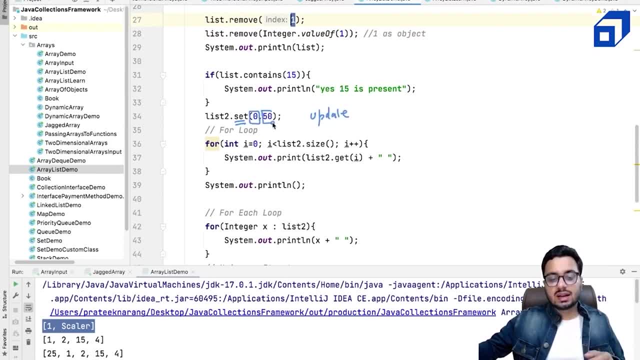 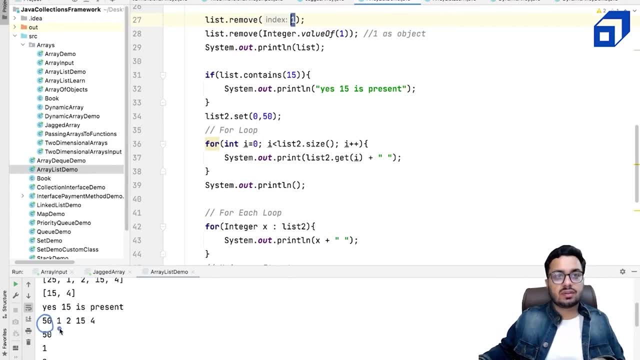 So if I want to say, okay, I want to update the zeroth index and this is the object that I want to store at the zeroth index. If I do this, you will see at the zeroth index instead of 25.. Now, the new element that I have stored, it's going to be 50. And apart from it, we 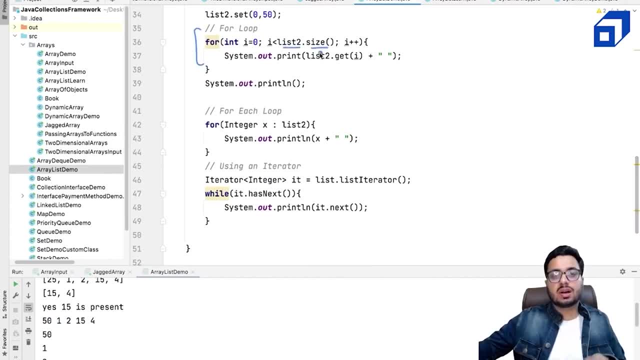 can iterate over the list. So list dot size gives me how many elements are there right, Not the capacity, but how many elements are currently present. That will give me- and I can use the get function to get the ith element from this list- That 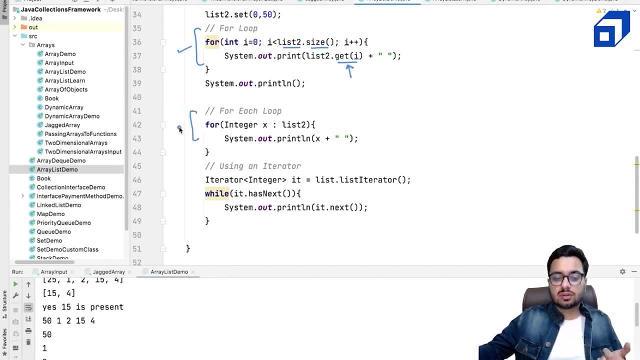 is one way of iterating over an array list. You can also use a for each loop if you want to iterate over the entire list. And third ways: you can also create an iterator object And while iterator dot has next, so has next tells me whether the next element is present. 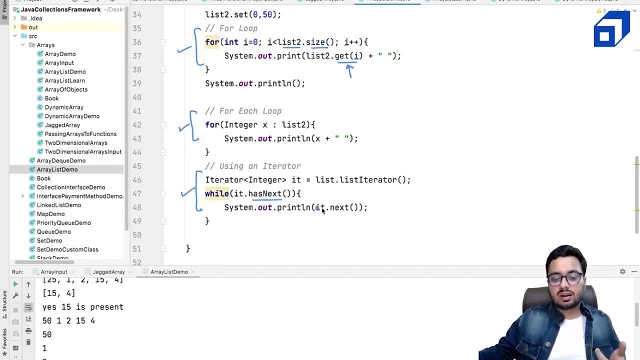 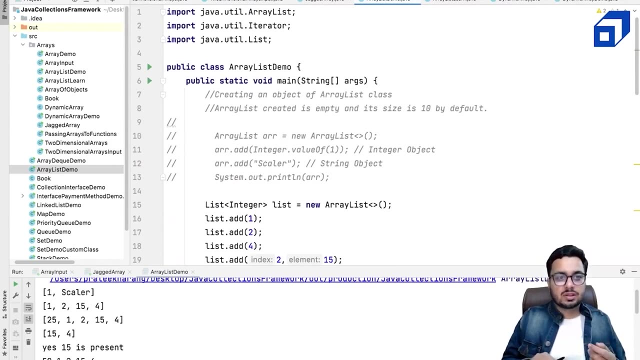 in the list or not, While it has elements, keep on iterating and you access the next element using the next method. So that is another way of iterating over the error list. So you can use this methods and you can work with error list while solving a lot of problems. Okay, So that is about 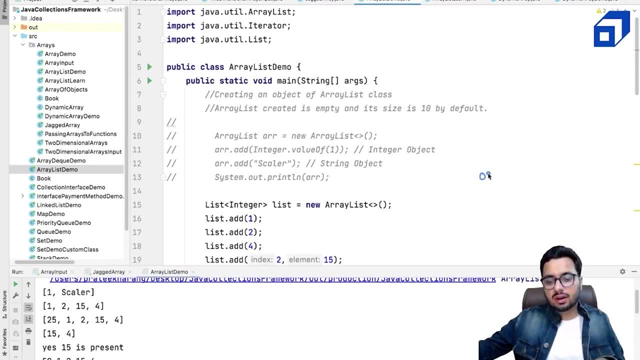 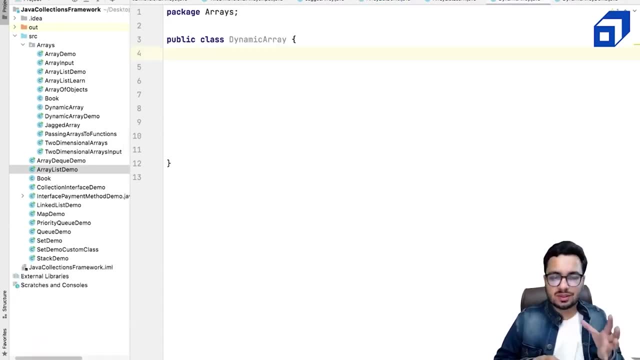 error list And, if needed, you can also refer the Java Oracle docs to go in more details of these. Let us come to the final part of this tutorial. So you so far you have worked with arrays, you have worked with error list, And now I want to show you, if you want to. 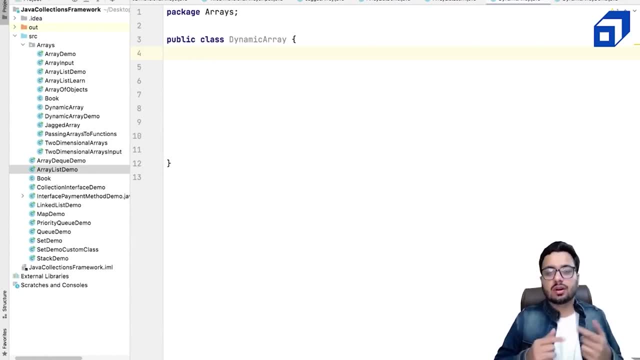 build your own dynamic array class, just for your better understanding of error list. was you're asked to implement an error list at your own, how you would do it? What we want to do? we want to implement a class called as dynamic array. What, what thing we learned? 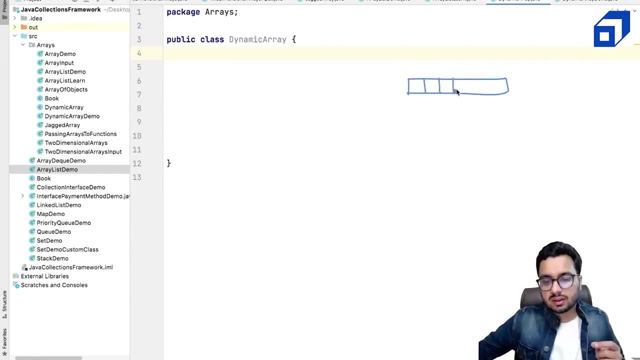 First thing is it internally uses an array. That means one data member of this class would be an array And this array would have some size. also, we will okay, it has some default capacity, right, This capacity And we provided by the user or we. it can have some default value as well. we will look. 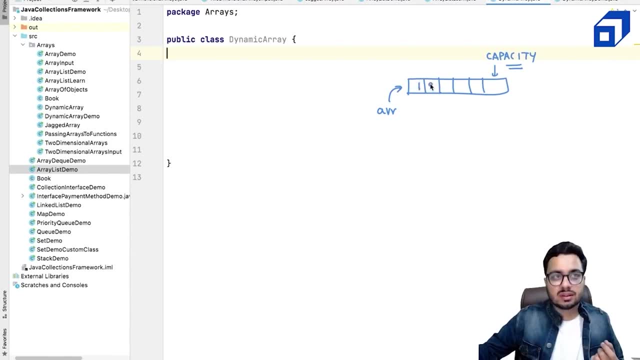 at that And then if you start putting elements, start adding in elements in this area you also need to maintain how much errors fold. maybe current size? maybe the current size is 3012.. If the next element comes, can I insert it at the current size index, Can I? 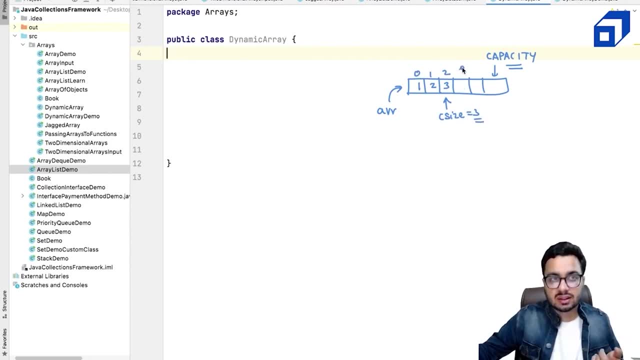 insert it at the third index. Yes, I will insert it at the third index. it is, the element is four And I will increment the current size right. So it is clear that I need one data member. that is one data member that is current size, one data member that is capacity and maybe. 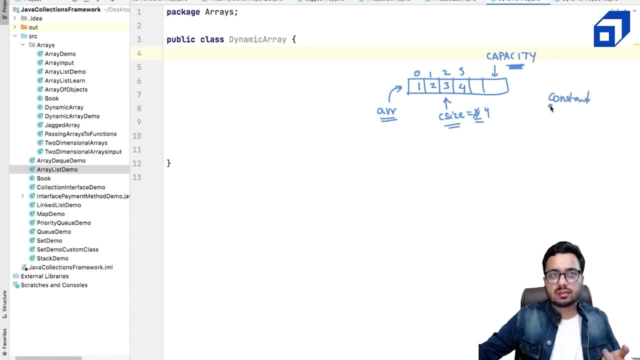 one constant where in which is going to store how much would be my default capacity, that I can call it as default, So, by default, the capacity of this area should be. so let us create these data members. I've created an array, Right, I've created a capacity, I've created current size and I've created a default for. 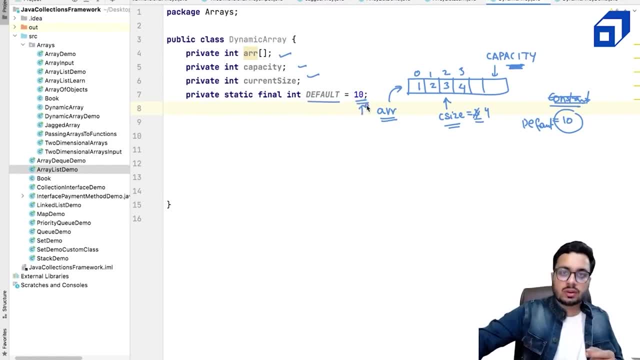 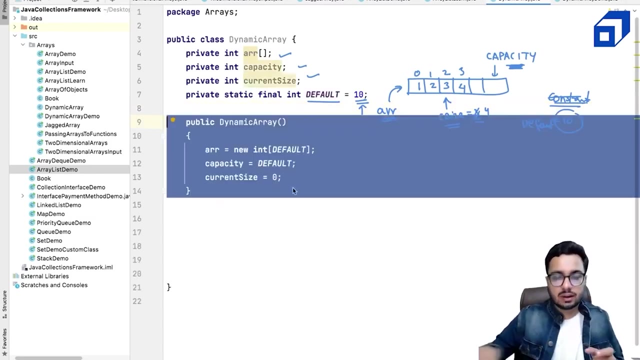 which the value is 10.. Now user says: Okay, I want to create a new dynamic array object. how you're going to initialize these variables? okay, Suppose I do not give you any default capacity, I will need a constructor. And in the constructor what I will do: I will initialize. 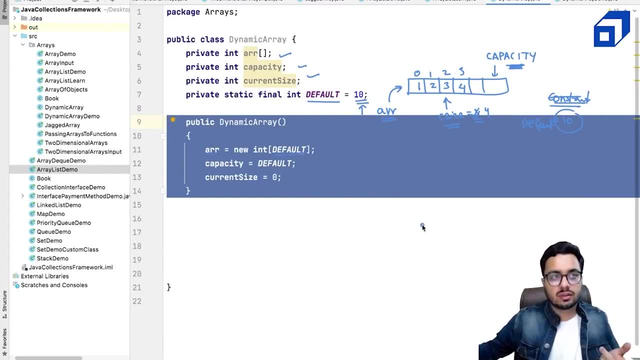 my array equal to the default size. Default of size 10 is okay. the capacity variable is also equal to default, right? Why I need this capacity? because capacity can keep on changing. If n size 10 gets full, I will make it 20.. If 20 gets full, I will make it 40. The capacity will keep on doubling. 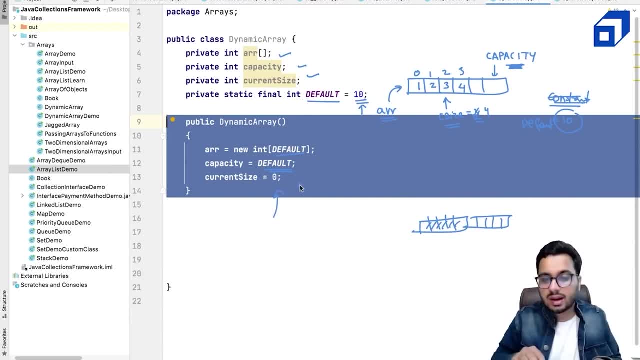 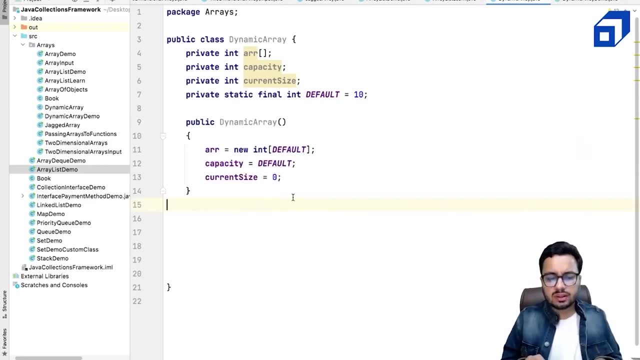 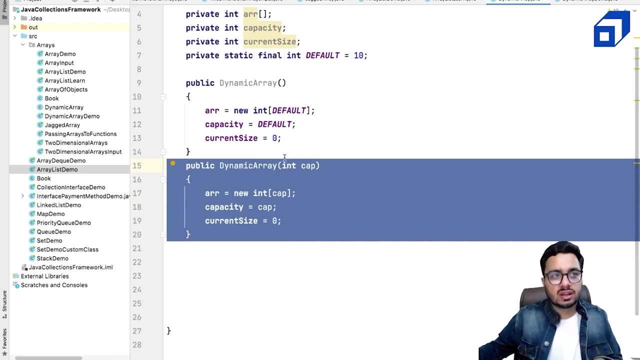 and current size. that is going to be zero. right, Because I have not added anything. But suppose if the user says, Okay, no, I'm going to give you the default size of the array. then how do I do it In the constructor? I will accept. Okay, you tell me the capacity. 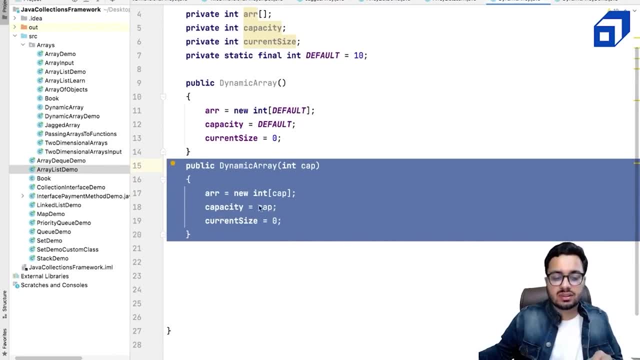 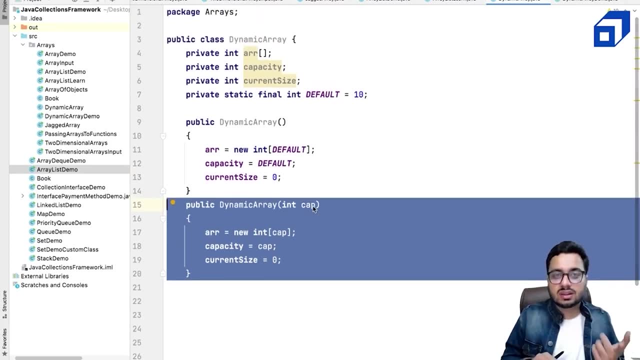 I will initialize my capacity equal to that capacity and I will create an array of that capacity. right And current size is still zero. Okay, so that is how the constructor is getting created. The third constructor, in which I get another list and then I create. 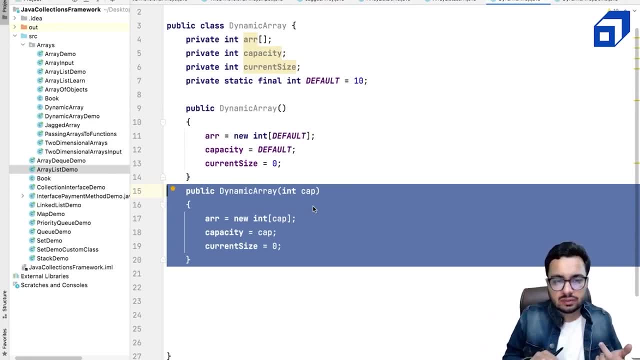 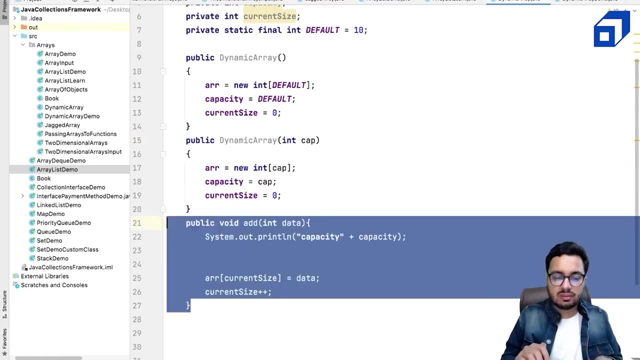 this array. I'm not creating that. I'm writing a simplified version of an array list. Now suppose I want to add something into my array. How should I do it? Very simple, I will define a method called as art, And I will. I'm just. 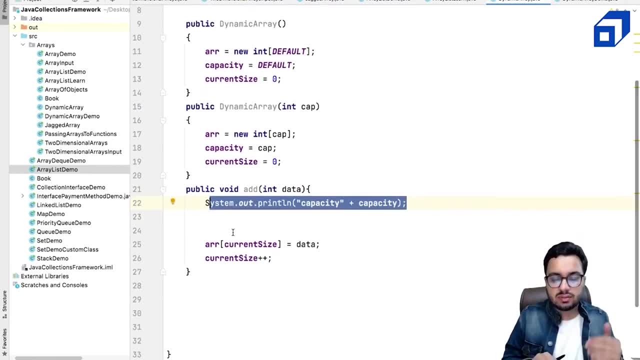 printing the capacity as of now, but I will remove this statement so that we can see while running the code I can the array of current size. this is equal to data Basically, in the beginning my current size, it is zero And I get some data. let's say data is five. 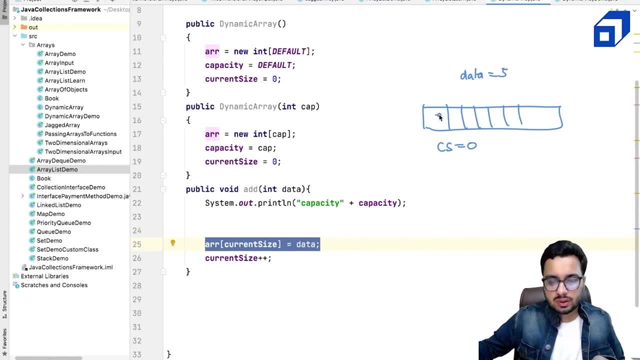 I said fine, array of zero, this should be equal to five. And I say current size plus plus, so my current size becomes one. So that means next time I will do insertion here Again. I get a data that is six. What I do, I put it here and 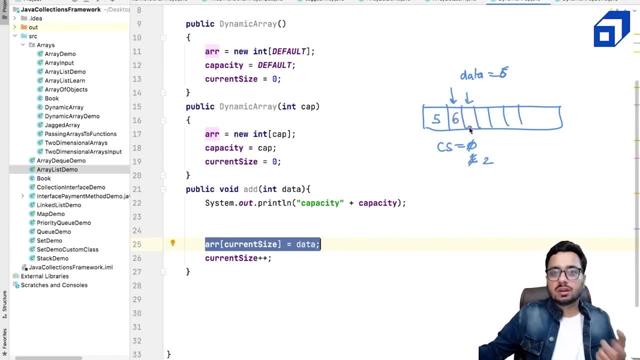 I increment the current size to the next time. my insertion will go here. Now suppose I keep on adding elements And after some time my current size becomes equal to the capacity. So my capacity was 10. And my current size is also 10. That means I have already inserted. 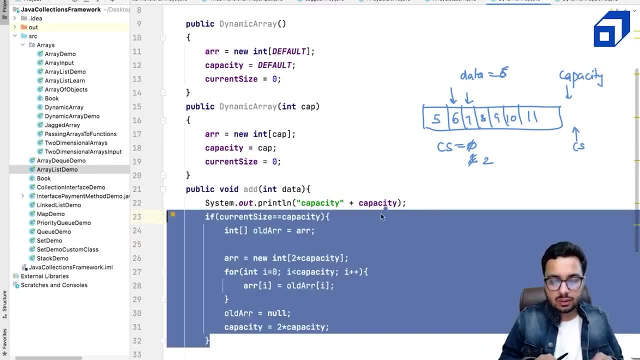 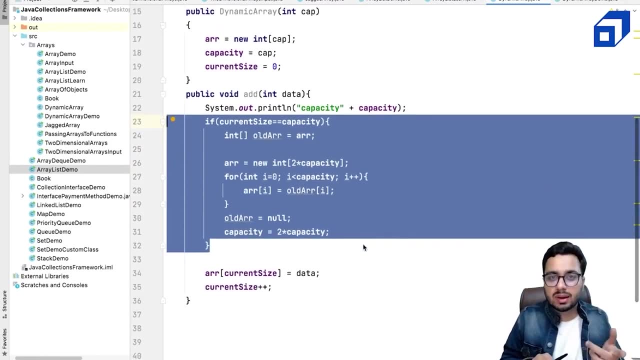 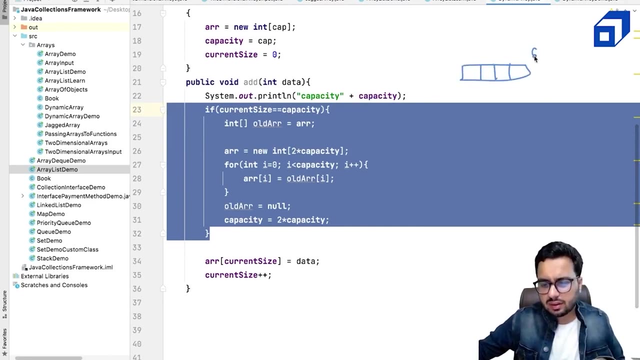 10 elements. If something like this happens, I'd okay my current size. it's going to be equal to the capacity. what should I do? I need to double my array. How do how I am doing it? let us try to understand that. So let's say I have an array of size of capacity, for I 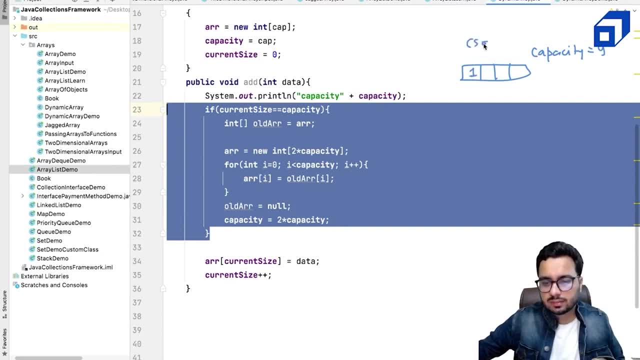 insert one element: current size becomes one. insert one more element: current size becomes two. I insert one more element: current size becomes three. I insert one more element: current size becomes more. current size is equal to capacity. If this happens, and this: 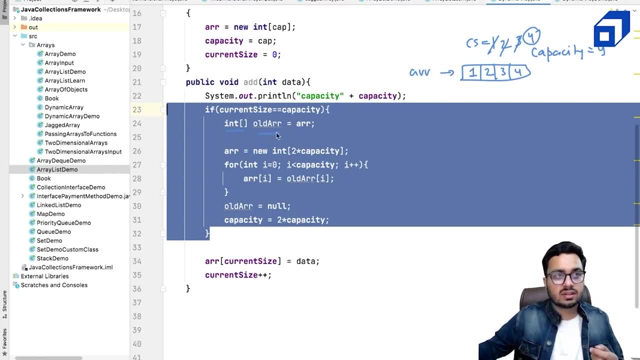 is my ARR. what do I do? I create a variable called as old array. I say, okay, old array, pointing to this ARR, the old array. then I say ARR, which is the data member of the class. it should refer to a new array which has a double capacity. it should have double. 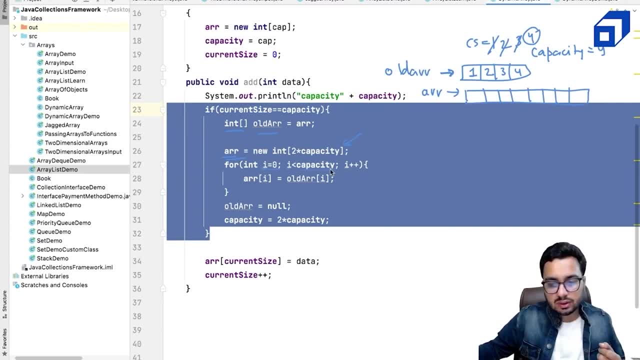 capacity. So that is what I do here. Then I iterate over the old array. old array, I iterate over these elements and I say: array of i, this is equal to old array of i. I copy all these elements here. okay, fine, I do it. what should I do? I say: old array, this is equal. 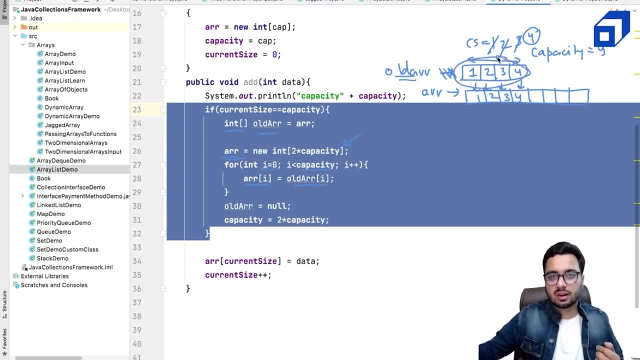 to null. so I break this connection. that means no one is pointing to this array now the garbage collector will delete it. here the garbage collector will get invoked and of course, for the new array we have updated the array property, but we have not updated the capacity property. the capacity 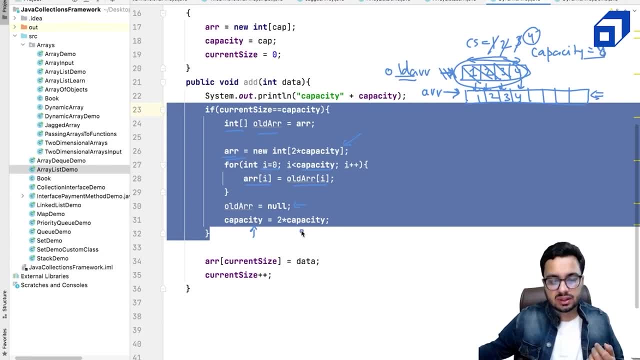 was still 4, but now the capacity should be- I'm saying capacity equal to twice of capacities. what? what do I do? I first check if my array is full, I double it and then I can insert data into. I say array of current size. array of current size is still 4, so 0, 1, 2, 3, 4. at the fourth index I can. 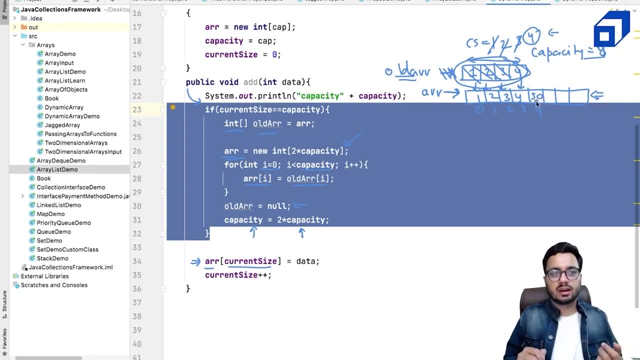 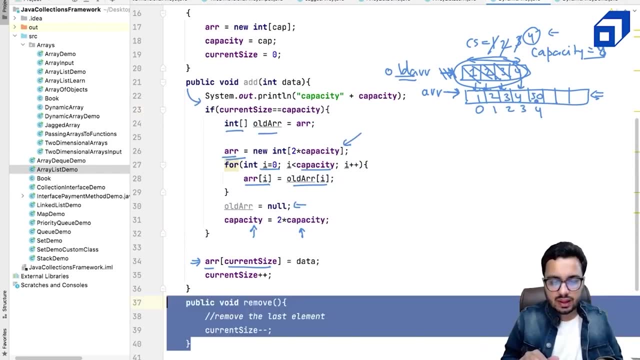 put the new data. maybe the data is whipped. I put it. that is how I implement the doubling of the new array. so I put it in the new array and I put it in the new array and I put it in the operation inside my array. now suppose I want to remove something, so removing is easy, right, I'm. 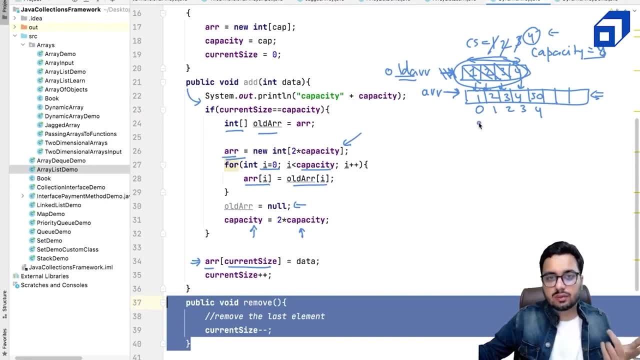 not removing from an empty array, so that check you have to. either you do not, either you put some conditions here or you throw an exception right. I'm simply saying okay, I want to remove an element. I'm simply removing the last, last element. so this is my current size. I said, okay, I'll reduce the. 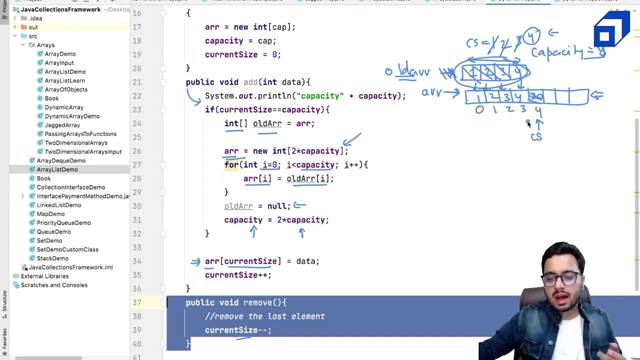 current size and it means, okay, I am going to remove an element. and I'm going to remove an element one step back- current size minus minus. so I'm removing one element from the array. the element will stay here, but next time you add something it will get overwritten, okay, and if you have to, 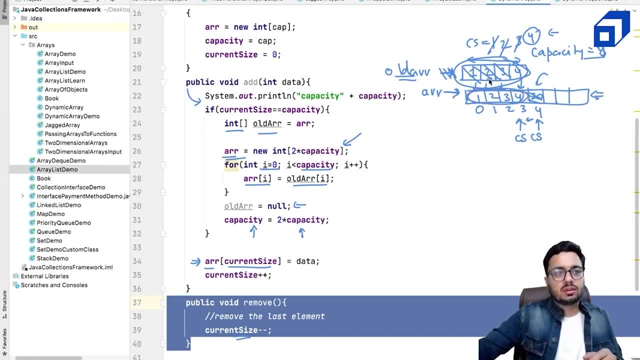 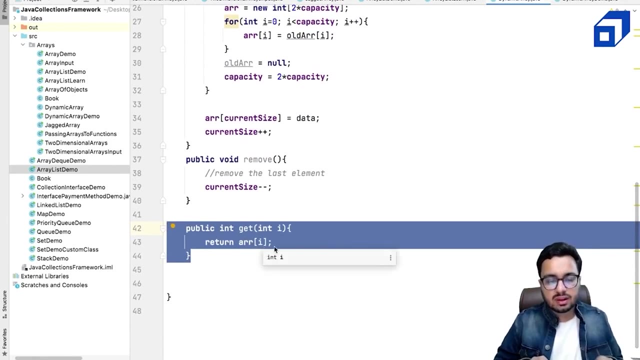 iterate. you will only iterate on on this range. doing current size minus minus will remove the last element as well. now there are some more methods we can implement. for example, if I want to get the ith element, that is pretty easy. you simply return array of i. if I want to get the capacity, how many elements my array list can hold, I can say: 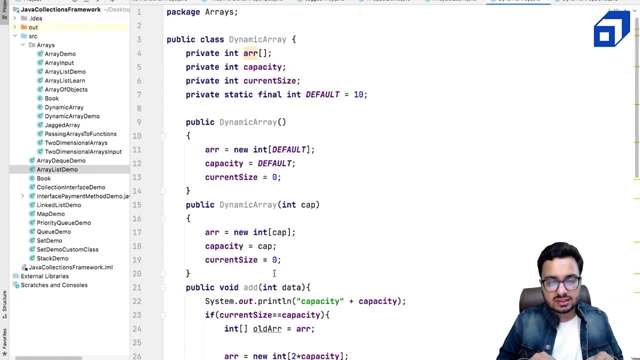 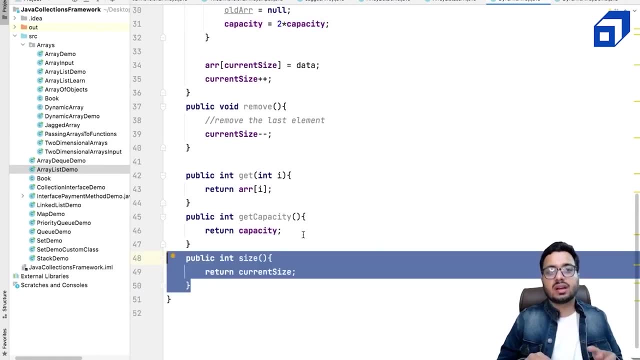 return the current capacity. I cannot use accesses directly because it is a private variable, so I have created a getter to return it. then if I want to get how many elements I currently have, I say okay, there is a function called size that I have implemented. it is going to return the current. 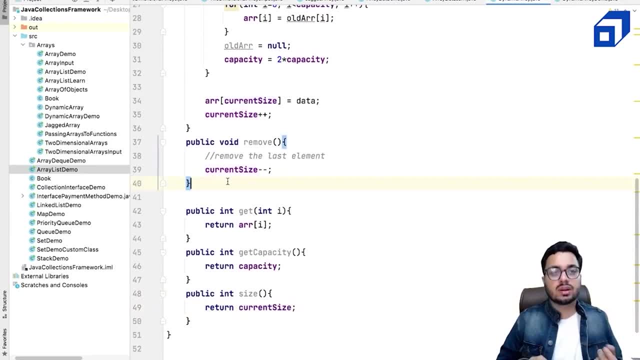 size. now you can create more methods. you can create a method called contains, in which you will implement linear search and you will tell whether that element is present or not, if you can implement a method called as index of, in which you will return the index of the element where it is present. so 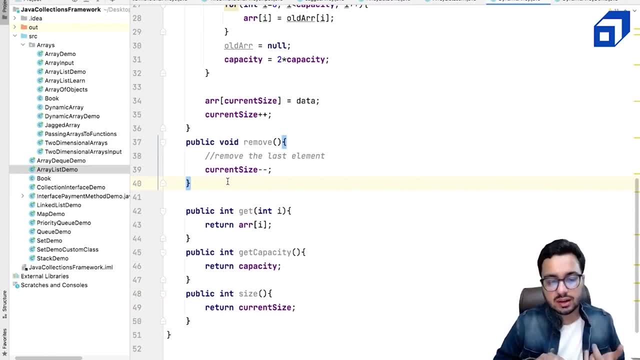 instead of returning a boolean, you can return an integer index as well, right? you can also overload the remove method, where you will get a integer value. so either you remove the element at that index or you remove that value, right, so you can do something like that as well, right so? 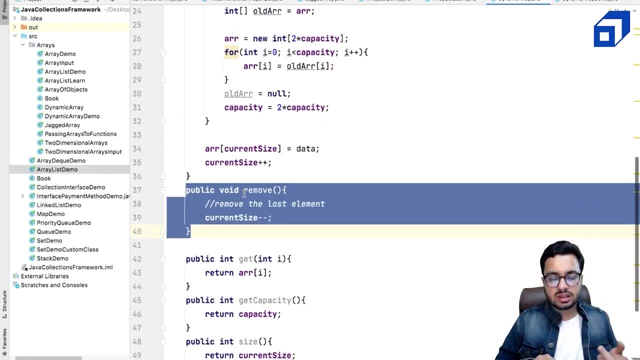 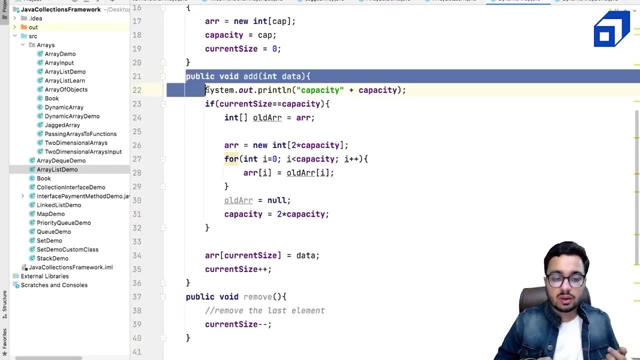 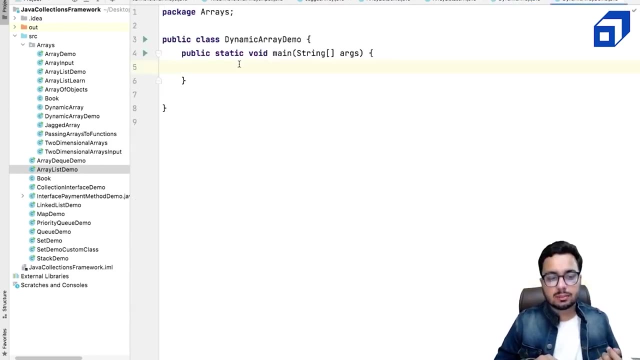 so I want to control the data, to go to the求 in this run feature, byakan, to test it here. the task par elements itself and perhaps I can also define the data. so that's how this text data creation is incredible. okay, let's test the mobility things. so let's say, now I'm working within an array. 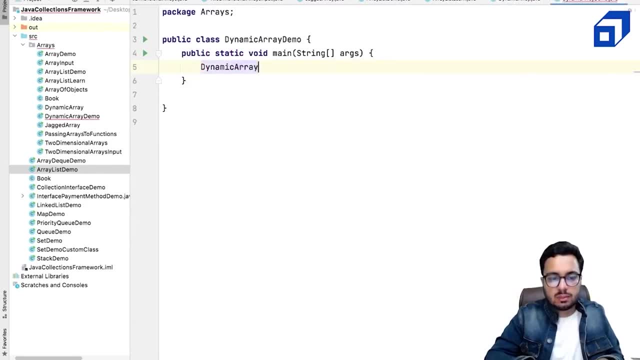 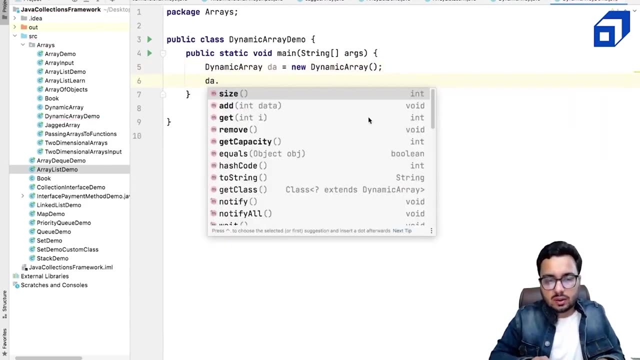 jenizlar tag class come into edit folder. let's comment on others. ok, so if we click on somebody, da this is equal to dynamic array and i want to use some methods inside it. now let me say default size is 5 instead of 10, so default to, as it is 5, da dot add 1. let me just add 5 elements. 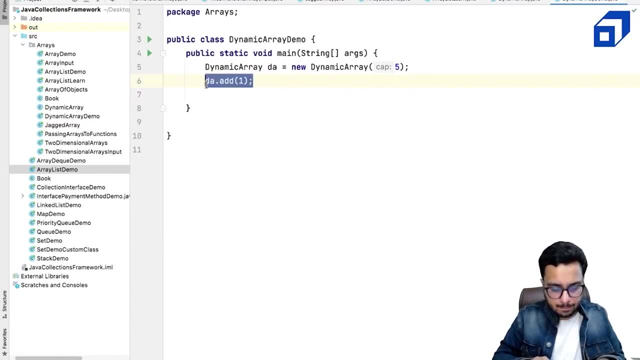 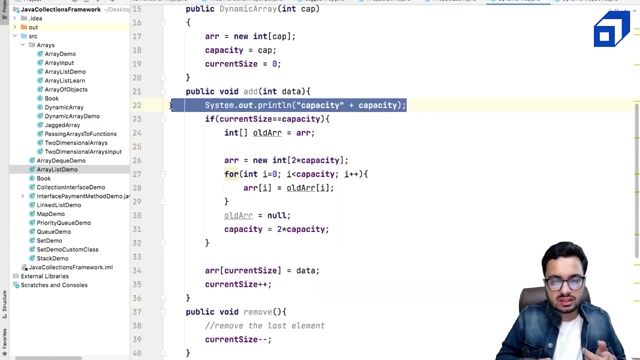 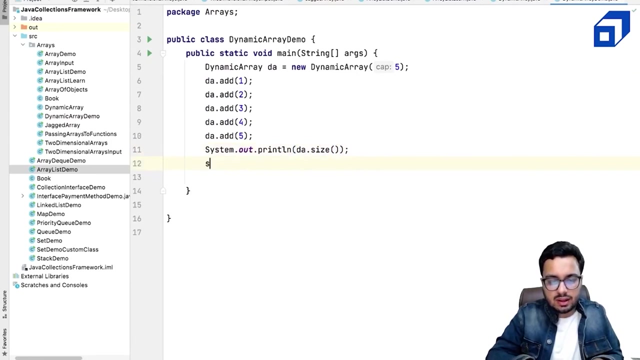 let me say 1, 2, 3, 4, 5. now, at this point, i want to see what is the size of the array and what is the capacity of the array. let us see sout da dot size and sout da dot capacity. both should be 5 at this. 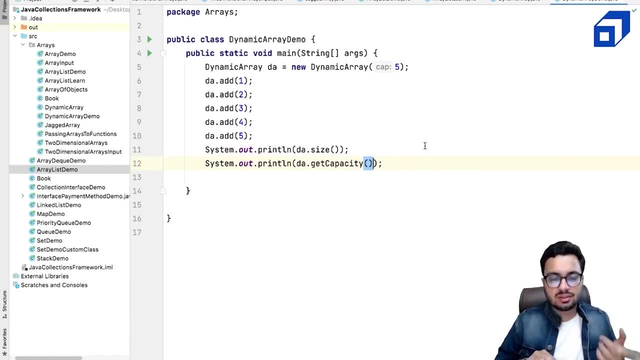 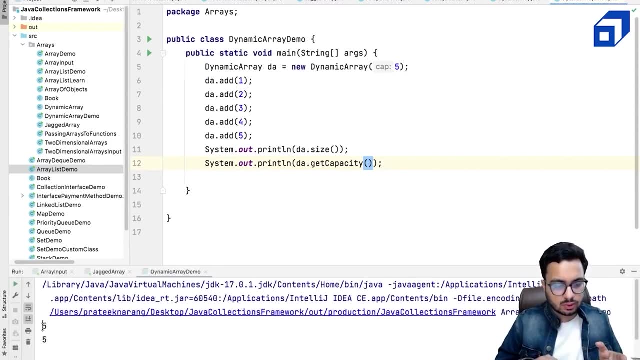 moment. but as soon as i insert the sixth element, the size should be 6 and the capacity should be uh, okay, so both are 5 at this moment. let me insert one more element. let me say: da dot, add 6. and now, if i add this element, you will see the doubling operation will get triggered. 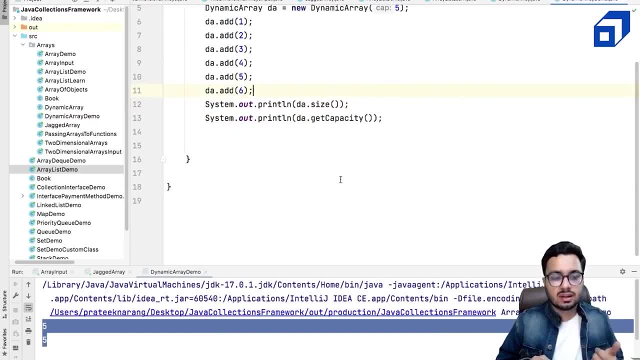 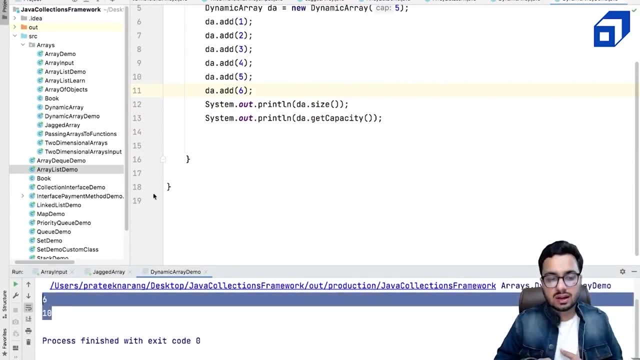 right, that means the capacity should be now 10, the size should be 6. yes, that is happening it. so your array of size: 5, it got full and as soon you add sixth element, it doubled itself. that doubling thing is happening, right, you can see here. now i can also say: okay, i want to add 7. 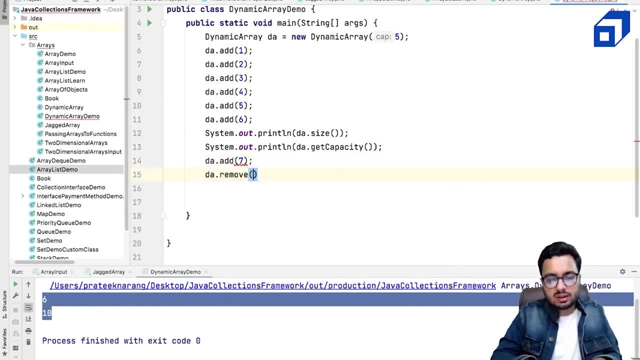 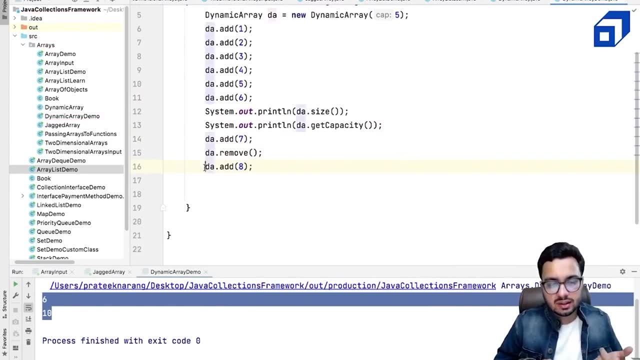 i want to remove the element and i want to add 6, and i want to remove the element and i want to remove the last element and then i want to add 8. that means i added 7, i removed one element, i added it, so 7 will get overwritten by 8. and if i want to iterate on this array and 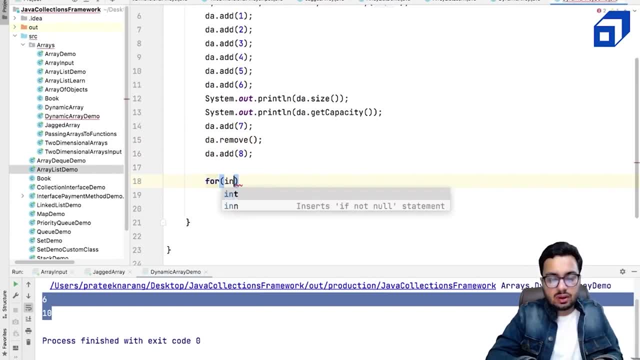 see it, what all elements are there. so i can say: for int, i equal to 0, i less than n, what is n? the number of? uh, basically da dot size, the number of elements present, i plus, plus, and i can say s out: i want to get the ith element. 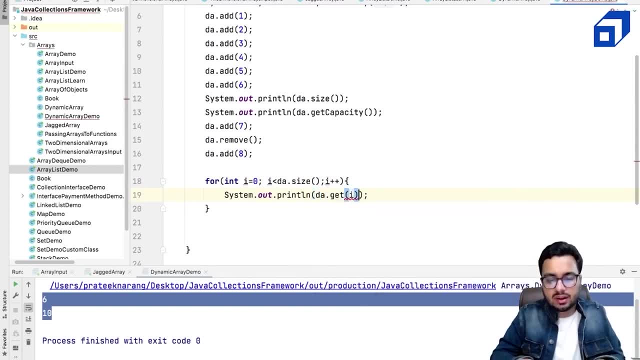 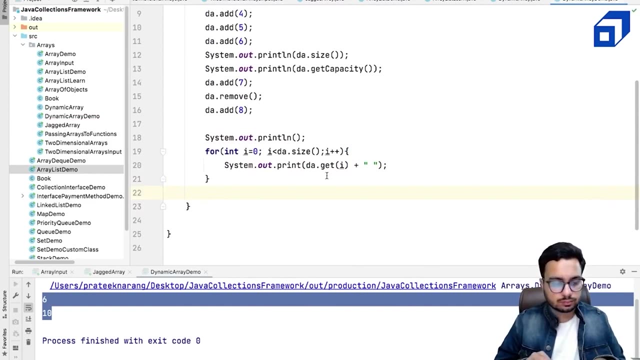 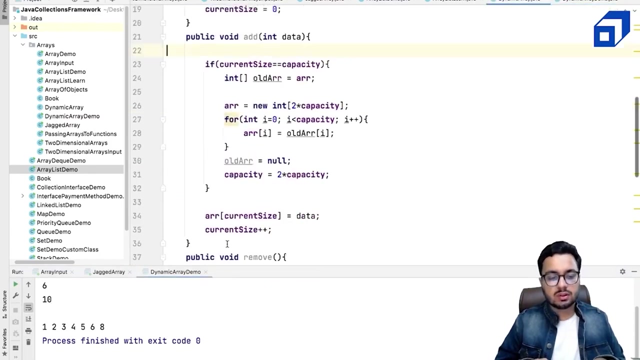 so i can say: da dot get ith element. i want to show them in a straight line. i'll do s out here and like this so you can see: like one, two, three, four, five, six, seven, eight. now you can also implement a method called as two string, which will, uh, simply iterate over the array and join all. 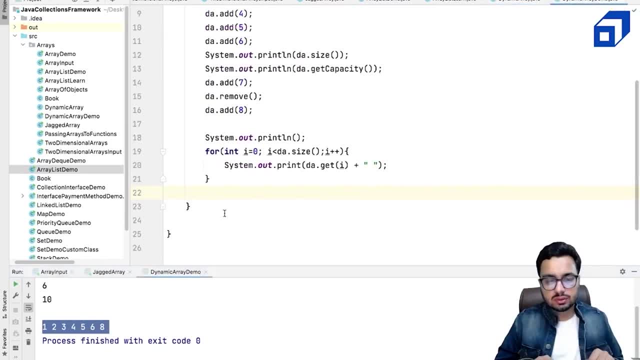 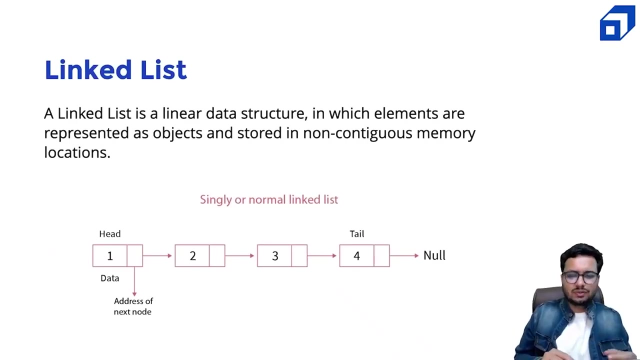 these numbers inside a string, so you can use the two string method also to print your dynamic array, right? so instead of traversing, you can give this as a method inside the dynamic array class as well. let us begin with linked list. what is a linked list? a linked list is a linear data structure. 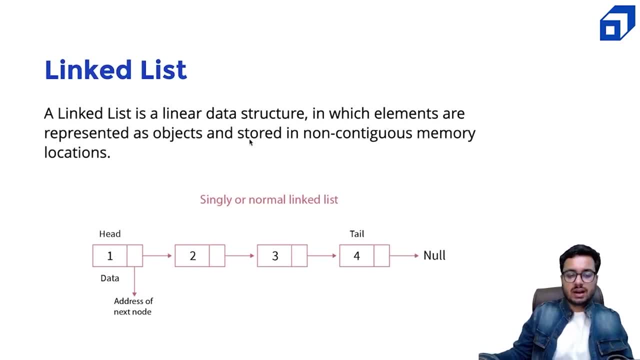 in which the elements are represented as objects and they are stored in non-continuous memory locations. okay, so one thing that you need to note about linked list is: it's a dynamic data structure, right? so unlike an array where you need to tell: okay, i want an array. 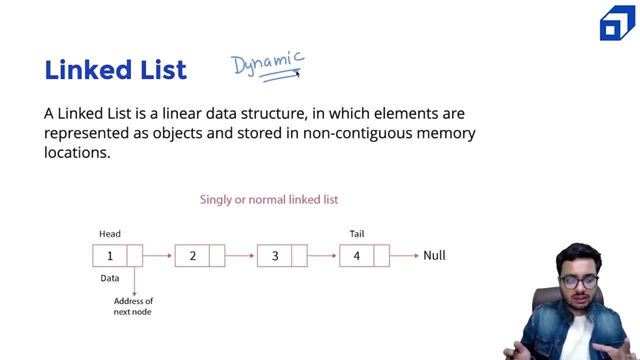 of size n. you don't need to specify the size of the linked list. every time you get a data, you create an object, you put the data inside it and you put it in the form of a chain or in in the form of a linked list, right? so why the name linked list? because we have lot of nodes. okay, each node is: 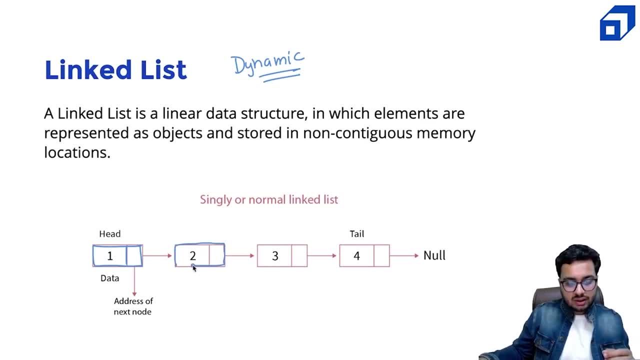 a object in a heap and these nodes are connected with each other, right, how they are connected, so each node is created at some memory. let's say this is a data structure, right, so we can write it in a name. the address is 205, so the previous node knows that the next node is present at this. 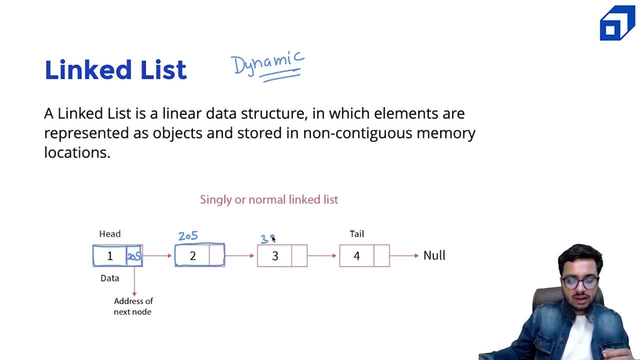 address. right, so two will know: the next node is present at some address, so that is also going to store there, right? so each node is going to store two things: one is your data and one is the address of next node, right? so if you know the address of next node, you can easily traverse. 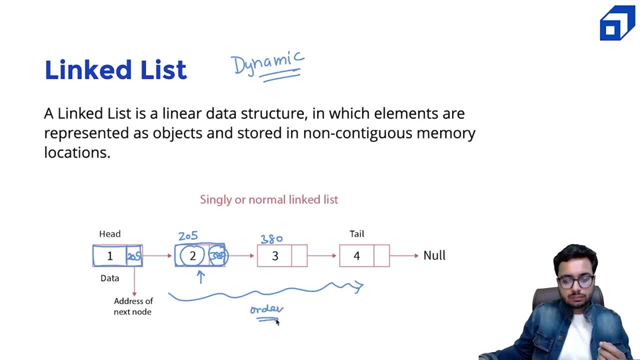 the data structure and you can also put things in an ordered way, right? so every time you get a new beginning, we can insert at the end. we can also insert in the middle, right, so it's up to you how you want to maintain the ordering inside the link list, right? one thing to note is it's a dynamic. 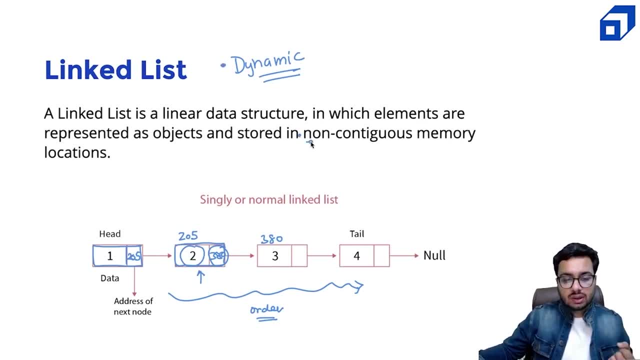 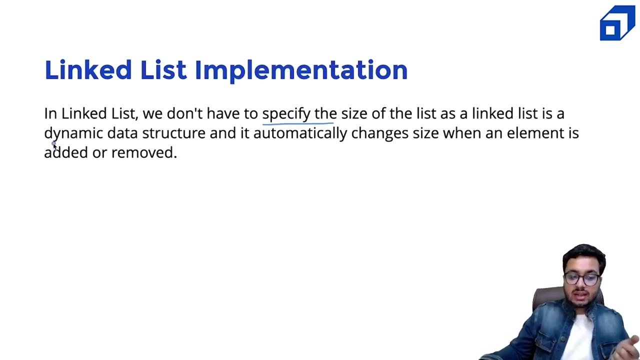 data structure and the nodes in which the data is getting stored. they are stored in non-contiguous memory locations, unlike an array, right? so that is what link list looks like right now. in link list, we do not specify the size, as i have already discussed with you, and it is a dynamic data. 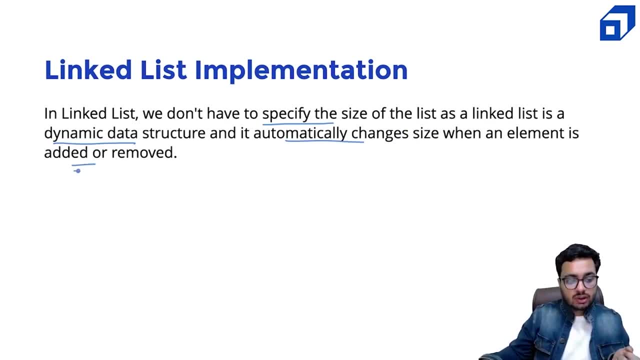 structure. it automatically changes size when an element is added or removed. so we'll go into the internals of how addition and deletions are performed on a link list in this tutorial. so while doing the implementation i will show you that. okay, if there is a node, how do i connect the? 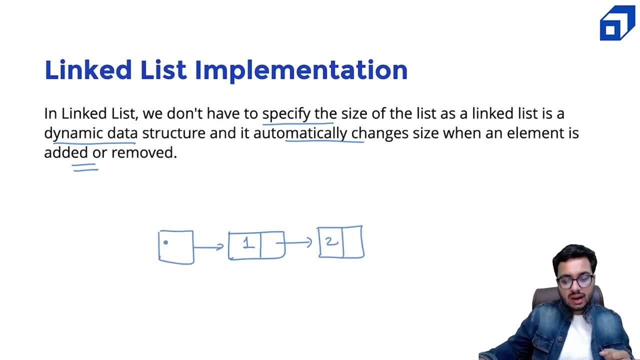 next node: how do i add something in the beginning? how do i add something in the middle? how do i delete something right? so the fundamental operations that we will be learning would be addition- okay, removal right and getting a node right. so i want to get a particular node i can. how do i get that node? 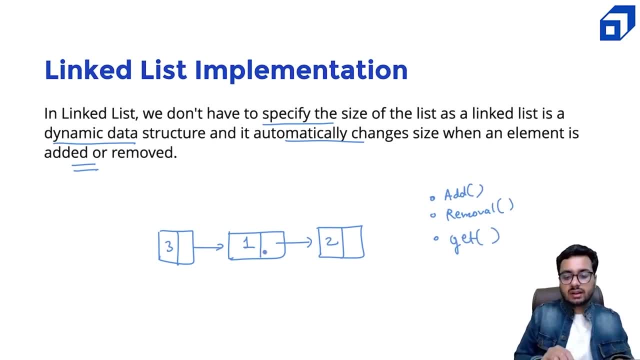 right. so given an index, i can iterate to that index, right? one thing that is bad about link list is if you suppose want to get the middle node right in array, you can say, okay, give me the ith element. so this, this property is called as random access. so link list is a bad data structure if you need. 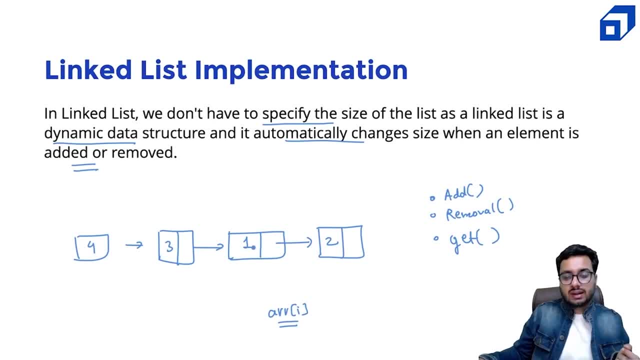 to access ith element. why? because you cannot directly get this element. you have to traverse till i positions to get this element right. so it's it's bad at getting nodes, it's bad at random access, but it is good at certain things that we will see all right. so, that being said, let us jump into the 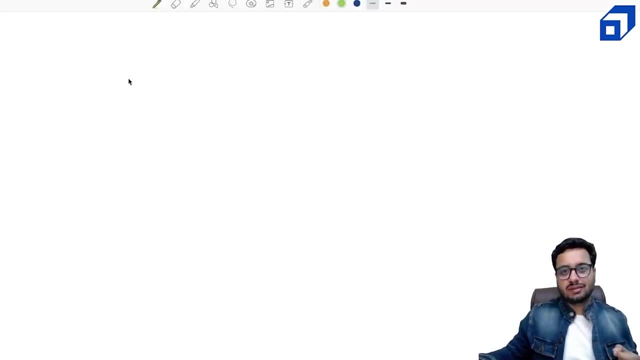 implementation of link list. now let us dive into the implementation of link list. so far, what we have learned is that link list is a chain of nodes in which every node is connected to the next node. okay, if there is a node one, it must be connected to the second node, let's say node two, right? the way to do it is that in every node we also store the link list in the next node, right? so if, for example, if this node is created at some memory location, let's say 206, then this node must store what is the reference of this node where it is created. right, and for the first node what we need. 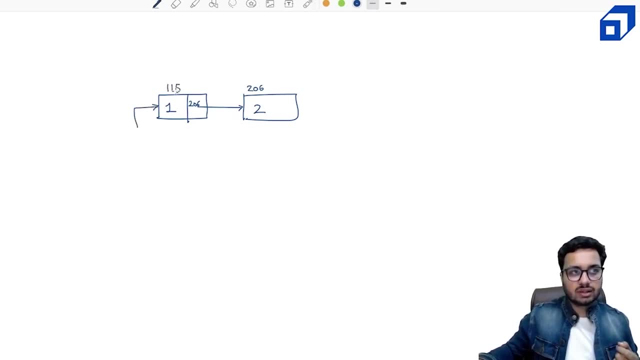 to do. for example, if this node is created at some some location 115, then we need to store this location 115 in a special variable. okay, we generally call this special variable as head, right? okay, and second node will store the reference to the third node and so on. right, so third node maybe. 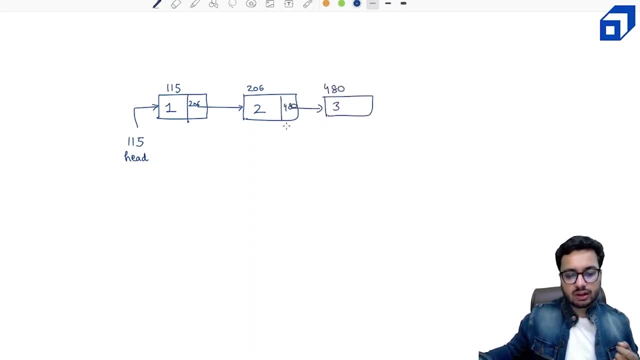 it might be at 480, so i might be storing 480 here right now. the first step in the implementation is that: how do we implement this structure? okay, this uh object that we see here. so we are calling this object as a node object. right, what i will do? i will say, okay, i will define a node class. 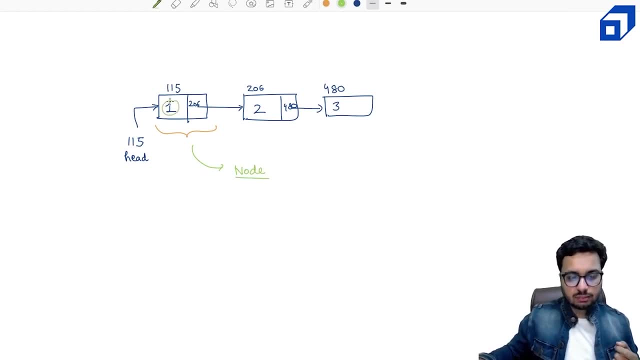 and this is capable of holding two things: one is my data and one is my reference. right, so each of these boxes is a node, right? so each uh node is going to hold a data. now, a data can be of a different type as well, so, just for the sake of simplicity, i'm treating it to be a. 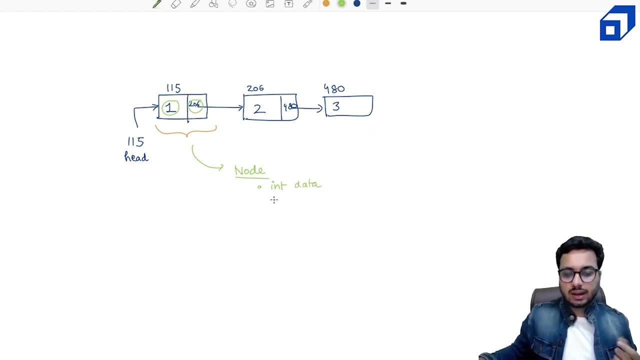 integer, but it can be an image, it could be a book, it could be any object, right? and second thing i have is a reference to the next node, right? so how do we uh, store a reference to the next node, right? so it's okay. uh, this will be of the type node and let's call this variable as next. 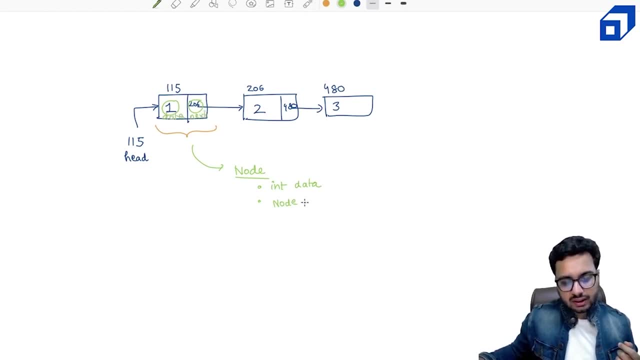 right, we have data and we have. next, if you are confused, i will explain you. uh, what is this concept? so let us first start with the code, let us create this structure and let us try to understand that. okay, inside the node class, you can have an object reference which is holding the address of the next node, right? so let us go into intelliJ. 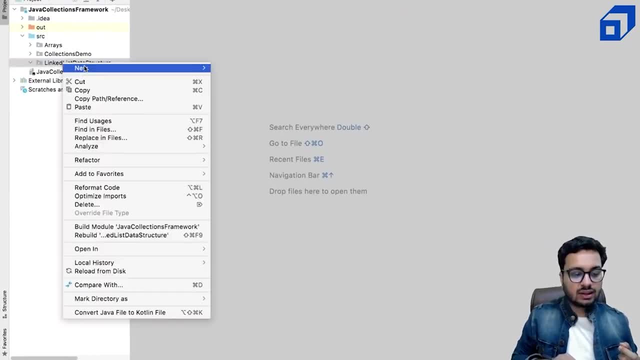 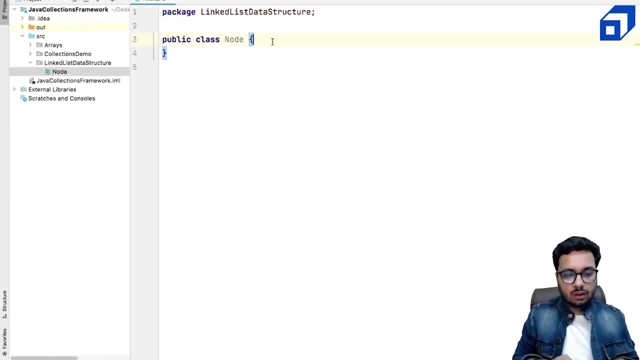 and I have created a package called link list data structure, and here I'm going to create a Java class called, as let's node dot Java. now it automatically creates a class for me, but it does not have data members. so how do I add data members? I can say: okay, I want data and I also want 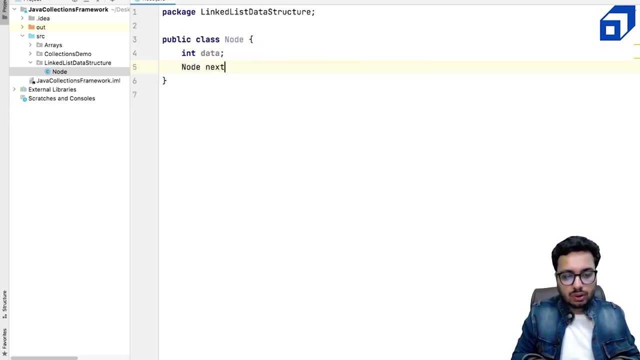 something called as next. so that will be of the type node. now, this does not mean that there is, there will be, an object inside an object. no, this is only a way, this node right, it's only a way to hold the address of the next node right. so this is of the type object reference. I will tell you. 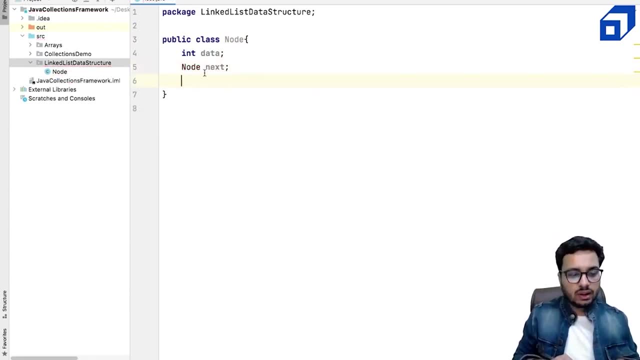 right. and let me do one more thing. let me add a constructor here as well, so you will see why we need a conductor. let's do one thing: let's create main right. let's create a linked list demo, another class in which I am going to test my functionality. in this class, I will create my main. 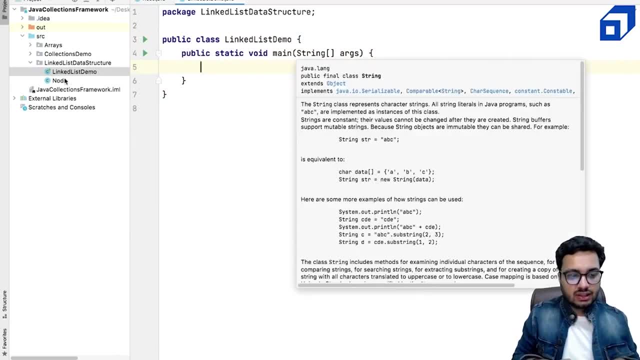 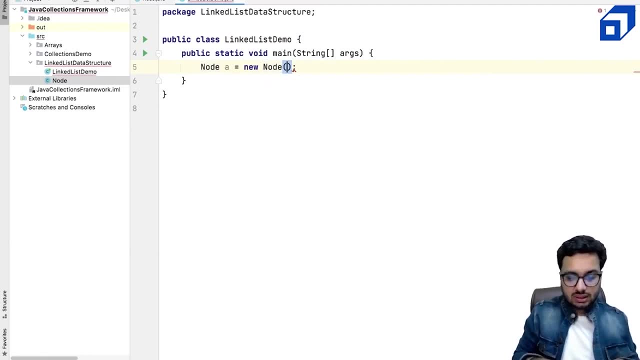 function, and in this class I will create my main function, and in this class I will create my main method where I'm going to test my functionality. right, let us create a node object, that's okay. no day, this is equal to new node. right now, this? no, this does not hold any data, right, so a is not. 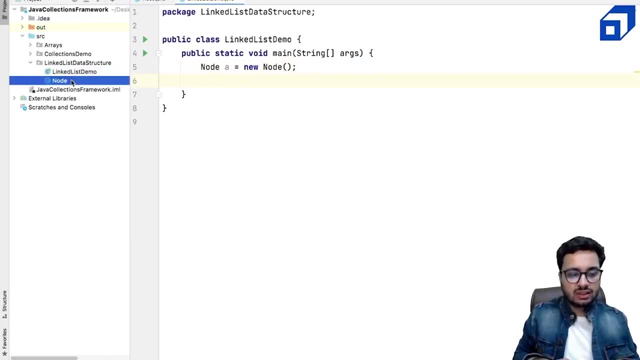 going to contain any data. by default, the value of integer is 0, right, and next would be null, right. so what I can do, I can joke: a. a dot data equals to 5, a dot next equals to null. and if I say, ok, s out a dot data, what I'm going to get, let us see. right, I'm getting this value as 5, which is: 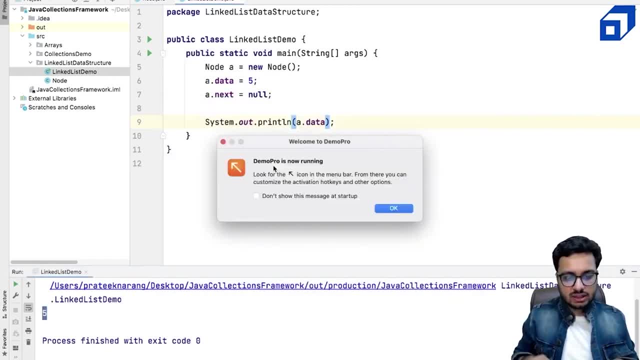 absolutely correct right now why this is happening. let's see what it did writing this code. it created a node right, and what is a? a is referring to this node, so a is a address. it is a object reference, so a is another bucket which is holding the address of the node right. so this I am going to write a. 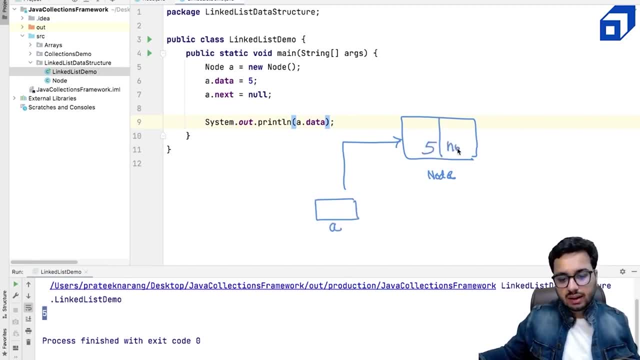 of this node. so this node has two things: one is my data and one is my null. so this is your data and this is your next. and this node has been created at some memory location in the heap right. this is my heap memory, so a uh, this address might be, let's say, five, zero, eight right. 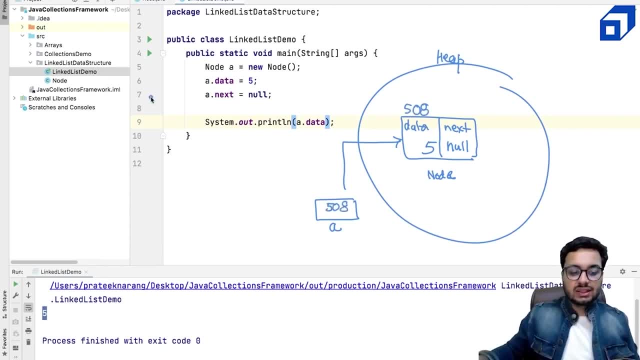 what is a? holding a is holding five zero eight. this is what is exactly happening behind the scenes. so in this case, this a is also an object reference right and it is referring to an object inside that object. i have one more reference. okay, how do i access this value? i access this value by: 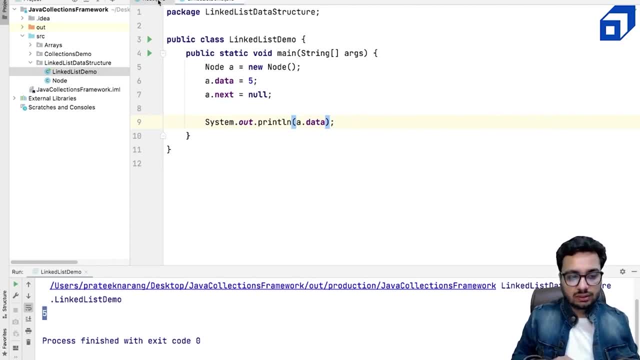 a dot next. so this is what is happening when you are creating this node: right, it is giving you, it's wrapping up two data members inside one bucket. inside node you have an integer value and a reference to the next node, right, if i say, okay, there is one more node, right, let's say, node b equals to new node. 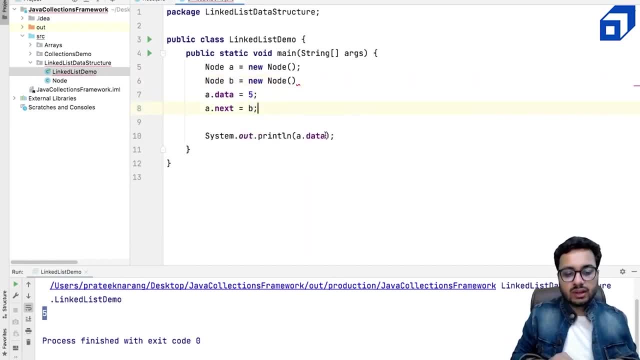 and i say, okay, a dot next should refer to b. so if i print out, what is a dot next? so a dot next is nothing, but it is the address of the b node that we have created, or the value that is getting stored inside b right now. if you see, this is the reference of the next node, right? so 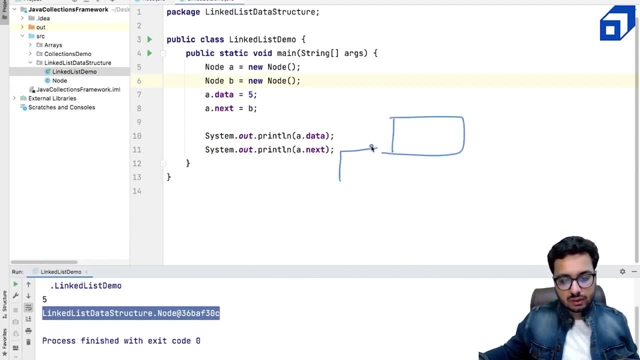 let me show you through a memory diagram. so a is referring to a node. okay, so a is five. b is some other node, so let me do it like this: so a is a variable that is holding this address, let's say 108. this value is 5 and b is 30c. right, so b is some other node. b is another variable that is holding this value: 30c. 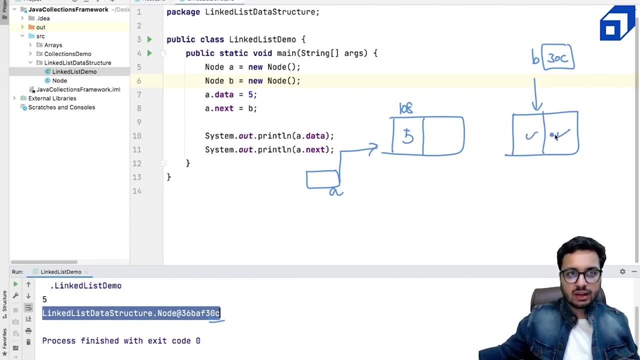 and this is the of next node. I don't have any data and null value, so it will be the default value of integer and next right. so that will be zero and null, right. so I have zero and I have none. now B is referring to this. so when I say a dot, next equal. 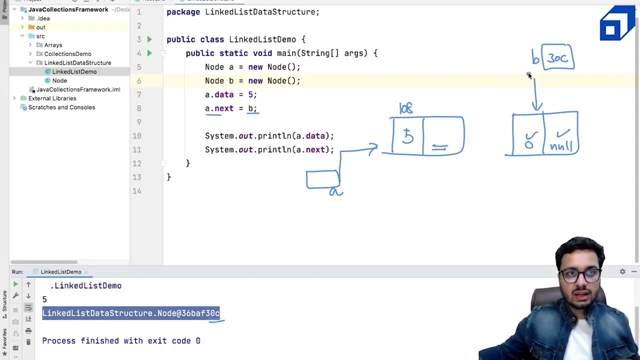 to B. so inside a dot next, which is this field, I am copying whatever is present in B. so I'm copying 30. see, it means in a way this B got connected with a right. even if I lose this variable B, this chain is still connected, right? this is? 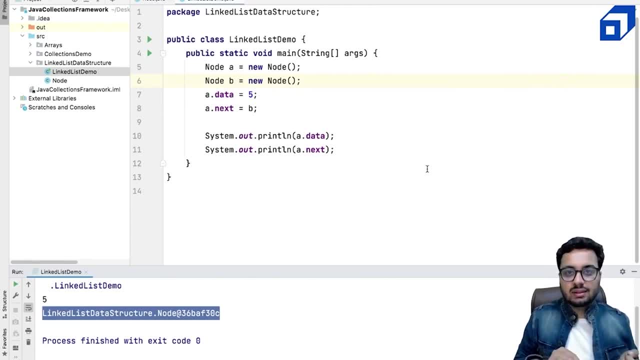 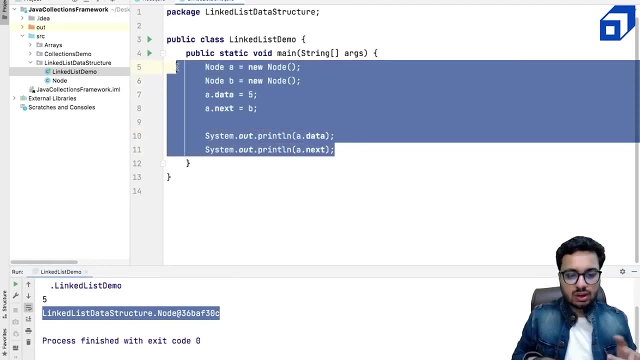 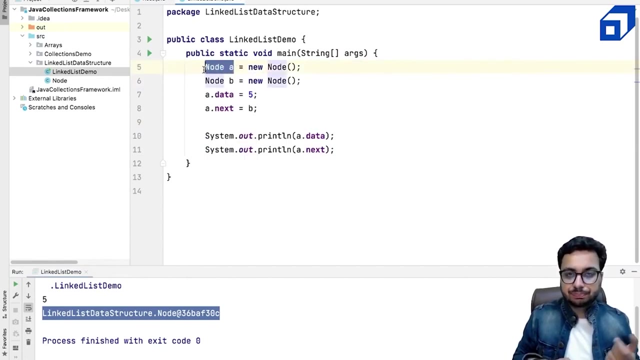 how we are going to work with nodes and we will write one more class that does all this manipulation of nodes. okay, we'll call that as a linkless class, right? so I hope this node concept is clear. what is a? what is new node? the new node is getting created in heap in this case. this is a reference variable here. 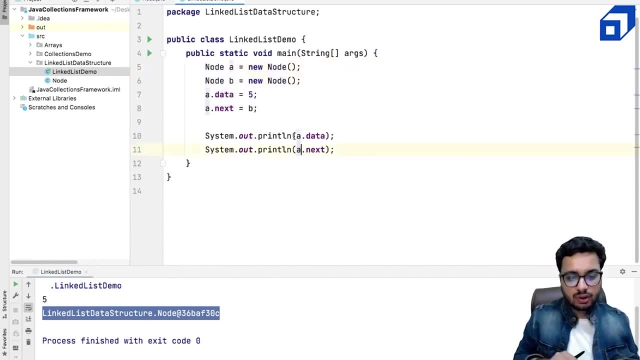 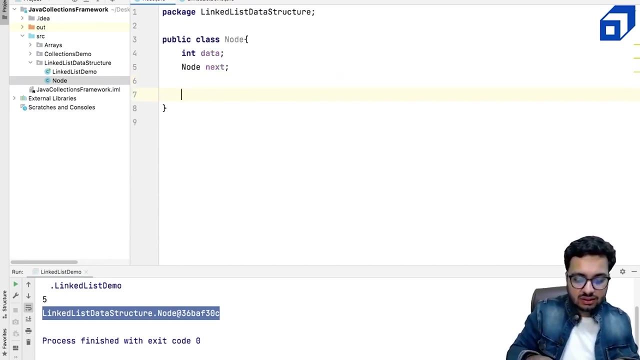 and this variable is created inside stock at this point. right, so what I will do? I'll remove all this code and I will do one more thing: instead of, like every time, doing a dot data equal to something, a dot next equal to something, I will define a constructor inside this. 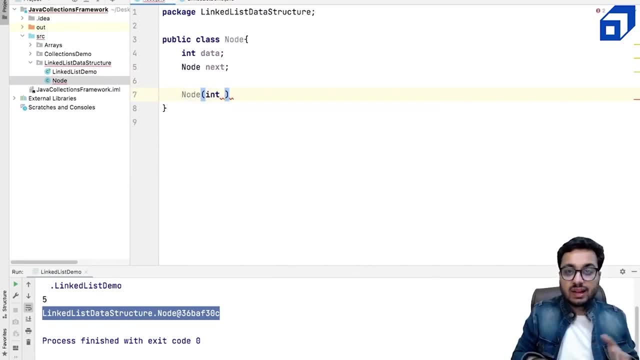 class, so I call it as node. it will accept some integer, let's say data. it will accept some value of next, but in General we will not know that value of next. ok, so whenever you creating a new node, you know the data. so I want to create a new node and you can click on that. it will change values. ok, so that. 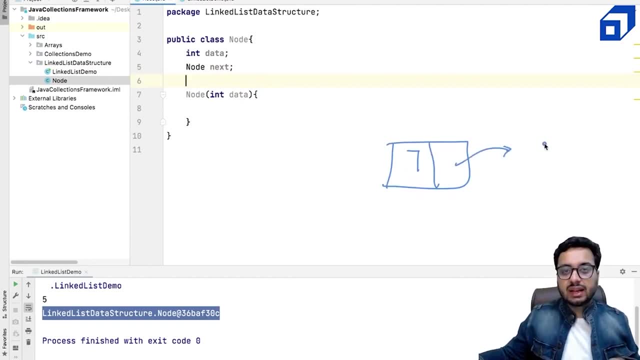 new node with data 7. what will be connected in the next node, we do not know at the moment. right, so what we can do, we can leave this variable initialized with the default value. right, so i can say this: dot data equals to data. so i'm initializing this variable with the data that i'm 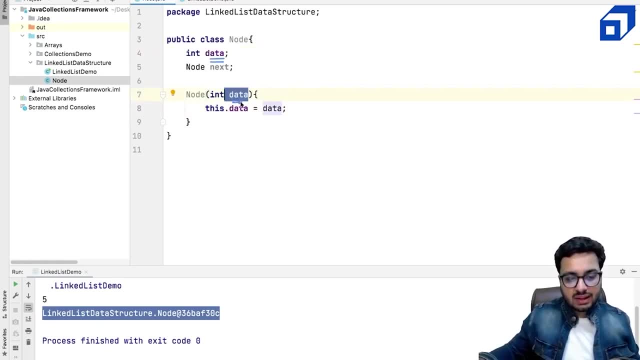 getting right. so since the two variable names are same, writing this here is important, so that compiler knows that we are talking about this data member as a attribute. right and next, what about next? so you can say: next is null, or you can do this dot, next is null. both are fine. 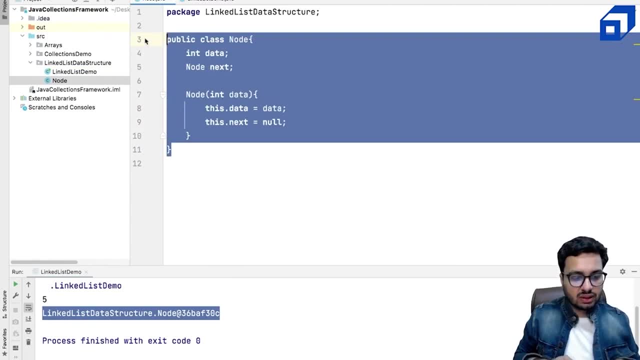 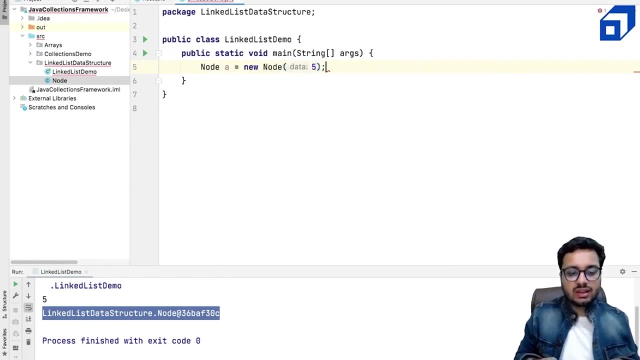 both will work right. this is the constructor for the node class right now. if you want to create a node a now, you will say okay, node a equals to new node. you just give the data as 5 and you say node b, equal to new node, you will say data is 6 and a dot next equal to b. this creates a very simple. 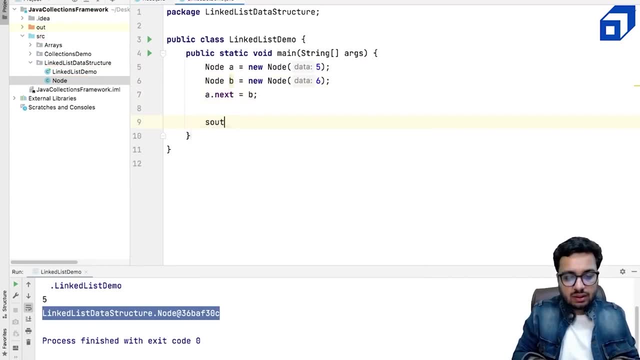 linked list in which we have two nodes. okay, if i say s out a dot data and show me what is the data in the next of a, so how do i do it? a dot next gives me the uh address of b dot data. so i'll say five, followed by six, right? 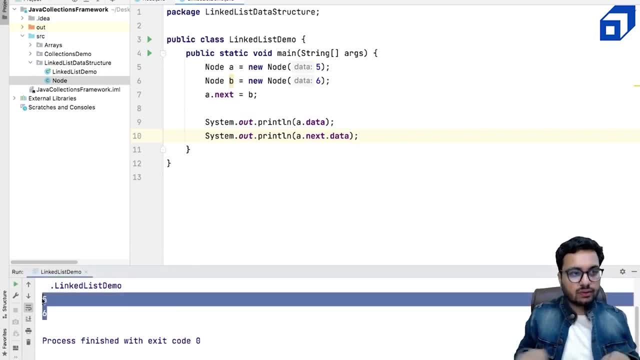 so i will see this. so i see five, followed by six. so what we did? we simply created a linked list in which we have just two nodes. this is a. this is b, right, okay. and a dot next is storing b. so a dot next is storing right now. you might say, okay, this is. 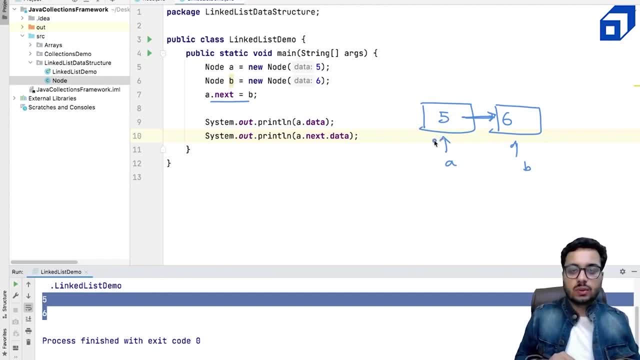 this looks very easy, but if i have to add 10 nodes, 20 nodes, 100 nodes, 1000 nodes, will we create so many variables and attach them manually? the answer is of course no. we will write an algorithm that does insertion in the linked list, deletion in this linked list, and it helps me to get. 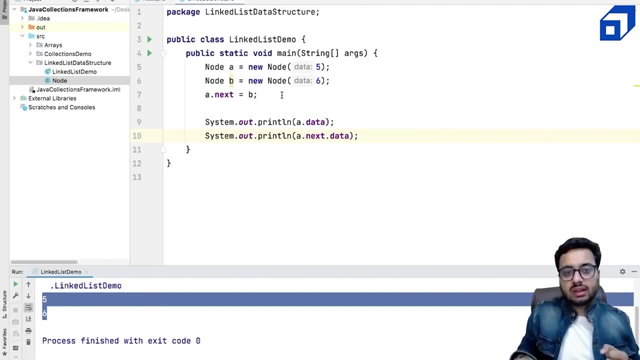 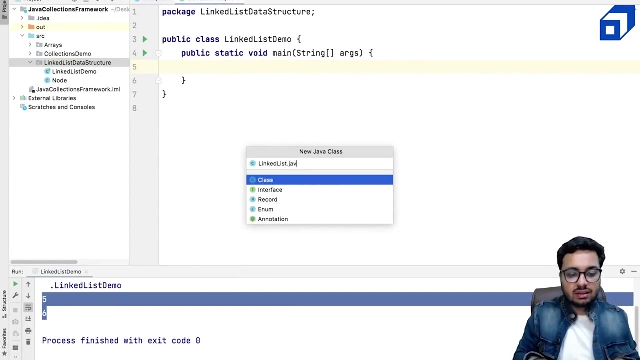 the nodes in the middle of the linked list or end at the end of the linked list or at the beginning of it, the link list right to do all these operations. what we will be doing, we will be writing our own link list class. so what i will do, i will create a new java class and i will call it as link list. 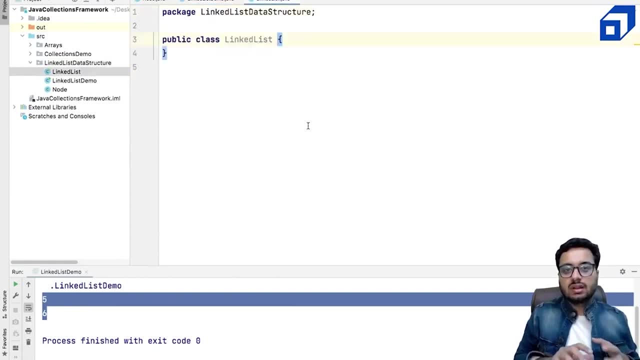 dot java, in which all these operations involving these nodes will be done. right, let's see the implementation of link list. so, let us see the implementation of link list. now suppose you are: uh, you want a data structure that is like in the form of a chain, right, and you want to build. 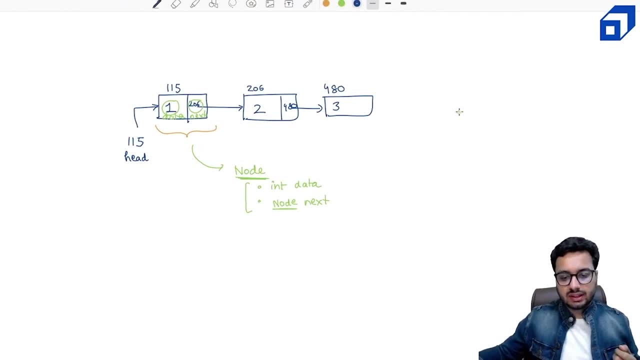 certain methods. you want to say, okay, i want to do addition in this link list. that means i should be able to add more nodes inside it. i should be able to remove nodes from this link list and i should be able to, uh, get the nodes from this link list. that means i want to read nodes from the link. 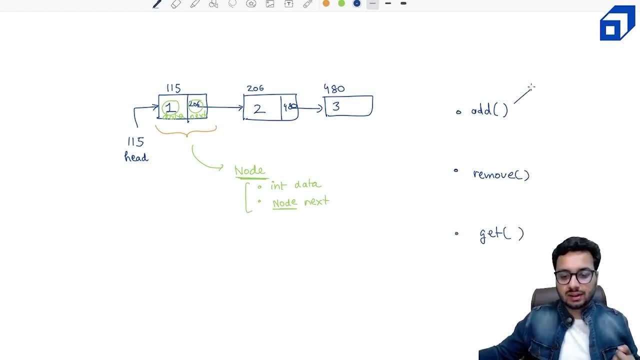 list right now, the add operation. it can happen at three places right to make the operation. maybe if there is a link list like this, you can say, okay, i want to add something in the beginning of the link list. so i can say, okay, add at the first position. or you might say, okay, i want to. 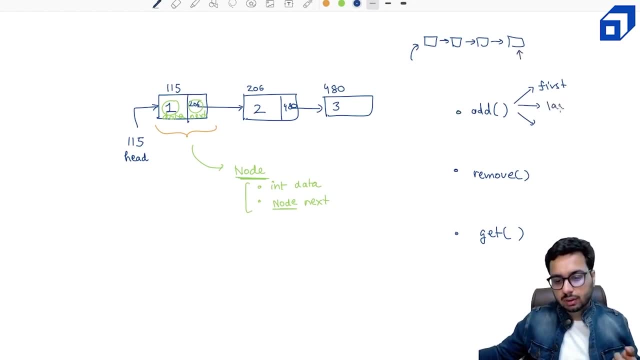 add something after the last node, right. so you might say, okay, i want to add at the last node. or i might want to say that that i want to insert something in the middle, so i might be doing something in the middle or at a given location. okay, add up at a given position inside. 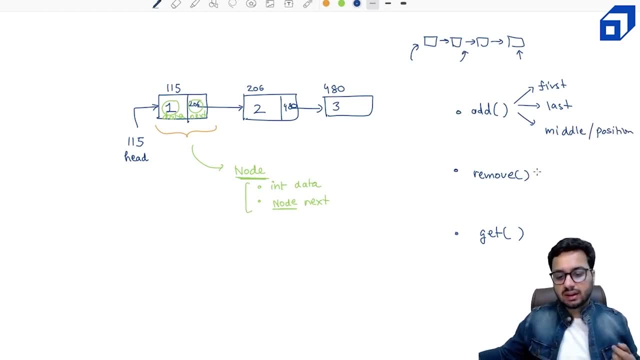 this uh link list right? similarly, remove can happen at the beginning. so i will say: remove first would be an operation, remove last would be an operation and remove at a particular position can be an operation. similarly, get me in the. okay, i want to read something. i want to get the first. 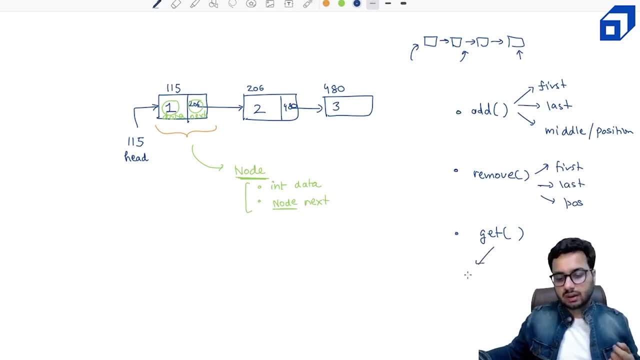 element, i want to get the last element or i want to get the middle element, right. so i will say i want to get first element, last element and element at a given position, right? so what we will be doing, we will be implementing these operations right now in order to implement these operations right. what is important? let us start by understanding. 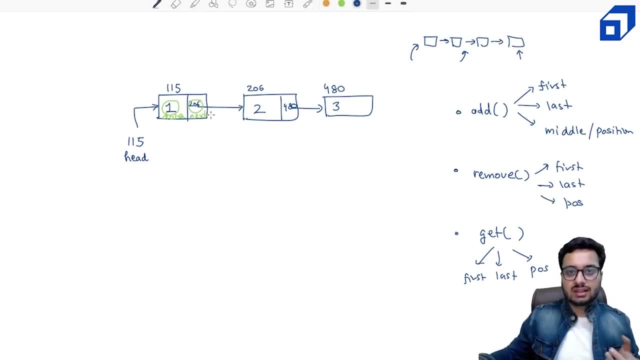 how my ad operation will work, right? so whenever you want to add something, so one thing you need to know is what is the starting point of the link list, right? so suppose you want to add something in the beginning, you must know the starting point. or you want to add something at the end? right, one way. 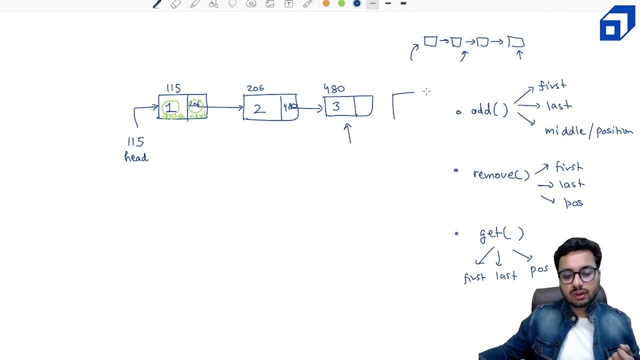 is if you're adding something at the end, right? that means if you're creating a node here, you need to know the starting point of the link list and update the next variable of this node, right? you would say, okay, um, in the ending of this node, i will attach this node one ways. you always iterate. 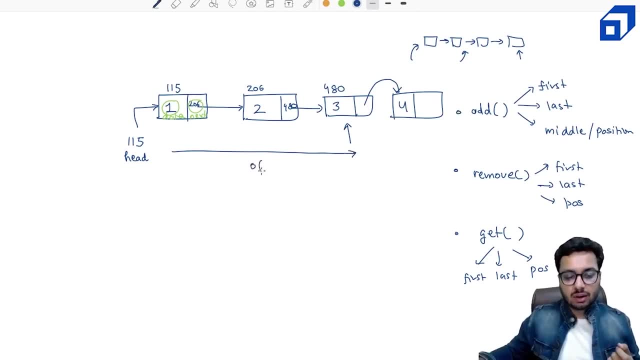 till this point, starting from the head, and this will actually take order of n time. if you iterate from here to here, it will take order of n time. so i don't want to do that. what i will do, i will say okay, every link list will at least know what is my head and what is my tail. i will keep another reference. 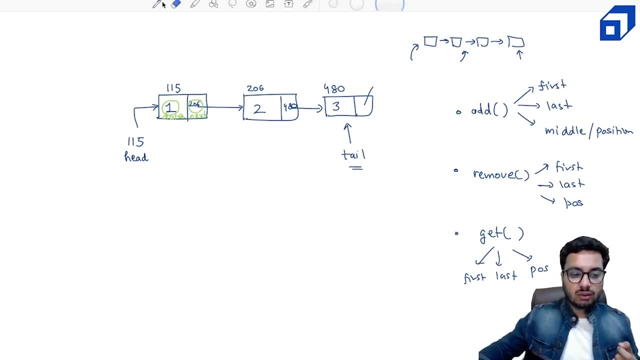 point to the last node of the link list. whenever you will add a new node at the ending of the link list, i'll say okay, i'll modify the tail node, i will attach the node and i will update my tail variable to go here, right? so let us see how these operations are implemented. so what i'm trying to tell you is: 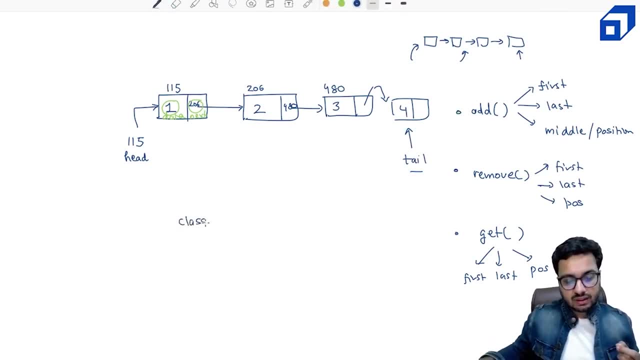 that if you're implementing a class called link list, this link list will have data members. okay, something that the link list should know. okay, some operations that the link list will does, right. so here are the operations. they will be part of the methods, right, and we will have some data members or attributes. what are the data members? what are? 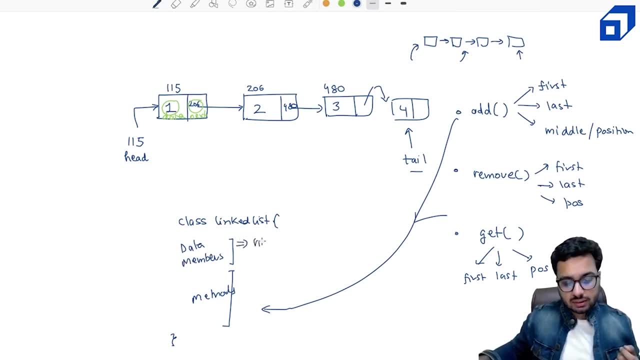 the things that the link list must know. one is head: what is my starting address? one is the tail: what is my ending address? so again, keeping this is optional. but i want to optimize certain operations. for example, add at last should not be in order n operation, it should be an order one operation. so i need to keep the tail variable as well. right, 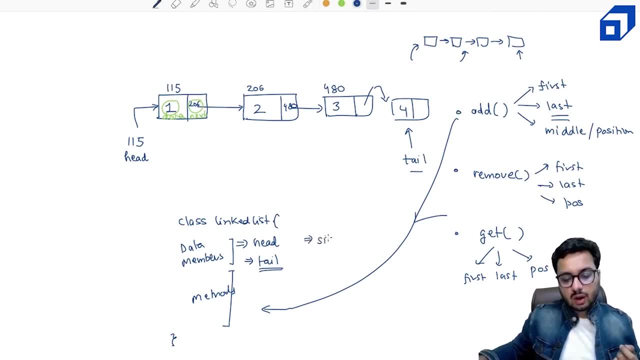 and maybe some optional information like size: how many nodes i have in the link list? okay, so maybe i want to implement a method like get size: how many items are already inserted in this link list? this is a useful operation. we want to check. okay, if the size is zero, that means link list is empty. 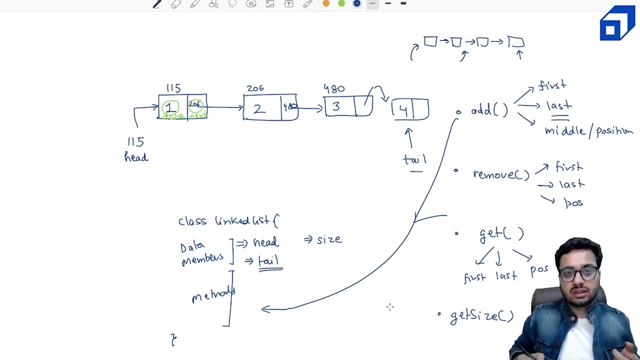 right. otherwise you can check. if the head is null, that also means link. this is empty, right, so we will also implement this operation like uh, get size. and maybe we'll implement operation like display. i want to show the entire link list, okay, or you can implement a method like two string: iterate on this link list and convert. 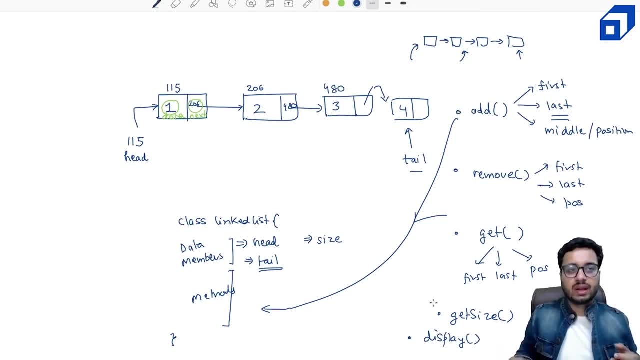 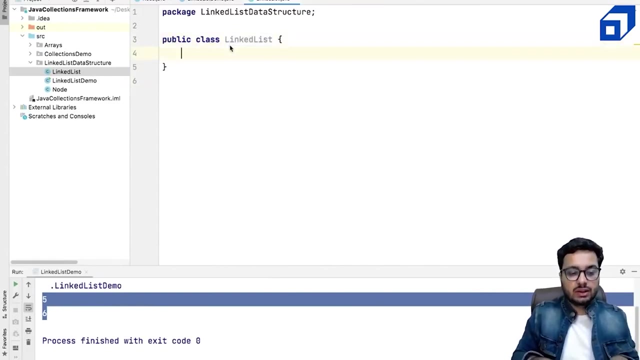 it into a string, so that is just like a display method. i want to show the entire link list to the user, right? so let us start by implementing these operations one by one. so this is my link list class. so, first of all, what i will do: i will add some data members and i will add a constructor to 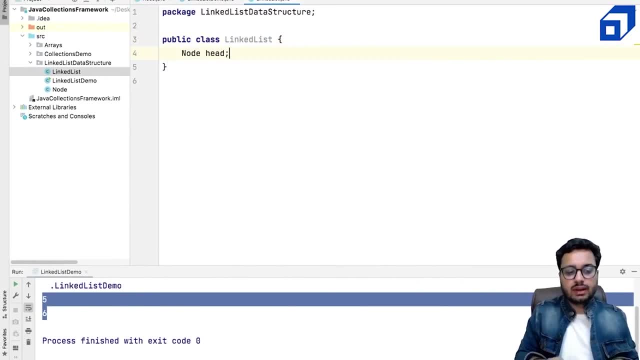 that. okay. i want to create a head, so node head. again. head is a object reference, hence it has a data type called as node. right then i will have node tail, and one thing i can do is i can make them private. so private node head and private node tail. i don't want people outside the 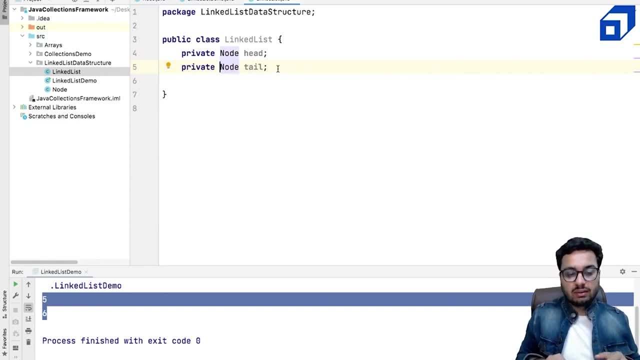 linkless class to know where is the head node, where is the tail node. so i will not expose this data outside the linkless class. right, and i can also say private in size. i'm not making it public because i don't want this size to be changed by someone outside. the size should change. 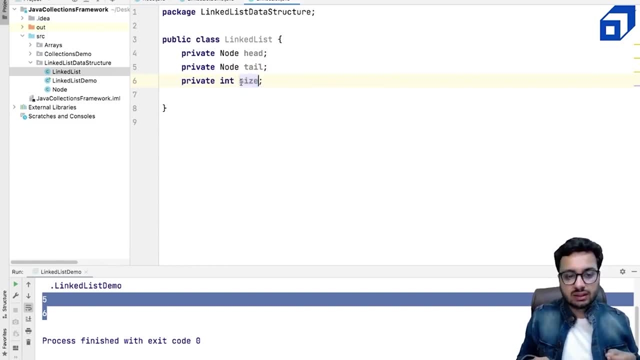 automatically when something is inserted or something is removed from the link list. so it should be a private variable only changed by the linkless class right. next thing i want to do is i need to initialize a constructor. okay, when, whenever user says, okay, give me a new link list, what should? 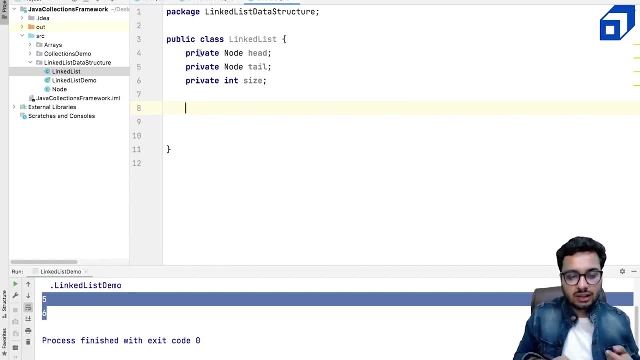 i do that link list will have zero nodes inside it, so i need to initialize these three data members. so i need to initialize these three data members, so i need to initialize these three data members. and what i want to do is i want to say head and tail, they will be null and the size would be zero. 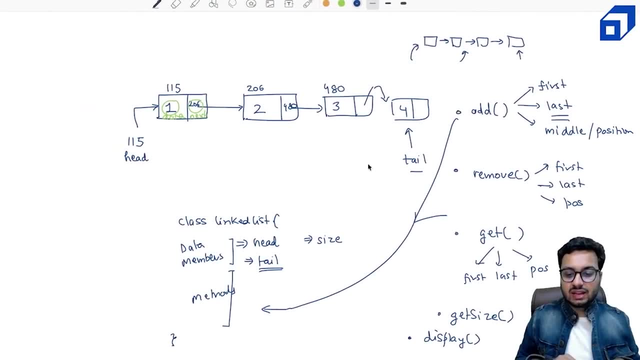 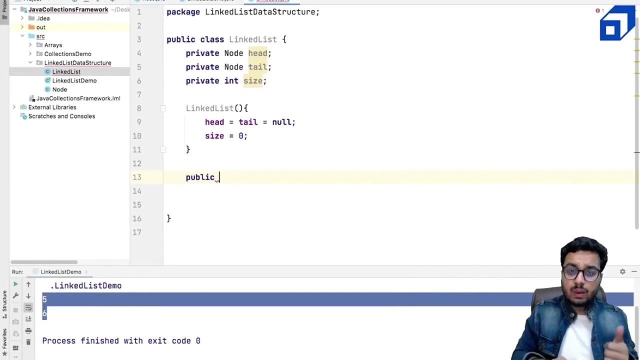 okay, so this is my constructor. now, what is the first thing i will do? i will, okay, i want to do an insertion, so i will add. i'll write three methods: one to add something at the beginning, something at the end and something at a given position in the linked list. that's okay. public method. 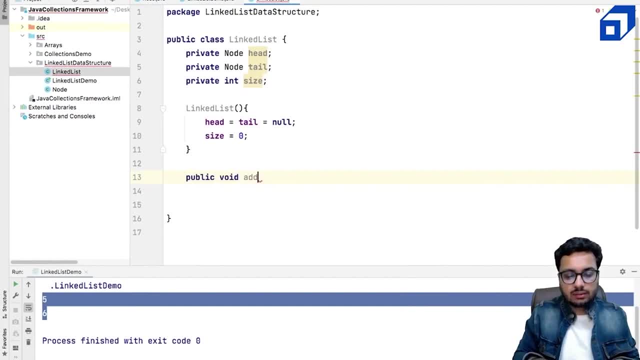 and the method is of the type void add, and let me call it as add first and public void at last and public void add at a particular position, so add art. in all the three uh methods i should know what is the data that i need to add and in the third method i should also know at what index i need to add. 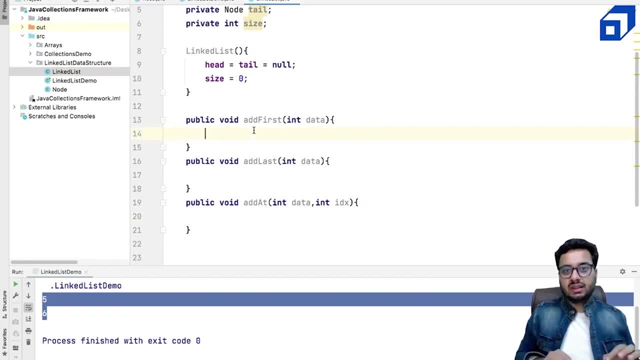 now take a pause and think how you will implement these methods. okay, if you are given a link list and you want to add something at the beginning of the link list, how you would add in? okay, so what will be the code behind this method? take a pause and think about it. okay, so let us discuss. 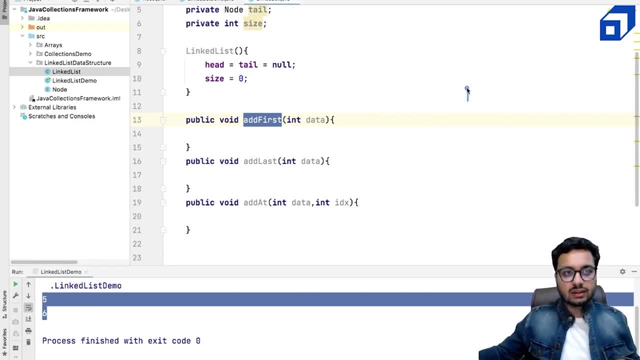 the first method: add first. now suppose you have a link list, right? let's say this is a, this is b, this is c, this is already there and head is referring to this node. i want to say i want to add another node, d, which is at the beginning of the link list, right? so how i will do it? the first: 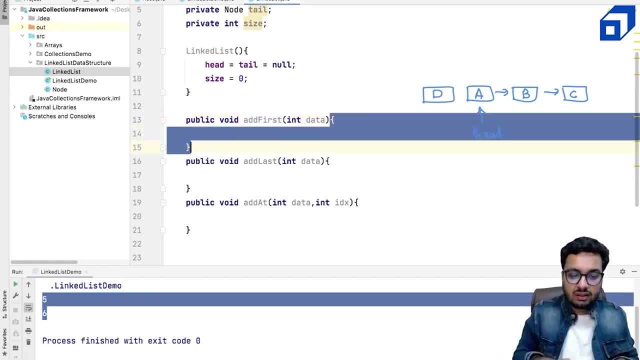 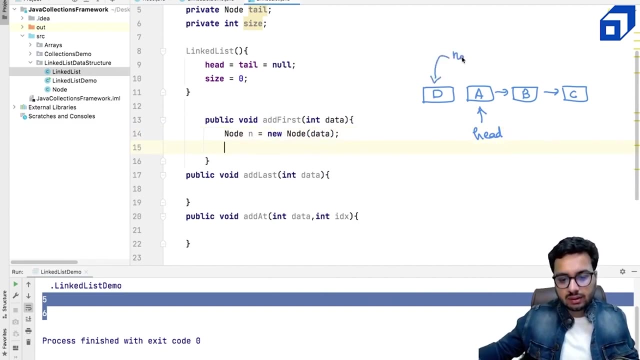 thing is, i need to create this node. so how do i create a node object? very easy, i simply say: let me create a node called as n. this is equal to new node and the data of this node is same as this data that i have given. so this creates a new node and n is referring to this node, right? 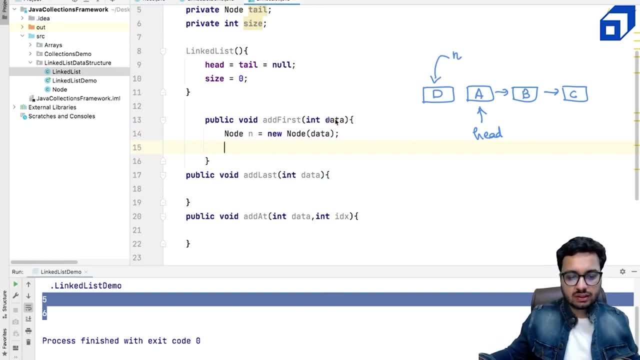 n is an object reference, a local reference created inside this function which is referring to this node. what should i do? how do i connect this? i would say, okay, n dot next should refer to the head. so if head is already there, n dot next should connect to head. so it it makes this connection. 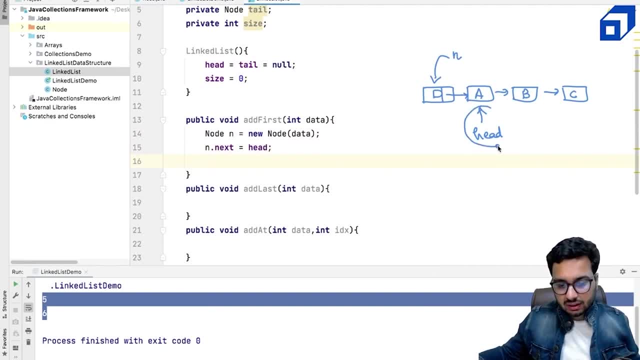 right. one thing i need to do is i need to say: okay, this head, it should move here. right, this head should not refer to a. instead, this head should refer to now, d, so i can say head is equal to n. this will work really well. and one more thing i will do is 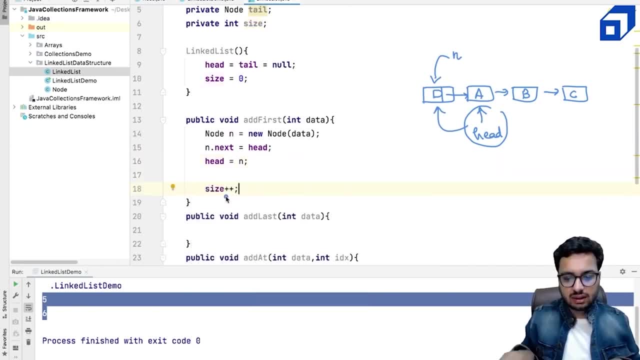 size plus plus, every insertion will increment the size of the link list, right? so this will work really well if the link list is already there, right? but suppose you are creating the link list for the first time and you call the add first method. so, head and tail, both of both were null. 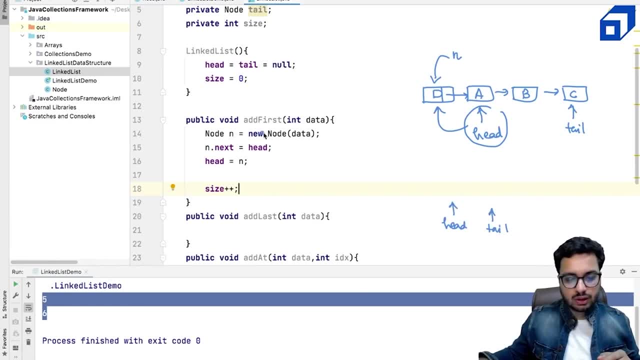 right. and you said: okay, i want to create a new node. so you created a new node called d and n. dot next is equal to head, so head was null. so d is next is also null, which is fine, right. and then you say head is equal to n. this head refers to this node, which is also fine, right. but the thing 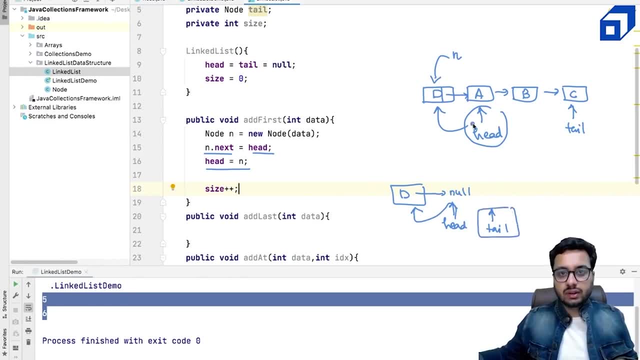 is the tail is not getting updated right whenever the first node is inserted. right? let's say, the first node is a, both head and tail should refer to this node, right? what i can do, i need a. i need to add a separate condition that if, what if the size was zero before adding this node? in that case, 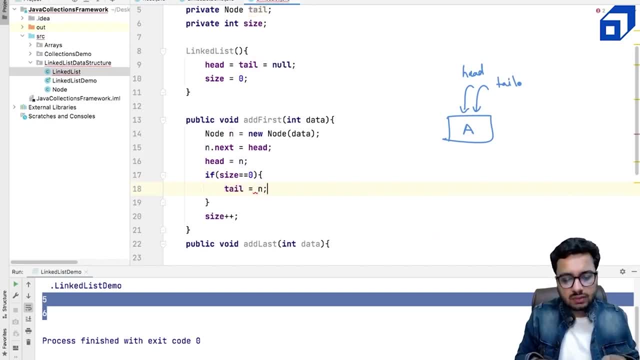 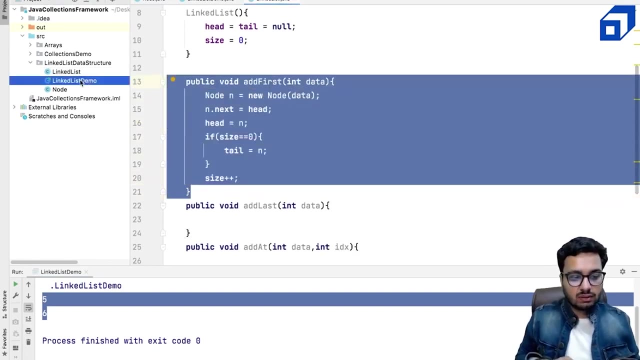 also get updated. so tail should also point to head or tail should also refer to n. right now, this is a special case when you have zero nodes. in that case, you also need to update the tape. right? this is my add first method. let us test the functionality of add first method. so what i will do? i will go in. 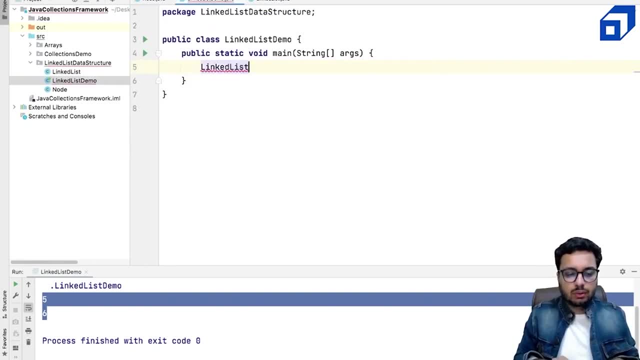 linked list demo. it's okay, i want to create a linked list, l. this is equal to new linked list. and now in this i can say, okay, l dot add first. and uh, i will give some data, let's say 10 and say l dot add first. 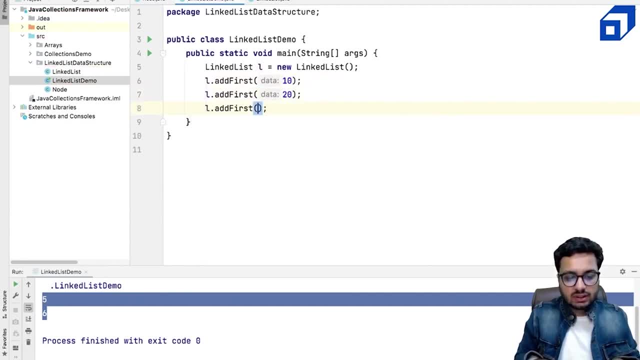 i will add 20 and then l l dot add. first i will add 30, right, so i want to see this linked list. so i will call the display method, which i have not implemented. so i will. we will implement the display method as well. right, let us go back into the linked list class and let us add one more. 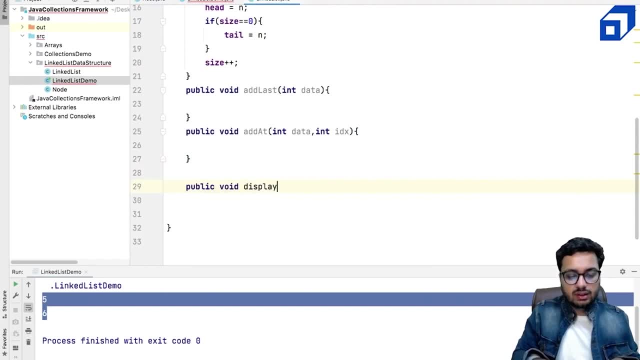 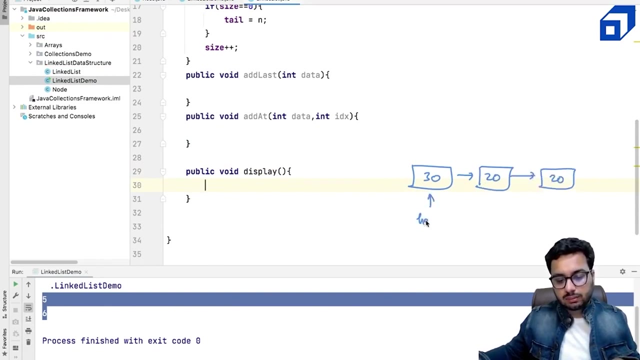 method: public void display, right. so how do i display the linked list? now it's going to be pretty easy. suppose the linked list is 30, followed by 20, followed by 10, right, and head is referring to this node. okay, tail is referring to this node. this is 10, right? 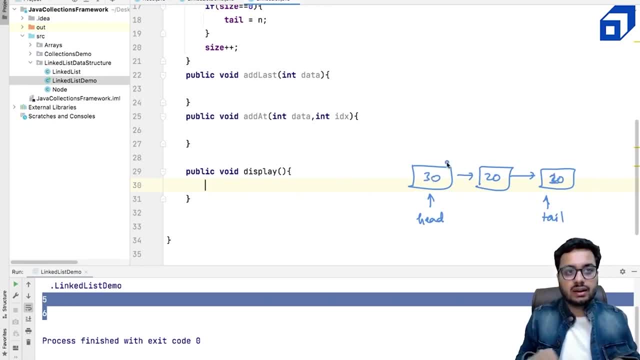 so tail is referring to this. so what i need to do? i need to start iterating from head till the end. so i will take a temp variable, i will print it and i will take temp here. i'll print it. i will take temp here, i'll print it. i will take temp here. right, what is happening? so once my temp reaches null, 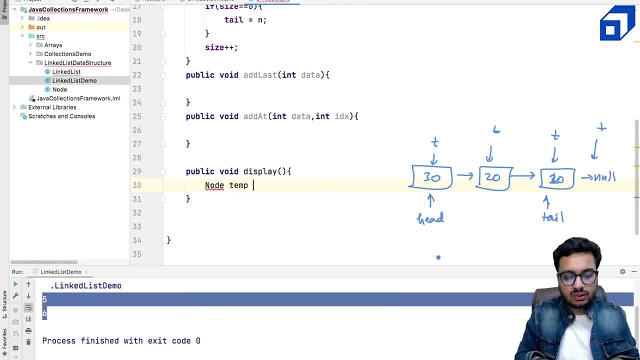 i will stop what i can do. i can say: node, temp. this is equal to null, so temp is again a reference. it's not a node, right? so sorry it's. it's equal to head. it starts from head. and while this step is not equal to null, what do i do? i print the node so i say: s out temp dot data and take this temp to the. 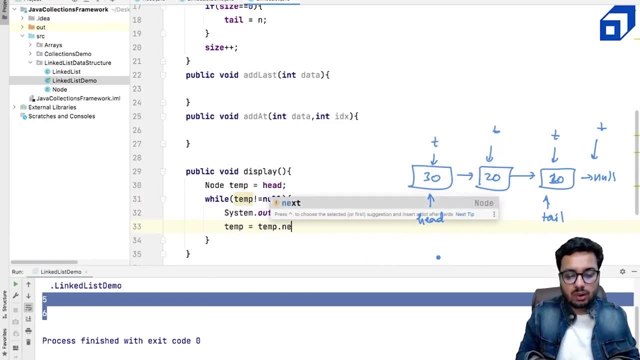 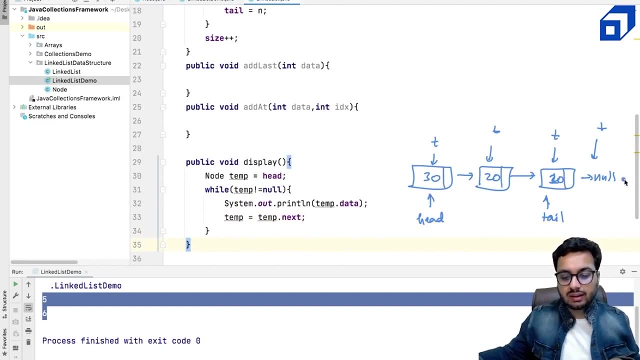 next node: temp equals to m. temp dot m goes to the next node. this while loop will help me to iterate on the entire linked list. right, so temp starts from head. temp is referring to this node. i print out 30. temp equal to temp dot next. so temp dot next means this value. so this value means this. 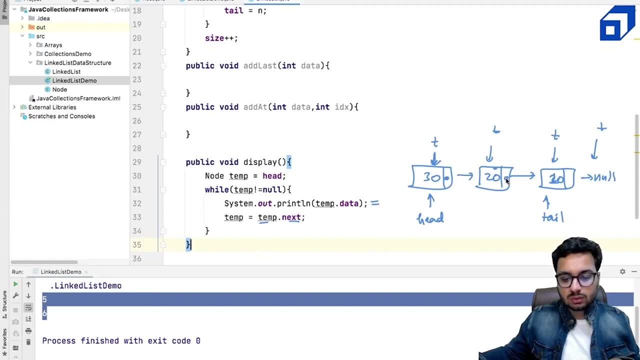 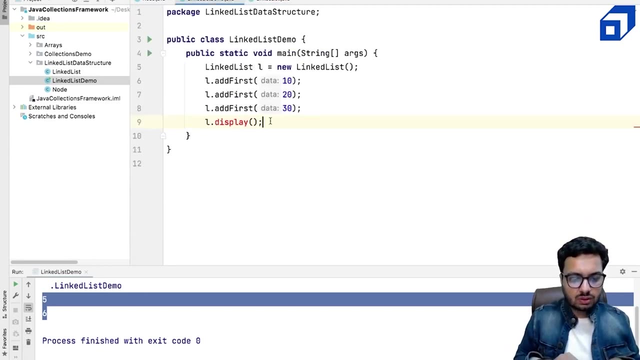 node. so temp goes here again. temp dot x means this value, which is this node. m goes here again. this is not null, this node is not done. so i say temp dot next, which is this value, which is now the temp actually becomes null and my loop stops. right now the display method is there and we can. 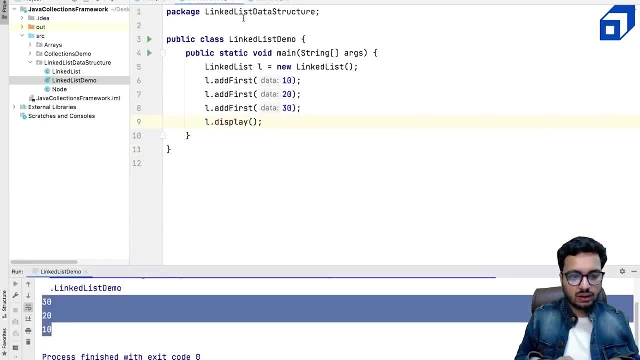 run this code. okay, so i see 30, 20 and 10, which is okay. that means my linked list is getting created. but to show you in a link here fashion what i can do, i can put a arrow here and i can put a new line here, right. 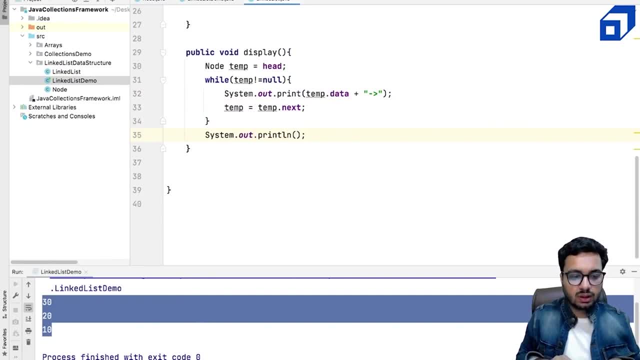 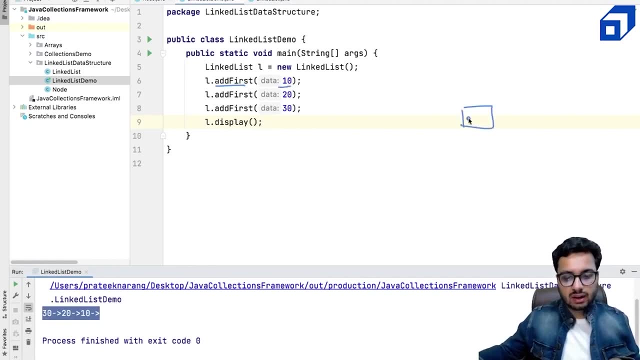 this will make the representation look little better. right, i'm getting 30, 20, 10.. if you look carefully, i added 10 in the beginning, so 10 got added. that means my head and tail- both were here right. then i added 20, in which 20 got added here and my head moved here right. then 30 got added. 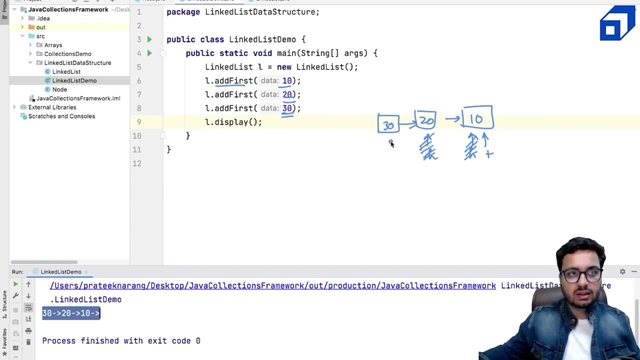 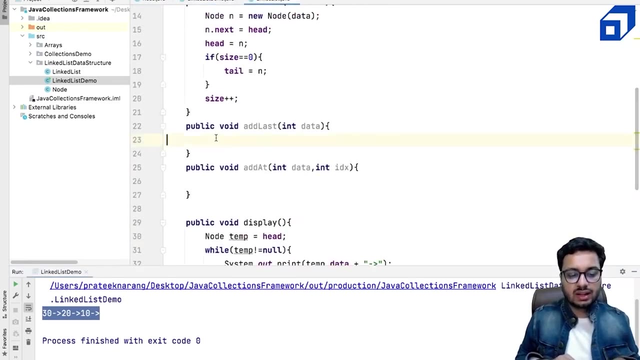 a new node was created. it got connected here and then my head moved here right. this is how the linked list is going to look like: 30, 20 and 10.. i hope you are able to understand the add first method right now, on the similar lines, what we will do. we will implement the method called as. 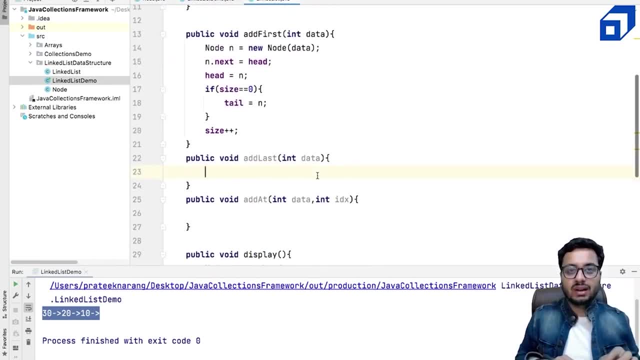 add last. now take a pause and think how you will implement the add last method. all right, let us see right now. suppose you already have a linked list- a, b, c, right, and i want to. i want to add a new node d, which is at the end of the list. so this is my head and this is my tail, right? so 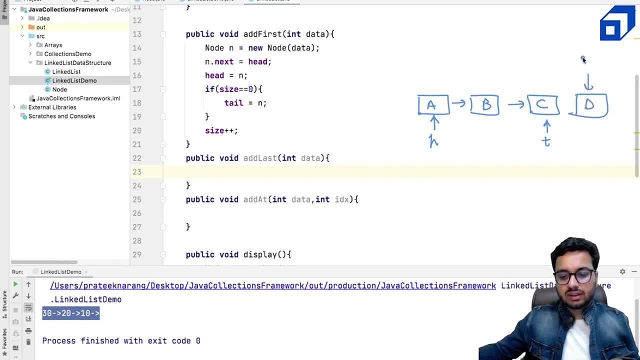 how do i add a new node here? first of all, i need to create this new node. so how do i do it? i can. okay, fine, node n. this is equal to new node and i give the data to this node. that i'm getting right. how do i connect this tail node with the new node? look, that connection is pretty easy. 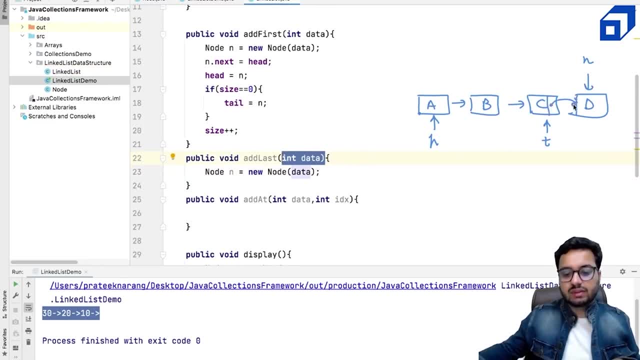 what i need to do. i need to update this value and give it the reference of this node, which is stored in n, right. so i need to say that fine tail dot. next, this is equal to the new node that we have created, right, so this makes the connection. 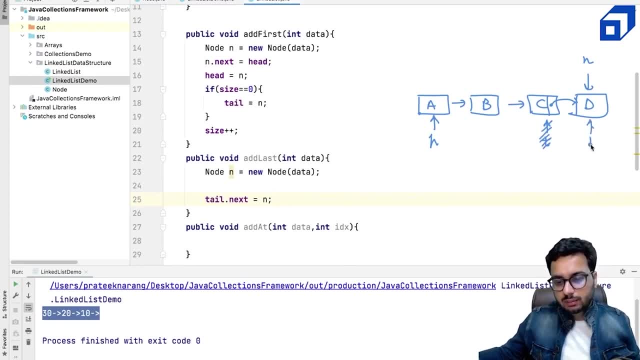 and i also need to say: okay, this tail should be here, because this, this node, is now the new tail, right, so i can say tail equal to tail dot next, or you can say tail equal to n, both are fine. right now, this tail has also moved, and one more thing we will do is we will just size plus plus now this: 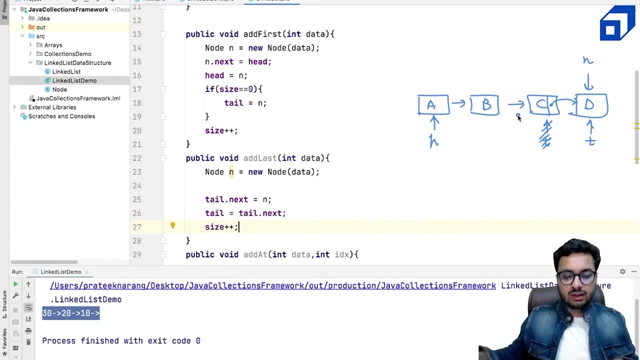 will work fine when the link list is already there, right. but think of a case when your link list is not created. that means both head and tail they were null and you inserted the first node by calling the add last function. you say, okay, i don't have a link list. that means if the size is zero. 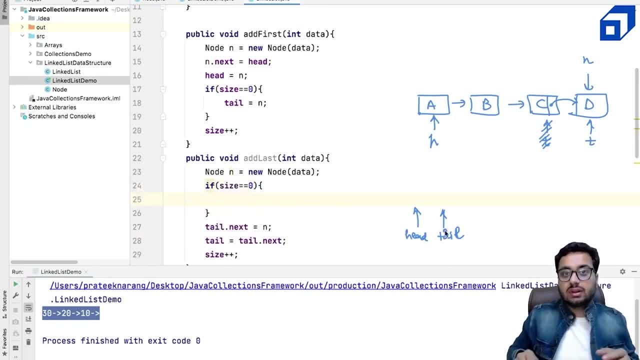 and you are adding the first node in the link list, then how should the update should happen, right. so you still created this new node n, right? uh, with with the data d, n is referring to this node. so in this case, both head and tail should get updated. they should point to this node, right? 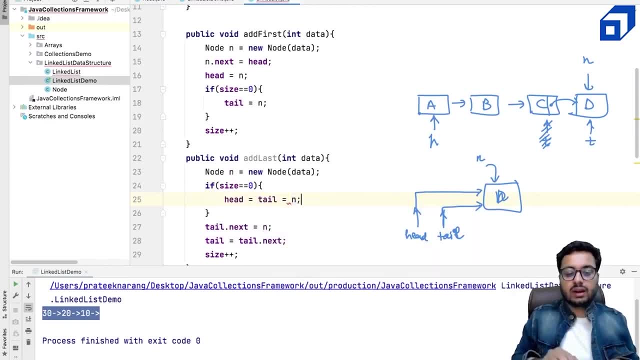 what i can do. i can say: okay, head and tail. they will refer to n. right, they will also store the address that is stored in it. right now, you might ask: okay, uh, what happens to this end? so n is a local variable. it will get destroyed after this function call is over. but head and tail. 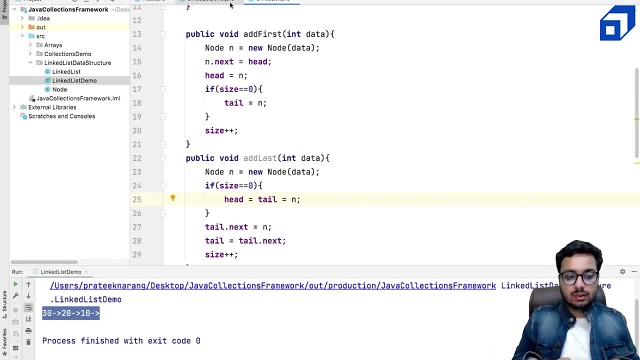 are the data members of the class. they will exist till you have the link list object in your memory, right? so they are not going to get destroyed, right? so n is a local variable. it will be over, right, and anything that is allocated using new will not get destroyed. why? because if someone is referring 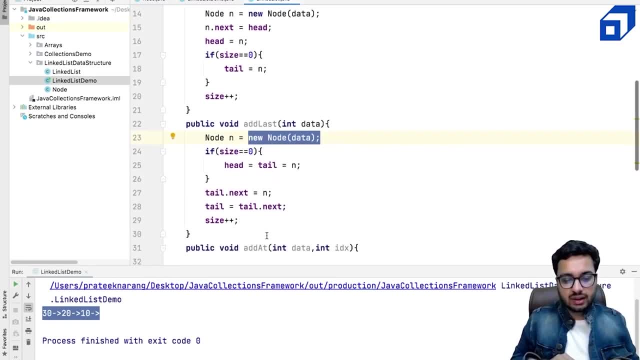 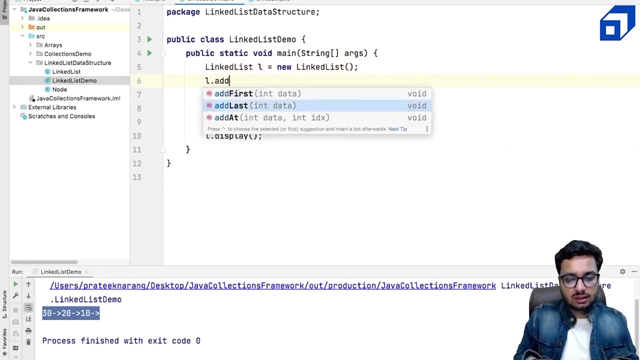 to this memory. that memory will not be garbage collected, right. so head and tail, they are referring to this. node n is a local variable. it will get destroyed, right. so this way, add last will work. so test our functionality. right is okay. L dot add last. maybe this is 40 this time. 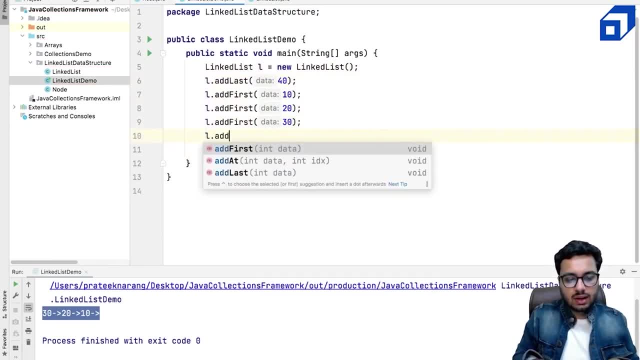 and again is okay, L dot. add last. this is 50 right now. if you look carefully, I'm adding the first node by calling add last function. first 40 was added. add first 10, so 10 was added, then 20 was added, then 30 was added. now again I'm. 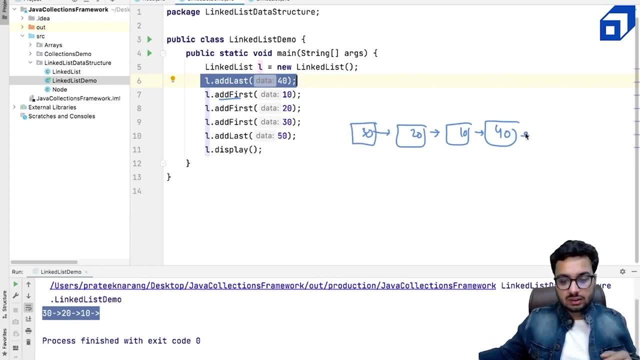 calling the add first method on a linked list which is already built. so 50 should get added right. so if I say L dot display right, which it will give me this linked list. let us see the output. we are getting this linked list: 30, 20, 10, 40, 50. 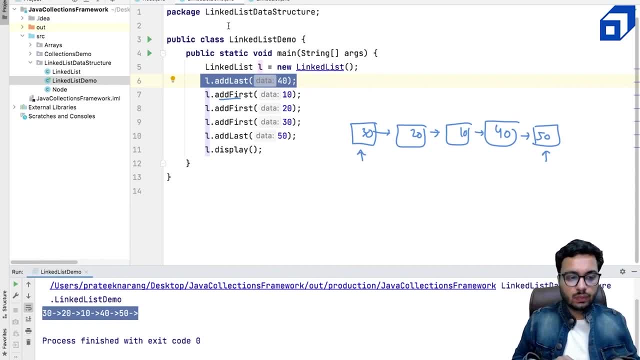 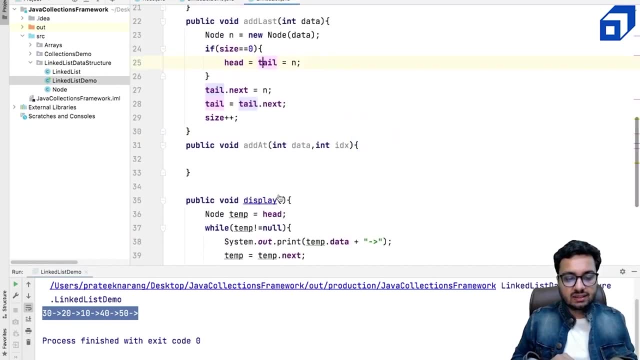 that means this is working really fine. okay, let us go back here and let us implement one more method. that is okay. give me the size right. okay, let us implement one more method. that is okay. give me the size right. okay, let us implement one more method. that is okay. give me the size right. how many nodes we have that's going to be. 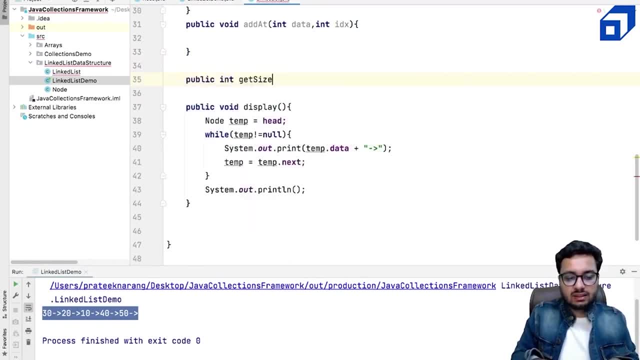 how many nodes we have. that's going to be how many nodes we have. that's going to be easy public int get size and what we are easy public int get size and what we are easy public int get size and what we are going to do. we are going to return the. 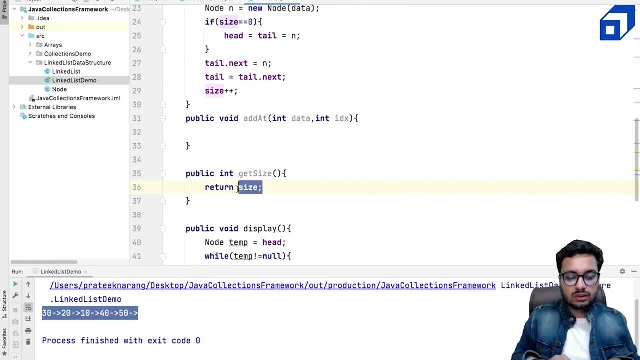 going to do. we are going to return the going to do. we are going to return the size of the linked list right now we are size of the linked list right now. we are size of the linked list right now. we are doing it this way because if you make 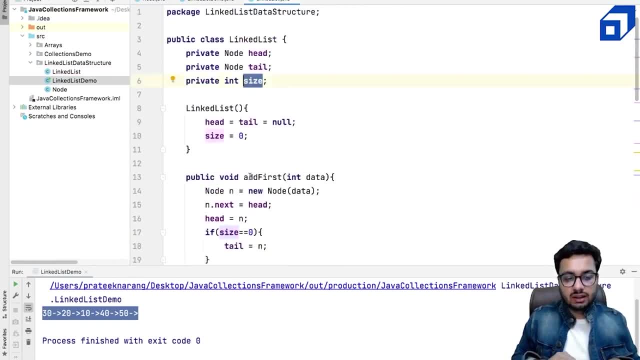 doing it this way, because if you make doing it this way, because if you make this size public, anyone can change it. this size public, anyone can change it. this size public, anyone can change it right. I'm only giving the getter to right. I'm only giving the getter to. 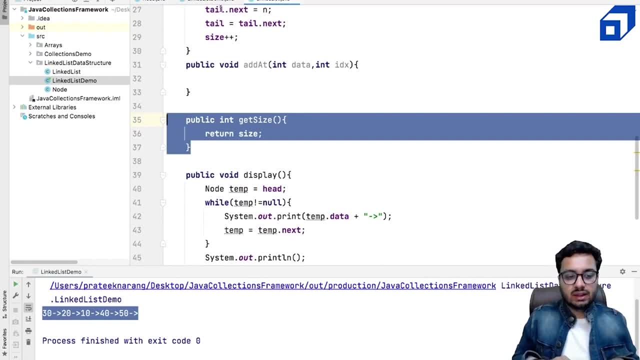 right, I'm only giving the getter to excess the size. I'm not giving any method excess the size. I'm not giving any method excess the size. I'm not giving any method to set the size of the linked list. okay, to set the size of the linked list okay. 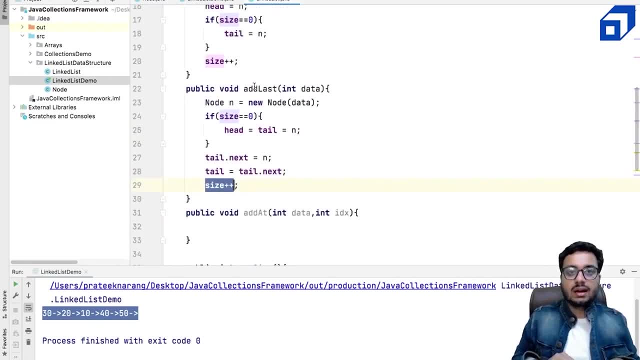 to set the size of the linked list. okay, that size should be updated only through that size. should be updated only through that size, should be updated only through the add and the remove methods. so this, the add and the remove methods, so this the add and the remove methods. so this is also fine. so I can say: L dot get size. 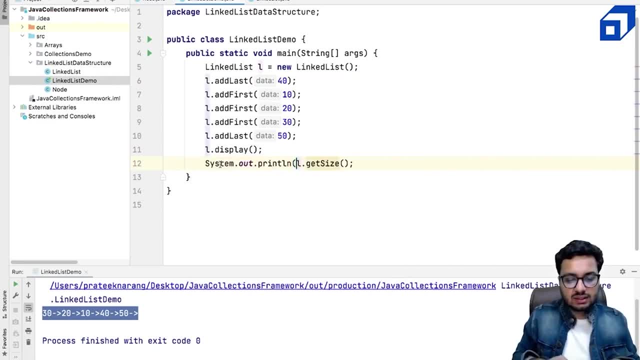 is also fine, so I can say L dot get size is also fine, so I can say L dot get size. and I want to display how many nodes I and I want to display how many nodes I and I want to display how many nodes I have in this linked list. 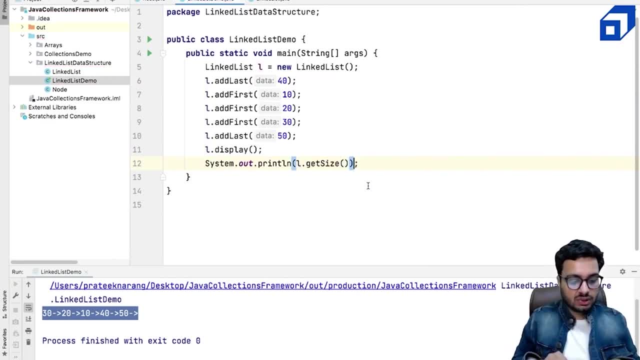 have in this linked list. have in this linked list. this is again a order one operation. this is again a order one operation. this is again a order one operation. right, right, right. I can see, okay, there are five nodes now. I can see, okay, there are five nodes now. 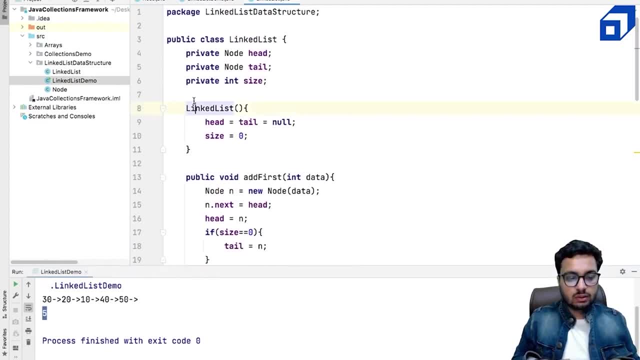 I can see. okay, there are five nodes now let us talk a little bit about the. let us talk a little bit about the. let us talk a little bit about the complexity. so your constructor is doing complexity. so your constructor is doing complexity. so your constructor is doing order. one work at first, it is also doing 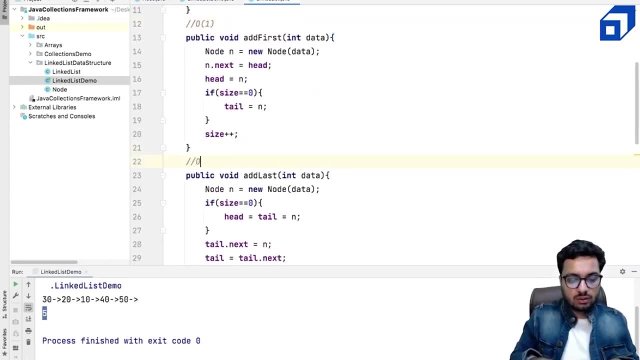 order one work at first. it is also doing order one work at first. it is also doing order one work. order one work. order one work. no loops involved. here also we are doing no loops involved. here also, we are doing no loops involved. here also we are doing order one work. 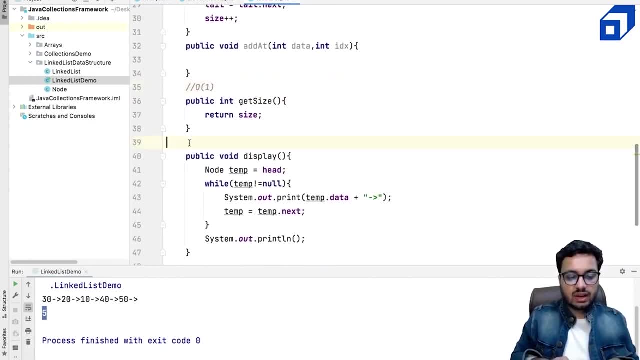 order one work. order one work, get size. we are doing order one work, get size. we are doing order one work, get size. we are doing order one work display. we are iterating over all the display. we are iterating over all the display. we are iterating over all the nodes. we are doing order of n work right. 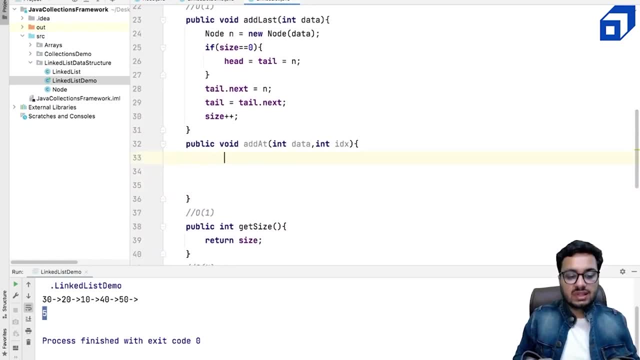 nodes: we are doing order of n work right. nodes. we are doing order of n work right now. the next method is add art right. so now, the next method is add art right. so now, the next method is add art right. so take a pause and think how you will. 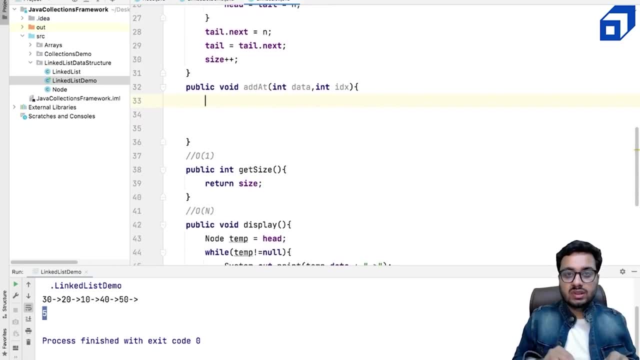 take a pause and think how you will take a pause and think how you will implement, implement, implement, add art method, add art method, add art method. and if you want to insert something in, and if you want to insert something in, and if you want to insert something in the middle of a linked list at a 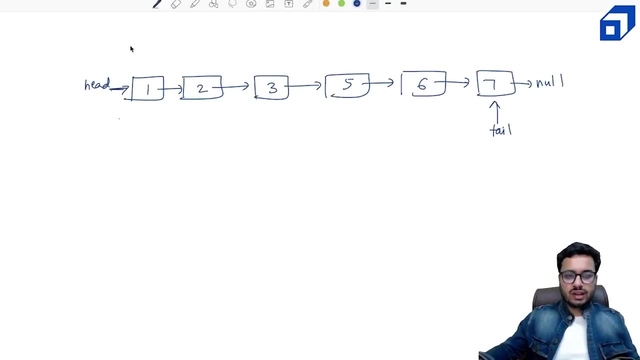 the middle of a linked list at a the middle of a linked list at a particular index. okay, so let us see it. particular index. okay, so let us see it. particular index. okay, so let us see it. do this insertion right now, suppose my. do this insertion right now, suppose my. 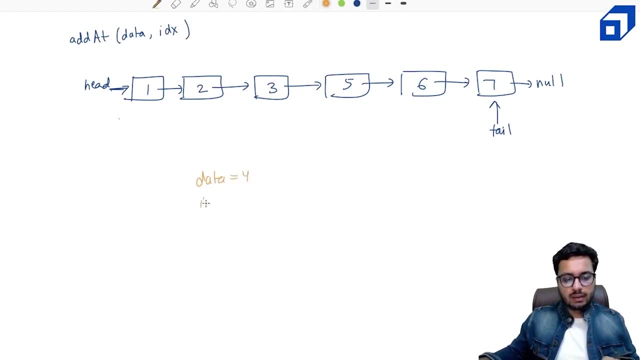 do this insertion right now. suppose my data is four, data is four, data is four and my index is three. that means okay, and my index is three. that means okay, and my index is three. that means okay. zeroth index. first index. second index. zeroth index. first index. second index. 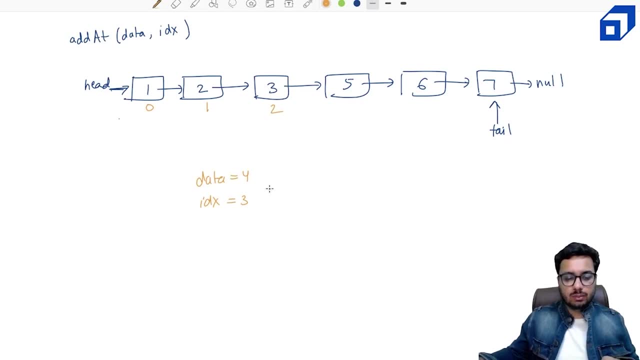 zeroth index, first index, second index: here i want to add, here i want to add: here i want to add, like at the third index, the new node, like at the third index, the new node, like at the third index, the new node should come right, should come right. 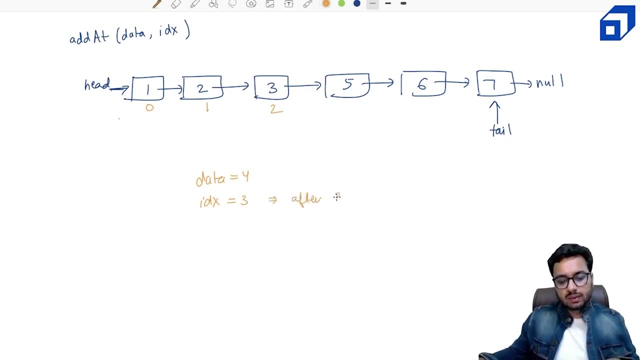 should come right. or you can say okay after three nodes, or you can say okay after three nodes, or you can say okay after three nodes, i want to insert, i want to insert, i want to insert the fourth node, so this is my, the fourth node, so this is my. 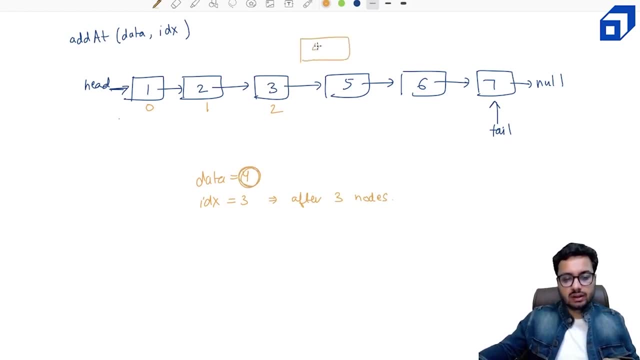 the fourth node. so this is my fourth node that i want to insert. fourth node that i want to insert. fourth node that i want to insert somewhere here, right, so how i will do it somewhere here, right? so how i will do it somewhere here, right, so how i will do it, right? so one way is: 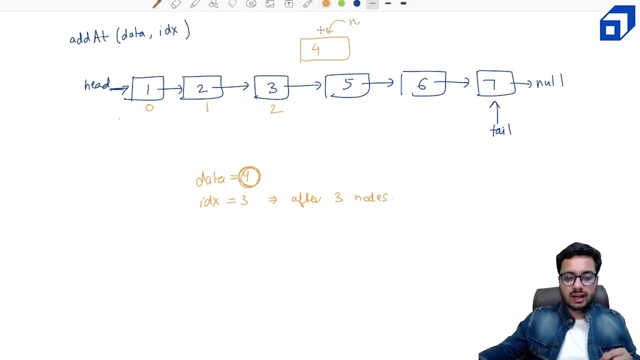 right. so one way is right. so one way is okay. i will create a new node n. okay, i will create a new node n. okay, i will create a new node n. n is referring to this node 4, right, but n is referring to this node 4, right, but? 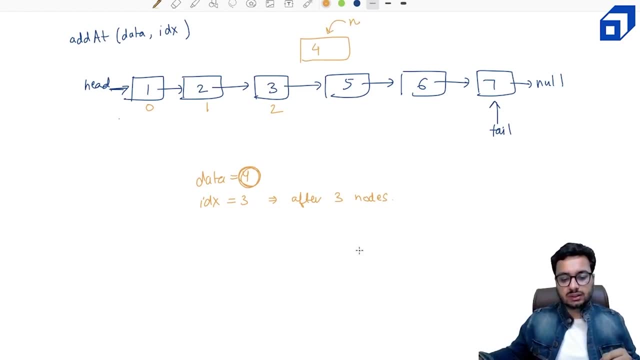 n is referring to this node 4, right, but how do i connect? how do i connect? how do i connect 3 with 4 and 4 with 5? right? so this is 3 with 4 and 4 with 5, right? so this is. 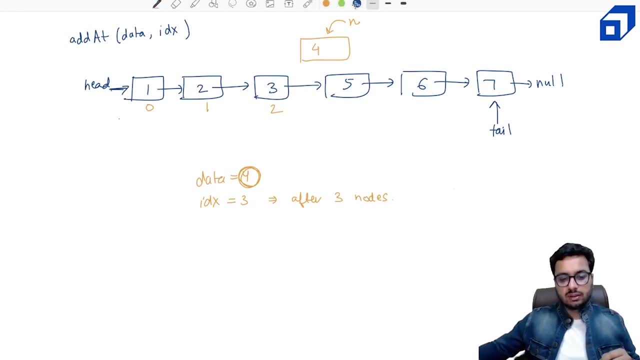 3 with 4 and 4 with 5, right, so this is going to be easy, going to be easy, going to be easy. how you can say, okay, let me create this. how you can say, okay, let me create this. how you can say, okay, let me create this. new node n. so node n. 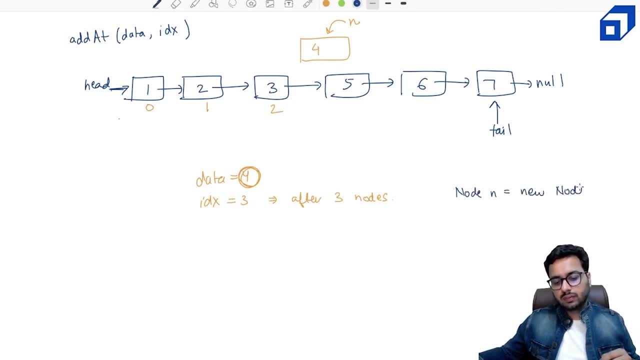 new node n, so node n. new node n, so node n. this is equal to new node. this is equal to new node, this is equal to new node. with my data 4 right now, with my data 4 right now, with my data 4 right now, one way is okay. i can say: 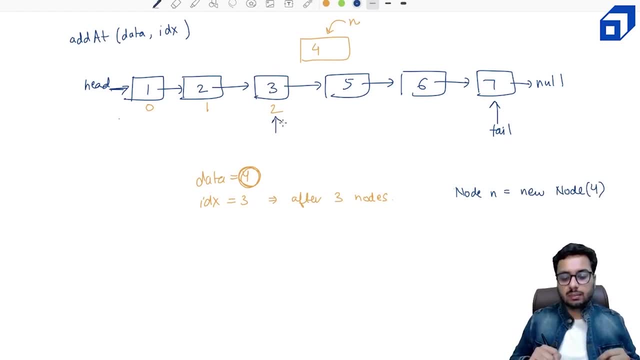 one way is okay. i can say: one way is okay. i can say: i need to reach this node right. how do i need to reach this node right? how do i need to reach this node right? how do i reach this node? i reach this node right. that means i. if i start from this: 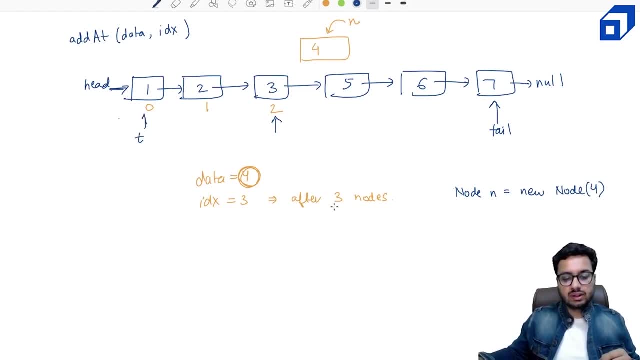 i reach this node right. that means i, if i start from this, i reach this node right. that means i if i start from this node, node, node and i want to reach the third node right and i want to reach the third node right and i want to reach the third node right after three nodes. i have to insert that. 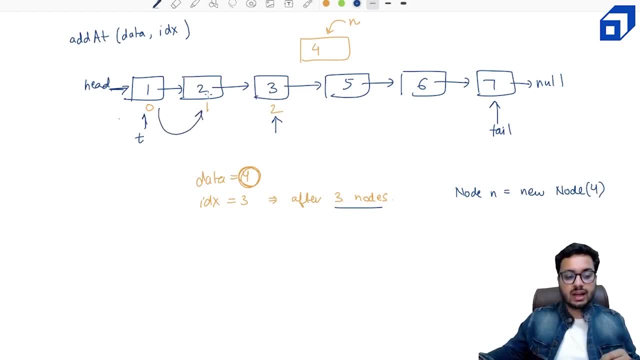 after three nodes, i have to insert that after three nodes i have to insert that means i have to reach the third node. means i have to reach the third node. means i have to reach the third node. if i take one jump here, i reach two if i 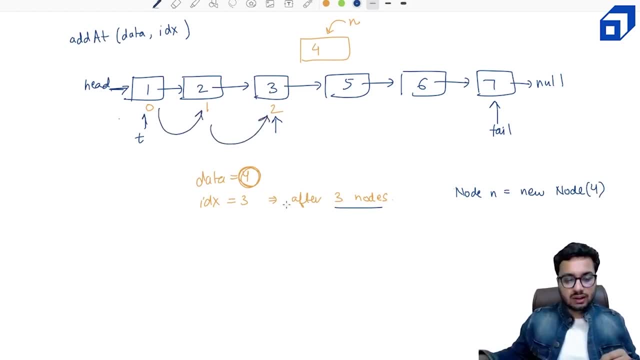 if i take one jump here, i reach two. if i, if i take one jump here, i reach two. if i take one more jump here, take one more jump here, take one more jump here, i will reach this node right. that means: i will reach this node right. that means: 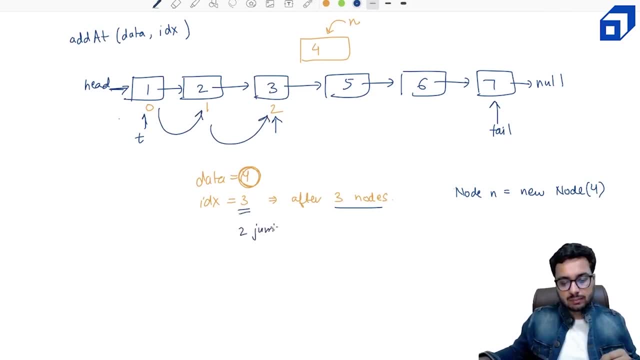 i will reach this node right. that means, in order to reach three, i need to take. in order to reach three, i need to take. in order to reach three, i need to take two jumps, right, okay. so if my index is two jumps, right. okay. so if my index is, 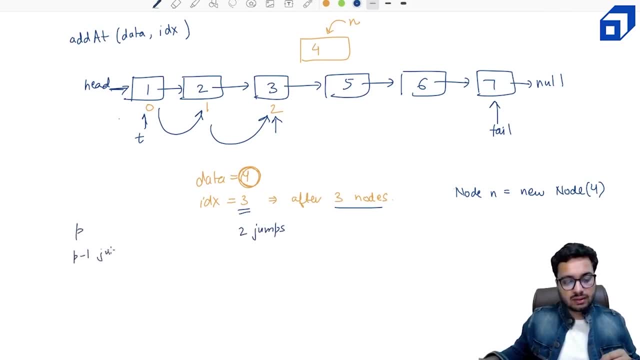 two jumps right. okay, so if my index is some p, some p, some p, right, i need to take p minus one jumps right. i need to take p minus one jumps right. i need to take p minus one jumps right for a particular position: p right for a particular position: p. 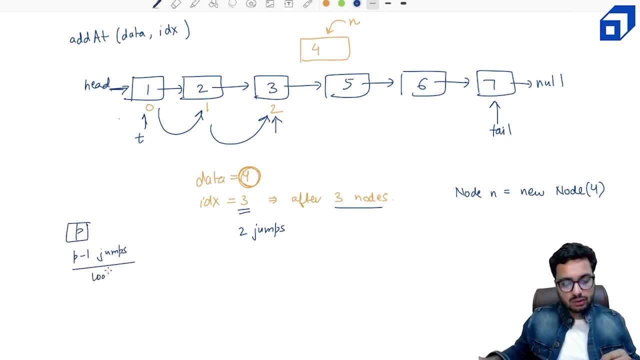 right for a particular position: p- i need to take p minus one. jumps this: we i need to take p minus one. jumps this: we i need to take p minus one. jumps this we will will. will do it using a loop right. let's say i've do it using a loop right. let's say i've. 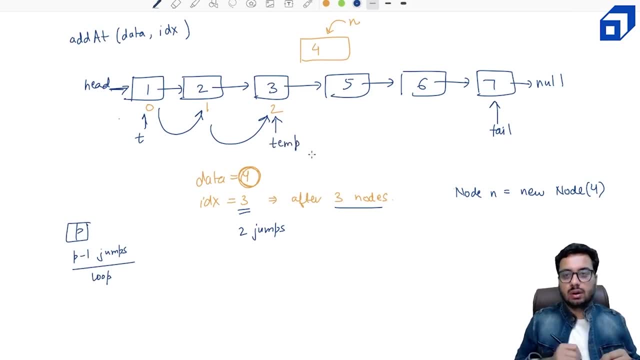 do it using a loop, right? let's say, i've reached this node and reached this node and reached this node and i'm holding this address in a variable. i'm holding this address in a variable. i'm holding this address in a variable called temp. right now how i will do it. 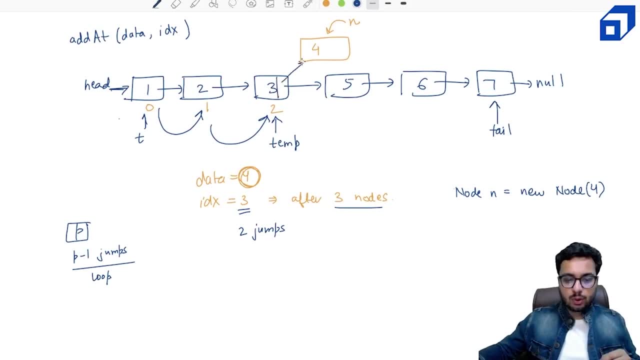 called temp right now how i will do it. called temp right now, how i will do it: right, right, right. so i can say okay, temps next should point. so i can say okay, temps next should point. so i can say okay, temps next should point to four. if i do this, 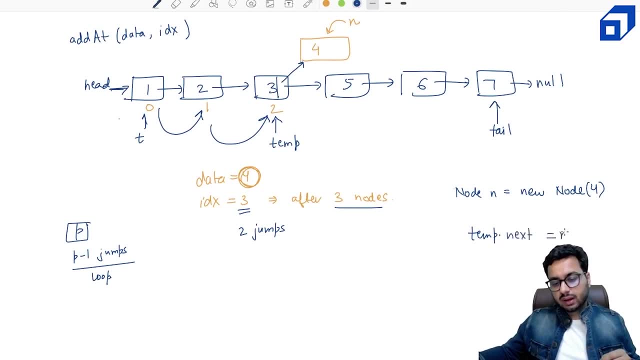 to four. if i do this to four. if i do this, temp dot next, temp dot next, temp dot next. should refer to n what loss i will have. should refer to n what loss i will have. should refer to n what loss i will have. i will lose the address of five. i don't. 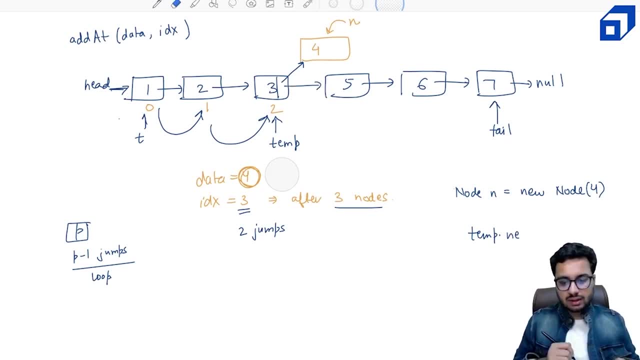 i will lose the address of five. i don't, i will lose the address of five. i don't want to do that right. want to do that right. want to do that right. how should i do it? i will say that. how should i do it? i will say that. 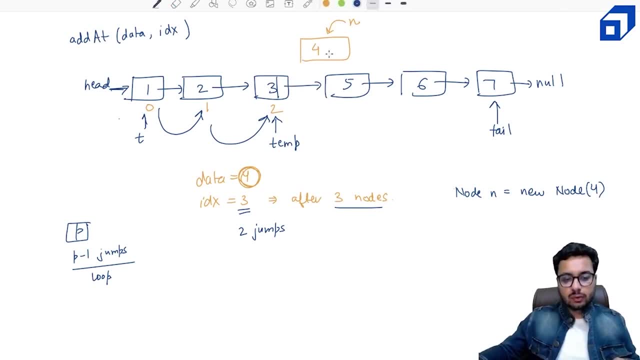 how should i do it? i will say that, before doing this operation, before doing this operation, before doing this operation, let me say that four should store the. let me say that four should store the. let me say that four should store the address of five. address of five. 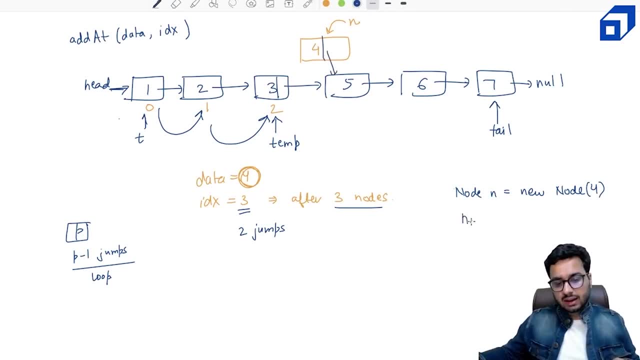 address of five. can i do that? of course, yes. how do i do? can i do that? of course, yes. how do i do? can i do that? of course, yes. how do i do that? i can say that. i can say that. i can say n dot next. that is the next of four. 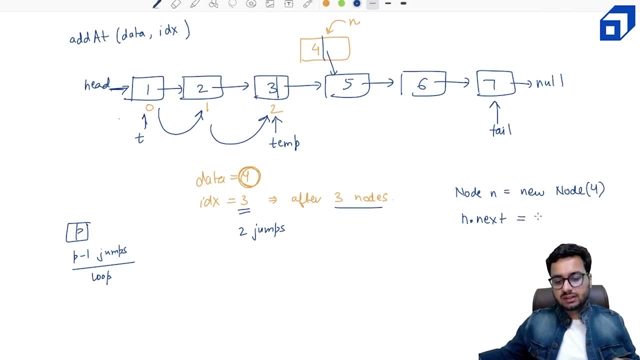 n dot next. that is the next of four. n dot next. that is the next of four. should refer to five. so what is the should refer to five. so what is the should refer to five. so what is the address of five? address of five. address of five. it is nothing, but it is the next of temp. 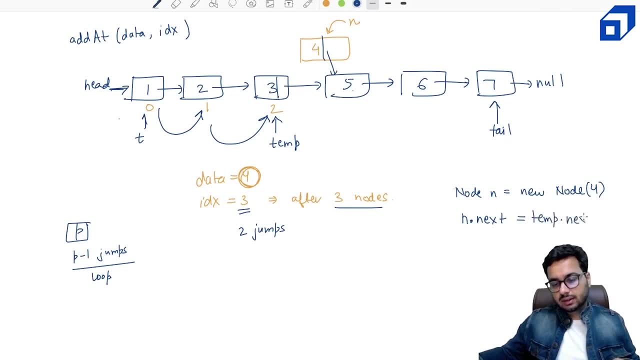 it is nothing, but it is the next of temp. it is nothing, but it is the next of temp. so it is temp dot, so it is temp dot. so it is temp dot next right. once it is done, can i update the next right. once it is done, can i update the. 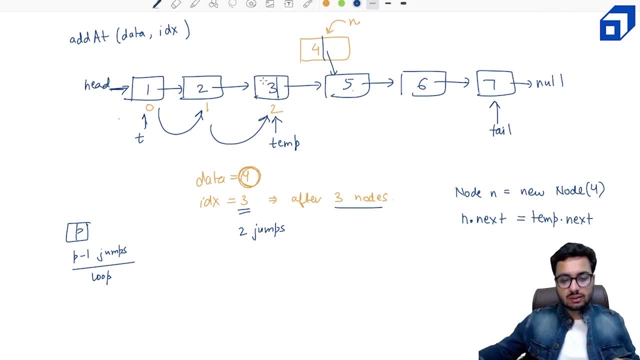 next right once it is done, can i update the address address? address: the next of three, of course. yes, i can say the next of three, of course. yes, i can say the next of three, of course. yes, i can say, okay, three is next. now should point to: 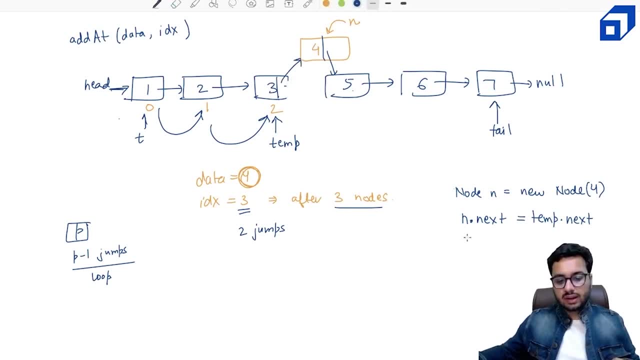 okay, three is next now should point to: okay, three is next now should point to four. and this link will automatically get four and this link will automatically get four and this link will automatically get broken. so i can say three is my temp broken? so i can say three is my temp. 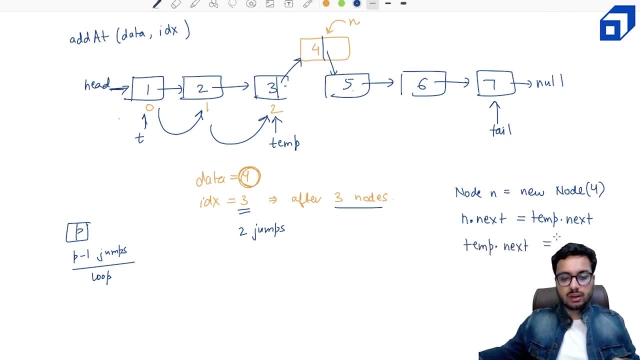 broken. so i can say three is my temp temp dot, next temp dot, next temp dot next should be equal to n, should be equal to n, should be equal to n. in just these three steps, i will be able. in just these three steps, i will be able. 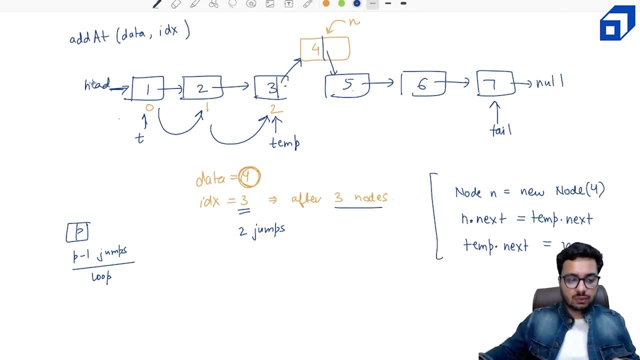 in just these three steps, i will be able to insert a node in the middle right now. to insert a node in the middle right now. to insert a node in the middle right now, we might have a special case where we we might have a special case where we 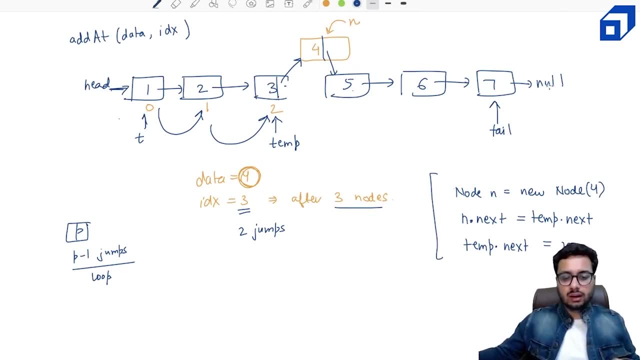 we might have a special case where we might need to insert a node in the, might need to insert a node in the, might need to insert a node in the beginning, beginning, beginning, or at the end, or or at the end, or or at the end, or we are getting an index which is out of. 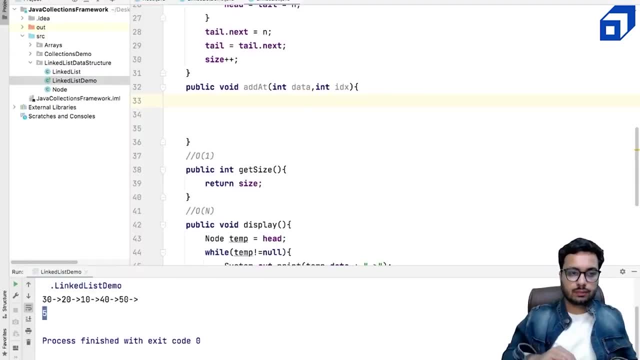 we are getting an index which is out of, we are getting an index which is out of bounds. so let us see how we will handle bounds. so let us see how we will handle bounds. so let us see how we will handle those cases, those cases, those cases. so first of all, i'm going to check if 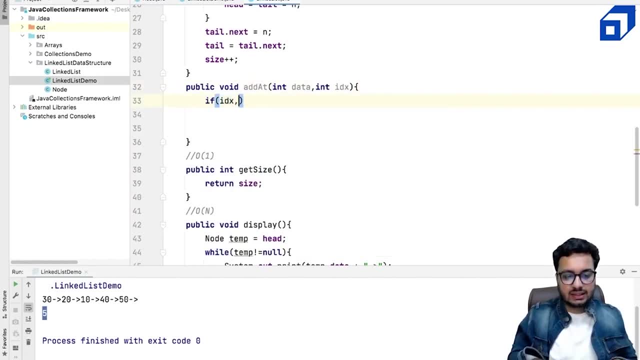 so, first of all, i'm going to check. if so, first of all i'm going to check if this index is out of bounds, right. so if this index is out of bounds, right. so if this index is out of bounds, right. so if my index is less than zero. 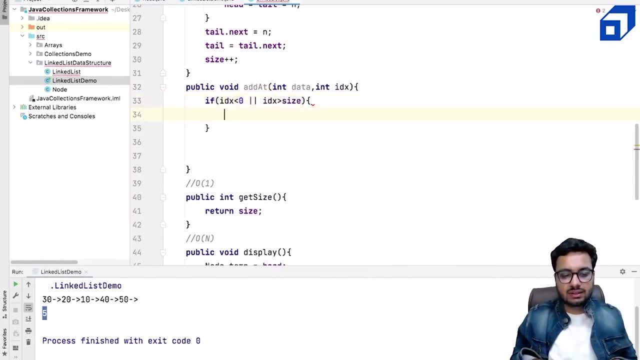 my index is less than zero. my index is less than zero, or my index is greater than the size of, or my index is greater than the size of, or my index is greater than the size of the linked list. that means the linked list. that means the linked list. that means i cannot insert this node right, so in 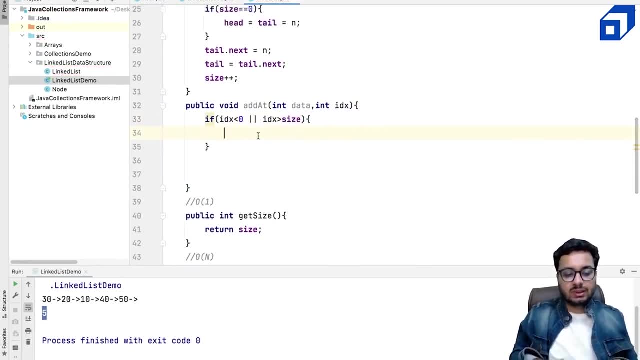 i cannot insert this node right, so in i cannot insert this node right. so in this case, what we can do is either we this case. what we can do is either we- this case. what we can do is either we, uh, simply return right, but that's not a. 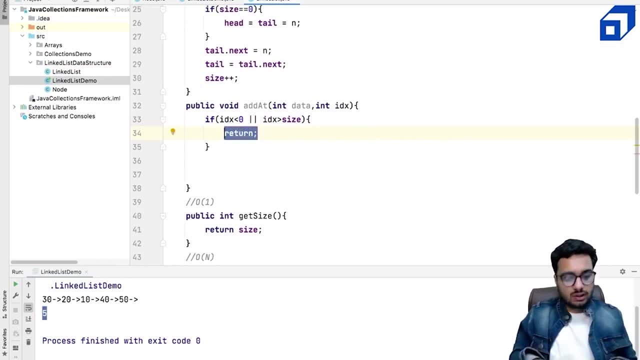 uh simply return right, but that's not a uh simply return right, but that's not a good idea. we should tell the user that good idea. we should tell the user that good idea. we should tell the user that you are doing something wrong, right, so. you are doing something wrong, right so. 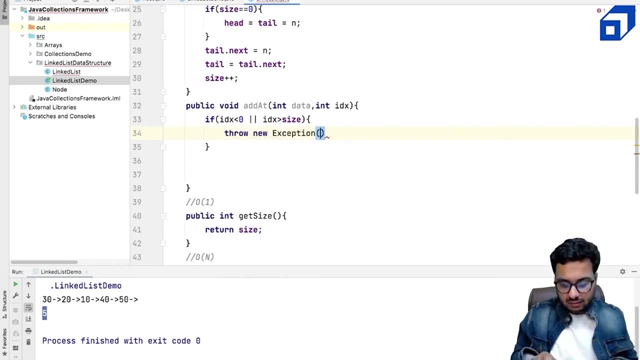 you are doing something wrong, right. so one way to do it is: we can throw a new. one way to do it is: we can throw a new. one way to do it is we can throw a new exception, exception, exception, and we can. okay, uh, index out of bounds. 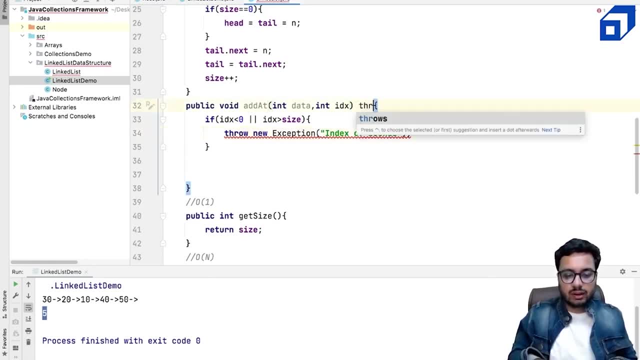 and we can, okay, uh, index out of bounds. and we can okay, uh, index out of bounds, that you're using the incorrect index, that you're using the incorrect index, that you're using the incorrect index. and here i have to say, okay, this method. and here i have to say, okay, this method. 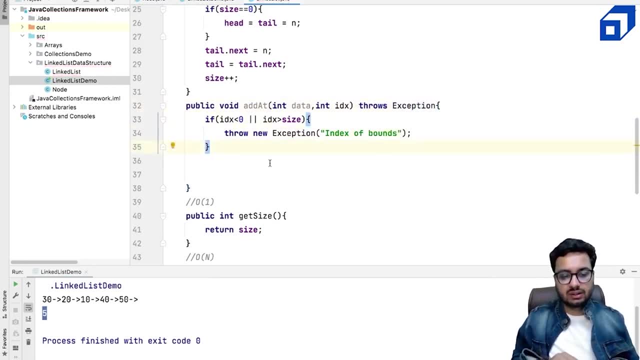 and here i have to say, okay, this method towards throws an exception right, so i towards throws an exception right, so i towards throws an exception right, so i can throw an exception in this case and can throw an exception in this case, and can throw an exception in this case, and an error will come in the main when this 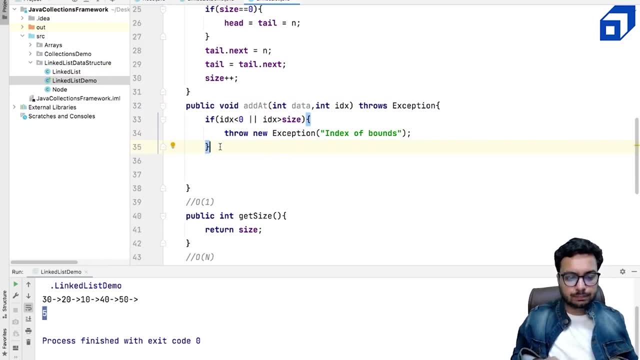 an error will come in the main when this. an error will come in the main when this program is executed. right program is executed, right program is executed, right and uh and uh and uh. now, if my index is zero, that becomes a. now, if my index is zero, that becomes a. 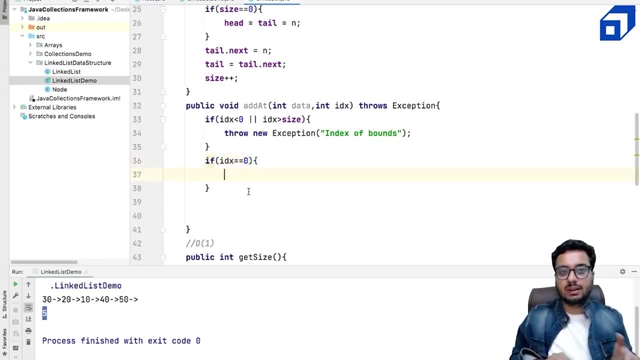 now, if my index is zero, that becomes a special case. special case, special case, that means okay, i'm trying to add that means okay, i'm trying to add. that means okay, i'm trying to add something at the beginning so that i something at the beginning so that i. 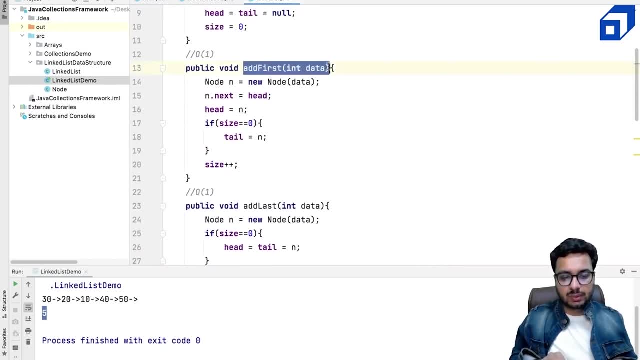 something at the beginning so that i have already, have already, have already handled. we can just call the add first handled. we can just call the add first handled. we can just call the add first method, method method with data right, so i can say: with data right, so i can say: 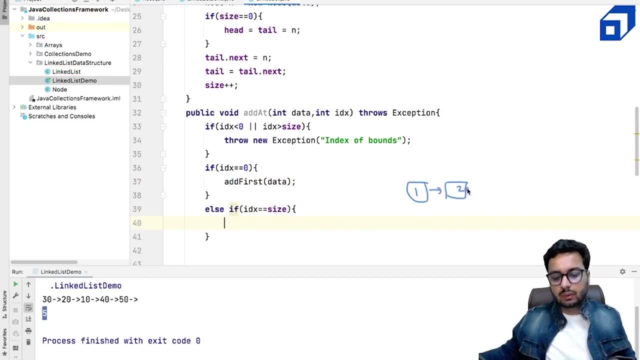 with data right. so i can say: this has three nodes, this has three nodes, this has three nodes, and you want to insert something at and you want to insert something at and you want to insert something at index three, index three, index three. that means you are inserting something. 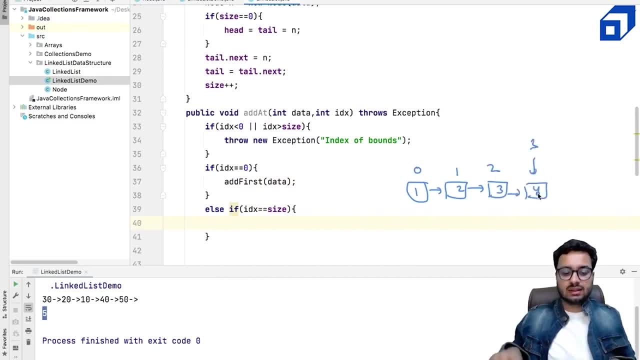 that means you are inserting something. that means you are inserting something here right, which is again at the here right, which is again at the here right, which is again at the ending of the linked list. in that case, ending of the linked list. in that case, ending of the linked list. in that case you can call the method at last and you 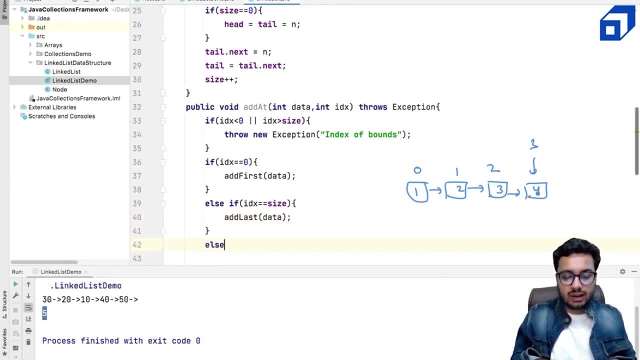 you can call the method at last, and you you can call the method at last, and you can give the data right in the else can give the data right in the else can give the data right in the else block. we have to write the exact logic block. we have to write the exact logic. 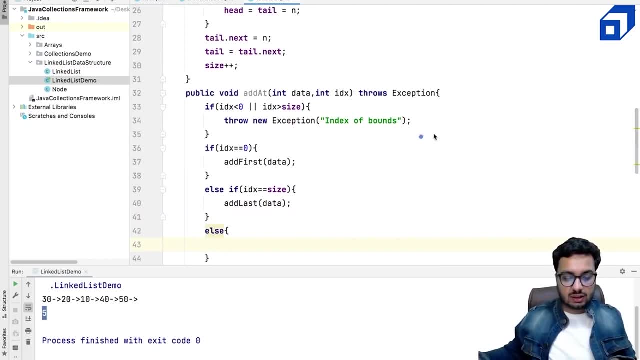 block. we have to write the exact logic that we are talking about right, so let's that we are talking about right. so let's that we are talking about right. so let's see how we will do it. suppose your. see how we will do it, suppose your. 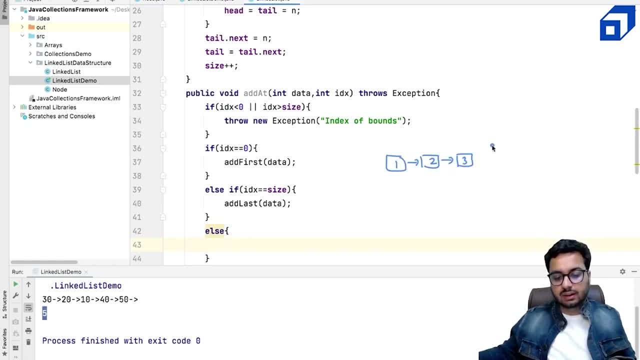 see how we will do it. suppose your linked list is like this: one, two, three linked list is like this: one, two, three linked list is like this: one, two, three, right, and i have five, six, seven right right, and i have five, six, seven, right right and i have five, six, seven, right. so i'm telling you that, okay, after three. 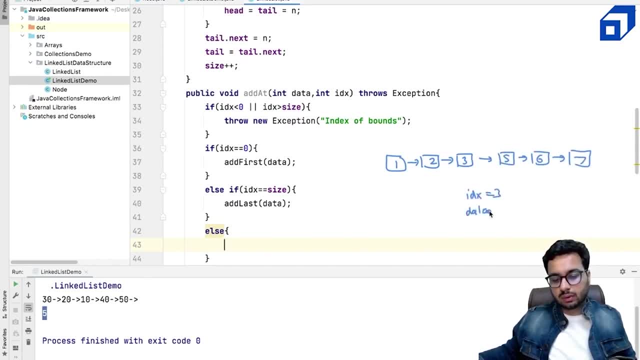 so i'm telling you that, okay, after three. so i'm telling you that, okay, after three. nodes, nodes, nodes. you have to insert a data that is four. you have to insert a data that is four. you have to insert a data that is four. right, so how do i do it? first, i need to 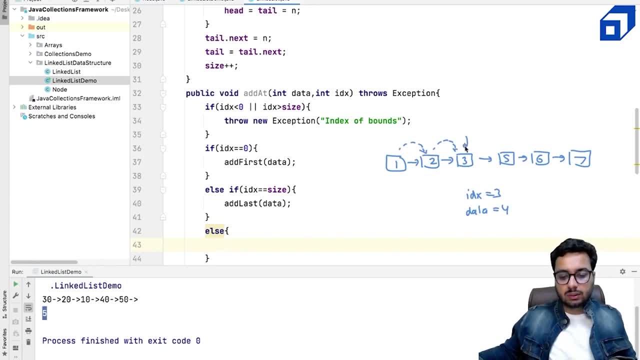 right. so how do i do it first? i need to right, so how do i do it first? i need to reach the third node right. so i need to reach the third node right. so i need to reach the third node right. so i need to take a temp. 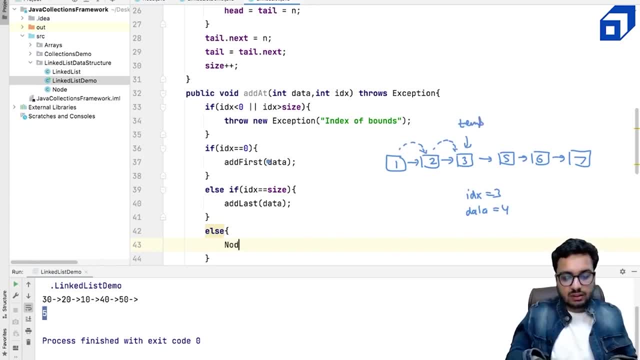 take a temp. take a temp and reach this node, so temp will start and reach this node. so temp will start and reach this node. so temp will start from head, from head from head. so i can say: node temp, this is equal to. so i can say: node temp, this is equal to. 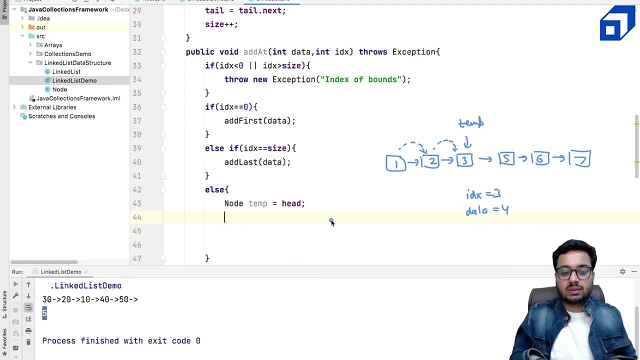 so i can say: node temp. this is equal to head. how many jumps i have to take head? how many jumps i have to take head? how many jumps i have to take? i have to take index minus one jumps, so i i have to take index minus one jumps, so i. 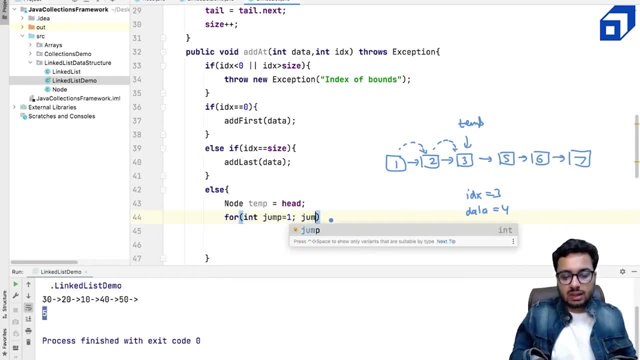 i have to take index minus one jumps so i can say okay for int, can say okay for int, can say okay for int. jump equal to one jump. equal to one jump less than uh. equal to index right jump. less than uh. equal to index right jump. less than uh. equal to index right jump plus plus right. or if it is, 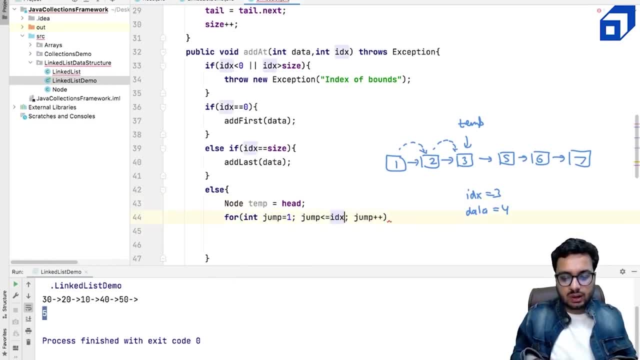 jump plus plus right, or if it is jump plus plus right, or if it is sounding confusing to you, you can say sounding confusing to you. you can say sounding confusing to you. you can say: less than equal to index minus one right. less than equal to index minus one right. 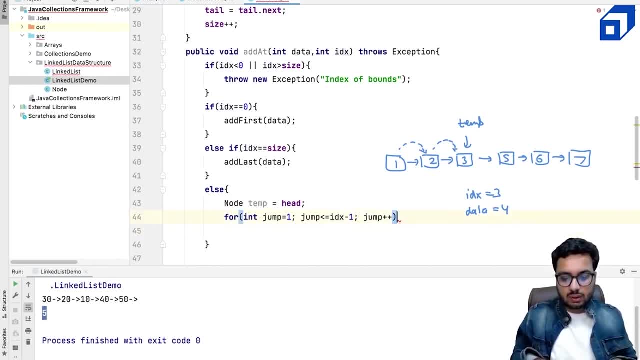 less than equal to index minus one right. these many jumps, as i told you, we have these many jumps. as i told you, we have these many jumps, as i told you, we have to take right now, in each jump, what we to take right now in each jump, what we. 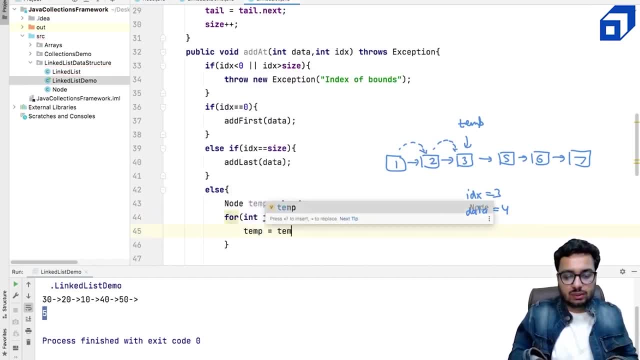 to take right now in each jump, what we should do. temp will take a step, so temp should do. temp will take a step, so temp should do. temp will take a step, so temp will go to the next node, temp equal to will go to the next node, temp equal to. 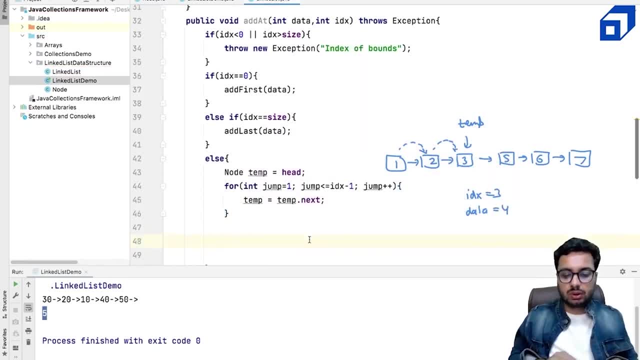 will go to the next node. temp equal to temp dot next. now i'm in a good position, temp dot next. now i'm in a good position, temp dot next. now i'm in a good position to do some insertion here. right what i to do some insertion here, right what i. 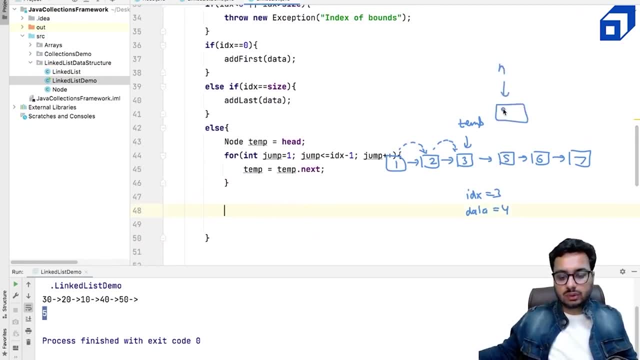 to do some insertion here. right, what i will do is okay. let me create a new node. will do, is okay. let me create a new node, will do, is okay. let me create a new node: n, n, n, whose data is four. i can say: whose data is four, i can say. 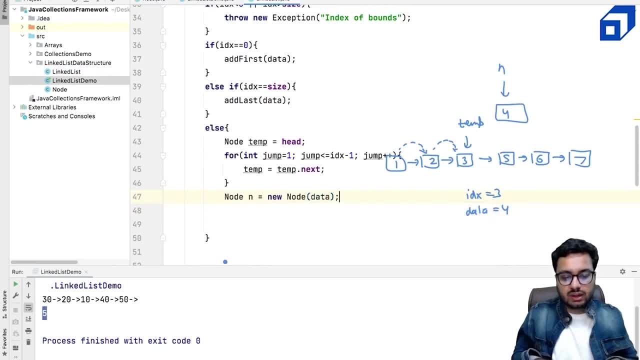 whose data is four, i can say: node n, this is equal to new node. with the node n, this is equal to new node. with the node n, this is equal to new node with the given data, given data, given data and n dot. next should refer to temp dot. 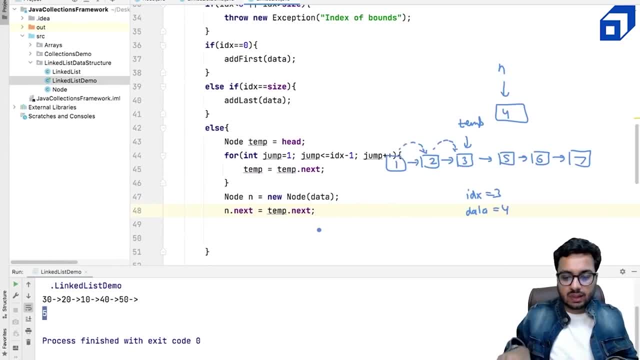 and n dot next should refer to temp dot and n dot next should refer to temp dot next, as we have just discussed here, as next, as we have just discussed here, as next, as we have just discussed here as well. right, well, right, well, right. so four should get connected with five. 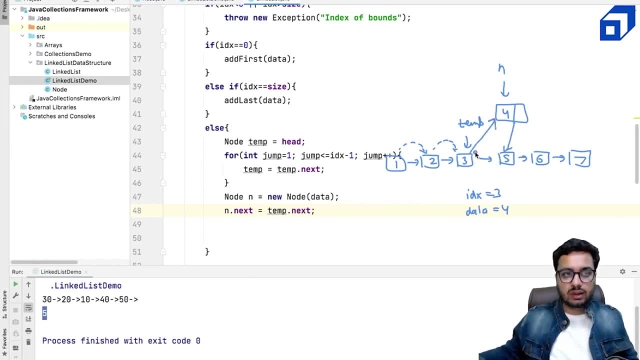 so four should get connected with five. so four should get connected with five. that is the first step. then i need to. that is the first step. then i need to. that is the first step. then i need to connect three with four, connect three with four, connect three with four, right? so how do i do it so? 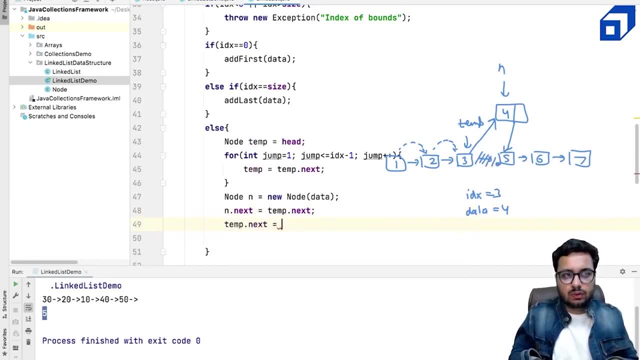 right. so how do i do it? so right, so how do i do it? so three is my temp dot, next three is my temp dot. next three is my temp dot. next should point to four. so four is n that's. should point to four, so four is n that's. 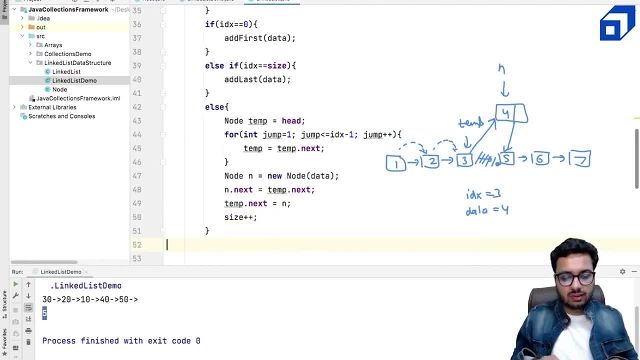 should point to four. so four is n, that's it, it it. and size plus plus size: we will update. and size plus plus size: we will update. and size plus plus size: we will update here. so here we are not doing size plus here. so here we are not doing size plus. 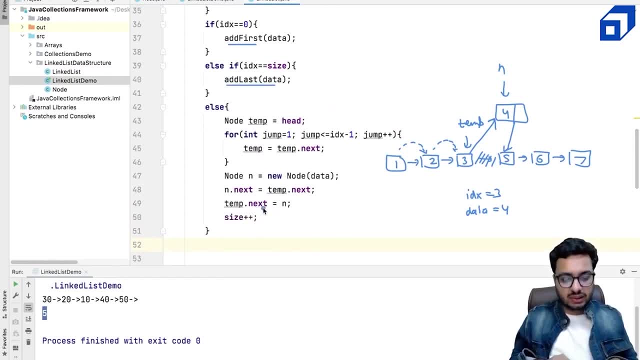 here. so here we are not doing size plus plus, because at first and at last will plus, because at first and at last will plus, because at first and at last will automatically increment the size right. automatically. increment the size right, automatically. increment the size right. that's it. so that is my insertion in the 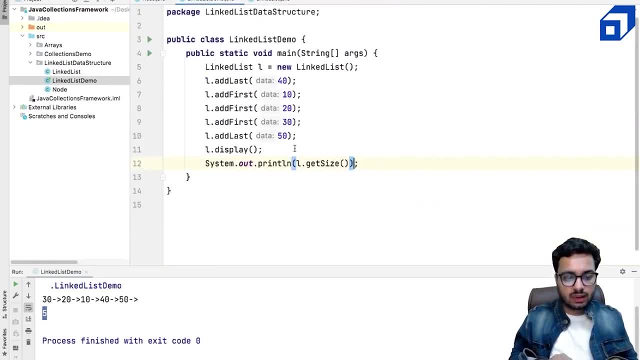 that's it. so that is my insertion in the. that's it. so that is my insertion in the middle. now let us run this code middle. now. let us run this code middle. now. let us run this code in main and see if it works really well in main. and see if it works really well. 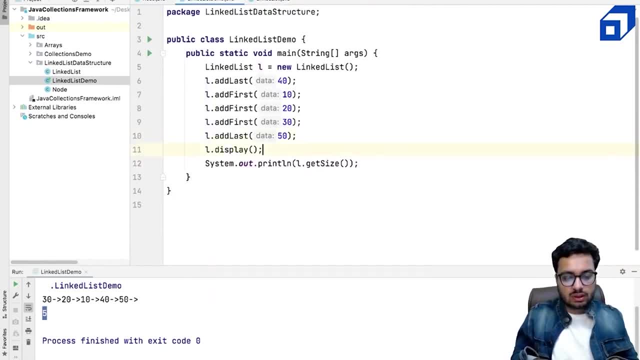 in main and see if it works really well or not. right or not right or not right now i can okay. this was my original link. now i can okay, this was my original link. now i can okay, this was my original link. list. list list. l dot add at index. 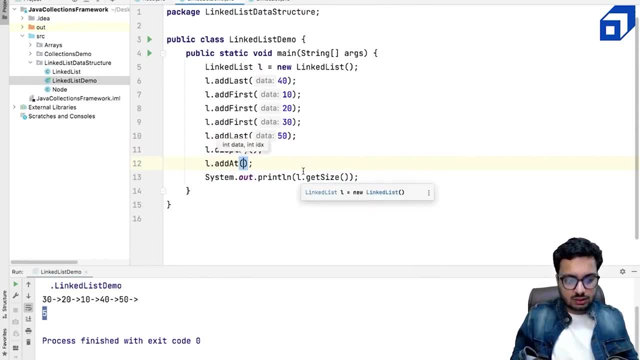 l dot. add at index. l dot. add at index. let's say i want to add: at some index: zero. let's say the data is zero, right zero. let's say the data is zero, right zero. let's say the data is zero, right. l dot. add at index. i want to add: 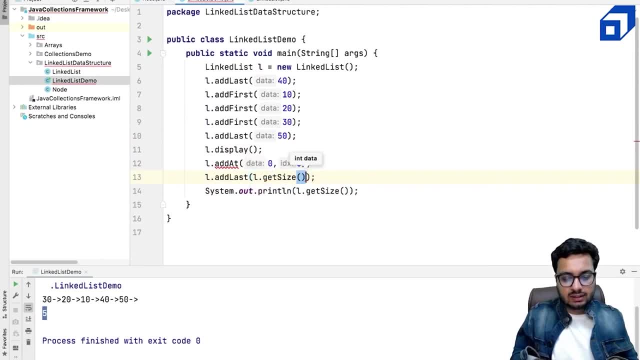 l dot add at index. i want to add. l dot add at index. i want to add something at the last index. so l dot something at the last index. so l dot something at the last index. so l dot get size, get size, get size. okay, now i'm getting a getting not add. 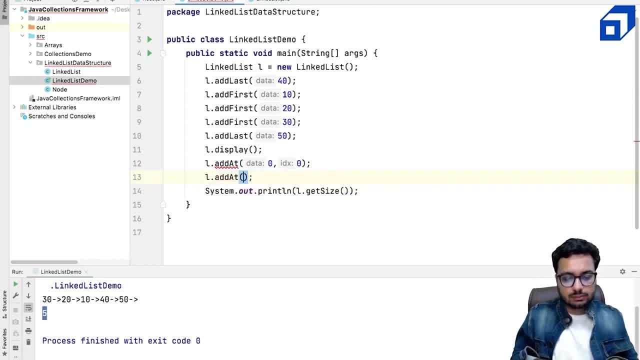 okay, now i'm getting a getting not add. okay, now i'm getting a getting not add last. but i can say last, but i can say last, but i can say add that. so index will be, let's say the last. so index will be, let's say the last. 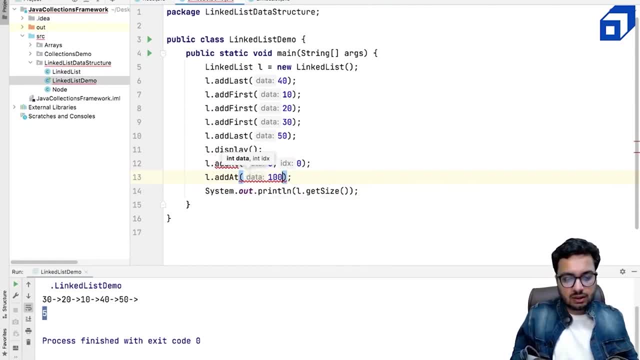 so index will be, let's say, the last index. so index, so index. so data is: let's say, 100 l dot get size. data is: let's say, 100 l dot get size. data is: let's say, 100 l dot get size. now again here. i'm getting this because 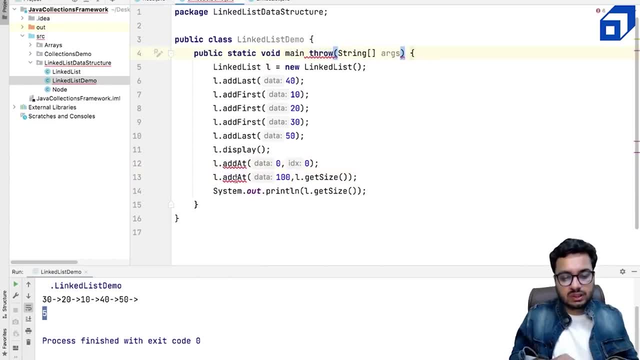 now again here i'm getting this. because now again here i'm getting this because i'm not written- throws exception, so main i'm not written throws exception, so main i'm not written throws exception, so main can also throw an exception because it can also throw an exception because it. 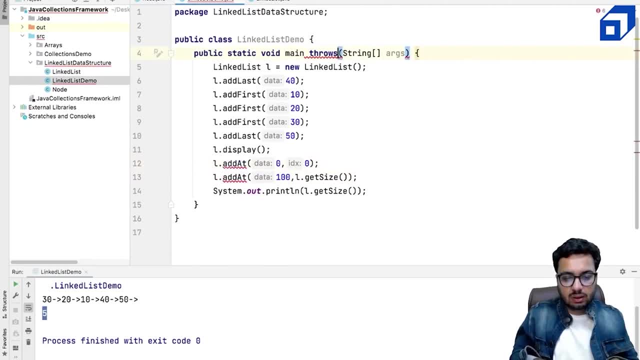 can also throw an exception, because it is calling a method that throws, is calling a method that throws, is calling a method that throws exception. so main can also, can also can also throw exception right. so we have to write throw exception right. so we have to write throw exception right. so we have to write this here right. and let's add something: 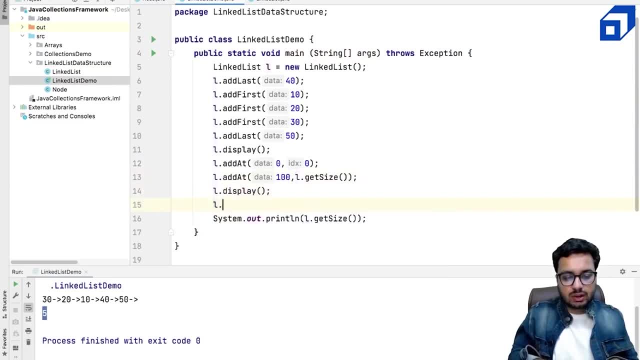 this here, right, and let's add something. this here, right, and let's add something in the middle as well. so l dot display in the middle as well. so l dot display in the middle as well. so l dot display, and i also okay l dot add at. 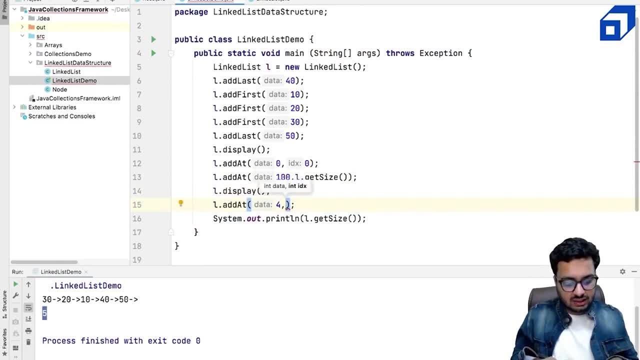 and i also okay. l dot add at and i also okay. l dot add at index 4. sorry data is 4. add some index. index 4- sorry data is 4. add some index. index 4. sorry data is 4. add some index. let's say 3. 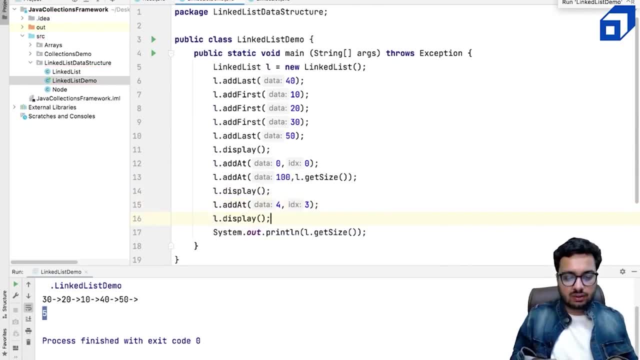 let's say 3, let's say 3, something like this. and again, let me say something like this. and again, let me say something like this. and again let me say l dot display, l dot display, l dot display. this will test over all the three cases. 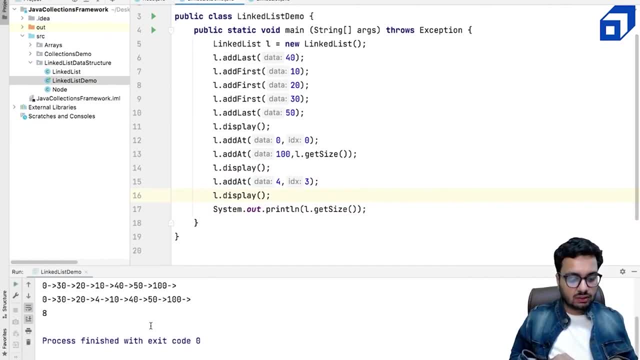 this will test over all the three cases. this will test over all the three cases and we should be and we should be, and we should be seeing that they should work fine, right. so, seeing that they should work fine, right. so, seeing that they should work fine, right. so in the first case, i added zero in the 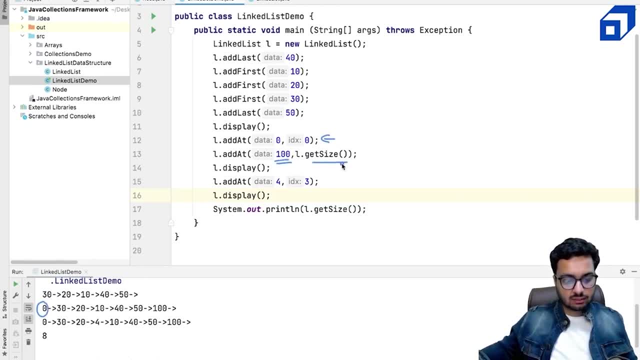 in the first case i added zero in the. in the first case i added zero in the beginning. fine beginning, fine, beginning fine. i added 100 at the end. i added 100 at the end. i added 100 at the end. fine working fine. then in this linked 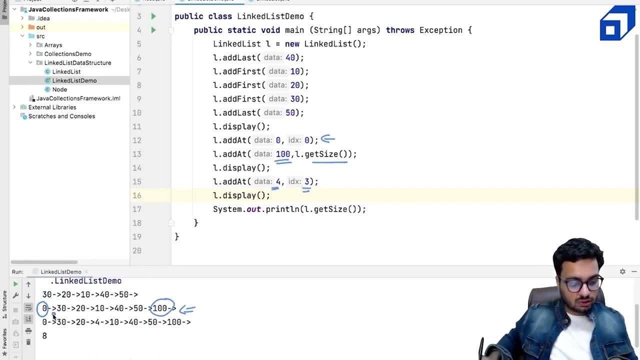 fine, working fine. then in this linked- fine, working fine. then in this linked list. i said okay at index 3, i should list. i said okay at index 3, i should list. i said okay at index 3, i should insert 4.. insert 4.. 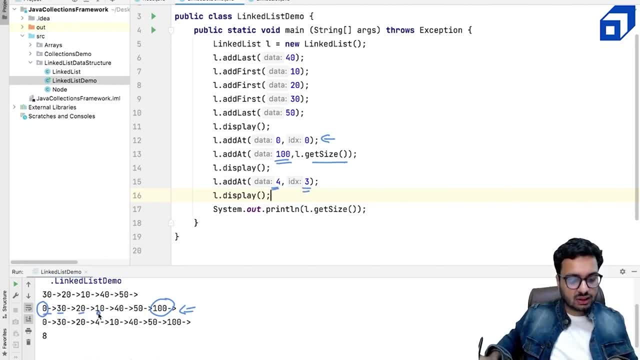 insert 4.. so 0, 30- 20. so 0, 30- 20. so 0, 30- 20. this is the third index, so before 10 i. this is the third index, so before 10 i. this is the third index, so before 10. i will insert a 4. so 0, 30- 20. i'm getting a. 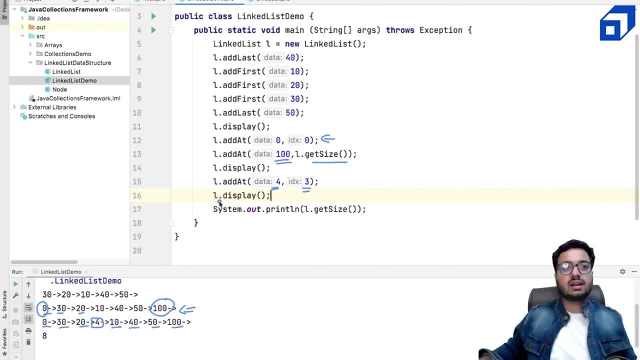 will insert a 4, so 0, 30, 20. i'm getting a will insert a 4, so 0, 30, 20. i'm getting a 4 here, 4 here, 4 here, then 10, 40, 50 and 100. that means in the. 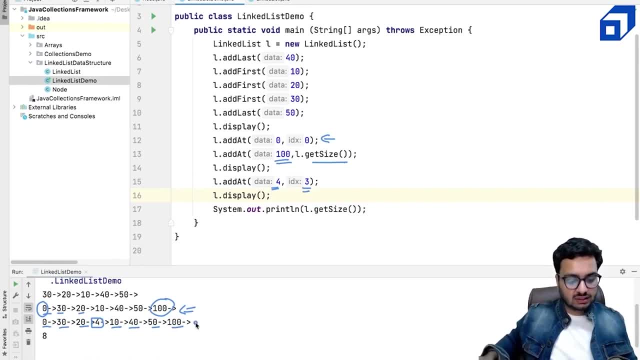 then 10, 40, 50 and 100. that means in the. then 10, 40, 50 and 100. that means in the middle. it is also working fine. middle. it is also working fine, middle. it is also working fine. and i display this list right and finally, 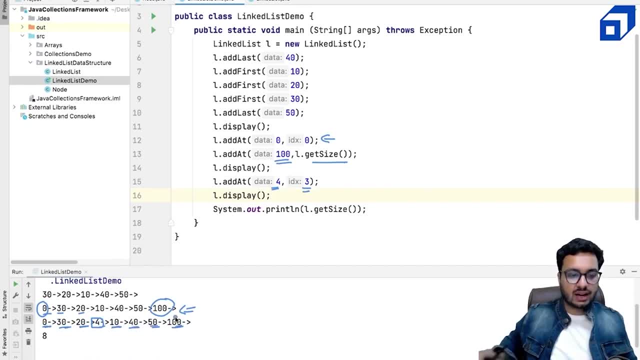 and i display this list right and finally, and i display this list right and finally, i have eight elements: one, two, three, four. i have eight elements: one, two, three, four. i have eight elements: one, two, three, four, five, six, seven, eight. that means five, six, seven, eight. that means 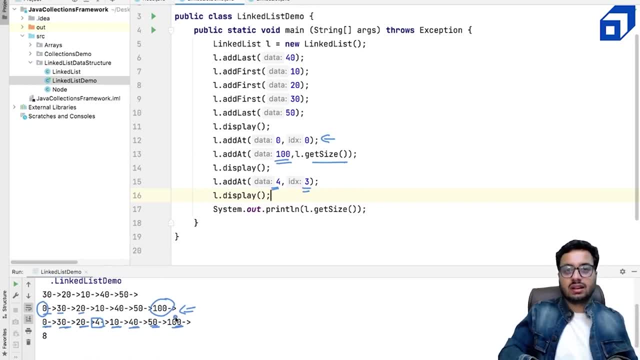 five, six, seven, eight. that means that size update is also working fine in that size update is also working fine, in that size update is also working fine in all the three cases right, all the three cases right, all the three cases right. so that completes part one. that means we 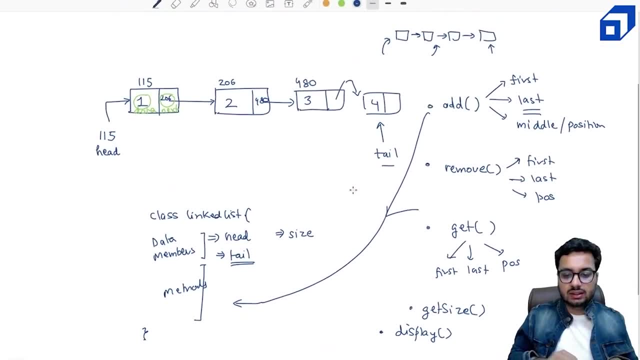 so that completes part one. that means we so that completes part one. that means we are able to add, are able to add, are able to add nodes in the linked list in all the three nodes in the linked list. in all the three nodes in the linked list, in all the three cases. 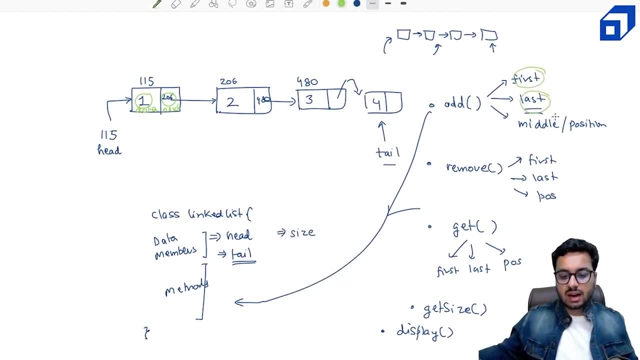 cases, cases. we have seen at first. we have seen at first. we have seen at first. we have seen at last and we have seen add. we have seen at last and we have seen add. we have seen at last and we have seen add in the middle right. next we will move. 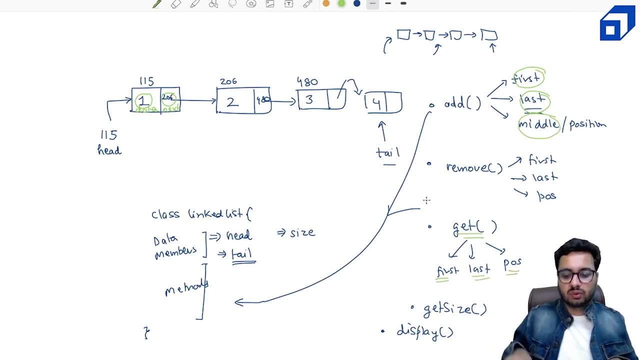 in the middle. right next we will move in the middle, right next we will move on to get on, to get on to get, and after that we will move on to, and after that we will move on to get, and after that we will move on to get the movement. so take a pause and think. 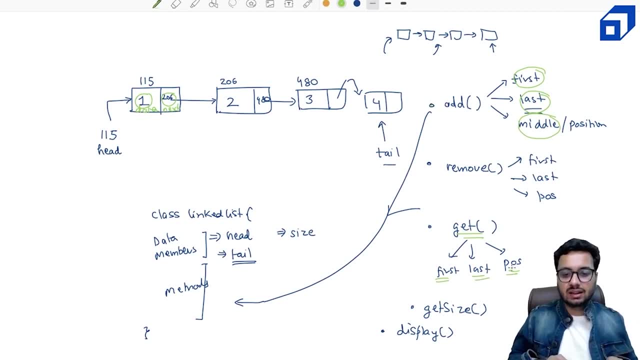 the movement. so take a pause and think the movement. so take a pause and think how you can implement these methods. get how you can implement these methods. get how you can implement these methods. get first, get last, and get an element at a first, get last and get an element at a. 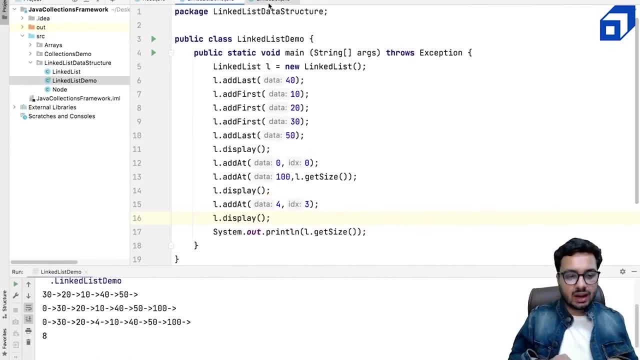 first, get last and get an element at a particular position. it's your time to particular position. it's your time to particular position. it's your time to code, and i'll just code, and i'll just code, and i'll just show you the add art method. right so? 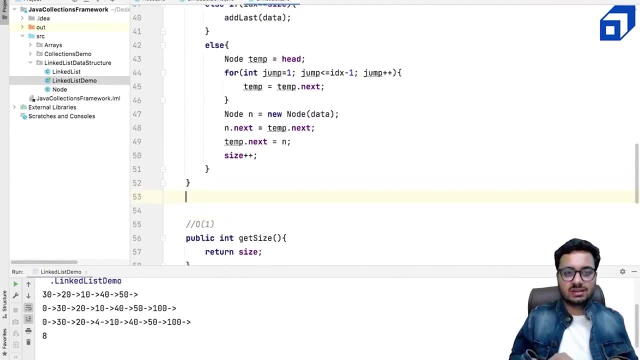 show you the add art method, right. so show you the add art method, right. so pause this video here and try to pause this video here. and try to pause this video here and try to implement these three methods. let us implement these three methods. let us implement these three methods. let us implement the get method right. so i need 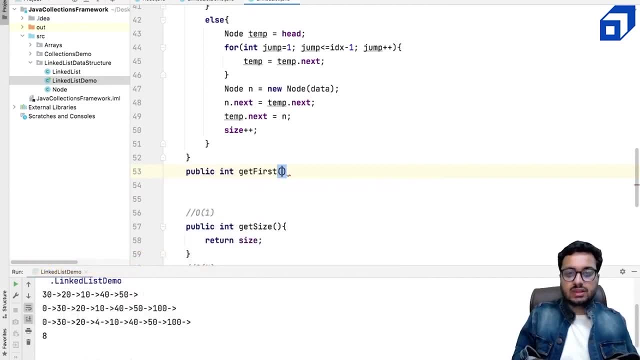 implement the get method right, so i need implement the get method right. so i need to write a method called public and get to write a method called public and get to write a method called public and get first. that means i want to get the first first. that means i want to get the first. 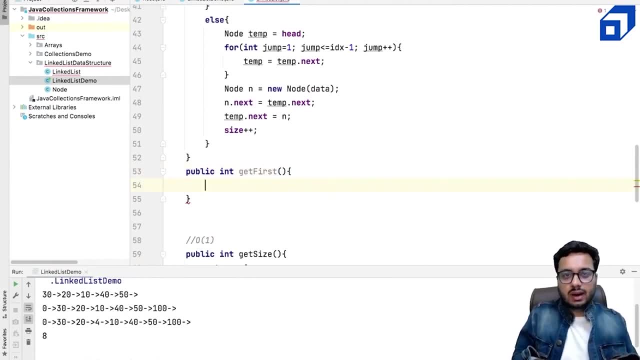 first. that means i want to get the first element of the linked list. but what if? element of the linked list? but what if element of the linked list? but what if the size of the linked list is zero? i do. the size of the linked list is zero- i do. 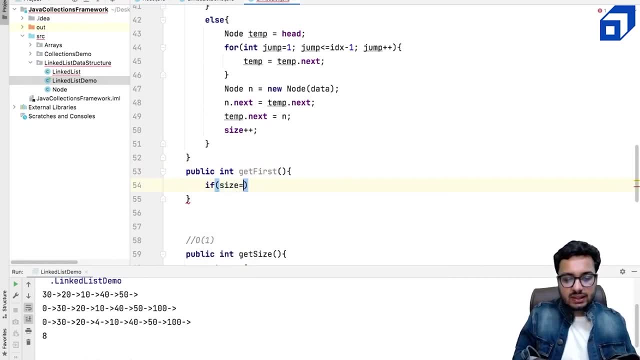 the size of the linked list is zero. i do not have any, not have any, not have any such elements, so i will have a special such elements. so i will have a special such elements. so i will have a special case, case, case. if size is zero, i can throw a new. 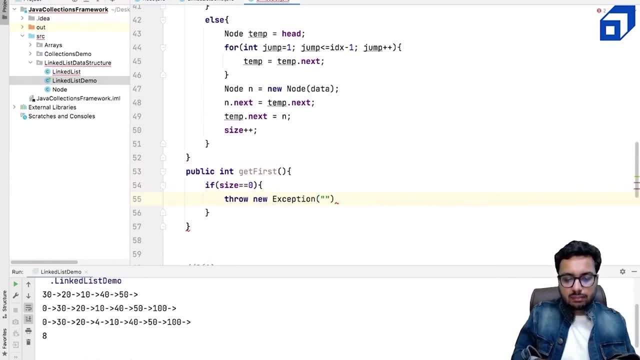 if size is zero, i can throw a new. if size is zero, i can throw a new exception exception. exception that the linked list is empty. right that the linked list is empty. right that the linked list is empty. right so linked list is empty. so linked list is empty. 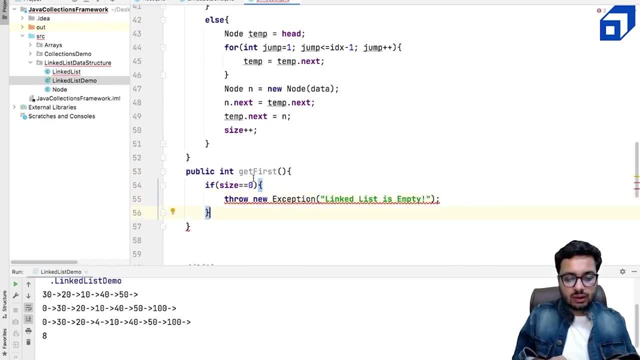 so linked list is empty. that is the error that i am trying to. that is the error that i am trying to. that is the error that i am trying to show to the user right, show to the user right, show to the user right, and here i have to tell that. okay, this. 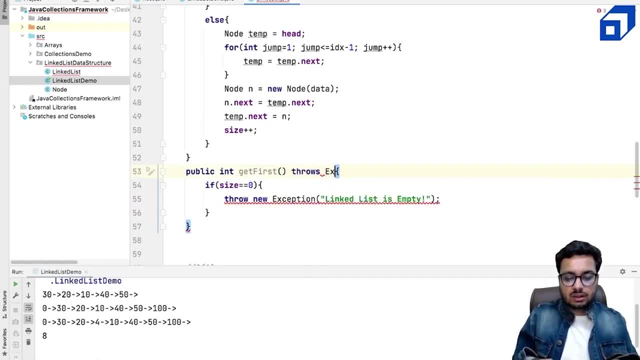 and here i have to tell that: okay, this. and here i have to tell that, okay, this method also, method also, method also. can also throw exception right. can also throw exception right. can also throw exception right. so throws exception. but if the size is so throws exception. but if the size is. 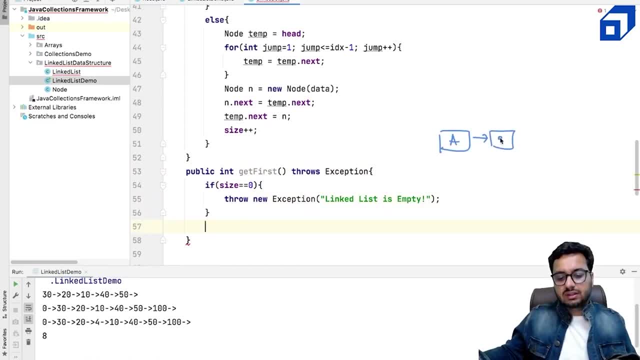 so throws exception. but if the size is not zero, the linked list is there. not zero, the linked list is there. not zero, the linked list is there. then it is pretty easy. we just need to, then it is pretty easy. we just need to. then it is pretty easy. we just need to return. 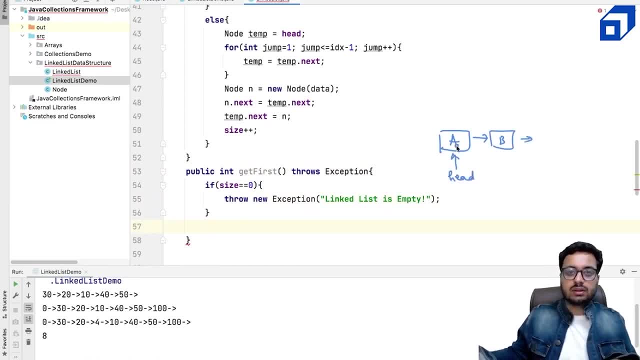 return. return the data present in the head node right. so the data present in the head node right. so the data present in the head node right. so head is referring to this node, head is referring to this node. head is referring to this node. access the data and return it. 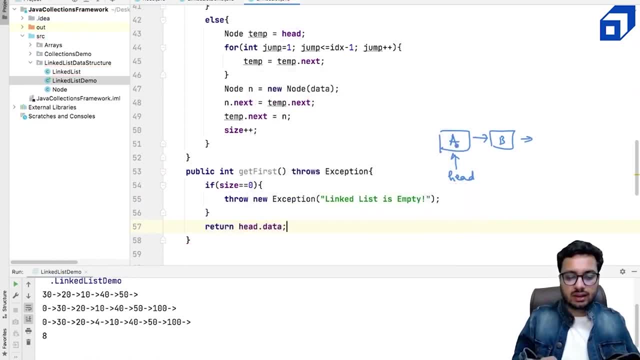 access the data and return it. access the data and return it, so return, so return, so return. add dot data that's it size will not add dot data that's it size will not add dot data that's it size will not change, change, change and this is what you will do, so similar. 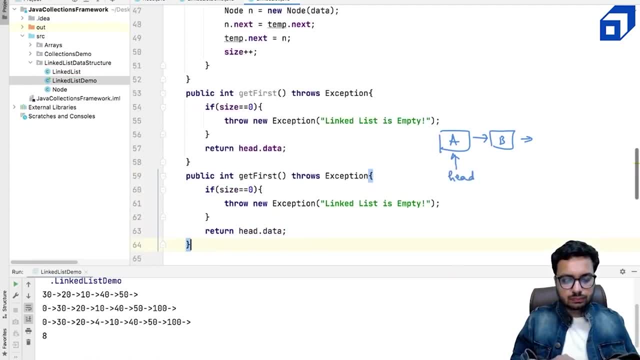 and this is what you will do. so similar, and this is what you will do, so similar to this, to this, to this: you can also write get last. you can also write get last. you can also write get last. so again, if the so again, if the so again. if the linked list is having size 0, then there is 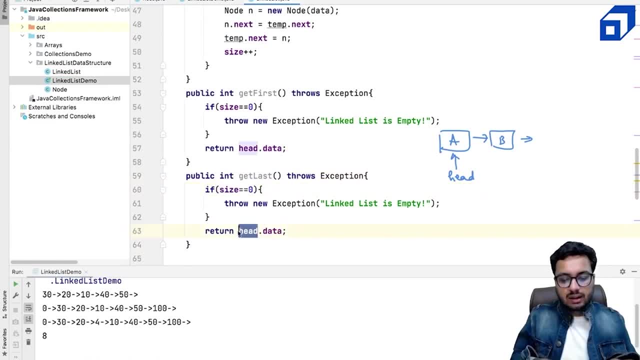 linked list is having size 0, then there is linked list is having size 0, then there is no last element. no last element, no last element. you will throw an exception and in that you will throw an exception, and in that you will throw an exception, and in that case, the last. 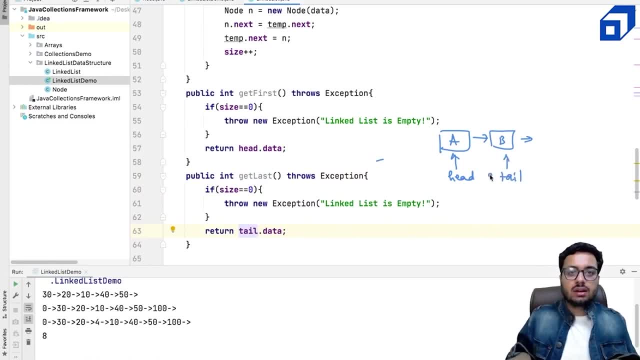 case, the last case, the last data will be at the tail node. right you data will be at the tail node, right you data will be at the tail node, right. you can say return. can say return. can say return tail dot data. that's it, if you want to. 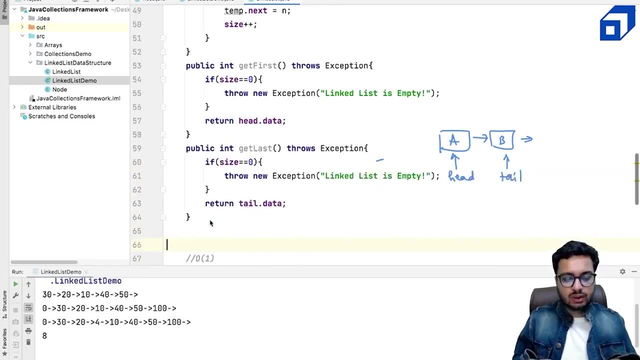 tail dot data, that's it. if you want to tail dot data, that's it. if you want to get something in, get something in. get something in in the middle. that is going to take in the middle. that is going to take in the middle. that is going to take one more step, because you will have to. 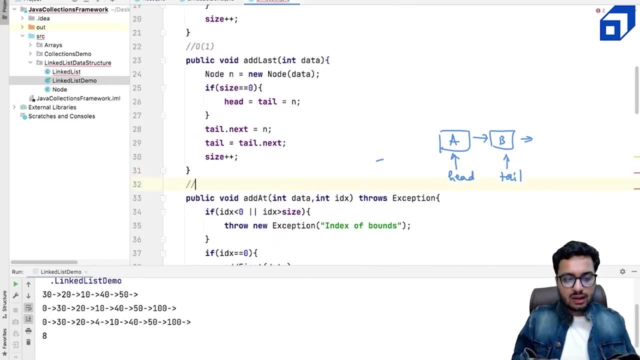 one more step because you will have to one more step, because you will have to loop through it right, loop through it right. loop through it, right, okay, so add that we did not discuss. okay, so add that we did not discuss. okay, so add that we did not discuss. it's going to take. 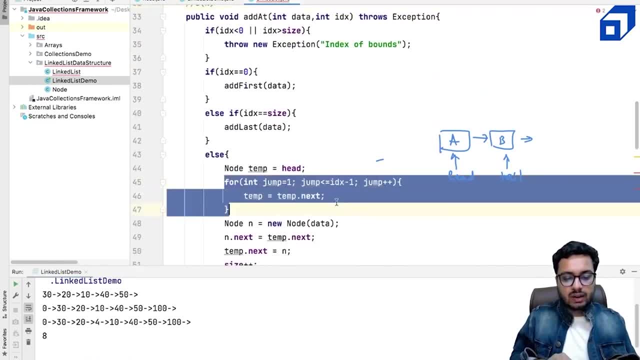 it's going to take, it's going to take order and time because your the worst order and time, because your the worst order and time, because your the worst case. you might have to case, you might have to case, you might have to loop till the second last or the last. 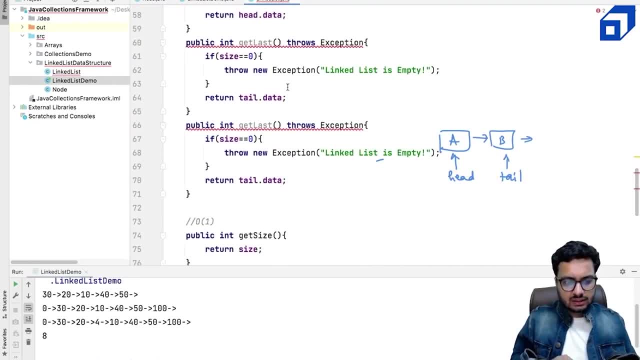 loop till the second last, or the last loop till the second last, or the last, one right, one right, one right. so get last. we have done. now this, this will be get at a now this, this will be get at a now this, this will be get at a element at that. 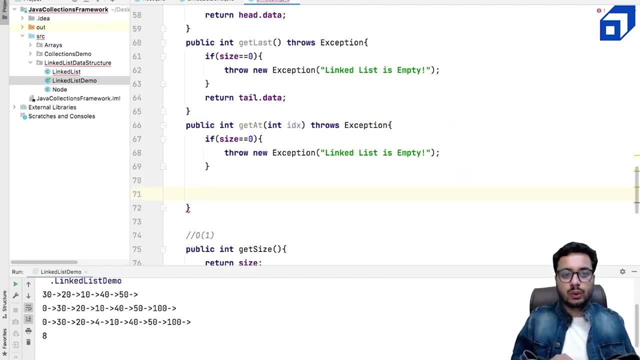 element at that, element at that- how it will work out. take a pause and how it will work out. take a pause and how it will work out. take a pause and think how you will do it. this is also think how you will do it. this is also 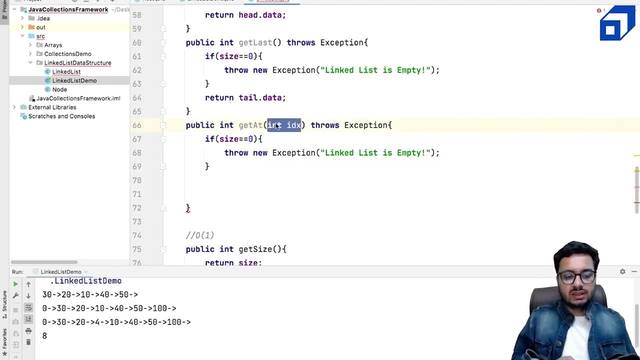 think how you will do it. this is also easy. right now, user is giving you an easy. right now, user is giving you an easy. right now, user is giving you an index. now it is possible that this index index. now it is possible that this index index. now it is possible that this index is also out of bounds. 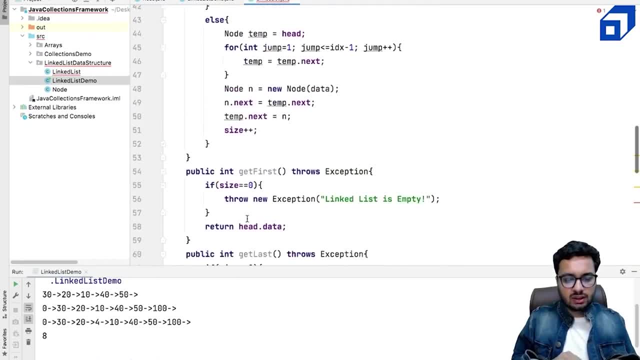 is also out of bounds, is also out of bounds, like we saw here right like in the case, like we saw here right like in the case, like we saw here right like in the case of addition. it is also possible that of addition, it is also possible that. 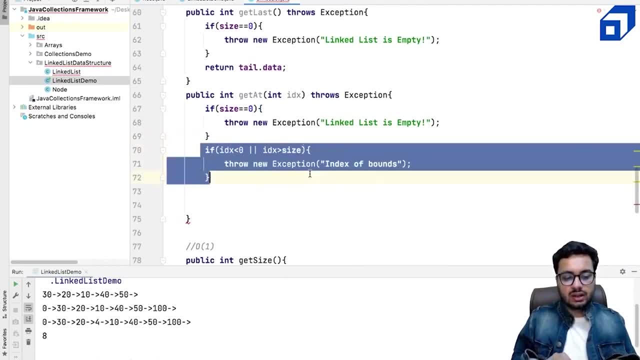 of addition, it is also possible that this index is out of bounds. so if index, this index is out of bounds. so if index, this index is out of bounds, so if index is less than zero or it is greater than is less than zero or it is greater than. 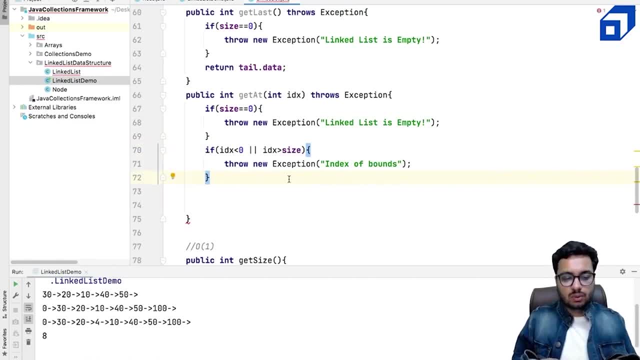 is less than zero or it is greater than size, i can throw an exception index out size. i can throw an exception index out size. i can throw an exception index out of bounds of bounds of bounds. then if this is not the case right, then if this is not the case right. 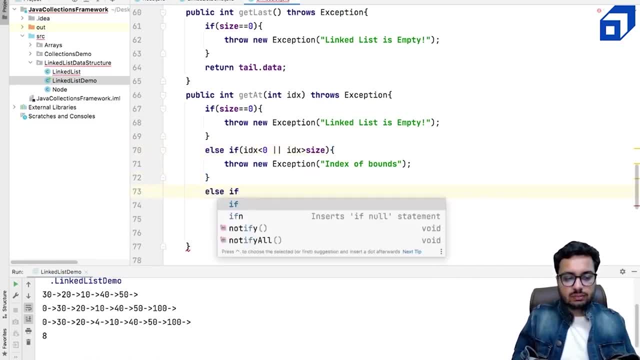 then if this is not the case, right. so if this is not the case, if the user, so, if this is not the case, if the user, so if this is not the case, if the user is is, is really giving you a valid index right, really giving you a valid index right? 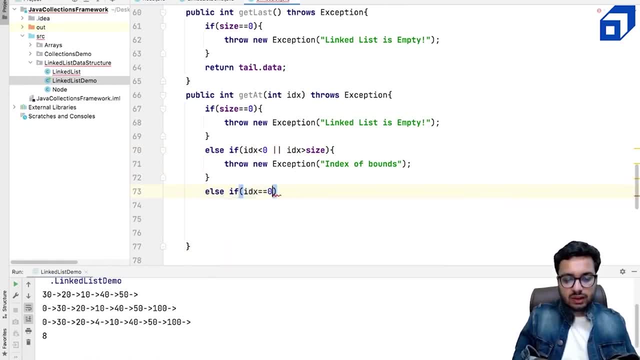 really giving you a valid index right, as if it is possible. you are talking as if it is possible. you are talking as if it is possible. you are talking about index 0, about index 0, about index 0. if that is the case, you can say return. 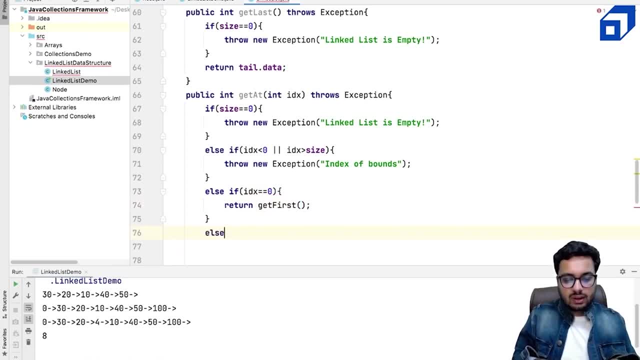 if that is the case, you can say return. if that is the case, you can say return, get first, get first, get first. this can happen, as if index is equal to. this can happen, as if index is equal to. this can happen, as if index is equal to size. 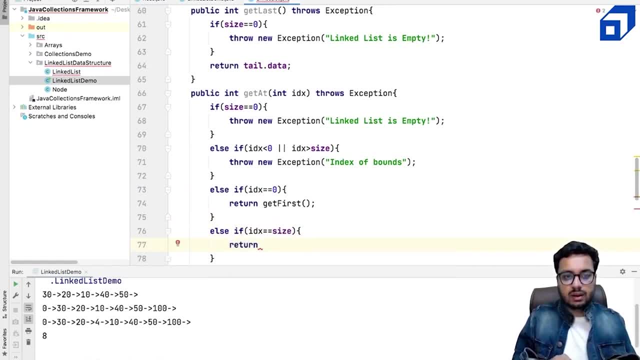 size. size: you can say return. you can say return. you can say return size or size minus one. size or size minus one. size or size minus one: it will be size minus one because the it will be size minus one, because the it will be size minus one because the last element will have an index size. 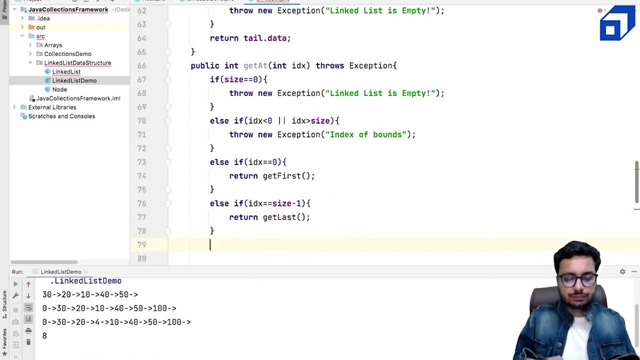 last element will have an index size. last element will have an index size minus one. you can say return minus one. you can say return minus one. you can say return: get last right, get last right, get last right. otherwise, what you need to do, you need to. otherwise, what you need to do, you need to. 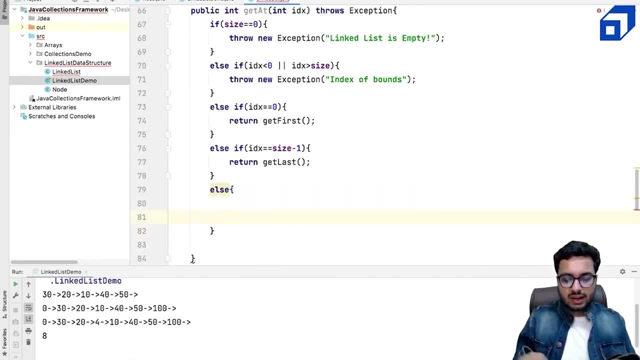 otherwise, what you need to do, you need to iterate, iterate, iterate on the linked list right, so that on the linked list right, so that on the linked list right, so that iteration part is easy, iteration part is easy, iteration part is easy. what we will do, we'll have, let's say, a, b, 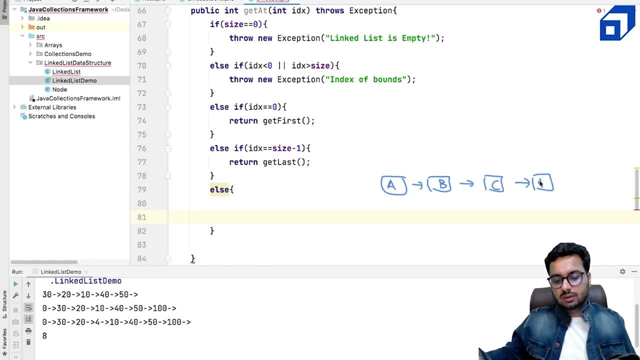 what we will do, we'll have, let's say a- b. what we will do, we'll have, let's say a, b, c, c, c, d and so on. right, this is index 0, d, and so on. right, this is index 0 d, and so on. right, this is index 0, 1, 2, 3, 4. right? i want to get something. 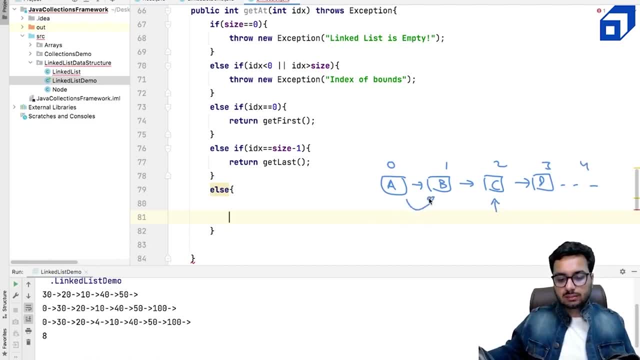 1, 2, 3, 4. right, i want to get something: 1, 2, 3, 4. right, i want to get something at the second index. what i need to do at the second index? what i need to do at the second index? what i need to do, i need to take one jump. 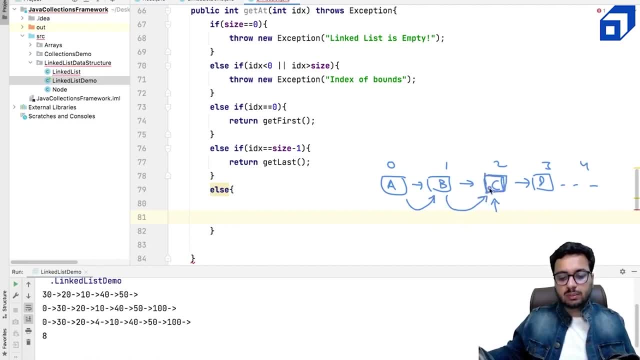 i need to take one jump. i need to take one jump, one more jump, two jumps to reach this, one more jump, two jumps to reach this. one more jump, two jumps to reach this particular index right. so that means particular index right. so that means particular index right. so that means take the number of jumps equal to that. 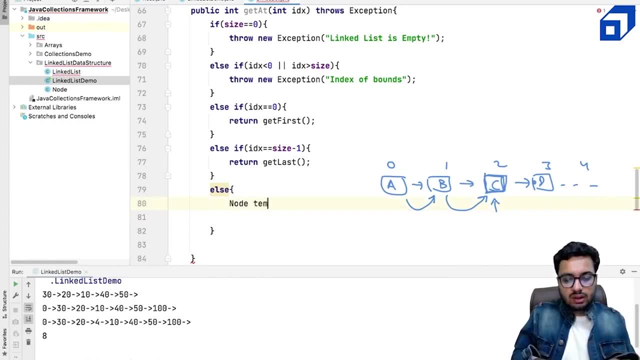 take the number of jumps equal to that. take the number of jumps equal to that index, index index. so i can say, okay, fine. so i can say okay, fine. so i can say, okay, fine, node temp that is equal to head, node temp that is equal to head. 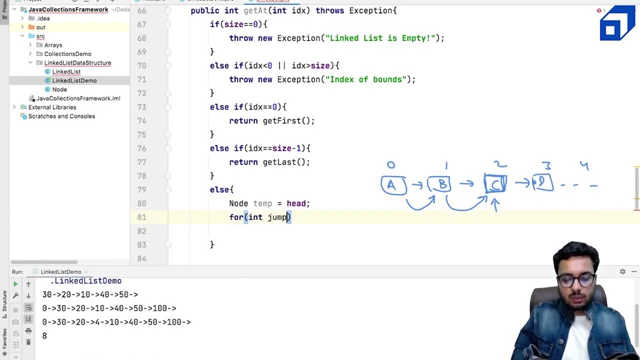 node temp that is equal to head and uh and uh and uh for int jump equal to one. for int jump equal to one. for int jump equal to one jump less than equal to index jump. less than equal to index jump. less than equal to index jump plus plus. 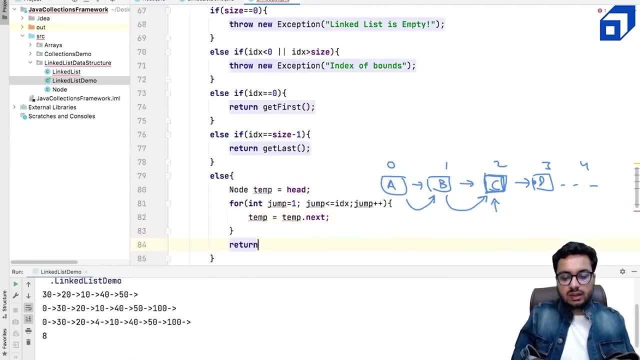 plus plus, plus plus temp dot. next. once i reach this node, i temp dot. next. once i reach this node, i temp dot. next, once i reach this node, i need to return the data of that node, so need to return the data of that node. so need to return the data of that node. so return temp dot data. that's it. 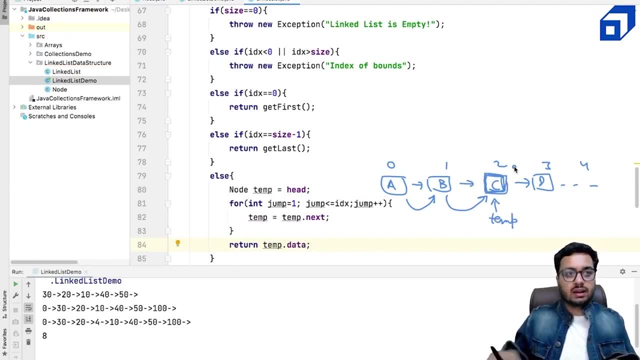 return temp dot data. that's it. return temp dot data. that's it. so i take my temp here, so i take my temp here, so i take my temp here and i return this data right. this will, and i return this data right. this will, and i return this data right. this will give me the data at a. 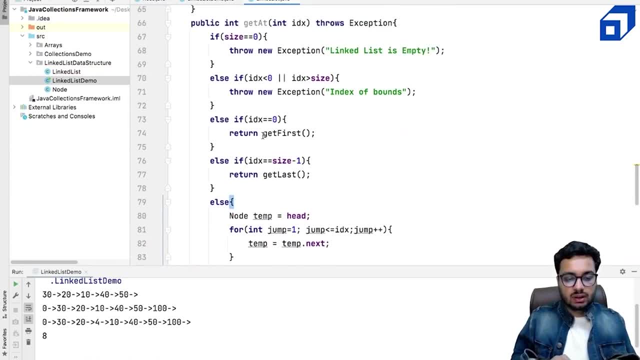 give me the data at a. give me the data at a given position. so that is my get at a given position. so that is my get at a given position. so that is my get at a particular, particular particular index, index, index. now let us test this code. so i want to. 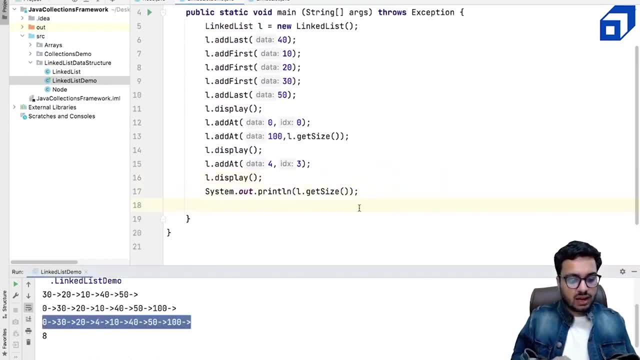 now let us test this code. so i want to now let us test this code. so i want to say okay fine, say okay fine, say okay fine in this link list that we have. i want to. in this link list that we have, i want to. in this link list that we have, i want to get the zeroth element. 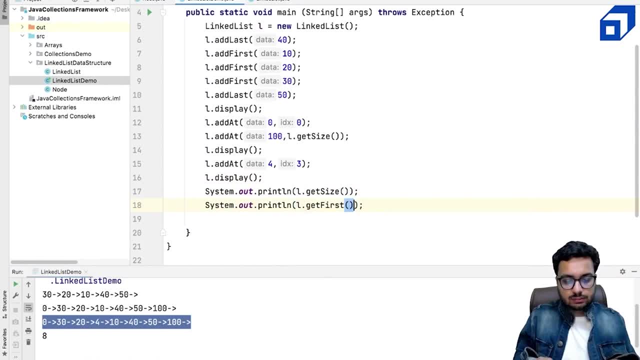 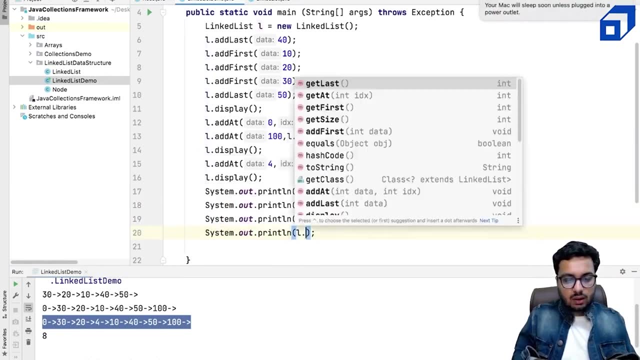 get the zeroth element. get the zeroth element s out. l dot get first s out. l dot get first s out. l dot get first s out. l dot get last s out. l dot get last s out. l dot get last and s out l dot. 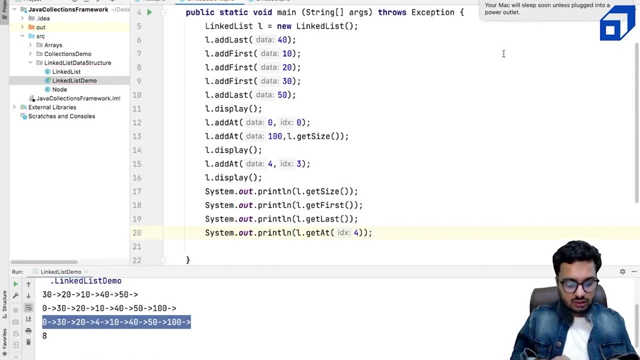 and s out. l dot get at and s out. l dot get at and s out. l dot get at index four, index four, index four. let's go and run this code the first. let's go and run this code the first. let's go and run this code: the first element is zero. last element is 100. 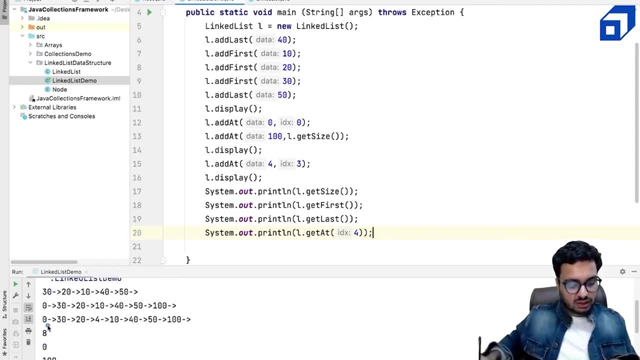 element is zero. last element is 100. element is zero. last element is 100. the fourth element is 10. let us verify the fourth element is 10. let us verify the fourth element is 10. let us verify the zeroth index: first index second. the zeroth index: first index second. 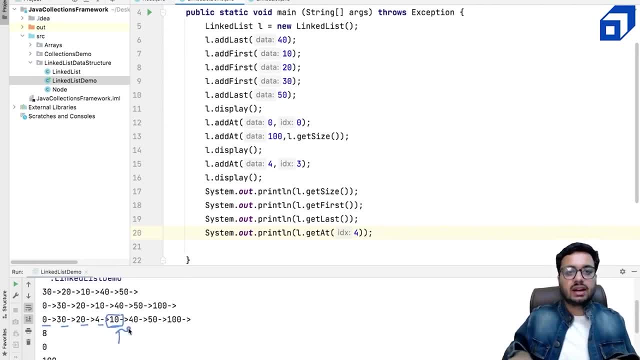 the zeroth index, first index. second index, third index, fourth index. so fourth index, third index, fourth index. so fourth index, third index, fourth index. so fourth index is really 10. that means my output index is really 10. that means my output index is really 10. that means my output is correct. 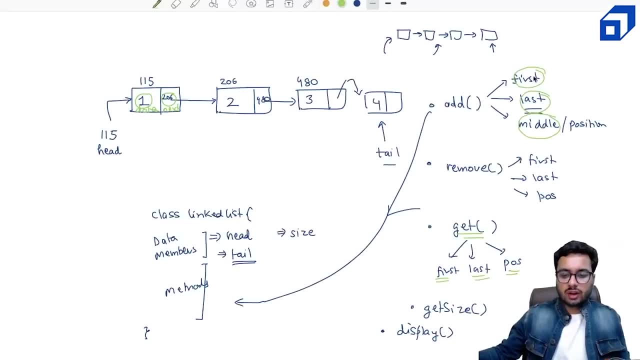 is correct is correct. that is how we build the get art methods. that is how we build the get art methods. that is how we build the get art methods. in the link: so far we have seen uh the. in the link so far we have seen uh, the. 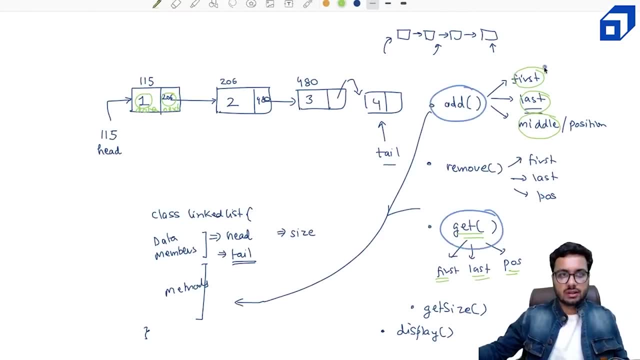 in the link. so far we have seen, uh, the add method, add method and the get methods: okay, all the three. and the get methods: okay, all the three. and the get methods: okay, all the three versions. so getting first versions, so getting first versions. so getting first, adding first. they all take order one. 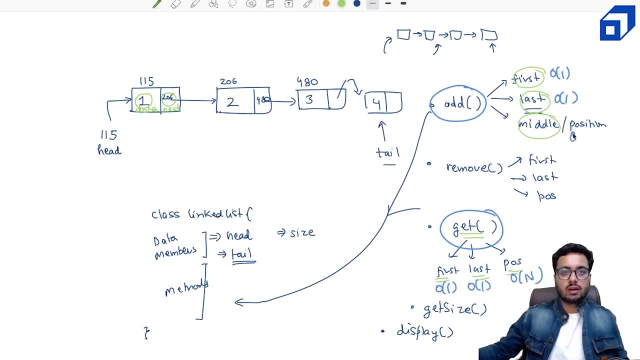 adding first. they all take order. one adding first. they all take order one time. but doing some work at a particular time, but doing some work at a particular time, but doing some work at a particular position, position, position: they take order of end time, right. so they take order of end time, right so. 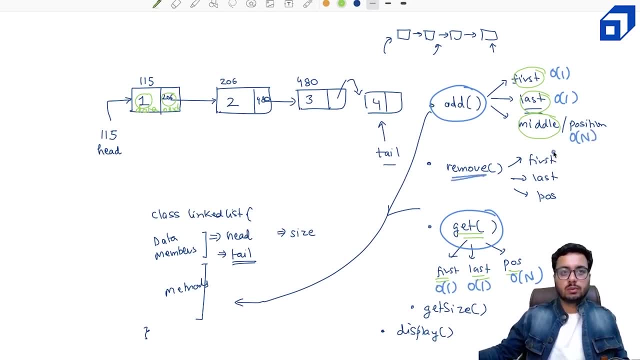 they take order of end time right. so other methods are all one, other methods are all one, other methods are all one. now we have the remove method. we want to. now we have the remove method. we want to. now we have the remove method. we want to remove first, remove last and remove at a. 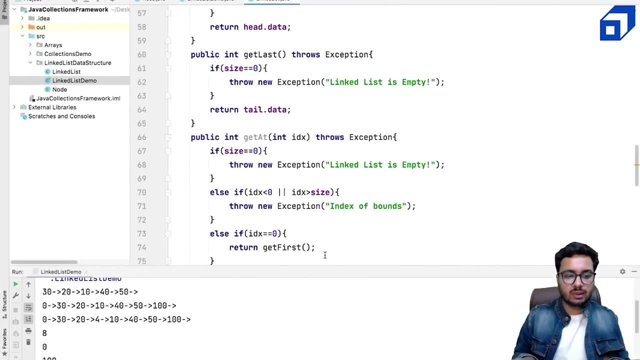 remove first, remove last and remove at a remove first, remove last and remove at a particular position, particular position, particular position. let us see how we will write these. let us see how we will write these. let us see how we will write these methods. okay, so what i will do? i will. 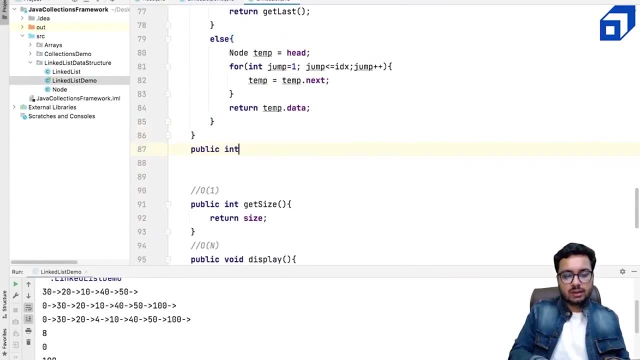 methods: okay, so what i will do. i will methods. okay, so what i will do. i will create- remove methods. public end, so create. remove methods. public end, so create. remove methods. public end, so remove. i will also get the data that has remove. i will also get the data that has. 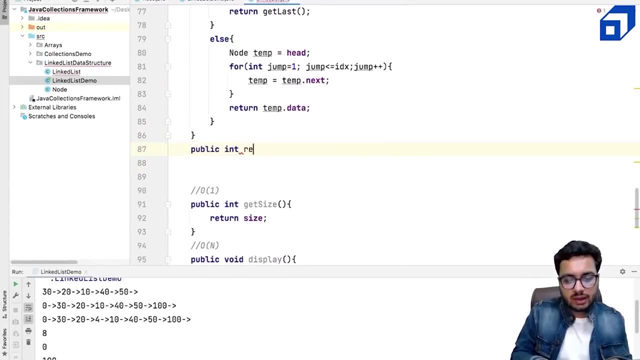 remove. i will also get the data that has been removed from that particular index. been removed from that particular index. been removed from that particular index, so return type would be int, so remove. so return type would be int, so remove. so return type would be int, so remove first. 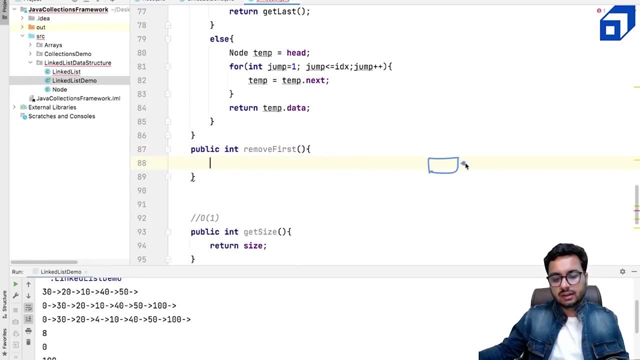 first. first, you might think it should be very simple. you might think it should be very simple. you might think it should be very simple. whatever is right at the head, whatever is right at the head, whatever is right at the head, i will, uh, return that right. so i want to. 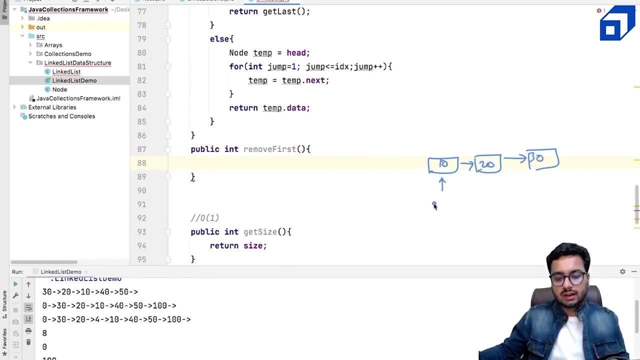 i will uh return that right, so i want to. i will uh return that right, so i want to remove this. let's say 10 is there- remove this. let's say 10 is there- remove this. let's say 10, is there 20 and 30. and this is my head. how do i? 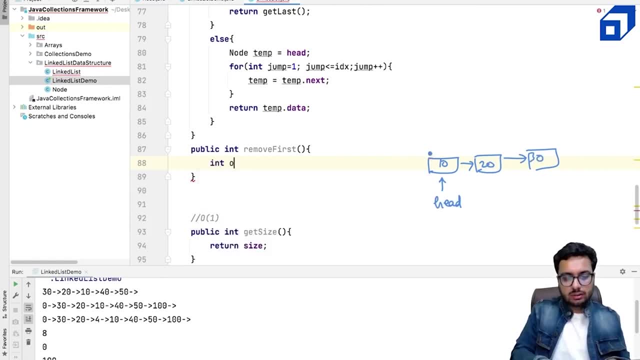 20 and 30? and this is my head. how do i 20 and 30? and this is my head. how do i remove this node? remove this node, remove this node. so one way is okay: you can store the. so one way is okay, you can store the. 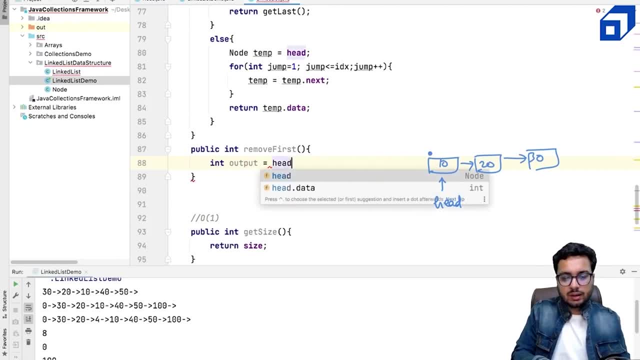 so one way is: okay, you can store the output, output, output that is going to be head dot data, that is going to be head dot data, that is going to be head dot data. and then you can say: okay, this head. and then you can say: okay, this head. 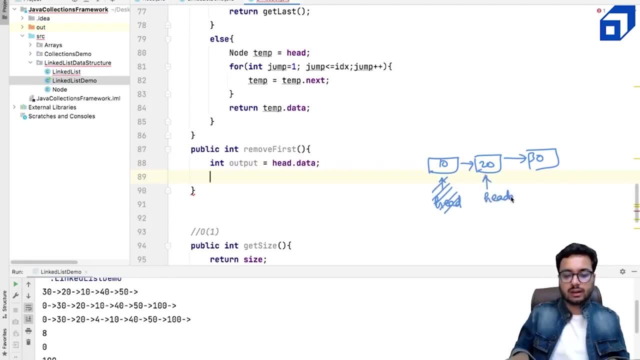 and then you can say, okay, this head will move to the next node, will move to the next node, will move to the next node. so head will go here. right, so head is. so head will go here. right, so head is. so head will go here. right, so head is going to. 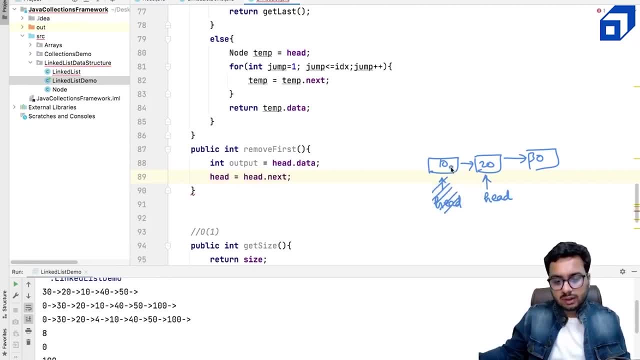 going to going to be at head dot next right, so doing this. be at head dot next right, so doing this. be at head dot next right, so doing this. will it remove this node? the answer is: will it remove this node? the answer is: will it remove this node? the answer is yes, so in heap. 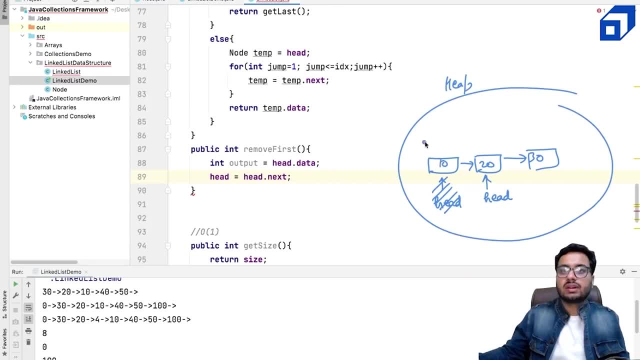 yes, so in heap, yes, so in heap. uh, this node, uh this node, uh, this node is a node that no one is referring to. is a node that no one is referring to. is a node that no one is referring to, what will happen? it becomes eligible for. 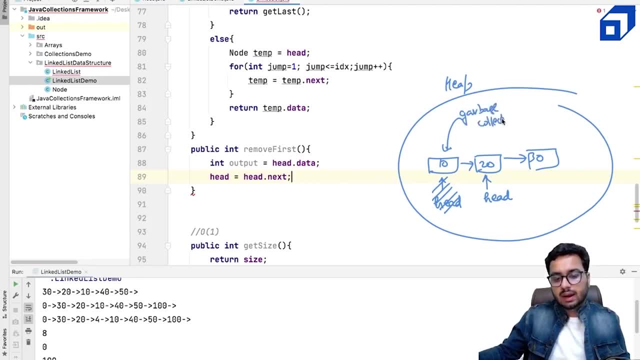 what will happen? it becomes eligible for. what will happen? it becomes eligible for garbage collection, garbage collection, garbage collection. the garbage collector will come. the garbage collector will come. the garbage collector will come and it will going to. it's going to sweep and it will going to, it's going to sweep. 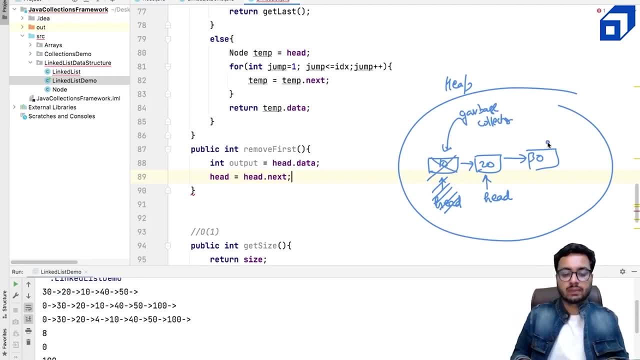 and it will going to. it's going to sweep away this memory. so that means now your away this memory. so that means now your away this memory. so that means now your linked list will be only this right linked list will be only this right linked list will be only this right. but there are a few special cases, right. so 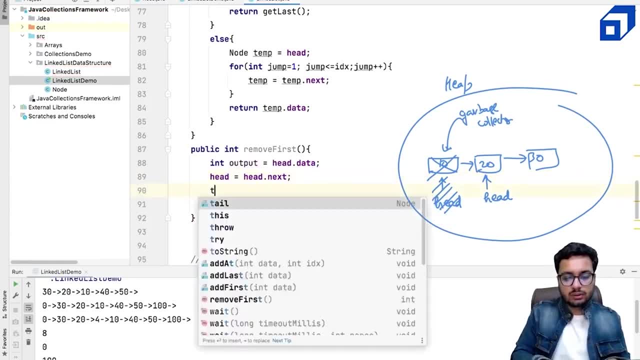 but there are a few special cases right so, but there are a few special cases right so i can say the output will be returned. i can say the output will be returned. i can say the output will be returned, that's okay. you also need to reduce the. 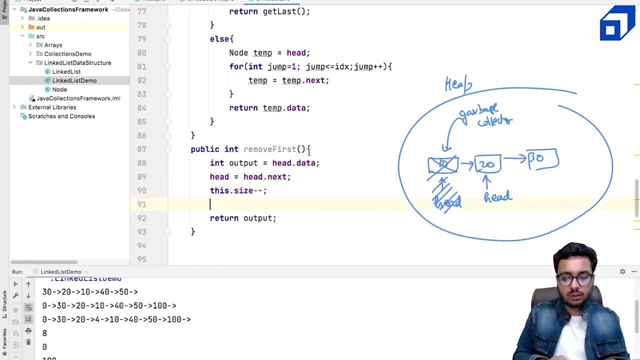 that's okay. you also need to reduce the. that's okay. you also need to reduce the size. this dot size minus minus. this is size. this dot size minus minus. this is size. this dot size minus. this is something we need to do right, but what something we need to do right, but what? 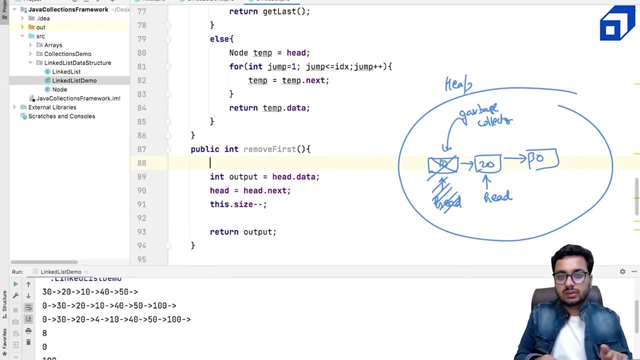 something we need to do right, but what is a special case is a special case? is a special case if the linked list is empty? can you? if the linked list is empty, can you? if the linked list is empty? can you remove the first element? the answer is no. 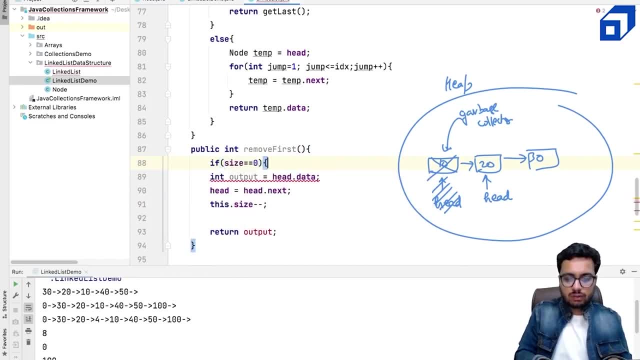 remove the first element. the answer is no. remove the first element. the answer is no. so we have to check if the size is zero. so we have to check if the size is zero. so we have to check if the size is zero, what we will do: we'll throw an exception. 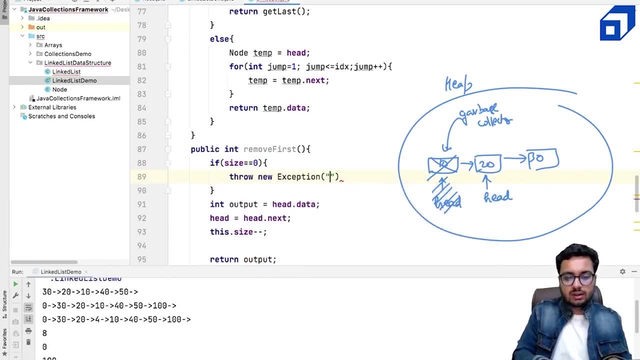 what we will do, we'll throw an exception. what we will do, we'll throw an exception. we'll say throw. we'll say throw. we'll say throw new exception, new exception, new exception. that linked list is that linked list is that linked list is empty right, empty right. 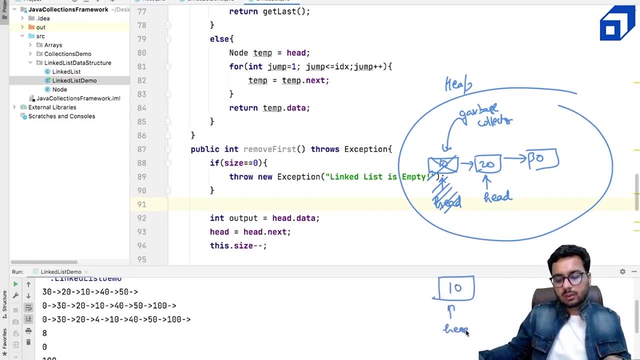 one node and both head and tail they were pointing to this node. will it form a special case? of course, yes, right, if this node is getting removed, what will happen to head and tail? they will be reset to null, right? if your original size was one, how do you remove it? you will set your head. 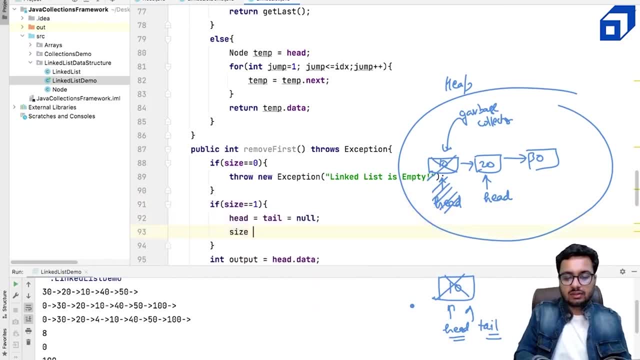 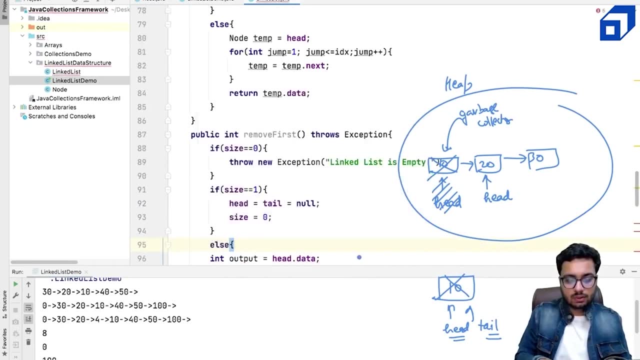 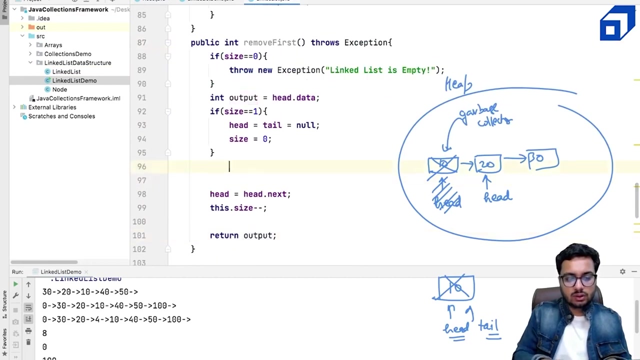 and tail equal to null. size will become zero. right, okay, and else sorry. yeah. so one thing we can do is this code we can move here: output is equal to head dot data. okay, and we'll of course return output. this code we can move in else case: right, that means if there are like: 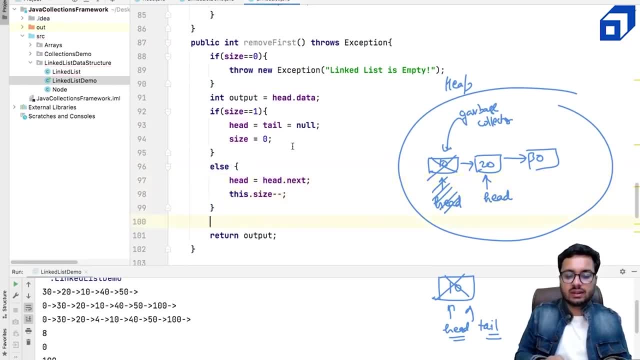 at least two nodes. in that case, tail will not be affected, right? so what about this case? else case: if there is 10, there is 20 and there is 30. so this is my head, this is my tail. even if my move, remove this node, head comes here. right, the head goes to the next place, size gets reduced, tail is not affected. 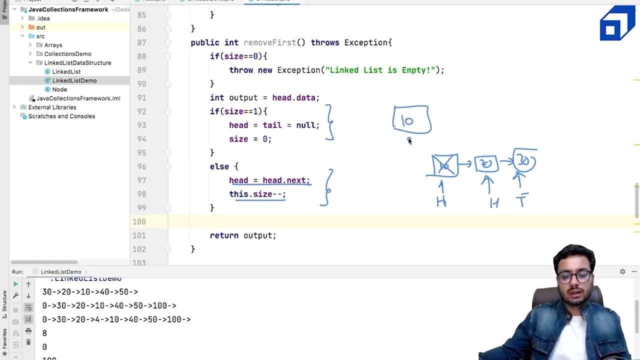 right. but if i have just one node and i remove that node, in that case head and tail, both way stuff in our case we can remove tail from this node. we can remove tail from this node. tail from this node. we can remove tail from this node. we can remove tail from this node. 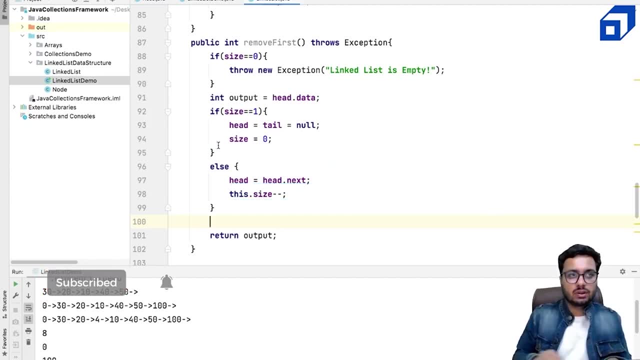 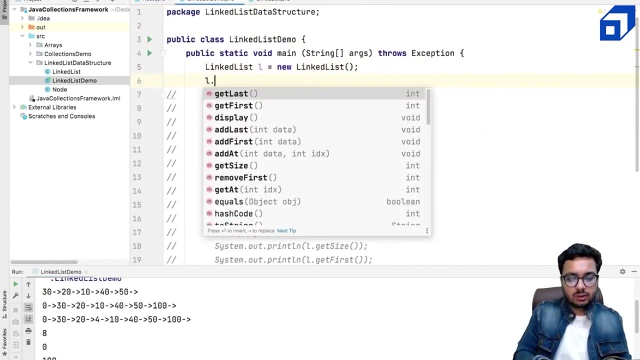 be affected. so they are reset to null and the size becomes zero. so that is how the remove first method should work. now let us test this method. let me create a new link list. let's say i add at the first position, let's say 10, then i add 20, 30, 40.. 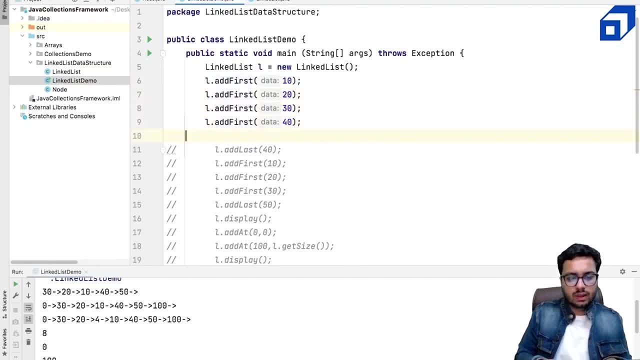 20, 30, 40. and i can say l dot display. then i can say l dot remove first and l dot display, right, so i'm getting 40, 30, 20, 10, fine, and if i remove the first element, 40, my linkless is 30, 20, 10, which is fine. 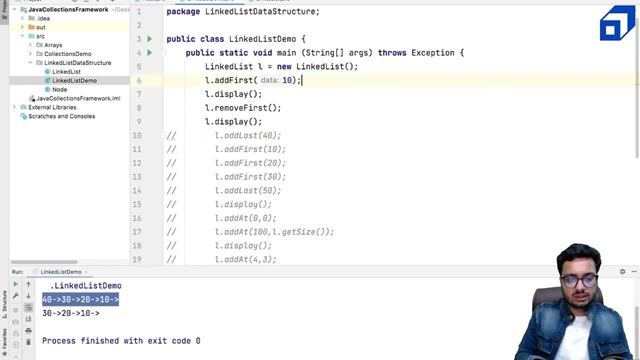 okay, if i have just one element in the linked list and let me see if it works well. so i have one element. i removed that one element, so my linked list is empty. fine, that also works well. right, and i can say: s out l dot size. i want to see if my size is getting updated properly. yes, the size is zero and i don't see any. 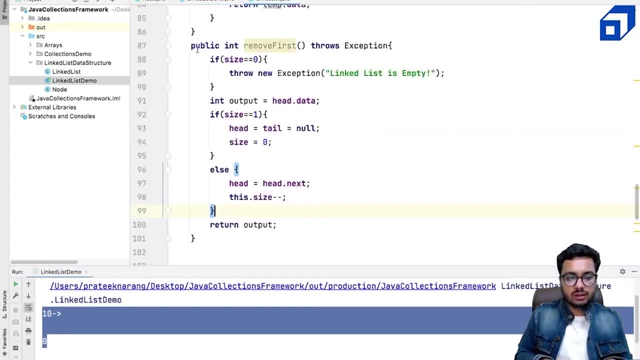 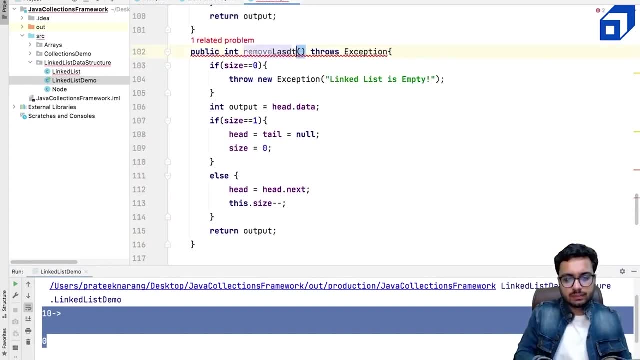 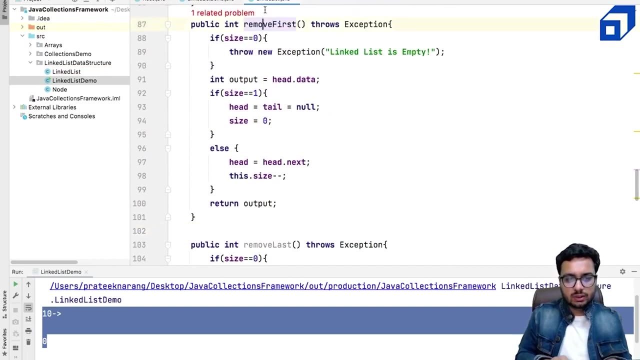 output here. that is how i will implement remove first method. now, on the similar lines, can you implement the remove last method? okay, just need to think what will change, what will happen to head and tail, how much time it will take. so this method. it's going to take order one time, right. 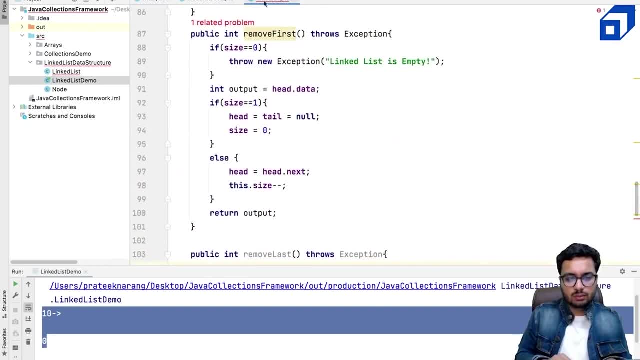 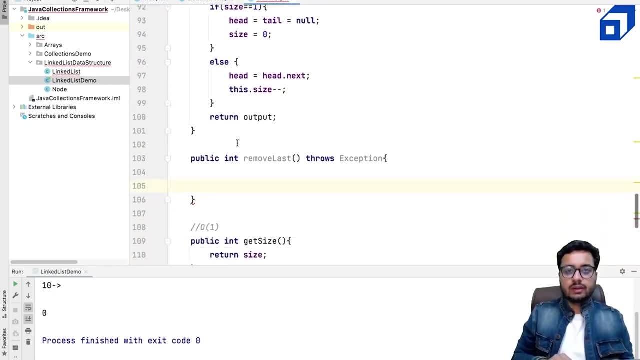 remove first, but you have to think how much time remove last will take, okay. so let's see. uh, remove last, okay. so first case is okay. if your linked list is empty, you cannot throw anything, you cannot remove anything. so if your size is 0, you will throw a new exception. okay then, similar to: 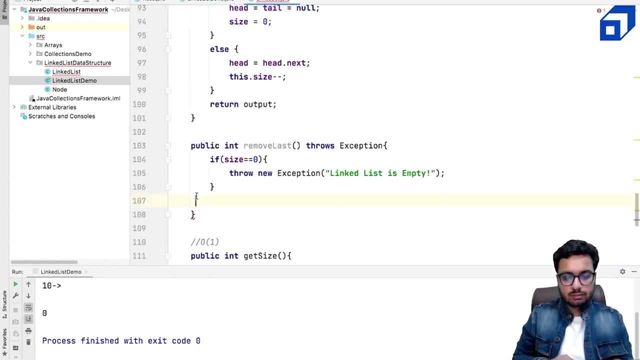 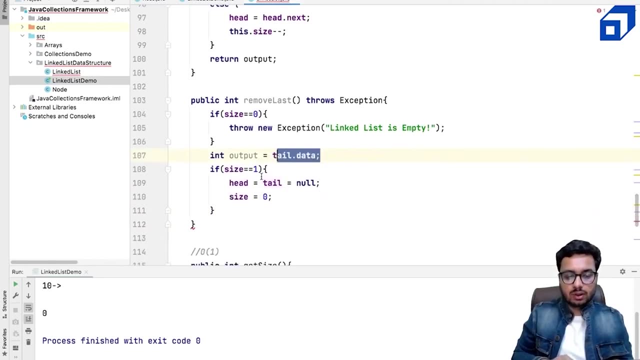 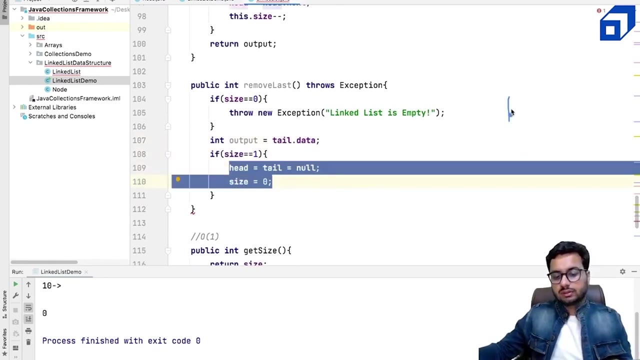 this one. your output in this case will be what your output will be now: tail dot data. you know, the last node is tail and that data is your output, right? so if your size is one, what you will do? you will reset your head and tail to null and you will. the size is zero. if this is only one node, both. 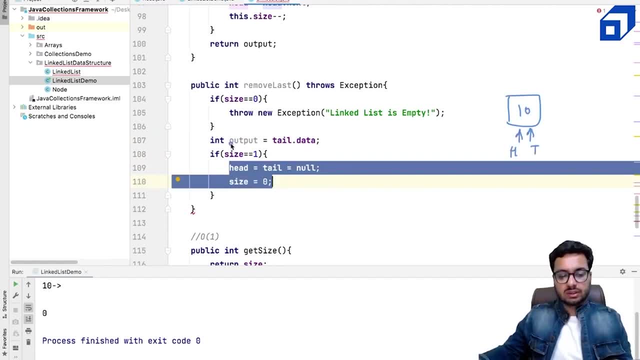 head and tail are referring to this node. you want to get this data. you store this data in a variable called output, that is tail dot data. original size was one. if this is removed, head and tail, they are reset to null and size becomes zero, which is correct, right? otherwise, if you really want to, 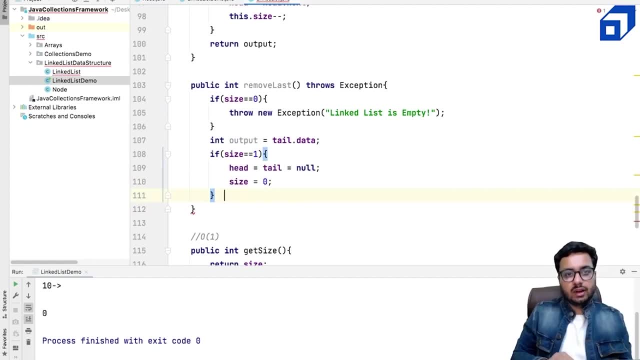 remove something right. so you will have to check that if your index is in the bounds, or is it zero, or is it the last index? sorry, you don't need to check here, because we are talking about remove last right, so you just need to remove the last node, right. so what i will do, i will say okay. 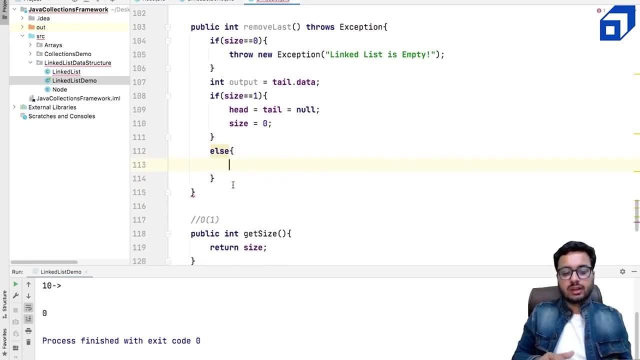 s. we have the other case. we know what node to remove if there are more nodes, right. there is one tricky thing here: that if it is a singly linked list, right, and this is your tail node, you are saying i want to remove this node, right, that means tail should be updated, tail should come here, the new. 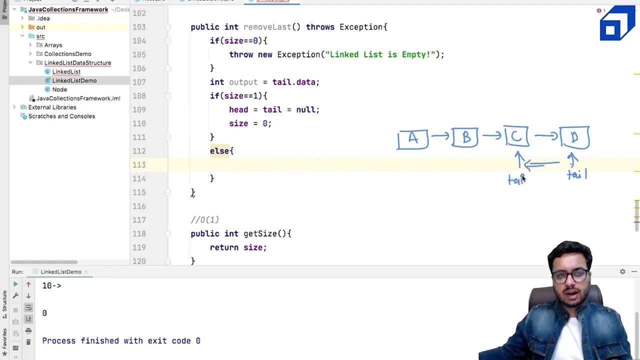 tail should come here right after removing this node. i have stored this d in in a variable called output, so output is tail dot data, so output is d. right, how do i bring it back? there is no way to do it, even if you maintain. okay, i will. 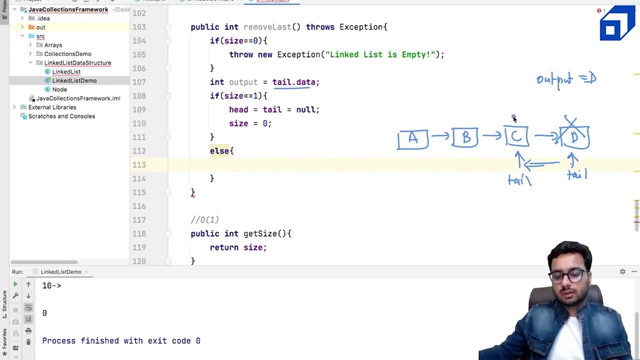 maintain previous of tail for every node. suppose this was the previous, but when you remove, see how you will get the previous. the answer is: we don't have an any order, one way of coming to the previous node. we have to iterate from the beginning to reach this node right so that i can update my tail variable right. so this is going to. 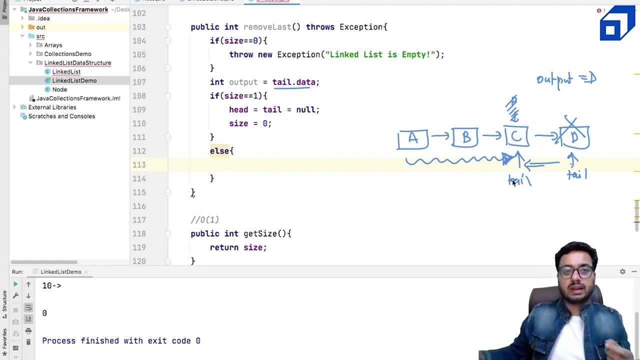 take time, right? or the other option is: you maintain a double prenup or should we write round one, because we have a function called si*node. but this will not take time if you write round one or you do nothing list in which every node is also connected back, right? if you do that, your remove last will work. 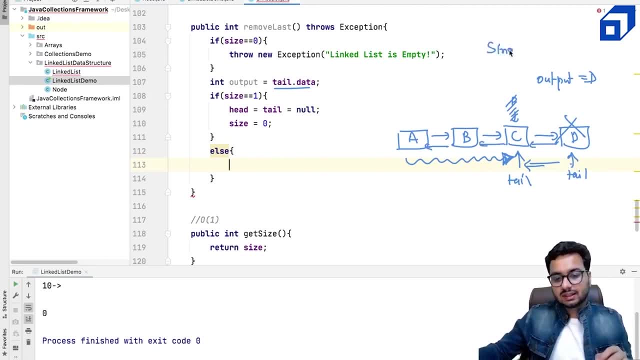 in order one time, but for now we have a singly linked list. that means we have only the next address, right singly linked list. in that case we have only one option: start from the head node and try to reach the second last node. so how do i do it? so i take a variable called temp, which 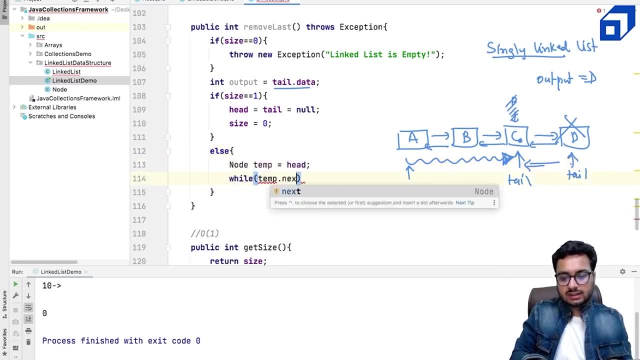 starts from head. i can say: while temp, dot next is not equal to tail, right, so what is the stopping condition? so when i reach this node, m, dot next. this is equal to tail, right. so this is the tail node, right? suppose? this is my c, this is my temp, and this is my tail node. this is my d, right, i'm? 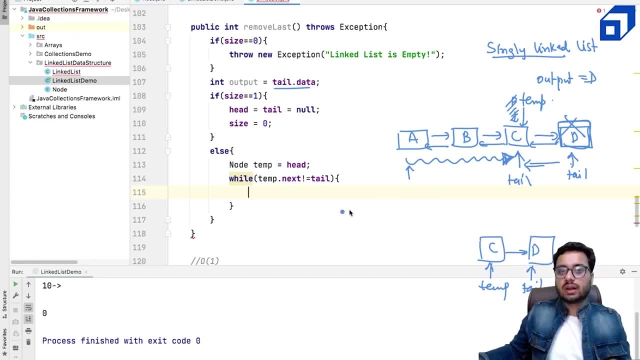 saying: while temp dot next is not equal to tail, right until this condition is not met i will take my temp to the next and next node. so temp starts from here, it goes here, it stops it. right, because c is next is equal to tail, so temp will stop at c. so i can say temp equals to temp dot. 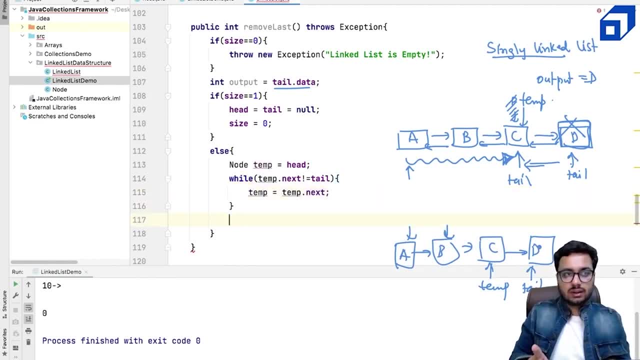 my temp stops at the second last node right now. why this is important? because i want to update the tail thing right now. at this point i want to disconnect d, this d i don't want. what should i do? i would say temp dot next is equal to null. so if i reset this variable to null, what will happen? this object. 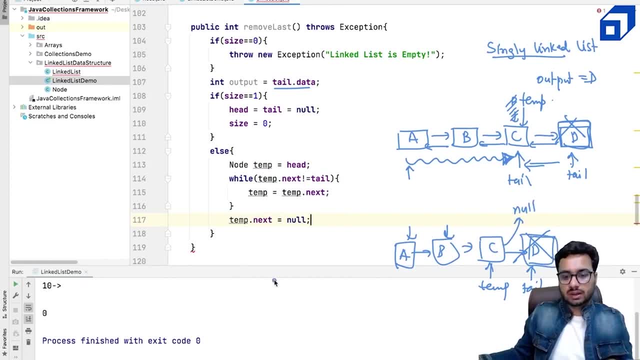 becomes eligible for garbage collection because no one is referring to this object, right? so garbage collector will come and sweep away the memory of d because there are no object references which are holding the address of this node. so this d will get deleted from the memory. and c is next is updated. correctly, right, but what about the data that we wanted to return, that is, 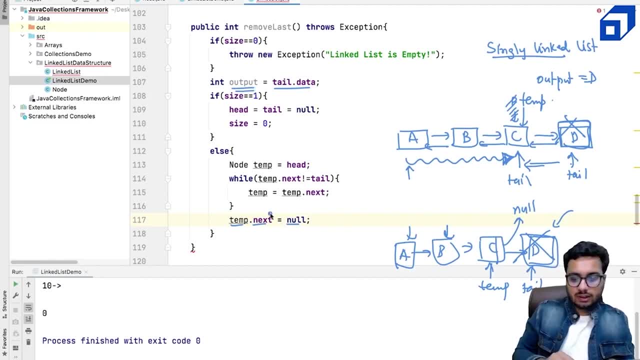 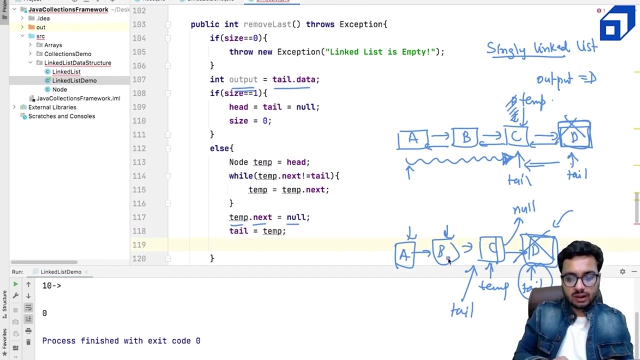 still copied in a variable called as output. right, so once this is done, what should i do? so temps next is now null. this tail should be updated, so this tail should come here. this tail will become equal to temp and the size will also get reduced. right, so here. 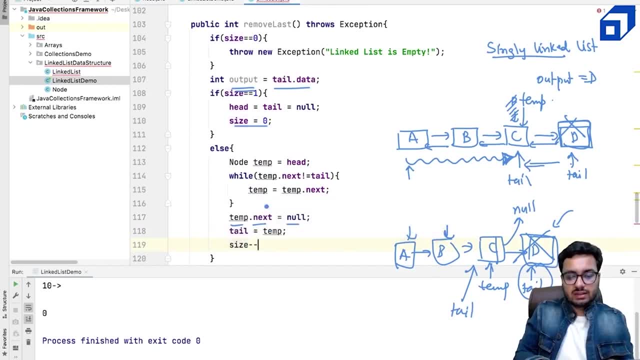 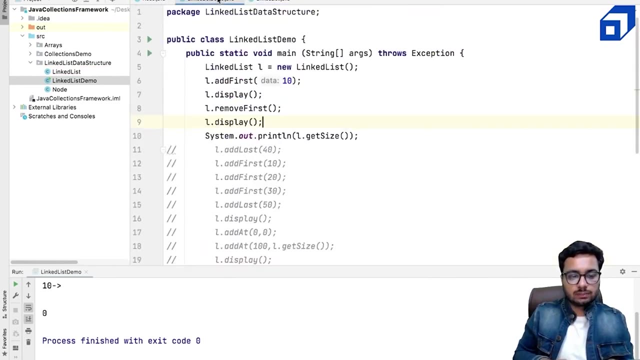 we have reset the size, so here it will be one less size, minus, minus. that's it, and i will return the output in both the scenarios. right? so return output in this case also. i'll return the output in this case will. i will also return the output. that is how remove last will work. and if i now show you l dot, remove last. 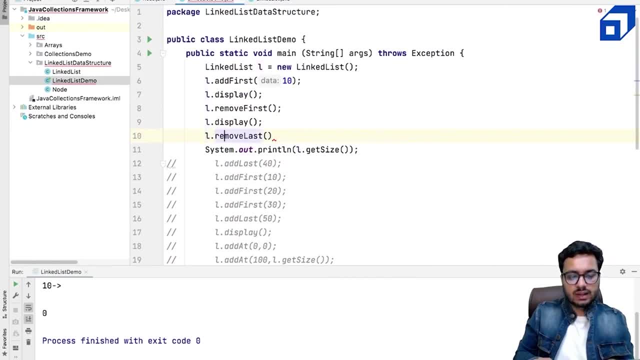 and uh, maybe if you want to output, that's okay. we just want to see the link list so i can say: l dot display. what do i get? okay, let me add some numbers only then we can see 20, 30, 40.. so right now i'm getting an exception because you know it's an empty link list. so 10. 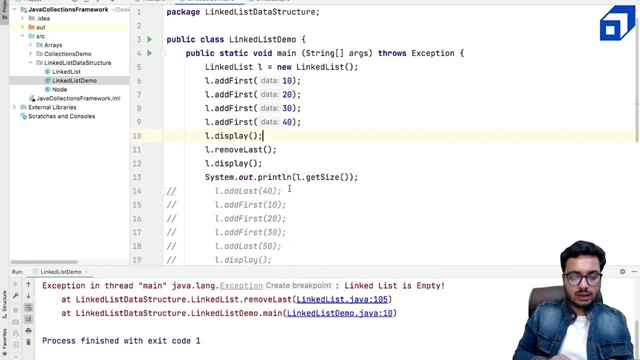 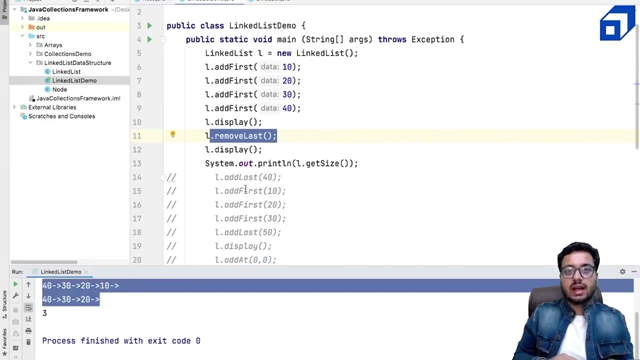 20, 30, 40 l dot display and then i called the remove last method. so this was the link list. i removed the last element. this is what i am getting and the size is 3 right, which is fine. that means the remove last is working as expected right now. the next thing we would like to do is any guesses. 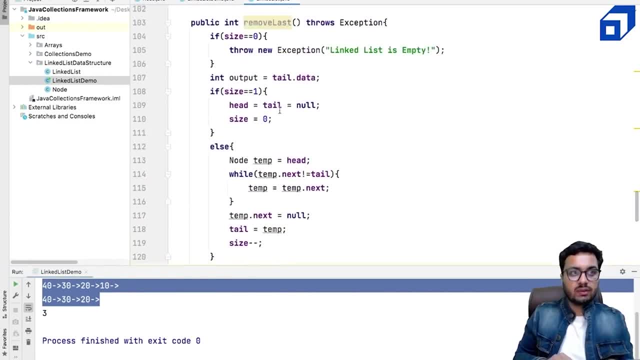 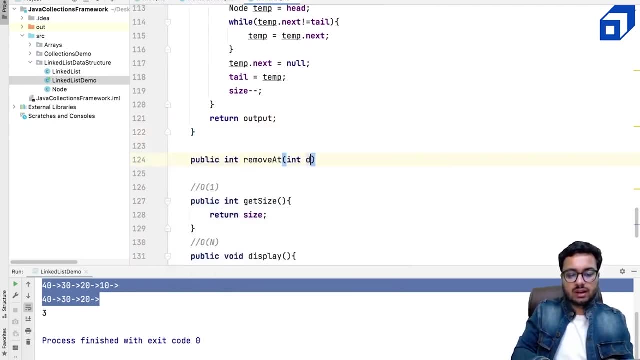 of course it's going to be remove at a particular index. so we want to write one more method: public int- remove art given index. so again, before i write the code, take a pause and think how you will implement this method. given a particular index, i want to remove something from that index. 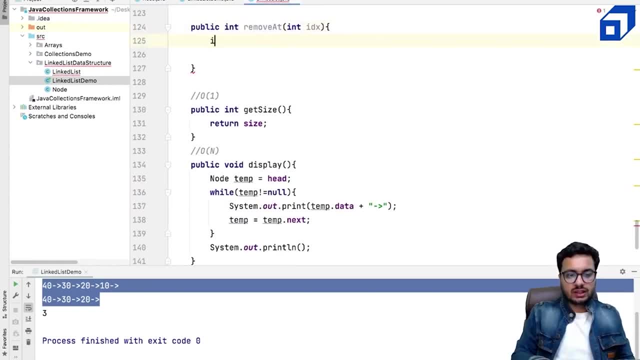 let us start it. take the index less than 0 and you can remove this by saying so. if the index is zero, let's say so. you are implementing a remove at right. so first thing is, if the size is 0, that means you cannot remove anything, so you will throw a new exception. 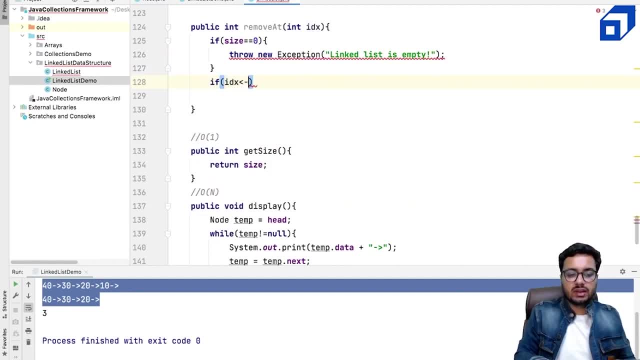 so throw exception. throw a new exception, annuals. okay, link list is empty. you cannot remove it. or you can check that if the index that you're getting is out of bounds. so if index is less than 0, even at size, we don't have anything. the last index is a size minus one. so if 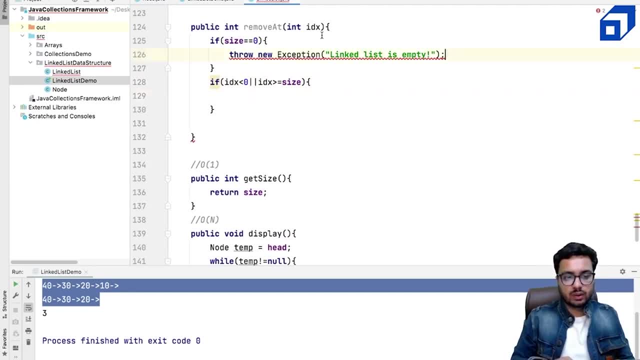 this is the case, I have to throw new exception. right, I'll throw a new exception and we'll tell that this method and throw an exception. all right, so the error is fixed. now what to do? I still want to remove it. so if my index is zero, that means I want to remove something from the head that we have. 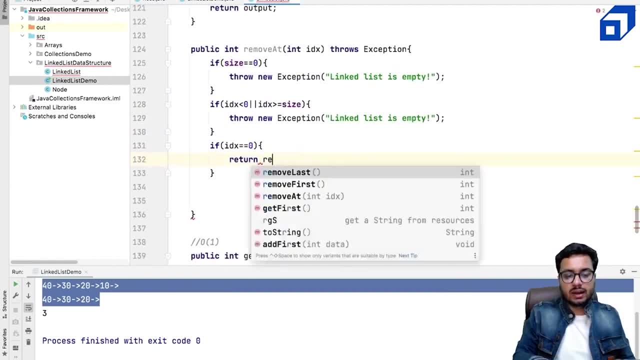 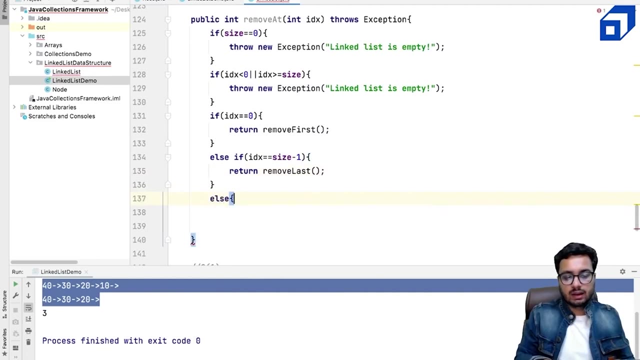 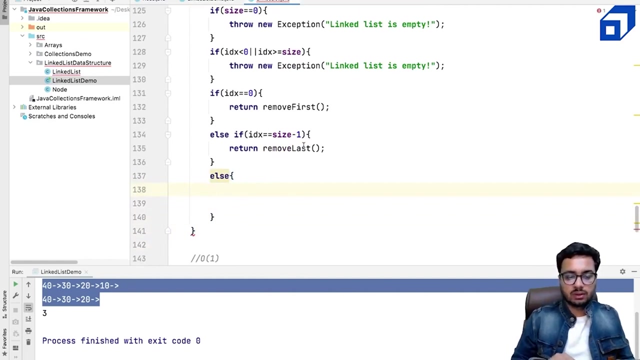 already implemented. so whatever is returned by the remove first, we will return that as if index is equal to the last, which is size minus one. we will return whatever is removed by removeLast method. and now is the time we will see the actual working of this method. right, how do I remove something from the middle? 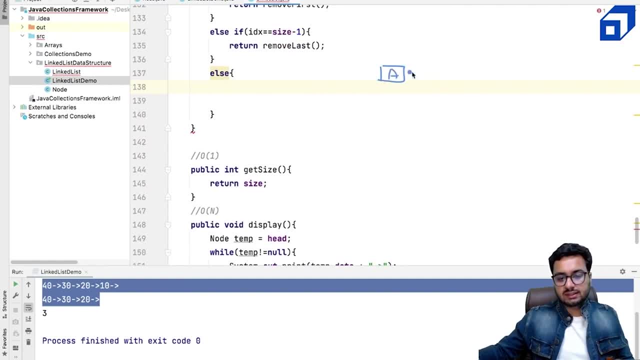 of the linked list. let's say, I have a linked list like this: a, b, c, b, c, d, e, f, right, and it's okay. i want to remove something from index 2 right: 0, 1, 2. i want to remove this element. if i want to remove this element, that means we should get connected with. 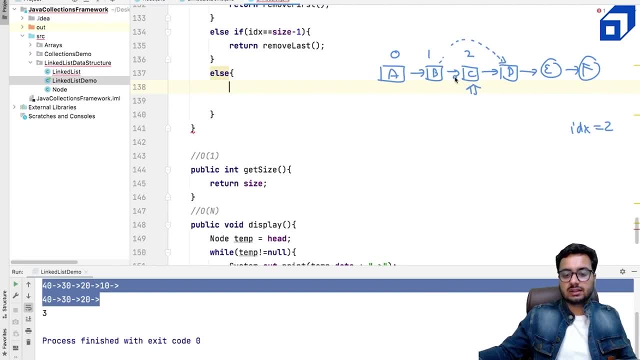 c right and this link from b to c. it should get broken and c should be garbage collected right. if this happens, c will be deleted from the memory, right. so how we are going to achieve this right? so first of all, we need to reach this node that is b right. so if my index is 2, i need to reach 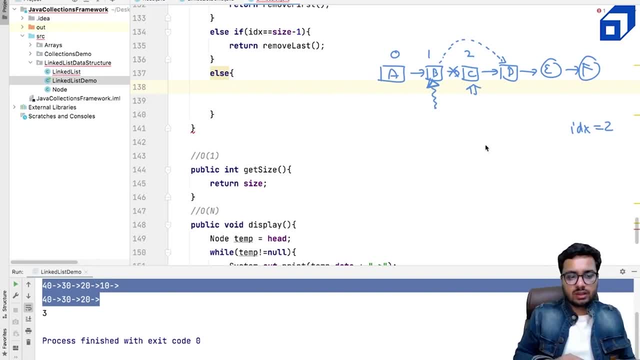 one node behind that index. so how do we reach that node again? fairly easy, i can say i will start with temp. that is equal to head, and if index is 2 that means i need to iterate 1 less than that index for int jump equal to 1, jump less than index. 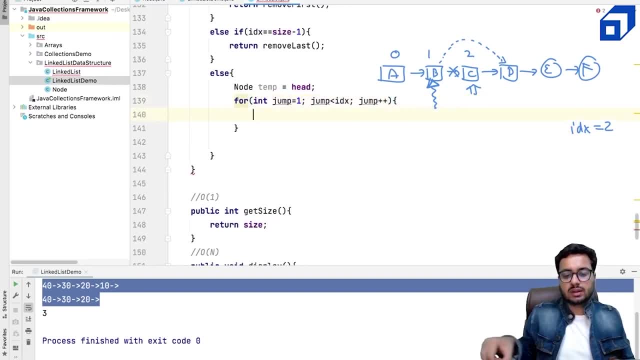 jump plus plus. so if it is 2, it's okay, i'll just take less than 2 jumps, that is, i'll take one jump. i will come here and at this node i will start doing certain operations, right? so first of all let me take temp to that particular node. now i am standing at this node. 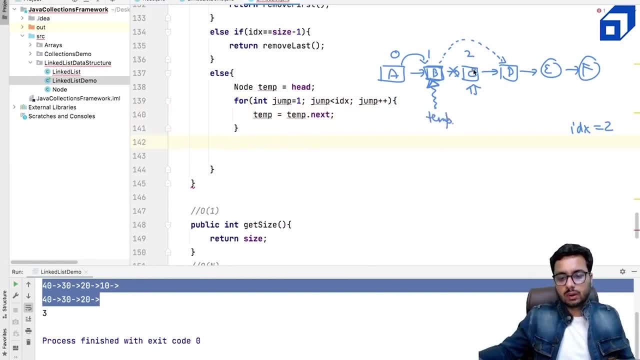 so what i want to do? i want to return this node right. i want to return the data of this node. i will copy it in a variable called output. output is nothing but um, temp, dot, next dot data. that is what my output is right, and i want to return that output. 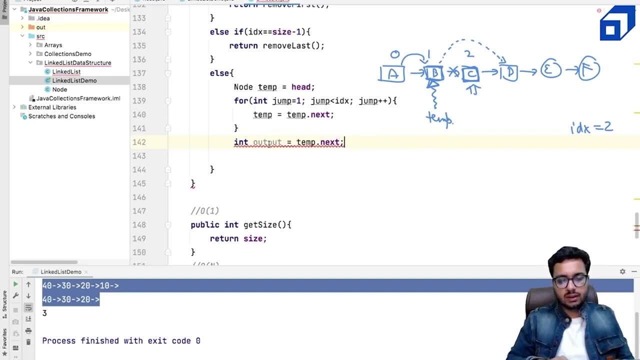 or let's say: this is my node, which is okay, either way we can do it. node called output. so this node is my output node and what i want. i want temp to connect with next of this node. so i want b to connect with t. so how we can do it. so temp dot next. 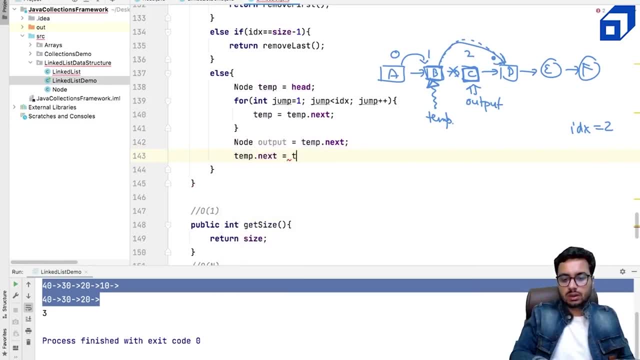 either you write it should be equal to temp dot next, which is my output dot next, so that is my d, or you can say output dot next. so again i'm connecting b with d. right now no one is pointing to t. it will become it will get garbage collected, right, okay? and if this node is garbage collected? 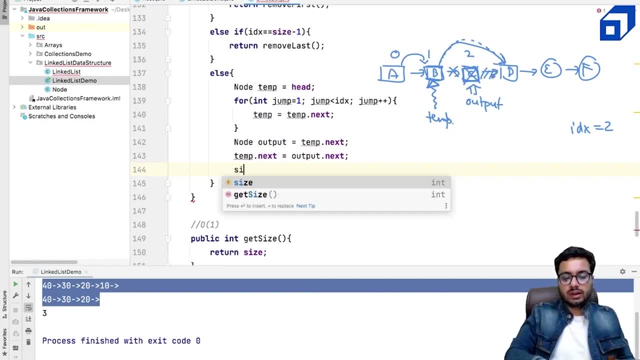 this link is automatically broken. so what i need to do, i need to say, is minus, minus, and i need to return output dot data. output dot data. this output is a local variable right. it is there only in this function. once i return output dot data, there is, uh, this: 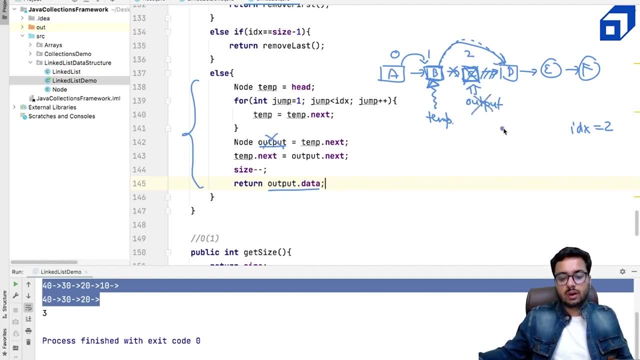 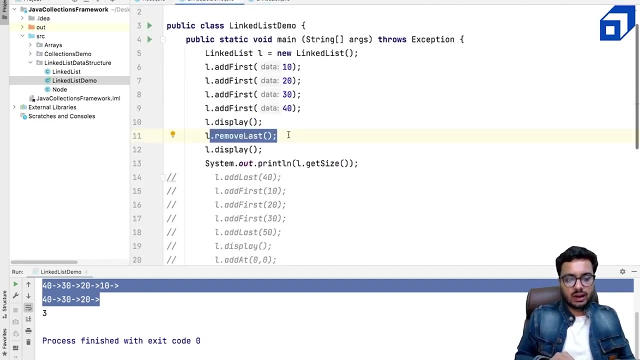 function call is over, output will will be out of scope, it will get destroyed and hence no one is referring to c. this memory will also be cleared off. that's it. that's what you need to do, right? so that is going to remove something from the middle of the linked list. right now i can test my code so i can say l dot remove. 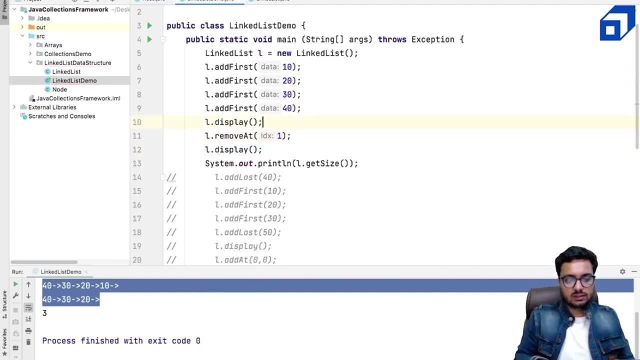 at index, let's say one, given this linked list. let's say remove. at index two, which is okay. show me what will happen if you remove something from index two. so this is my linked list and if it's okay, remove index two. zero one, two twenty is gone. i get forty, thirty and ten. that. 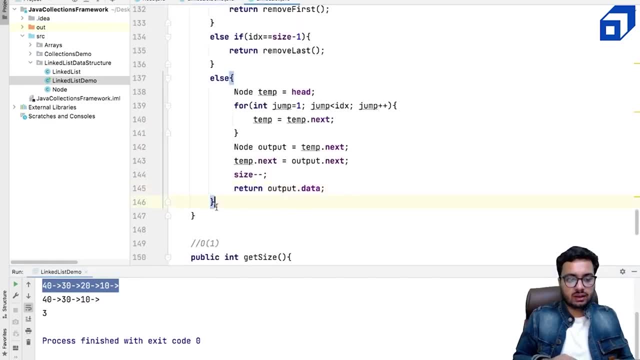 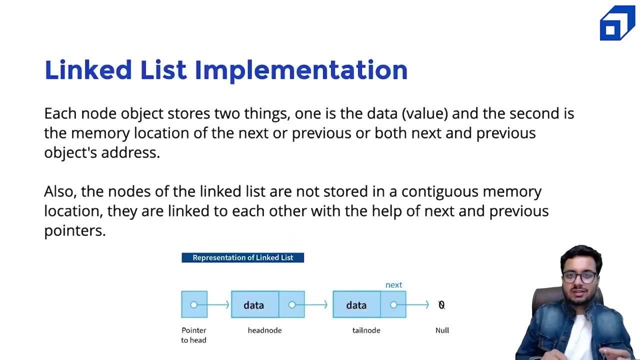 means the code is working absolutely fine. this is how we can remove something from the middle of linked list. so far, we have seen the implementation of single linked list, right so, in which we said: every node is going to store the address of the next node, right. but what happens in real scenarios you might need? 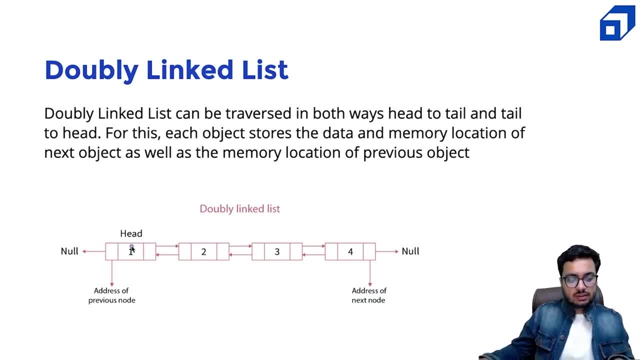 sometimes a doubly linked list. so what is a doubly linked list? just like you were storing the next, you will also store the address of the previous node. that means each node is now holding three things: data data, the next reference and a previous reference. so two will hold the address of three. two will also. 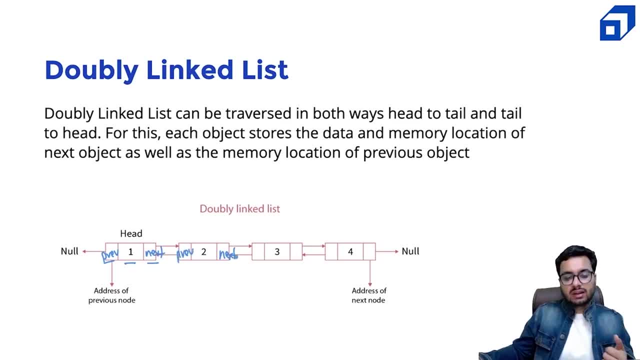 hold the address of one right now. the advantage of doubly linked list is that you can reverse in both directions, right? for example, we were doing removal at tail in which i said: okay, i want to remove this node and i want this tail to come back, so i, if it is a singular linked list, i have to. 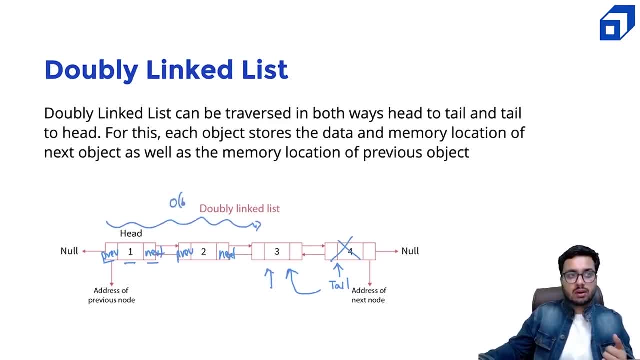 iterate from the front to reach this node, which is going to take order of end time, right, but if i do this in deletion at end for a w linked list, i can just come back to the previous node. okay, because four knows the address of three, so i can update my tail pointer very easily. right, so it comes at the 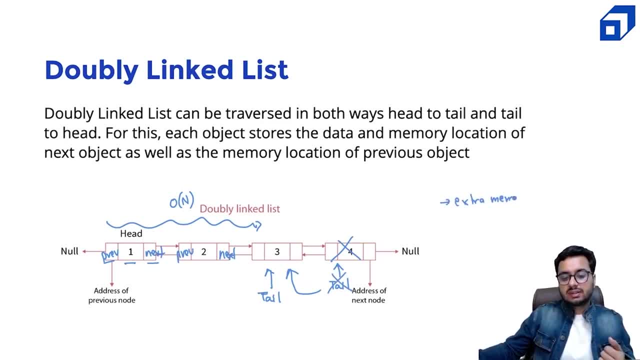 cost of extra memory, but it can save some time. for example, if you want to delete something at the end, it can then be done in order one time. insert at end can be done in order one time. insert at head can be done. it can be done in order one time. remove at head can also be done in order one time it should. 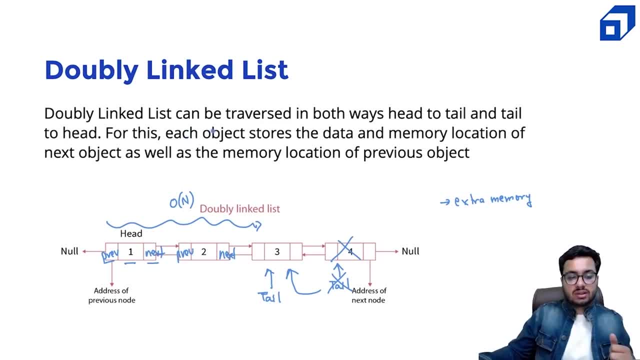 both ends. you can do insertion and deletion in order one time, right? so each object stores data and memory location of next as well as the previous object, right? so this is something you can implement right now. there won't be a lot of change. for example, if you're making a method to 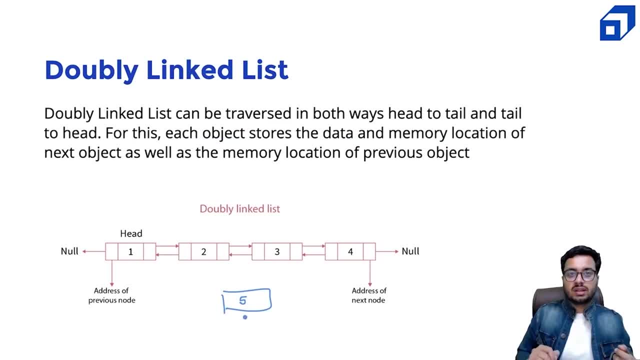 insert something in the middle. let's say, i want to insert five here. what are the variables that you will have to update? right? so? so you will have to update that two's next should point to five. okay, but if you do this first, what will happen? you will lose the address of three. 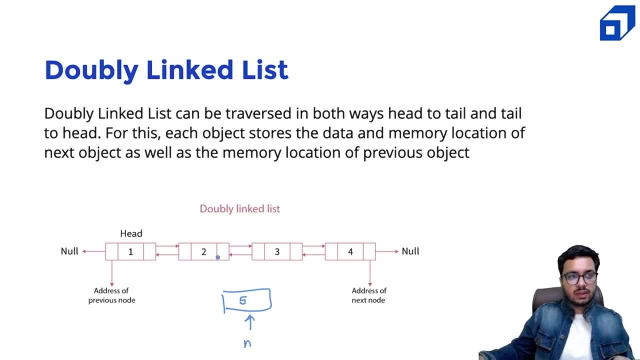 i will do, is it's okay? let me create this new node five, and let's say this is my temp here. i want to insert it. so five's next will point to two's next. five gets connected with three. right, i can also say: five's previous can point to them. so five also connects connected with two. right now i just need. 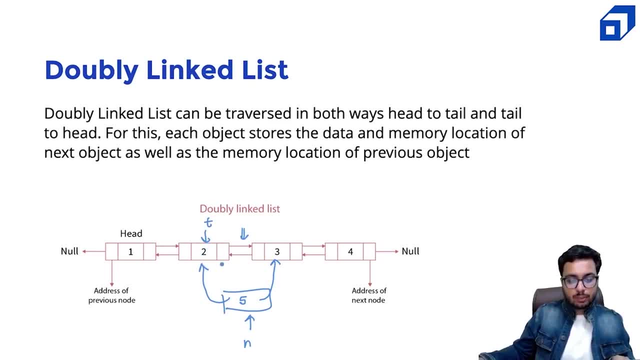 to change these variables. so i can say t is next will point to n, so two is two, points to three right. and i also need to say: is previous right or we can do it other way? right? we can first say that this node, which is the next, 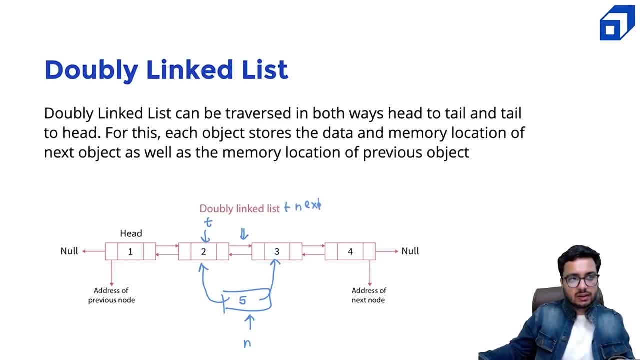 of two. so t dot next, dot previous. three is previous, should point to n. so this link will get like this: this link is gone. now what you can do, you can remove two's uh next and make it point to end so you can say this will get connected here. so you can say t dot next. this is equal to: 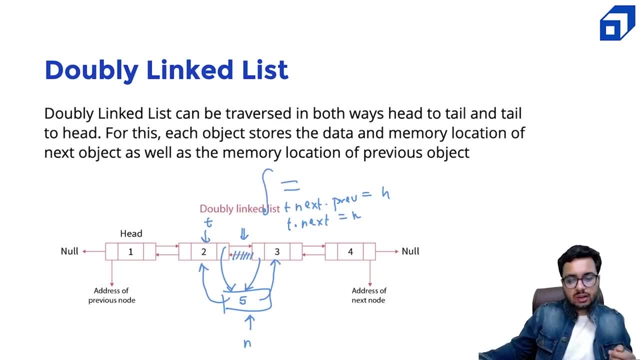 n right? so again, you just need to think logically and you need to execute these instructions in a particular order so that your updates are correct. you are not making any changes which are inconsistent, right? so again, all the operations get remove. uh, add, you can try creating those. 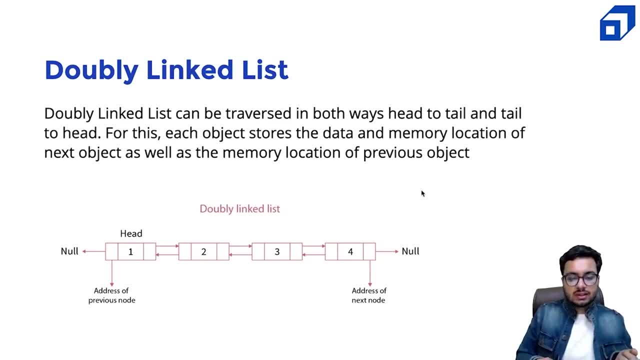 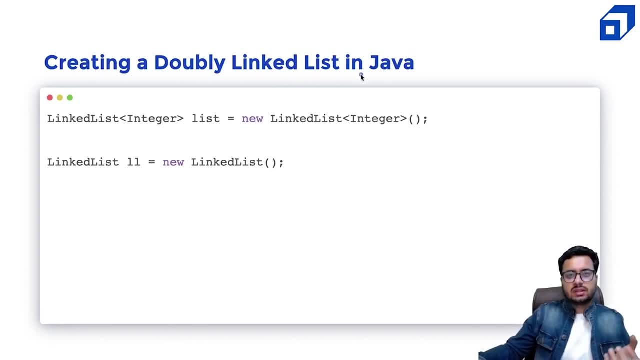 operations on a doubly linked list as an exercise, right? so let's talk about what happens in java, right? so if you want to use this class inside your collections framework, then this class is already implemented. so there is a class called as linked lists. so it's part of javautil package as a part of collections. 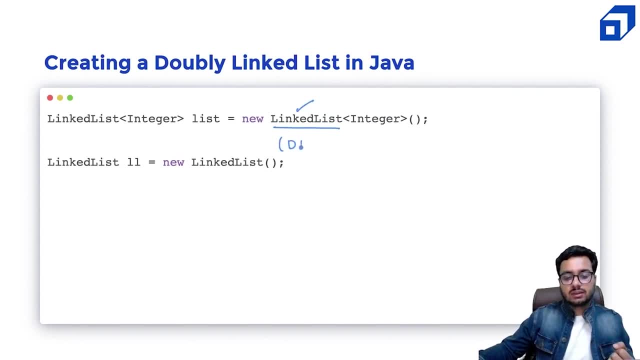 framework. by default, this class internally uses a doubly linked list, right? so if you're using this class directly in solving problems, you're getting a doubly linked list by default, right? so if you want to learn more about this, i have covered collections in my dsa tutorial. 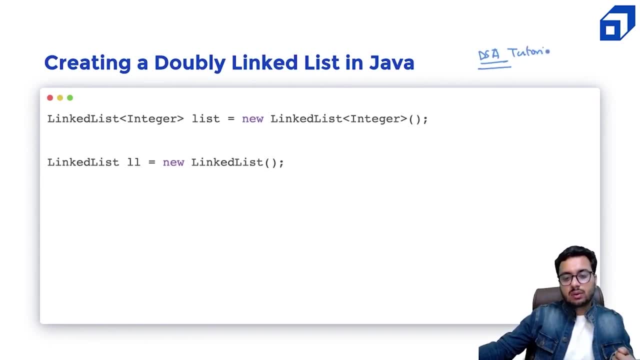 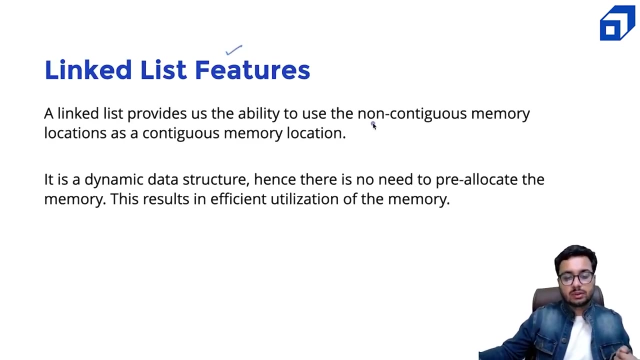 on the channel. you can watch that and learn how do we use the inbuilt doubly linked list or inbuilt linked list class. you can definitely learn about the methods of that as well. right, so let us quickly revisit the features of linked list. right, so it provides us an ability to use the non-continuous memory. 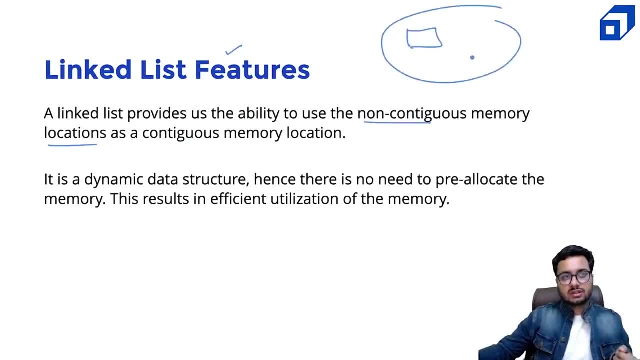 locations right. so if you have like different chunks of memory available in different parts of the heap and you cannot create a big array, but what you can do is you can use some memory here, some memory here, some memory here, just connect those chunks right. non-continuous memory parts can be utilized efficiently using a. 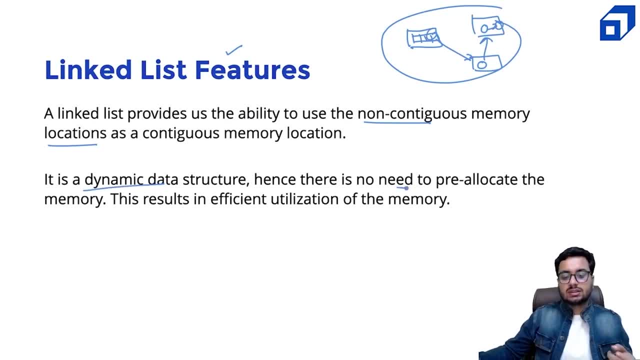 linked list. second advantage is it's a dynamic data structure. there is no need to allocate pre-memory and again this results in efficient utilization of memory. for example, if an array, you say, okay, i need thousand elements, but only suppose 100 get used up, then what is happening? 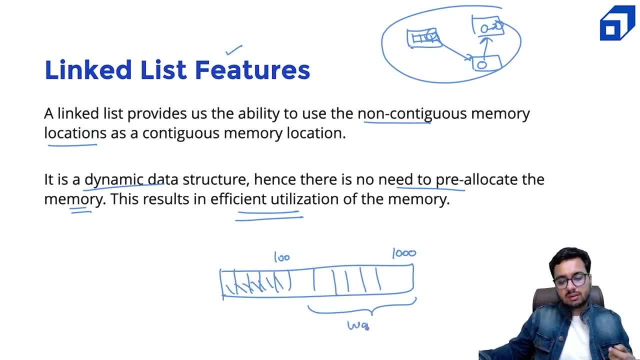 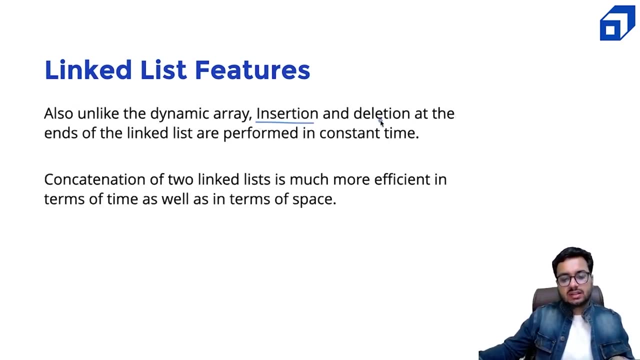 all this memory is: uh, it's a waste of memory, it's not efficient utilization of memory. so, linked list, you create memory on demand and hence you only use that much memory. that is required, right, okay. and if you are using a doubly linked list, insertion and deletion at the ends of 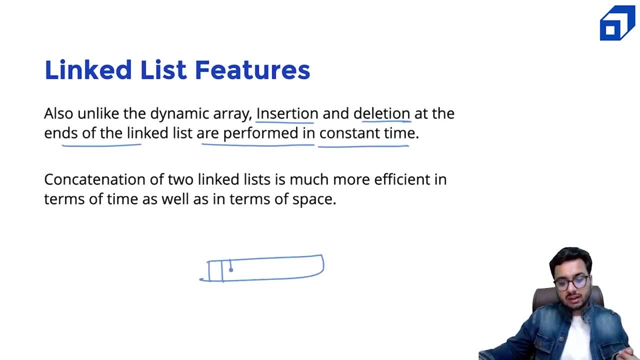 the linked list. they are performing constant time. so if you compare it with an array and if you have to do some insertion or deletion in the beginning, right, you will know that it's going to take order of end time because i have to do shifting, if i insert something or if i delete something. 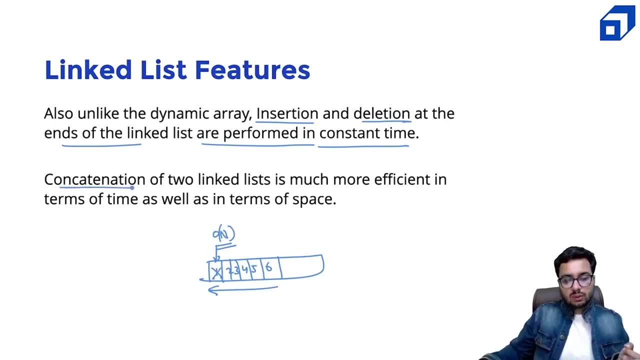 again, i have to shift all the elements right and joining two linked lists. it's much more efficient in terms of space and time. so, if there is one linked list and there is another linked list, right. so think, if you have to join two arrays, you have to copy all the elements from one. 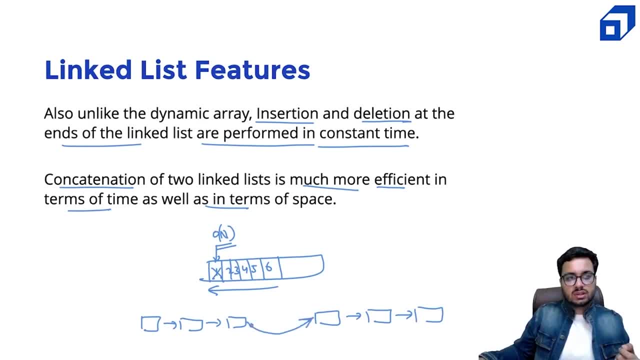 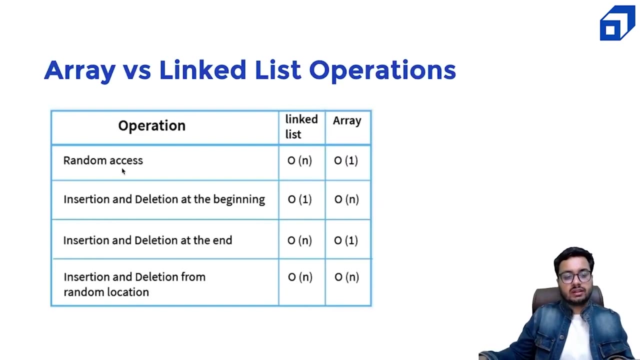 array into another array. but if you have to join two linked list, you just need to connect the tail of one with the head of other linked list and that is going to be an again an order, one operation. so it saves both your space and time. right, so that is all about linked list. so a quick. 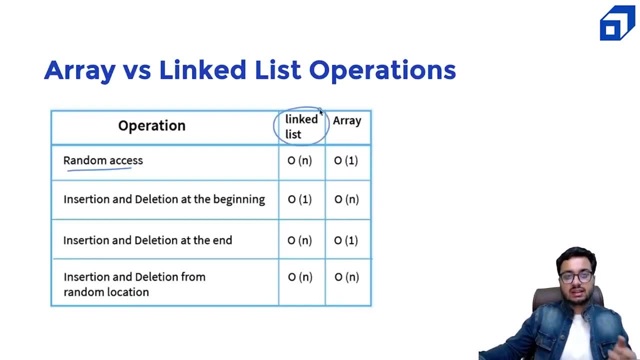 revision on the operations. random access. if it is a linked list it's a bad thing, right, because it's going to take order of end time in an array. getting the ith element will take order one time. insertion at deletion at the beginning: order one time in an array. it's going to take order and time. 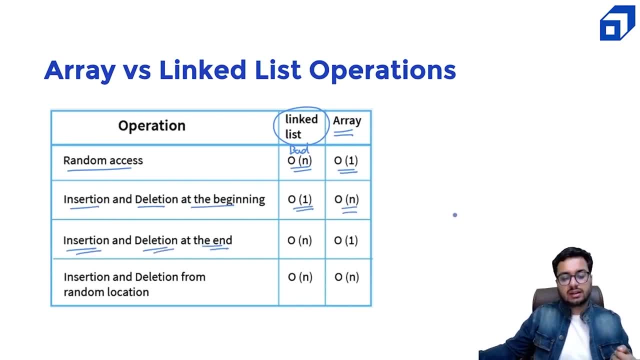 as i just discussed, insertion and deletion at the end, right. so this, if it is a double linked list, it can be done in order one time. right in an array also, it can be done in order one time: insertion and deletion from a random location. so if you are doing somewhere in the middle, both are going to take. 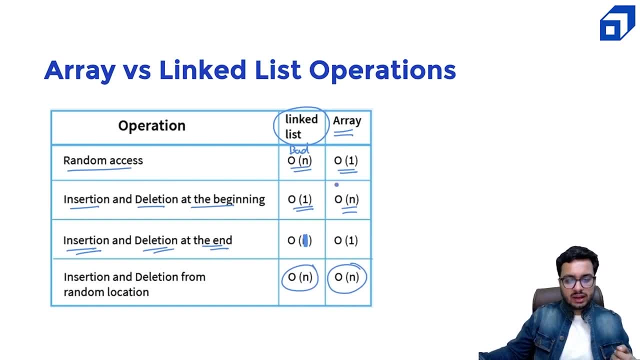 order end time: right. so in an array, this part is bad. insertion and deletion: at the beginning, random access is good. in a linked list, this insertion deletion part is good, but random access is bad. so you can see, each data structure has its own pros and cons, so depending on upon. 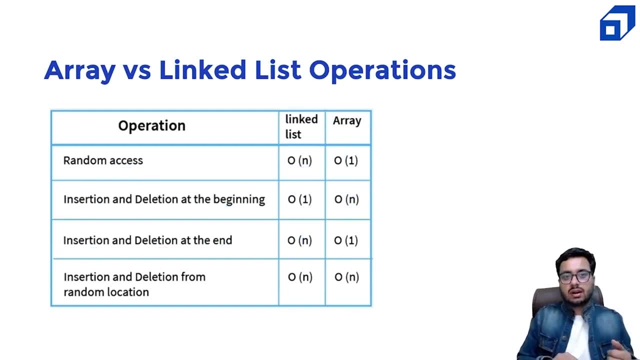 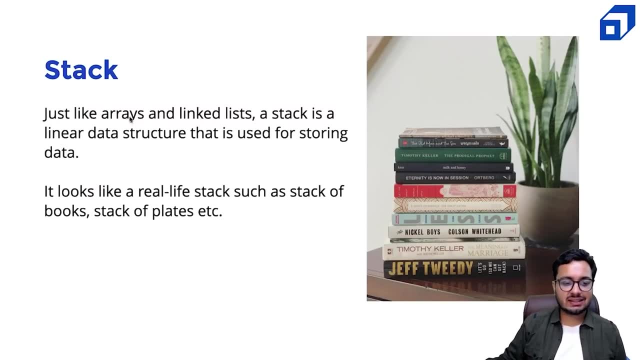 the problem. you have to decide whether you will go with a linked list or an array. let us talk about stacks today. so, just like arrays and linked list, stack is a linear data structure that is used for storing data. right, and it looks very much like a real life stack, such as. 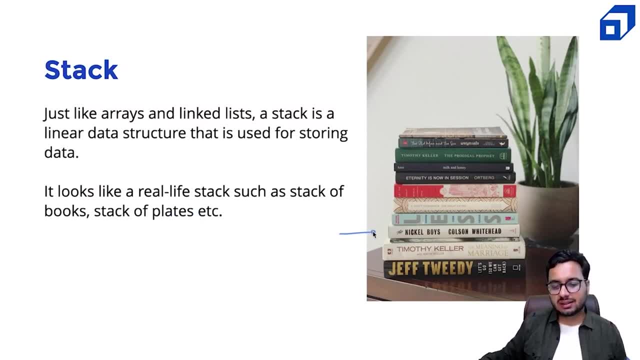 stack of books, stack of plates and so on. right, so you might have guessed the kind of behavior this stack will show. so what happens is you can insert something. if you want to put a book, that book must be inserted from the top right. you cannot insert books directly in the middle right you. 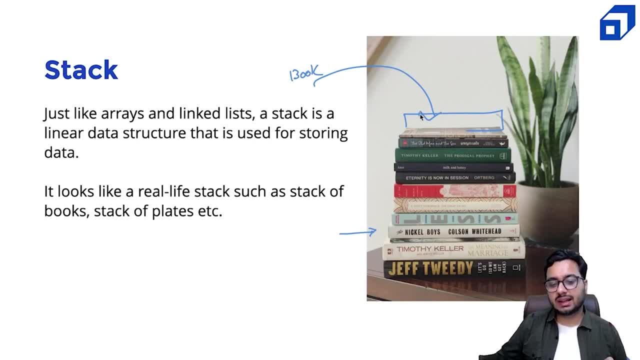 can insert books directly in the middle, right. you cannot insert books directly in the middle. you cannot insert a book at the bottom of the stack, right? basically, any book, let's say c++ book, it goes on the top, then a python book, it goes on the top of the stack, right. so this is how it's. 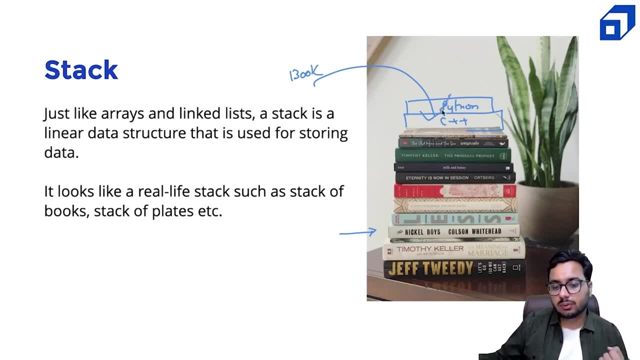 it's going to be. and if you want to remove some book, you will have to remove the topmost book first, then you can remove the next topmost book, then you can remove the next topmost book, right? basically, it's a data structure in which insertion and deletion they are done only at the one end. 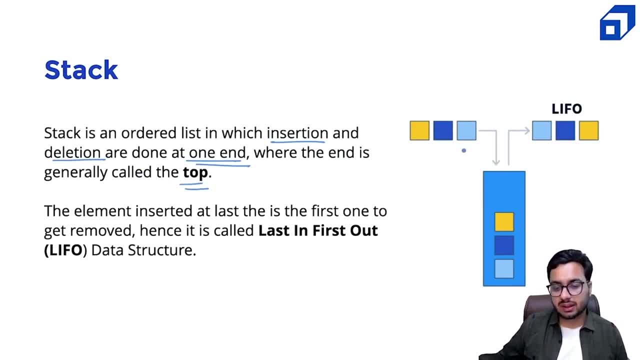 where end is called as the top of the stack, right. so you cannot insert a book at the bottom of the stack, right. so if you are pushing something, this blue goes, then this blue goes and then this yellow goes. okay, the item which is inserted at the last right last item, it is at the top of the stack. 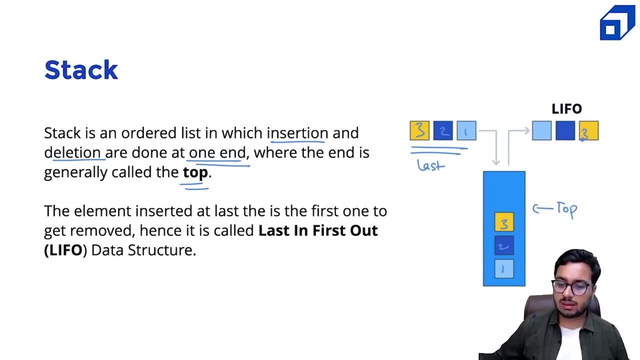 right now. if you want to remove something, this three will come out and this two will come out. then this one will come out. the last item is the first one to come out, so hence this behavior is also called as last in first up right. so when you do a 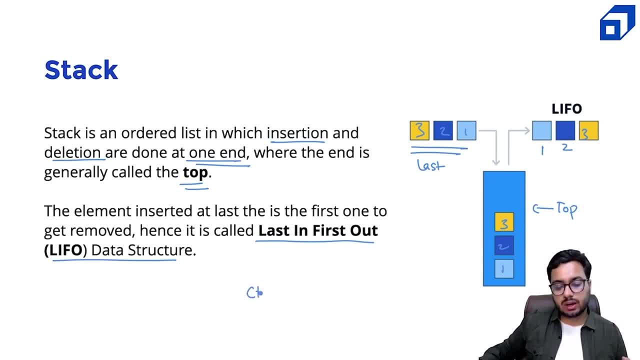 execute these operations on your computer: uh, undo, undo, redo, you do, right, so you, when you do ctrl z, so the last operation has been reversed. when you do again undo, the previous operation gets reversed, right. so stack is a useful data structure if you want to implement recursion, if you build 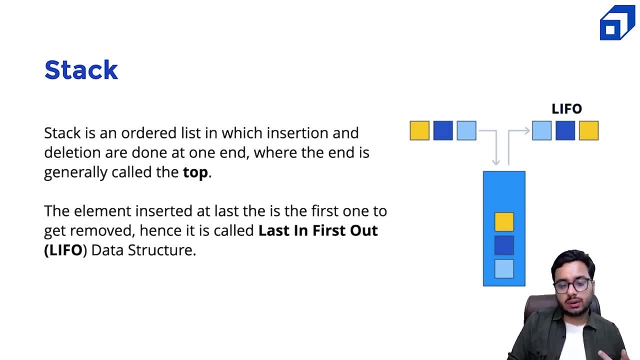 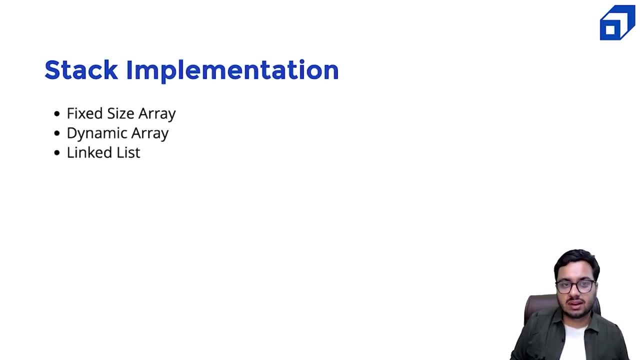 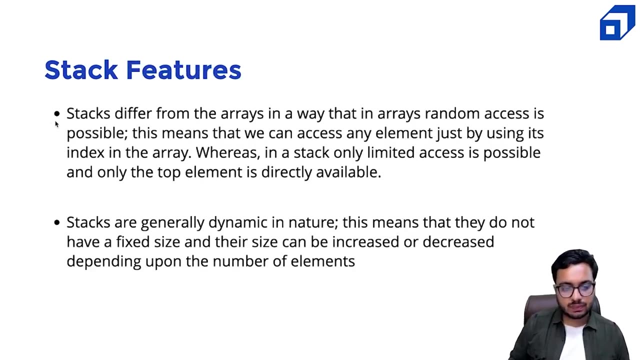 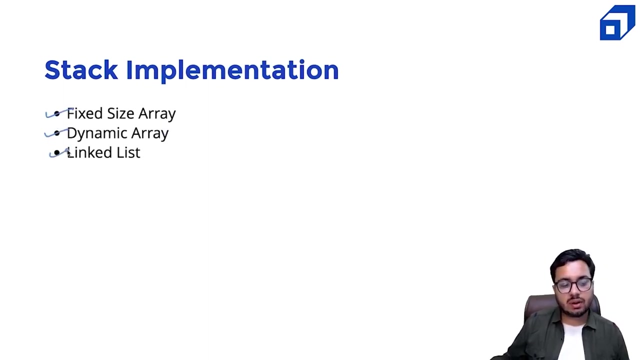 if you want to build something like an undo redo stack, you can do that right and problems where this last in, first out behavior is important, stack can be used here right. talking about implementations of stack, we will discuss uh three implementations. we will discuss uh one using fixed size array, we will see dynamic array right, or an array list, and we will also see 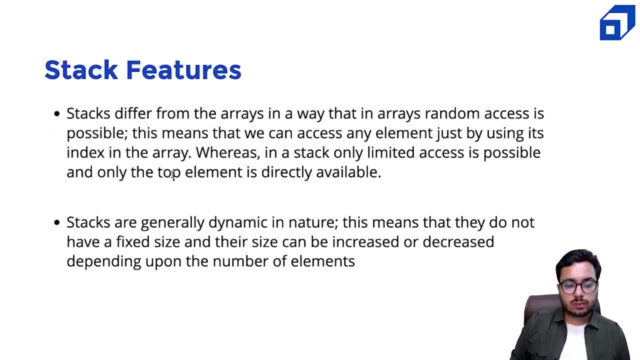 using a linkless right. so we'll go into the implementation details, uh, very soon. but before that let us also talk about features of the stack right. the stacks are different from arrays in a way that in arrays random access is possible. that means you can any ith element, but in this case, stack only limited excess is possible. that means only the. 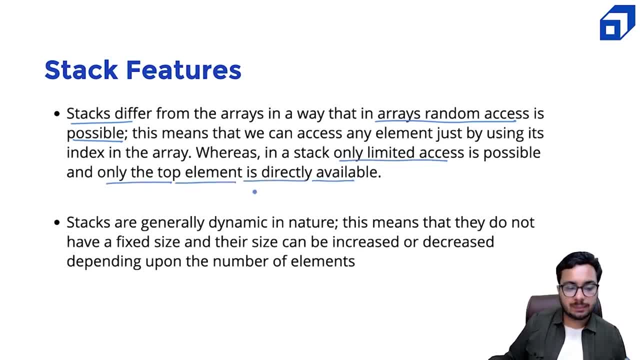 element which is at the top is directly available to us right, and stacks are generally dynamic in nature. in general we can have a fixed size stack as well, but generally we can push and pop elements so the size of the stack can keep on changing right. so generally we do not say it's going to. 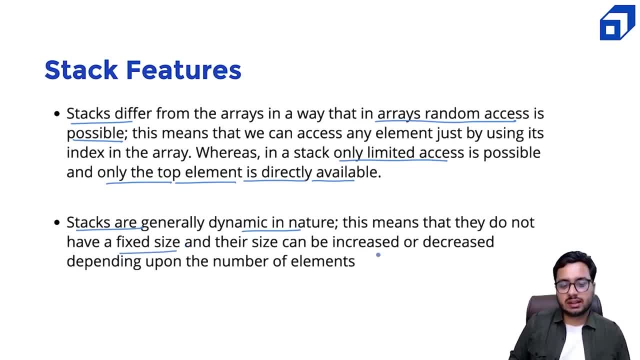 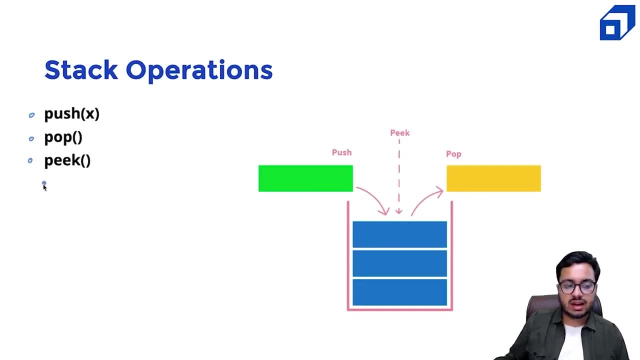 have any fixed size, right. if you use an array list or a linked list, you will be able to implement a dynamic stack, right. so three fundamental operations that we will have with every stack. it's okay, we want to push something. push something at the top of the stack you want to remove. 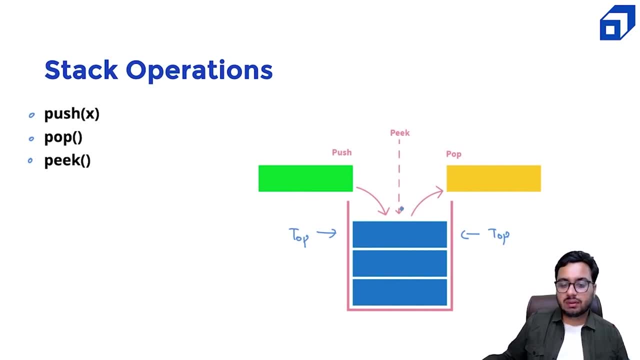 something again that happens at the top of the stack and we want to peak. that means we want to get the element at the top. we are looking for the element, so we call it as peak, sometimes also called as a top right. we want to seek the top most element. that is about stack. and now let us jump. 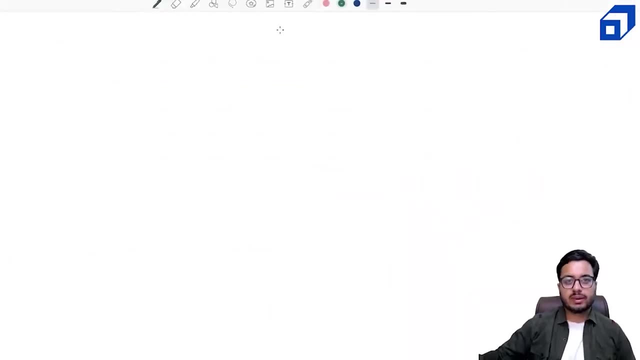 into the implementation of stack. let us talk about implementation of stack. so we will be discussing two implementations. one is stack that uses a fixed size array, and the second implementation would be a dynamic stack right which can use a array list or a linked list. okay, so we will discuss. 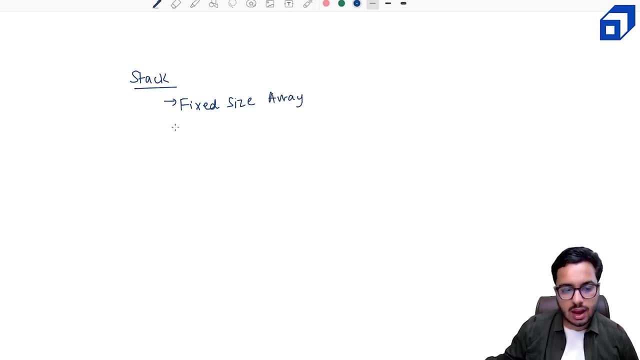 a fixed size array implementation and another implementation using dynamic array, which is called as array list, or we can also use linked list, right? so one of those data structures we can use to give the behavior of a stack, right if you are using a fixed size array, right? so you have to think of a container which is 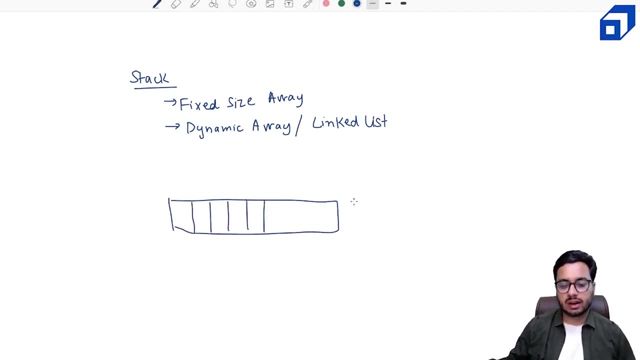 getting filled and getting empty only from one end, right? that means if i say okay, every insertion will go from here, right? so one, two, three, four, five. if i want to insert six, i will insert something from this end. if i want to remove something, i will also remove something from this end. and if i want to. 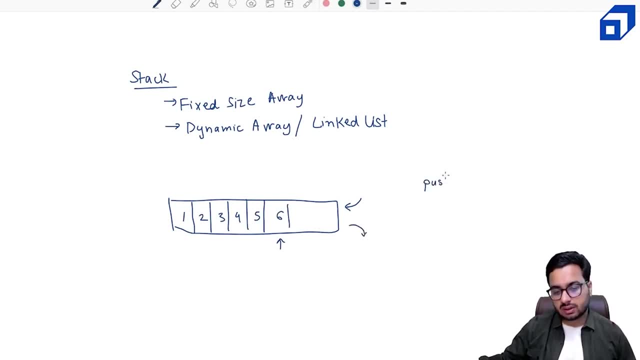 insert something from this end, right, so i can say, okay, i'll push something into the stack. so that means i'll push six and if i pop something, that pop will also remove six. right, and there is one more method that we would like to implement that? okay, i want to see what element is at the top of. 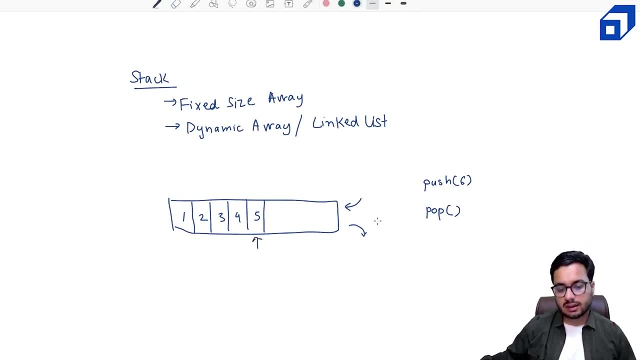 the stack. so if you remove six- and we call this method as peak, right? so if i want to see what element is at the top of the stack, that element would be your five right? these are the three most important operations that we need to implement on a stack right now. clearly, we can use a fixed size array to do it right. so, internally, 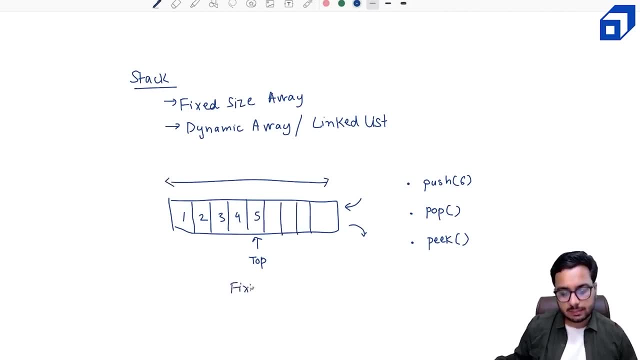 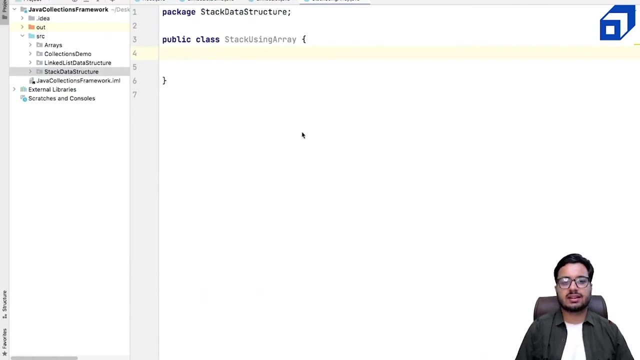 it's okay. there is an array which is having fixed size and we can add elements from this end into the array and we can also remove elements from this end of the array. so let us see how we can implement a stack class in our code. let us start implementing the stack using a fixed size. 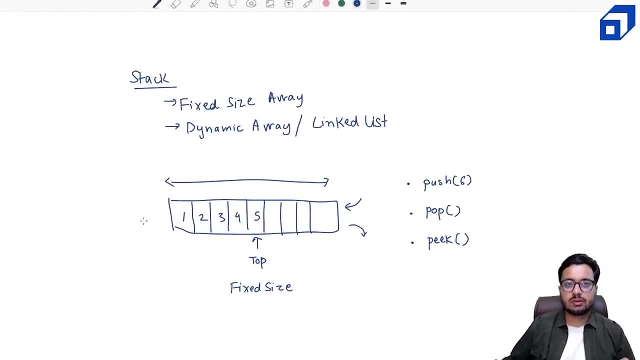 array right now. if you look at this fixed size array, what are the three things you will need in this class? one is the name of the array or the container in which you are going to hold data. another is the top variable that is going to move as you insert and delete elements, and another 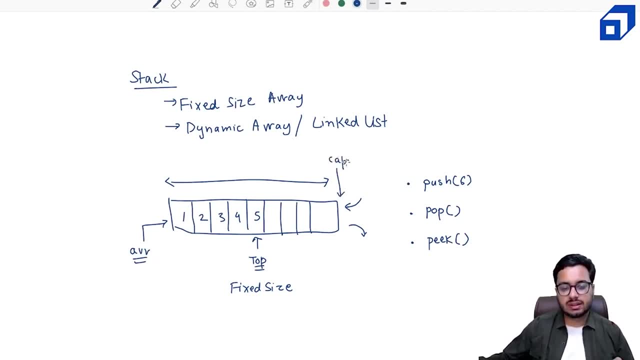 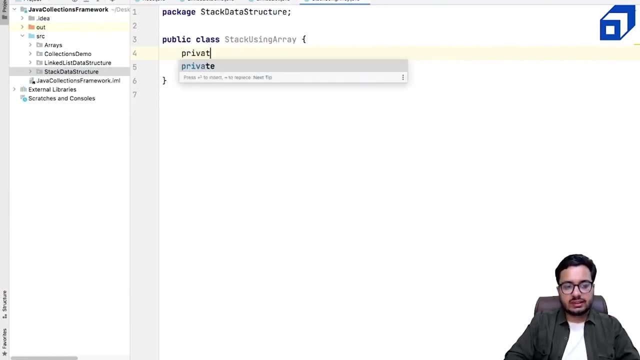 thing we need to know is: what is the maximum capacity of the stack? right, what i will do. i will define these three attributes as data members of the class. first thing i will have is a private array, which, which we call it as data thing i will have as top and another thing i will have as a constant default capacity can be treated. 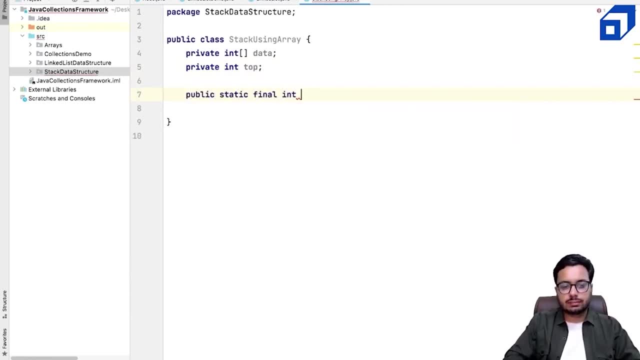 as a constant, so public, static final int. i can say default capacity: right, and this is equal to 10. right now i need to define a constructor so i can say, okay, stack using an array. there is a constructor and i'm not getting any default capacity, so that means my array size will be 10. 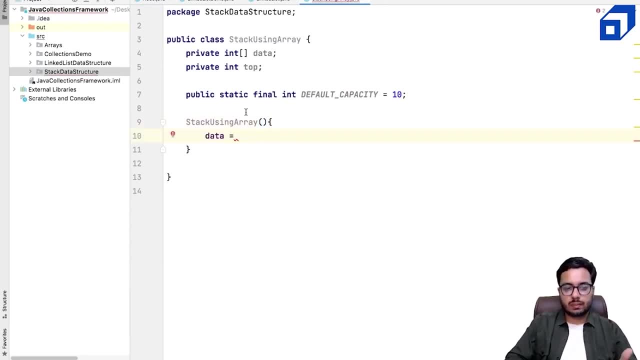 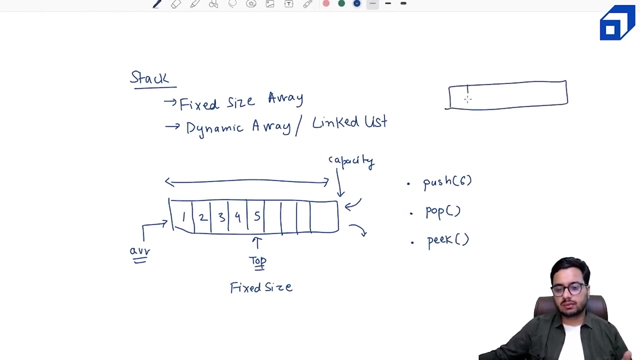 in this case. so i can initialize my data array, so i can say: this is equal to new int. how many integers the default capacity? right? and what is the initial position of the top? so top is the index at which i'm going to store the element, uh, at which i am stored the last element. so in the beginning i can say my top is at minus. 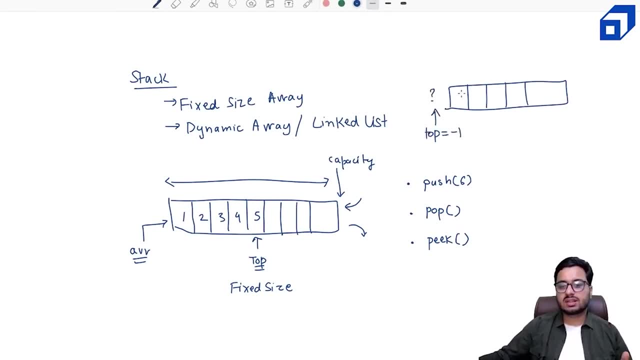 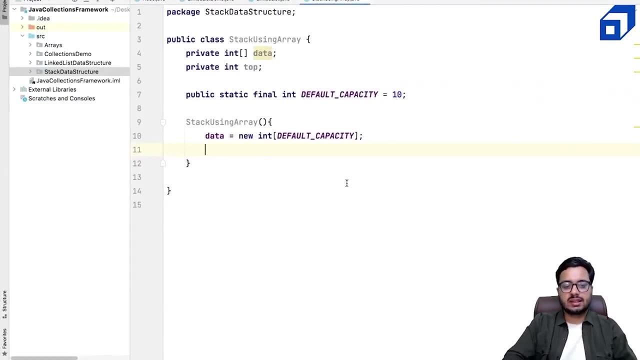 one why? because i have not stored anything. when you insert something you can say: okay, three is there and top will come here, so top will move after you can do the insertion. so i can say: initialize my top variable as minus one, so i can have another constructor in which. 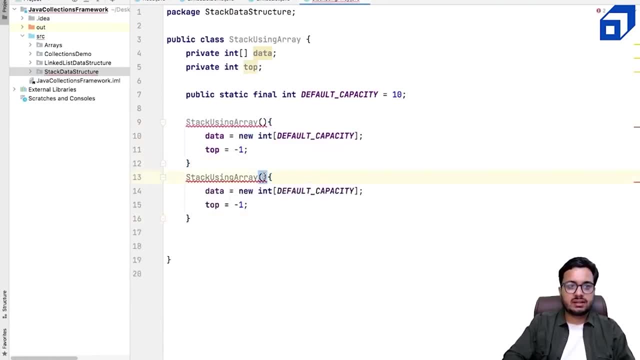 i'm getting some capacity as user input, so i can say, fine, i'm getting some capacity. so in this case i can say, okay, the array that i'm creating, it has this particular capacity, right. or you can also put put a check that if your capacity is less, 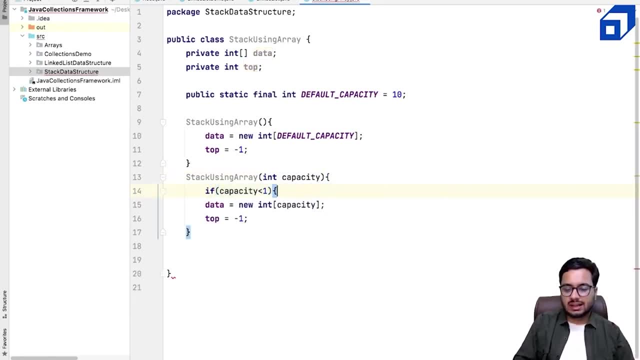 than one right. that means, is it negative or zero? in that case we can throw exception. so i can just throw new exception: uh, invalid tax capacity, right. so something like this we can do and here we can say: okay, this function can throw an exception, those exception. so this is: 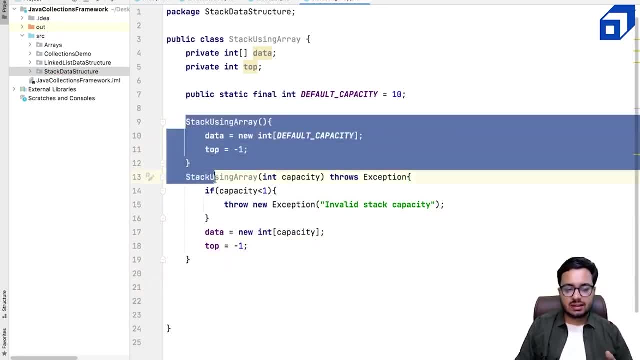 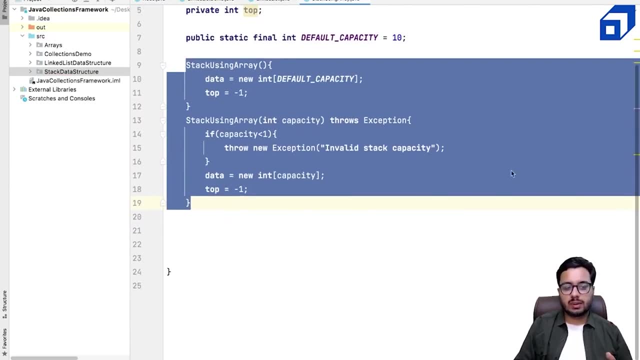 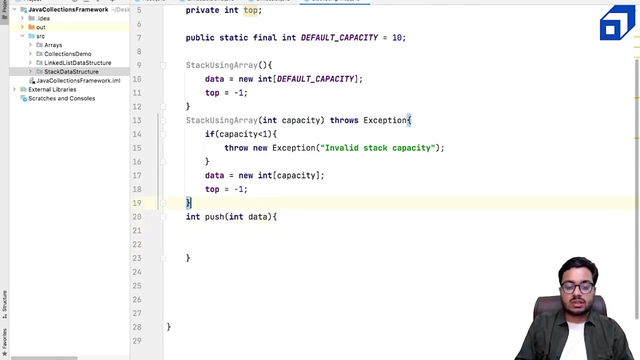 how we will create the constructor for the stack class. right, and we are using a fixed size array. now we have to, uh, define three functions. okay, we have to define a push function. okay, i want to push something into this stack, so i'm going to get data right now. we have to check whether my stack is full. 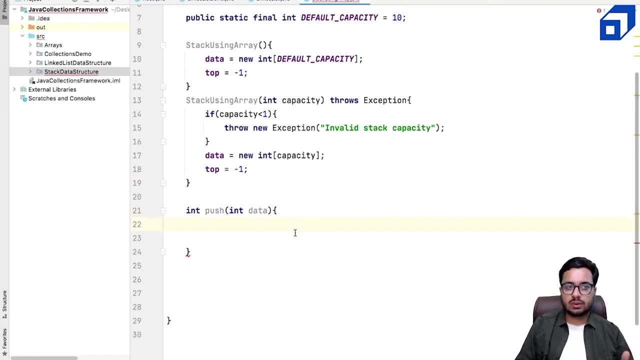 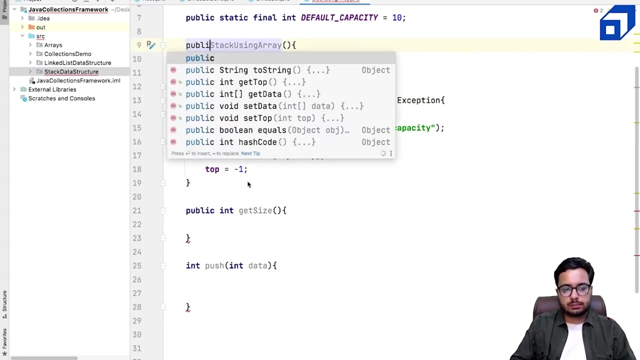 or not. only i can push right. so how do i check? how do i check? right? so let me do one more thing. let me also write a function that will, that will give me the size of the stack, right, so i'll say public and, um, get, the methods would be made public. i want to see, uh, what is the current size of the? 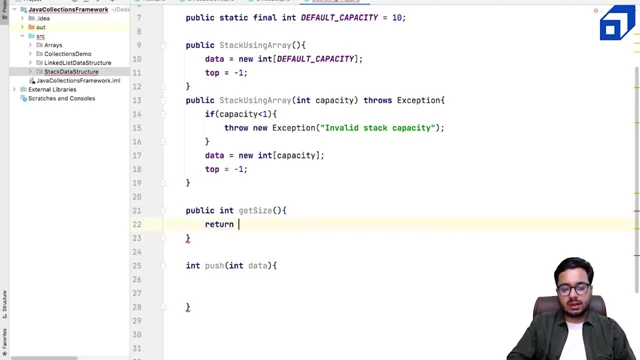 stack right. can i say: uh, the current size is nothing but the value of top plus one. so in the beginning top is minus one and if you have not inserted anything, this output will be zero. so minus one plus one, it will be zero when you inserted, let's say something, so top will be at. 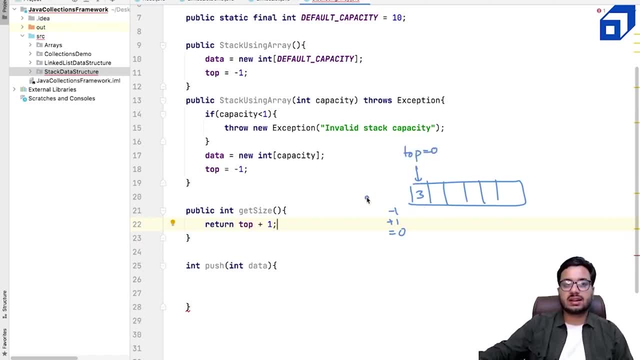 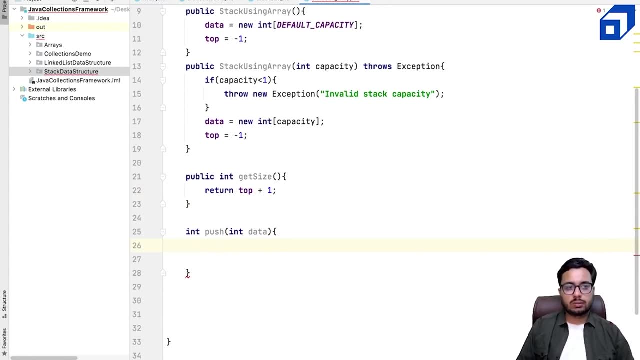 index zero. what is the size of the stack? the size of the stack is one, right. so when you're going to push, how do you check whether the stack is full or not, right? what you can do, just think about it. okay. so what we can do is we can check that whatever is the current size of the stack. 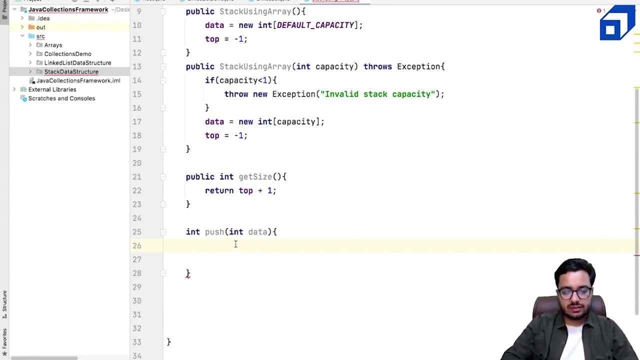 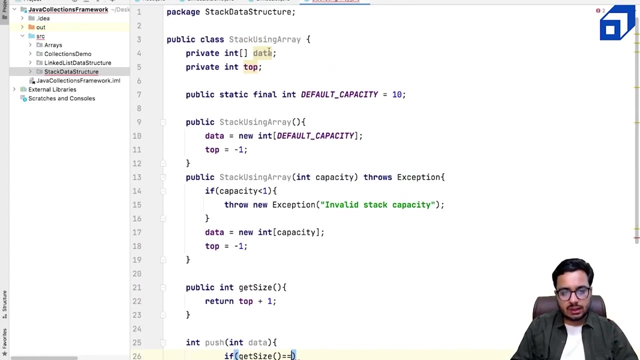 is it equal to the array capacity? right, so i can say, if i can call the get size function, which is basically giving me top plus one, is it equal to the capacity of this tank? right, so how do I know? so I can say that capacity is nothing but array length? right, so array has a property called as. 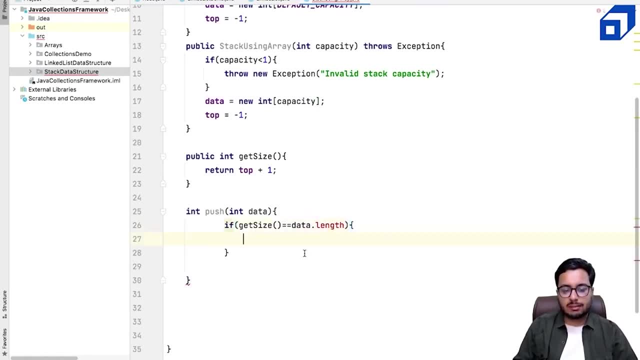 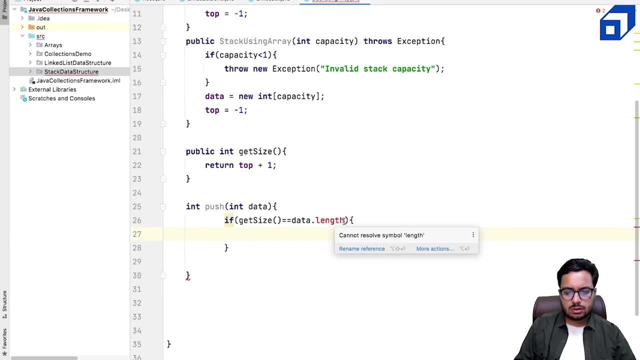 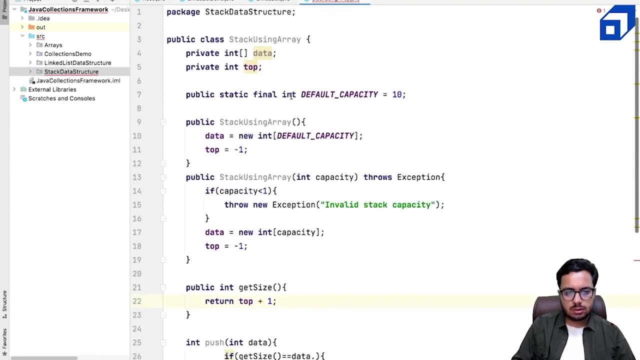 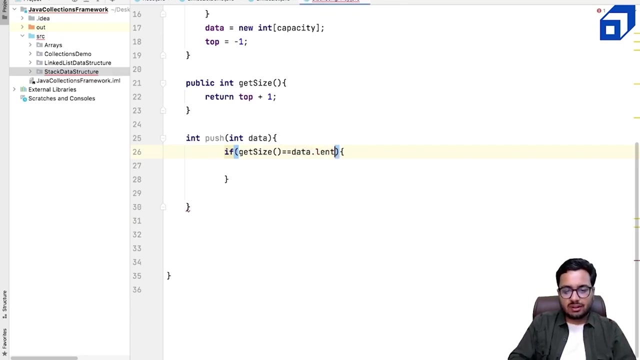 length. if these two are equal, that means my array is already full. okay, so we have here getting a error here: data dot length. because of this reason, data is a variable here and data is also an array here. right, I need to make it something different. I need to. 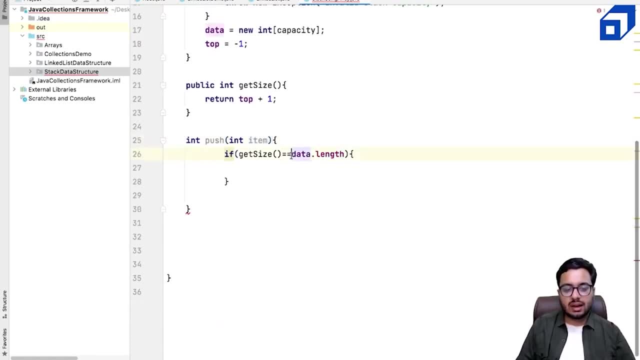 say: this is some item that I'm pushing into the stack and now this data means the arrays right if they are equal. so in that case I cannot push anything more. so I can say: throw new array exception and the exception name is: stack is full right. so that is some message we can. 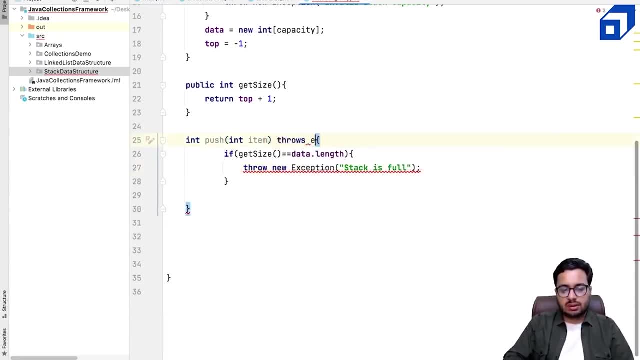 display and we can tell. this method also throws exception. all right, but if? if this is not the case, so what I will do? I will increment my top. that is okay. fine, increment the top variable and at the new position of top you are going to store that item, right? 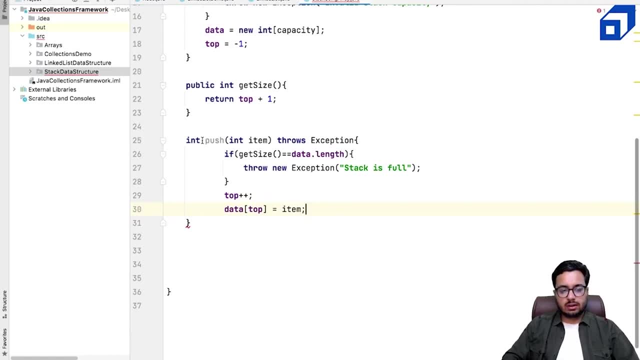 that's it. if the stack is not full, right, so function can be made as void public, void push. so we don't return anything right now. what is happening? that your top was here. I said push three, so my top comes here. and I put the item. I say push four, my top comes here. 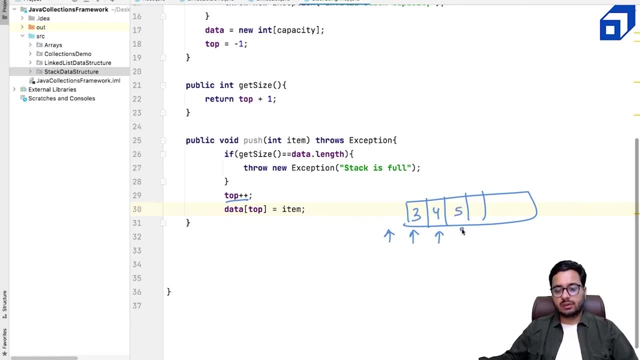 and I put the item again. I push five top comes here and so on. right, eventually, if your top top plus one is this value, that means if my stack is full, okay, so get. size is how many elements I have currently stored. it's a six, seven and the capacity of there is also five. so if it is there, 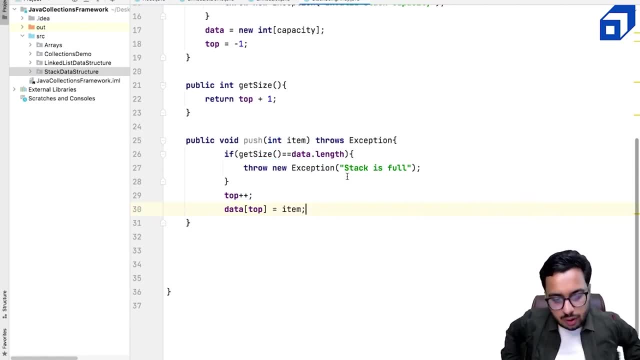 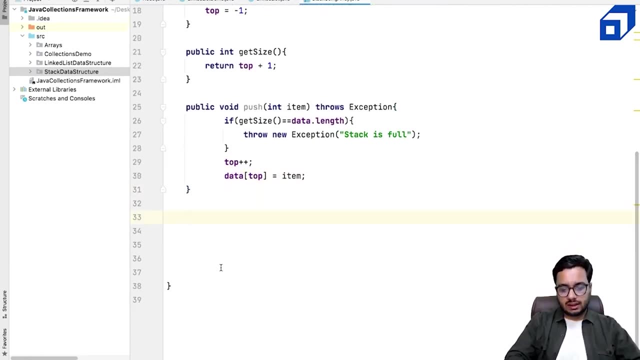 so I can say stack is full right. so that is how we can perform the push operation on the stack right now. let us talk about how do we remove something from the stack. right now I can say I will have public int pop. okay, I want to remove the topmost item. so again here what you can do. you can make a check that if 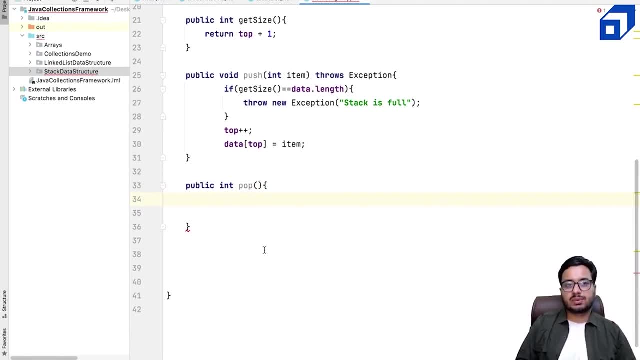 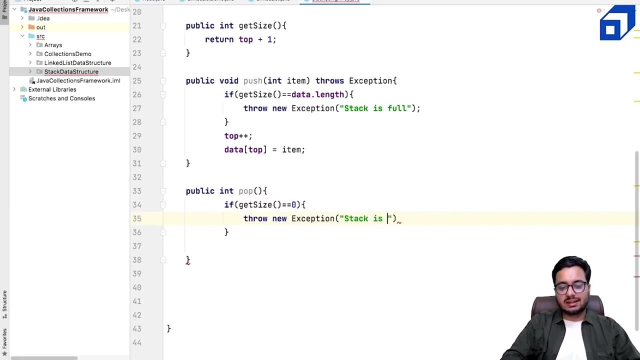 my stack is empty, right, then I have to throw an exception. I cannot pop from an empty stack. so if get size tells me, okay, this size is zero, there are, there is no data in the stack, so you can say: throw new exception. stack is empty, right. and here we can say this method: 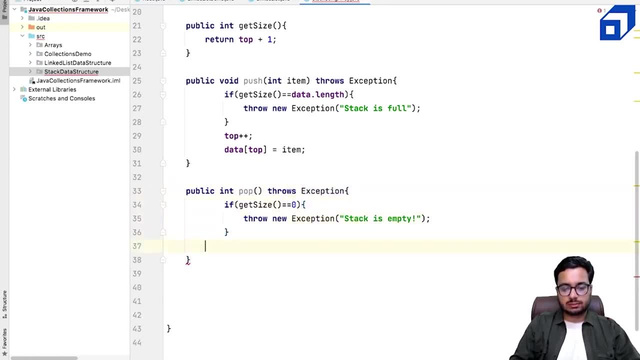 shows exception, right? okay, if this is not the case, I can easily remove something from the stack. I will store my answer. so, answer that I want to return it will be a data of top right. what I can do, I can reduce top top minus minus and I can return the answer that I have. let's see what we 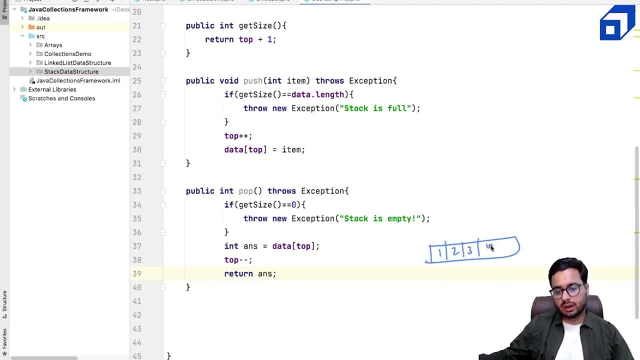 are really doing so. we are saying, okay, one, two, three, four, this is my top, right? I want to remove this. so I can simply say, okay, this top will come here and I will copy this four in a variable called answer and I will return it. right now you might say, okay, if I print the stack, I might see four. that's not going to be true, because 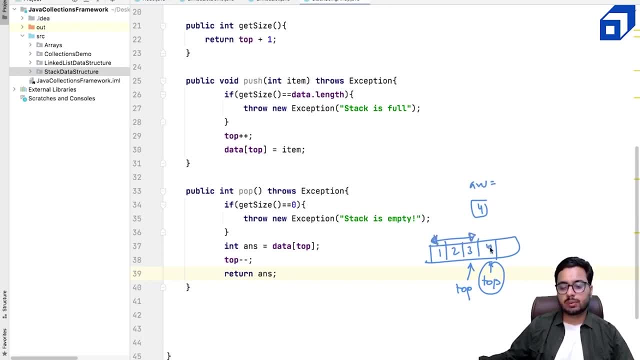 we will only print up to one, two, three, right up to top right, this data. if you want, you can make it zero or you can keep it as it is right. so just to make it little more more clear, I can say: answer of top. I'm making it zero so that, oh sorry, rate of top. I'm going to make it zero so that it looks. 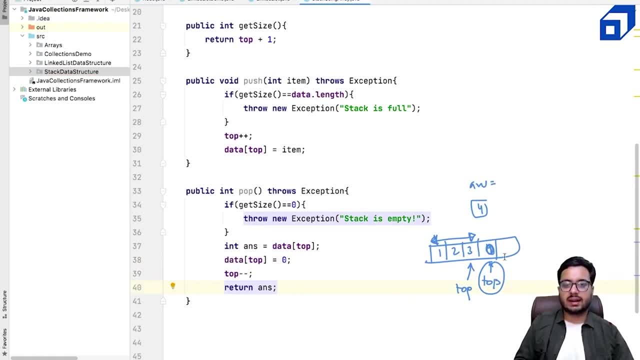 good when you try to, uh, look at the entire array, right, so I'll. so, in general, you are not going to look at the whole array, but only the array till the top. but that's okay. so this is an optional step if you would like to do right, because data can be zero, also right. so again, this is an 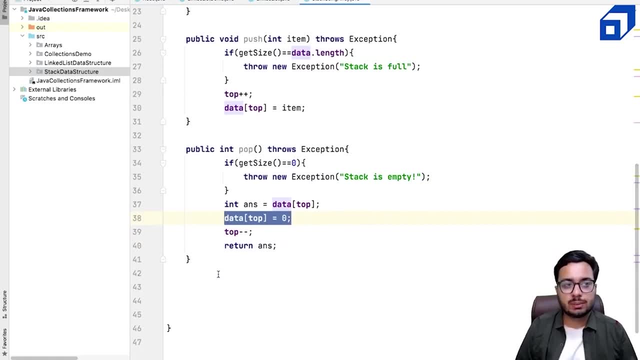 optional thing if you want to. that is how you will remove something from the stack. right now we have the method to look at the topmost element, right? so sometimes this method is called as a top, sometimes it is called as peak, right, if you want to look at the peak method? uh, it's pretty easy. 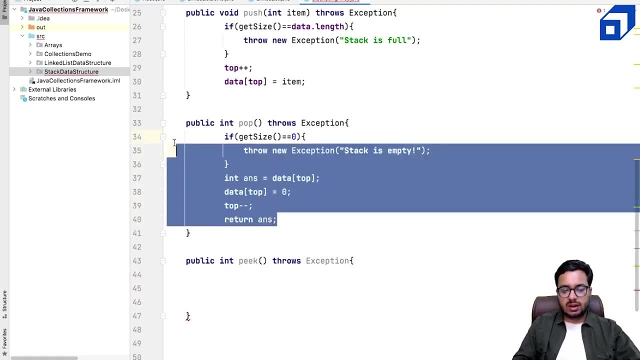 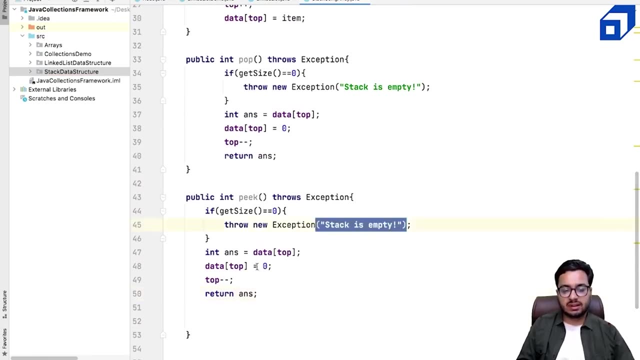 you just need to do the similar thing, right? so it's okay. if the array is empty, then you can throw a new exception. that stack is empty, otherwise you get the data but you don't remove it. so that's it. you can, or you can simply return data of top. okay, the topmost element you can return directly. so 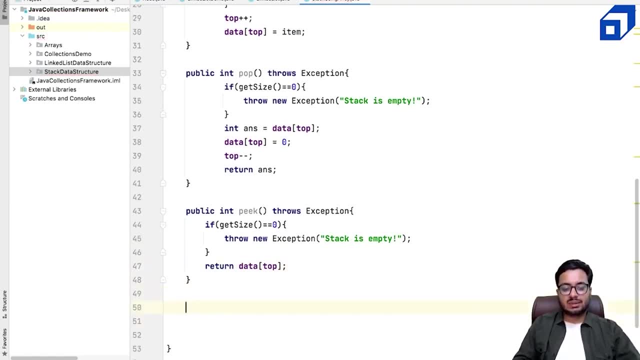 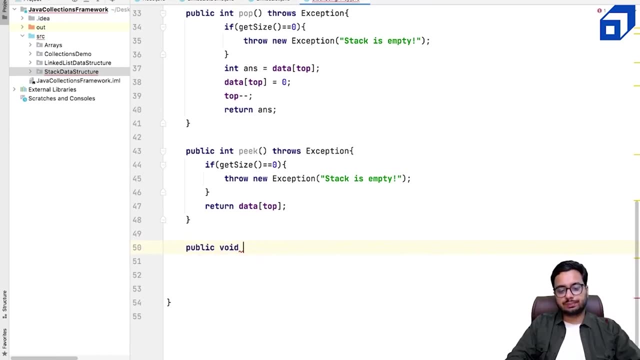 that is your peak method, right? let us add some more methods. if you want to print the stack, so I will print everything up to top right. public void display. so I can say for int, i equal to top, i greater than equal to zero, i minus minus. so I will iterate on the items in the reverse order. so if it is like one, two, three, four, 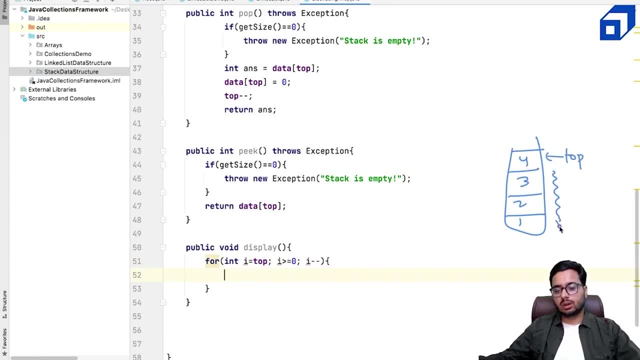 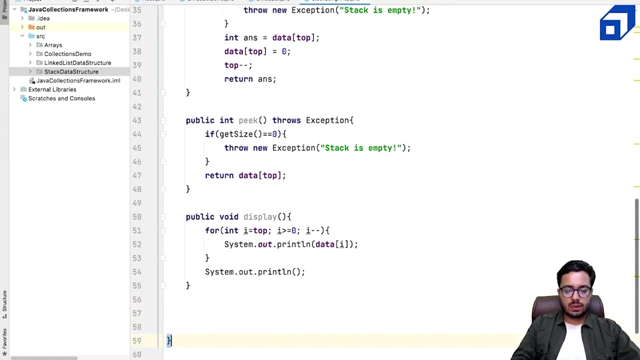 I will first: okay, I'm going to print from top to the bottom, right, like this, so what I will do. I also okay s out data of i. that's it right. so that is my display method and I can give a new line here. I will put a line in here and I will put a line in here so that my stack will be empty. 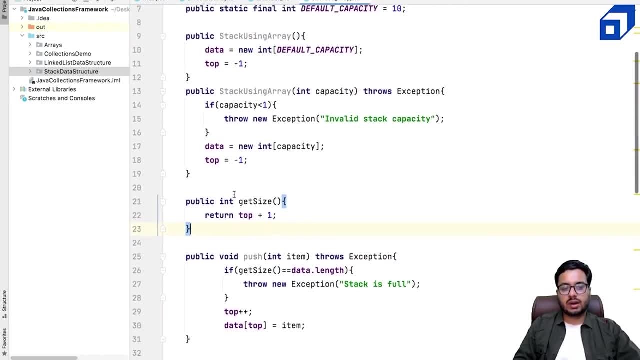 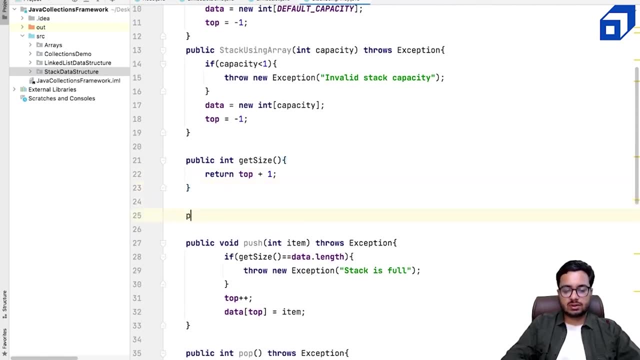 so any other methods if we would like to write. so maybe we want to write a method called as is empty or is full, so we can write those method as well. so I can. I will write is empty method, whether the stack is empty or not. so I can say public and public boolean is empty. so this is helpful when 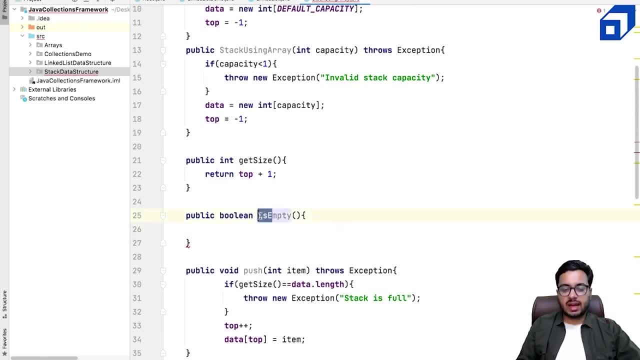 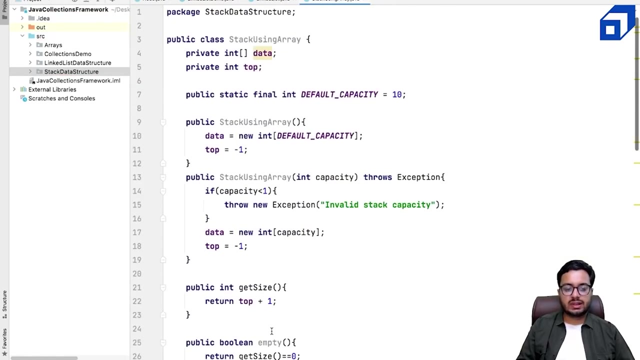 you want to continuously remove elements from the stack, and until the stack is not empty. so this used right now I can return. if my get size is equal to zero, this expression will evaluate to true or false. I think this looks good. next we will test the functionality of this stack that. 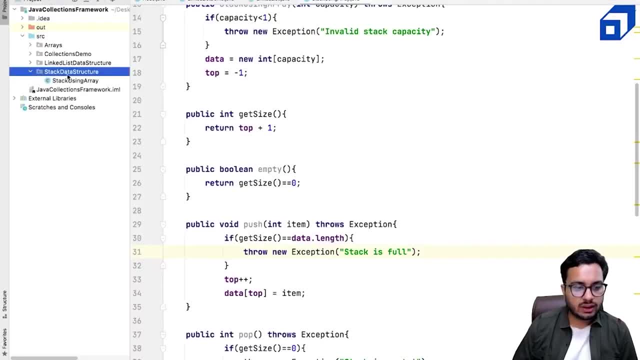 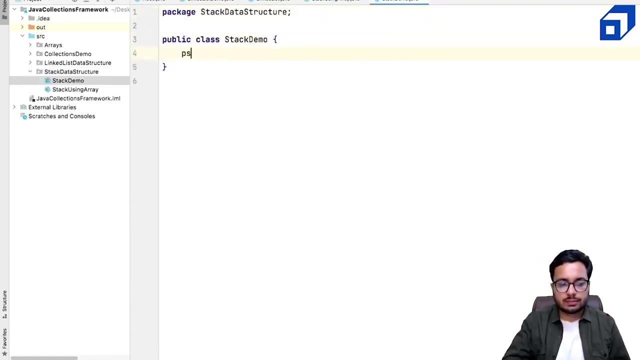 we have created. now let us write one more class so that we can test the functionality of this stack class. so I will call it as a stack demo. dot java- right. so in this stack demo we will create a stack object. so main method is there, like in the stack s. sorry, this should be stack using an. 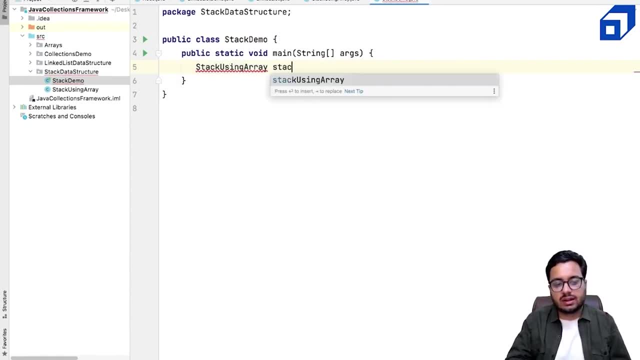 array right. stack using an array- I call it as stack. this is equal to new stack. new stack using an array right. I've created the stack object, or just call it as it is. push some numbers into it so I can say: s dot push 1, a start. push to a start, push 3. so we have to push method can throw an exception so I can say: 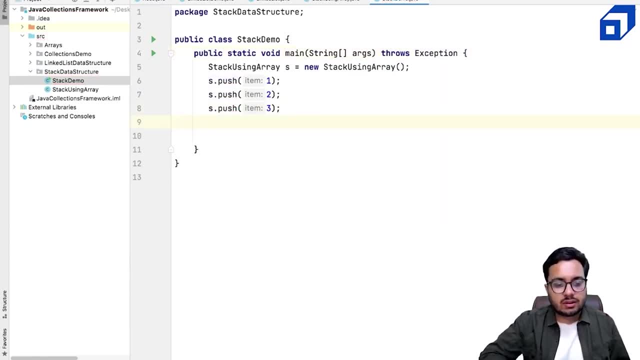 main can also throw an electrical connection, the s dot push 3, 4, 5, whatever it is right, and then we can try to extract items from the. so four, five, six- i've added six items. i can say okay s dot display show me, uh, the stack right. let us run this and see what do we get right. and at the same time i will 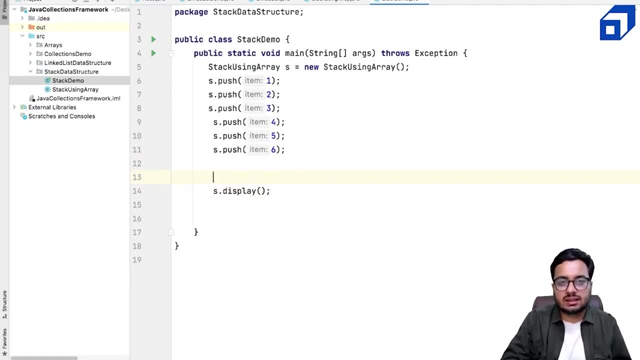 do one more thing. i will pop items from the stack until the stack is not empty. so, while the stack is not empty, what i will do is: okay, give me the topmost element so i can say s dot peak. print the top most element, so s out uh topmost element and remove it so i can say s dot pop, right a pop. 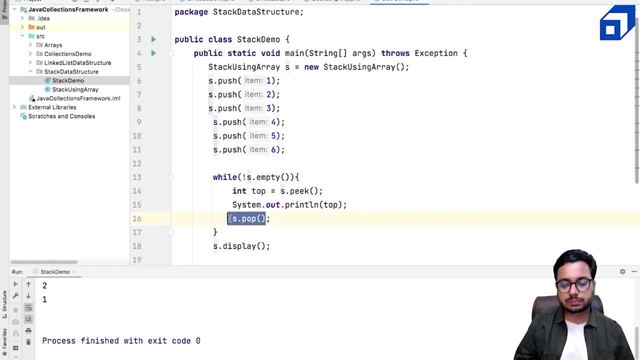 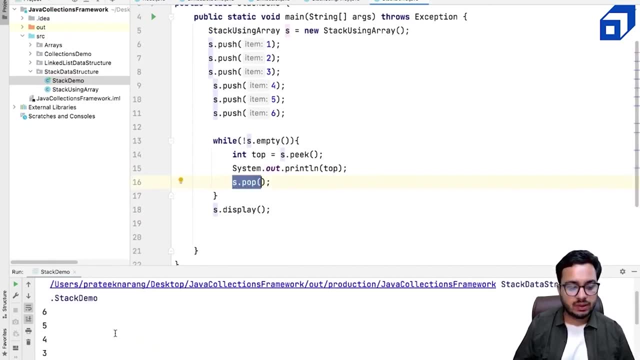 function you can also use, uh, because it also gives you the element and remove it. right, but here we are not reading the value from the pop, we are just reading the value from the peak function. so when we are printing it, you see six is at the top, then five, then four, then three, then two and then one. right, if? if i do not call the display, 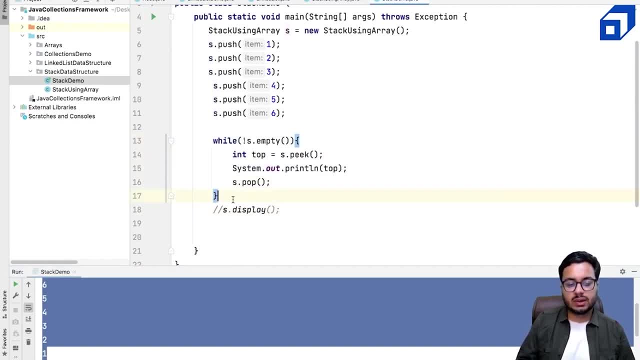 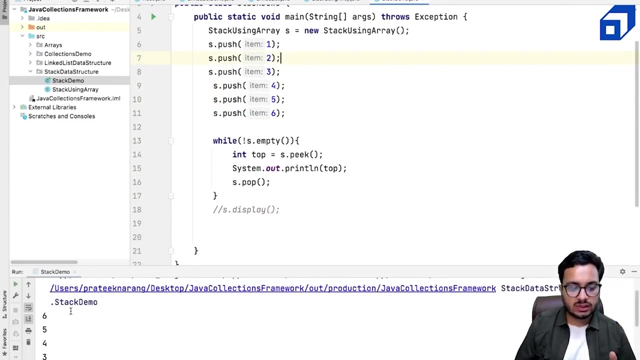 method. instead, i use this while loop: what is the first element that will get removed? that will be six, last in, first out, then five, then four, then three, then two and then one. let us go and run this code and we will get a same output by removing all elements from the stack as well. right? 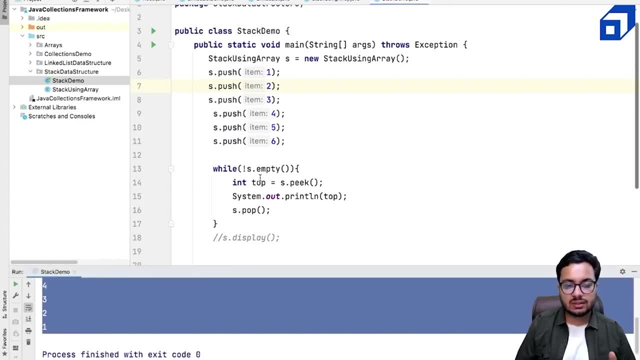 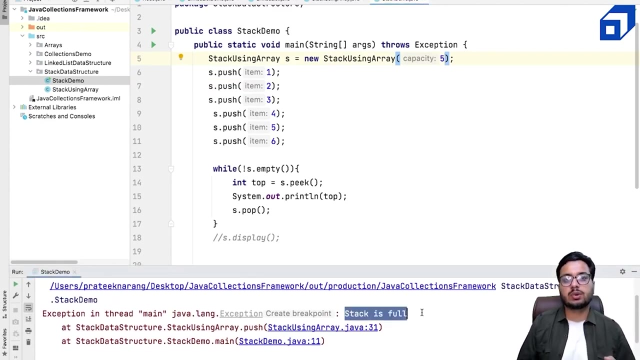 so you can see that means our class is working perfectly fine. by default, the capacity is 10. if i show the capacity is 5 and i try to insert six elements, then this code is going to throw an exception that the stack is already full and i cannot push any more elements into the stack. 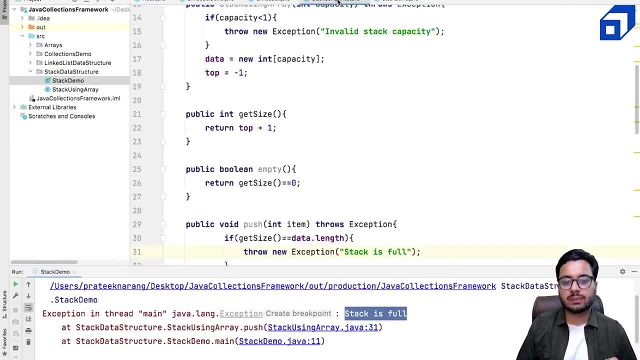 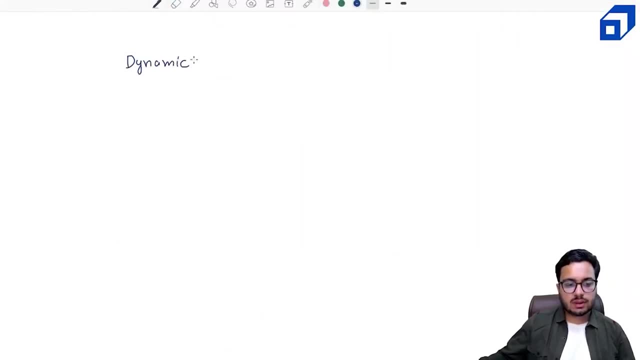 the next implementation of stack we will see using a dynamic array and a link list. let us talk about dynamic stack now. there are two options to implement it. one is you can use an array, or one is you can use a link list. so when i say array, we can use a dynamic array, right? so suppose you are implementing the 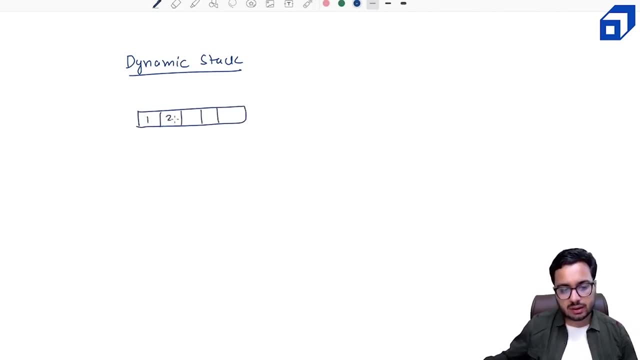 stack using an array and at some point, your array got full. okay, your current size is equal to capacity, right? what you can do is using the same logic as array list inside your push method. what you will do, you will find i will create a new array of double the capacity. if this is the 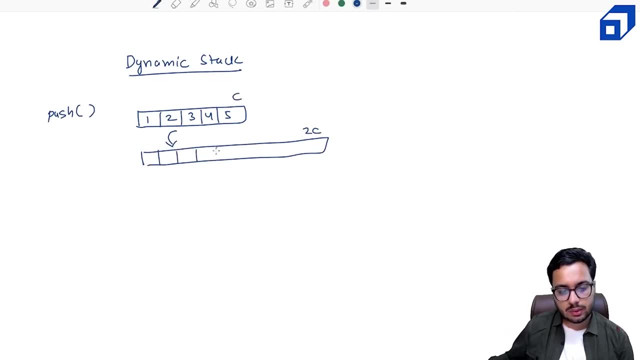 this is c. i will create an array of 2x of my capacity and i will copy the elements here, right? that is how my push method will get changed, right, and pop will remain same. i am not going to shrink anything, so pop will remain same. even the top method will remain same. no changes, right, nothing. 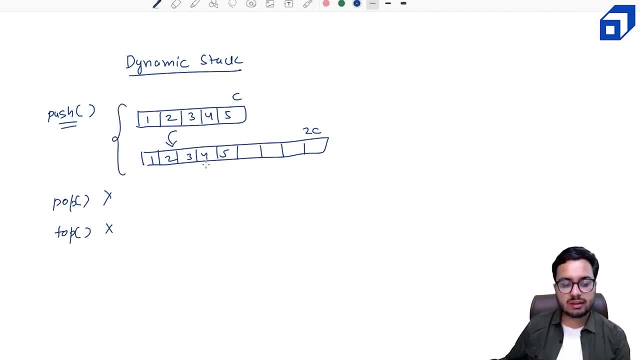 changes here, only in the push method. we are going to change. array will not overflow. instead, it will get a doubled right. and again, this copying is an expensive operation, right? so we should make sure that this is not happening, happening too frequently, right? that is why initial capacity is important, right? so that is. 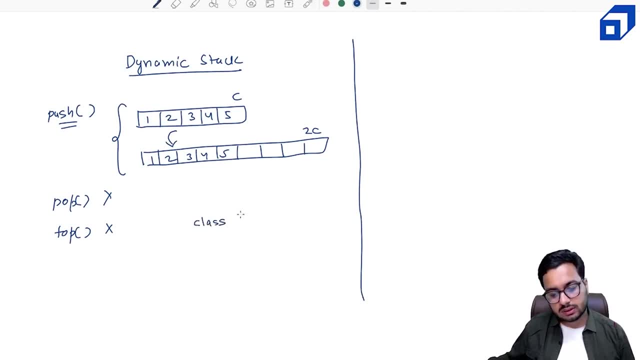 using an array list right now if you want to discuss it in the code so you can say: okay, i have a class called stack. so either you can keep a error list object here, right, because we have already implemented a list. it can be your implementation. it can be library based implementation as well. 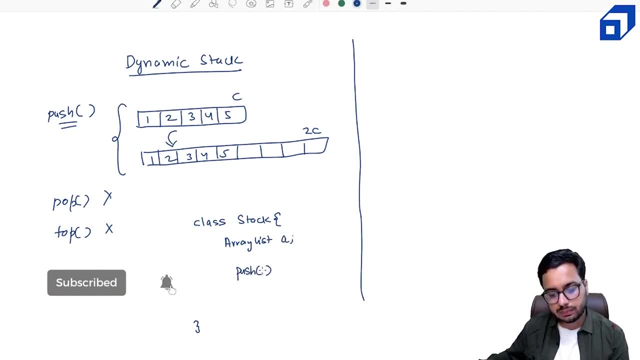 whenever you go get a call for push some item i, you can simply say: okay, a dot, add the item i. so add function. we know it adds at the end of the array list. the code becomes even simpler, right? or if you don't want to use, uh, the inbuilt class, right, what you can do, you can take the manual array. 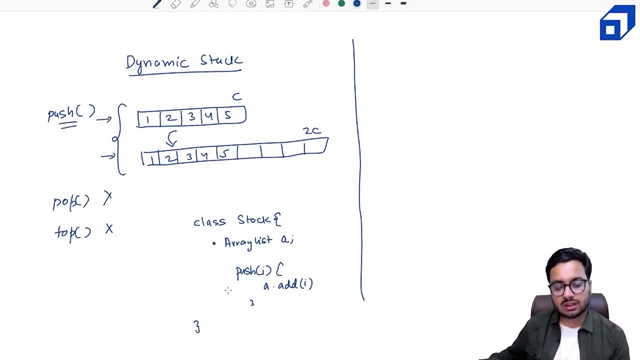 like we did in the previous example and write the doubling logic inside the push method. so i'm hopeful that you will be able to do that part right. another option is you will only output your sawdon as one. so sorryox, step one right. you can choose your network or as their code, location or destination. then you tell the kingdom instead of the area method with add function. so if you will not make a column, Katrina, etc by the function, we can add two where the googles inside the item. like you want to add laser into the executability function for curated errors is the right thing to make it as all the here cool stuff, bro, mouthwash right. 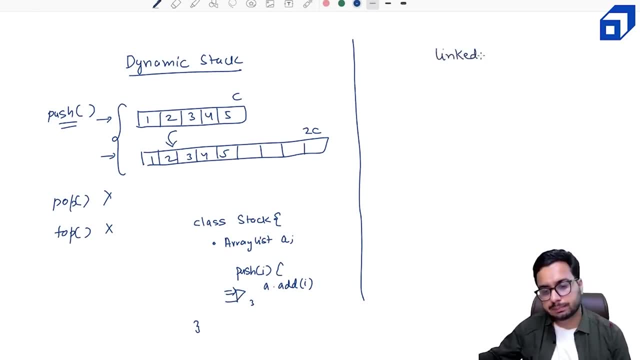 another option is you can use a link list also. right now, suppose we are building a stack. i got one, so i insert that node into the link list. my head is updated, tail is also updated right now, suppose you. you got two now. the question is, where should i insert two? should it? should it go? 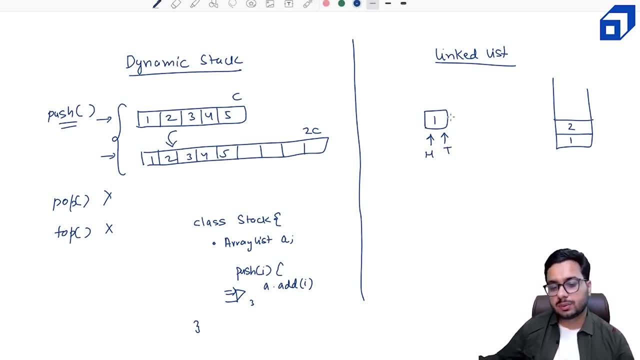 at head or should it go at tail, right? one option is okay. if i put it at tail, insert at tail. if i do it, this tail will go here, right? okay, and suppose i got three. then you can again insert it at tail. this tail will go here, and three is also inserted right now. the question is if i want. 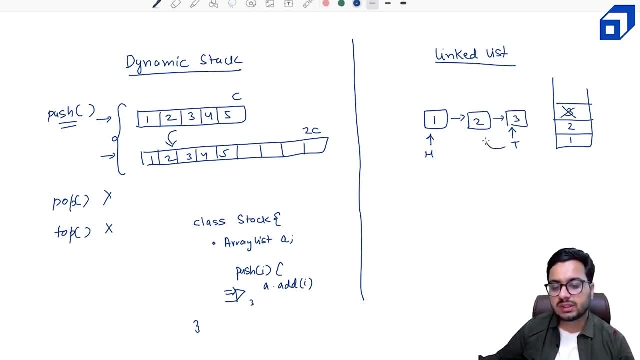 to remove something. if i want to pop out three right, how do i move this tail back right? i cannot move it back in order one time right, i have to traverse from the beginning. this is going to be time taking. so push is going to be order one, but 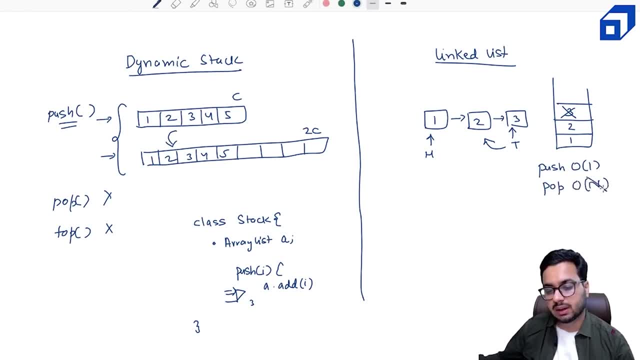 my pop is going to be order of n, which is not acceptable here, right? so hence i need a better implementation using a link list. let us do one more try. suppose i got one and both hadn't till they got updated. right now, if i want to insert two, two will go here. i will create a new node. 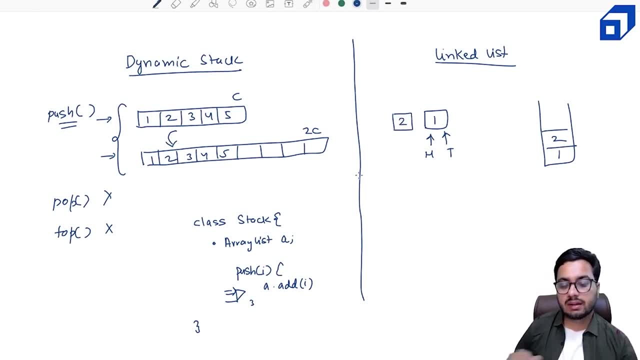 okay, and i will connect this node with the head. so basically, i'm inserting at the head, only this head will move here. fine, right, because that that we have seen how to insert at head. then i insert three. i create a new node connected with the previous head. 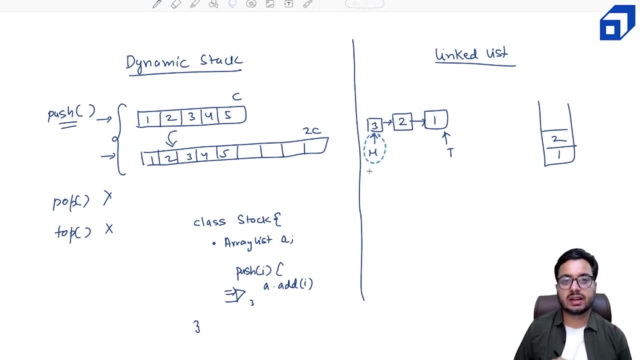 and i update this head right. this head can come here right now. if i want to remove something, i can say, okay, i want to remove the topmost node, i want to pop this node right. how do i remove it? this is now pretty easy, how we can say, okay. 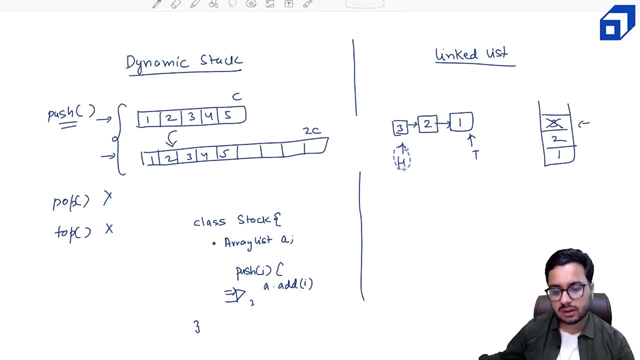 fine, let me move the head from here to here. and this node now becomes eligible for garbage collection. right, that means popping is very easy. even looking at the topmost element is very easy. so the element at the head is the element at the top. so again, if i want to remove this thing, my head, 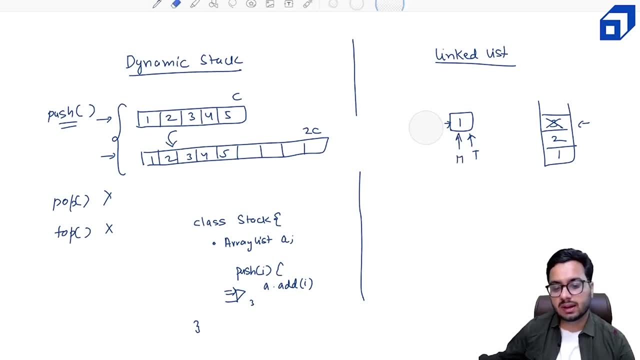 will go here and the node 2: it will become garbage collected. so using linked list also, building a stack is very easy. if you want to insert something or you want to push something, you can say: okay, i will call the add front method of the linked list right, or insert front, whatever it is, and if i want to pop something i will say remove. 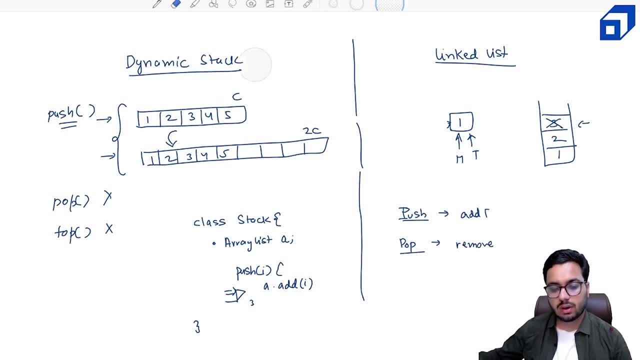 from the front. okay, i think add first, we call, called it as add first. i need to add at the first position and i need to remove at the first position. right, and peak is nothing, but it is the get first. i want to get the first element, the linked list, right. that is how it's going to work, right? so regarding the implementation, 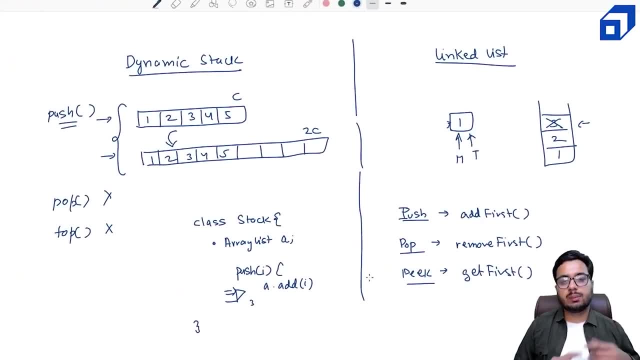 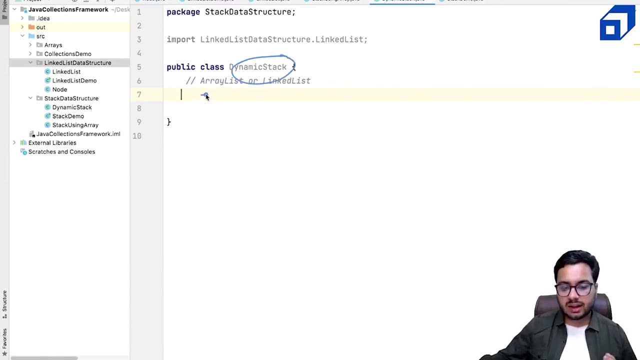 i think it's now pretty easy, given that we have implemented arraylist, we have implemented linked list, what you can do. you can also put that code inside your dynamic tag class as well. right now, three options: either you write entire code- that is option number one. you define the node, you write. 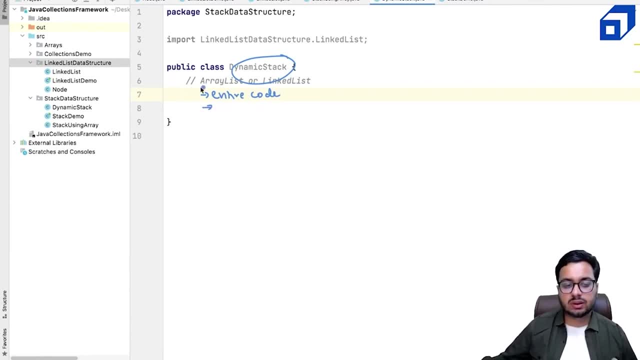 how do we insert at front? second option is you can use, uh, the linked list class that we have created or the arraylist class we have created, so you can use your library version. okay, if you don't want to do that, you can also use the collections um arraylist or the collections linked list, right? 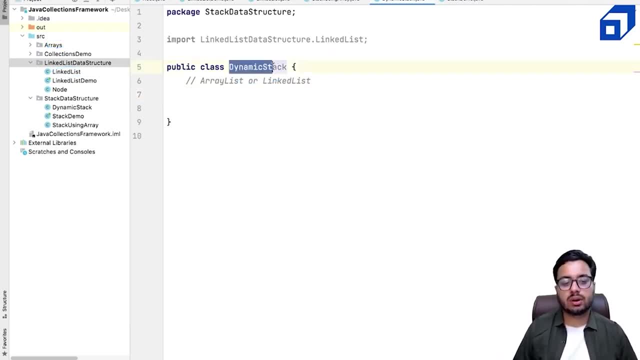 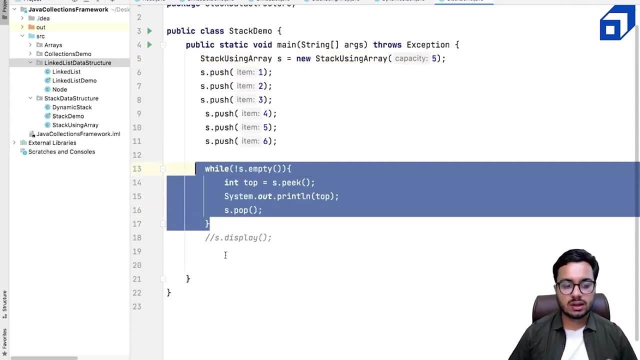 any, any code you can use to build your own version of dynamic stack. right and the behavior wise, it will have same functionality, except that it will not get the same functionality, except that it will not get full unless your system memory is not full, right. so that's all for dynamic stack hope. 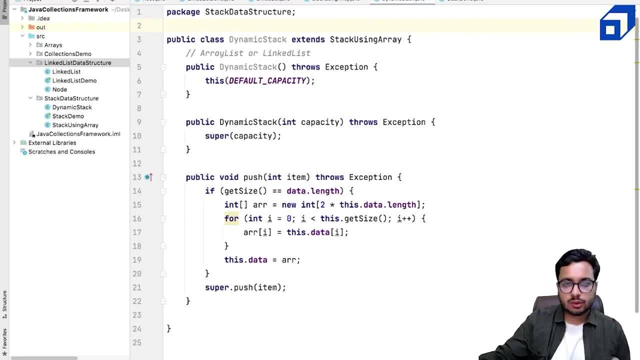 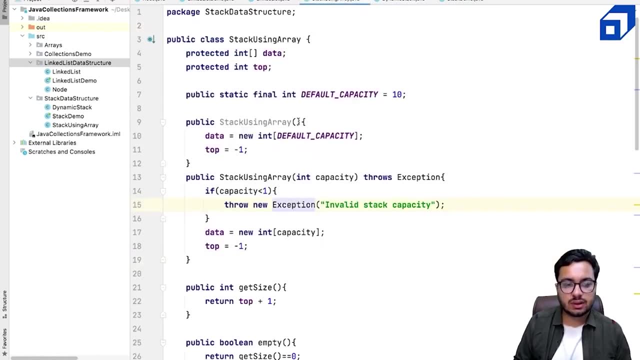 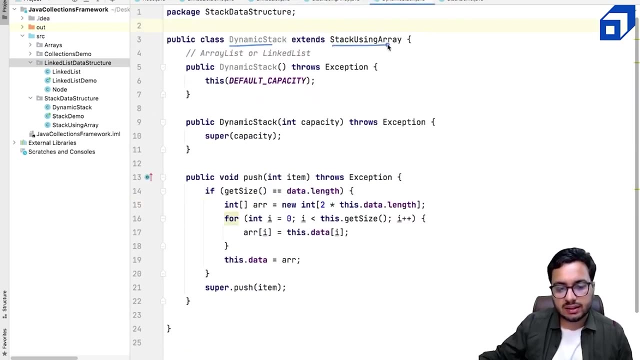 you understood the functionality of dynamic stack. okay, i'll show you one more implementation of implementing dynamic stack using the stack using array class. so this class we have just written. so what i'm doing, i have created one child class called dynamic stack and it is extending the stack using array class that we have just written. so inside this class, i 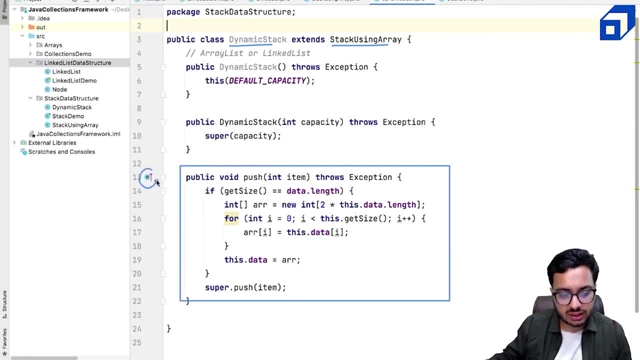 have only updated the push method. so basically i have overwritten this method, right, and i have provided two constructors so that i can provide, uh, build the dynamic stack object, right. so the first constructor does not accept any capacity. so i call the constructor. so this is basically calling this method with the default capacity. so i say, okay, go and create a start with the. 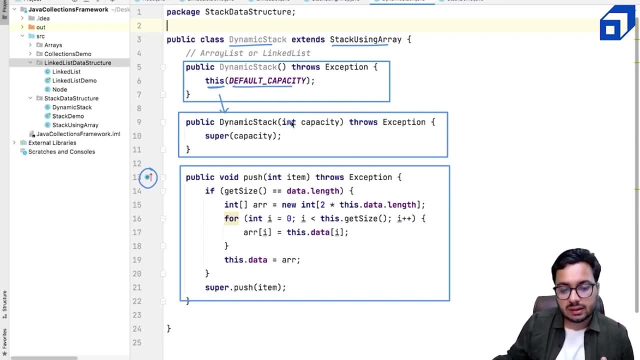 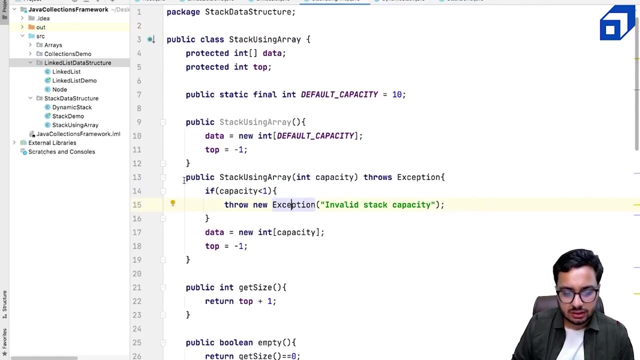 default capacity, right, and if i get a capacity from user, then also i can. i call the constructor of the parent class. so super is for calling the parent class and i give the capacity. okay, you go and call the constructor that is here, right? so this constructor is getting called right and i. 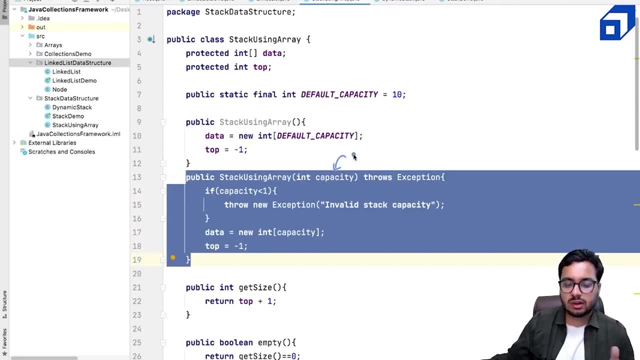 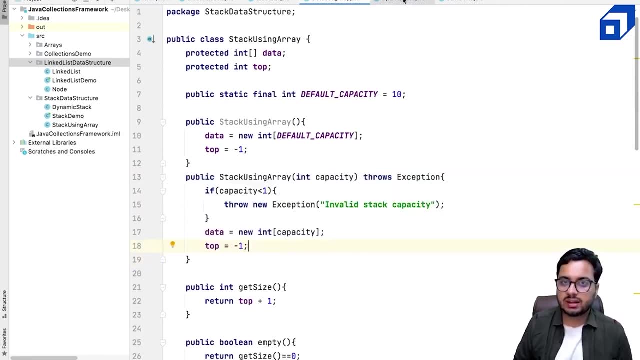 pass in the capacity. so either i pass in the default capacity, that is 10, or i give the user defined capacity. right, so i give that. so this calls the parent constructor and initializes that array right of that particular size, right? so pop method. i call the pop method and i give the user 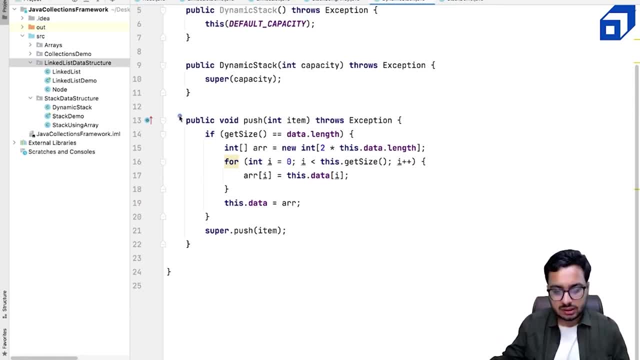 told you, it's not going to change the peak method, it's not going to change in the push method. if my array is full, right. so if get size is equal to data dot length, right, and what i will do. i create a new array of twice the size, i copy all the elements into the new array, okay, and i say, okay, this dot. 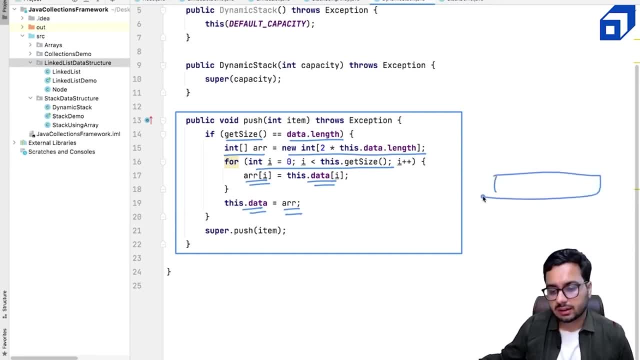 data should, uh, now point to this array, right? what happens? so data was pointing to the old array. right now data is pointing to the new array, so this reference is gone. that means this array will be garbage collected, right? so this is arr. error is a local variable, it will be destroyed, but data is a class member, so it will. 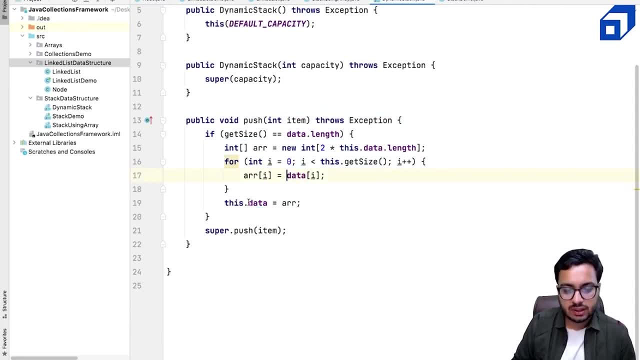 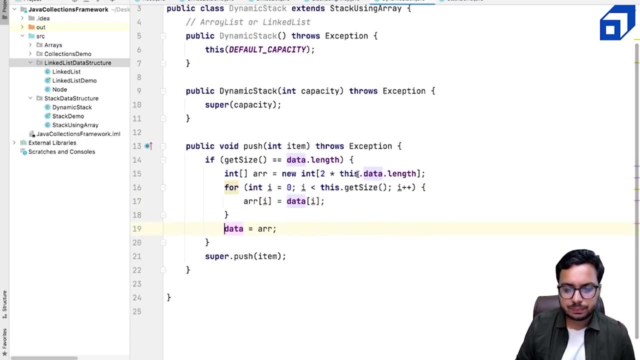 not get destroyed. so using the- this keyword is optional. it is for more clarity that we are talking about the data member, very, not any local variable, right? so that is what we are doing here, and then, after we expanded the array, we call the push method of the parent class. 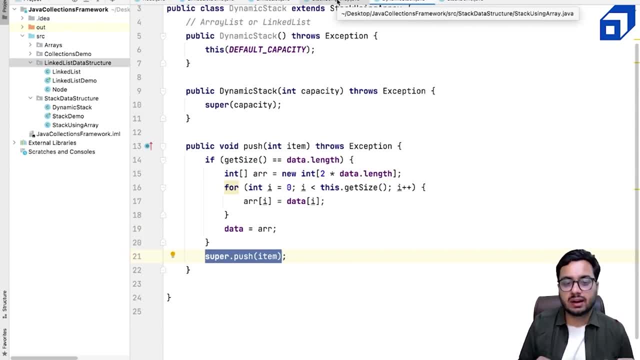 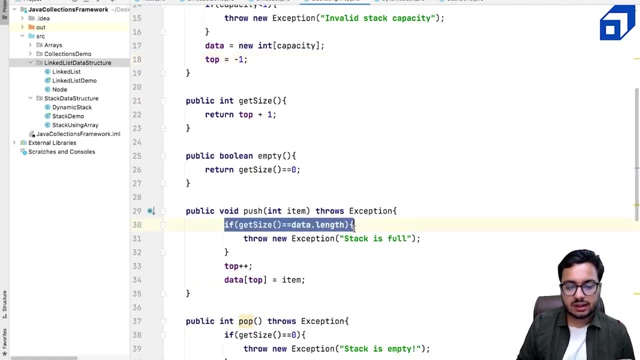 in the parent class. now, if, if your array has already expanded, you will never get this condition. this condition will never be met. which condition? that data dot length is equal. so exception will not be thrown. and what will happen? top plus plus and data of top equal to item. so this code will: 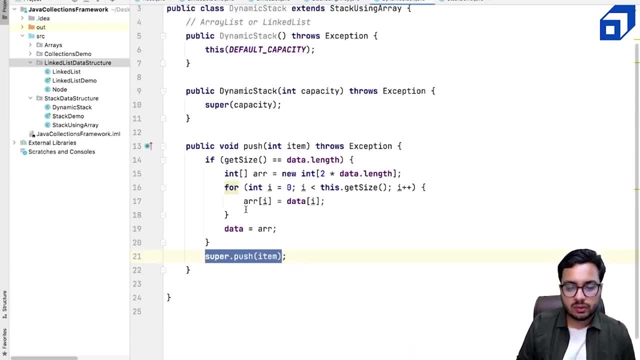 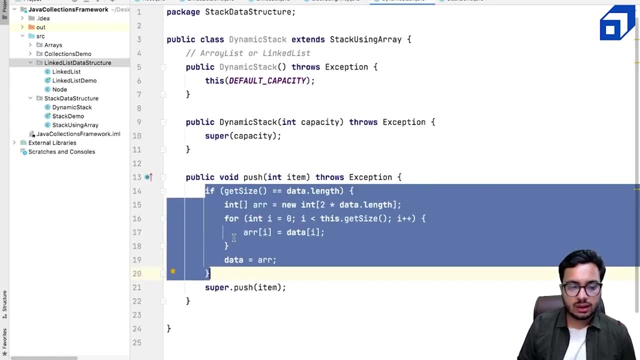 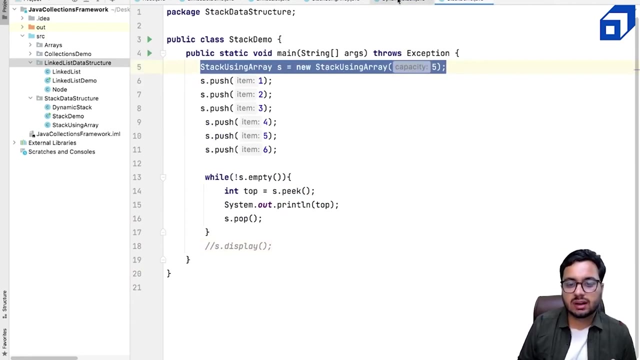 actually execute. if condition will not be true, before calling the push method of parent function, i simply expand the array. in case of a dynamic array, this is what i rarely do and it will work. so what you need to do, you need to replace this stack with the dynamic stack. you can try it out. 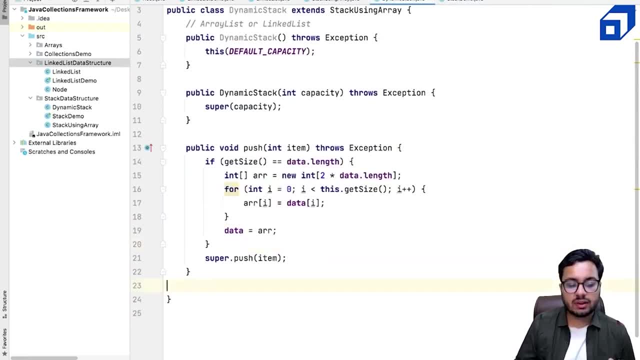 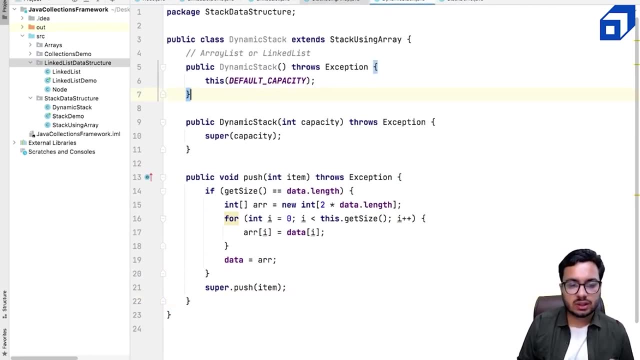 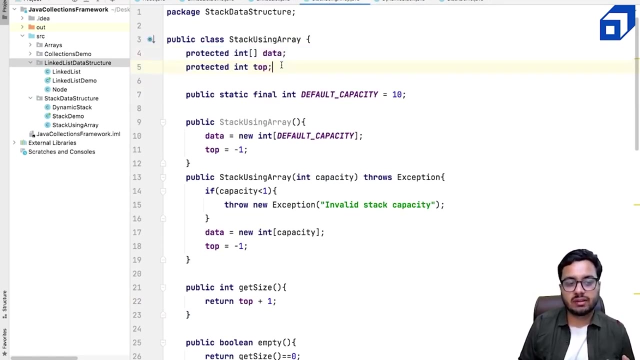 and it will work right. so that is another way of using inheritance and creating a dynamic stack object for you. one small change i wanted to discuss was i did a change that i made these data members, which were earlier private. i made them as protected. now, right, why? because i want to use these data members in the child class as well, right so. 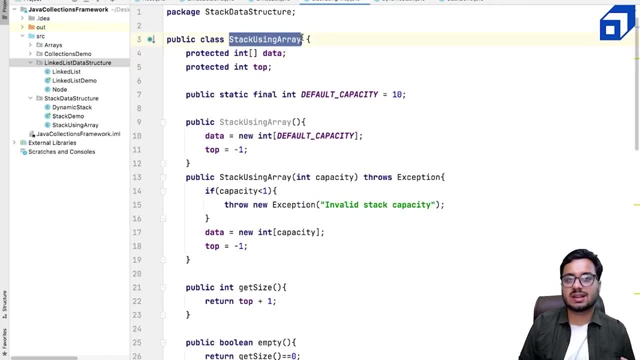 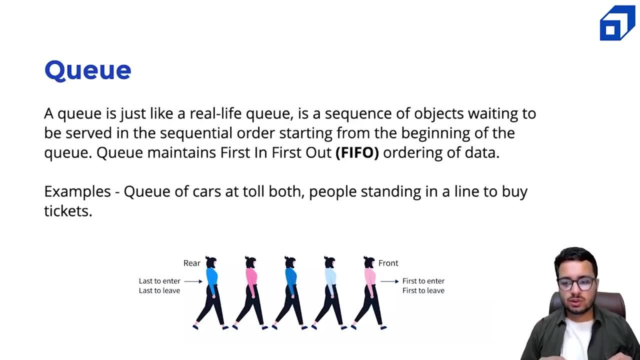 that is the only change i have done in the class called stack using an array. so let us start by understanding the fundamentals of a queue. what is a queue? a queue is just like a real life queue. so, in most general terms, a queue represents a sequence of objects. 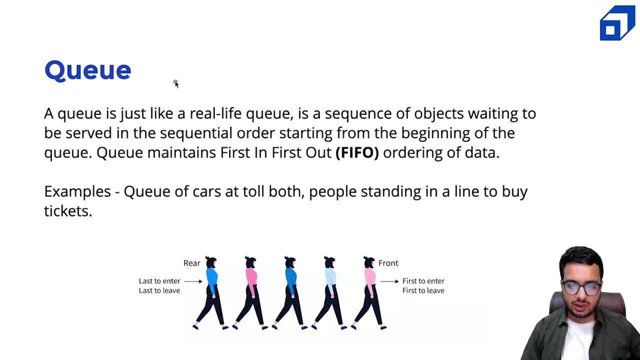 waiting to be served in a sequential order. okay, so one thing you need to remember is that a queue is also a linear data structure, like other linear data structures you have seen so far- arrays, array, list, tags, linked list, q, q is also a linear data structure that stores the data in the 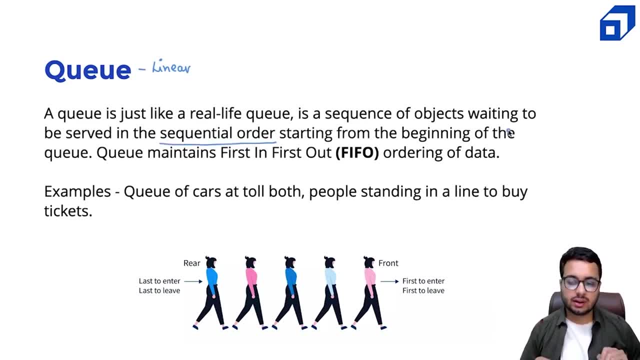 sequential order starting from the beginning of the queue. right. for example, if you go to a bank right, the person who enters the queue first it is at the front of the queue, second person is behind it, third person is behind the second person, and so on, right. so in general, q has two ends. one is called as front, from where the people will be served. right. 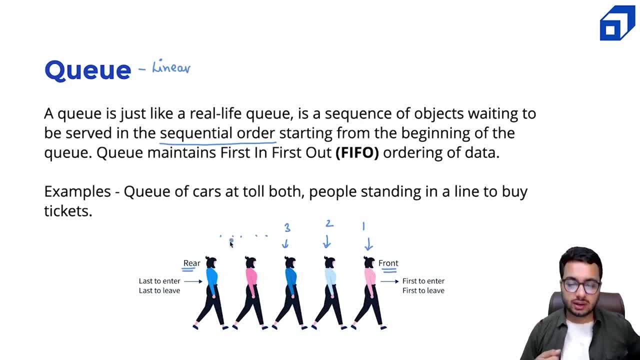 and one is the rear end, from where people will join the queue right. basically, insertion of data will happen from this side and removal of data will happen from the front side. right- people at the front. once they are served, they will get removed from the queue. right now, this queue can. 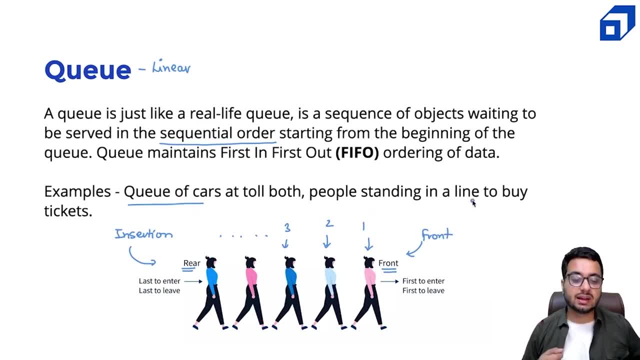 also be seen as queue of cars at a toll booth right, people standing in a line to buy the car tickets right. and in the world of computer science, we use queues a lot, right. for example, many people are uploading videos on youtube and youtube has maintained a queue so that people who 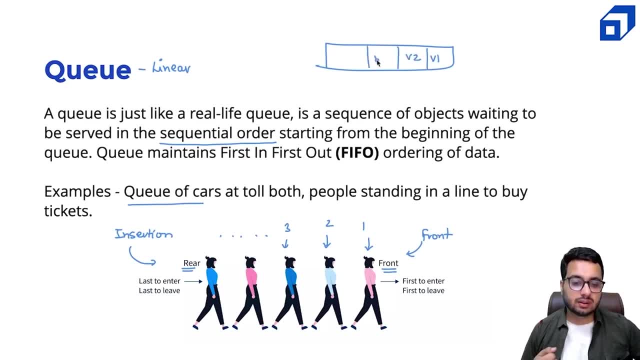 have uploaded videos first, their videos will be processed right. we might maintain a queue of videos on the server waiting to be processed right. similarly, on in software applications, for example, an application has to perform several tasks, it might maintain a queue of the task that it needs to perform so that our work gets done right. so q is again a very important, very interesting data. 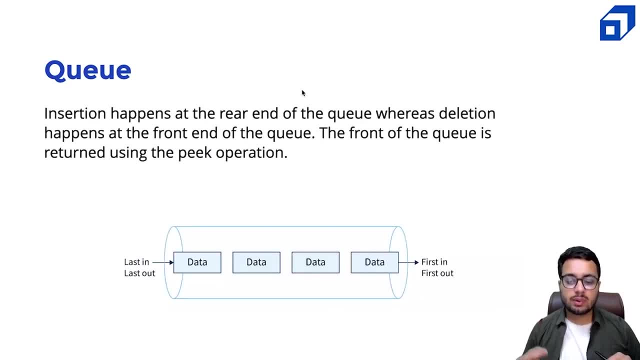 structure. right now let us talk a little bit more about the operations. so, as i discussed, one fundamental operation on the queue is insertion right. i want to insert something into the queue right. so the kind of queue that we are discussing, current now it is called as FIPO queue. first in: 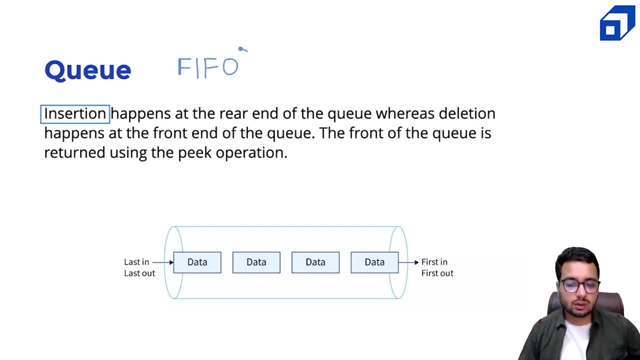 first out queue. why? because the person who joins the queue first is the first one to get served right. in a FIPO queue, insertion happens at the rear end of the queue, so this is your, let's say, rear end, whereas deletion happens at the front end of the queue. so this is your front side, right? so anything? 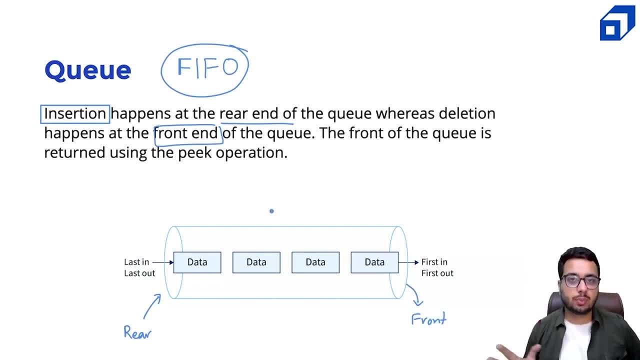 you cannot say: okay, i want to remove something from the middle of the queue. that is not possible. only the data which is at the front of the queue will be removed. right, there is one more operation. so we have seen insertion. we have seen deletion. right, we will discuss how these operations are. 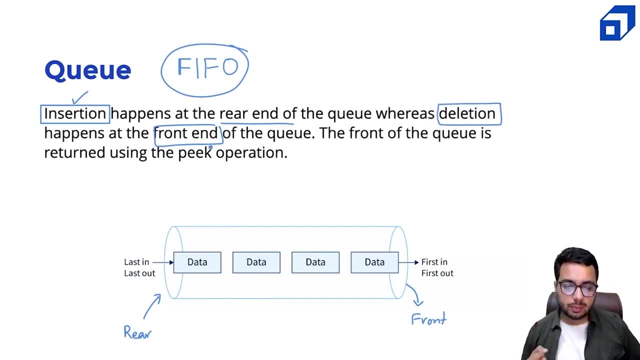 implemented using other data structures. right, there is one more operation that is called peak, so i want to look what is the front element? okay, who is standing at the front? we call that operation as peak. so just in case of stack, if you remember, the peak operation returns. 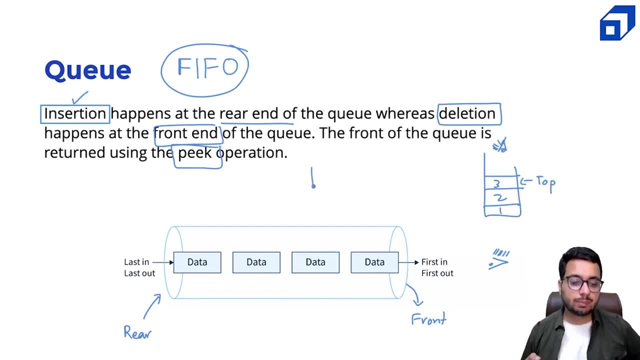 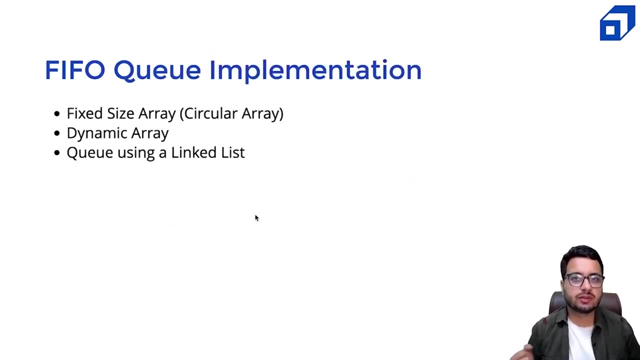 the top of the top element of the stack in a queue. peak operation should return the front element of the queue right, the person who is standing at the front of the queue. that is what peak operation will do right. so as a next step, we will look at the implementation of a 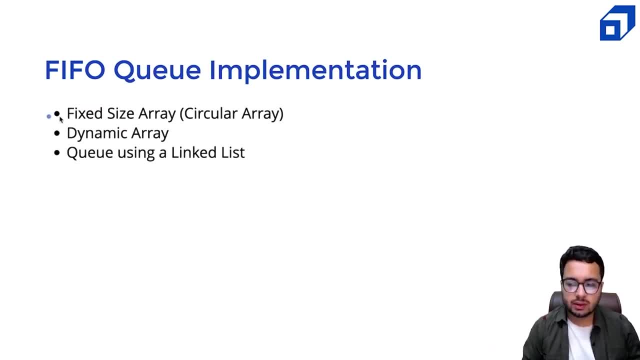 FIPO queue- right, so there are three common ways to implement a queue. we can use a fixed size array- right, and we will see how this array will behave as a circular array when we are going to implement it. okay, so in this case, uh queue will have a limited capacity because the array size is fixed. 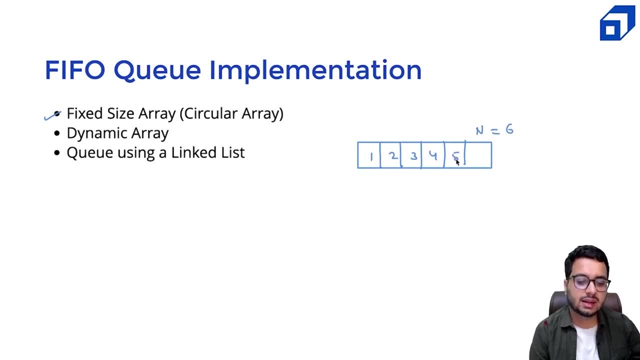 suppose n is six, so i cannot have more than six elements in this queue at any given point. right second is: i can use a dynamic array. i can write my own logic for creating a dynamic array. for example, if my queue gets full, i will define i will double the array. 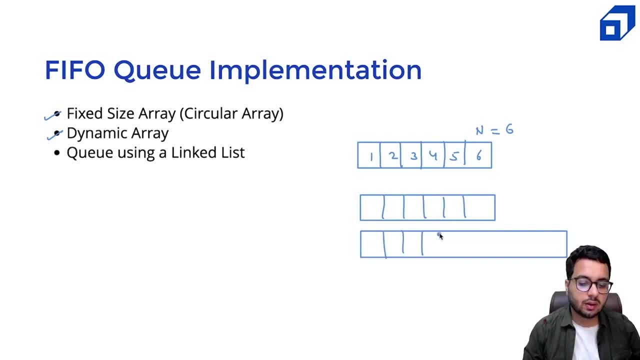 i will create a new array of double the capacity of the given size right now. if again the queue gets full, i will again do the same thing. right, this is called as implementation using a dynamic array. the other option is: if you do not want to write the functionality of doubling, it is already. implemented inside your queue, and when we're doing that, we use pointer which is called search可以上回到数ét r? svr. the other option is, if you are not wanting to write the functionality of doubling, it is already implemented inside your phone library. again, then we will use the keyword presented for finetuning to create new MH. 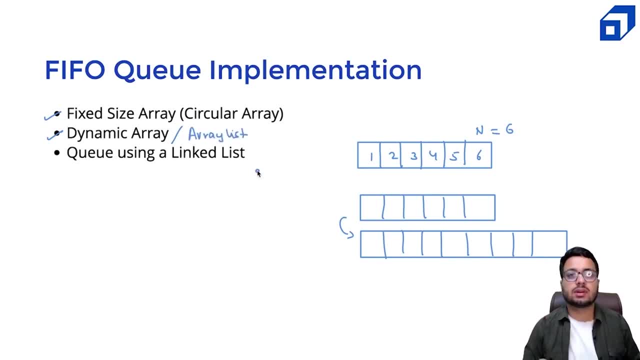 arraylist class. you can also implement queue using a arraylist, right? third is: we can use build a queue using linked list as well, right? you know, linked list is a dynamic data structure, so we will look at how a linked list can be used to implement a queue as well, right? so let us start. 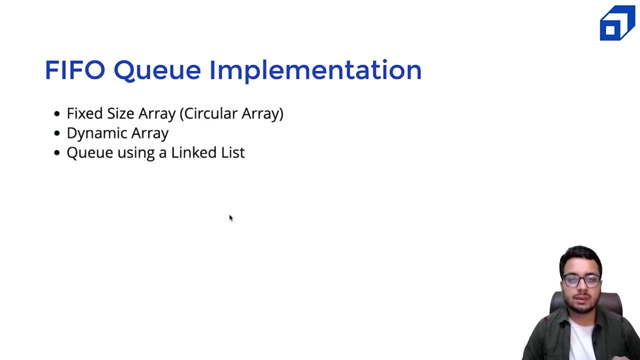 with the first implementation, that is, implementing a queue using fixed size array. now let us talk about how we can implement operations on a queue using a fixed size array. so the three operations that we need to build are nq, dq and peak. so nq. nq means i want to insert something into the queue. 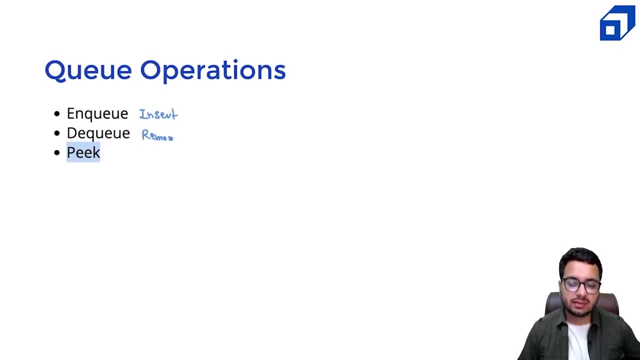 aq means i want to remove the element at the front and peak means i want to get the element at the front. these are the three things that we will have in a d4 queue. first in, first out. right now, let us see how we can use a fixed size array to create these operations on the queue right. 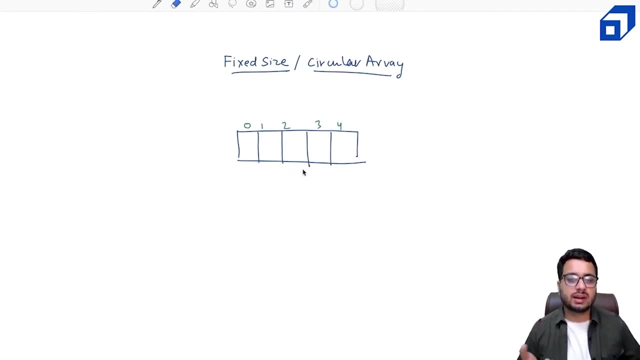 so in the beginning, i should know if something is coming, at what index i will insert it into the queue and at what index i will remove it from the queue. right, what i will do is: okay, let us take a variable called front, and it is here, right, we can. 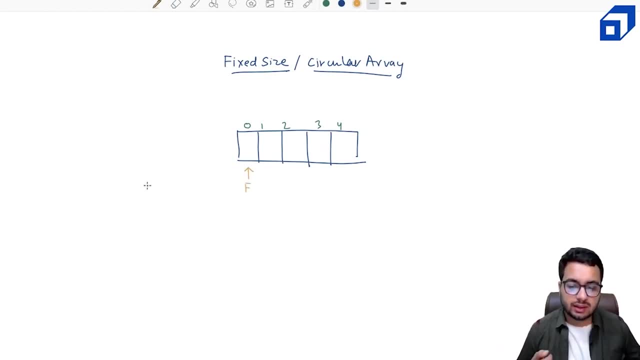 also take another variable rear, but again, that is optional if you are maintaining the size of the queue in the beginning. size is zero. front is also at zero. that means, um, nothing is inserted in the queue. yet right now someone says: okay, person, one is going to join the queue and i will insert it. 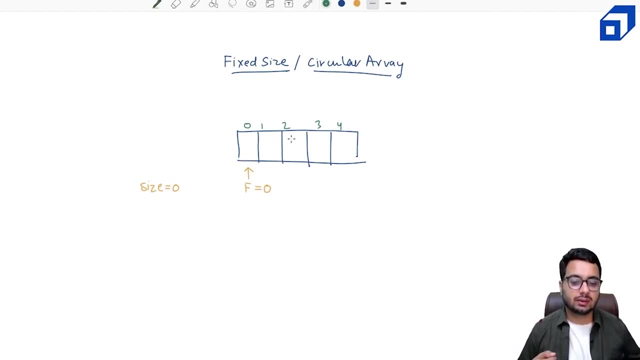 right, what i will do. i will insert it at the rear end. okay, so how do i compute the rear end? let's see, the rear end can be said as front plus size. i will tell you why, right. so what is front? front is zero. what is size? size is zero. so zero plus zero is zero. so i can insert person one here in the queue. 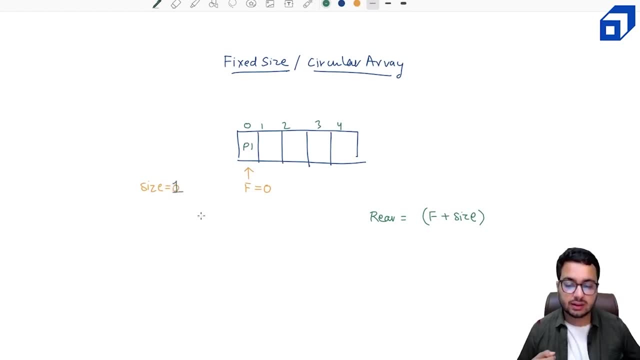 right and i will increment the size. the size will become one right size is going to become one right. so i'm not going to change the front. look carefully, i'm not going to change the front right now. uh, it was zero plus zero. that's fine. right now i can say again: i want to insert person two. okay, i want to insert person two at. 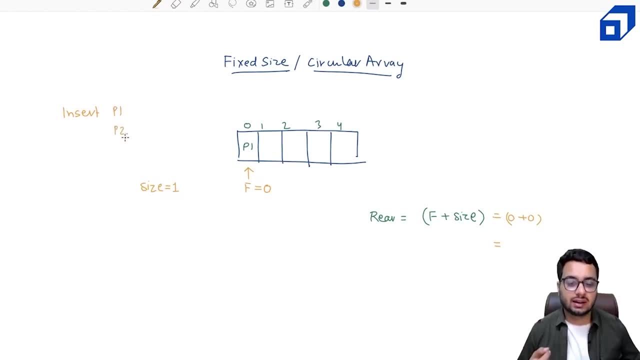 what index i will insert. i will insert it at the rear end, right. so what will be the rear my, what will be the rear value? now? it will be f plus size. so f is zero, fine, size is one. it is going to be one. i can insert person two at this index. very good, right now, let's say one more person wants to. 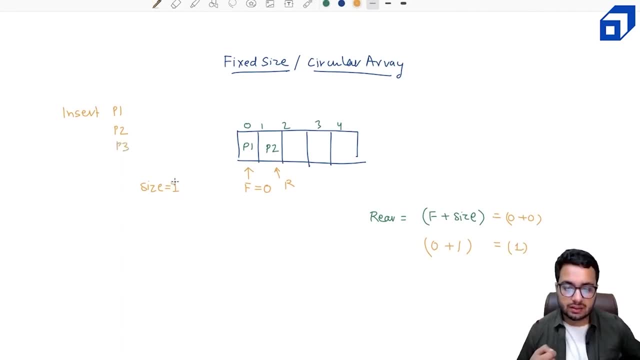 join the queue. so i want to insert person three. right size is already two, right, i've inserted two elements, but what index i will insert? i will insert it at the rear index. what will be the index? zero plus two. that is going to be two. that means person three will be inserted here and this. 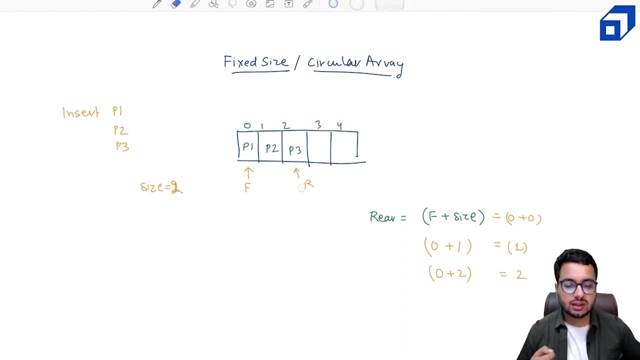 is the new rear, okay, so front is not changing, rear is changing. in this case, again, i want to insert person four. let's insert person four. so size is already three. now, right size is already three. so what will be the new index? zero plus three, it's going to be three. i can insert person four at this index and my rear is already. 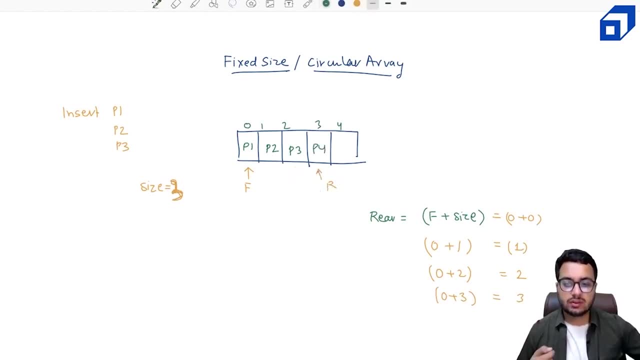 here right now. suppose i've done a lot of insertions. i want to remove something, right, so i have inserted till person four also, and i want to see how my front is going to change right now, suppose i want to remove something. i want to perform dq, right? so that means i got a query to remove the front element. 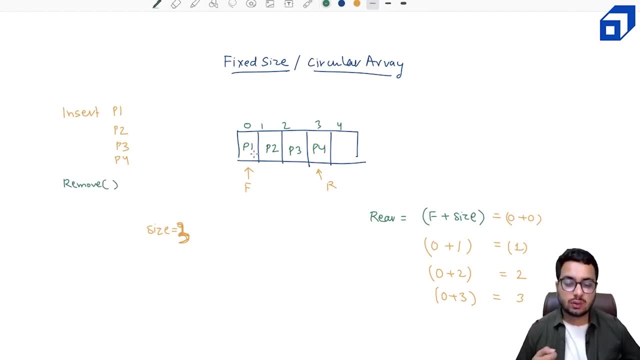 the front element will get removed right now. how do i remove it? if i move this f one step forward and i will have to reduce the size. right now the size was four because four elements are there in the queue right. my size becomes four. from four it becomes three and i say, okay, f should move one step ahead. so 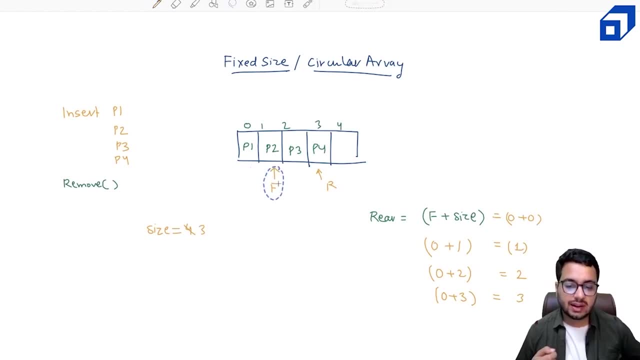 it's okay, i'll take this front one step ahead. that means this p1 is- uh, it's kind of a- removed, it's not there, right. so the area between front and rear, it is the content of the q right now suppose i want to insert something more right. so what i will do, i'll again do um front which is at: 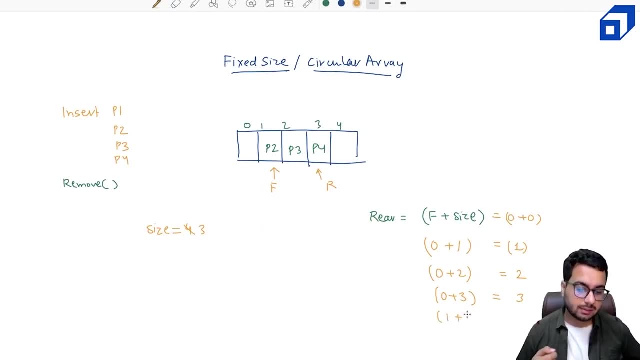 one, okay size, which is at three, look carefully. so one plus three, i get an index four. that means the next insertion will happen at this index. can i insert something? of course i can insert something, because q is not yet full. i insert something at this index right now. suppose i want to do one more insertion. 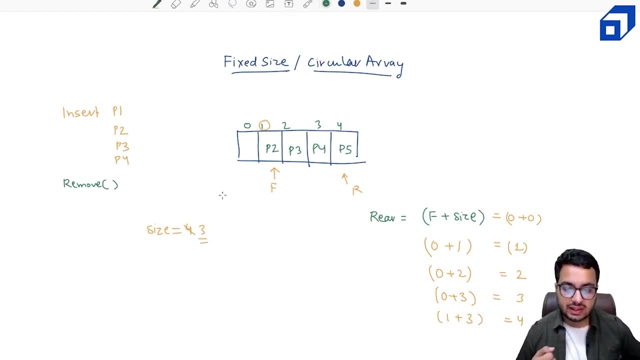 again, um, what is the value of size? now, size is still four, size is four, right. so what will we do? is the value of rear? so it will be front, which is one, plus rear, which is at uh, which is plus size, which is four, right, it is going to get five. now, is this five a valid index? is this five a valid index? 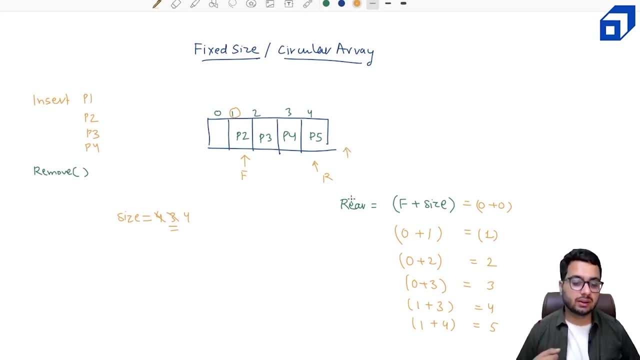 the answer is no. right now i will get a problem that if it, it will give me index out of bound exception, but q is not yet full. q is not yet full, so how should i handle this case? right, the way to handle this case is treating this array as a circular array. right? if you exceed four, you should come back to this index. 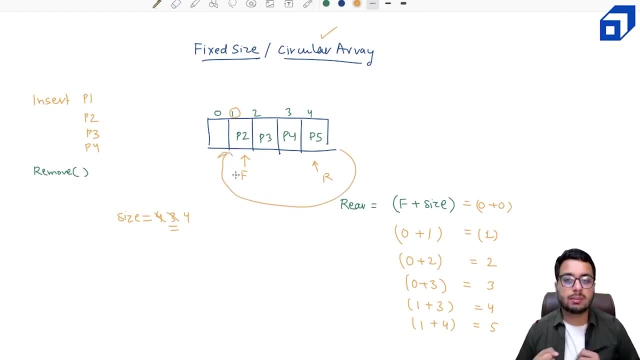 you should kind of rotate and you should, you should come back here right now. how do i achieve this? i have to say, take a mod with five. every time you hit a five, you go back to zero again. you start filling the queue from this index. now suppose i got this. uh, p5 i have already got. i want to insert. 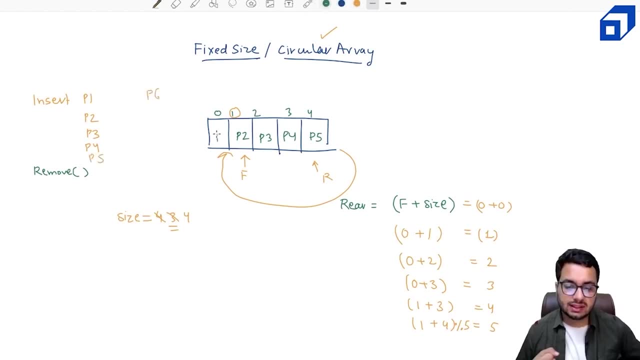 p6. this p6 will get inserted here. what i'm saying is the rear will not be updated using this formula. the rear will be updated by using front plus size mod of the capacity of the queue. the capacity is five right, so i have to take a mod with capacity. so that means if you hit the capacity, 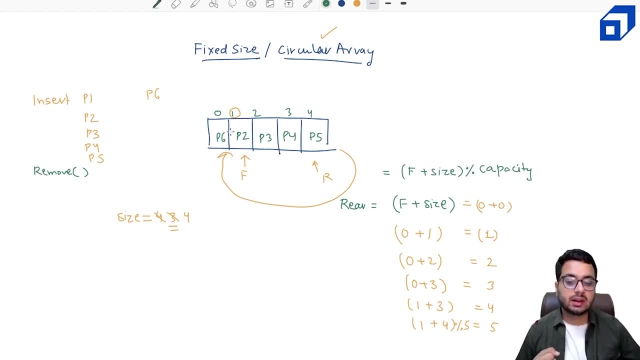 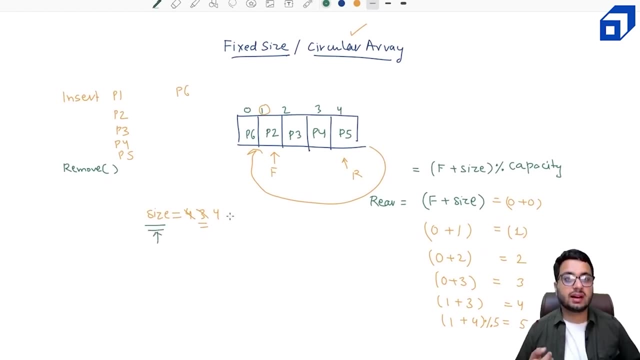 if the rear index hits its capacity, it will be again shifted back to zero. so why did? your? q is not full. you, you have to check that. okay, if my size is five and i have only four elements, right then i can add more. the size is five and i have already added. 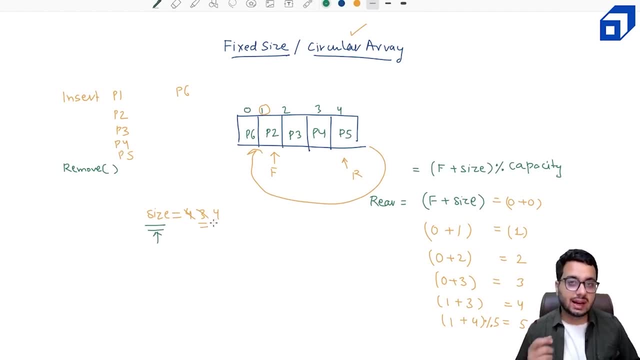 uh, if the capacity is five and the size is also five, in that case i will throw that the q is full. i cannot insert anything more, right, so i will insert it here right now. my front is still at p2, right front is still at v2, but my rear is here, right? 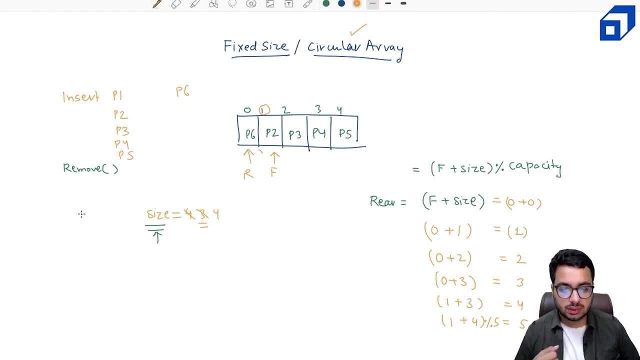 now someone says, okay, i want to remove something. or let's say, i want to insert something right now. what is the size? the size is five. can i insert something more? the answer is no right. so what? you will check that if your size is equal to the maximum capacity that we have allocated, i cannot. 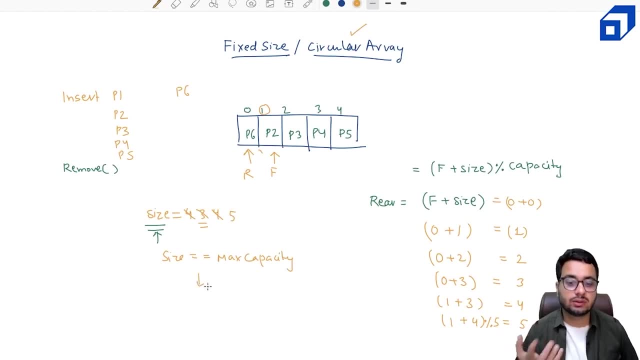 insert anything into the queue so i have to throw some kind of error. that queue is full, right. now again, let's say i want to insert, uh, perform the remove operation, right, so how, i will do it as a fine, i'll move this front from here to here, i will reduce down the size from five to four and 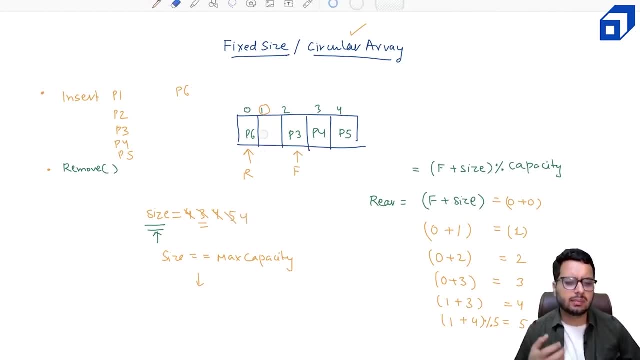 this makes that p2 is not there, right? so p2 is not there. i'll either make it zero or i'll just keep keep it like this. right now i can insert something. right, i want to insert something. so what is my front? front is at two. what is my rear? i'm sorry, what is my size? the size is five, so two plus five. 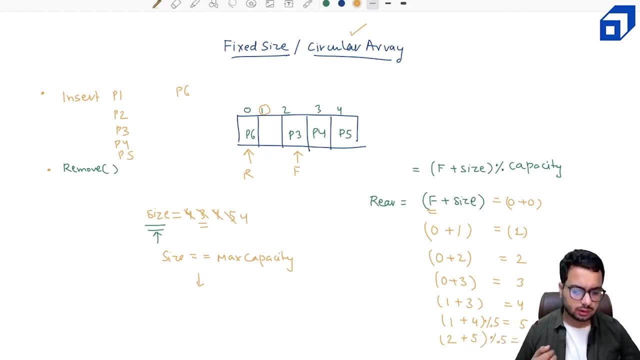 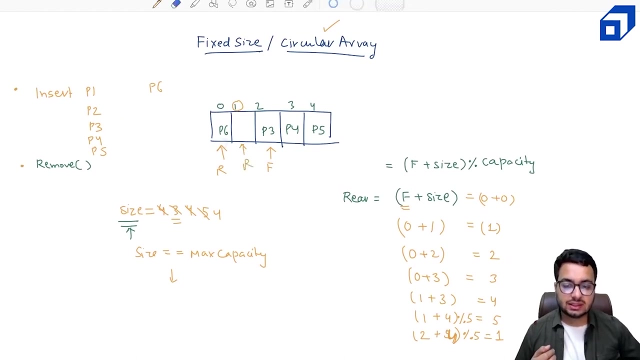 mod five, it gives me two. oh sorry, the size is actually four. the size is four. so two plus four, that is six mod five. it gives me one. two plus four mod five, it's one. that means the rear should come here and the next insertion will happen at this index. so if p7 comes, that person 7 will be stored. 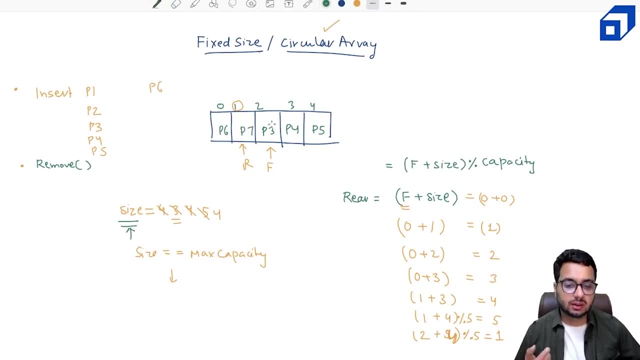 at this place again. if you want to remove something, you will remove from the front. so the front is p3. you will read the elements in this order right. the elements will be removed in this order right. one thing you have to notice when you're moving your front right. 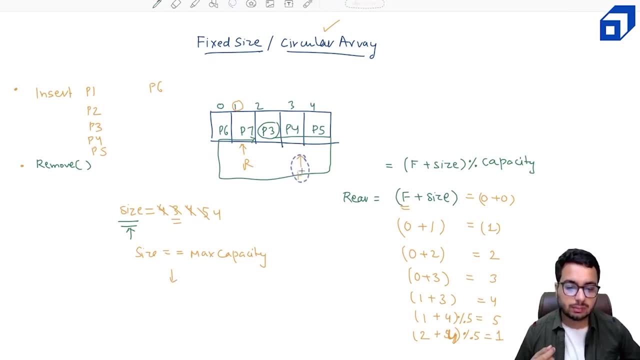 your front will also go like this: it will go to p3, p4, p5 and again it should come here- p6, p7, right? basically, what i'm trying to say is that when, when you're doing this operation, that uh front will move like f, equal to f plus one. right here also we should do mod with the. 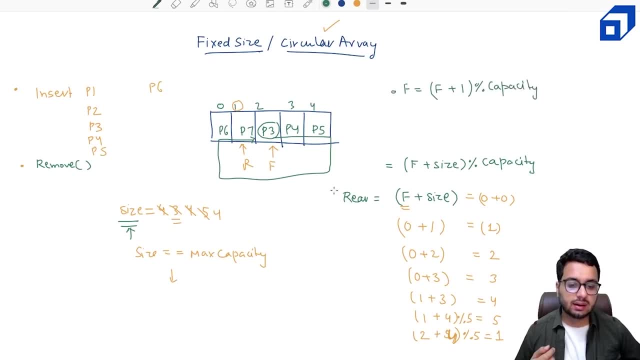 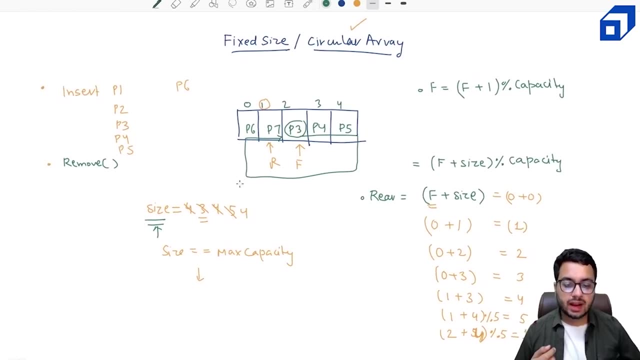 opacity. try to read the different outputs, all thegs, so that my both front and rear move in a circular fashion inside there, right at any given point, right? um, i have to check. if the queue is full, i cannot insert something. if the queue is empty, i cannot remove something, right? 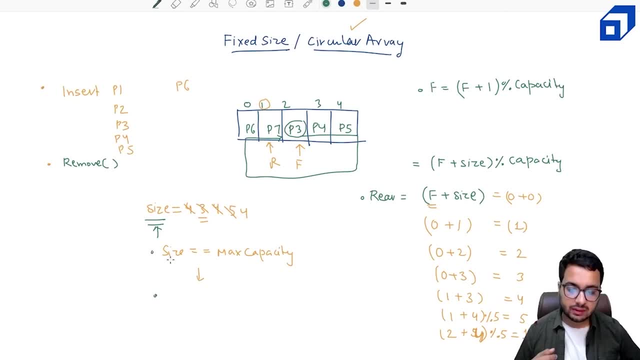 so we have to handle two cases: that if size equal to maximum capacity i cannot insert, and if the size is zero i cannot remove. right, so that is lose capacity, ofending the ofending the voyages, for that matter. its not change right. and so i have to handle two cases: that if size equals max capacity i cannot insert, and if the size is zero i cannot remove. 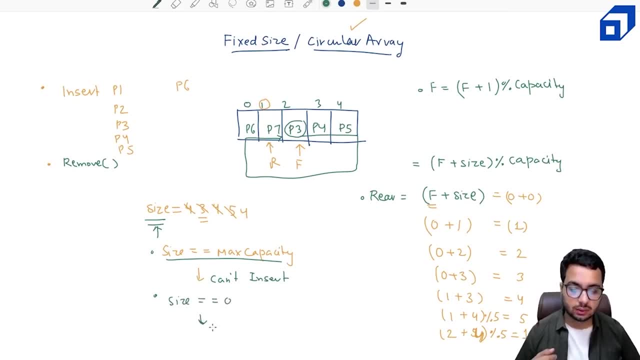 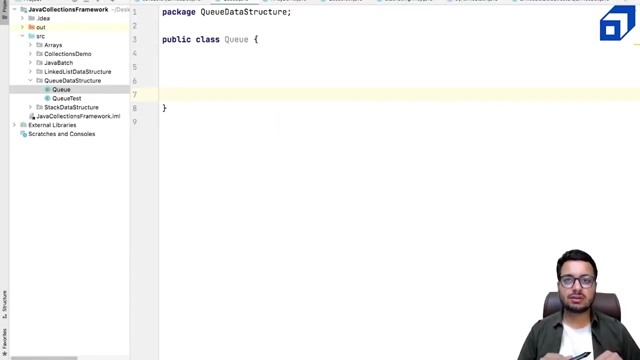 if the size is zero, i cannot remove, right, So these will become our special cases in the code. right, I cannot remove. I hope you understood the logic for the fixed size queue And now we will jump into the implementation. Let us start implementing queue using a fixed size array. I will be using Java, but you. 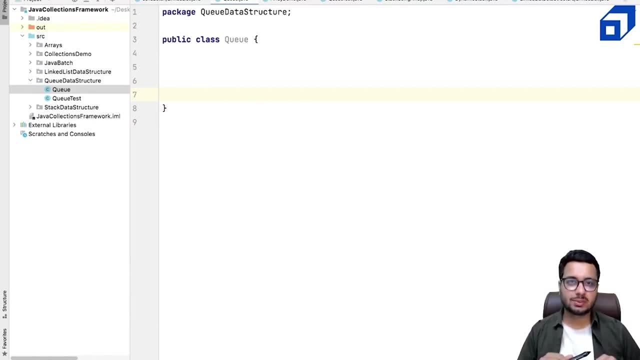 can use any language of your choice for the implementation. Let's begin. The first thing I will need to do is I need to create a class queue And I need to define few data members, As we have discussed earlier that, if you're using a fixed size array, we will need object. 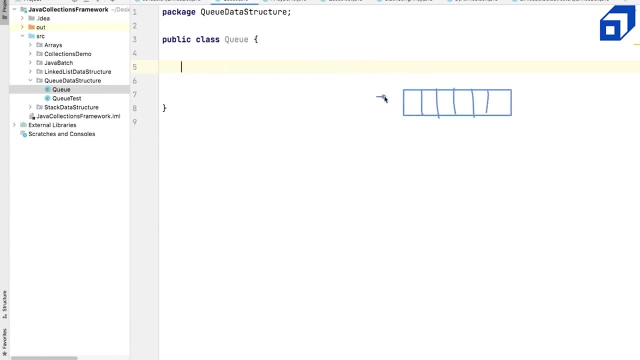 reference to store this array, right? So you can call it anything, I am just going to call it as ARR, right? So let's create this variable data member. so I will say private. it's an integer array And I need to define what is the maximum capacity of this queue, right? 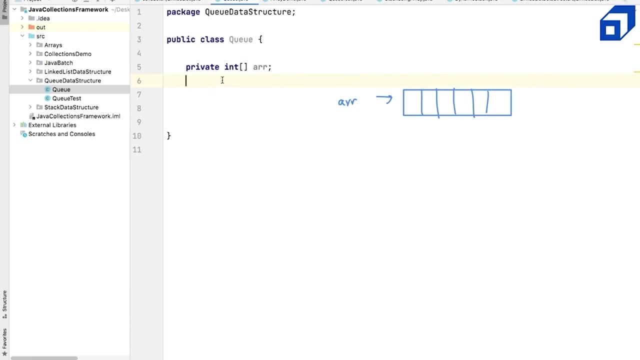 So that I will define using a constant. because I'm taking a fixed size array, I will say: okay, fine, Constant will be a public static final int called as default capacity, and this is equal to 10.. One thing: I need to notice: that if someone is inserting data into this queue, what is? 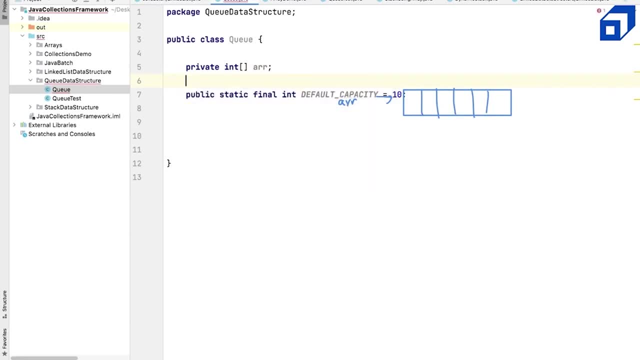 the current size of the queue. So I will take another private variable to denote the size of the queue. right now, in order to perform operations like insertion and deletion, I must know the front of the queue. So I'll create A variable that is private int, and I call it as front right. 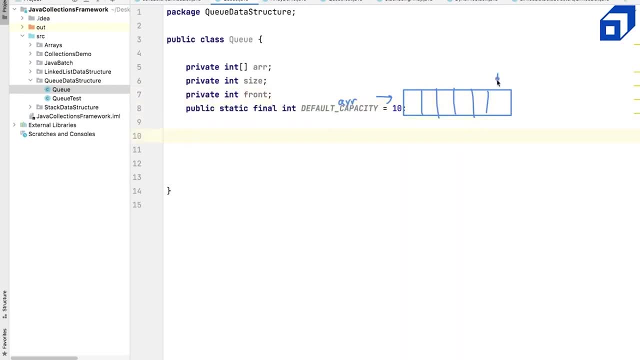 These are the four data members that we will need. So one is your capacity. let's say that is 10, then there is your front, which is initially at zero, and there is size, which is, which will be also at zero, right? 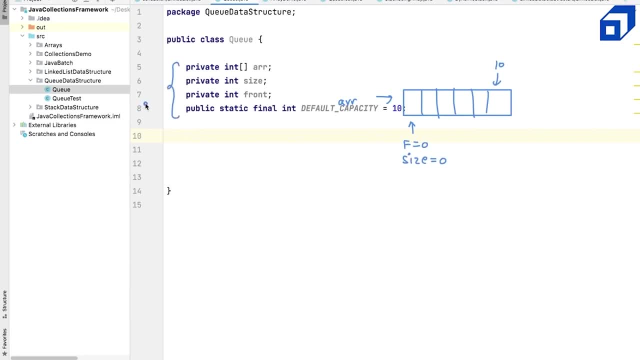 Now we need to initialize these data members. So that part we will do in the constructor for the queue right. So I'll define: let's create a constructor and in this constructor I'm going to, I'm going to create a queue right. 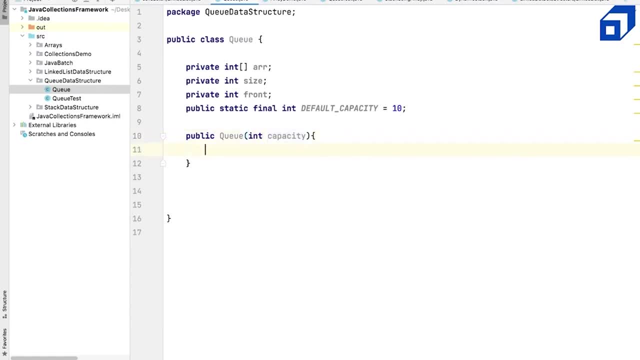 So maybe I'm going to get some capacity as input, right? If nothing is given, I will use the default capacity. So I'll create actually two constructors: One is the parameterized accepting capacity and other one does not accept any capacity from the user. 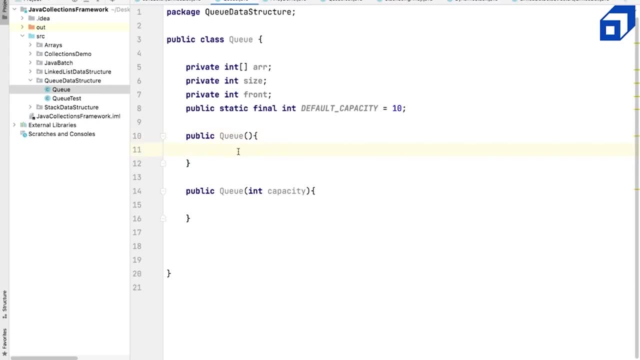 So in this case, we will use the default capacity. So one thing we can do is: uh, from this constructor, we can directly call this and we can talk a fine. So you can call this contractor and give default capacity as a parameter to it, right? 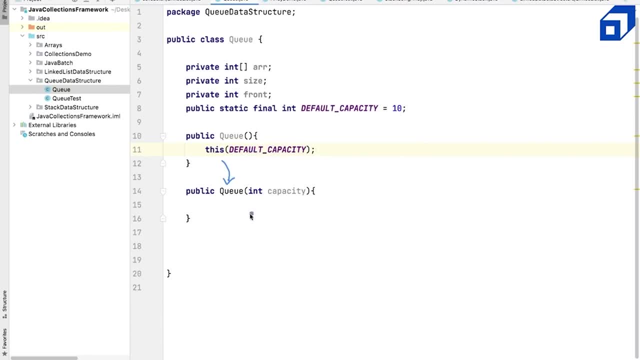 So that will help me to avoid creating an area here, and that part I can do directly here. right, Let's see how we can do it Now. if my capacity is less than one, if someone gives a wrong argument, maybe a negative capacity, 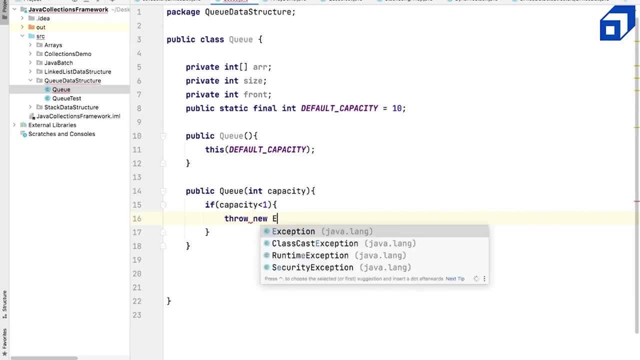 In that case my code should throw an exception. so I can say: no new exception, that, uh, invalid capacity. You are giving it to me, right. And also we need to define that this throws an exception, right? All right, Now let's do the actual work. 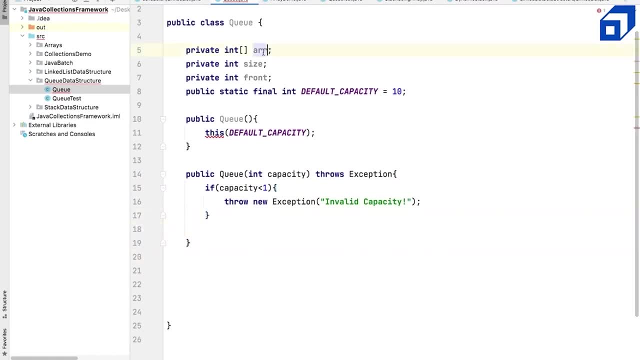 The actual work is that we need to initialize this area and try, need to say that fine, This area, that I have right. So again, I'm using this um, which is optional here, but, uh, it's a good thing to do because 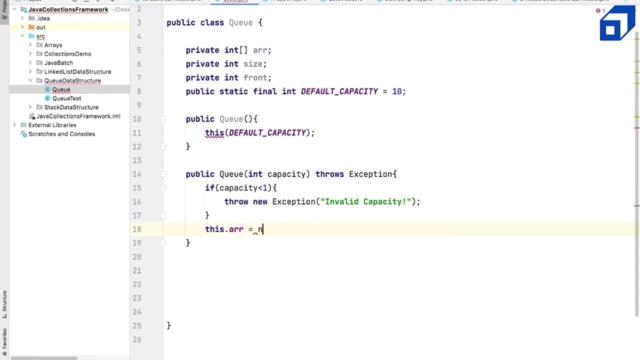 you are clearly referring to the data. member of the client. So this dot area should be a new area of capacity right Now. this capacity can come, as an argument, from the user directly, or if the user does not give, then this contractor will be called and this capacity will come from here, right? 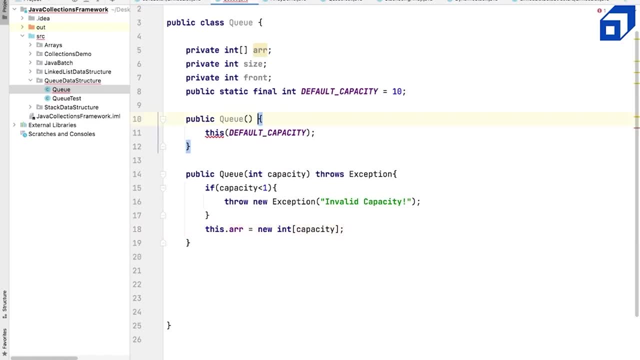 That will be your 10, right. And here also, we need to say that this method can also throw an exception. So this is how we have initialized our area. Now we need to initialize the size and the front variable. Okay, So initializing them is pretty easy. 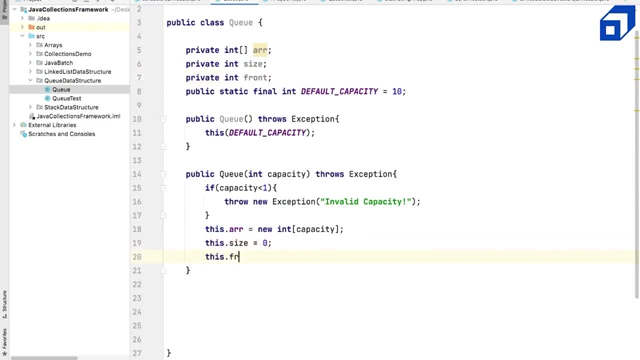 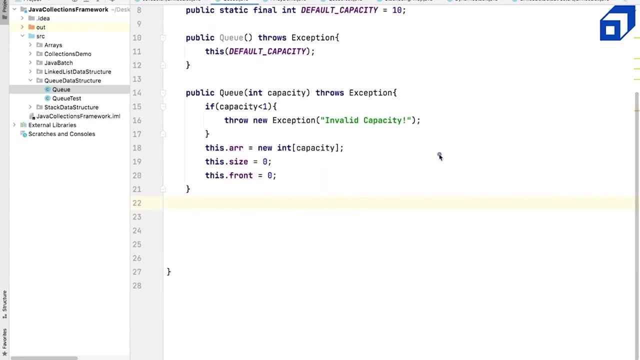 So I can see this dot size- It is a zero, and this dot front- that is also zero, right? So I hope this is clear. So we have created a new queue of given capacity. It can be fixed. size, It can be, uh, given by the user as well, right? 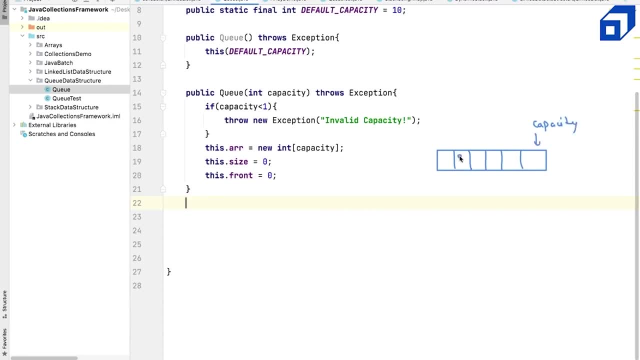 So we have a capacity. right, It's a capacity in this case is one, two, three, four, five, six. So capacity is six, Front is zero and is referring here, And the current size of the queue is also. you know the queue has been initialized correctly. 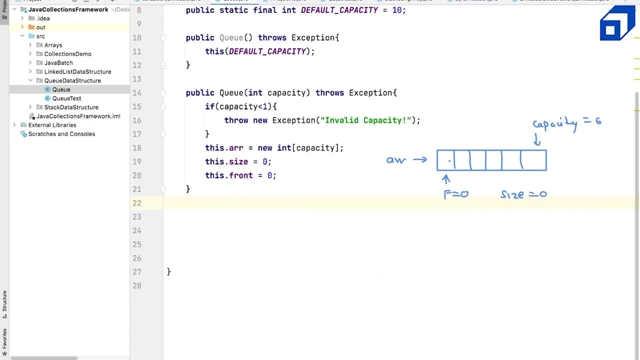 Now the next operation that we need to build on this queue is NQ. I want to push something into it So I can say: public void NQ and I'm going to get um some data or value to add into this queue. 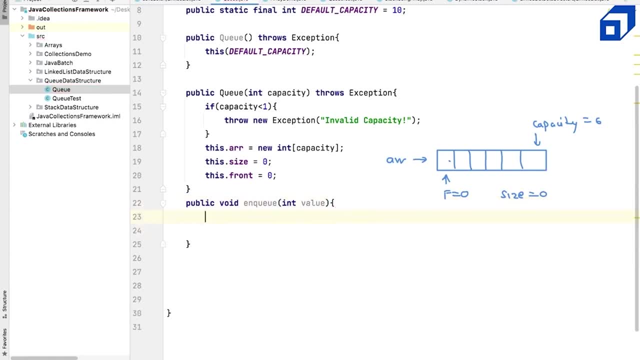 Now, since it is a fixed size queue and it is possible that queue is already full. So how do I check if the queue is full? I can simply say that, fine, If the current size, if this dot size, that is my data member, it is equal to the capacity. 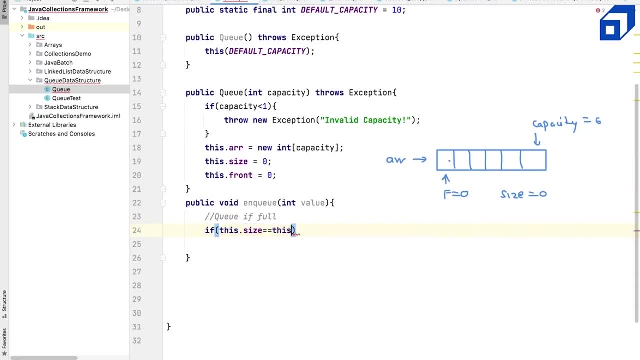 of the queue. So what is the capacity This dot array, dot length, length of the given array? Then I can say through new exception that my queue is, And here I can say that this method also throws a exception. but if the queue is not full we can insert. 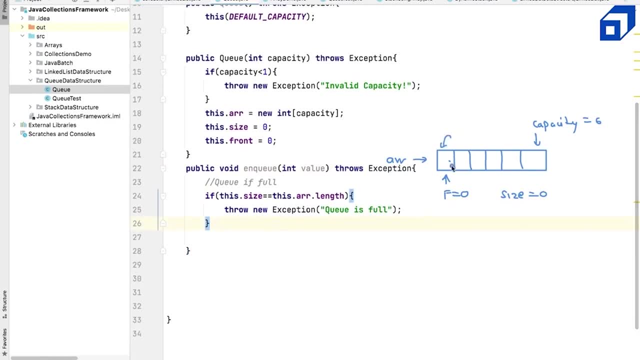 it right. So if the queue is not full we can say, okay, fine, we will push something at a rear index. So we will need to compute that rear index and see how we can compute that. So I can say the rear index according to the formula is the front index plus the size. 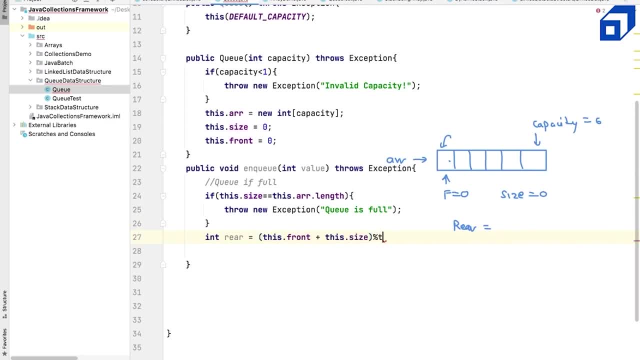 And then we have to take the mod with the capacity, So that capacity is nothing But this dot array, dot length. that is the capacity. Now, in this case we will be zero plus zero. mod with six. in that case it will be zero. 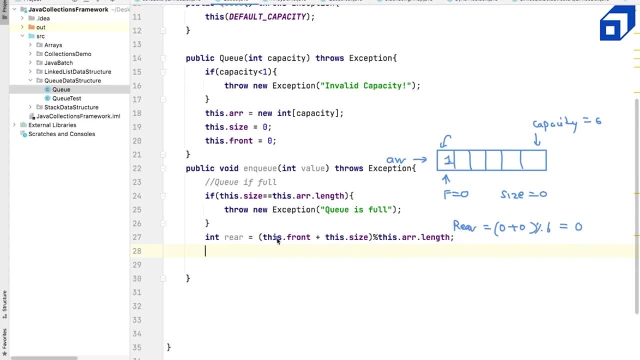 So I will insert something here, and then again, size will also increment, So we will put the data, So we'll say this dot array- at the rear index. I want to put the value, I'm storing one and I need to upgrade the size. 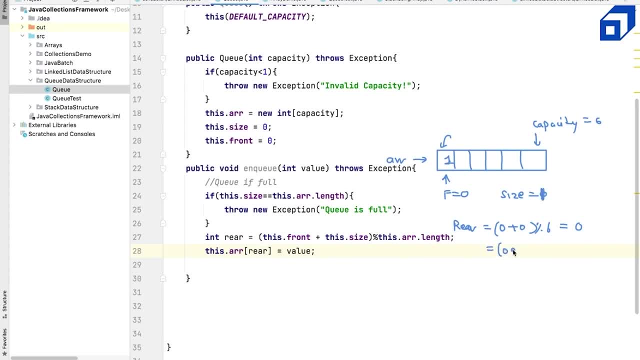 I need to say: the size is now one, So. So next time the rear would be zero plus one mod six. Next time the insertion will happen here. Maybe I push two, So I'll do the insertion at this index. In order to achieve that, I have to say this: dot: size plus, plus. so I need to increment. 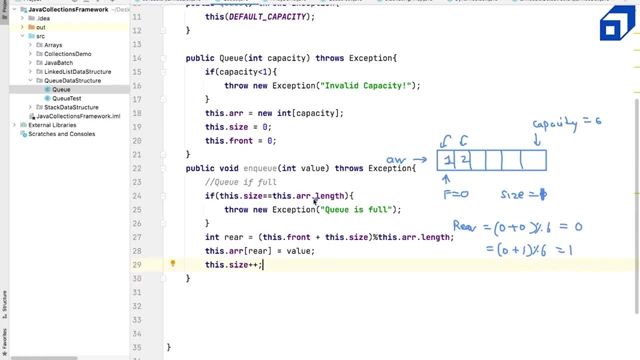 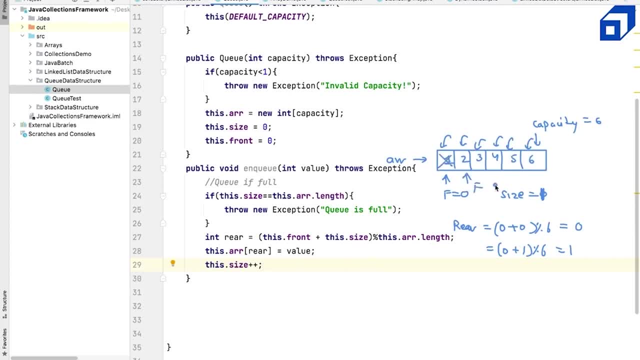 So It gets removed. So your F will come here. right, Let us look at the remove method as well. In that case, you can call the method as a public. Now, either you can make it as void or you can make it as int. 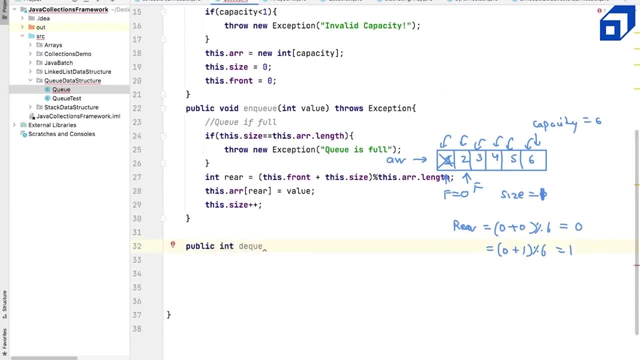 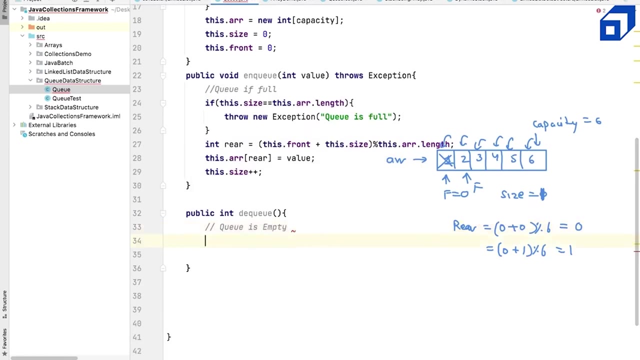 So you also want to return what has been extracted from the queue, Right? So in that case you can make the return type as int. Now this method can also throw an exception. If your size is zero, That means queue is empty. You cannot remove anything from this queue. 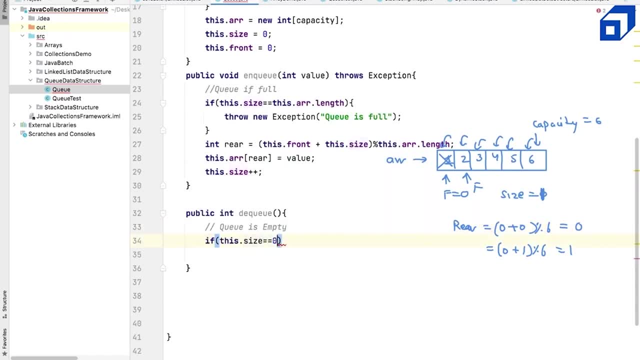 If this dot size is zero, what you should do, you will say, okay, throw new exception, that queue is empty. But if this is not the case, I can say, throws new exception here. sorry, throws exception. But if this is not the case, what we discussed, what we will do, right, so we will store. maybe. 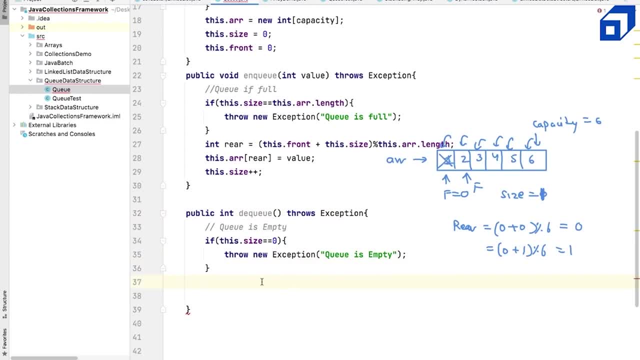 this data. one will store this one here against. okay, our output. the answer that we want to return is present at this dot array of front or this dot front, whatever. So you can definitely return this answer, but you have to update your front and you. 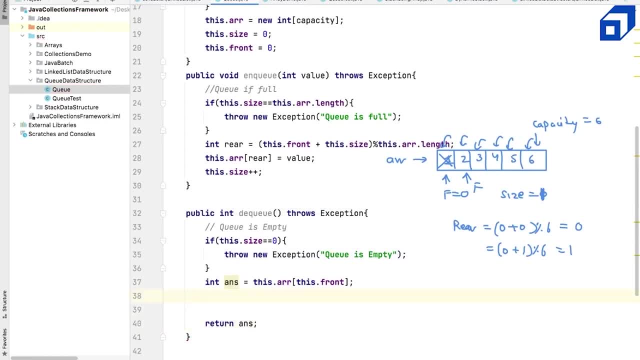 have to update your size as well. Right, So you will find this dot front will move. this dot front equal to this dot front plus one mod capacity. So capacity is this dot array, dot length and the size will reduce this dot size minus one. 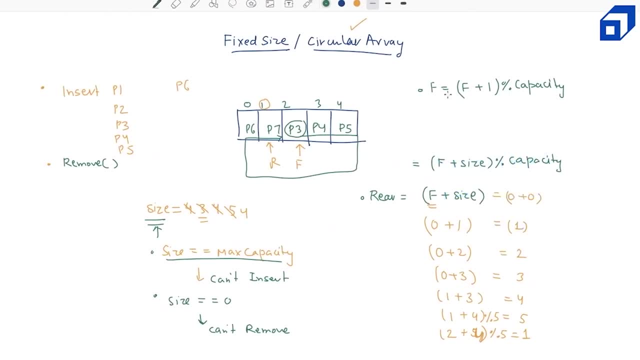 If you remember from the diagram, this is what we discussed earlier also- that this is how my front will change in case of removal right. Okay, And this is how I will compute rear In the case of insertion right. We have already discussed how it's going to work. 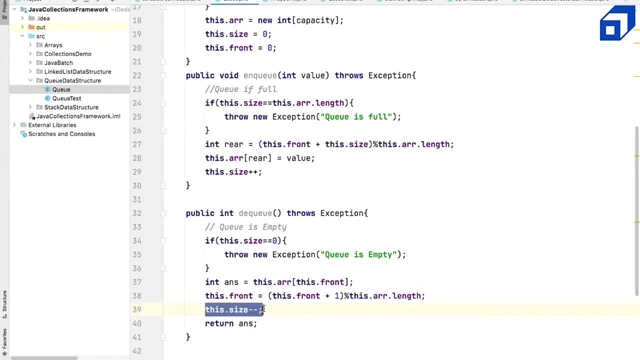 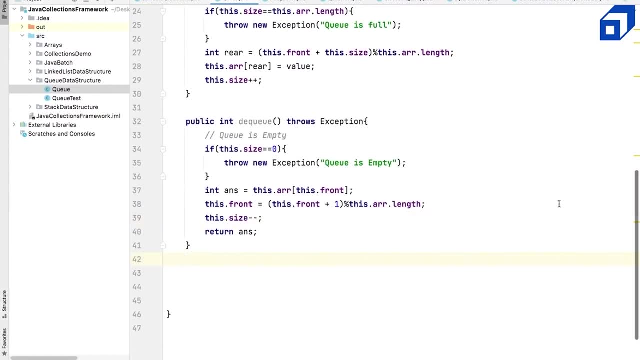 So I'm changing the front and I'm changing the size as well. This is my DQ method right Now. let us write some more methods that would be helpful. So one method would be peak. If I want to look at the front element, I can define public int peak. 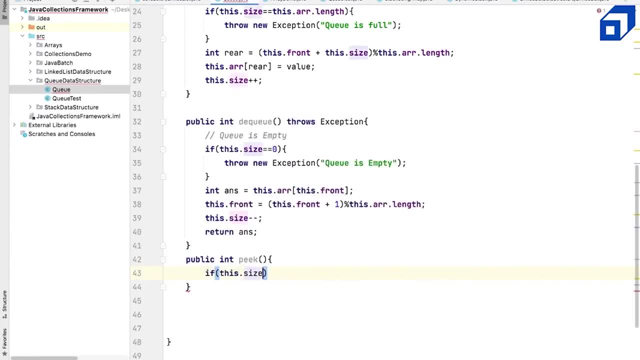 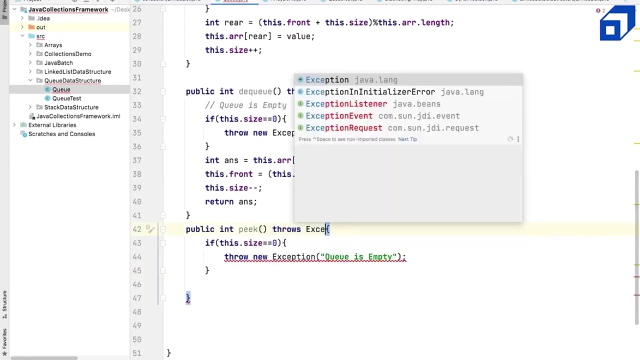 If, again, the queue is empty, I cannot look at the front element. So if this dot size is zero, Okay, So I can say fine, um, so, new exception: the queue is empty. You is empty. That means I cannot remove anything from this queue, otherwise. okay, let's just fix the. 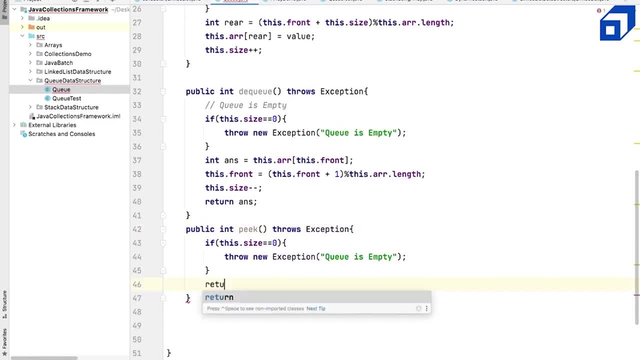 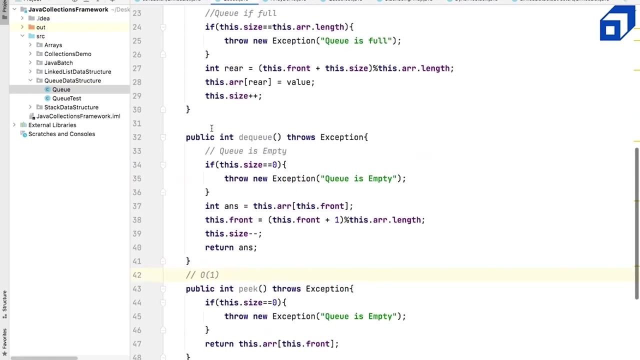 error. Otherwise I can say: return the front element, this dot array of the index, which is this dot front. Okay, That, that is my peak method: Return the front element. So the complexity of this method would be order one here also DQ method. 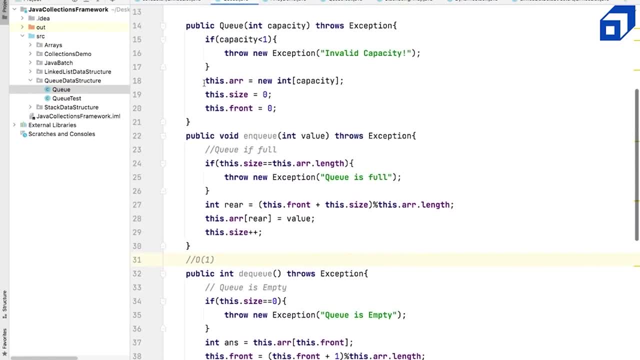 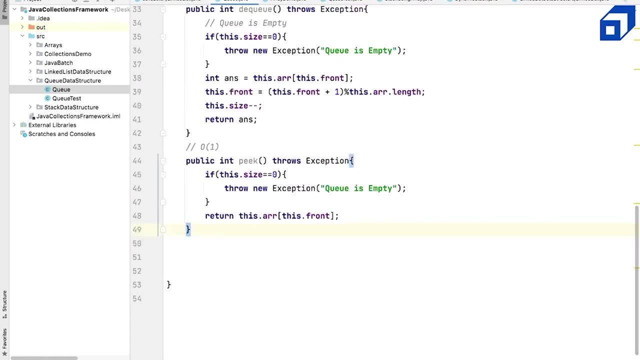 It will be also order one, the insert method. that is also going to be order one. The constructors are also order one part from it. We can make two, three more methods. One is to check if the queue is empty or not. That can be a Boolean method. 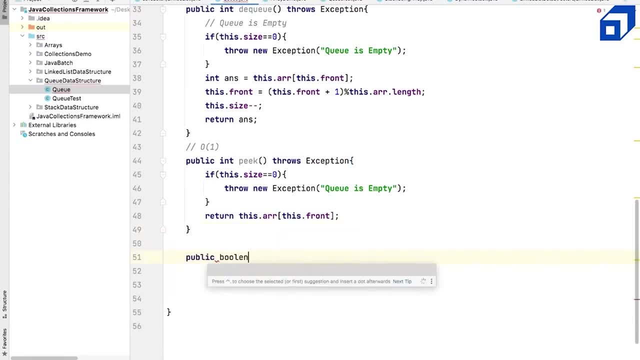 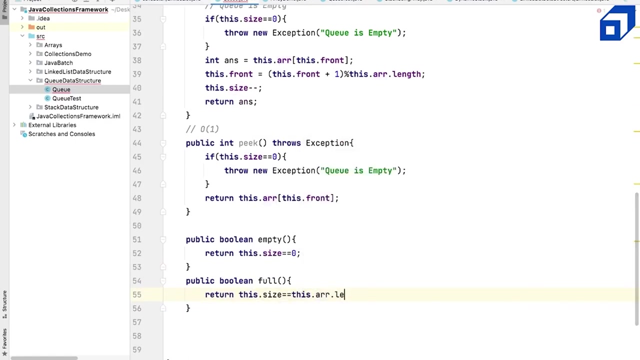 I can say Public Boolean is empty or just empty. right, I can return. true, If this dot size is equal to zero, I can make a method called public Boolean full, so I can return if this dot size equals this dot array, dot length. okay, that will tell me if the 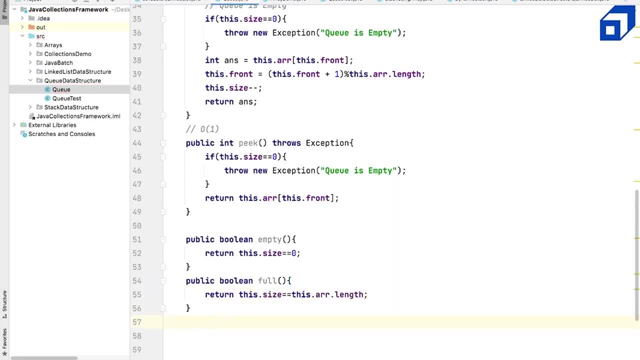 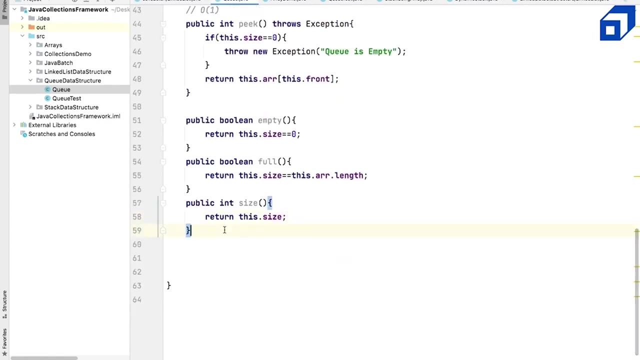 queue is full. What else I can also make a method to get the size, public int size. I can return this dot size from this method. Anything else that you think would be helpful? Maybe just a method to print the entire queue, right? 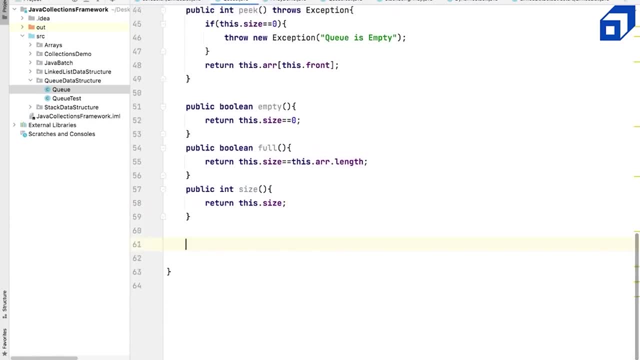 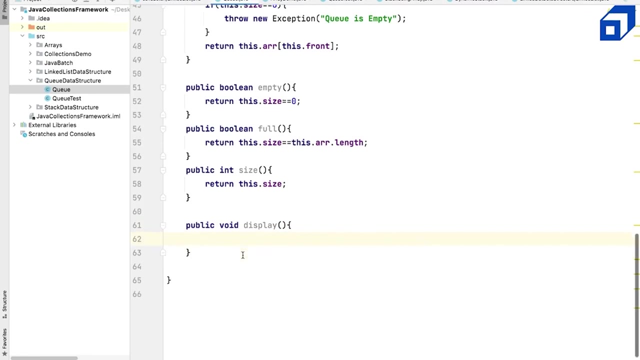 So maybe I want to display the entire queue right In Java, this method is called as two string, which is present in the default class. I need a way to look at- Okay, All the elements of the queue, right. So right now I'm not going to iterate from front to rear. 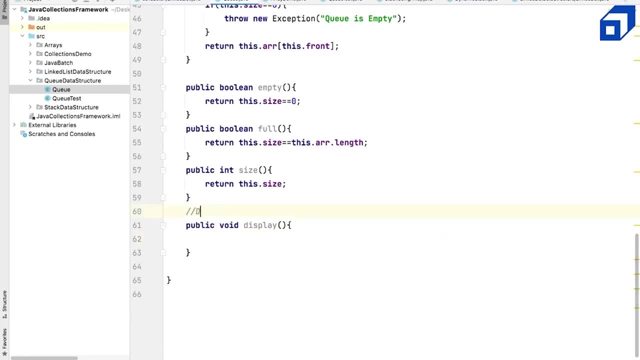 I will just display the array, So it's more of a method for debugging, not for doing anything else. Okay, I'm just going to print my array, or we can say we can print one simple way you can do it As out: at is dot two string. 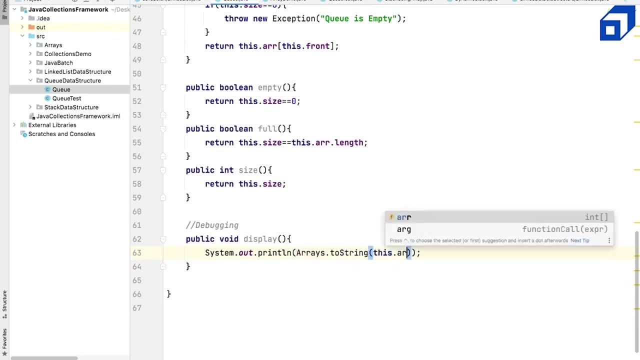 And you can do this dot error right. But now, instead of doing this, you can also say that fine, I would print elements from rear to front. Suppose this diagram is your queue, so maybe I want to print the elements from rear to 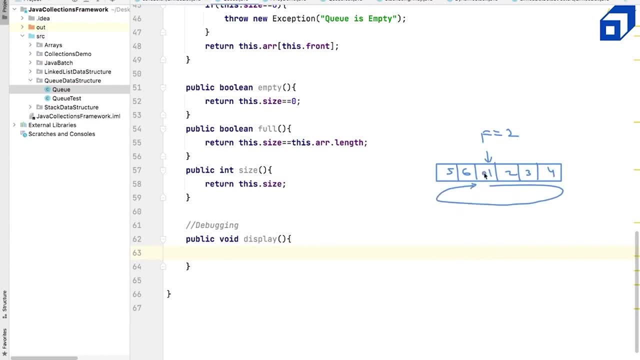 front, right or front to rear. So how I can do it right now, suppose if my friend is at two right. So I want to print, Let's say one, two, three, four, five, six. So I want to print all the elements from front to rear of the queue. 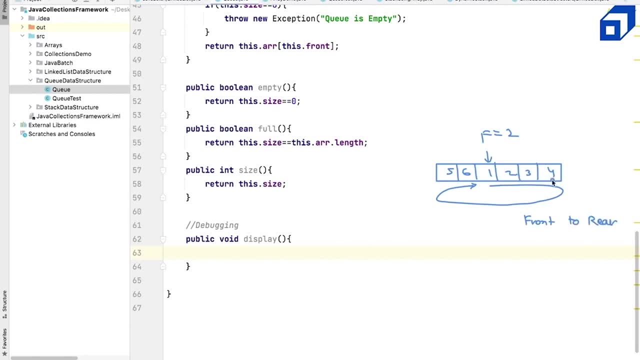 I want to display all these elements, So my output should be one, two, three, four, five, six. So how I can do it? very easy, I can. I know this index, I can compute this. I can compute this. 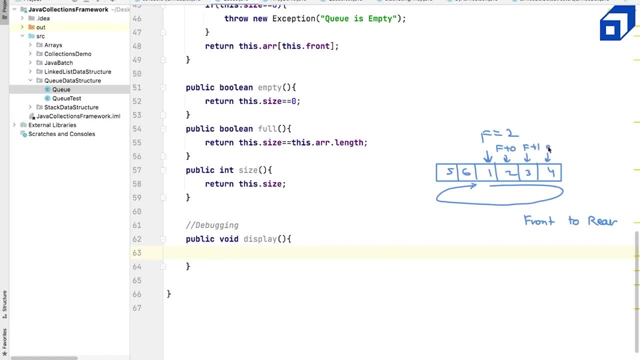 I can compute this. So this is F plus zero, This is F plus one. This is F plus two. This is F plus three. This is F plus four. right, And of course you have to take the mod so that you can rotate in this. 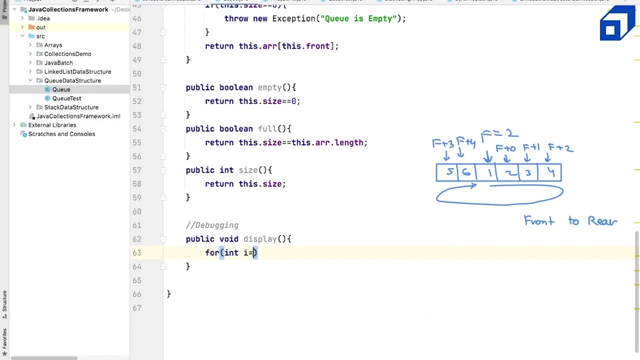 Circular fashion. So very easy. I can say, for hint, I equal to zero, I less than this dot size, And I can say, okay, the current element, the current index will be nothing but this dot front Plus. I take a mod with this dot capacity, that is array dot length. 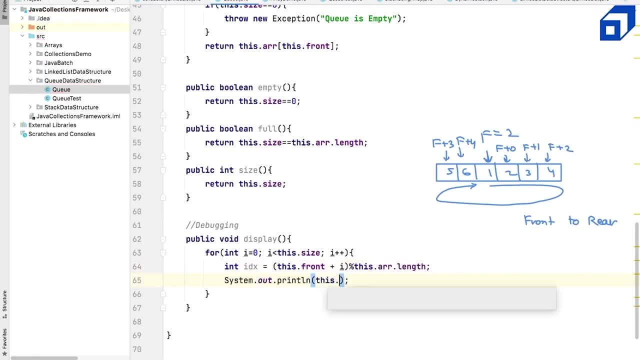 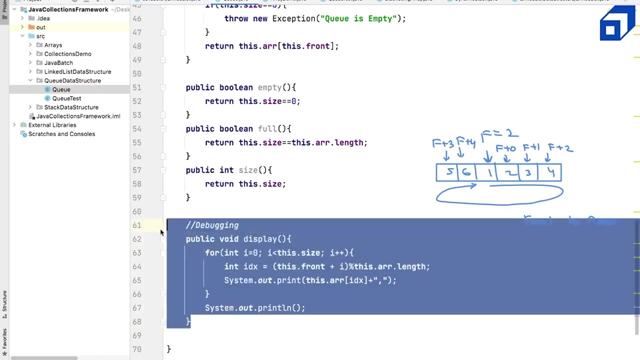 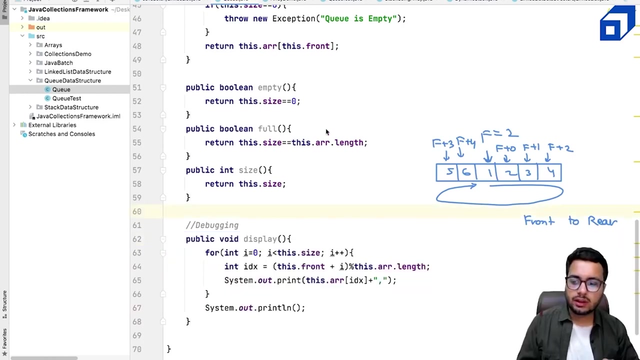 Now I can say S out that in elements of this dot Array of index followed by a comma, and S out, This looks good to go. This will print all the elements from front to rear. Now let us test our functionality in the queue test file. 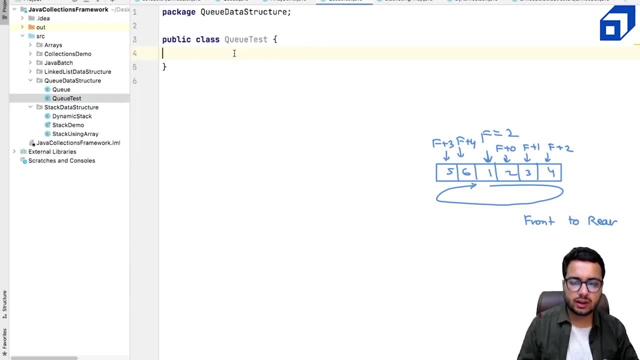 So we have created a queue test. So here what we need to do, we need to create a queue right, So we'll say PSVM. That is the main method. Now we can create a queue object to queue equal to new queue. 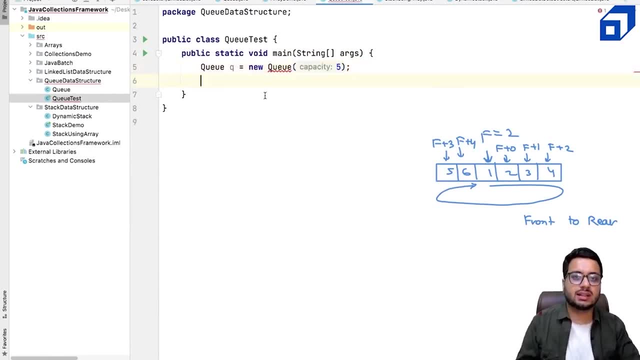 Let's say the capacity is five. Now I want to add certain elements to it, Those exception. right, We have to tell that main can also throw in exception here. Now, capacity is five, What do I do? I say, okay, fine. 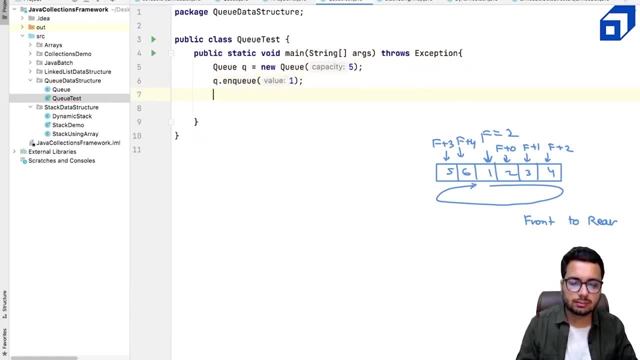 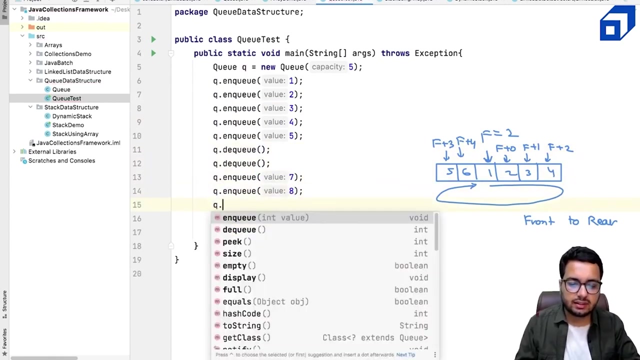 Let's push you dot NQ one. It's a two, three, four, five. Then I remove something. Let's say Q dot EQ, Q dot EQ, And then I can say seven and eight, And then I can say Q dot display right. 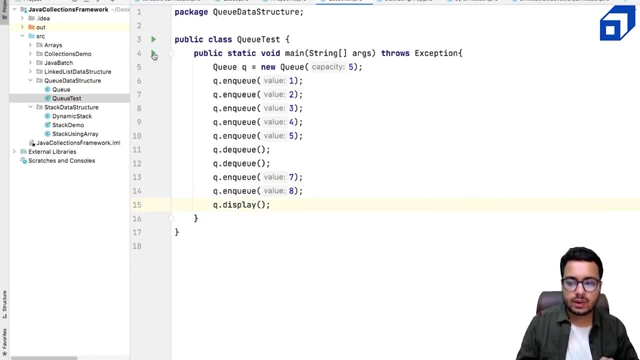 Now let's see how this queue should look like. Let's go and run the code. I inserted one, Two, One, Two, Three, Four, Five. The queue was full. Then I removed something right, So I removed this. 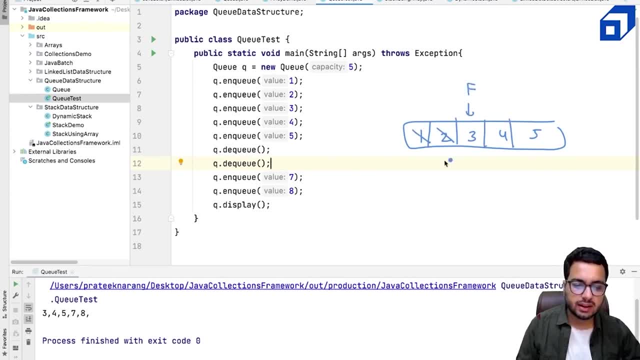 I removed this. My front is here, And then I NQ'd seven and eight. So seven and eight. they will come here, right? So if I now print my queue it should be like this: Three, four, five and seven, eight. 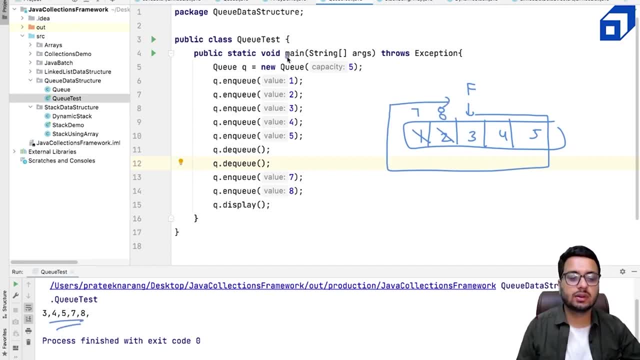 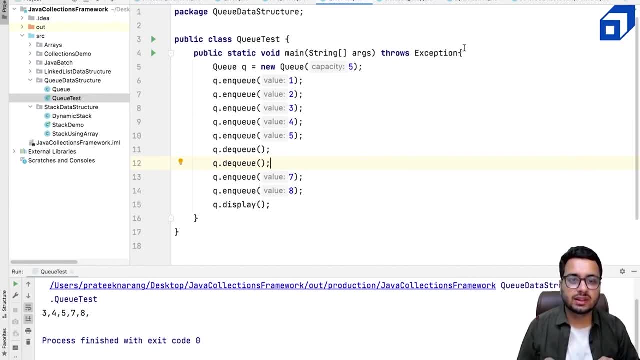 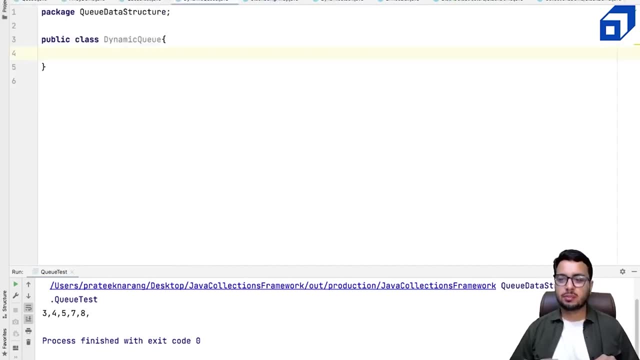 So I hope you understood the implementation of queue using a fixed size array. Next we will jump into the dynamic array implementation of the queue. Let us now discuss the implementation of a dynamic queue. right Now, there are two ways. One, you can use a link list, or you can use a dynamic array as well. right, 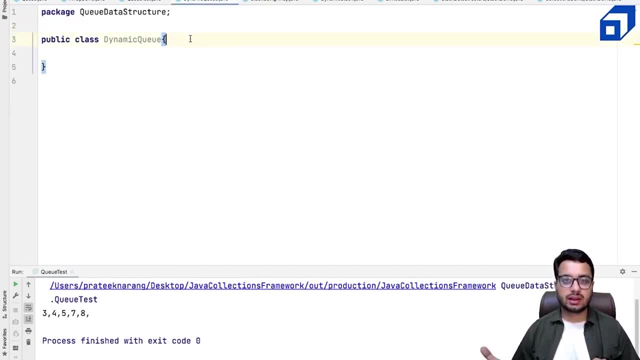 In this implementation, I'm going to show you how we can use a dynamic array functionality And we are going to extend The implementation of the queue class by adding this functionality. Okay, So queue. we have already written What I'm going to do. I'm going to create a class for dynamic queue, which will be the 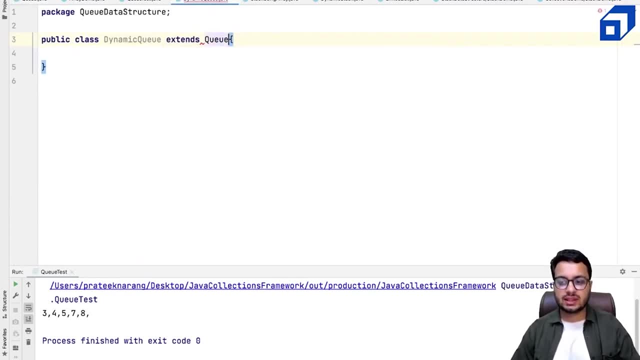 child class of the parent class. So dynamic queue extends the queue class right Now. one thing to notice that this dynamic queue, it's going to behave in a similar way. The operations NQ, DQ, P, they will remain same. 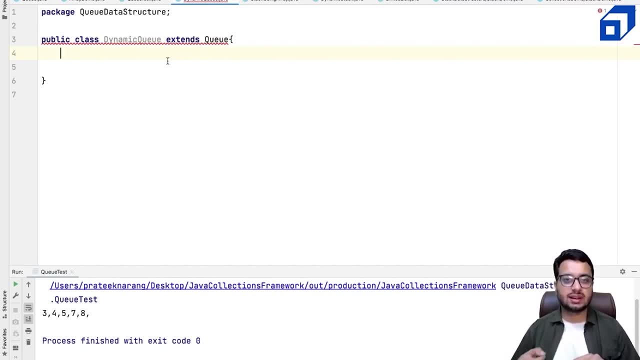 The only thing is the logic in the insertion operation, That is, NQ operation. It's going to change right. So first of all, let us start by creating the constructors for this class. So I can say public dynamic queue. Again, there can be two types of constructors. 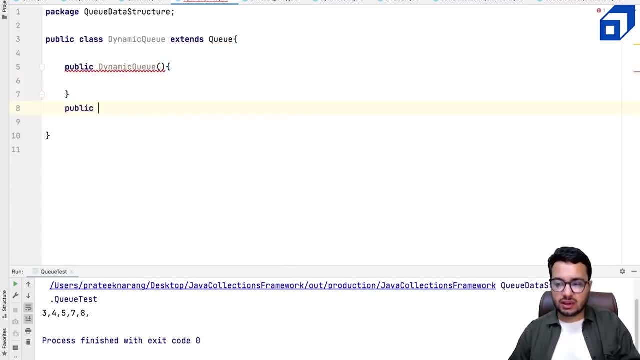 One without the capacity and one with the capacity right. So public dynamic queue where I'm going to accept some capacity right Now, in this case in the first constructor. what I'm going to do, I'm going to simply call the second constructor. 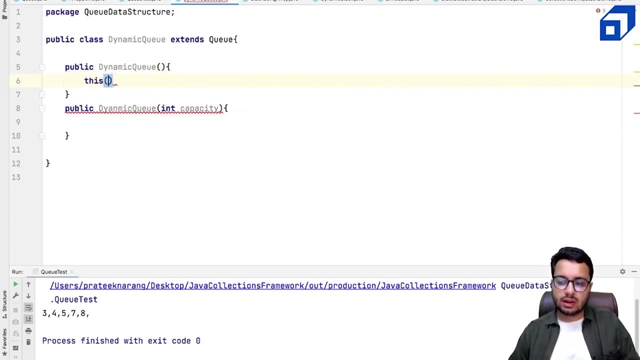 With default capacity. So I can say this and call it with the default capacity. Basically, what is happening: if I want to create a dynamic queue object in which I'm not getting any capacity, So I make a call here. If I get a call here, again what I can do. I already know how to create an array of given. 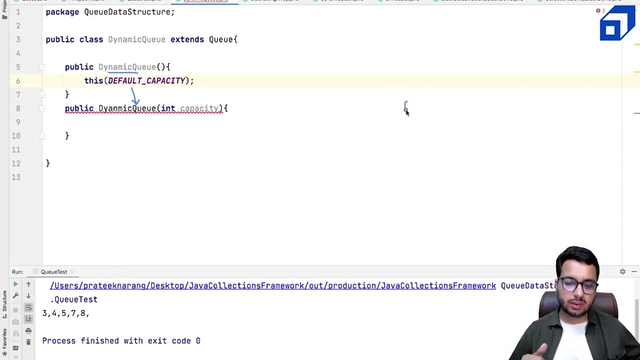 capacity that I'm doing in the parent class, right. So queue is my parent class, Dynamic Queue, Dynamic Queue is my child class If I want to create a fixed size array in both, if I get a call here to create a dynamic. 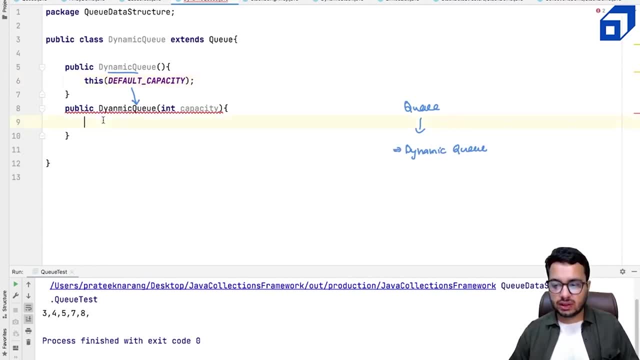 queue. I can redirect the call to the parent constructor So I can say super and I can pass in the given capacity. that I'm getting right. Basically, I'm calling the constructor of the parent class right Now. this is a spelling mistake. 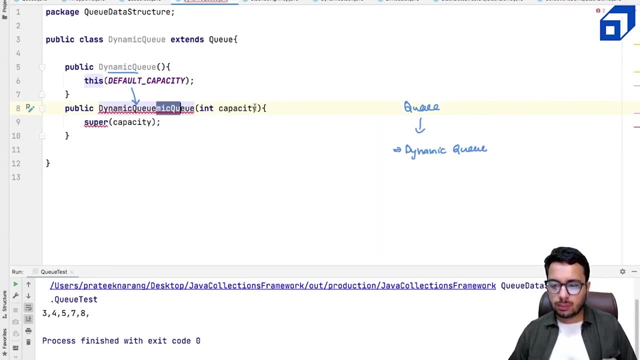 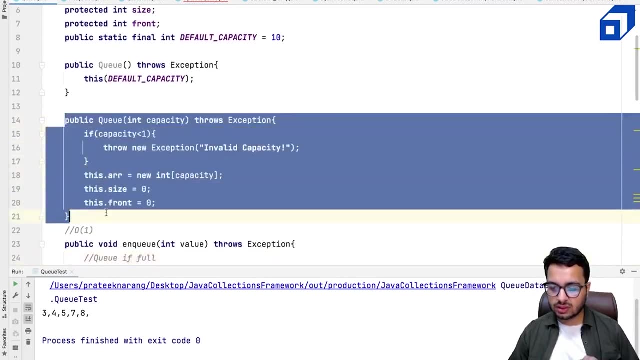 Dynamic queue. Now the parent class constructor, if you look carefully here, right. So basically what is happening? the call is going to come here to this constructor. So we are already initializing the array correctly. size is reset to zero, front is set to zero. 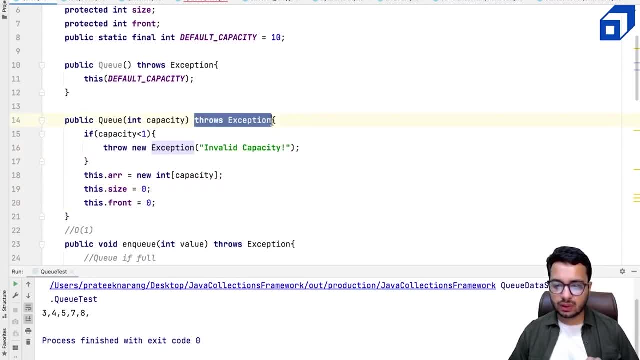 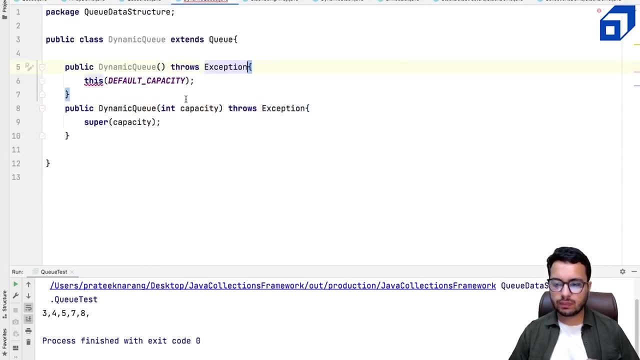 and we are also throwing the exception. We can also say that our dynamic queue can also throw an exception. This can also throw an exception. Now the errors are resolved Right. The constructor part is set. Now. there won't be any change in other methods except enqueue. 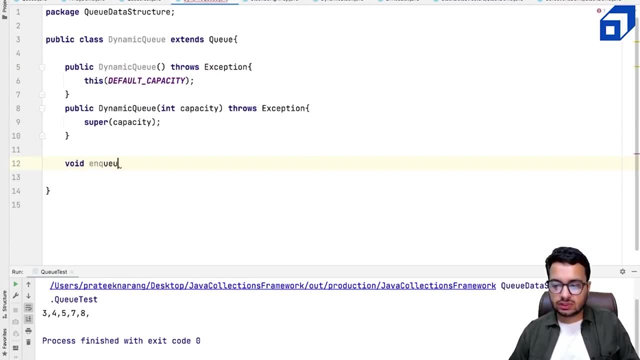 Let us see If I want to enqueue something, let's say public void enqueue. So I'm going to overwrite the method that I have written for insertion. You can see we are overriding this method right Now. there are two things we have to do. 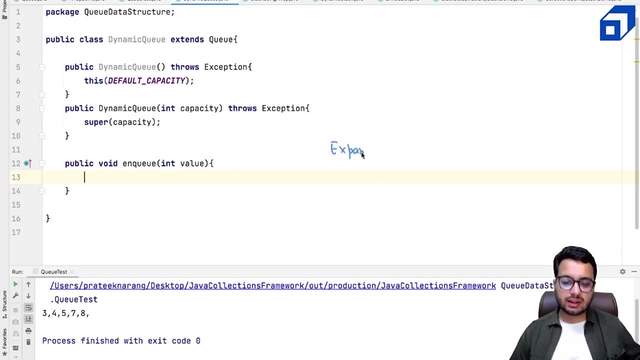 We have to expand the array right And then we have to put the element. if the queue is full, okay, put the element right. Expand if queue is full. And then we have to put the element right. This functionality we were not doing in the previous implementation. 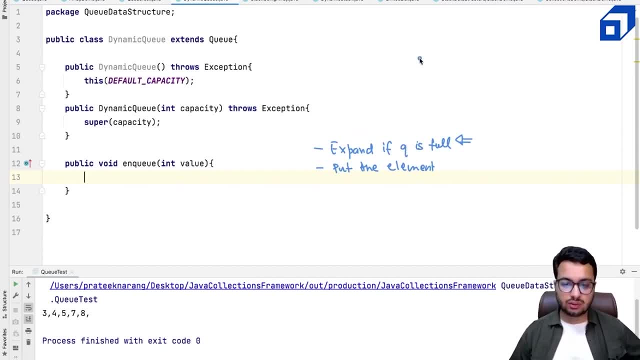 Now we have to do this functionality right. Assume that your queue looks like this. So suppose queue is like this: Right, Right, Right, Right, Right, Right. Like this: One, two, three, four, five, six. 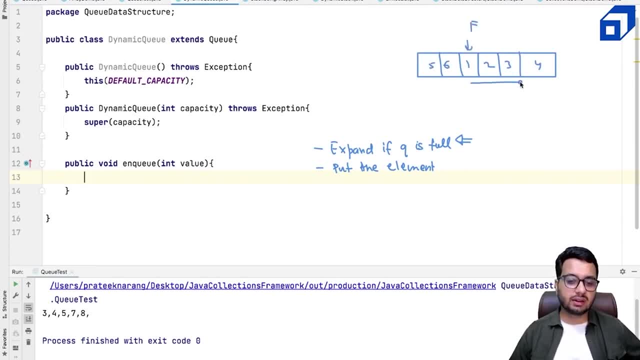 Right, And suppose my front is here. That means if I want to read data, I will read the data in this manner. Right? So my capacity was six, Size is also six. That means my queue is full And I want to create a new queue, a new array, basically with double the capacity. 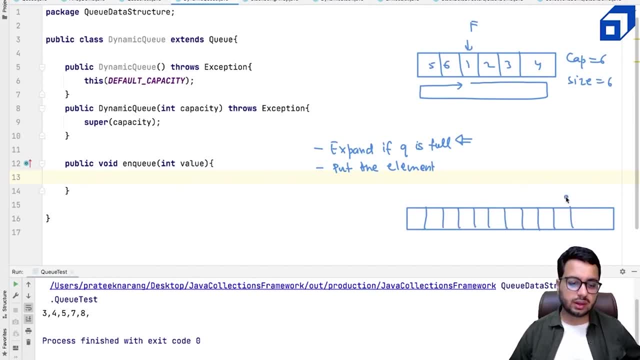 Right, Let's just say that this is going to be 2x twice of the original capacity And if I want to copy this data data, can i copy it directly? can i say i'll copy five, six, one, two, three, four. will that be correct? 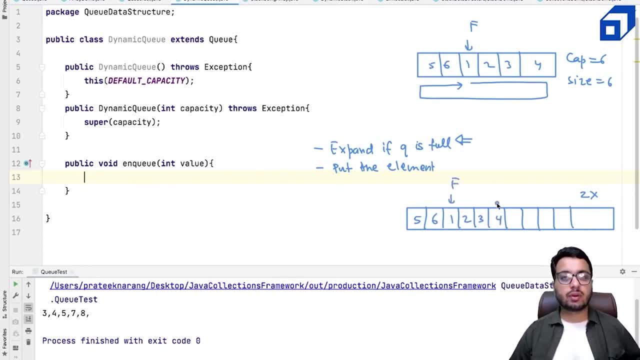 the answer is no, why? because if i want to do a next insertion, right. so at what index the next insertion happens? it happens at front plus size, right? so in this case front is at two, fine, size is six. next insertion will happen at the eighth index. that means i will start filling from this. 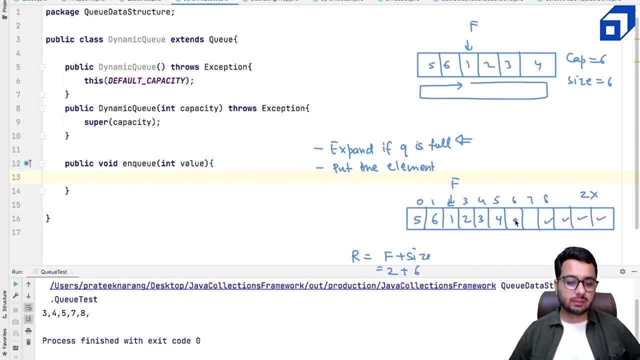 index. but is it correct? the answer is no, right, because what happens at these places we don't know, right. so the correct way of doing the copy is: you create a queue of double the capacity, right? you iterate over this part. let me change the color. you iterate over this part. 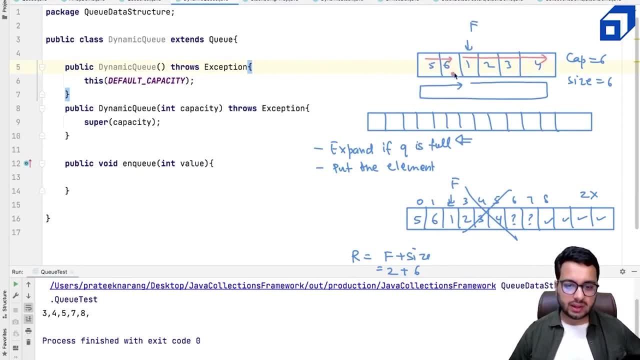 in a circular way and you copy the elements here, right? so you copy one, two, three, four, then you copy five, six. this is my front, this is my front now, if i want to do an insertion. so my rear would be front plus size. front is zero, fine, size is six. i'll start. 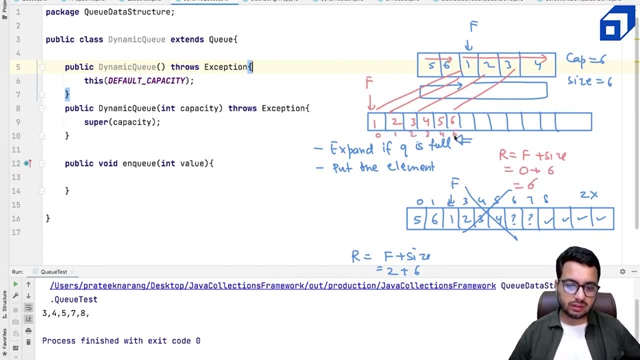 copying from the sixth index: zero one, two, three, four, five, six. that is correct. so if i want to something, that insertion should happen at these places, right. so let's see how we can do this right. so let's say: this is my original array, this is my temp array, in which 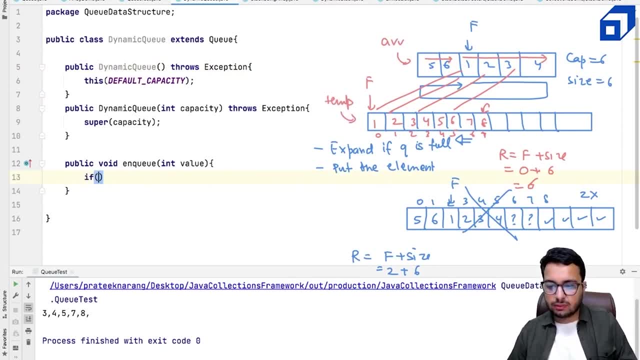 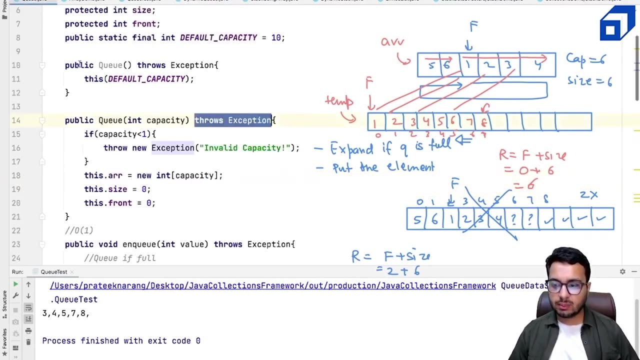 i'm going to perform a copy. i will say if what, how do i check the size? if this dot size is equal to this dot array dot length right now? one thing: you will notice that these members were earlier private. i've just made them protected. now, right, i've made them protected so that i can use them. 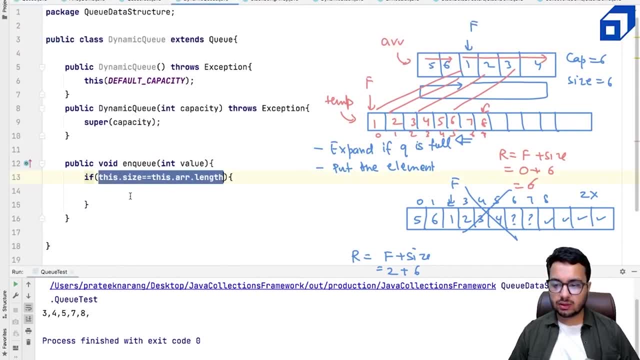 in the child class, right coming back here, so i can access the data: members of the parent class, because they are now protected, right? so what i have to do? i have to create a new array of double size. so let's say there is a new array called temp that is equal to new and of size twice. 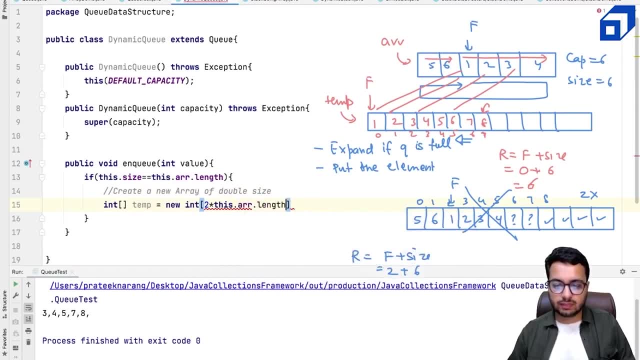 of this dot array, dot length. so this is created. now i have to copy the data so i can say for this dot array, dot length and i equal to zero, i less than this dot array, dot length, that is the size right. or you can say this dot size, both of them, they are equal, i plus plus right. i'm going to run. 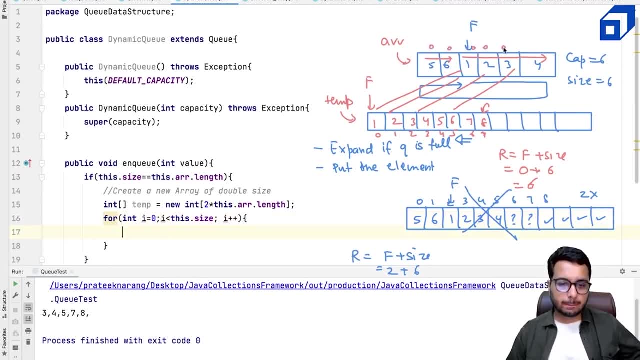 a loop these many times, right? okay, so i'm going to iterate over these positions. seven, eight will come later. right, i need to copy these values right, so i can say temp of i and add the ith index in the temp. what should i copy? i can say temp of i and add the ith index in the temp. what should i? 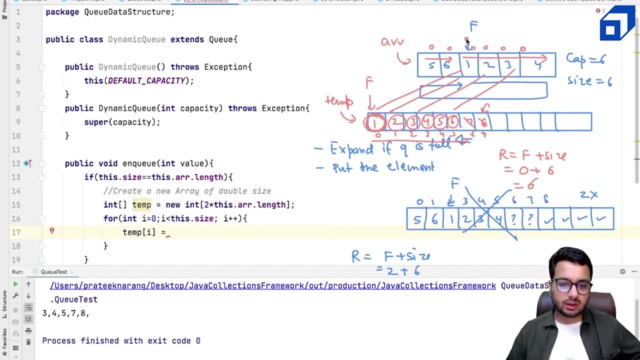 copy. at this index. what should i copy? i should copy the element from the front, so this is f plus zero. then at the next index i should copy this: lu, this is f plus one, then this is f plus two, f plus three, f plus four, f plus five and so on. right, so i can say this is going to be equal to. 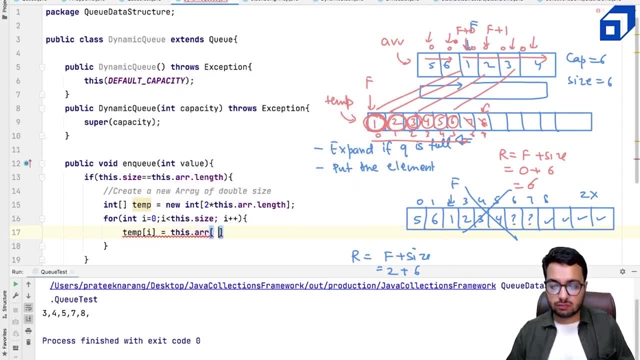 uh, this dot array of, let's uh find the old index. so this is going to be this dot original front plus the original size, with the original capacity mod right. so the elements at the um at this particular index right mod, this dot array, dot length. this is what i need to do, right, sorry, this dot front plus this dot plus i. sorry, that's a mistake. 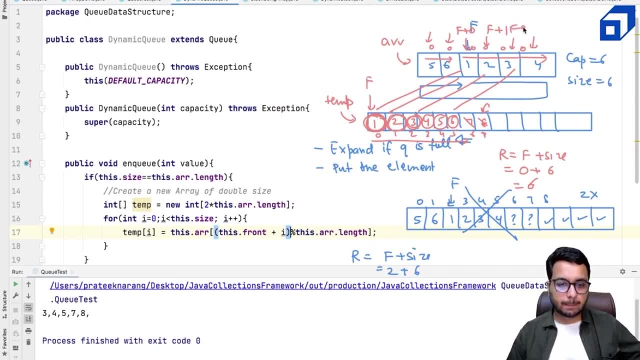 f plus zero, f plus one, f plus two, f plus three, nine, basically the ith element. okay, so the element at, let's say, temp of three will be equal to array of f, which was, let's say, 0, 1, 2 plus i. i is uh three. 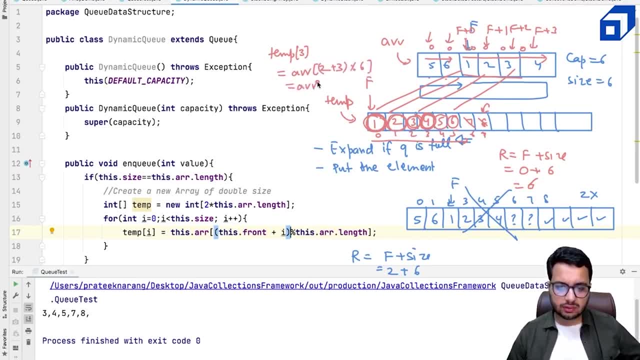 mod six, so it will be array of five. so fifth index: zero, one, two, three, four, five, five. so that element is four. that's correct. so at the third position i'm putting the value, that is, four, right arrow five. this is what i need to do, right? so just like we did in the display method. 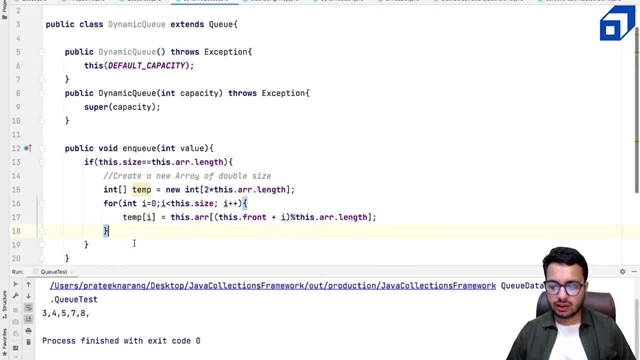 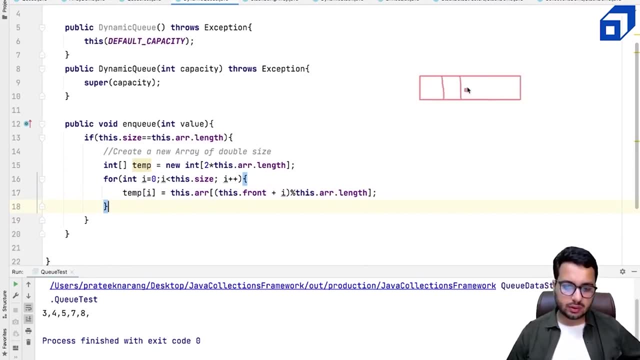 in the queue. that is the same logic we are using here right now. once this is done, temp array has been created, right, so i've erased all of it. i'll just do it once again. it was like one, two, three, four, five, six, right. this is my front now. i've copied this data like this: one, two, three, four. 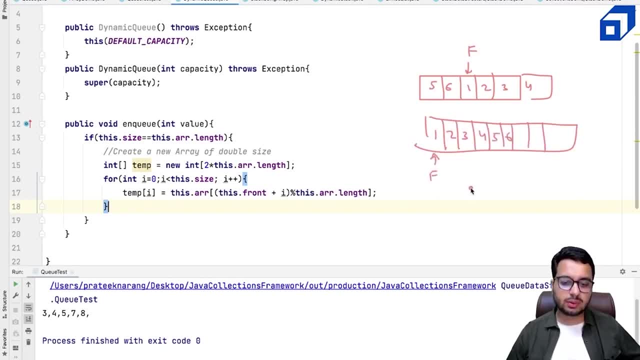 five, six. so i have to reset the front here. right, this should be the new front. okay, and this was my array. this was my temp, right? one thing i need to change is that this error should refer to this memory. this connection should get broken. i can see this dot error. this will be now referring to temp. 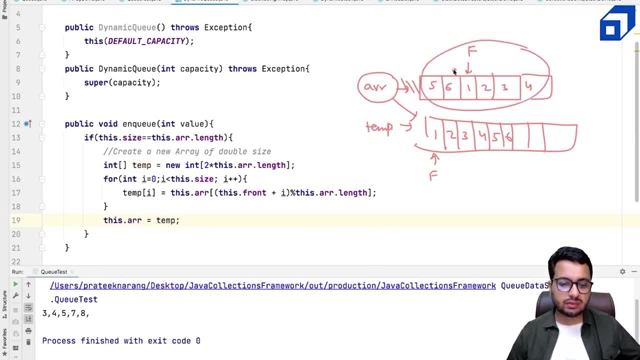 object and now doing this, no one is referring to this memory. so garbage collector will clean up this memory and this dot front will be set to zero right. but have i really done insertion as of now? the answer is no. we have still not done the insertion part right. so how do i? 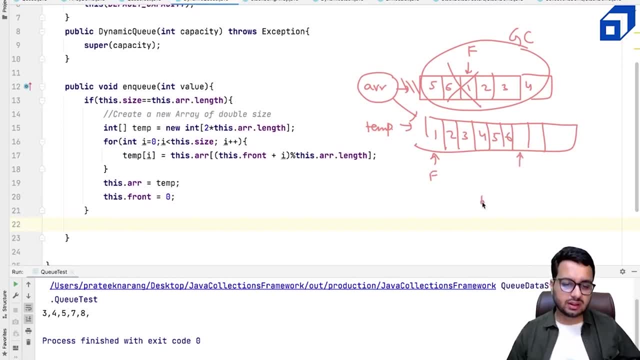 insert i can define at this position, which is rear- rear is my f plus size mod capacity. i will do error of rear equal to the value that i'm inserting and i will do size plus plus. right now this code i'm already doing in the enqueue method of the parent class, so i can. 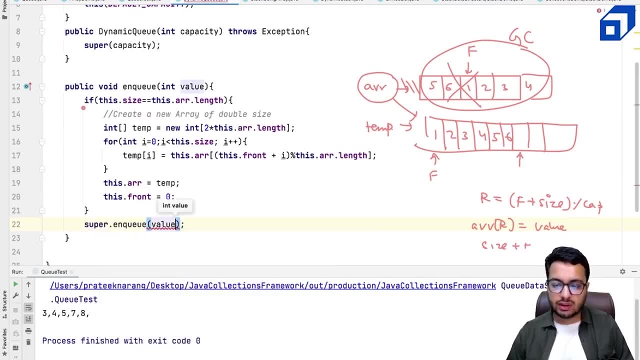 just call that method superenqueue and i can give value right now. this method will get to know that the array has been changed because error is now referring to this memory, right, and it will try to push something into this method to the new array because we have changed ARR, which is not referring to the new array, right. 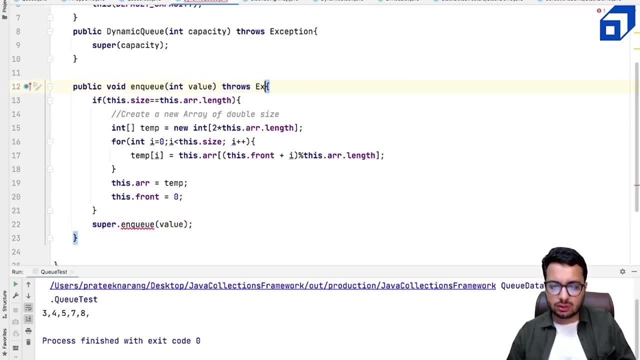 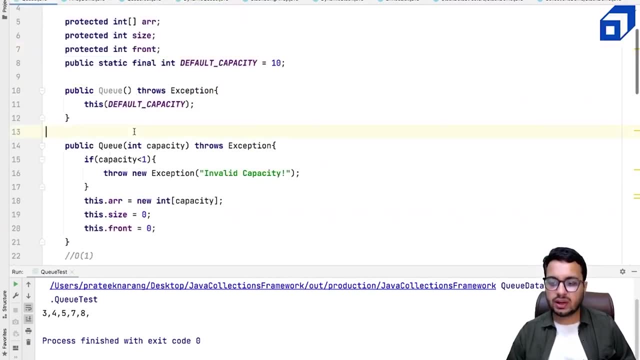 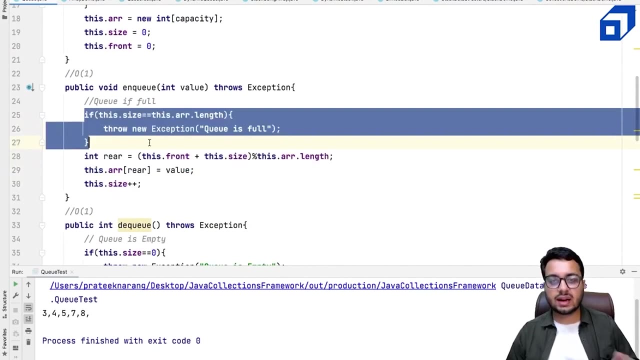 I can say this method can also throw an exception. those exception, this error, should get resolved. let us look at the NQ method of the parent class. so here what is happening? this is what we are doing right now. this condition is handled in the child class. if Q is full, double it. 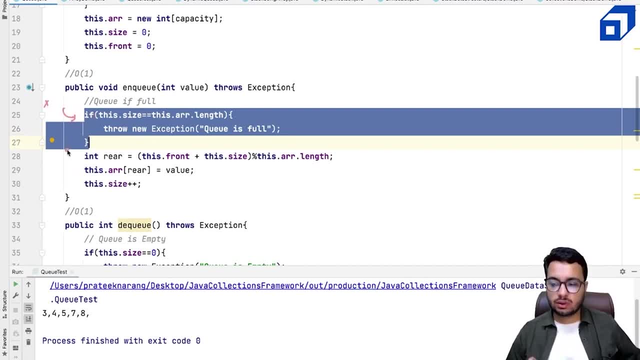 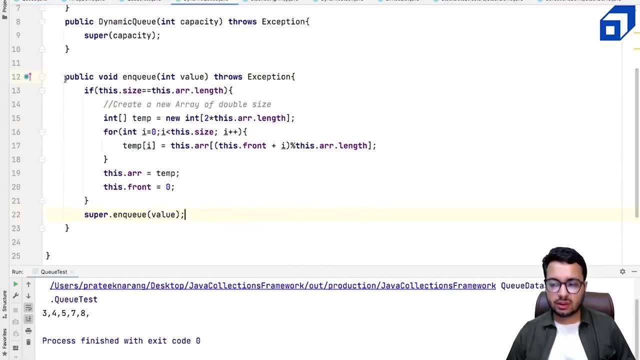 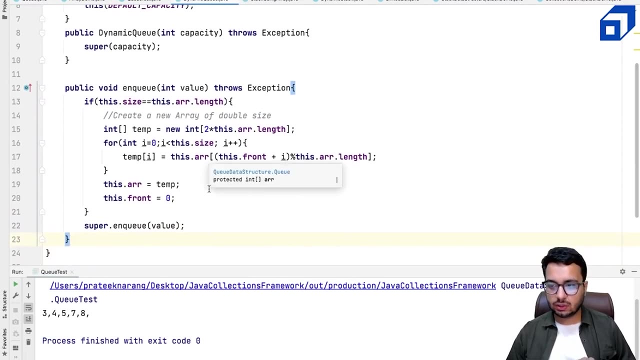 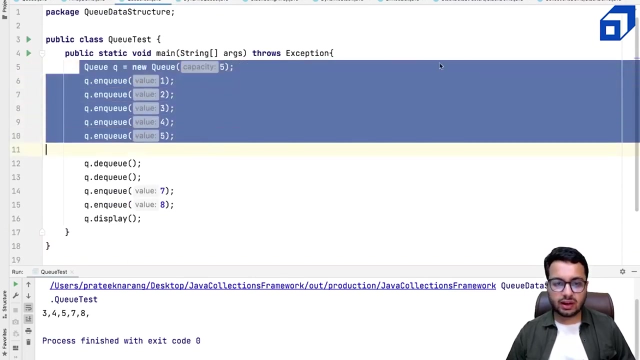 when you come back into the parent method, this condition will not be true. what code will execute? this code will execute, right, that is how we have implemented dynamic Q using a dynamic array. right now, let us test our functionality. let us go back into qtestjava, right? so earlier I was creating a Q of fixed size. if I try to, let's say, push six elements, 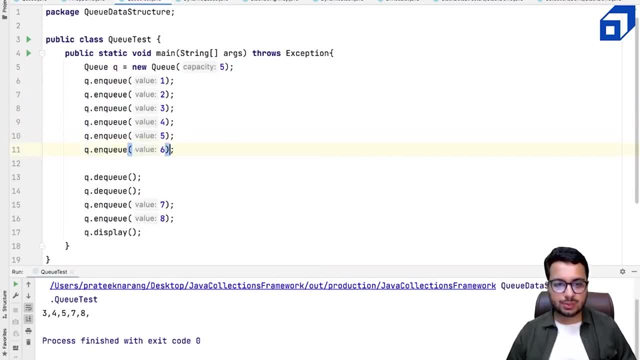 in a Q of size five, I will get a exception right. I'm using the fixed size Q. let's see. so I'm getting exception. that Q is full right now if I replace this Q object with the dynamic Q object. let me show you. if I do this, I should be able to hold it right. yes, I'm able to hold it. I. 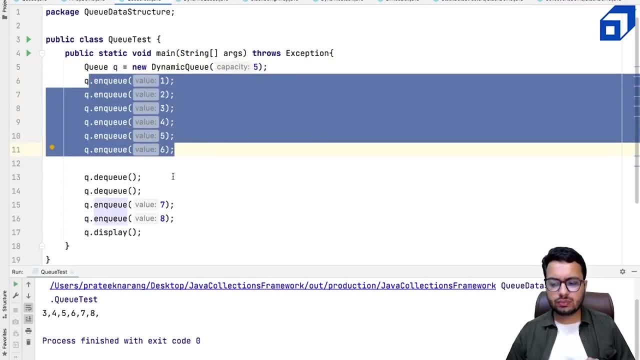 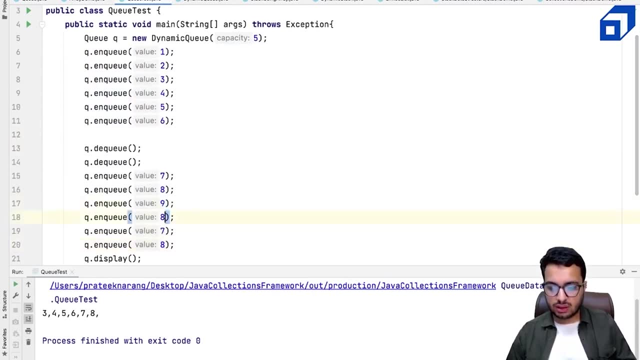 do not get any exception, because Q is getting expanded right and even I can put more elements. I can define him. let me put 9, 10,, 11,, 12 and so on. so let's see what output do we really get? I'm getting everything. 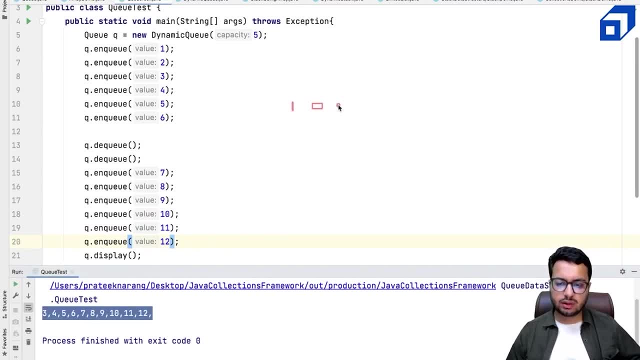 from 3 to 12, which is correct, right. so we inserted 1, 2, 3, 4, 5, 6 and you removed 1, 2 elements at the front. then you insert 7, 8, 9, 7. ah, there is a universal minimum distance more than one. 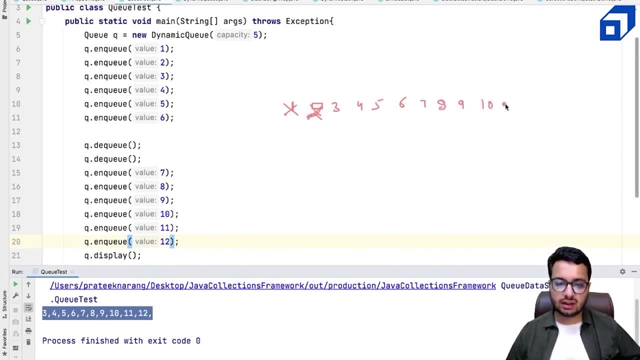 two just for the inside of masks structure. so I just get the output here. I actually get the whole night. máximoalsa, the result I dreamed, state in. I mean, if it looks like you know three models, let's see if thisехai eight, nine, ten, eleven, twelve, okay, irrespective of the initial capacity, which was five, you are. 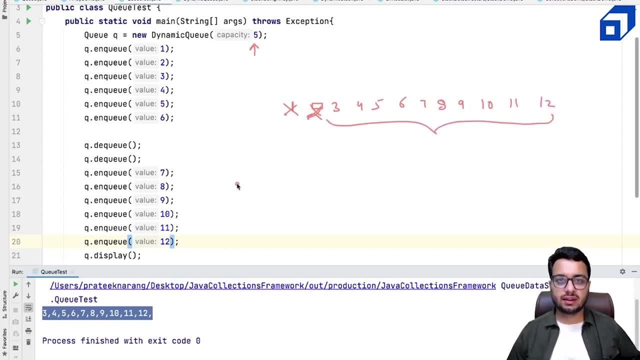 able to hold more elements because your array is getting expanded during the insertion process, right? so in this case you will never get it. q is full exception, unless you run out of your uh deep memory or something like that, right, that is uh dynamic q using a dynamic array, right? 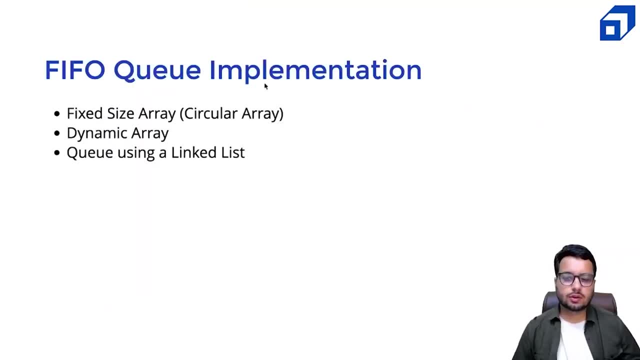 next we will discuss dynamic q using a linked list. so so far we have seen uh two implementation: fixed size error implementation and dynamic error implementation. we have seen right. you can also use a error list object: uh, if you want right now. third kind of implementation, why will involve a linked? 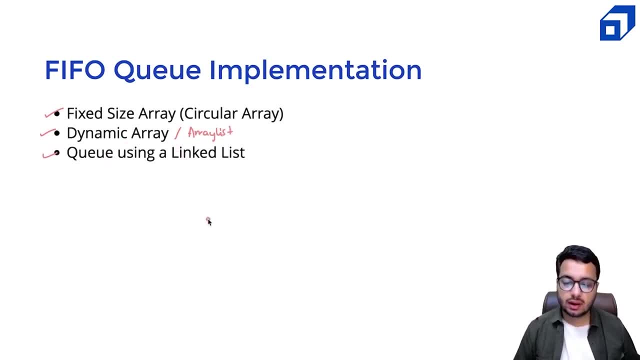 list, because linked list is also a linear data structure. right now, you might ask how we can use a linked list. it's pretty simple and very intuitive as well. now suppose you are inserting something, so one is at the beginning, then you insert two, then you insert three, then you insert four. right now, if i ask you: uh, this is. 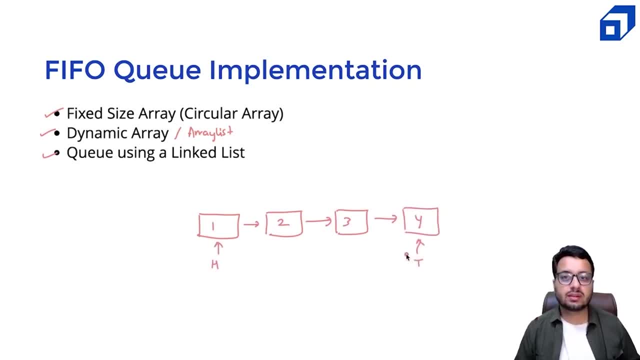 let's say head and this is tail, right? if i ask you where is the front element? right? so i want to get the front element. so that is one. if i want to remove this element, can you remove it? of course, yes, you can say, okay, i will move this head here. and that means this: 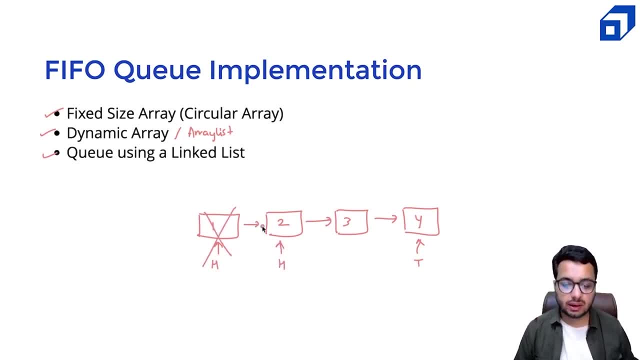 element will be removed. if i want to read the front element again, that element is at present at the head of the linked list. if i want to insert something, it should go at the rear end. so where is the rear end? the rear end is at the tail right, so you can easily insert something here and your tail 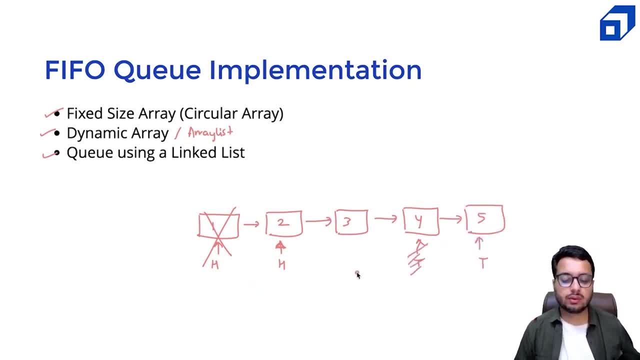 will come here, right, so your head and tail- uh data members will behave as front and rear for the linked list. so this will be your front, this will be your rear. you can always insert at the rear end which is insertion at tail, and it will be a order, one operation. 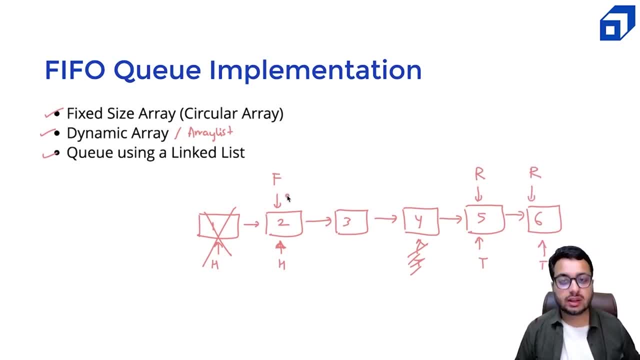 and you can always remove from the front end, which is again going to be a order, one operation, right. so very simple implementation. and we have already covered linked list. i will not write the code using linked list. once again, you can either use the same class object, so in your queue class you can say: fine, i'm, i'm going to create a linked list object, linked. 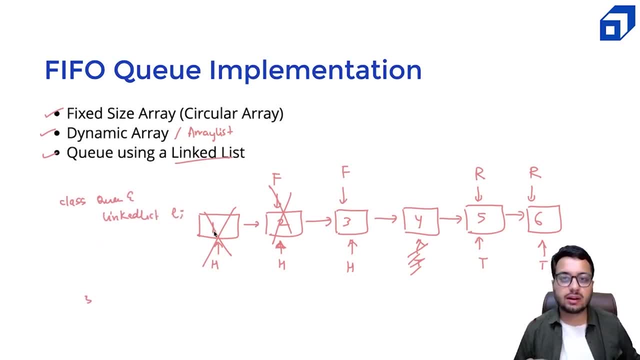 list l, and whenever you want to enqueue, you add it to the linked list, and whenever you want to remove the first element of the linked list, okay, so those methods can be implemented, or you can implement all those methods from scratch as well. right, so that is about uh implementation using a linked 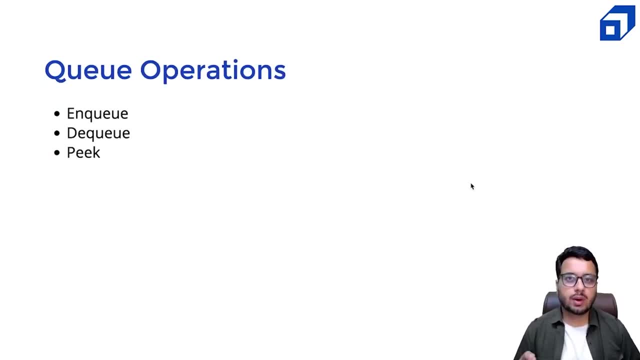 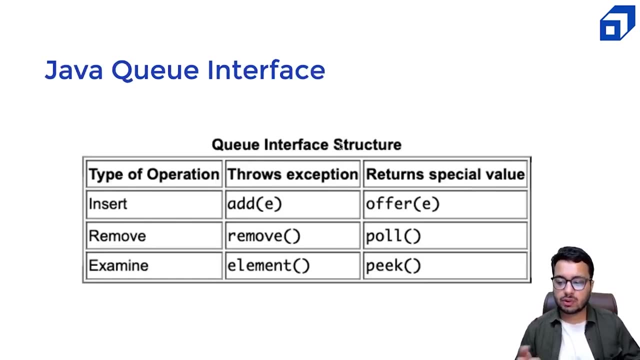 list. now, before we wind up this tutorial, i want to talk a little bit about the java queue. that is part of collections framework, right? so the java queue supports, uh, three types of operations. so one is your insert, remove and examine. right, so examine is like getting the front element right now. 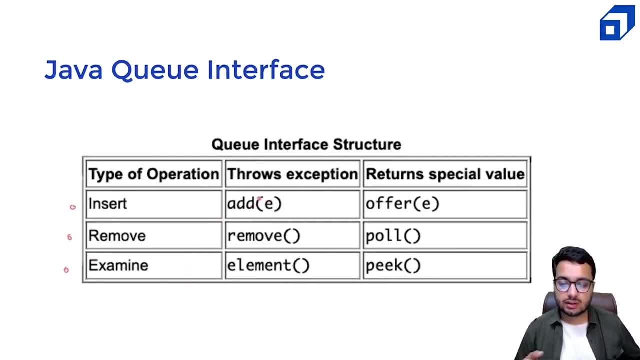 there are two variants of the methods that are provided, so in one variant the methods throws an exception. like the variant that we have coded, those methods throw an exception. if you want to add something, the method is called as add instead of enqueue. right, so you will say: okay, i will create. 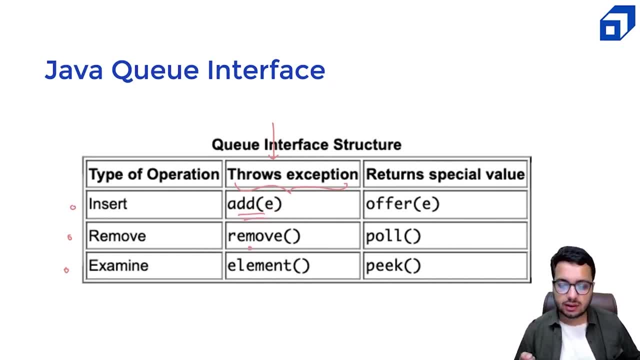 a queue object and i will call the library method add- right. if i want to remove the front element, the method is called as remove instead of dequeue, and if you want to get the front element, it is called as element, right. if the queue is empty, it will throw an exception. right, and the second set. 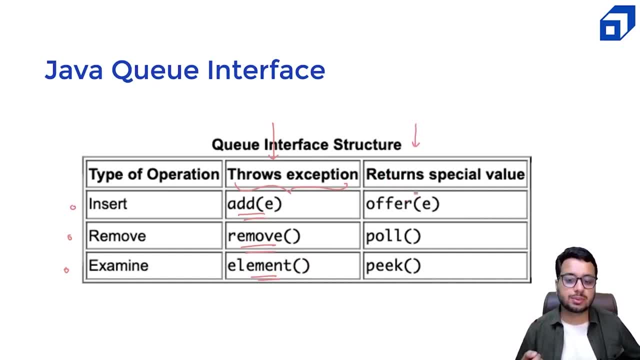 of methods. they are also same, but instead of throwing an exception, they will return a special value, maybe boolean value, whether the operation was successful or not right. so add and offer their equivalent methods, remove and pull their equivalent methods, element and peak their equivalent methods. okay, so i've discussed about queue interface in my java collections. tutorial on. 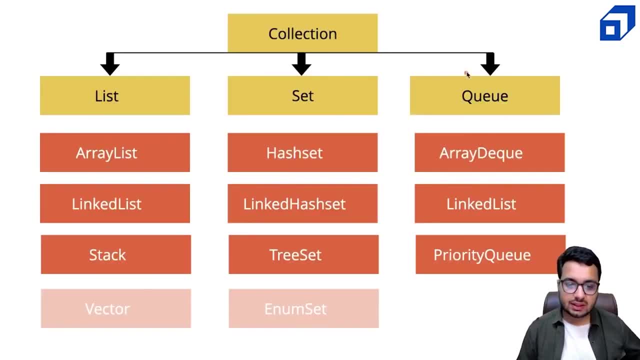 the channel right. so what we talked about is: let's see what we talked about here. so let's see what we talked about here. so let's see what in java queue is actually a interface, okay, and there are three implementations. there are three classes that implement this cube. so your linked list class: it implements your fifo queue. that we 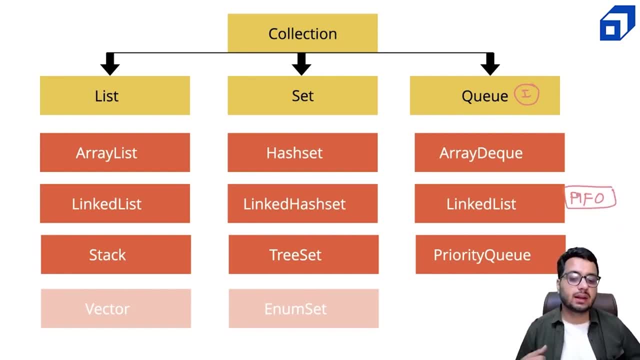 have just seen that we can build a queue using a linked list, okay, and there is something, there is a class called as aerodeck. so aerodeck is a class that implements another kind of queue in which you can insert and remove from both ends, right? so it is called as a doubly ended queue. so in this case, 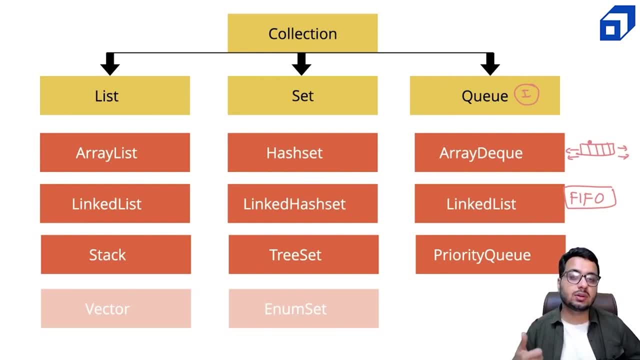 the behavior would be different. you, you can add at first position, you can add at last position, you can remove at first position, you can also remove at last position. so it starts. it is a doubly ended queue. it's called as deck right. it's not dq, it's called as tech right. it's a different type of queue. 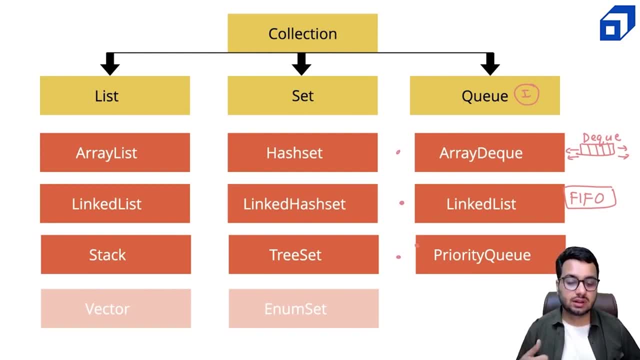 and third type of queue. it's called as a priority queue, which we will of course discuss. it is based upon the concept of keep data structure. in this case, the elements don't maintain a fifo ordering, but they maintain a priority queue. so when we look at this, you will see that in this case, even full promfu- 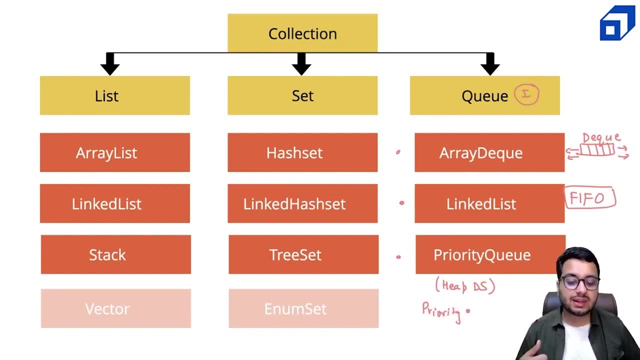 file or other file case. it will contain a saying in this case. now i'll like to say that the type priority ordering. so again, it's a big topic. we will discuss it separately. but if you want to see the code demo how these different queues are, how these classes are different in behavior. 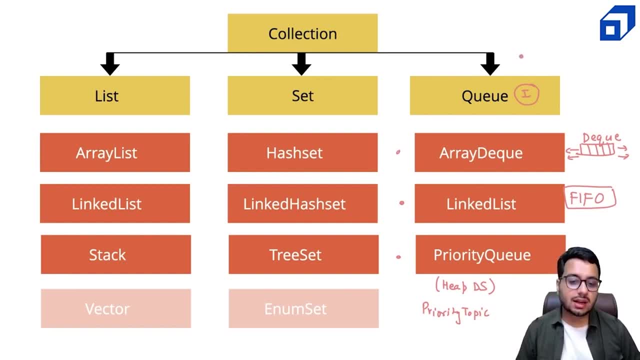 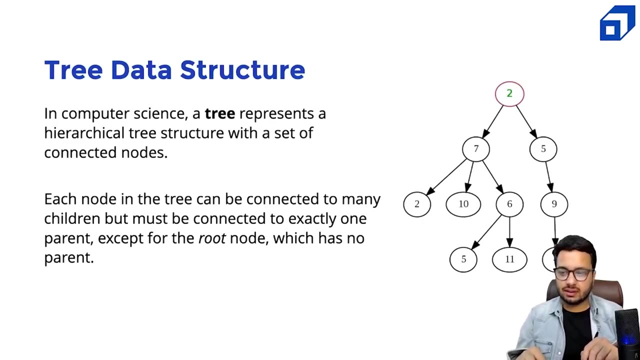 check out my video on data structures and in which i have discussed the complete collections framework as well as different implementations of queue as a part of that video. let us start the topic by understanding what is tree data structure? in computer science, a tree represents a hierarchical structure with a set of connected nodes, right? so, for example, if you look at this, 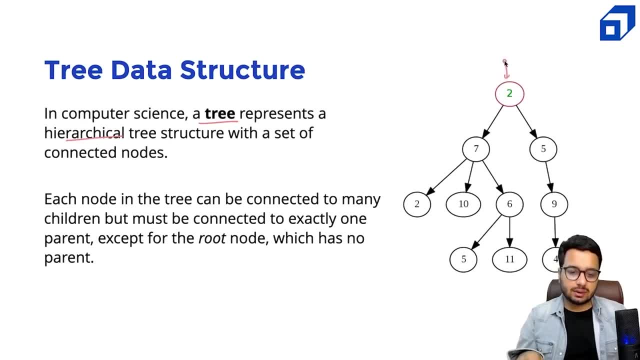 diagram. this actually represents a tree and this node, it is the starting of the tree. it is called as a root node. right, we will discuss where it can be useful. so in this structure each node in the tree can be connected to many children. so this is a non-linear data structure. the first 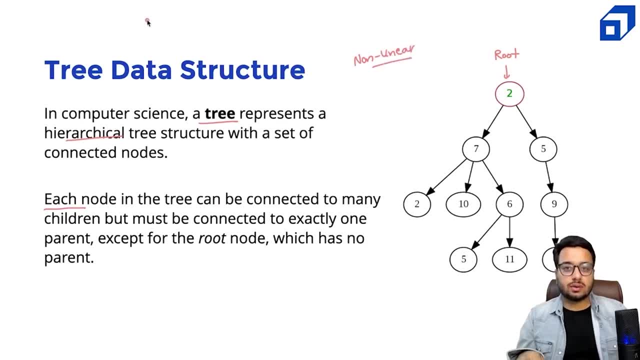 non-linear data structure that we are covering is a tree. so far, we have talked about array, we have talked about linked list. all of those data structures were linear data structures because they were following a sequence. here there is no sequence. here there is a hierarchy, right, so each 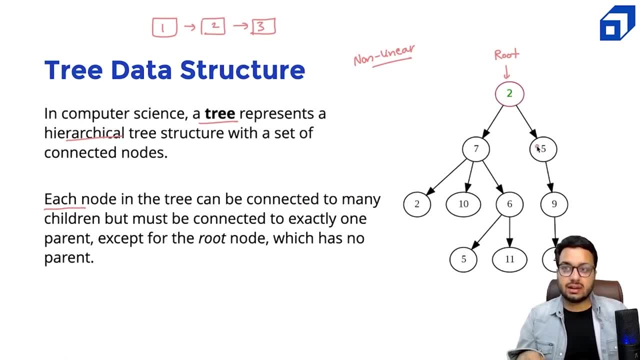 node can be connected to many children. so two is connected with seven and five. it is connected with two children, so seven and five. they are children of two but must be connected to exactly one parent. so each node must have one parent. i cannot say seven will have two parents. no, 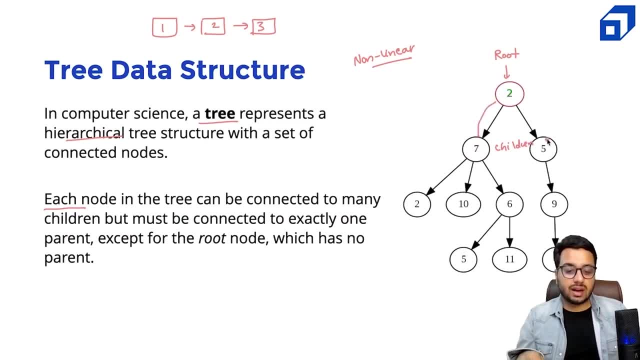 seven will have only one parent, that is two. five has only one parent, that is two. two has only one parent, that is seven. ten has only one parent, that is also seven, right so, except for the root node, which has no parent. so root node has no parent, rest all the nodes, they have one, one parent, right. 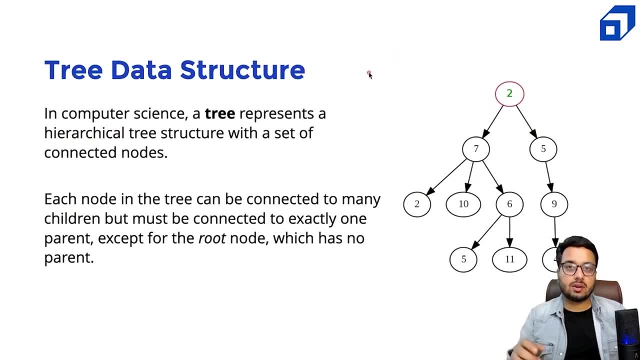 now. because of this, there will be an interesting observation. suppose you are creating a tree in which you are going to have n nodes. okay, for example, i have three nodes here, so how many edges you will have except for the root node? for every node that you will have that you will add, there will be an edge. 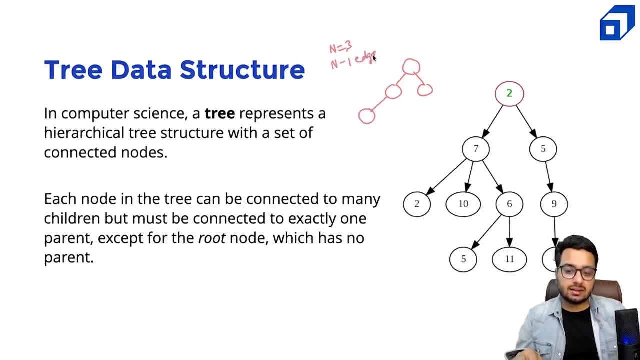 so there will be, of course, n minus one edges in the tree, right? so in any tree that you are going to create, irrespective of is it a binary tree or not, each node is going to have an edge. so if you are going to have an edge in the tree, 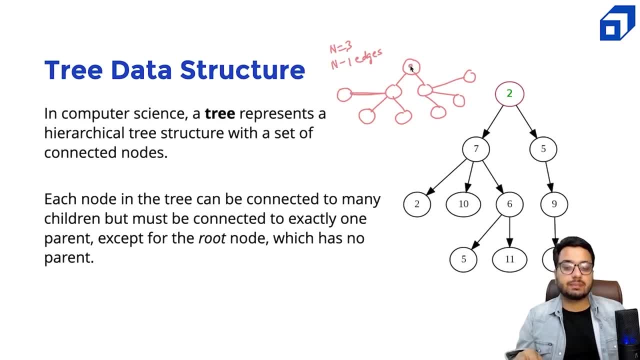 the node that you add will add a edge in the tree except the root node. okay, so root node does not add any edge in the tree except the root node. if there are n nodes in the tree, there are, there would be n minus one edges. okay, because root node has no parent. rest all the nodes that you add. 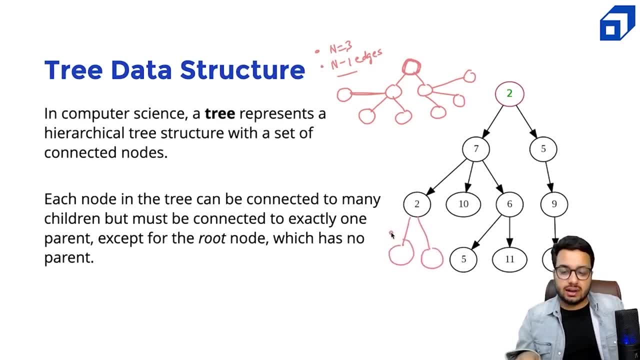 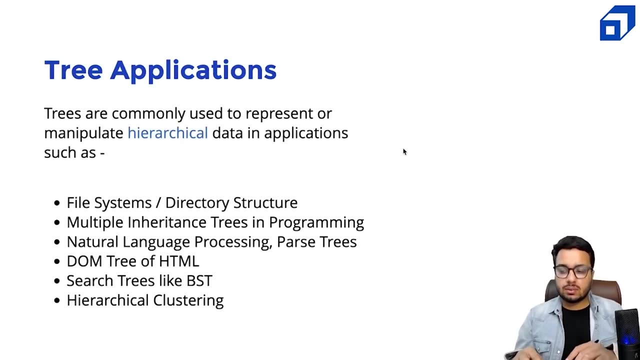 they must be connected to a parent through an edge right. so this is an interesting observation. you can note. so in n every tree there will be n nodes and there would be n minus one edges in the tree right. so that is tree data structure. now let us talk about where this data 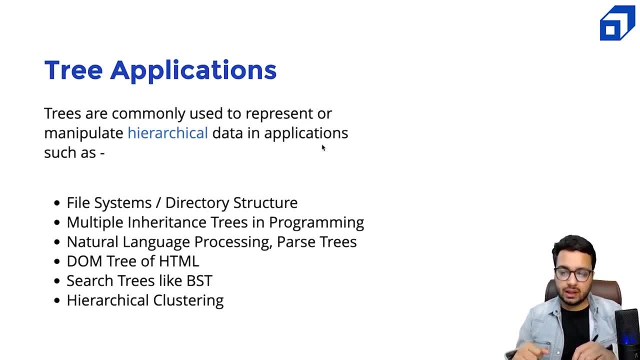 structure can be used, how it can be helpful in computer science. okay, basically, trees are used to represent or manipulate hierarchical data in applications such as file systems or directory structure. right, so all of you have worked with a file system. so what happens in a file system? you say, okay, i have my pc in this, i have certain drives. 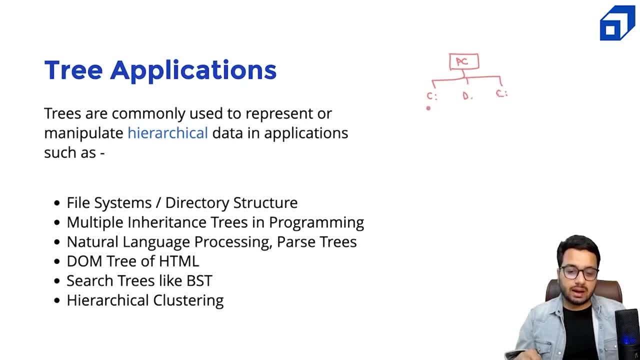 c drive, d drive, e drive, and then inside this i have folders f1, f2, f3, f4, and here also i have folders. then i have sub folders- right, maybe i have photos here. maybe i have some documents here right now. we often do operations like that. okay, i want to move these photos from here to here, right, so? 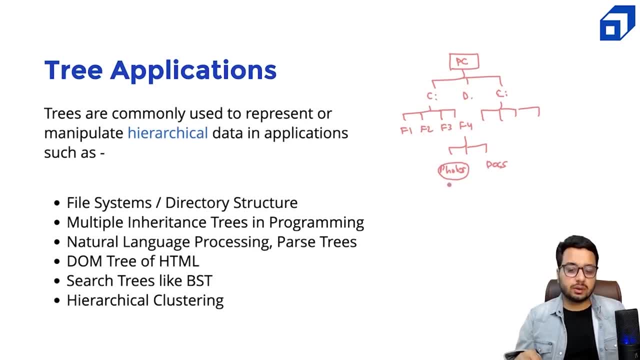 what is going to happen? you're not going to copy this data. you're going to say, okay, i'll cut and paste. so if you simply want to move these photos from here to here, what do you need to do? you do not need to copy this information to some other part of the disk. you only need to change the reference, right. 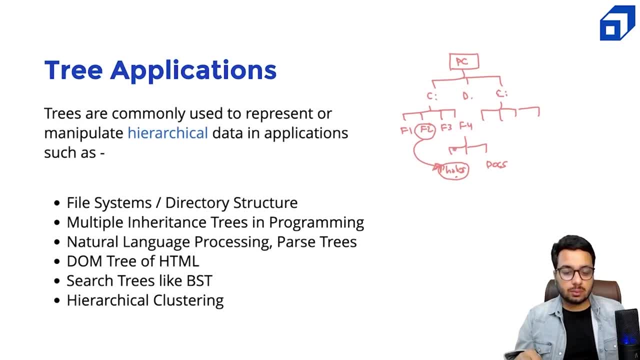 that. okay, earlier this reference was stored by f4, now this reference is stored by f2. basically, the links, right, the links to the folders and subfolders. they can be easily changed if the data structure is implemented using a tree, right? this is something we will discuss. right, the file system is a good example of 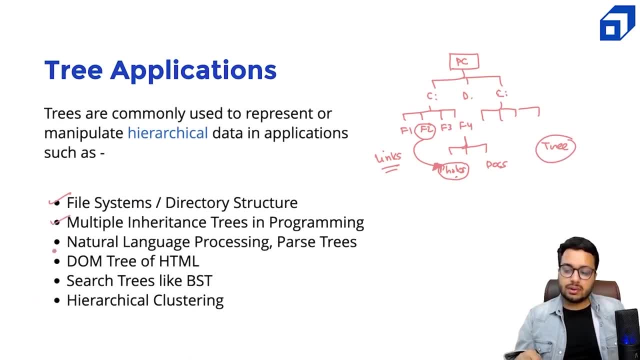 a tree data sector right- multiple inheritance trees in programming. so this is used when you are using object oriented programming concepts and you have a class c which is going to inherit from a class a, it is also going to inherit some methods from class b, right? this is, uh, not exactly a tree, i would say, because 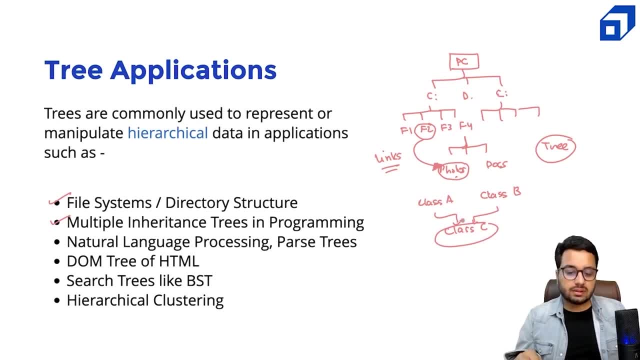 this node. this is inheriting from two different classes. irrespective of that fact, basically, the trees are internally used by the compilers to see what methods would be part of the class that you have implemented using inheritance. okay, then again in natural language processing, basically whenever you have a sentence, for example, i am going for a party right now- this. 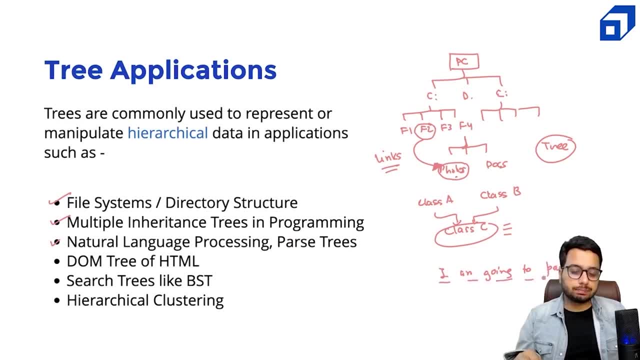 sentence can be broken down into two parts. one is the input and the other is the output. so this is orton equals one is the identity of the other. so again, i will just criticise you for not dealing adequately with me & stop there. we will discuss the code in a bit, but already ligby to get into. 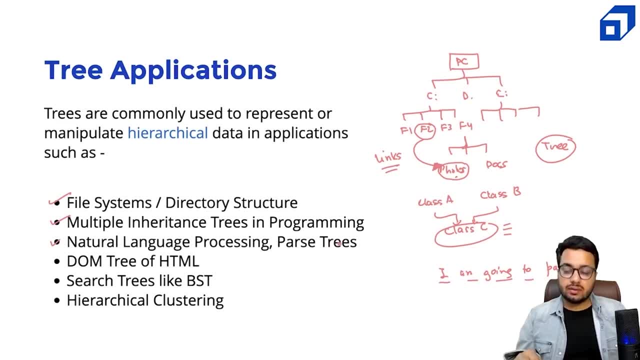 uh, certain components, maybe you have a verb, maybe you have a subject, maybe you have a predicate, or you have even for language parsers, okay, so what are your parsers? So whenever you write code, uh, it goes through a language parser so that compiler can figure out if there is any. 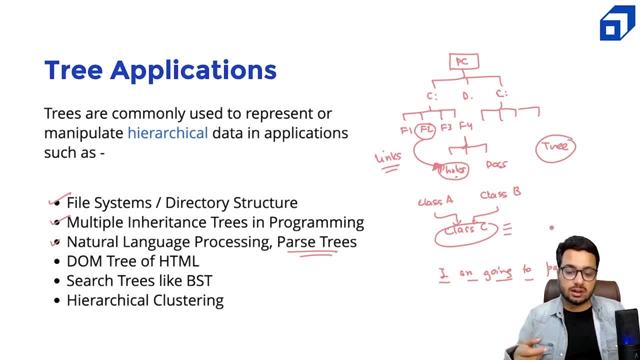 error in the code is it's having the correct syntax or not. so they again form a parse tree of that code, right? so again, it's an interesting concept that you will learn in compilers right now. right again, they are used a lot in understanding of the language. okay, then in html there is a dom. 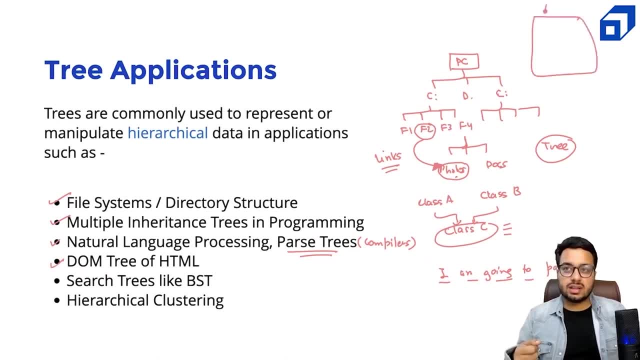 tree. so whenever you open up a website, right, you see there is a html code. right inside html code there are a lot of tags, there is head, there is body. right inside body there is a paragraph, there is a div, there is a image. right, if you look carefully, this whole document forms a. 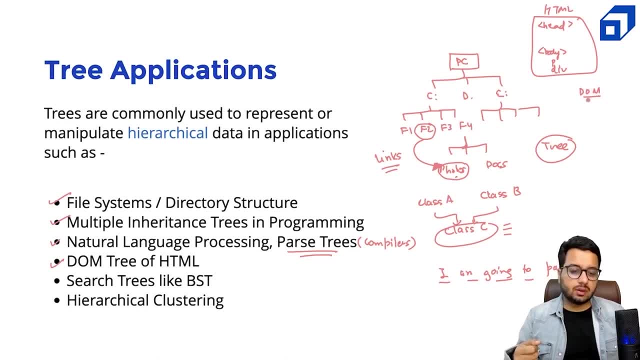 dom tree. so inside dom tree you have head, you have body. right then you have certain elements, you have div, you have paragraph here you might have image, you might have some text it. what is happening? you want to say, okay, i want to click this particular button and on clicking, 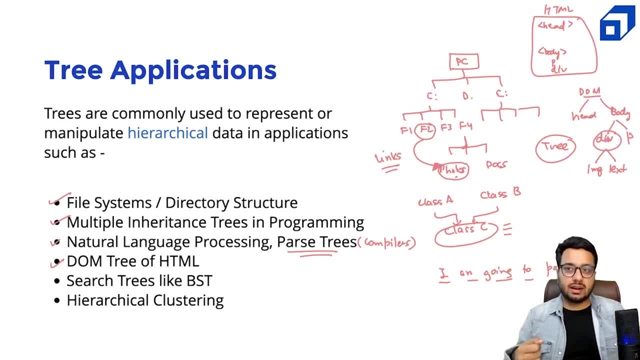 this button, this div will change its color right. so how do you fetch elements from this huge web page? so there are methods like doc. element by id, document. dot get element by tag name. so what it is doing it is traversing this dom tree. it is a tree of objects. okay, it is a tree of objects, uh, in your web browser. 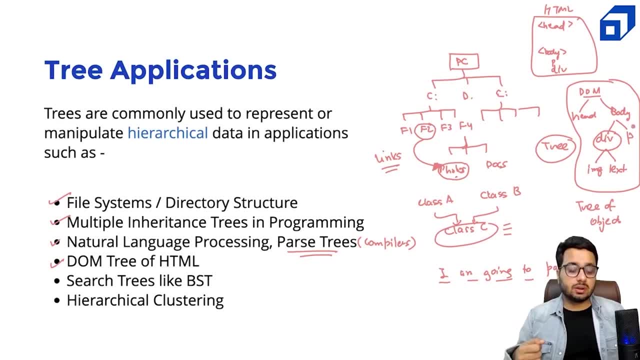 again. it's behind the scenes, so it is doing some kind of search operation on this tree and it is trying to manipulate this tree right? for example, you scroll your web page and a new item is added from the bottom, so maybe it is adding something in in the list, right? 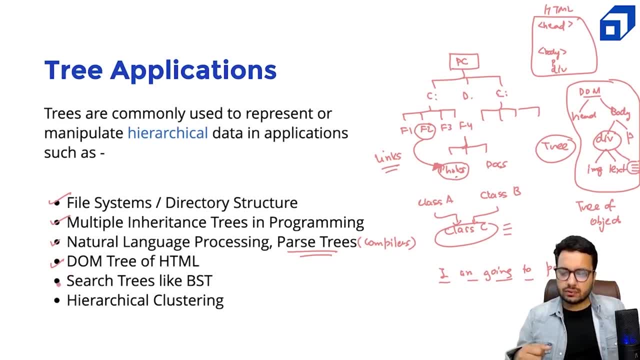 so your tree is getting modified, right then, of course, there are trees which are used in search operations, like binary search tree. there are trees which are used to implement data structure, like map self-balancing trees. okay, so they are used to perform faster searches and keeping data ordered. 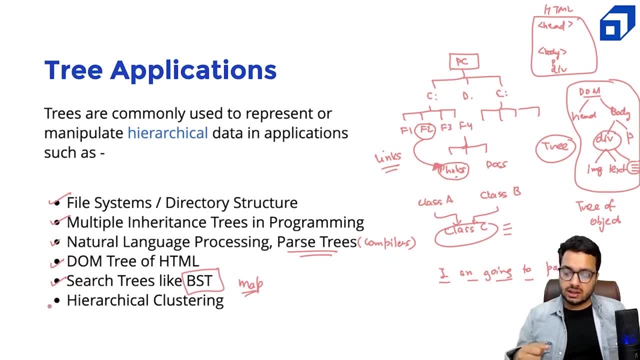 we will talk about bsts in the coming class. in machine learning there is a concept called as hierarchical clustering. so it is a part of a clustering technique okay, where i want to group together something like that. so i'm going to do a little bit of a search operation and then i'm going to 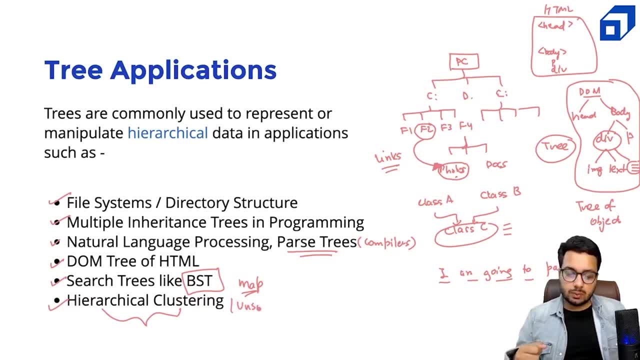 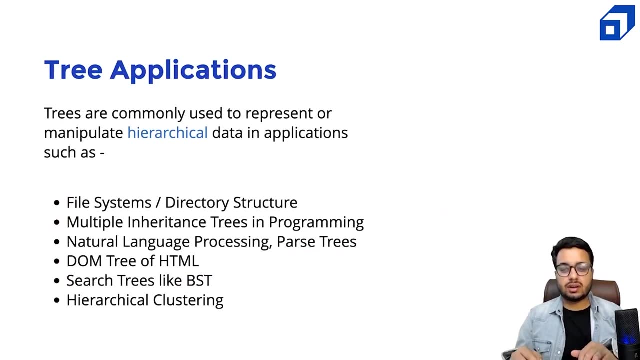 together similar items. it comes under a part of unsupervised learning, so there also the tree data sector is used right. so you we see lot of applications are there and that becomes very important for us to understand the tree data sector. so in this video we will be talking. 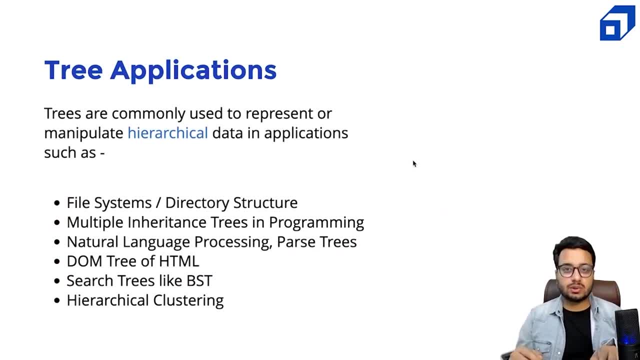 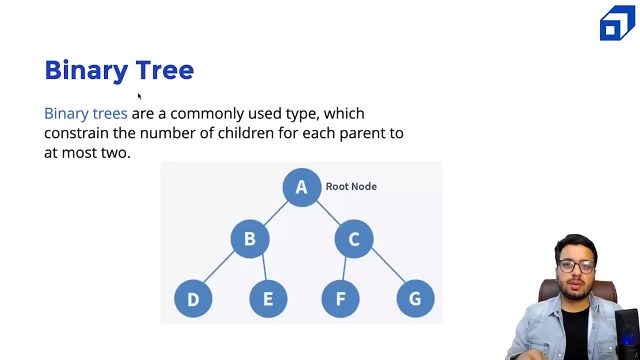 more about binary trees in general, because that they are the most common ones that are widely used. okay, so let us start with binary trees. so let us start by understanding what is a binary tree. so, as I discussed, it is the most commonly used tree structure in which 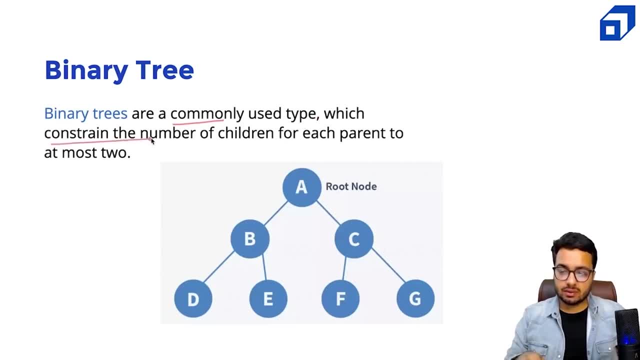 you can have at max two children. okay, so it contains the number of children for each parent. to add most to that means node can have zero children. for example, in this case, the nodes D, E, F, G. they don't have any children. they are also called as leaf nodes, the nodes which 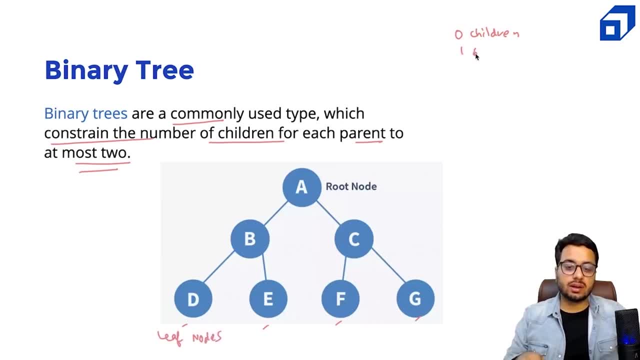 don't have any children. they are called as leaf nodes. node can also have one child right, or it can have two children right. it cannot have more than two children. for example, if i draw a few structures, you have to tell me whether it is a binary tree or not. is it a binary tree? the answer is yes. each node has zero child. 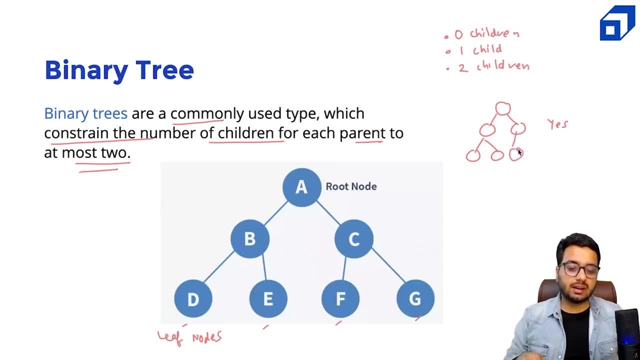 one child or two children. right, okay, is this a binary tree? the answer is yes. so this node, the node c, it has one child. a and b, they have two children and def, they have, they don't have any children. hence, in this case we have three leaf nodes. so this is again an example of a. 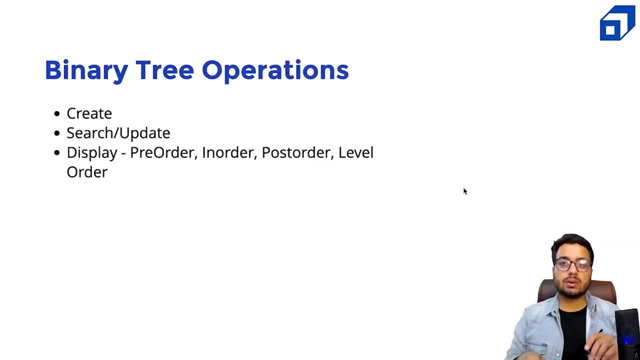 binary tree. right now, what we are going to learn in this tutorial? we are going to learn about different operations. how do we create a binary tree? how does the node structure look like? how do we perform search or update operation on a binary tree? how do we display a binary tree? and there are uh four popular ways to do it: pre-order traversal in. 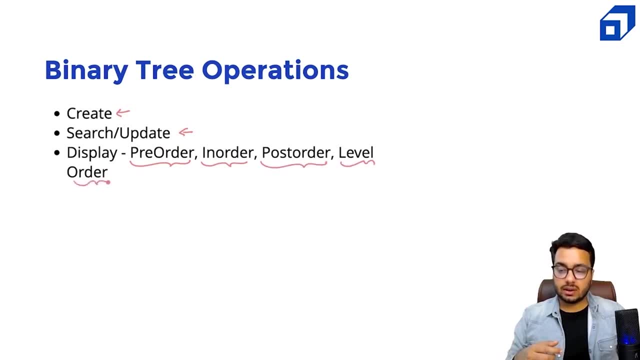 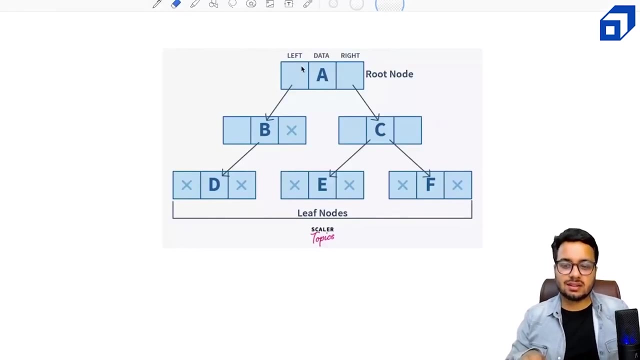 order traversal. post-order traversal, level order traversal. okay, so we are going to look at all those, all these things one by one, and we'll be starting with, uh, creation of tree. first, let's begin with that. let us talk about creating the tree. so first of all, we need to understand the 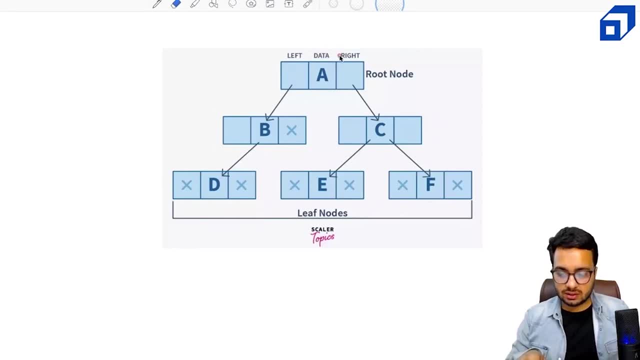 structure of the node that is going to create the tree, right? so in this tree, if you look carefully, there are so many nodes and this box represents one particular node. okay, that is the root node, right? so i have the root node. now, what is this root node going to contain, or any node going to? 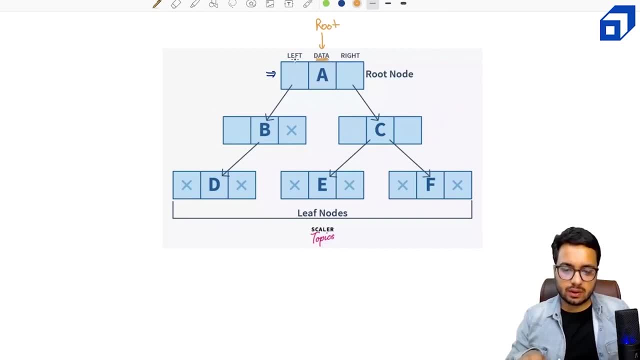 contain. it is going to store three things: one is your data, one is the address of the left node, one is the address of the right node. okay, in java we also call it as reference. right now, suppose this object b it is created at some memory address. let's say, uh, 250, right? 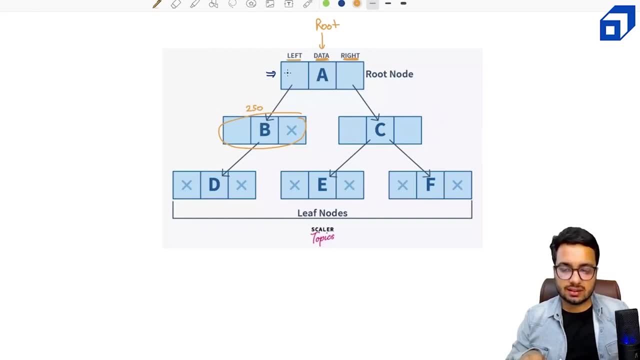 this is the location of b in the heap where it is created. so a is left, is going to store 250. let's say this is created at some location- 380. so a is right, is going to store 380. right, a itself is created at some some location. let's say 400. the root is going to store 400. okay, so root is. 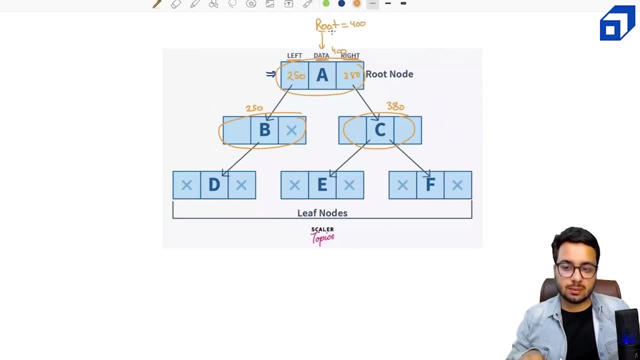 not a node. root is just a reference to the root node. okay, so root variable is holding the address of the root node right now. b is left, is referring to d, so d is created at some location, let's say 560.. so here we will have 560.. now d is left and right. they are. 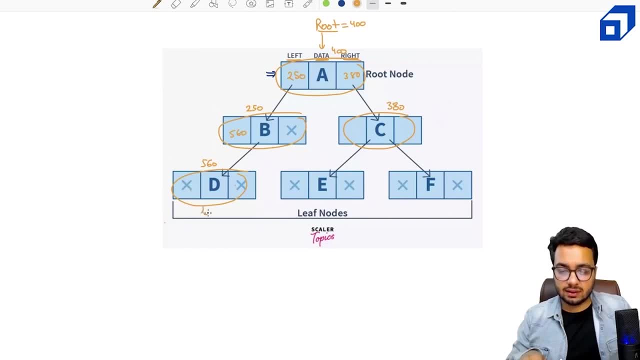 they are null. they don't refer to anyone because d is a leaf node, right, so d is a leaf node. e is a leaf node. f is also a leaf node, so they are left and right, they are null. now b is a node with a single child- right, because it does not have any right child. hence this value is also null. and 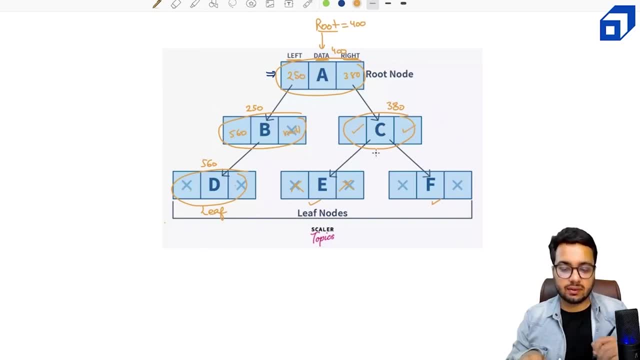 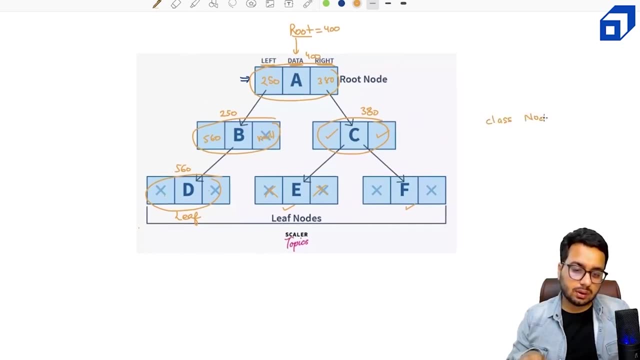 here i will store the address of e, here i will store the address of f. right, so i hope you are familiar with this value of the node. so i need to implement a class called node, in which i will have three things. one is my integer data. data can take any type. just to keep it simple, i'm taking it. 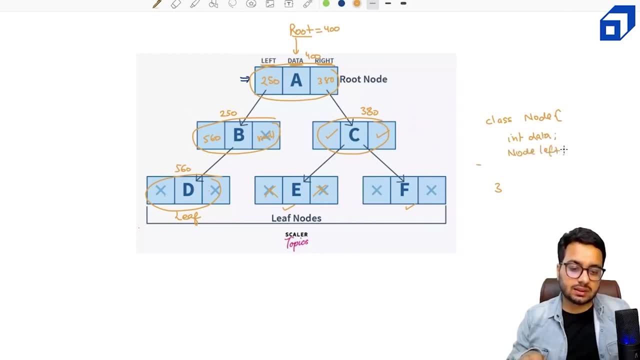 as a integer one will be my: node left, a reference of the next left node, and node right, a reference to the right node. if the left and right node does not exist, then i will set this value to null. right now let us see in the code how can i implement this node class. 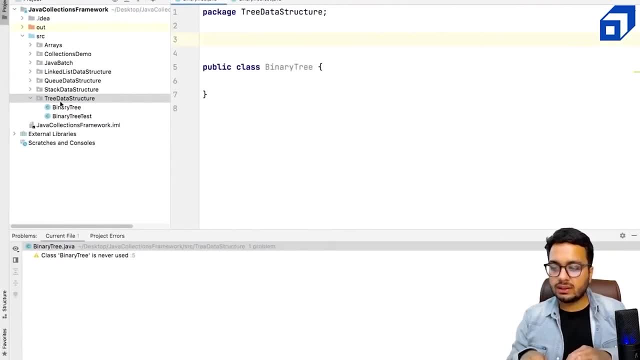 so let us go to intellij. now i am going to implement the tree data structure. i have a class called binary tree. i have a class called binary tree test. both are empty classes as of now. in order to build binary tree class, i need to define that. what is node right, so node will. 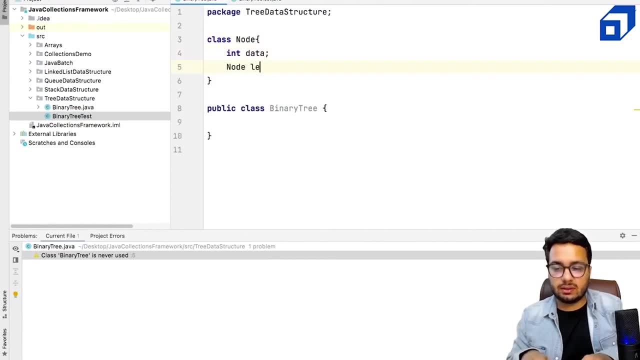 have three things: one is my data, one is my left and one is my right. apart from it, i also need to give a constructor here that whenever a new node is constructed, what data it should take. so it's okay, data i will know, but at the time of construction of new node, i do not know what. 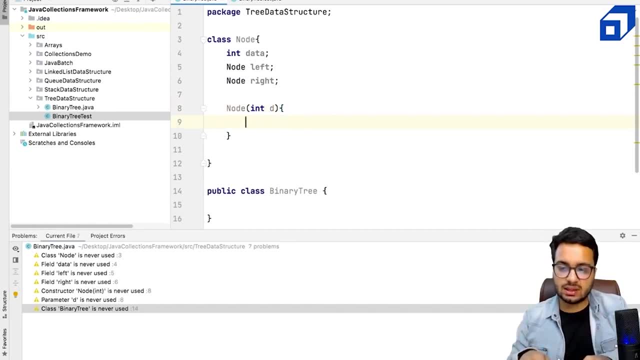 node will go into the left? what node will go into the right? so i will simply say that my data this is equal to d, and left and right, they will be set to null by default. so whenever you are creating a new node, you do not know the left and right uh nodes. so these will be. 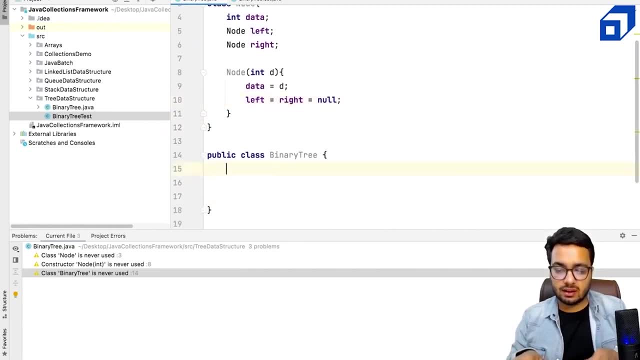 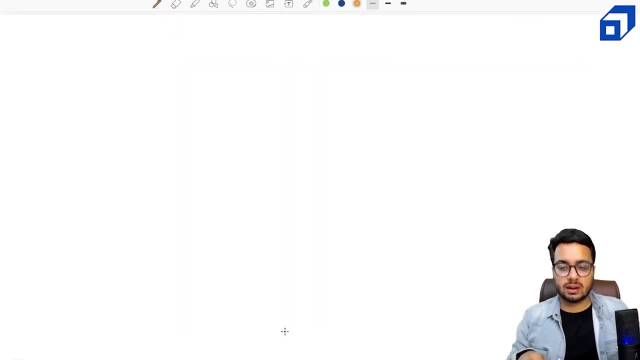 set later. right now comes the binary tree class. now suppose we want to create a tree like this. okay, or let me take up another example in which i have numeric data so i can say: okay, let me create a tree like this, one connected with two, and then it is connected with three. right, let's say very, 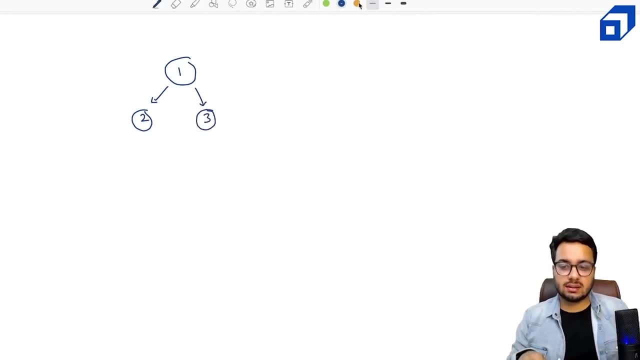 simple tree, three nodes now how you will read this tree. the first thing is: how do i read this tree? the first input i will get is the root node. okay, user will enter one. i will say: fine, input is one. okay. so i will create a node called root node and root node is going to point to this node, right? 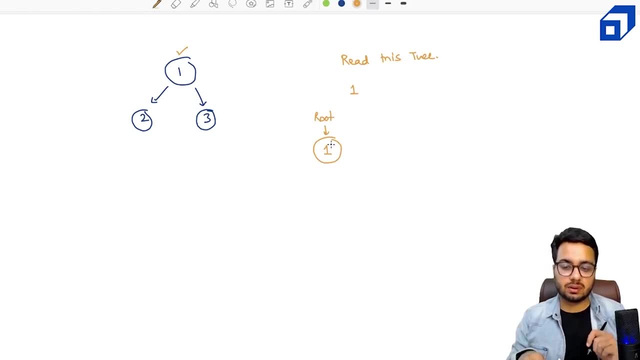 and in the left of this i will again read from the user. right, the user says: okay, fine, the next node is two. so i'll define, i'll create a node called two. i will attach it in the left of one like this: okay, and now what is the next one? i will read: right now it can happen that i have something. 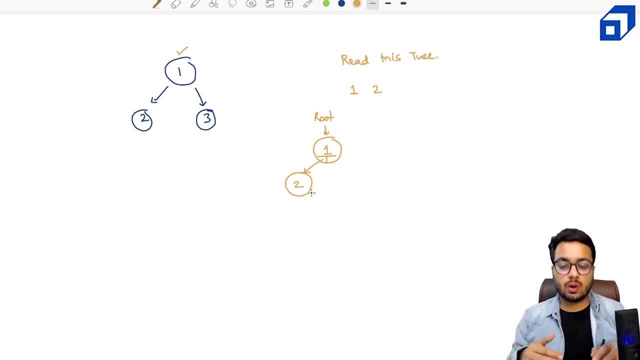 in the left of two, or i have something in the right of two, or i i have something in the right of one right. so i do not know the way we are going to do it is we are going to read now what is there in the left of two. okay, so if the left of two is null, right, i will input minus one. so minus one in. 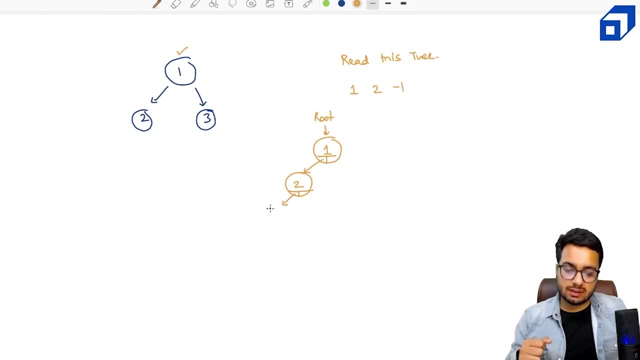 the input will denote that near is nothing here. so i will simply set this value to be null. right what is right of two, i'm again going to say it is minus one, so i will set this value to null right now. this option is gone. i've read it. this option is gone now. i can only read this. 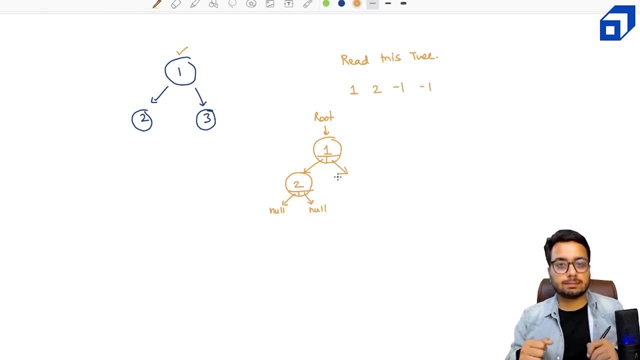 so i'll come back here i will say: fine, this two is done. now try to read what is there in the right of one right, so it's okay. the next input is three. i will create a new node and i will attach it, of course, here, but before that i will read what is in the left of three, right, so attach. 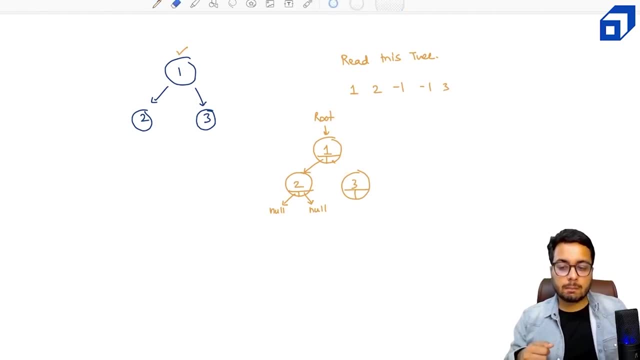 part will happen a little later. right, i'll read what is in the left of three. so this value would be minus one, minus one what is there in the right of three. again i say minus one. now this node is constructed, or in a way i can say this subtree has been constructed. 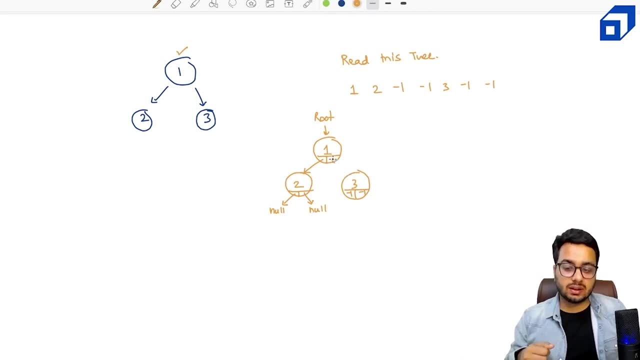 so once it is constructed, i will return it back to the parent. so the parent is one, it will get connected here, right? so this will become more clear once i write the code. the idea is: i will, of course, do it for a bigger tree as well. this is little tricky, right? so what the idea is, we are 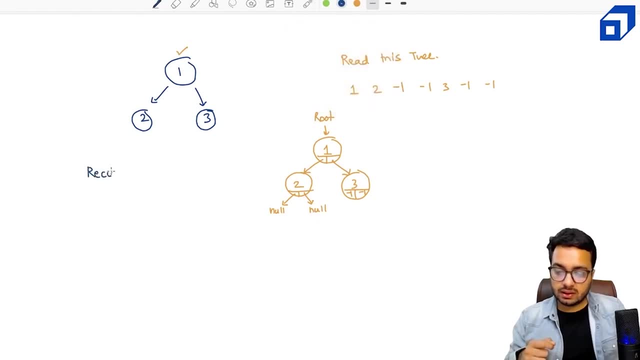 going to build a tree recursively. we are going to build recursively, right now how we are going to build a tree recursively, many tree operations. they are recursive in nature. right, that's okay. fine, i will build the root node. that is one. then i will build the complete left subtree in the above. 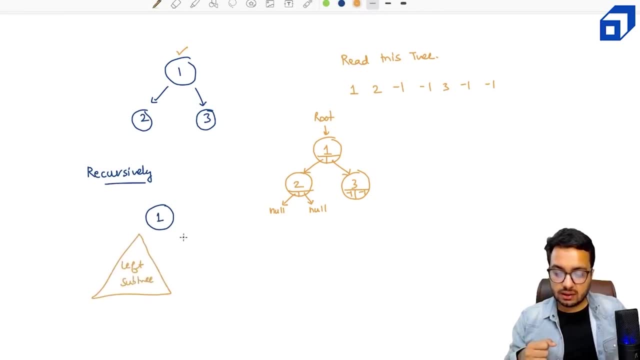 example, the left subtree has only one node, so it looks easy. right, i will build the complete right subtree, right? okay, i will build the complete left subtree and i will attach it here. one. i will build the complete right subtree and then i will attach it in the right of one. 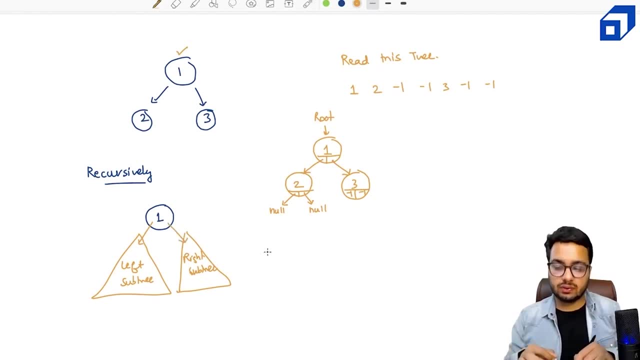 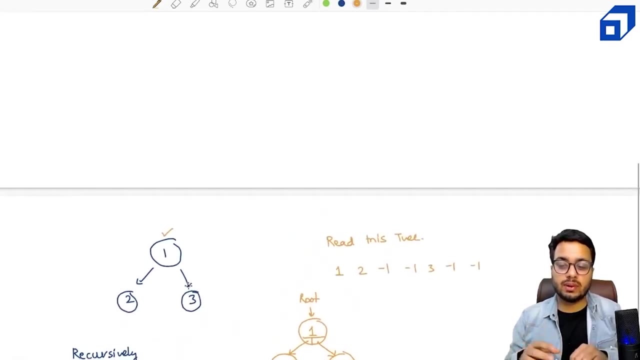 so we will do it for a bigger tree as well. so let us jump into the code first and try to see how this can be written. of course, i will do a drawing and explain you how you can build a more complicated tree like this with the same code. okay, let us go into the 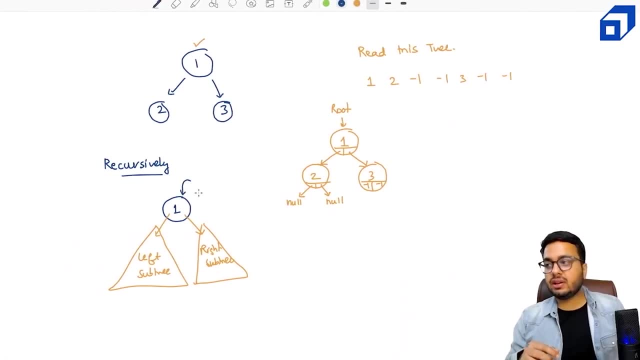 binary tree class. one thing is for sure: that every tree must know what is the root node. what is the root node. so this is something that will be the property of the tree. every tree must know what is the root node, just like in a linked list. every linked list knows. 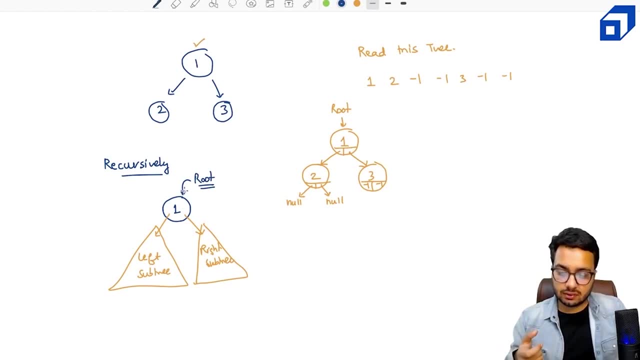 what is the head of the linked list? what is the tail of the linked list? so, in in case of three, you must know that. what is the root node, right? so one thing is there. i am going to read this tree, so user will, uh, input will come through the user, right? so let us see the tree construction part. 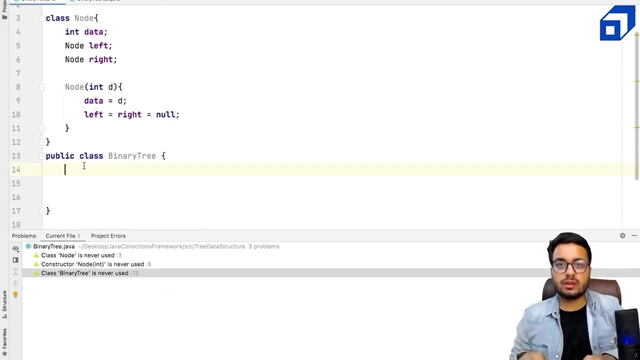 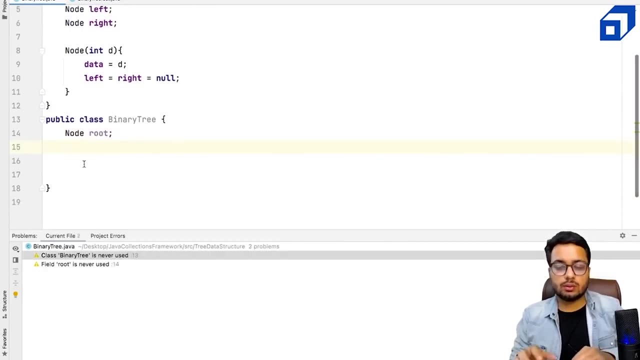 so, in this binary tree class, what i am going to do, i am going to first define the data members of the tree, so i have only one data member. that is the root of the tree. right now, this root should be initialized where it should be initialized, of course, when the tree is created. so when the tree 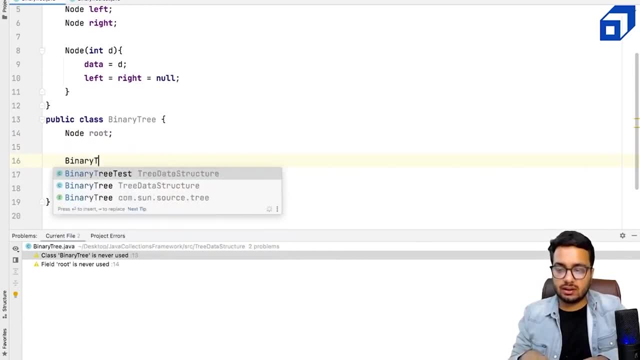 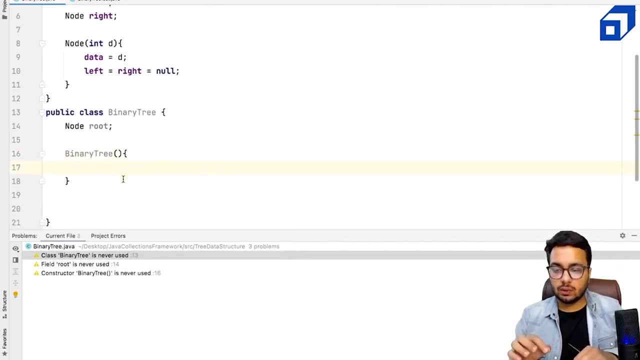 is created. it is created, then the constructor is called. i need to define a constructor called binary tree. right now, in this constructor, what i need to do? i need to take input from the user. so in order to take input, i will need a scanner object. i will say scanner se. this is equal to: 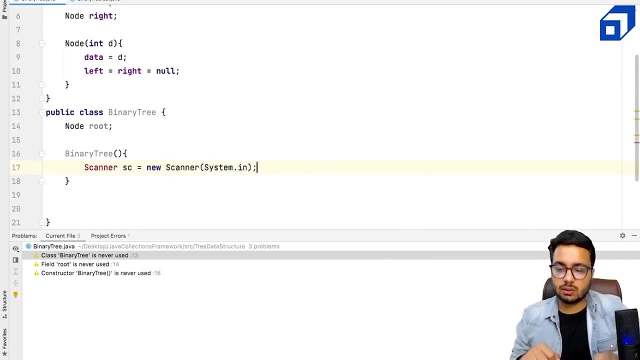 new scanner system. dot in. so scanner object is used in java to read inputs. so i have imported the scanner right now. the building of the tree is recursive in nature so i will create a helper function to do it. so i can define node. let's say, create tree and to this: 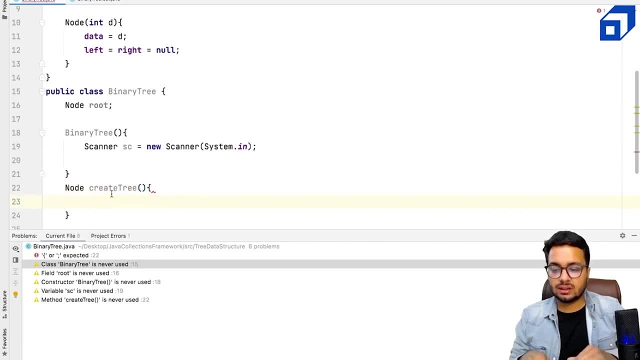 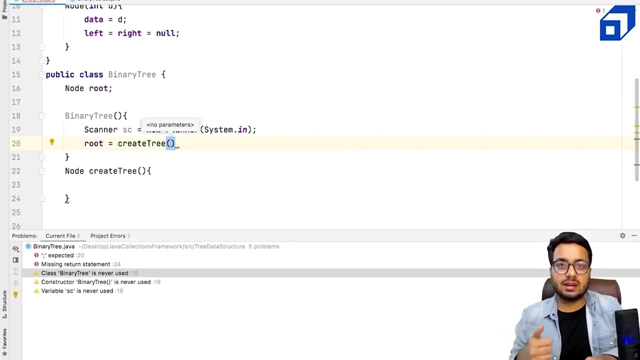 create tree method. i am going to supply the scanner object so that this method will actually read from the user. okay, i will define. the root should be initialized by calling the create tree method. so create tree is a helper method getting called in the constructor that will read the tree. 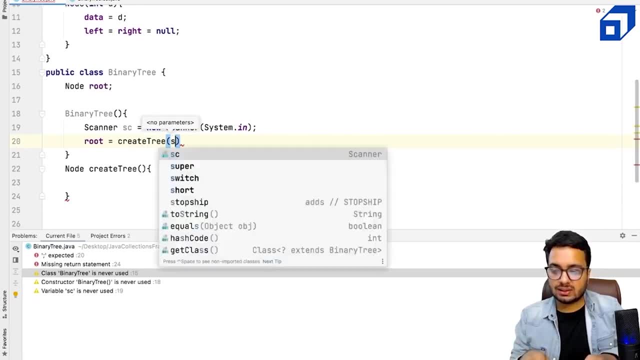 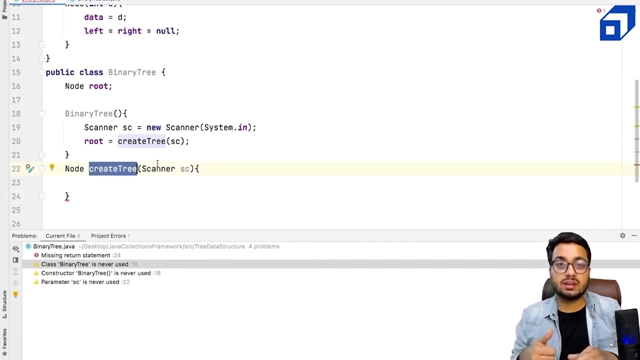 from the command line. right now, i'm going to pass the scanner object here so that i can use it to read data from the user, right? i'm no, i don't want to create this object again inside this method. okay, so i'm creating it once and that object is being circulated. 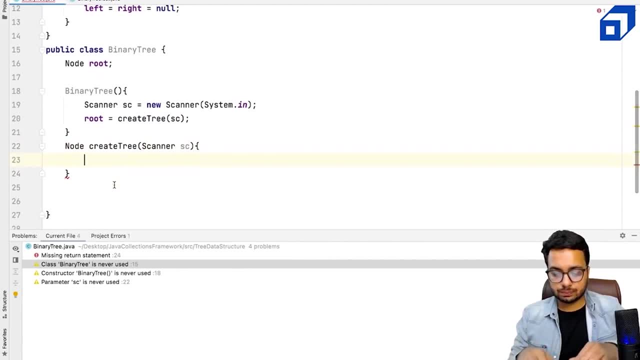 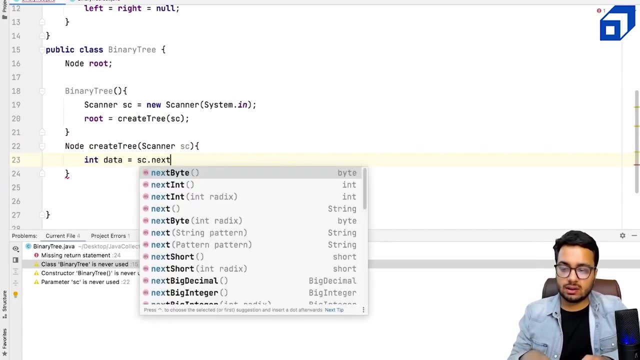 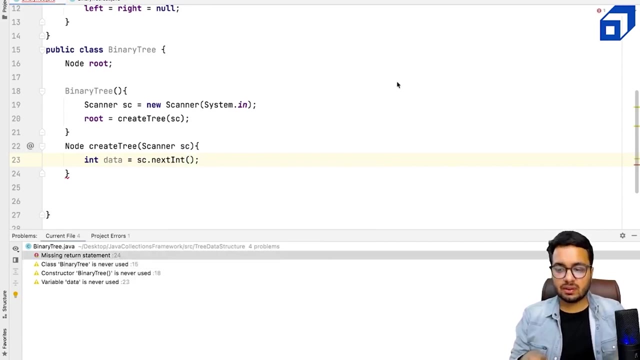 across all the recursive function calls that are going to happen right now. suppose i read something i can say, okay, uh, data that i'm going to read is scanner dot next int. so i'm going to read something. all right now i have read something from the user. let's say: this data is one right. what i want to do. 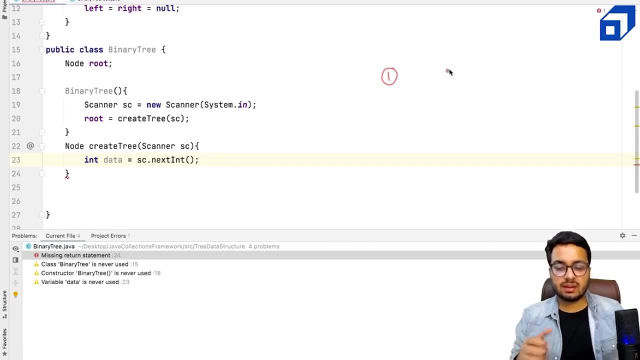 okay, this data can also be minus one, right? i'm asking: okay, tell me what is the next data? so i will actually have a two, two types of case. one will be my base case. if my data is minus one, then what should i return? i will return a null. that means okay, i don't want to attach any node here. 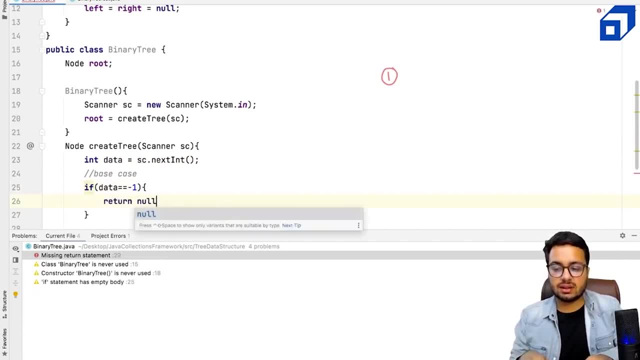 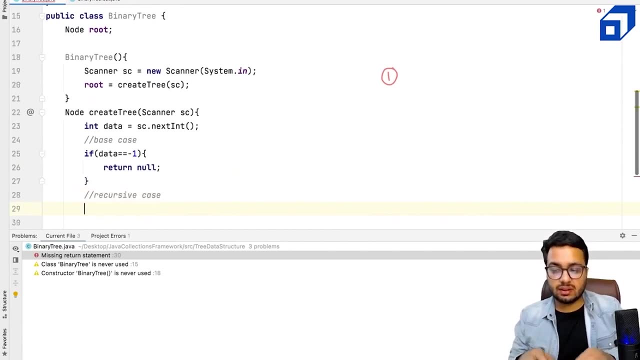 that sub trace just null. i will return null, but if it is not minus one, if it is something else- basically i'm talking about the recursive case. for example, if my input is one, what i will do? i will create a new node. i'll say: fine, i'll call a node root. this is equal to new node. 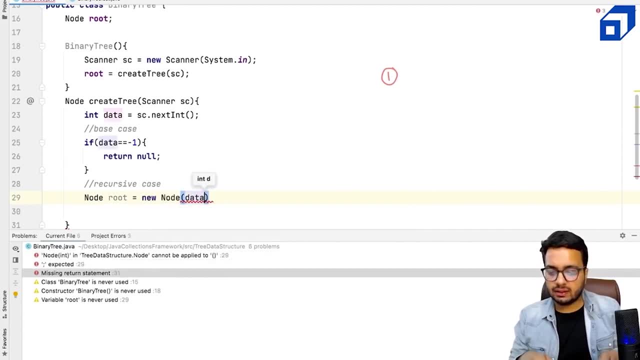 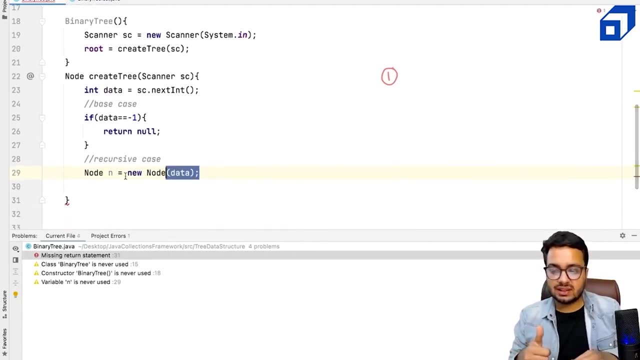 and i give it the value data, right? if root is confusing to you, just call it as n, right? i create a node called n which is initialized with this data. so suppose my input is one, right? so i say n is a new node. now what should i do? i need to read the left sub tree. basically, i need to create a left sub tree. 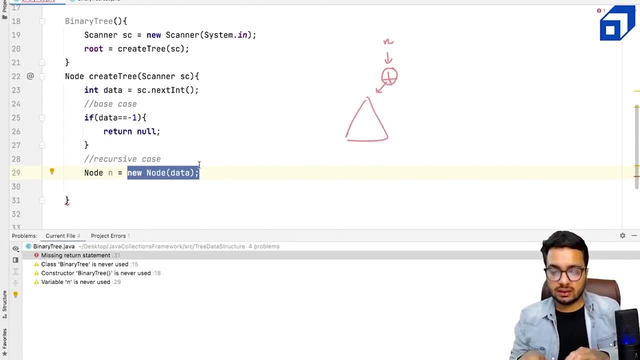 here and attach it here right. what i can say? that in the left of n, n dot left should refer to a new tree which is equal to create tree. again, scanner will get passed. what should n dot right point to? n dot right should also refer to a new tree called create. that is returned by. 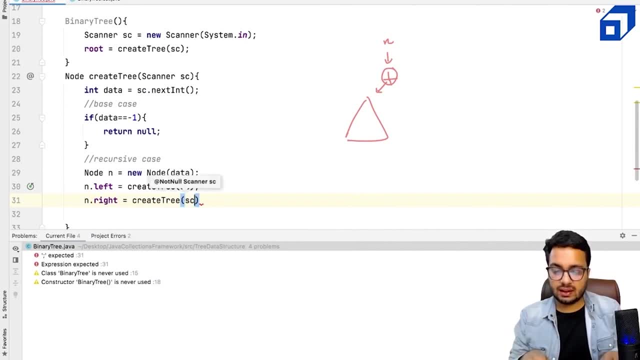 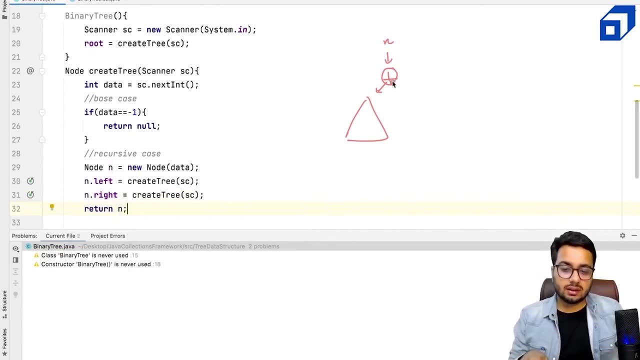 the create tree method and again, the scanner is going to get passed and then i can return what i'm saying: that n dot right should also point to a new tree: left sub tree, right sub tree. this is the recursive way of constructing the tree. now you might ask: okay, how does this method will? 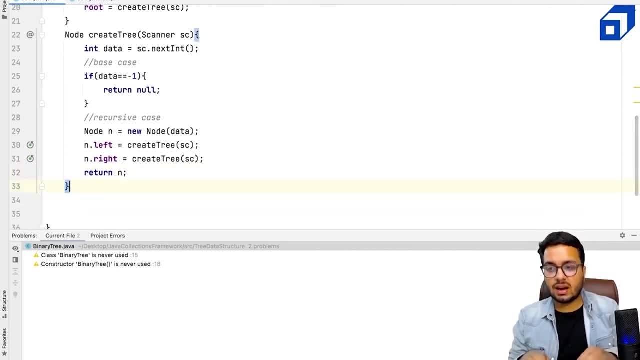 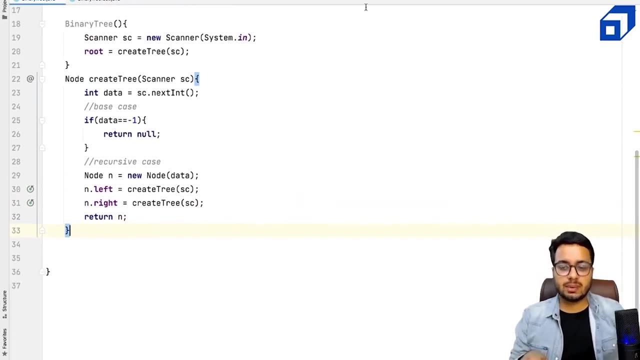 actually work. i will show you it will actually work. let's see how it's going to work, right? so let us take an example of a more complicated tree. or let's first start with a simple tree, right? let's say, i have a tree like this: one, two, three, eight. for this tree, what is my input going to look like? so input will be: 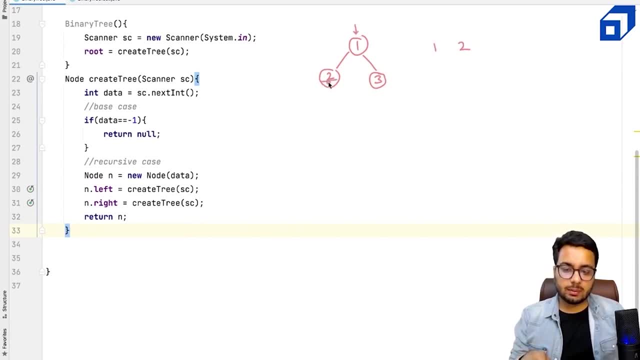 one, then it will be two, then it will be left and right of two, which is minus one minus one, then it will be three, and left and right of three, which will be minus one minus. so, given this input, i actually want to create this kind of a structure. let's see how it's going to happen, right? 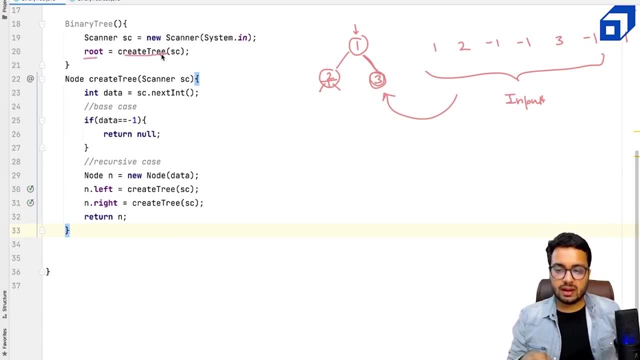 so i said, fine, uh, root is equal to create tree. i call this method create tree. it reads something from the user, so one integer it's going to read. so it's going to read one. so data is not minus one. fine, i come here node and this is equal to new node. so basically i have a stack call. 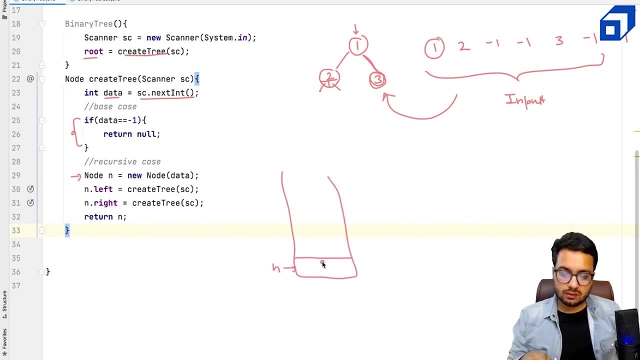 in which n is going to say n is a new node. where the data is going to be is 1. fine, now n dot left. it makes a new call: n dot left, right. so i said, fine, in the left of 1 i want to create tree. 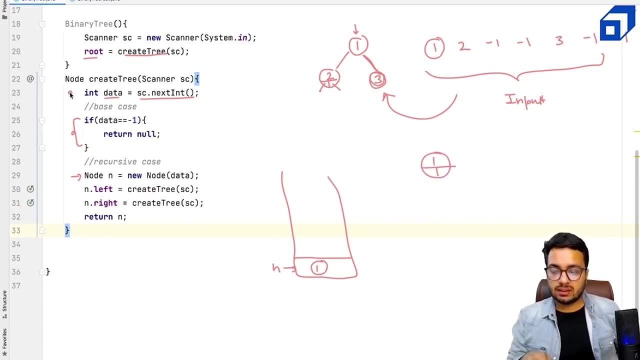 so again, create tree is called. if you come again in this function you read something from the user, so you read 2. fine, you said: fine, i create a new node n. ok, new node n is created. so earlier n was here, now the new n is here. right, it's a local variable, it is. 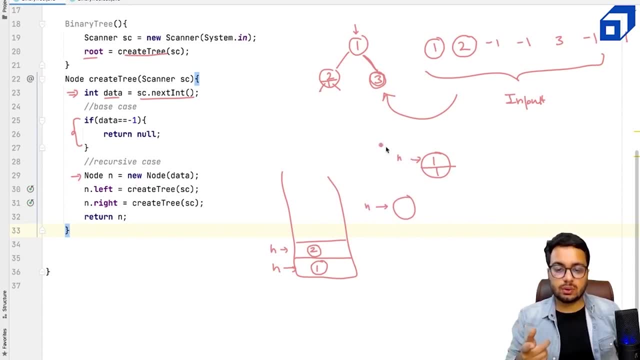 created in every stack. call, right, it is here. this is equal to new node where the data is 2. fine, now n dot left. this is equal to create tree, right. so again i call, i make a function. call create tree. go and do something right. so i've made a call for here. right now, if i 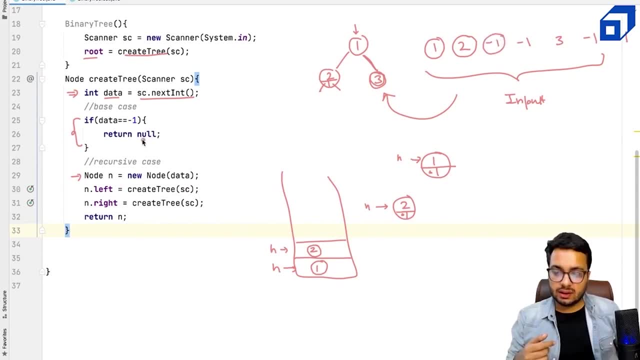 go and read what is the next number. it is minus 1, so i return null. basically, what happens? so 2's left made a call and it got a value that is null. so 2's left starts pointing to null. now what is the next call that is going to happen? we are in this stack. 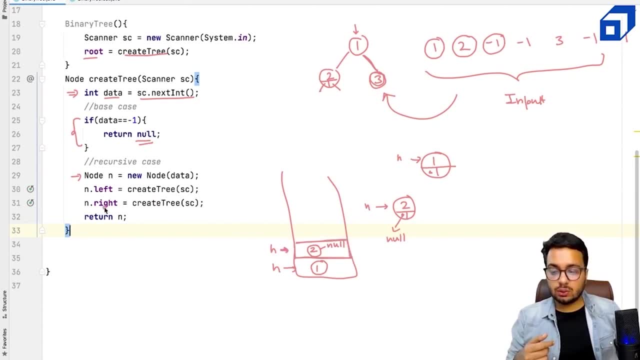 and i make a call that 2's right. this is equal to create tree. so i make another call here and this value is also null. once these two calls are over- this one and this one- i return n. so i return this n back where i return it to the place from. 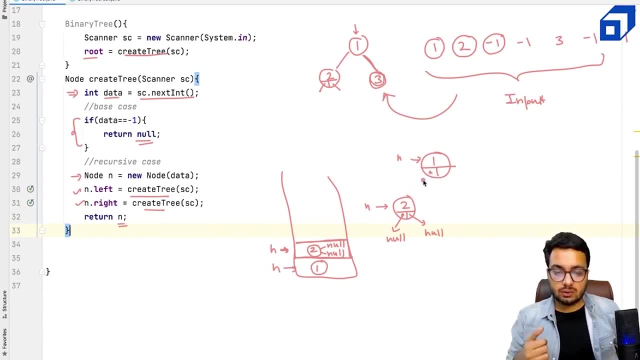 where it was called. so who called it? one called it. one gets to know that my left should refer to this node. so by returning this n, this answer goes back to the previous function. and once left is now connected with now, what is the next call we are going to make? so once left is now created, so 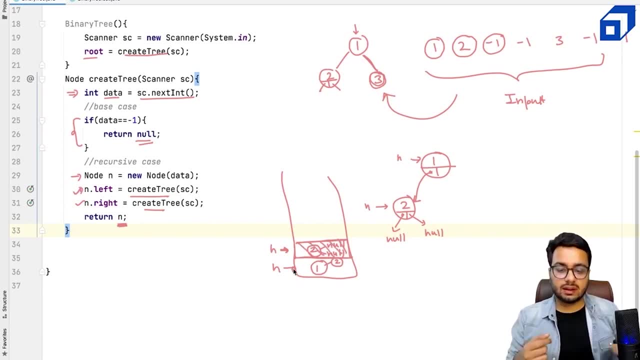 this call is over once. left is now created. right now one says, okay, fine, my left is created. i am pointing to 2. i will make a call to update my right. so n dot right. this is equal to create tree right. so this was already read. again, a new function call is made. you read the next number, that: 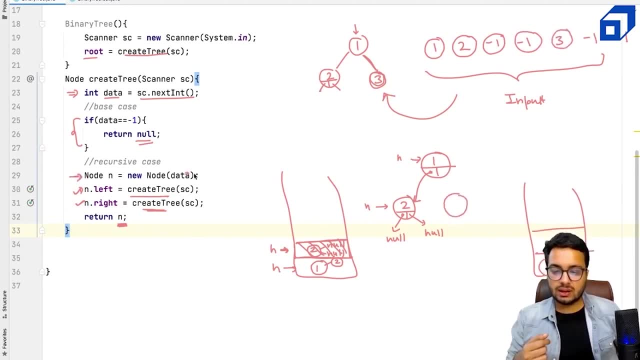 is 3. you create a new node from line number 29. you said the new node is 3, n dot left. this is equal to create tree. so 3 is left. makes a call to create tree, which again reads the data that is minus 1. so you return a null. so 3 is left. says okay, make a call. that call. 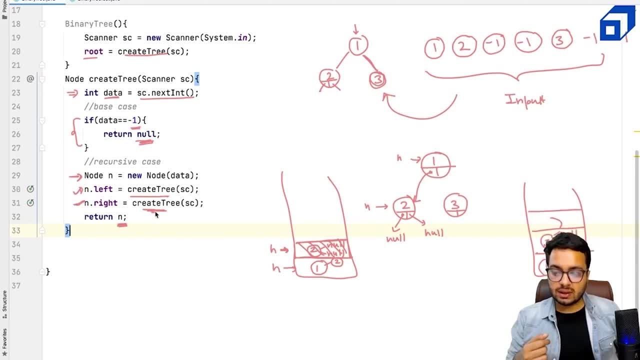 says i will return null. now 3 is right. says make a call to create tree. it goes and reads a number that is minus 1. again it returns a null right. and then you return n. now n is this right? so it returns 3 back. when you return 3 back, what happens? who called 3? so ones right. 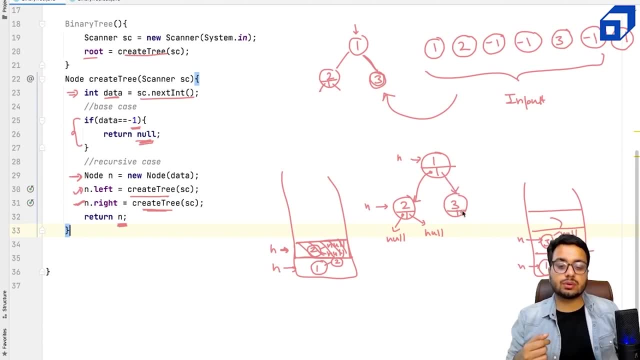 made a call to create this tree, so ones right is now going to store the address of 3, so it gets connected here from here. if you return n, where does it go? it goes back to the constructor because this made a call to create tree. finally, root is referring to the address of 1 right. 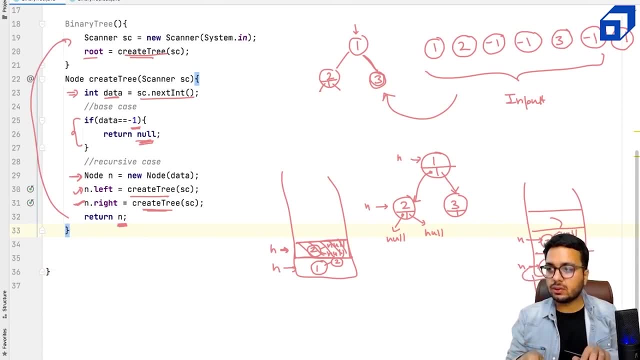 okay, i will hide myself so that you can see the root is referring to this one, right? so this is how it is happening, right? so this is a small example demonstrating that you can see how this small tree is constructed using this code. right now i will run this. 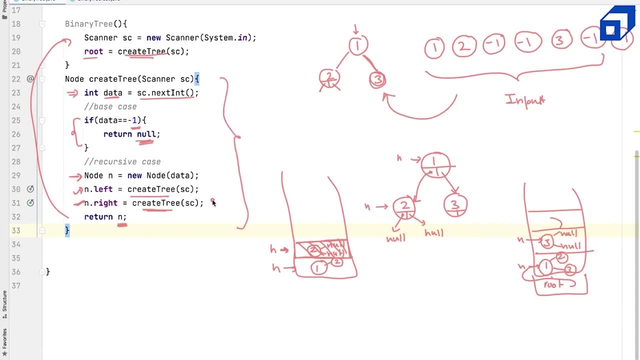 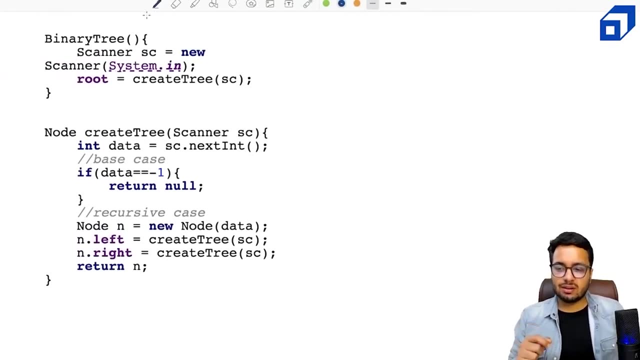 example on a. run this code on a bigger example as well. now, some of you might not be convinced that, whether this code will work for a bigger tree or not, so let us rerun this code on a bigger example. okay, so this is the method: create tree. that again, i am explaining with. 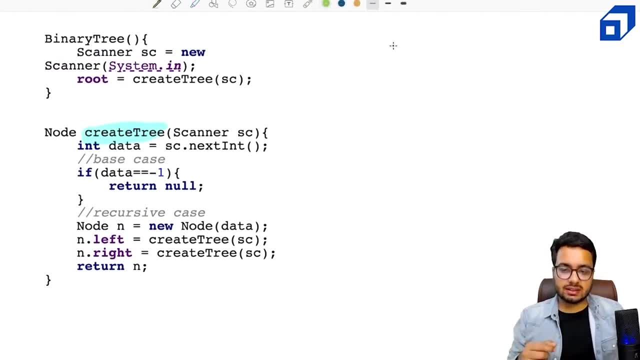 the big, big example. let's say i have a tree which is which should be built like this. let's say i have one, i have two, i have three, i have four, i have five and maybe i have six. now what input should i give? so, first of all, i will give the root node, okay, so input will be one, then i will. 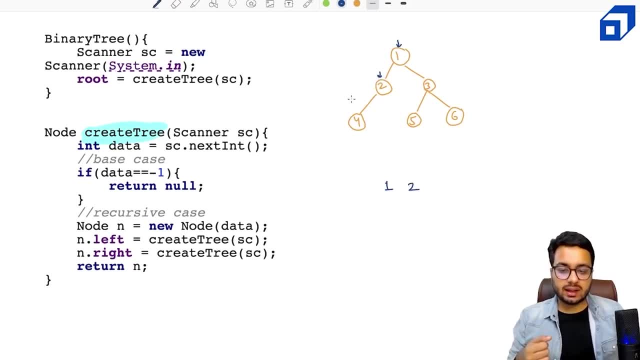 go left, input will be two. then again i will go left, input will be four. then i will go left of four, which is minus one. i will go right of four, which is also minus one. okay, then i will come back because four is done. i will come back, i will go in. 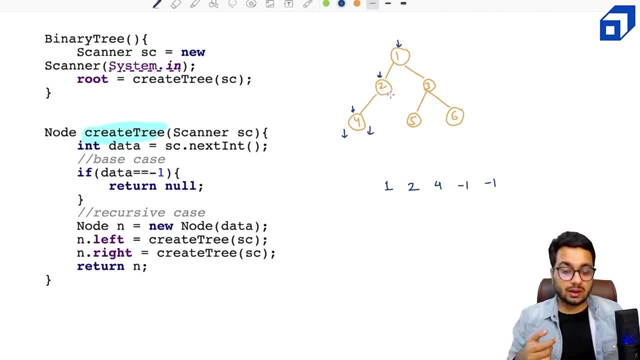 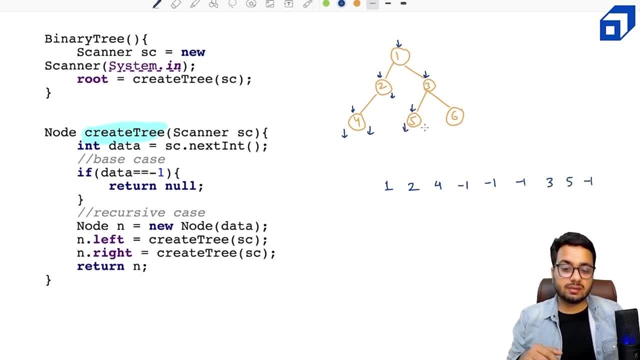 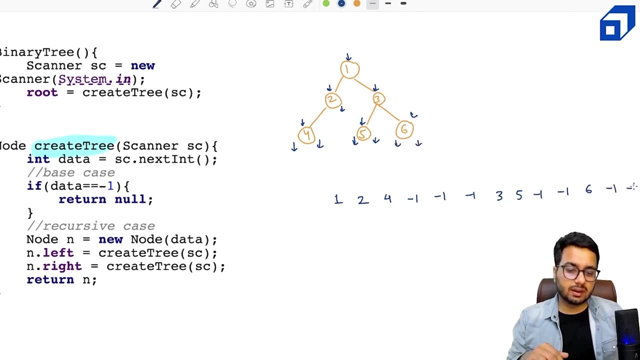 is five. i will go in the left of three, which is minus one, right of five, which is also minus one, then i will go back. i will go in the right of three, which is six, then left of six, right of six, minus one, minus one right. so the goal is given this input. 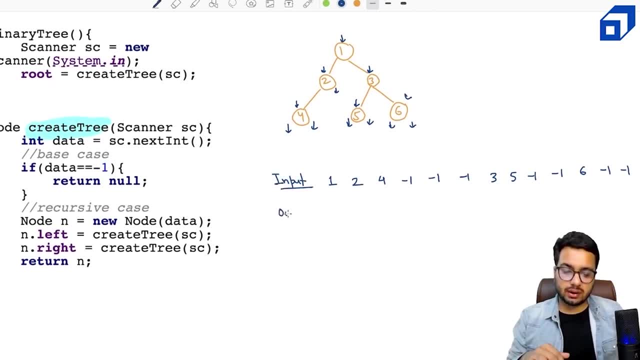 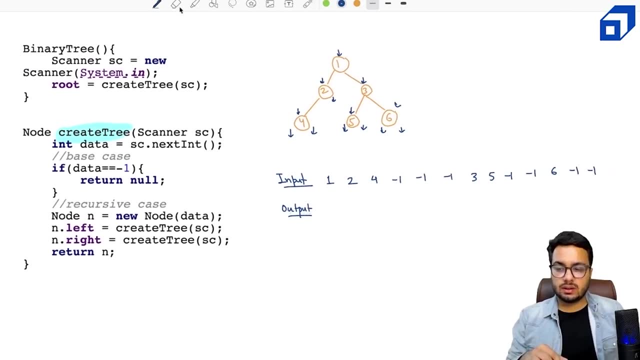 i want to create this tree structure in the output from this input. i want to create this tree structure. now let us see how we are going to do it. so again, i'm going to read some data. so i will read the first number. that is one. i will say: fine, data is equal to scanner dot. next end, it's not minus one. 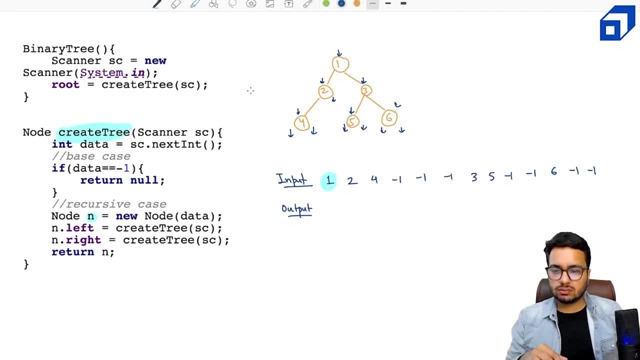 so i create a new node, n right, so fine, let's create a new node and that is having data one. let me draw the stack as well, side by side. so n is referring here right now. what? so, if you want to learn key, what is the function that is currently executing? so that is. 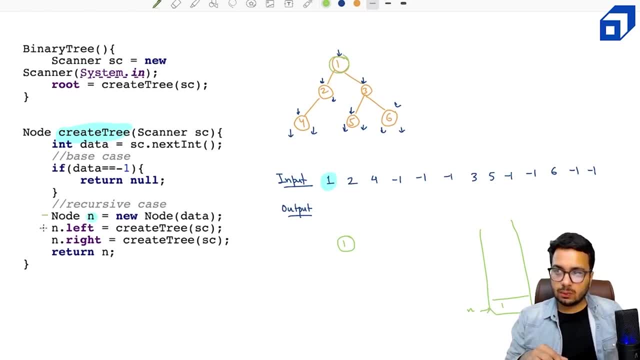 at the top of the stack, so n is created. now you make a call n dot left equal to create tree. so you are making a call to create something in the left of one right, so one makes a call for the left part. so again you go call this function. you read data, so data is the next number, that is two. 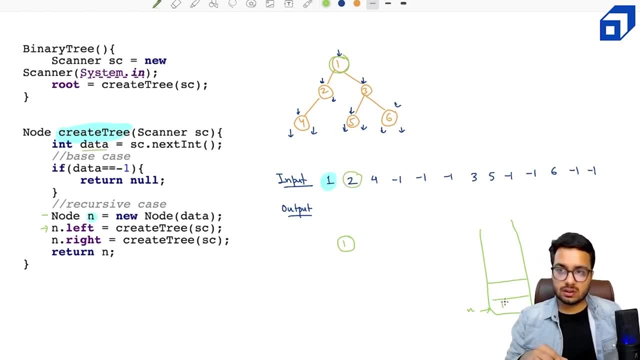 fine, you again create a new node. now this function is paused, this function is paused here. you said: fine, i'm going to create a new node and that node is two. that node is two right now it is not connected. it's not connected with one. and again you say: i want to connect something in the left of two. 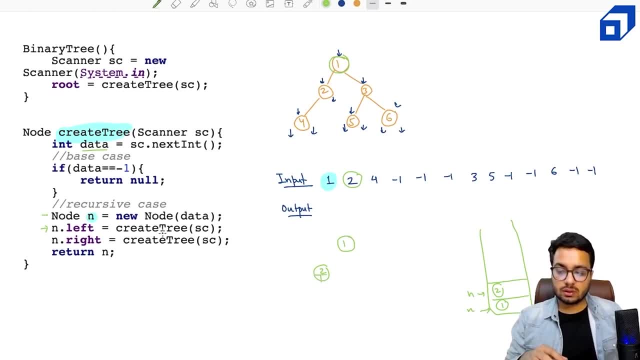 what will be that something? again you make a function called to create tree. so again this is paused and it is expecting to build its left tree. so you again call the function create tree. you read the data. so now you are going to read four, you, so you read four. 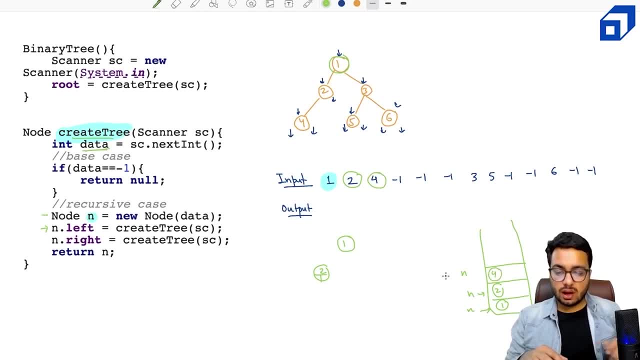 you read four. now four says: okay, i am, i am a new node and i will create something in my left. a force left makes a call to create tree. the force left again makes a call to create tree and in this case you read data. the data comes out to be minus one and if the data is minus one, you 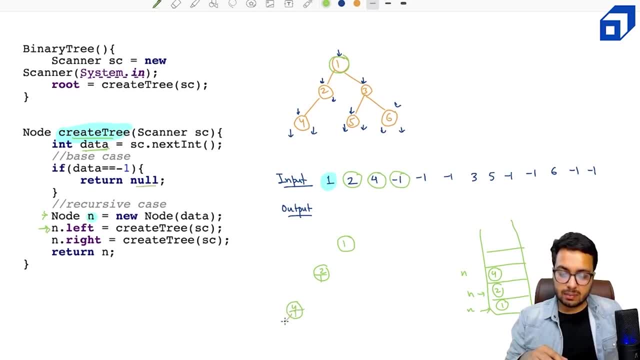 return null force. left gets to know that my value is null, so a null is returned from this function. so you read four, you read four, you read four. now four says: okay, i am, i am a new node. now four says: okay, i am, i am a new node. and this is the function which is attached with left of 4. 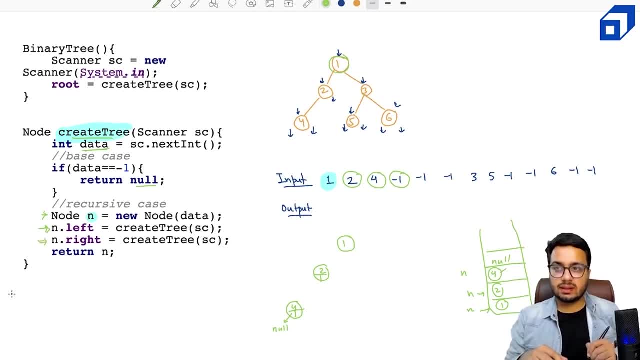 and then you hit this line for the first time in this function: call right n dot right. this is equal to create tree. now you say, okay, i will again call create tree. i will read this number. this number is again minus one. it returns a null in the right. also, force left and right. 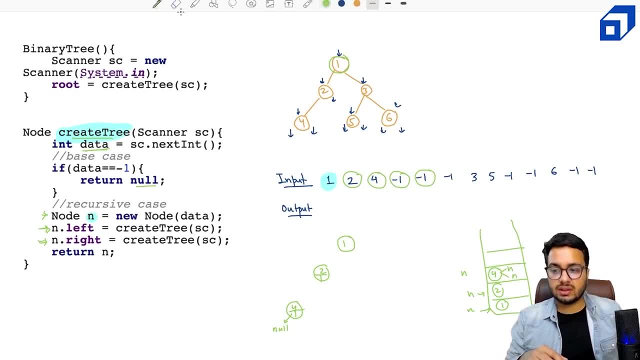 they are null. that means the subtree of four has been created. this subtree is finished. i will return n. this is null and i will return n. n is this where this return value will go. it will go back to the place from where it was called. so who called it? 2 is left. called it. so 2 is left. is now connected. 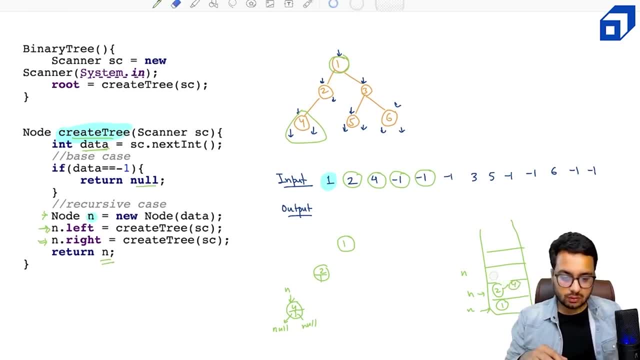 with 4 and this function call is over. right, so 2 is left, is connected with 4 right now. this is the point where this connection has been established. right so 2 made a call to 4. 4 said: okay, i will build myself, i will build my left and right, which are null, and now i will return myself. right so 2. 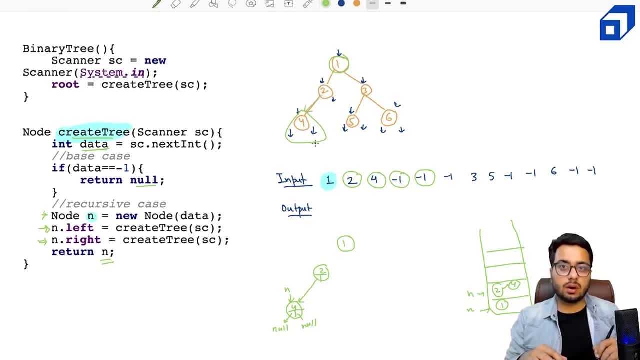 is left is over. now what will happen? 2 will make a call on the right, the right subtree. 2 makes a call here: n dot right. this is equal to create tree. now what do i read next? again, it is minus 1. so i return a null. i return a null from here. so 2 is right is null. so 2 is right is null, it's not. 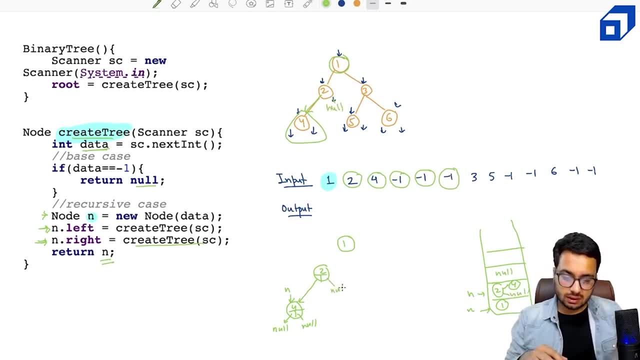 referring to anything. right, so this value is null. you now: 2 is left is done, 2 is right is done. i read. i say return n. so return n means what is the function that is at the top? at the top, i have this function. i'm going to return this subtree. 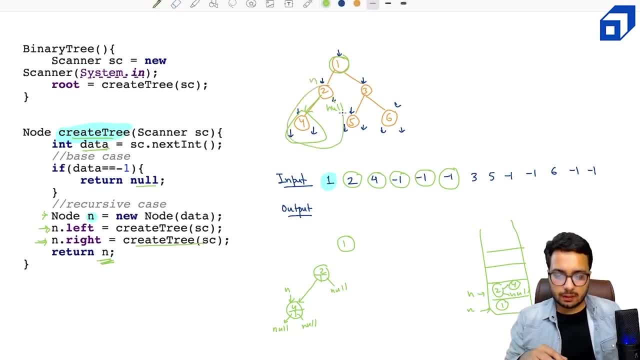 this whole subtree back to 1. so basically, 1 will get to know that my left points to this n and hence the left subtree of 1 has been built. now i will build the right subtree, right, okay. so 1 will say: okay, fine, my left subtree has been built. this is over from the call stack. 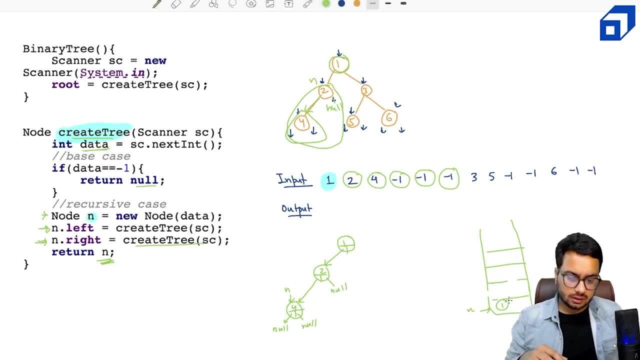 so once 1 is now connected with 2 and 4, right, this tree. 1 will say: okay, now it is my turn to call the right. so once left is done, it will execute this line: n dot right. this is equal to create tree. now you again make a call. next number you read is 3. so you create a new node called n. this is the. 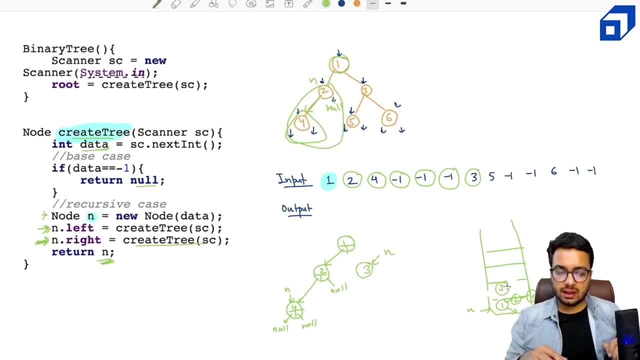 new node, so 3 is created. and then you again make a call to the left so you read a number: 5 is created. this is new node. then you again make a call to the left minus 1, so 5's left is null. again you make a call. 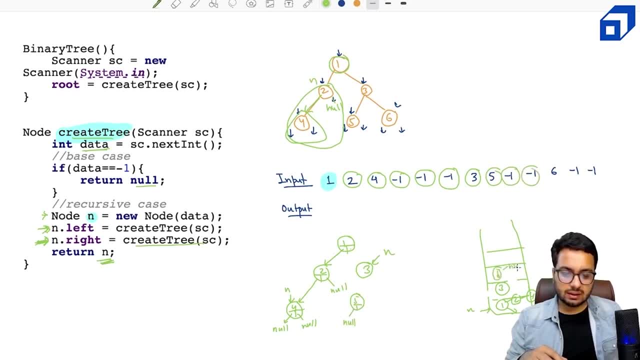 on the right, so 5's left is null. again you read minus 1, so 5's right is also null. then you return n, so you return 5. so 5 gets attached in the left of 3.. so 5 is returned. it gets attached in the left of 3, so 5 goes here. then again, what's going to happen? 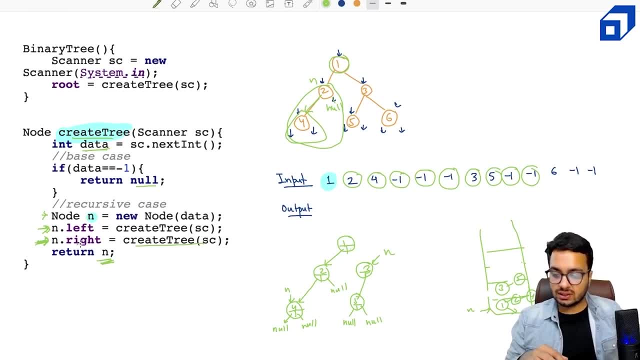 you will say: okay, i want to build something on the right of 3.. so 3's left is done, 3's right's done. so i'll again make a call. it will read 6. a new node will be created. 6, okay. and again you say: 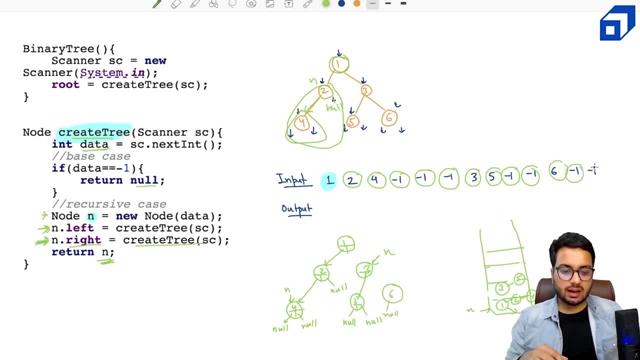 okay, i will read the left, which is minus 1, i'll read the right, which is also minus 1, and then i will return n. when you return n, this 6 is returned back to the right of 3.. so this 6 is being attached here and then you say, okay, i'm going to return. 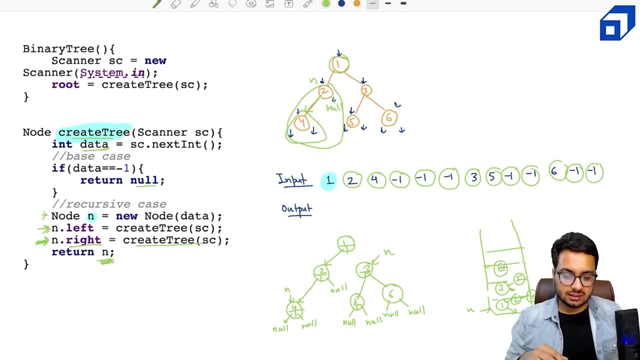 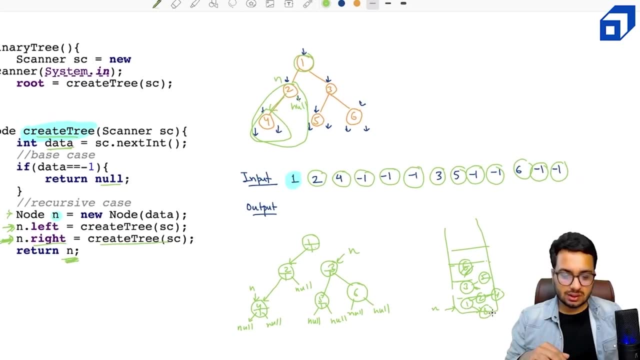 n. so when you return n, you return this 3 back to 1.. so once once right is going to point to this sub 3, 3, 5, and this subtree is attached with one. so finally we'll, when you are here, this call is over, right, so you will return n, so n will be this node, and it is. 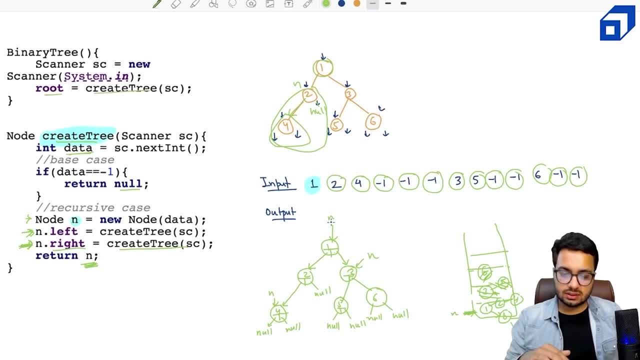 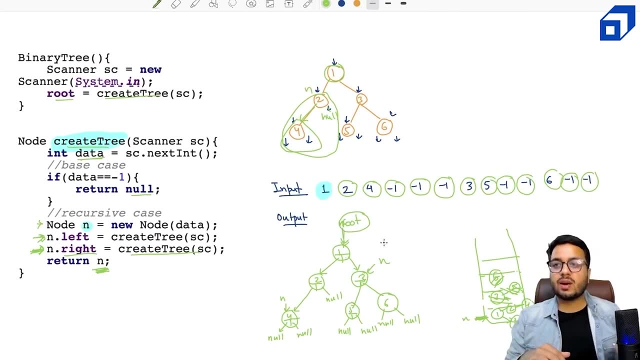 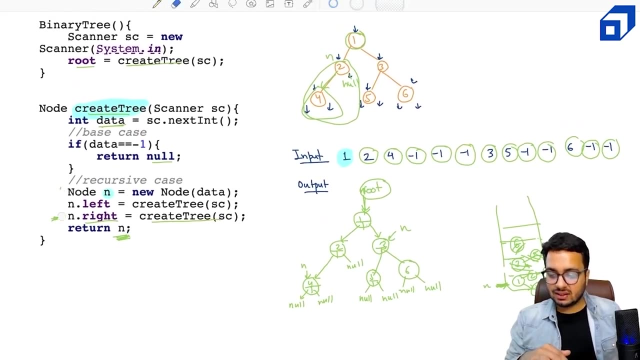 returned back here. root equal to create tree- this- this becomes the root of the tree, so root is a data member of the class and hence root of the tree gets updated. i hope you are now convinced that how this structure can be made so easily with this recursive function. okay, with this. 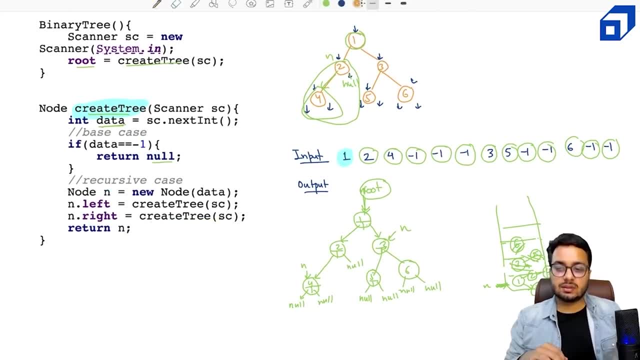 recursive function. okay, now this way of building the tree. it is called as pre-order. right pre-order means: first we are building the root node, then we are building the left sub tree, and then we are building the right sub tree, then we are building the right sub tree. right now we have 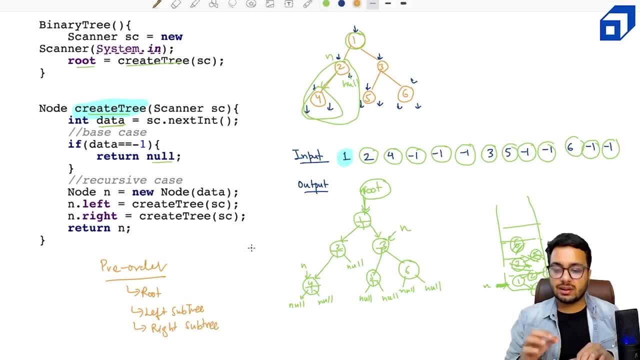 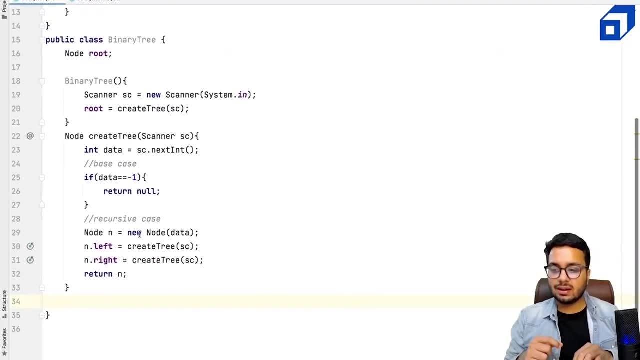 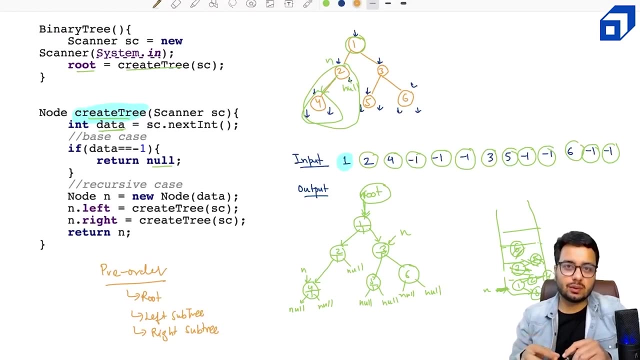 built the tree using a pre-order recursive. build tree function right or create tree function okay, right. next we will look at how we can print this tree in a similar way. now let us talk about tree traversals. okay, so tree traversal is a way to iterate over all the nodes of the tree, right? 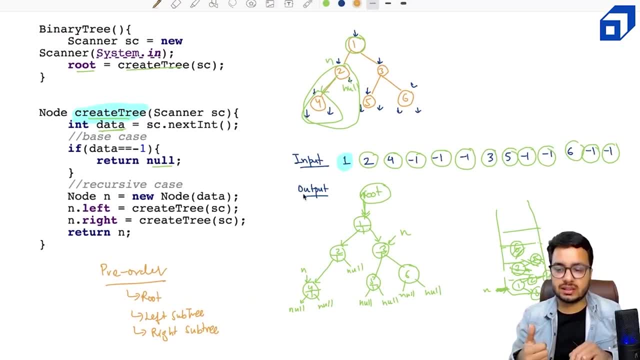 now, this traversal can be helpful if you want to perform operations like counting the number of nodes, searching for a given node, updating a given node right. so in order to do all these operations, we must know how to traverse a given tree right. so a tree has been built, a tree has been created. 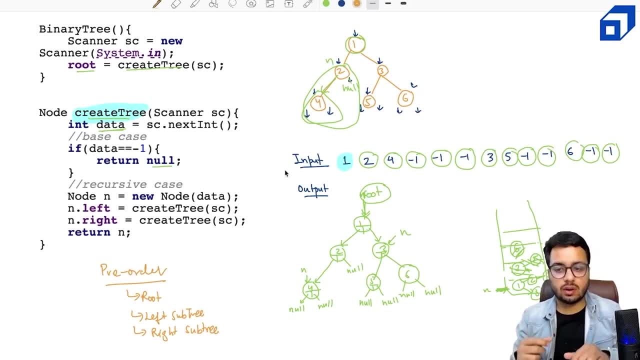 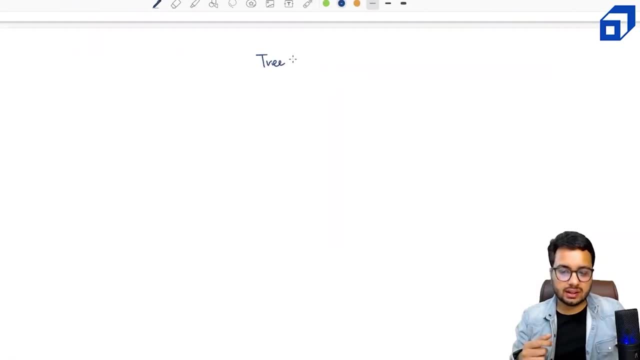 we want to do all these operations, we must know how to do all these operations. we must know how to. we want a way to go to each and every node of the tree, right? so, as i discussed, if you want to do a tree traversal, there are two broad techniques, right so, tree traversal, one is your recursive. 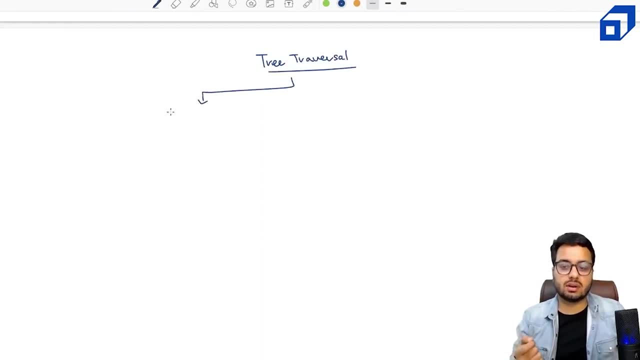 technique that, okay, you start with the root node, then you iterate recursively on the left tree and the right tree, right. there is a recursive way of doing it, there is a iterative way of doing it. so we will discuss all these ways. now right, then recursive way. again, there are, it depends upon the ordering. okay, the way is same. we basically 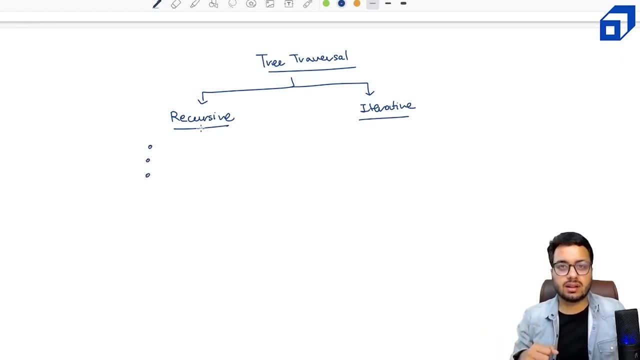 recursively iterate on the left and right sub trees, but based upon ordering. there are three different ways. one is called as pre-order reversal, one is called as in order traversal and one is called as post order reversal. we will be looking at all of them in iterative. there is only one way, that is called as level order reversal. 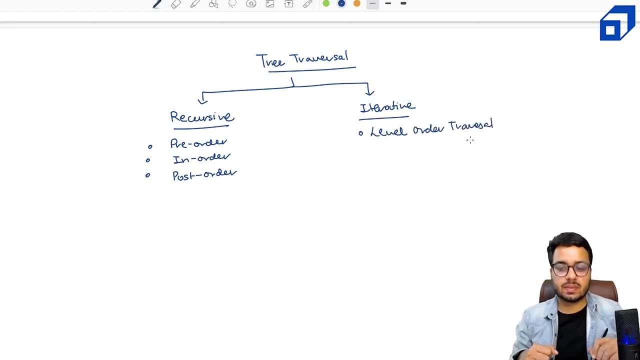 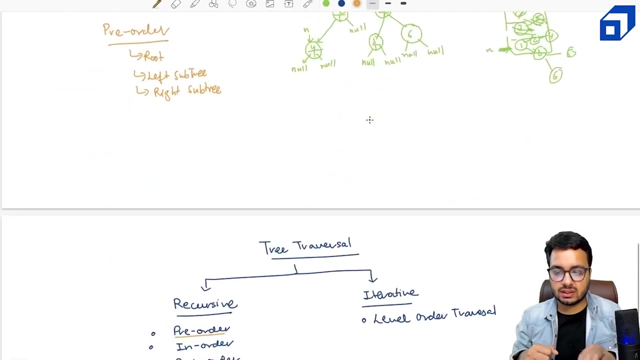 right. so all of these traversals, they are going to travel all the nodes, but the order in which you will see the output it will be different. so let us start with the pre-ordered reversal. given this, as the tree right one, two, three, four, five, six, I will just redraw this tree. 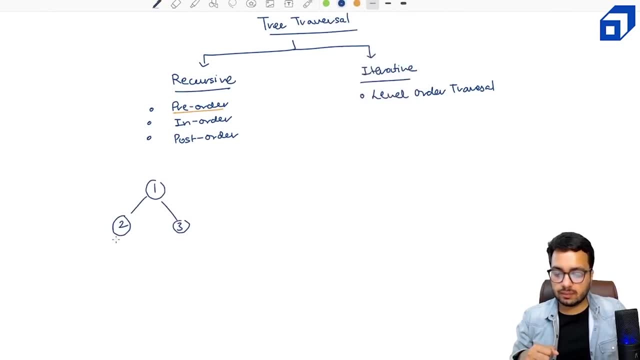 one, two, three, four, five. what is this? pre-ordered reversal says that? fine, what I will do? I will travel the root node, then I will recursively traverse the left subtree- okay, this will be a recursive call- and I will recursively travel the right subtree- again a recursive call. okay, it is very similar to the build function. what we 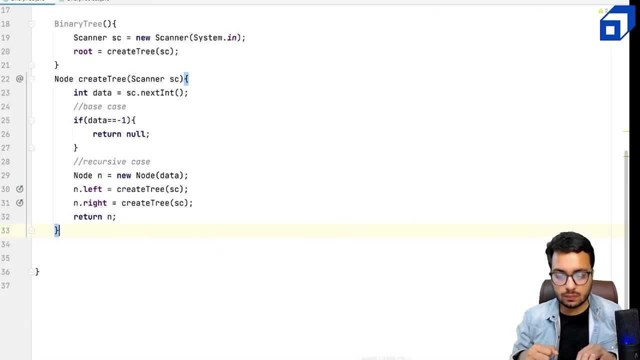 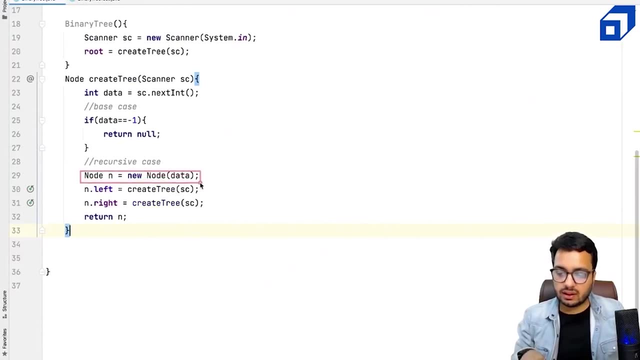 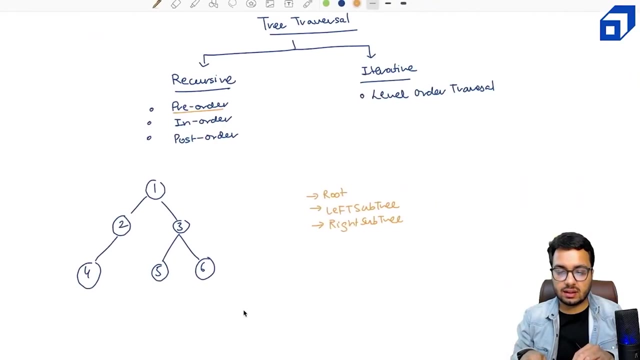 are doing in the build function. also, if you look carefully, we are for first building the root node and then we are recursively building the left tree and then we are recursively building the right tree, right, if you see, in this case the output will be very similar to the order in which you have built the tree. so if you start, 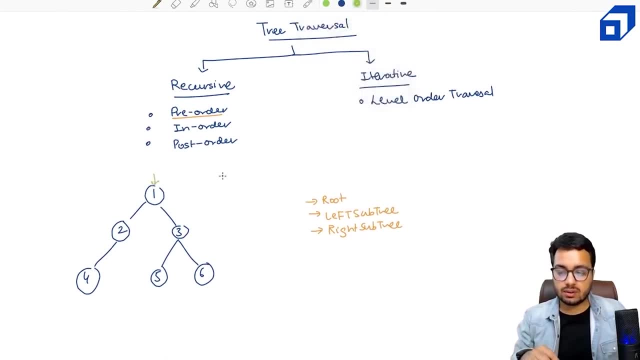 traversing you will define. I will start with the root node, I will print one, I will go to the left subtree, so this whole is my left subtree. so I will print the root node, that is two, and then I will go to the left sub tree. So left of 2 is 4.. I will print 4 and I will go to the left. Now left. 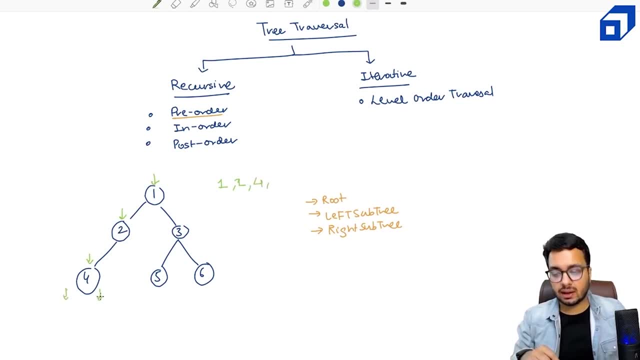 is null, So I come back. I will go to the right. Right is null, I come back. 4 is done. This whole tree has been printed, So I come back to 2.. I will go to the right of 2.. Again, it is null. I will. 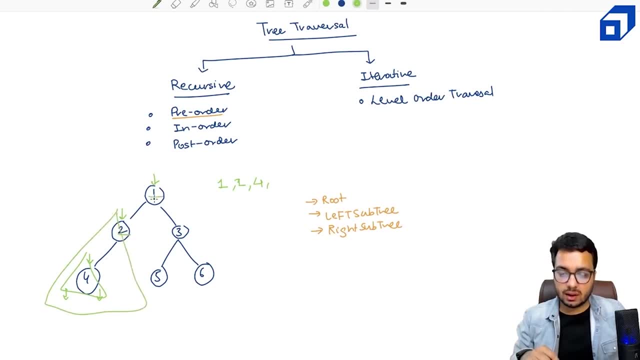 come back. So this whole tree has been printed. I go back Now. left of 1 has been printed, So I go to the right of 1.. So I come to 3.. I will print 3.. I will go left Now. I will print 5.. I will go. 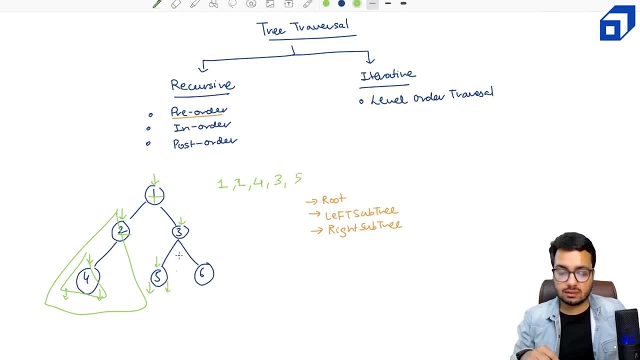 left. I will print right of 5.. Again null. So 5 is done. So this whole tree has been printed. I will go back, So at 3, else okay, Let's go right, I will print 6.. I will go left. I will go right, Nothing. 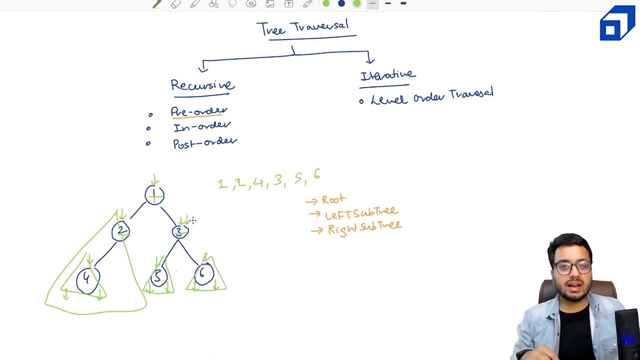 happens. This whole tree has been printed. I come back Now. 3 has been printed, So root has been done. Left of 3 has been done. Right of 3 has been done, Well written, So this whole tree has been printed. 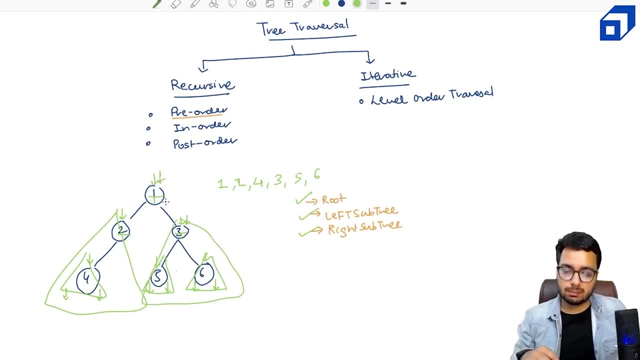 I come back and at 1 I see 1 has been printed already, because before printing left and right, I print 1.. This output is called as pre-order output, in which before printing left and right nodes, I print the root node Right. So 1,, 2,, 4,, 3, 5, 6.. This will be the pre-order. 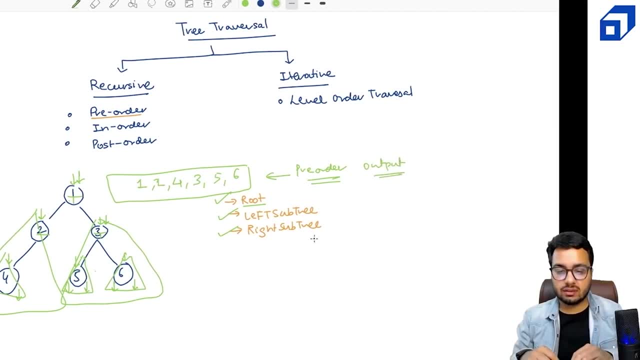 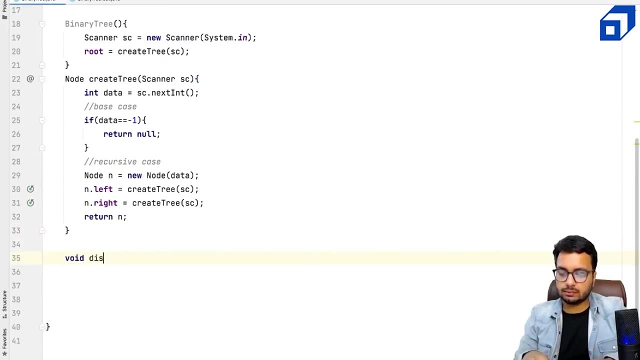 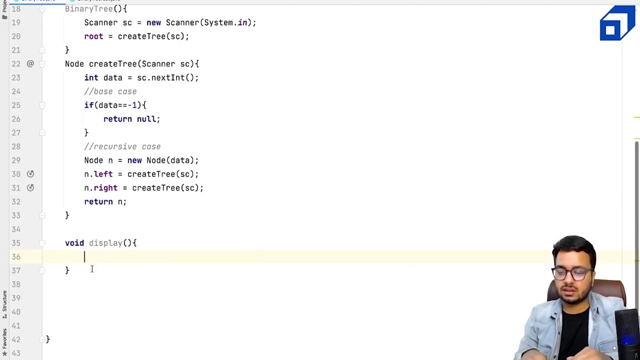 output for this tree Right Now. let us see this thing in our code as well. Let's write a pre-order print method, Let's write a method called void display, And this is going to be the method that will display the tree Right. So inside this logic can be changed. I can display a tree in a pre-order. 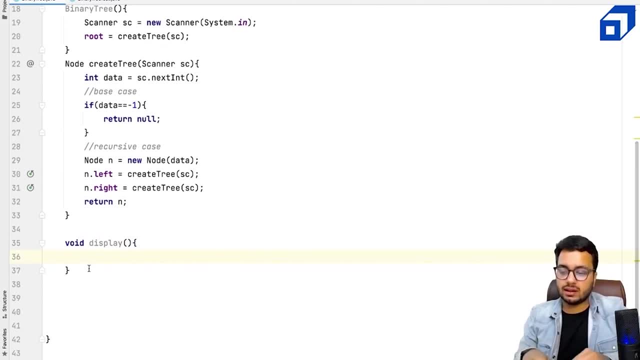 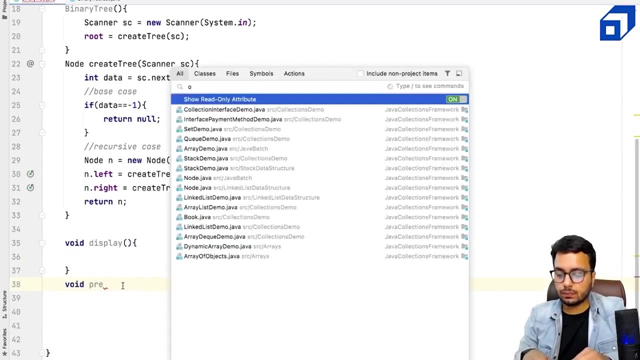 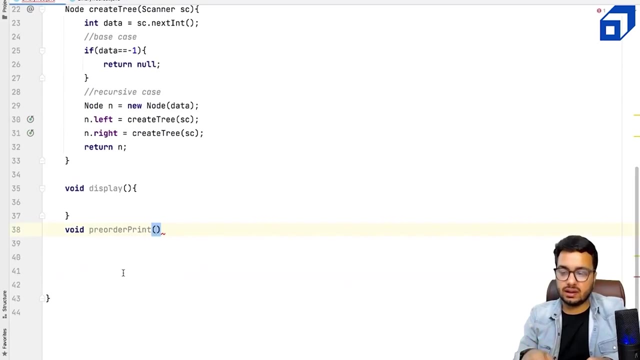 way or in a level order way or any other way, Right? So I will again create one more helper method. So I will say void pre-order. So void pre-order print. Now this is a recursive function, So I have to tell at what node I'm currently at. So I will start with the sum node, that is, root node. Okay, 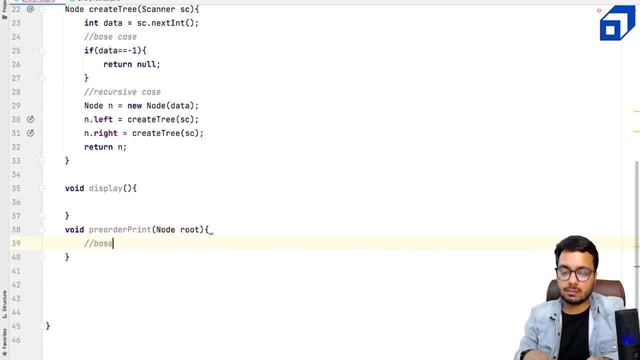 So what I will do? I'll say, fine, I will have a base case. What will be my base case? What is the smallest tree I can get that? the tree is null, the root is null. In that case, I don't need to. 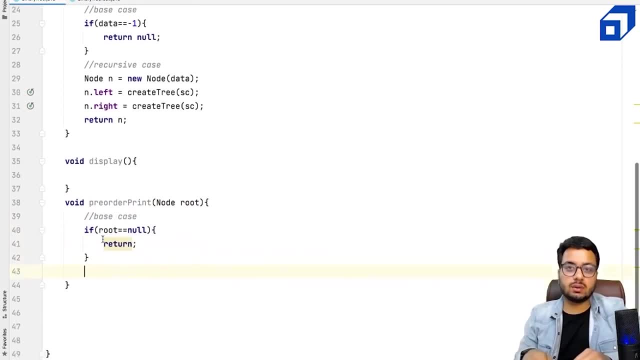 print anything. I will simply return. Otherwise what I will do: I'll print the root data And I will go back and print the root data. And I will go back and print the root data And I will go on the left and the right tree. So I will say: fine s out root dot data. Go and print the left. 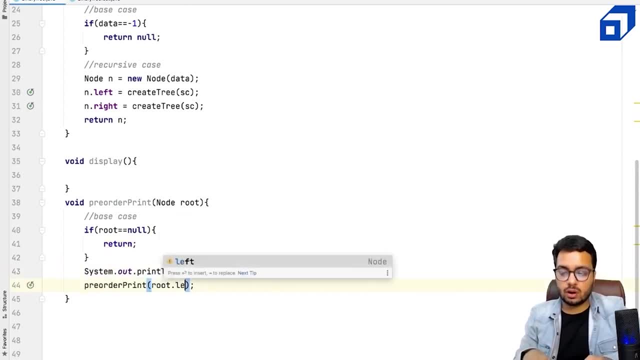 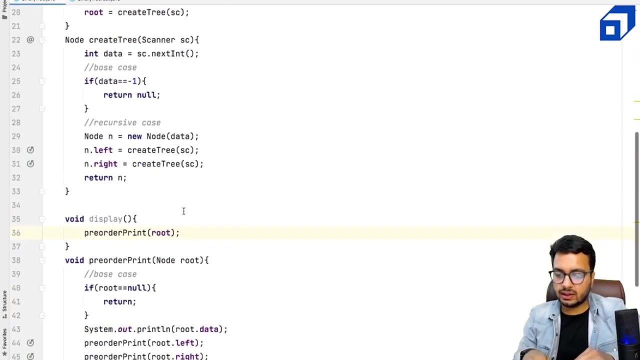 sub-tree recursively. So pre-order print- root dot left, then pre-order print- root dot right. That's it, And in the display method I can call pre-order print with the root of the. Now let's do one thing. Let us test our binary. 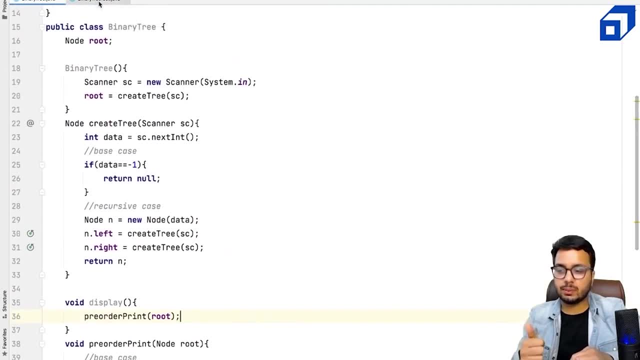 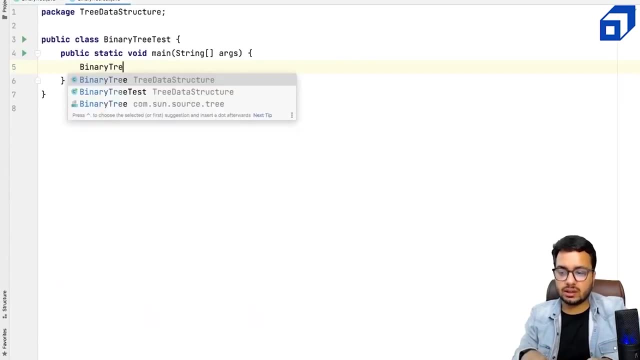 tree Because we have the create method. we have the print method. Now I can create a binary tree and try to print it. I can define: I want to create a binary tree object. This is equal to new binary tree. I have defined the class. Now, as soon as this constructor is. 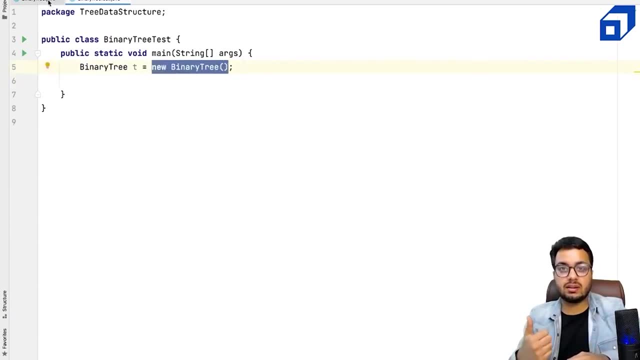 called your tree will start getting built because we call the create tree method here. right Now I can call tree dot display. Now think of any tree that you want to make. we will give it as an input here. Sorry, I should run this file. 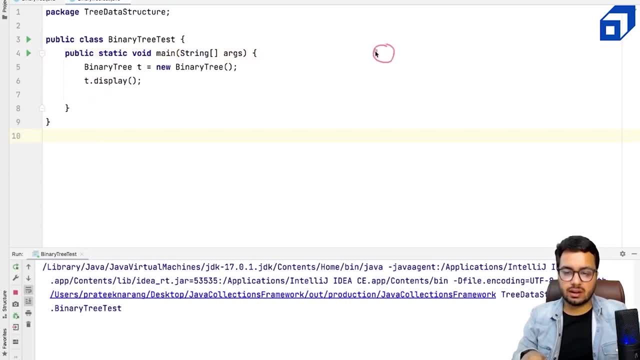 Now this is waiting for the input, right? So let me draw a tree. let's say tree is 123456.. Now how this tree will be given as input. So you will input one, then two, then four, then left. 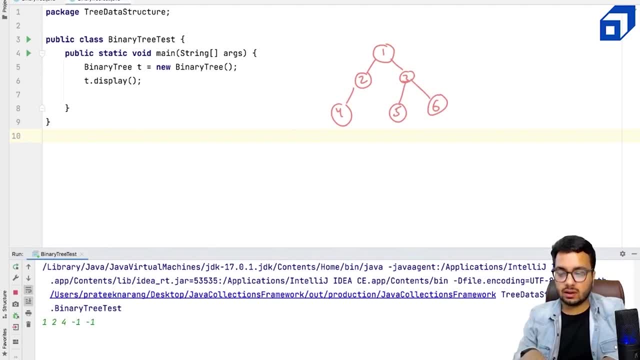 of four minus one, right of four minus one, right of two minus one, then three. then you will input five, left of five, right of five, right of six, right of three, that is, six left of six and right of six. Okay, the same input that I have shown you in the example. also, This input is: 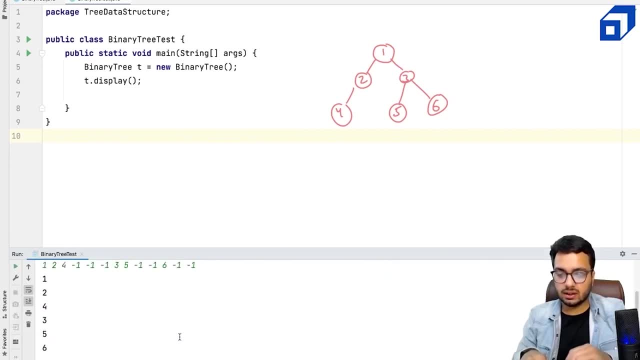 given, And now I'm saying that let me print this tree. What I'm getting? I'm printing one, I go here, then I go to two. fine, then I go to four. fine, then I go to three, I come back, I come back. 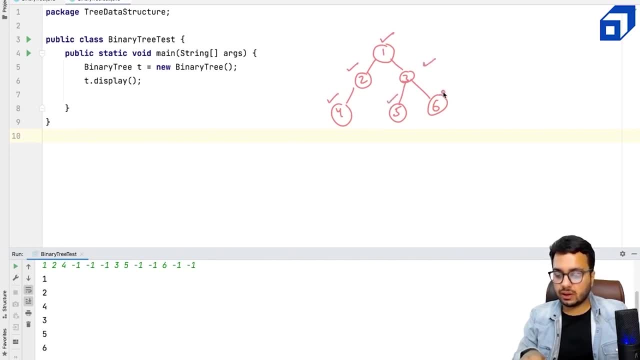 I go here, yes, And I go here five, and I go here six. Absolutely correct, right? So if you look at, this was a pre order build, right? And this is actually a pre order print. If you see the output. 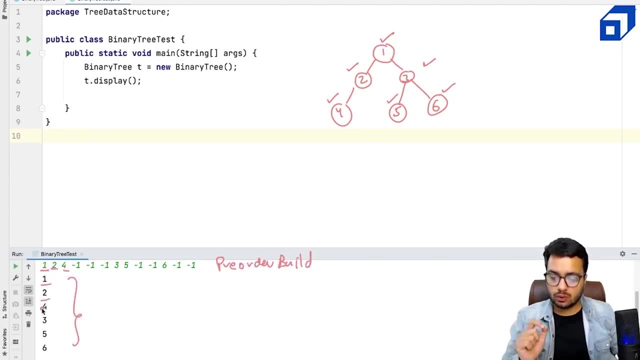 will be exactly same: 112244 minus one. I'm not printing skip, skip, skip. then three, five, three, five, absolutely correct, minus one. I'm not printing Six, six, right, That means my both functions are working fine: trees getting built correctly and trees also getting 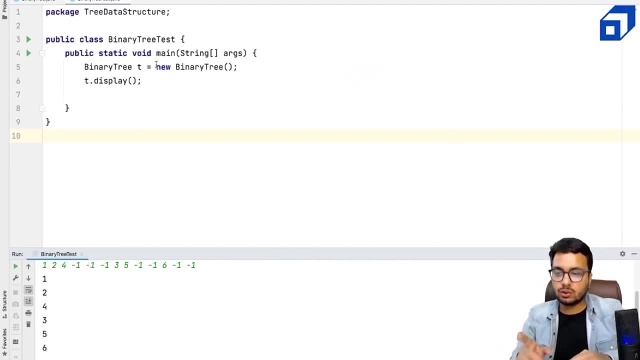 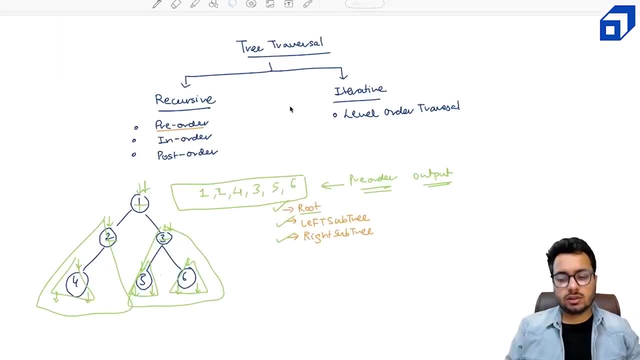 printed correctly as well. Right Now I will show you two more variations of this print method that is called in order print and post order print. Now let us discuss the next type of recursive printing that we call as in order print. Okay, I hope pre order is clear. Now we are moving. 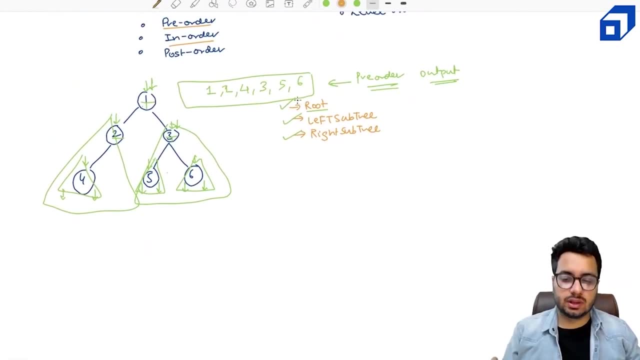 so nothing is going to change. the order of printing is going to change. okay, so earlier it was root, left subtree and right subtree. now what we are going to do in order means root will be printed in between. so before you print the root, you will print the left. 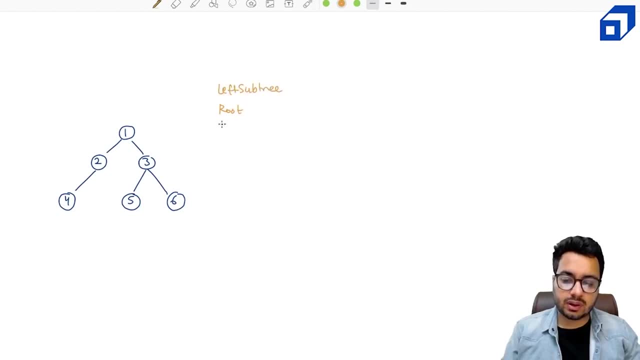 subtree, okay, and after you print the root, you will print the right subtree. that is what the in order printing would mean. let us dry run this logic on our code and see what do we get in order, what I want to do. so I will start from the root node. I want to print this: 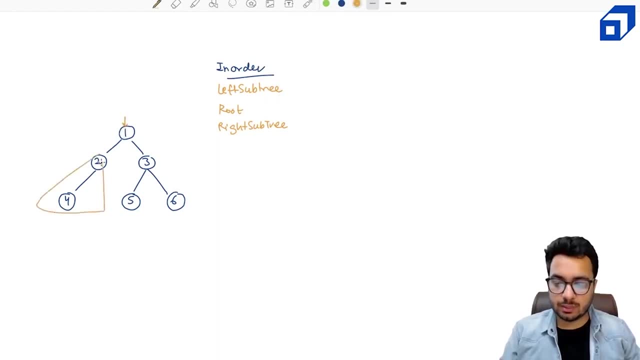 root node. but before that I will have to print the left subtree right now. at the left subtree again, if I am at 2, I have to print the left subtree. so that means I will have to print 4.. So I have to print the left subtree now. 4 will be the first output that I will get now. 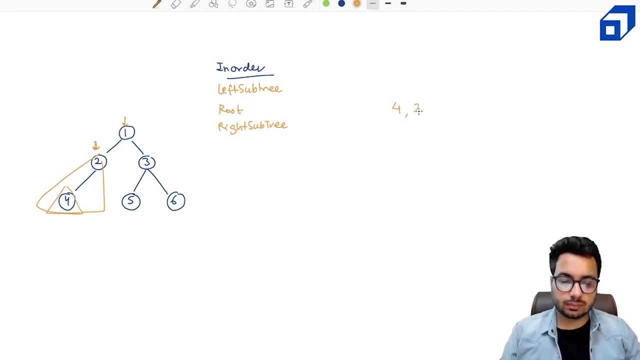 I will print the root. so what is the root? the root is 2. alright, then I will print the right subtree. so right, subtree of 2 is null. right, then I can go back to 1. so for 1 I have seen the left subtree is already printed. then I can print the root. so I will print 1 and 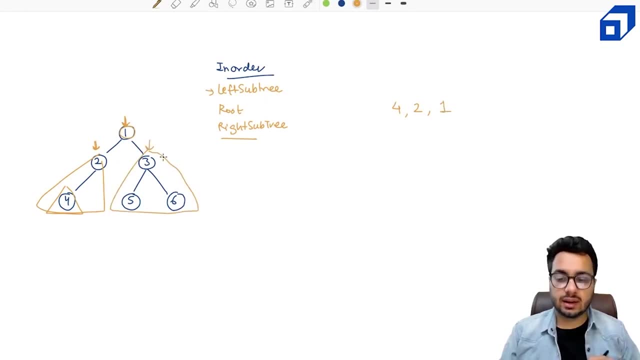 then I will print the right subtree. now I am at 3, right. before I print 3, I will have to print the left subtree. only one node. i will print five, then i can print the root node, that is three. then i can print the right subtree. that is six, right, this will be the output we can expect by traversing this. 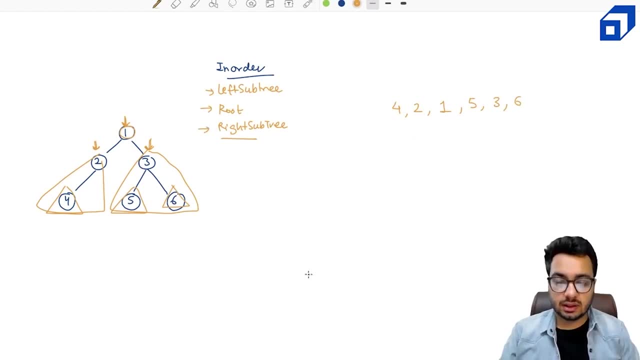 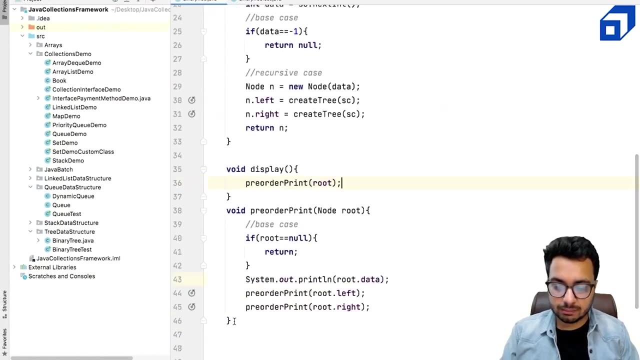 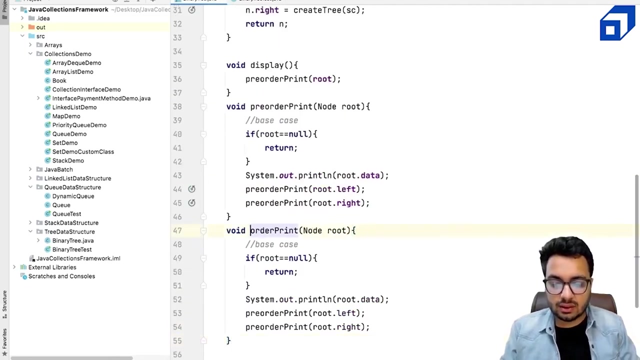 three in a in order fashion. so let us jump into the code and see what we will change. right, just like the pre-order print method, what i will do, i will create one more method called as in order print. so in this case, the root will be printed in the middle. 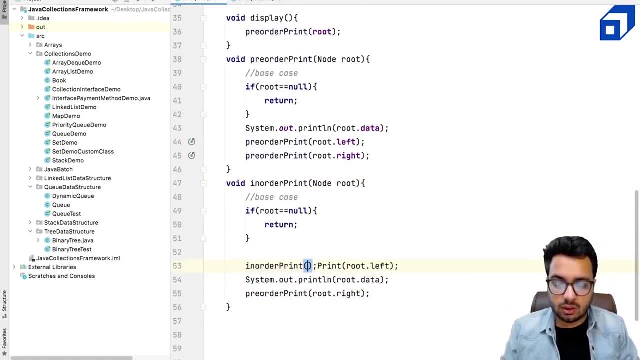 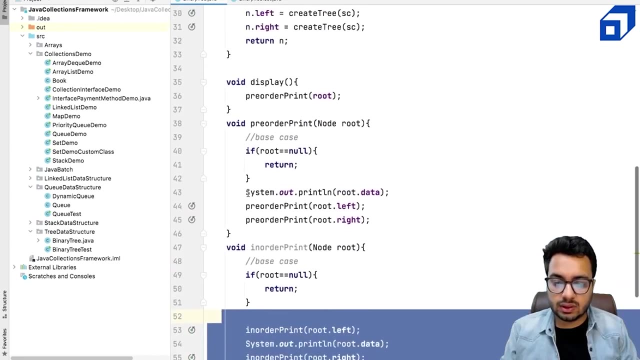 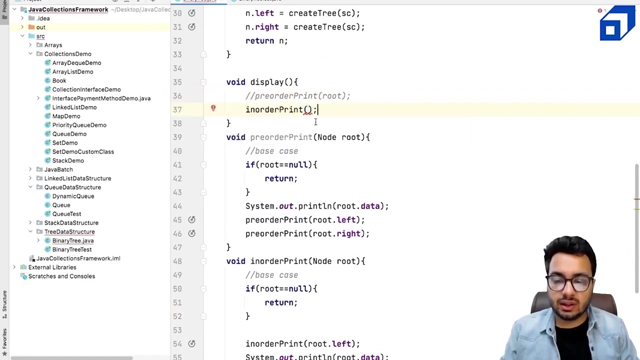 and this call will be now in order print root dot left. and this will be now in order print root dot right. okay, now in the display method, instead of calling pre-order print, maybe let's just call in order print. this time i want to display the tree using 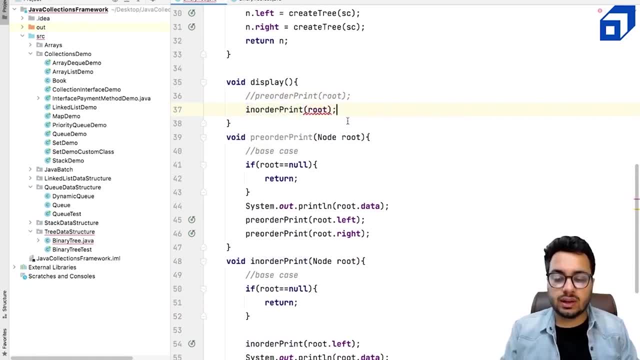 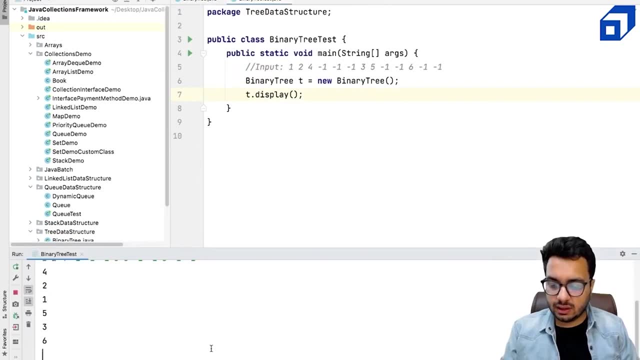 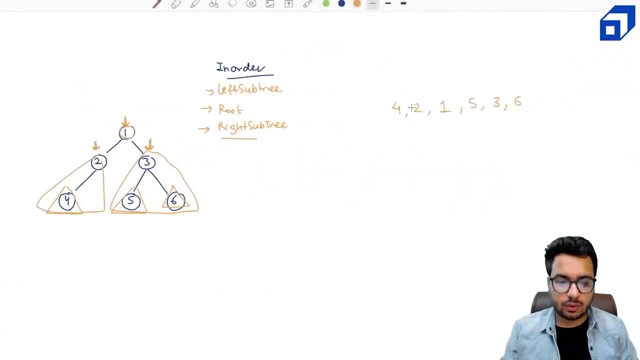 in order print. i will pass the root of the tree as a parameter here. let us give the input for this tree and see what output we get. we are getting four, two, one, five, three, six. is it the expected output- four, two, one, five, three, six? the answer is yes. right now you. 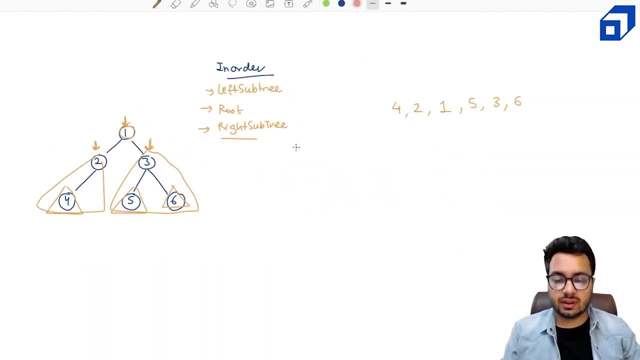 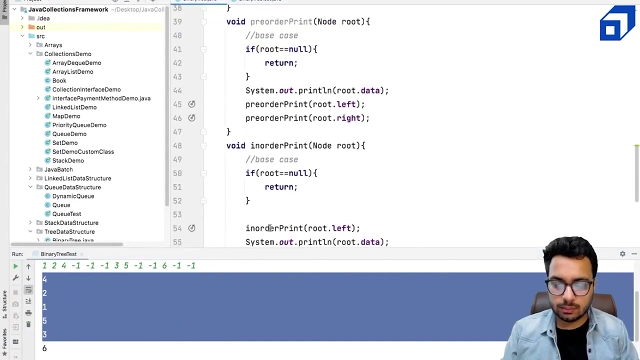 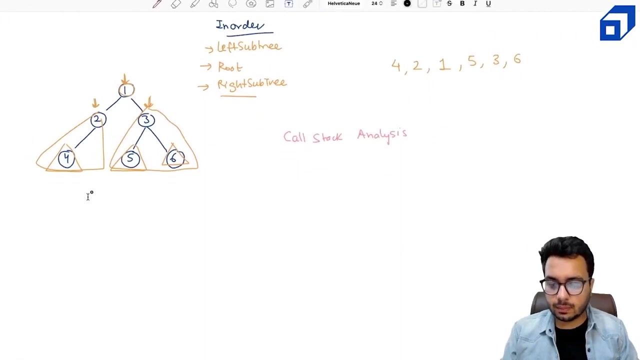 might be interested in doing a call stack analysis of this, right? so let us see how we can do the call stack analysis as well. right in the beginning, what is happening? uh, let me also copy paste the code. this is the code, right? let us do the call stack analysis. 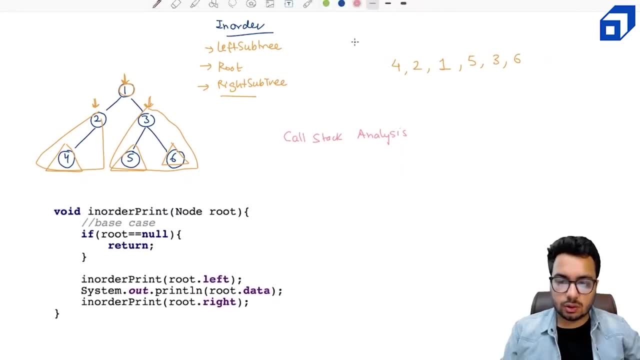 this is the method that we are calling, right? so the call stack is empty. so we called in order print where the root node is 1. so I say root is 1, but I'm not going to print it. so root is not null. I will just call on the left. so I make a call here, right? so that means root is now 2. I am at. 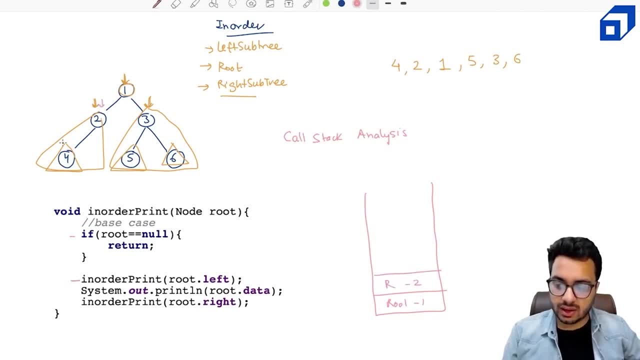 this node, but I'm not going to print it again. I make a call on the left. that means root is 4. okay, I'm not going to print it because root is not null. again, I make a call on the left. when you make a call on the left of 4, you actually come here. this is null. if this is null, you return. okay, so you. 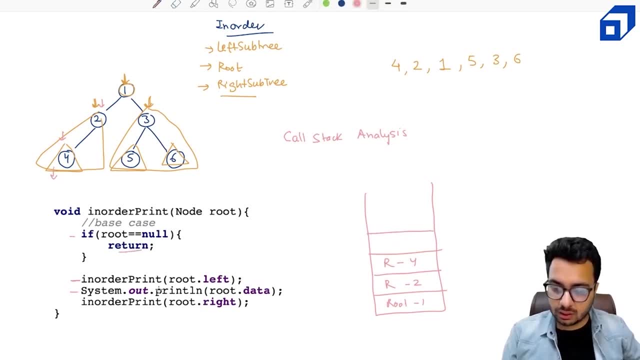 return. then you make a call, then you print the root data. so that means you print 4. this is the top of the stack and this is the root that we are talking about, so you will print 4. then what's going to happen? you will say, okay, I'll go right. so right is null. again you make a call to null. 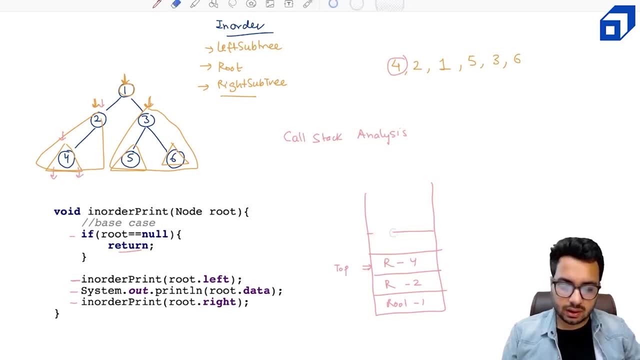 and you return. so you come back. so again, you are here now for 4. you have done all the three things: left is done, root is done, right is done, so you return. so from here you go back, and this is gone from the stack right now. what is the new top right? how do we come back to 2? this is how we come back to the 2. 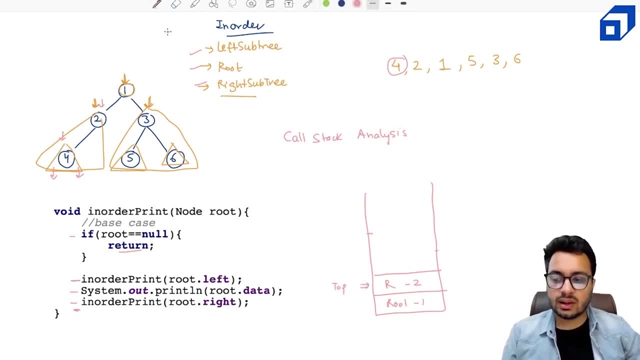 so the new top is this: now, this is the root node that is currently we are talking about. have I printed the left? yes. have I printed root dot data? no, I will print it now. have I printed the right? no, so I make a call on the right of 2 that is null, and I again return. then this is done, so I come back now. 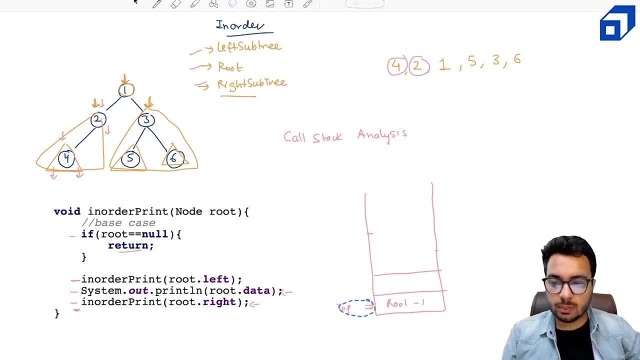 what is the top node? the top node is 1. so have I printed left? yes, have I printed root dot data? no, I will print 1 and I will make a call on the right. so I make a call on this tree right. so again you do a similar process. you come at 3 right, so root is 3. then you make a call on the right of 2 and you 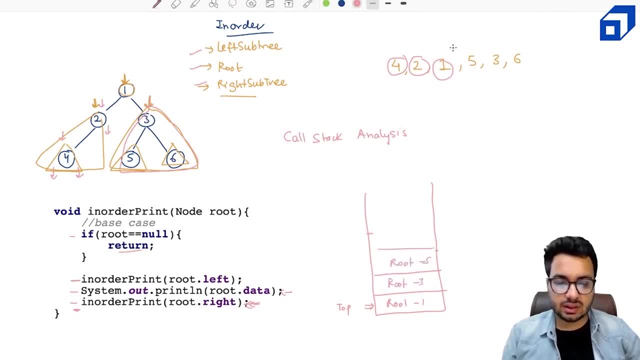 make a call on the left of 2 and you do a similar process. you come at 3, then you make a call on the the, then when you come back to the, all right. so we came away from the top and you come back to the. 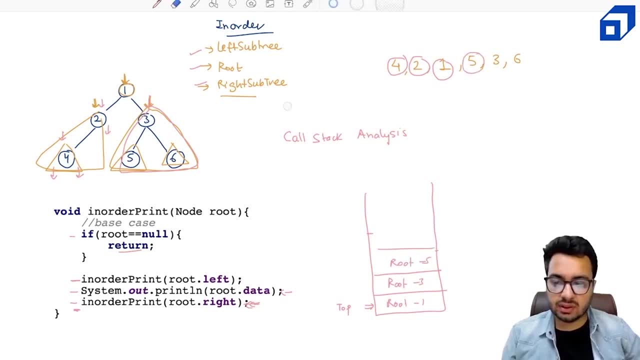 right. and now you came in to get the root code right. so rice is beaten, the. so oh, that R is the left, that is root is 5 to 5, left is no. so you print 5 or the right is null. you come back. so The V is done. then you go back. the new top is now 3, 8 it was 5, now it is 3 or 3 says ok, my left. is done, I will print myself and then I will go right. So I will be 6. you come here. you went here. then you claim here: fix, now root is 6, left and right their null. so rather you left, it will get the root 0. so because I see that in all the right, so I go back and you see what will come here: 1 another. 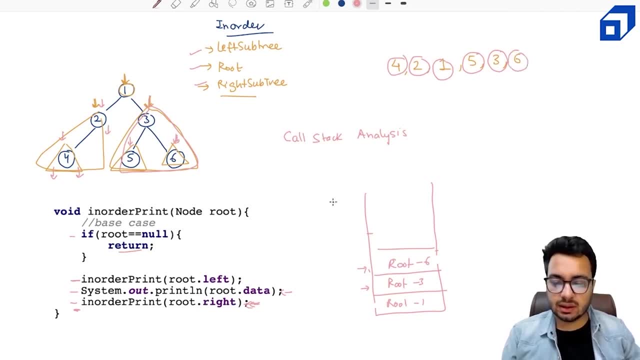 they are null, so six will get printed. right is null right, and then six will be popped off right then. so for three: right is also done, so this call is over right, and you come back at one. so for one: left is done, root is in right is done, so this call is also over right. 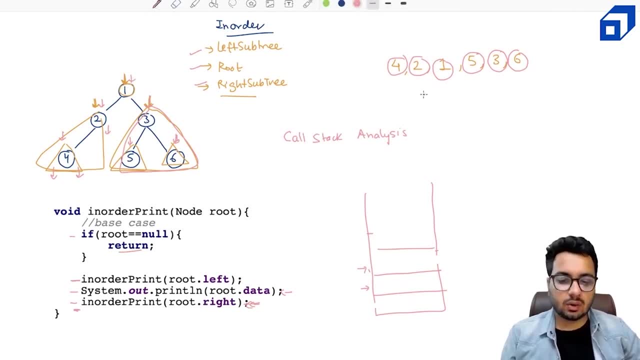 finally, the call stack will be empty and this is the output that you will get right. so i hope you have understood the in order traversal. now make a bigger tree and try to generate the output for that particular tree, right. and next i will discuss post order traversal. let us talk about post order. 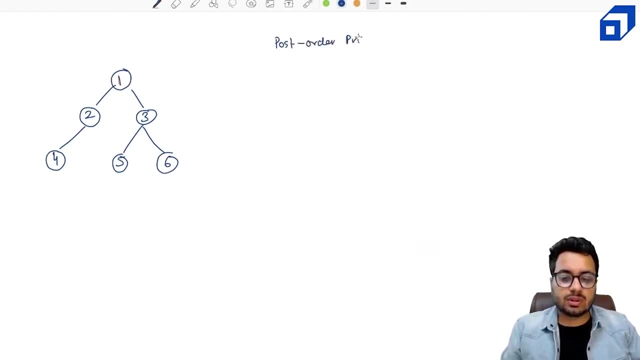 print. so, as the name suggests, post means the word after. okay, so in this case, what we do, we print root in the last. so first we print the left sub tree, then we print the right sub tree, recursively of course, and after then we print the root right. so if this is the tree, once again, what i will do, i start with. 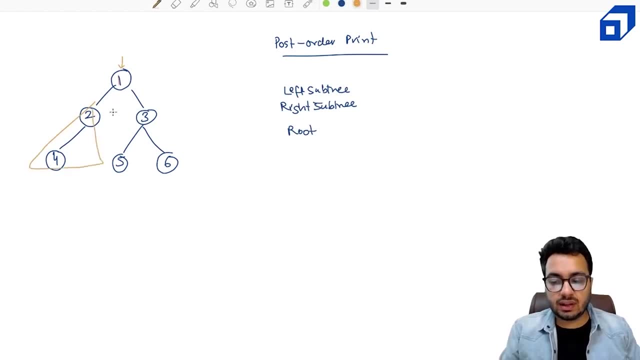 one. but i have to first go in the left sub tree, then i have to go in the right sub tree and then print one right. so at two. i again have to print left sub tree. that means i will print four right, then i will print the right sub tree. so right of true is null, then i will print two. i will print. 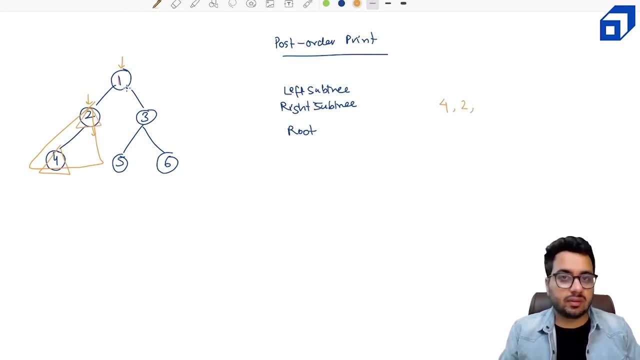 two right, then at one i have to print left, which is done, and then i have to print left, which is done, and then i have to print left, which is done. i have to print right sub tree, and then i will print two. so at three i will, okay, print left. 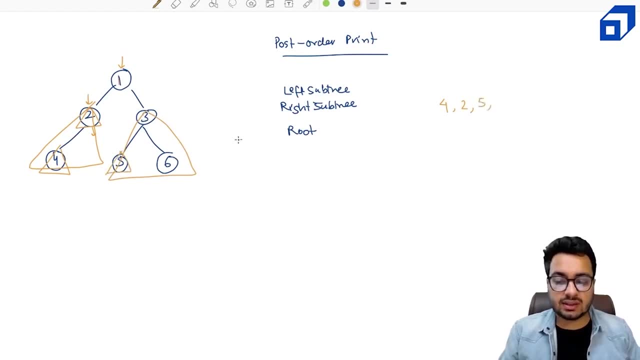 sub tree, which is five, then print the right sub tree, which is six, then print the root. that is three now for one left sub tree is then right sub reason. then i can print the root. that is one night. so this is what the post order output would look like. right, you might be asking: uh, why do we need? 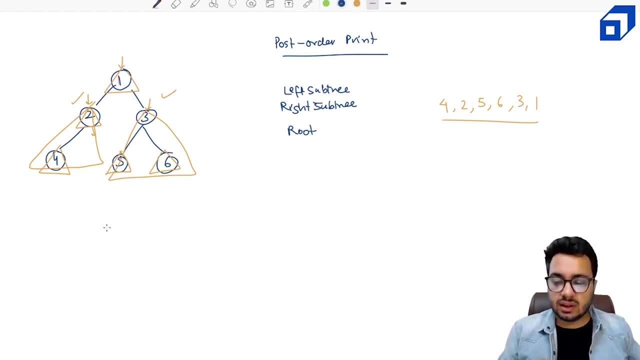 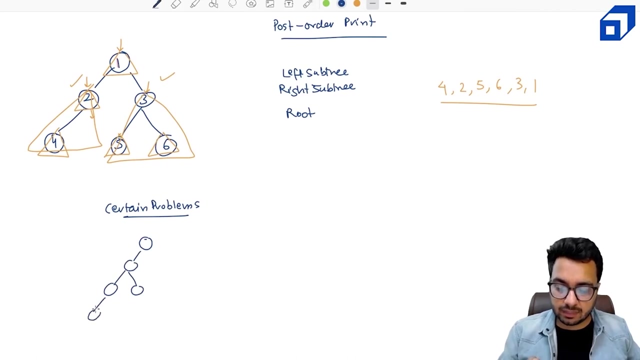 so many traversals. okay, for example, what happens in certain problems is in certain problems. you are expecting that. you are expecting output from the left and right subtree, for example. given a tree, i want to calculate the height of the tree. right, for example, i want to calculate what is the height of this. 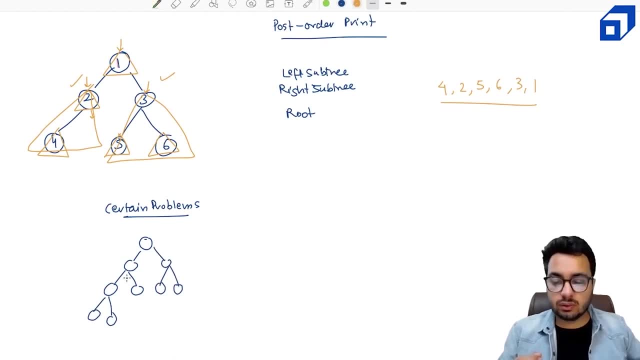 tree right. so in order to calculate height, what you will need, you will need to know that. what is the height of the left subtree? let's say this height is three. what is the height of the right subtree? this height is two. then can you say recursively, at this root node, the height is: 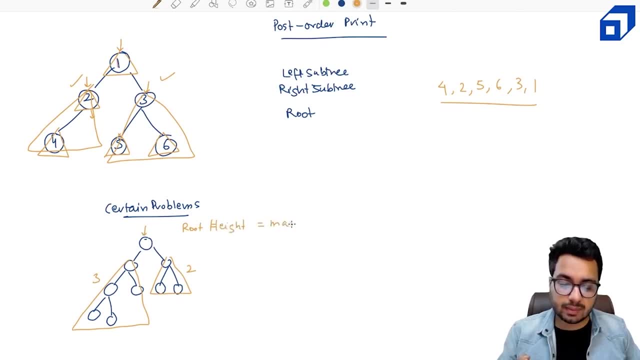 nothing, but it is the maximum of left and right, okay, maximum of the answer that you are getting from left comma, right, and one more than that. so can i say the height will be four. what is this? this is the answer from the left subtree. what is this? this is the answer from right subtree. so what? 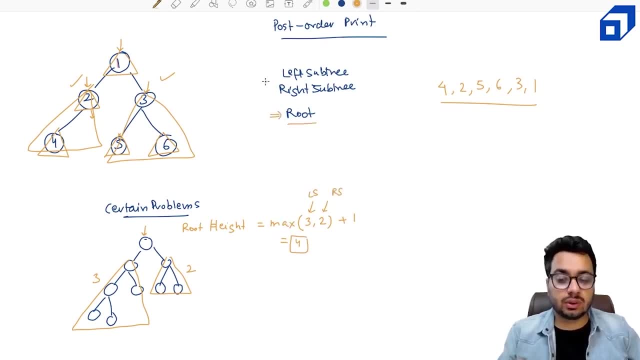 i'm trying to claim is, in order to build the answer at the root node, you need the answers for the left subtree and right subtree and hence, in problems like these, you would of course need a post order reversal right. so that is the idea when you need answer from the uh child subtrees. 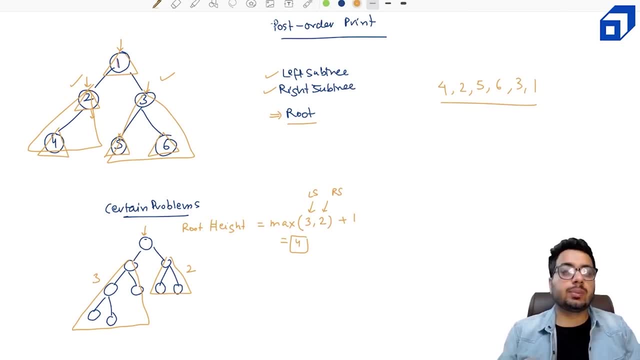 to calculate the answer at the root node, you will definitely need post order reversal there, right. so now let us write the code and then we will do the dry run of that code. so writing code is very easy. so i i'm in the in this class. so if root. 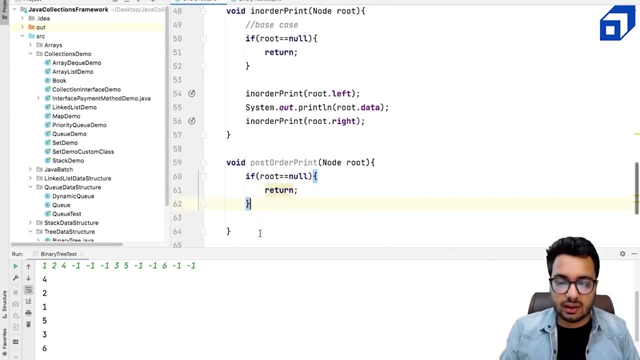 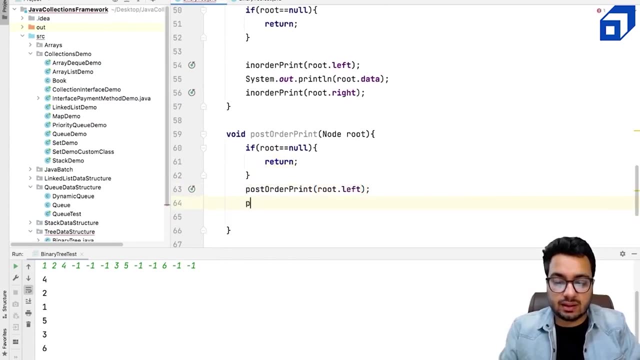 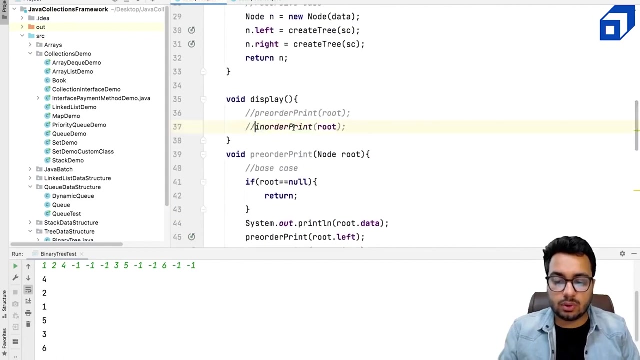 is null, i will return right. then what i will do? i'll go on the right left: post order, root dot left. then i can say post order print, root dot right, and then i will uh print the root node. so s out root dot data. right now let us go and um call post order print in our display method. 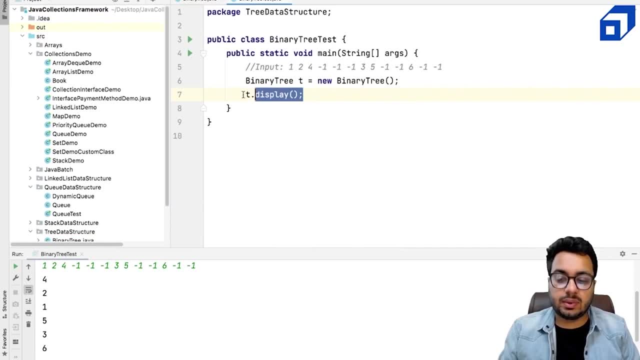 just pass the root here, so t dot display. it's calling the post order print method. now for the same input. let's copy this input and we will see what output do we really get? now we have given the input. i'm getting four, two, five, six, three, one. is it the same output? 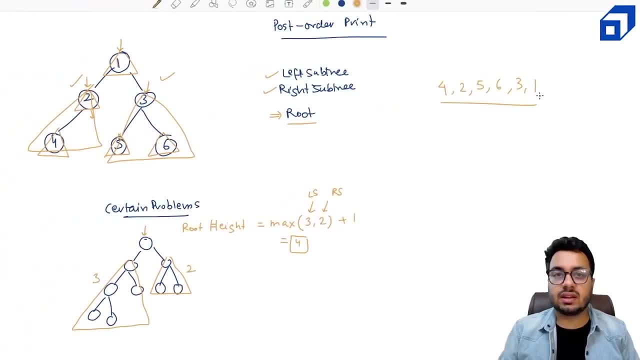 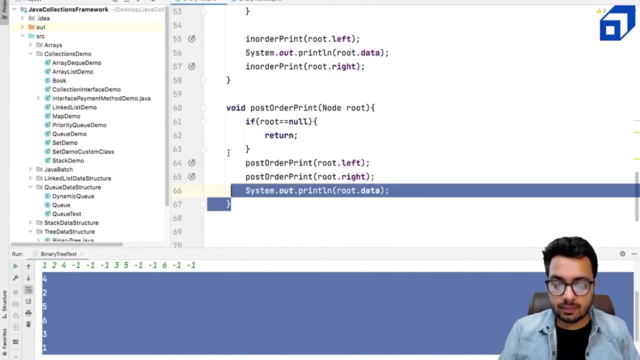 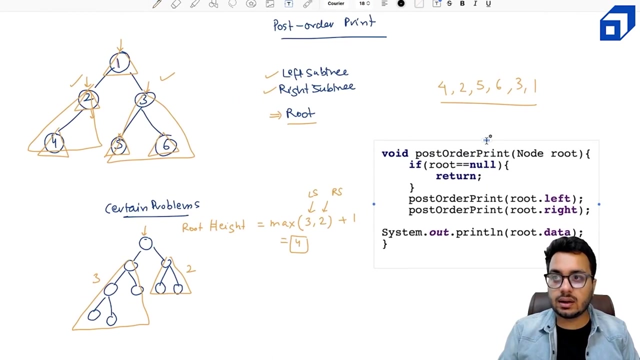 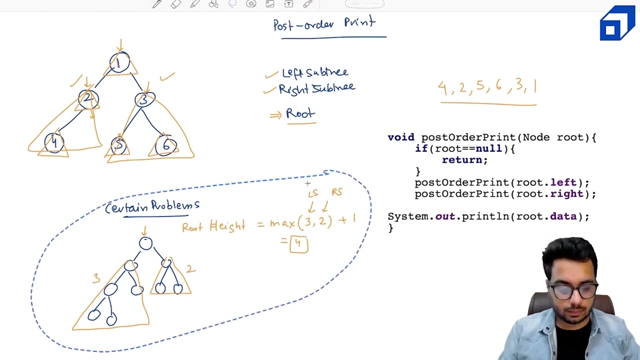 as we have got four, two, five, six, three, one, absolutely yes. now let us do a quick call stack analysis of this method as well. so i'll copy the code, i'll put it here and let us do a quick call stock analysis. let's say: this is my call stack. in the beginning i give one as my root node. the root is one. 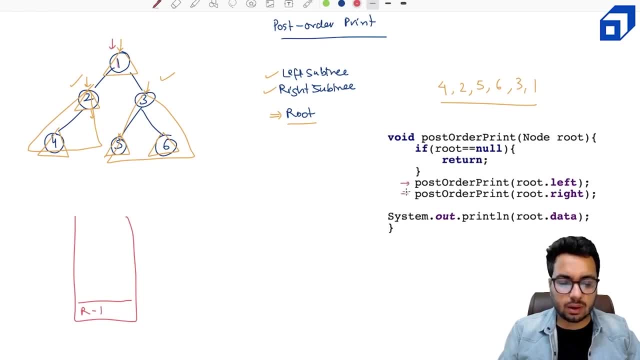 then i say: okay, uh, make a call on the left. my root is two. i make a call here now. code is paused. right call will happen later again at two. i make a call on the left. i come here. root is four. a four makes a call on the left. left is null. i. 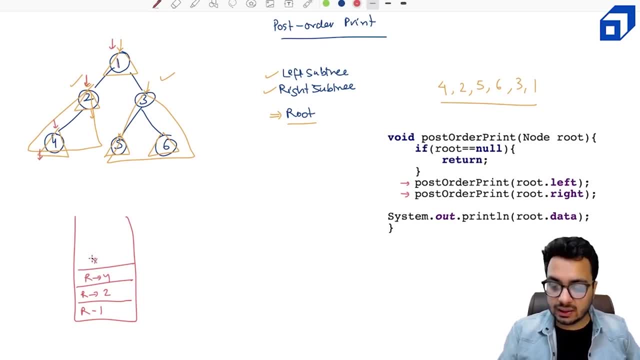 return. then four makes a call on the right. right is null. again i make a call and return. now i can say: print root dot data. i will print root dot data. this is the top of my stack. i will print four right. then uh, if four is gone from the stack, what is the new top? the new top is two right. that means i. 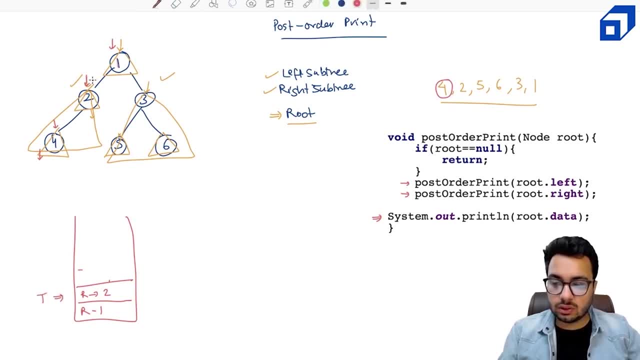 am in this function. i am at two, so i am printed the left. i make a call on the right, so two says okay, go and print the right, right sub trace null. i return. then what happens? left and right, they are done. i will print root dot data. that means i will print two right. now. two is also gone. we are 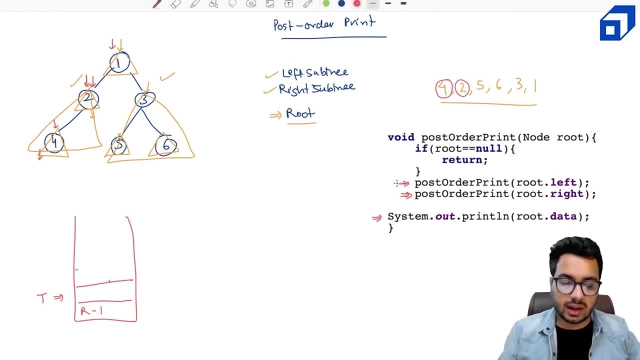 done. so. one is at the top right- we are done, we are done. two is also gone, we are done. so one is at the top of the stack. now, at one I said: okay, go left, which is already done. left is done, go right, I come here. so now one makes a call to three. now three says okay, go left. three: 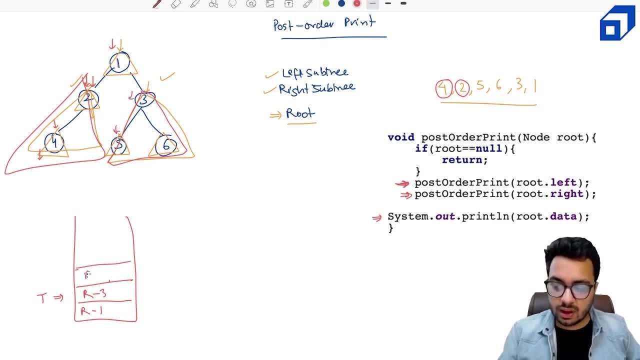 makes a call to five. r5 goes here and r5 says: okay, go left, which is null, go right, which is null, and hence you print five. so you will get five as the next output. now, once five is gone, you're back again at three. three says: okay, my left is done, this is done, I will go. 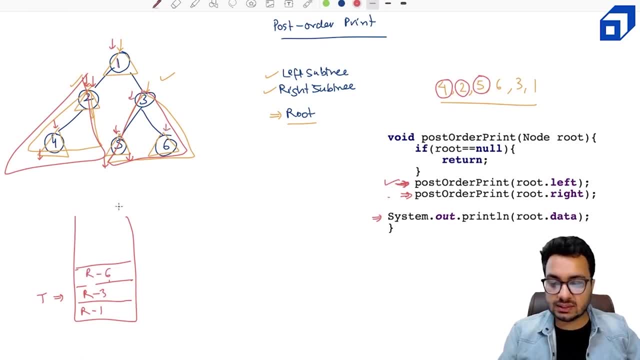 right. so I go to root node. that is six. the root becomes six in this call. so this is the top six says go left, null, go right, null, and hence you will print six right, and then six is also gone from the call stack. then what happens? you are at three. three says okay, my 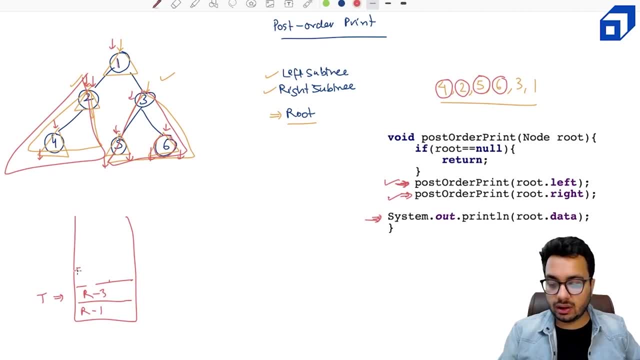 left is done, right is done. I will print root dot k data. so I will print three. I will get print three. three is also gone from the stack and now top is at one. so for one, left is done, right is done, and hence you will print the. 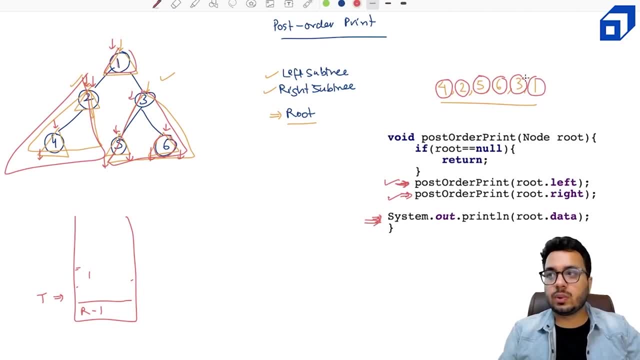 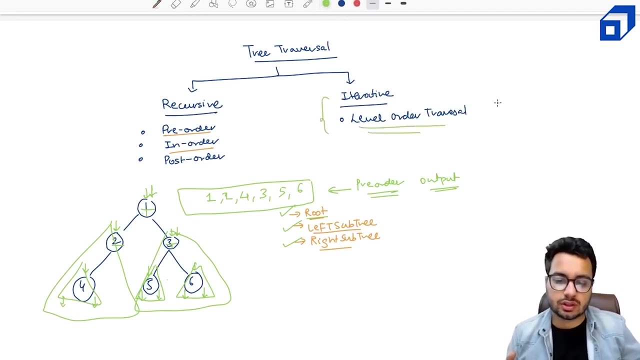 root dot data. that is one right. this is the output of the post order print. I hope you have understood post order traversal. next we are going to discuss the level order traversal. okay, let us jump into the iterative traversal, which is also known as level order traversal. so that means we won't be using recursion. we would be using some kind of iteration to 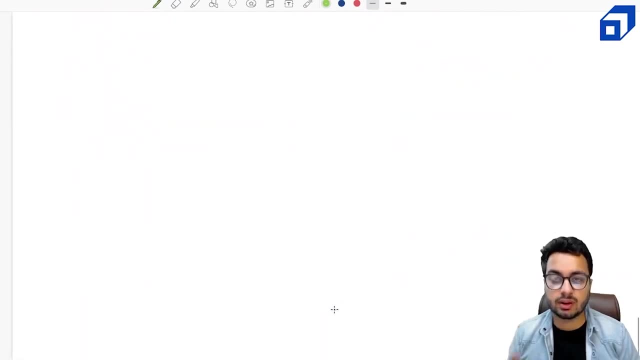 iterate on the tree. okay, oh, some kind of loop, right, let us take this example of three once again. and idea is, instead of going in a depth, first manner: okay, so in all the traversals that we have done so far, what is happening? they're starting from the root node we are. 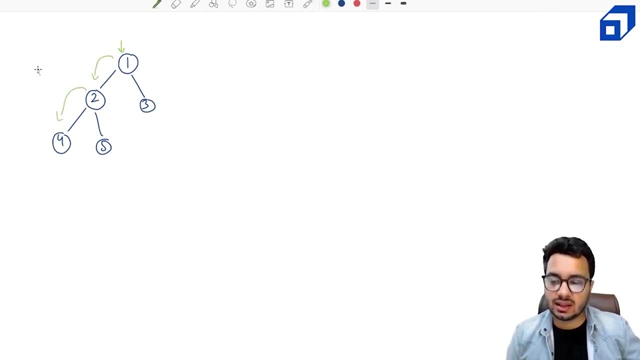 going here, then we are going here. so all these traversals, they are depth first traversals. that means you first go deeper into the tree and then that's how you- i trade, okay, so your pre-order, post-order and in order, they are depth first traversal. right, but now the traversal that we 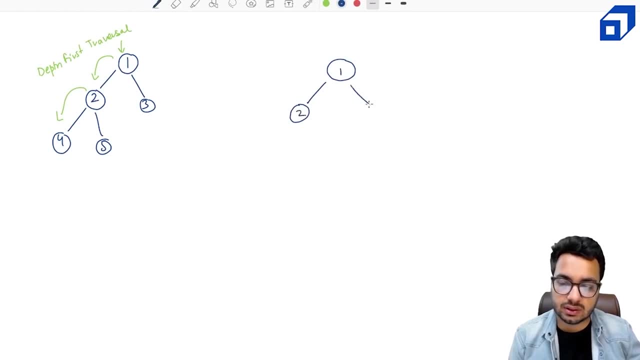 are going to do now. it will be a breadth first traversal. that means if i have a tree like this, i will be going across the breadth of each level, this level, this level, this level right. that means i can expect an output that is one, two, three and four, five, six, right. so level order. 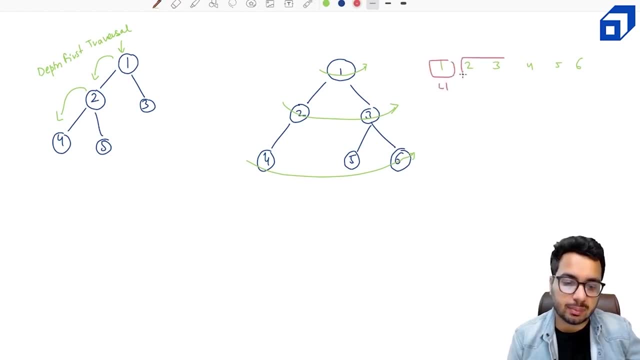 traversal. so this is my level one, then i am printing level two and then i am printing level three. okay, what is the level? all the nodes which are at same distance from root node. so level one, all the nodes are only one node. it is at distance zero from the root node, or let's say, level zero. 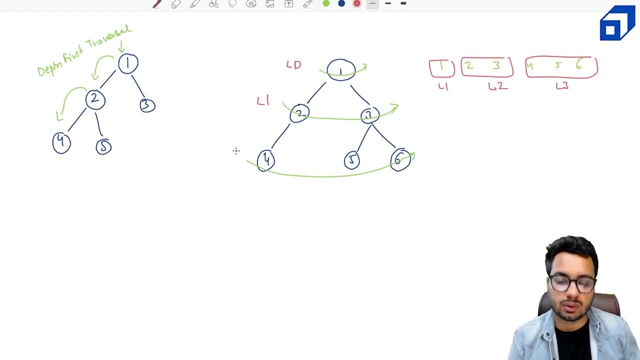 level one, all the nodes are distance one from the root node, and the is my level 2, all the nodes are at distance 2 from the root node. if this is also known as breadth-first traversal, right breadth first traversal, right now let us see how we can achieve this kind of a traversal. 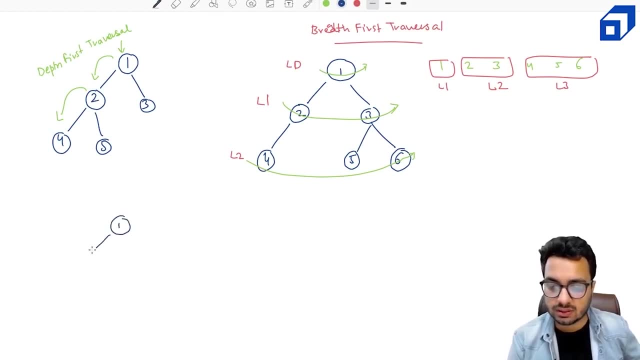 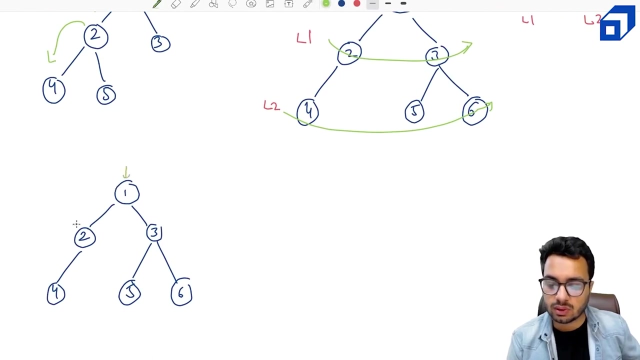 right. let's draw this tree once again now. if you look carefully, if you start doing any traversal, that is a recursive traversal right, from one you come to 2 right and at 2 you do not have a direct way of going to 3 right. so that means with recursion it will be very 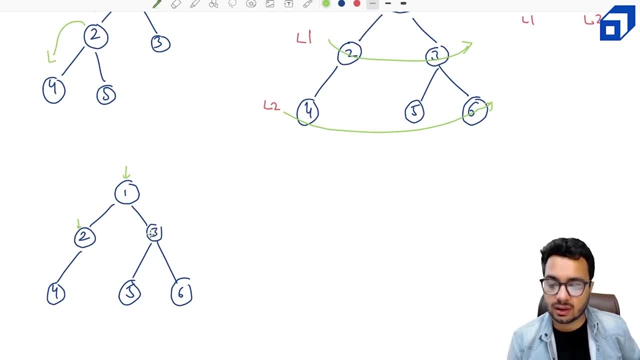 difficult for us, from 2, to go directly to 3 right, and if we go to 3, we outside, we don't know a way to come to 4 right, so we cannot go back and forth, right. so how this is achieved? this is achieved by using a concept of 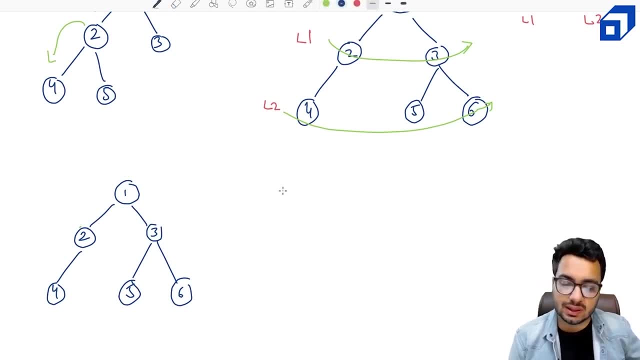 a q data structure. okay, what we will do? we will create a q- q- you know it is a before data structure. first in, first out. so in the beginning i will push this node in the q. fine, right. and then i will say: okay, like q dot, push root. now i will pop one node from the q. 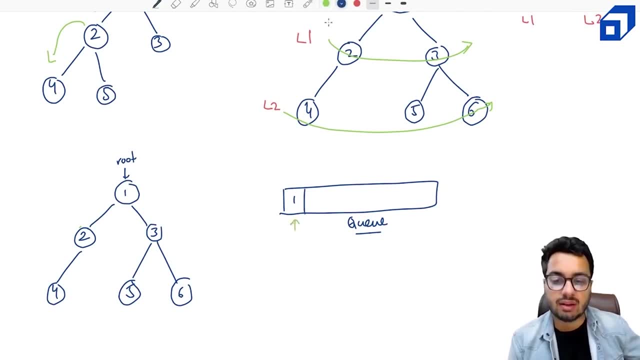 so i will pop this node and i will push the children of this node into the q, so i will print it. output will be one. this is popped and what are the children of one? children of one are two and three right now. how do i know the children? because i'm not going to store an integer value. 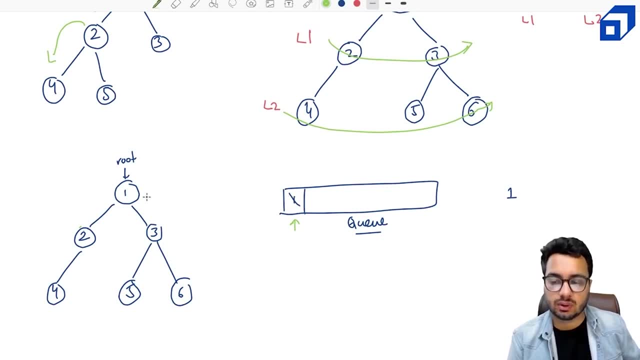 here. i'm going to store the reference of this node, right? so i'm going to say, okay, this root is the address. of this node is stored here. so if you know the address, you also know the child values, right. so you know the children are root dot left, root dot right. i will push. 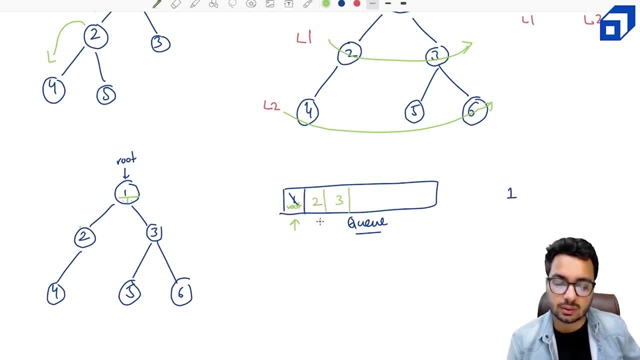 theので. we will repeat this over and over so that administration becomes fix. so if you the reference of 2 and 3 in the queue, right next i will again pop one node. i'll say, okay, let's remove 2, let us print it and let us push the children of 2 in the queue. so 2 has only one. 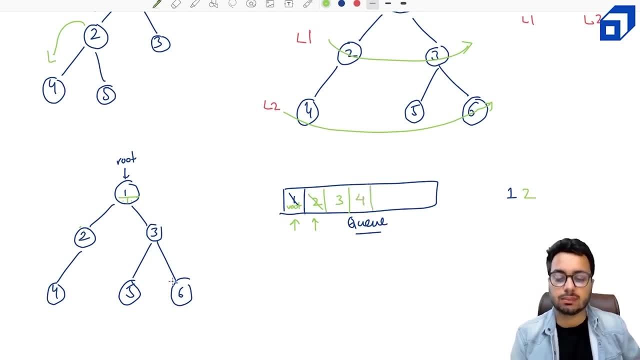 child, the 4, will be pushed into the queue. right again, repeat this process, pop one node. so now you're going to see that, okay, 1 is done, 2 is done. the next node is coming is 3. right, i will pop it, i will print it and i will push the children of this 3, okay, into the queue. so i will push 5, 6, so 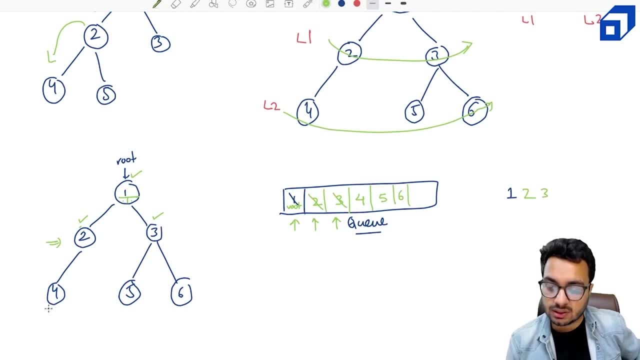 you look carefully, when the second level or the first level is popped, the next level is already in the queue, right? the next level is already in the queue. let's say, i have some more nodes. let's say i have, uh, 7, 8 and 9, right? so let us just extend this example a little bit now. 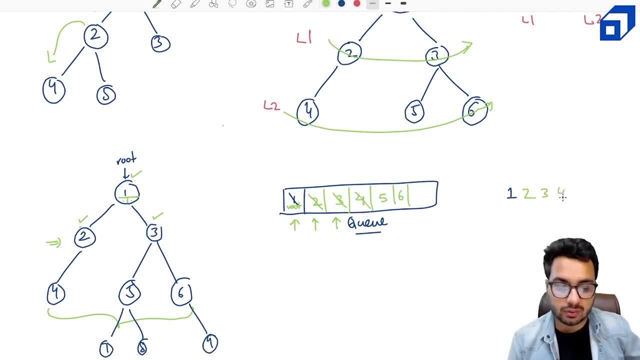 you. i will pop 4, i will print 4. this will be removed. 4 does not have any children, so nothing will be pushed. next, i will pop 5, i will print 5 and i will push the children of 5 into the queue. so i will push 7 and 8 into the cube right next. i will pop 6, i will print 6 and i. 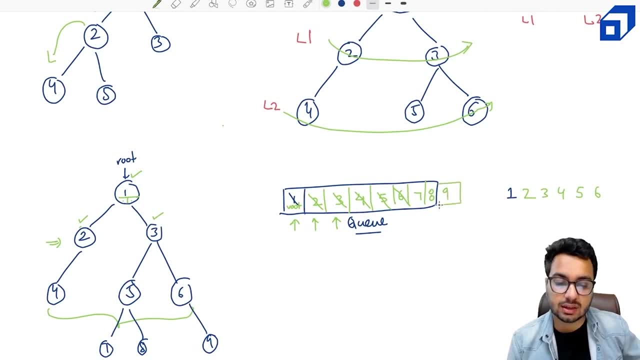 will push the children of 6 into the queue, so 9 will get into the group. next i will pop 7, i will print 7 with delivery data here. the second step is another step. if you run with this method, you can and no children, so nothing will happen. next i will pop it, print it: no children, nothing will. 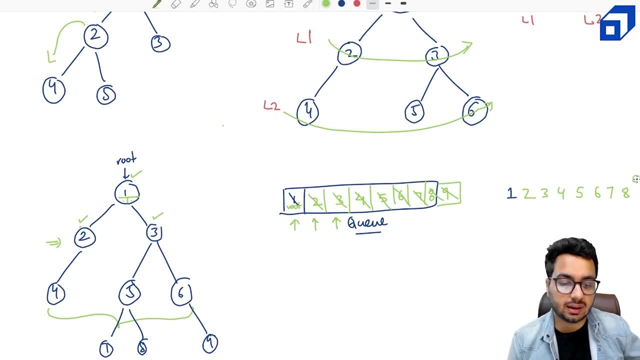 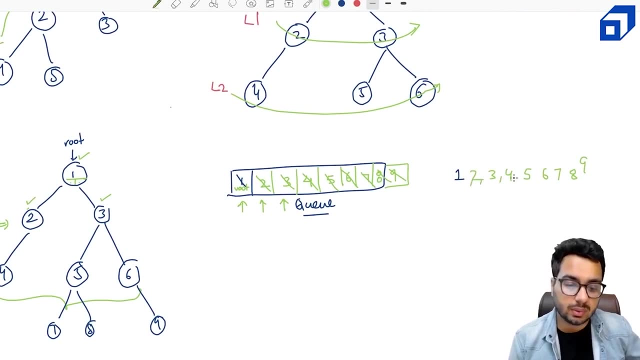 happen, i will pop nine, print nine and the queue is empty. right, so no children. so queue is now empty. this will be my output of level ordered reversal, right? i hope you are convinced that this is the correct output for this tree. right now, let us look at this implementation in our code as well. 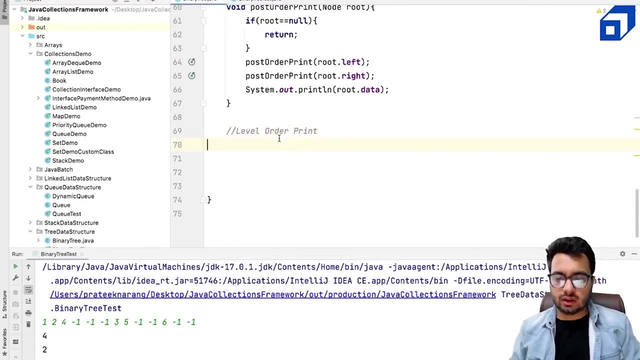 let us discuss the implementation of level order print. so i'm going to create a method called as void, level order print, and first of all i will. i will need a queue object, right, and i also need to pass the root here. so i'll say, okay, fine, i'll need a queue of node called queue. this is equal to: 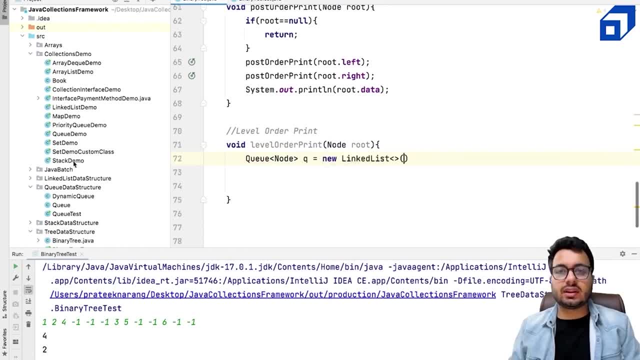 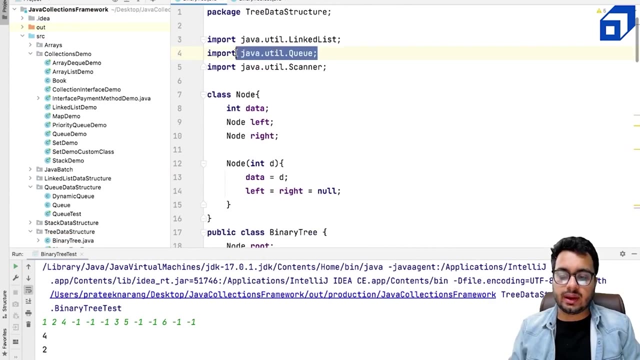 right and i will need a queue of node called queue. this is equal to new linked list. so in java, queue is a interface and linked list is a class that implements the methods of the queue. right, we need to import this from the util package, okay? so linked list is imported, queue interface is also imported. so to start, 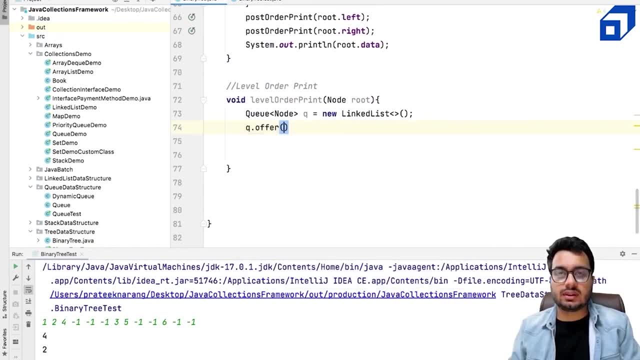 with. you can say: okay, queue dot offer, that is your add operation. right, and i can offer root inside the queue. that means i can add queue, right. i said you will do some work while the queue is not empty. so, while the queue is not empty, what you will do? you will pop out something. you 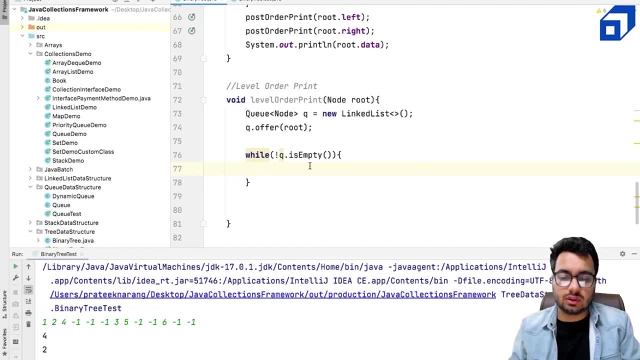 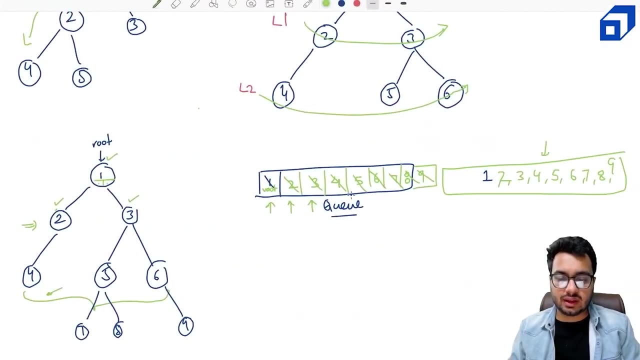 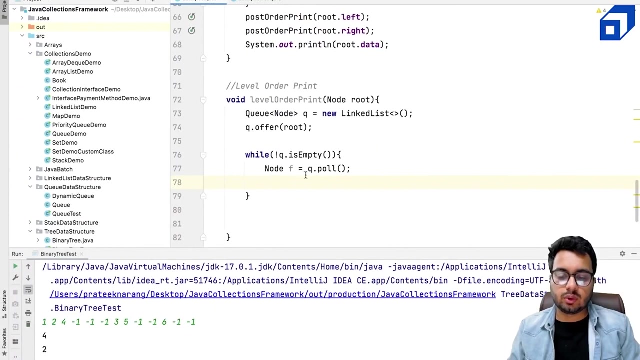 give me the node which is at the front of the queue, the node f. this is equal to q, dot, whole right. so this removes the first node. like we have seen in the diagram, we are always removing the node at the front of the queue right, so this is going to remove it and return it. right now i can print the data of this node so i 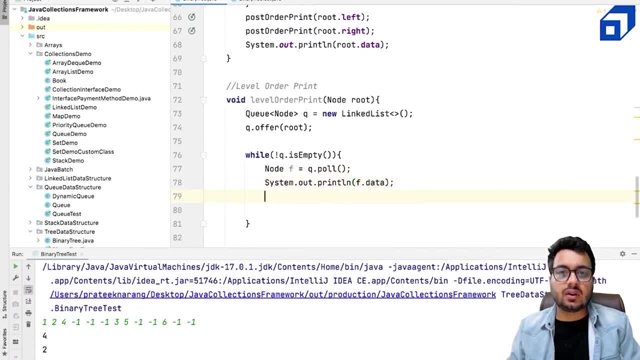 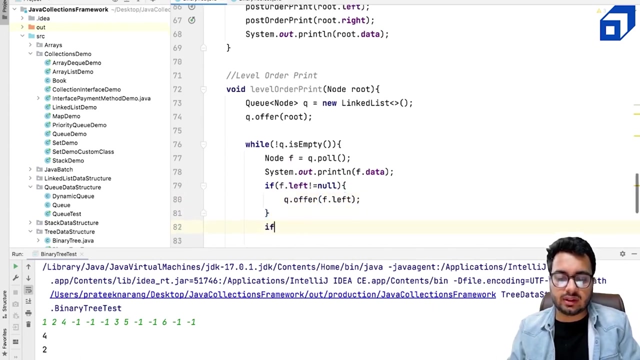 can say s out f dot data. and now i can check if the left and the right side. if they are not null, i can push them into the queue. if f dot left is not null, i will say q dot, push f dot. sorry, q dot offer f dot left. and if the right child is not null, 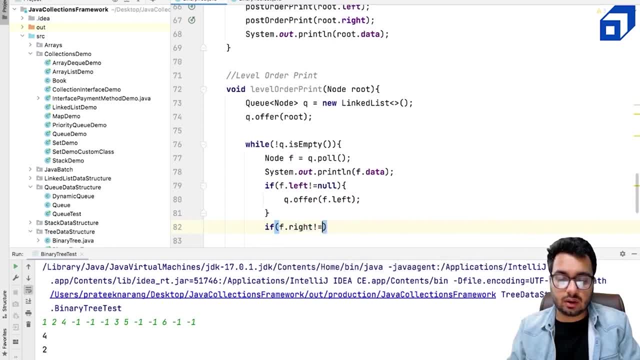 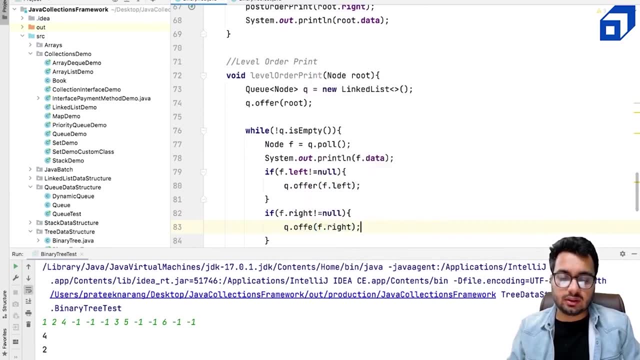 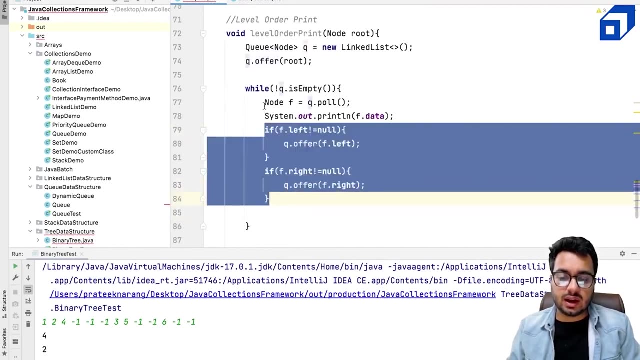 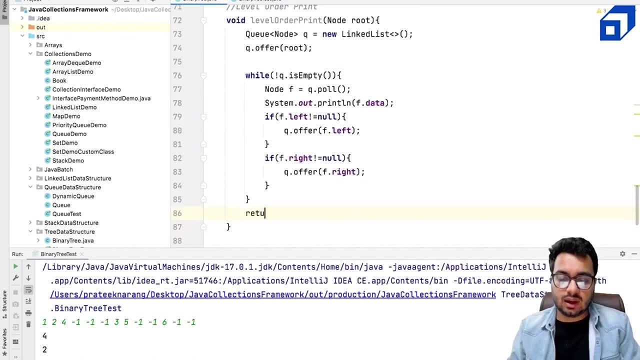 but if- yeah, if the right child is not null, i can say q dot offer, f dot, right. so in this way, q is getting filled using these if conditions and it is getting empty from the queue. so i can say q dot offer from the front using this whole operation. right, that's all that is the code, and now i can just run. 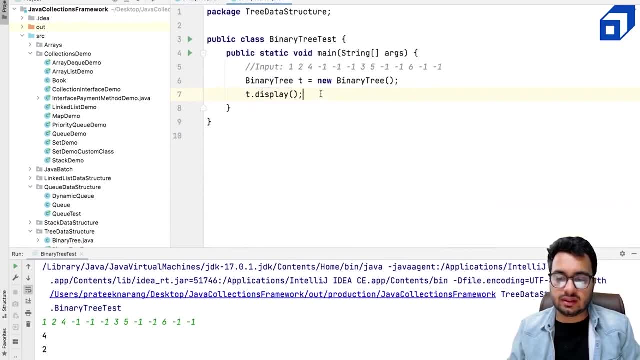 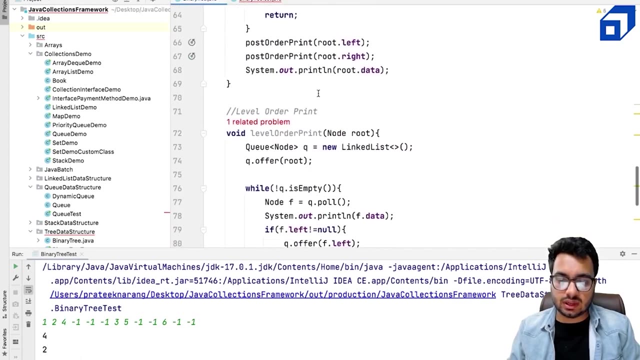 this code in the display method, or here i can say: uh, t dot level order and okay, root. so it's better to call it uh internally because root. i don't want to access it outside, so, okay, i'll just call it from it, from the front, using this whole operation. right, that's all. that is the code, and now i can just run. 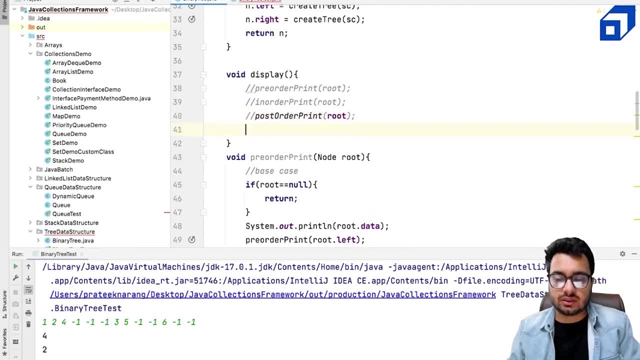 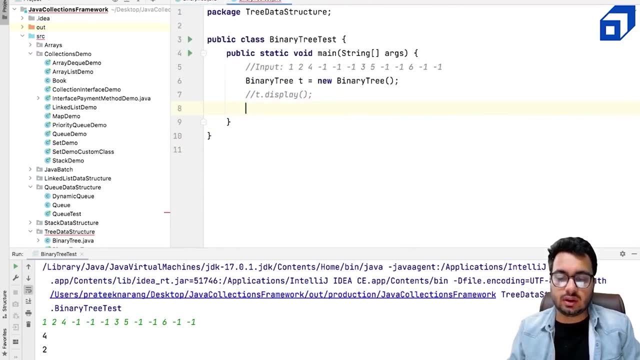 the display method because we are testing the functionality so i can say level order print. so here i can just call t dot display. so now my tree will be displayed in a level order fashion. let's see what output do we get. so for the given tree i'm getting one, two, three, four, five, six. 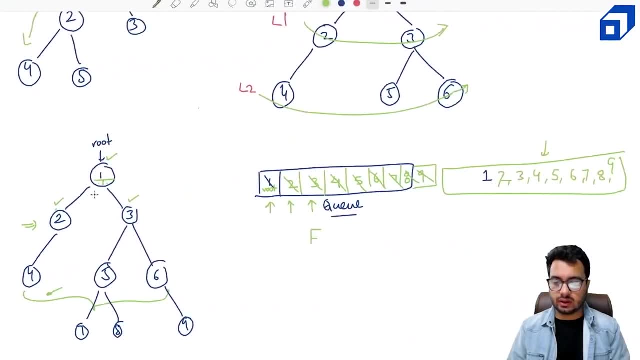 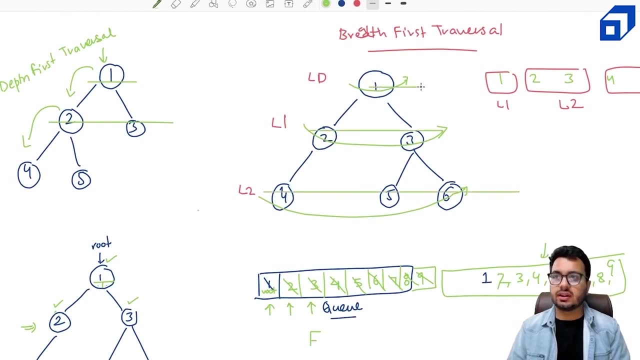 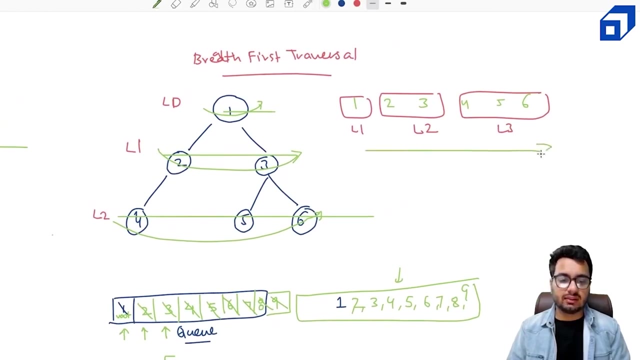 which is correct. and uh, if you look carefully here for this tree, i'm getting one, two, three, four, five, six. yeah, this is the tree actually, so i'm getting the correct output, which is this. so i hope you understand the level audit reversal and how it is achieved. 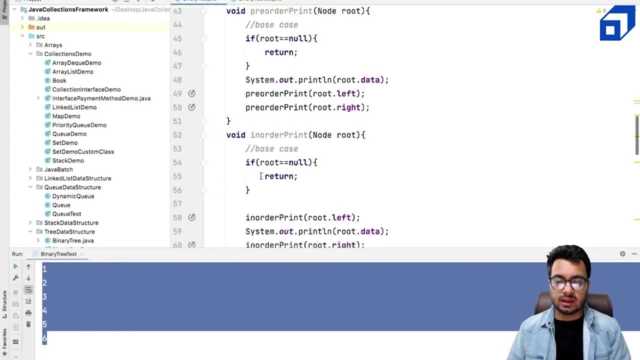 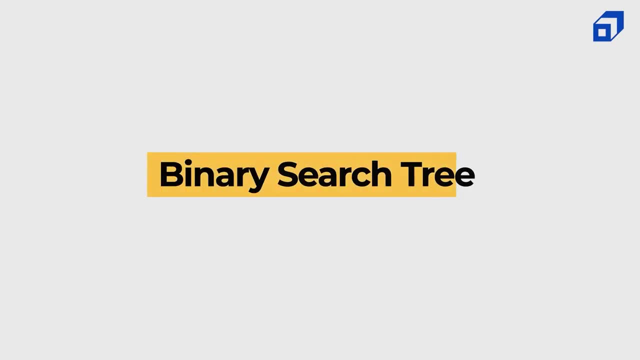 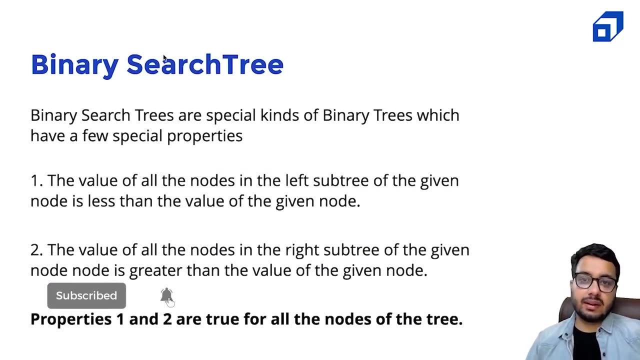 using the q data structure. the code is very simple and you can also do a dry run of this code at your own, so let us start discussing binary search tree data structure. so right now we have learned about binary trees, which we said. it is a tree in which every node can have at max two children. 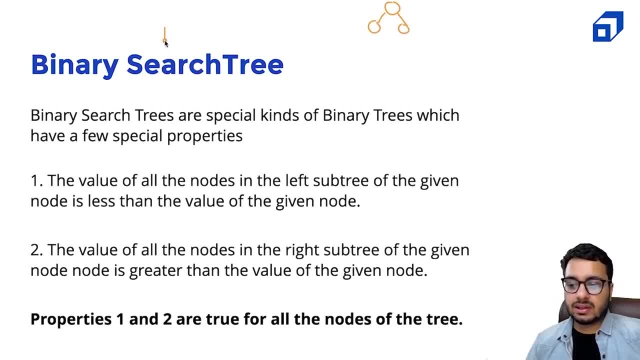 a binary search tree is a special kind of binary tree which is optimized for the search operation. okay, so that is why the name called binary search tree. in short, we also call it as bst. the bst is a special kind of binary tree with the following properties. the first property is: 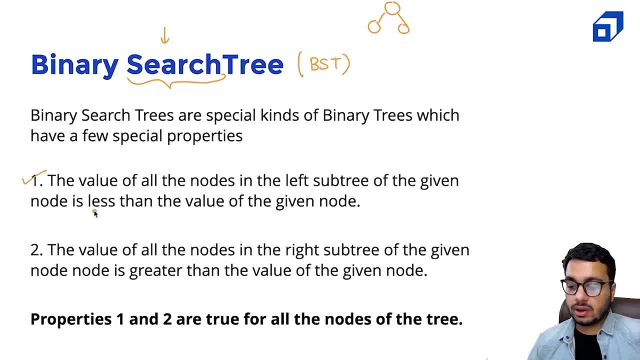 the value of all the nodes in the left subtree of a given node should be less than the value of given node. for example, if this is the root node and it has certain value, for example, this value is 8, then all the nodes which are in the left subtree, they must be less than 8, okay, and 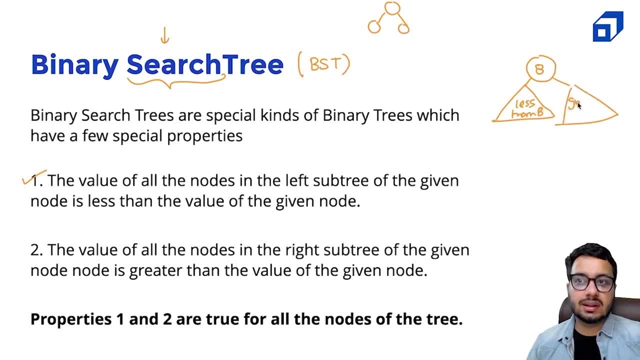 all the nodes which are in the right. they must be greater than 8.. this is the bst property right now: how this makes searching easy. for example, you are searching for 5, you don't need to have to traverse the entire tree. you will have to say, okay, i will go into the left subtree, right. 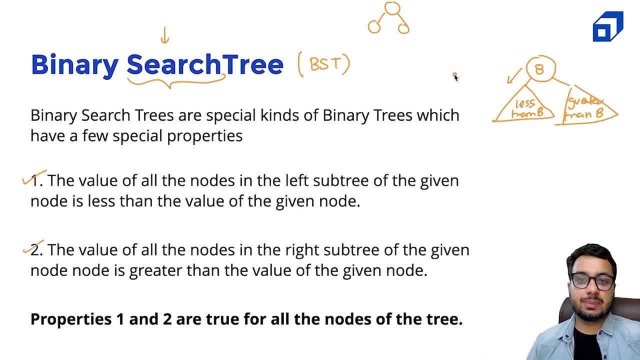 now this property that we are talking about, that nodes in the left subtree would be smaller, nodes in the right subtree would be greater. it is not just applicable for the root node, but it is applicable for all the nodes of the tree. okay, so we will see an example. 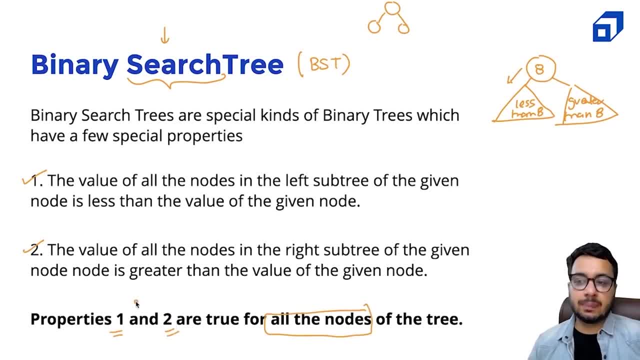 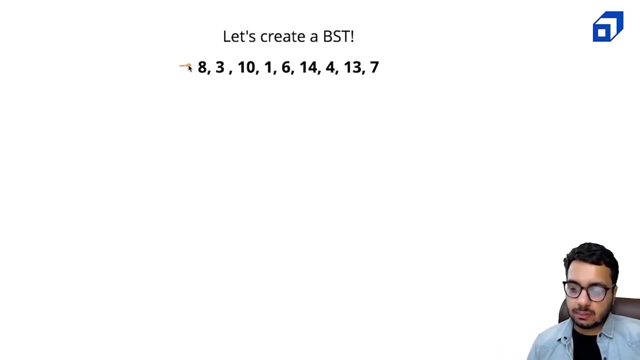 of how do we construct such a tree where every node follows the bst property. so this call this, we call as the bst property right or the bst properties. so this is what makes this tree very special and efficient as well. right now, suppose we are given this data and we want to create a 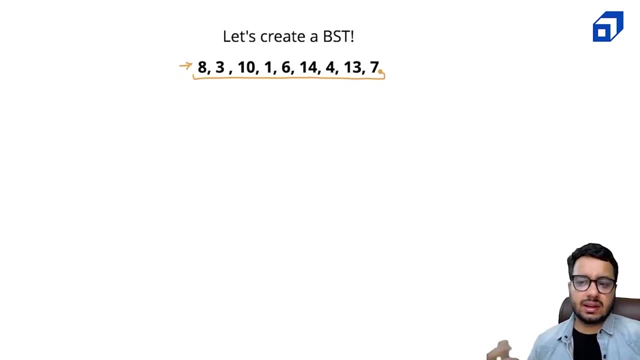 binary search tree from it right now, how we will create it. let us discuss. so, first of all, we are getting eight right, so eight will be the root node because my tree is the bst property. right is currently null, so eight becomes the root node right now. next element that i'm getting is three. 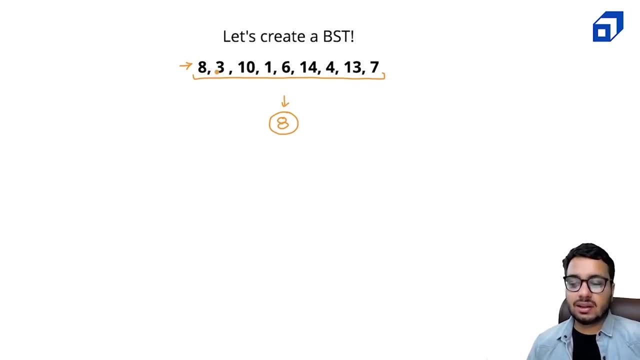 eight, now three. i know it. it is less than eight, so it will go in the left subtree of it, so three will go here. next i am getting 10, so 10. i know it is greater than 8, so it will go into the right of it. it will get connected here right now i am. i want to insert 1, so again, i do not. 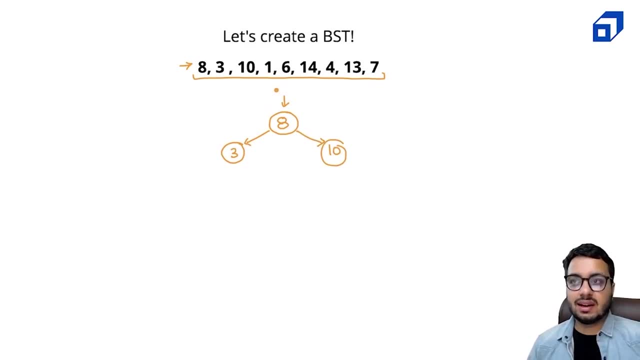 know where it will go, so i will start from the root node. so 1 is less than 8, i will go left. 1 is less than 3, so i will again go left. i will insert 1 here. then i get 6. 6 is less than 8. i go here now. 6: if you compare with respect to 3, it is greater, so it will go here. 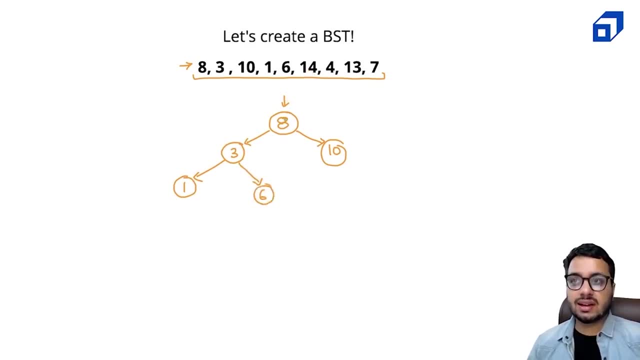 6 gets inserted here. then we have 14, so 14 is greater than 8, i go here. it is greater than 10, so i go here, so 14 will get inserted here. then i have 4. 4 is less than 8, i go here. it is greater than 3, i go here, but it is now less than 6.. so i have to. 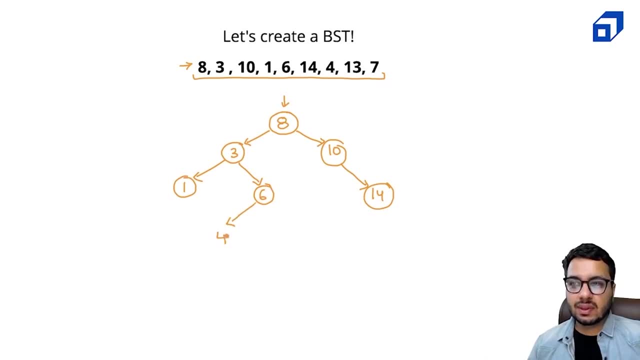 travel the branches accordingly. so that means 4 will get inserted here. then i have 13.. so 13 is greater than 8, go here. 13 is greater than 10, go here. 13 is less than 14, so you will go here. and finally, i have 7 right. so 7. if i start with respect to root node, let's go to root node. 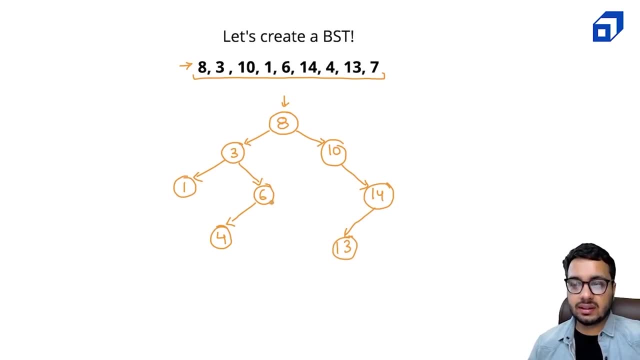 then 8 go here. greater than 3 go here. greater than 6 go here. 7 will get inserted here right now. this is how the binary search tree is constructed. okay, so we have discussed how do we create a binary search tree. so we have to insert all the nodes one by one, right? 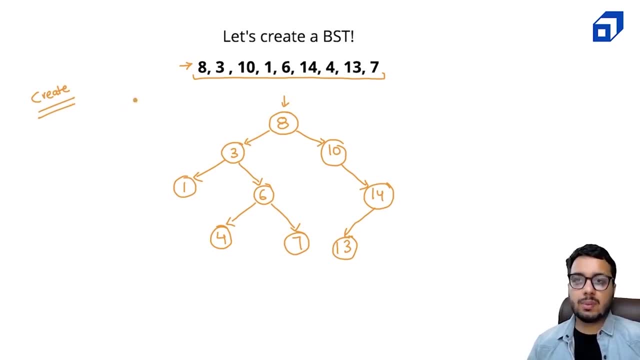 now how much time it will take to insert one node, right? so it will depend upon what is the height of the tree. now suppose if this tree height is h and i want to insert a node, so in first case i have to travel one branch, for example, if i want to insert, let's say, 20, right? 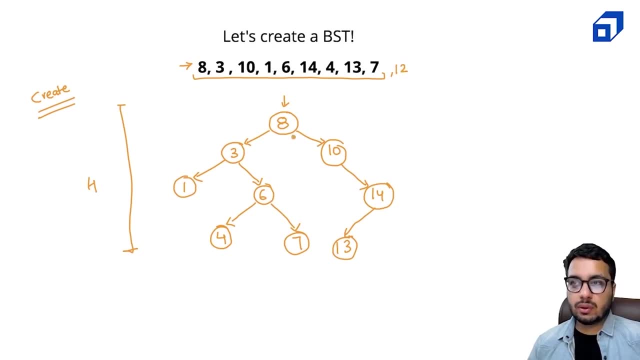 or let's say, i want to insert 12. right, what i will? i have to do. i have to start with 8. go here. it is greater than 10, i have to go here. it is less than 14, i have to go here, and it is again. 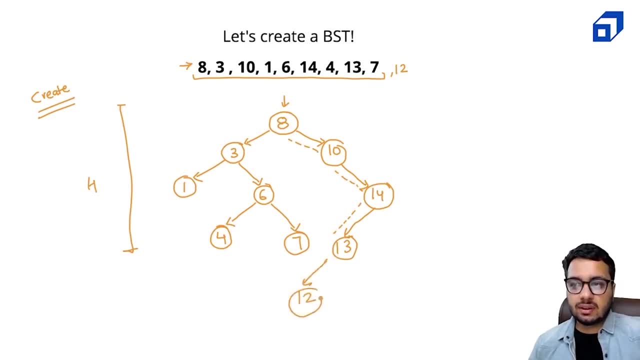 less than 13, so i have to go here and insert. so this is how 12 will be inserted in the tree right now. let us talk about searching. okay, how do i search for a given node? now, for example, i am, i want to search for. let's. 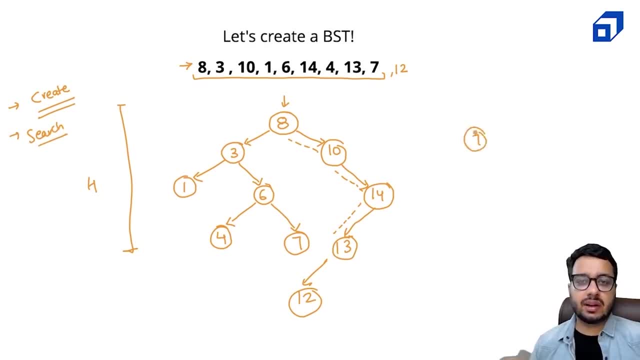 say 7, right, where is 7 present? or if it is present or not. so i just want to output yes or no, whether this is present or not. so i start with it. if 7 is present, it must be on the left, so i go here. 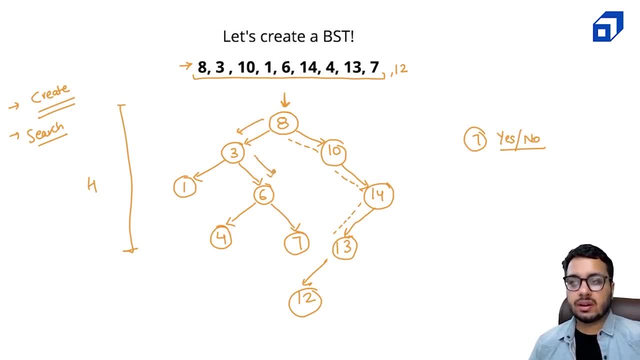 at 3: if 7 is present, it must be on the right, so i go here. at 6: if 7 is present, it must be on the right, so i go here. right now i hit a node which is actually 7, right, that means if i am again performing an operation. 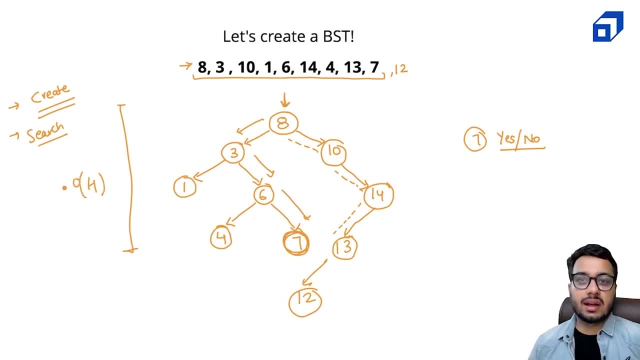 like search, i will do it in order of s time, where height, in the worst case, can be n also. for example, if you say okay, i want to insert these nodes into the binary research tree. it will form a skewed tree like this: 1, 2, 3, 4. right height can become n also, so that is why i'm not saying order. 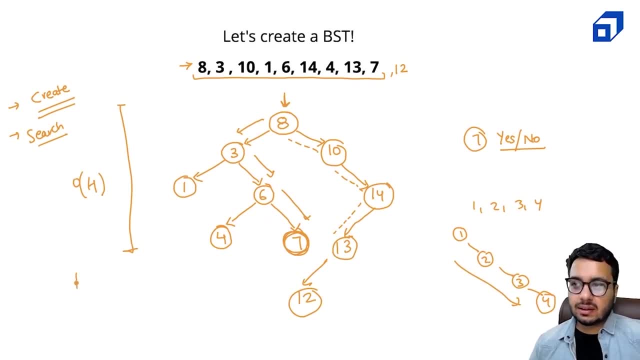 of n or i'm not saying order of login, right. So the height in the worst case will be- can become order of n, right, and in the best case, if your tree is a fully, completely balanced tree like this, okay, in the best case, if a tree is like 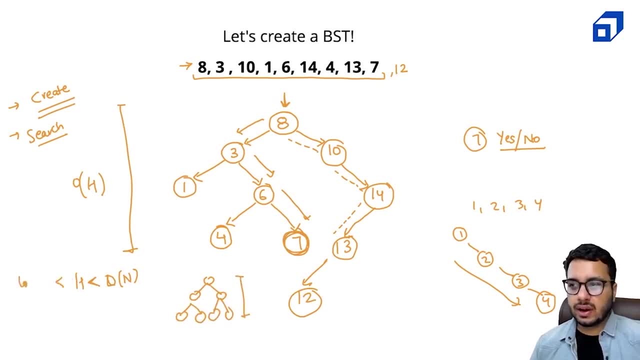 this. the minimum height it will have would be log of n, right? So height will be greater than log n, greater than equal to log n, and it will be less than equal to n. So height lies in this range, right? So, accordingly, the creation and the searching time: okay, not about creation, but 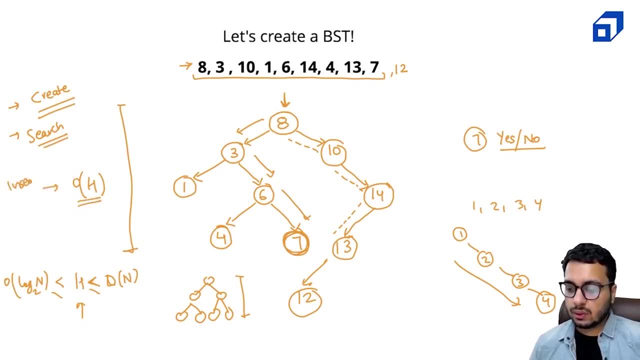 inserting one node. okay. So inserting a single node will take order of h time, where h is the height of the tree. Searching for a given node will take order of h time, where h is again the height of the tree. I hope you understood the fundamental concept behind binary search tree. 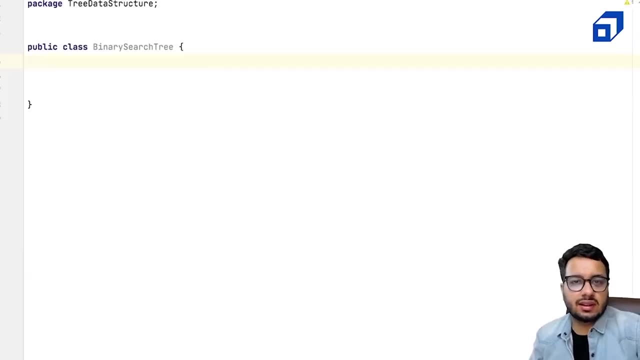 and now let us dive into the implementation of it. So let us start by building a binary tree. binary tree. So let us start by building a binary tree. So let us start by building a binary tree, binary search tree class. okay, So in this class, what this class should know? that? what is the root? 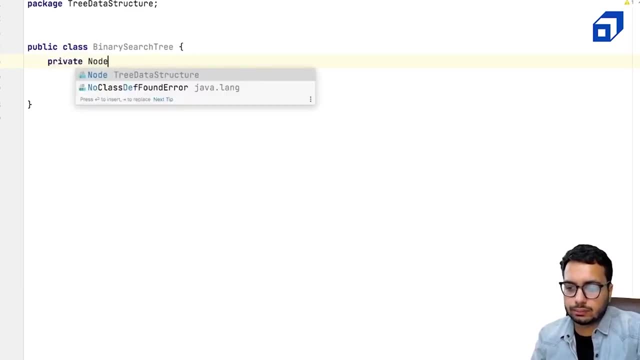 of this tree. So I can say, okay, private node, root. So I have a root node which is a private member because I don't want a outside world to access this root directly. right Now. I want to initialize this root node by creating a tree. right, So I can say, okay, there is a binary search tree. 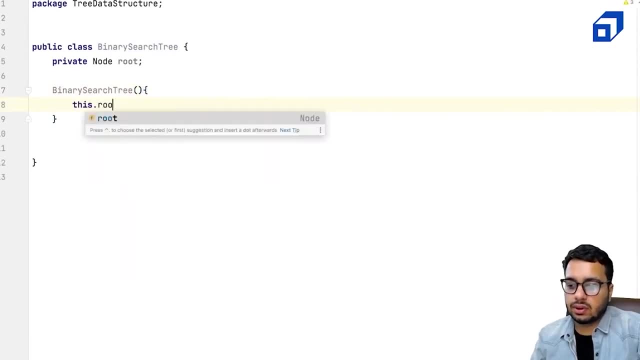 constructor and in this case I can say this: dot, root. this is equal to some build tree method that I am going to create right Now. let's see what is this build tree method going to be So I can say, okay, public void or public node, build tree. Build tree is going to read data. 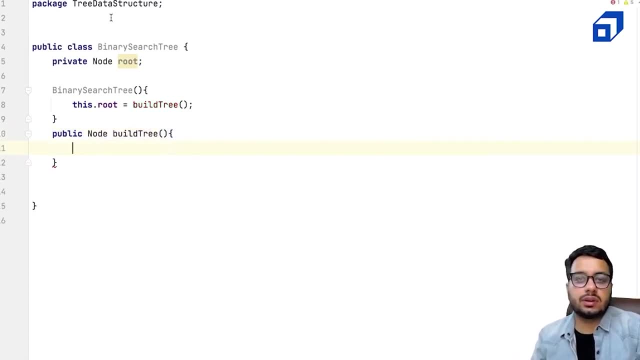 from the user and it's going to insert all the nodes into the tree one by one. okay. So in the example that we took, we said, okay, we will take these nodes and we will insert them into the tree one by one. So if you take eight, you insert it into the tree. then you took three, you insert it. 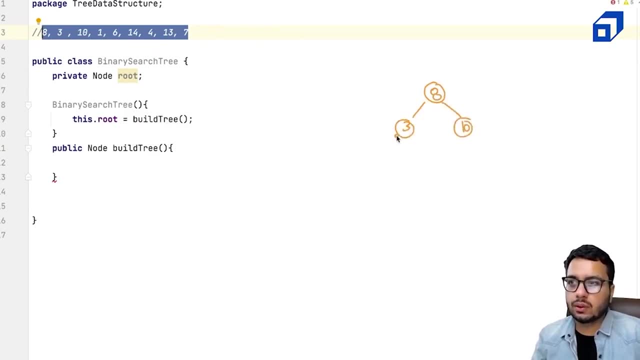 into the tree, then you took 10. you insert it into the tree, then you took one, and so on. right, So we what we have to do. we have to insert nodes into the tree one by one. So we will also build a insert method that will do the work for us. right Now. how do I read this data? So I will read it till I hit. 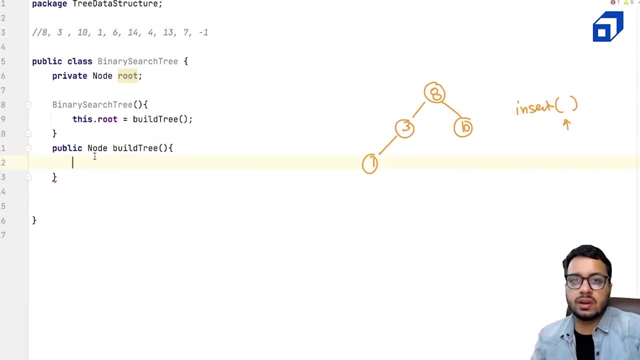 minus one, right, So this is one way. or you can ask how many nodes you want to insert and then you can read n numbers. both are fine, right, So I can do this as well. or I can say: okay, I will read n followed by n integers, right? So right now I'm doing it this way. that, okay, I. 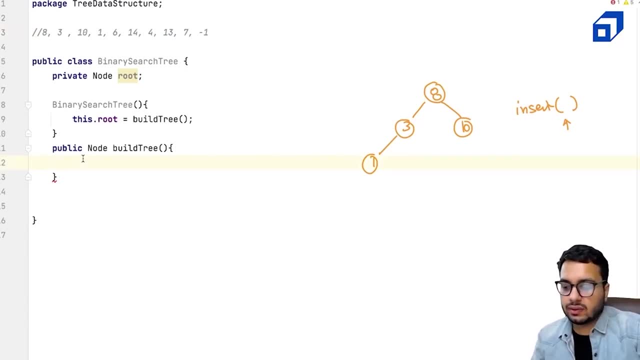 will read everything until I hit minus one, So I can say, okay, fine, scanner equals new scanner. and now I'm going to read data. right, So I can say: int data: this is equal to scanner dot, next int. While this data is not minus one, what I will do, I will insert. 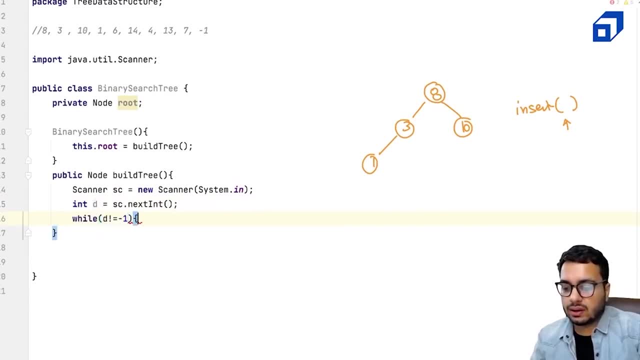 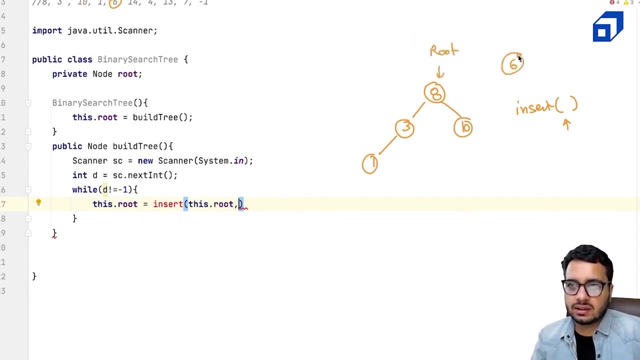 nodes into the tree. So while data is not minus one, I can say, okay, this dot root is given by the insert function and what I need to insert? I will say, okay, take root and take this data, insert it into the tree, Okay. so, for example, if I want to insert six, that's okay, fine, take this root node, take this number six and go. 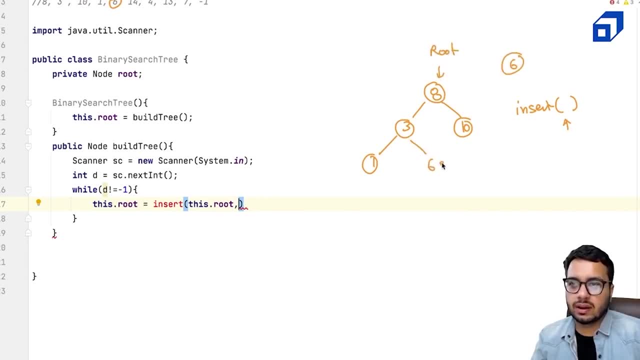 and insert six into this tree, So maybe six will go here, right? Something like this I'm going to do, So I will give data as well, right? And finally, I can, okay, build tree is going to return root, right? That is fine, right? Or you can do it like this as well. 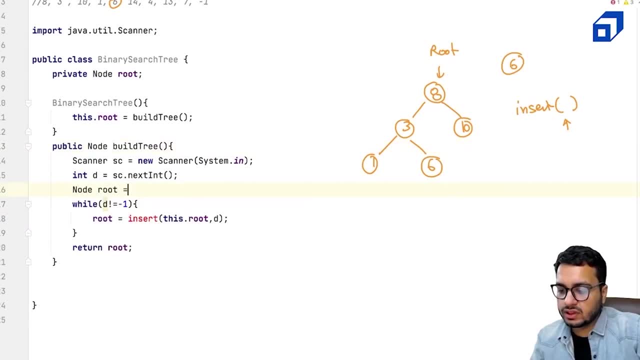 node root, which is initially null. You can say: say it like this as well: So I'm finally returning the root node, which will get a dated here, And this root is the data member root. that is here. Now let us write the insert method. 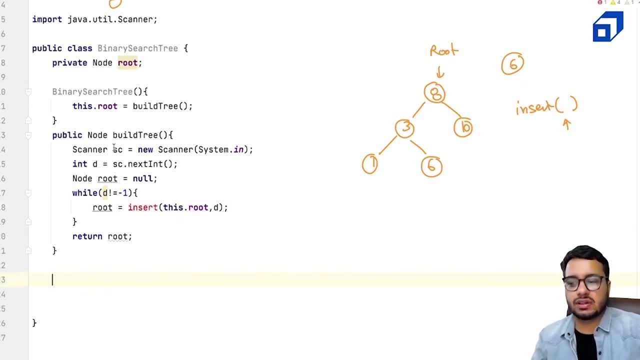 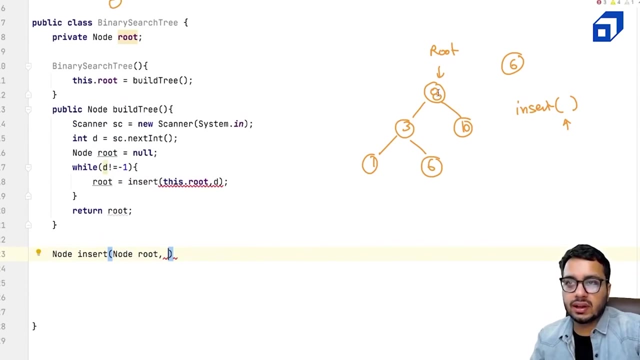 that is going to insert data into this tree. This is just like a wrapper function. Okay, The actual insertion will be done by the insert method. I want to say: OK, node insert. I'm going to get root node Now. this root node is in the beginning. it is this root node, But it's going to be recursive function, so this: 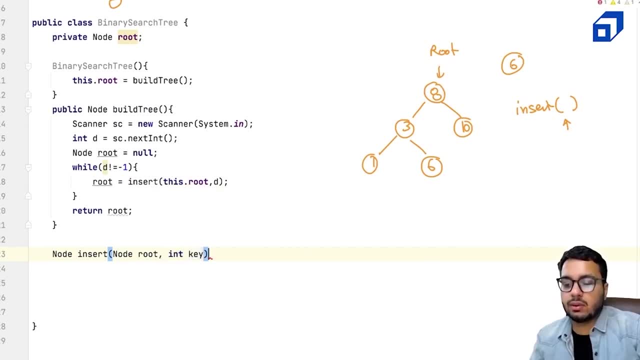 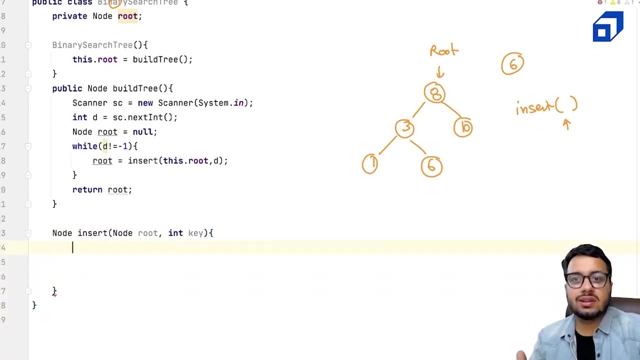 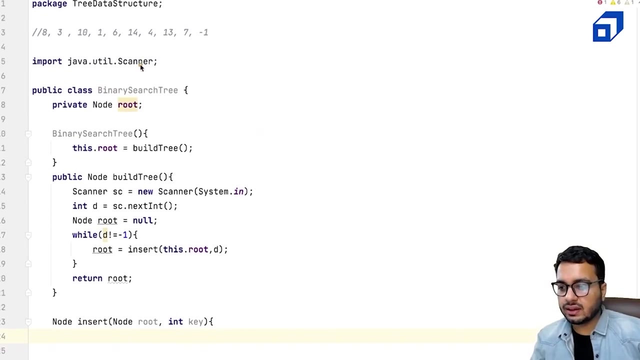 root node is going to change right and the key that I want to insert right. okay, so I'm already getting the key. now can you think how this insertion will work? okay, let us take an example of beginning. what is going to happen in the starting? in the starting you are going to insert: 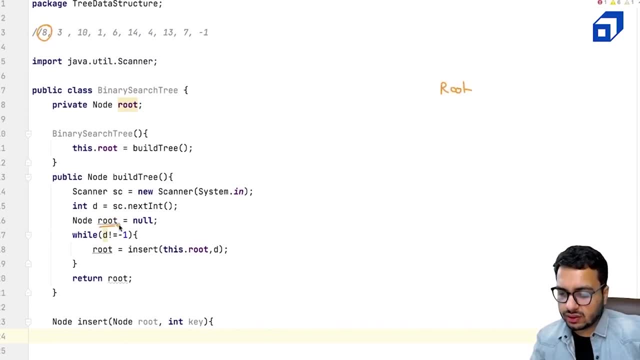 8, so root is null. so here the root is null and the data that you're getting is 8. so if the root is null, can I say inserting? it is very easy, just create a new node and return it so your root will get updated. so you can say: okay, root is equal to insert. you give the current root node, maybe you. 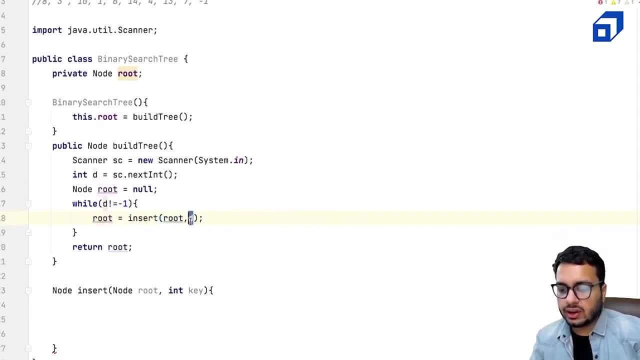 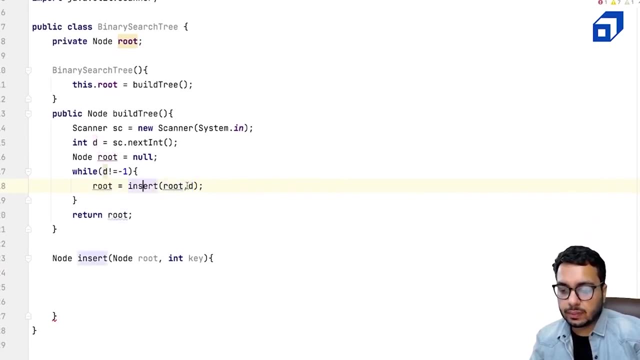 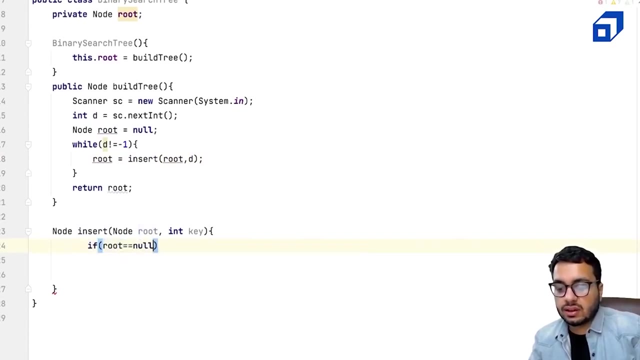 can give this root node, that is fine and you can give the data right. so what is going to happen? you're going to say, fine, I'm inserting. I'm inserting something into a null tree so you can say: if you root is null, that means you can insert it directly. you can create that node and you can. 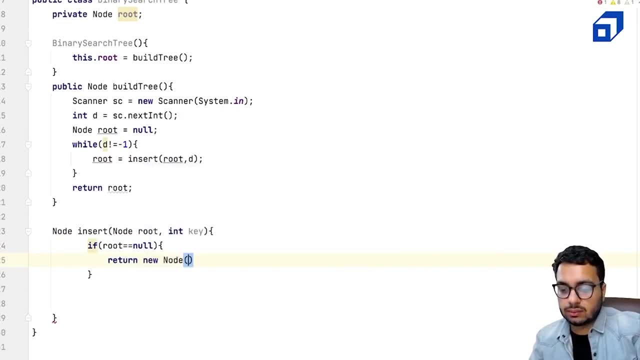 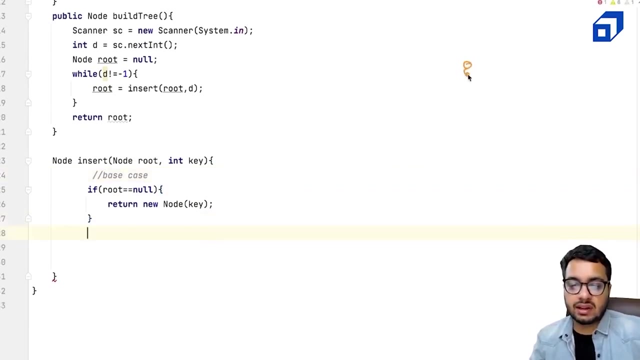 return it. so you can say: return new node and the data is equal to key. so this, this will also act as a base case and it will also help us in the beginning to create the actual root node of the tree, right? but if this is not true, for example, I've inserted 8 now, so root is pointing here, right? 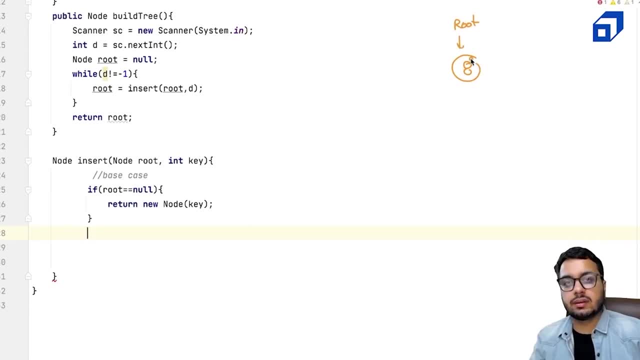 and suppose I want to insert 3 now this 3 is given input to this tree, right, so I will compare. is 3 less than 8? so I will compare if root dot data. sorry, if key is less than root dot data, then what should I do? I should go and 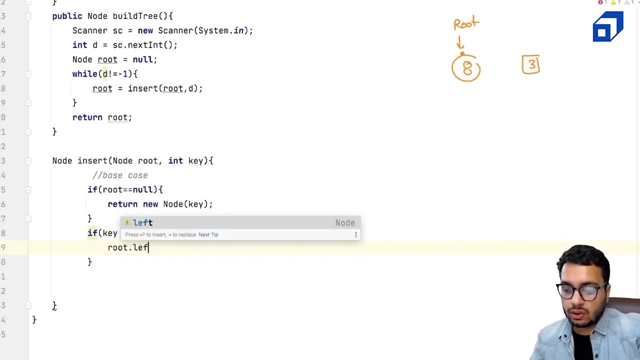 insert in the left subtree right, so I can say, okay, root dot left. now. this will point. this will point to a new subtree in which 3 has been inserted, so root dot left. this is equal to insert method again where in the root of left, and the key will remain it now. this is a very important step. you have to see it what I'm saying. 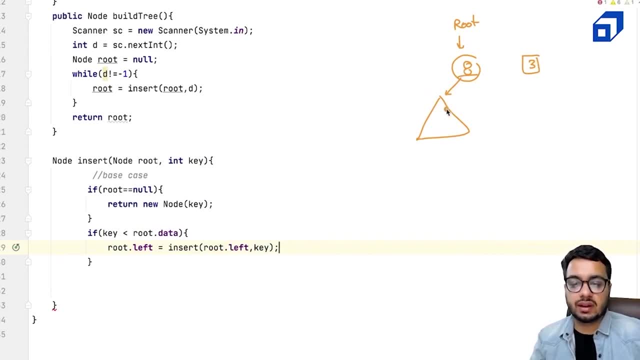 is that: go and insert 3 in the left subtree of 8. so if you hit this, what will happen? your root will come here again. you will observe that root is no, so you will return new node of that key. so you will say: okay, fine, i'm going to create a new node, 3 and i'm going to return it where. 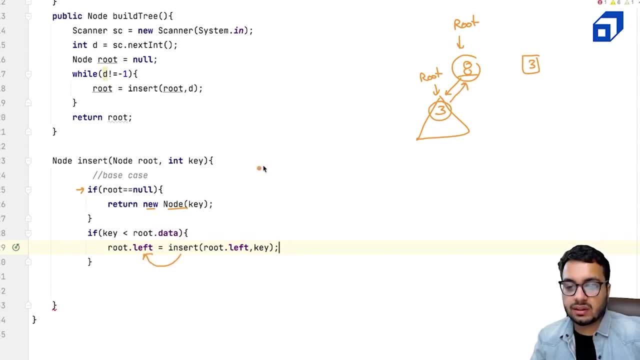 you're going to return it. you're going to return it from here. that means it will get updated in the left of it. so this is how three will get connected in the left of it. okay, let me finish the code. i will do a complete dry run. okay, and the complementary case: okay, we can make it less. 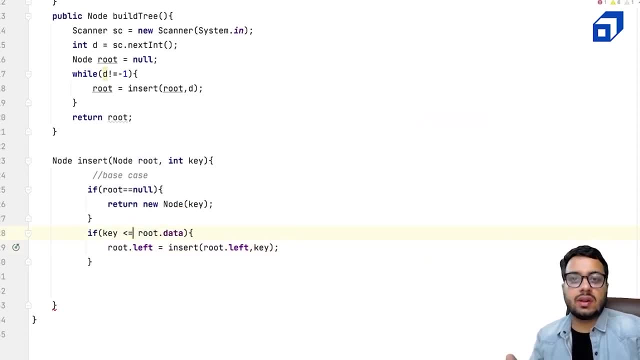 than equal to. so if duplicate elements are present, all of them, they will go into the left separate. else this is not the case. else, root dot right- this is equal to insert root dot right comma. that means, if it is greater, go and insert that node into the right subtree and update. 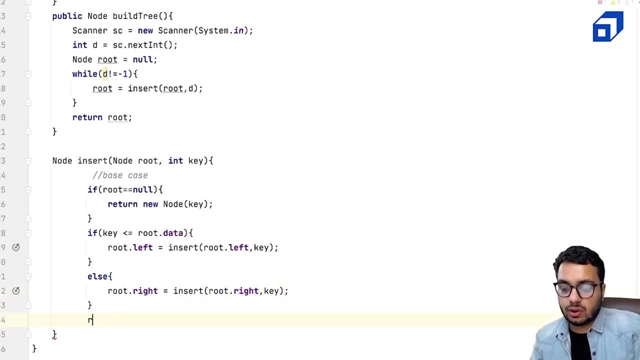 the root dot right, okay, and once it is done, what i have to say? i have to say: return root. right now. this is important because every function is expecting that address of a tree or a subtree or a function is expecting that the address of a tree or a subtree or a function is expecting that. 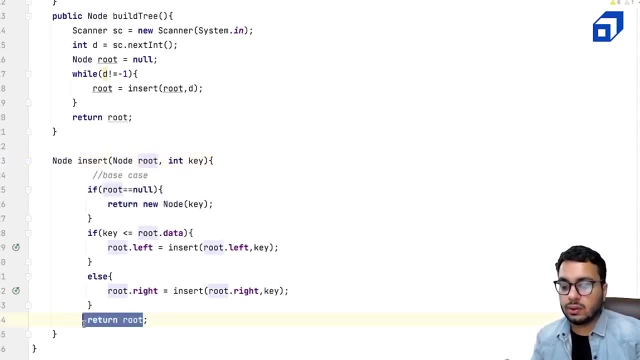 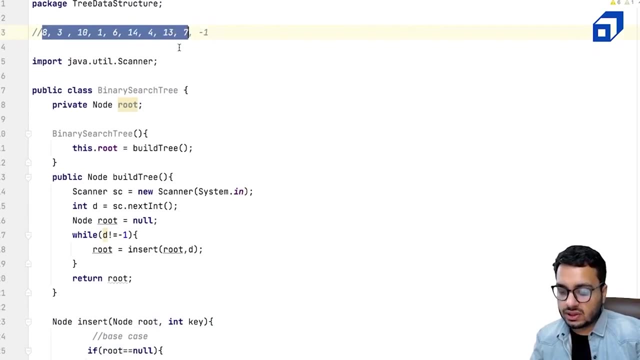 a root node will be returned. so we are going to return the current root. now let us take an example of, let's say, eight, three, ten, one, six, and let us try to insert some of these numbers into a bird tree. okay, so i'll just take this example and i will dry run this function. 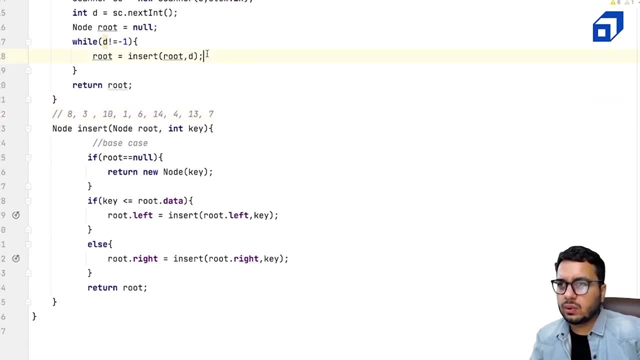 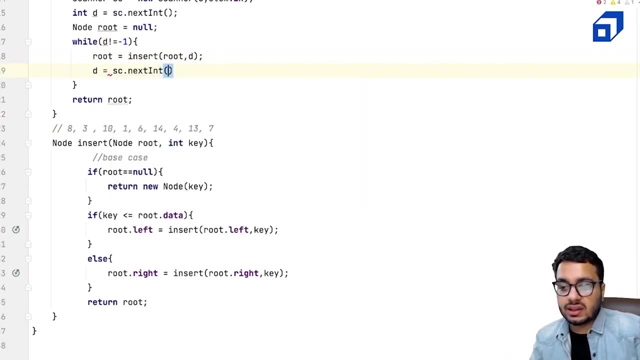 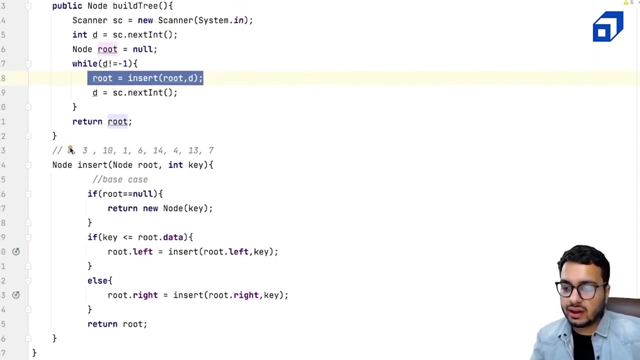 what is happening. oh, okay, i think i missed out one thing here. i will have to read the data again also. so i have to say data equal to scanner dot, next data. so i'm inserting a number, okay, and then i am reading the next number, right? so first of all i will read eight. fine, so if 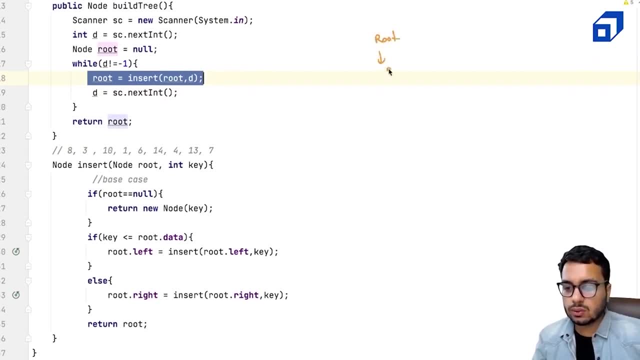 for eight. root is null, the root will point to it: is okay, return new node of key, so insert call is over. next time i am reading this number three using this line, data is equal to scanner dot. next end data is not minus one, so is okay. root is equal to insert into this tree, right? so root is now eight. and i'm saying insert dot minus super jazz. and you can also find this after i run these percent number under cocoa and i'm again using the line. data is equal to scanner dot. asking data is not minus 13, so is okay. root is equal to insert into this three, right? so root is now 8 and i'm saying insert. 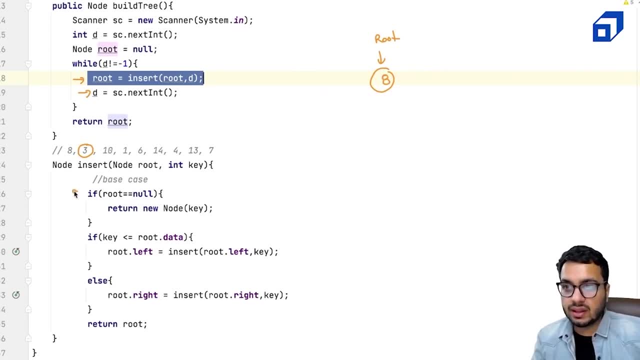 three. so if you want to insert three, what? what will happen? the base case is not true. you come here. if key is less than equal to root data. yes, root dot left. this is equal to insert root dot left comma key right. so i will draw this call stack as well. so i have eight, so eight makes a. 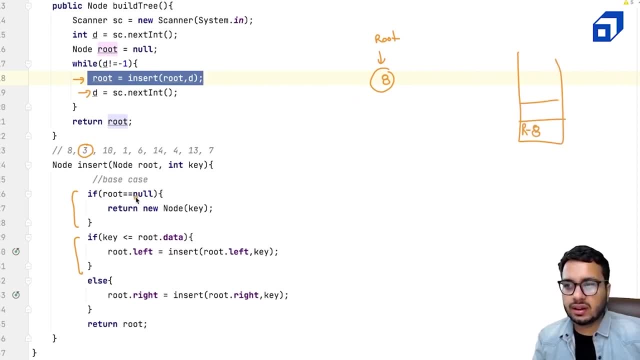 call on the left. the left is null. so you hit the base case. you say: return new node of key right. so it returns a new node three. so this function returns a new node three. now where is this three getting updated? so three is getting updated in the root dot left. so it is getting connected in the 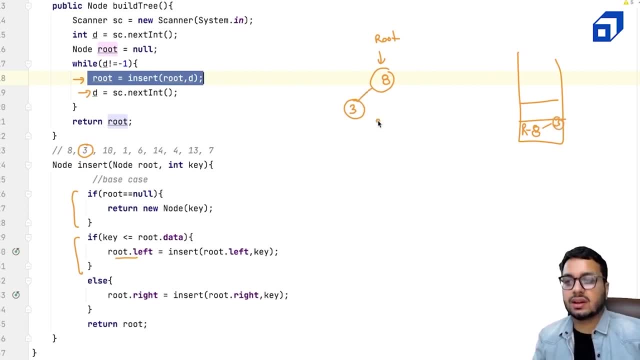 left of it. so this is how it is getting connected, right. so this is over. and now from this function, call you return root. you return root. so you basically return the address of 8 back into the build tree function. okay, now you want to insert 10.. okay, you got 10.. again, you compare 10 with. 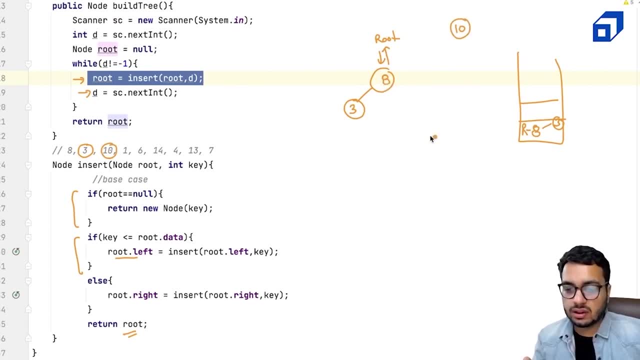 respect to 8, right. so what happens? you call the insert function, take this tree, insert it now. root 8 is not null, 10 is not less than root. so you come into the else block. you say: root dot right. this is equal to insert root dot right comma key. a root dot right. this is null. that means you. 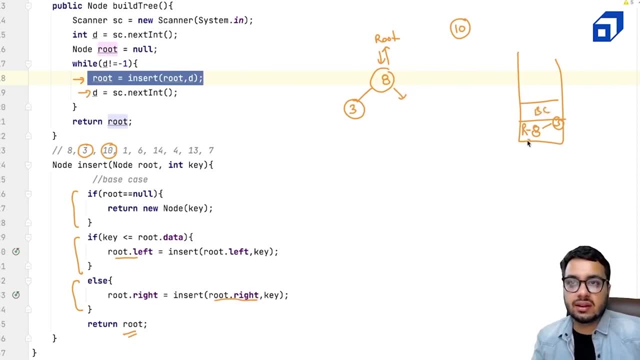 again hit the base case. this base case returns a new node, that is 10.. where is this node returned? it is returned to the previous function, which is this, and where it is getting updated. so 10 is getting updated in the right of 8. so you get 10 here and this base case is over. so 8 is connected with 10. 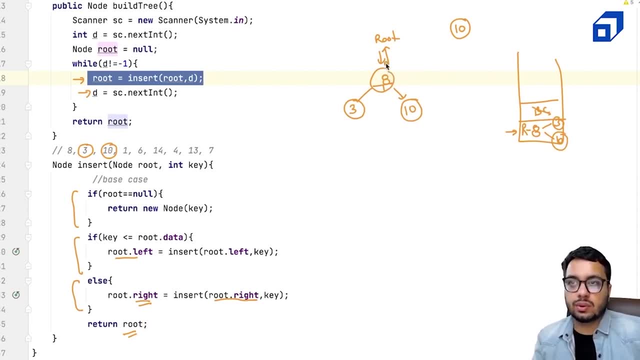 and you return root. so what is the root node? this 8 is the root node, so you return this address back into the main. right now comes the next node. you read one and you want to insert one into the this particular tree. so now this is the tree: 8, 3 and 10. right now you want to insert 1 here. 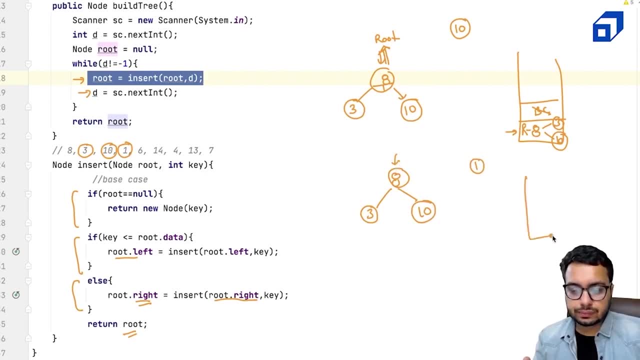 1 is less than 8, fine. so it says: go and insert 1 in my left sub tree. it makes a call here, right? it makes a call here now, when you reach 3, so your root is 3, right, and you again compare, is 3 is 1. 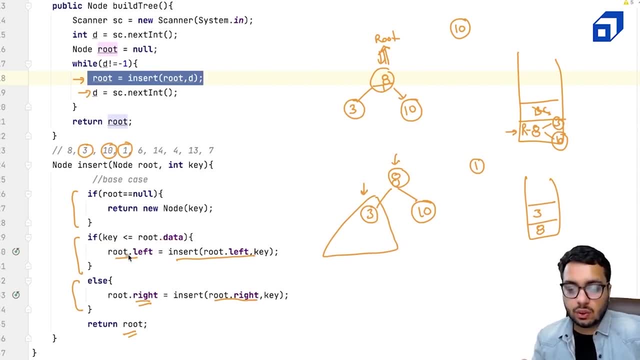 less than equal to 3. the answer is yes. so you again make a call: root dot left. this is equal to insert root dot left. so you make a call here. so you make a call in the left of three. now this value is null, so you return a new node. 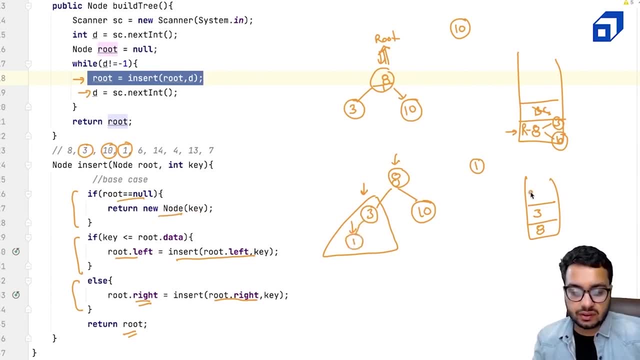 that is one. this one is updated in the left of three. so you return one, one gets attached in the left of three and then you say return root. effectively, now you're returning the address of three back to it. now eight's left is again. earlier it was referring to three, now again it is referring to three. but 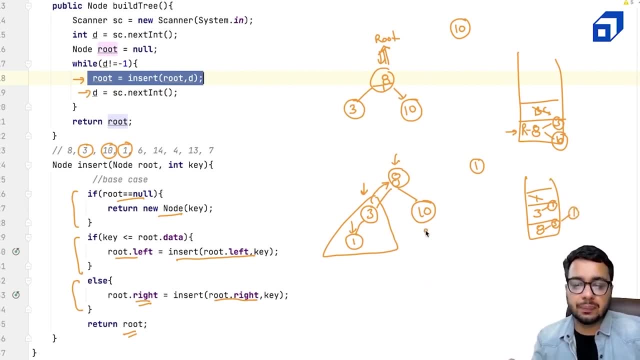 now which three. one is also attached. okay, so that is what i was saying, that one gets inserted in the left sub tree of eight. right, so this is again updated. so earlier it was storing the address of three, now again it is storing the address of three. and again you say: okay, from this function i am going to return root, so you are going to. 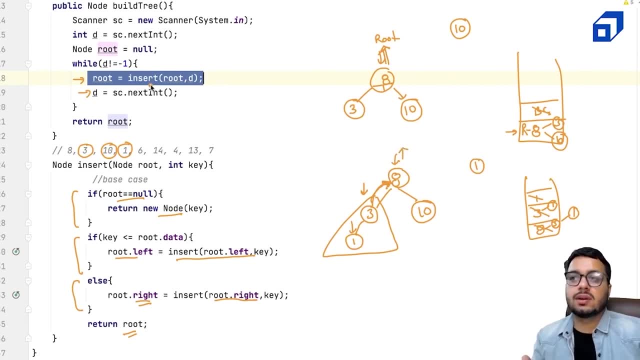 return the address of eight back into the built tree method. okay, let us do one more insertion and let's say i want to insert six. so six is less than eight. so this is now the tree: eight, three, one and ten. now six is less than eight. i go here. six is greater than three. i go here. 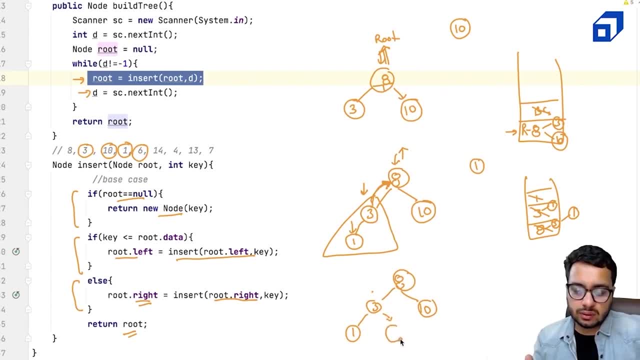 so again what happens? this is null. so you return a new node, so you create six, so that address is attached in the right of three, and from three you say return root, so three gives us address to eight and eight gives its address back to me, right? so by keep on doing this you will be able. 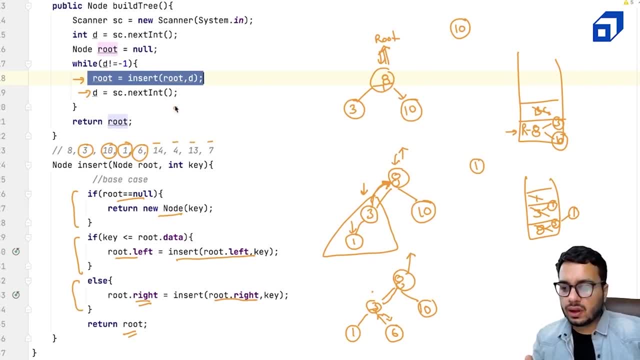 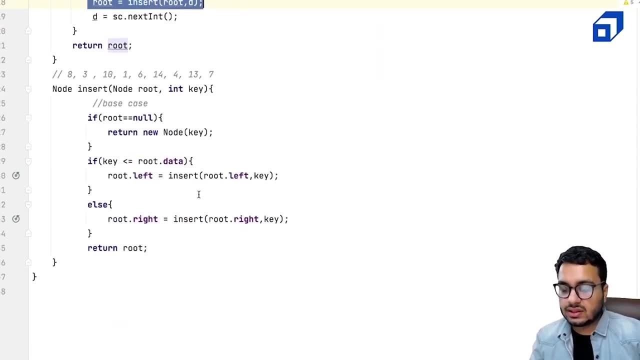 to insert all the nodes until you hit minus one into this tree, right? so i hope you have understood the insert method. the insert method is going to take order of edge time to insert one node into the tree right now. let us write in this code and see if it works. 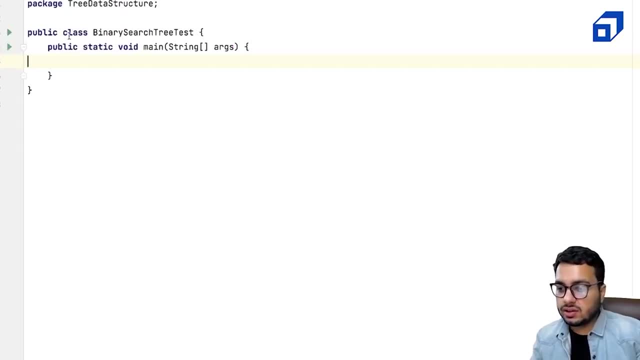 okay, i want to execute this code dry run. we have already done so. i have a binary search tree test class. i have created a main method. so i have to create a bst object here. so i have to say binary search tree bst. this is equal to new binary search tree. 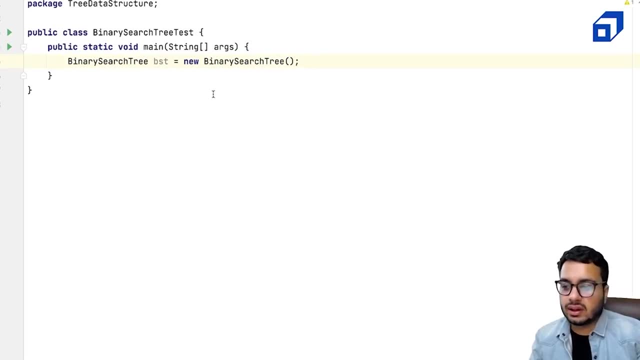 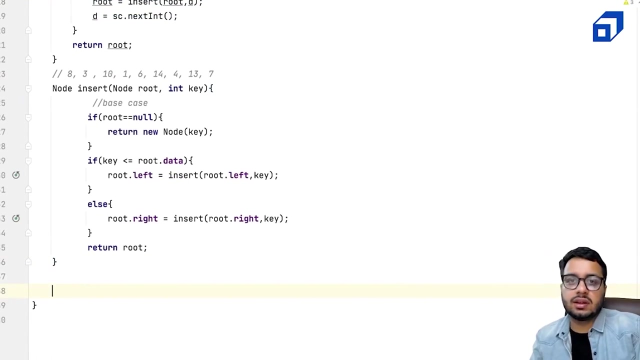 this will automatically trigger the build tree method and it it will start reading input from the user. okay, but if i want to display this tree, maybe i have to do some kind of reversal as well. so I go into the binary search tree class and here we can write a method for. 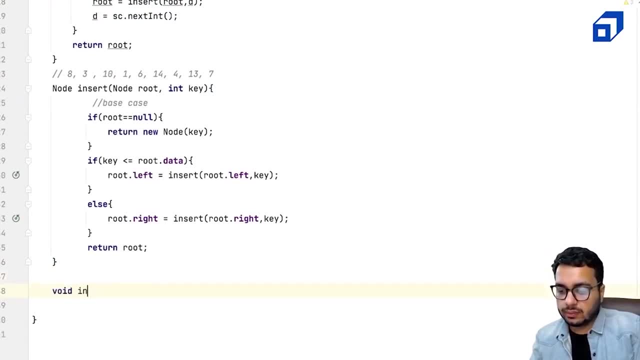 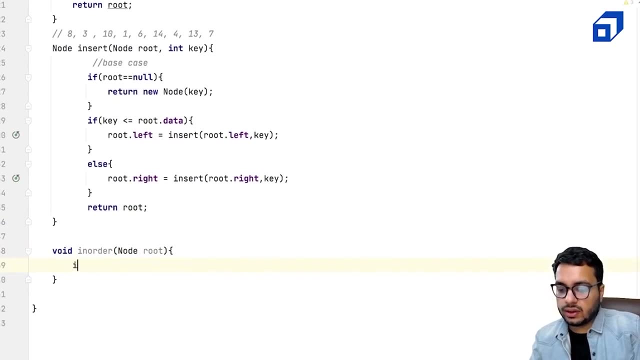 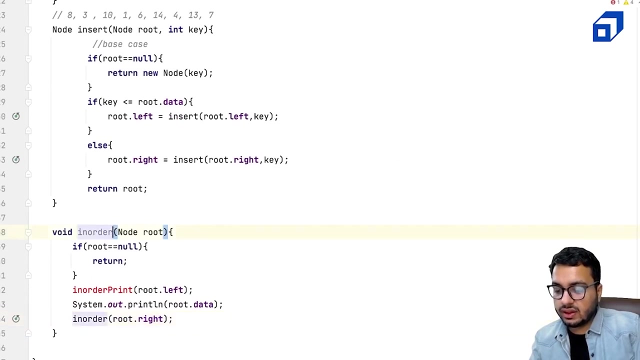 doing the in order print of this tree, right, so void, in order. I can say node, root and here I can say: okay, if root is null, do nothing, otherwise do a in order print on the left sub tree, print the root data and do a in order print on the root dot, right, so let's call this as in order print. 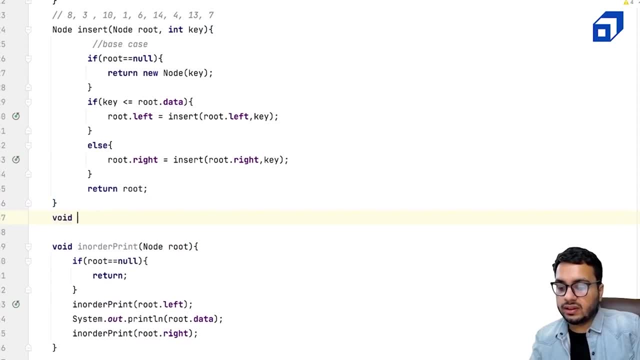 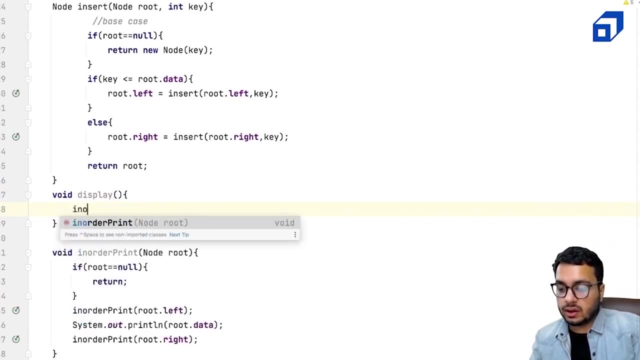 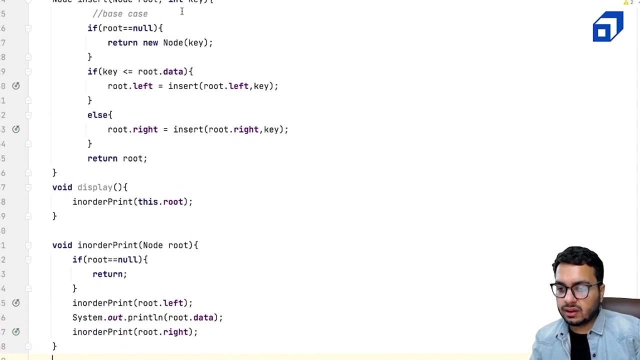 in order print. okay, let me create a display method from where I will call the in order print method so I can say: okay, uh, in order print, and here I give root. or you can say this dot root, both are okay. this dot root means we are talking about the data member root. okay, so display method is done so. 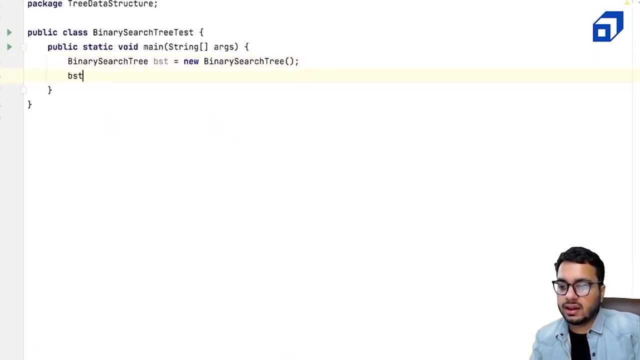 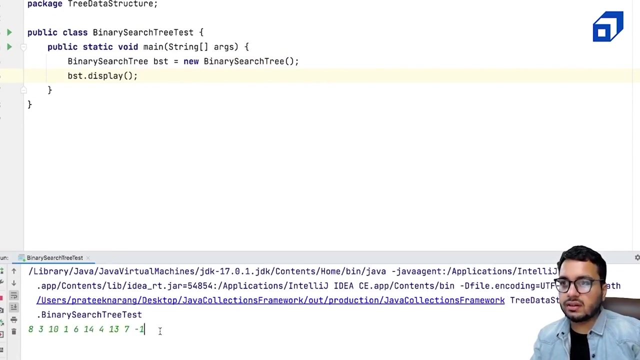 I am going to create the BST and I can say: BST dot display. let us execute this code. the build is complete. it is waiting to uh, waiting for us to give input, so let us give the input. and here we got some output. so this is the output. 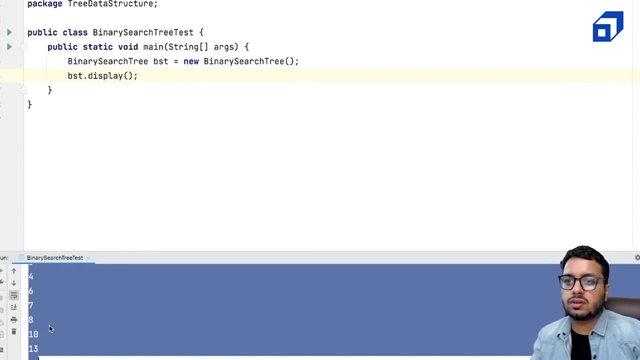 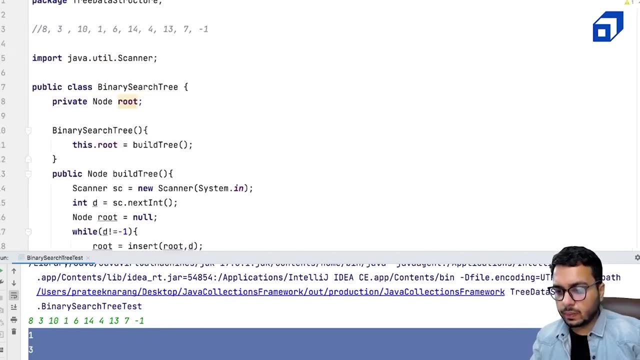 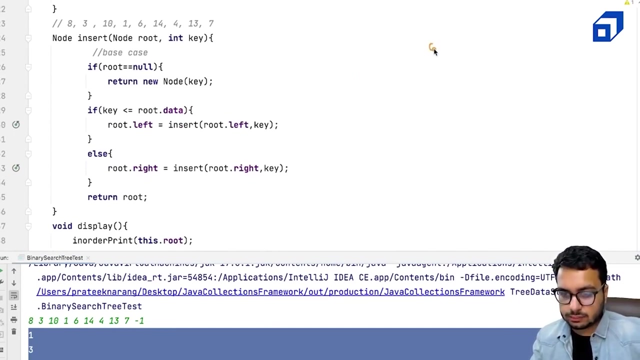 of, in order, traversal of this tree and this output looks sorted. let us see, uh, what output we should ideally get. so let us quickly create a tree with these numbers. so I have, uh, eight, I have three, I have ten, I have one, I have six, I have 14, I have four, so four will go here. 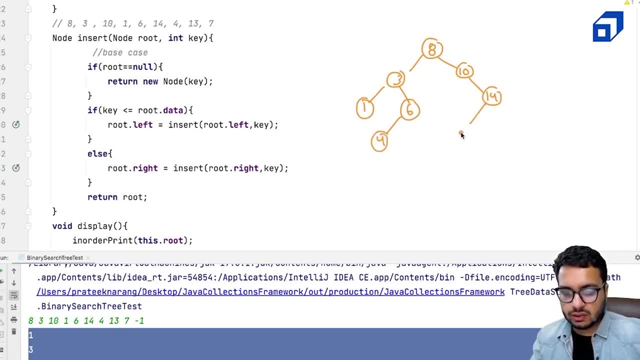 then I have 13, so 13 will go here. then I have seven, so seven will go here. that's it right now in order. traversal that means before printing root node you will print left and then you will print right. so now we know all the nodes in the left chapter are smaller, all the nodes here are greater. 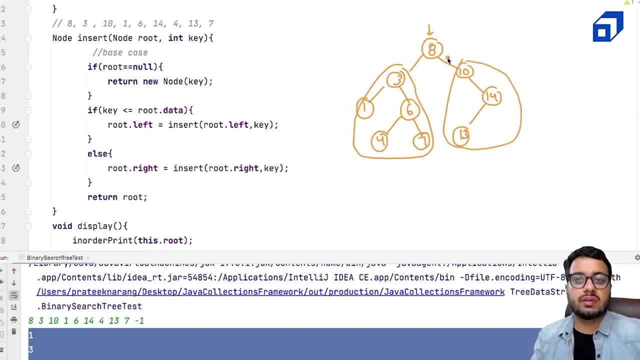 right, and if you do it for every node, you will observe your output will be sorted. so at three. if that is okay, go left. that means I will print one, then you will print root. that is three, then you will print the right sub tree. so for six, you will print left, root, right. so you will print four, six. 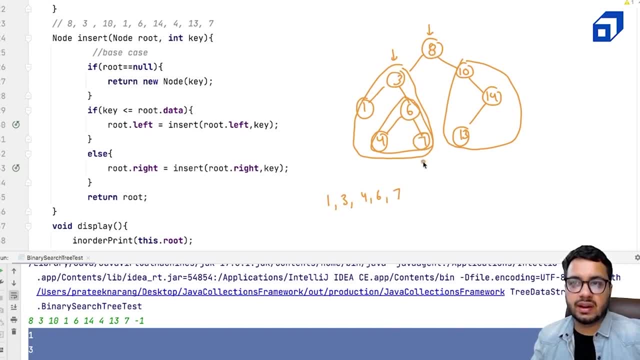 seven and then you go back here for eight. left sub tree has been printed, so you print root and then you print right. so you come here at 10, you circle left, which is null, then root, which is 10, then the second again, you will print 13 and 14.. so this is the expected output of in order traversal. let us 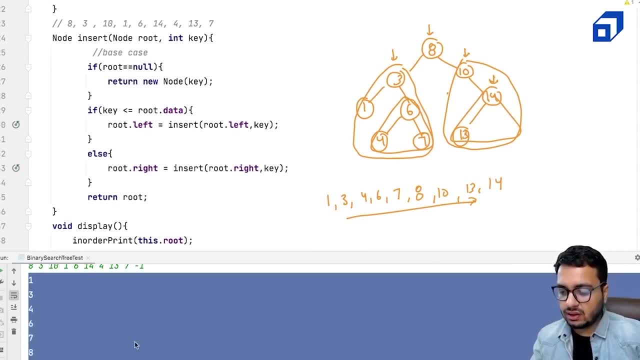 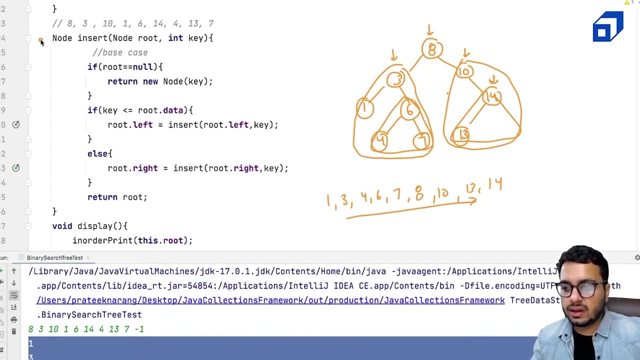 verify if it is correct. so we are getting 1, 3, 4, 6, 7, 8, 10, 13, 14, which is absolutely correct. so that means our build tree and the insert methods. they are working perfectly fine, right? so I hope you. 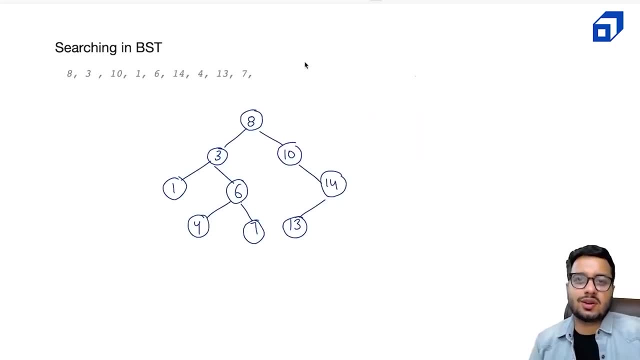 have understood the insertion in a binary search tree, so now let us talk about the search operation in a binary search tree. so, given this BST, I want to search for a particular node. for example, let's say I'm given that I am searching for a key that is two. how do I search for two? right, so I will start from the root node. I will 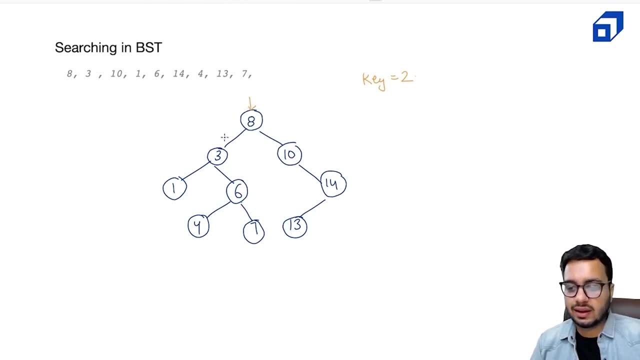 compare eight with two. so I will say, okay, two is less than eight, so I will go here, I will go left. two is also less than three, so I will go here, and here I compare if two with one. so what happens? if two is present, it must be on the right of one. so I go here, so I go in the right of one. but 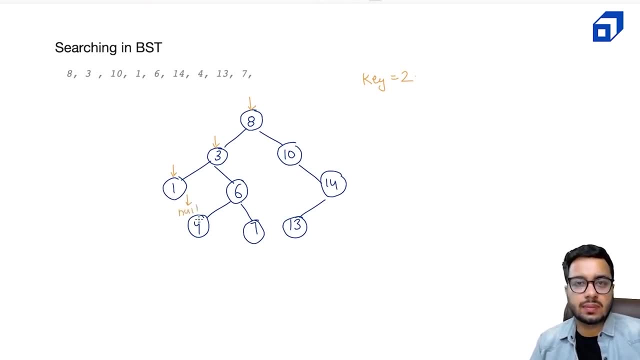 as I reach here, I see that I am hitting a null value. that means two is not present, right. so one of our case would be that if I hit a node that is null right, that means the given key is not present, so I can simply return false. that will be one kind of a base case. right now, suppose I am not searching. 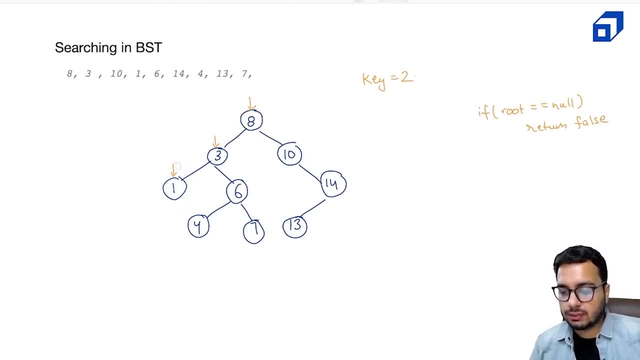 for two, but I'm searching for, let's say, uh, seven, right, so seven is present here, so let's see how we can do it now. if I compare seven with eight, I know it is less than eight, so I will go left if I come to three. 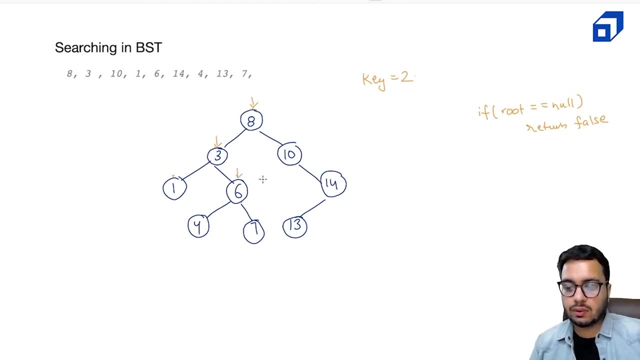 seven is greater than three, so I will come towards right. and at six, seven is greater than six, so I will again come towards right. so now I am hitting a node where my root data matches with key. so what should I return? of course I should return true. so if root data matches with my key, I would be returning. 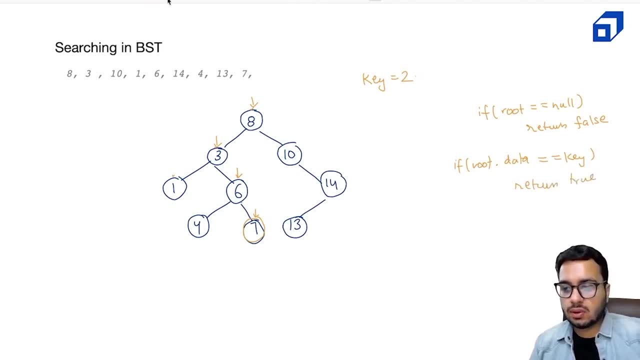 through from the method. right now, let us talk about a recursive case. if we are searching recursively, so what exactly we are doing right? so we are saying that, fine, I am going to compare root node with- uh, the given key. let's say that the key is seven. so I'm comparing eight with seven right now. if the key is not, 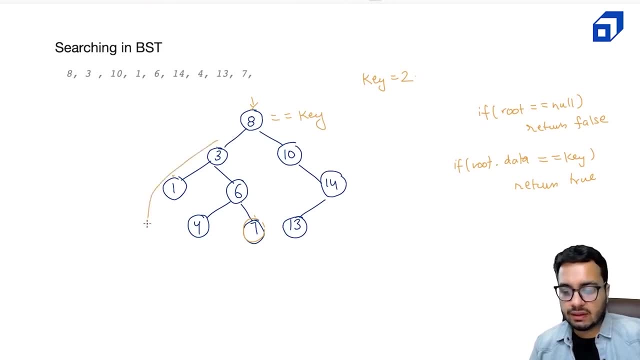 matching. so what? I'm saying that okay, if the key is lesser I will search in the left subtree. whatever is the answer of left subtree, I will return that answer. now, suppose the left subtree says true, that key is found, I will return true. but if the left subtree says false I will go and search. I will not go and search. 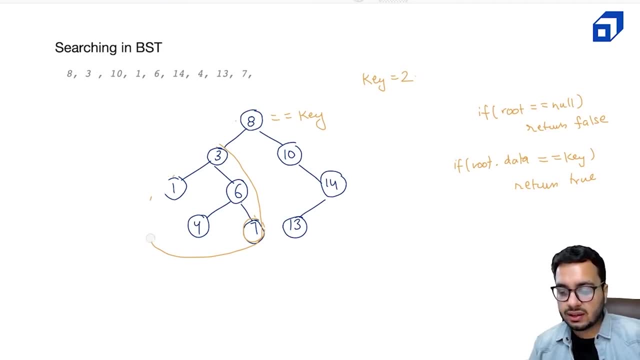 in the right subtree. why? because I am already checking whether I should go left or I should go right. right, because if the key is less than or equal to, it will be present in the left subtree. if the key is greater than or equal to the root node, it will be present in the right subtree. let us take 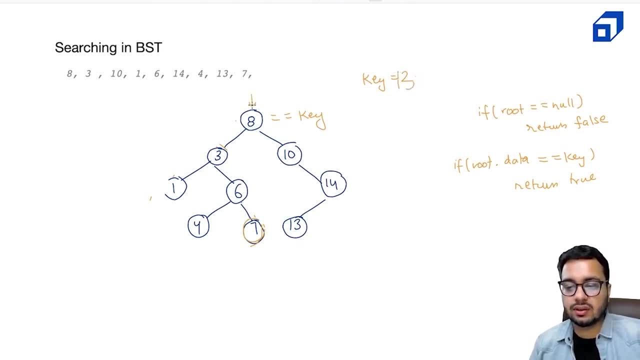 an example of 13: right. so now 13 is greater. so I will not make a call in the left subtree. I will make a call in the right subtree. now, at 10, 13 is greater. what I do. I say: okay, go and search in the right subtree. at 14, 13 is less. 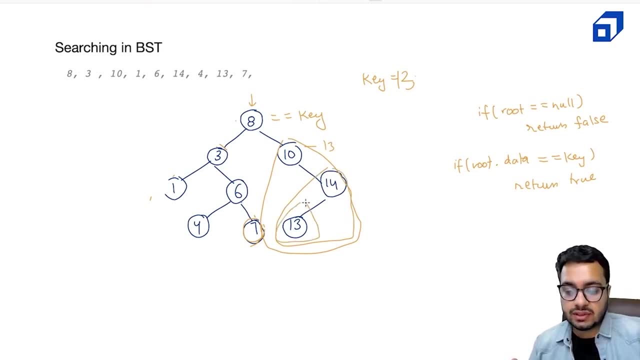 than 14.. so what do I do? I say: go and search in the left subtree. now, as I reach this node, I say, okay, this matches my key. so what I will do? I will return true, this 14 will also return true, this 10 will also return true and this 8 will also return true. so this is how true will be propagated back. 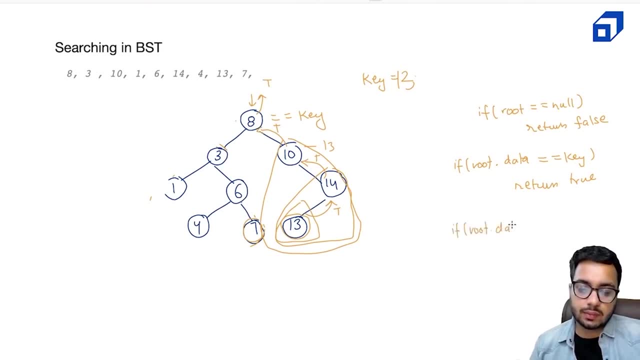 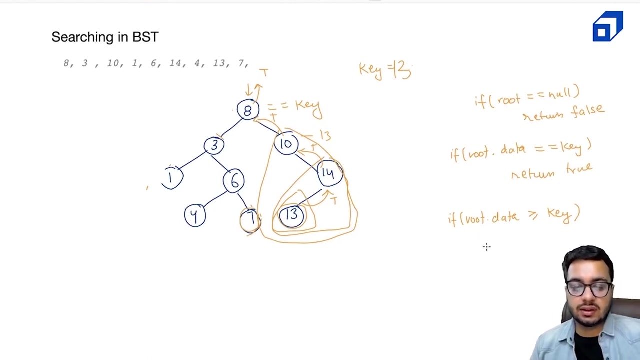 what I have to do if root data is- uh, let's say root data is greater than equal to key. right, so that means key is less than equal to root data. that means I will return the answer of the search method by calling the left subtree. so I will say, okay, return whatever has been returned by. 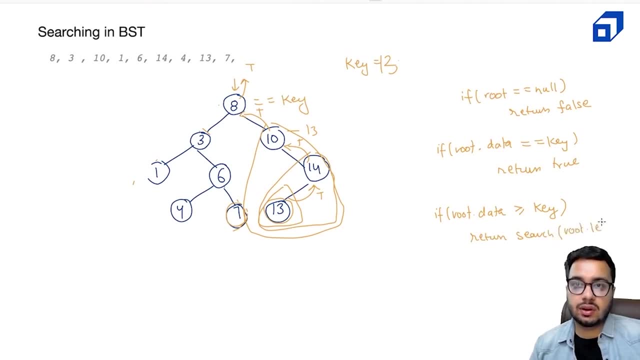 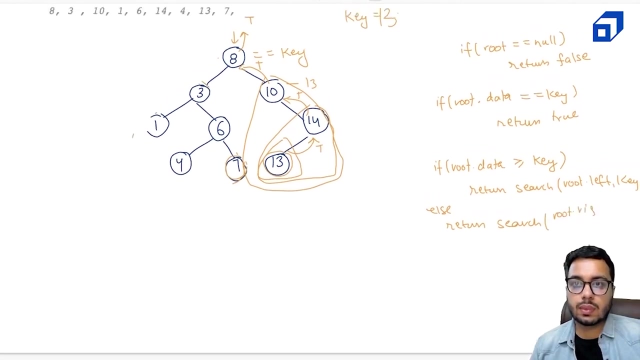 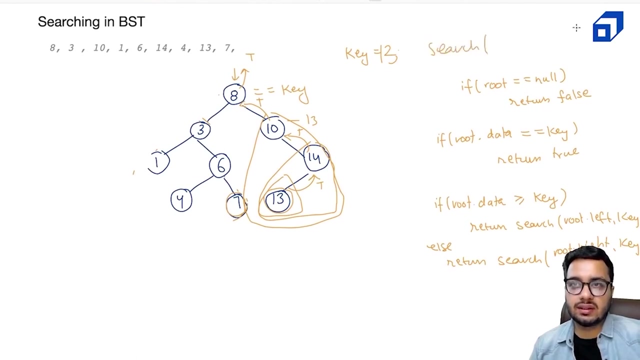 the left subtree for that key. so root dot left, ôn key right. otherwise I'll say: return whatever has been returned by the search method by calling it on the right tree. so root dot right. so this will be my search method. now let us quickly write this method in our code as well. 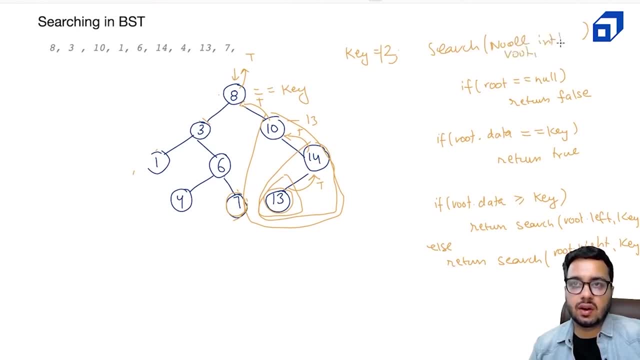 and then we will see whether this works correctly or not. it should. it should work right. so this- I'm writing it recursively, can also write it iteratively, right? so the only thing that you need to do is you need to travel at max from the root node to one of the leaf nodes. in the worst case, that means the complexity of 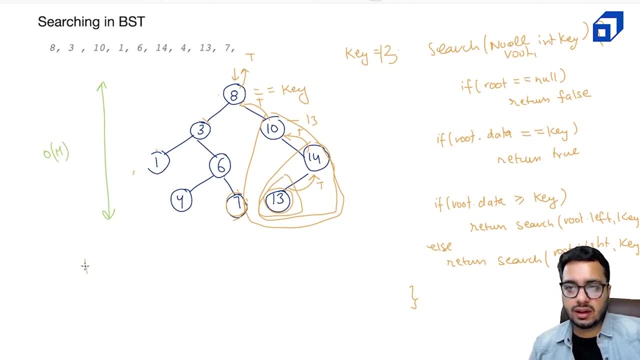 this method will be order of h, where h can lie between n and log n, right? so in the best case scenario, when the tree is perfectly balanced, your height will be log n. in the worst case, if all the nodes are on one side- that is called as a skewed tree- your complexity for search operation will be. 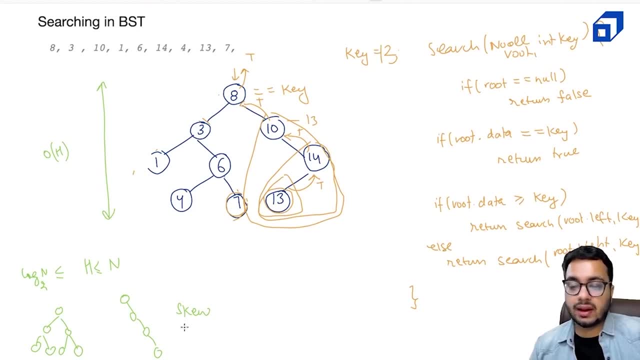 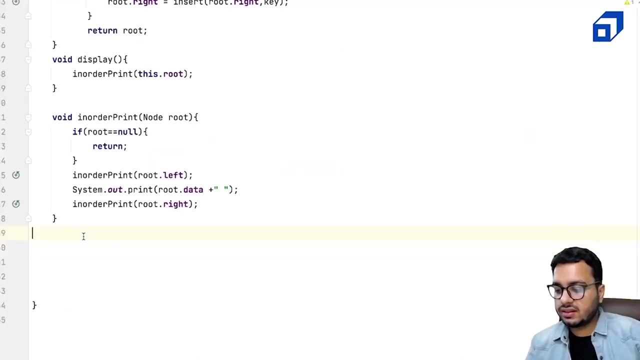 order of n. now, it is much better than binary tree, because in binary tree you have to search for across all the nodes, but here we know that we have to move in one direction, either left or right, but not both. okay, let us quickly code it up and see. so let us write a method called search, so it. 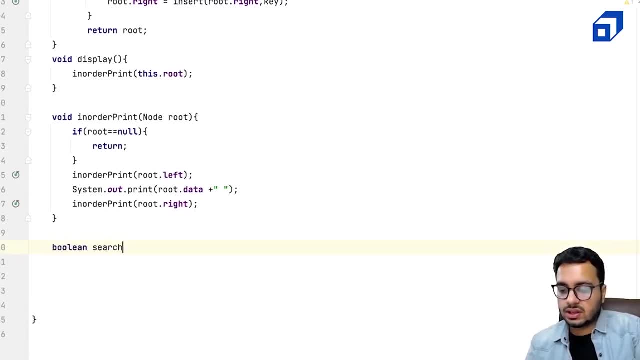 will have boolean return type so i can say: boolean search, i am going to get the root node and i am also going to get uh, the key that i am searching for. okay, let's say this is some search uh function. right, so it's a recursive function, so i have to. 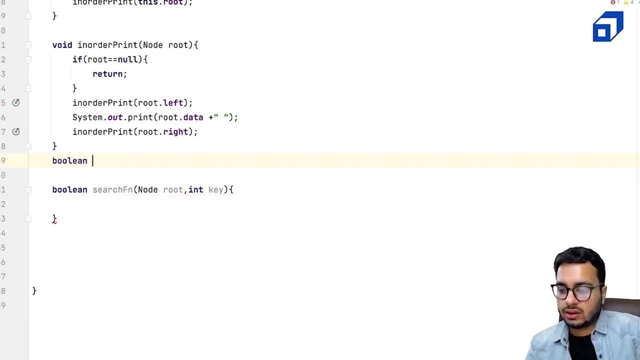 write a wrapper function as well, so i can say: boolean search, uh, where i am just getting the key, so it will return whatever has been returned by the search function, and here i will pass the root node and the key. now let us see how to do this. so i am going to write a wrapper function. 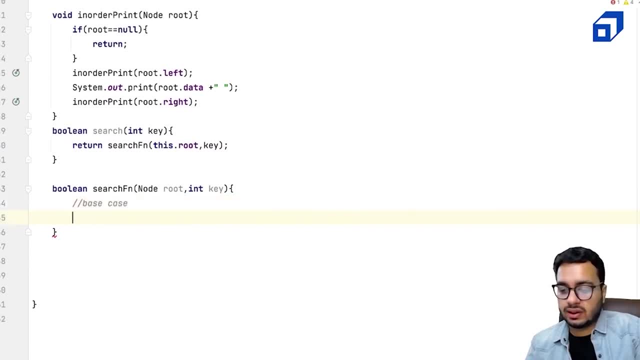 let us see how this can be done. so i discussed there will be two base case, so you can stop. if your root is null, that means the key is not present, so i can say return false in that case. but if your root matches with the key, you can return true in that case. okay, otherwise i have 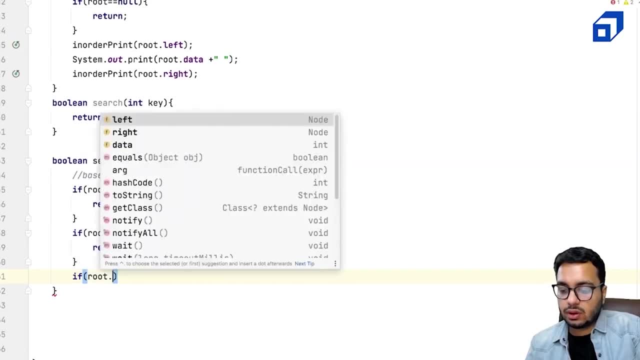 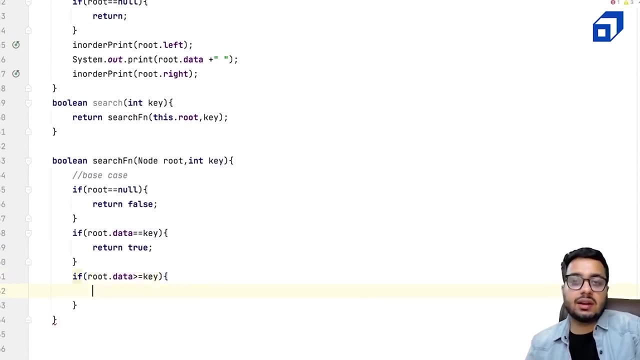 to compare. okay, so i have to say: if root dot data is greater than equal to key, or you can say key is less than equal to key, or you can say key is less than equal to key, or you can say key is less than equal to root data, then you have to call the search function on the left and you have to. 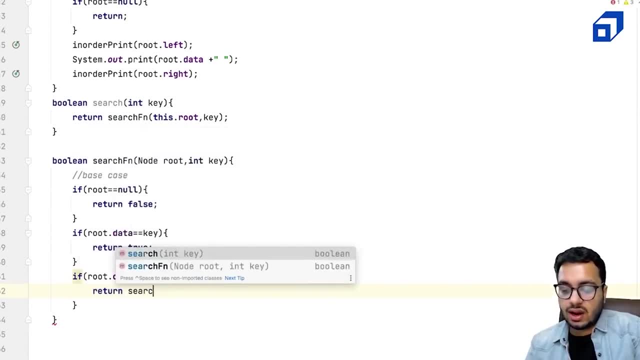 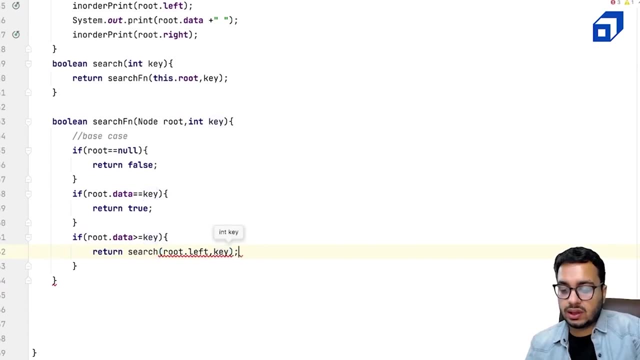 return whatever that function is returning. so you return the output of the left chapter. so search in the left chapter. that is root dot left comma key. else you can return the output of the right chapter. so root dot right comma right. so this will be your search function. recursive function is the 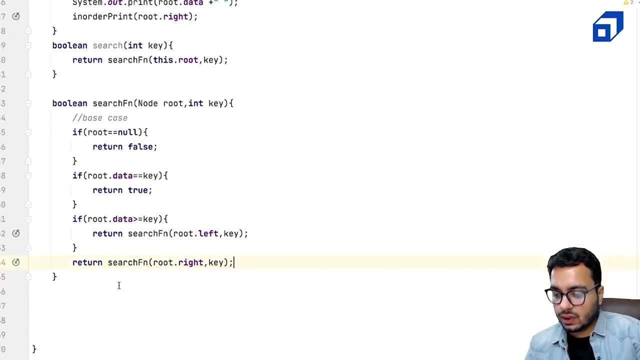 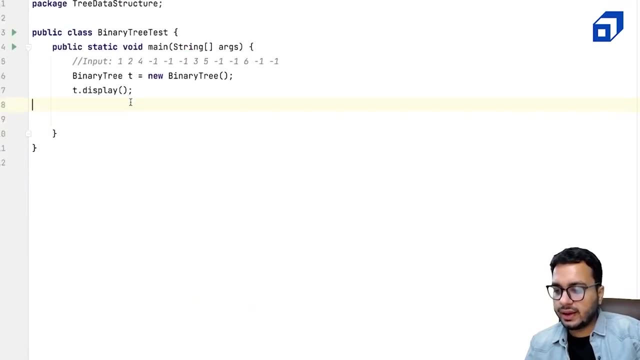 search function. so this looks good. now let us test our method. so here i can okay s out p dot search. let's say i'm going to search for four. sorry, this is not, uh, the correct file. i have to do it in binary search tree. so bsd dot search, i can say let us search for 4. 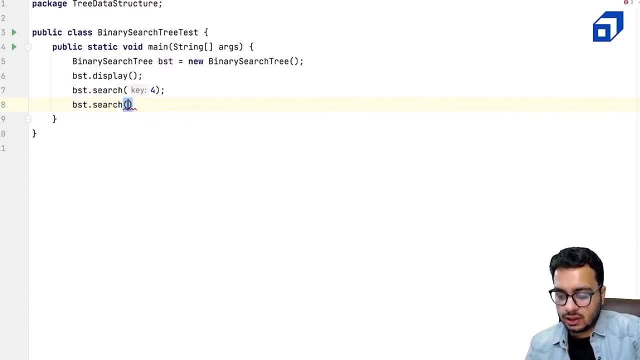 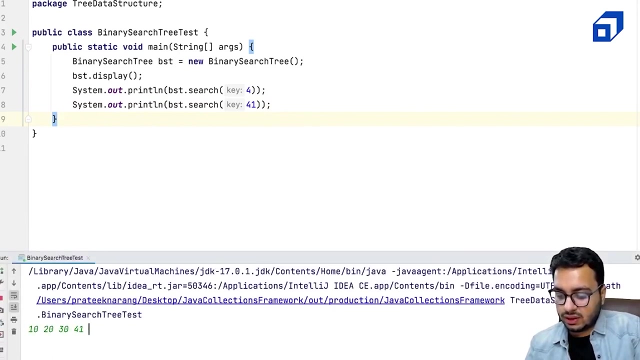 and bstsearch, or let's say 41, right? so i will s out output and same here. this looks good to go and let us do this same thing. let us run our code now. let us give some elements, let's say 10, 20, 30, 41, 3, 5, 6, 8, 9 minus 1, right? 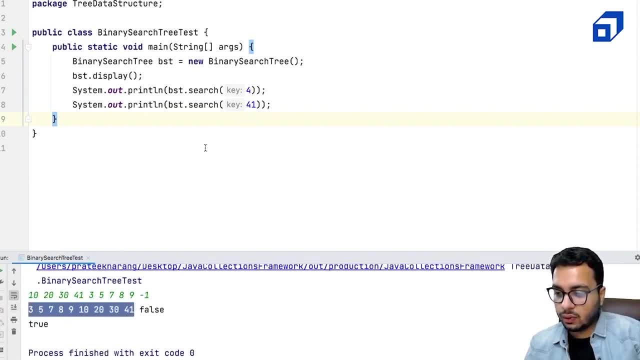 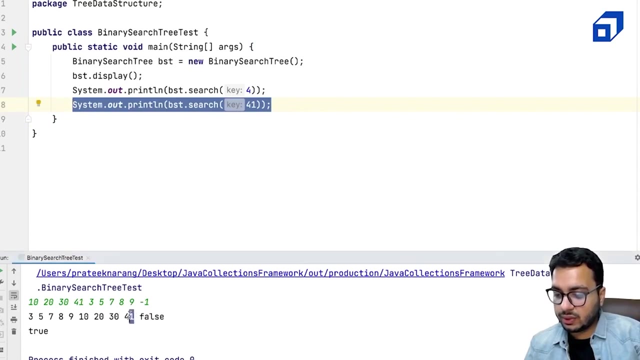 this creates a tree. and for the value 4 i'm getting an answer false, that 4 is not present. and for other values i'm getting the tree is: uh, the 41 is present. the 41 is present here. right, and you can see in order. display is looking sorted. 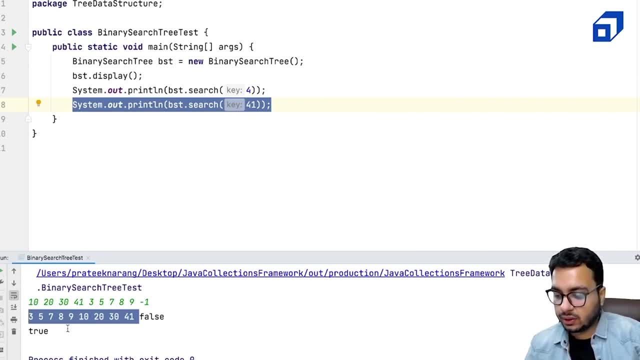 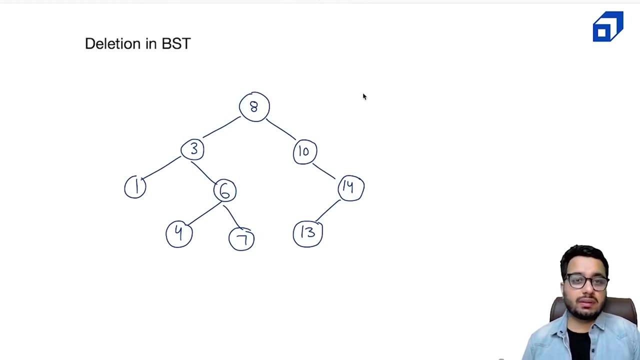 and 4 is not present in this and 41 is present. okay, so this is how the search method is working. i hope you understood the search method really well. next we will move on to deletion. let us discuss deletion in a case of a binary search tree. so deletion means that: okay, i've given a particular node and i want to remove that. 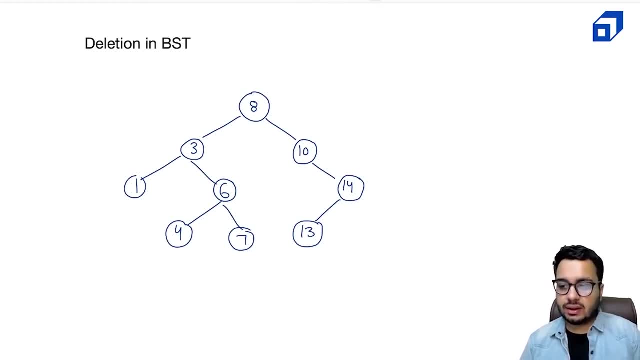 node okay. for example, someone might say that, okay, let us delete 13, or let us, you know, delete 3 or let us delete 8, right? so if you observe closely, there are three kinds of nodes. okay, so there are nodes which have no children, also called as leaf nodes. there are nodes with zero children deleting. 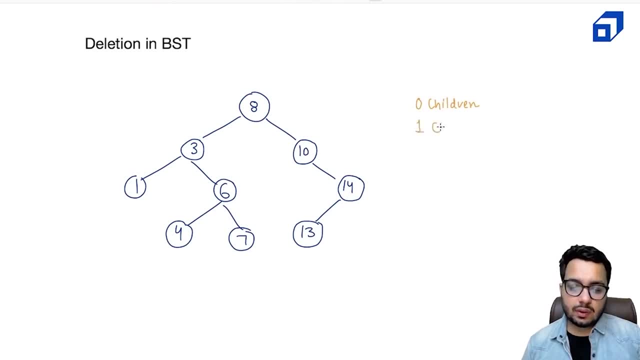 them is very easy. there are also nodes which have one child. deleting them is slightly more difficult. and there are nodes which have two children. they are even more tricky to delete. okay, for example, node like eight. if i want to delete this node, then how would my tree structure would look like? so we have to discuss all these scenarios now. 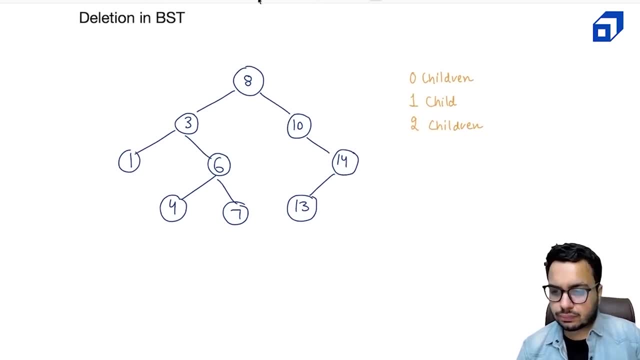 right, let us start with scenario one and let me create a copy of this tree as well, so that i can use it right now. suppose i want to delete a node like four, or i want to delete seven, or i want to delete 13.. so deleting it is very easy. so suppose let's say i: 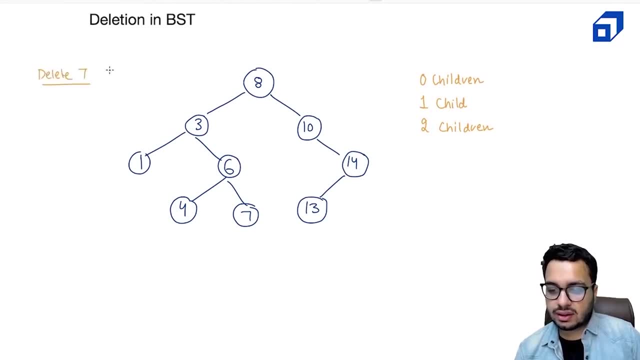 want to delete seven, right. so that is my case one, case number one. so in that case, what i need to do? first i need to search for seven. where is this seven located? right. so i need to reach that node. so i start from it. i say, okay, seven must be on the left. so i go to three. 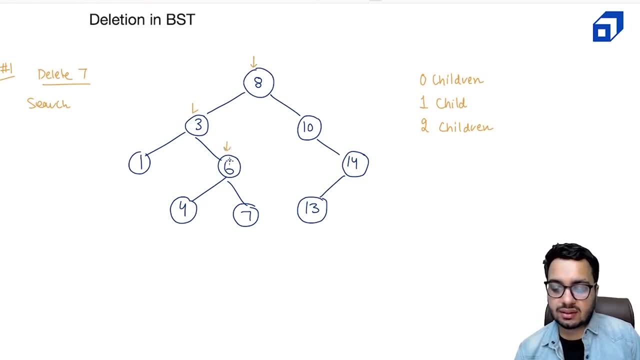 so three says seven must be on the right. so i go here now. six is seven must be on. uh, right. so i go here right now. if i reach this node, what should i do? i would say, okay, fine, this is the node that i want to delete. i will somehow delete this node and i will return a. 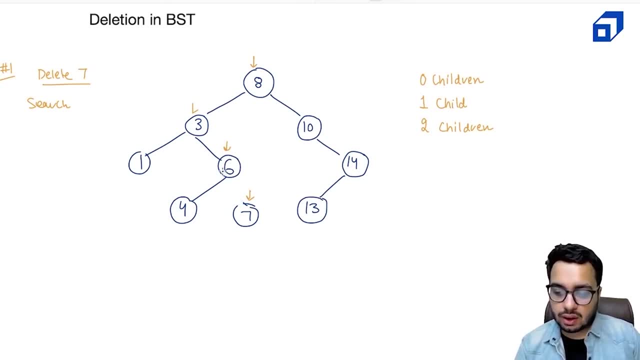 value null to the parent. so basically what i will do: in every call i will try to change the tree, i will say okay, in the right of six i will attach a null value and this node is now referenced by no one. so that means this will be automatically garbage collected. okay, so garbage collector will. 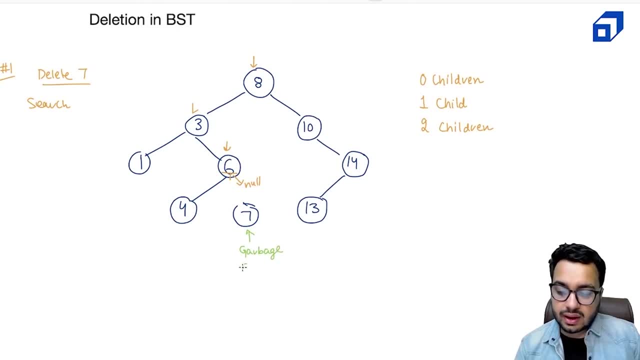 come and it will get garbage collected because no one is referring to this node. okay, so garbage collection mechanism will clear out the memory occupied with by this node. so what, what i need to do is i need to reach this node and if this matches with the data that i'm uh finding out, i 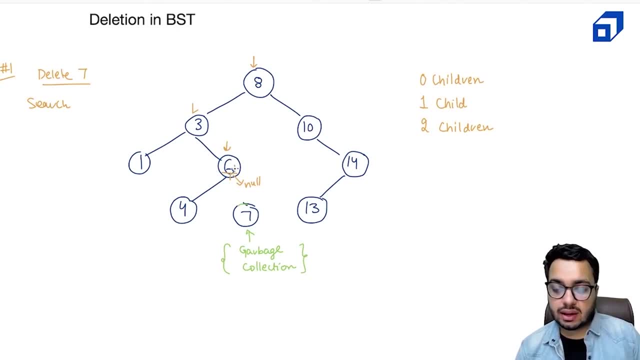 have to return delete null. okay, so when i return null value, that will get updated in the right of 6. that means, uh, the return type of the function will be of the type node. it will not be a void function. there will be a function and, as you can find root dot right, this is equal to some delete. 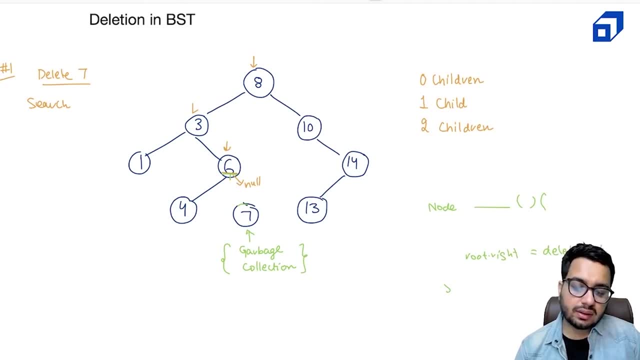 node and uh, delete node returns a null value which gets attached in the right of six. okay, so this function is delete node, something like this. i will be doing so just to give you an idea how it's going to work. so, basically, we are going to update the right reference in the parent. 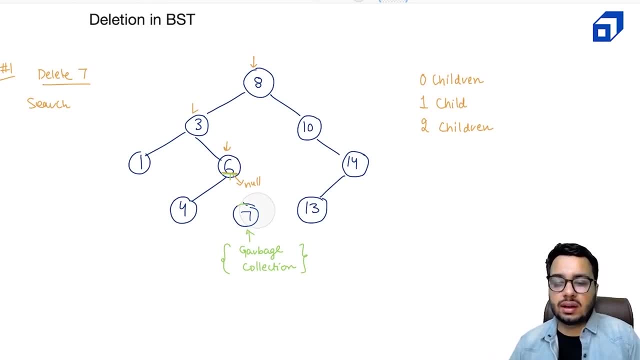 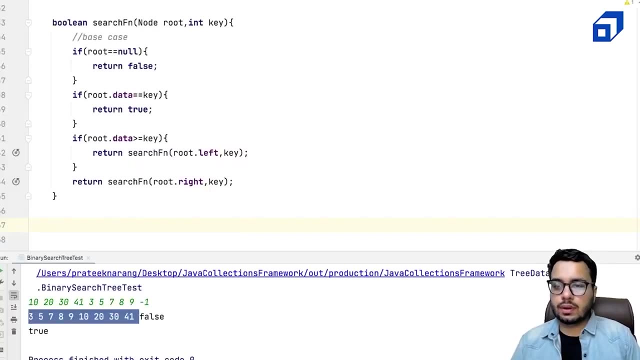 that is case number one. this is how it will be deleted. now let us write the code and see case number one, and then we will discuss case number two and case number three. so i am in the uh file called binary search tree dot java, which we have written. 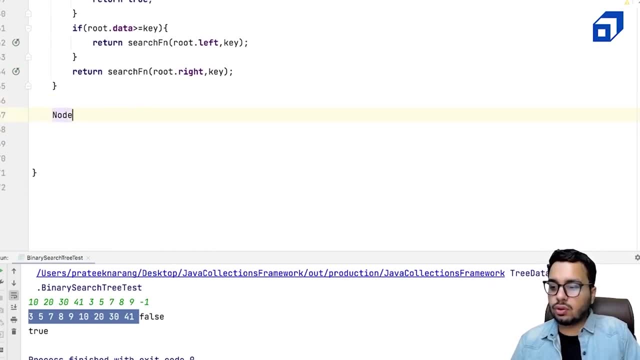 now we are going to define a method called as node remove, and here we are going to accept the current root node and the key that we want to delete. right, of course there will be some base, which we will see, okay, and there will be some recursive cases as well, right? so one thing that. 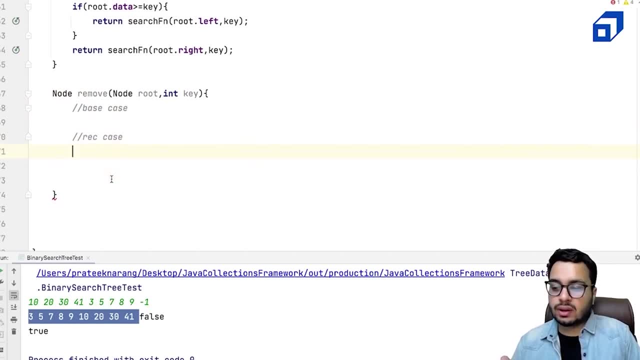 i told you that first we have to search for the node. okay now, uh, three possibilities can happen. so if you are at eight and that the node that you are deleting is also eight, then you can do work there. but if the data is lesser than eight, you have to go left. if the data is greater than 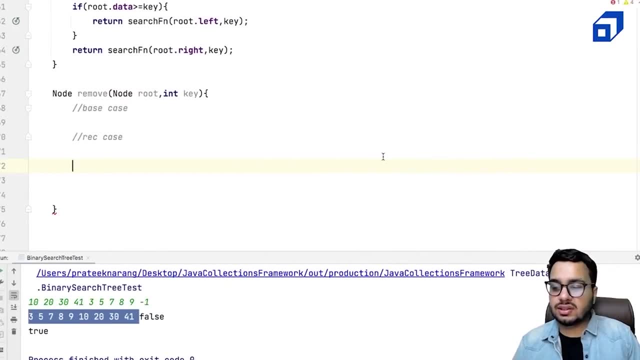 eight, then you have to go right. so first let us do the searching part. so if the key that you are that you want to remove is less than root dot data, in that case you do not need to do anything at the current root node. what you need to do is make a recursive call in the left sub tree, for example. 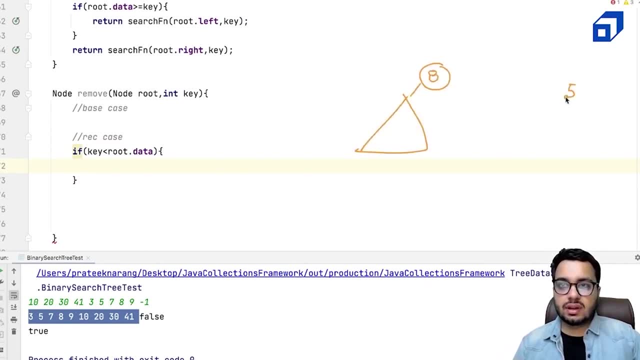 this is eight and i want to delete something which is five. a five is not present here, so what i will say? okay, i'll say: go and remove five from the left sub tree. the remove function will go and remove five from the left sub tree. so you say root dot left and key. go and go into this. 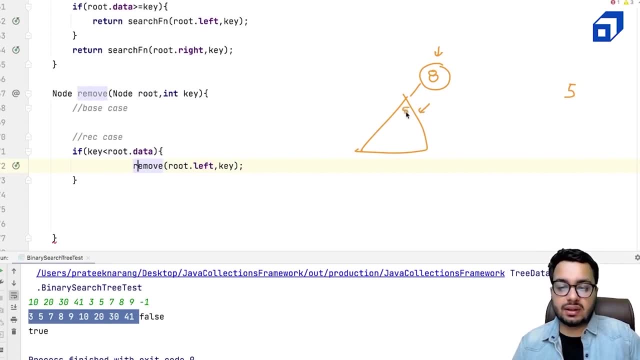 tree and remove it. now, it is possible five might be present here, or five might be present here, or five might be present, and we do not know right. so, whatever it is, uh, after removing five, whatever is the new root of the tree, that will be given back to me. so i will say, okay, eight dot left, if this. 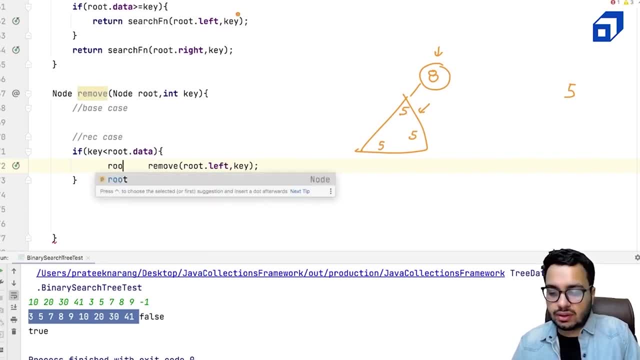 is equal to remove. so i can say root dot left should be updated by the reference of the new left sub tree that i i'm going to get now. it is possible that here the node was 6 and nothing changed. still, I will get the address of 6 back here, right, so that. 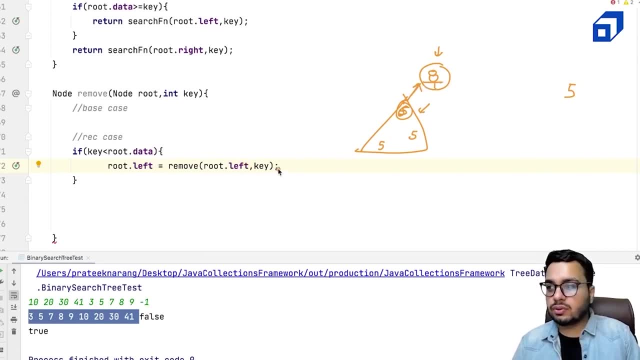 is something we have to do. the root dot left. this is equal to remove. so I make a call in the left sub tree to remove it. so this is a recursive case. right else it is also possible that key is greater than root data. that means I have to do the same thing but in the right sub tree, for example. 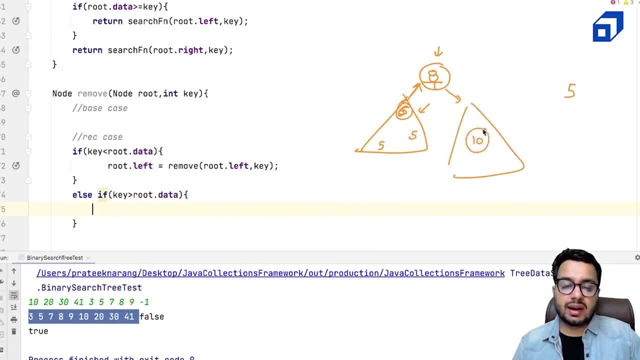 I want to remove 10, I can say, okay, go and remove 10 from the right sub tree and whatever is the new tree, give the reference back to me. I can say: root dot- right, this is equal to remove root dot right comma key right. else that means this is the node where I have to do the actual deletion. that 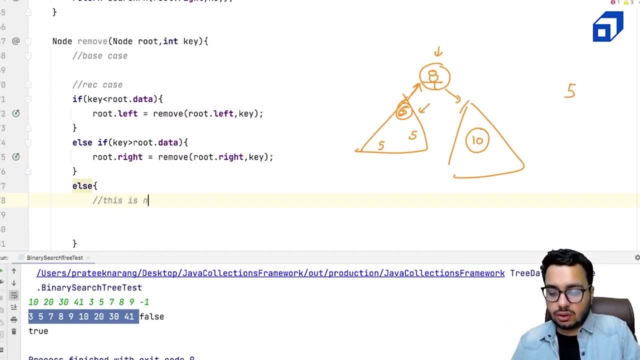 means it is the case of equality right. so this is the node to be deleted. now I said there can be three cases. case number one, that I have a node with no children, and that's the actual deletion of the node with no children. so that's the actual deletion of the 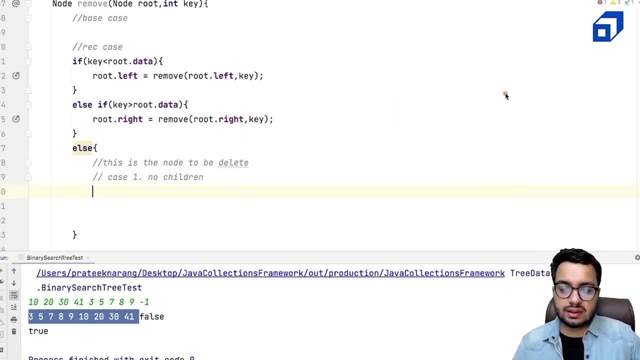 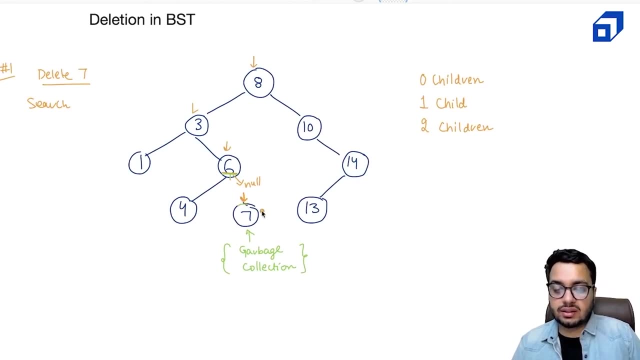 case, it is pretty easy that, for example, if you are talking about a node like this, uh, a node like seven, right, so if you have already traversed till this node and you want to delete this node, it matches seven. so what i can say? i can simply say: return null, right. i can simply say: 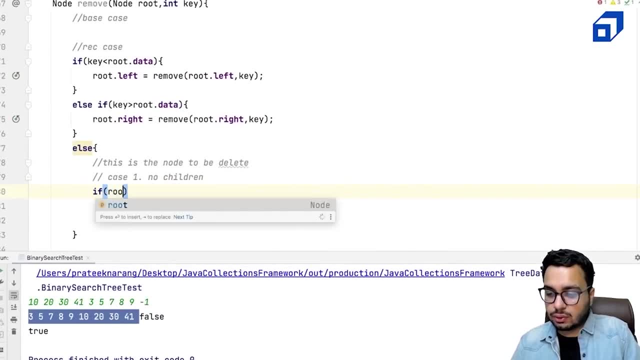 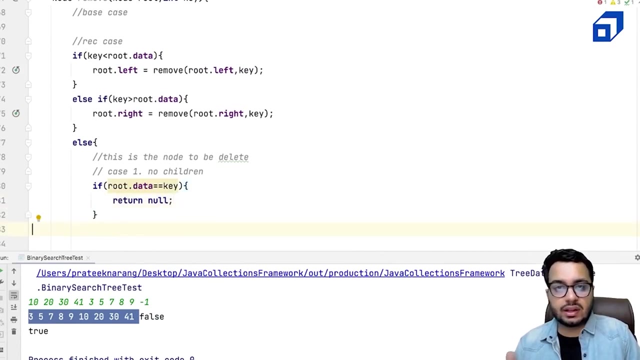 return null. so i can say if root dot data matches key, i can say return null. now this null will be attached in the uh back in the parent right. so if it was present in the left, so left value of the parent will become null. for example, six and seven right. so six made a call on the right. that okay. 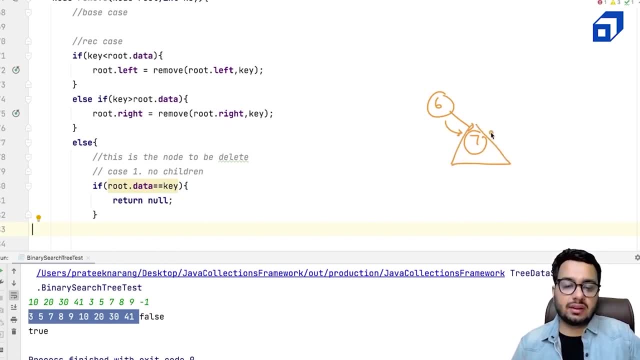 delete, uh, the seven node from this subtree. now, seven is equal to seven. so i'm saying: return null, right, this null is returned. and root dot right called the remove function, which returned null. so this remove function returned. eventually, what will happen? the right of six will start referring to null and from six we will. 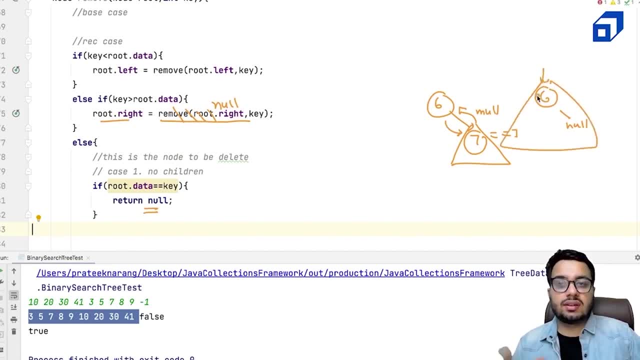 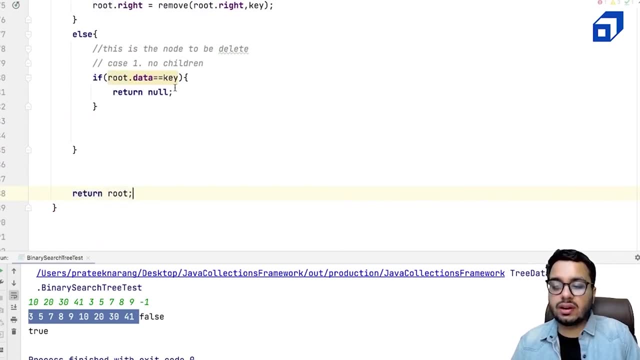 return the address of this subtree, which is nothing but this node itself, right? so finally, what? what we have to return? we have to return root also, right, like if we are not returning null, that means, if we are returning from some other node, we have to return the same root. that. 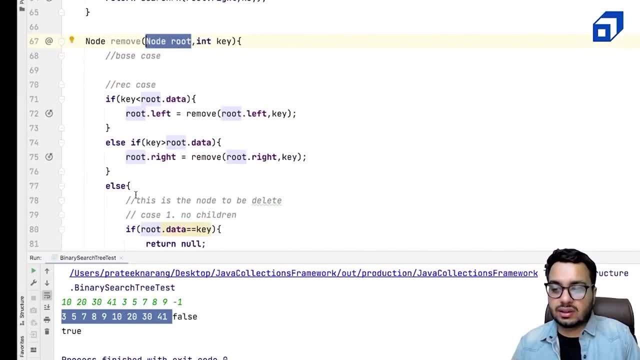 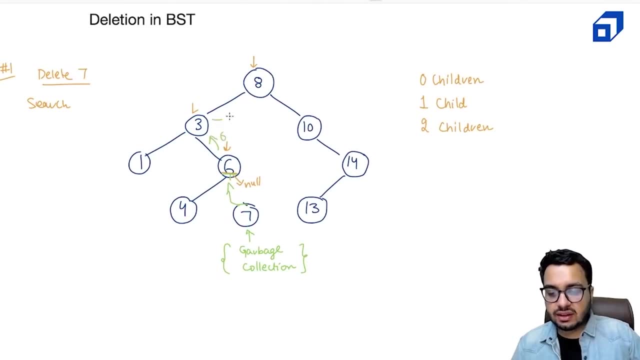 we were getting as input. so six will return its address. so seven returns are null. okay, which gets attached here. six returns six. three returns three. eight returns eight. okay, this is how it's going to happen. so we have discussed the case with zero children. now let us discuss the case. 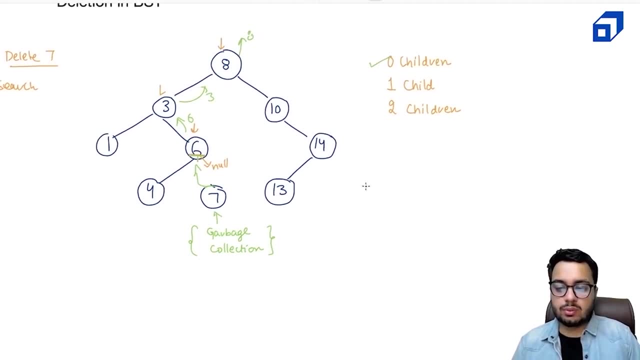 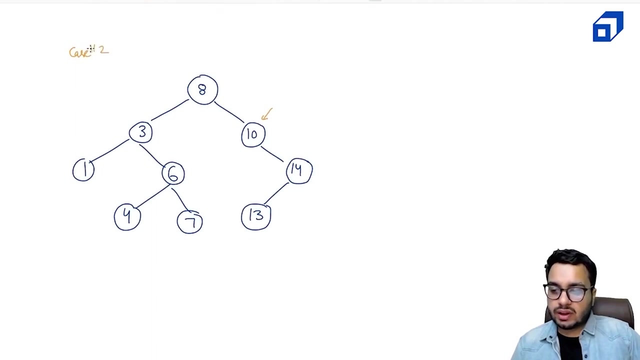 when we have one child right now. suppose i want to remove 10 right now. look at, look at this, i want to remove 10.. so let me draw this diagram again. right, i want to remove 10 right now. this is case number two, where i have one child right now. if you look carefully, if i want to remove 10, what should i do? 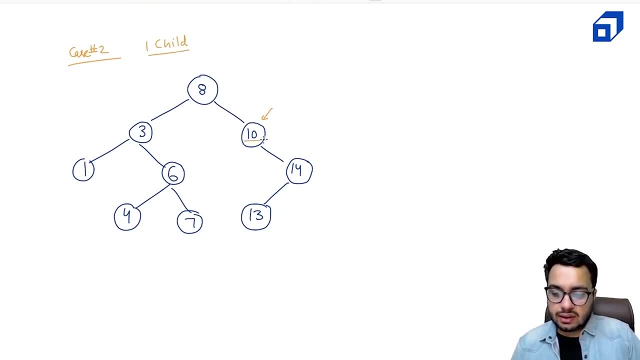 right. so that simply means that it is a node which has either a left child or it has a right child, right? if i want to remove 10, can i simply say that whatever is the left subtree or the right subtree of 10, this will get connected directly here and then will be removed. so if i simply say: remove 10, 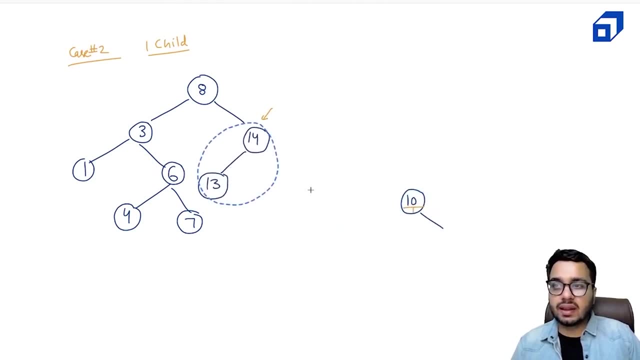 and this child will be connected here. is it correct? is it a bst? the answer is yes. for 8, 14 is greater and for 13 is less than 14. so it is correctly placed. okay, what i'm trying to say is, if you have 10 and if you want to remove 10, right. 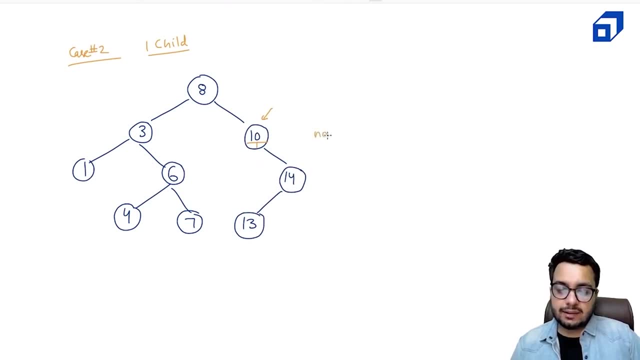 so you have to actually return the non-null child of 10 back to 8.. what is the non-null child? so this is the right subtree, right? if you want to remove this node, you have to return the reference of this right subtree back to it. so 8 will point to 14 and the remaining subtree will get attached. 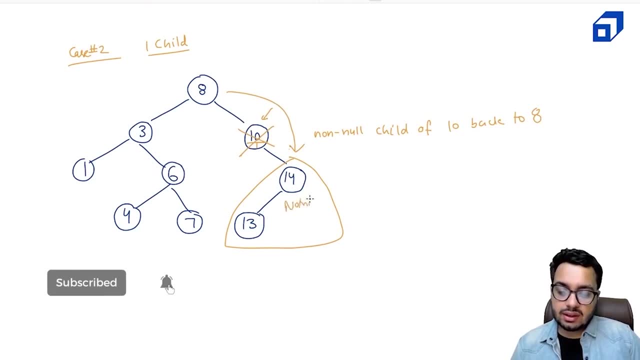 as it is. so nothing changes in the subtree. nothing changes in the subtree, right? okay, this is the point that i'm trying to make, right? so how do you reach 10 by the search mechanism that we have already written? right? i want to delete 10, so 10 is greater. so i will come here now at this node. 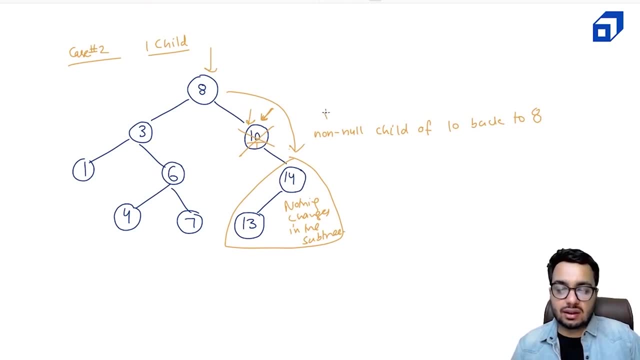 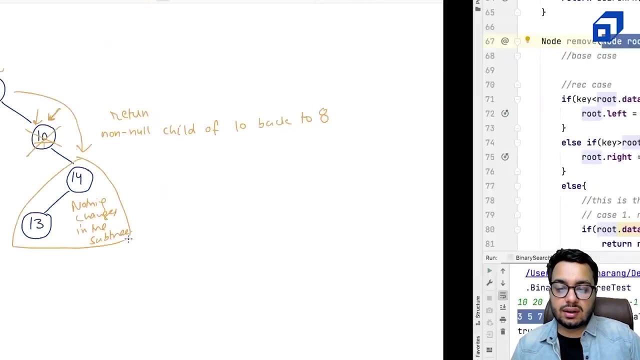 10 is equal to 10. what should i do? i will return the non-null child of 10 back to the parent. this is what i have to do. now let us see how we can write it in the form of code. all right, okay, so i. 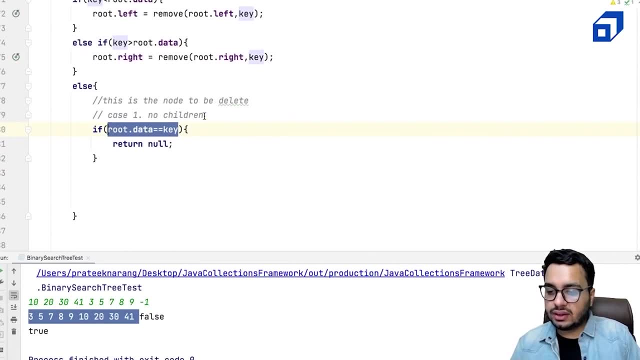 think i have made a small mistake. this is a node to delete, so of course the data will be equal because we are in the else case, but case 1 was no children, okay, so i need to fix this case. so the condition would be: both left and right of that node are null, okay, so i'm fixing a small mistake. 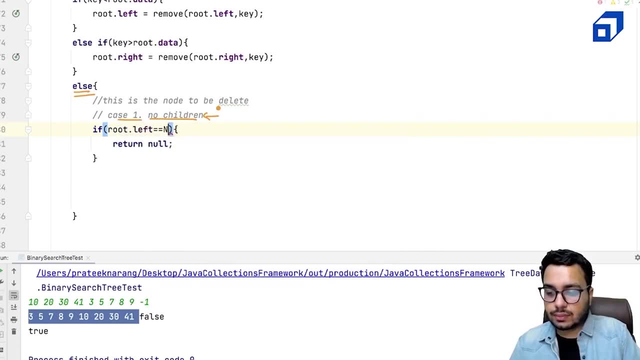 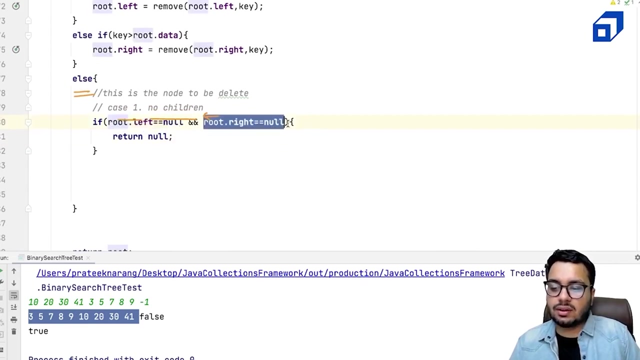 here root dot left is null and root dot right is also null. null would be capital, a small small, so i can return null right. so root dot left is null and root dot right is also null. that means, if it is a leaf node, okay. now let's talk about case two. that means exactly one of 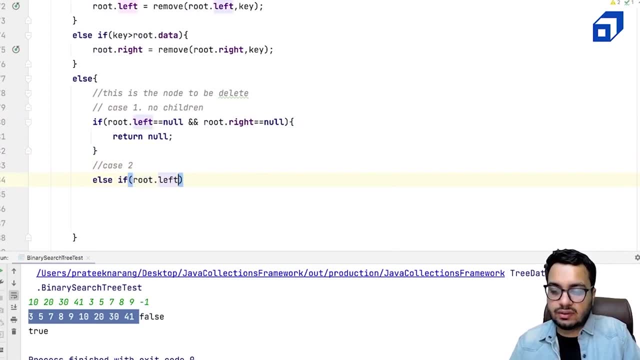 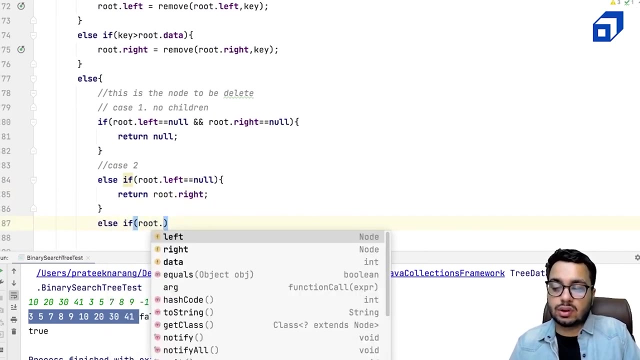 the child is not null. so else if root dot left is null, that means the left child is null and the right child is not null. in that case can i say i will return root dot right back to the parent. else, if it is the other way around, if root 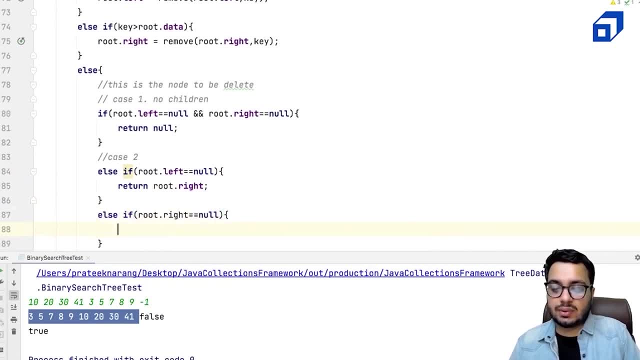 dot right is null, that means the right subtree does not exist. so we are at a node where the right subtree is null but the left subtree is existing and i want to delete this node. so what i need to do, i need to return the address of the left subtree back to the parent so i can say: return. 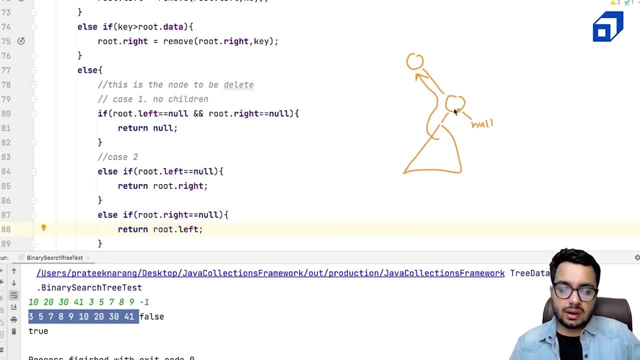 root dot left. now what's going to happen? this will get attached here, but do you really think that this node will be deleted? do you think this node will be deleted? the answer is yes. why? because who was storing the address of this node? the address was being stored. 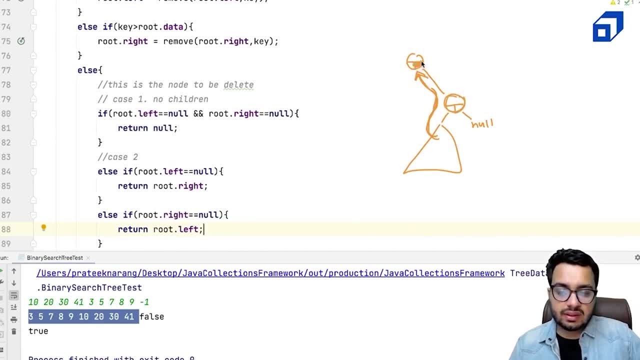 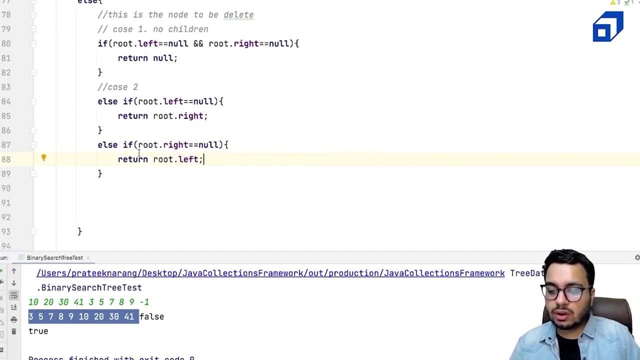 here. if this is updated, if this is updated, if the right of this root node is updated, then no one is referring to this node. that means, in a way, this object becomes eligible for garbage collection. so this will get deleted, right? so this is what we need to do now. we have a third. 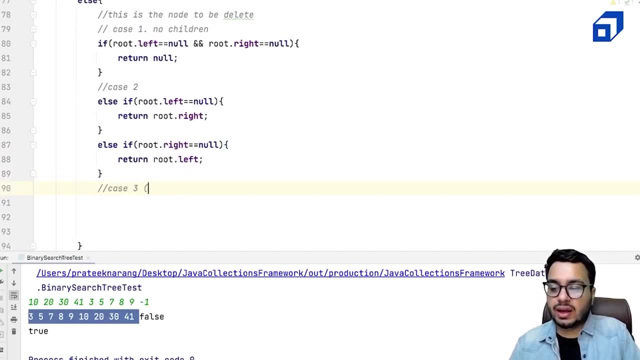 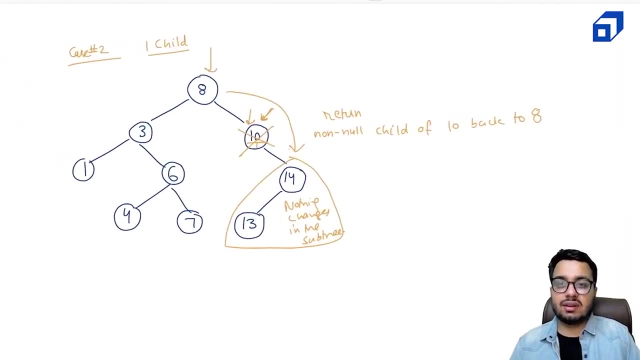 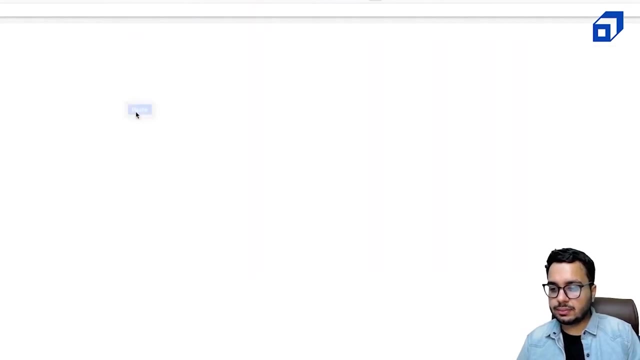 which is case three. that means a node has two children. we need to delete a node with two children. so let us discuss how this case three will work. let us discuss case number three. this is the tree, and suppose i want to delete a node which has two children. so it can be any node which has two children. so let's say i want to delete it right now, if i 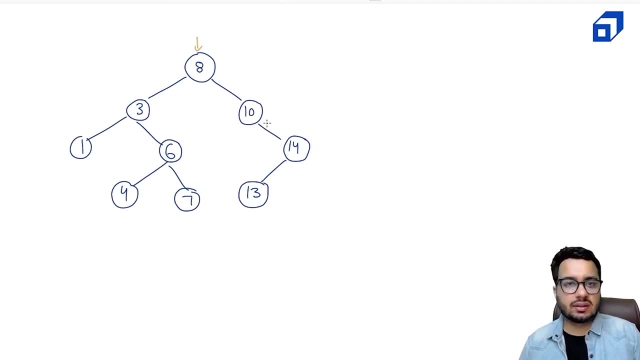 directly delete it. this tree will be split into two parts, which i don't want. this tree should remain same, right, this tree should remain same. so what i can do is i need a way so that i do not disturb the tree structure a lot. right, if i talk about in order to reversal of this tree, i get 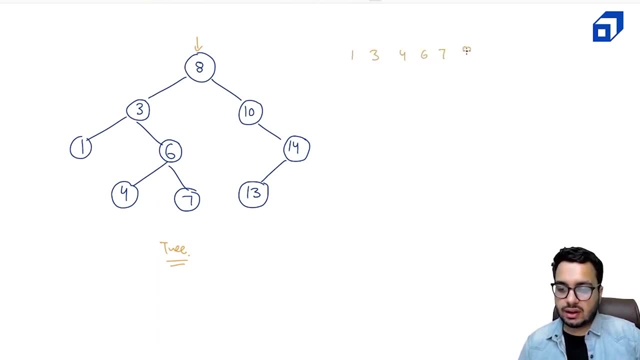 one, three, four, six, seven, eight, ten, uh, 13 and 14, right. so this is what i get, right. if i want to delete eight, the new root node should be either seven, okay, or it should be either 10.. so one of them should become the replacement of. 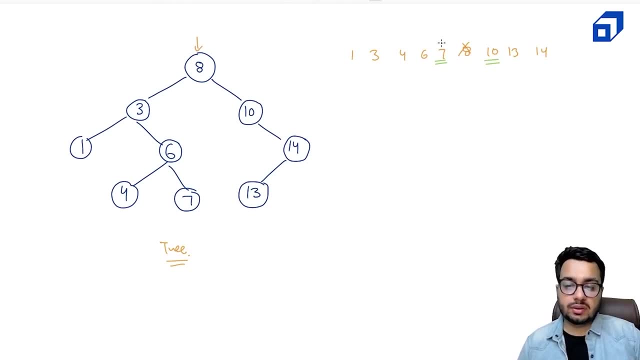 this node right now how i am going to do it so it can be the largest node in the left subtree. that is option number one. right option one is make the largest in the left subtree as the root node. right option number two is make the smallest in the right subtree. 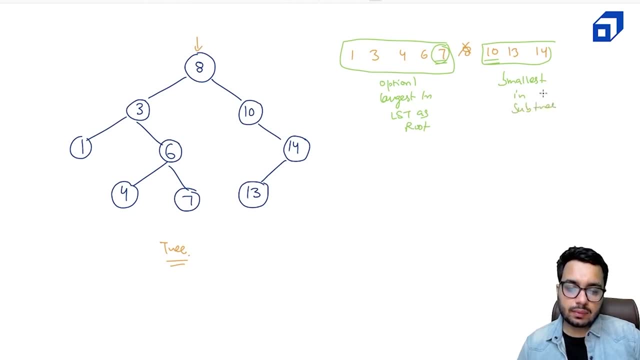 as the root node in the right subtree as the root, so you can use any of these options. okay, so if i show you, if i make smallest in the largest in the left subtree as the root node, in that case seven will become the root node. okay, now how it is done. let us see now. suppose you have reached the. 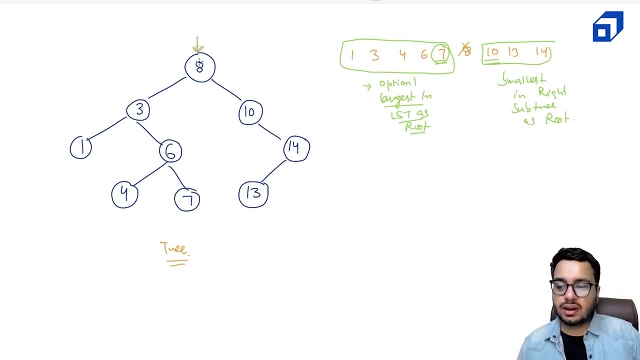 root node, the node which you want to delete, and it has two children, right, so you will. okay, i'm going to find out the largest node in the left subtree. so how do you find the largest node in the left subtree? you start from this node and you try to keep on going right. you always go right. 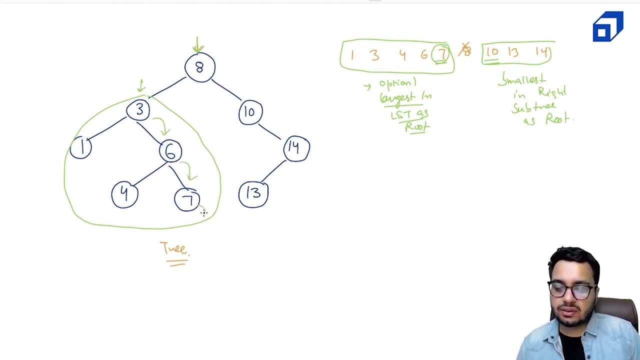 and eventually, when you stop here, because the right of this node is null, so you, you have to stop at this node and you will have to say, okay, this is the largest node and i will put this node here right now. putting means i will copy the data. so you will copy the data 7 here, so this data is copied. 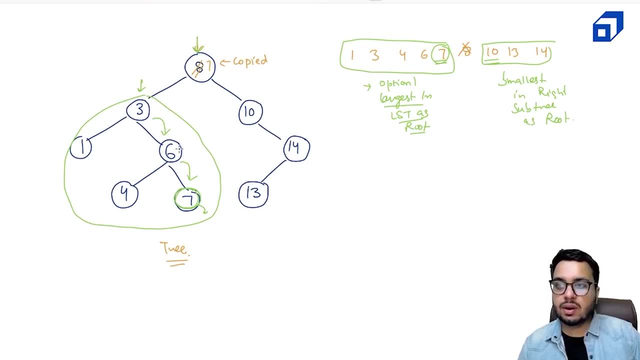 i'm not changing the node structure, i'm just copying the data. so 7 is copied here right now. if you copy 7 here, what you will observe? you will observe this: 7 is duplicate, right. this is present two times. this is duplicate right now. what i can do is: can i make a recursive call to remove? 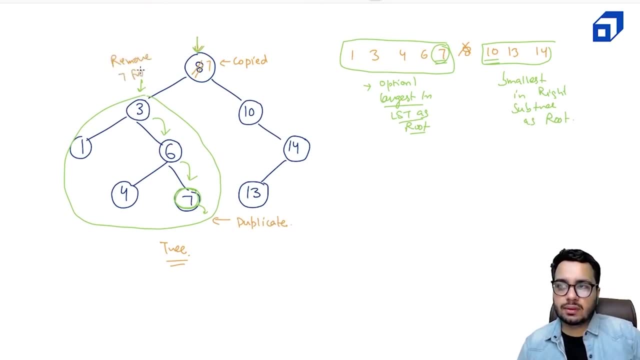 7 from this subtree, from this particular subtree? can, can it be done? the answer is yes. if i remove 7 from this tree, then my work will be done right now. if you look carefully now, 7 will be a node which has either- okay, it will have- either no children, for example, in this case, or, if it is, 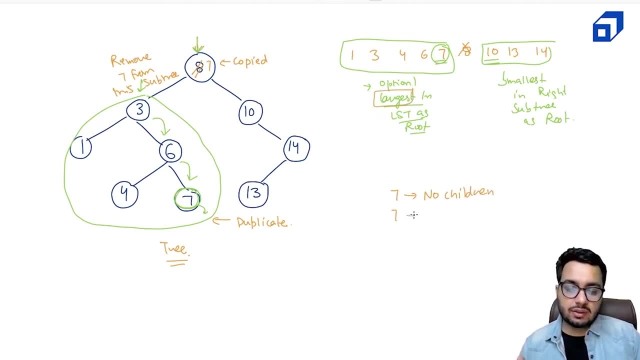 the largest node. it will not have any right child. right can have a left. child can have a left sub tree right. seven can have a left sub tree right. that means if i'm recursively removing seven from this tree two, two things can happen. seven does not have. 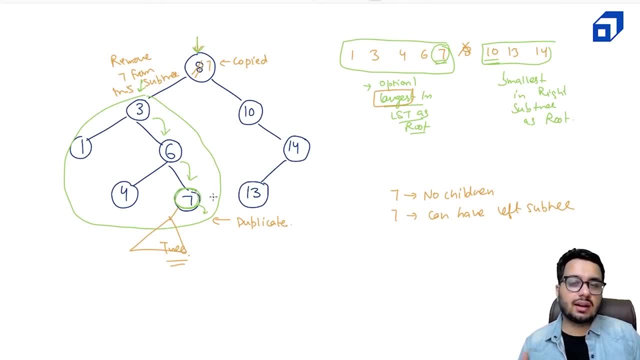 any child. so it will fall back to case number one, that a node with no children, so it can be easily removed. i can return a null here. right or seven has a left sub tree. in that case that sub tree can be returned here and it will be correct to attach it. why? because all these nodes they are 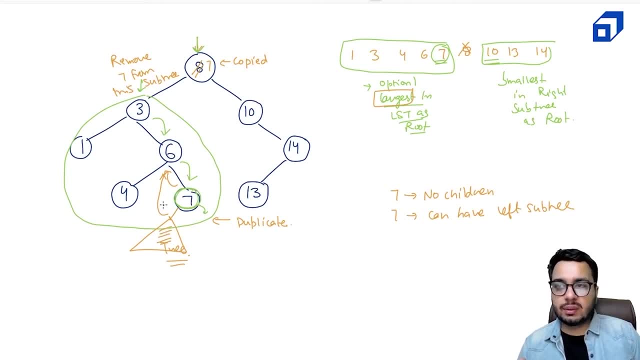 greater than six. but they are less than seven they can be attached directly in the right of six right. so seven still can be removed. so this, if this is the case, it will handled by case number one. if this is the case, it will be handled by case number two. that a node has one left child or 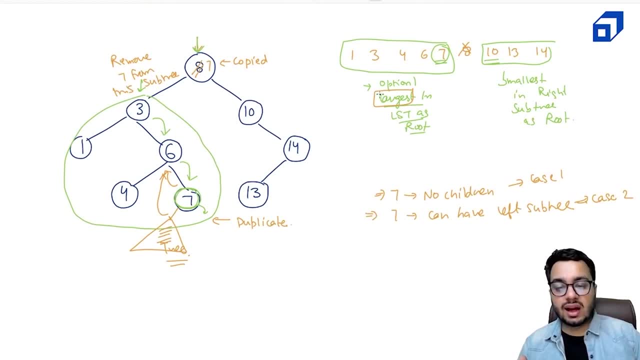 right child, right child, right child. but it cannot have both. okay. so you can see, largest node can never have a right child, okay. similarly, the smallest node can never have a left child because it is a bst it, if it is a, has a left child, then it is not the smallest right. so we are going right until we don't find anything on the 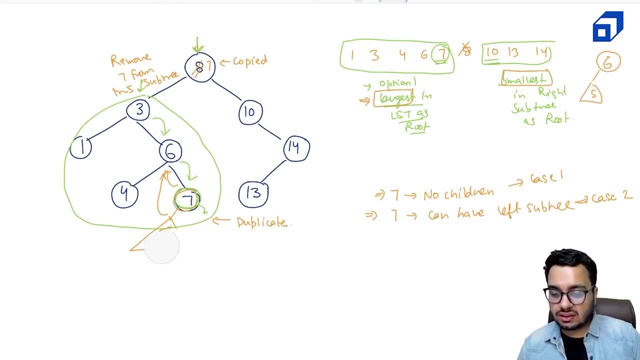 right, so seven can be replaced. okay, so that means, in this case, seven is not having any left child. i want to remove this node. i will make a recursive call on this left sub tree to remove seven, and so seven will be removed, and this is how the tree structure would look like. right? so i hope you are. 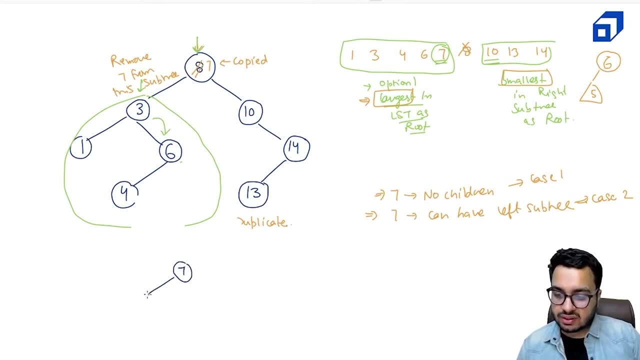 able to understand. new tree would look like this. it will be seven, three, one, six, four, and here i have 10, 14 and 13. this is how the new tree would look like. if you talk about the inordered reversal, it will be 1, 3, 4, 6, 7, 10, 13, 14. is it correct? 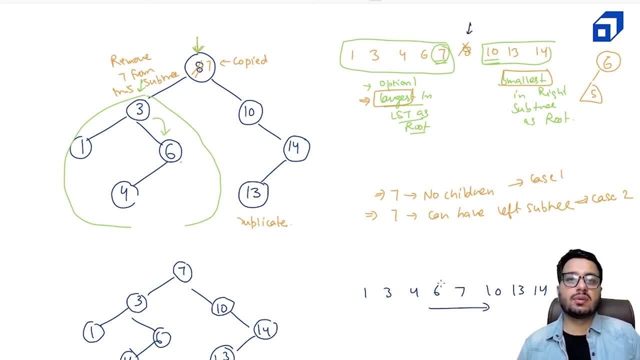 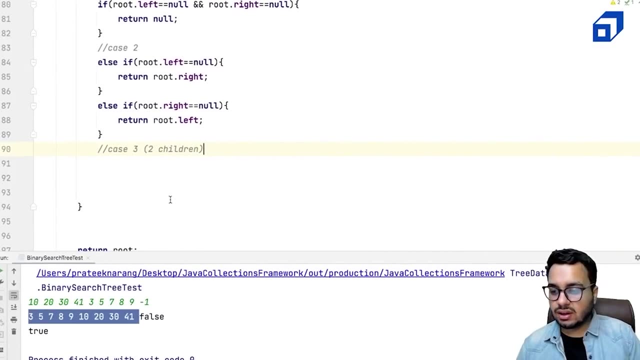 of course it is correct. is it removed? yes, it is removed from this reversal. right now let us look at in into the code how this can be actually done, right? so i have case 3 where the node has two children, so this can be handled by the else block. so what we need to do, we need to uh. 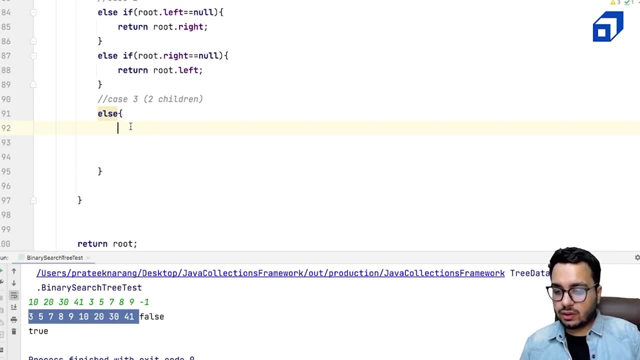 the first we need to do is we need to find the max node in the left sub tree. okay, so i can. okay, i will take a temp variable node: temp. this is equal to root dot left. so i can say: while temp dot right is not equal to null, so i will move this temp towards right. so temp equal to m dot right. so 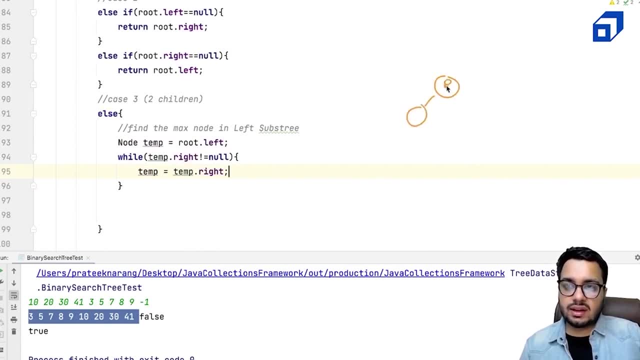 if you are confused what we are doing now. suppose this is the tree eight. let's say i have, uh, five, six, seven and i have some nodes here as well. right, i'm saying, okay, i want to find the largest in the left sub tree, so i start a temp here. so temp dot. right is not null, so temp goes. 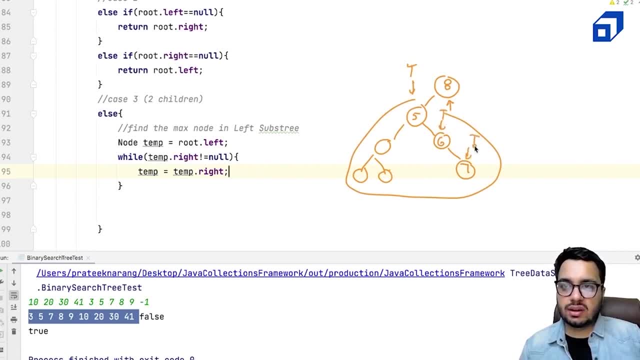 here again, temp dot right is not null. temp goes here now, temp dot right is null. so what? what do i do? i stop. so even if it has a left sub tree, temp will stop at seven right. okay, so we found out the node. now what i need to do is: i want to find the largest in the left sub tree and i want to find the 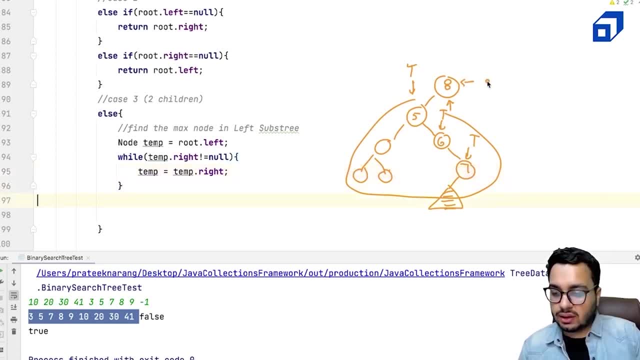 largest in the left sub tree. so i need to do: i need to replace the data here so i can say, okay, fine, root dot data will be replaced by temp dot data, the data of the temp. so i copy this seven here right now. what i need to do? i need to recursively delete the node 7 from the left. 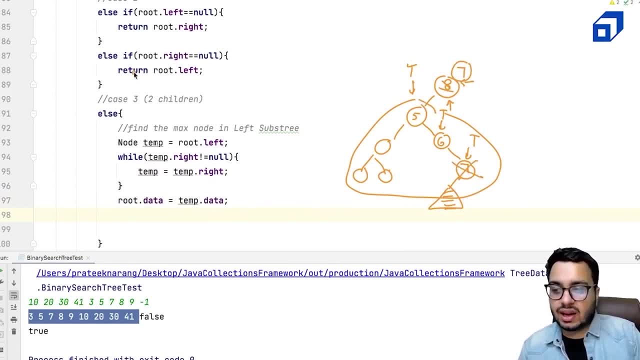 sub tree. can i call the remove function? yes, because it will either lead to case 2 or case 1, which i have handled right, so i can say: okay, fine, now my function is to remove the node with temp dot data from the left sub tree, so i can say remove. 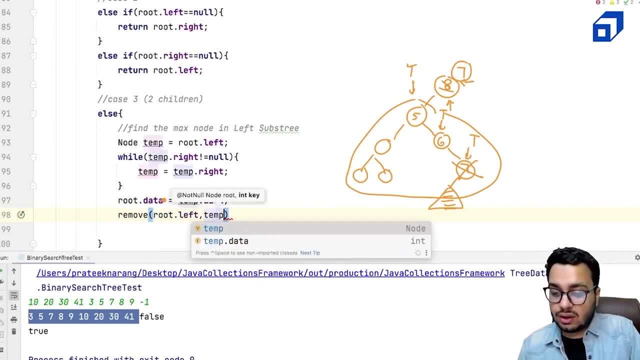 root dot left. the node is called temp dot data. i'm not. i don't want to remove 8 now, i want to remove 7 now. so that is why the value is not key, but it is temp dot data. but after removing this, something will be updated right. so i am standing here, i am making a function call on this left sub tree, so 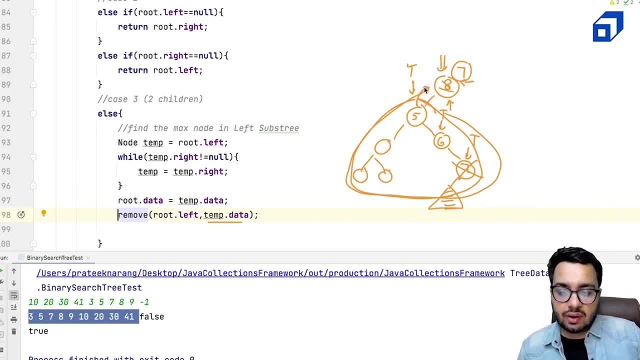 this left sub tree will tell me the updated address of the left sub tree or the updated reference. so i have to say that root dot left, this is equal to remove right. so whatever is the tree after removing, please tell me. it's a root dot left, this is equal to. 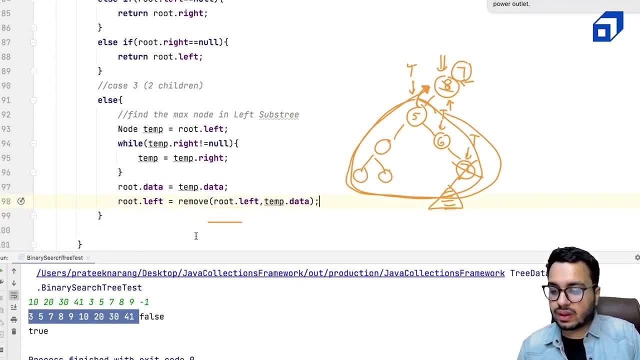 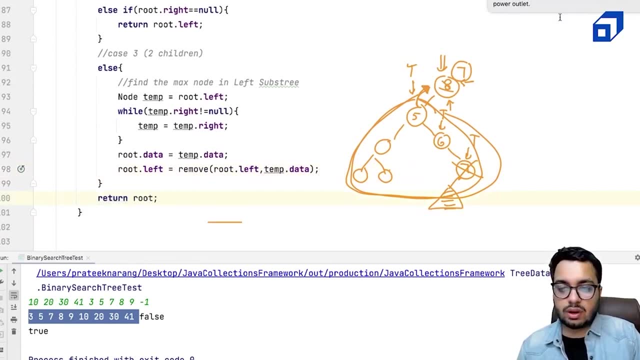 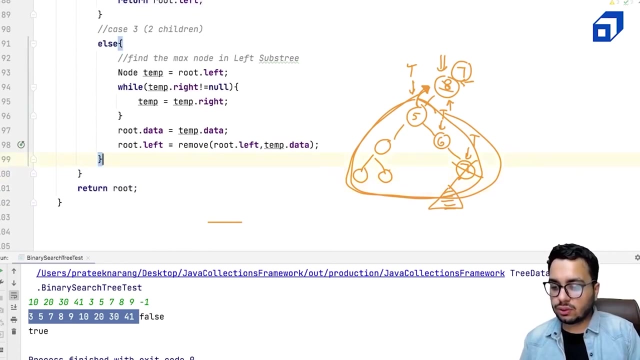 remove, right. so once it is done, what should i do? i will simply return the address of the root. so this is something we will do, right? so i'll tell you quickly what. what is happening here, right? okay, return root. we have already done at the end, so, no, no need to do it here. so we have three cases. 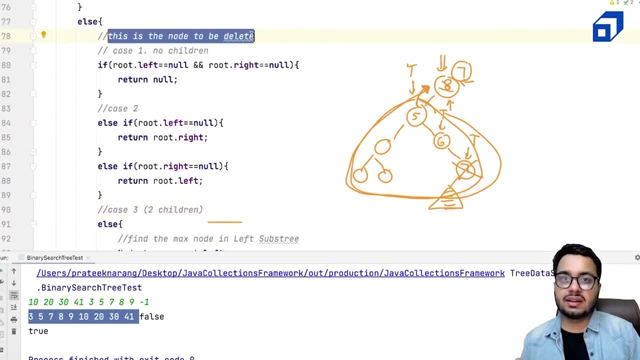 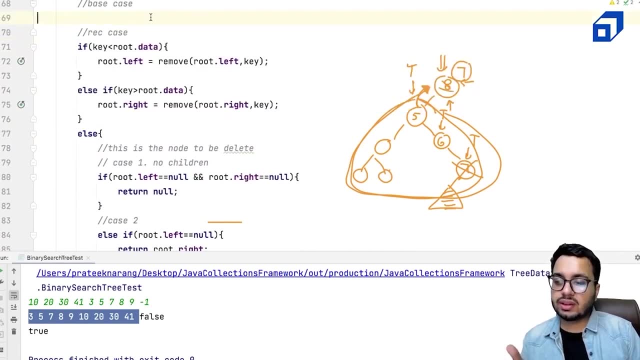 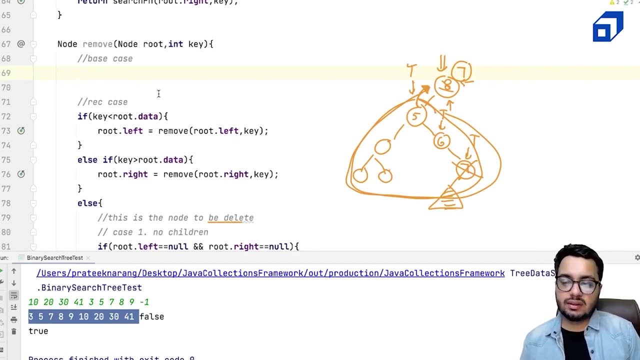 when we are at the node which is matching the given key that we need to delete. okay, we have two recursive cases which are, uh, basically helping us to reach a node. okay, so there will be a base case also. right, the base case would be that if node is not present, so if node is not present, we might end up at a value that is null. 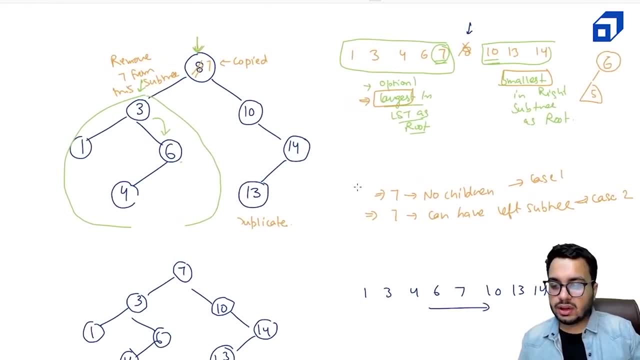 right. so i will show you what will be the base case. now suppose i want to delete uh. let's say i want to delete uh 41 right now. i start with, let's say, 7. i say, okay, 41 is greater. i go to 10. 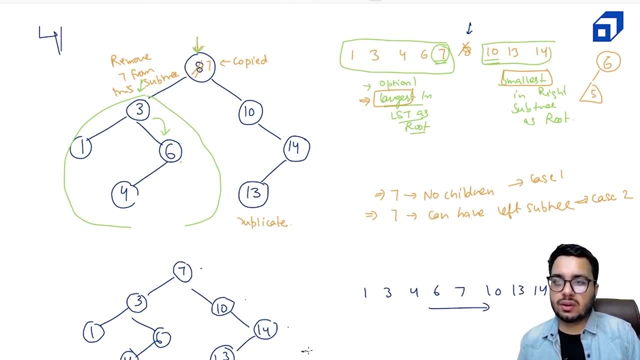 it is greater, i go to 14.. now it says it must be on the right, so i go here. so basically, the right of 14 is null. if i reach a value that is null, that means the node is not present. so it is just like the search method where we were returning false. here we will not do. 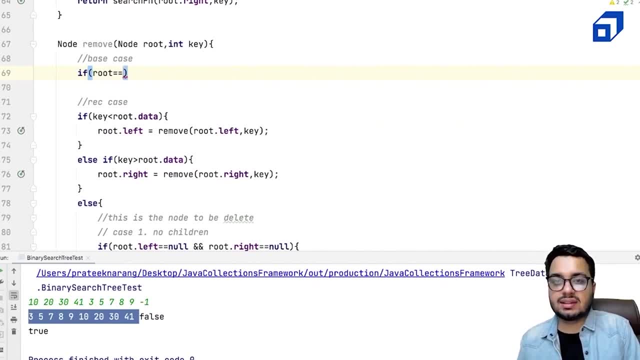 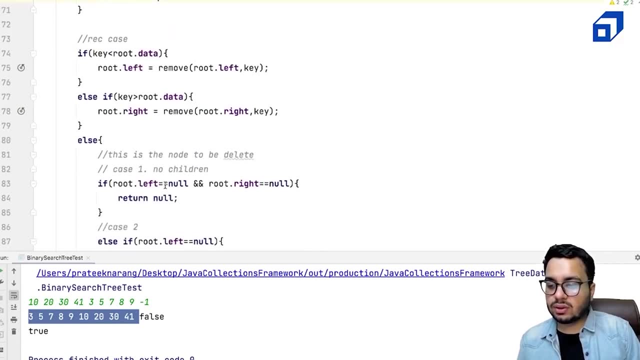 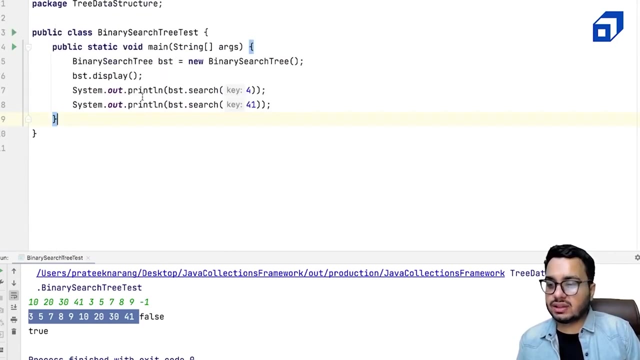 anything. so if root becomes null at a certain point, right, so i can say, okay, i'm also going to return null, right? so this, i think, makes the code complete. now let us test our functionality by going to binary search tree test file. okay, so, okay, i was all doing searching earlier. 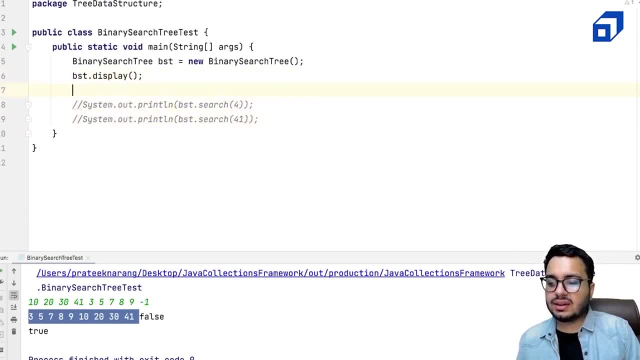 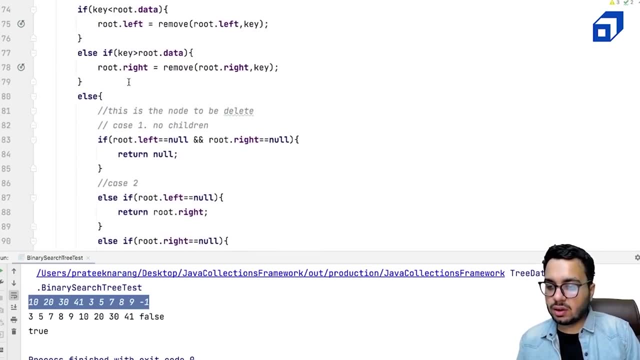 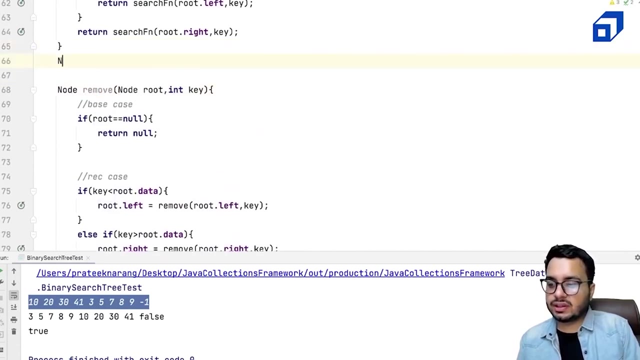 now i can say, okay, uh, i will remove something and then i will display the tree. okay. one more thing we have to do is we cannot call the remove function directly because we have to supply the value of root, so we will create a wrapper function. let's say: node, remove key. let's or let's avoid. 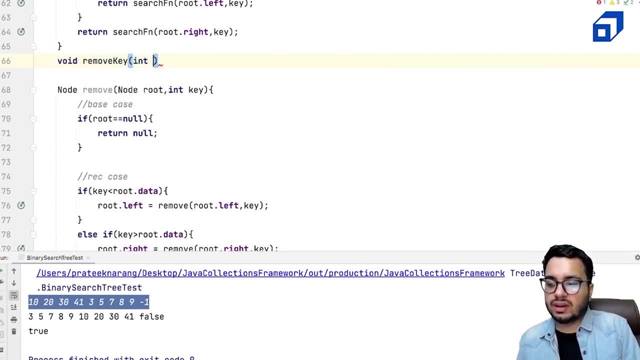 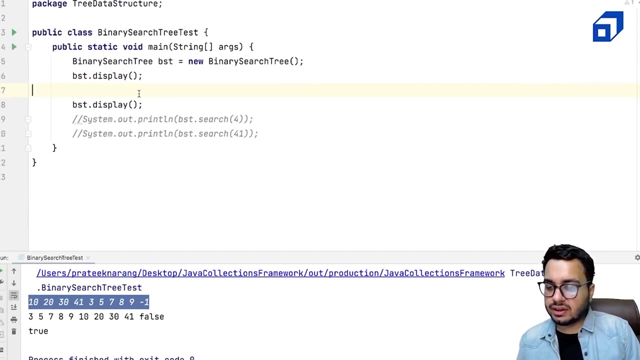 remove key. this is the method, and here we will only accept the key right and from here we will say: okay, let us call the remove function, where we will give the actual root and the key here. so now from binary search tree test we can say: okay, bst dot, remove key. and here: 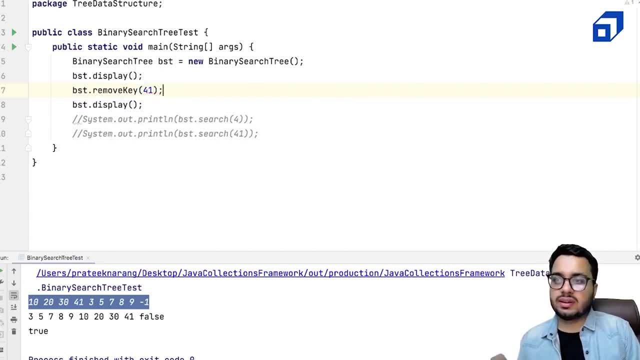 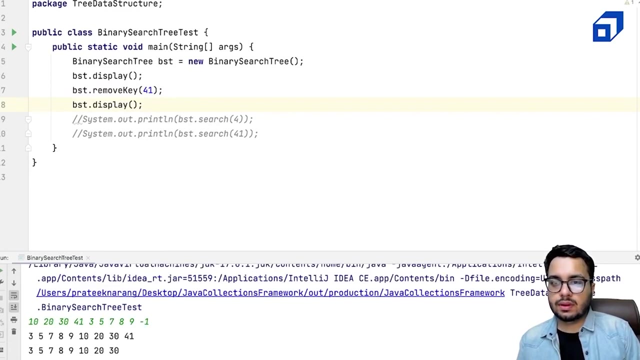 i can give some key, let's say 41. now, if this is present, it will get removed. so i will give this value. and let's say, i want to display this tree, so i have given this particular input. so this is the tree: before printing, before removing, then i 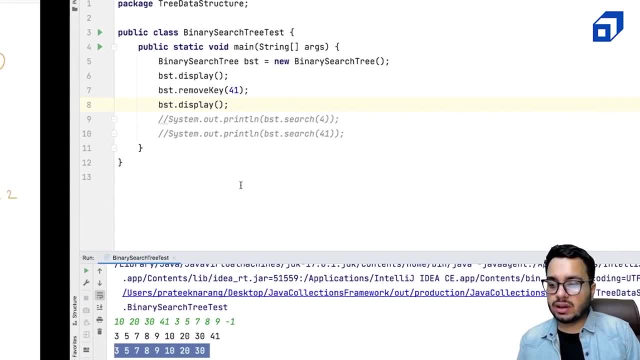 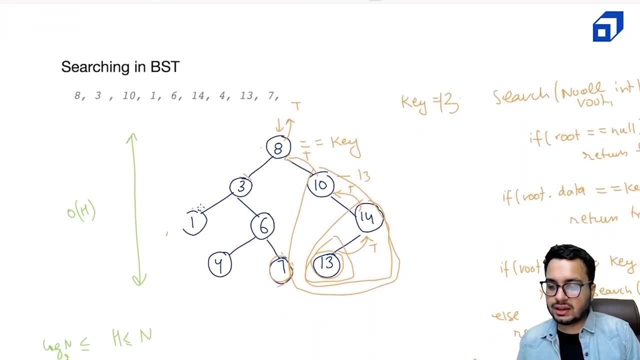 removed 41 and this is the tree. right, we can experiment with this tree as well. that we had for this tree. uh, the input was 8, 3, 10, 1, 6, 14, 4, 13 and 7.. let us try to play with this tree as well. 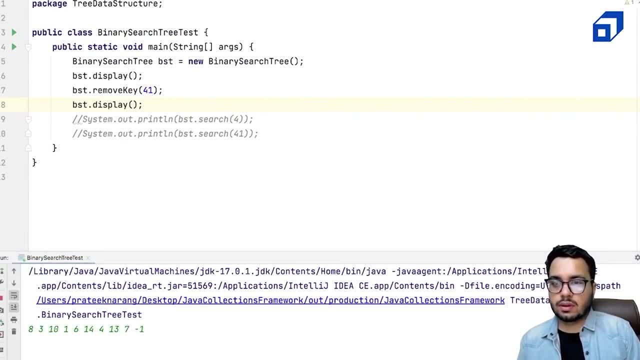 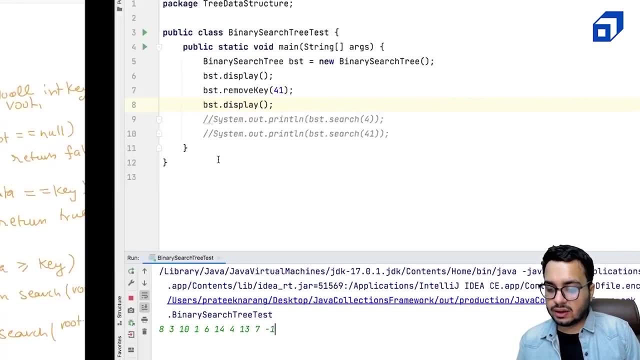 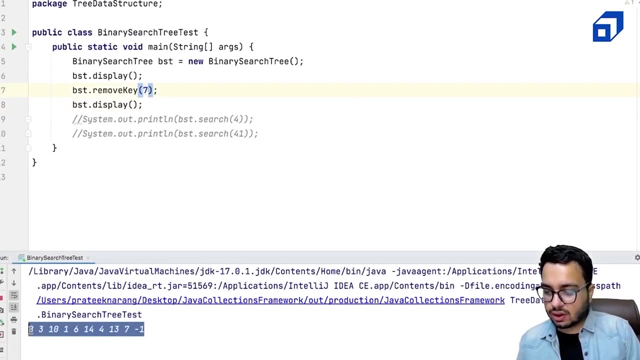 so i will quickly type the input. so this is the tree from the diagram and uh, from this tree, let's say i want to go with case one, where i want to remove, let's say, 7, i will give input as it's a 7 or i can ask the user. 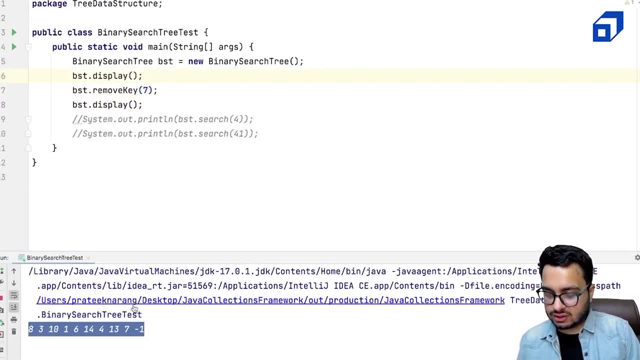 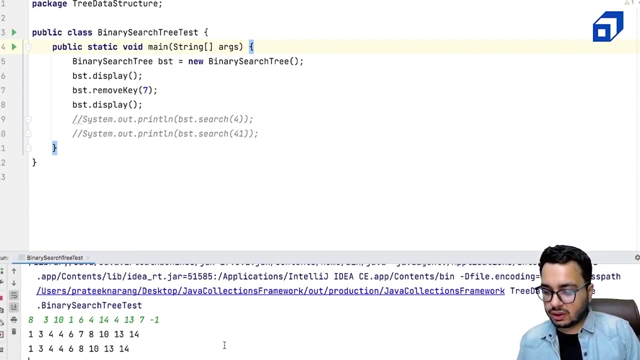 for the node to delete. okay, that that is also doable. i will just rerun this code and i want to get 7 from this tree. let's rerun it. uh, so let's say sorry, this is the wrong input we have given. all right, so this is the input we have given, and now from this input i have removed seven. 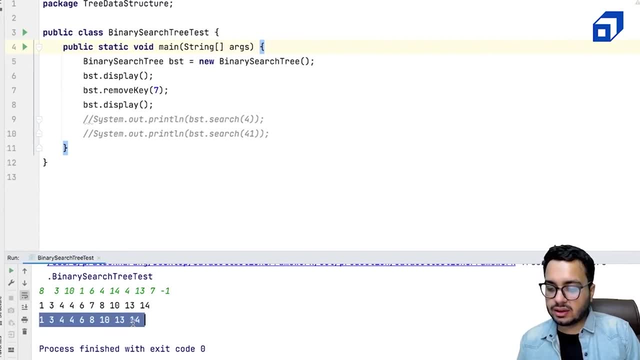 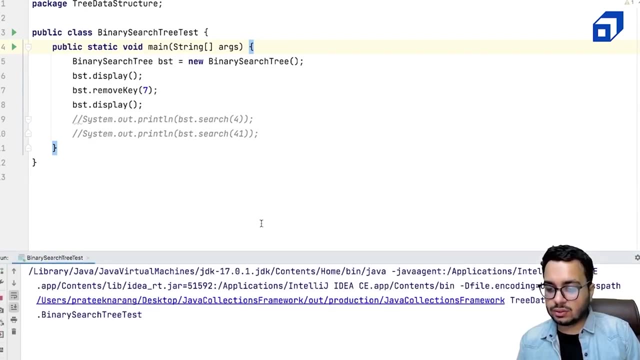 so you can see the seven has been removed from this tree, right, so that means case one is working fine. now let us rerun this once again. and let us discuss case two, where i want to remove, let's say, 10.. so the same input goes, but i have to remove 10, so i have to rerun this code once again. 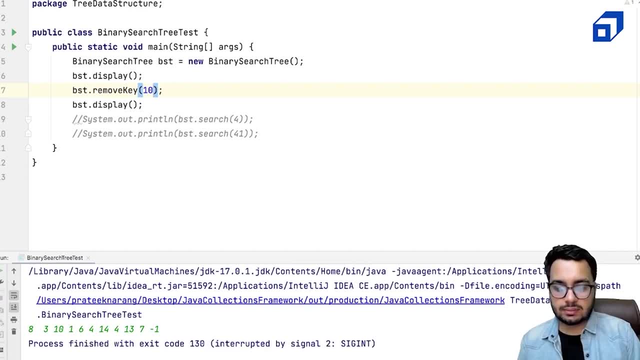 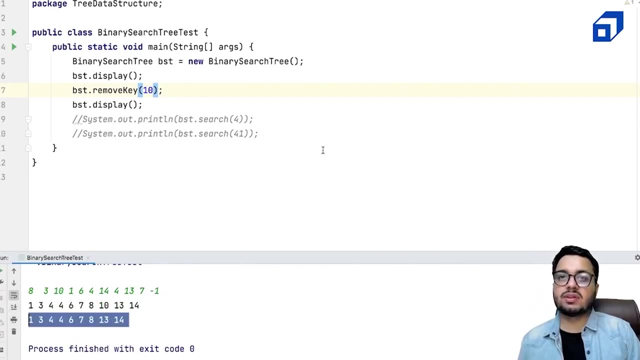 i will stop it and i will rerun it. let's say i'm removing 10.. now from this code you can see 10 has been removed. that means it is working fine for case 2 as well. case 3. let's say i want to remove it, so i want to remove 8. 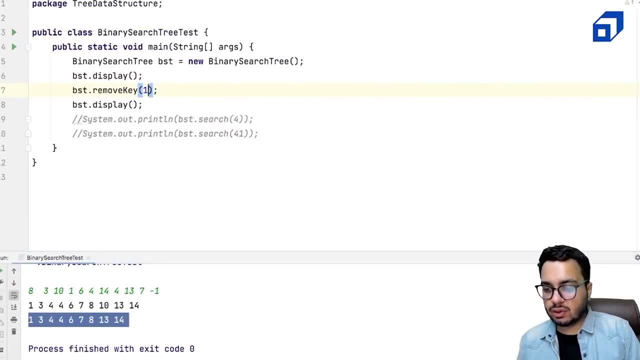 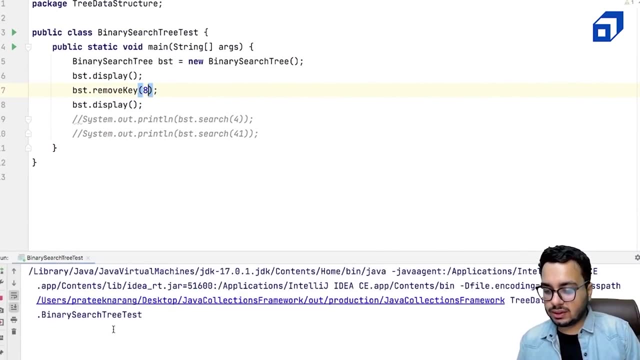 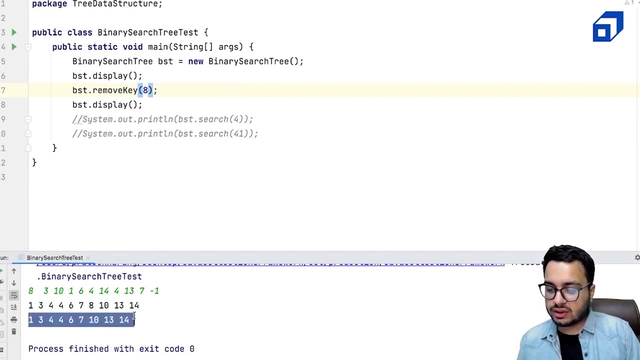 i will rerun this code and let's see now, after removing it. you can see this is the in order traversal of the tree, which looks correct. okay, so in this case i have removed 10. so i want to remove 8 and i will rerun this code. 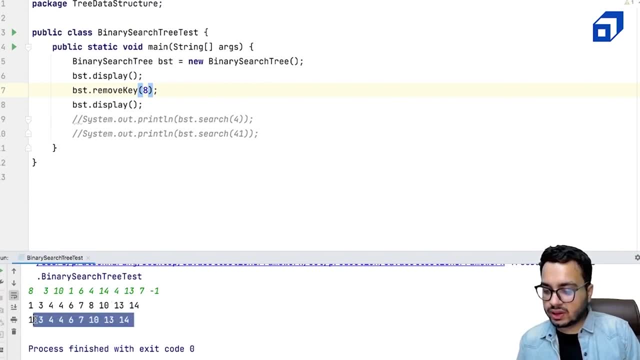 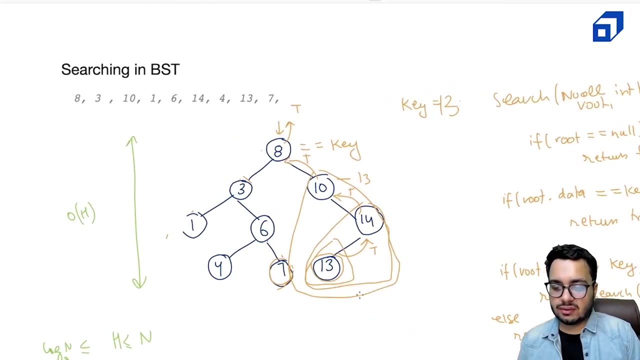 code. i have two fours, which is okay, but you can see eight is removed and eight was the root node of the tree. right, that means it is working fine for all the three cases. that's about how you remove a node from a binary search tree. okay, if you want a small dry run, we can do it once again. 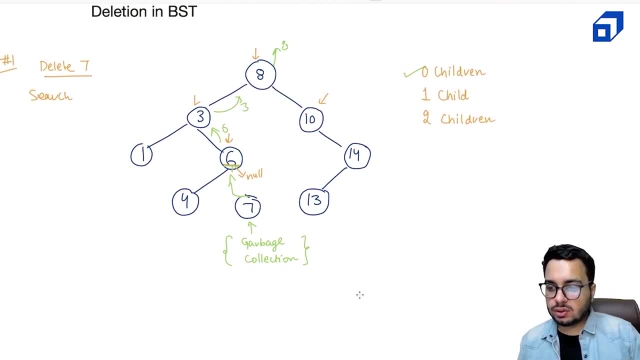 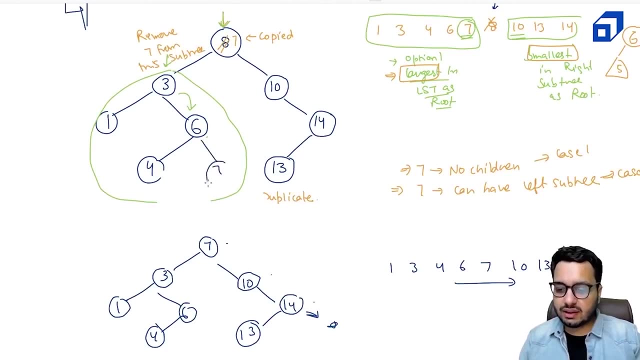 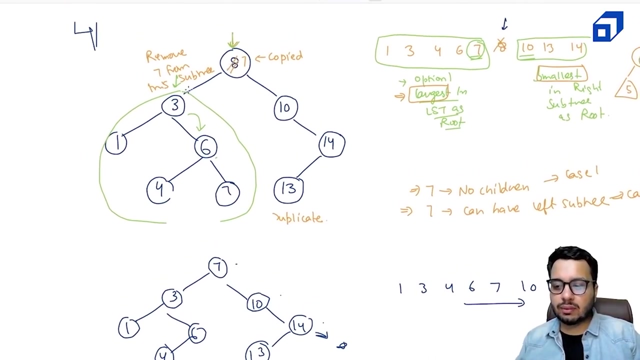 uh, let's say, now you're removing it. so, as i discussed. so what are you doing? uh, you had seven here, right? so you say, okay, i want to remove eight. so i will. i will go in my right subtree, in the left subtree, and i will try to iteratively find the largest node. 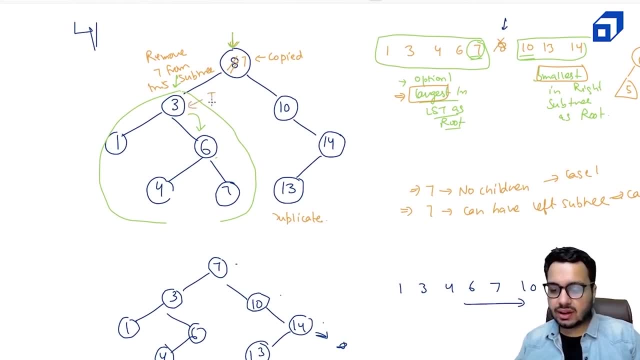 so it says: okay, this is okay, temp is here. temp goes here right, is not null, temp goes here, right. then i say root dot data. this is the current root where i want to delete. so i say root dot data, this is equal to temp dot data. so seven is copied here. then i make a recursive. 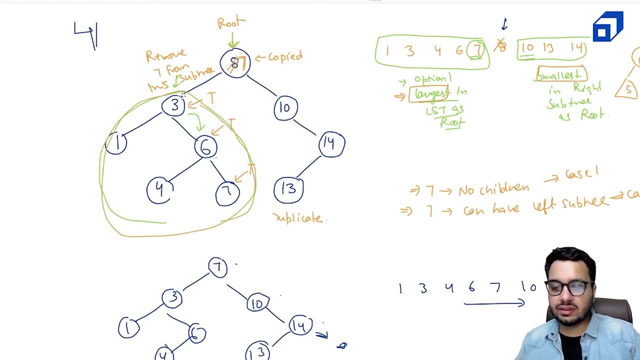 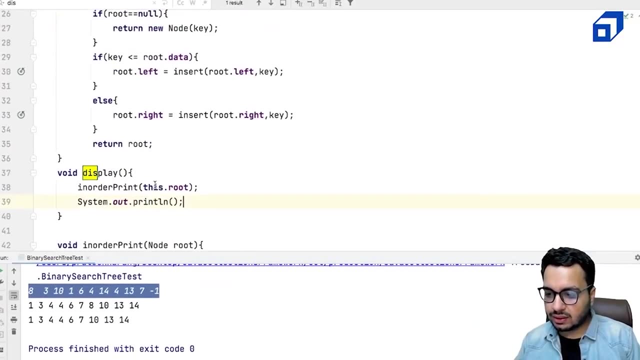 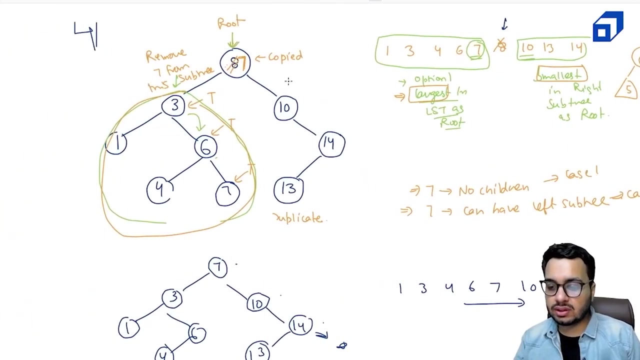 call on this is okay. root dot left. this is equal to remove. okay. uh, if i talk about in the code, i'm making this uh change here. uh, i show you. this is the remove function. so i'm saying root dot left. this is equal to remove root dot left and temp dot data. so i'm not saying remove it, i'm saying remove 7 from this tree, because 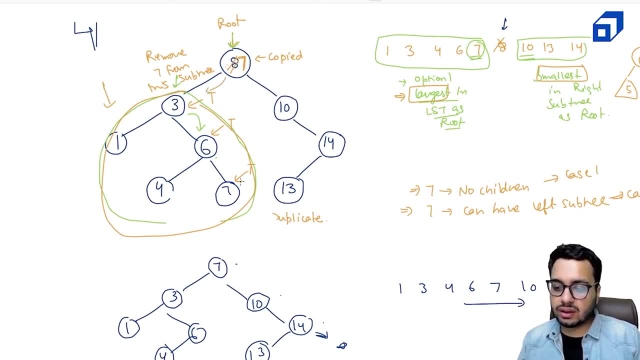 so i guess i can say: root dot left should point to a new tree in which seven is removed. so now i say seven, i want to remove seven from here. so seven is greater than three, i go here. seven is greater than six, i go here, so i reach finally seven. if i reach seven i say return null. now 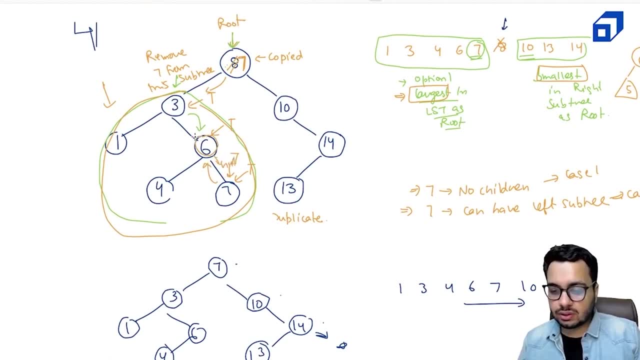 six right is pointing to null and as a return root, so six is being returned. so three refers to six. this node is gone. and from three i say return root, so seven now refers to this three. so this is what is happening when i am doing a recursive call for deleting seven from history. i hope all those who 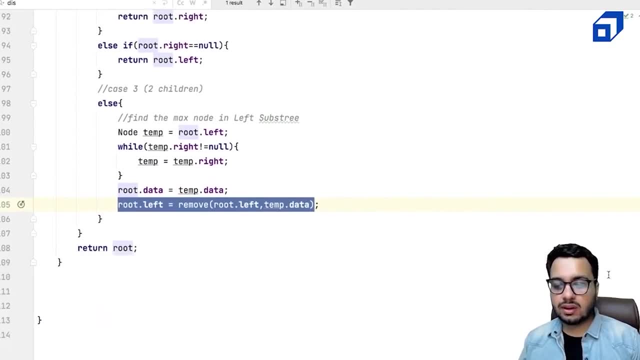 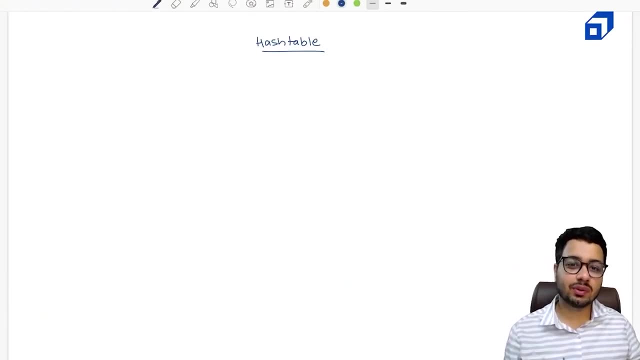 had a doubt. now it is clear, and this is how removal in bst works. let us try to understand what is a hash table and how it works. okay, so you might be already using hash table a lot of times and it is known by different names in different languages. for example, in java it is called as hash map. 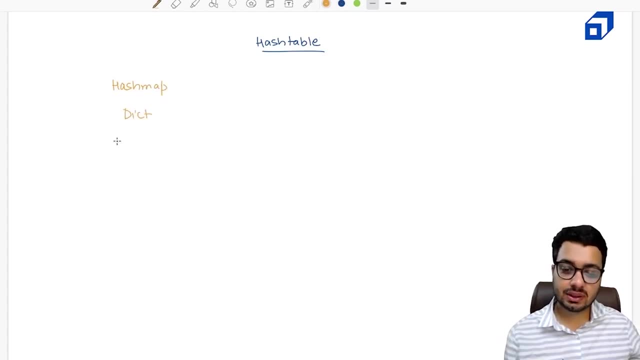 in python. it is called as dictionary in c plus. plus it is called as unordered map, right, so there are different names, but the internals of the data structure they are same in different languages. okay, so hash map in java, dictionary in python and unordered map in c plus. 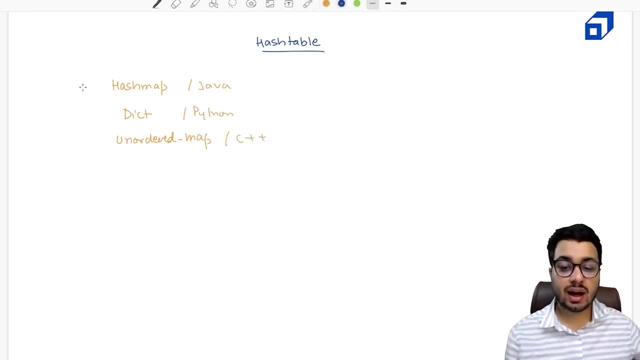 plus, and in, of course, in other languages as well. you have this data structure that is available, right? so the reason why we are going to study this data structure is it is very, very powerful, right, and it is used a lot, right. it is used a lot, right? so when i'm saying it is used a lot, 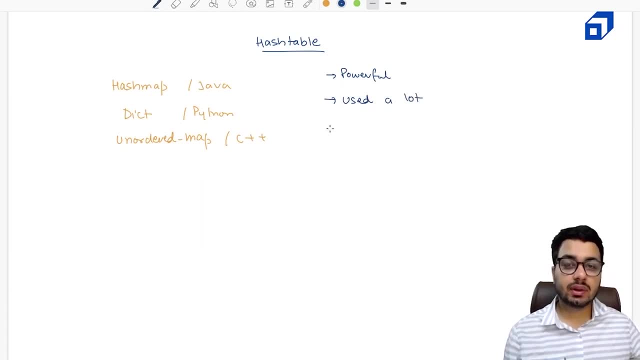 so not just business logic. so when you're dealing with your problem solving, when you're building real software, you would often require a hash map to store data in the form of key value pairs. okay, so it stores information in the form of key and the value pairs, but not just that we can. 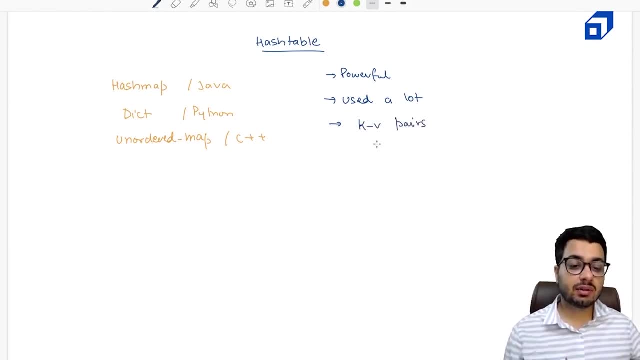 also store key value pairs in the form of a list right. why it is powerful? because it allows us to do operations like insertion: i want to insert a key value pair, i want to look up for a particular key right and maybe i want to delete a particular key right, a key value pair, so i can just give okay. 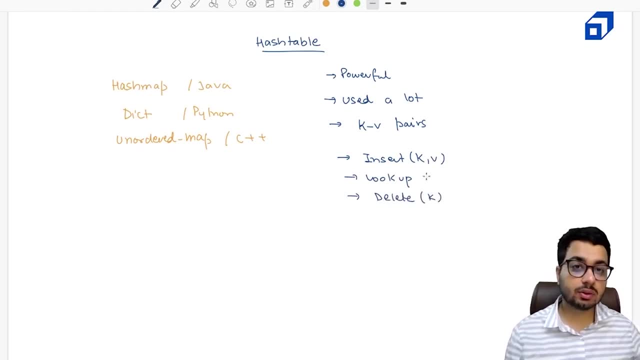 this is the key. delete the corresponding value and the key. so delete the key value pair. given the key, lookup means the search right. i want to search for a particular key, if it is present or not, and if it is present, what is the associated value with that particular key right? so these are the three. 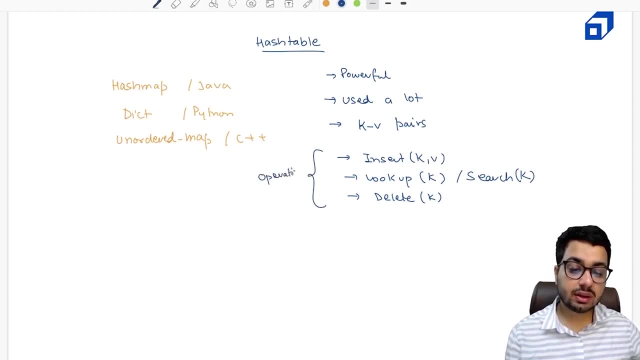 important operations associated with the hash table right, and the good thing about these operations is why this is so popular or why this is so powerful: because these operations are performed on an average, in order one time. so order one on average, that means most of the times these operations will. 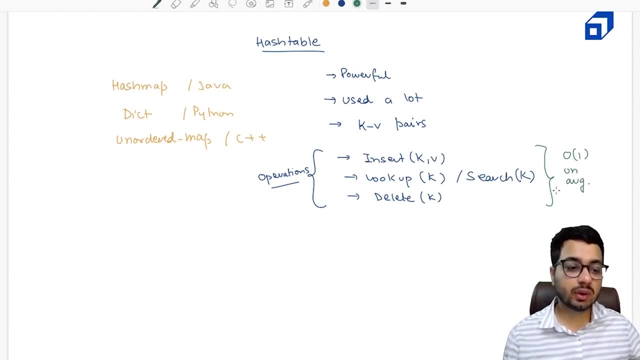 be performed in constant time. okay, so we will discuss the scenario when they are not performed in constant time. but you can say, okay, most of the practical scenarios, these operations would be performed in order one time by the hash table. right now let us discuss where this can be used. 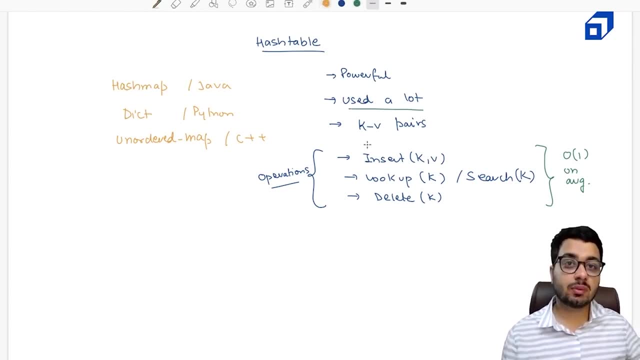 okay, so i discussed that it stores information in the form of key value pairs. okay, suppose you are building a application for a restaurant and user item. a user of wants to order particular item, right? so user says, okay, i want to order a particular item, so i can order a particular item. 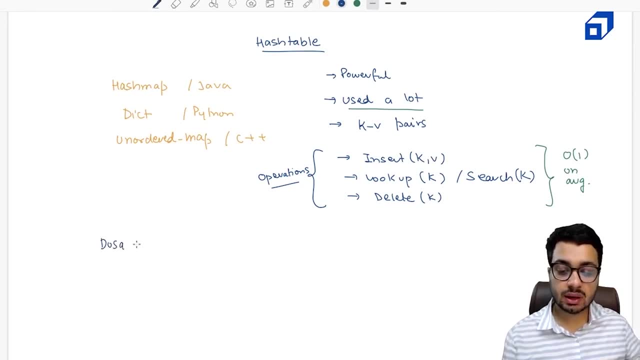 want to uh check if dosa is available and what is the price of the dosa. the restaurant owner might instantly reply that, okay, the cost of the dosa is 100. right, so given this key, you are telling the value in order one time. okay, maybe i want to order some coke. maybe this is priced at 50. 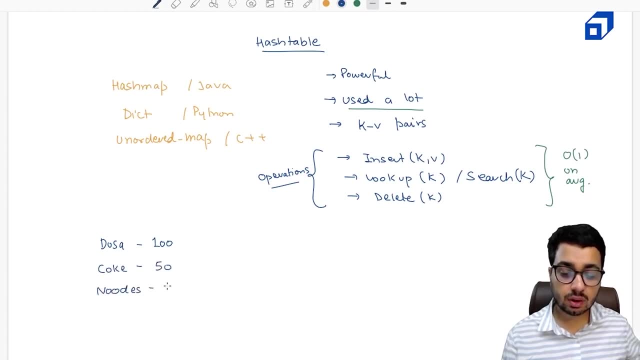 maybe i want to order some noodles, right? this is cost, costing maybe 70, right? so what can happen with this menu? what are the operations we might be doing on a restaurant menu, right? so if we are building an online menu, we might be adding a key value pair. okay, a new item has been added. maybe. 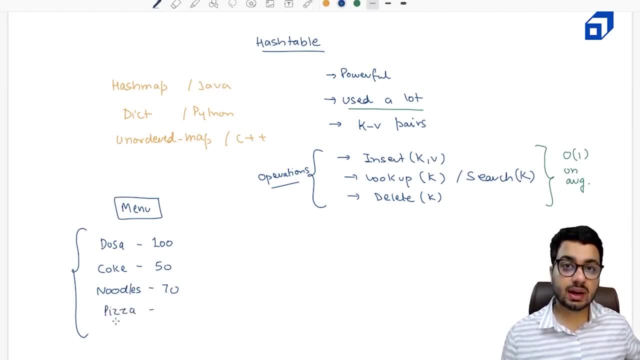 a pizza has been added, so you will supply. okay, pizza has been added and it is associated with some object, or in this case, that object is nothing but an integer object only, right? so the cost of pizza is is 250, right? so i can say i want to insert a new key value pair. that is doable. second is i 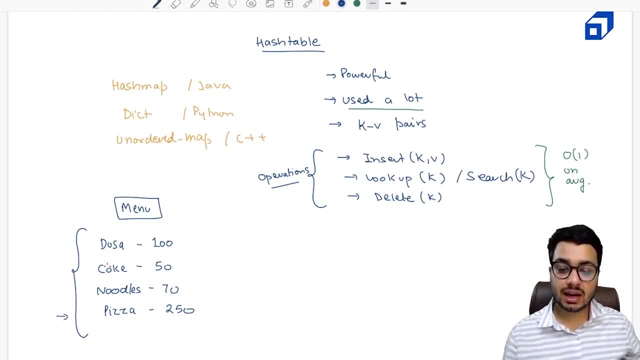 can look up now. i can ask what is the price of the coke, so the hash map will tell me in order one time. yes, the price of the coke is 50 rupees, then i can delete. i can say: okay, coke is not in the stock, delete coke. so it will be deleted from the table. so these are the three operations that our hash 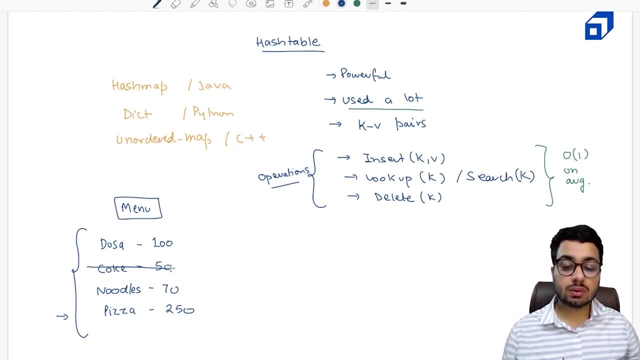 table is going to support right now. of course, we saw that this can be used in business logic. when you are building an application, a hash map can be useful data structure to use. right, because it provides fast lookups, fast inserts and fast delete operations as well. right but one. 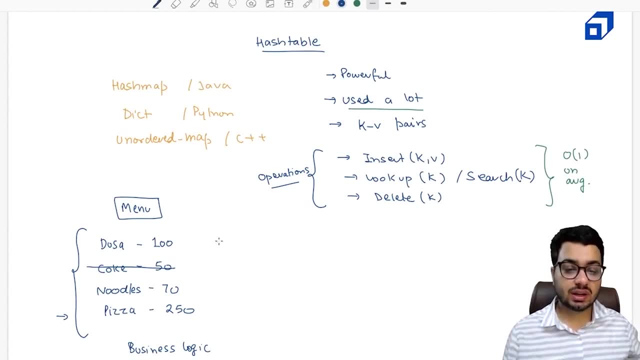 major application is also in the language runtime, right? so whenever you are working with a language like java or c, plus, plus, you know, uh, you create certain variables. you say create certain classes. so you say, okay, i'm going to create a variable, uh index, and i'm going to say: this is 10, right. 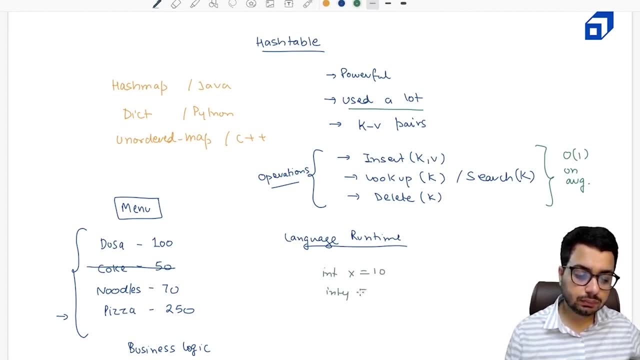 then it's okay, into y. this is 20, right? so what happened is how these uh variables are stored. so these variables are actually stored in the memory, right. x is a bucket that is storing 10, y is a bucket that is storing 20, right? but when you want to make a change, you want to. okay, x is equal to x plus 2, right? so 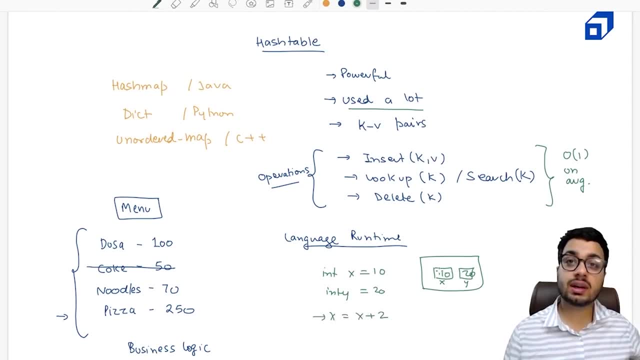 your compiler needs to know where is this x located so that it can go to that location and change that bucket. now suppose this bucket is at some address abc, right? let's say abc20. right, this is some address written in a hexadecimal format, right? so the compiler maintains a symbol. 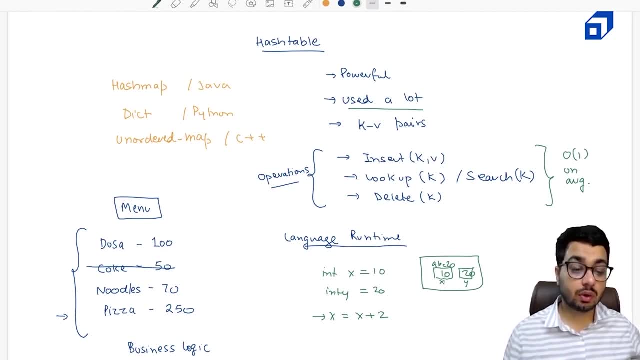 table for all the variables and the classes that you are going to, all the objects that you are going to create. so there is a symbol table, right, maintained by the compiler, right. so this symbol table will tell that, okay, x is a bucket which is present at this location. abc20. right now, when you 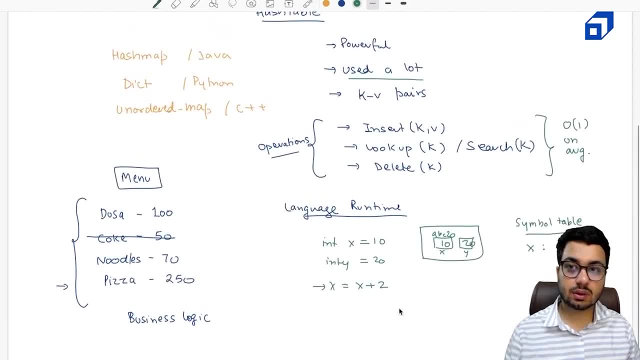 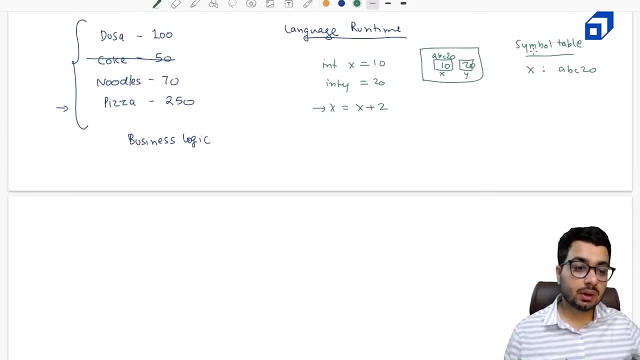 do this operation, x is equal to x plus 2.. so i'll just scroll up a little bit. when you're doing this, operation, x is equal to x plus 2. so the compiler will look at the symbol table. where is x located? it will go to that location and it will make the change right. 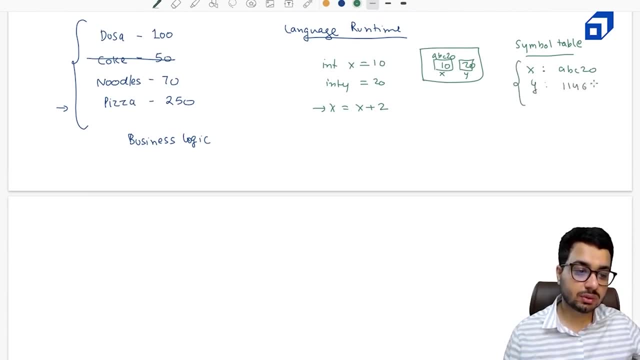 similarly, y is located at some location, maybe one one four six two right and maybe right. so one one four six two. this is some other location for y, so y will. it will again look up at the symbol table where is y located. it will go to this location and it will make the change in the y right. similarly, if 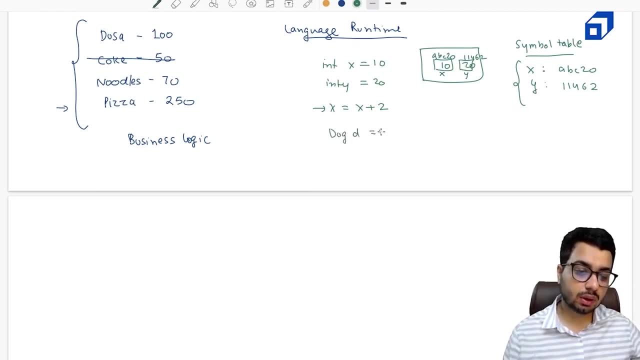 you create some objects. let's say dog d. this is equal to new dog, so this dog object is created at some location in the heap right. so similarly, your d will be mapped with some address right now. what is your symbol table? a symbol table is also of a form of a hash table right. 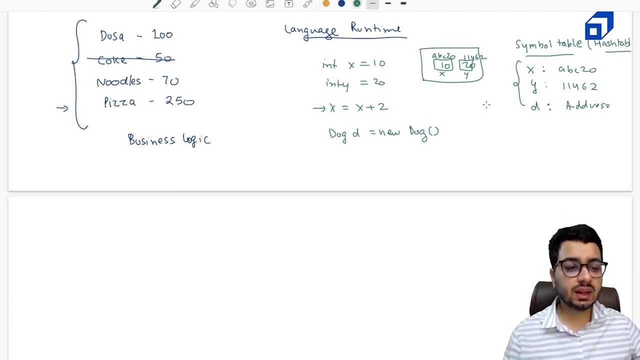 it is also a form of a hash table right that your compiler is maintaining and it is called as symbol table right. similarly, when you have classes and objects right, so use your symbol table to create a new class called dog. dog has certain properties, right. let's say it has a. 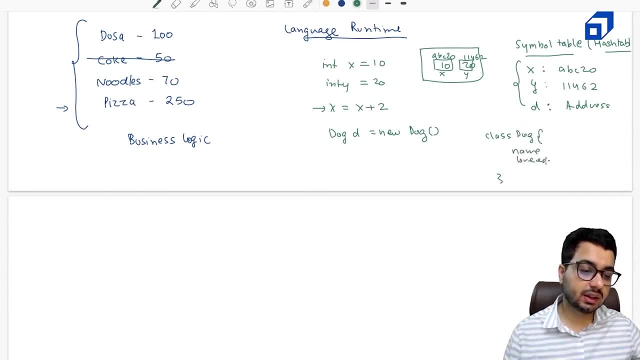 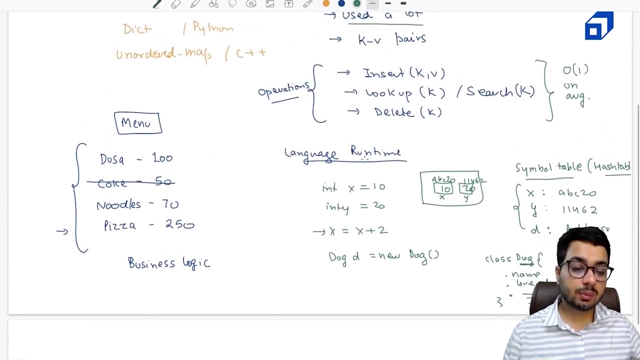 certain name, it has a certain breed, it has a certain method, right? so what is happening? so you are also. you are able to map dog with various attributes and various methods, right so all these features? right they are. they are powered by the language runtime and language runtime. 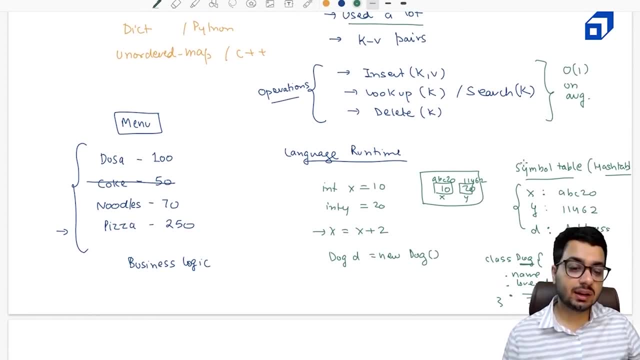 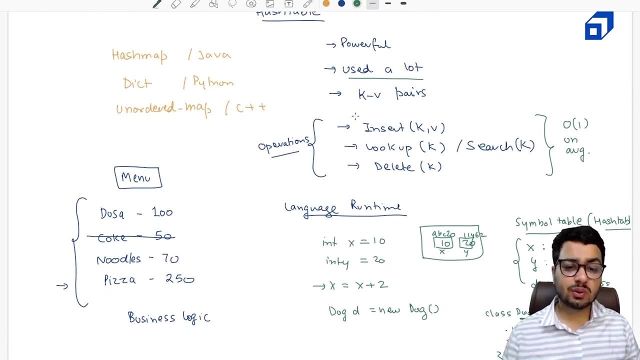 might be, is actually used in the hash table internally so that you can do lookups very, very fast. okay, if this functionality is slow, your language will become slow. so that is another application of hash table. it is used in the internals of the language. so i hope you got a good introduction about hash table. now we 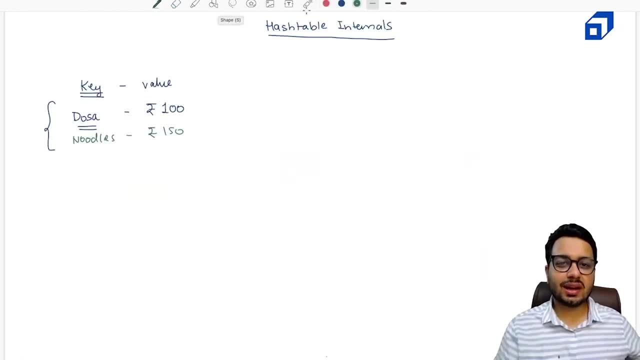 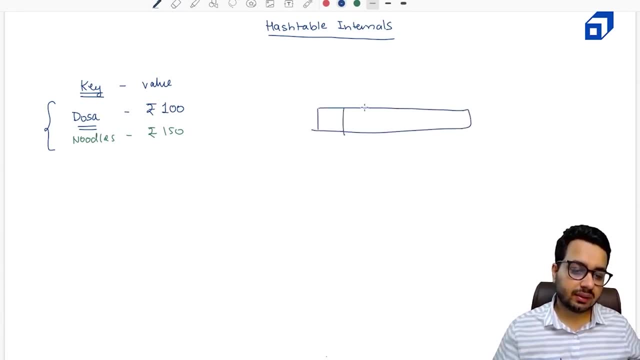 it can be an array as well, okay, of some size, right? so basically, whatever data we are given, we have to map this data with a certain index in this array, right? so suppose i'm getting dosa right. so the first step of a hash table is that we have to hash the key value, right? 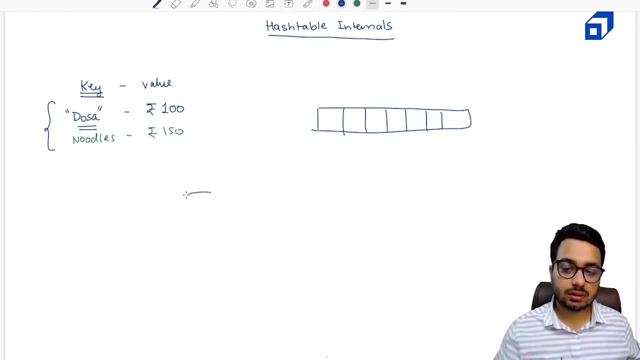 we have to produce an integer location for a given key. now, given key- in this case i'm taking it of the string type, but it can be any object, right. it can be student, it can be book type of object. you need to tell the hash function how the that integer value will be computed, right? 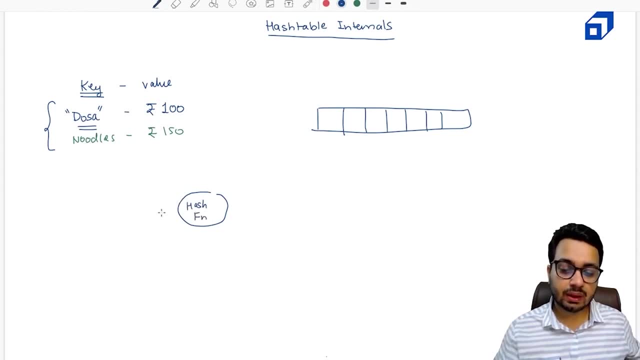 so right now, i am assuming that there is a hash function which is going to accept some key, let's say dosa, and it is going to produce an integer location, right? so maybe that integer location is zero, one, two, three, four, five, six and so on. right, maybe dosa will get stored here and 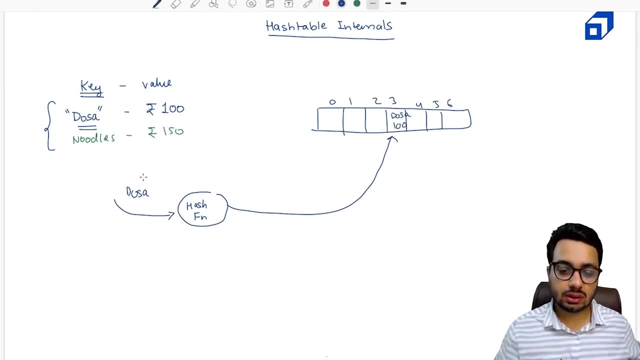 the value will also get stored here, right? i got noodles, so noodles will go also go into this. maybe i get a location six, so maybe noodles get stored here and 150 gets stored here right in the same location, right? so what is this hash function doing? hash function is taking input, a key, and it 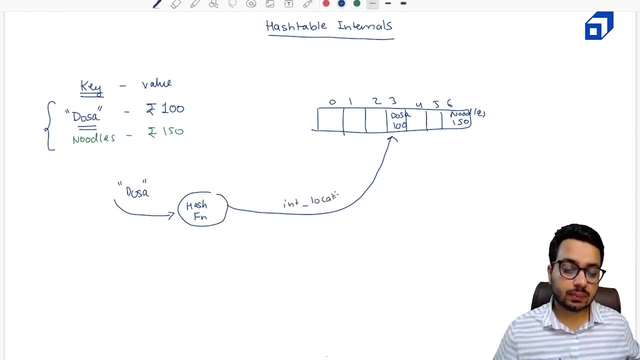 is producing a integer location in the array right now. you might have some questions, right, how big this array should be right now if i have six keys. and if, if i have six- uh, let's say six size of the array right- and i have 12 keys, then of course i cannot store 12 keys. 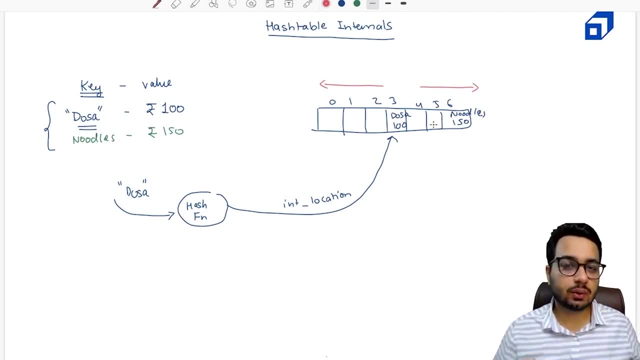 in this array, right? so it's going to cause problems, so we will look at how to handle this very soon, right? this is not the completely correct implementation. we are going to discuss it step by step, right? so the idea of hash function is that it is going to produce a unique integer location. 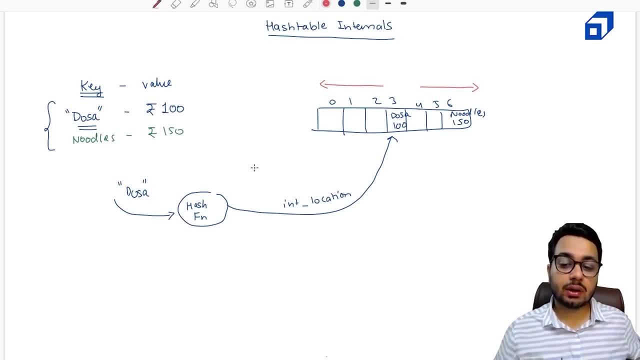 for every key, but it is also possible that for two different keys they get mapped with the same location. for example, if i get something like coke and this, since this is a mathematical function, it might compute a similar location for the same location for the same location. for example, if i get something like coke and this, since this is a mathematical function, it might compute. 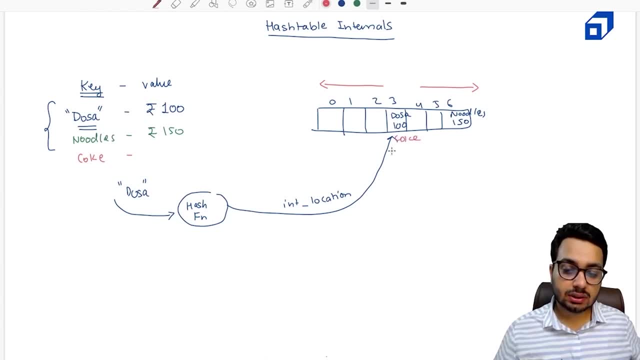 location as well, right. so it might say, okay, coke should also go here, right, so this is called as a collision. we will discuss how do we handle collision, right, so maybe 200 something, but the idea is how big this array should be, right. so one thing we need to note is that this in if it is: 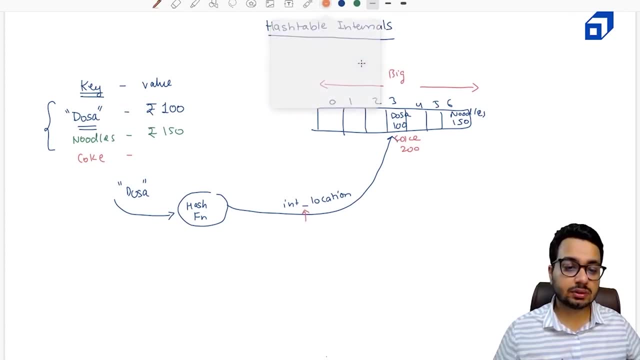 producing an integer, then integer can take any value, right? so integer can be in the range, maybe 0 to 10. it could be in the range 0 to 100, right, it could be even in the range of 0 to int max, right? so means like if i talk about every possible integer that can be generated, this range can be int max as. 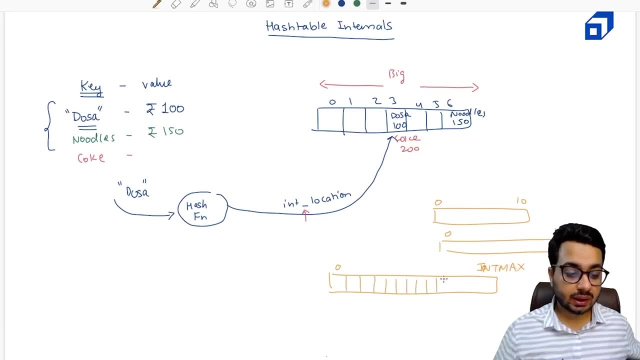 well, right, but do i really need to create this big array? okay, int max is approximately 10 power, 9 elements, right? if i talk about how much space this array will take in the physical memory, this will come out around 16 gb, right? so will you need 16 gb of an array, right, or can you? 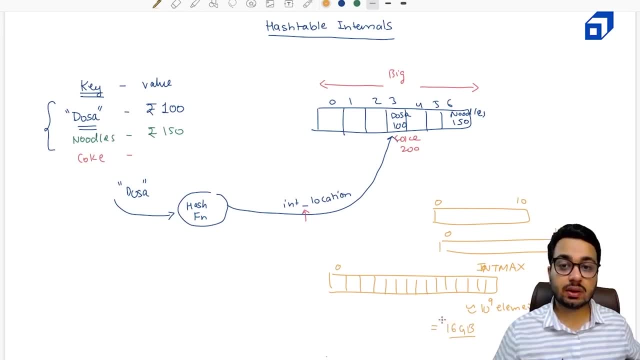 create this big array? the answer is definitely not. we cannot create this big array because this amount of continuous memory might not be available. and secondly, suppose you have created this big array and you have only 1000 keys in your key value pairs in your data set, right then? 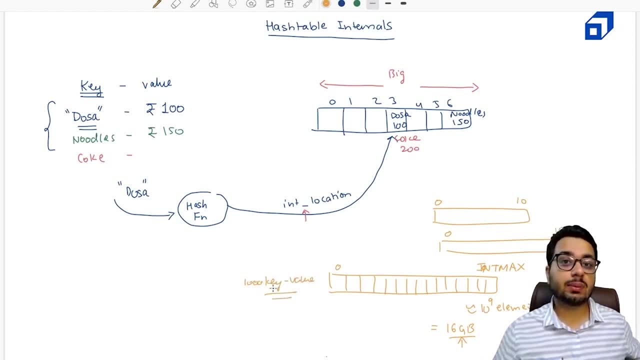 you are allocating space for 10 power 9 elements and you just need space for 10 power 3 elements. that means you are doing lot of- uh, space wastage, which is not a good option. right then, how big this array should be? it should be roughly of the order of number of keys that. 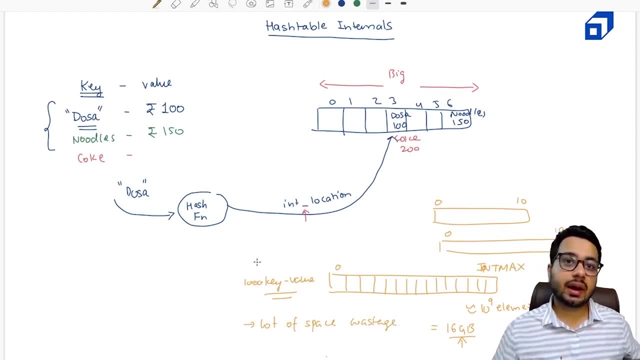 you are, you want to insert, right, so you, if you have an idea, okay, i want to insert somewhere around 1000 keys, then it is good enough. this array should have around 1000 buckets inside it, right? or if you want to insert maybe around 500 keys, it should be of the order. this much, right? so 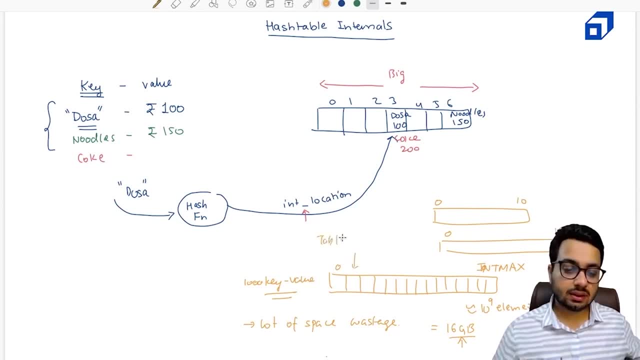 what i'm going to say, that table size should be of the order number of key value pairs that you're going to expect right now. it might happen that you expected 500 keys, but in practice, since the data was dynamic, 700 keys came right. so we will also look at techniques to grow this table. 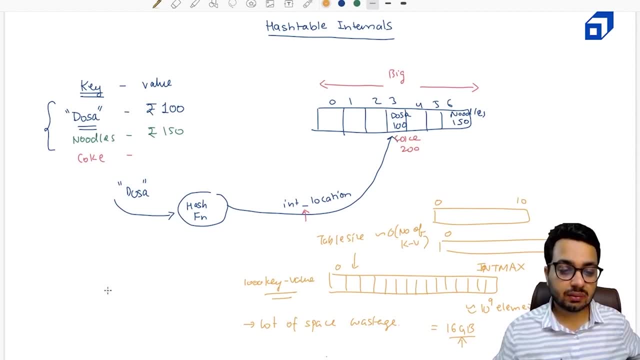 dynamically during the insertion process, right? so that is something we are going to study, right? what happens if there is a collision? how do we grow the table? how do we initialize the table? so all these concepts we are going to see next. so let's begin starting with the hash function. we will talk. 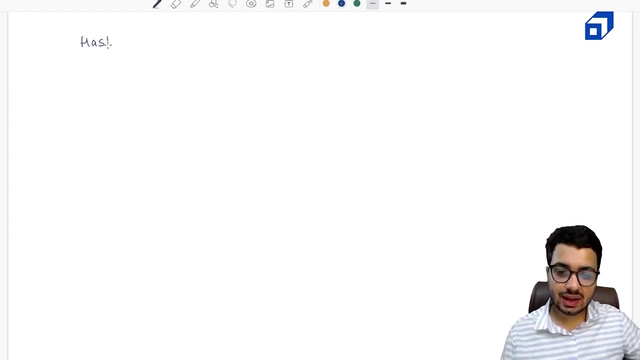 about it in a moment- and deletion in the hash table. so we are discussing hash function, right? so, as i discussed, hash function can accept a key. okay, input is a key. it can be of any, any. it can be any type of object. for our case, i'm just assuming it to be a string and i want an integer. 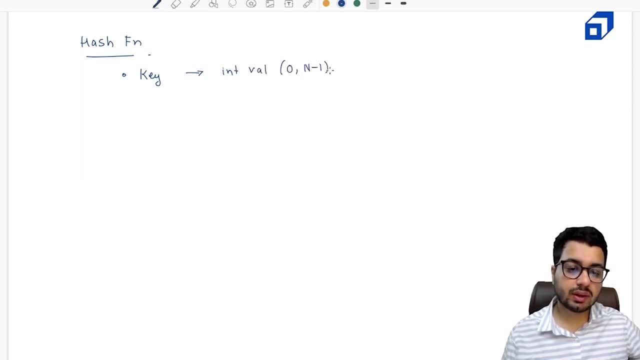 value in some range. okay, in some range, that is, from 0 to n minus 1, where n is the size of the table, size of the table that I am implementing right. so, for example, just to keep things simple, I am going to assume that I have a small table where the size of the table is just 7. so 0, 1, 2, 3, 4, 5. 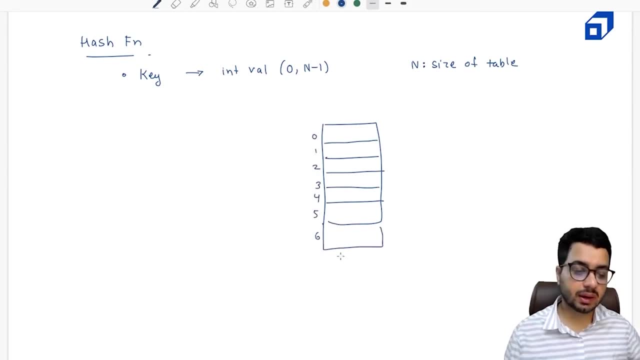 and 6, so indexing is from 0 to n minus 1. so I have this array right, or I call it as table as well. so this is having a table size of 7. right now I have a hash function which knows how do I convert. 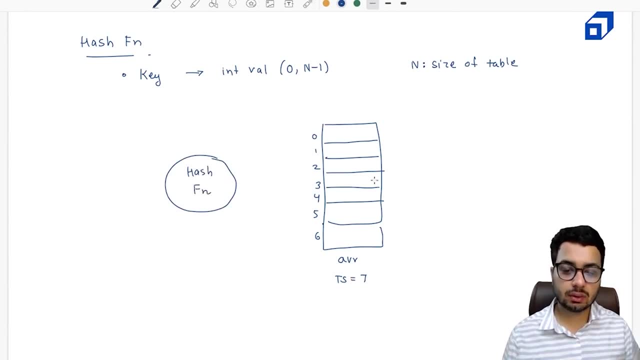 a given string into a numeric value. so suppose I'm getting a key like dosa, comma 100 right. the goal is to generate a integer, map it with a integer right and that value should not be random. it should be same always. so whenever you ask dosa, you have to tell me at what location this dosa. 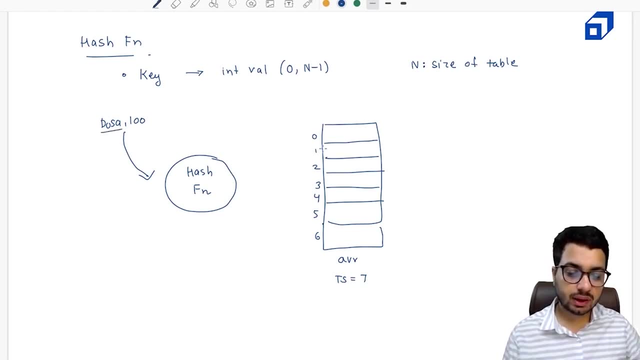 is present. right, the goal is to convert this dosa into a number in the range 0 to 6. right, how do I do it? one simple way would be that I iterate over the ASCII values of dosa, add them and, since this addition will produce a number much larger than 7, okay, for example, your capital A right it? I think it has. 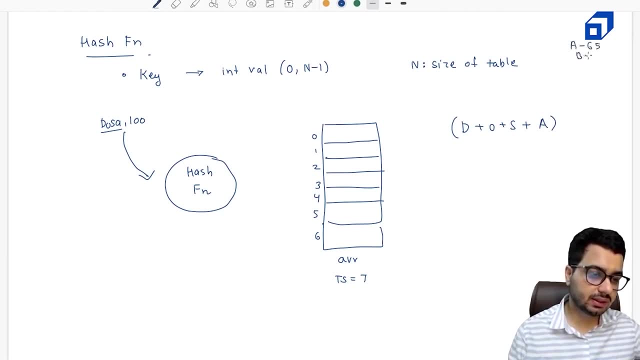 a ASCII value of 65, b is 66, b is 67, so d will be 68, right? so similarly, here you will have certain values: 68 plus something plus something plus 65. this is going to produce a large integer, right, maybe of the order 200 to 300. 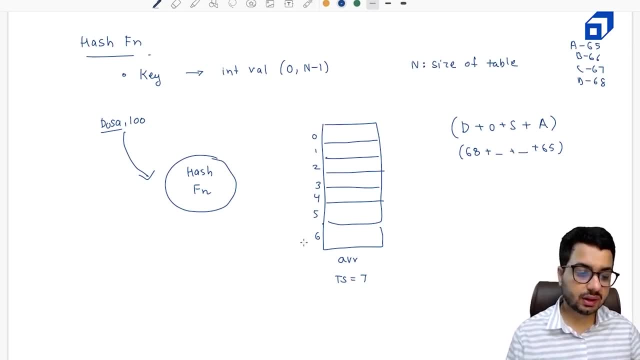 right, but I want to map it in the range 0 to 6, right? so what I will do. how do I reduce a bigger range, which is some larger range, into a smaller range, right? I can say, okay, fine, this can be easily done by using a mod operator, right? so I can say: mod with n, so I can take a mod with n, so let us. 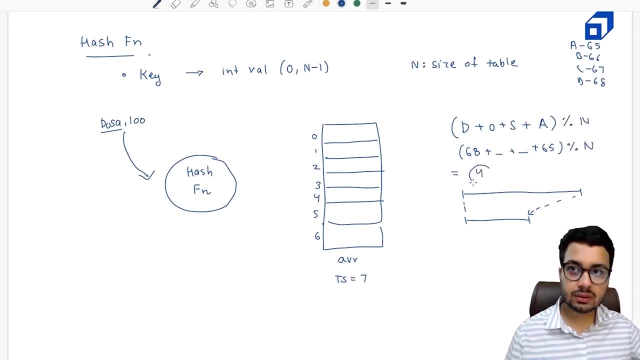 assume that this mod gives us an answer that is 4, so that will be called as a hash index. okay, so basically the index on the table produced by hashing, the hash index is, let's say, 4. so that means dosa will go at this particular index and this value will be stored at this place, right? 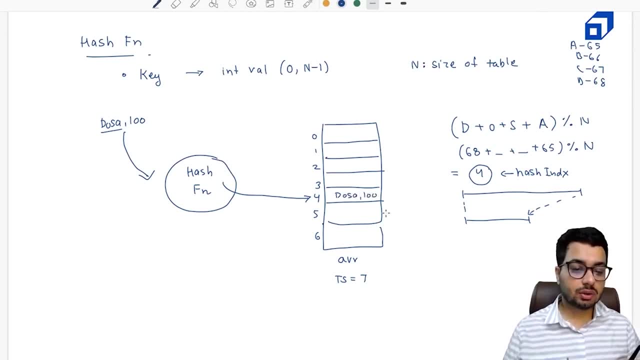 now the question is: what should I do? maybe I am getting another key right in which the result is also 4. right, the result is also 4. so can this happen? the answer is yes. so I can say: okay, I have maybe coke and maybe 150 right, I do not know. I add the letters of coke right and I take a mod with n. 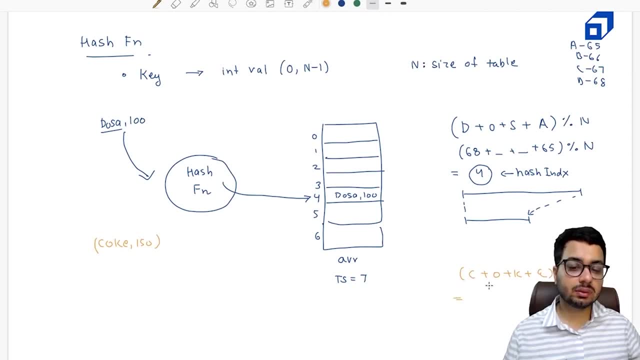 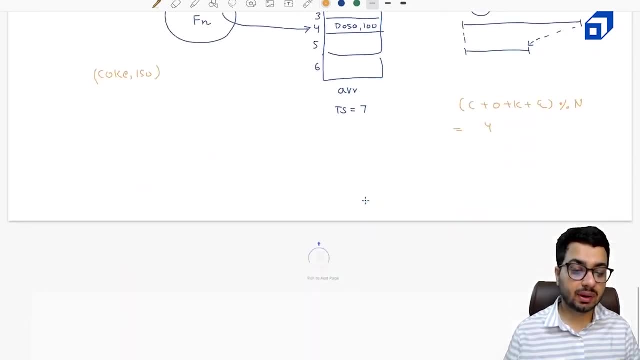 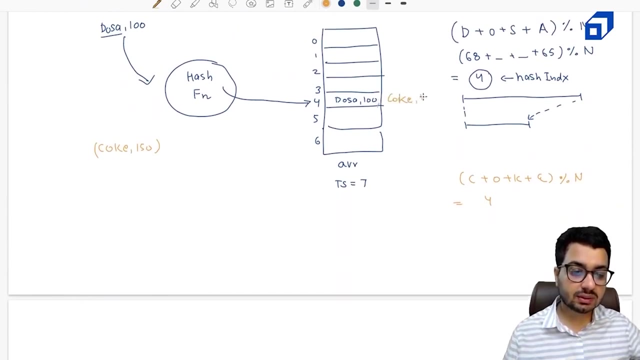 right mod with n can produce the same result for many numbers, right. so maybe this also leads to 4.. what happened here, right? what happened here? the coke is also fighting for the same position. that means I also want to store coke here right now. this thing is called as a collision, right we have. 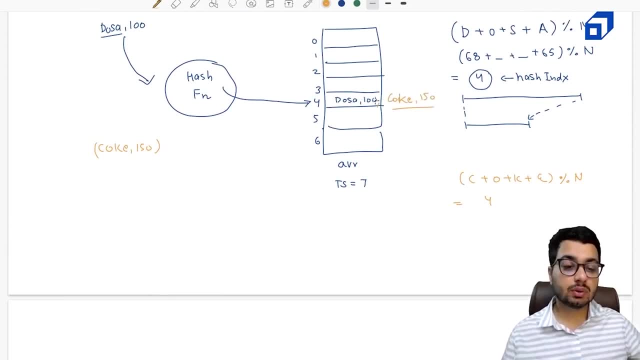 space for only one key value pair, but we want to store maybe two or more key value pairs at that particular location. right, so this is something called as a collision. right so what happens? right so what is a collision? so collision is a scenario in which, basically two 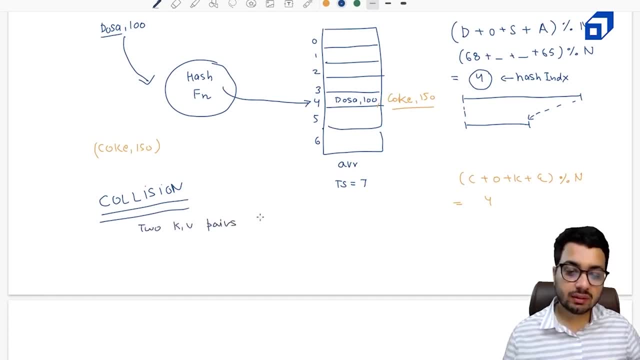 key value pairs, two or more key value pairs, they get mapped with the same bucket, mapped with the same bucket. so this, what does this mean, right? can we avoid collisions? the answer is no. can we reduce collisions? the answer is yes. so the one in the second column will be the next column. then multiply it, right, this volume, also the second column. 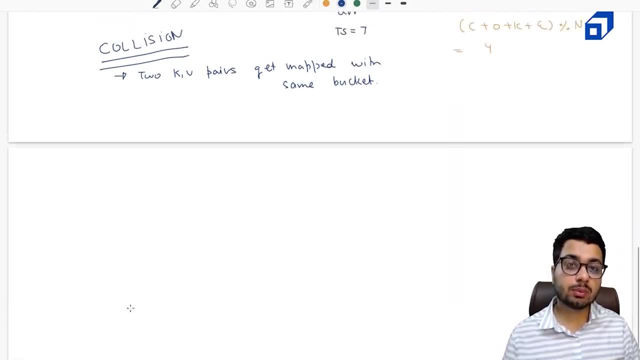 will be one column and the second column will be two columns. if you wanted to just divide two of them, yes, right, so we will talk. talk about both the things, right? so in order to reduce collisions, right, what we need is we need a good hash function. so we will work on both the fronts, right? so 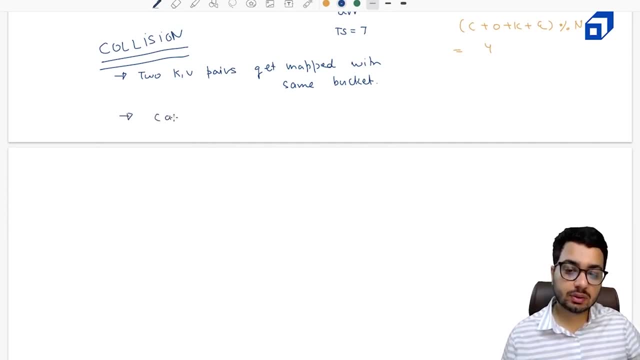 collisions should be it. they cannot be avoided, right? so how? irrespective of how good a hash function is, collisions cannot be avoided, but they need to be handled right. so cannot avoid collisions, right? okay, but i can reduce the chances of collisions, but chances of collisions can be reduced by using a good hash function, right, but chances of collisions can be reduced. 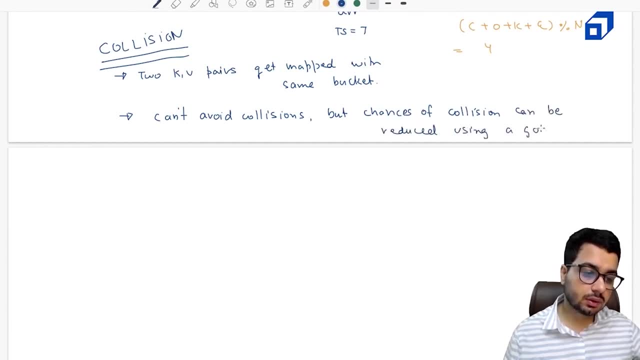 using a good hash function. right, using a good hash function. now how do we design a good hash function? we will discuss by taking an example of string right. and secondly, since you cannot avoid collisions, so even if the collision is happening, you need a way to handle that collision right. so they still need to be handled. 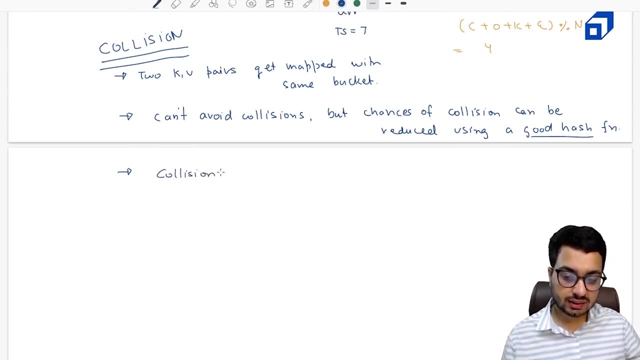 so we need something called as a collision handling scheme, right, collision handling scheme. this is something we will discuss very shortly. right now, there are two important things here. one is: what is a good hash function? second is a good. second is we need a good collision handling scheme. so first, good hash function will reduce the chances of collisions, but they still can happen. 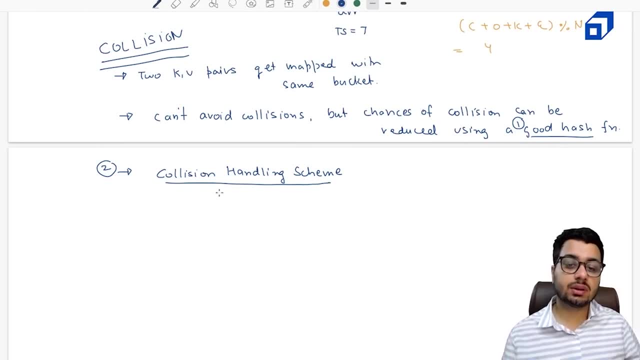 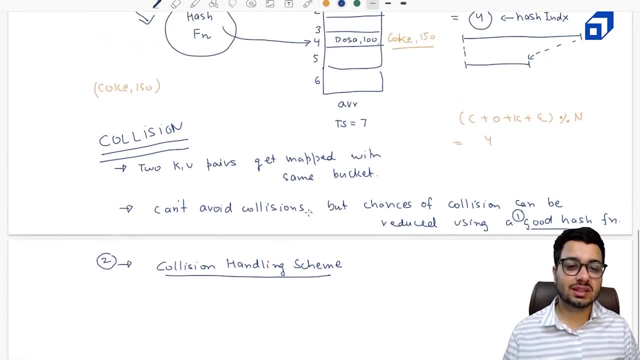 so if the collision is still happening, we need to handle it using collision handling scheme. so let us discuss what is a how do we design a good hash function and how do we design a collision handling scheme. next, let us discuss the properties of a good hash function. right, 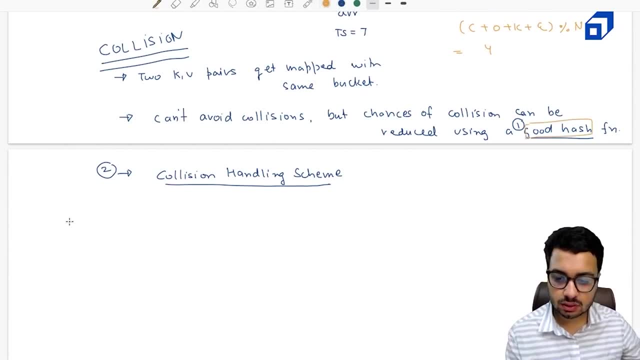 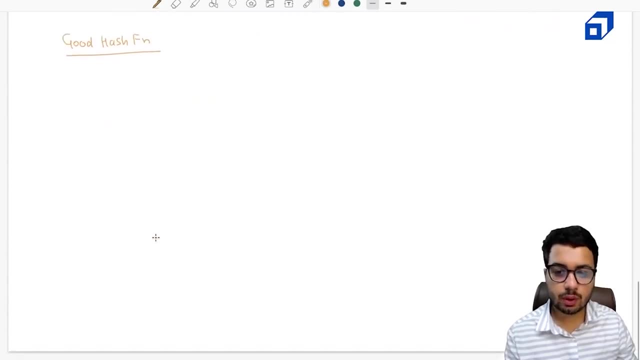 so i am going to discuss the properties of a good hash function, right? so basically, a good hash function should have two properties. first, it should ensure a more of a uniform distribution- okay, it should ensure more uniform distribution, right. and secondly, it should be fast to compute, right. 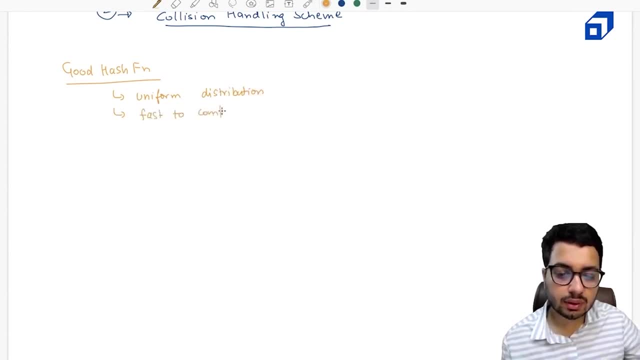 so that means we do not spend a lot of time in computing the hash index itself, right, for example, in our case, what we were taking. i will take examples of two hash functions. okay, so let's say example number one, in which i am simply adding the ascii values and taking a mod with 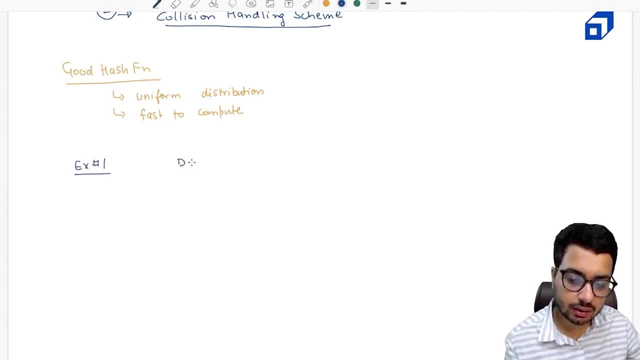 the table size. so i'm saying, fine, i will add dosa d plus o plus s plus a, and i will take a mod with the table size right now is: is this function fast to compute? yes, because i just need to iterate on the uh letters of the key, right? so when, when i'm talking about, i'm going to insert many key. 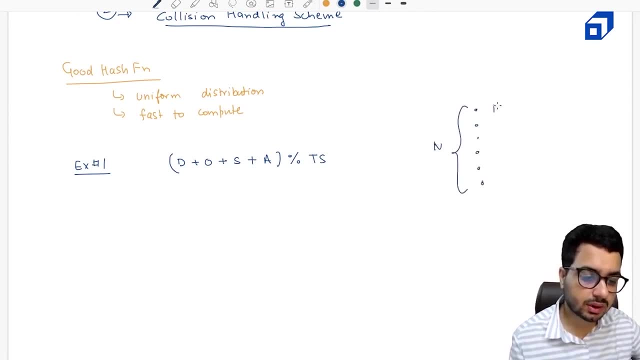 value pairs. so what is n? n is the number of key value pairs. okay, so key one: value one. key two, value two. right key three: value three. i want to insert many key value pairs. so my hash index does not depend upon the value n, but it depends upon how big my 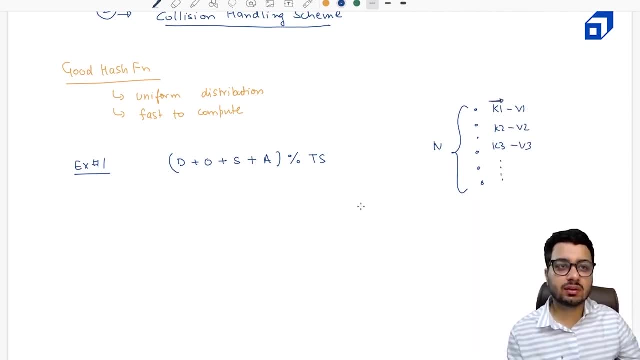 key is. so, in general, the key would be small. let so we can assume that. okay, if it is a name of a person and the phone number is the value, the key would be maybe maximum 50 characters or 100 characters. so, yes, in this case this is a fast hash function, right, but is this hash function is going? 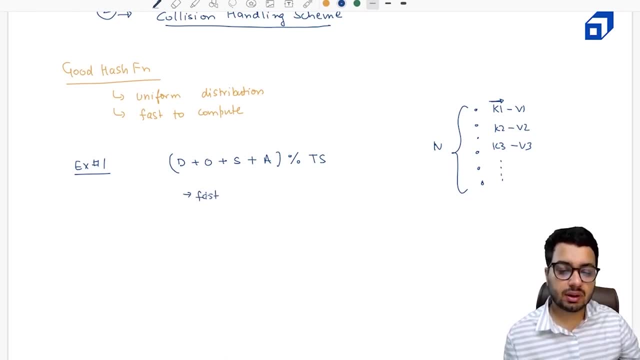 to minimize the chances of collisions. maybe not right. why? because if i talk about english language, right, in english, lot of words they are anagrams. that means uh, lot of words have same set of letters in them. for example, let's say the word is tab right, so it is made up of t, a and b. and if you add 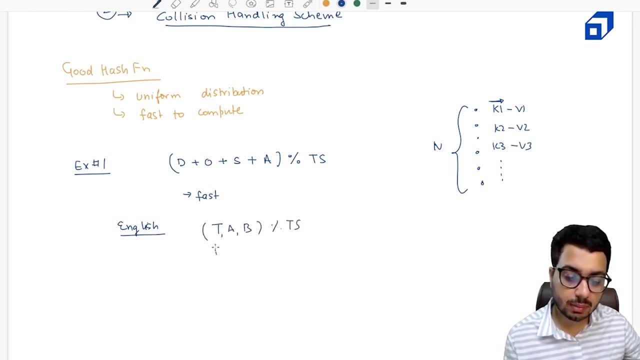 you will get certain sum right. but if i talk about the word bat right, it is also made up of same letters. so in this case we are sure that these two are going to collide because our hash function is doing a very simple sum right. so in: maybe of course there could be other words also. maybe the word is mango right. 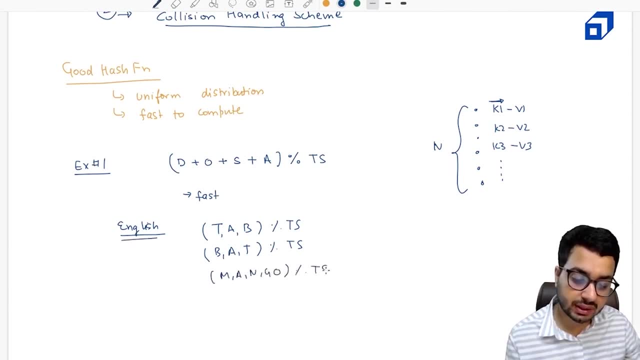 now, it is possible that even if you do a mod with table size, you might end up at the same index, right? so we do not know. so in this case it is of course difficult, uh, to tell whether the collision will happen or not. but it may still happen, right? but here we are sure that a collision will happen. 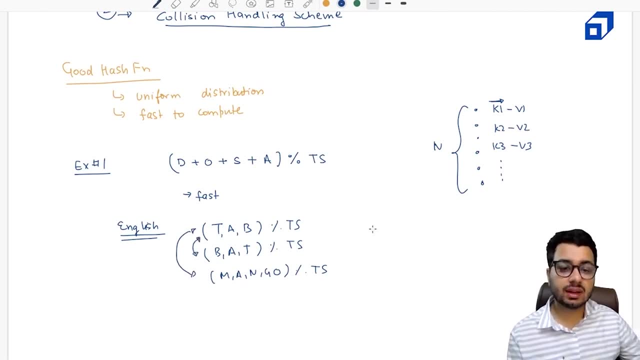 right. so many words in english. they will have such a scenario, right. so what we can do is, instead of doing a simple addition, right, we can do a weighted addition, right. so this is like a simple addition of rsk values we are doing right, so a better way would be. 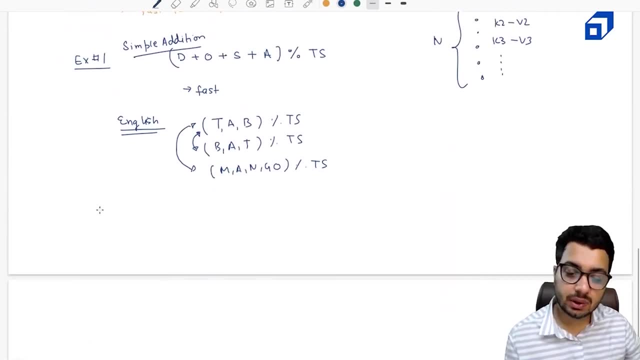 that you do not do a simple addition in your hash function, but you do a weighted addition, right? so example two of building a hash function would be that you do some weighted addition, right? so that means you are going to multiply each letters value with some weight, right? so, for example, i choose a weight. maybe generally it is a prime. 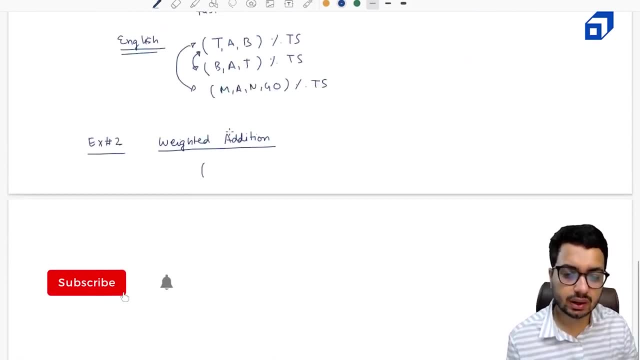 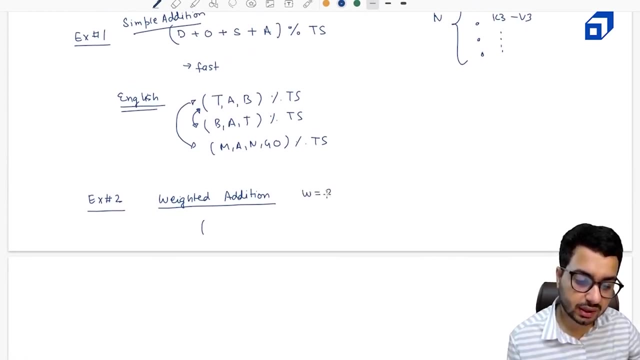 number right. so maybe i choose a weight as let's say 31, right, or 29, right. what i can say? that fine, i will multiply dosa with powers of 2.. so let's say the weight is 29, so 29 power 0, that is 1. 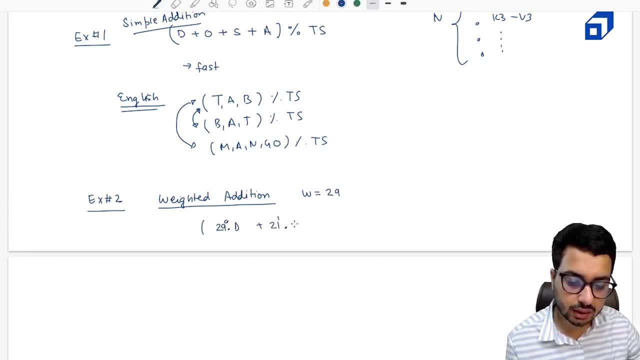 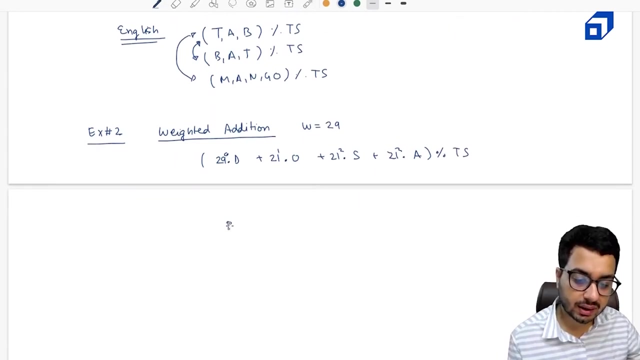 into d plus 29 power 1 into o plus 21 square into s plus 21 square into a. and then i take a mod with table size right. what i'm trying to claim is now: if you do it for bat and tab, it is less likely that you will have a collision, right? so i'm saying you multiply. 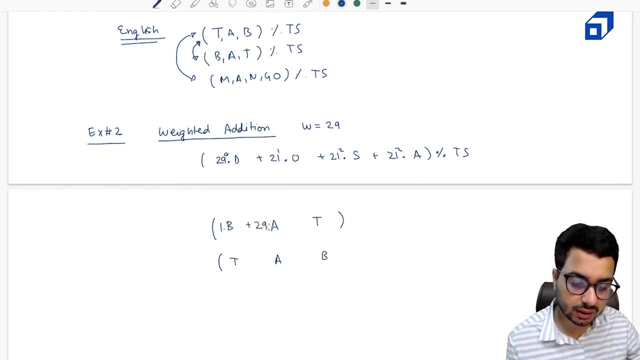 29 power 0, which is 1, this is 29 and this is 29 square right. and then you like, it's a weighted addition again, 1 plus 29 into a, plus 29 square into b and, of course, mod with the table size, mod with the table size right now. earlier we were sure. 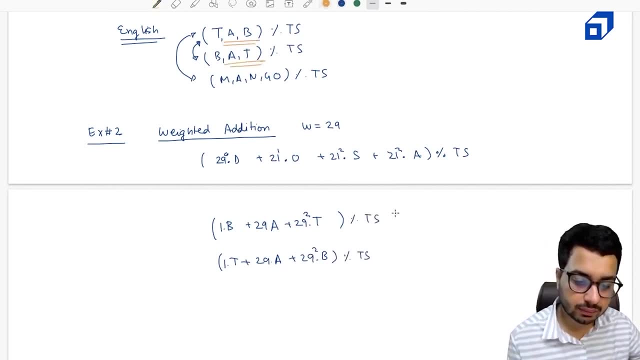 that these two values, ah, will surely collide. now we can forget. the chances of the collisions are less. okay, so there is a less chance of collision, right? so these are the factors that you can keep in mind, that, okay, if i'm building a hash function, can i modify it some? 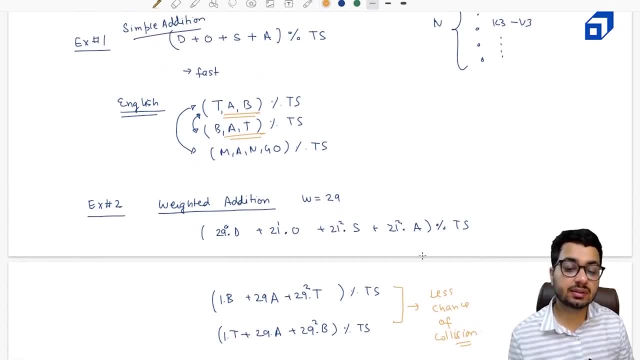 way so that it reduces the chances of collision and it is fast to compute right. so here also it is to compute right. maybe, if you have a string with in which the length is too big, maybe you can restrict that. okay, i will consider only the first 10 letters of the string for this weighted edition. 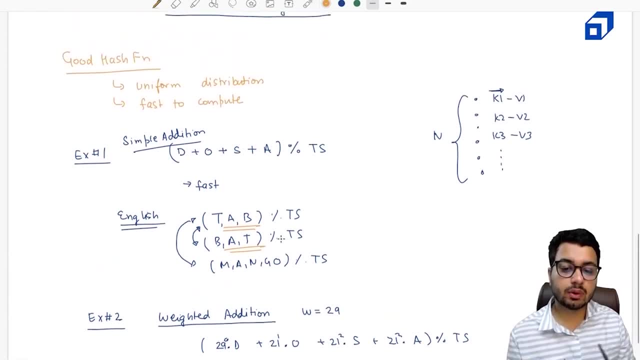 that can also be done. right, so, that will even make the function a bit more faster, right? so, if you are thinking that the keys are too too long, you can restrict to maybe the first 10 letters or maybe something like that. right? so now we have a good hash function, which is the second one. the second 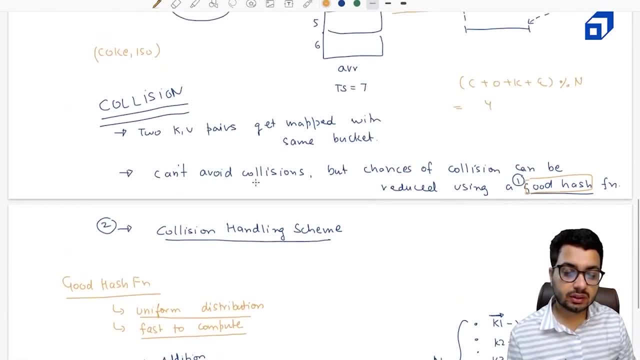 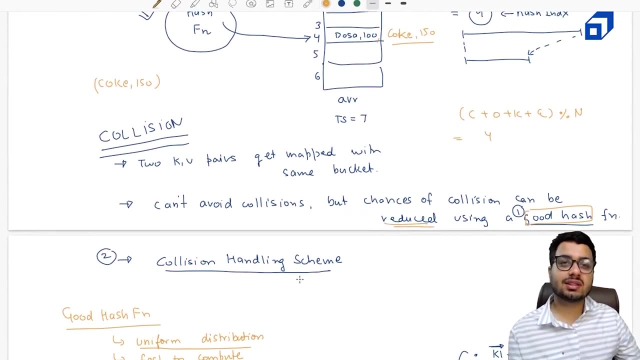 one is obviously better. we are doing weighted addition, so it is going to reduce, uh, the chances of collision, right, but a collision can still happen, right? so how do we handle if still a collision happens? so here comes a collision handling scheme, right? so let us discuss about. 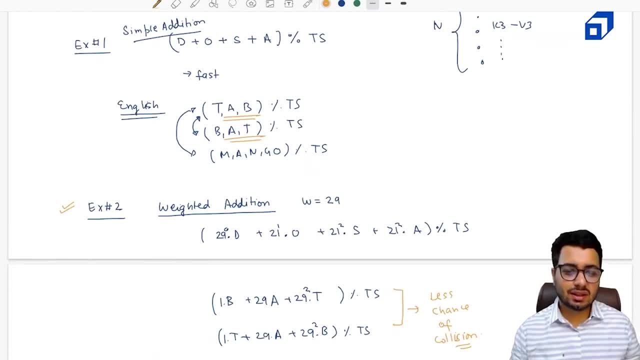 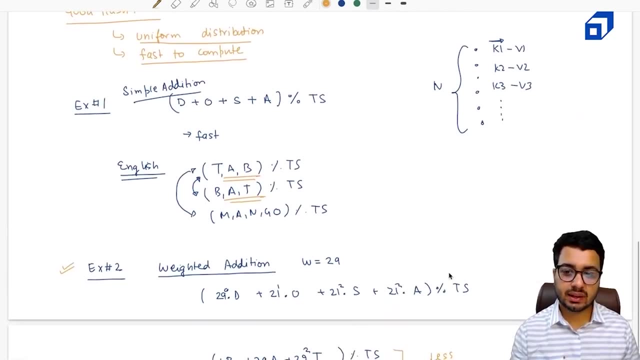 collision handling scheme now. so you have seen how do we design a hash function. now we need to discuss how do we design a collision handling scheme right? so collisions can still happen. we need to handle them right. so let's see how do we design a hash function. now we need to discuss how. 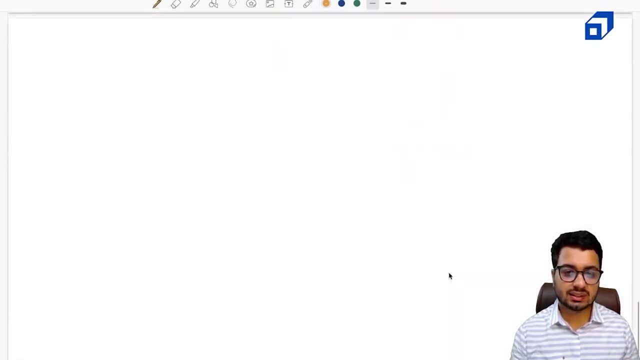 do we design a collision handling scheme right? so collisions can still happen. we need to handle them right. so let's see: how do we design a hash function? now we need to discuss how do we design a collision handling. let us talk about how do we design a collision handling scheme right. 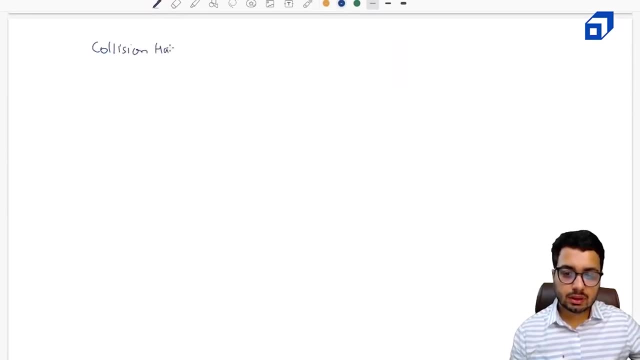 collision handling scheme. right, so there are actually multiple schemes, but i would particularly particularly discuss one scheme, right? so in this case, what we can do, we can do something called as separate chaining, so we are going to discuss only one scheme. there are other probing techniques as well, right, so i will discuss separate chain. 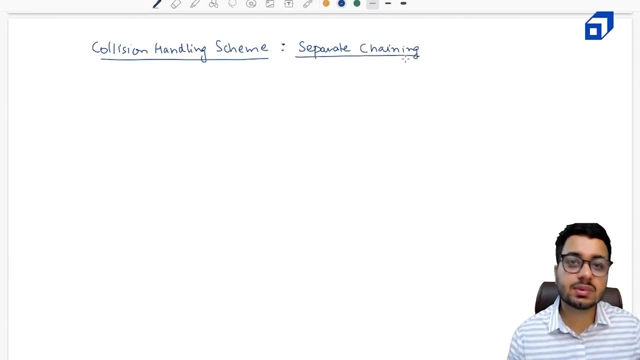 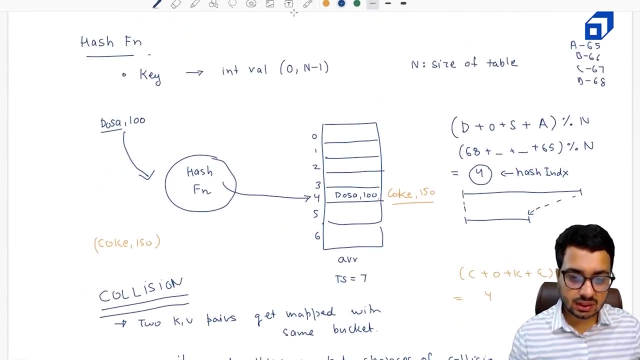 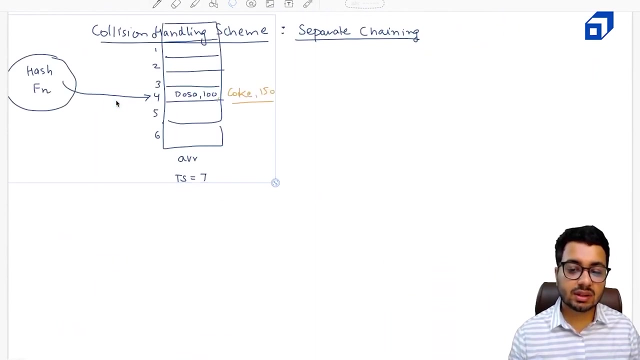 chain technique, right. so this is one of the most popularly and widely used schemes in implementing a hash table. right now, i'll just copy the diagram that we have seen earlier. this is the diagram, right, so let me just copy it. uh, so here we go. the idea is that if a collision happens, what should we do? right, that is what needs to be addressed. 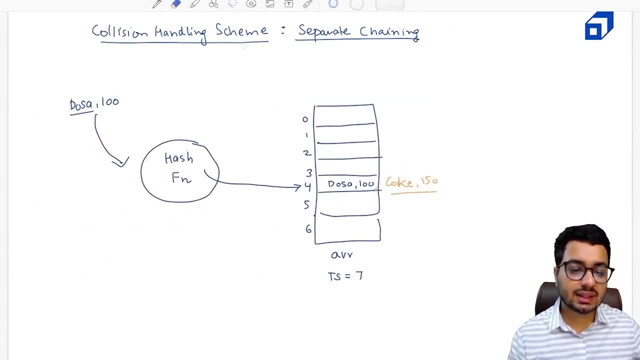 right, that is the problem right there. okay, so what we are going to do in this example, we are going to address using a technique called as separate chaining. so suppose if we got dosa and it get get mapped with index 4, so what we will do will not store it directly inside this bucket. 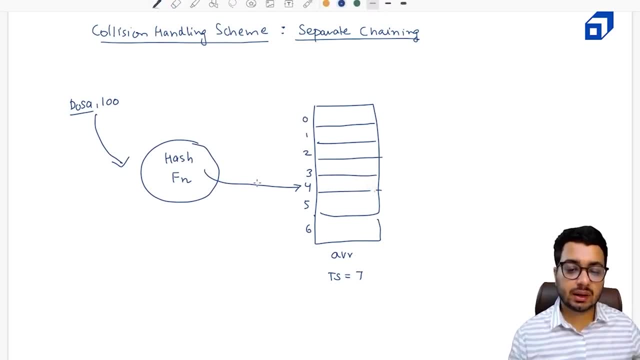 but instead, every time we get a particular bucket mapped with dosa, we will start a chain from there, right? so what? what is a chain? a chain is like a linked list, so it's exactly a list, right? that means each bucket is actually going to hold the address of the first node of the list, right? so for? 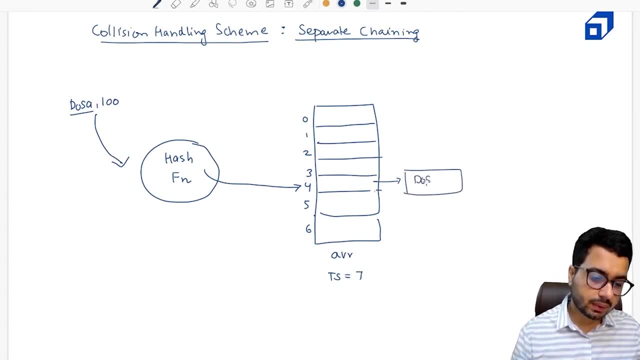 for, for example, i'm going to store dosa comma 100 here right now. suppose i got coke comma 150. the coke goes into the hash function and maybe this time i get two, so i will start a chain from two and coke will go here, coke comma 150. it will be stored here right now. suppose i got something. 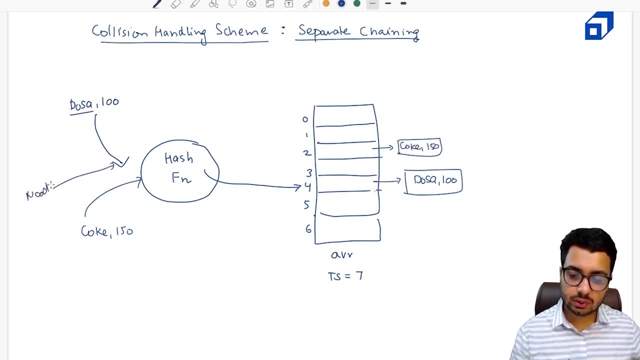 like noodles, okay, and noodles is going to have a value, let's say 120. now noodles, if it goes to the hash function, let us assume the hash function computes the index 4 right now. at index 4 we already have dosa. so what we will do? we will also try to store noodles at this index. how? 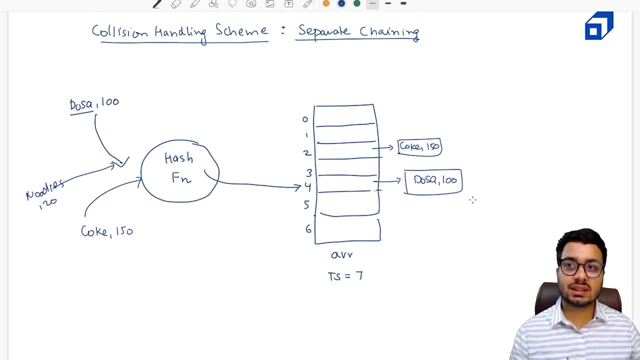 so we can- okay, we can- add noodles to this linked list. now, suppose this is some address. let's say: this is, uh, 150, this is 270, right? so this is storing 270, this is storing 150.. so each array bucket is actually storing the head of the linked list, right? 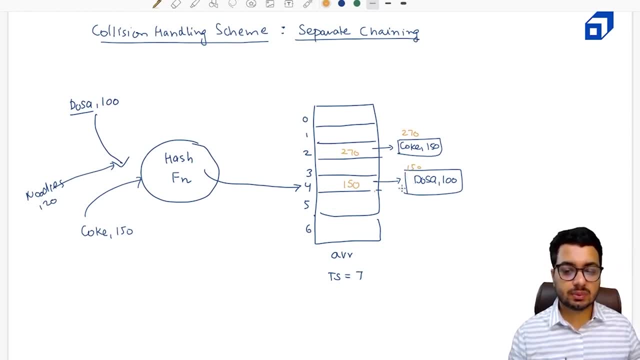 now how we can insert noodles in this chain in order one time. it's pretty easy, so you can. okay, i will create a bucket called noodles. let's say this bucket is: uh, this node is created. so i'll create this node n with the given key value pair: right, so it's a new. 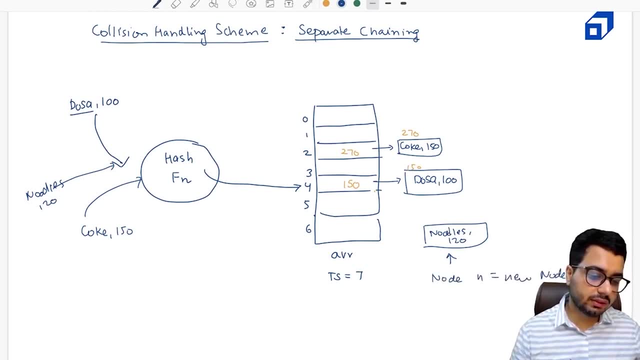 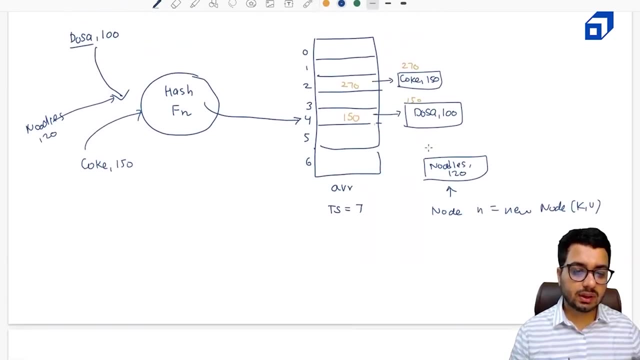 node with the given key value pair right now in this new node. what should i do? like? how do i add this node in this linked list? right, so, i can. okay, this is some array, right so? or this is some table. i can say array of: uh, and let us also compute the index, so i can say index. where i want to store this is given by the. 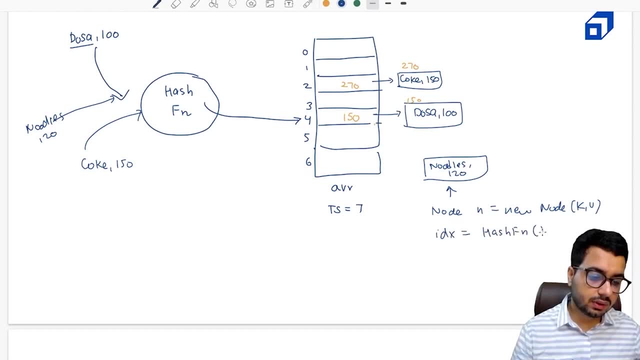 hash function of the given key right. so i got to know that. so now i am going to compute a board, the index also. so at this index i need to store noodles. so one thing i can do is either i can insert at head or i can do insert at tail, since i'm not maintaining the tail of the link list. 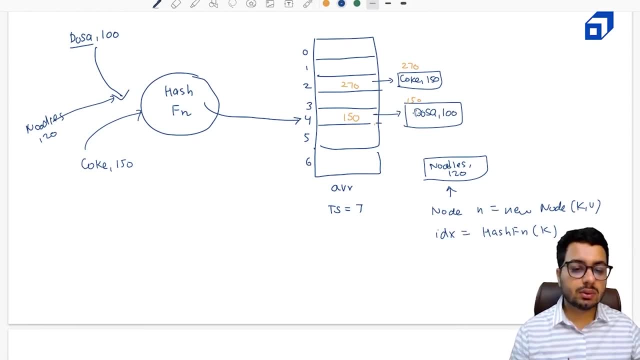 explicitly, but you can maintain. if you want, i can also do a direct insertion at the head, right, so that means we can say, okay, uh, this node 4 will refer to noodles and noodles will connect here. so right now, this is connected here. so what i can do, i can ask noodles to connect with dosa, right, so 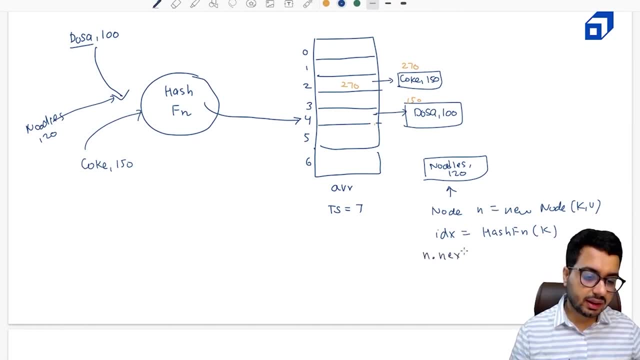 i can say n dot next. so in every node i'm also going to have next field right, so that i can actually form a chain just like a link list. so every node is going to have a next field so i can say, okay, you should connect here right. so i can say n dot next should be equal to array of index. 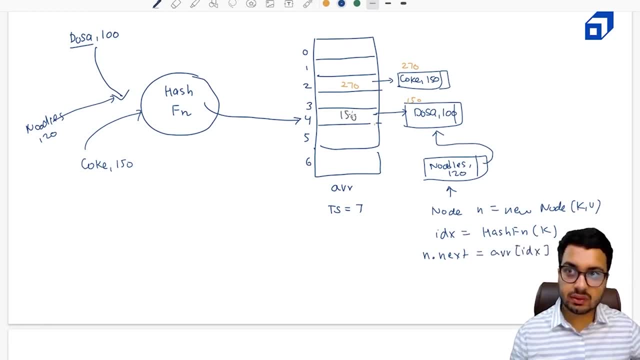 array of index is storing 150, so that 150 will be copied, so i can say n dot next should be equal to array of index. right, and now i can update array of index to point to this node so i can say array of index should point to n. so basically i'm changing this connection like this: 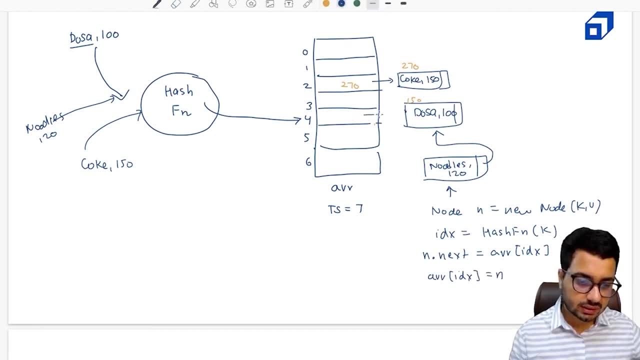 n is what. whatever it is, this will be now referring to this node. if you look carefully, we have actually formed a chain, right? so this is, let's say this is some address. let's say 480. this is now storing 480, right? so you can see. 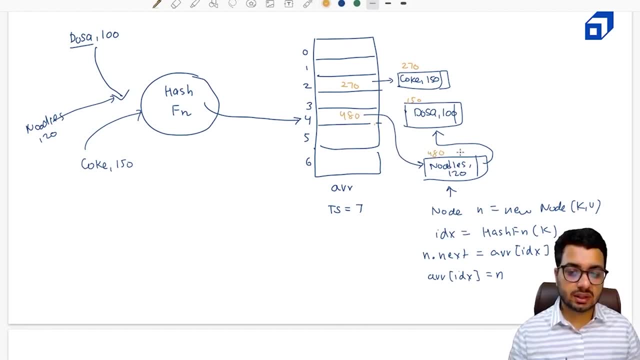 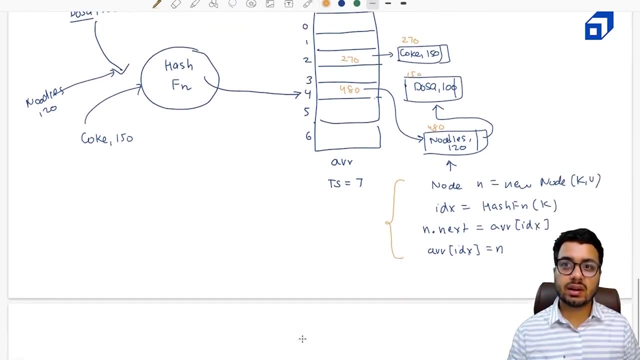 we are actually forming a chain, right, we are actually forming a chain. so this is exactly how the insertion is going to work and this is the code to insert, right? do you think? will it work in order? one time? absolutely yes. this insertion will be always order one, right, because we are 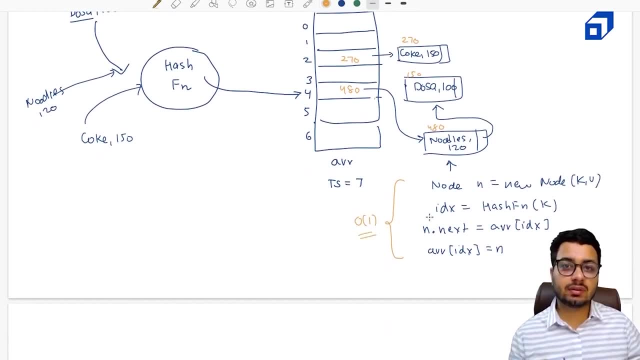 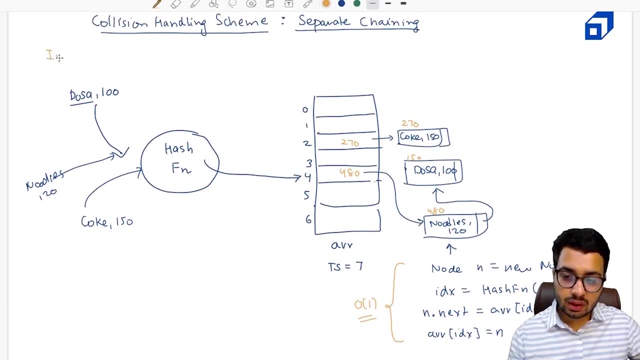 inserting something at the head of the link list. irrespective of the chain length, the insertion will be always order one, right. so i hope you have understood insertion, but is it done? the answer is no. we are not yet complete right. we have to still discuss one more concept, but that concept i will discuss after discussing searching. okay, so this is still. 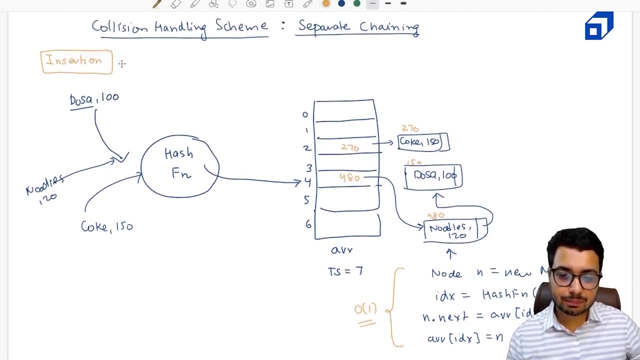 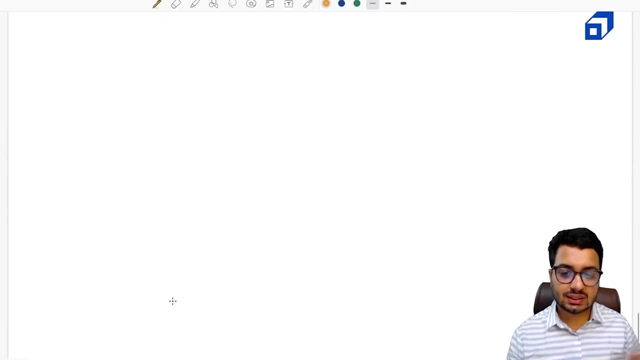 not complete. so this is insertion part one, right? okay, so there is something more to the insertion that is going to come up. right, let us discuss searching- how we can actually search in such a scenario. right, so we are discussing searching now. right, so we are discussing searching now, right. 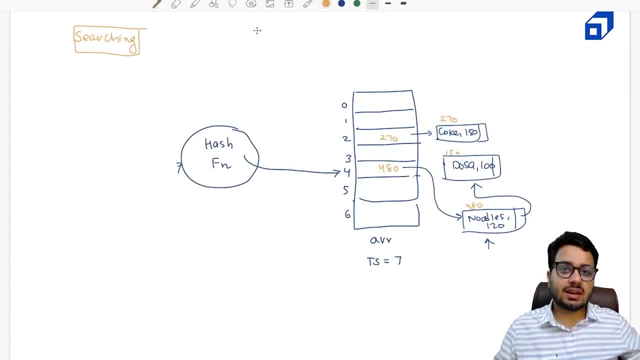 so now, what is the purpose of searching? the purpose of the searching is that, given a key, i want to look up for the value of that particular key. right, if i ask? okay, i want to know what is the price of dosa, how i will find it. so, first of all, dosa is a key. this is given as input, so dosa will. 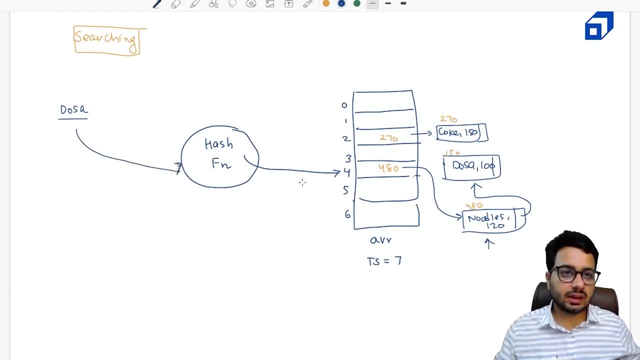 go to the hash function. the hash function will generate a index where this dosa can be present. in this case, hash function gives me an index 4.. that means now at index 4 i actually have a chain right. so now at index 4 i actually have a chain right. so now at index 4 i actually have a chain right. 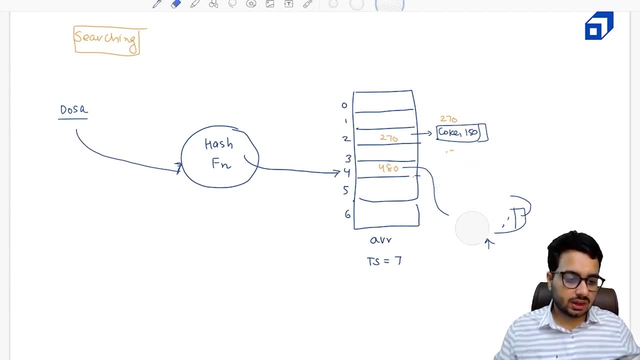 if i write it little more clearly. so this chain looks like this: i have noodles and which is like 120, and i have dosa, which is part of the chain, and this price is 100, right, and of course the next is none. now i have to iterate on this chain. 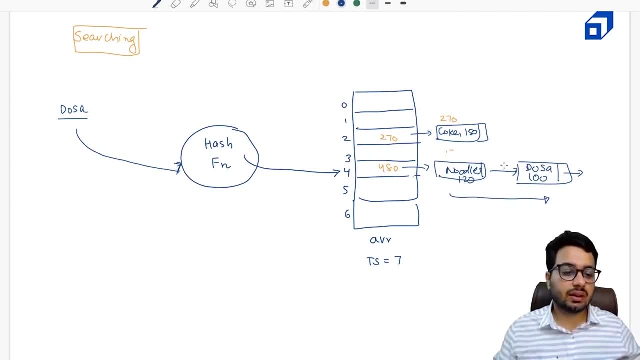 to check if this chain can contain dose or not. so if i iterate on this chain, i will find a dosa at this particular position, and once i find dosa i can return the value, that is 100. right, that is how searching is going to be performed. so we first find the bucket. 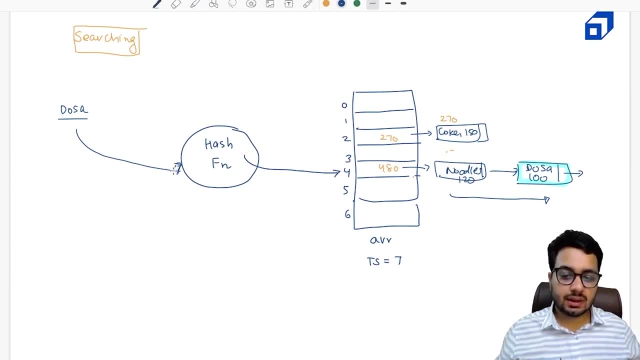 where the hash function is telling me: okay, in this bucket you have to check and in this chain, dosa can be present. dosa may not be present right now. you might ask: okay, if we have to iterate the chain, then what is the time? complexity of this operation. my answer is: it will be order of. 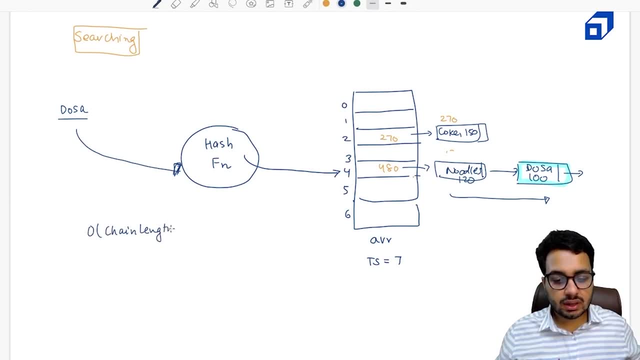 chain length right now. how do we figure out chain length? okay, can this chain length become very large? the answer is yes, it can become very large, right? so the key to successful search operation is that we have to ensure that this chain length is very small. okay, so we have to ensure. 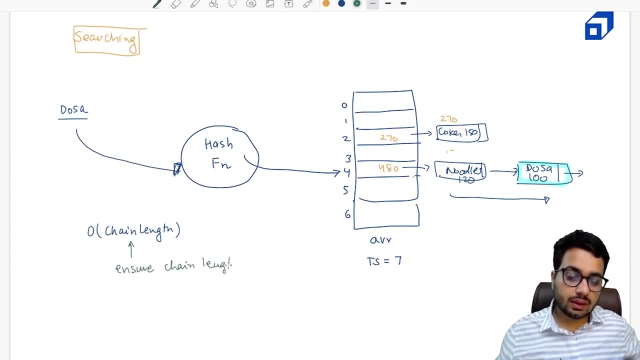 that chain length is very small, right, maybe two to three nodes, or maybe three to four nodes right, and this is achieved using a concept called as rehashing and load vector. so we will discuss this concept. ensure that the chain length is very small. so, if the chain length is very small, 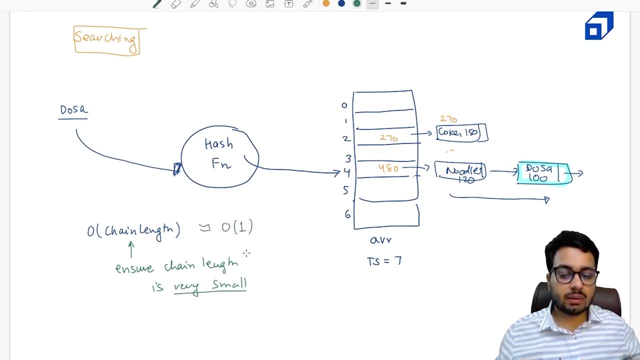 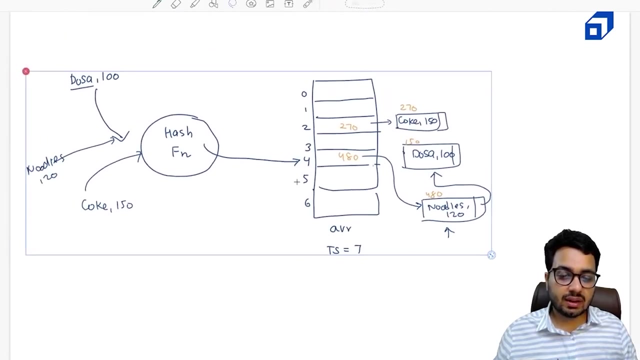 we can say: okay, on an average, this operation will be order one. maybe. i say: okay, the chain will have only three nodes, two nodes, right. but now let us discuss how this chain length will be decided. right, how this chain length will be actually decided right now, suppose i have a hash. 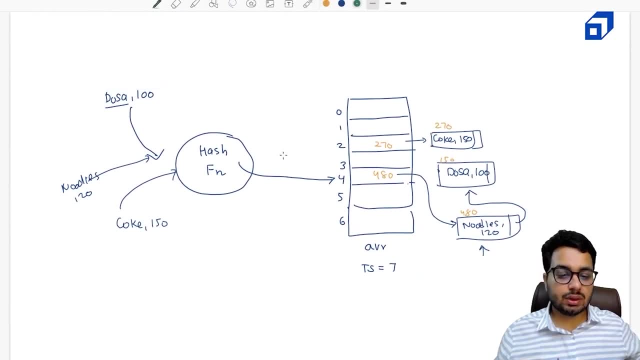 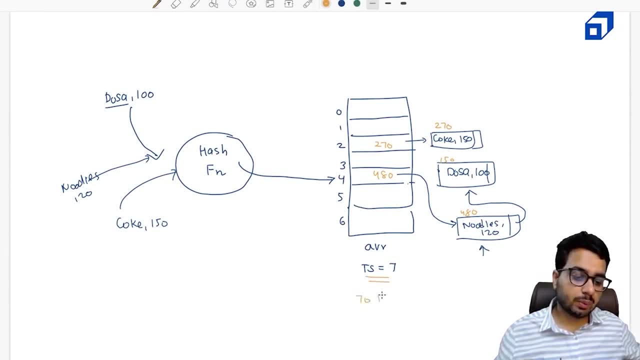 is seven and i insert 70 key value pairs inside it. right, what will be the average chain length if i talk about the average chain length in this case? so i can say, okay, i have done 70 insertions across seven buckets, so it will be 70 upon 7, that is 10.. 10 is a big number. i do not want to keep this much. 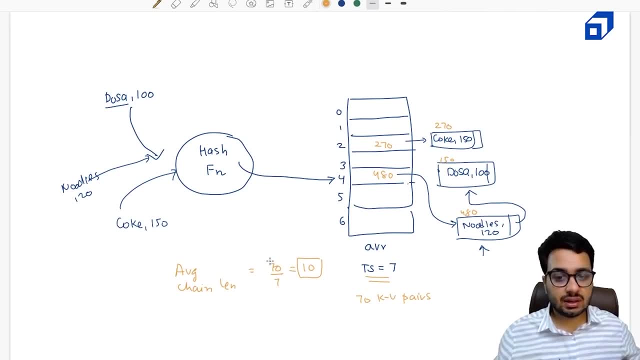 chain length, right, so this quantity that i have just written here, it is actually called as load factor. so load factor is a technical term for the average chain length. okay, so how do we compute load factor? so we say, okay, total number of key value pairs that have been inserted into the hash table. 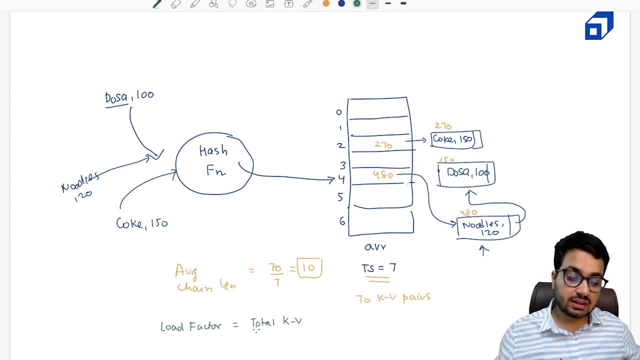 so total key value pairs i have inserted upon my table size- or in other words you can check current size- the number of key value pairs that have been inserted upon table size. that could be another way of writing it right, so i write this one. looks little more better to me. so in the current scenario, if you have 70 key value pairs, 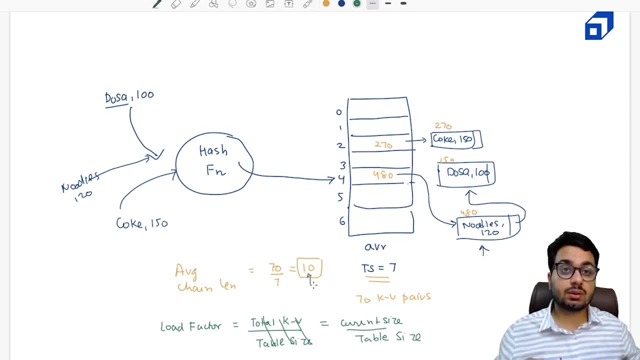 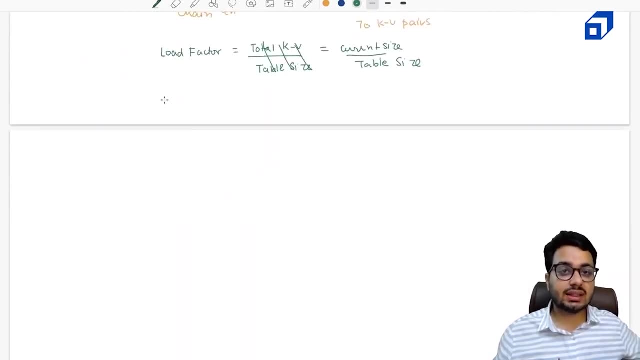 inserted in seven buckets. this is 10. it is actually huge, it's bad, right. so what do we need to ensure? we need to ensure that our load factor does not exceed a certain threshold, right. so in some languages it is one, in some languages it is point seven. so, whatever is the case, we need to. 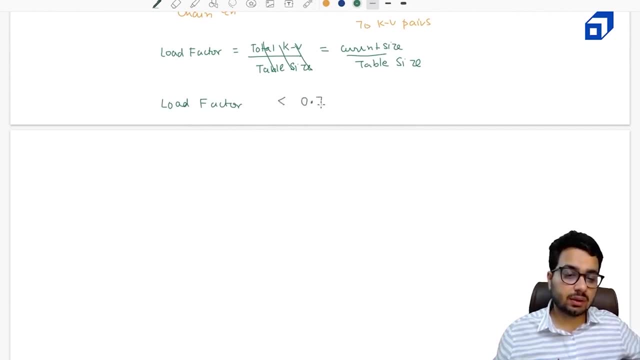 ensure that it does not exceed the threshold value of, let's say, 0.75. right now, what does it mean if i have, let's say, 10 buckets and i insert seven key value pairs? so what will be the load factor? it will be point seven. that means, on an average, every chain has less than one node, right so? 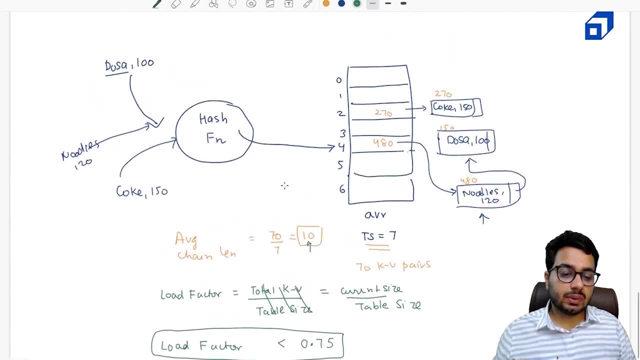 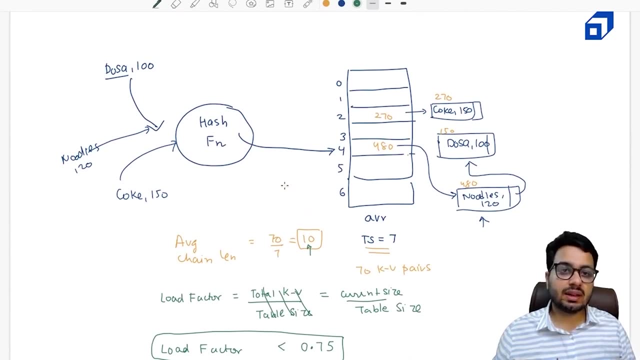 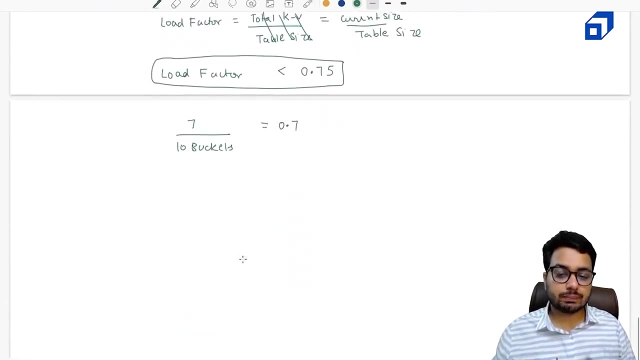 that also means that my table size will be slightly bigger than the number of keys i want to. so if i want to put, let's say, 100 keys, then my table size would be of the order 150, right? something of that sort, right? so that is something we need to ensure right now. how do we ensure that our table 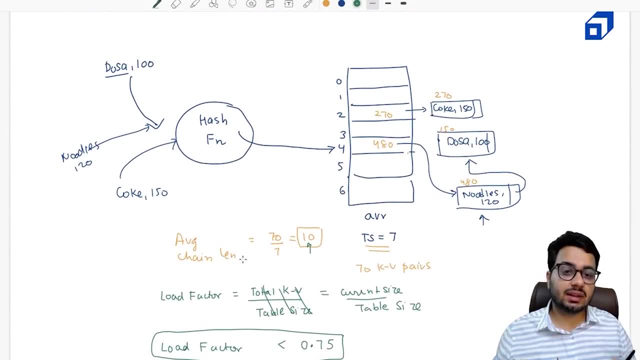 grows dynamically as the data in the table is increasing. right, one thing you can do is, if you have an idea that, okay, i'm going to insert somewhere around 70 keys, you can initialize your table size um around 150. you can insert about 70 key. oh, so that means i have more than one. 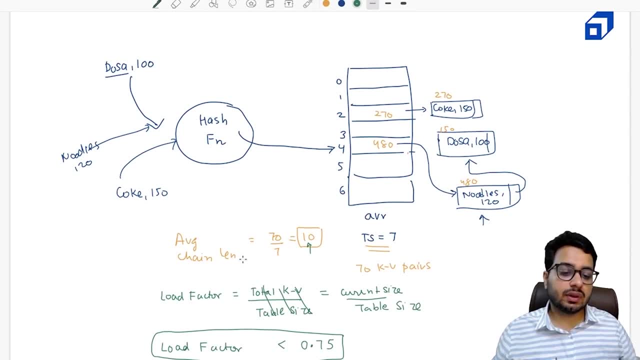 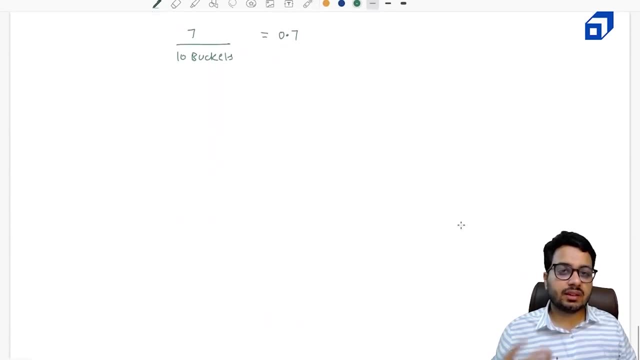 okay, so generally it is a prime number, right. so if it could be like 103, something of that sort, right, or 107, right? so you need to ensure that if it is a prime number, it it ensures a slightly better distribution, right of the keys, right? so what i'm going to do? i'm going to do insertions. 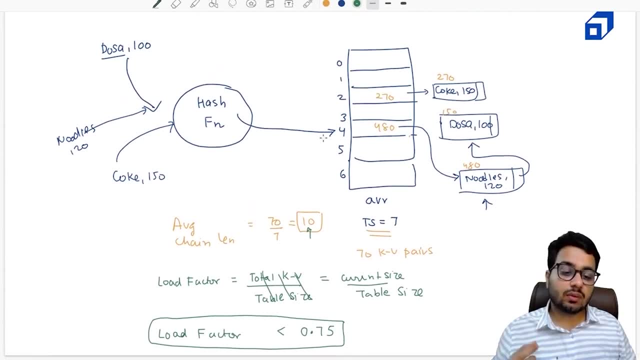 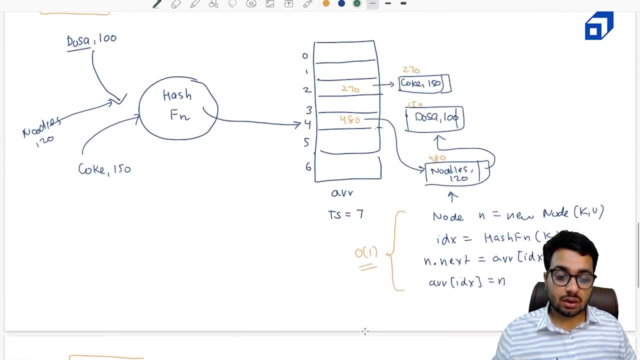 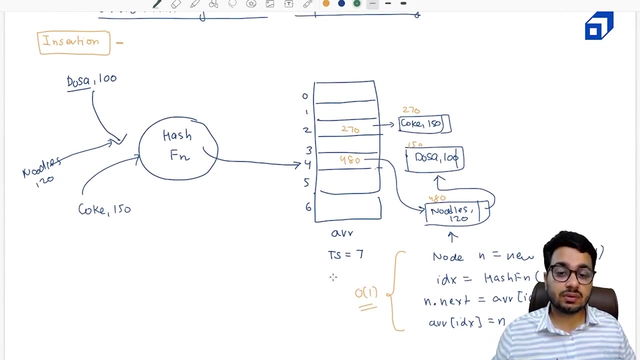 and i'm going to show you how the load factor is going to change and what happens if the load factor exceeds the certain threshold. so, going back, i'm going to discuss the insertion logic once again. and now, apart from doing the insertion in the chain, we will also discuss the concept of 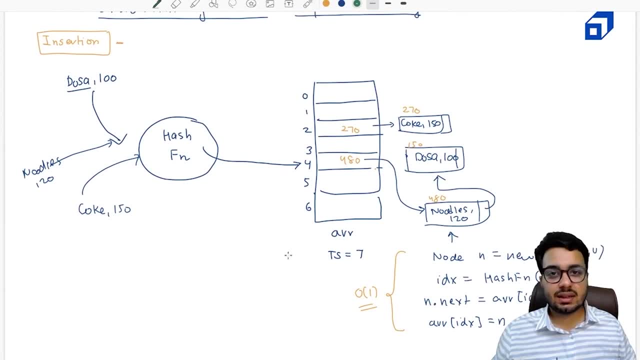 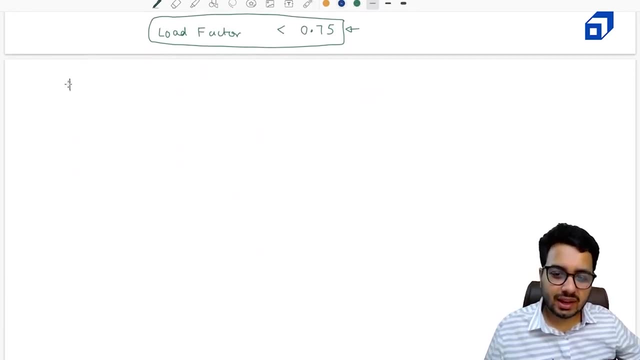 rehashing and how do we increase the table size dynamically? let us talk about rehashing according to the load factor. let us talk about rehashing right. so rehashing is a mechanism that is going to help us expand the table size and bring down the load factor. let us try to understand insertion and rehashing. 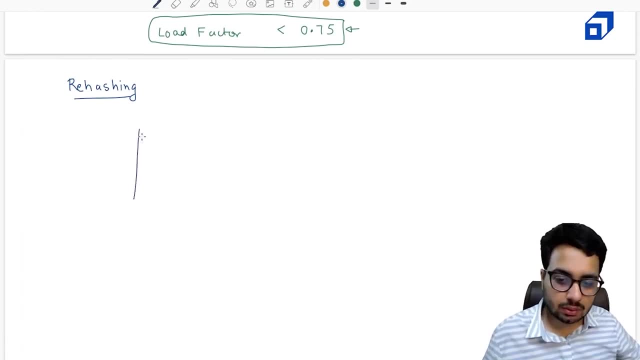 procedure with the example. okay, for example. now suppose i have a table which is of size 7: 0, 1, 2, 3, 4, 5, 6. right now i'm going to insert certain key value pairs inside it and i will calculate the load factor during the insertion process. for example, i insert a right, so the 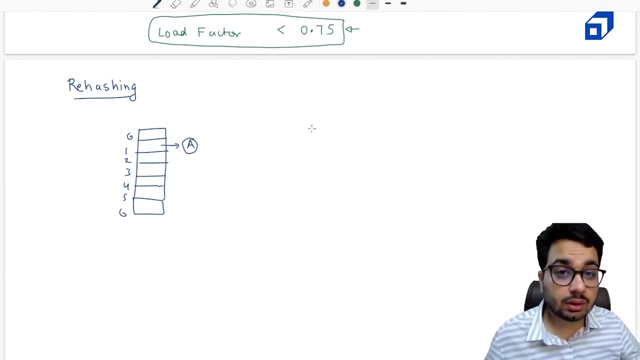 locations are decided by the hash index. so now the load factor will be 1 upon 7, which is 0.14, right, which is well below the threshold. okay, so our threshold is, let's say, 0.75. so it is below the threshold. i will not do. 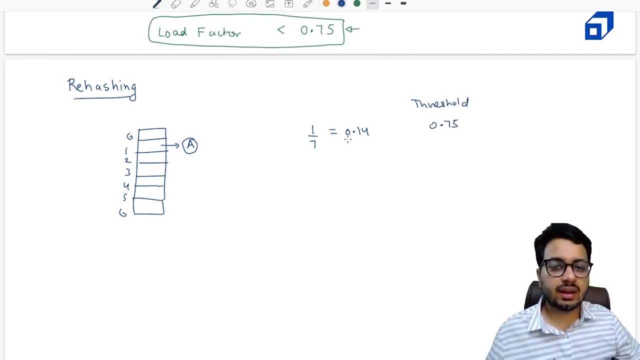 anything. that means on an average, every bucket has 0.114 elements inside it. right, if i say okay, i will insert b, maybe it goes here. now my load factor is 2 by 7, which is about 0.28. right, then i insert c. maybe a collision happens and c goes here, but then on an average, each bucket has now. 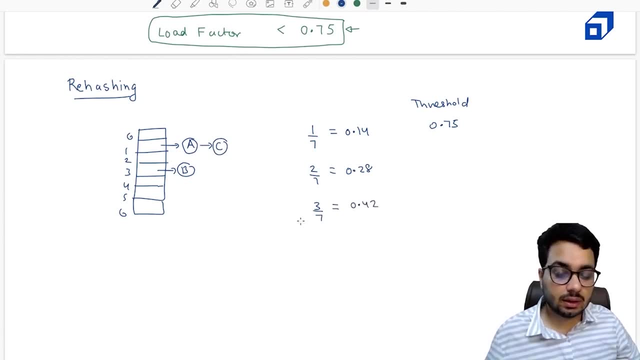 0.42 elements, so it is 3 by 7. that is my load vector, right, and maybe i insert d, so it's going to be 4 by 7, right? so it's going to be around 0.56, right, so it's it's around 0.57. 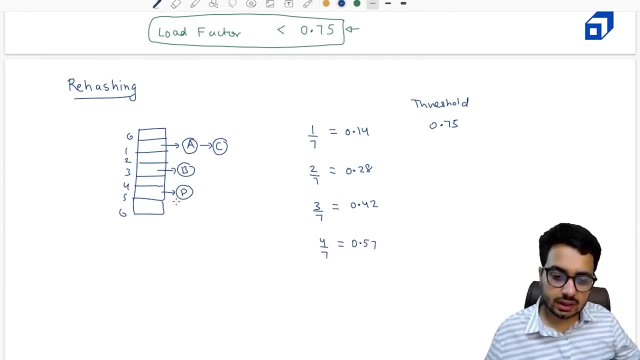 on the calculator. and similarly, if i insert, let's say, e, maybe e goes here right, so it is five by seven. it's going to be around 0.71. it is still below the threshold. then if i insert the sixth element, maybe f, it goes here and it collides right. so it's going to be six by seven, which. 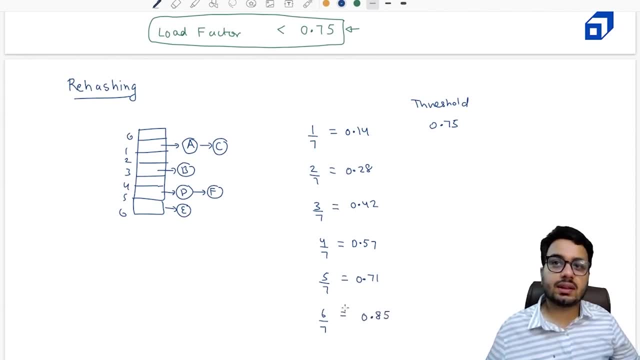 is around 0.85. now, at this point, what do i see? i see that the load factor right has reached 0.85. that means it is close to one. that means, on an average, every bucket has around one element. each is the time to grow the table right. so what is the table? this is my table. i want to grow this table. i. 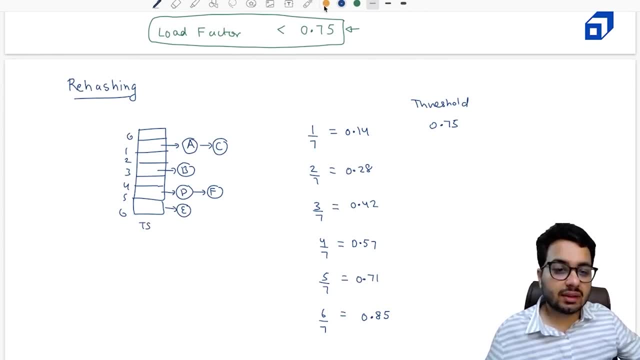 want to make it bigger, right, what i will do? i will create a new table or a new array, right, which is approximately double of the given size, right? so maybe this table size was seven. so i generally look for a table size which is a prime number, right? so this new table size could be, let's say, 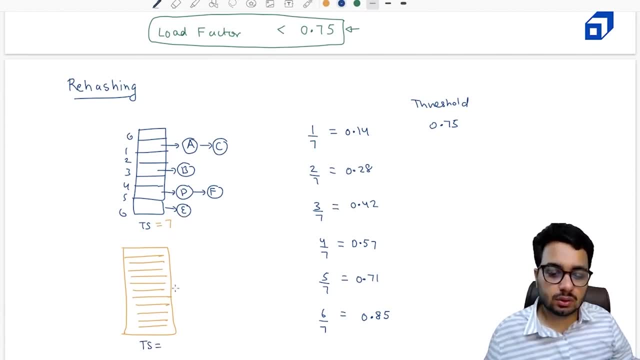 7 into 2 is 14. what is the nearest prime number, close to 14? it could be 13 also. it could be 17 also, let's say this is 17, right? so i'm taking the next biggest prime number right now. what i 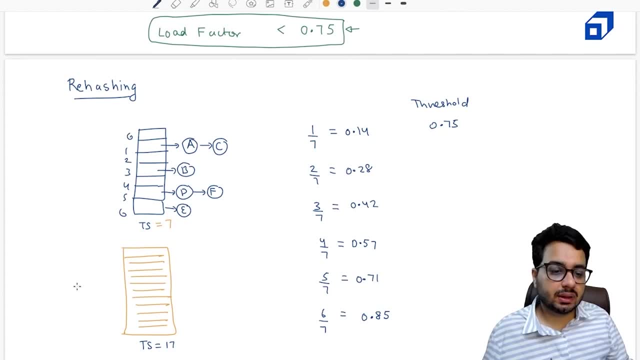 will do. this table is empty, right, this table is empty, and my goal is to remove all the entries from this hash table and put it into this hash table. now you might ask why can't we, uh, use this hash table, right? the reason being, um, your table size has changed and your hash index 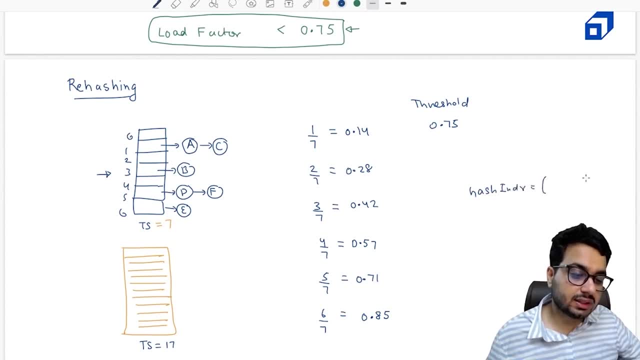 that we saw right. so we saw it was a weighted sum. okay, it was a weighted sum of um, the letters of the string taken with, taken mod, with the table size. now table size has changed so my hashing will also change. that means if i now insert a. earlier it was going at position one. it might go. 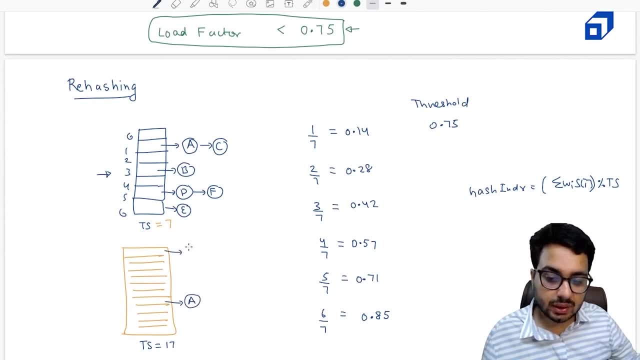 at certain some other position. so a might go here, c might go here, b might go here and d might go here. and since the number of bucket they have also increased, that means my distribution will also change and it is possible that the number of collisions that are happening they might reduce. right, so what i have to do, i have. 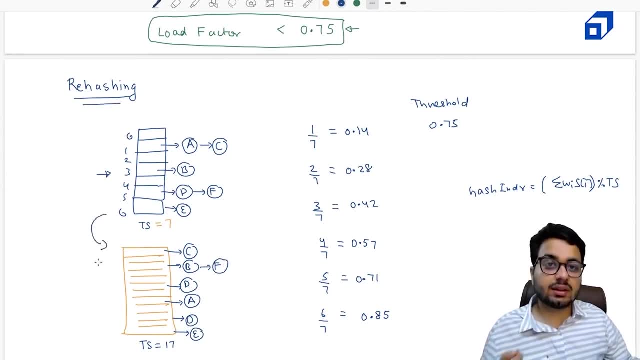 to do rehashing. so this is what rehashing is. so we have created a table of size, double the capacity, right, and we, we iterated over every chain in the original table, every node we added again into the ninth. uh, use buffer. ok, todas, okay. so by using warfare we are going to directly Ef. 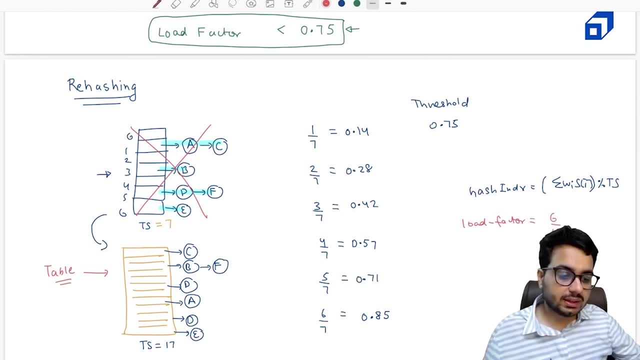 this means this: i will be playing a steady to all my shots, train resh, command to. and if here i say Vous, i am the disk. this network is 6 upon 17. this value comes out to be 0.35, 0.35, right, so i can keep on adding more entries into. 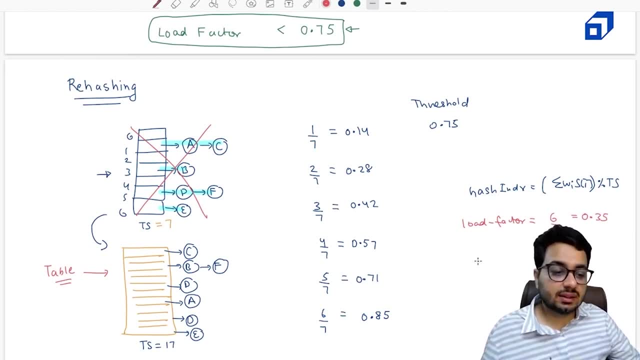 this table right again if again, it exceeds the threshold. what i will do? i will execute rehashing once again right now. what i'm trying to say is that this rehashing is a special mechanism that will be triggered from the insert method when my load vector exceeds the certain threshold. 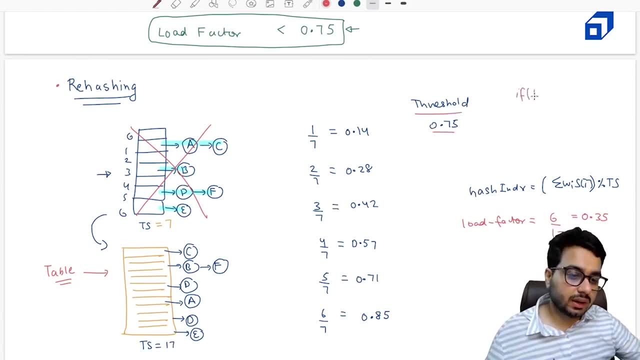 right, so it will be some condition like: if my load vector exceeds the certain threshold, i will have to call the rehash method from the insert function, right? so this is something i will show you in the code as well, right, but i hope you're understanding the reason of rehashing, right. 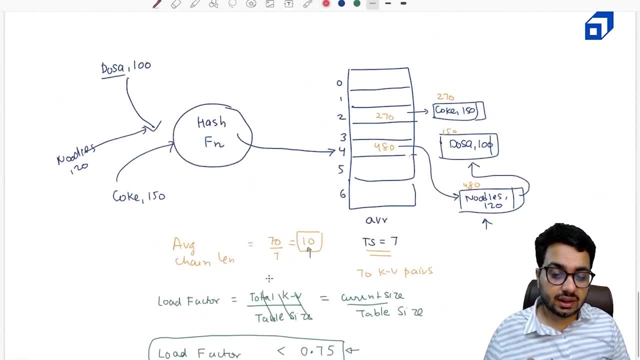 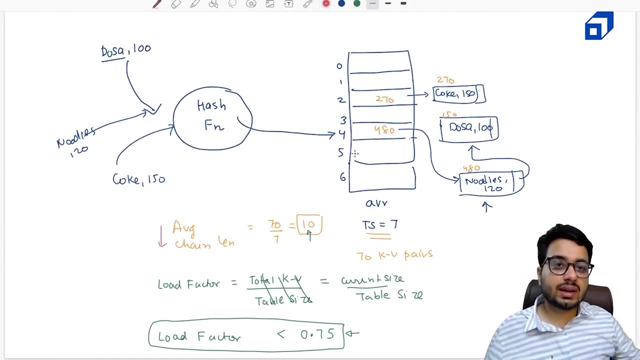 what is importance of rehashing. so if you have done rehashing right, can i say the average chain length will be always less than one. that means, on an average, no bucket has more than one node right? so it might happen that some buckets may have zero nodes, some buckets might may have two or three nodes, but i'm going to say this: 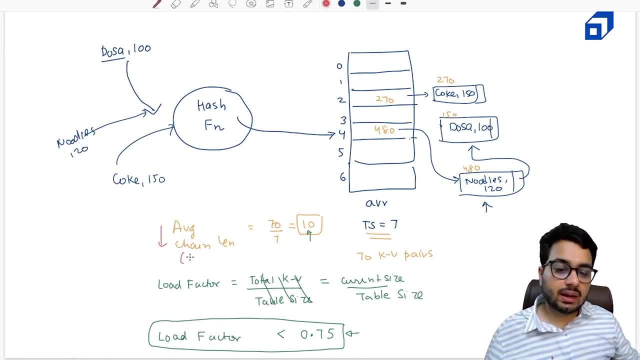 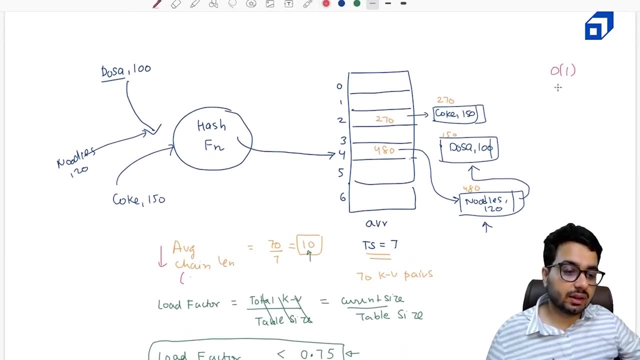 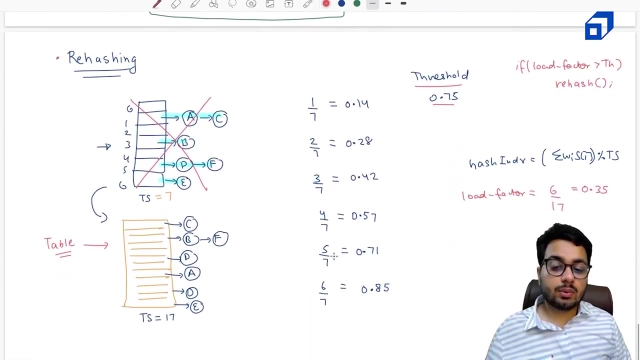 average chain length will be a very small number, and it it is, it can be treated as constant. so that is why we say that our search is order one on average right, order one on average right. that is what what my search operation will be right now. another point: what is the complexity of? 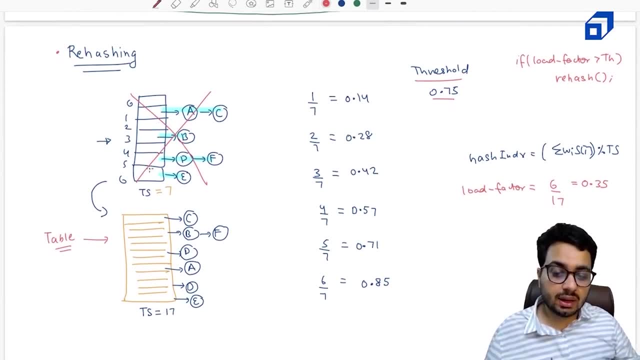 rehashing, right. so of course we have to iterate on the entire table and put all the keys into the new table, so it is going to take order of n time, right then, how my insertion can be order of one. so, if you look carefully, this rehashing is not happening again and again. so it is happening. 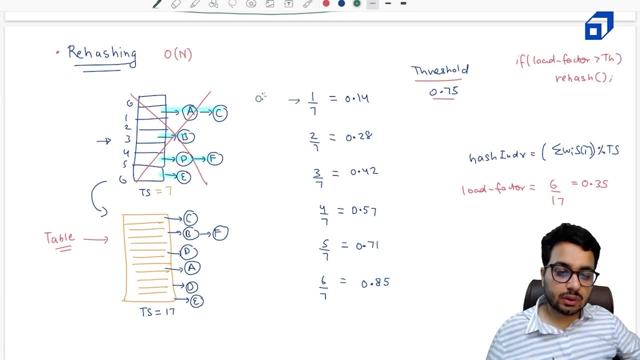 once in a while. so you inserted this element, you took order one time this element. it took order one order one time. order one time. order one time. and at this point we saw that load vector is increasing and it is going to trigger the rehash function, so it is going to hit order of n time. 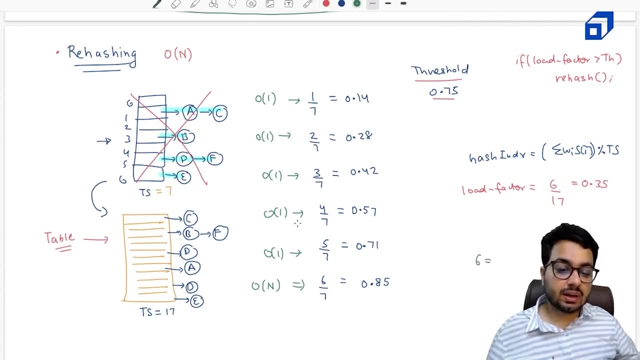 right. so can i say that for six elements i spent it constant time, but for one element i spent order n time, right? so if i talk about on average how much time i spent on each element, so again if i take an average, it's like a worst case. right inserting six is like a worst case, worst case. 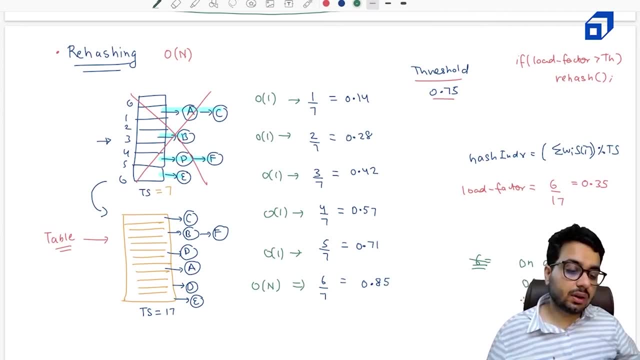 it can go order of n, but on an average we are spending order of one time in doing an insertion. right, you might ask how can i bring down the time of rehashing? so if you know that, okay, i am going to insert about 500 keys. so you make sure in the beginning that your table size is big enough. 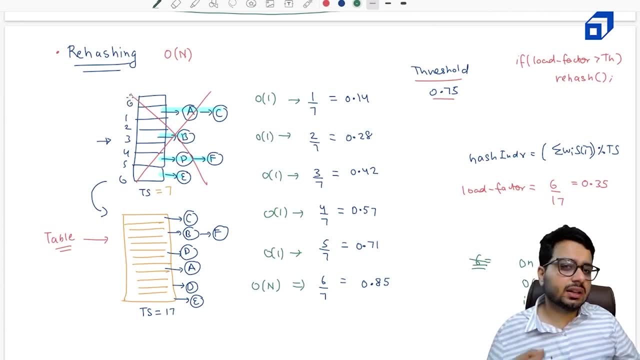 so that rehashing is never triggered, okay, or it is triggered very, very rare, right? so the correct thing is that if you have a large enough table, okay, it should not be too big, that you are using too much of memory, and so you have to make a balance between effective memory, memory utilization. 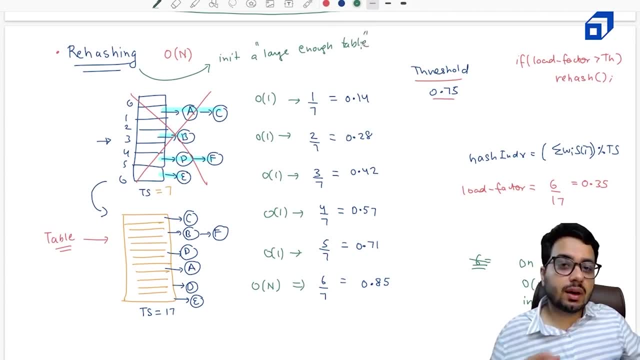 so you should know from the historic data, okay, how. how big table should be sufficient. so if you are storing phone contacts, you know in general people might have 500 to 1000 contacts, so you can initialize a table of the size around 1000, right? so it is just large enough. just large enough. 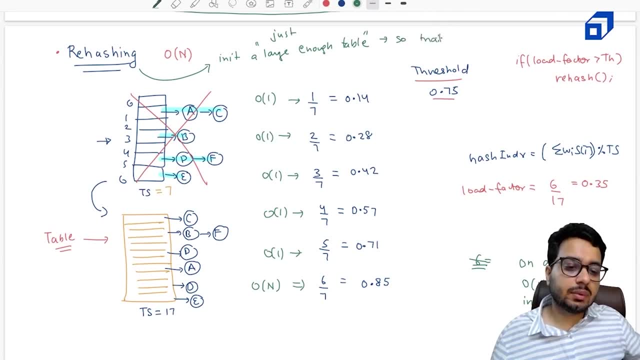 so that rehashing is never triggered, right, or it is triggered maybe just once, right, it is never triggered, right. so this is something we can do, right to make sure that almost every insertion is order one, right. so i hope you understood the concept of rehashing and i'll 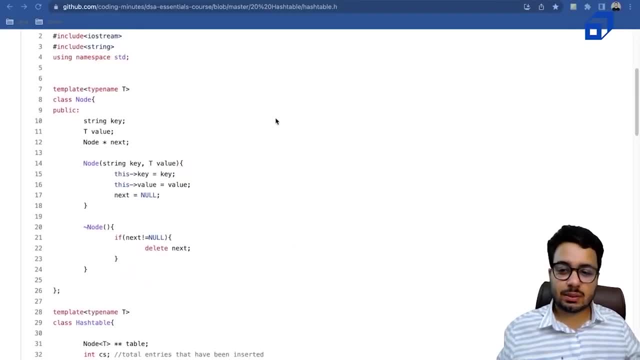 show you in the code as well. let us discuss the implementation of hash table. so i'm using c plus plus, but you can also use java or any other language to map the same functionality in in your own language, right? so first of all, i discussed that hash table is a table and in this table is going to: 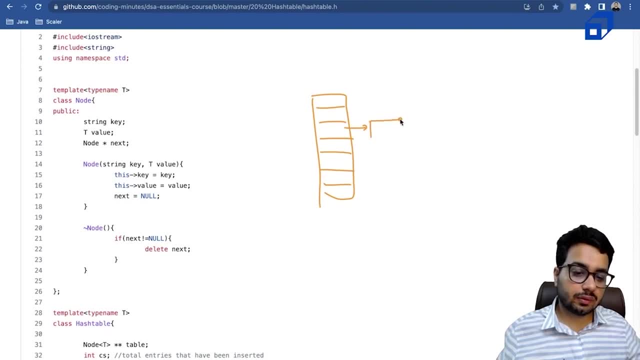 contain the address of it. it is going to contain the head of the link list. so link list is made up of nodes, so node will store key, a value and the next field, right. so that is what i've defined in the node structure. so i'm using templated classes, so it's like generics in java and 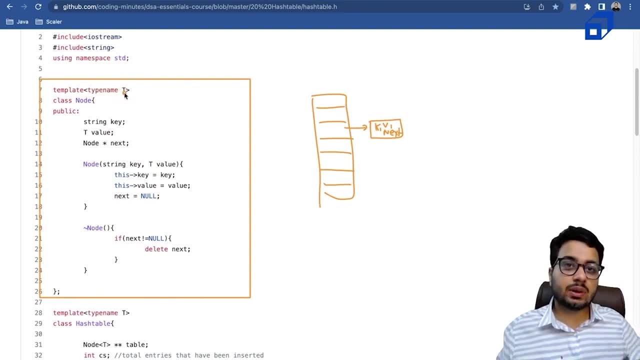 templates in c plus plus. these templates allow me to hold data of any t type in my node. right for keeping things little simple, i'm assuming that my key is always a string, but it can be of other data types as well. for that also, you need to. 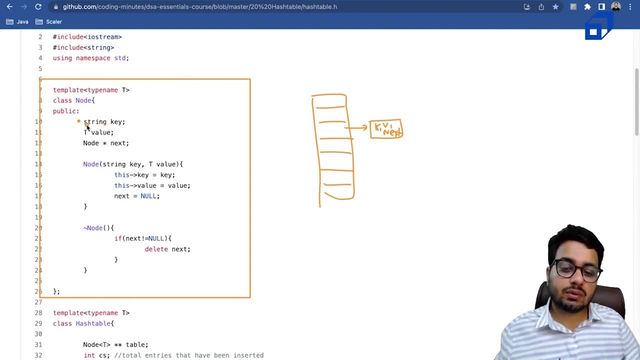 use templated classes and you need to provide a way to convert that data type into a hash index value, right? so for now i'm dealing with strings only, but i'm saying the value can be of any type. it could be end, it could be string, it could be float, because we are not computing any hash on the 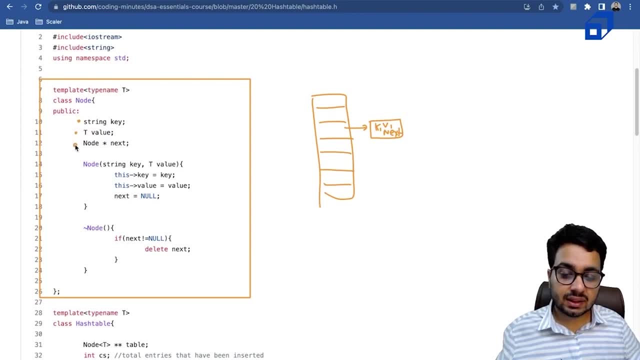 value. we are just going to store that value as it is. and third thing is the next property, that is of the node: right, whenever i initialize the node, i set the value of key, i set the value, which is the value, and by default, i set the next as now. right, and this is my constructor. 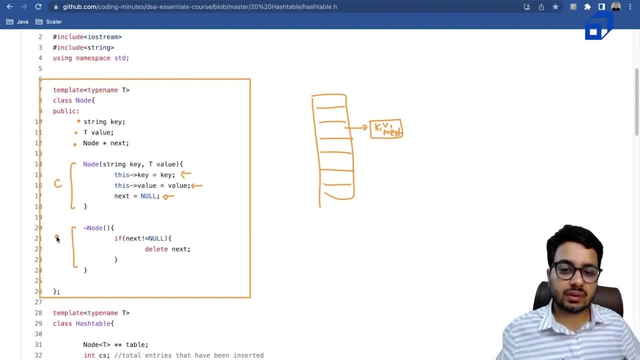 and if i want to delete a node, so this deletion will happen. if i am deleting a certain value or i'm doing rehashing and i want to delete some data, right, this is actually a destructor which says that next is not null, delete next. so basically it is a recursive way of deleting the node right, so that 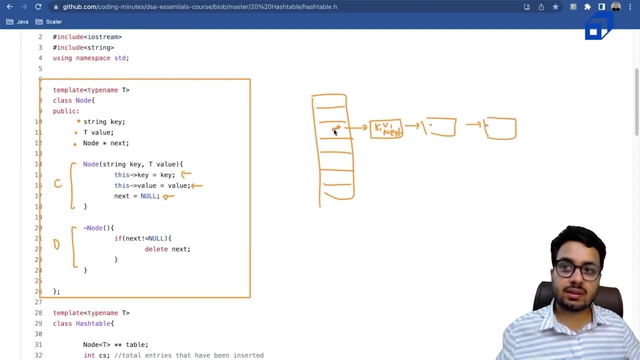 means, if i uh make a call at this point, it says: okay, if i'm going to delete this node and if the next is not null, first delete it. if the next is not null, first delete it. so it it's a way in which i can delete the entire chain at once, right? so this is something, um, which you can also like. it's. 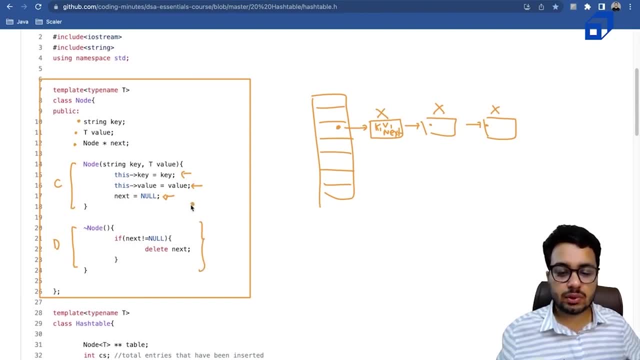 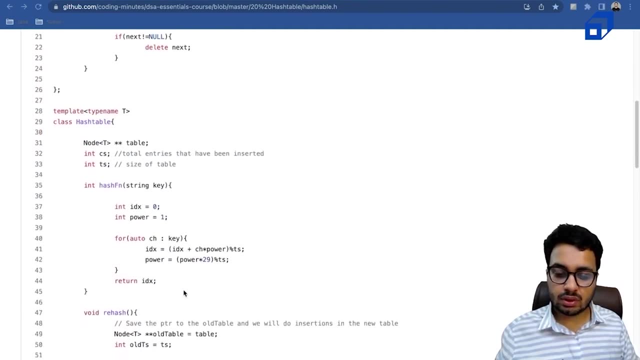 uh, it can be implemented in other way also, right, so, you might not necessarily do the same thing, but in my case i'm doing it. i will tell you why, right so? uh, that is about the node constructor. and now let us come to the hash table class. right, what i have done, i? 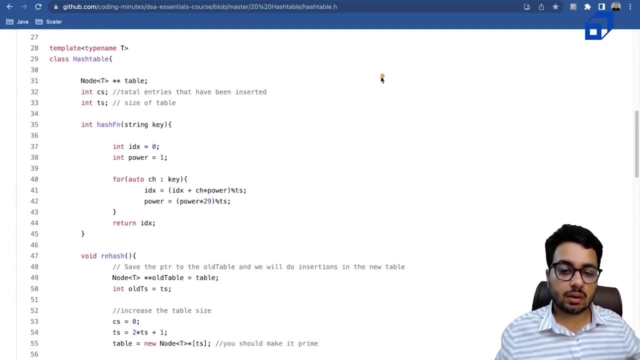 am actually keeping a two dynamic array called table. so table is referring to an array, right, you might ask. why star star? because, see, uh, each, each bucket in this array is going to hold an address of the node, so it is of the type node star, right. and what is table? table. 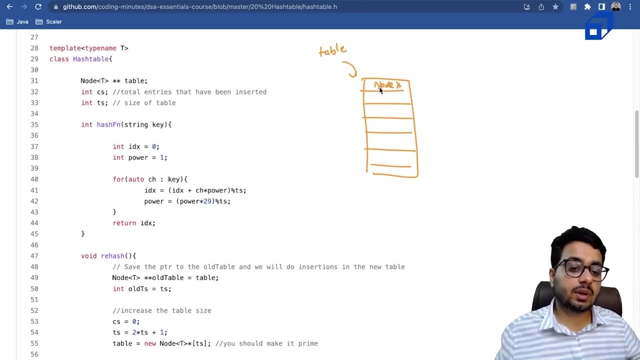 is a pointer to an array of pointers, right, because each bucket is going to point to the head of the linked list. so each bucket is of the type node star. hence the type of the table is node star, star. right, it is going to be a dynamic array referring to an array of pointers. okay, so i have a table. 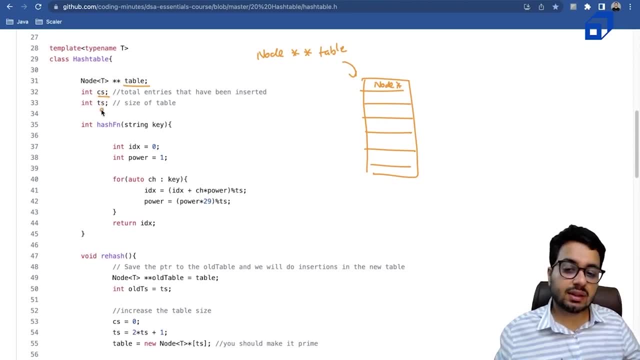 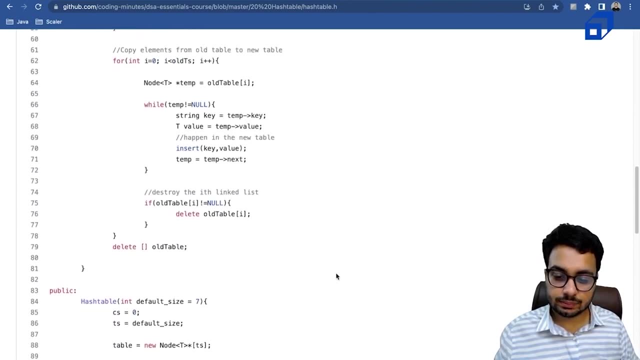 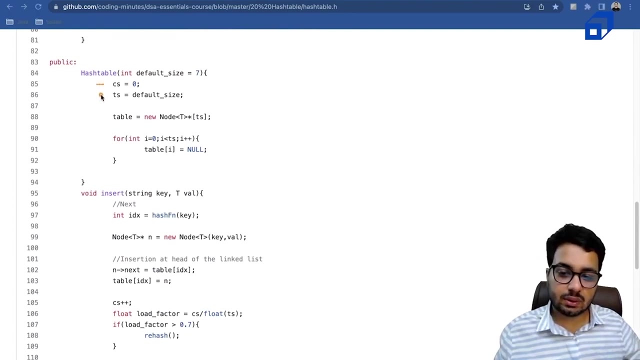 which is not initialized at the moment. i have current size, i have table size, so current size will be zero in the beginning. so i will show you, uh, the constructor for this. yeah, this is the constructor. so whenever a new hash table is created, right, so current size is set to zero. table size is set to default size. 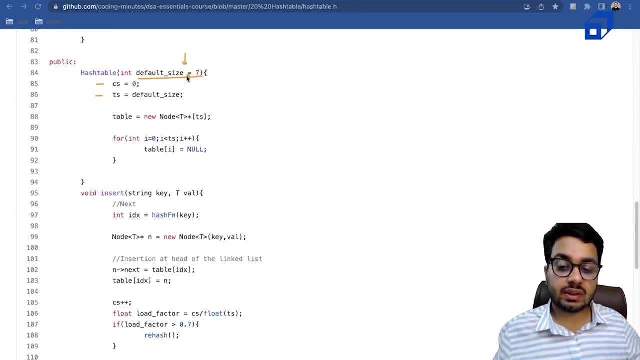 i'm taking a parameter with the default value of seven. so if user gives me, let's say, i want a table size of one zero seven, it will be one zero seven. but if nothing is given by default, i'm taking it very small and it is seven. right, then i initialize my table array. 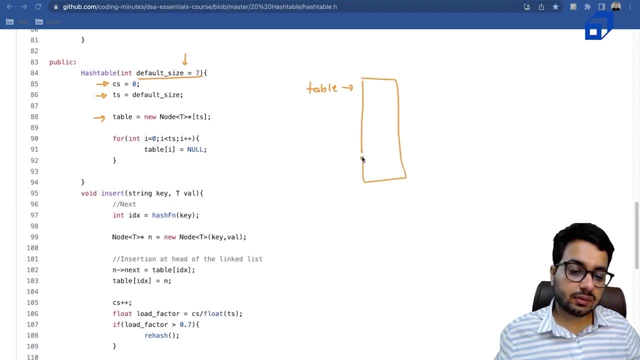 so table is an array that points to an array of node star and this is of size, table size. so these many buckets i have initialized, and by default in every bucket i am putting a value null right. so this is null, this is null, this is null right. so instead of having garbage it, 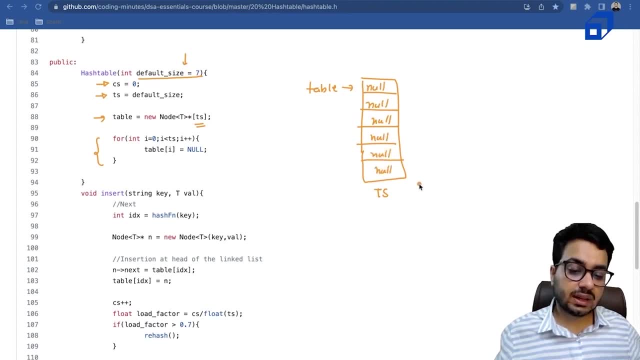 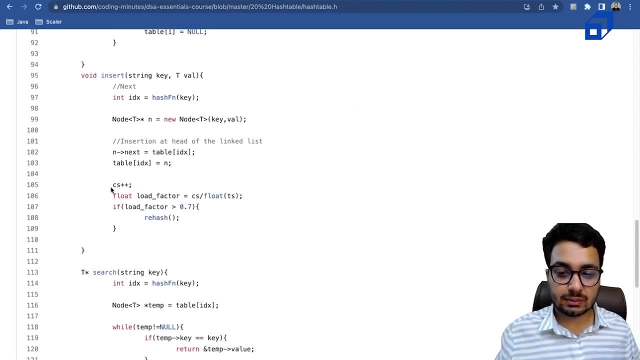 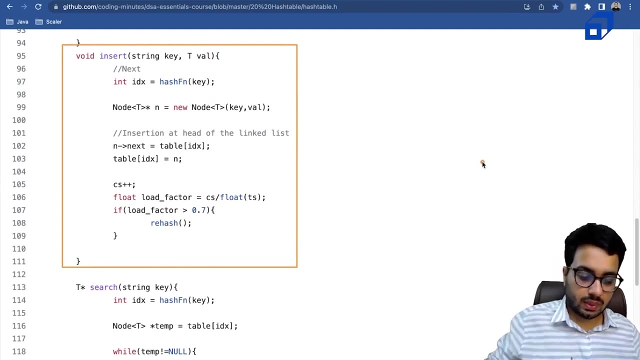 is better to initialize everything with null. that is how that hash table has been initialized. i hope you don't have any doubts till now. now comes the interesting method, that is, insert right now if i want to insert something right. so my table is ready, so table is here, my hash function. 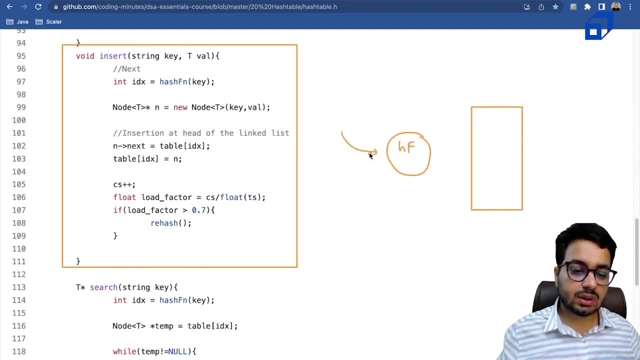 is also ready. okay, i'll show you the hash function. let's say i want to insert dosa, comma hundred. what do i do? i will show you the hash function. let us understand the insert. so my key that is dosa. it goes through the hash function and i get an index. so maybe the index is. 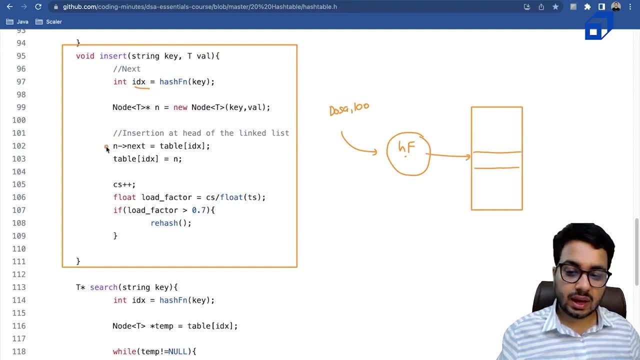 four, right at this index, what do i do? i will create a new node. so i say okay, there is a new node called n, which is dosa comma hundred. in this line. i do this work and i say n dot next. this is equal to table of index. so table and this is index. so n dot next will point to whatever this. 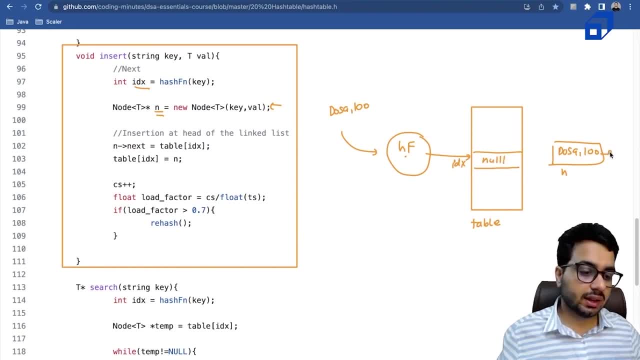 is pointing to. so it is currently pointing to null. the next starts pointing to null, right. then i say: table of index is equal to n, so this index is going to hold the value n. so n is, let's say, two, four, eight. that is the address of this node. so 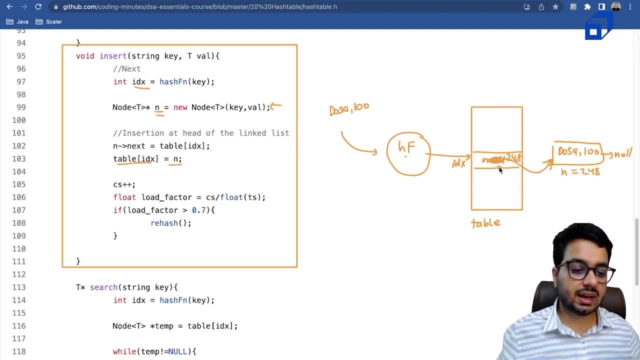 it is going to store two for it, right? so this is how this node gets attached to the beginning of the table: current size plus plus. so current size becomes one. then i compute load vector, so which is one upon seven. is it greater than point seven? the answer is no, right. so if it becomes, then i 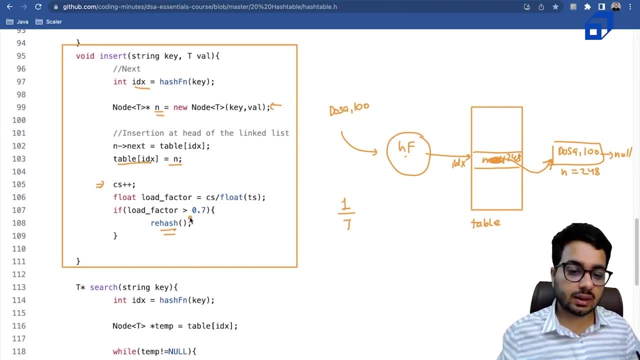 will trigger rehash. i will show rehash method also. right, so this is about the insert functionality. i hope you are getting it. let's say i'm inserting one more node, which, at the index, four. so i just want to show you how the chaining is going to work. let's say i inserted noodles, and for noodles also. 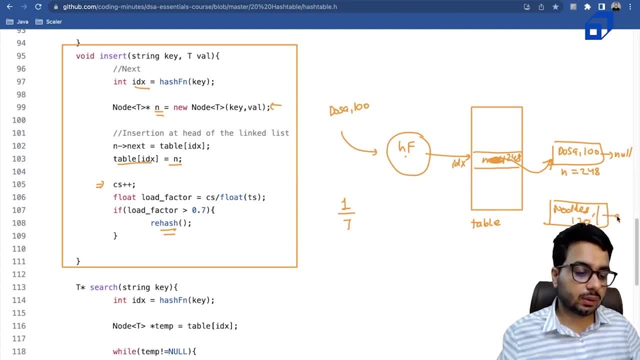 i got an index four, so noodles, comma 120, i created a new node called n, right. then i said n dot next is equal to table of index. table of index is storing this value, so noodles starts pointing to this value, right, and table of index is equal to n, so this connection is broken and this starts. 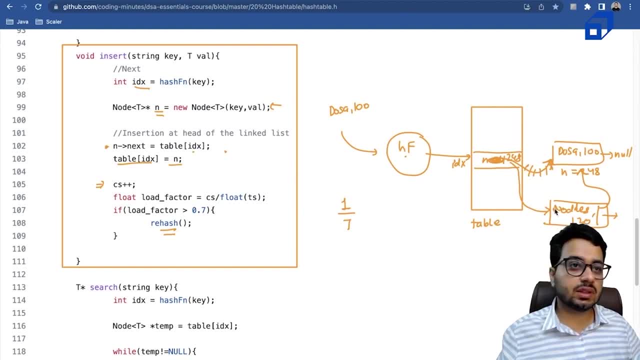 into this node, right? so you can see, in a way we are forming a chain in which noodles is getting inserted at the head of the linked list, right? so this is nothing but insertion at the head of the linked list. current size plus plus. so current size is two. load vector is two by seven, which is again. 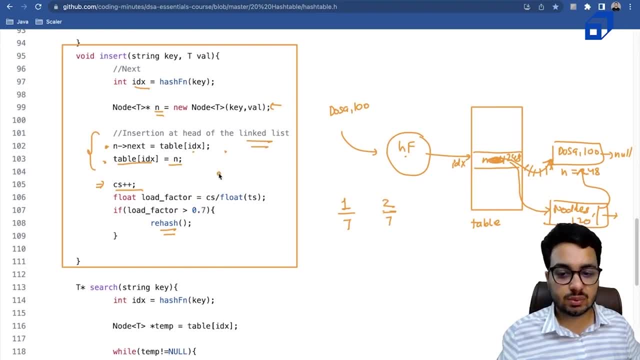 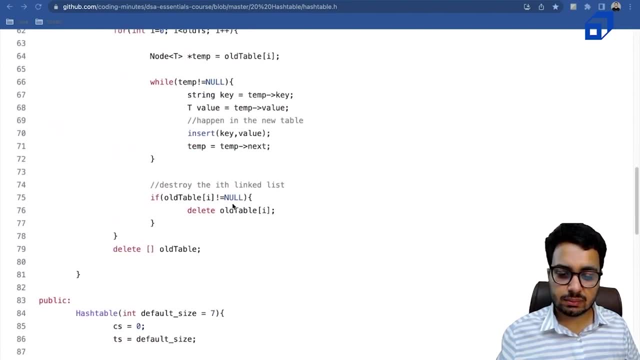 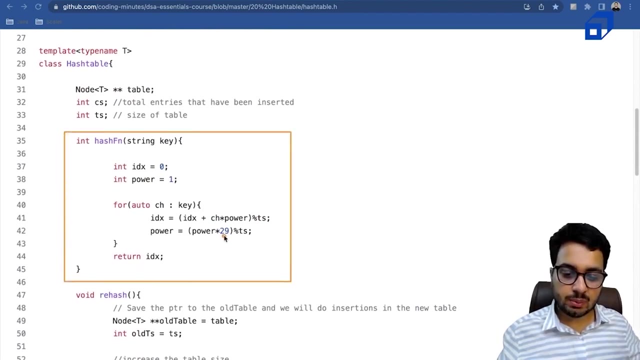 less than 0.7. so hence i do not trigger rehash at this moment. right, so i hope you insert. you understood the insert method. next, i want to show you the hash function that i've used here. the hash function, i've made it as a private, so what i'm doing, i'm simply multiplying the numbers. let's say: 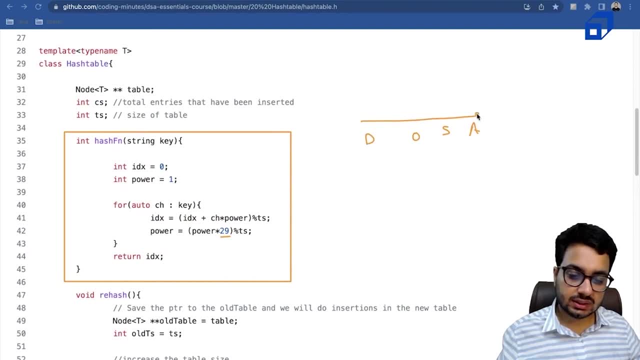 the word is dosa. what i'm doing, i'm iterating over this and i'm multiplying it with powers of 29. so it is one. so initially it is multiplied with one, then in the next iteration power becomes into 29, into 29. next time it becomes, power becomes again power into 29. so it gets multiplied with 29 square. 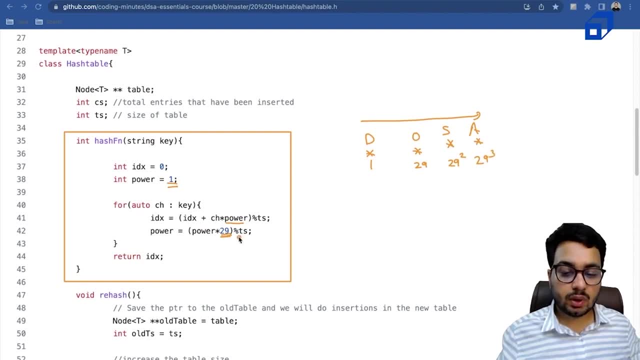 and again it becomes 29 cube right. so, in order to avoid overflow, i am doing a percentage mod at each step, because if, if you take mod at the last, uh, or if you take mod at each step, you know this is the property of mod, so mod can be taken at each. 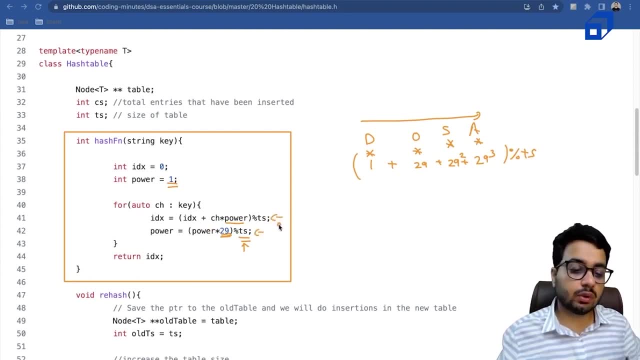 step as well, so this is a better thing to do because it helps us to avoid overflow. right? i'm taking a mod with power also and i'm taking the mod in the answer also, so i get an index which is in the range zero to table size. 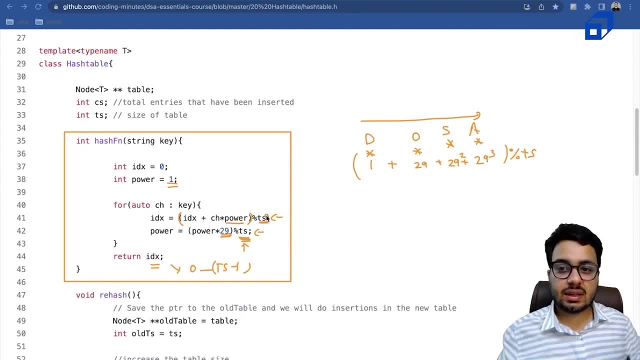 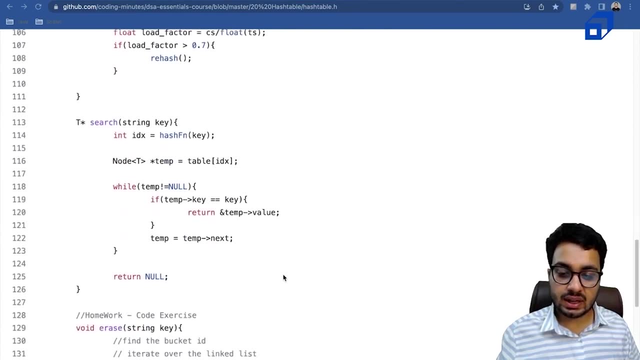 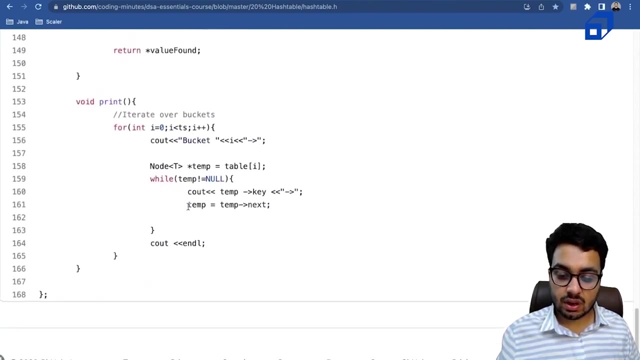 minus one, because i'm doing a mod with table size. so i hope you understand the hash function as well. right now, what i need to do is i need to understand the rehash method right. so if we understand the rehash method, our insertion will be complete. so i have written a rehash method as. 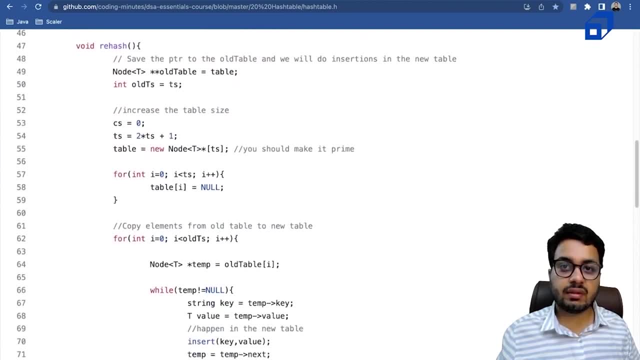 well, which is actually a private method as well. so what i'm doing in my rehash method? that suppose i have a old table, actual table. in this i have inserted some keys, let's say a, b is there, c and d is there. what do i do? i say, okay, old table is going to point to table. so this was my table. now, old table is. 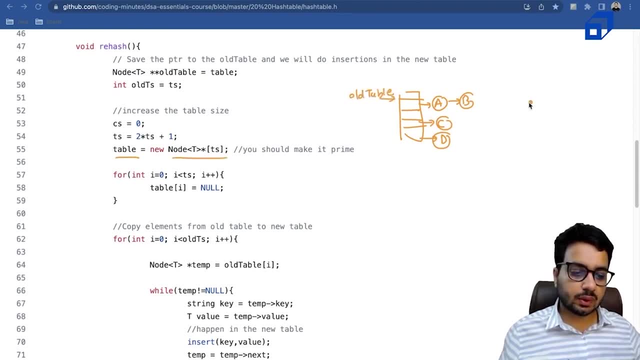 pointing to this table. i create a new table, okay, which is almost double of the previous size, plus one. i'm just making it as a odd number instead of making it as a prime number. so i'm saying: this is my table now, which is also the data. member of the class. right. 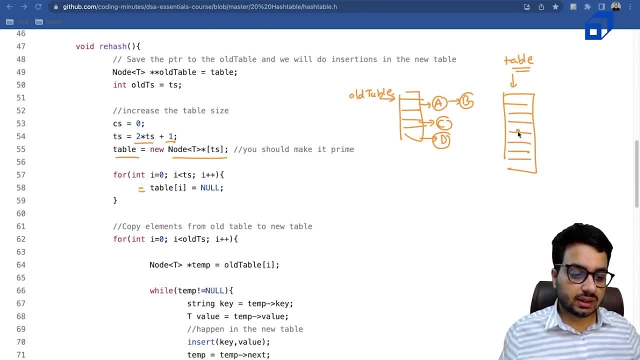 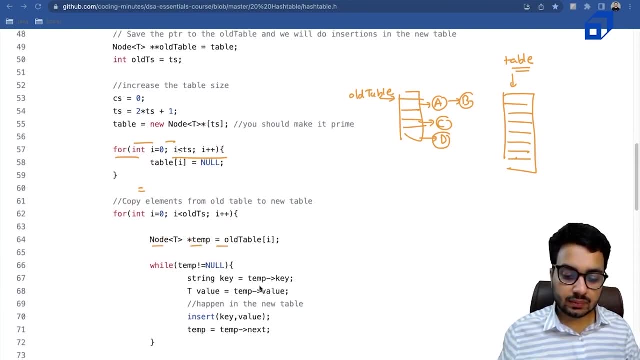 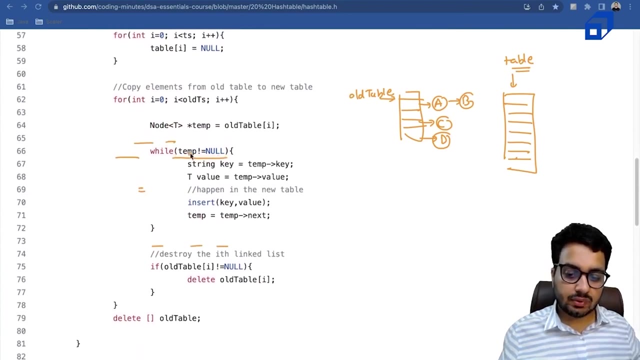 so what do i do? i initialize it with null, so all these values are set to null. and then what i do? i copy elements from the old table, so i iterate over the old table. and how do i do do the work? let me show you. so i do do it like this: i take a temp variable, which is the ith row, so temp starts from. 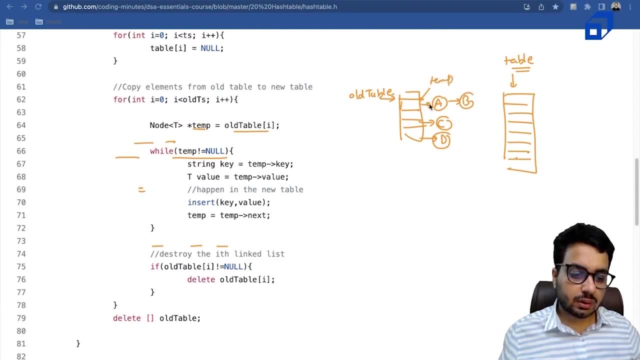 here. okay, temp is referring to the head of the linked list and while temp is not null, so i copy the key, i copy the value, so i say, okay, give me this key value pair and i call the insert method. so insert method. we know, by default it acts on the table, which is the 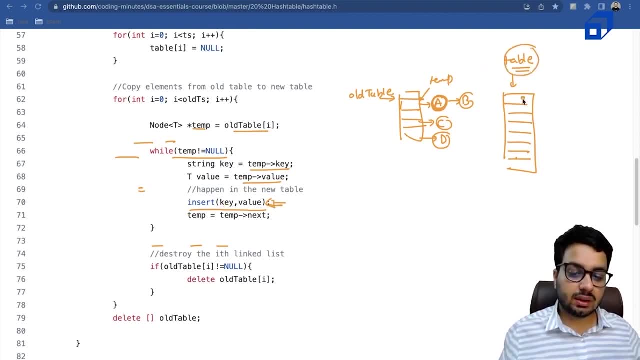 data. member of the class. so it is going to insert automatically in the new table right and temp goes as next. so temp comes to this node again. i copy b i and insert it in the new table right. so once it is done i make a destructor call. if old table of i is not null, delete old table of i. so in java. 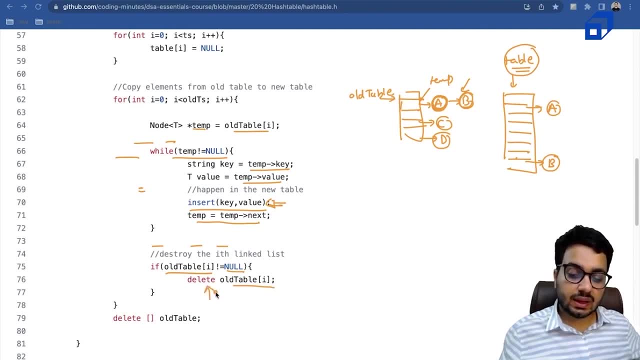 took garbage collection. but in c plus plus, we have to use explicitly, we have to invoke uh, the destruction of this or this entire link list by saying delete old table of i. so i initiate a destructor call from here which makes a call to a. is being it being a recursive destructor. a makes a call to b. this way, this entire row is deleted. 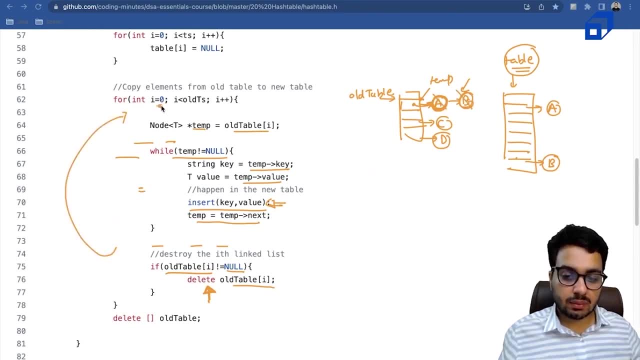 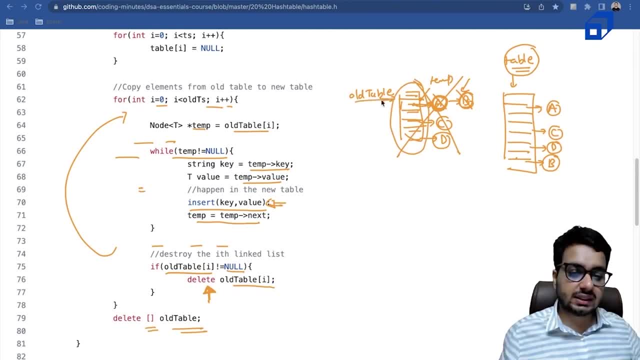 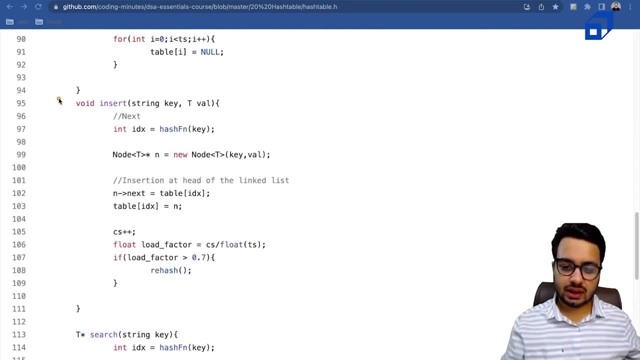 so i say: delete old table. this old table is gone and since it is a local variable, this is also destroyed, right. so till now you have seen the insert functionality and we discussed that. uh, the function rehash will be triggered from the insert whenever load factor exceeds the threshold. 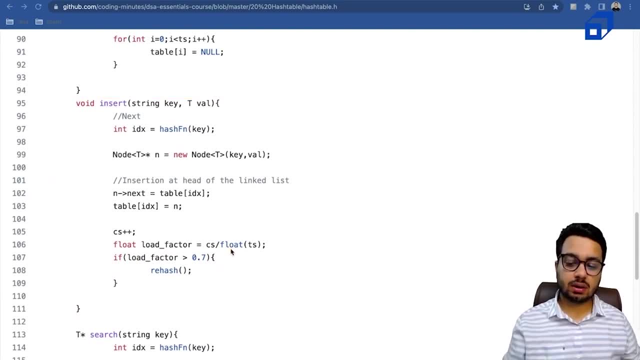 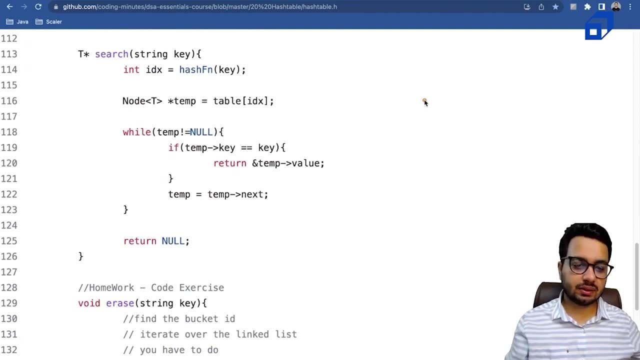 okay, so we basically double the table size here right now. let us talk about searching a little bit. how do we actually do searching in a hash table? so searching is pretty easy. so if you have a hash table right and you want to search for a certain key, let's say dosa, so that key will go through the 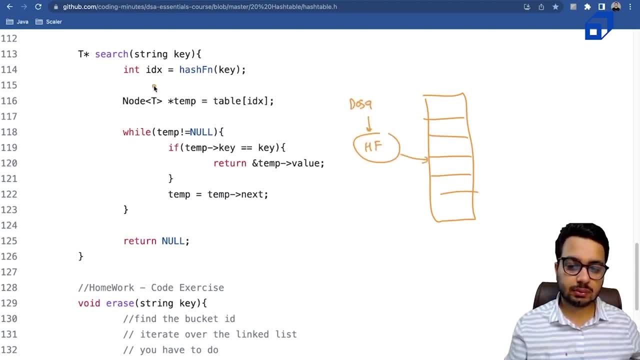 hash function. the hash function will tell you the bucket. so maybe this is the index of the bucket and in this bucket there might be a chain in which dosa could be one of the item, right? so maybe this is some x item, some buy item, some red item. so you need to iterate on this chain linearly, right? so 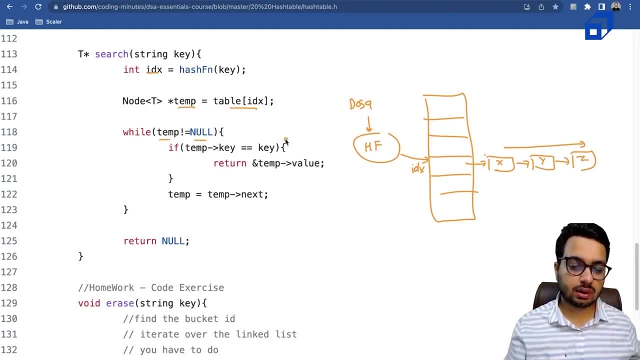 i start temp from this node while temp is not null, while i do not hit the end of the chain. i compare: is the key of this node matches with the given key? if i'm that, i'm searching. so if that happens, i return the value. otherwise i go to the next node. if i hit end of the chain, that means 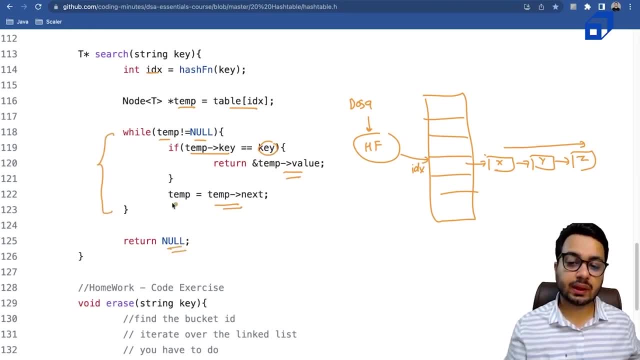 i would not found the key, so i return null. in that case, right, this is how searching is done. right, so, on an average, what we are saying? that this chain length is so small? right, because of the rehashing and the load factor that we are maintaining. right, so we can say, okay, iterating over a very small. 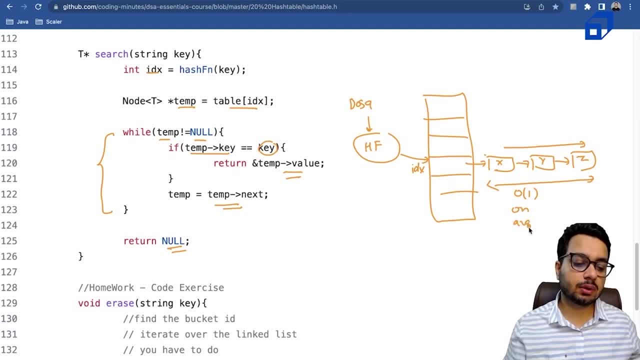 linked list will take order one time on average. okay, so we are not talking about the worst case. the worst case scenario might be like this: a single bucket has all the n nodes inside it, right? so basically, chain length is of the order end. but this is a very less likely scenario because 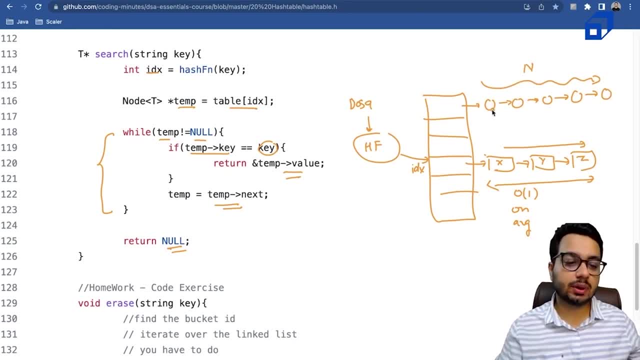 this can be only possible if your hash function is too, too bad. it is producing the same bucket for many different types of keys. okay, in general, it's not going to happen. so that is why we say, on average it's going to be order one most of the times, right. so i hope you have understood the 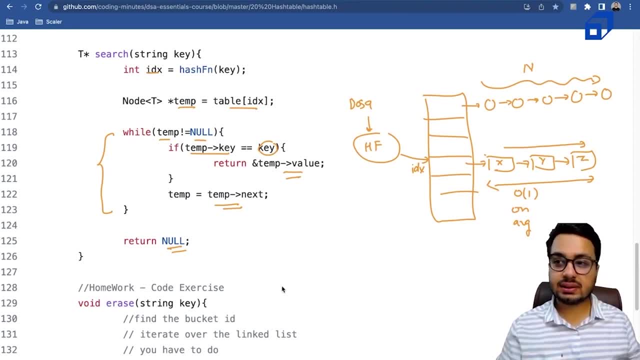 search functionality as well. right on a similar lines. you you might have to do erase as well. you might want to delete a particular key as well. right now, how to delete a particular key right now. how you have to do it now. this is pretty simple. if you know how to search, then you can. 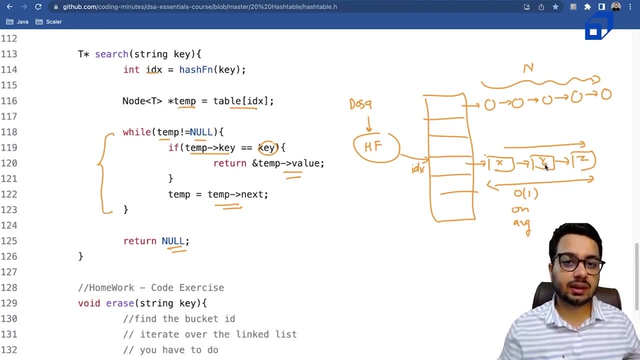 also know how to delete, right? so suppose i want to delete a key, that is y, what i will do. i will pass y to the hash function. it will give me the index. i'll find this linked list. now the problem boils down to deleting this node from the linked list. now you have to handle these cases, this node. 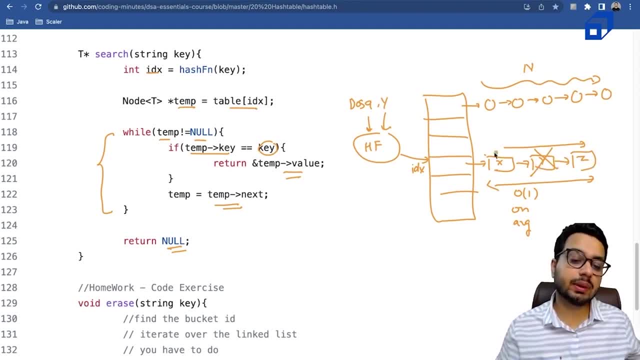 could be the last node in the linked list, it could be middle of the linked list, it could be beginning of the linked list, right. so if you know deletion in a linked list, you can easily handle the code to erase a particular key value pair from the hash map as well. let us talk about graph. so graph is. 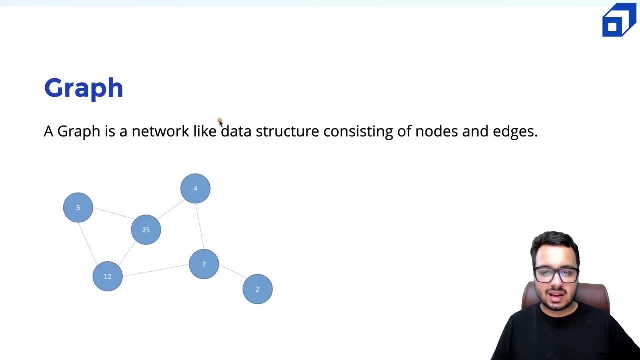 a network, like data structure, consisting of nodes and edges. so it is a data structure. that means it is able to hold data and the data is in the form of a network- okay, and consisting of nodes and edges. so if i look at this figure, all these circles- they represent a node- and all these lines. 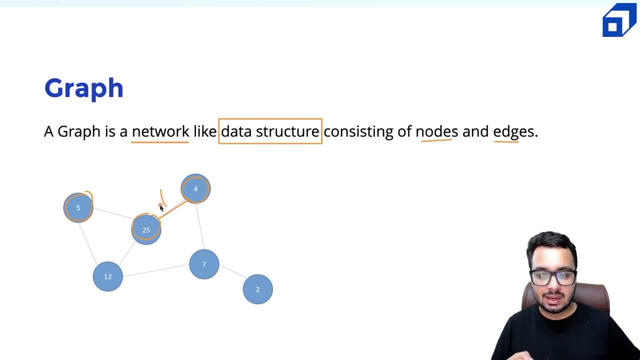 they are representing a connection between these two nodes. for example, this edge is connecting node 4 and 25.. so can we think of any real life example where the data might have connections in between certain objects? of course yes. if we talk about cities, then cities are connected with each other through connections which we call as roads. if we 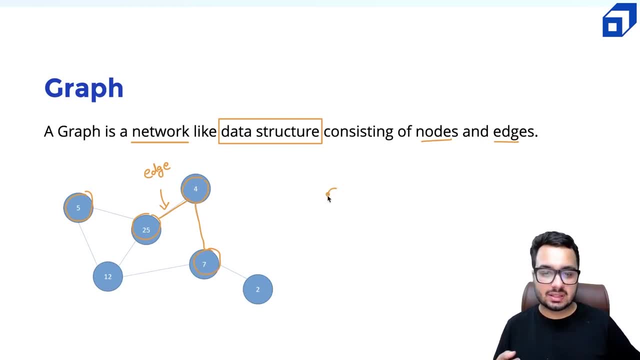 talk about a social media graph, for example, this is person a and he is connected with a person b and a is also connected with a c. so we say b and c are friends of a, or a and b are connected. a and c are connected if i talk about, uh, this person d. 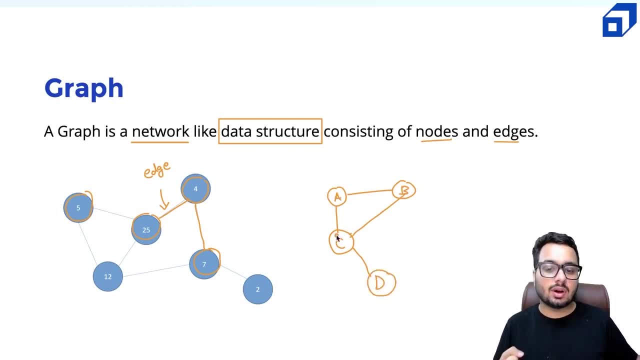 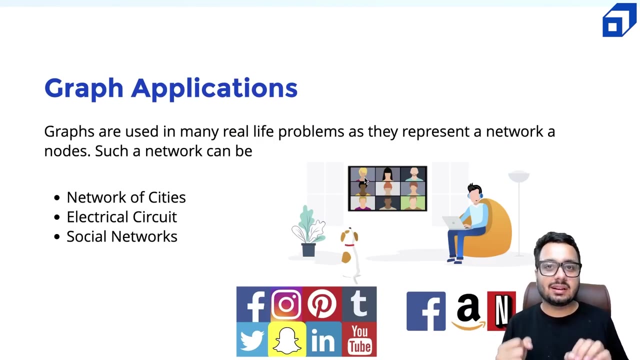 is it connected to a? we say no, the person a is not connected with d or d is not connected with a, because there is no direct edge in between them. so if i add a edge they also become direct connections. so there can be many, many applications in real life where graphs can play an important role. 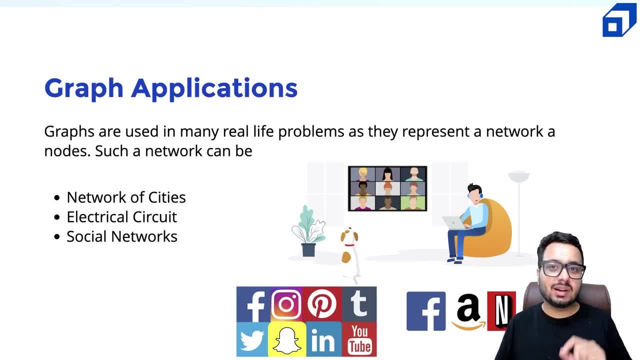 let us try to understand the applications first, then we will dive deeper into the implementation and coding. so graphs, as i said, they are used in many real life applications and they represent a network of nodes. such a network of nodes can be a network of cities, a network of places, landmarks, anything. it can also be an electrical circuit. 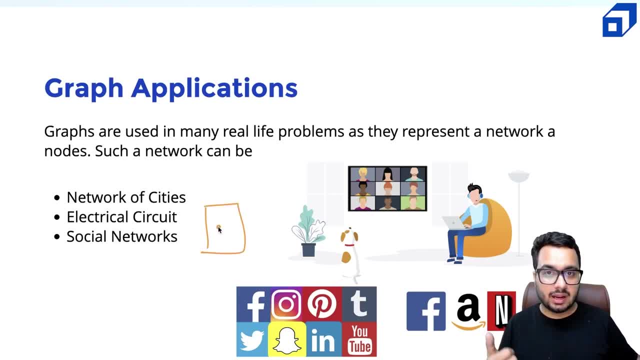 when you use, when you use your mobile phones. it has something called as a circuit. okay, it has a motherboard on which you have elements, certain small, small embedded systems on it, and there is a wire connecting these, any elements. so it is possible that we want to find out the most optimal route for the wire so that we can 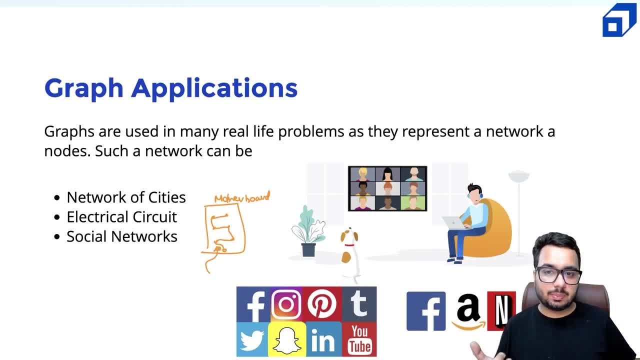 reduce the cost. okay, because it is a copper wiring, it can be expensive. it can be. a graph algorithm can be used here to minimize the total length of the wire. that can be used to connect all the components in this circuit and, of course, social media networks. we have just. 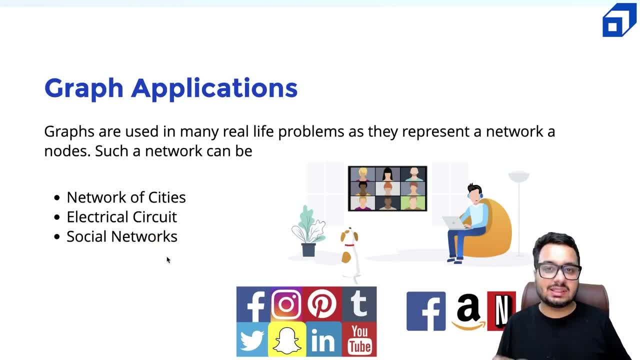 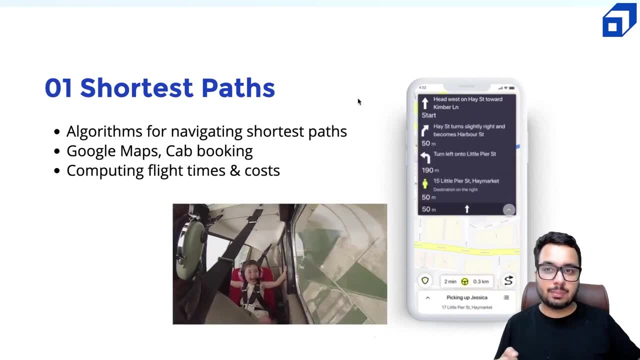 discussed that facebook, twitter, linkedin all these networks. they can represent graphs, so let us go into the applications in little more detail. the first example is an example of shortest paths. we often use apps like google maps, uber, cola and many other apps to compute to in our daily life. 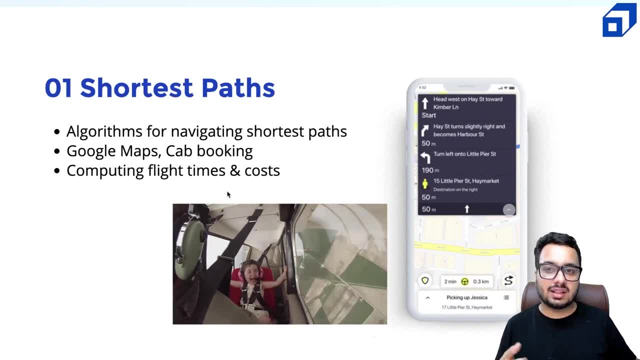 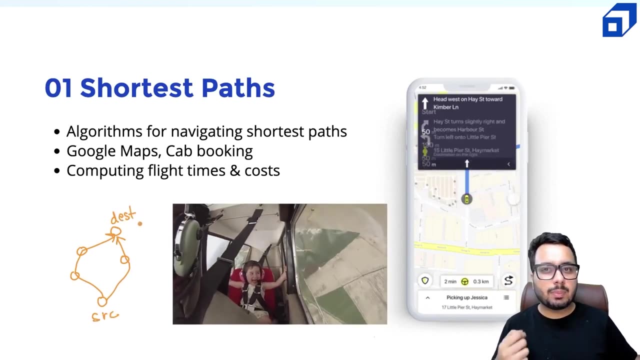 okay. so these apps, they try to figure out what is the shortest path between the set of nodes that are there, and should i go from this route or should i go from this route? if you want to do such a calculation? okay, if you want to go from source to a destination, then what path would be best can be easily devised. 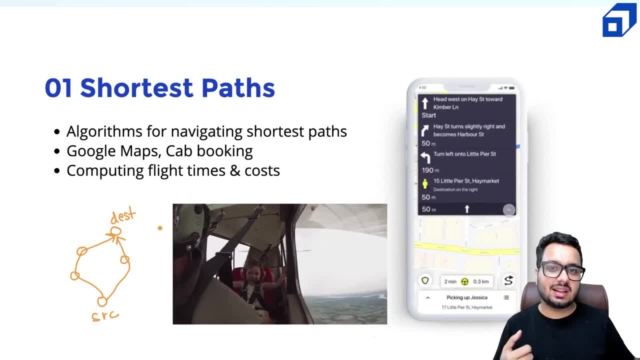 using a shortest path algorithm, known as dykstra's shortest path algorithm. we will discuss that algorithm in this series. then, of course, if you want to book flights, okay, you want to say, okay, i have to go to this region. maybe there is a flight which cost 80 and there is a flight which cost 20.. 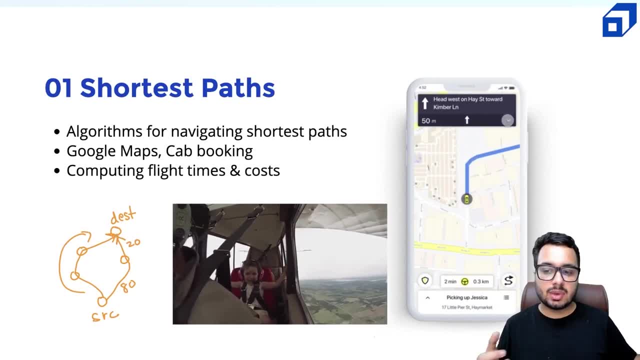 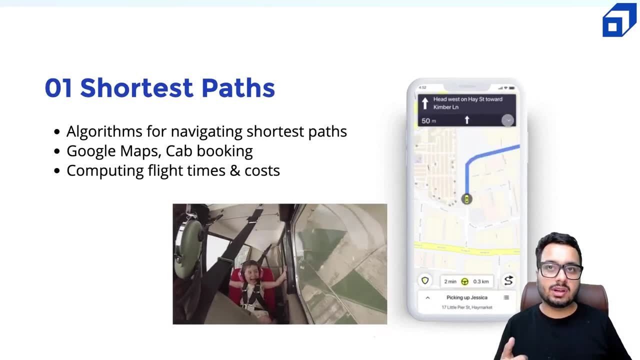 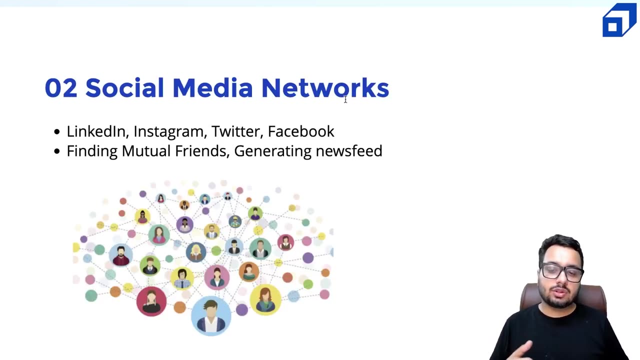 should i take this flight or should i take these three flights? maybe they are cheaper, but they are taking more time, so there might be trade-offs again. you have to look at what you want. what is your requirement? do you want to optimize for time or do you want to optimize for the total cost of travel? the social media networks i have discussed. 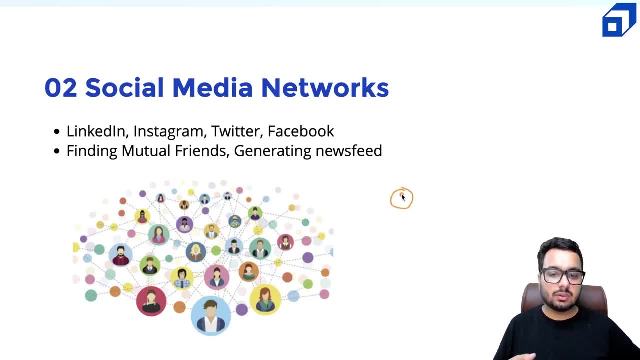 so i will give you one more example. in some networks when you connect with a person, for example facebook, so if a and b are friends, then this connection is bi-directional. that means a is b, b is connected with a, but in some other networks this connection is having a direction. 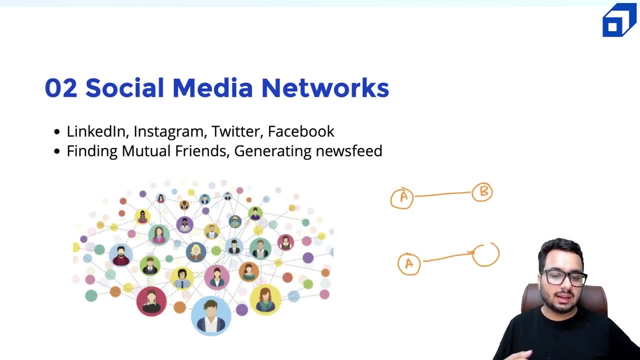 for example, on twitter, if a follows b, it does not mean b is also following a. so these edges, they can be bi-directional or they can be one directional. so we call such a graph as a directed graph or directed edges. okay, so this graph has directed edges because a is following c and b, but 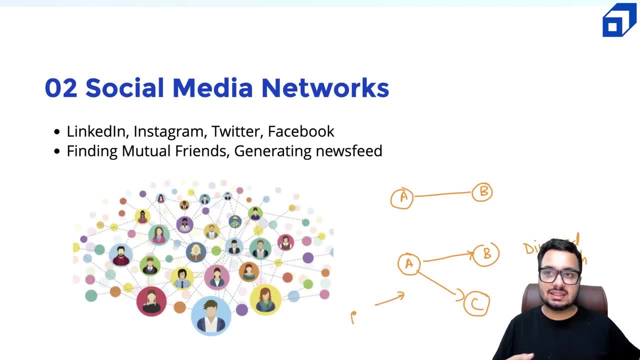 is not following this. so in such a case this is called as a directed edge, and in example of facebook it is called as a undirected edge, because there is no fixed direction. if a and b are friends, then b is a friend of a and a is also a friend of b. right now, these kind of representations. 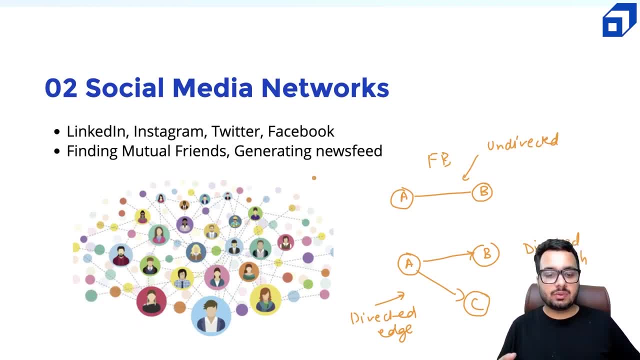 the graph, like representation, is important to build algorithms. if you want to find mutual friends, if you want to generate news feed, so for example. if you want to generate news feed, so, for example, a, it will see the post from b and c. if b is following someone, then this person's post will. 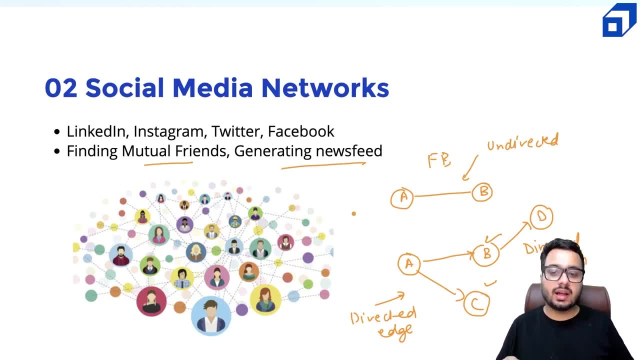 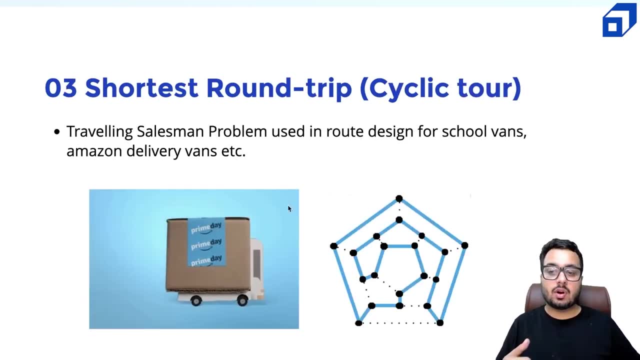 not be visible to it. all these algorithms require graph like representation of the objects involved. then there is also something called as shortest round trip, if you think of a traveling, if you think of something called as a school van. okay, what is the purpose of school van? it will start. 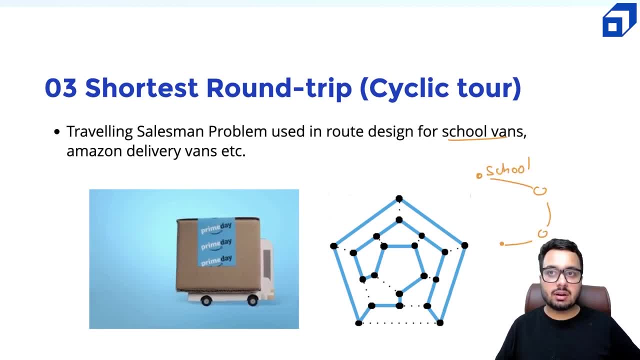 from school and it will drop all the children on the way and it will come back to its location. so, in this case, what is happening? we are doing a cyclic tour. we are coming to the source by covering all the points in the city where we need to drop the children. now it is possible that multiple routes can be devised. 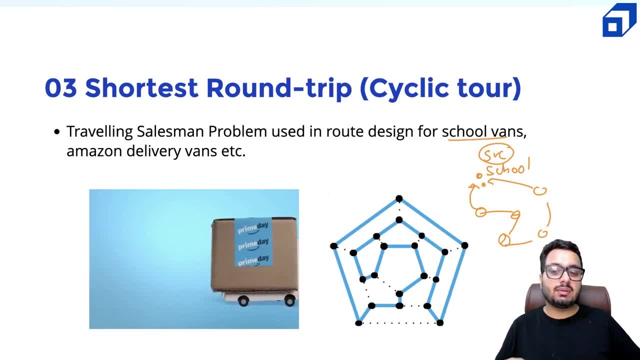 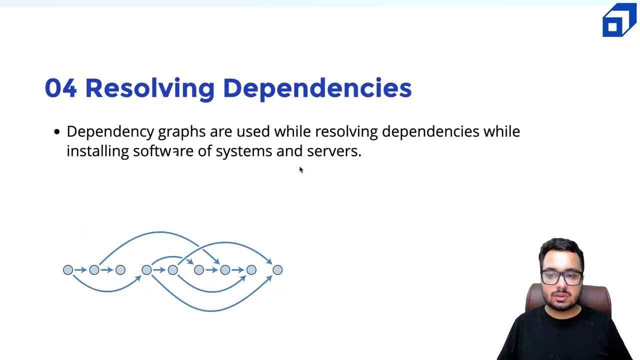 but we want to devise a route which costs minimum. so such route design can be used in for amazon delivery vans, for school vans, and this is a very famous problem in graphs, called as traveling salesman problem. we will also discuss this problem in the coming series. let us talk about one more application. so when you are installing software you might have seen that. 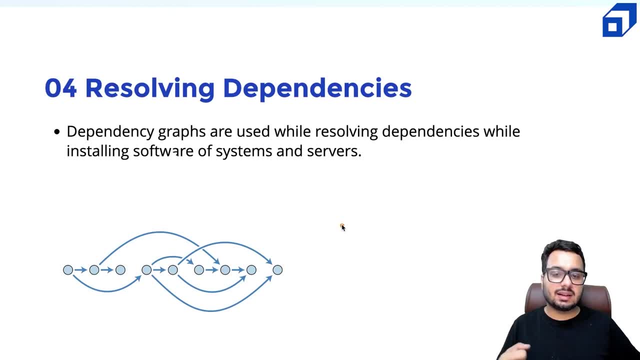 the software is installing list of dependencies in a certain order. for example, you have to install a software x for x, you need something called as, let's say, uh, c, c is dependent upon something called as b, b is dependent on upon a and there is something called as d. x is dependent upon d. 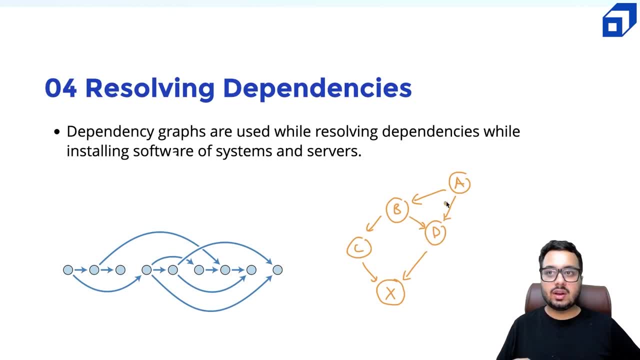 and d is also dependent upon a and b right now. in such a scenario, if i have to install the dependencies, what is the first thing i will install? of course i will install a. if i install a, then b and d. they do not have any dependencies, so either i can go with b. 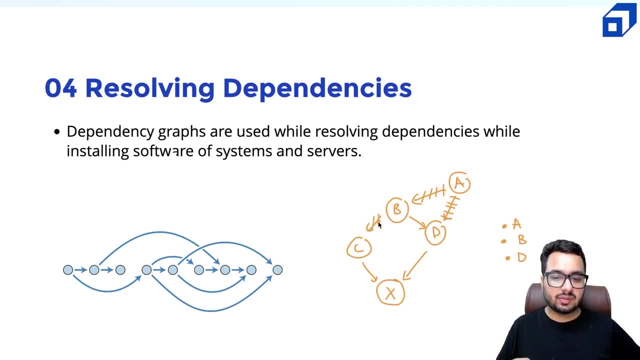 or i can go with d, so i can install b and d. if i have installed b and d, then X has only one dependency, that is C. so I can install C and then I can install X. so if I install the dependencies in this order, right, my. 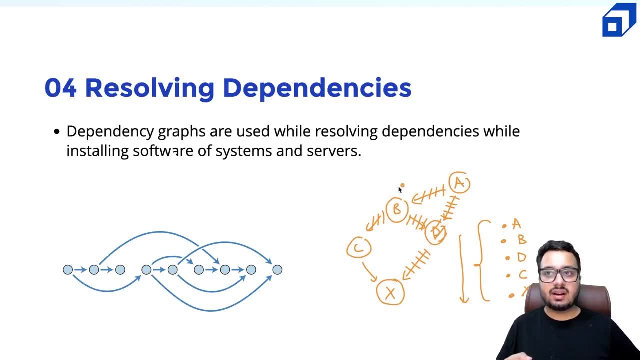 software will be installed correctly. so this kind of a graph- it is called as dependency graph and it is an example of a directed acyclic graph. that means there is no cycle, it is directed, and from this graph we need to figure out what is the correct order of installation of software. right, it is. 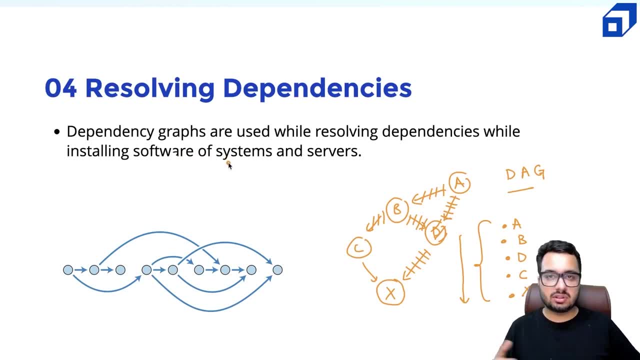 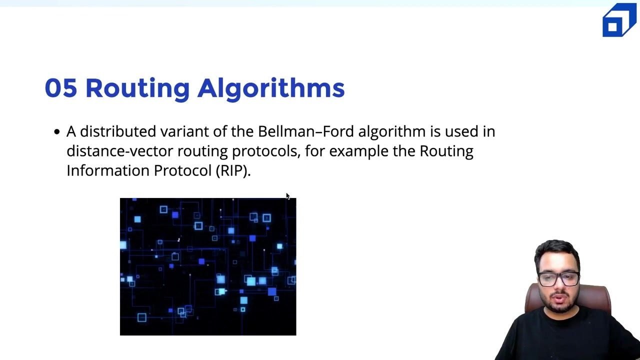 often used while installing software on systems, on servers. when you're installing libraries and modules, they follow this particular order, and this dependency graph can be easily created using a graph algorithm called as topological sorting. we will learn about this algorithm in the coming series of videos. okay, that is another application of graph. let us talk about one more. 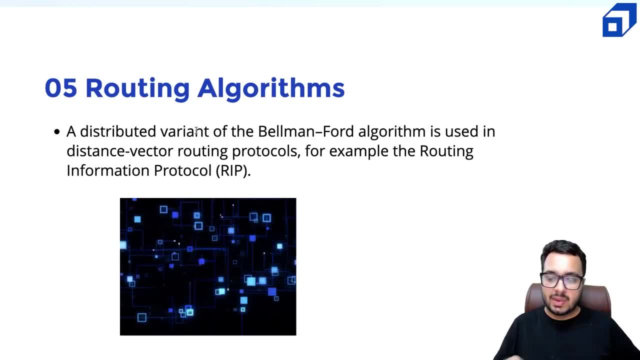 application that is routing algorithms. so Bellman Ford is a very popular graph algorithm that is also used in finding shortest paths. now this algorithm is also used in routing algorithms. so when you? so you know, the world has lot, lot of routers, and these routers are continuously exchanging data packets. so which data packet should go? 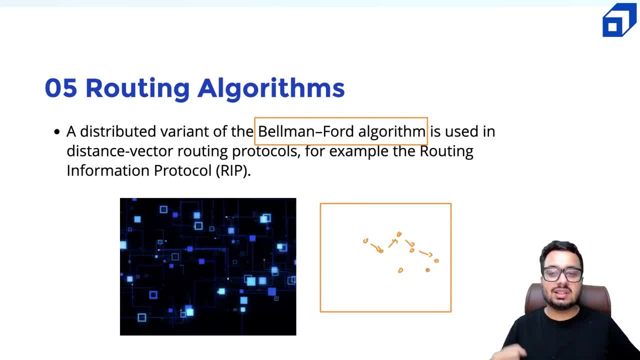 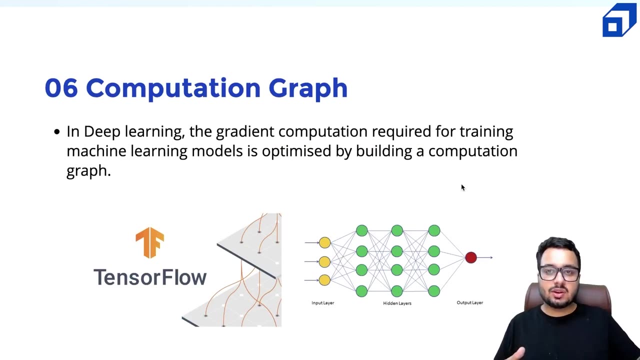 there and what is the shortest time in which it can reach to the desired location. all this routing is done using a distributed version of Bellman Ford algorithm, which is again a very interesting algorithm in itself. so let us talk about one more application. so if some of you have done machine learning, 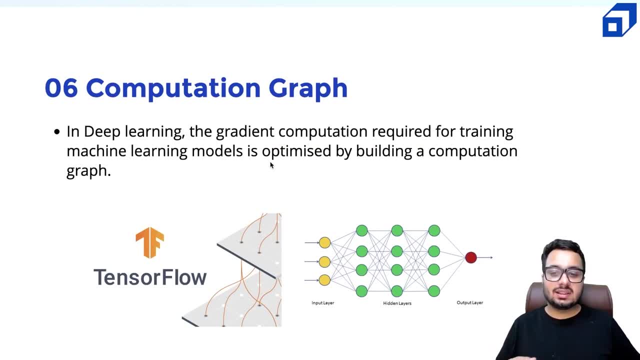 then you know, in deep learning, the deep learning models, they do gradient computation, which is an important step in training of the machine learning models. okay, this: these gradients are used in back propagation to adjust the model parameters and the way these libraries, like tensorflow, pytorch, they have built, they build a computation graph of these gradients. so 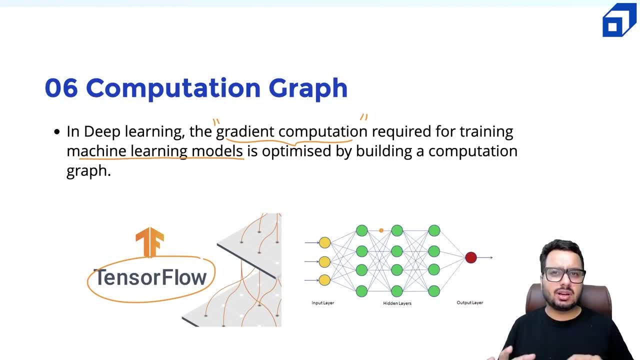 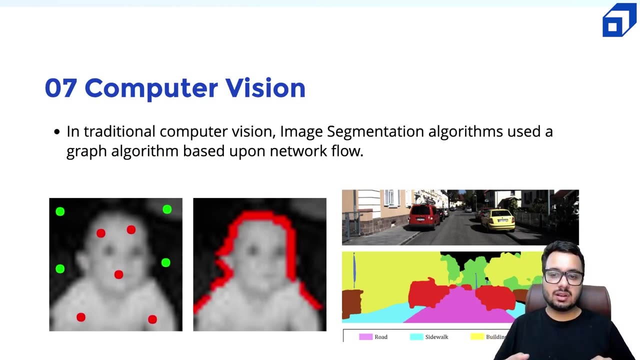 that the computation can be optimized, so you do not need to worry about how to how to construct the graph. the libraries like tensorflow, pytorch, they automatically do it for you. again, this is inspired from the idea of graphs itself. and in traditional computer vision, what happened? image segmentation. 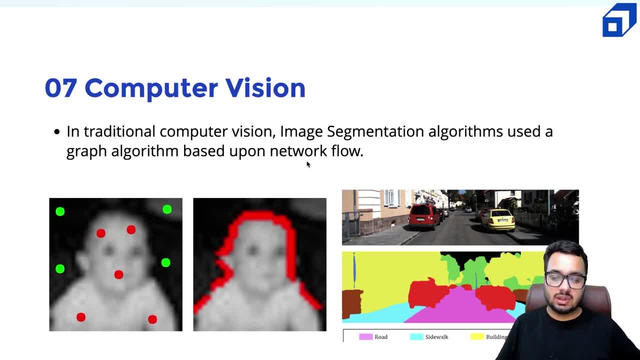 algorithms were used which were based upon the concept of network flow, which is again a graph based algorithm. if you do not know what is image segmentation, so image segmentation is basically extracting out objects from an image. it's like drawing a boundary on an object that is like one, one entity in 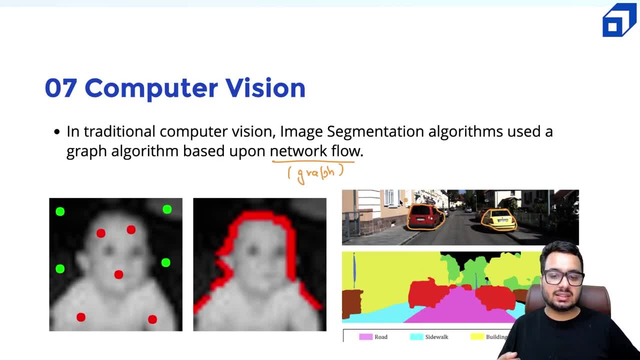 case of this example, the car is one object, the building is another object, this footpath is another object, the road is in another object. so this, these kind of algorithms, are often used in self-driven cars. but in today's world we have deep learning techniques for image segmentation, but the traditional way of 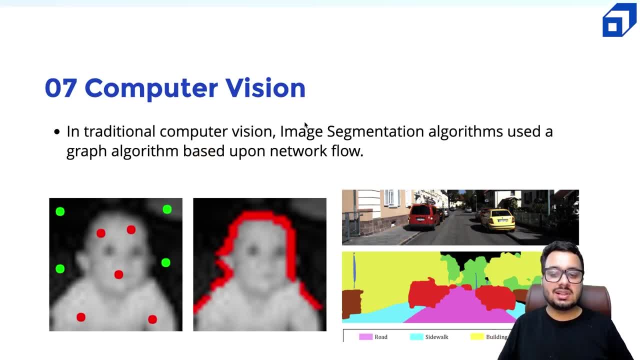 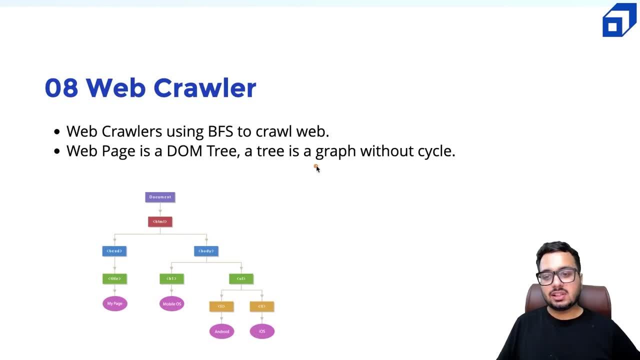 doing this. segmentation was based upon a graph algorithm called network flow. again, let's do one more application in web crawler. so basically, when you want to build a web crawler, for example, you want to crawl Amazoncom and you want to scrap the entire website. so when you go to 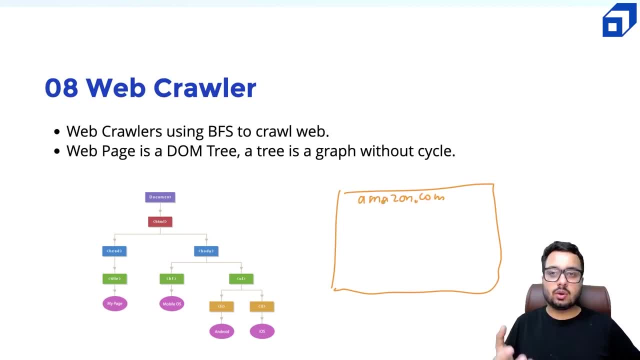 amazoncom. what happens? you load the code. the code is loaded in the browser, so in the code you will see it. there are a lot of products and with each product there is a hyperlink. so you want to go and scrap all those products. so what do you do you? you build a web scrapper that reads these links, add them into queue. 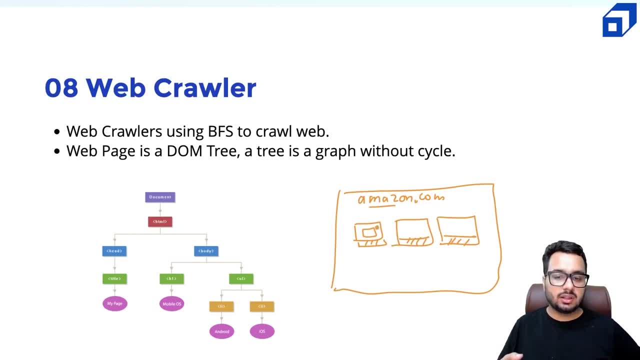 maybe this is some TV button, okay, so you go to that page, it opens up and then again there are many, many links here, so you can also use these links, crawl further, right? so it's like a tree traversal. so web crawlers use breadth first search to crawl the web. so if you have built a web scrapper, 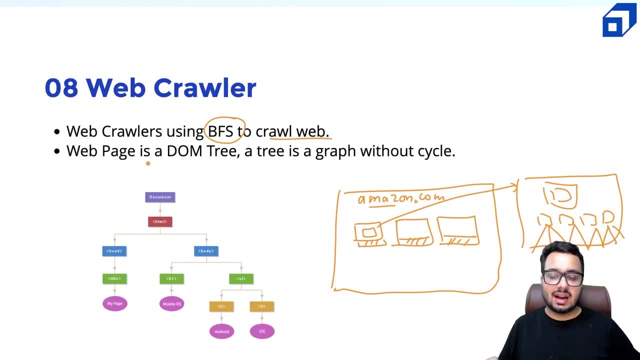 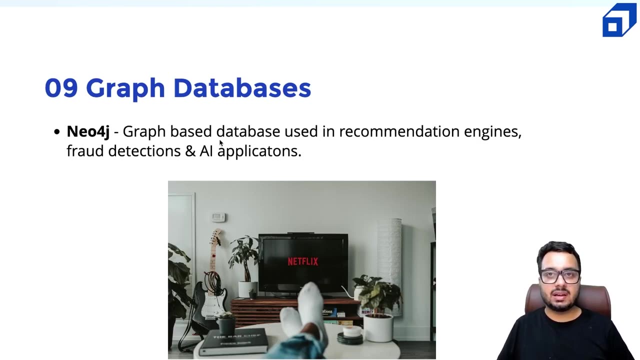 you would have know that you often do a BFS like thing and you traverse the dom tree, and a tree is also a graph. okay, a tree does not contain a cycle, but it is also a graph example. so let us do one more application. nowadays we also have databases that are inspired from the idea of graphs. 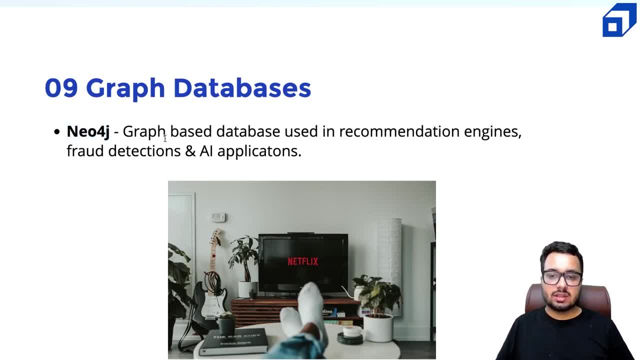 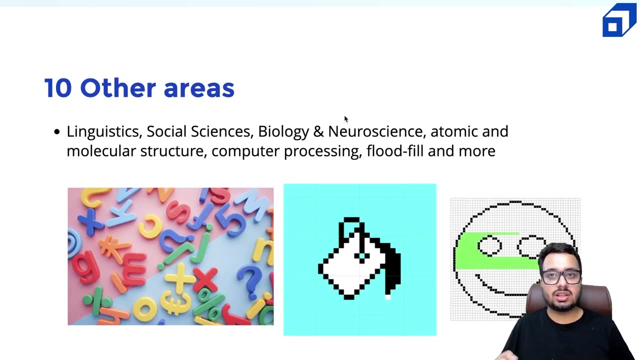 one such database is called neo4j, so these kind of databases are used in recommendation engines, fraud detection and many there are based applications. apart from it, there are lot of other applications of graphs, such as in linguistics, Social Sciences, biology, neuroscience, atomic and molecular structure, computer processing, flood fill and more so. what is this flood fill, this? 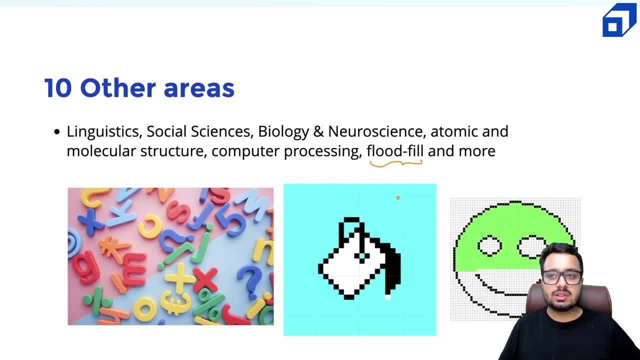 is an interesting application. looking a lot for afraid of the ways that we're I often cover in my course. when you use a paint bucket tool like this and you drop it in an object, It automatically fills the color till it hits the boundary, like you see. you can see here right. 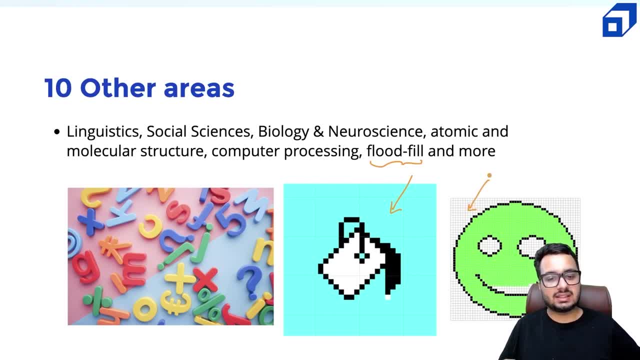 So this again is an example of graph and this matrix is an example of a 2d Implicit. it's a 2d matrix which is representing the implicit graph. So we will discuss about what is the implicit graph and how do we build algorithms on implicit graph. that will be covered as well. 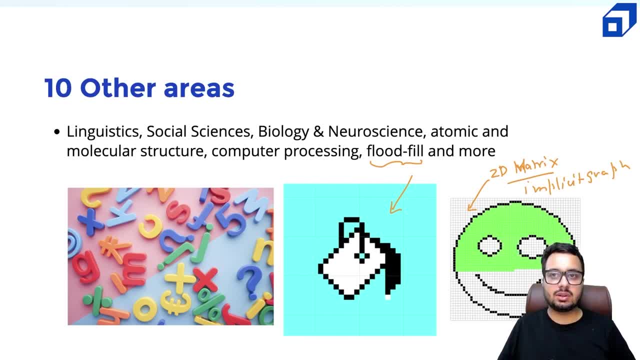 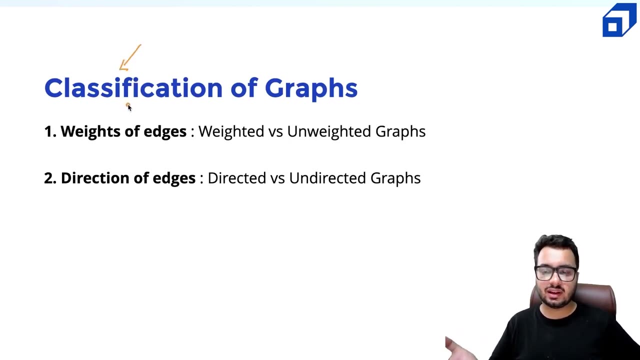 So that's about the applications. next, We will dive into the more technical concepts and understand how a graph can actually be created and stored inside The memory. next thing I want to talk about in graphs is classification of graphs. though We have talked briefly about weighted and unweighted graphs, Let us try to understand with some more examples. 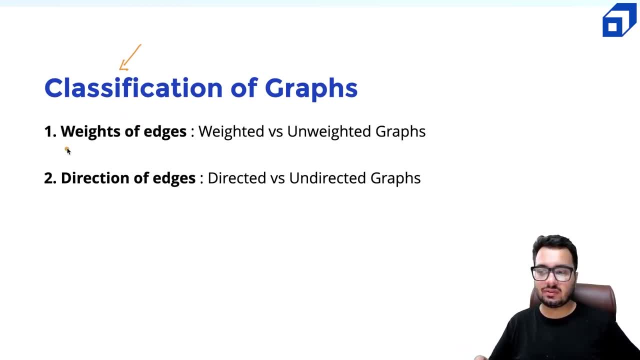 Basically, there are two criteria for classifying graphs. one is weight of edges. There can be graphs in which there is no Weight associated with the edge. That means each edge is treated equally. each has a unit cost. Okay, you can say, okay, It is a unweighted graph. such a graph is called as unweighted graph. 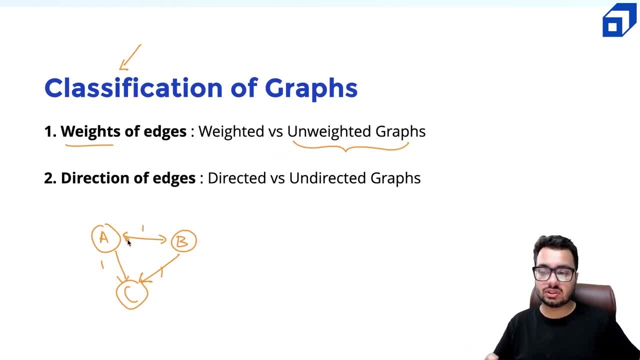 But it can be scenario. For example, if you talk about roads, Each road might have a length or it might have a time to travel from B to Z. It was some kind of weight or maybe some kind of fuel cost, so we can say that in such a scenario, each 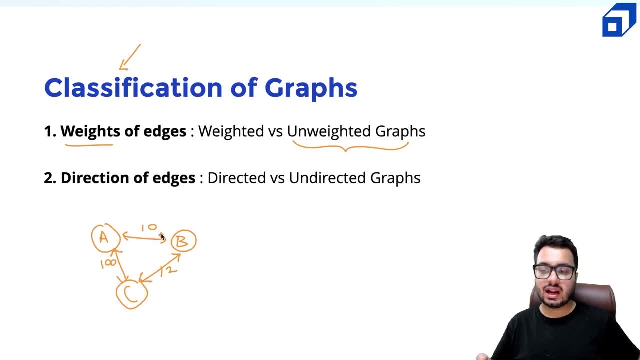 edge Is having a different weight and we need to store that weight as well. Okay, so earlier if I am representing the edge as A comma B in an unweighted graph, now I have to represent edge as A comma B, comma 10. That means the time to travel from A to B or the edge weight from A to B. 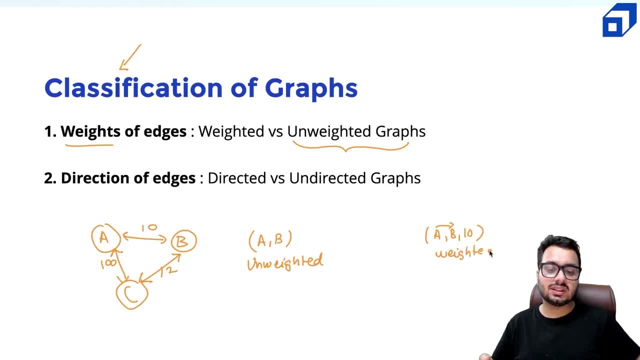 So this is a case of a weighted graph, right, That means in the implementation. Also, you will have to store this weight associated with the each edge, and then there is direction of edges. now there can be scenarios where the edges are not having any specific direction for 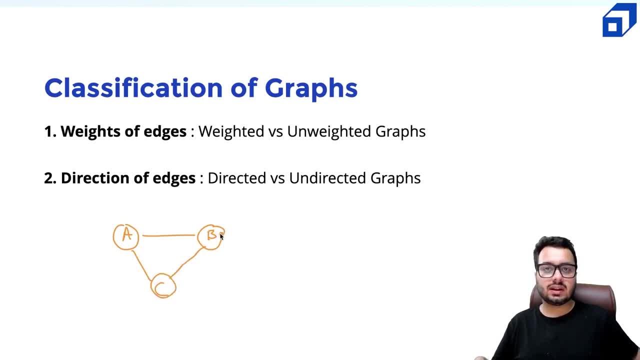 example, talk about Facebook friends. if a and B are connected, they are connected. that means a is a friend of B, B is a friend of a, but edges can have a certain direction. for example, a Twitter graph: if a is following B does not mean that B is. 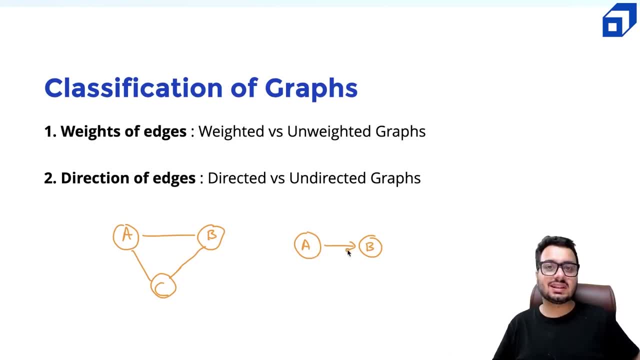 also following it. so in this case, edge will have a certain direction. that means a is following B and a is following C and B is following C, something like this. this is an example of a directed graph. and wait, so this is an example of undirected graph. 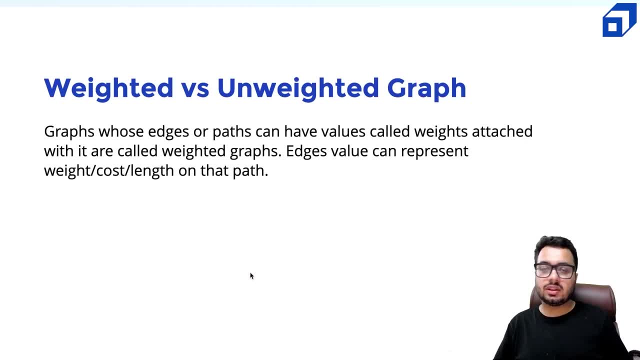 let us look at some more examples. okay, so we have discussed graphs whose edges or paths can have values associated with them. they will be called as weighted graphs. edge value can represent either the weight or some kind of cost or length of that path. for example, in roads it might be the 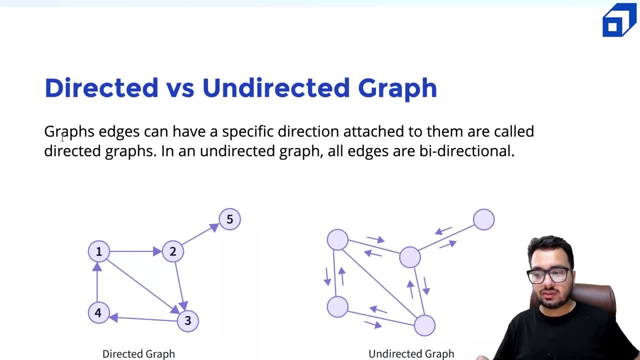 distance in kilometers. so directed, undirected graph. we have already discussed graph edges- can have specific direction attached to them. they're called as directed graphs. okay, now, in such a scenario, you might have two way to do this. you can go from 1 to 2: there is an edge. from 2 to 1, there can be edge. 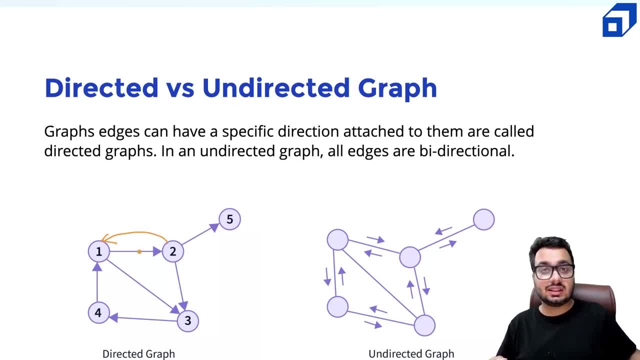 as well, and it is possible a different way. it is associated with each of it and, for example, we are going from Delhi to Bangalore by a flight. now this flight might cost you 4k, but this flight might cost you 5k. this is an example of a 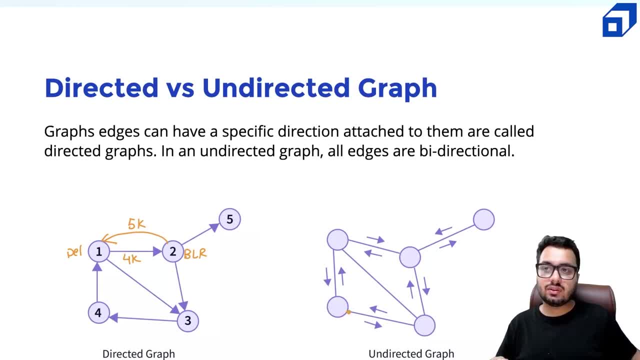 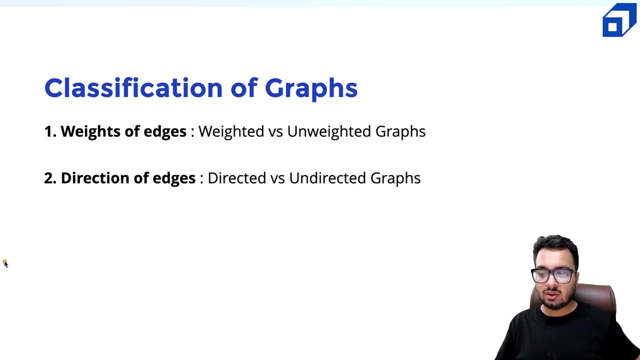 directed under weighted graph. in an undirected graph there is no direction of the edge. that means you can travel in both directions. you can go from A to B to A, for example, in roads. I hope you are under able to understand through these examples. so let us try to make a matrix and let's summarize right. I can say: 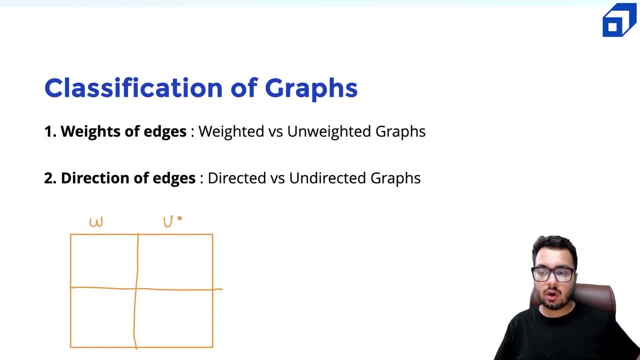 graph can have weights, weighted graphs or unweighted graph. they can have direction or they can be undirected. what? what would be an example of for directed and a weighted graph, for example, from A to B? okay, and there is a cost associated with it. this can be your graph of. 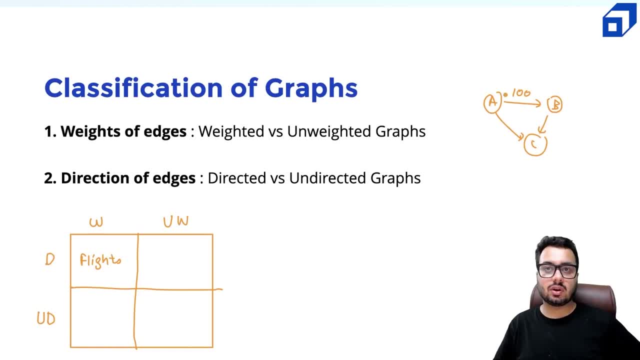 different flights across cities because flights will have a cost and they will have a direction. if there is a flight from A to B, it is possible that there is no flight from B to A, or B to A flight has a different cost. this will be a directed and a weighted graph. let's look at an example of a directed and unweighted. 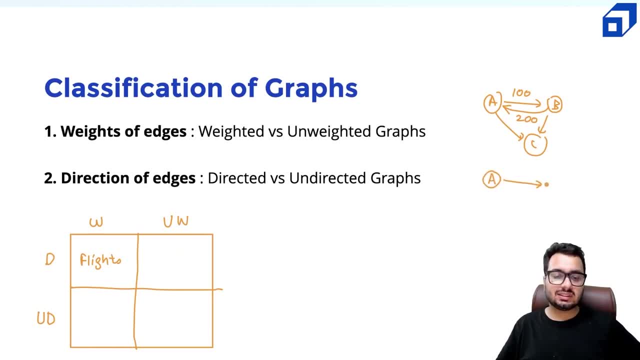 graph. I talked about topological sorting, in which we said that there are certain tasks and there are dependencies. for example, B is dependent upon A, C is also dependent upon A and C is also dependent upon B. so this is an example of a directed acyclic graph. okay, so this is. 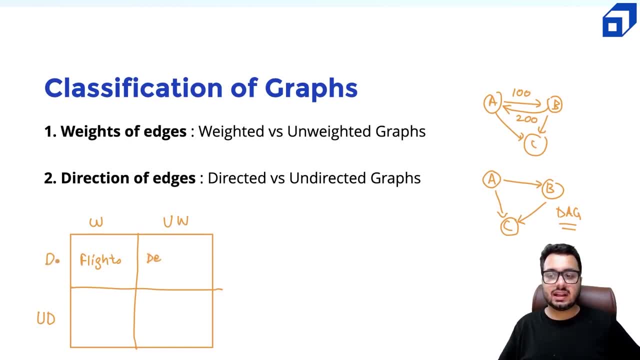 an example of a dependency graph. in this graph there is a direction, but there is no weight. it is an example of directed and unweighted graph, so an example is dependency graph. okay then, this is an example of undirected but weighted graph. so I want a graph in. 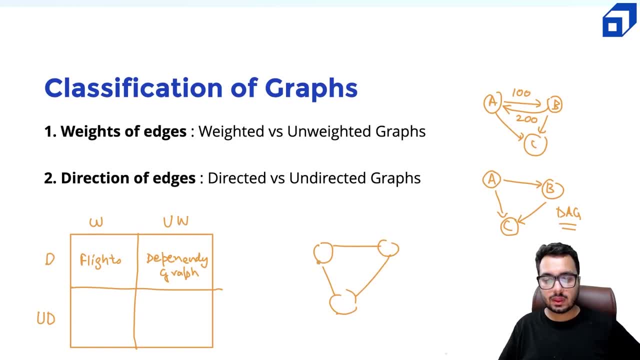 which there is no direction but there is a weight, maybe the road network. I can say, okay, the roads are generally two-way, so there is, there is a cost, so there is a weight, but there is no direction. so 100, 200, 10, 20.. 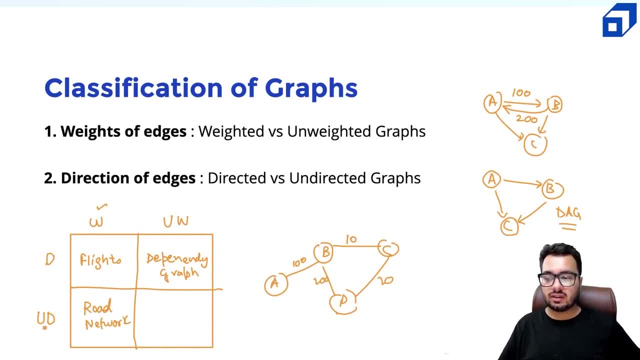 this is an example of undirected and a weighted graph. then undirected and unweighted graph. so that means no direction and no weights as well. so it could be simple: Facebook graph in which you are representing who is connected with whom. A and D. they are friends, so there is no weight. so maybe Facebook friends graph, okay, or Facebook. 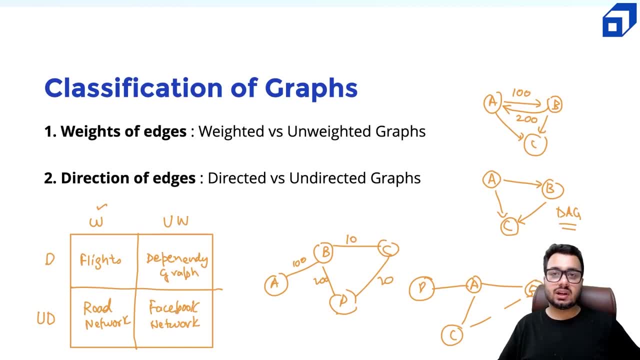 Network. so it is possible that it is unweighted. but depending upon how Facebook implements it, this graph can also become weighted. Facebook might represent the score, a friendship score, on each edge, how strong these two people are, how strong their bond is. so it is possible that this graph can be made as weighted also. so I hope. classification of graphs. 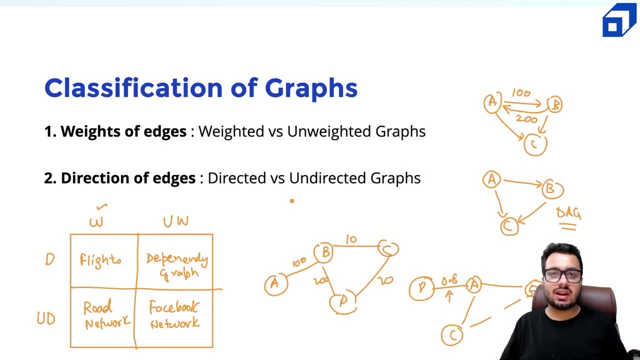 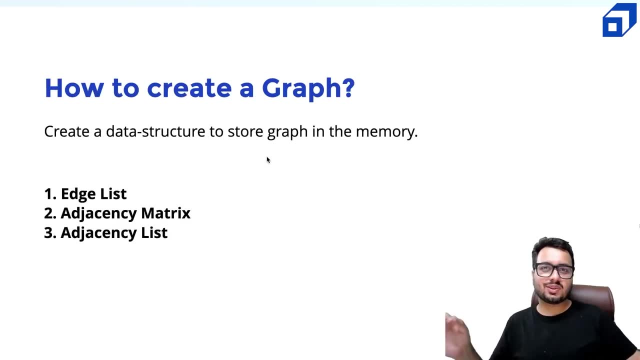 is clear through these examples, and next we will dive into the implementation: how to create a graph and store it on your around. now the next question arises: how do we actually create this data? how do we work with it? so there are three common representations for graph. one is called as edge. 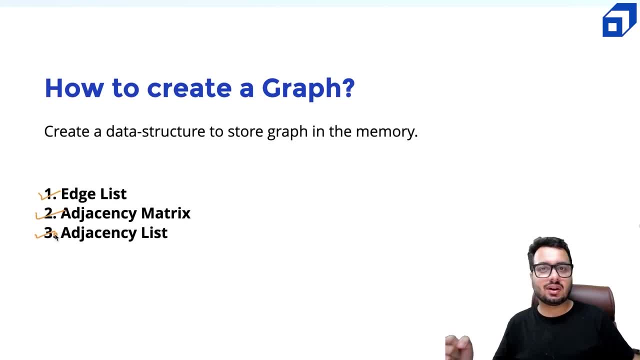 list. one is called as adjacency matrix and one is called as adjacency list. we will go over all of them one by one. each representation has its own set of advantages and disadvantages, but in general, this representation, which is called adjacency list, this is the most popular and most commonly used. 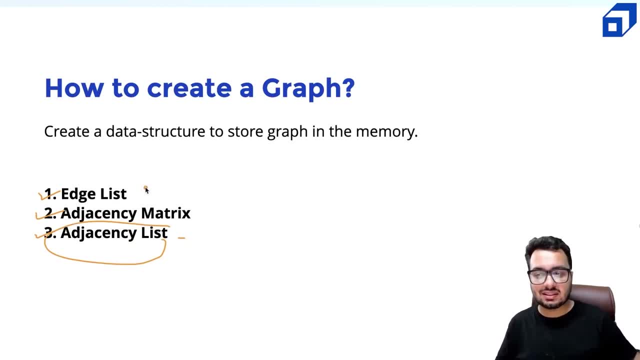 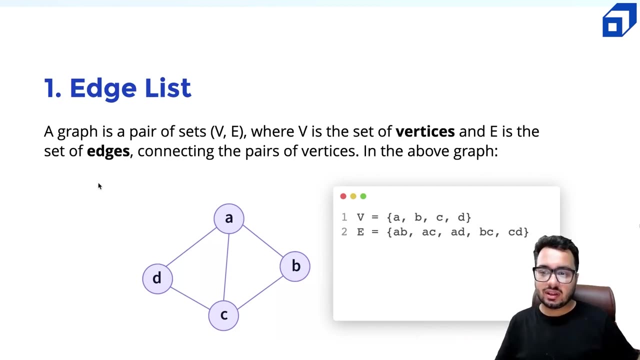 in many algorithms. but this does not mean that edge list is useful or adjacency matrix is useless. they are also useful. they have their specific applications in certain type of algorithms. so let us discuss edge list first. and what is the edge list? so in a edge list, we represent 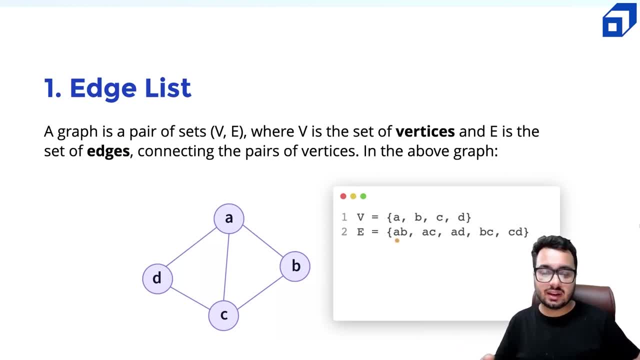 graph in in terms of list of edges, right? so suppose we have vertices a, b, c, d, so we will make a list of vertices and if we have edges, we will note down what edges we have. we have a b, so a b is an edge. we have a c. 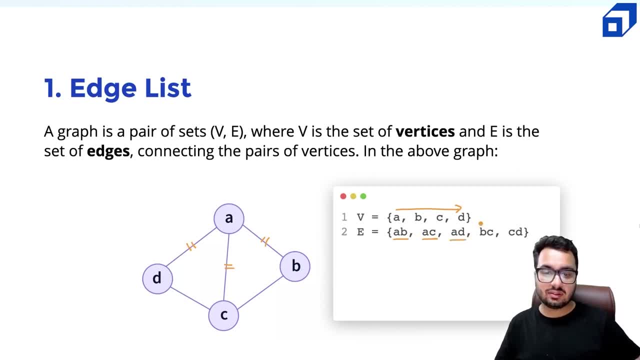 we store that. we have a d, we store that. we have b- c, we store that. we have c d, we store that. so right now, i'm assuming this is a undirected graph. so when a- b is an h, it also means b. a edge is also there. that means if you can go from a to b, you can also go from b to a as well, right? 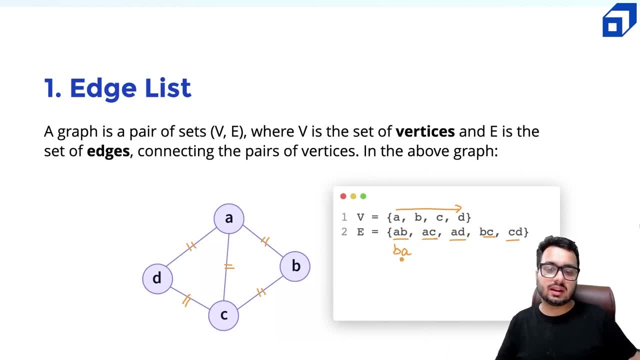 similarly, if you can go from a to c, you can go from c to a as well, right? so in my code i will be storing two copies: ad is there? da is there? bc is there? cb is there? dc is there? right, i'll be storing it like this. that will be more helpful, because if i am at d and i want to look at what nodes i can. 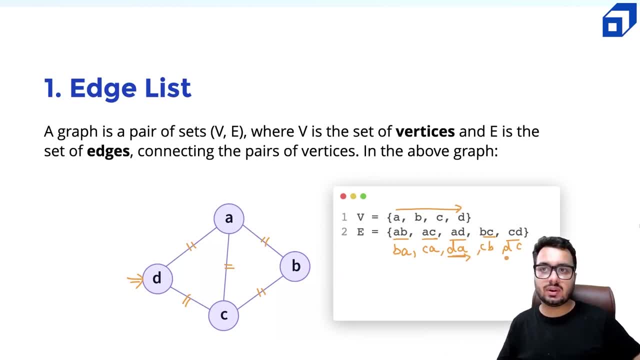 visit. so i can clearly look at this. there is an edge from d to a and there is an edge from d to c, right, so i can look at this. or you can say, okay, i'll iterate through the whole list. of course you have to iterate through the whole list and you have to look at what pairs contain d right from. 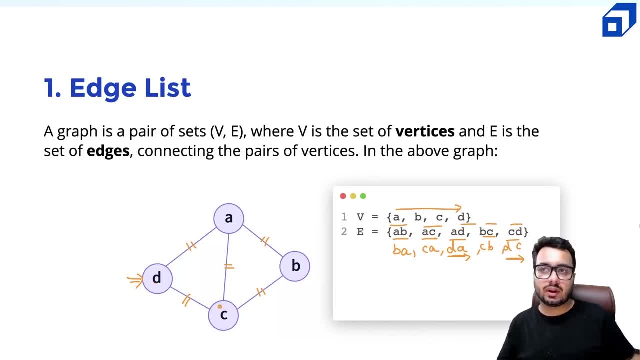 that you can get this information from d, where you can go right, but this kind of representation is pretty, i would say, inefficient. if you have to find whether there is an edge between, let's say, b and d, i want to see whether there is an edge from b to d. the answer is it is inefficient because you 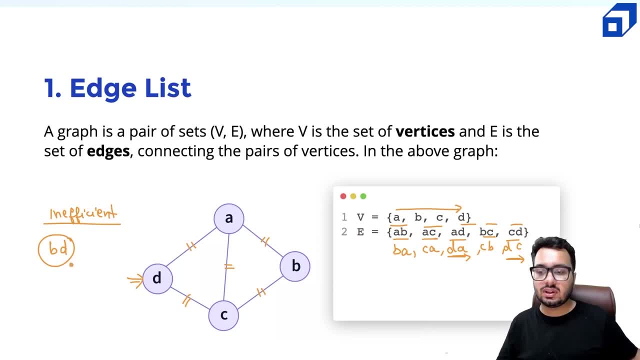 have to spend. you have to do a linear search over the whole list. so that means you have to spend order of e time looking for whether such an edge exists or not, right? similarly, if you have to do an operation like: okay, give me the neighbors- immediate neighbors- of b, right. this is now a very common operation in graph algorithms such as bfs. 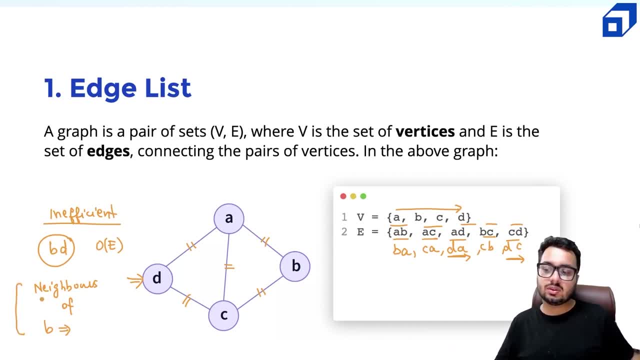 dfs, the extras. we often need this operation, right, the neighbors of b. so what are the neighbors of b? so again, you cannot tell directly, you have to iterate over the whole edge list to find out what are the neighbors of b. so again, you cannot tell directly, you have to iterate over the whole edge. 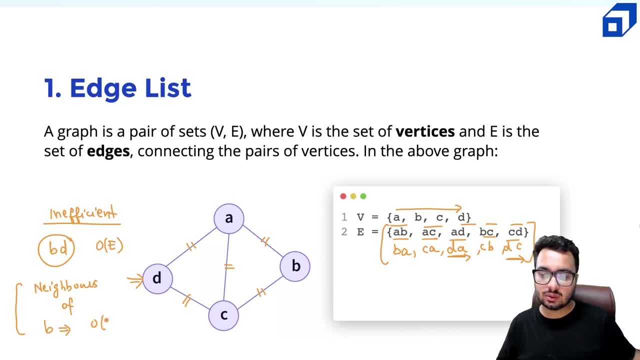 list to find out what are the neighbors of b. again, this operation is going to be inefficient, it is going to take order of a time, right. but one thing this edge list is good at: for example, suppose this was a, this graph was a. let's say a weighted graph. let's say 10, 5, 2, 1, 6, 8. and i want to pick. 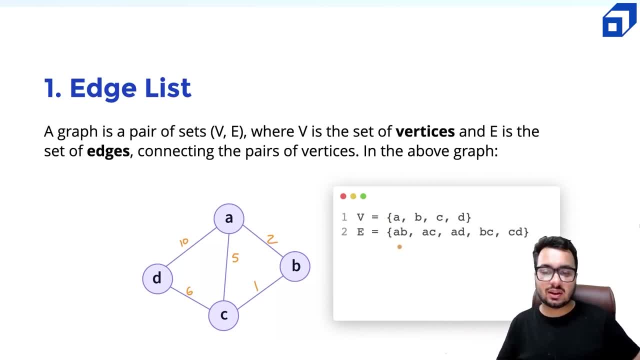 edges based upon their weight, right. so now, in such a scenario, i will be storing three things in an edge. so i will be storing a, b, followed by 2. i will be storing a, c, followed by the weight right. in case of a weighted graph, i need to store three things, right. 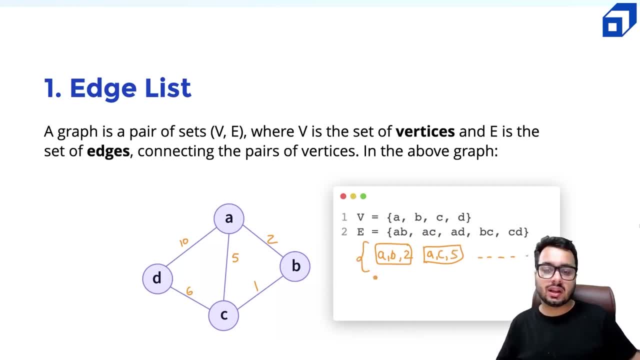 and so on. maybe i want to pick edges based upon their weight. so what i can do, if i'm i've stored all edges in the form of list, i can easily do sorting on this list. okay, i can do sorting on the list in like e log e time, right, e log e time, and i can pick edges, maybe based upon their weight. 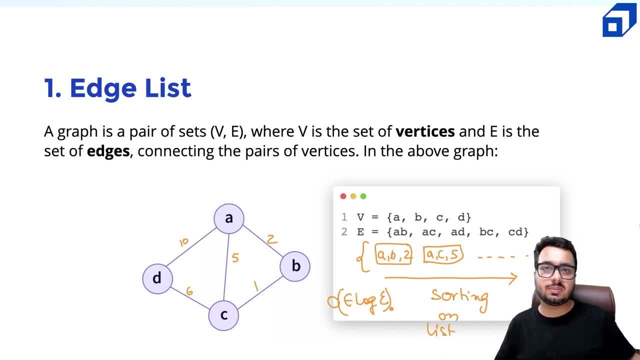 right? or according to some criteria, right? so maybe i want to do sorting on the list based upon weight. so this kind of algorithm is actually helpful when we deal with a topic that is called as minimum spanning tree, right? so when we are building a minimum spanning tree algorithm, we actually need 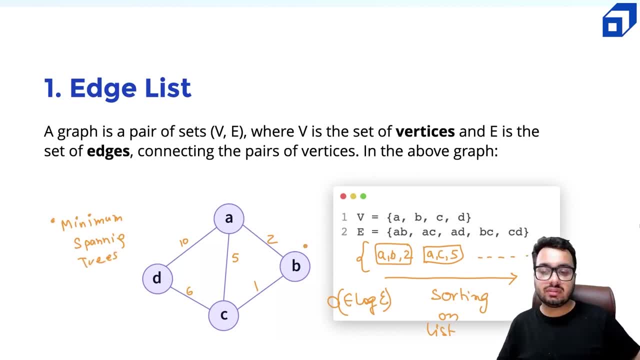 to pick edges based upon weight in such an algorithm. we will go with the edge list kind of a representation. right, so that means this representation is also useful, but it depends upon the algorithm. what kind of operation do we want? do we want to get neighbors of a node, or do we want 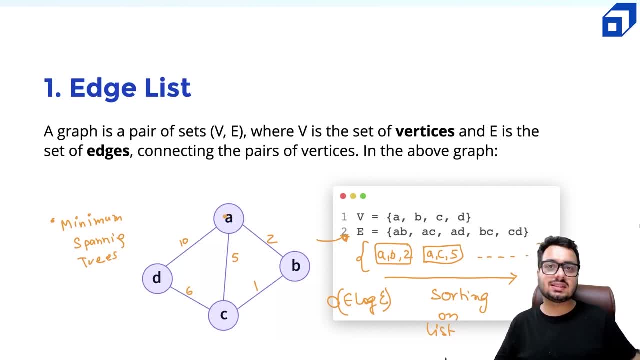 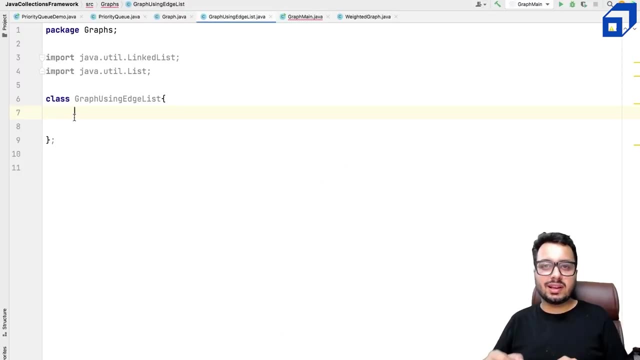 to sort edges. so if you want to sort edges, then edge list is the representation that we will use. so i hope you are able to understand edge list. and now, in the next video and now we will discuss the code of edge list. so i am going to show you how we can create a graph using edge list. 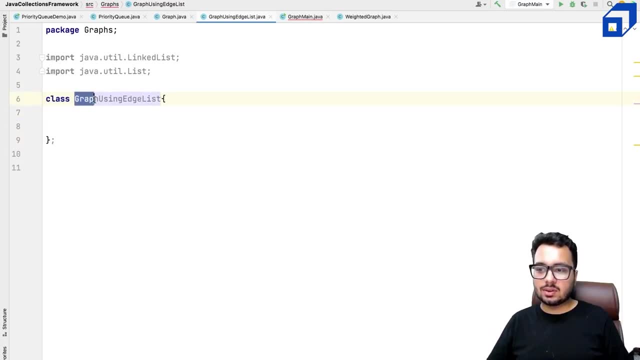 so i am in my intellij id and i am going to create a class called as graph, using edge list. this class will be responsible for holding the data of the graph effectively. what i am going to do is- i am going to keep things little simple. i am going to fix. 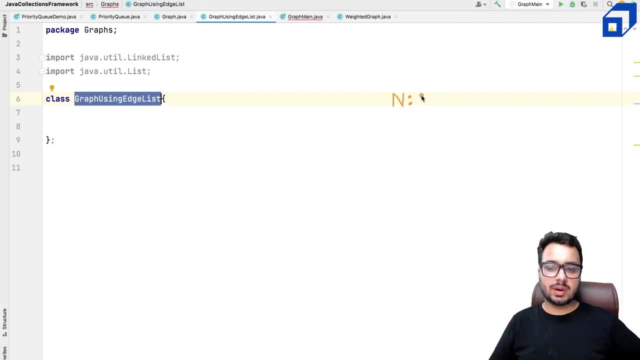 number of nodes- let's say number of nodes- is given as input by the user. let's say: user says four nodes. i am not going to take input the names of nodes. i am going to assume that the nodes are always numbered from zero to n minus one. so this is from zero to three. right, this is something. 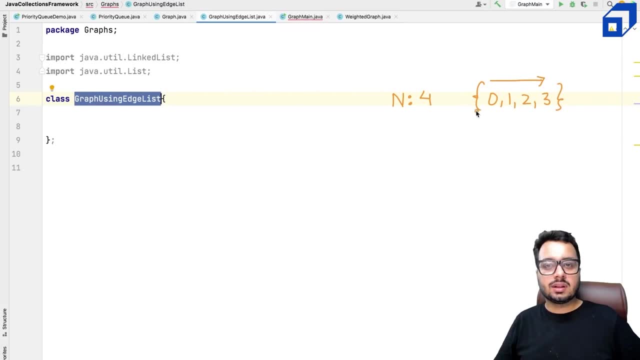 which is very common in many coding problems and we often use. we make this assumption okay and you can verify from the problem statement. if this is not the case, then we will discuss it separately, right? so number of nodes are four and let's say, the graph looks like this: zero, one, two, three, right? 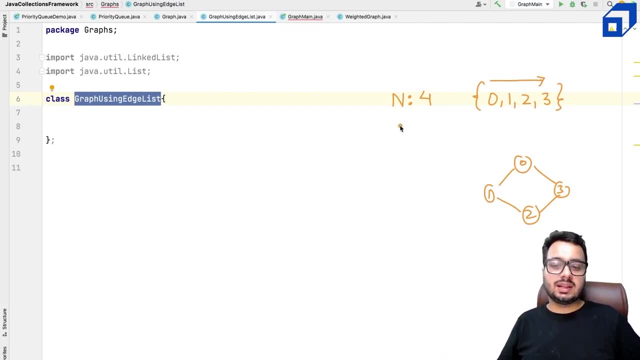 so what is expected in the input? that you will be given how many edges are there. so number of edges will be input, that is also four, and then you will be given the names of edges. so zero comma one is one edge. zero comma three is another edge one. comma two is another edge two. comma three is another edge. 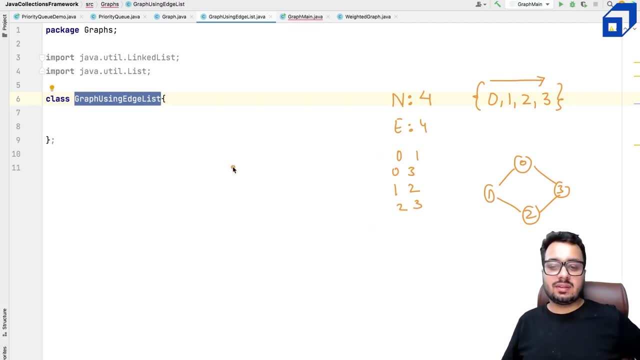 numbers input. so what is our expectation? that this graph should be able to hold these pair of edges. so 0 comma 1, i want to hold, 0 comma 3, i want to hold, 1 comma 2, i want to hold and 2 comma 3 i. 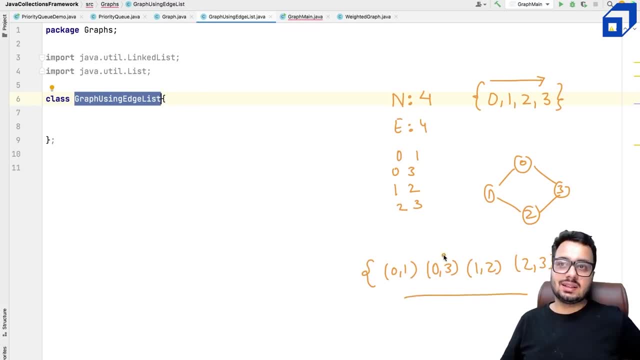 want to hold right now. if you look at this list, can you visualize this graph? of course, yes, right. that means this information is sufficient to store this graph, right? what i'm going to do in this graph class is i'm going to make a list which is able to hold the following edge: right now: it is. 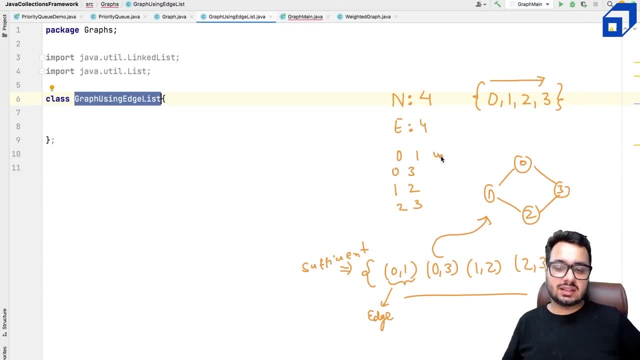 possible that each edge might have a certain weight, let's say some weight: w1, w2, w3, w4, right. in such a scenario, i can add w1, w2, w3. it will be list of edge, where each edge object is a collection of three numbers, in this case right. so what we can do is we can define a class called as edge right. 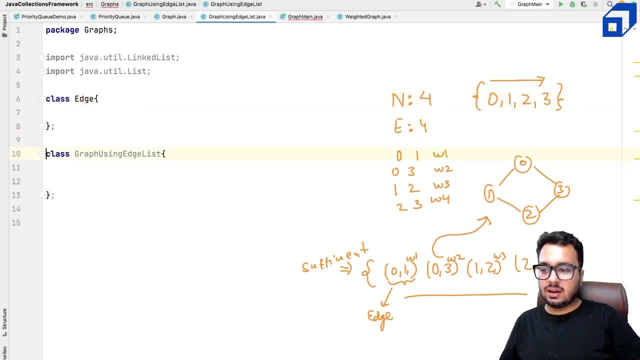 we can define a class called as edge right, and in this class i can have three things. one is maybe the source, so i call it as u, i have v and i have weight right, so that means, uh, the triplet. if there is an edge from u to v with a weight w, i'm going to store a triplet u v- w and i'm going to create an edge. 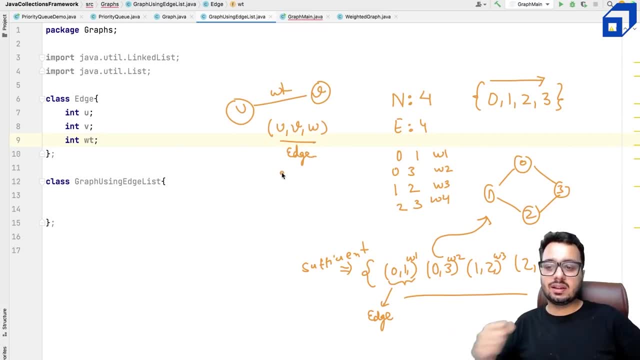 object out of it. right, then i can make a list of edges. so i hope you understood the concept. let us dive into coding. so i need a constructor for the edge class. so the constructor is going to expect u, v and w right for one edge object. so i can say: this dot u equals u, this dot v equals v. 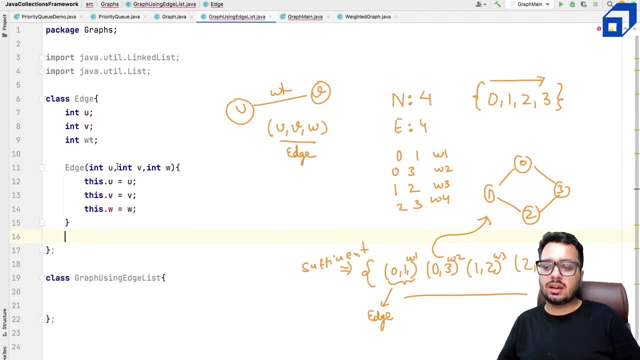 this dot, weight equals weight, right? so later on i want to print the edges, so i might need a method to display an edge, right? so i can just do string method, which is going to show me which is going to print, which is going to return a string. 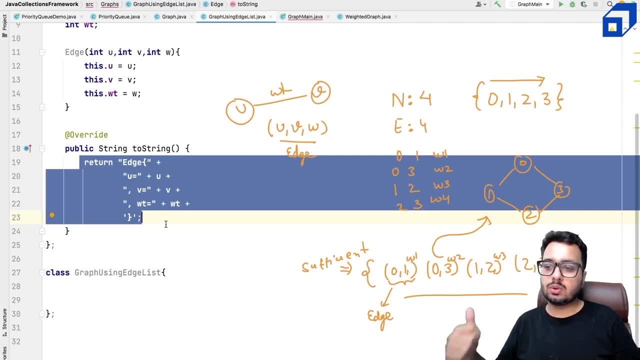 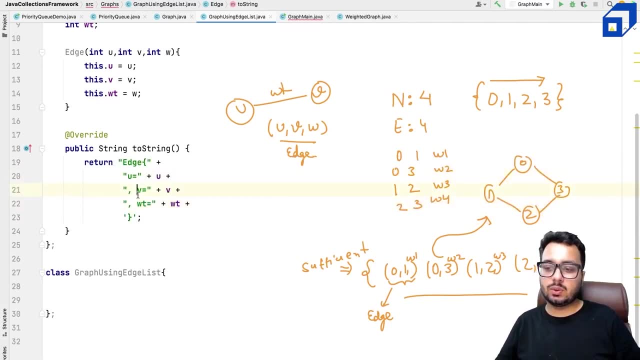 representation for this edge. so this will be helpful when we are going to print the edge. so if i want to do s out an edge, i will see that the edge will be printed like this: u equal to something, v equal to something and weight equal to something. 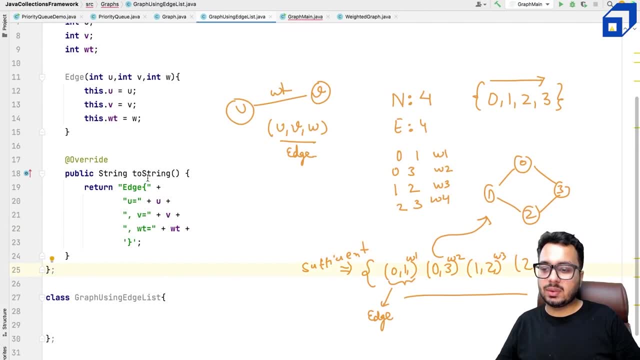 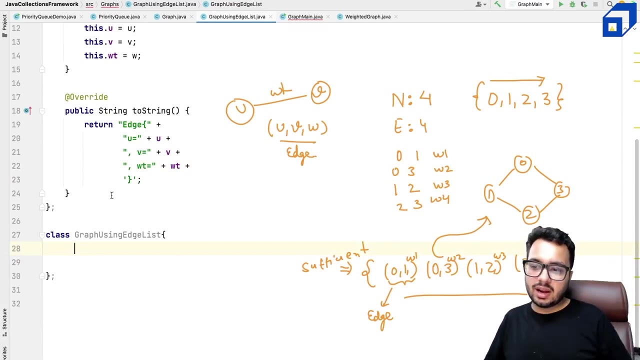 this overwrites the default uh two string method, right, and it is auto generated by the id form, right, so i have the two string method with me, right? this will be helpful if i'm going to display the graph. that means i'm going to display this edge list in the output, so i don't have to like. 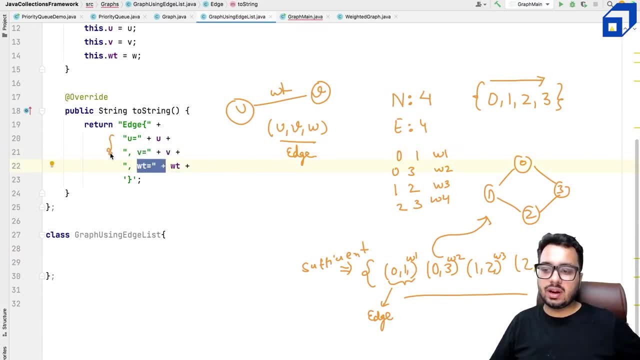 i don't have to write for each edge i have. i don't have to do this work because it this method will be called when i'm going to print it, so i can simply say: s out some edge, right. so something like this. we can do so now, coming to this actual class: right, so let's make this class as public. 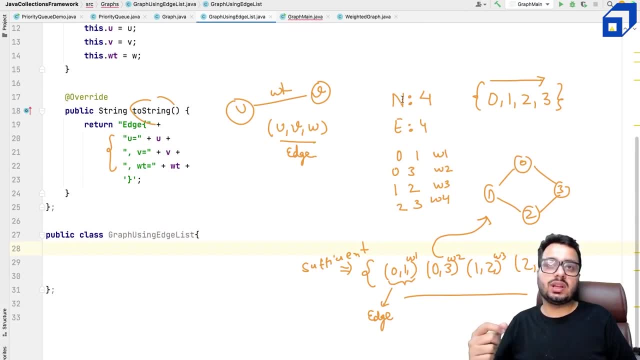 class what information it needs to hold. it needs to hold how many nodes we have, number of vertices, number of edges is optional because it can be judged by the length of this list. right, the user is going to enter the edges and we are going to store them. right, so that is simple and 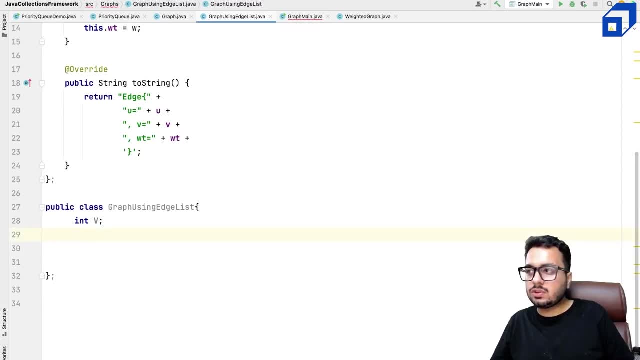 let's have a constructor- right so the construct, and apart from it, we need a list of edges- right, so let's have the type edges. help. let's create the constructor graph using edge list. in this constructor, i'm going to get number of vertices which i can initialize. 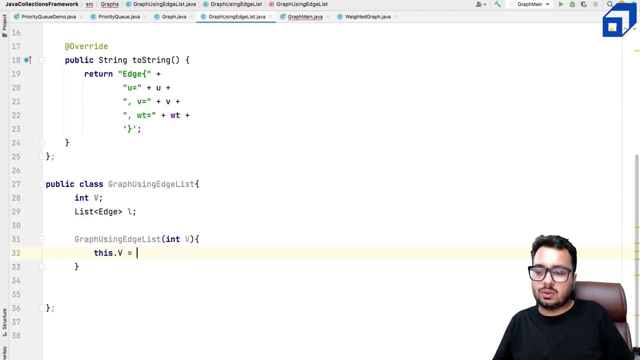 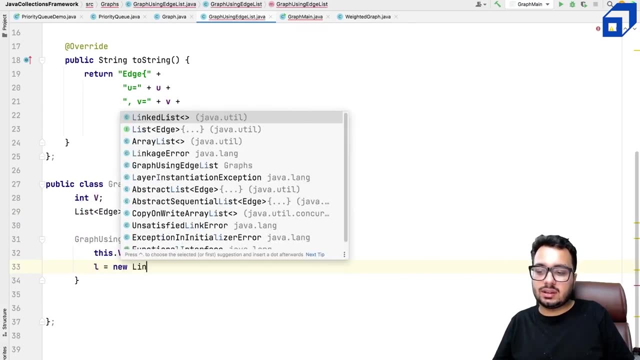 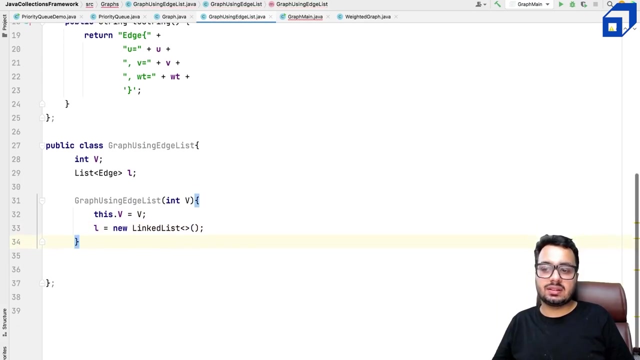 this will be list of edge, so i can say this: dot v equal to v and i also need to create this list. so l is a new list, so it can be a linked list or an array list and i can say it is an empty list, right? so when, when a graph is created, it knows how many vertices it has. 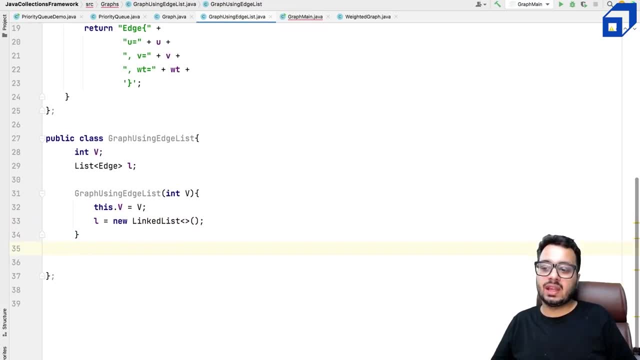 and it creates an empty linked list. okay, now i want to add edges in this graph. maybe i need to create some method. add edge u, comma v, and wait right, i want to push an edge into this graph. i can simply say: uh, if there is an edge from u to v, so i can say: 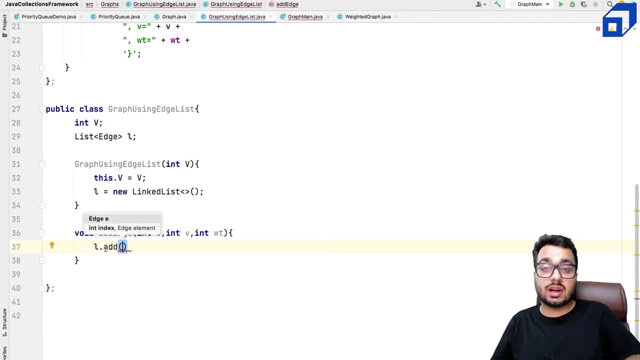 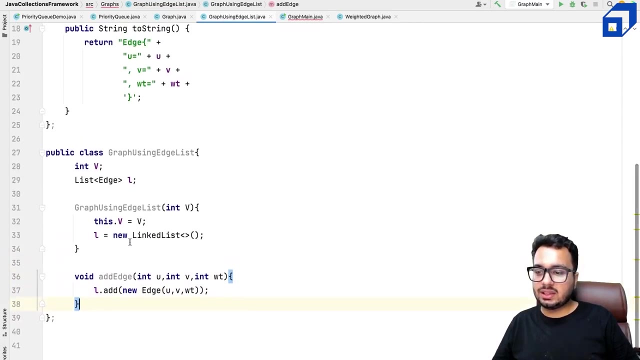 um l dot add what i should add. i should add a new edge which goes from u to v and is having a following weight. so i'm doing it for a directed graph. right, i'm going doing it for a directed graph. so i think this implementation looks complete to me. now let us test our 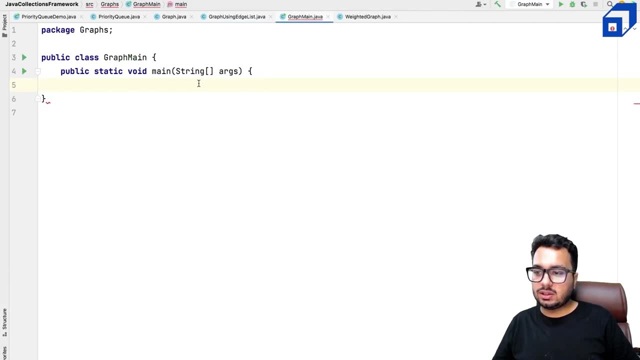 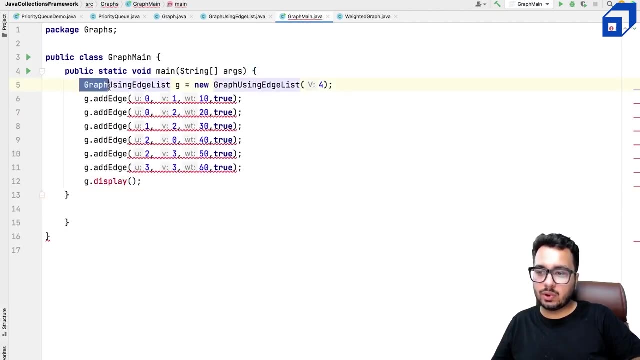 implementation by going to main right. so here what i need to do, i need to create a graph object, which i am doing right, and then i'm saying that, fine, okay. so here i've passed one more parameter which is going to tell whether the graph is directed graph or undirected graph. so this: 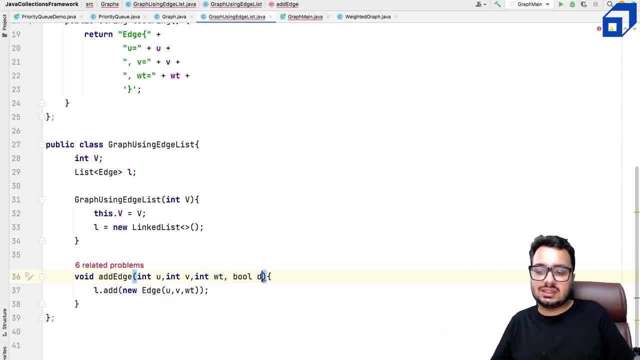 is an optional thing. if you want to accept that, okay, this is a directed graph, then you can add just this edge, but if it is an undirected graph, you also need to do one more uh line of code where you are adding the edge from u to v, right, so you are saying that? okay, a and b are connected. that. 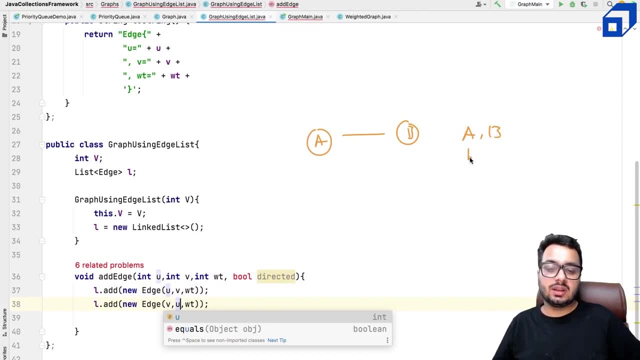 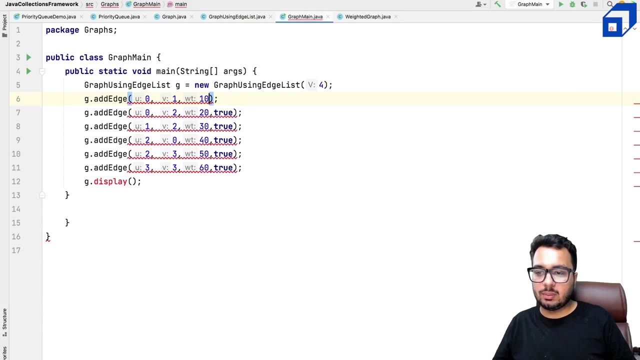 means a is a friend of b. there is an edge from a to b, but there is also an h from v to a right, so you can do this thing in case of undirected graph. that can be handled by putting a if condition here. but for now i'm keeping things simple and i will modify this code a little bit earlier. i did it for. 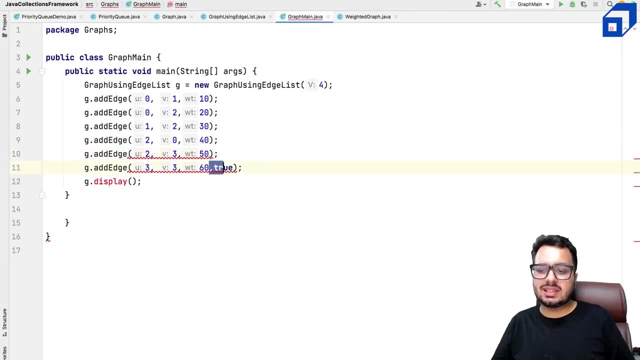 undirected graph. right, so it's. it's just a signal, the graph, whether you want to add this edge, like one time or two times. right, and now i want to display the graph. i basically want to display the edge list, so i created a graph object using this class. new graph: i initialize the number of: 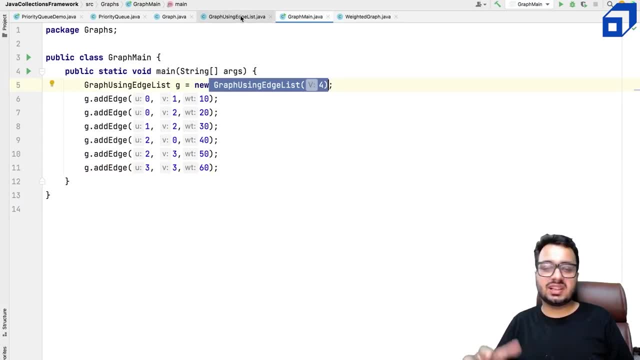 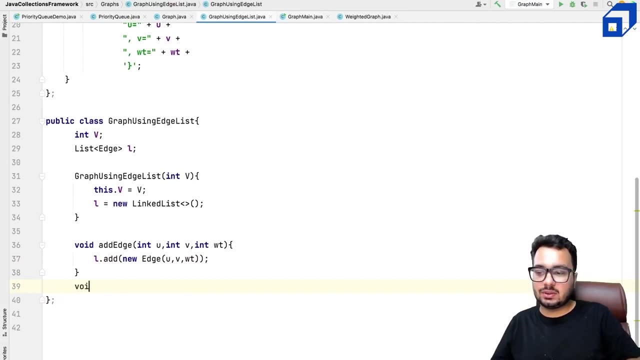 vertices, which actually we are not using as of now, but this might be helpful in future, right, for some other use case. now, if i want to display this edge list so i can say, okay, void display, okay. or let me see if i can do a two string thing here, right, so here i'm going to modify this, right. 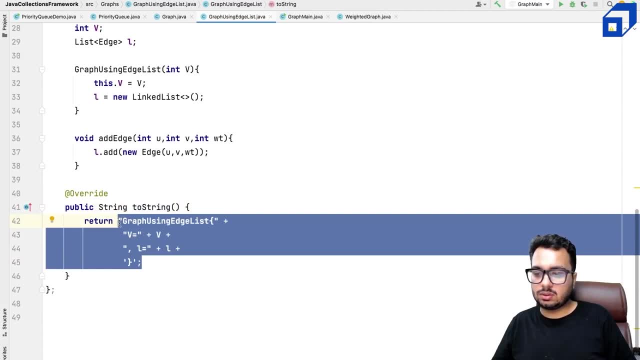 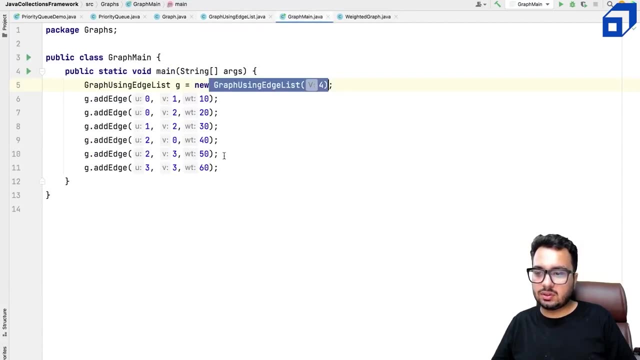 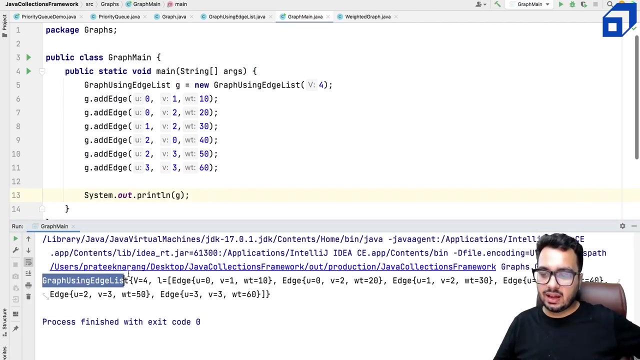 i'm going to, or this is fine, actually, this is fine, so it is going to return a list. let's see what does it return. right, i'm going to say s out graph. show me the graph, right, so let's go and run this code. okay, so this graph says that. okay, i? i know two things. i have vertices, which are four. 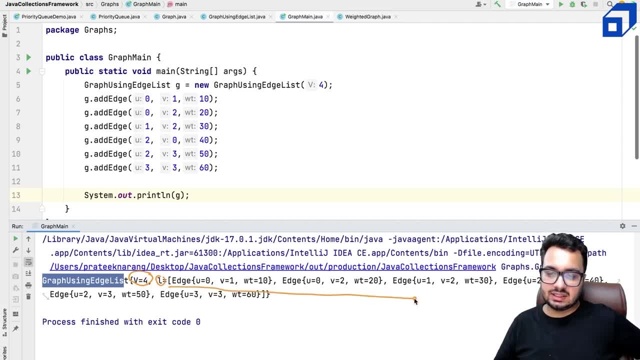 and i have a list of edges, which is this list: okay, there is an edge from zero to one with weight 10. so, zero to one- weight 10, zero to two weight 20. zero to two weight 20. one to two- weight 30. right, so you can see, this is completely fine and we are able to see, uh, the edge list that we have. 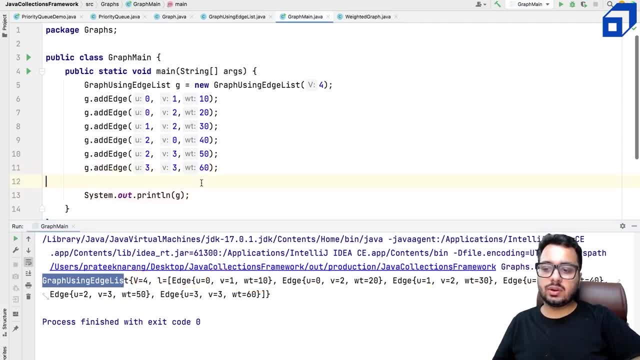 implemented. that is the idea behind edge list. now you can use this edge list to do sorting. so right now i have hard coded values here. but what you can do, you can ask the number of edges, put a for loop, take input those edges and inside the loop you can call this function. 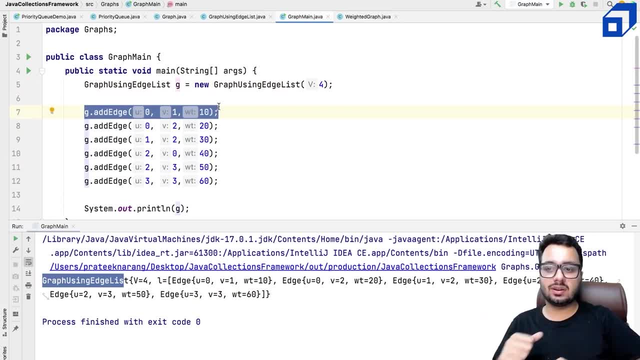 g, dot, add edge, and this is going to add all the edges in your graph, right then? generally, i've discussed how the input is given. number of nodes is given, number of edges is given, followed by list of edges, is given, right. so pairs like 0 comma, 1 comma, 10, followed by next pair, 0. 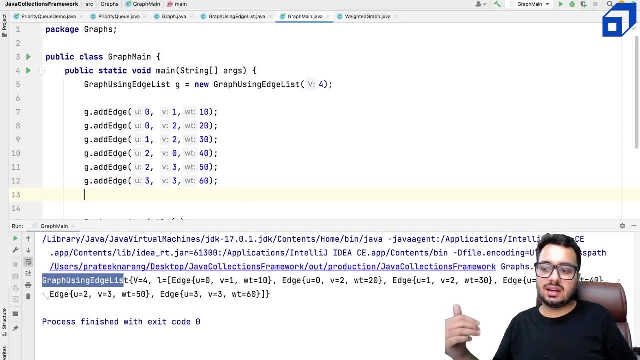 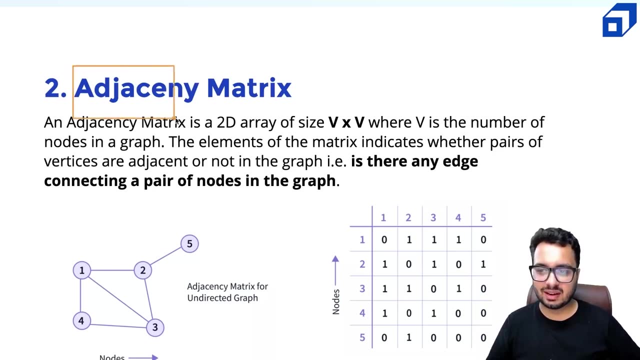 comma 2, comma 20: right, this will be input. you can scan it and call g dot, add edge to add it in your graph line. so i hope this representation is clear. next we will discuss another implementation, the next representation of a graph. it is called as adjacency matrix. 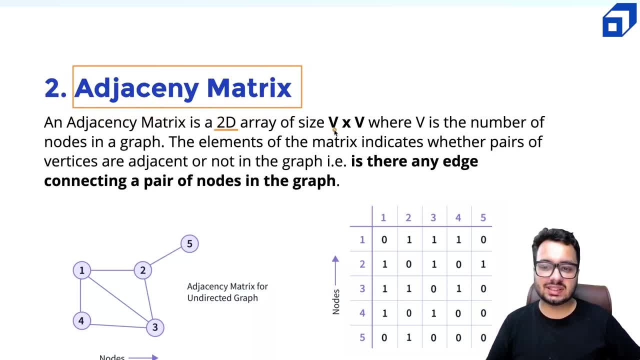 so what is this? it is a 2d matrix which is of the size v cross v, where v is the number of vertices of the graph. the number of elements in the matrix indicate whether pairs of the elements of the matrix, actually not the number of elements. the element of the matrix indicates whether pairs. 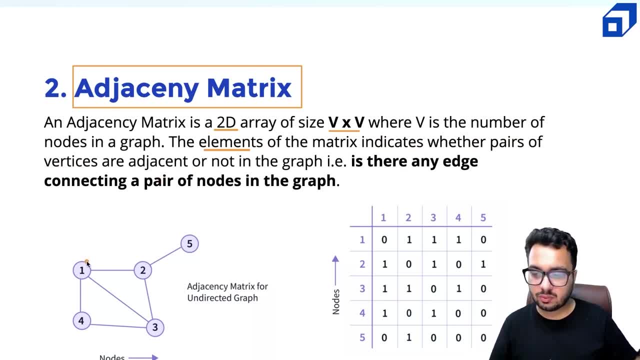 of vertices are adjacent or not. basically, if there is an edge from one comma two, right. so what we will do, we will have a adjacency matrix, okay? so in this case there are five nodes, so there is a 5 cross 5 matrix, right, and there is an edge from 1 comma 2. so what we are doing, 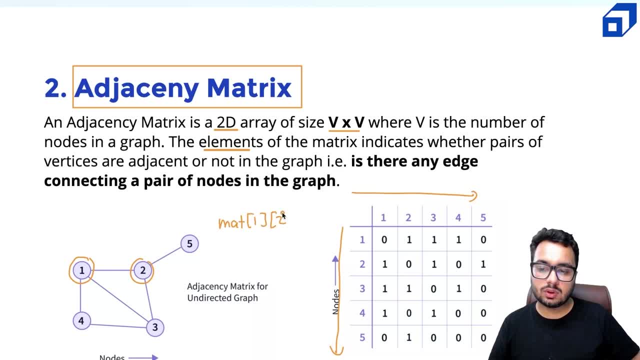 we are saying that matrix of 1 comma 2 will be true. so if it is a unweighted graph, there is no weight, so i can simply set this edge as true. so 1 comma 2 is true, or it is 1 right and similarly. 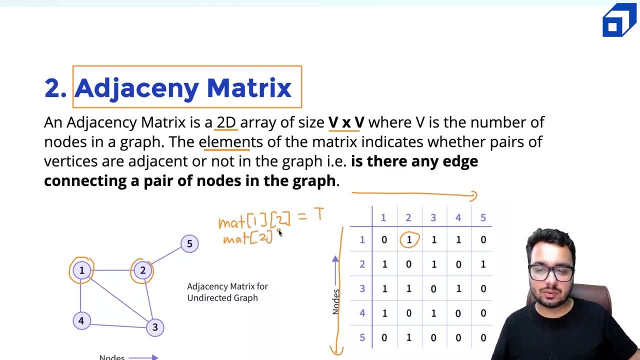 if it is a undirected graph, there is no direction. so matrix of 2 comma 1 is also true, right? so this value is also true. so this value 1 comma 5, this is 0. so this basically indicates there is no edge from 1 to 5, right? so if there is an edge from x comma y, then in in my matrix, matrix of x comma y. 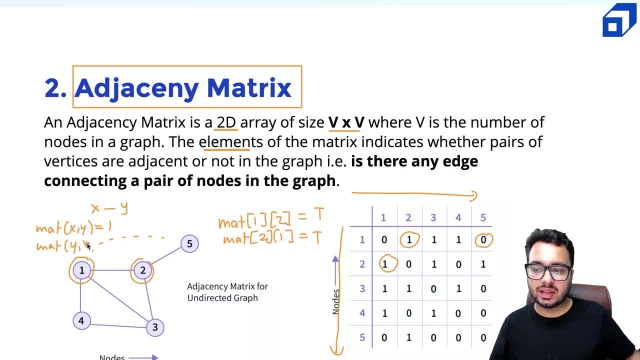 will be set to 1 and matrix of 1 y comma x will also be set to 1. that indicates that x and y, they are connected right. so this is pretty simple, and the problem with this approach is that as your n grows right. so if let's say, you have thousand nodes, 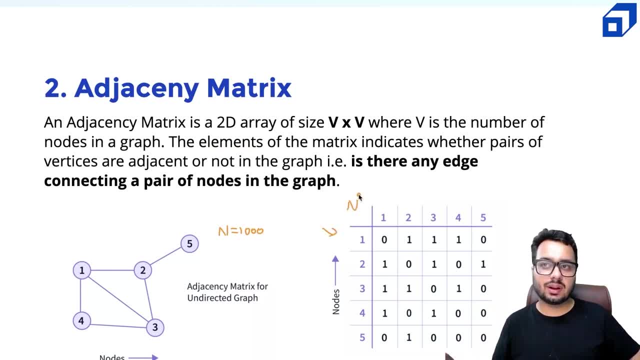 right. your matrix will be of the size n- square right. that means it will have 10 power 6 elements. so if n is, let's say, 10 power 7, your matrix will be of the size 10 power 14. you won't be able to. 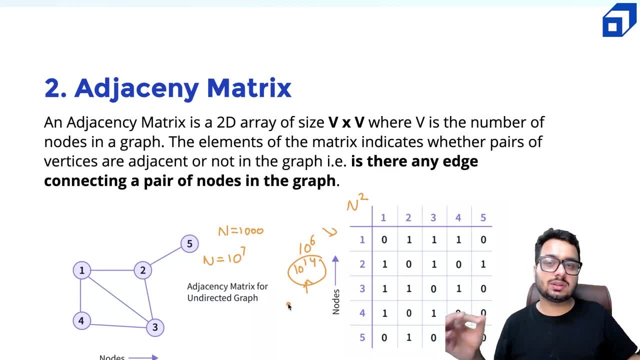 hold this big matrix in your memory, right? so it is not suitable for large number of nodes. okay, it is suitable for small number of nodes, but again, there are certain advantages and disadvantages for this right. one is one disadvantage. one disadvantage for this right is that n is not suitable for large number of nodes. 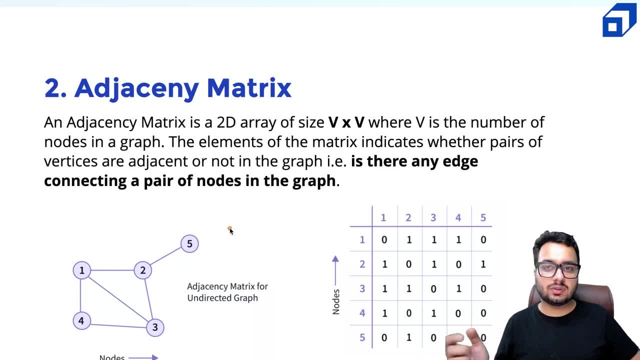 is that you are going to waste a lot of space. so in most of the graphs, if you have n nodes you might not have n square edges. that means lot of zeros will be there in the matrix, which is leading to space wastage. secondly, if you want to find neighbors of one, what nodes are connected with one? 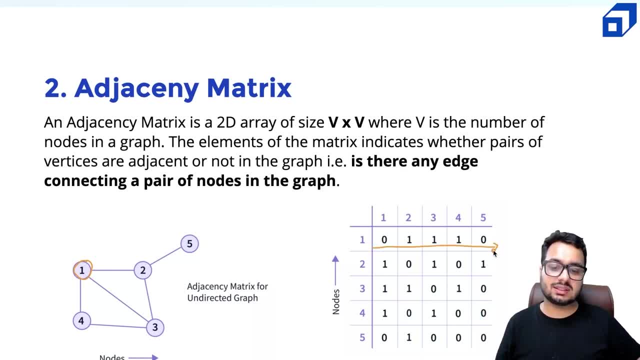 there is no way you have to iterate over this whole list, which is going to take order of uh. order of v time. right, because there are v vertices here, you have to go to each vertex and check whether one is connected with it or not, right? that is again a problem we do not want to. 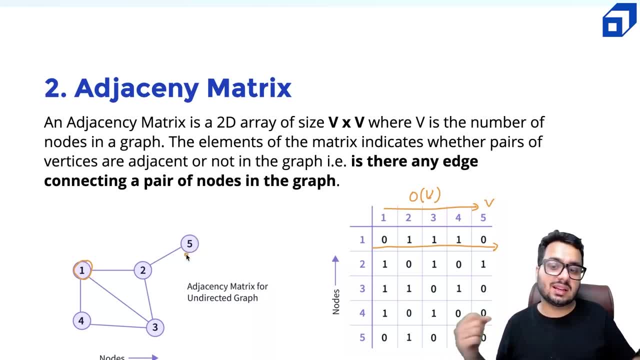 go to five because one is not connected with five, but we are still iterating right. so this is a major disadvantage. that means you cannot get neighbors of a node. in order to get neighbors of node, you have to spend order of free time, which is not very efficient operation right. 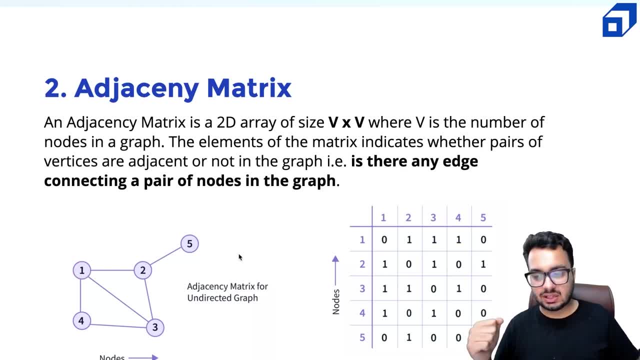 but there is one advantage as well. what is the advantage if i have to check if there is an edge between one comma three, eight, so that check can be order one? why? because you just need to go to one comma three, this index, and check: yes, this value is one, so you can check. yes, this value is. 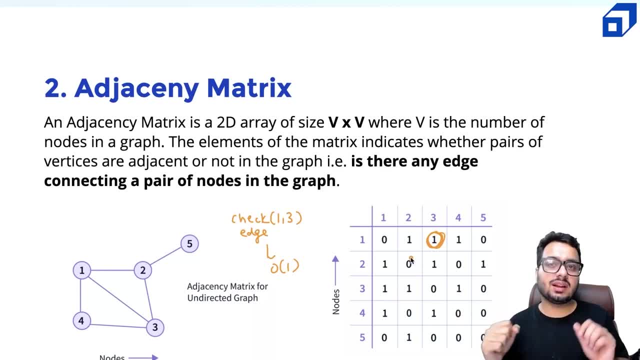 one. so that means i can figure out whether an edge is present between two nodes or not in just order one time. right now you might ask what if the graph was a weighted graph, 1 comma 2 was having, let's say, w weight. in such a scenario, instead of storing 0 or 1 here, you will store 0, followed by weight. 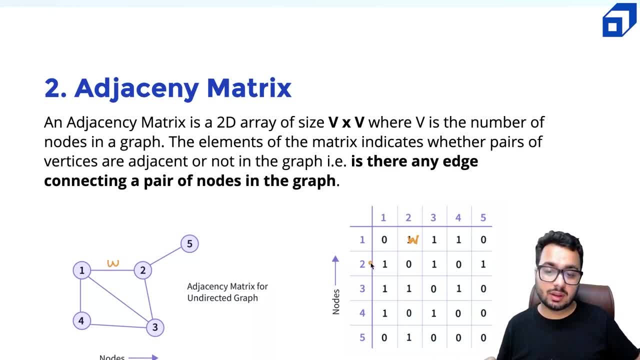 right 0 and weight. so 1 comma 2 has having w weight. so 2 comma 1 is also having w weight right. so you can store integer values. 2 comma 5 has 8 weight, so 2 comma 5 you can put this value as 8. 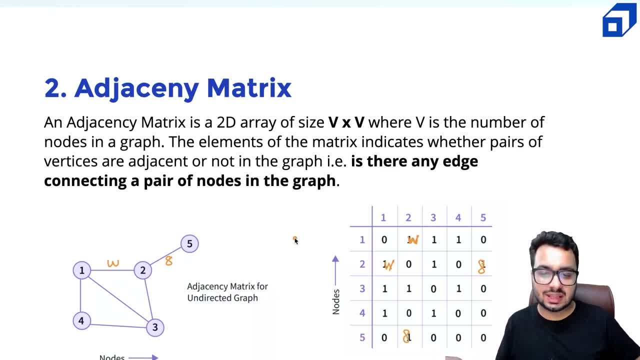 and 5 comma 2 has also it right. so, depending upon the use case, this matrix can be integer matrix or it can be a boolean matrix, right? so i hope you understand the concept of adjacent and c matrix. now let us look at the implementation of adjacency matrix. let us 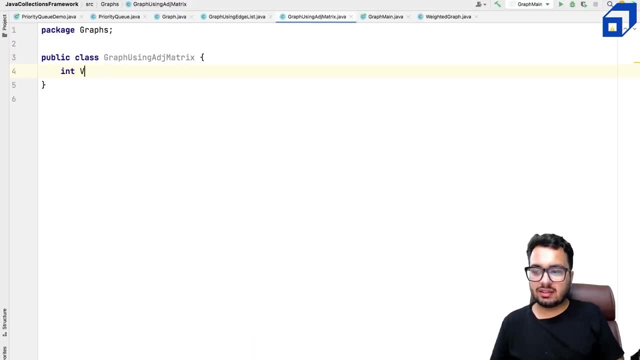 implement graph using adjacency matrix. again, i will have to keep number of vertices and i will have to keep a boolean matrix so i can say a boolean, some matrix, let's say, called adjacency matrix and we will initialize this matrix in the constructor right. so i have graph using adjacency matrix. i'm getting the number of vertices. this dot v equals v. 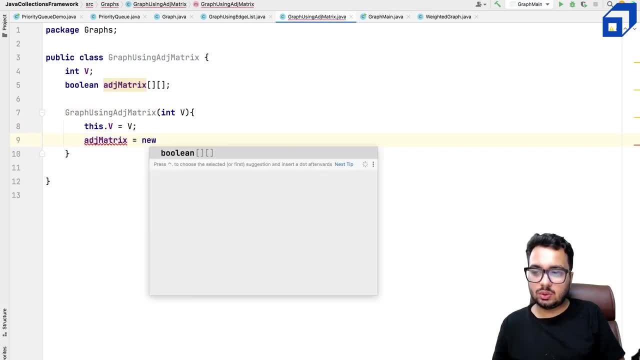 and adjacency matrix equals new boolean of the size v cross v. so i hope this matrix, this initialization, is clear by default. i think all the values would be false and now we can write the add edge function right. so i'm not going to take the weighted graph because i've taken a boolean matrix. 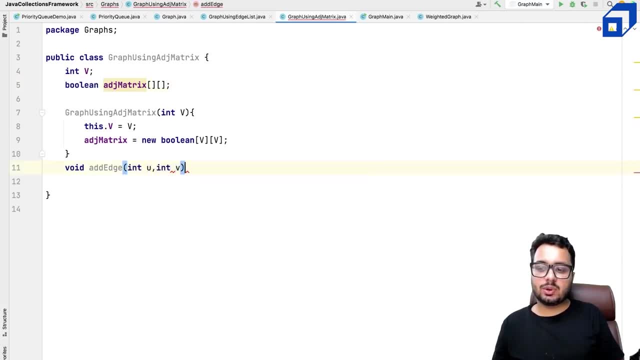 so i will take only two parameters: the edge from u to v, and also, i'm assuming the graph is a undirected graph, right? but if you have a directed graph then it is even easier, right? so if there is an edge from u to v, what i need to do in the matrix? 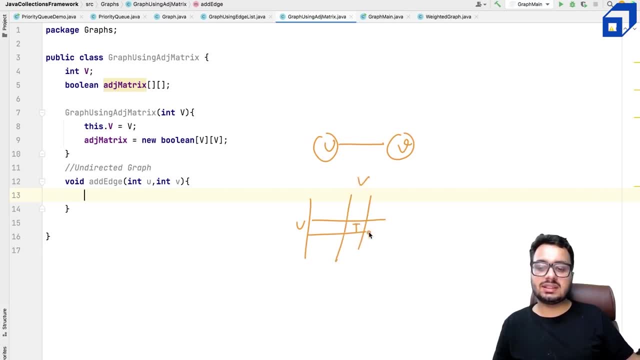 for the u-th row and the v-th column. i need to mark this as true, so i can say: adjacency matrix of u comma v will be marked as true. rest, everything is false, right. and adjacency matrix of v comma u. this is also true, right. so the other way around we also have to do right. 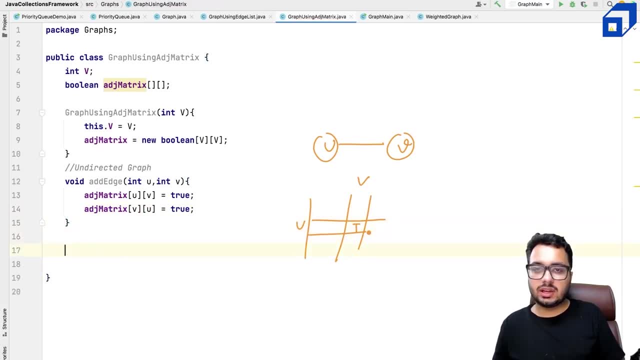 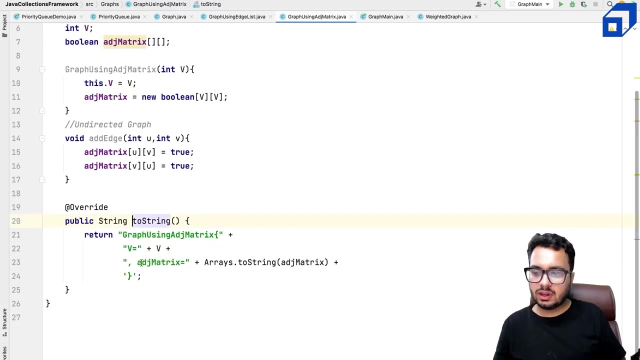 so that's it now, what we need to do. we need to test our code right. this adds an edge to our graph. and now we can have a display method, right, that is going to display the matrix. so i can add a two string method here which is going to display the vertices and the adjacency. 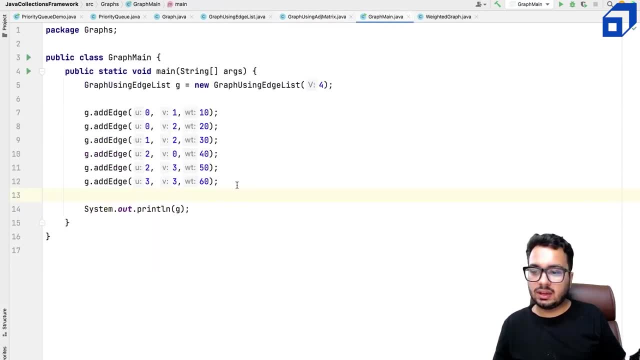 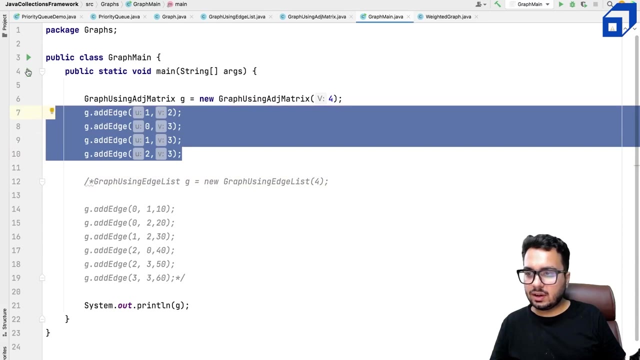 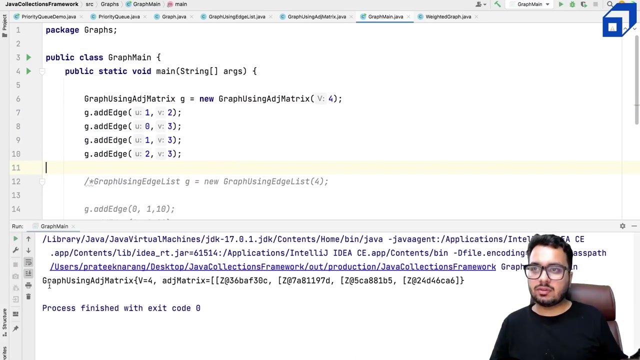 matrix. let's go to main here and now. i have to create a graph using adjacency matrix. i've added few edges and now let us go and run this code and let's see what output do we get? now we are getting okay. in this graph, object we have four vertices and now adjacency matrix is: 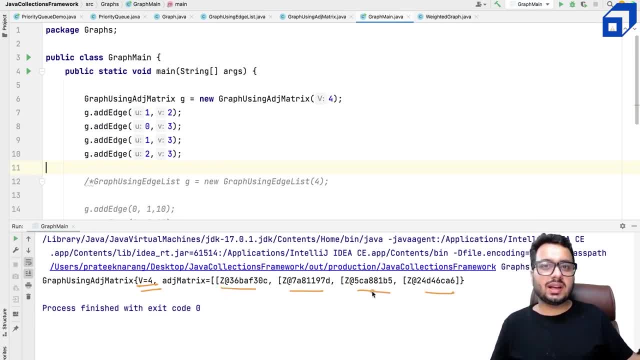 being displayed like this. so this is actually how a 2d array is stored in java, right? so if i talk about a 2d array, a 2d array is a 1d array of rows, right? and each row is actually point is storing. 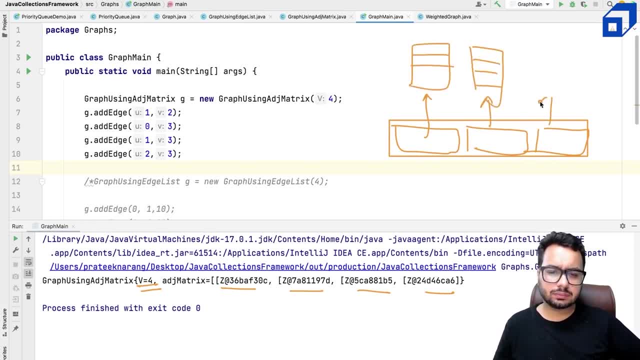 the address of an array. right? this is how it is being done. right? this is how it is actually done. 2d array is an array of rows. row is, let's say, this row is 30c. this is 97d, right? so what we are printing is we are printing. 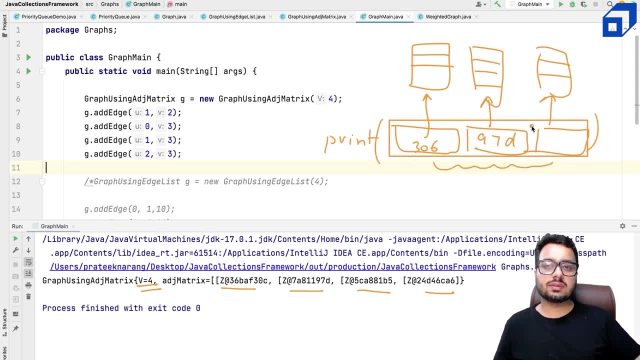 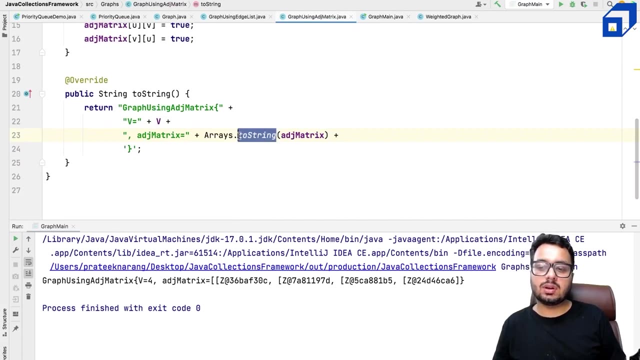 the address of each row of the array, right. so this is the address of a 1d array, 0th row, first row, second row and third row, if i want to handle this uh in a correct manner. so i have to say that we do not want to convert this 2d matrix into string directly. we have to use a method called. 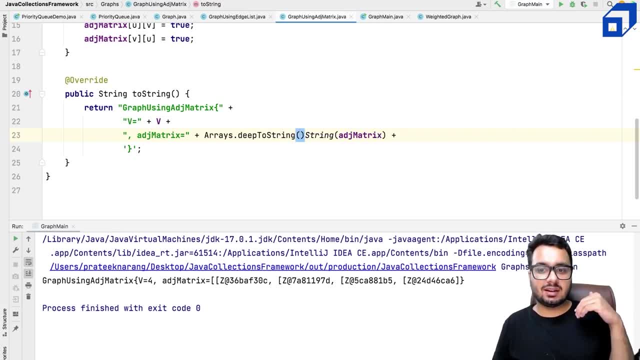 deep to string. that will actually iterate deeply into each row and then it will print: convert the contents into the string, right? so i'll do it like this. this will actually give me the string like representation of the full 2d array. right? let's go and run this code. 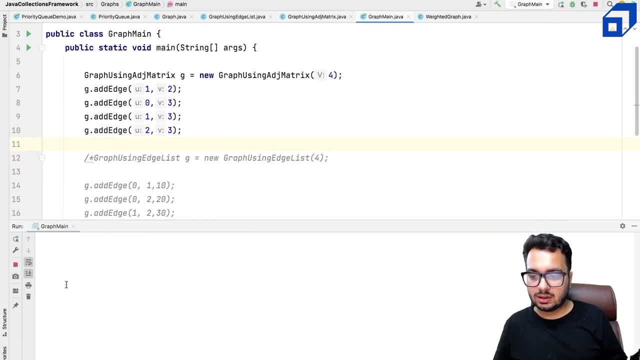 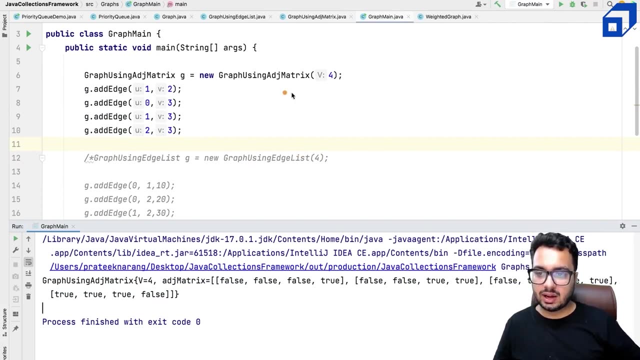 once again and see what do we get. yeah, this time i'm getting the correct adjacency matrix, so i will draw it for you. so what i did? i give four vertices. let's say 0, 1, 2 and 3. then i said 1 and 2 are connected. 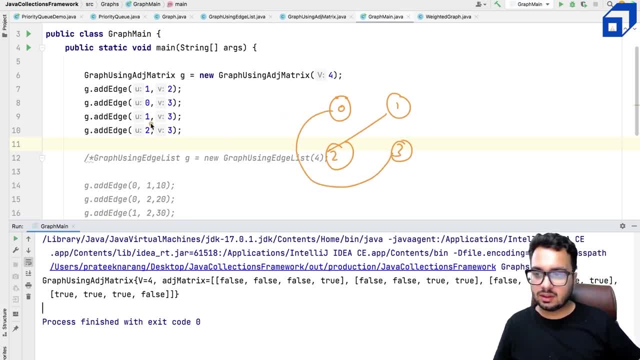 fine: 0 and 3, they are connected okay, 1 and 3 are connected okay, and 2 and 3, they are connected okay. so this is how the graph looks like. and then i have a 4 cross, 4 matrix: 0, 1, 2, 3, 0, 1, 2, 3. so it is false, false, false, true. so here i have a true here: false, false, true, true. 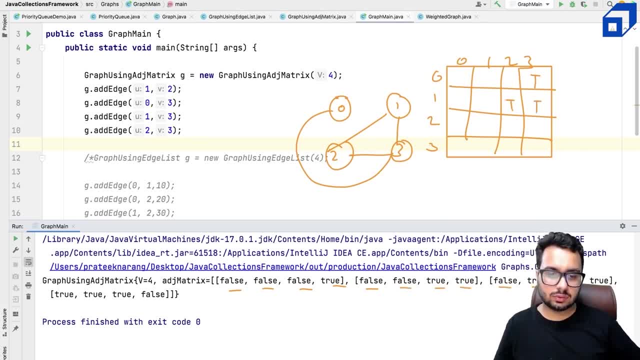 so here i have true, true, false, true, false, true, so true, true. then i have true, true, true, false, tt. if you look at this, zero, so zero is only connected with three, so we have a true here. then look at one: one is connected with two and three, so one is connected with two and three. 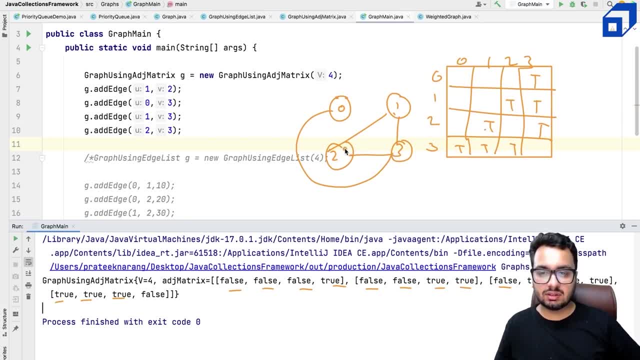 look at two. two is connected with one and three. two is connected with one and three. correct. look about three. three is connected with zero one, two. so zero, one and two. yes, this is a correct representation of the adjacency matrix for this graph. i hope you understood this concept pretty. 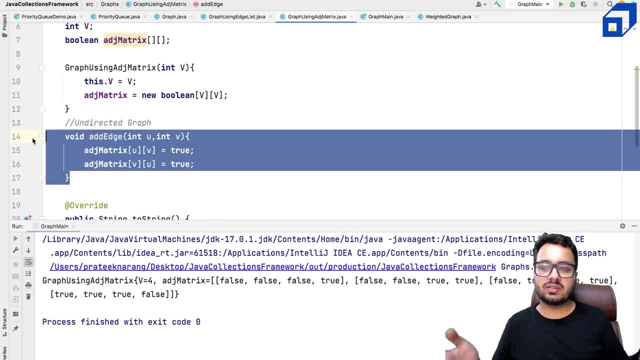 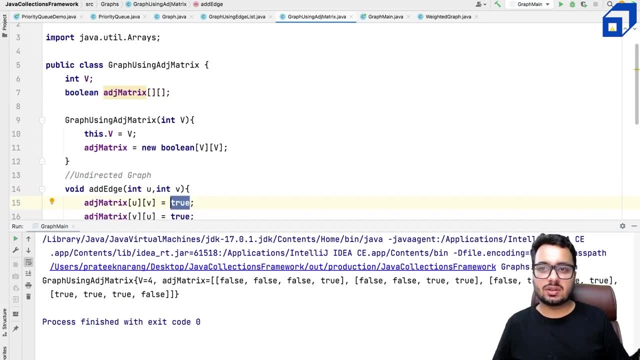 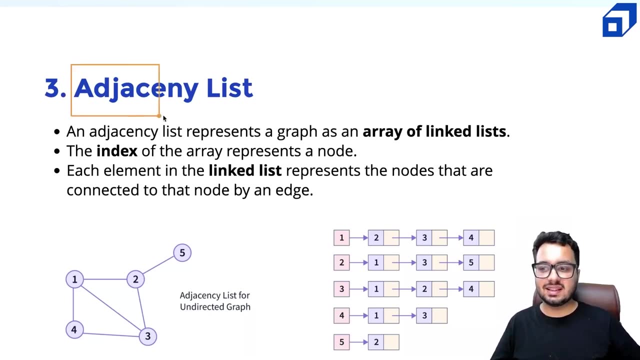 easy, nothing fancy in it, and you can easily modify the code for a directed graph by making this as a integer matrix and putting the weight here right. so that's all. next we will discuss adjacency list. now let us talk about one more implementation of graph that is called as adjacency list. 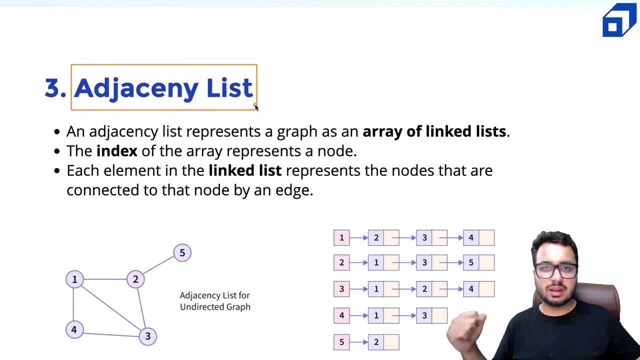 this is the most widely and most common used representation in many graph algorithms. what do we do in this representation? the adjacency list represents a graph as an array of linked lists. the index of the array represents a node. so we will try to understand now. suppose i have. 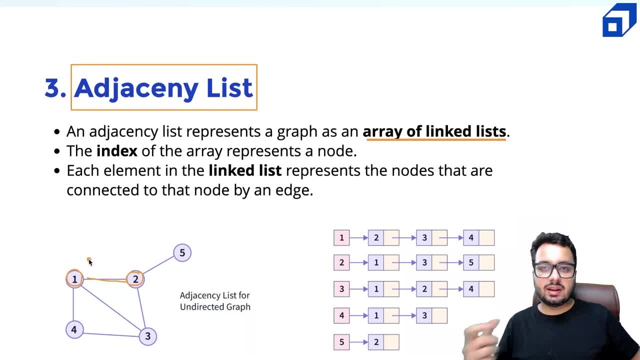 one, two, two. there is an edge, right. so what i really want to do is that, with no node one, i actually want to store all the neighbors of one. so one is connected with two, one is connected with three, one is connected with four. right, basically, there is a key value mapping. 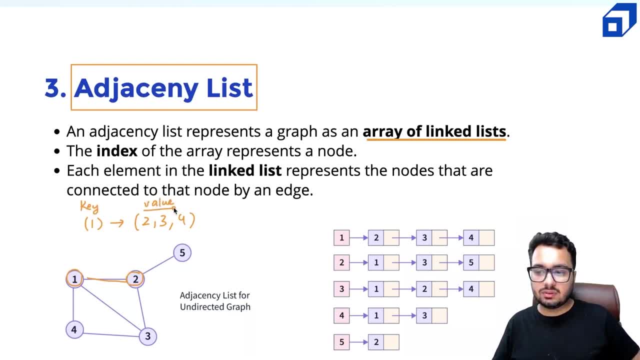 so key is one value is the list of nodes with which it is connected. one way to store it is that we create an array. now suppose there are five nodes. so here they have assumed a one based indexing. there will be a zero based indexing, right? what it is saying that it is a linked list, right? so if 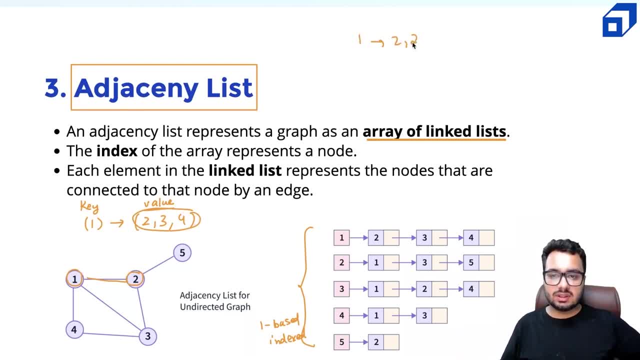 you talk about one, one is connected with two, three, four. similarly, if you talk about two, two is connected with one, three and five. so i know two is connected with one, three and five. three is connected with three is connected with four and two right so, and one also. so it is connected with one, two and. 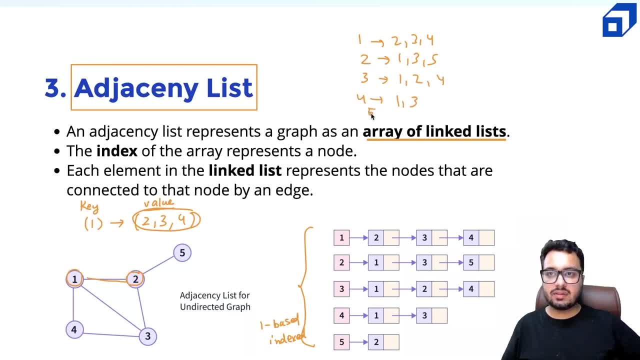 four. four is connected with one and three and five is connected with two. right, so each of this is like a linked list. we can definitely add more to this linked list, for example, if five and six are connected, so i can, okay, in linked list of five you can add six and in six at the sixth position. 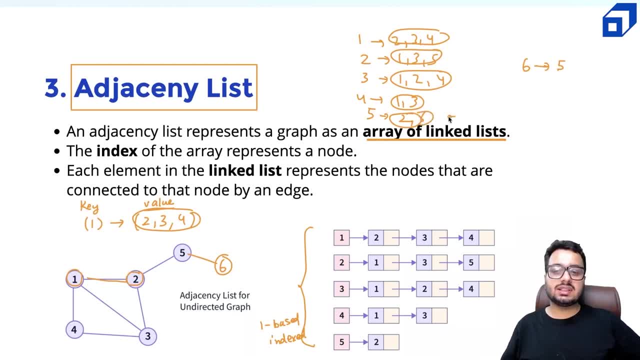 you can add five. okay, so why we are using this linked list? because it is easy to add into this, so we can easily do a add operation. right, but how many linked lists do we need? do we need one linked list? no, we need an array of linked lists. so this: 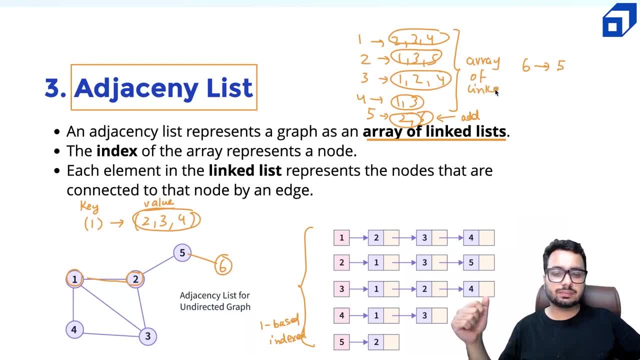 data structure is an array of linked list. right. so right now it we are assuming a one based indexing, but it will be zero based indexing. if i talk about array of one, area of one is nothing but it is a list, what about array of two? area of two is nothing but it is a list. and what does area of two denote? 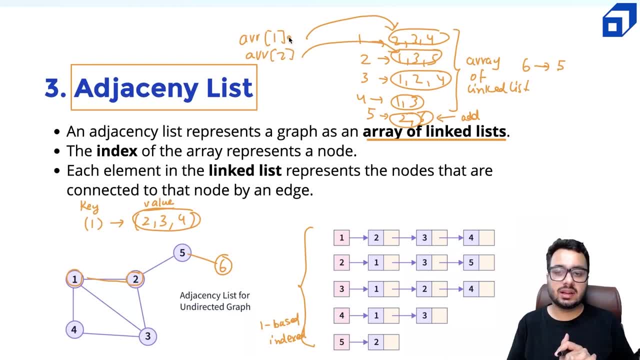 area of two denotes a list containing neighbors of two, right? so if we implement this right? so what we are going to store? we are going to store this, this, this, this, this, and we are going to form an area out of it, right? so this is what an array of lists look like. some of you might ask what happens if nodes are not. 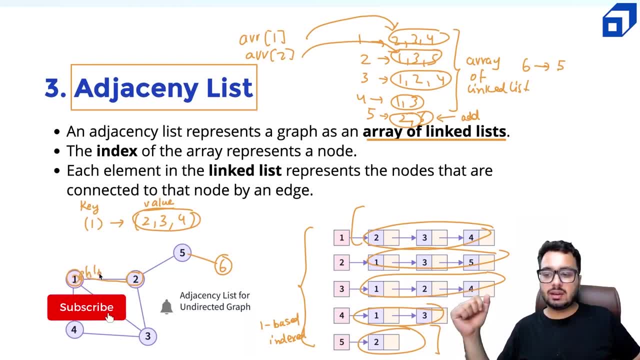 numbered one, two, three. suppose they are numbered as delhi, mumbai, jaipur. in that case, in instead of using an array of lists, you can also create a hash map where the key is a string and the value is a list of string. that is also possible, right, that is also a way to implement a 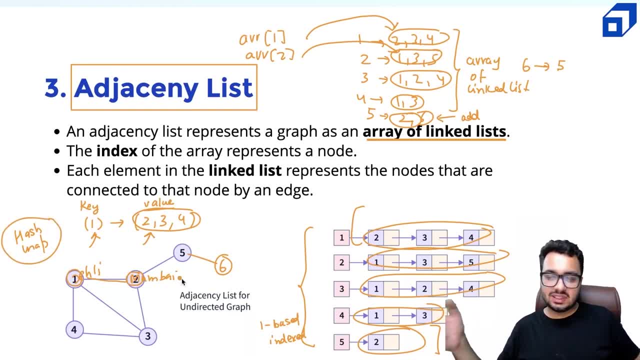 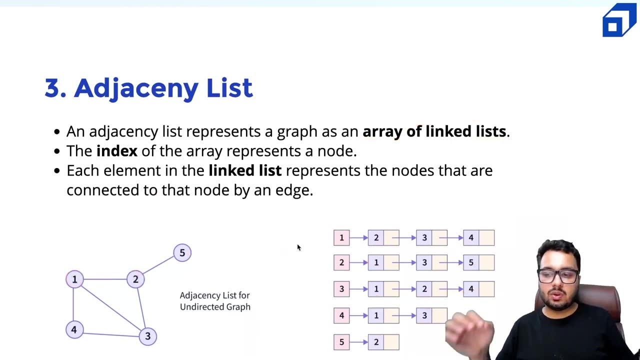 existence a list. so in in case of zero based numbering, it becomes easy, because array indexes are numbers themselves. but if you have something complex like delhi, mumbai, jaipur and the bad, you can also use a hash map in place of it, right? so i hope you are. 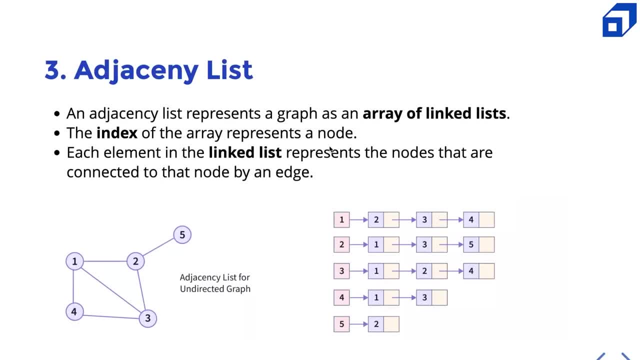 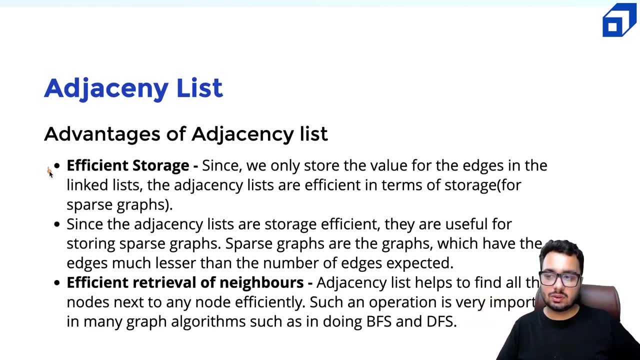 able to understand this concept. now let us talk about advantages. advantages of this representation. so the first advantage is efficient storage. we are not wasting any space, unlike we did in adjacency matrix right. we are only storing the value of edges where the edges actually exist. so it is efficient in terms of storage right. they are also useful for storing. 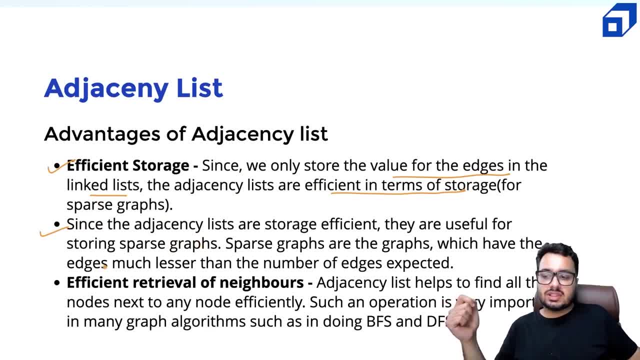 sparse graphs, that means um, which have much lesser edges compared to like what will be a dense graph. so if you have five, five edges and you have, let's say, v square edges, in that case that means every node is connected with every one. in that case adjacency matrix can be easily used, right. but if you have five vertices, 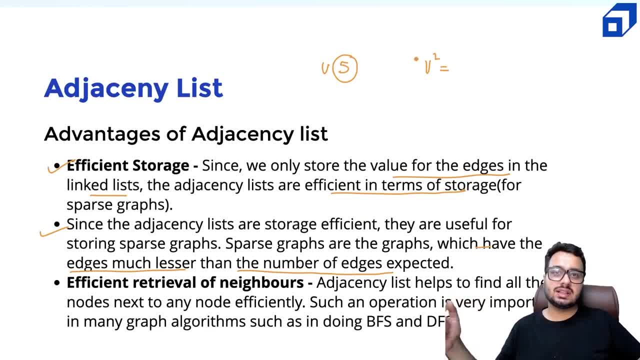 seven edges. it's kind of a sparse graph. right number of edges is much less than v square right, and the biggest advantage is efficient retrieval of neighbors. as i told you that this is an important operation than we frequently do in algorithms like bfs and dfs, we can easily find: 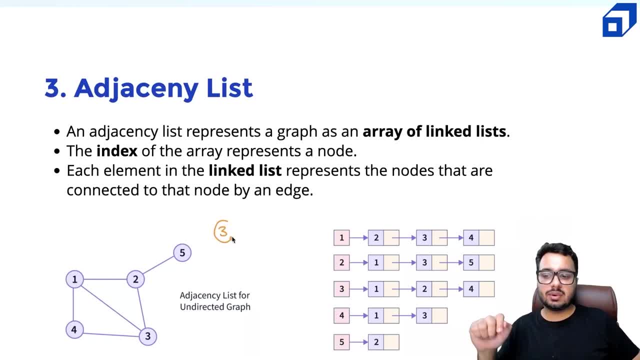 neighbors of any one node. so if you have a number of edges like this one, we can find the number of edges of any node. if i ask you, okay, find neighbors of three, what you need to do? you need to go to array of three, which is an order, one operation, and then you need to iterate on this list. so basically, in 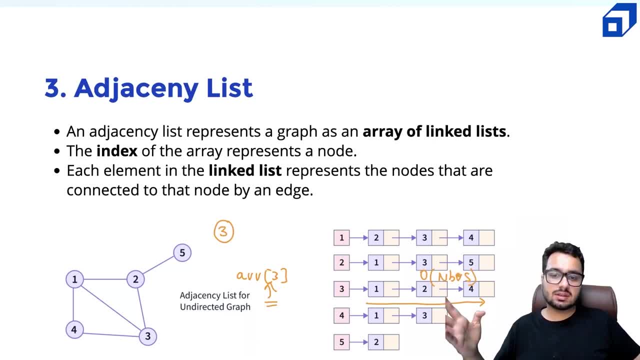 order of neighbors time. if three has three neighbors out of hundred nodes, you can get those three neighbors in three units of time. you don't have to traverse the whole list of nodes, right? so this is a very efficient operation. because of these two reasons it is a very widely 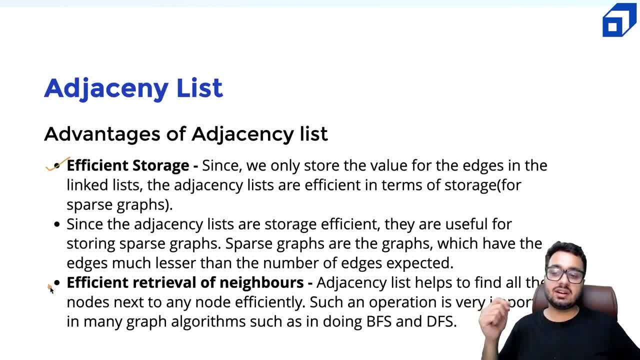 used. one is efficient storage. second is efficient retrieval of neighbors. this makes adjacency list a popular choice for graph representation and is used in many algorithms such as bfs, dfs, shortest path algorithms and much more. now let us discuss implementation of adjacency list. let us start implementing graph using adjacency list. so we are discussing. 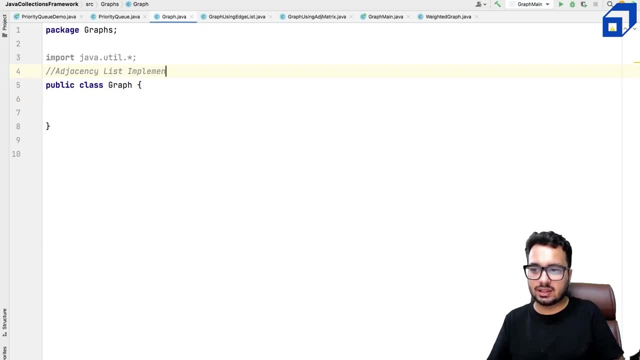 adjacency list: implementation for the graph. one thing we need is the number of vertices. next, what do we need? we need an array of linked list. so how do i create it? i can say list of what list of integers if i simply write adjacency list. this makes one list object. but i need a array. 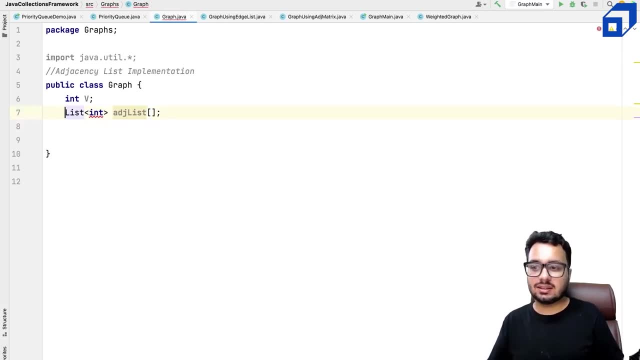 right now i need to initialize this array inside. okay, this will be integer here, right? because my collections does not accept primitive data types, so i need to initialize this object in the constructor itself. what is the size of this list? that will be known when we are creating the. 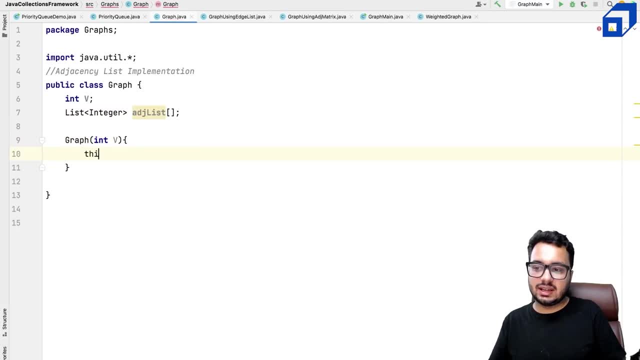 graph object. so i can get the number of vertices and i can say this: dot v equals v and i can say this dot exists in the list, this is equal to new linked list of integer and how many objects i do do i need? i need v- number of objects. okay, so i have created an array in which this adjacency list. 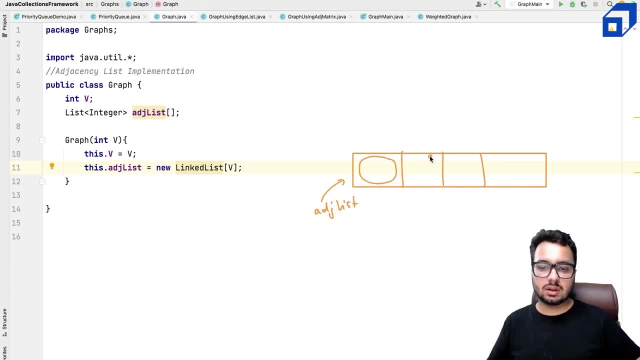 right, but right now this object is not created, right? only an array is created. so what i need to create? i need to create a linked list at each index. so how do i do it so i can? okay, i will iterate over this. i equal to zero. i list them. 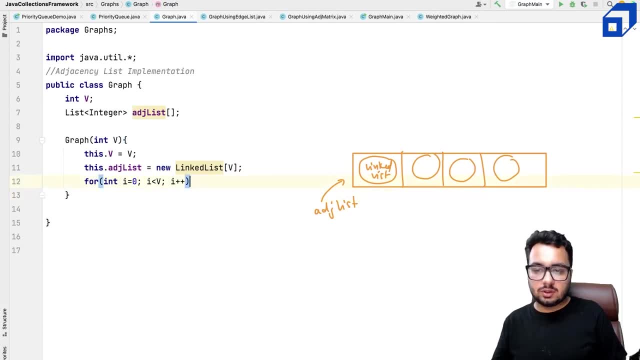 nv. i plus plus right. so basically, when i say i'm creating this area, that means the array bucket can hold the address of a linked list. but right now that is null right. so what do i want? i want this bucket to hold the address of a linked list object. how do i create this linked list object? i have to. 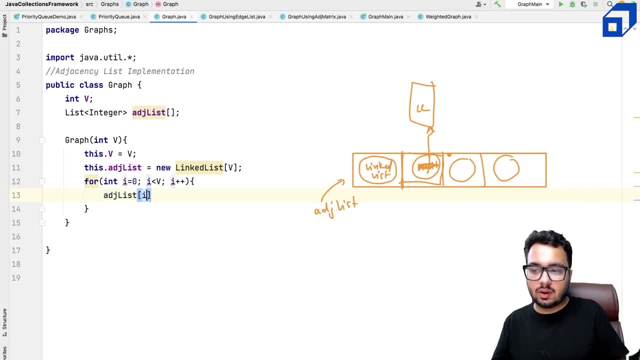 use new right. you have to say: adjacent to list of i. this is equal to new linked list. this, actually, it's an array in which each element is a linkless object. right, This is the correct way of constructing the adjacency list. Now what do I need to do? I need to add elements into the 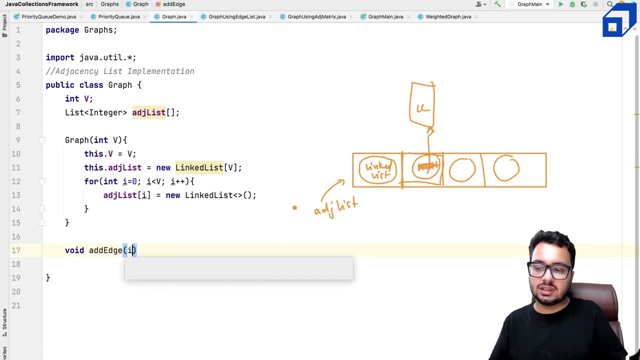 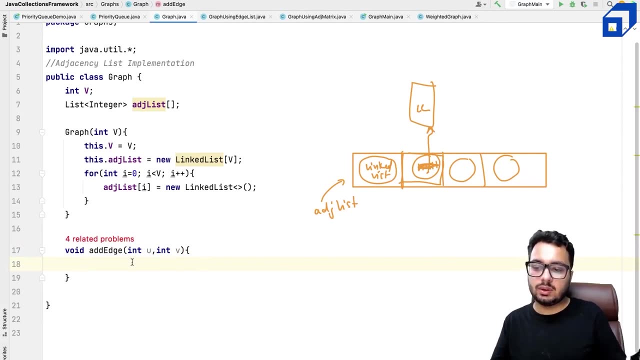 linkless right. I will have a function called void- add edge edges from u to v. what do I do? now I can say: okay, if there is an edge from u to v, what should? I will do And maybe I can. 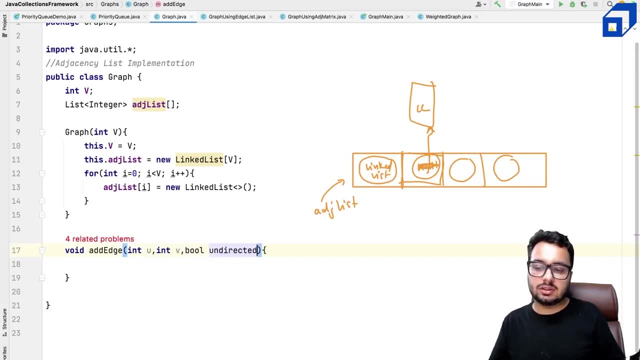 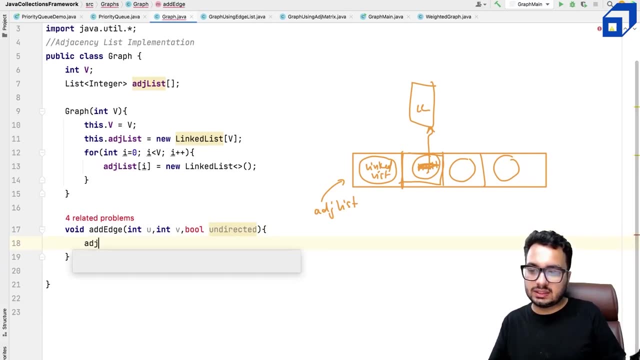 accept. is it a undirected graph, right? If it is true, I will also add an edge from v to u, right? So I can say: adjacency list of u dot, add v, something like this: And if it is a undirected: 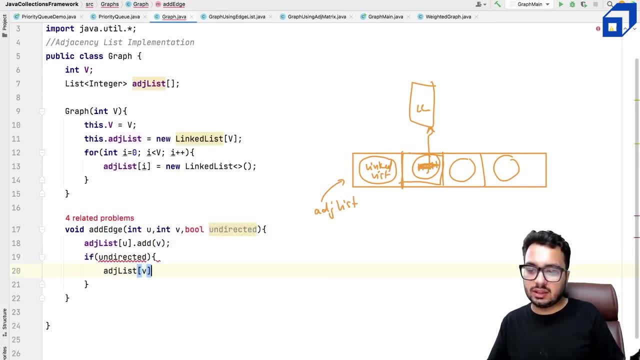 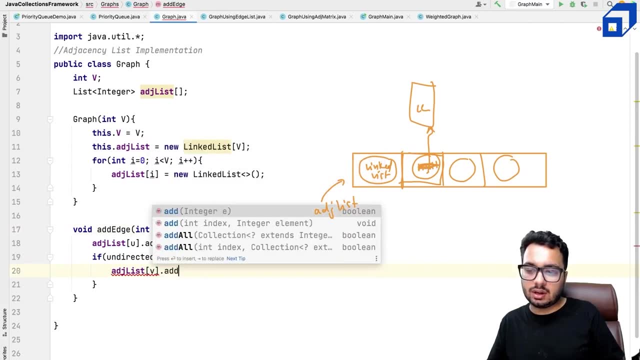 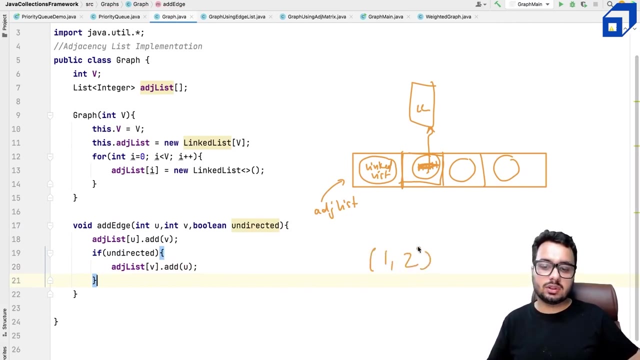 graph I can say adjacency list of v, So it will be Boolean right, Boolean C++. adjacency list of v. dot. add something like this, Basically what I'm saying, that go and add an edge from one comma two, so 0123.. So in first link list it will add two. 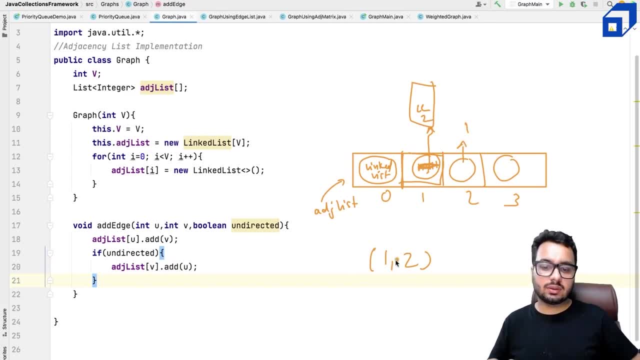 And in second list it will add one. then I say: okay, go and add one comma three. In first list it will add three, And in third list it will add one, something like this, Basically, if one is: 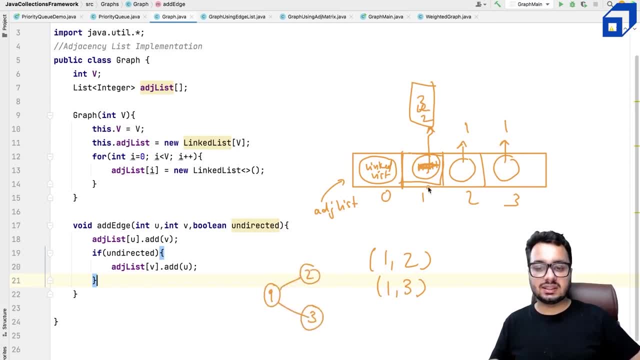 connected with one, then it will add one. So in first list it will add one, something like this: So if one is connected with two, one is connected with three. If I read this I see one's neighbors are two and three right. So if I write it a little more clearly, the two and three they have been. 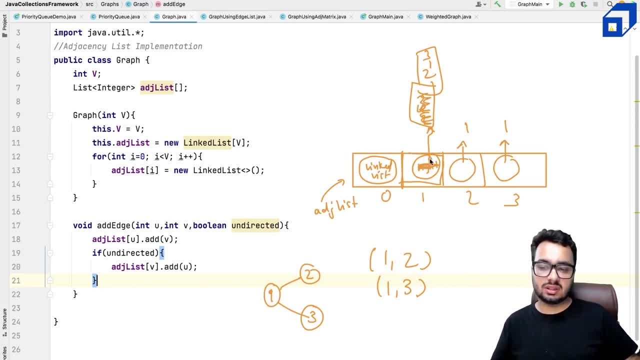 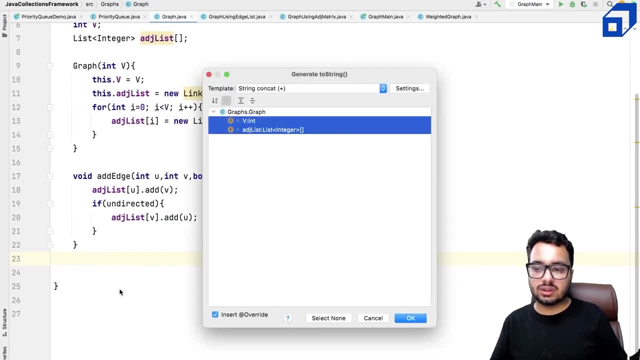 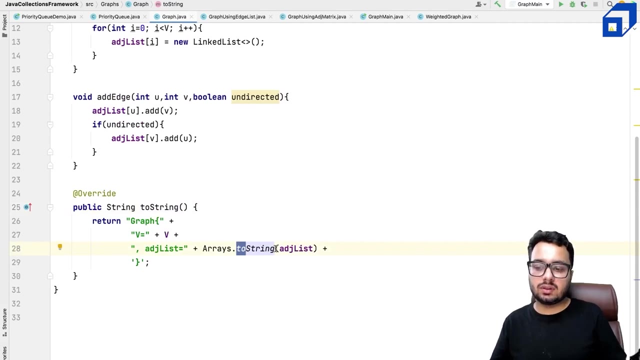 added into the link list, which is at the first position, right. So this is how the add edge function looks like. Then I can display the graph, So I can write the to string method, which is auto generated, And here, similar to the previous case, normal to string will not work. I want to. 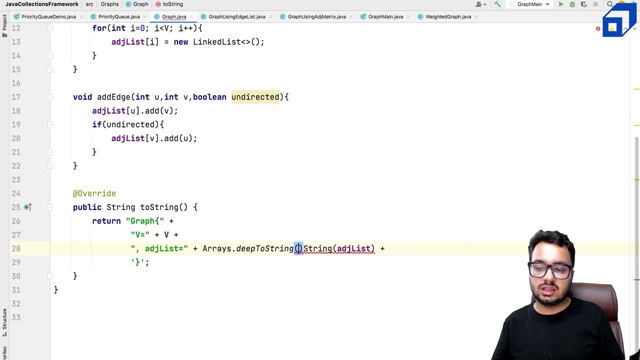 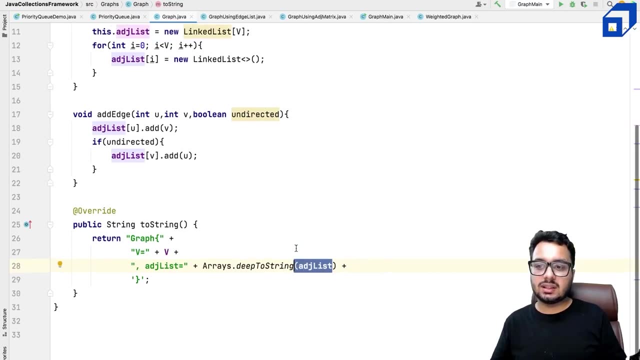 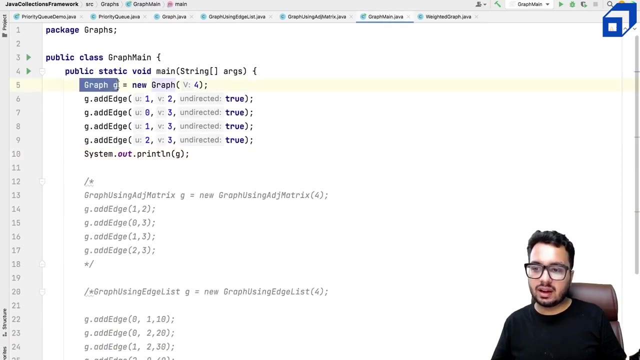 iterate deeply into into the data structure. I will use deep to string method And this adjacency list will be converted into a string, like representation, that I can print. Now let us come to our main, which is here, And I have created a graph, I'm trying to add edges in it And I'm trying to print it. So this I have already written. 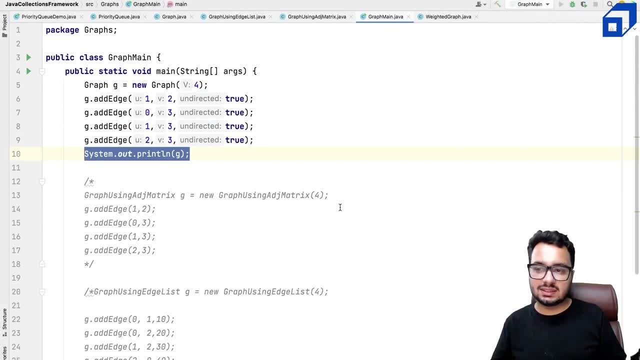 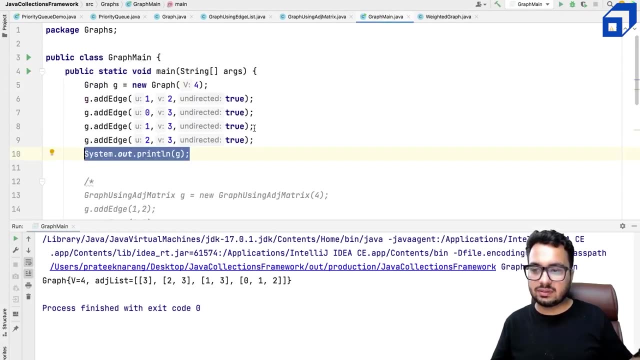 before. So I'm just going to run this And you can see the graph class we have just constructed. now Let us try to visualize this. graph One is connected with two. fine, undirected graph zero is connected with three. Okay, one is connected with three and two is connected with three. This is 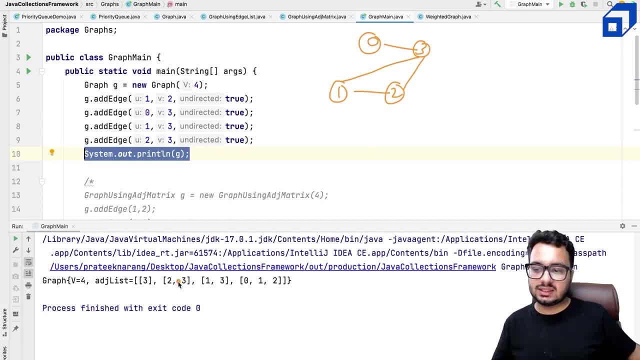 how the graph looks like. And now, if you talk about the adjacency list, zero is connected with three. okay, one. one is connected with two and three. one is connected with two and three. that's correct. So, list of one. it is storing the neighbors of. 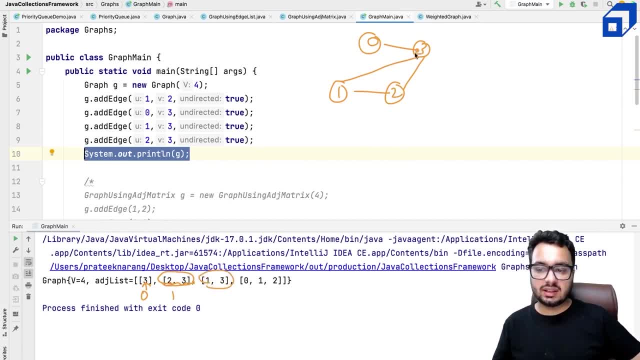 one. list of two. two is connected with one and three. Absolutely correct. What about three? three is connected with zero, one and two, So three adjacency list of three storing neighbors of three. This is how this 2d array- Okay, it's, it's. it's not a 2d And it's a. it's a array of link lists. 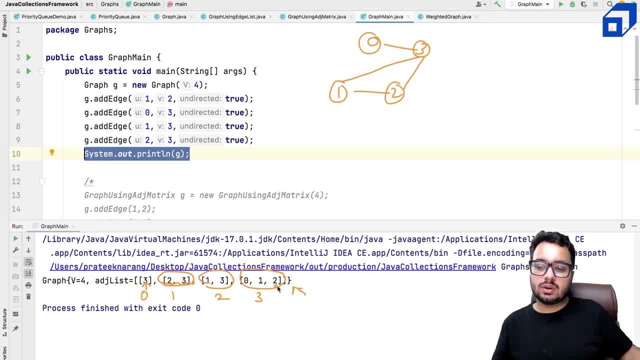 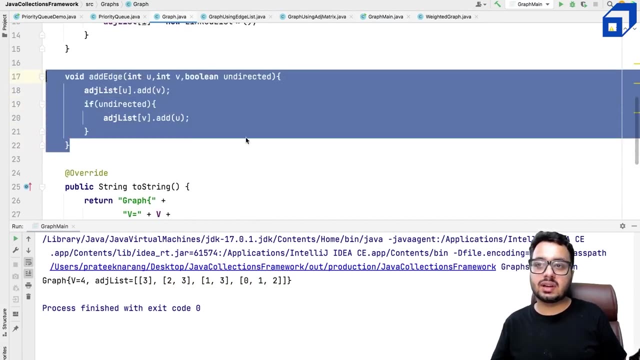 right. Each link list is denoting the neighbors of the ith node right. That is the adjacency list implementation. I hope you are able to understand this implementation. So pretty easy, nothing fancy, nothing difficult, And if you have more complex data, as I told you. 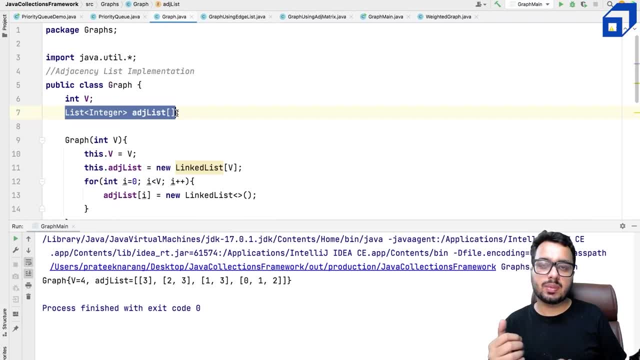 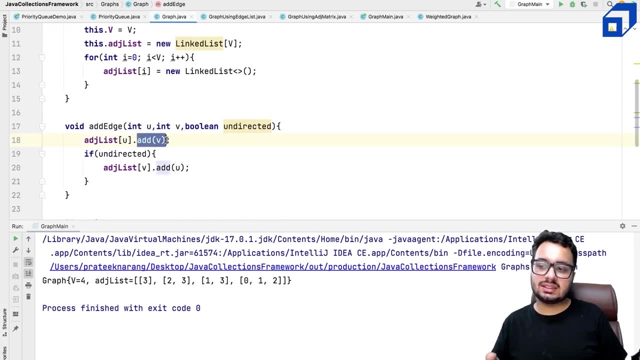 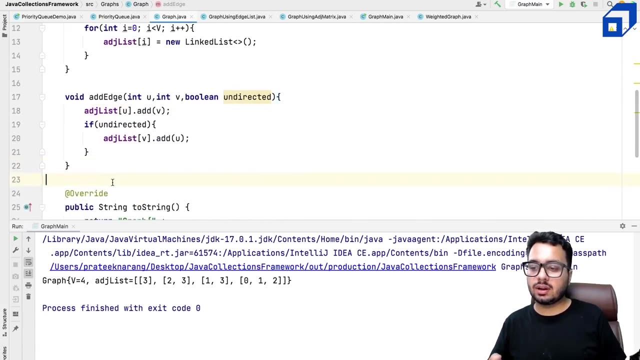 instead of having this, you can also have a hash map where key is your this: this will become your key And this will be added into the list corresponding to that key right? That's all for this implementation. Okay, so we have discussed the most commonly used implementations. 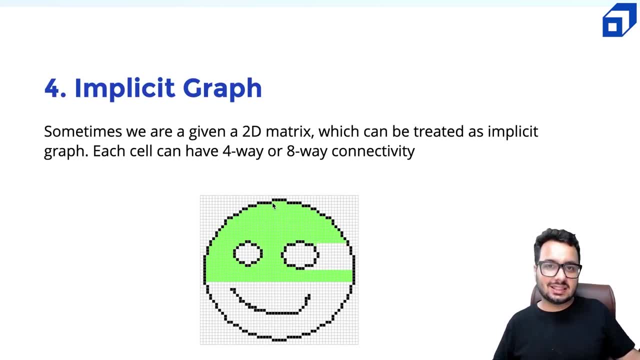 of the graph: adjacency list. adjacency matrix, edge list. there is one more representation that is sometimes convenient for certain type of problems, Okay. so sometimes we are given a graph in which we are saying, okay, there is a 2d matrix And it is given that each cell is connected with. 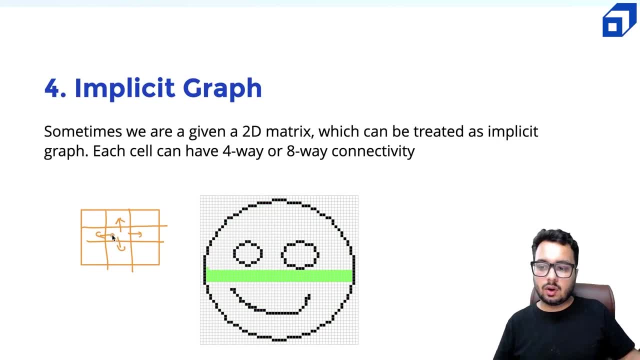 let's say the four neighbors, something like this: Or each connect cell is connected in the four neighbors which are of the similar color, right, And you have to do something right In this case, what you have to do, you do not need. 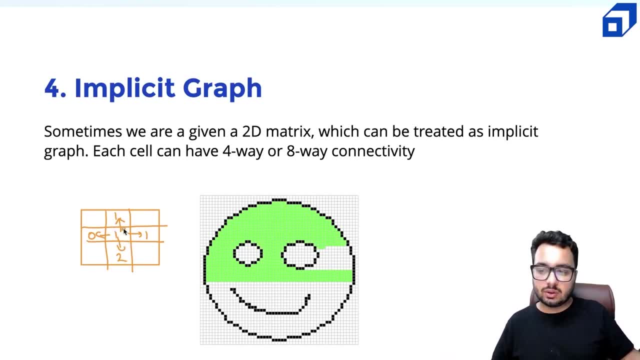 to construct a graph, you can directly deal with the matrix, right? So if I say, okay, what are the neighbors of this one? either it will be four way connectivity, it will be mentioned in the question, then you can go in these directions, Or it can be eight way connectivity. that means the diagonal. 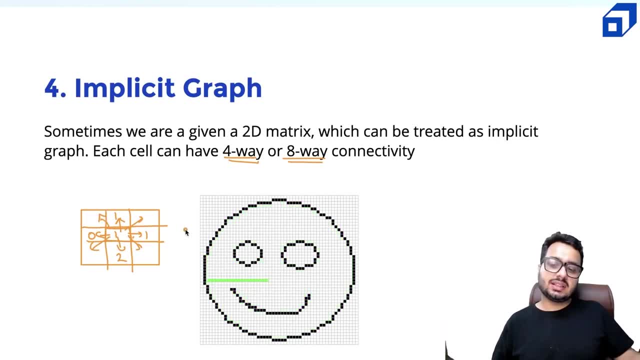 directions are also included. This kind of representation is helpful in some areas. algorithms like flood fill- right, So what is happening in flood fill? there is a two day image which is made up of some pixel values. right, So you're filling the color until you hit the. 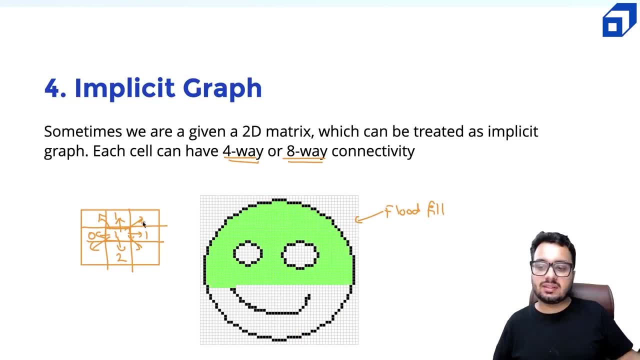 black boundary And how are you finding the neighbors? you're going in this four way connectivity or doing the eight way connectivity right. This is not possible for every type of graph But certain problems where graph could represent an image right Or the neighbors have. 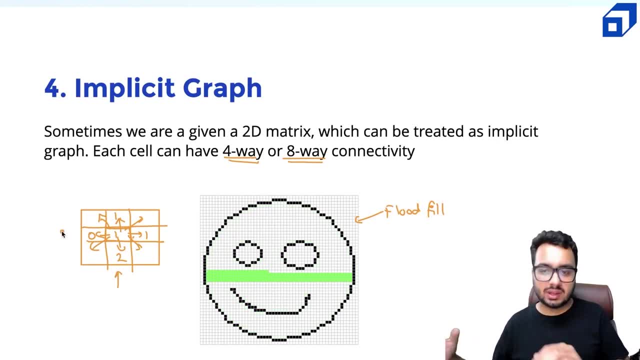 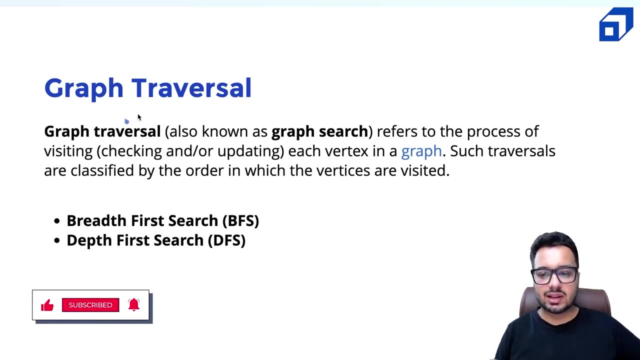 this kind of relationship where they can be represented using a 2d array, right. So we will deal with these kind of problems in the series And I hope you learned a lot of concepts from today's video. Let us talk about graph traversal First. what is actually is a graph traversal, So graph traversal, also known. 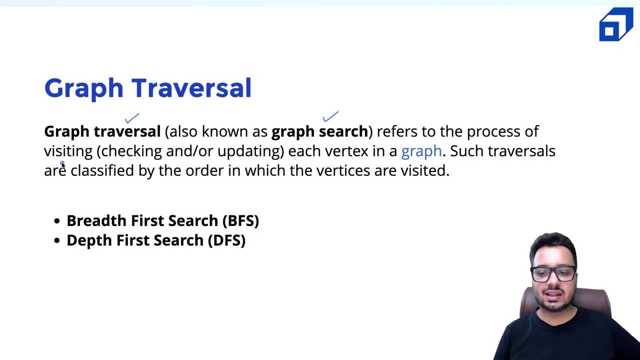 as graph search is a way or is a process of visiting each vertex in a graph. Such traversals, as I told you, are classified into two types. One is BFS, which stands for breadth first search, which is an iterative way to traverse the graph, And second one is a recursive way, called depth. 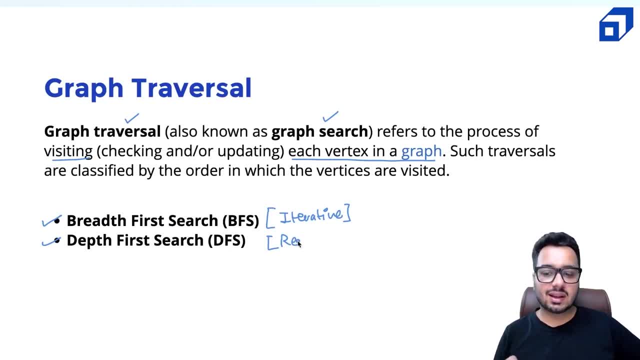 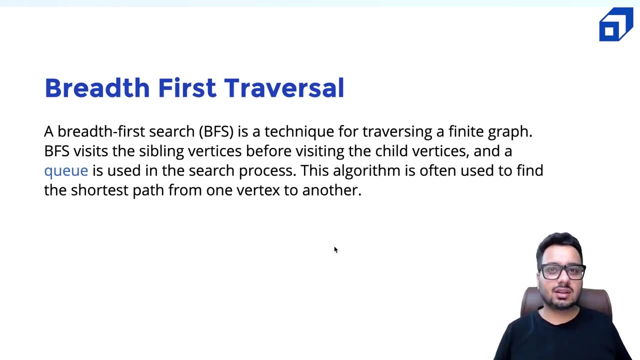 first search In this tutorial, we'll focus on BFS and its applications. So BFS actually has many applications, And one of the most commonly used application is finding shortest paths in undirected graphs. We'll also look at such applications in this tutorial. So let us start. 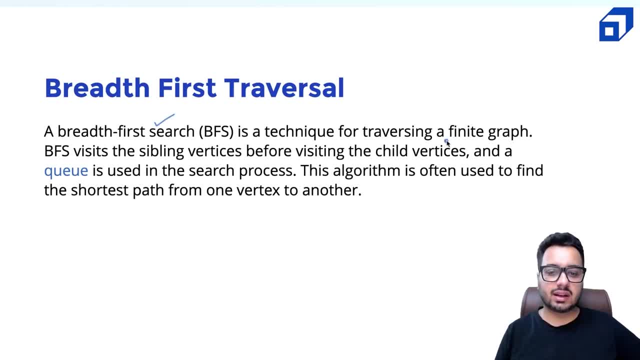 talking about BFS. It is a technique for traversing a finite graph. That means the number of nodes in the graph would be finite, And the way it works is it visits the sibling nodes before visiting the child vertices. So what does it mean If you have something like a node A and it has children like B and C, and then you 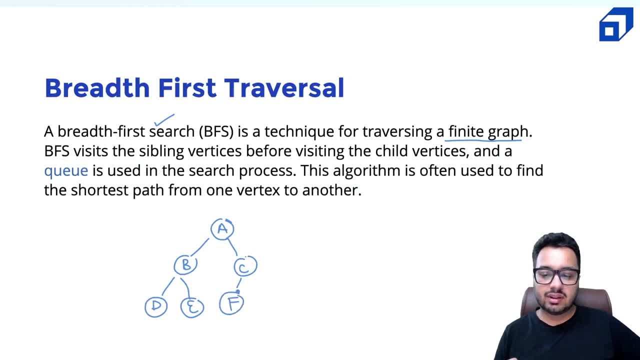 have some children like D and E and so on. The way it works is, if you look at in the form of a tree, suppose this graph is a tree. Now, this is not a tree, because I'm added one more edge here: The. 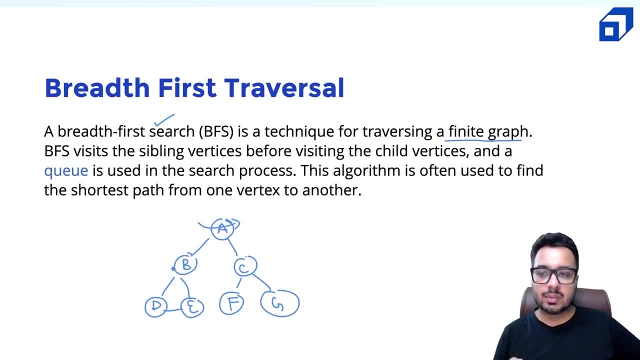 way it works is it will visit this node, then it will come at B, but it will visit sibling of B, that is C next. So it will visit BC, then it will visit D, E, F, G and so on. In a way, if you look at in the form of a tree tree, like traversal, it is like a level order, traversal. 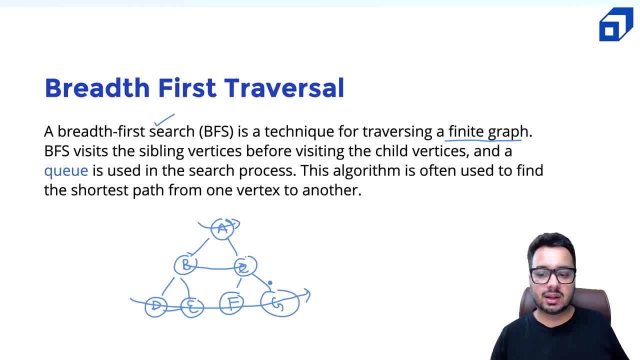 that we have done in a tree, But in a graph it will be quite similar. But there is one catch. The catch is graph contains a cycle. right, We have to make sure that we are not visiting a node which is already visited. For example, from this node one, if you visit two, and two is connected. 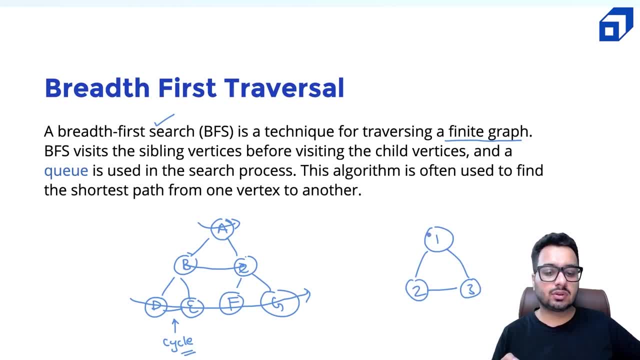 with three. three is connected with one, So there is a cycle. If you okay, we'll visit one, I'll visit children of one, that is two, I'll visit three from three now. you cannot go and visit one again, right? So 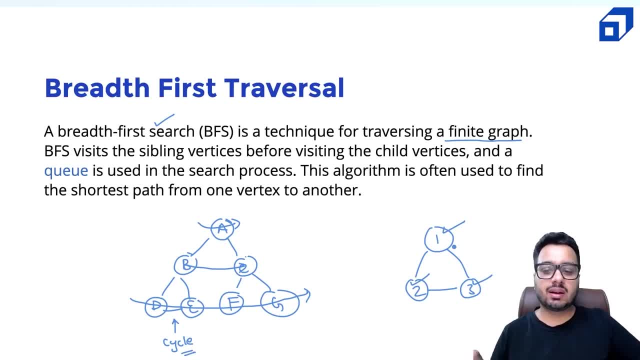 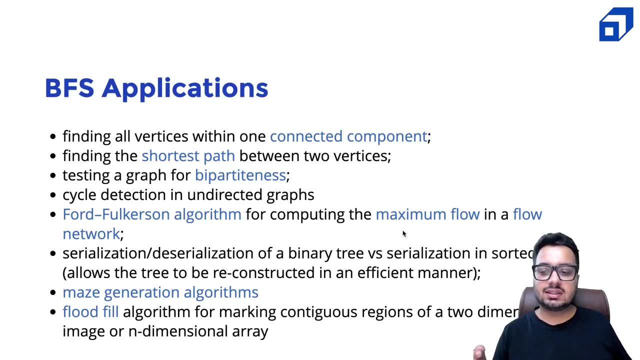 this is something we have to make sure is handled properly by our algorithm. Before I dive deep into the algorithm or into the code, let us try to understand some applications of BFS. BFS is can be used to find all the vertices within a connected component. 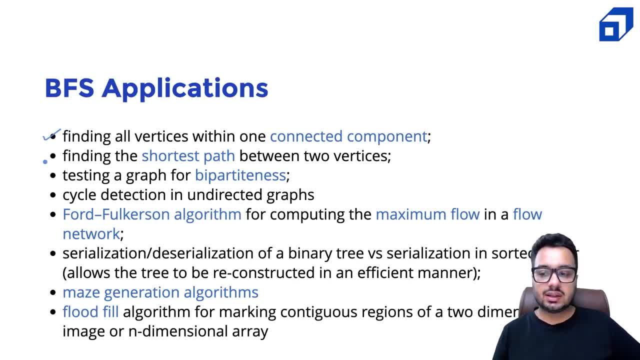 So we want to see what parts of the graph are connected. It is also used to finding shortest path between two vertices. in case of undirected graph, That means all the edges are unweighted. graph, That means all the edges. they have equal weight. there is no weight assigned to any edge. 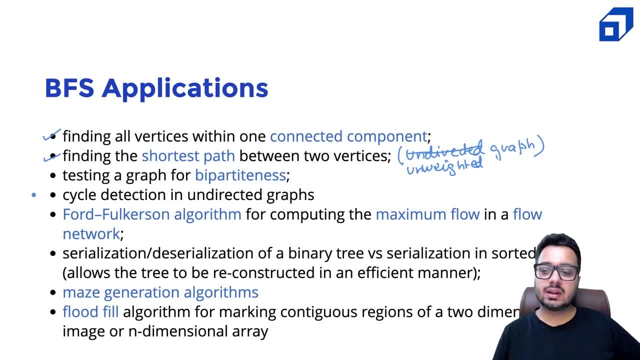 If it is a weighted graph, then we have to use a different algorithm. It can be used to check a graph for bipartiteness. it can be used for cycle detection in undirected graphs. it is also used in ford fulkerson algorithm. 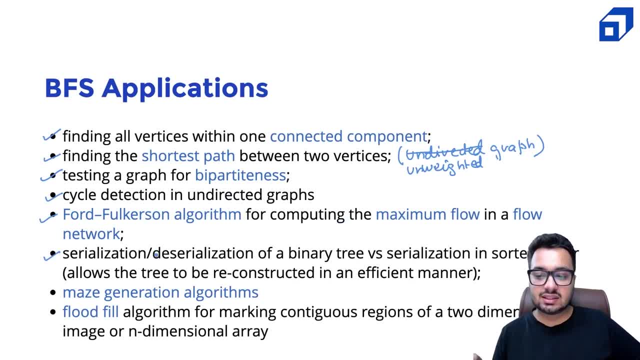 for maximum flow. it is also used in serialization- deserialization of binary tree. it is also used in maze generation algorithms and it can also be used in algorithms like flood fill. there are many, many applications, and that is why understanding this algorithm becomes very important. so let us 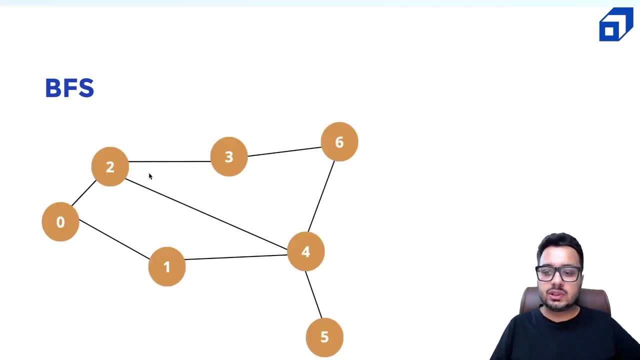 now dive deep into the algorithm. now suppose a graph like this is given. so what kind of graph it is? in my case it is a unweighted graph and it is also a undirected graph. that means edges don't have any specific direction. if zero and two are connected, two and zero are also connected. 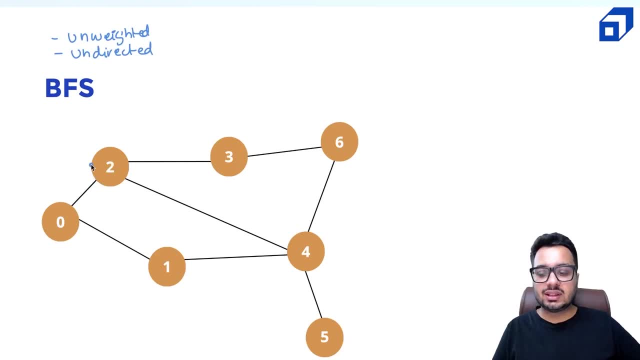 so we can go both sides right. so now in this algorithm, what is the input? the input is a source vertex. that means you are given a starting point. from that point you have to traverse the whole graph. the starting point could be zero, it could be three, it could be six, it could be any node. so just to keep things, 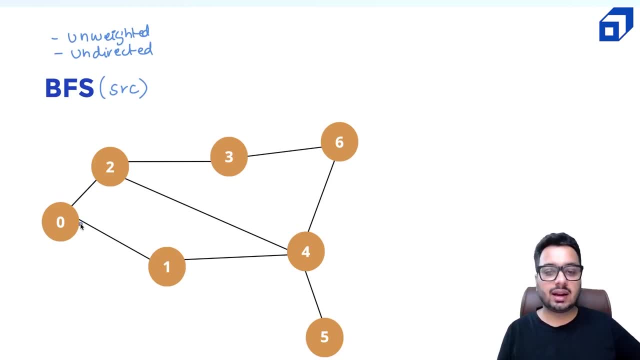 simple. i'm going to take zero as my starting point, right, and let me also draw the adjacency list that could be possibly a input for this algorithm. so that means zero is connected with two and one, one is connected with zero and four. so that means zero is connected with two and one, one is connected with zero and four. 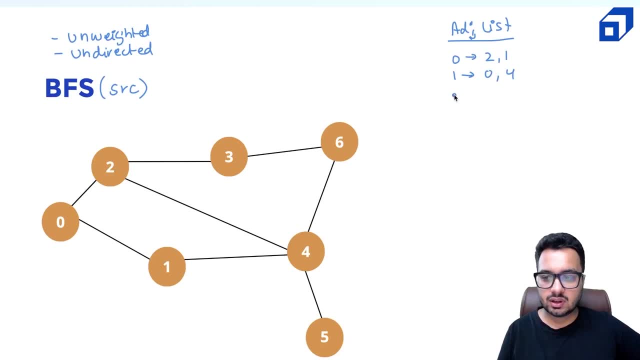 so neighbors of one are zero and four. neighbors of two are zero, three and four. so zero, three and four. neighbors of three, they are two and six. neighbors of four. they are one, six, five. i'll write it as one, five, six. then i have neighbors of five, which are only four, and neighbors of six, which are 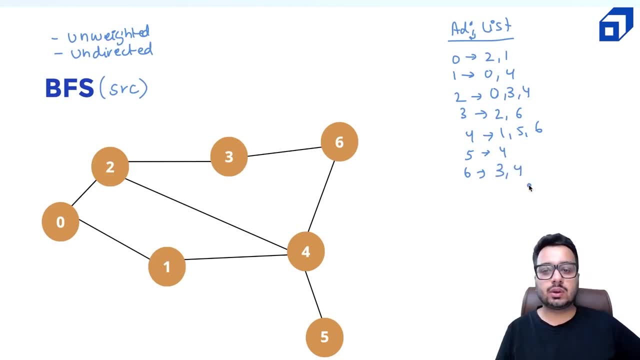 three and four. right one thing: i told you that if you start from this node, right so what we need to do, we need to. we'll be using a queue in this algorithm. you will understand why this queue is going to be very, very helpful. let me draw a data structure here which is a cube. apart from it, we will also need something. 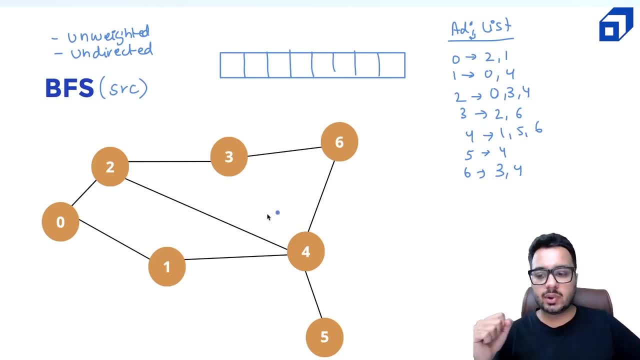 to maintain whether a node has been visited or not. right, because the graph contains a cycle and it is possible that we are coming to the same node again and again, right? so this is a queue. it is a empty queue as of now. right, the queue, you, you. 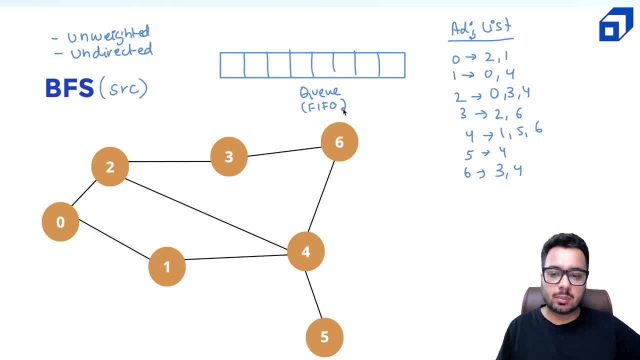 know it has a fifo property- first in, first out property, right. so it is a fifo queue here. and apart from it, i'm making one more data structure which is going to denote whether a node has been visited or not. so zero, one, two, three, four, five, six. i think this is sufficient. we don't need so we will mark whether a node is visited or not. so right now, it is nothing. it's marked. nothing is something ordered on that. a node is not busy right right. so now, if i compare these two together and if i consider its right side, it should be something that will be safe, or not. it should. be some kind of thing that is a 0,1,2,3,4,.5,5, whatever is right, it should be enough if this dass the no is upstairs, that if there is some kind of no and not it should say something or that anywhere, so we will build. 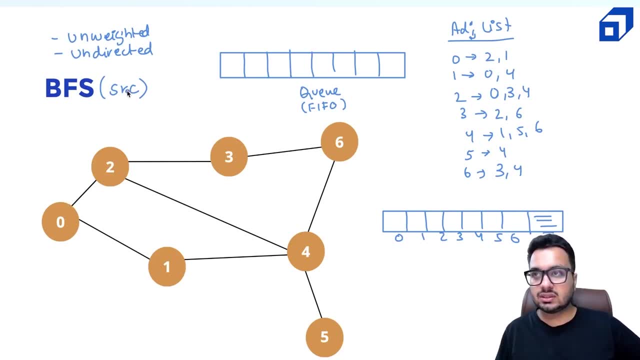 nothing is marked, nothing is visited. we'll start from this node. that is the source node. let's just assume the source node is zero. we'll mark it and we will put it into the queue. zero has been visited. zero goes into the queue and i am going to mark it as visited. so here the circle denotes the queue. 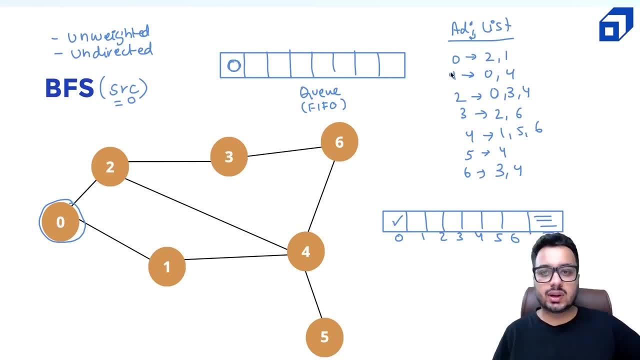 has been visited now what you will do next. you will look at this adjacency list. you will find out the neighbors of zero. the neighbors of zero are two and one, so you will pop this node out. the node is zero. you will look at neighbors of zero. that is two and one. you will mark them as. 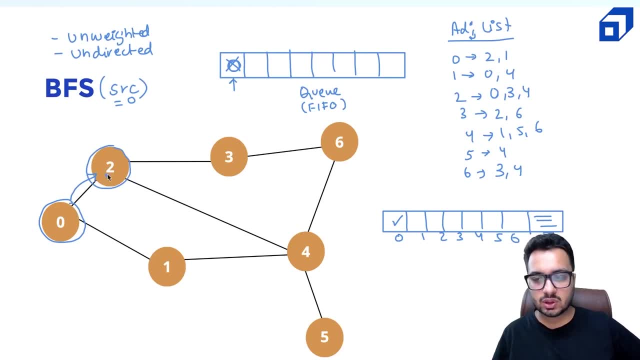 visited and put, put them, put them into the queue so you, from zero, you can easily visit two and you can easily visit one. what i'm trying to do is i'm marking one and two as visited and i'm putting one and two into the queue. so first i visited two and then i visited one. both of them they are into. 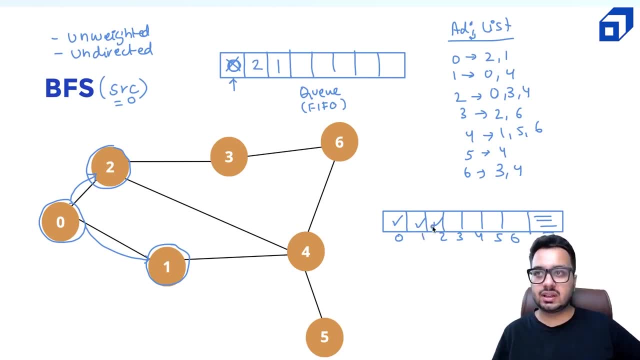 the queue. that means i have marked one and two as visited. now what you will do next? now you simply have to pop out a node from the queue every time and do the same process again. so now you will remove two. look at the neighbors of two, which are zero, three and four. now zero is already. 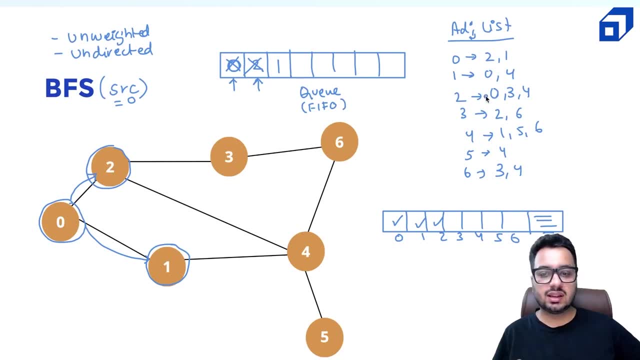 visited, so you do not do any work at zero. then three and four. three is not visited, you can visit three. so mark three as visited, put it into the queue. and mark four as visited and put it into the queue. okay, now two is gone. two has been removed. next node you will get from the queue. it is going to be. 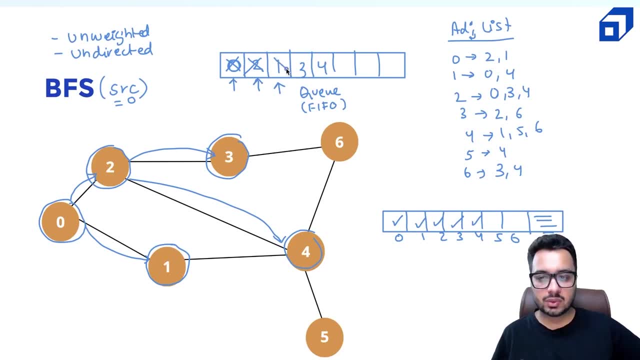 one. so you will remove one from the queue and you will mark neighbors of one as visited. so neighbors of one, zero and four. look at zero. zero is already visited. four, four is also a neighbor. four is already visited. so you do not do any work. so you do not do any work, right? so in the meanwhile, you. 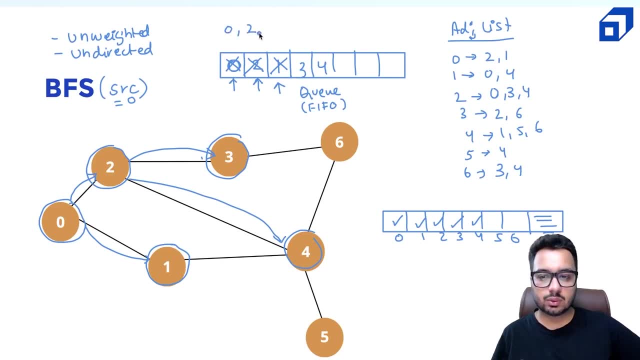 can print the nodes that you have seen far. so you have seen zero, you have seen two, you have seen one. next you will pop out three. so remove this node, print this node. look at the neighbors two and six. the two is already visited. do nothing at two. six is not visited. mark six as visit. put it into the queue. so. 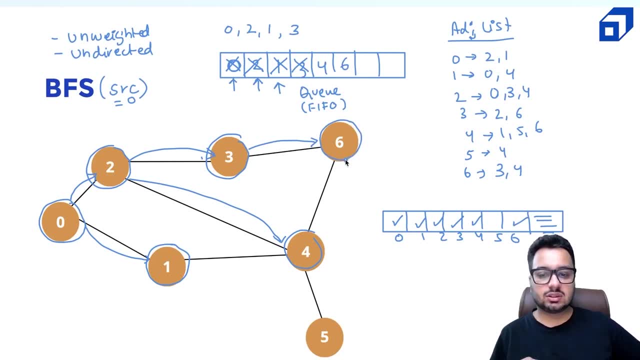 you have to. you have traversed six as well. the six is now also into the queue. next you will pop four, so print four. look at neighbors of four. four neighbor is one which is already visited. its neighbor is five, which is not visited, so you will visit it. put it into the 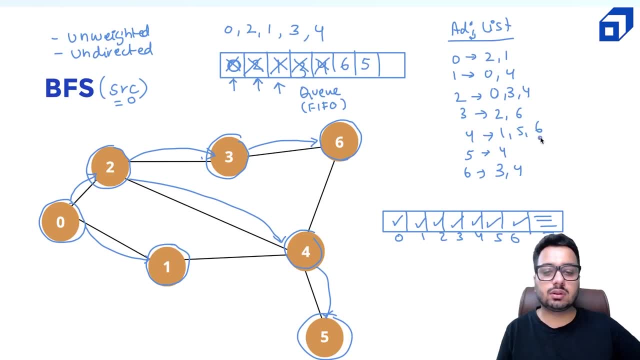 queue. six is already visited. do nothing to do here. right next you will get six from the queue, remove it, print it. and now look at neighbors of six. six neighbor is only uh, three and four, right, but both of them they are visited. so you will not do any work. so next you will remove five. 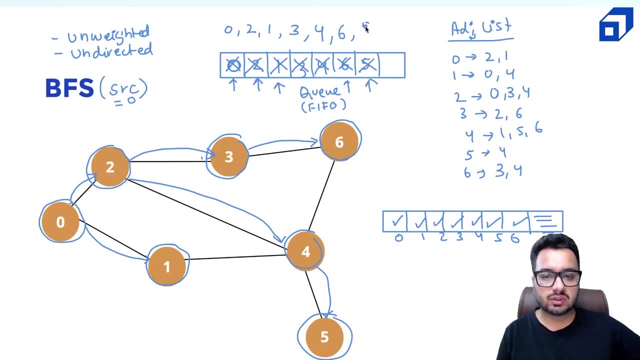 five, neighbor is four, so this is also removed. four is already visited, hence you do not do any work. and now what you can say is that your traversal is done. right, your traversal is done. so what happened during this traversal? we visited each node once, and in the worst. 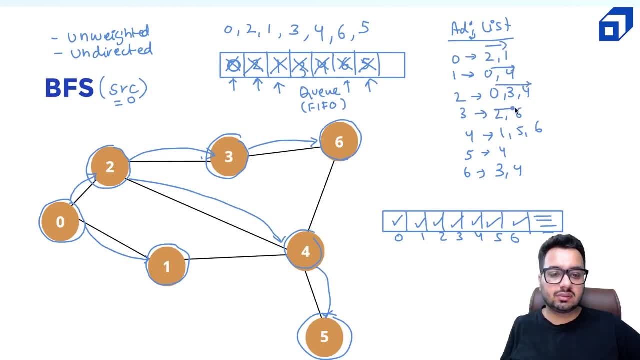 case, we are traveling through all edges once, right? so what we have done, like we have traveled through through some edges and we also checked that- from four i can go to one- so we did check this edge. right, we did check this edge. one was already visited, so we did not mark anything here, right, so we did not. 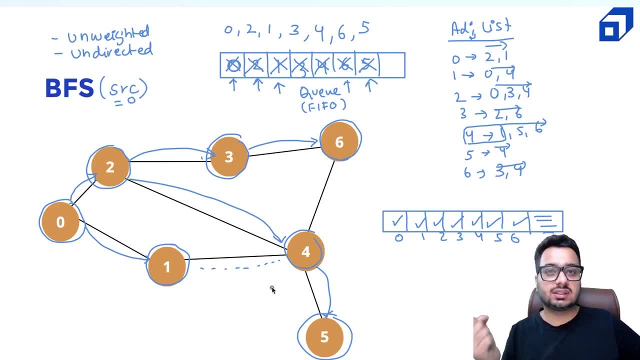 mark it in anything here. what i am trying to say is, when you are running this algorithm, each vertex is going into the q once and this it is coming out of the q ones, and when you are finding the neighbors of a node, you are traveling through all the edges, right. so all the edges are being covered at most twice. for example, 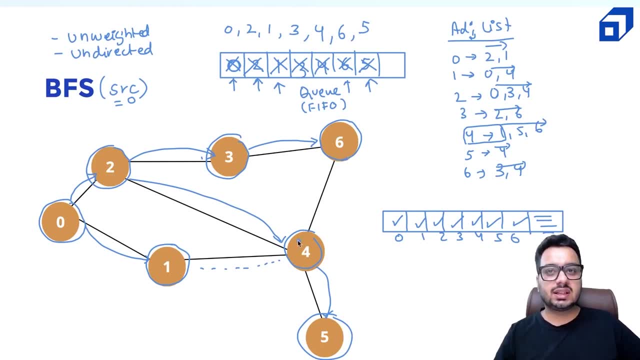 neighbor of 4 is 6. neighbor of 6 is 4.. each edge is counted at most two times. so if i talk about the overall time complexity of this algorithm, it will be linear in terms of number of nodes and number of edges. this is what we are doing, right, so i hope you have understood the basic. 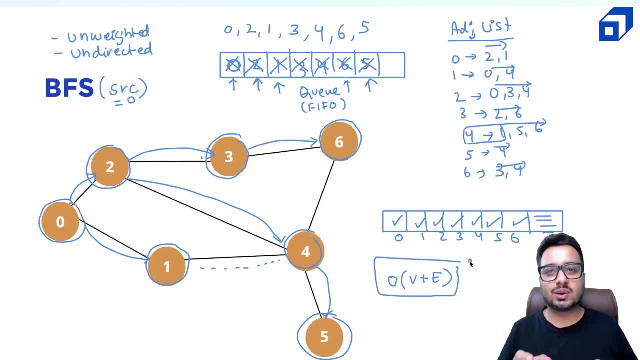 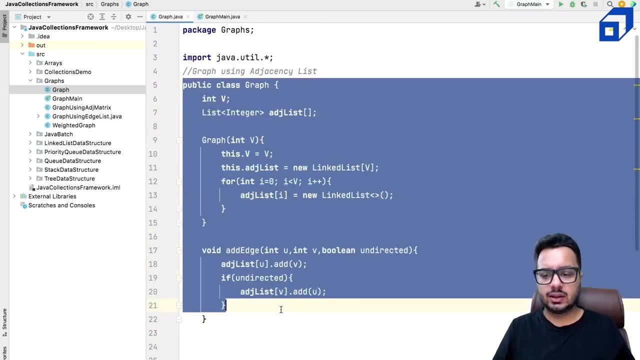 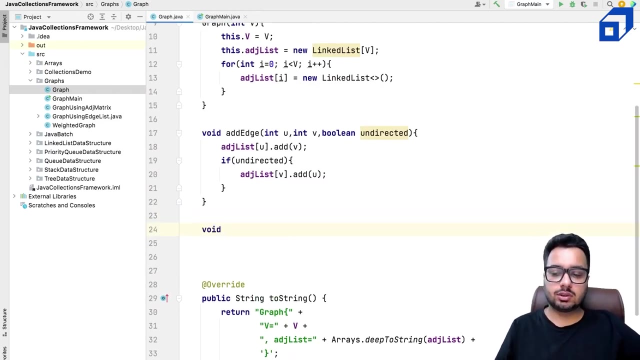 bfs idea. next we will look at the implementation and code this algorithm. let us discuss the implementation of bfs. i already have the boilerplate code ready, which is basically adding edges into the graph. the bfs function is something that i'm going to write now, so return type is void. we do not want to return anything. the method name is bfs, but what we 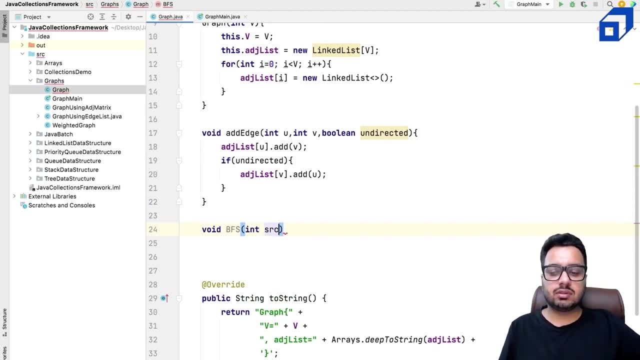 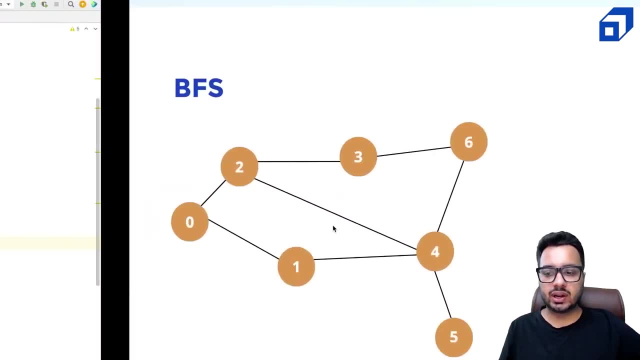 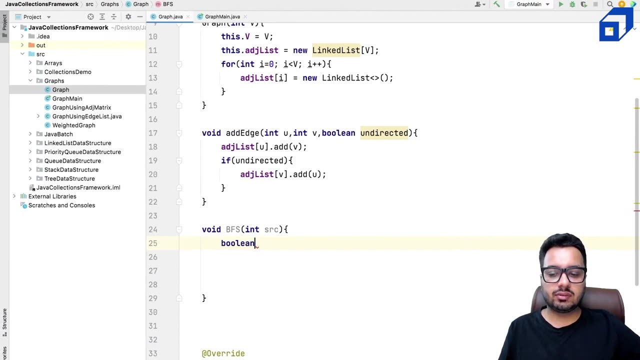 we may expect, as input is one source node from which we should start doing the bfs for this graph. so this is the graph. so i told you we will be needing two data structures: one to maintain whether a node has been visited or not. i can maintain a boolean visited array and this will 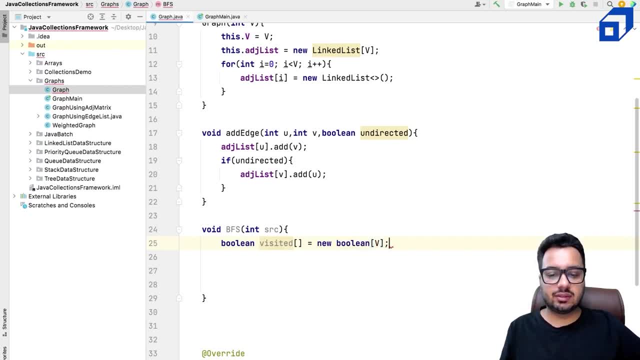 be a array of size v, where v is the number of vertices in the graph. next thing i will need would would be a data structure, q. so in java we have q as our interface, so i'll create a link list which provides me with the implementation of q as well. so linked list of integers. we will just call it. 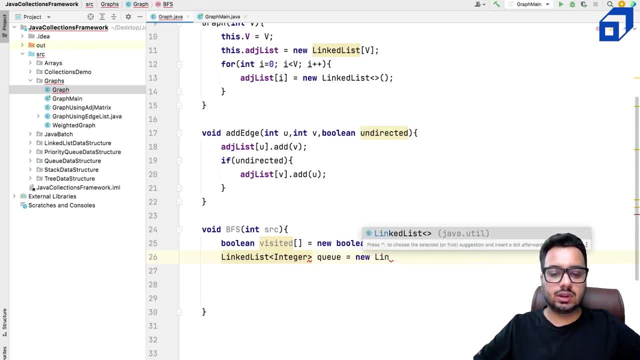 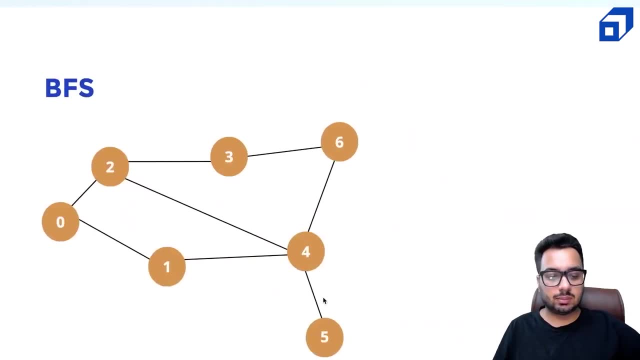 as q, and i will say this is equal to new linked list. all right, so that are the. these are the data structures that we will be needing. now let's start with the algorithm. so, in the first step, what i will do? i will start with the source node: mark it as visited, push it into the queue. 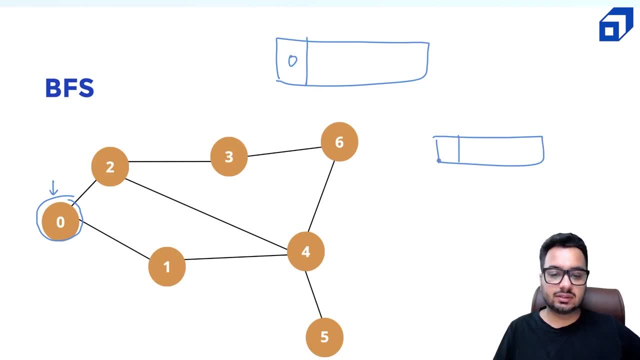 so i have to do three things: mark it as visited, so visited of source is going to be true. so i will say, okay, this is going to be true. and then i will traverse the neighbors of this node. so first thing i will do is i will push this into the queue. 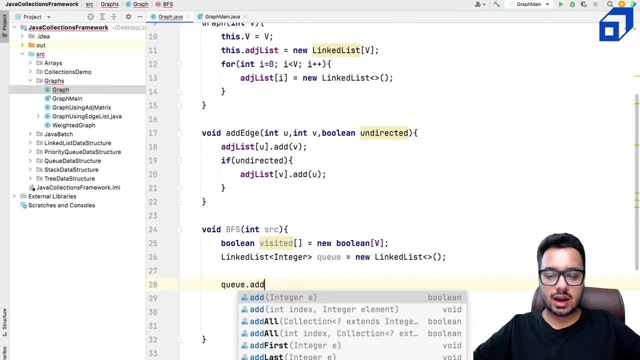 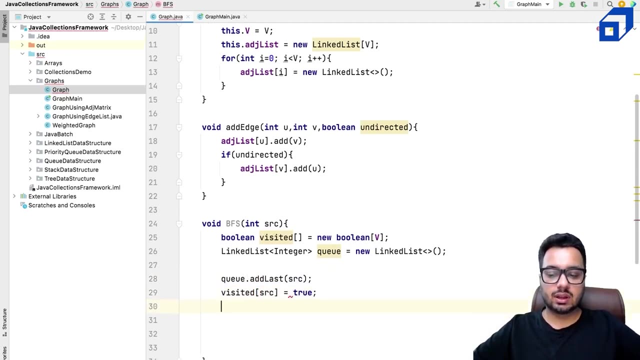 so i can say q dot add last. the node is source. okay, and second thing i will do is i will mark this as visited, the visited of source. this is going to be true. now, what can i do? now i can say while my queue is not empty, so i will stop once all the nodes. 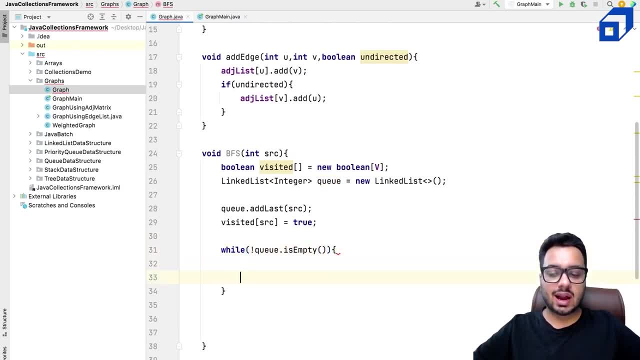 have been swapped out. so how do i add into the queue and remove from the queue? so you know if you have to add something into the queue that addition will happen from the ending, so add last and if you have to remove something from the beginning, so we can call. 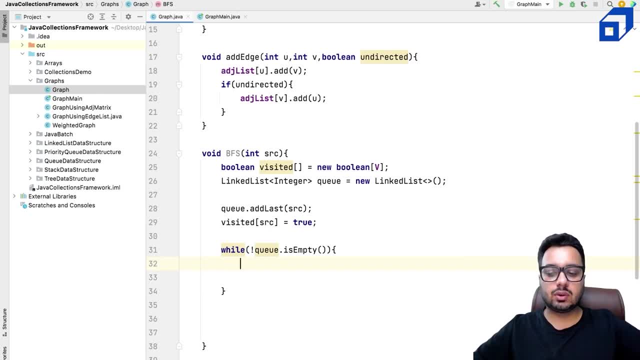 remove. first method, i can say: okay, the node at the front of the queue, so that's the last cloud of the queue, so we get the кр. similarly, once i have that added, i'm not going to add anything into the q now that i have added. i will stop this once all the nodes have been popped out. so, guys, what you know if i do add, move into the. 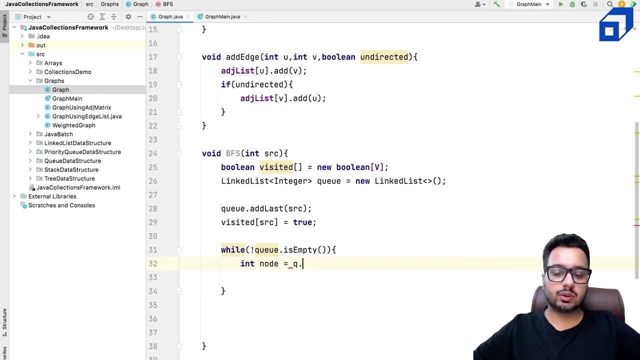 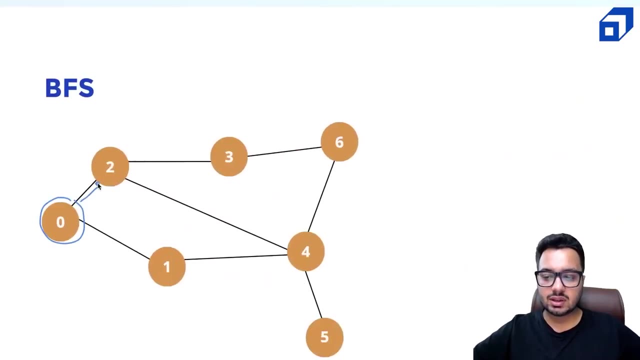 is int node. this is going to be q dot remove first. All right, now what can I do? I can say okay for this node. so node that I've removed from the queue is zero right. So I need to traverse. what are the neighbors of zero to zeros? neighbors are there in adjacency. 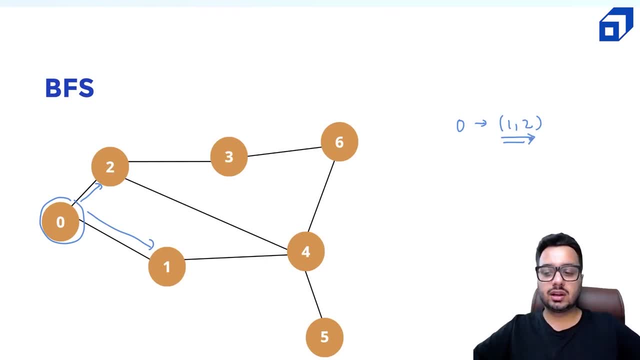 list. So they are one and two. So what I need to do, I need to traverse on these neighbors. If the neighbors are not visited, I will mark them as visited and I will push them into the queue. This is what I do. I can do okay for every neighbor, Okay. so to get the neighbors 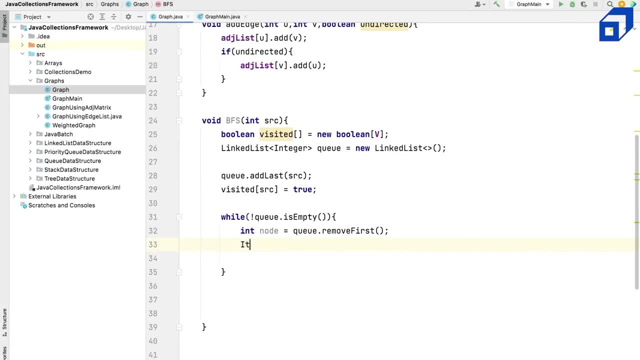 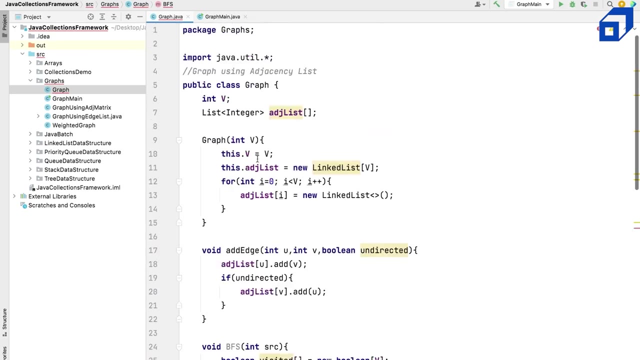 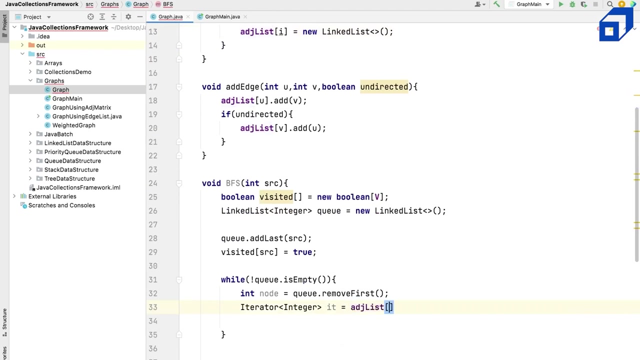 what we can do. we can use iterator. I can create a iterator of the type integer and call it something like iterate it, and now I can say: give me the neighbors of this particular node. So if you know, then this is the adjacency list. So I want to iterate on this adjacency list of the node So I can say, okay, while it dot. 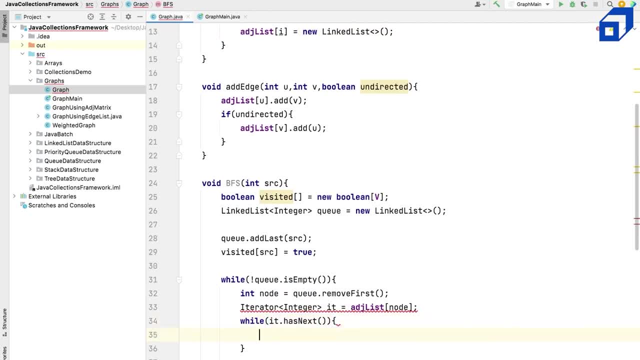 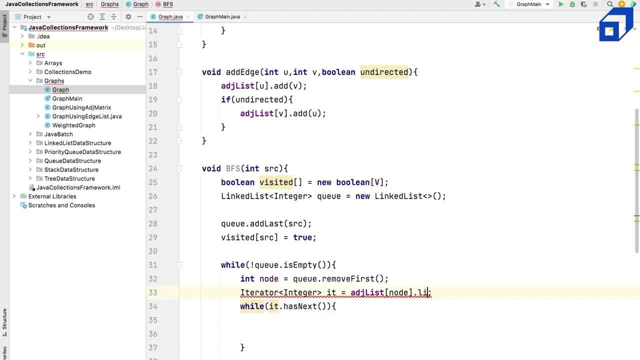 has next. that means the next node is present. Basically it is a way to iterate on the adjacency list, But you have to call a method called list iterator, because we are iterating on the linked list. So zeros, zeros, neighbors are one and two right, So these are stored. 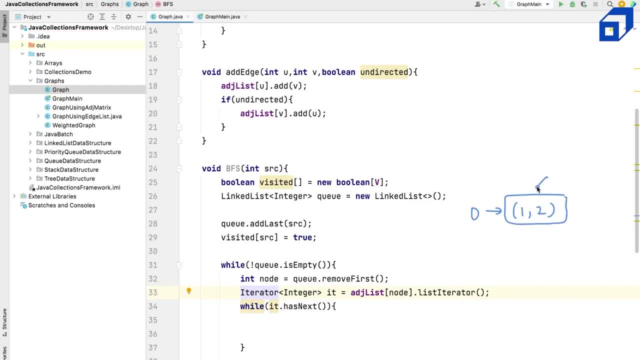 in a list Which is which was a list object. So adjacency list of node is a list. we have to get the iterator using this method, This iterator, it will iterate over these nodes until the list is not finished. it will go over these neighbors. Now I want to get the node right. 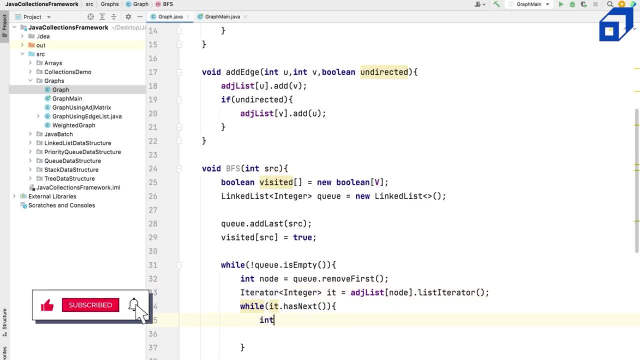 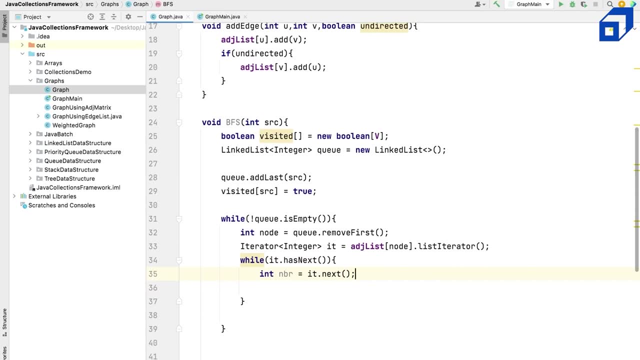 So how do I get the node? I can do: okay, the neighboring node is nothing, but it dot next. That is the neighboring node. And now what I need to do. if it is not visited, if not visited neighbor, what do I need to do? I need to market as visited. I can say visited. 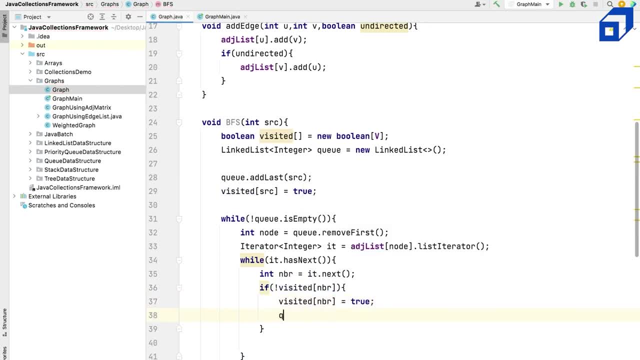 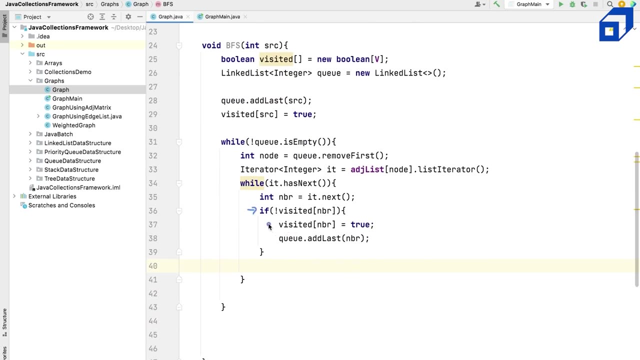 of neighbor. this is equal to true And I need to add it into the queue. I can do q dot add last, And the item is neighbor. we are iterating over all the neighbors And if the neighbor is not visited, we simply mark it as visited and we push it into the. i hope this should suffice. and one more thing. 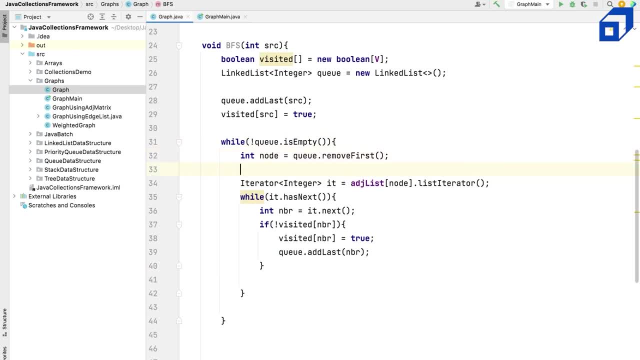 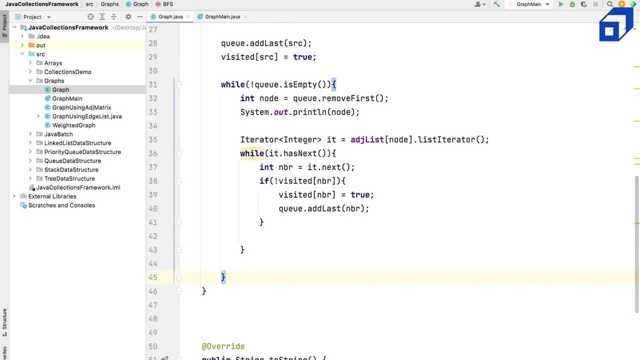 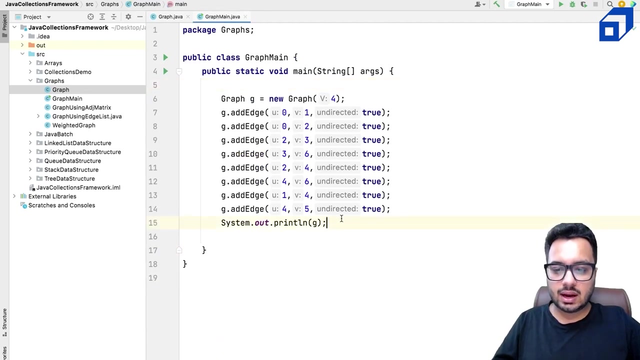 we can do in the while loopers. we can print out the node. we can see what output do we really get? i can say: s out node. now let us test our algorithm on the graph i have already constructed. so let me show you in graph main. i will go: and this is the graph, same as this graph. and now we 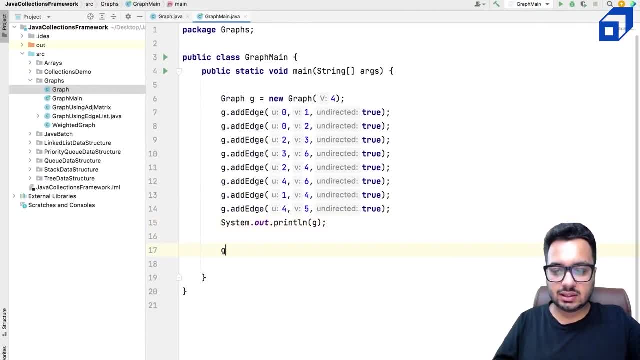 are going to run bfs function on it. i can say g dot, bfs. let's say the source node is zero, so let's go and run this code and see what output do we get. we should get all the nodes from zero to six because we are doing a. 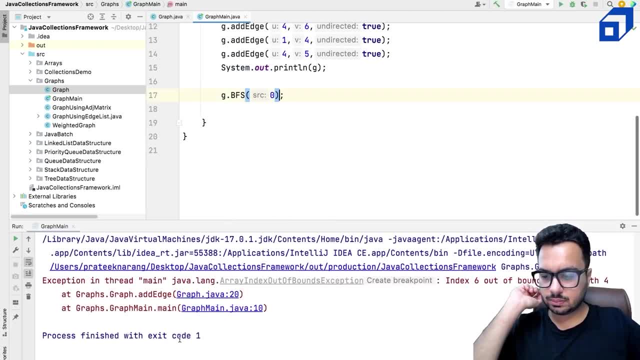 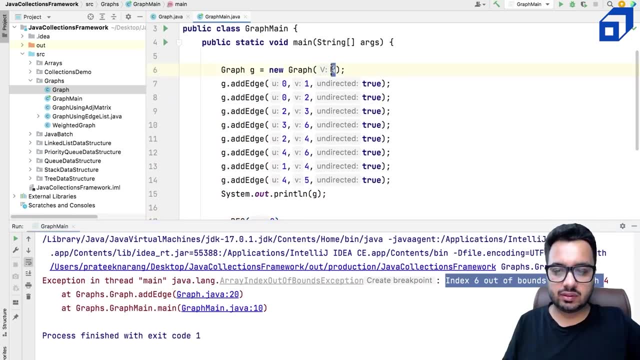 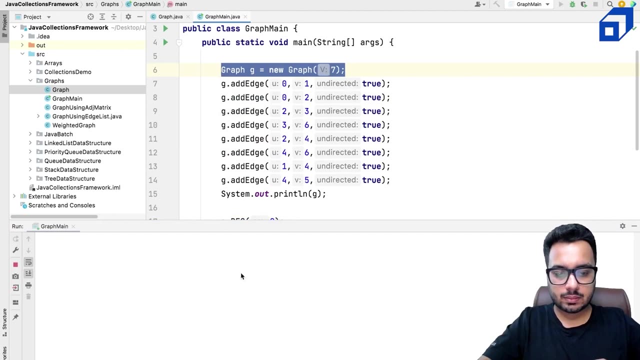 you graph traversal. let's see the output. okay, we got an error index six out of bounds for an error of length four. okay, so here we have to give. we have seven nodes actually. input needs to be fixed, okay, so this is our adjacency list and we are getting zero, one, four, three, six, five. 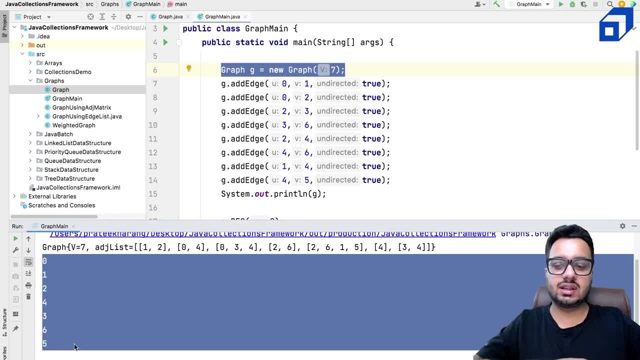 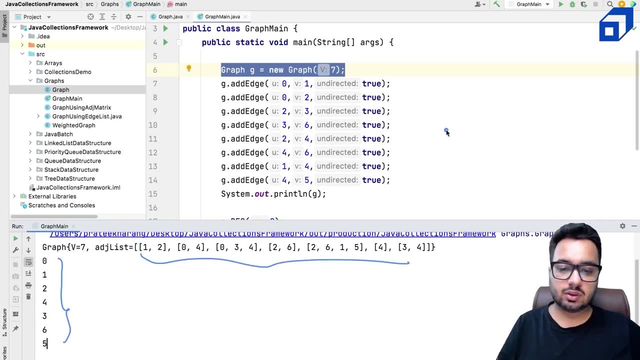 so we are getting all the nodes. that means the graph traversal is correct. now the exact output will also depend upon the way you have stored these nodes, okay. so you said, okay, zero's neighbors are one and two. after zero it will print one and then two. but if you say in my adjacent 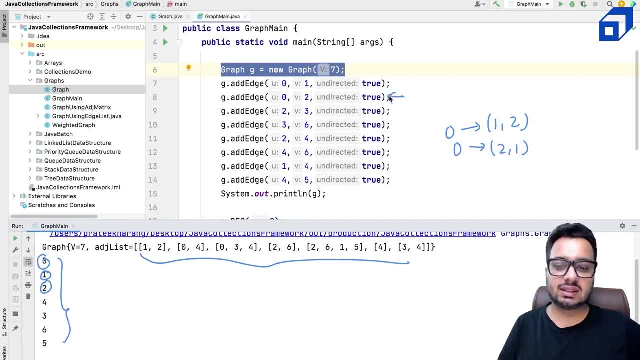 list. i will store two and one first. that means i will add this edge before this edge. then the output will be zero to one and so on. so right now our goal was to visit all the nodes which are which can be reached from node zero. so we are getting zero and two and so on. so i have to go to 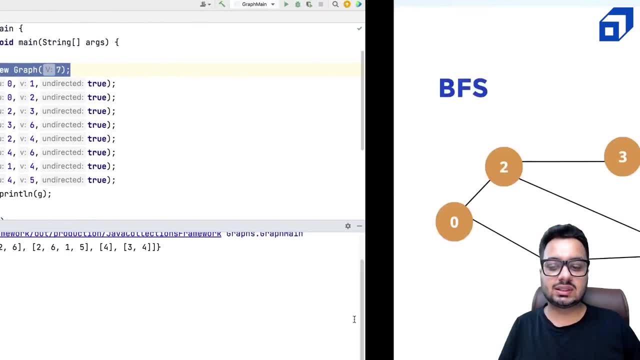 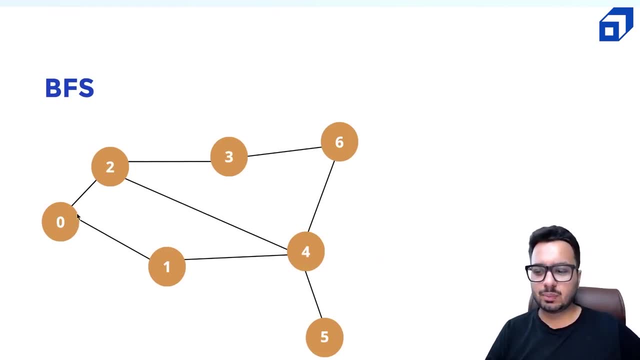 this node number and get two nodes, and then we are getting zero and two and so on. so we are getting one, two, four, three, six and five. that means this output is correct. we are able to reach all the seven nodes, including zero. now let us discuss one application of finding the shortest. 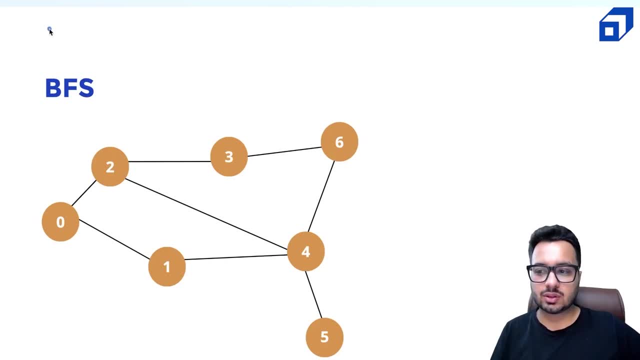 path from the source node to all other nodes. okay, so what we are going to do, we are going to do shortest path from source to all other nodes in a undirected graph, in a unweighted graph. an unweighted graph. so this graph is a example of an unweighted graph. so graph can be directed. 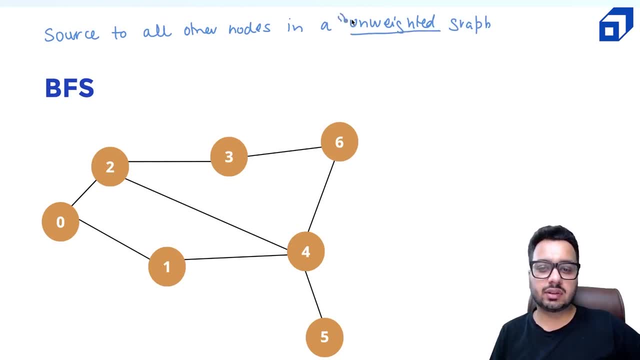 or undirected, but it must be an unweighted graph for the bfs algorithm to work for finding the shortest path. okay, so we are going to talk about bfs- shortest path algorithm. so the algorithm is very simple and it is very similar to just doing bfs. let us try to visualize. 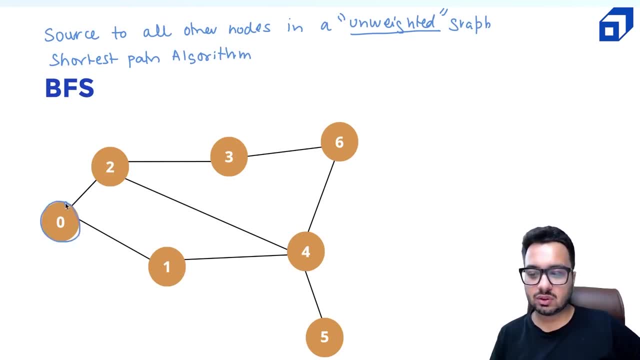 what we are doing in bfs. we are starting from node 0 and we can mark the distance of 0 as 0, and from 0 we are visiting the nodes 1 and 2.. since we are visiting a node for the first time, we will be updating their distance and we will be saying: this distance is 1. 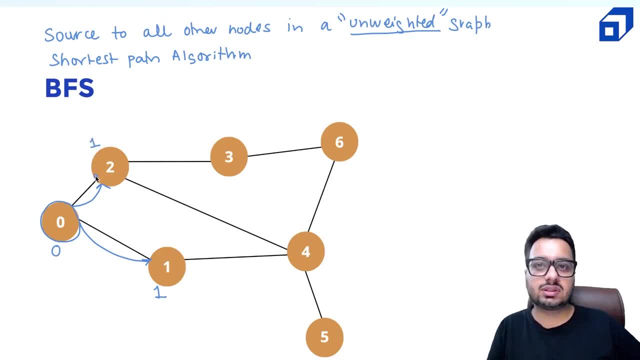 and this distance is also 1 because we are coming from 0 and 0's distance is 0.. next, you know in the queue what you have done. you have said, okay, 0 is there. then you pushed 1 and you pushed 2, and so on. 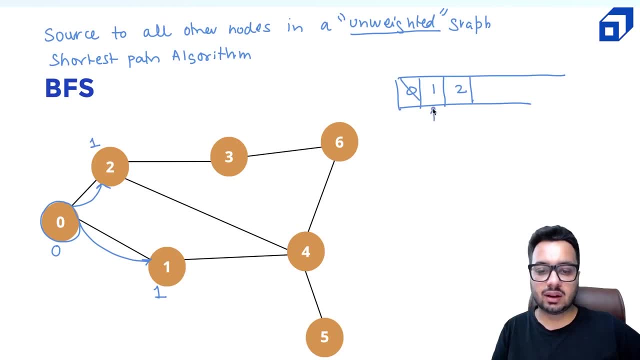 right now. next, next item you will pick is one and you will update the neighbors of one. neighbors of one is, let's say, four and zero, zero is already visited, so you will not go there. so you will say, okay, since i am visiting four via one, this distance must be two, the distance of four, i can say distance. 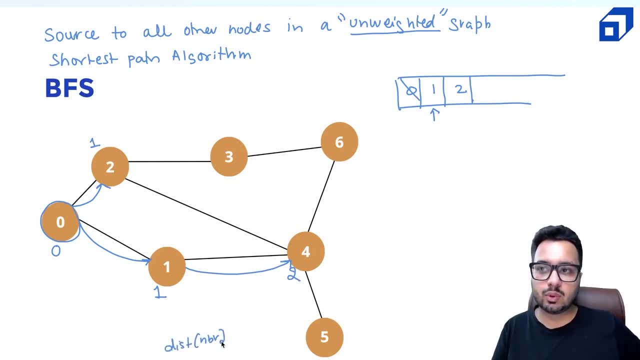 of. uh, the neighbor is one more than the distance of the parent. so parent is one. okay, distance of parent. parent node is one, child node is four. or the neighbor node is four. four's distance is one more than the parent. so i will visit four and i will push four into the queue. so next i will. 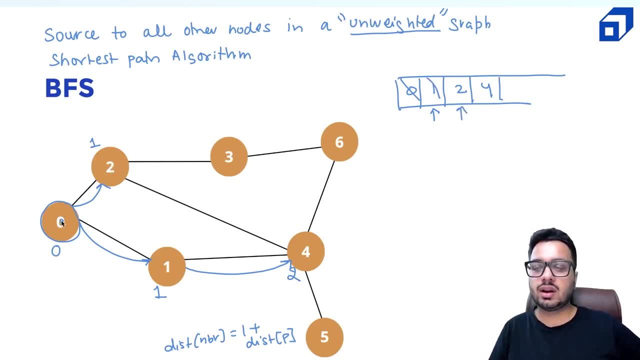 remove two. the two's neighbors are zero, already visited three. three is not visited, so i can visit three and i can. okay. this distance is going to be two, so i will push three into the queue, and two's neighbors is also four, but four is already visited so we will not update it. 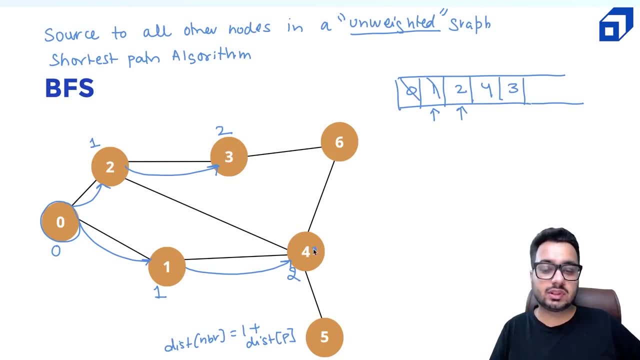 is not possible that you are reaching a node later which is already visited and the distance will get minimum. it's not possible in case of a unweighted graph. if it would have been weighted graph, this was this could have been possible. right now, four is already visited and since you 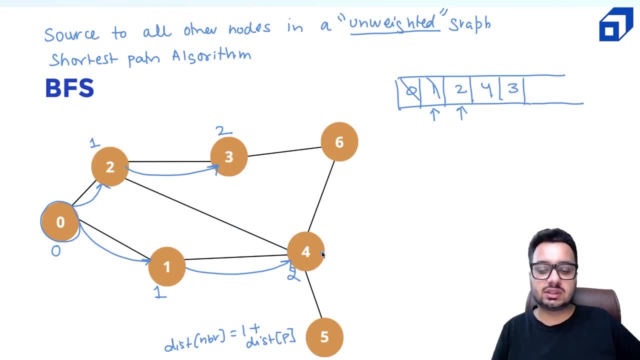 are reaching from two. again, node is already visited, so this distance will be either greater or equal to two. so it is, we will not update it, so we will not do anything at four. so two is done, it's work. next we will pop out four, and four can now update its children. so four children are. 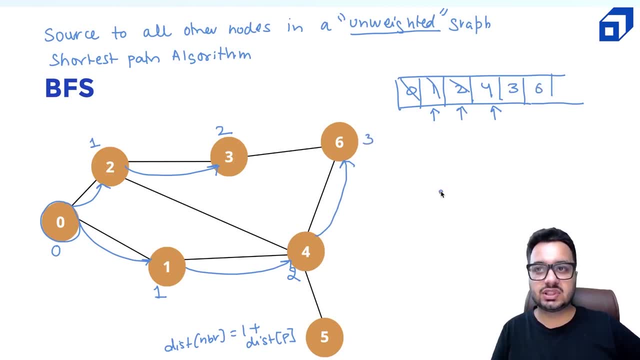 six. this distance is three, so you push six. and four can also update five. this distance is also. you can push five. next you can pop out three or three again. it will try to visit six, but six is already visited, so hence you don't do any work. then you try to pop out: uh, six. 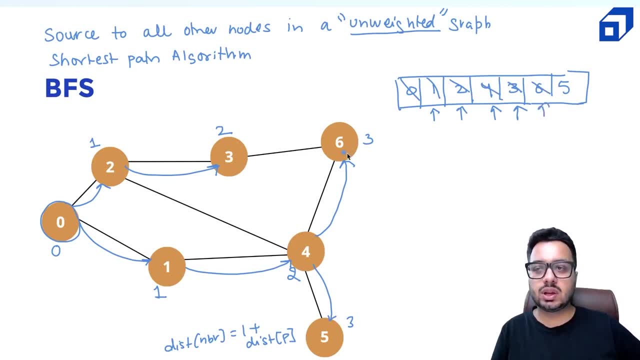 so you can remove six easily, but there are no nodes, no neighbors of six which are not visited. when you pop out five, there are no neighbors of five which are not visited. so if you look at these values, you will find that these are the shortest distances from zero to all these nodes. these are the shortest distances from zero to all these nodes. 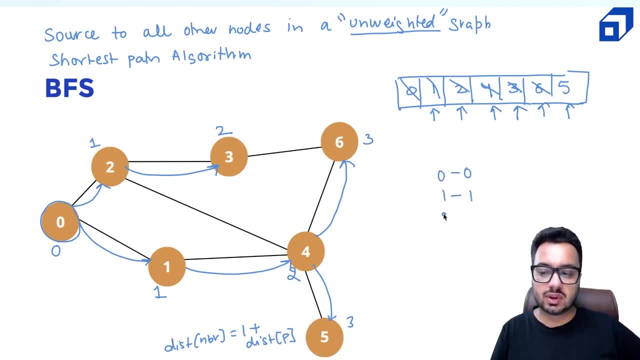 so that means distance of zero is zero, distance of one is one, distance of two is one, distance of three, distance of four is two, distance of five it is three, and distance of six it is three. so one observation we can make out from here is that bfs visits nodes in increasing order of their distance. 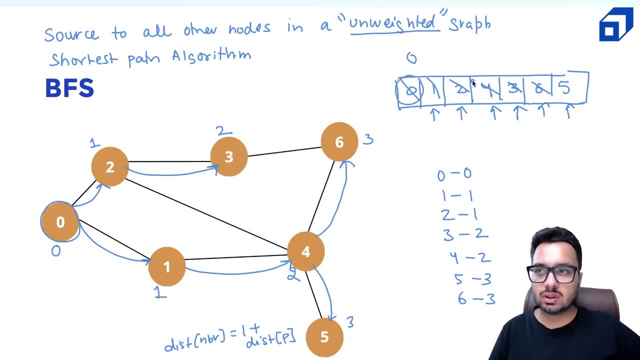 from the source node. this distance was zero, these two distances were one, these two distances were two and these two distances were three, eight. so this is an observation, right. so when i said you can get any ordering, so that means between these distances. the ordering can change, so bfs might produce an. 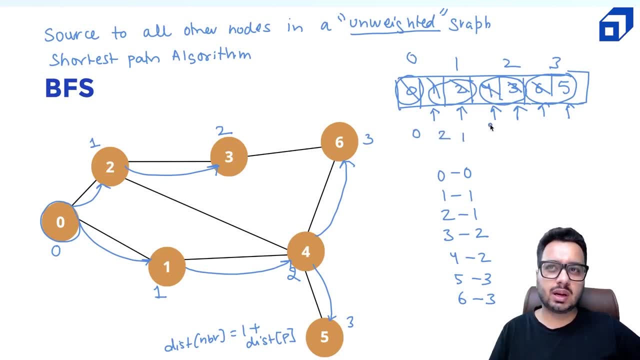 output like 0 to 1, it might produce 4, 3, it might produce 3, 4, 5, 6 might get 5, 6 or 6, 5, right to different orders, but the distances of these nodes will be in in in increasing order from the source. 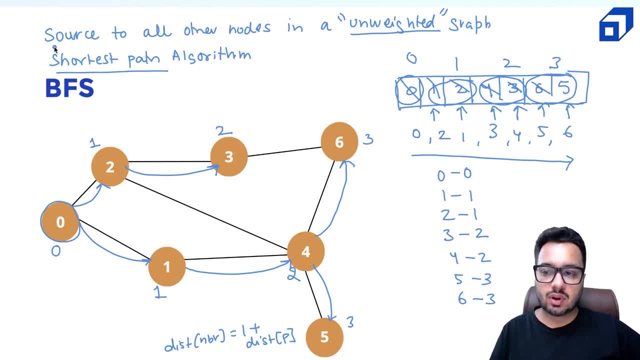 node. that is how we can find shortest path from source to all other nodes in a unweighted graph by simply using the fs. in the next part we'll show you the code changes that we need to do for this algorithm. so it is very simple. take a moment, pause the video and think what changes you will make into the code. 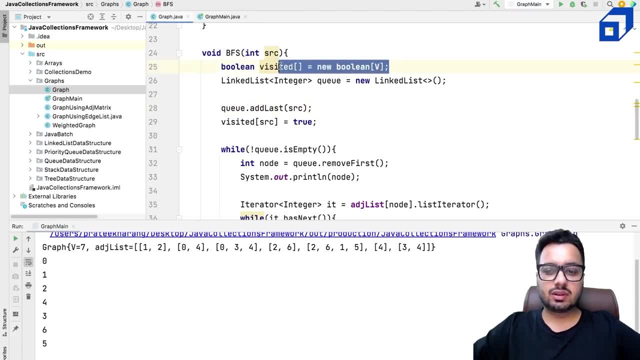 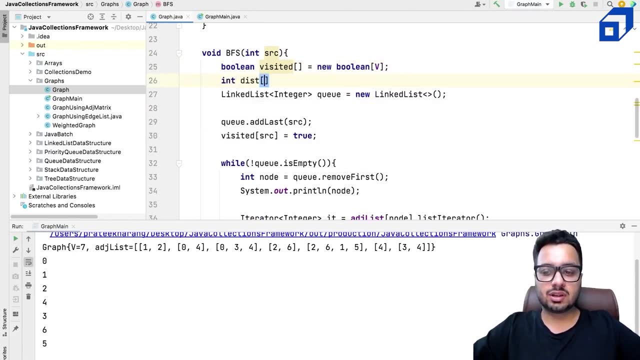 all right, so let us discuss the code changes. now, apart from the visited array, what you need to do? you need to maintain a distance array, the distance of each node from the source node. so you can. okay, i need a distance array which is of size v and in the beginning you can say distance of source. you can update that distance of source as. 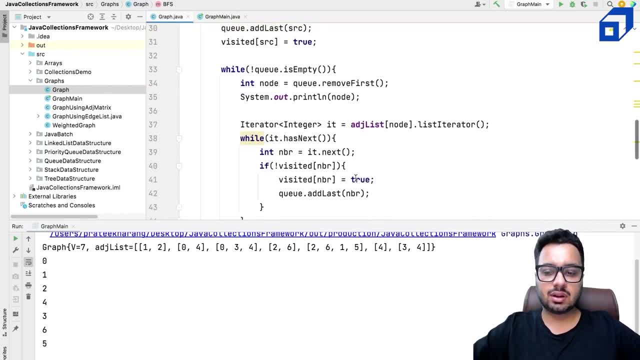 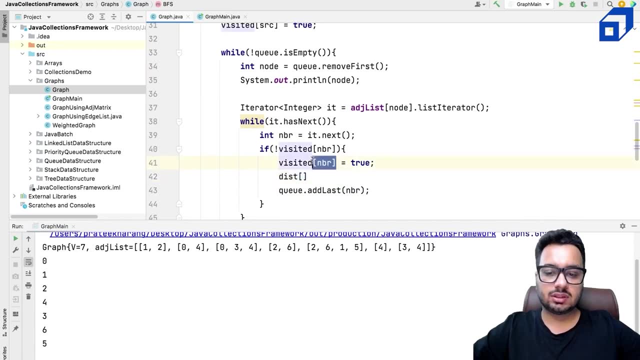 0 and rest is very simple: as you are visiting more and more nodes, you need to update the distance. so again, okay, i'm going to visit the neighboring node. so when i'm visiting this neighboring node i can say distance of this neighboring node is one more than the distance of the node. 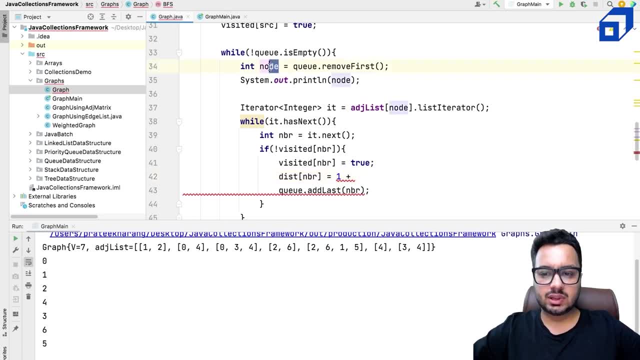 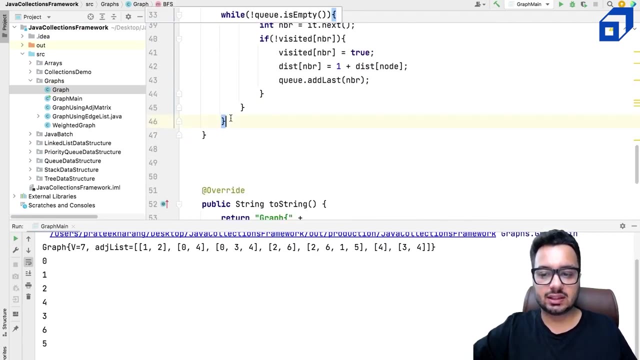 that is parent of this node. so that node is nothing but this node. so this node is distance of node. so that's it now what we can do in the same function. maybe we can either return the distance array or we can just print the distance array. so here i can say: 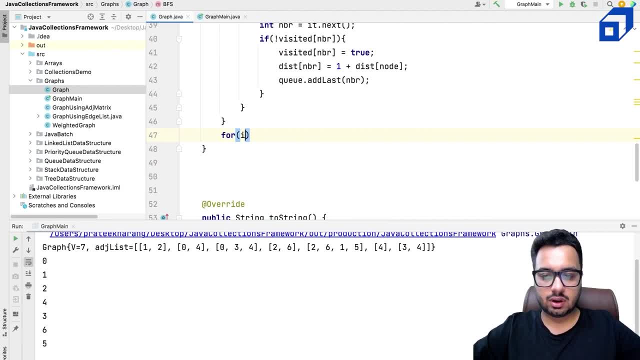 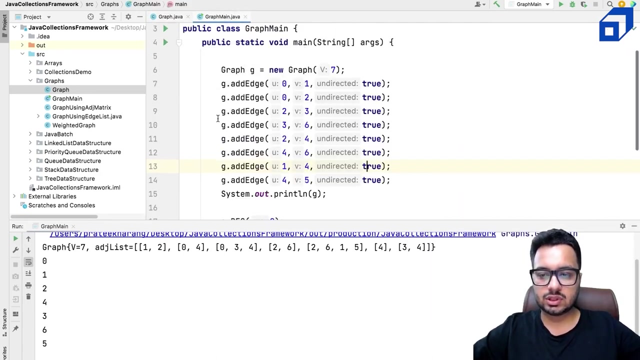 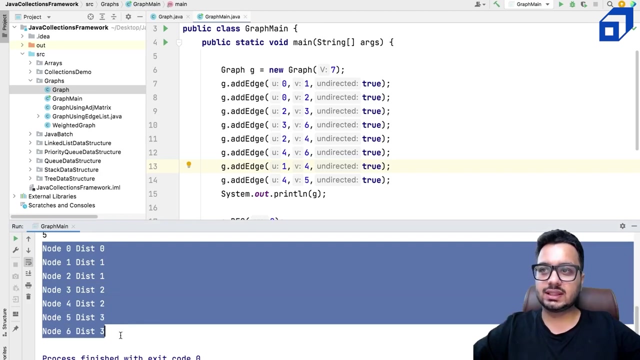 let's just iterate over the distance array: for i equal to 0, i less than v, i plus plus. i can show the node which is going to be i, followed by the distance which is distance of i. so let's go and run this code and we should see we are getting node 0 at distance 0, 1 at 1, 2 at 1, 3 at 2, 4 at 2, 5 and 6. 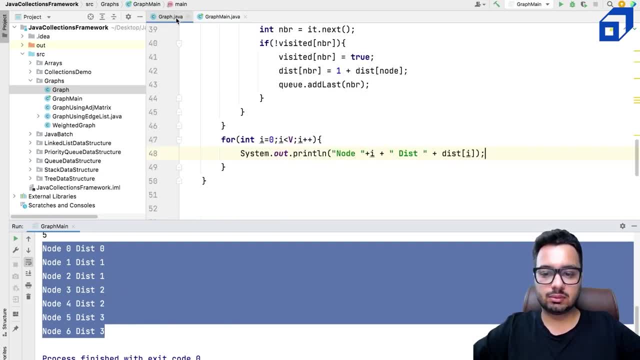 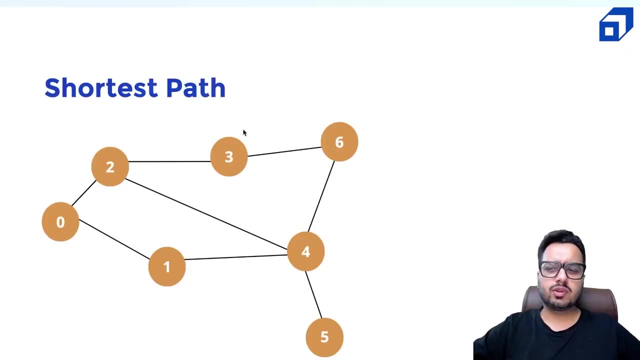 there at distance 3.. this is how easy it is to make changes in the code, and now we have made shortest path algorithm using bfs. now some of you might be wondering that, okay, we have figured out, but we have only figured out the distance. actually, what if i actually want to figure out? 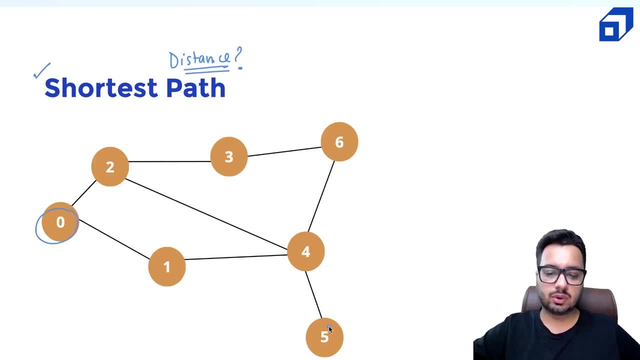 the exact path from, let's say, 0 to some node 5, right, maybe i want to find out what is the shortest path. should i go like this, or should i go like this, or should i go like this? what will be the shortest path from source to destination in a unweighted graph? so again, this thing is very simple. 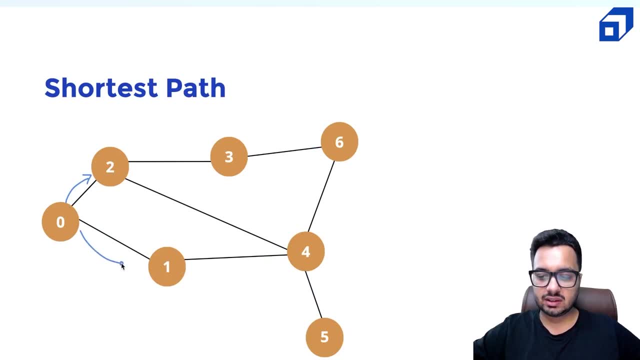 what we were doing. we were doing bfs: 0 was visiting 1 and 2, 1 was visiting 4, 2 was visiting 3 and 3 was visiting 6. no, i think it was like this: 4 was visiting 5 and 6 and then. 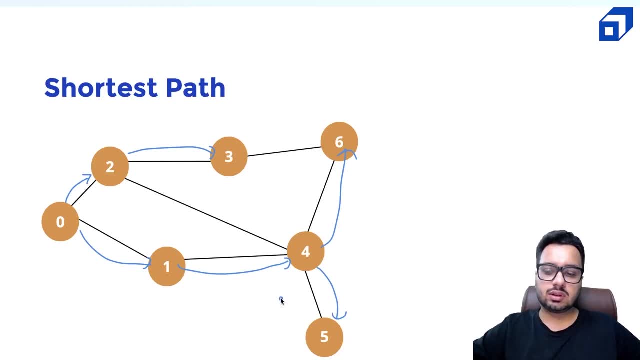 3, something like this. we did right. so now again, if you want to find out the shortest path to reach 5, you will know that, okay, 5 was visited from 4, 4 was visited from 1 and 1 was visited from 0. right, what you can get, you can, you can actually store the parent, so you? 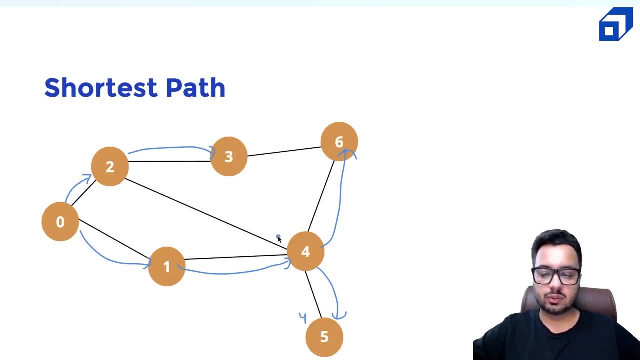 can store: parent of 5 is 4, parent of 4 is 1, parent of 1 it's 0 and parent of 0 is, let's say, 0 or minus 1. anything you can put, what you can do, you can store these parents for every node and then 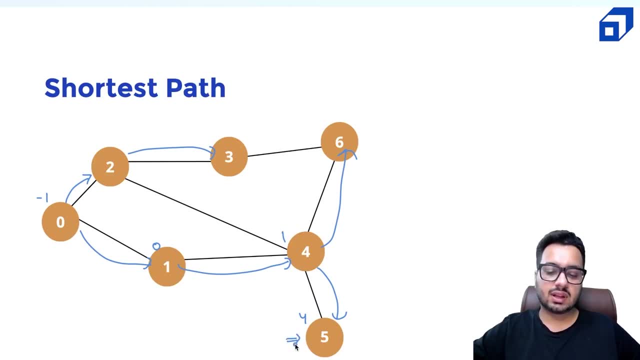 you can do trace back and okay, i'll start from 5. and okay, from where i should go, this is my destination node. so is the parent of 5? how do we arrive at 4? where is the destination node? okay, we arrive at five. we came from four so i can go to this node. okay, how do i came at four. i came from. 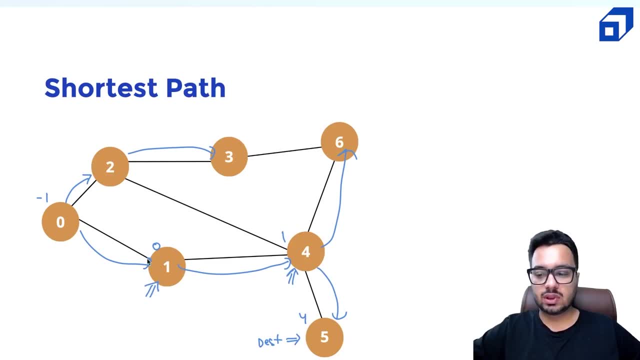 one, so i i can go to this one. how do i came at zero? i will go to zero. okay, how do i came at one? i came from zero, so i go to zero. who is the parent of zero minus one? that means we have, uh, finished the entire path. in this way, you will be able to store five, four, one zero in a array or in. 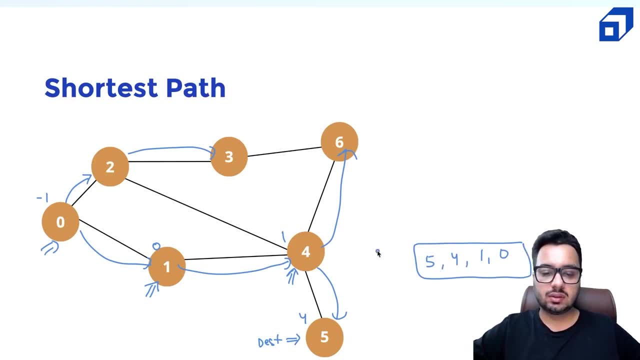 a array list, so this way you can also print the shortest path from the source node to the destination node. the only changes in the code you need to make is you need to create a parent array and when you are visiting from a node to to a neighboring node, so you can say, okay, parent of. 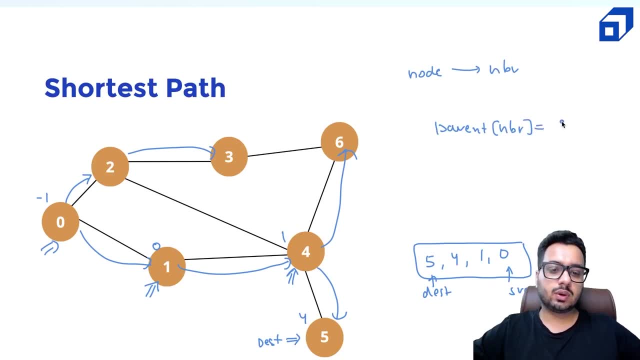 neighbor will be equal to node, something like this, and then you can simply put a while loop at the end. once all the nodes have been updated, your bfs has been done, and okay, while i don't get the source node, let me travel back from the destination node, so you 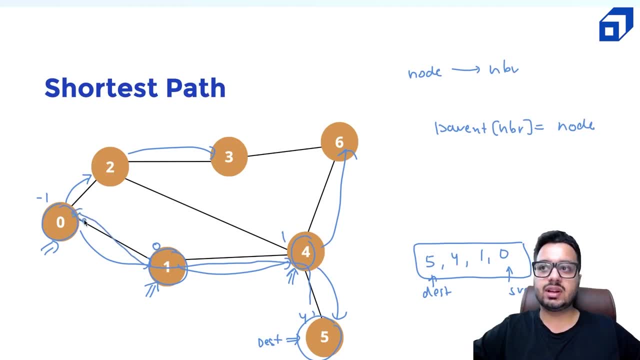 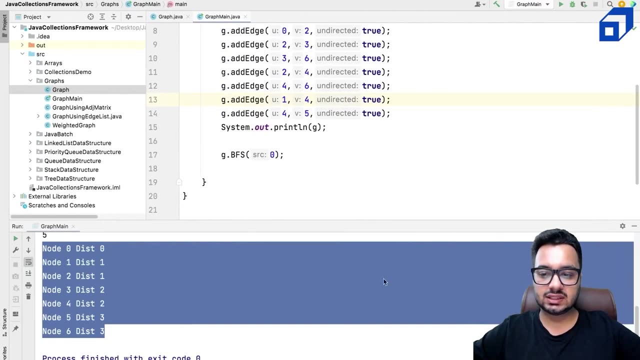 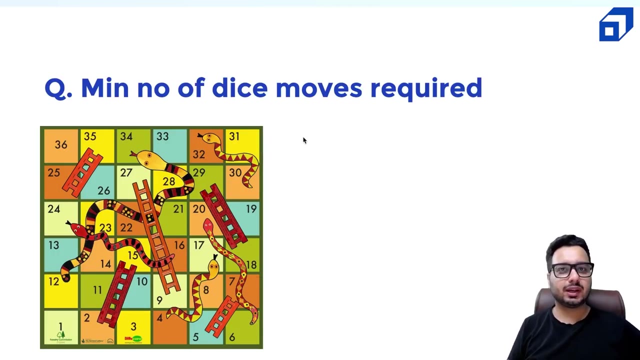 will travel this way. you will travel this way and you will eventually reach the source. so this is something you have to try, you have to figure out, you have to make the required code changes in the algorithm that we have discussed. now we will discuss one application of bfs in solving. 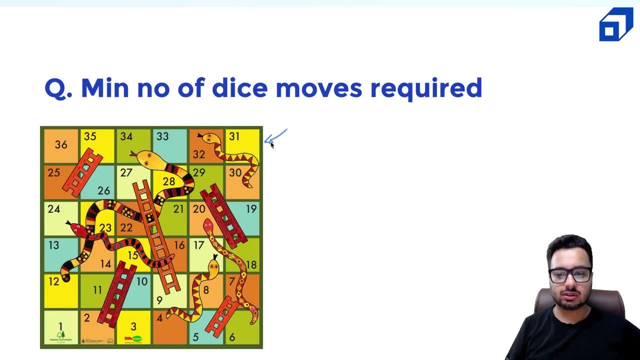 a problem. so we are given a snakes and letters board which looks like this, and what we need to do is we need to find out the minimum number of山. yeah, so our bf1 is represented by hotel company and second nine we need to give it this code name, right? so let's just put this code name here. 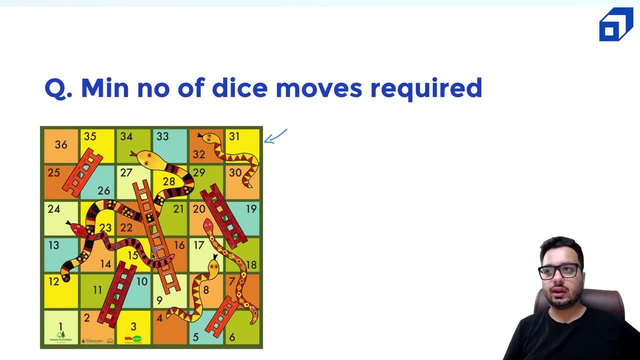 that's coming. currently, um go, it's coming, that's coming. we have to find out the minimum number of number of moves that are required to go from source, which is from cell one, to destination, which is cell number 36. so first of all, we need to decide whether it is a graph problem. so if 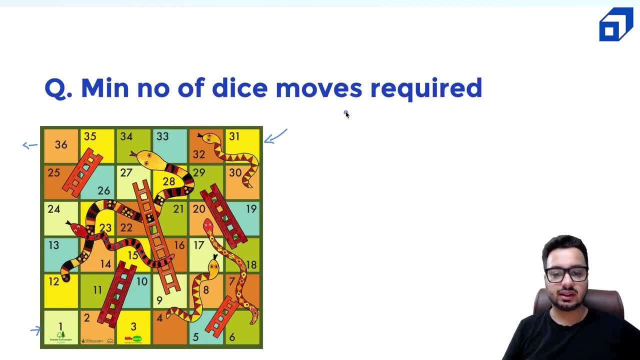 you look carefully you can analyze that. we can clearly see there are 36 vertices. there are 36 nodes where you can go so clearly we see vertices. but how do we decide the edges right? basically it. the question is: there is a regular dice, so on your dice you can throw any number of your choice. 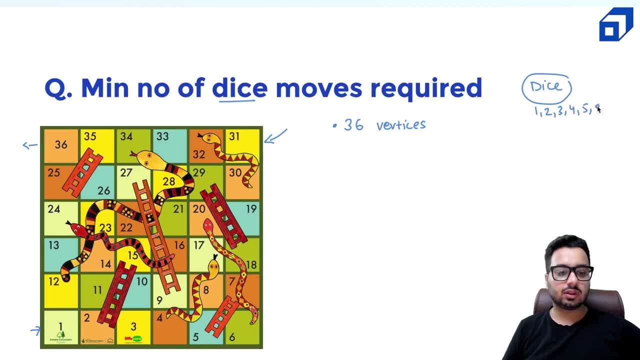 from one, two, three, four, five, six, right. the rules of the board are very simple. whenever there is a ladder, you can climb that ladder, but whenever there is a snake, you will be cut by the snake and you will reach the tail of the snake. so you can cut down from head of the snake and you can. 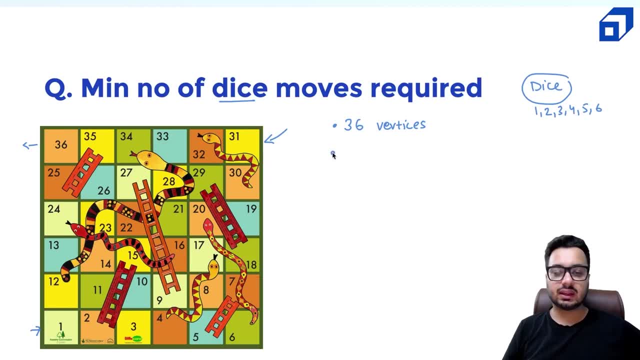 reach the tail this position right. so basically, like in any snakes and ladders gone, you have snakes which can cut you down and bring, bring you down, and there are ladders which you can climb and move to the top. the question is how many minimum number of dice moves will be required. 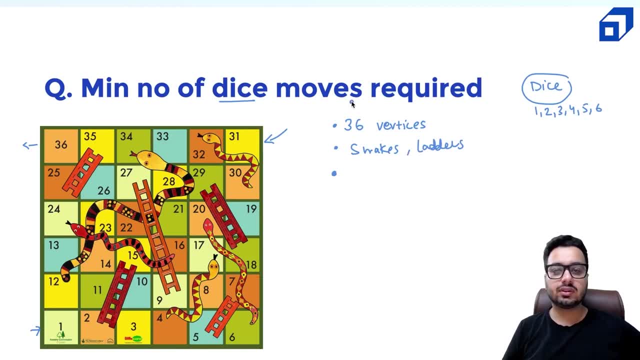 to reach this destination. so you can assume there is only one player. it's not a two-player game. so the question is only about finding the minimum number of dice. we need to think carefully what kind of graph it is. if you analyze carefully, you will analyze that. if 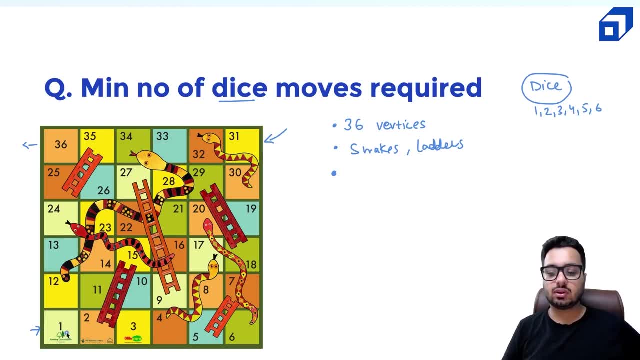 we count the. if you look at the dice moves. so at one you can throw a one that means you can reach two. but at two there is a ladder that means you will reach 15. so if i talk about this edge- there is a edge from 1 to 15 in this graph- then if at 1, if you throw 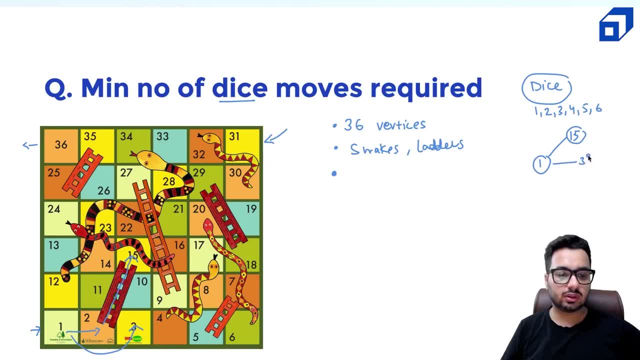 a dice 2, you can reach 3. there is an edge from 1 to 3. also, if you throw a 3 on dice, you can reach 4. that means there is a edge to 4 as well, and all of these edges are directed. 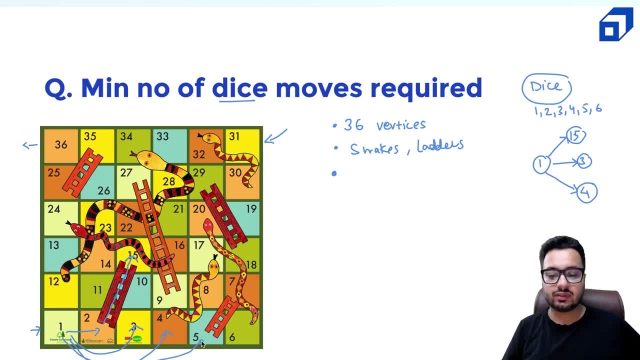 edges and then if you throw a 4 you will reach 5, but on 5 there is a ladder, so that means the edge is from 1 to 7, right, and if you throw 5 you can reach 6. that means there is an edge from 1 to 6 also. 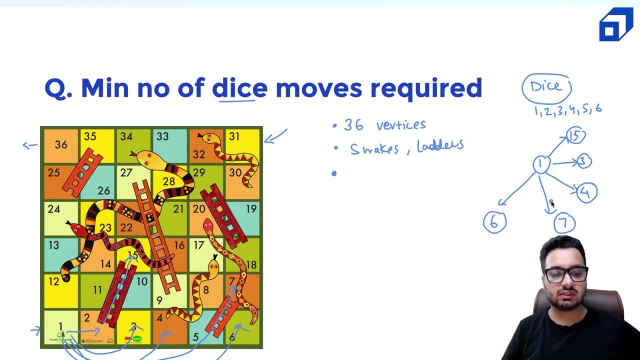 right now, if you throw 6 you can also reach 7. that means it is the same edge. we will not count that edge again. again, starting from 2. so 2, there is a ladder, so we do not need to do anything. then you would go at 3. so from 3, again there are edges. 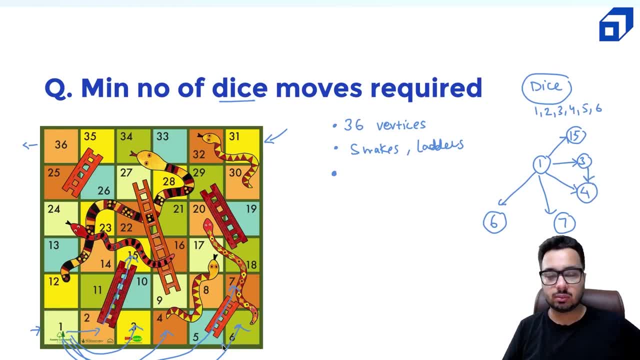 so there is an edge from 3 to 4. if you see carefully, from 3 you can go to 4, and so on. from 3 you can go to 7. also from 3 to 7 there is an edge, and so on. that means how many edges? 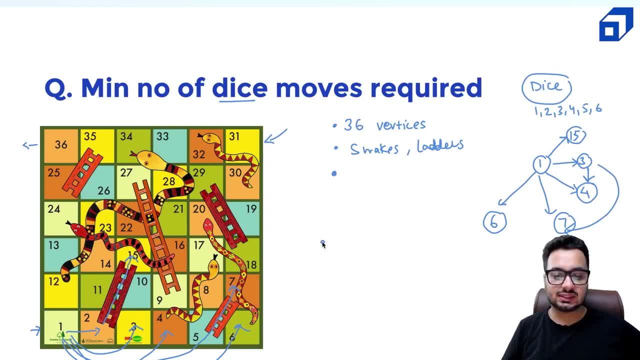 i have. so i have approximately 6 edges, starting from each vertex, from approximately 6 edges from each vertex. okay, so if the vertex is v, i can go to v plus 1, i can go to v plus 2, i can go to v plus 3, v plus 4, v plus 5. this would have been the case if there was no snake. 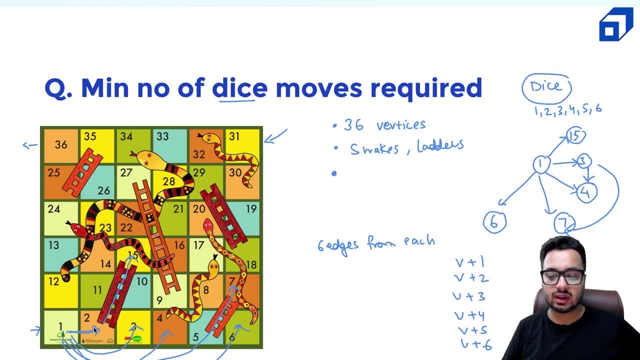 and no ladder. but now what is happening is suppose i go to v plus 1. here there is a starting point of the ladder, so that means i will reach at some other position. so that means there might be a factor which will add up or which will be subtracted, and that factor will come. 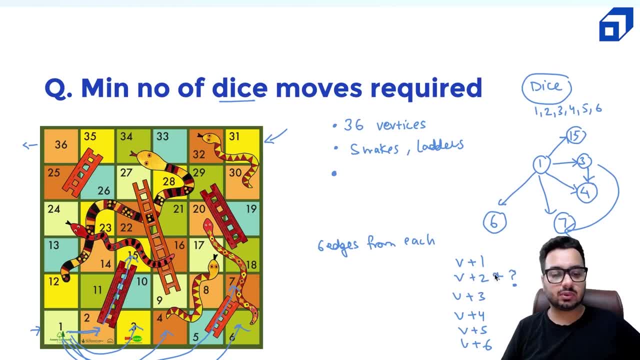 from if there is a ladder at that position or if there is a snake at that position. right, that is what i am saying: that it is an example of a directed graph. so that is what i am saying: that it is an example of a directed graph. it is an exam. is it a weighted graph? the answer is no. it is an example of unweighted. 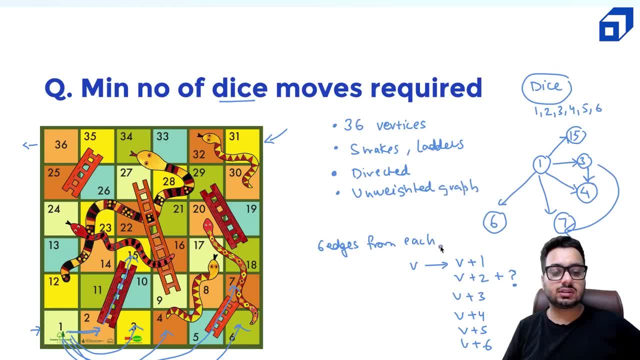 graph. that means all edges are equal, because the cost to cover in any edge is dice throw. so it does not really depend what number you throw on the die. each move is counted as one throw right. so if you analyze carefully, you will see it, it becomes an example of a directed 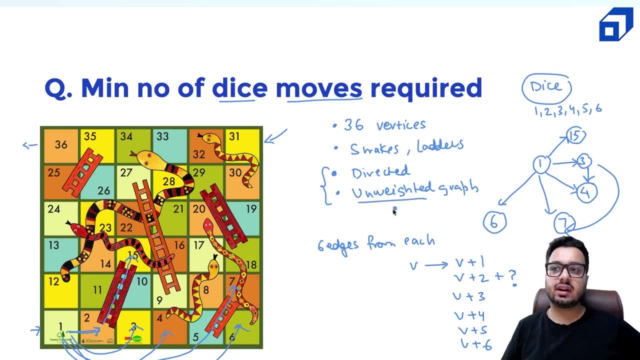 unweighted graph. and if it is unweighted graph we can use the bfs shortest path algorithm to find out how do i reach this node right. so in this case, if i analyze little more carefully, i will see: from 1 i can go to 15, from 15 i can throw. 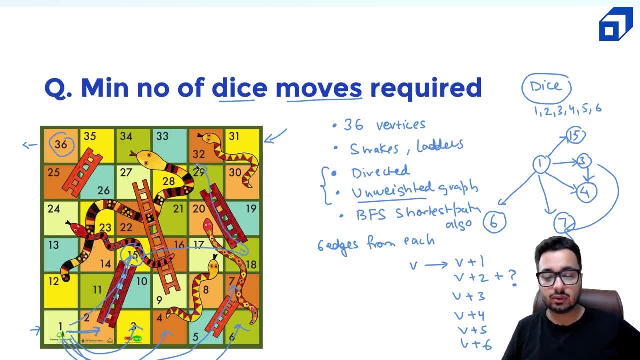 3 and i can reach 18- 18. there is a ladder. i can reach 29. in order to reach 29 i just need two moves, then i can throw one to reach 30 and then i can throw six to reach 36. so i guess in four moves i can easily finish this game. so i hope the problem statement. 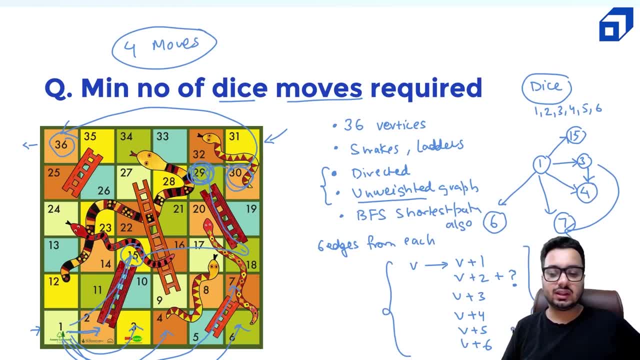 is clear. now it's your turn to figure out. how do we construct such a graph? take input such a graph. so, regarding input, you will be given the number of vertices, the number of snakes, the number of letters, as well as the position of the ladder, for example, two to 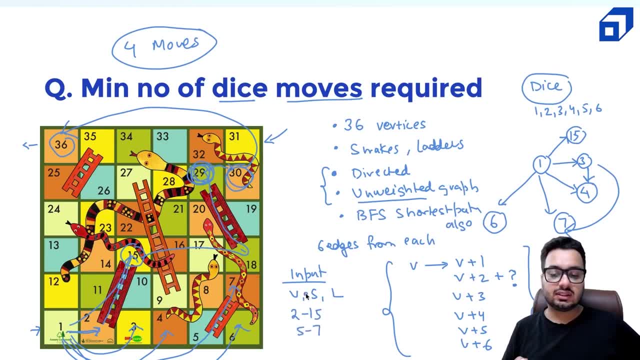 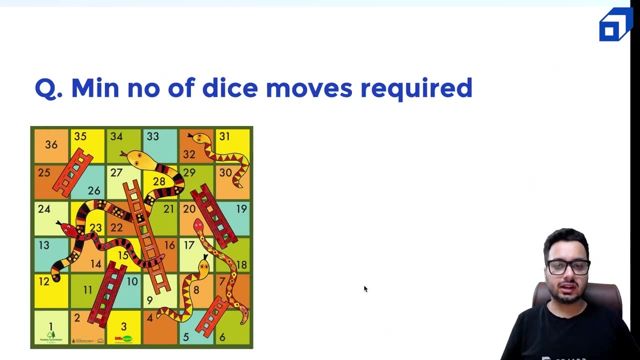 15: there is a ladder. five to seven: there is a ladder right. similarly, positions of snake will be given as pairs. 17 to 4: there is a pair right. so take a moment to think: how do you input such kind of a graph and how do you make your bfs algorithm run on it? all right. so let us discuss. 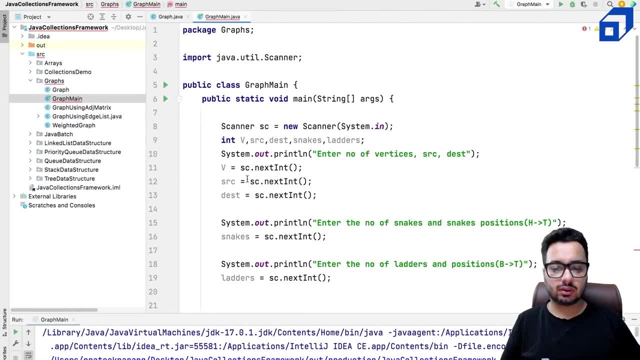 how we are going to build the algorithm. so i have written some boilerplate code. it's not the complete code, so i'm going to read some, some inputs. i'm going to ask: enter the number of vertices, source and the destination. so i'm going to read these three things. after that i will 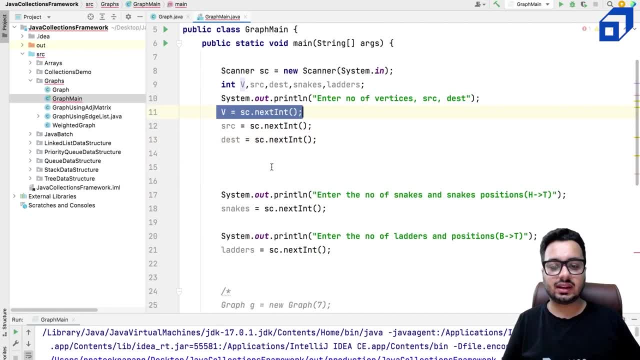 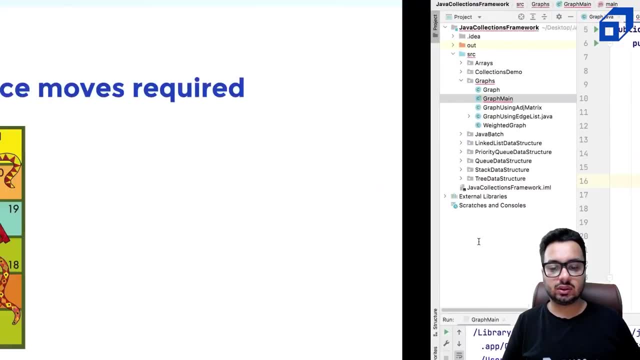 create a graph, since i know the number of vertices right. i can create a graph object, or i can do it later on as well. that's fine, and i'm going to read the number of snakes and their positions. so in our scenario we have one, two, three and four snakes. number of snakes in my case are four and 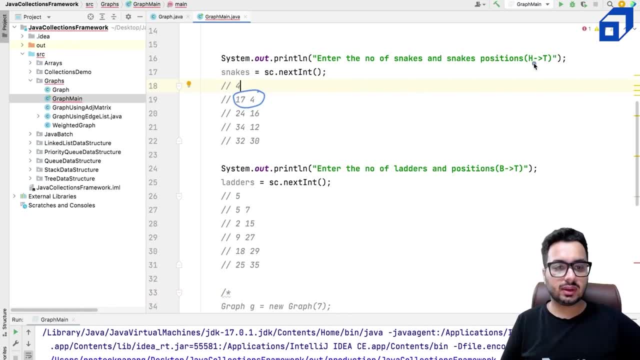 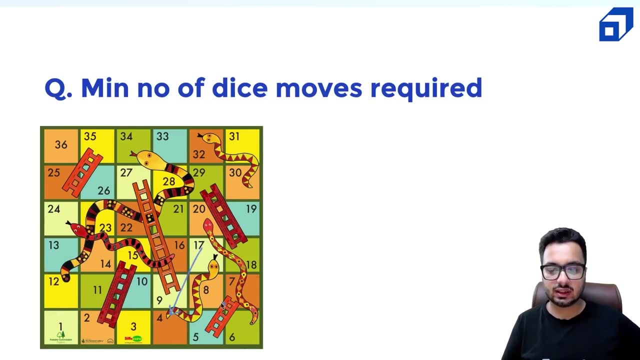 these are the positions of the snakes: 17 to 4. so i'm taking in this direction head to tail. so that means 17 to 4. if there is a snake, you look carefully, 17 to 4, this is the snake. similarly, i'm reading the letters in this direction: 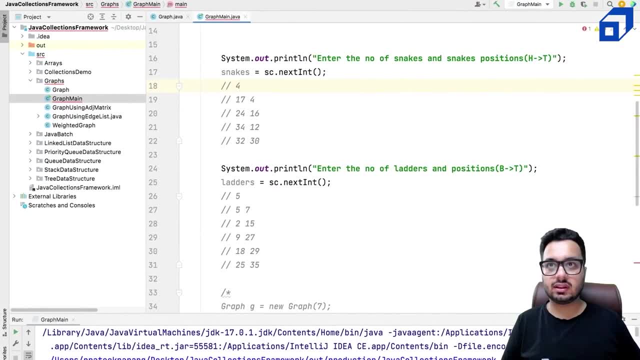 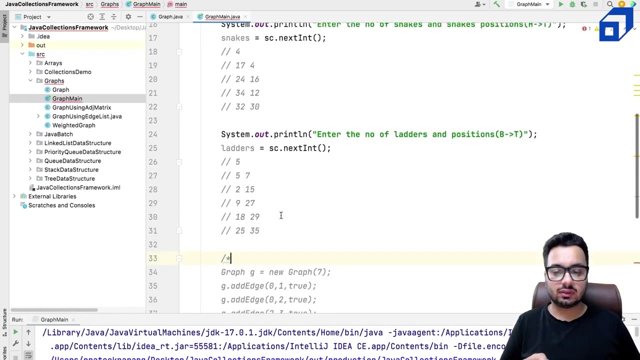 five to seven, there is a letter. so five to seven: there is a letter. the question is: how do we like handle this data? what should i do with this data? first of all, i need to read this and i need to make sure that this data is used in my construction of the graph. earlier we were 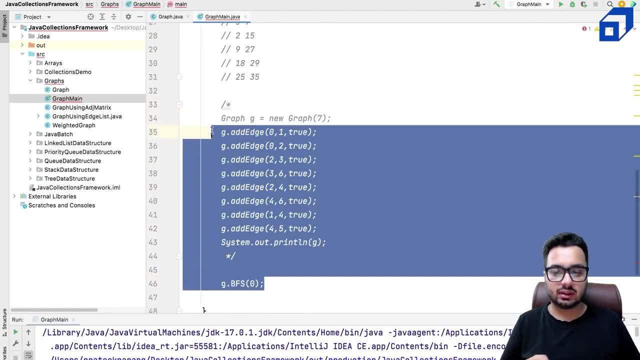 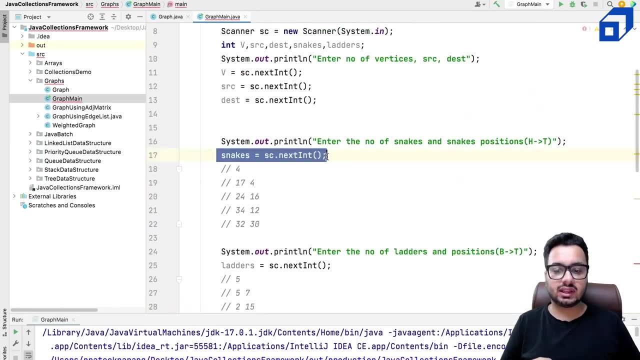 creating a hard-coded graph, so we'll not do that thing here, right? so we'll create our own graph. the first thing is: here i'm just reading the number of snakes. i'm not reading what snakes i have, so i need to implement logic for that as well, right? 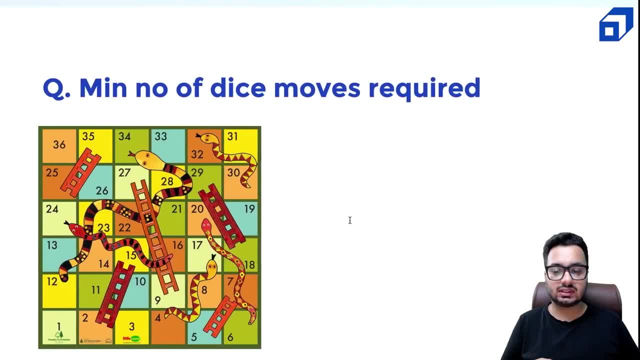 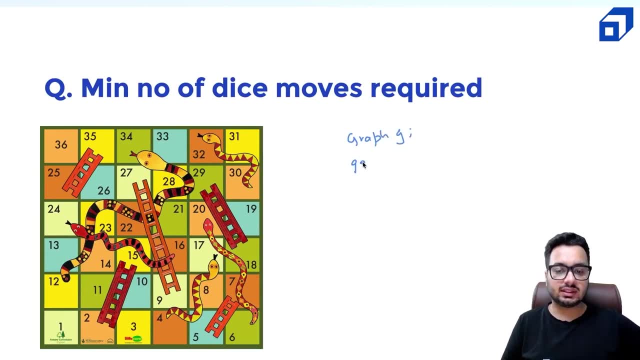 this part. i'm going to do it right now. so let's try to understand how we will actually create a graph. so we'll create a graph- object see- and we will, of course, we'll try to add edges to it. add edge now in edge. you need to know that from where the edge starts and where the edge ends. 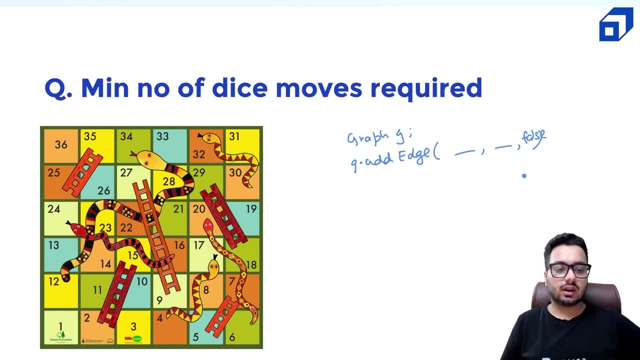 right, and it is a directed edge, so it's not a undirected graph. so i will set this third parameter. now, if, if i talk about vertex one, so i told you, from one i can go to, let's say, vertex i, i can go to, i plus one, i can go to i plus two, i plus three, i plus four, i plus five, i plus six and plus. 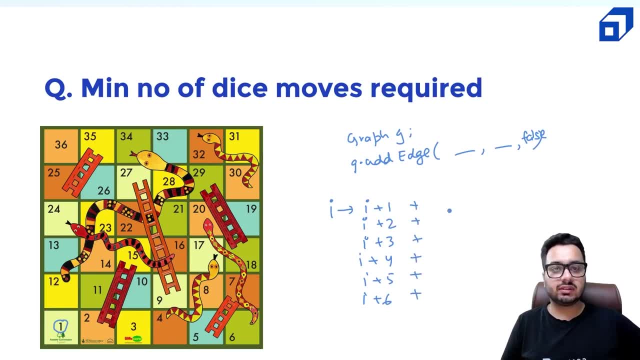 something right. this value could be zero. this value could be positive value. this could be negative value. what is this something going to be? it will depend upon whether there is a snake or a letter. starting from that position, for example, i plus one, so at two i have a letter. 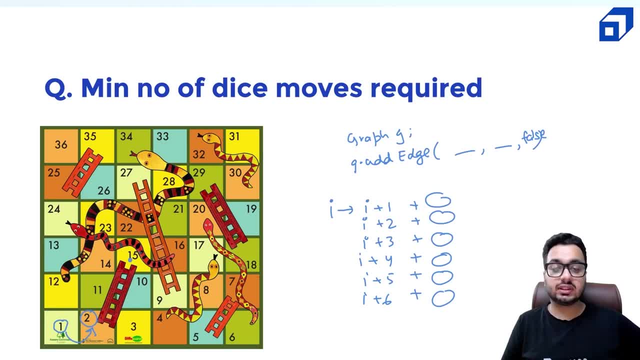 gives me which actually takes me to 15, right, which which is actually taking me to 15. that means i'm getting a jump of 13, right? so, for example, if i is one, i take a move of one, i reach two and two. there is a letter which is giving me a jump of 15 minus two, right? so basically there. 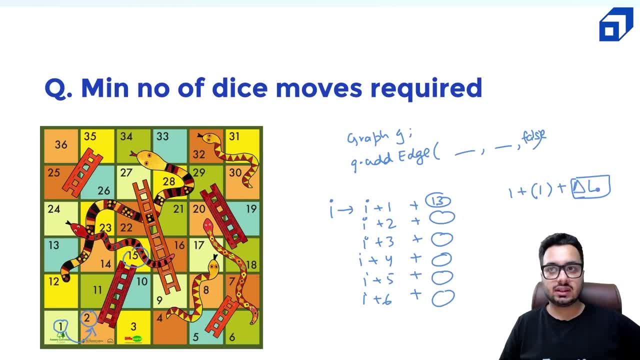 is a letter, so the delta that is given by the letter, right. so if i go to, let's say, uh, i, i plus three, so there is no letter here, so this delta will be zero. this delta will be zero, i plus four, i reach five. at five, i actually reach seven. so this delta is two. how do i compute this delta? 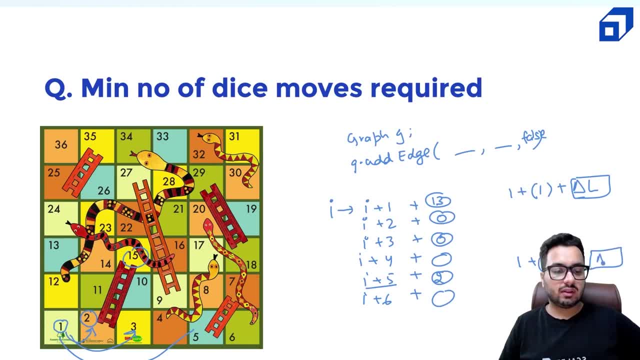 this delta, i have to compute and store it in a array. i have to compute and store it in an array. so that means in an edge. this becomes a starting point and this becomes the ending point of the edge. so this delta is very easy to compute. for example, you are given there there is a letter. 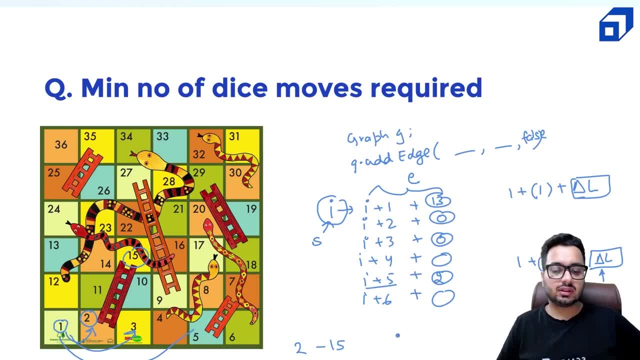 from 2 to 15.. you can easily say: okay, i am going to store it in an array and i am going to store it in some kind of array. let's create a board array, right, so it's. it's a 1d array of 36 positions. 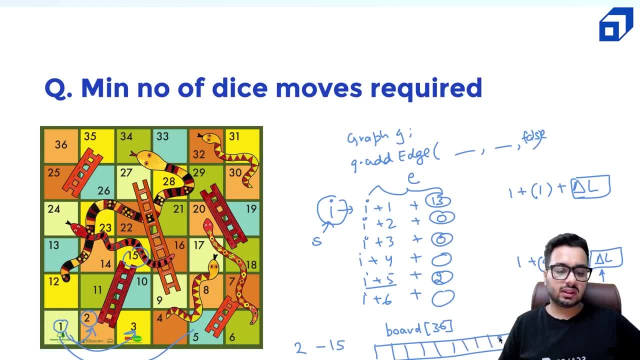 and in each position i'm going to store a delta. if someone says: okay, there is a letter from 2 to 15, that means at the second position in this array i can store 15 minus 2, that is 13.. so at the second index in this area, i can store 13.. so if there is a snake at, let's say, 32, which takes me, 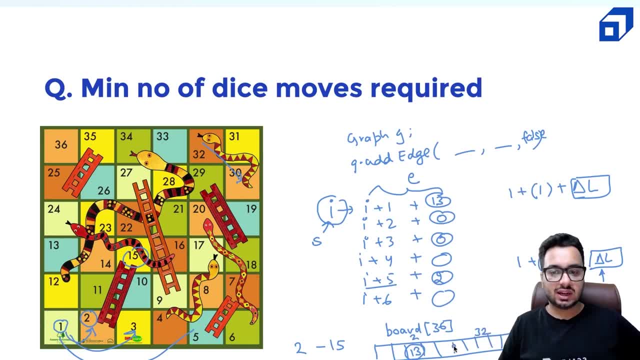 at 30.. let us assume this index is 32.. so at 32 i get a delta of minus 2.. so if i reach 32, effectively i reach 30.. so 32 minus 2.. this is how i'm going to do it. once all the edges have been inserted into the graph, i can easily run. 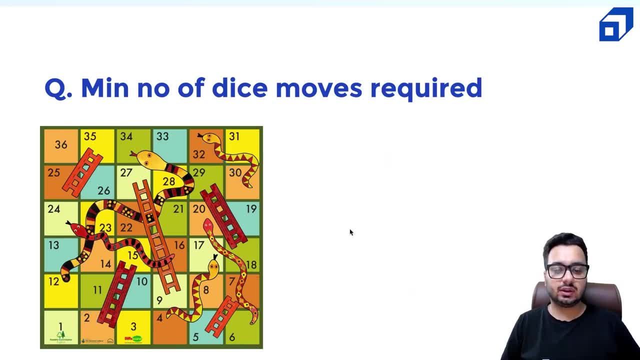 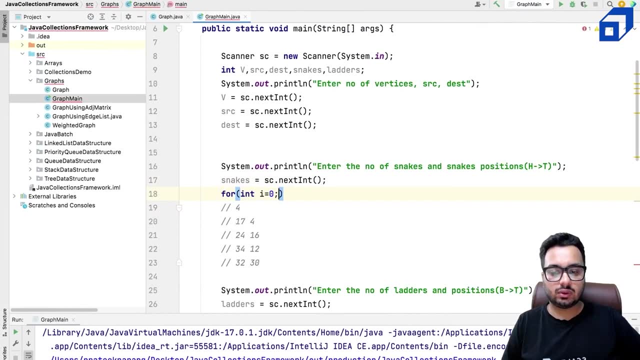 bfs on it. so let us try to insert all these edges into our graph. what i'm going to do, i'm going to run a loop. let's say for i equal to 0, i less than snakes, i plus plus. i can showcase snake as a head. 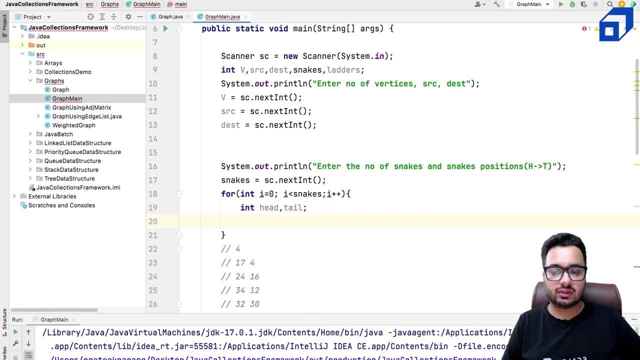 snake has a tail. so i'm going to read these values so i can say: head equal to scanner dot, extent, tail equal to scanner dot. next int. and i'm also going to create a board array so the board array can be created here. so int board and this is equal to new and 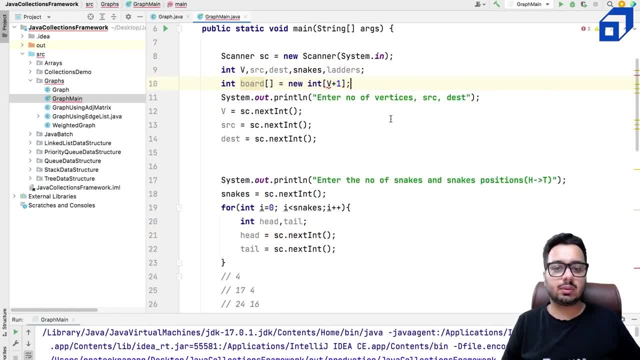 how many. so i'm going to do v plus 1, because it is a one base indexing here. so i've created a board array. oh, i have to move this code here because v is not input yet, so this board array will come here, or you can do it like this: that's fine. that's fine. board array is now. 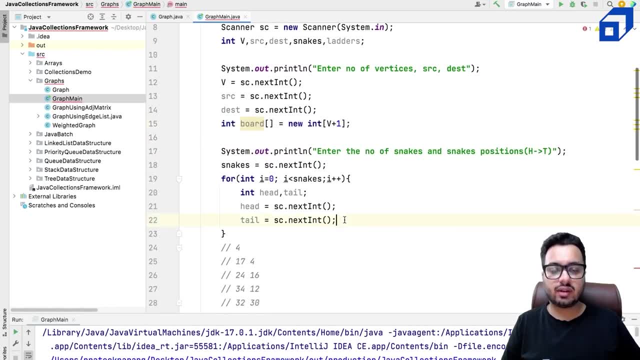 created. so now, when, when i'm reading the snakes right, so i have to update the board array so i can say, okay, board off head in case of snake, the snake is going to bite from the head right, the board of head will store a value that is equal to, because now it is giving you a decrement, so from 17 you are going going at. 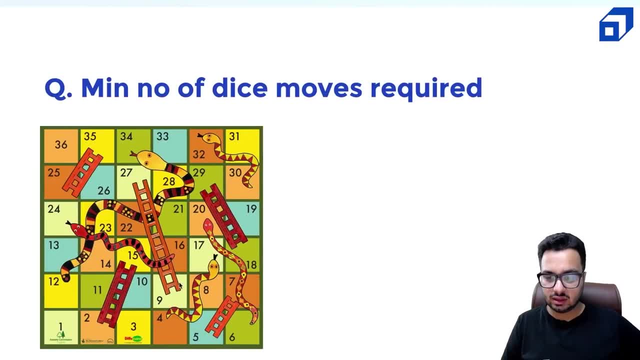 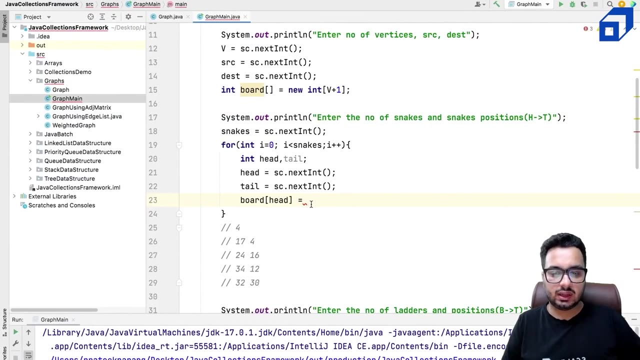 4. right, let's look, look once again. from 17 you are going at 4.. the board of 17 should say that my value is nothing but 4 minus 17.. so this value should be minus 30.. so this is how it should be. so it should be equal to tail minus head. so tail is a small value, head is a. 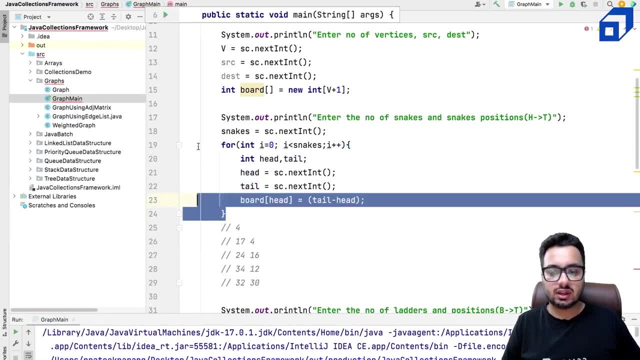 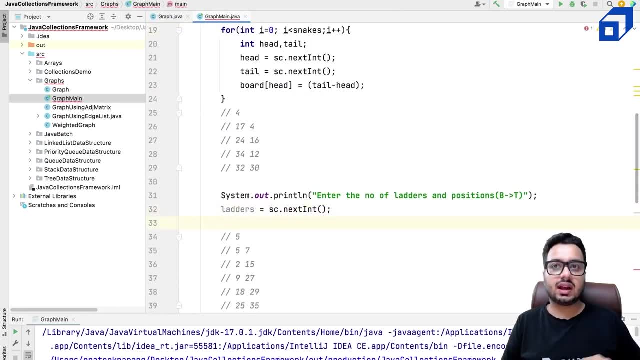 large value, so this value needs to be equal to tail. this is how it should be, so this is how it is needs to be negative. this will update the board array for snakes. similarly, we need to update the board array for letters and we will utilize this array while constructing the graph i will show. 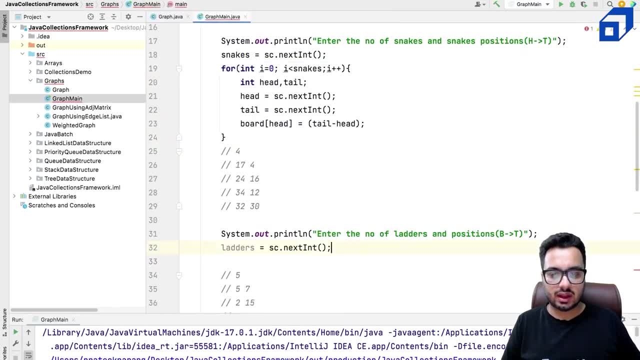 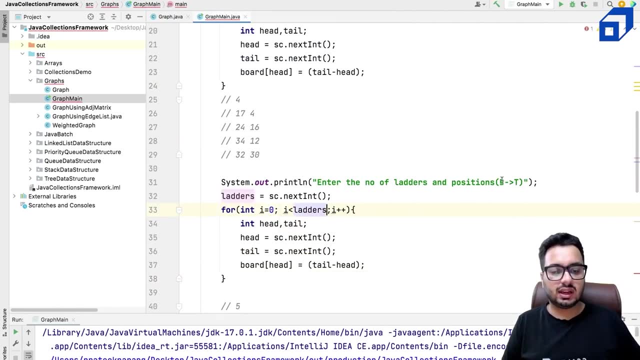 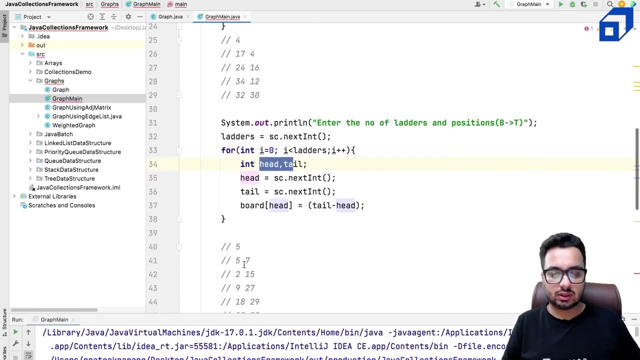 you how make a similar loop? i have the letters instead of snakes here, i will have letters. now the letters are given in this fashion: bottom to top. so letter also has a head and it also has a tail. so tail is this. number is smaller, this number is bigger. tail minus head would be a positive. 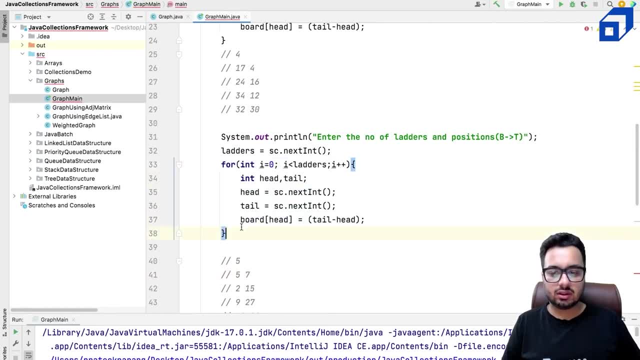 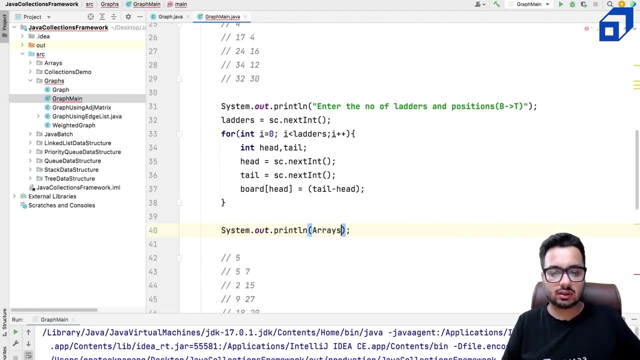 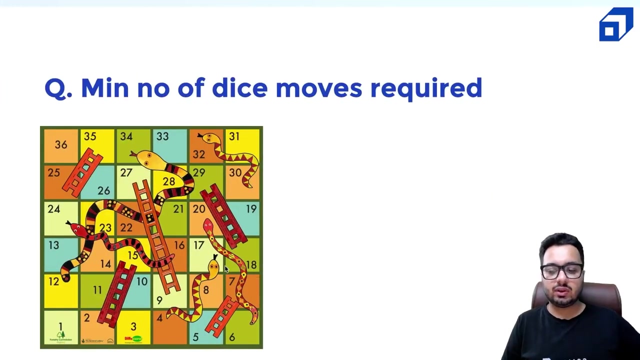 number here. that is fine. so i think board array looks fine so i can just display you the board as well. i can say s out at is dot to string and i can give the board array. now i have this board array, i have these delta increments. again, i need to figure out how do i insert all the edges. now that thing is fairly simple. you need to. 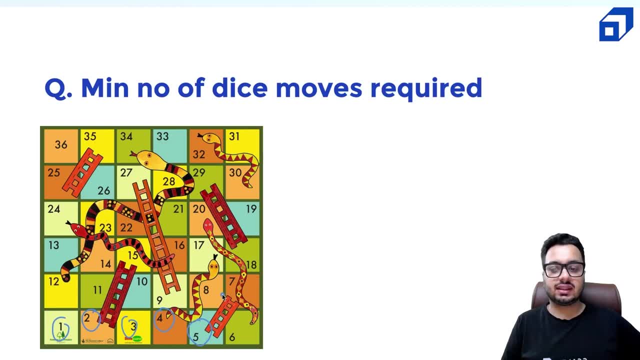 go to every vertex and create the next six edges that will start from that vertex. for example, if i start from five, or if i start from i, i can go to i plus one plus board of this position that you have reached. if you do five plus let's say some number, five or five plus four, you reach nine. but 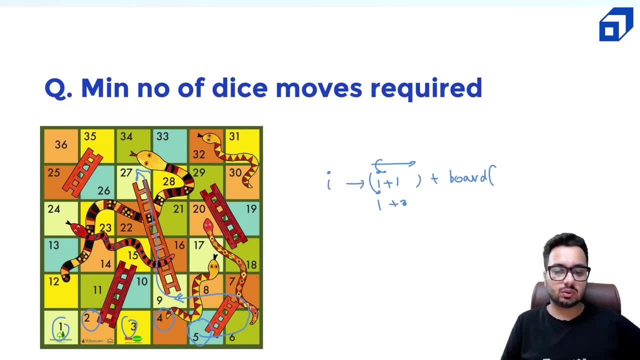 position you actually reach 27, right, i plus two, plus board of this position, i plus three, up to up to i plus six, basically from ith node where i can go. so here i'm going to use the board array to decide where i can actually go. so this will be board of i plus one, board of i plus two, and so on. 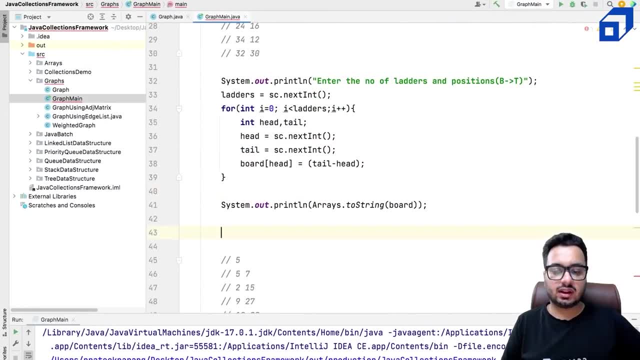 so let's see here as well, let's create the graph now. so i have graph g, how many vertices i have. i have v vertices, so i'll just keep v plus one because it is one based. so we we are also adding zero here. this is equal to new graph. 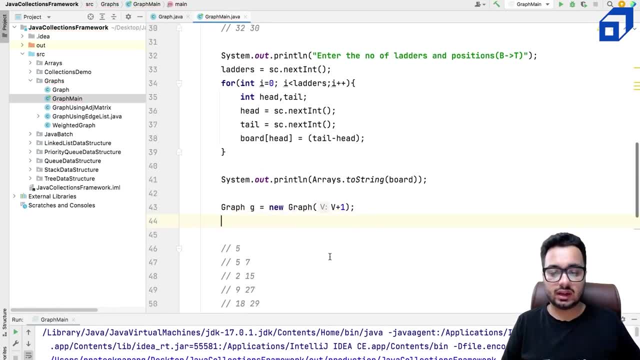 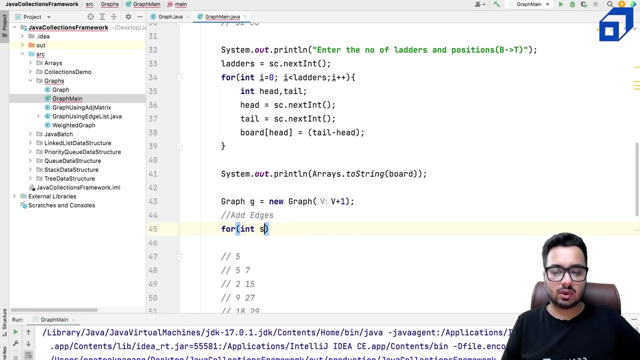 new graph of v plus one vertices. all right, i have to add edges, right, so i can do okay for int. let's say source which starts from. or let's say i'm going to add edge from i to something, so i to some j. okay, so if i goes from, i can start from source, which is one the smallest node i can go till. 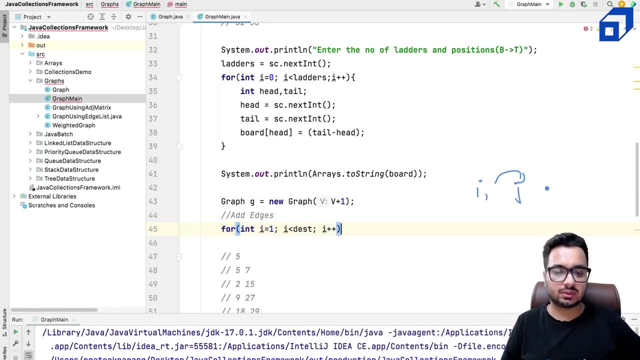 less than destination. that is my last node. i plus plus. so i'm going at every node and i can throw a dice at every node. i can throw one, two, three, four, five, six. so i can throw a dice. dice can take a value one. the maximum value dice can take is six and i can say: dice plus, plus. 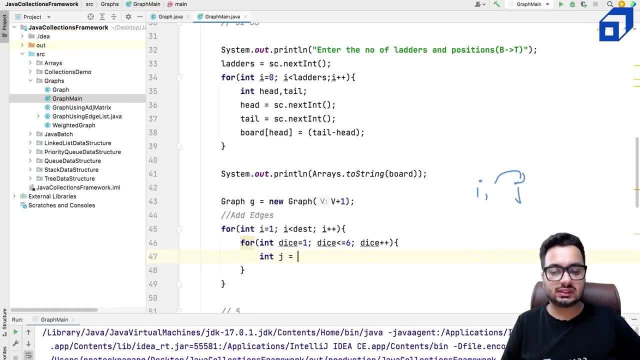 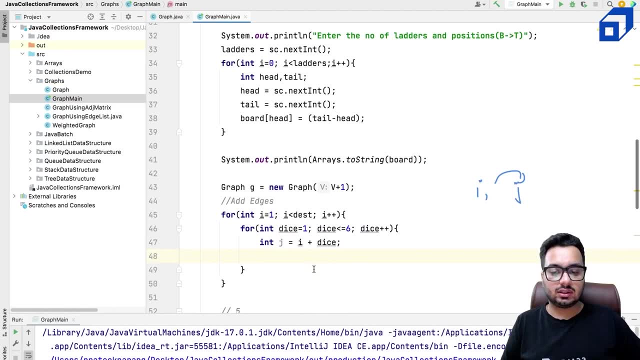 kay, and so what's okay. so what is the node at where i'm reaching? the jth node is i plus dice, but this is not final. i also have to add delta, so i can j, okay, j equal to j plus board of j. so in this value, what i'm saying is: 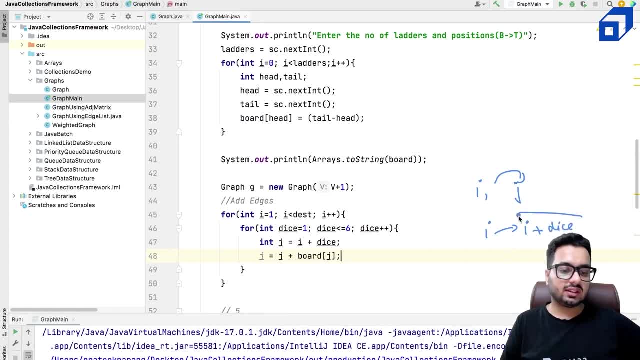 from i, you throw a die, you reach i plus dice. now, at this position, it is possible that there is a ladder. the ladder gives you a jump of 13. to add this factor also, that is stored in board of j, but if there is a snake, that takes you down. 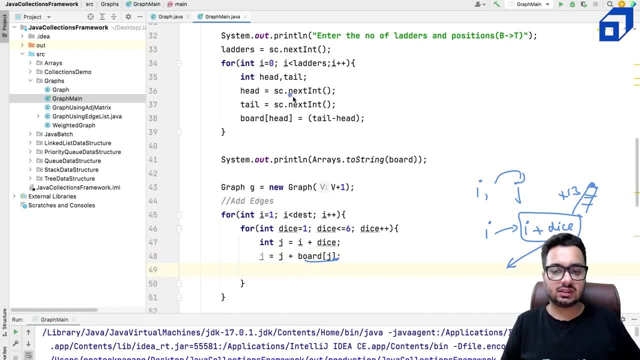 so you have to decrement this value. also that addition subtraction is already handled in the board array. now if j is less than equal to destination, that means i do not want to add any edge. that goes out of the board. so i can say g dot add edge. so u is my i, v is my j and it is a. 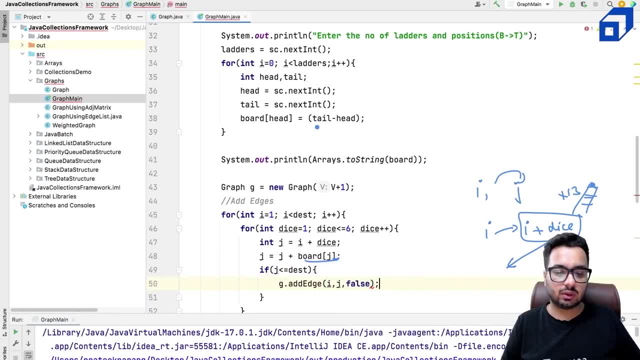 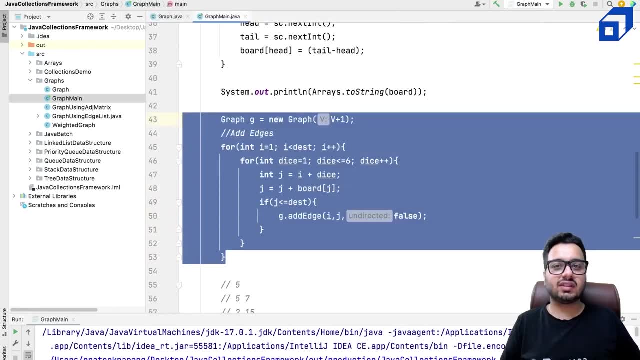 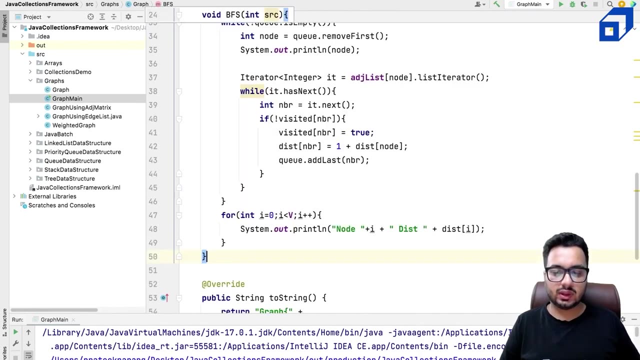 it is not undirected graph, so this value is going to be said to be. this completes the graph creation process. now what we need to do? we need to run bfs algorithm on it. so, as you know, we have already implemented the bfs algorithm. i'll just copy this code and tweak it a little bit so that we can do. 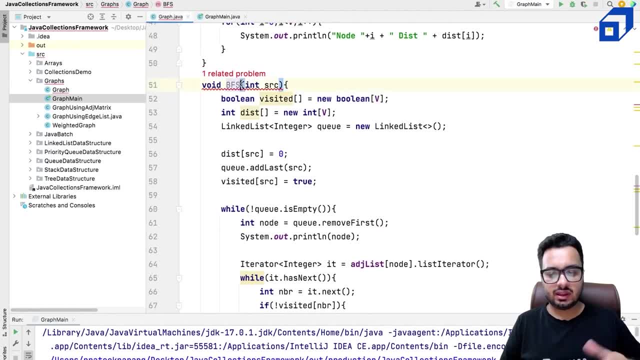 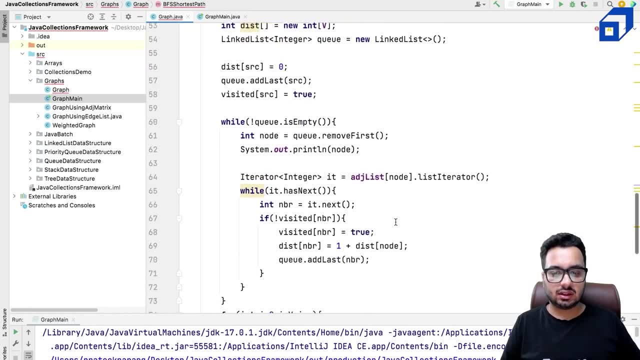 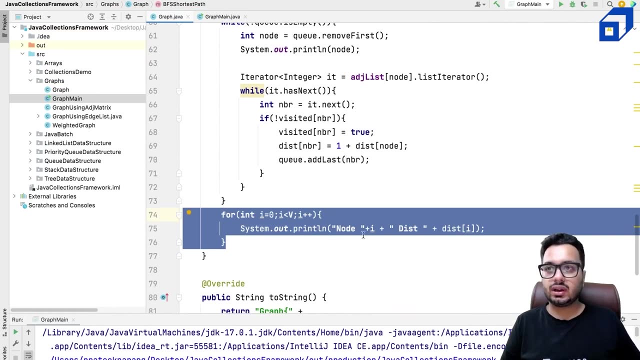 it. for this particular problem i can say bfs dot s path. so in this case i am getting source, i am also getting the destination. so if the user is interested in finding out uh, minimum number of moves. so you do not need to print distance every node, you can simply return the distance of destination and you can change. 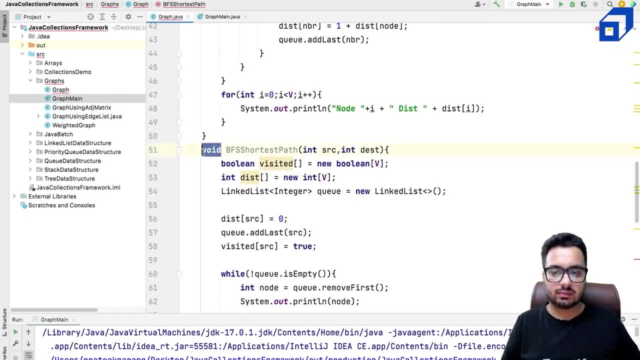 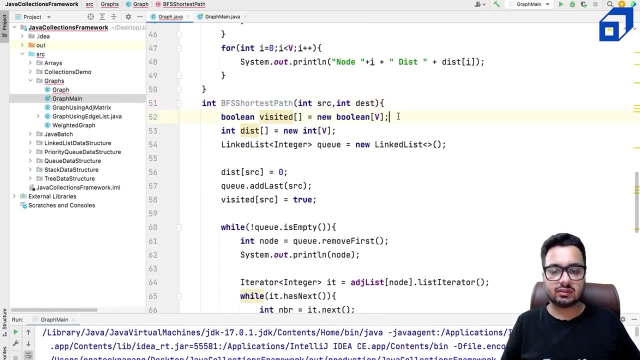 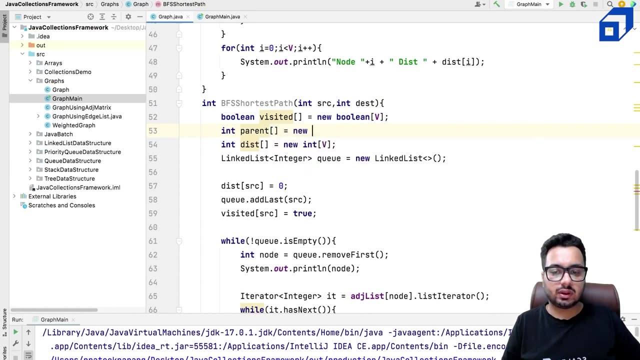 the return type to integer. this can be done. now, one thing might ask is: user might ask you to give the path. also, as i discussed with you, along with the visited array you can create a parent array as well and you can say, okay, this is equal to new, new integer of v, and here you can say okay, 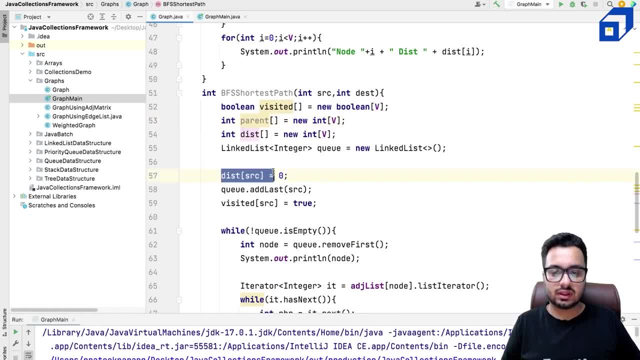 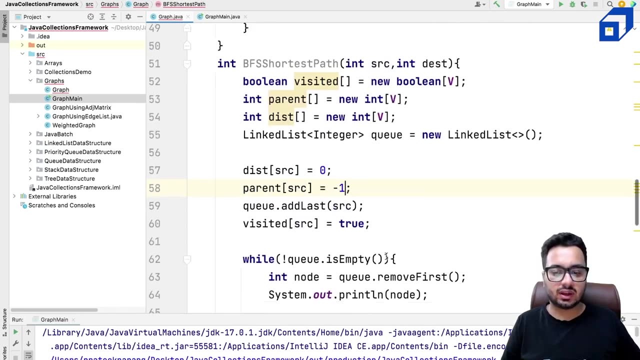 for first node, that is, my source node, the parent is, let's say, minus one. so, parent of source, this is minus one, or you can set this is the source itself, something like this, so that you can know right right now i can. i'm just saying this is going to be minus one and whenever you visit a node, 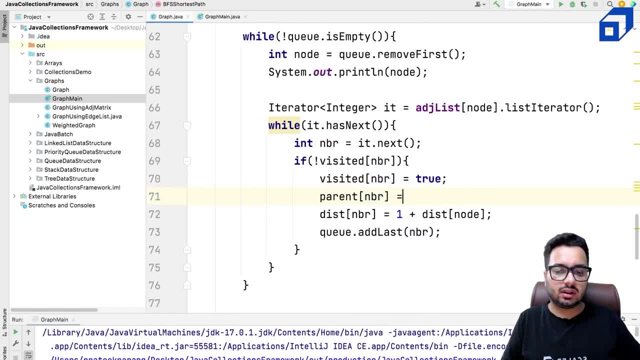 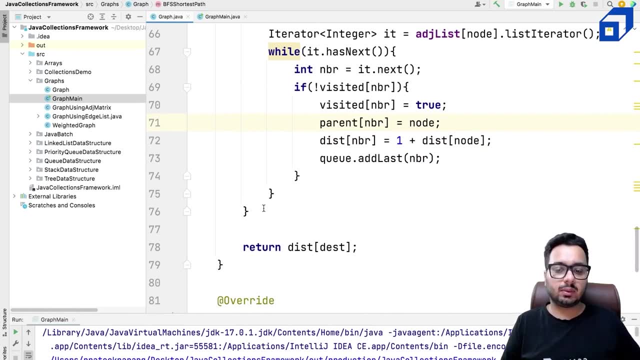 you can set the parent. parent of neighbor is going to be the node. now, as i told you, you can backtrack and you can find out the complete path as well. let us discuss that thing as well. if you want to do the path printing, that is fairly simple. you can start from the destination node. let's say: 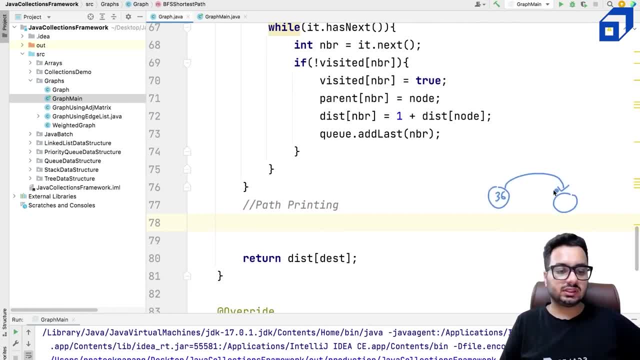 36, now 36 nodes from where i was visited, so maybe the parent of 36 is 30 right, so i can start from this node, reach this node again, ask the parent, go back, go back and so on. i can trace the path until i hit one or minus one, something like that, so i can define. uh, i take a temporary value which is: 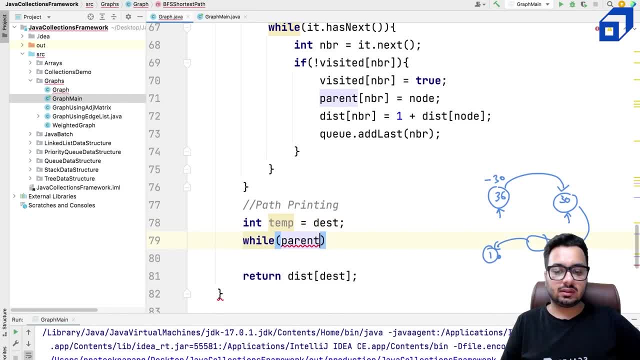 destination and i can say: while parent of destination or while parent of temp is not equal to minus one, what do i do? i say, okay, fine, i will print out the destination. i will print out the temporary node. persistent node. call as terminal node temples of destination node or residences of destination and um kernel of hisАnrias to parent of ему, sustenance node. ok, dispatch, i will print out the destination, i will print out the temporary node. so basically, just this kind of thing. okay, i will� 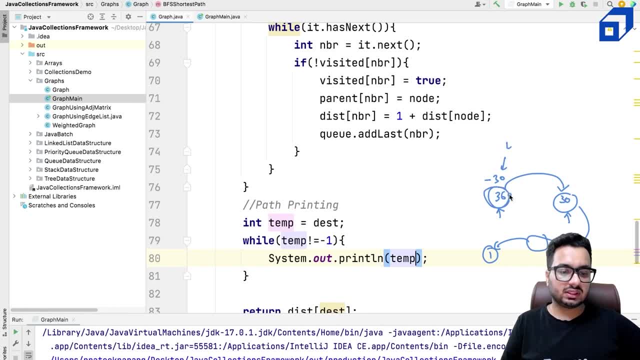 what I'm saying is the temporary node is this temporary node is 36. I will print it out and I will go here. this will become the new temporary node. but how do I update this temporary node? so fairly simple: temp equal to parent of temp. at every node I take it back to the parent, so this: 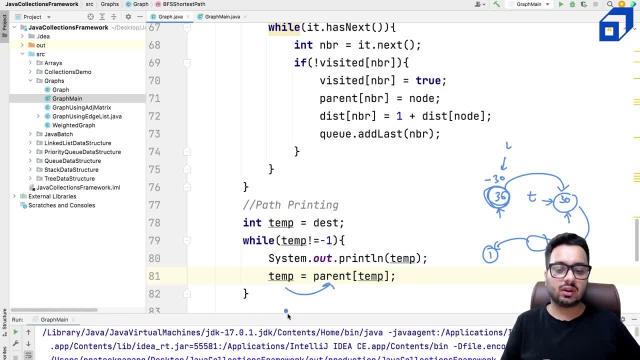 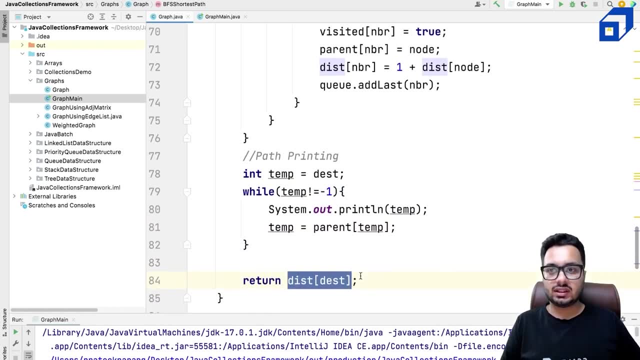 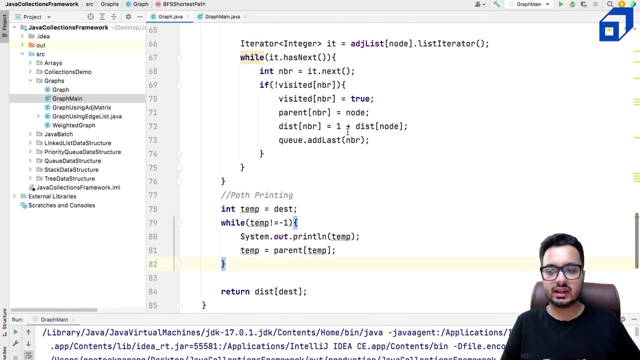 is basically going back to the previous node in the path, how it was discovered. then I'm saying: return the distance of the destination. now let us go and run this code. I think it should be fine. yeah, it seems fine. let us try to execute the code. so I have given the input. I've just combined the. 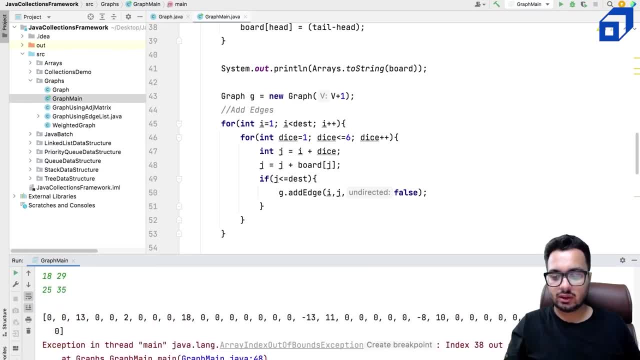 input and I'm giving it, but now I'm getting the error. actually I'll tell you what. what is there? so it is saying exception in thread main index, that it out of bounds. so in main day this is the array. so this is going out of bounds. why this is happening? because 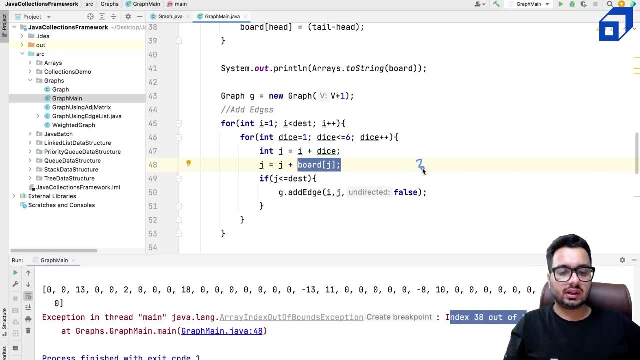 if you add something to, let's say, node 35 use, okay, I will take a jump off 3, you will actually reach 38. so you actually I'm checking it here. so instead this check should be done here, right? so when I'm doing this value here, when I'm computing this J, so I should do this thing here if J is less. 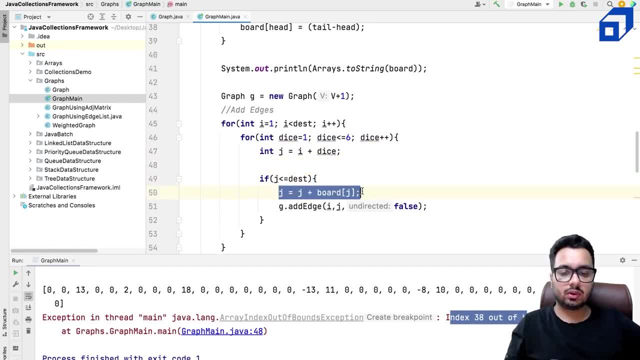 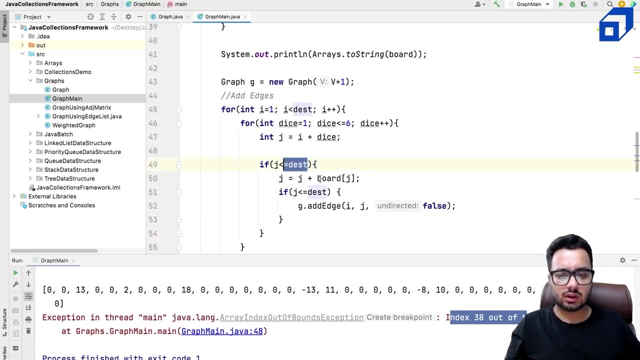 than equal to destination, then I should do J equal to board of J and again I should check if J's. you can do it here, that is fine. so if J is now less than equal to destination, then you can actually add that edge. I think this would be okay. or you can do two conditions here, right? so you need to check that. 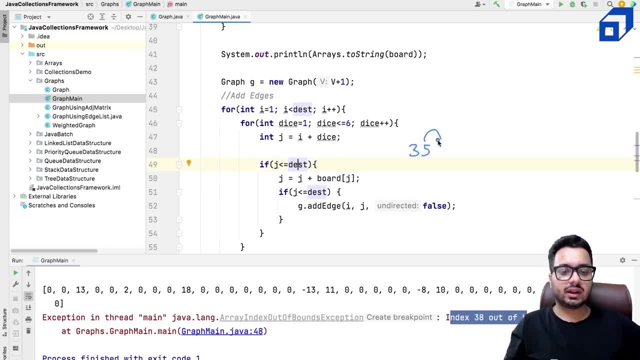 see what is happening is I added something here. I said, okay, 35 plus 2 or 35, let's say 33 plus 2. okay, and suppose there was a letter here. right, it might. it's not going to take you out, but what I'm? 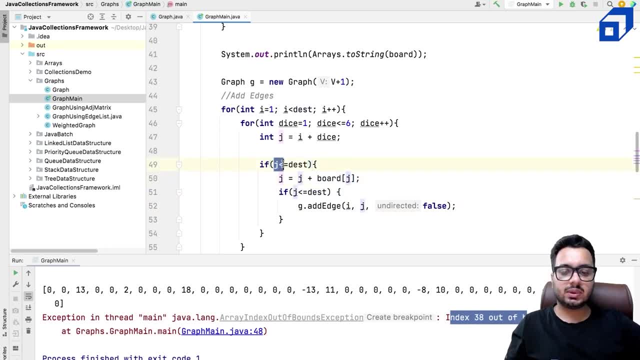 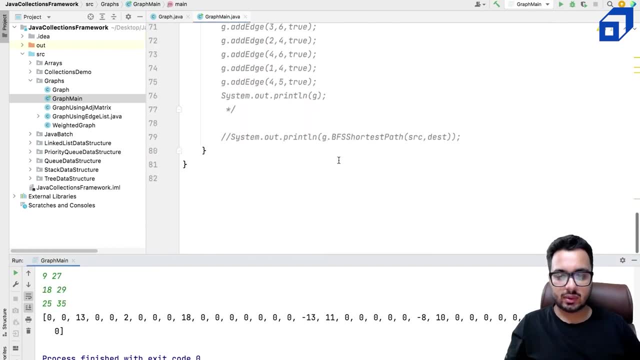 checking is that when I'm adding this value board of J, they must be less than destination, and when I'm adding the edge, that edge must be less than destination. let me run the code. okay, so I think I commented out the shortest path. let's re-run this code, and it should be good to go now. 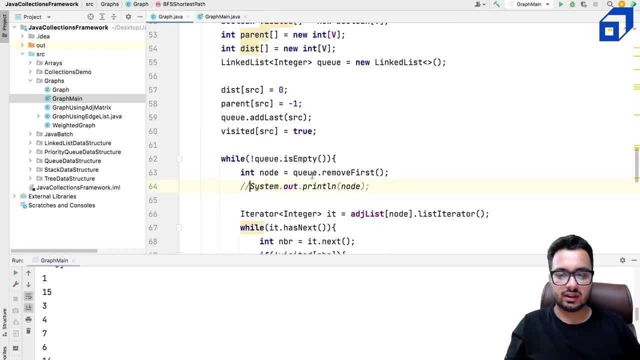 so we do not need to print each and every node while traversal right. one more attempt and then we should be good to go. we are doing bfs, we are printing the output of reversal, which we don't want, so let's paste the code and here we are getting. yes, this is the 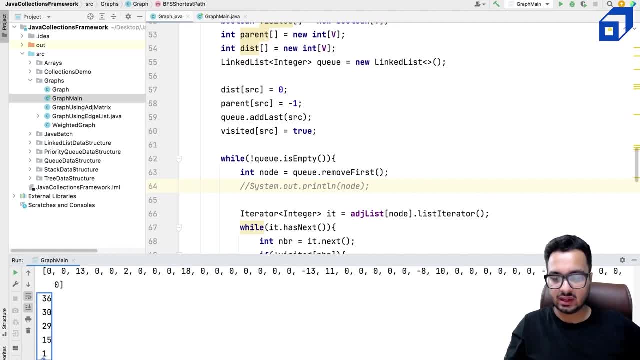 correct output. we are getting the path and we are getting the shortest length. that is going to be four. if i show you, this is the path that we are getting from one we went to 15, 29, 13, 36 and it took four number of moves. four moves were required to cover this. you can verify also. 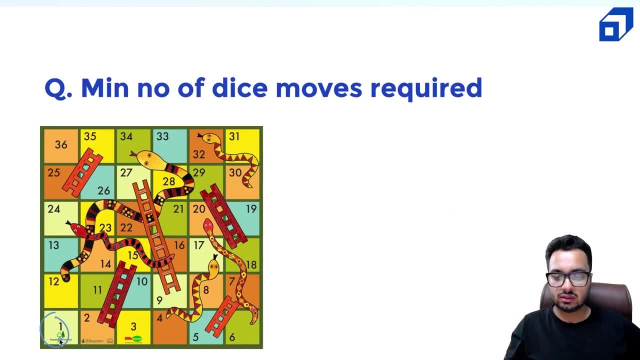 1, 15, 29, 30, 36. from 1 we went to 15, then we went to 29, then we went to 30 and then we went to 36. yes, these are the four moves that were used, so i really hope you understood this algorithm really. 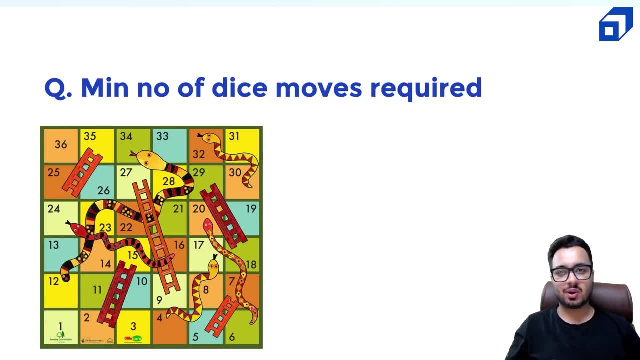 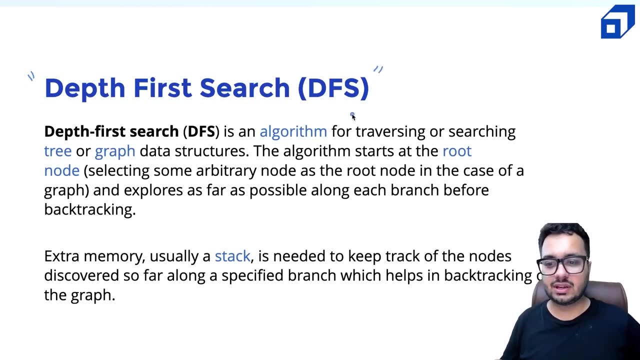 well, and the application of bfs we have seen through this problem. let's try to understand this algorithm called depth first search, or sometimes called as depth first traversal. it's an algorithm for traversing the graph or searching the graph. it can be used on tree, so on tree the pre-order. 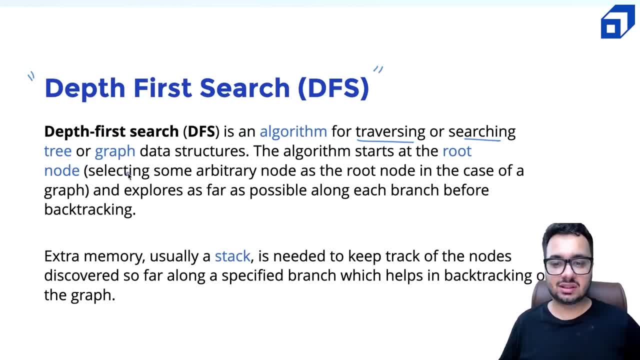 traversal that you have done. it's actually a depth first search. the algorithm starts at root node, so in in case of graph there is no root node. so you can arbitrarily you can select any node as the root node and or you can have a some specific node and you have to explore as far as possible along. 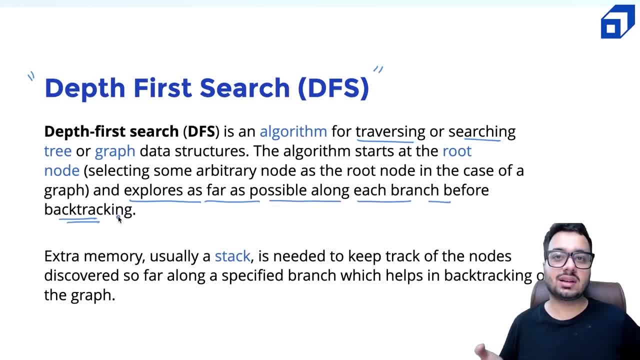 each branch so you can have a specific branch before doing the backtracking. so we'll try to understand this through an example. and of course, this algorithm, since you are doing it recursively, uses extra memory, which is usually a stack. so if you're using a stack, in case of recursion it will be created. 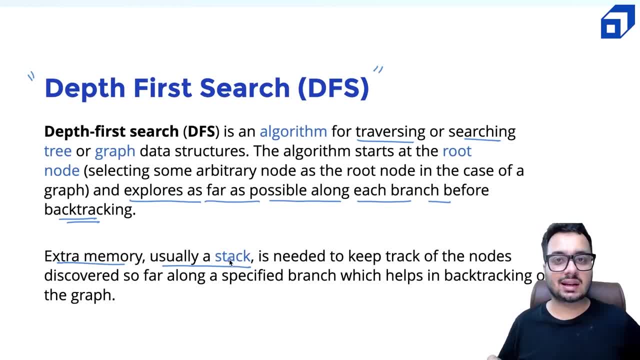 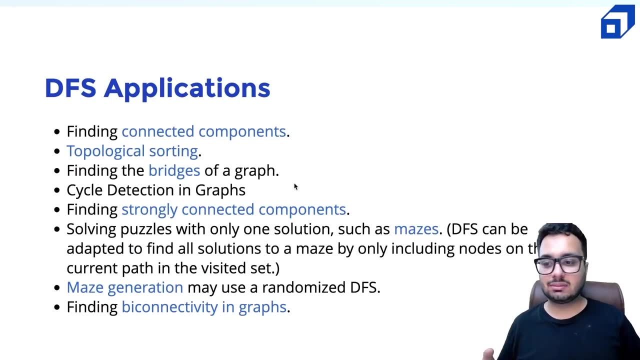 automatically. even if you are doing this algorithm iteratively, you can maintain a stack like data structure and do the work which is needed to keep track of nodes discovered so far along a specific branch, which helps in the backtracking in the graph. so let's go ahead and run this concept while when we are running through the algorithm and this dfs. 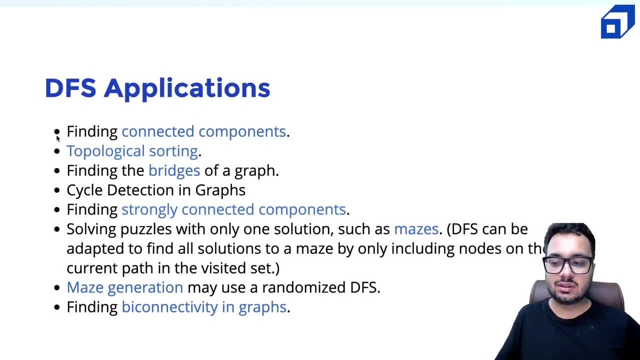 has many applications, some of the applications i have listed down here. it is used in finding out connected components. you can also use bfs here. basically, you want to look at what components of the graph they are connected. so, for example, if this is a graph, this whole thing is one graph. it. 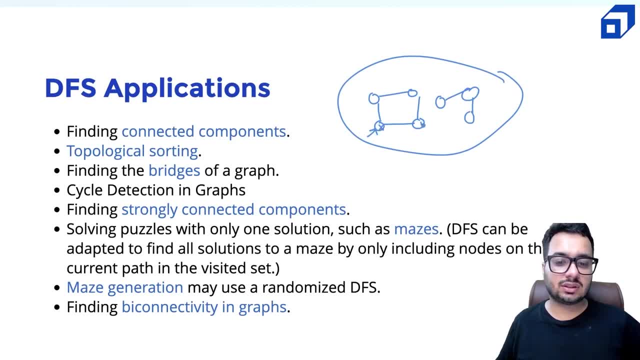 has two connected components. so you can do a traversal from this node, which will actually visit this whole component, and you can do a traversal from maybe this node, this whole component. so we'll do a separate tutorial on connected components. topological sorting: it can be used. it is also used in finding out bridges in a graph cycle detection. it can be. 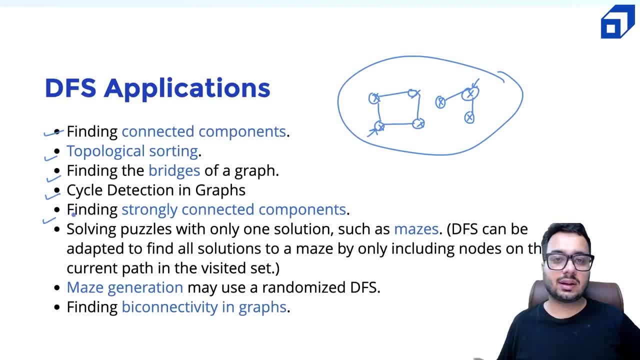 used. we'll look at cycle detection in this tutorial. strongly connected components is a different concept which is used in directed graphs. so dfs again is used there and it can be used to solve puzzles with only one solution, such as mazes. if you want to find out a path. 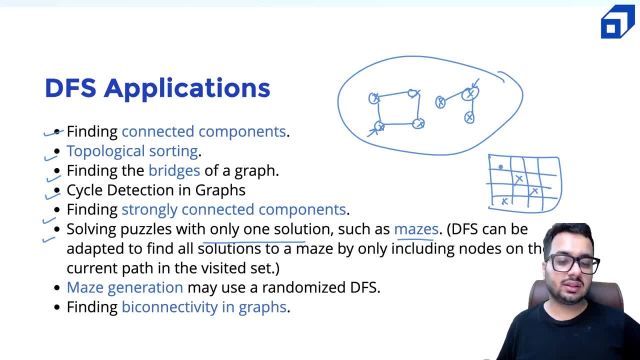 maze. maybe there is only one solution so you can easily use dfs along with backtracking to find out that particular path. it can be used in maze generation with the randomized dfs algorithm and it can also be used in finding by connectivity in graphs. so let us try to understand the algorithm. 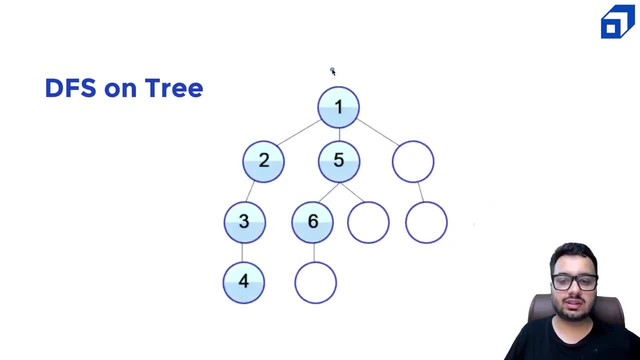 next. so dfs can also be used on a tree. so if you have this tree, so what this dfs will do will? it will start from, let's say, root node, it will go in this direction and here, here, here, then it will backtrack and it will enter into these branches. 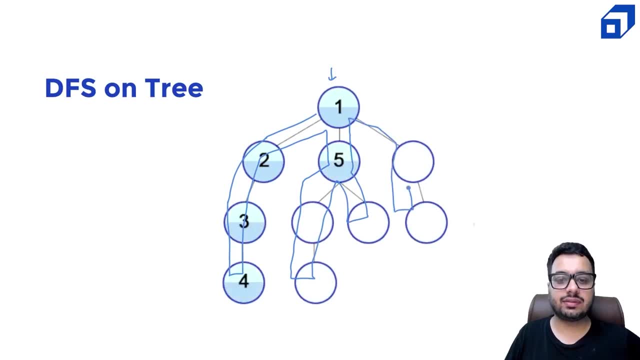 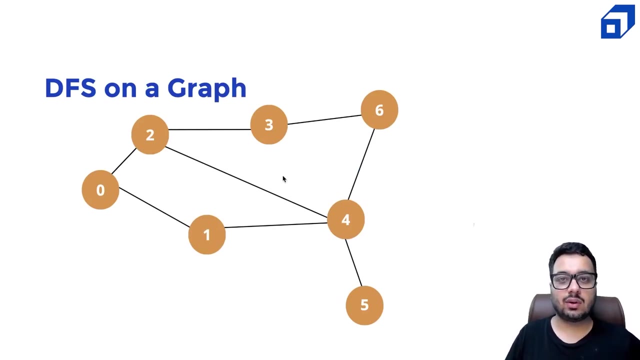 so it's just like a pre-ordered reversal that we have done on trees, but in case of graphs, the situation is little different. why? because graphs can contain a cycle, so we have to see what to do in case of a graph. let us try to understand, with the help of this graph, how dfs will actually work. 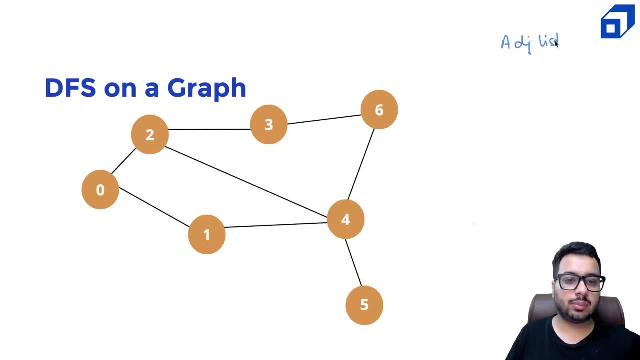 let me draw the adjacency list as well. that will be input and that is how the graph is actually, but this is how it looks like. so we have to add these two symbols that went from 0 to this one. with 0, we have the neighbors which are 1 and 2. with 1, we have the neighbors 0 and 4. 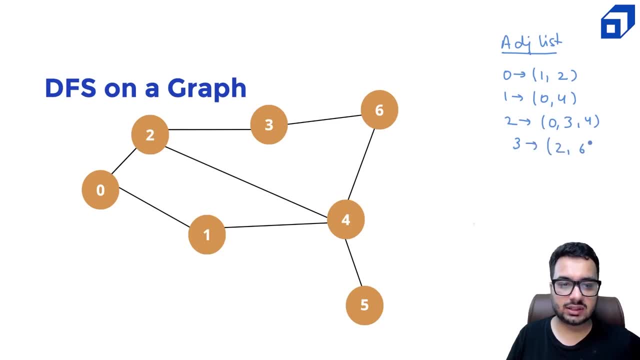 with two, we have the neighbors 0, 3 and 4. with 3, we have the neighbors 2 and 6. with 4, we have the neighbors 1, 2 and 6- 5. we have only one neighbor, that is 4 in the list of the graph will look like: now we need to understand how this df is actually going. 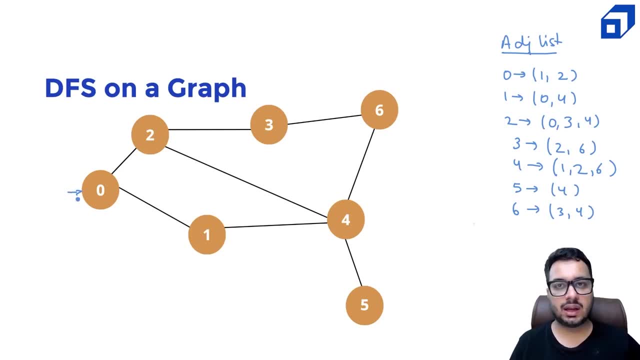 to work. so we are going to start from this node. it can be any node, so i'm going to take 0 as the starting node from the source node. and now, since the graph can can contain a cycle, i need to maintain a visited array. so i'm just drawing it here. so initially, nothing is visited. so this is: 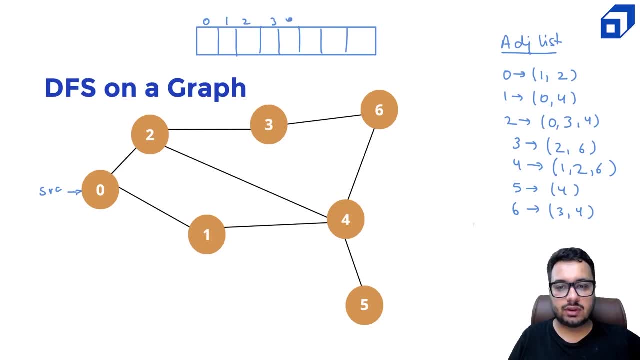 a visited array: zero, one, two, three, four, five, six. so i need this much error, right, i'll? i'll call it visited. this will help me to ensure that i do not visit the same node again. if it is already visited, we'll just backtrack, we'll go back. so i start with zero. i said: fine, i will mark this as visited. 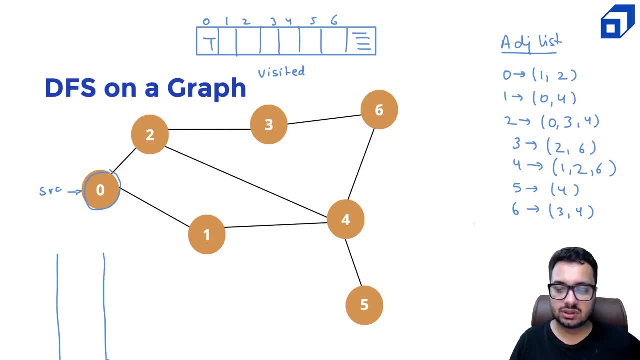 and since it's going to be recursive algorithm, so this node is in the stack. now zero can say: okay, what are my nodes? neighbors? neighbor of zero is one, so it will pick this node, the first node. i will try to iterate, but first i picked one and i will make a dfs recursive call on one, so i will go to this. 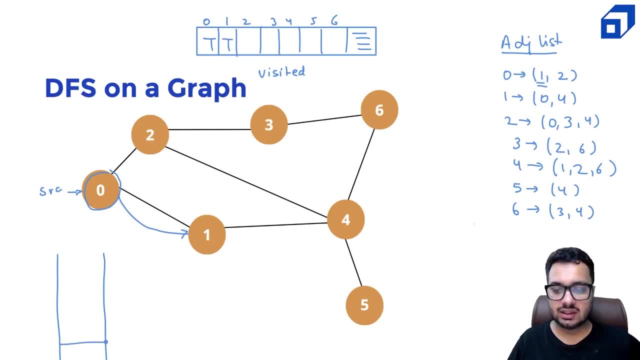 node, so i'll mark one as visited. the one is in the stack also. and now from one i can go to some neighbors, right. so once neighbors are zero, zero is already visited, so i will not go here, i will. if i go, i just come back, right. so i say, okay, this. 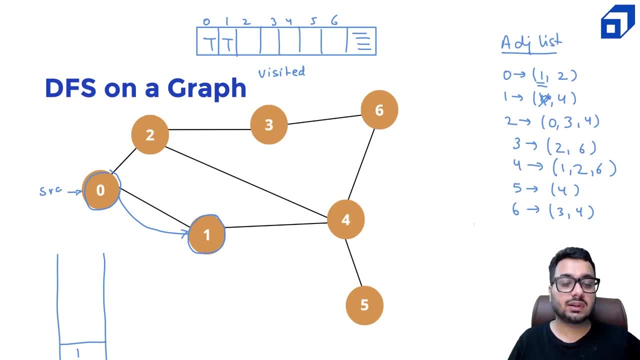 or i will not go. so this node is not visited. this zero is already visited, so i will not make a call. but what about four? four is visited, so i'm iterating on this list. so four is visited. right, so i may a. four is not visited, i make a call on four. 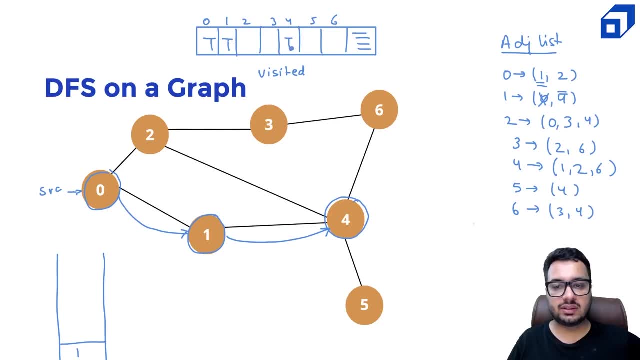 so i go and visit this node four. so four is marked as visited and four goes into the stack. so i think on the diagram you should also see a zero here before one. you have a zero right. so this, this portion got little cropped out from the screen. so zero one four. this is how the stack looks like. 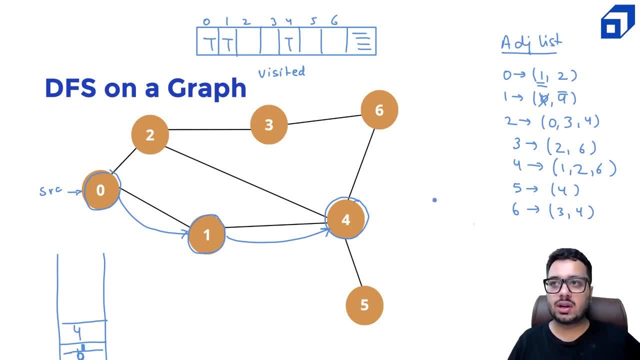 at the moment at four. i again do the same work. i look at what are the neighbors of four. the number of four is one, which is visited, so don't do any work. the neighbor is two, which is not yet visited. now what four will do? four will visit two. i'll go and visit this node, so two is visited. 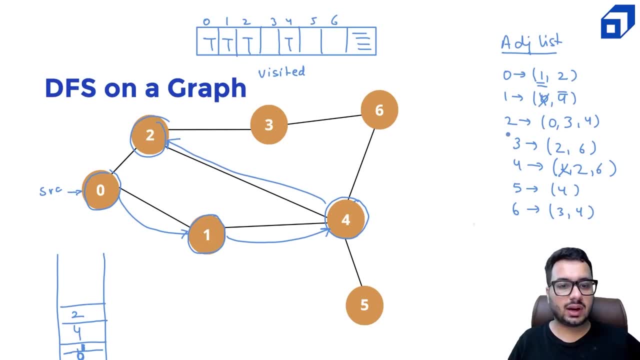 and two is now part of the stack. now at two, i look at what are the neighbors. the neighbor is zero, which is visited. the neighbor is 3, which is not yet visited. so i go to 3, this node, i mark this 3 as visited and i come to 3. so what are neighbors of 3? so it is 2 and 6. 2 is visited. i don't do any. 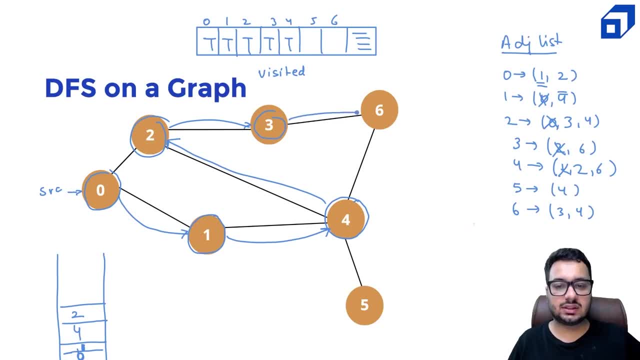 work. 6 is not visited so i go and visit 6. i go here. so 6 is marked as visited. so 3 is 3 is in the stack. 6 is in the stack now at 6. i look at the neighbors. the neighbors is 3 which is visited. 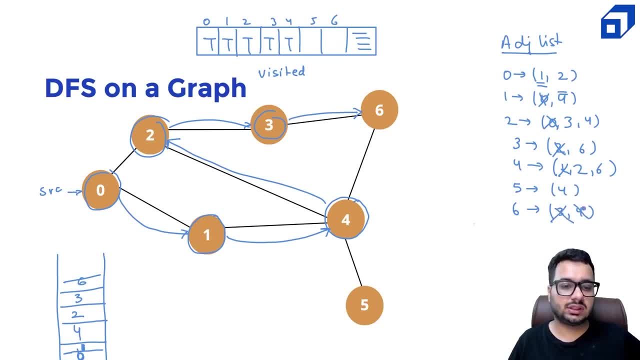 don't do any work. another neighbor is 4, which is also visited. so don't do any work now, what i can do. so 6 is already visited and 6 does not have a neighbor which is not yet visited. right, so what you will do? you will go back. this is important. so this is backtracking, so you come back at 3. 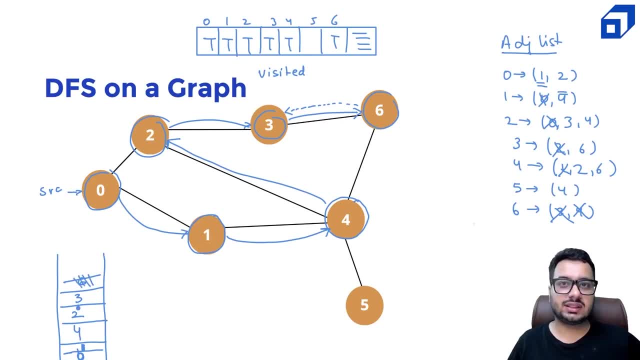 so from 6 you are now coming back at 3. so 6 is popped from the stack now at 3. you look at, i was running a loop. i was trying to traverse the neighbors and i already went and explored 6. this is over. so from 3 i cannot go anywhere else. this list is. 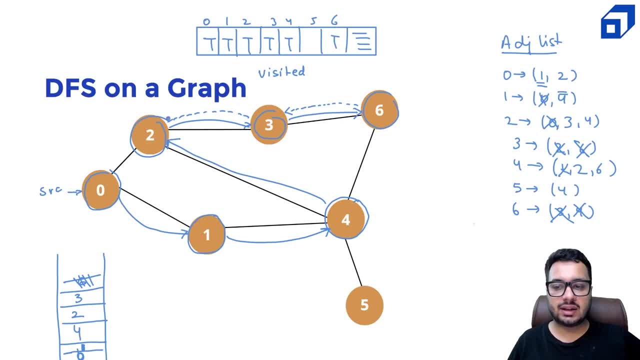 over, so i will just go back. i will backtrack. i will come back at 2. so at 2. i see, okay, i was at. i went to 3. 3 is visited. can i go to 4? 4 is also visited so i cannot go to 4. so 2's neighbor. 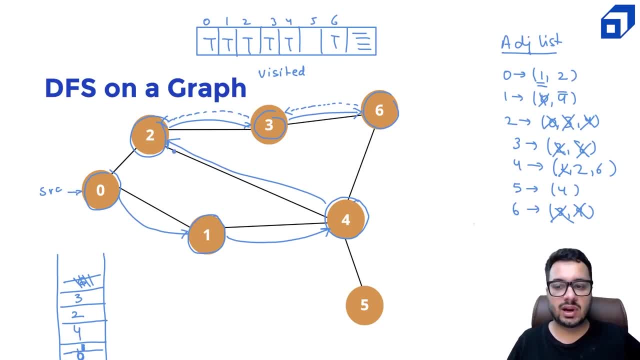 have been visited. so i can say, okay, just, let's just go back from 2. i go back to the previous 2. i i came from 4, so i come back at 4, so this is backtracking. now at 4 i can say, okay, i went to 2. 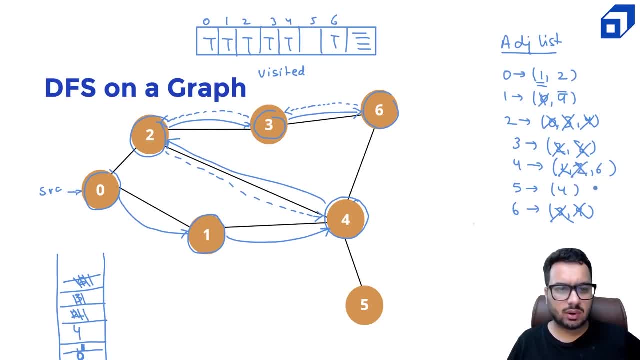 so 2 is visited. what about 6? so sorry, what about 5? this neighbor is 5, actually 4 has a neighbor that is 5, 4 has neighbors 1, 2, 6 and 5, 5 and 6- actually 4 neighbors. it has 1, 2, 3, 4. yeah, 4 has 4 neighbors. 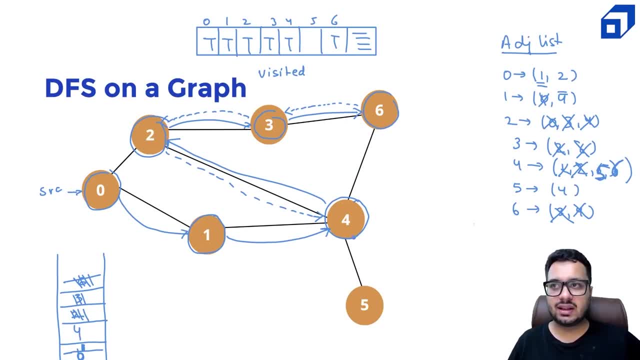 it will look at 5. can i visit 5? the answer is yes, i can visit 5. so 4 will make a call five and five will say: okay, i am visited now. so if i talk about the order, right, so it it was like zero one, two, three, six. and then, sorry, zero one, zero one, four, two, three. zero one, four, two, three. 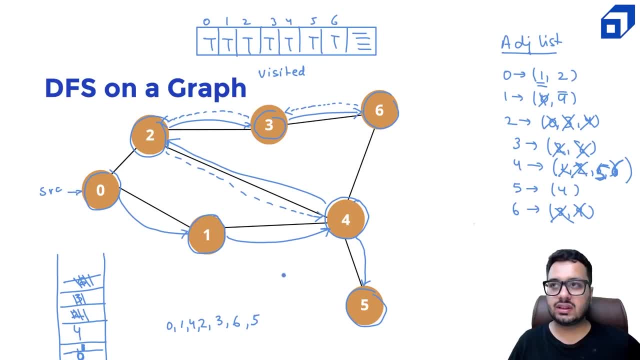 six. and now you are actually visiting five. right, you are now visiting five from six. you come back three, you come back to two, come back to four. and now four will say: okay, four has a neighbor, that is five, it is not yet visited. it will go and visit it. and five will say: okay, i can only go to four. 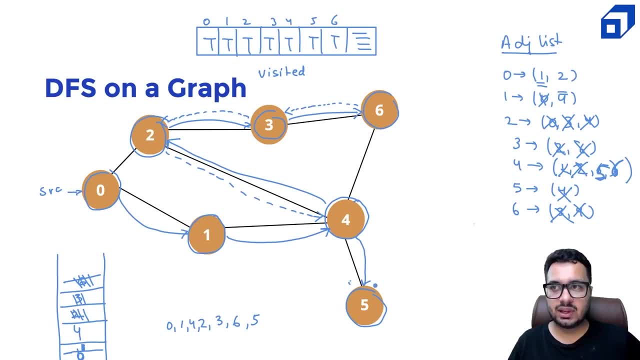 but four is visited, hence i will go back. it will simply return i. i go back to four. a force is okay. five is visited. what about six? six is also visited. six is not visited by four, but it is visited by three. it will not go to six. also, a force is. 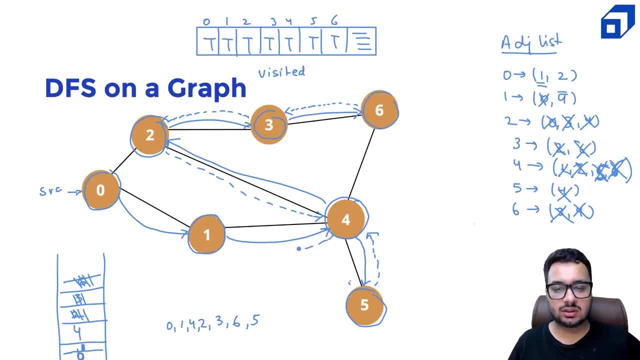 okay is okay, all my neighbors have been done. i will go back. it will come back at now. one. right, so here after four you went to five. five is over, four is over. now you come back at one. one says: okay, all my neighbors have been visited. now i will just pop, i will come back at zero now in the stack. 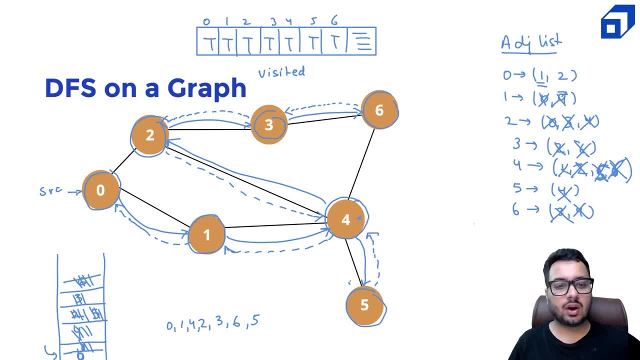 you are in this function zero. zero says fine, all my neighbors. one is visited. now zero looks at two. two is also marked visited in this array, So it says okay, my list is also finished, So I'll just go back. So this is also popped up from the call star. This is how the DFS algorithm works And given 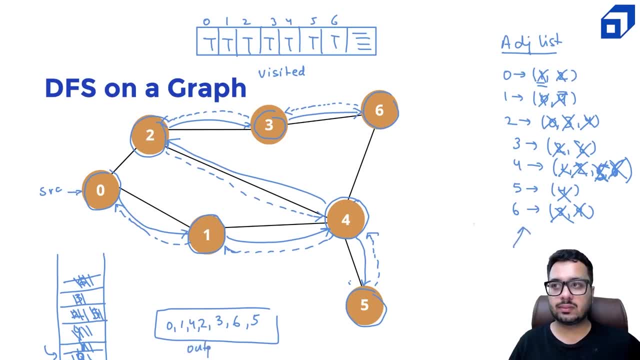 this adjacency list. this will be the output that we will get. So the idea was to traverse all the nodes, And this is what we will get by traversing all the nodes. I hope you understood the algorithm fairly simple. If the graph has multiple different components, then we 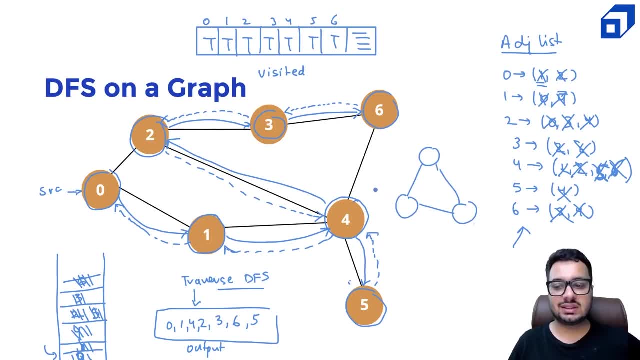 will see that you need to initiate DFS from one node in each component. Okay, so this is something easy that can be done later on, But first of all we'll focus on this simple DFS algorithm, where we are assuming there is only one component. Okay, so we are assuming. 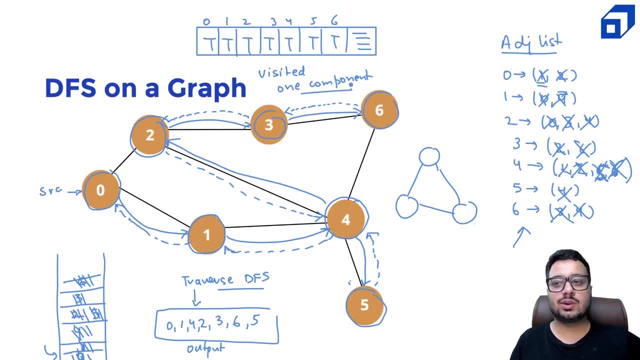 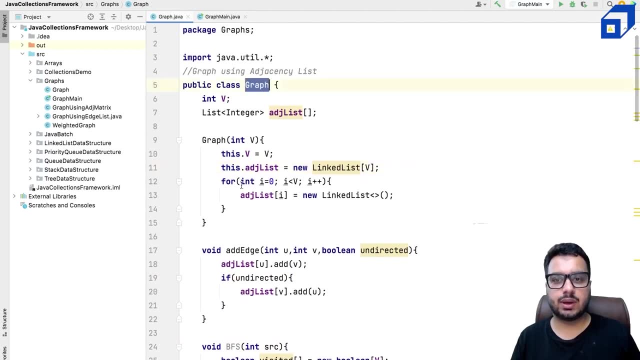 one component in the graph. as of now, Let us code this algorithm. Next, let us look at the implementation of DFS in Java. I already have the graph class, which is implemented in the previous tutorials. In this, I'm going to add a DFS method And 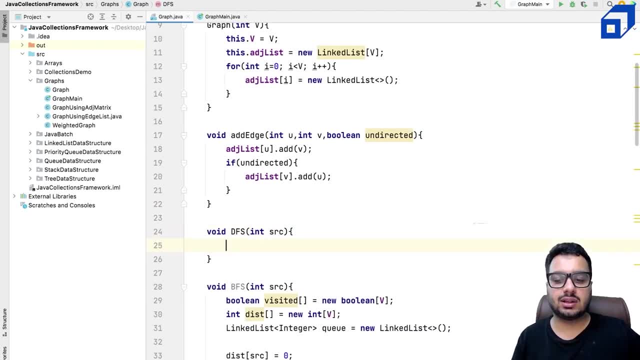 this is going to accept the source node from where I'm going to start the DFS. I'm assuming there is a single component in the graph. So what I need to do? so, firstly, I need to build a visited array. that is the data structure we will be needed So we can keep thinking. 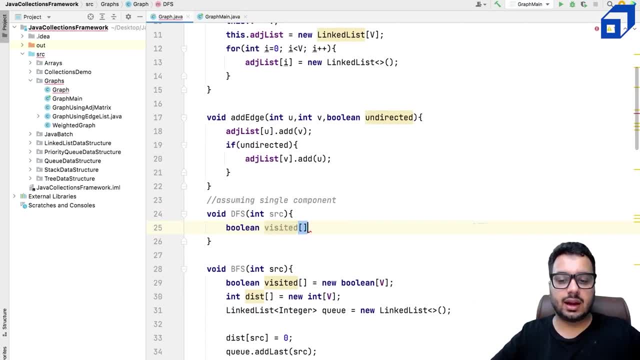 about this simple. we can create a boolean visited array and this is going to be of size v, that is the number of vertices in the graph. so initially everything will be set to false and in java, by default a boolean array is false. now i actually want to do this traversal recursively, so i cannot make this. 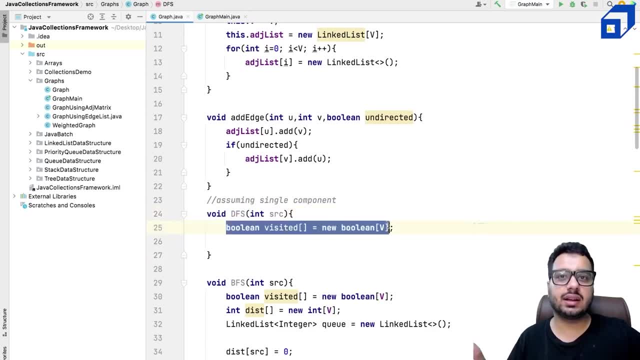 as a recursive function, because i cannot create this array again and again in the recursive function. so what i want? i want this array to be shared across all the function calls that i'm making so for. that is why i need to create another function which is going to help this dfs. i can 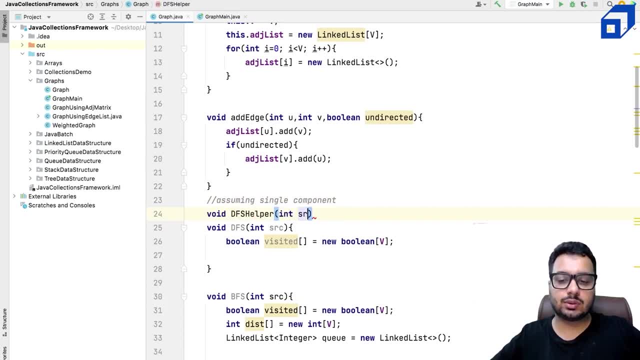 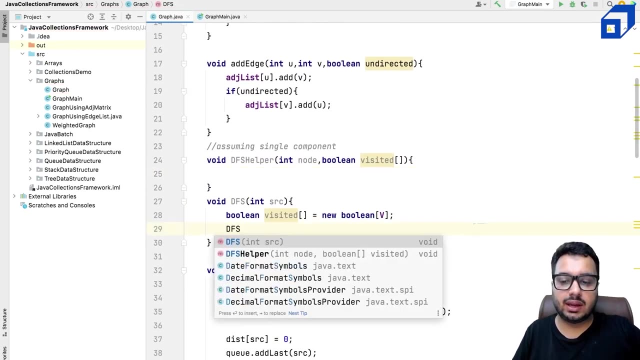 call that as dfs helper, and here i'm going to get the source node, or the node, the current node where i am, and the boolean visited array. so this array will be passed and it will be shared across all the function calls- right, you. so i can simply make call to dfs helper and i can give source node and the visited array. 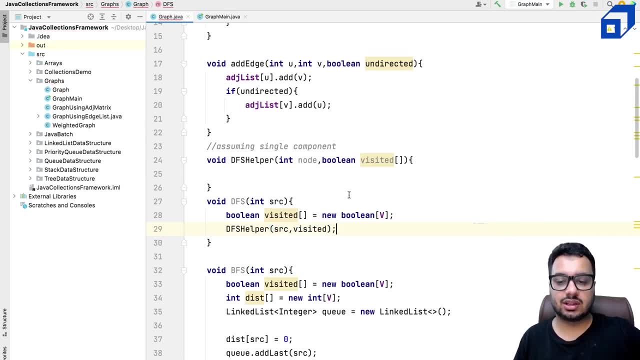 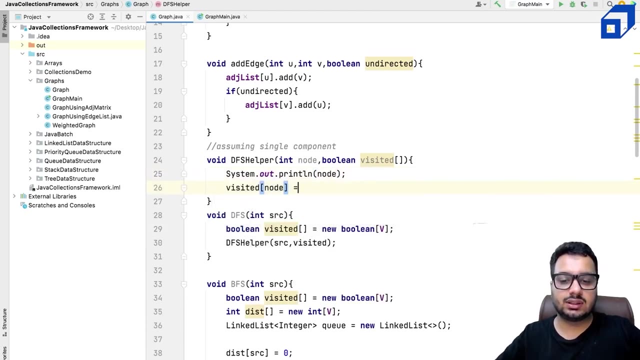 as input to this function right now. here what i need to do: as soon as i come to a node, the first thing i will do is i will mark that node as visited so i can- okay, i can print out that node, that is fine, and i can say: visited of that node. this is equal to true that, yes, i have visited this. 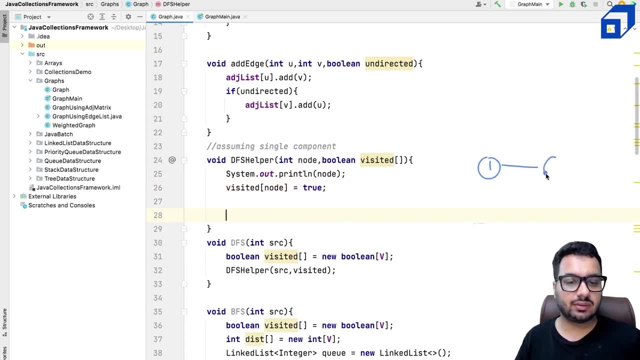 node. that is fine. let us take a small example. let's i have one, two, three and four and five. let's say this is the graph. so if i start from this note, so i will mark this as visited. now i will look at neighbors of one, so one's neighbors will be, let's say, two and four. 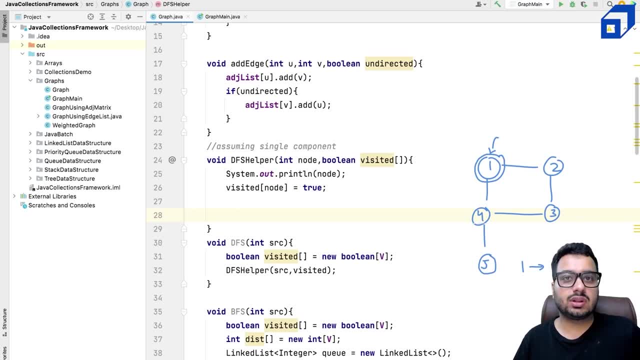 so i'll iterate on this list and i will go to the neighbor which is not yet visited. so right now two is not visited, so i will make a call to two. okay, so how do i do it? and that one is gonna be visited and i will make a call to on, probably between I'm getting two. 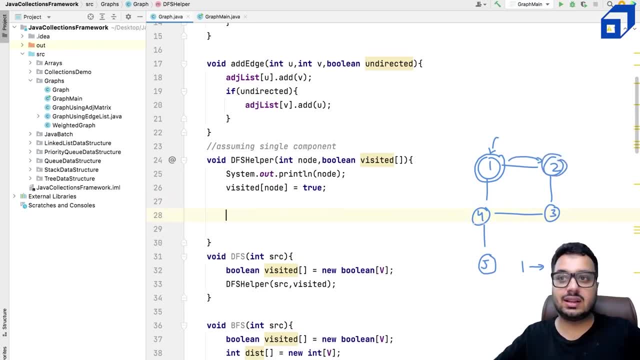 Okay, so how do I name this? mc isame was doing this plus and it has been changed to, and that's maybe what I have to do now. okay, so how do i do it? to iterate on this list? we need to create a list iterator. i think this. 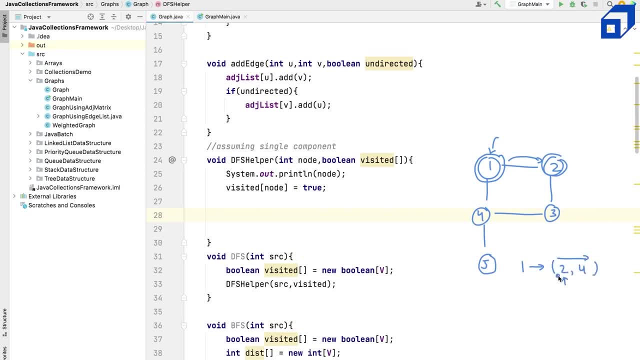 part was not visible, so i'll just hide myself. what i'm saying is that one has neighbors two and four, so i'll make a call at two first. so how do i get that? for that i need to create a list iterator first, so i can say: fine, let us create a iterator. iterator. 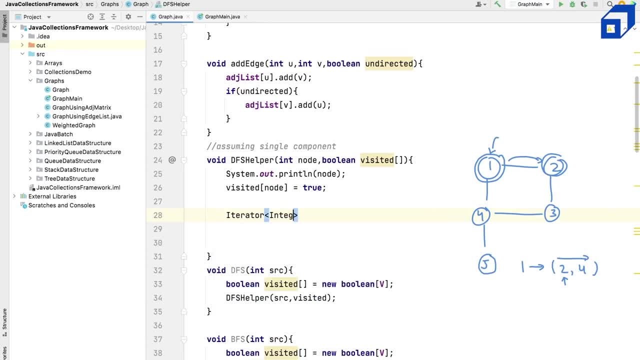 of the type integer- let's call it it- which is the iterator to iterate on this list. so i can say, okay, adjacency list of this node which is, let's say, zero source, in my case dot list iterator. so using this iterator, we can easily iterate. so while i have items in this list, while it dot. 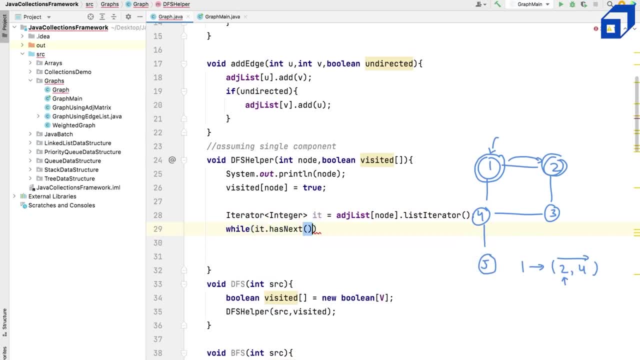 as next what to do, i can, okay, give me the neighboring node. so the neighboring node, this is given by it dot next. so i will now check. is two not visited? yes, two is not visited. so how do i check? i check from the array. so two is not visited. 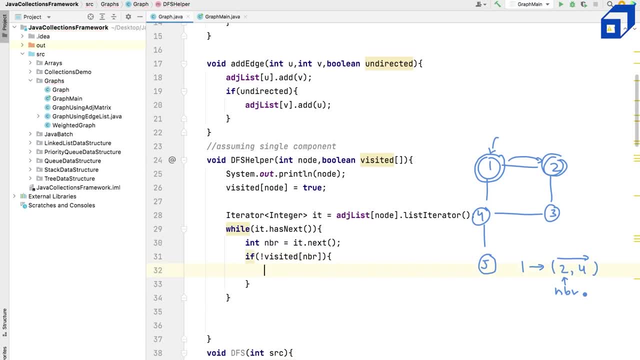 neighbor, then what to do? i have to make a recursive call so i can make a call to dfs helper. give it the node- the node is neighbor- and give it the visited array. i'll show you what's going to happen in this scenario. so i have this. let's say one, two, three, four, five. 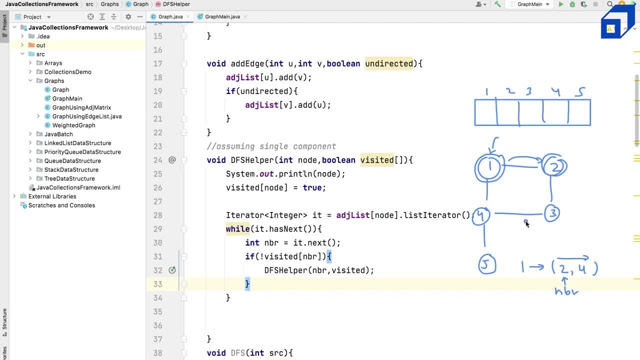 so generally in in the code the indexing is assumed to be zero based, but in the example i took it one based. but hopefully you will understand that part. so i check. one is connected with two and four. so two is not yet visited, so one is visited. so as soon as i get 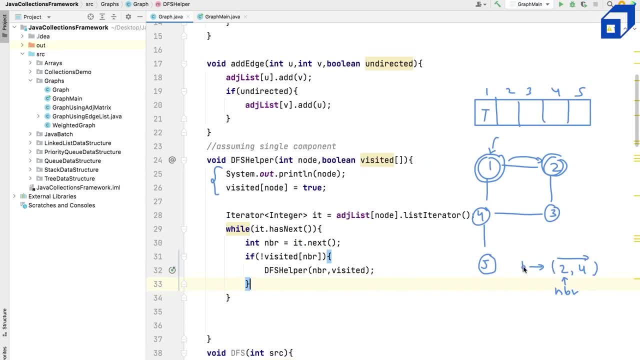 come to one, I mark one as visited. then I iterate over the neighbors of one. I check two is not visited. I make a function, call on two, So two is now visited. Now I look at neighbors of two. So two has neighbors, which is one, and three Out of this, one is: 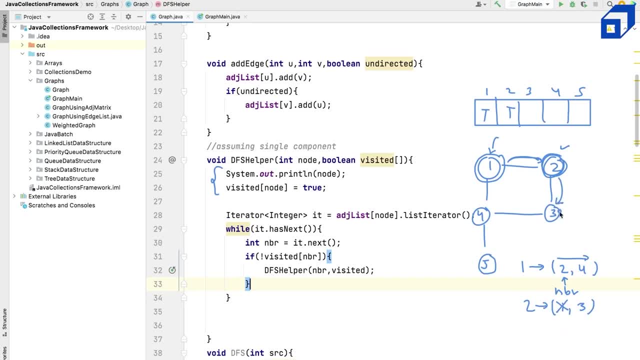 already visited, So I don't do any work. So I'll make a call at three As soon as I come to three. three is visited And three has neighbors again two and four. Three looks at: okay, two is visited, So I'll make a call at four. At four I have again neighbors which 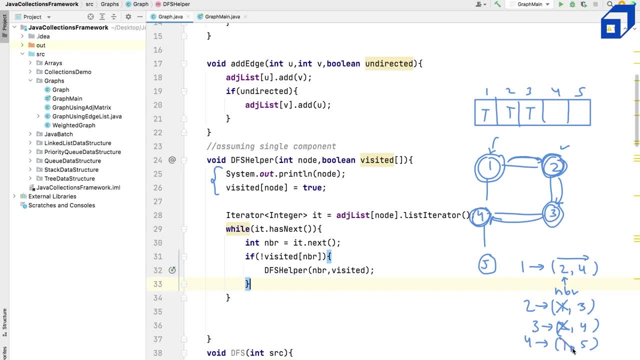 are one and five. So four says: okay, one is visited, don't do any work, make a call at five. So four visits five. So five is now visited. Now five has only one neighbor, four, which is visited. So this loop will not run for five, because it will iterate over the 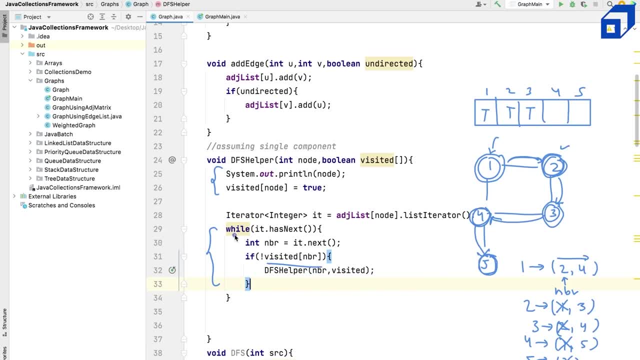 neighbors. So three is visited on four and four is already visited. So this, if will not execute and while will not do any work, so you will simply return it from here, we will come back. So you come back here At four. you see, five is done. The list of four is. 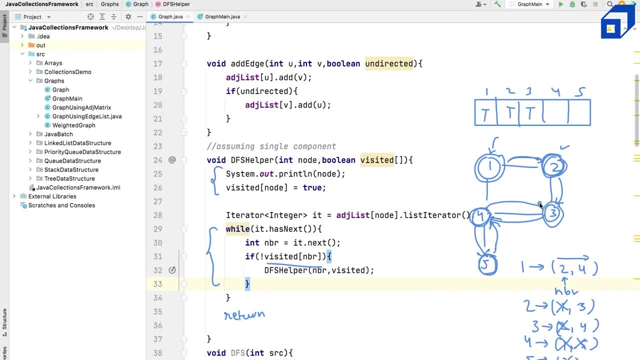 also finished. So this loop is over. four goes back to three. Three says: okay, I can go to four. this is also done. So three: these loop is also over. you go back at two. you have gone to three. that's also done. 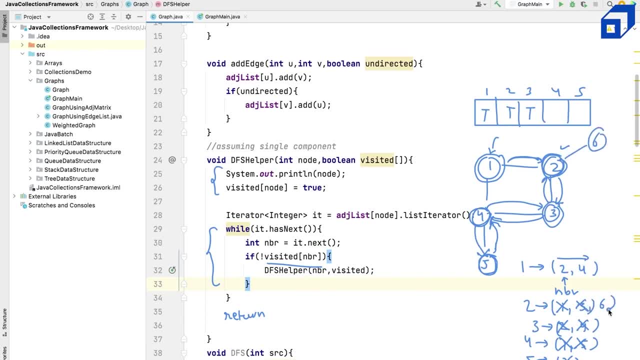 Suppose there is a node, six here, right. What will happen now? who will say: okay, yes, I can go to six, the two will go to six and six will get visited and you will come back. And of course, these: 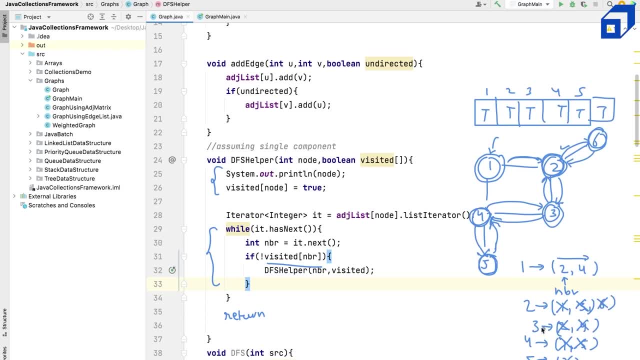 nodes are also marked visited. This loop is also now over. Now at two you will say: okay, my list is done, I will go back. it will go back here. One will look at: okay, can I go to four, but four is already visited, Hence you do not go. you do not make a call at four. 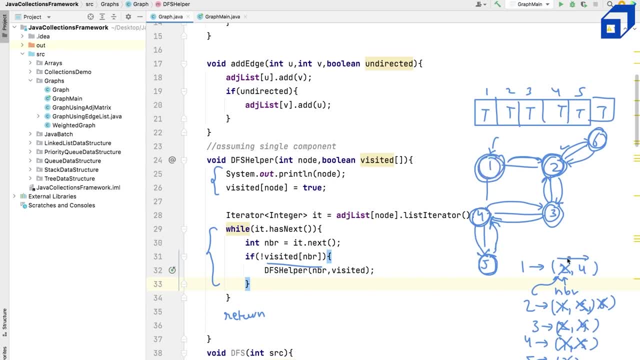 So this edge is not considered, And at one you can say: okay, this list is done, because four is also visited And hence I go back. This is how it will go back into domain. So in this case the output would look like 12345.. And then you have gone to six as well. This is how the DFS is going. 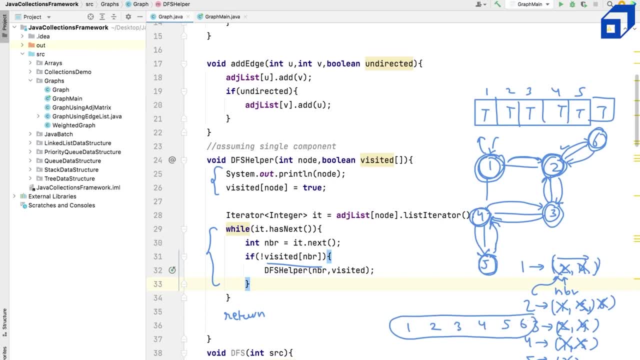 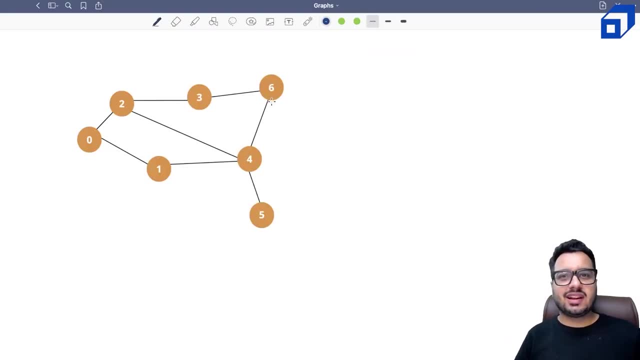 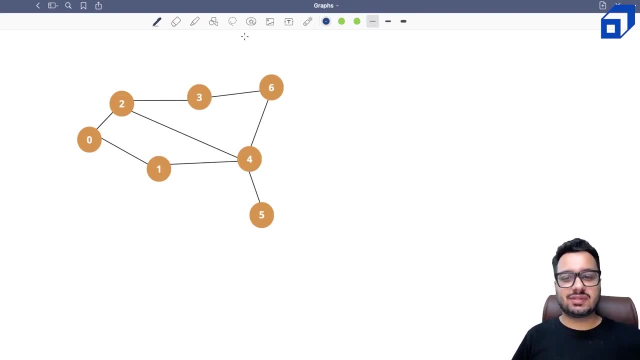 see what happens. So let's start with our code. The next thing we will learn is how do we do cycle detection on graphs. Basically, we will do this algorithm of cycle detection on two types of graphs. One is on undirected graph, which is given here, And secondly, we will do it on directed. 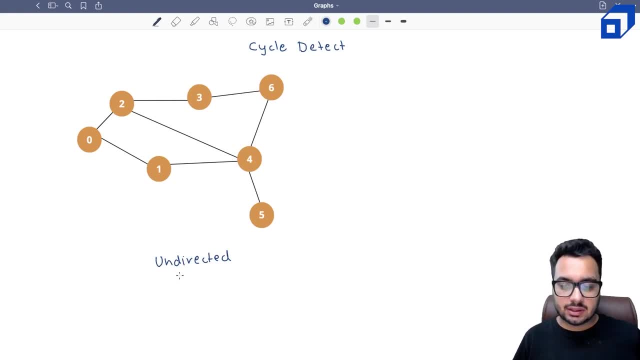 graphs in which the algorithm will change a little bit. This graph is an example of an undirected graph. Now, how do we detect a cycle in this? I can use BFS or DFS, Right, Right, you remember? the fundamental difference between a tree and a graph is that a tree is always not. 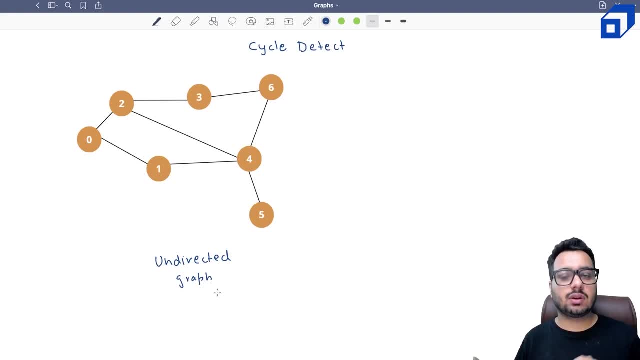 containing a cycle tree does not contain a cycle, but every tree is also a graph. basically, if you have a cycle in a tree, it becomes a graph, right, and every tree is also a graph. so if i give you an example, let's say this is node a, it is connected with b and it is also connected with c. 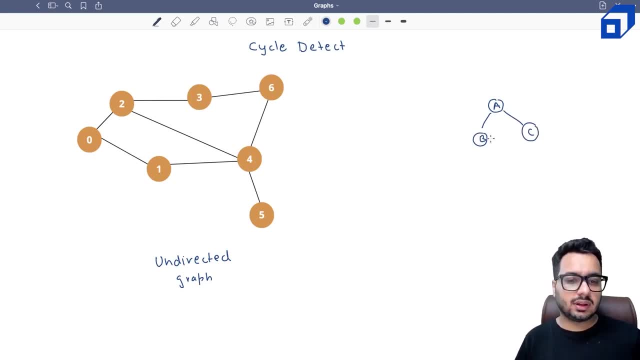 so right now it is a tree, right, and it is also a graph. but if i add this edge, it definitely becomes a graph, right, it is not a tree now because it contains a cycle, right. so now, what is the significance of cycle, or how do we detect a cycle? so it is pretty easy. let's say i start traversing. 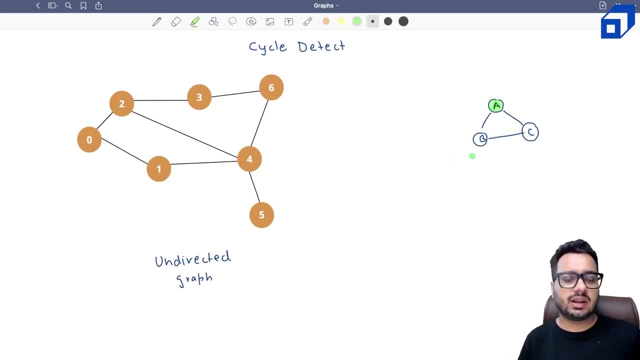 this using any algorithm. it's a bfs or dfs. let's say, start with a and i make a dfs call on its child that is b at b. i make a dfs call on its child c and c will now look at its neighbors, it will see, okay, i. 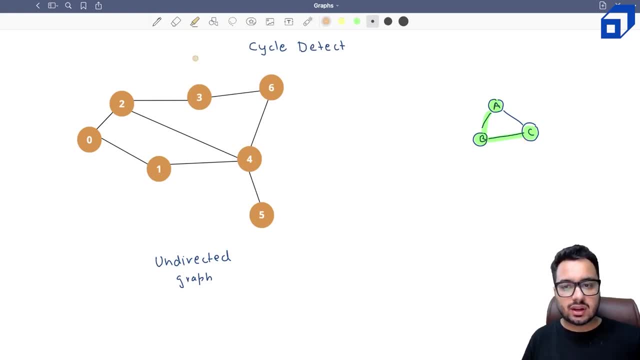 discovered a neighbor right now. c has two neighbors, so one of the neighbor is, let's say, b right. so if c looks at b right, b is already visited. but is it really a cycle? the answer is no. i cannot say that this edge is going to create a cycle. the answer is no right. let's say there is one more edge. 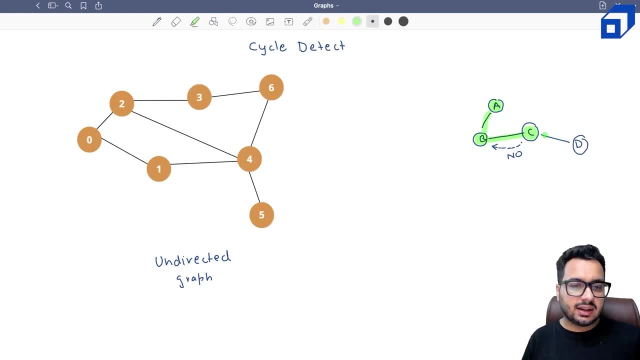 from c to d. c makes a call at d and it visits d. is this edge causing a cycle? basically, the answer is again no, right. so what is the difference between this edge, this edge, right, basically, before visiting d, d was undiscovered, he was not visited, but b was discovered. b was 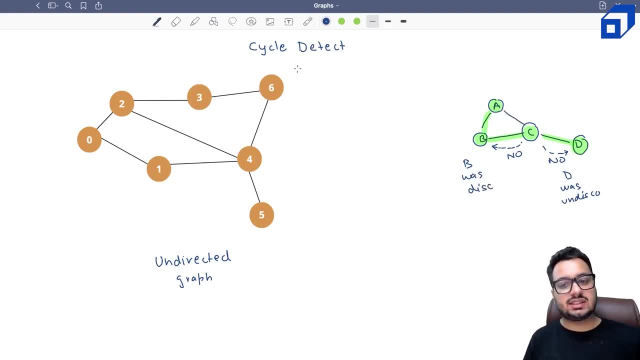 discovered. now suppose i create one more edge, which is this edge right? so if i now see makes a dfs call on, let's say, a right, but as soon as i make this call, i see okay, i'm landing at a node which is visited and i can say it is a cycle right, it is a cycle right. 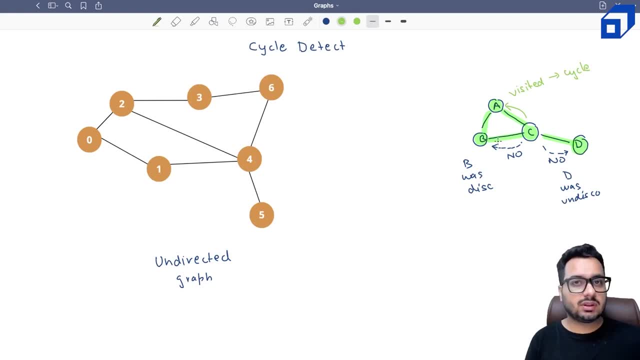 basically, what i'm trying to say is that b was also visited, d was not visited. so here we are sure there is no cycle. but here the answer is no, because b was discovered but it was parent of c, it was parent of c, it was parent of c, whereas from c when you go to a, a was already visited. 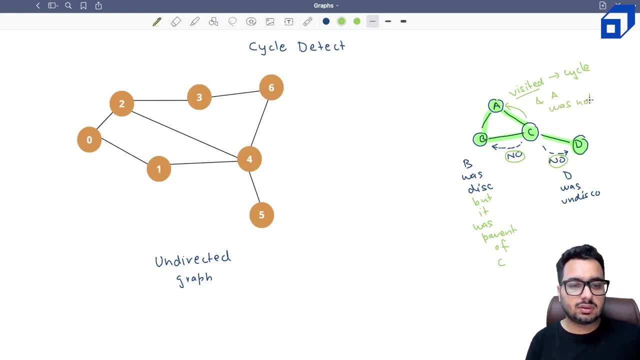 and a was not the parent of c. a was not the parent of c in the dfs call. so this is the condition that if we encounter a node which is already visited and it is not the parent of the current node, then we can definitely say yes, there is a. 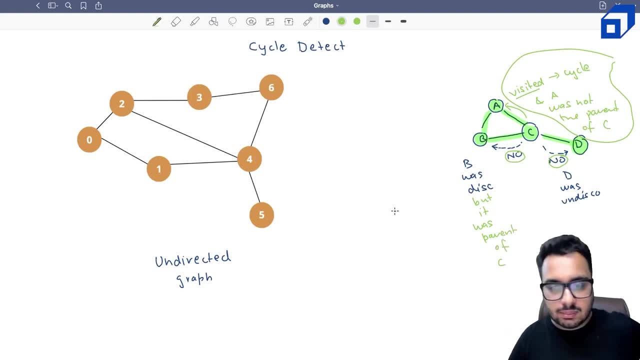 реvey, which is already visited and it is applying, say that we go to throwing about the other node, the redundant ok expression in dfs. then as soon as we add and before we use put string, we have to float with at the end of this row and so that we get there. 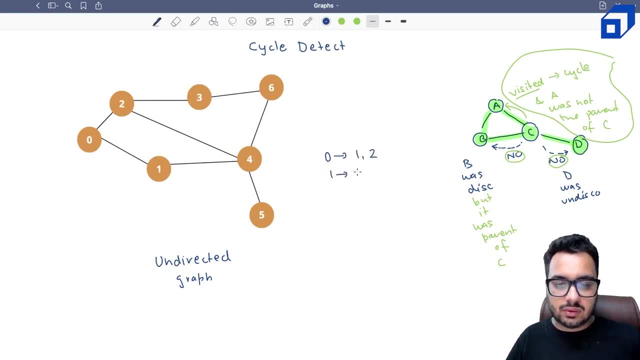 we can also add another friend, which is also a word we know it would be if y, if y is thought to be the spirit of the speaker, 모바일 Sahara. we are told that for the secret that you get connected with one, two and six, then five is connected with just four and six is connected. 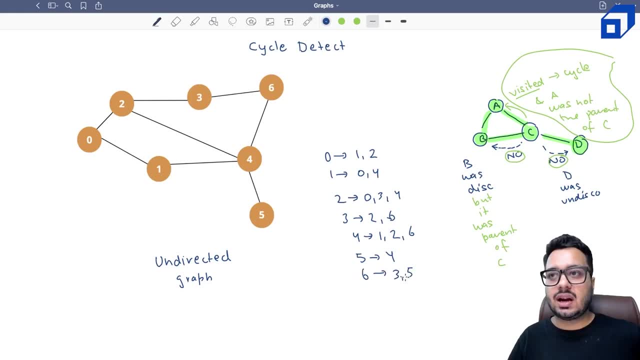 with three and five. right now, suppose, i start doing a dfs from node zero and i want to check if there is a cycle or not. so i start from this node zero. i said, okay, go and make a call at its neighbor. so one is the neighbor. it is not visited. so right now my goal is to iterate on this, but i 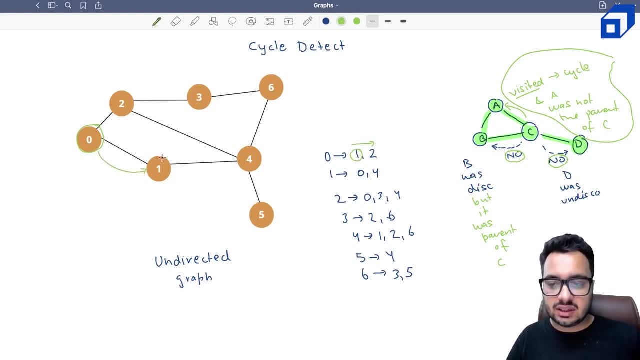 make a dfs call on the first node that is not visited. so one is not visited. i go here now at one. i look at the neighbors. the neighbor is zero, but if you look at zero, zero is already visited. zero is visited, but zero is also the parent of one. so hence we have to skip this node. we will not. 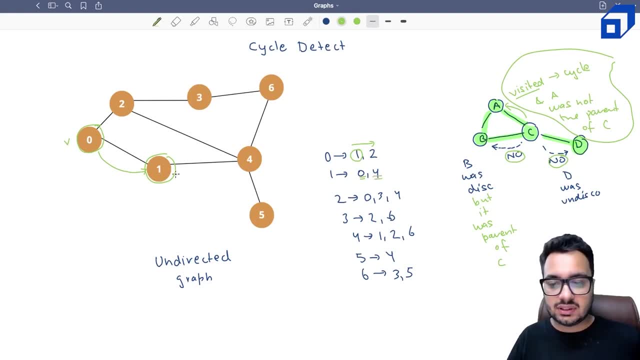 do anything at zero. what about four? four is not yet visited, so i go and make a dfs call at four right now. we come at four. four is now marked. marked as visited. one is visited. zero is visited. four's neighbor is one. so i will not do any work like c's neighbor. 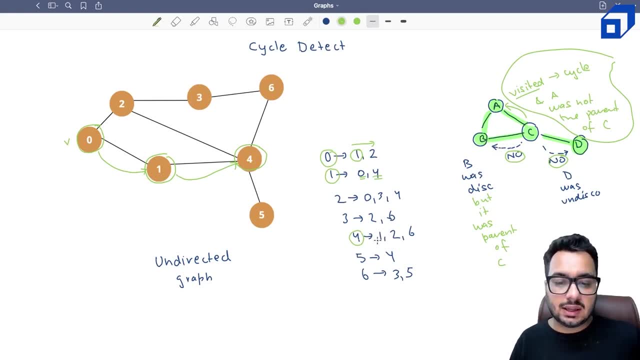 is b, b is visited. four is one is visited, but one is parent, so we will skip it. what about two? two is not yet visited, so i can go at this node and i can mark it as visited right now. look at two. now two has a neighbor, so i can mark it as visited. so i can mark it as visited. so i can mark it as. 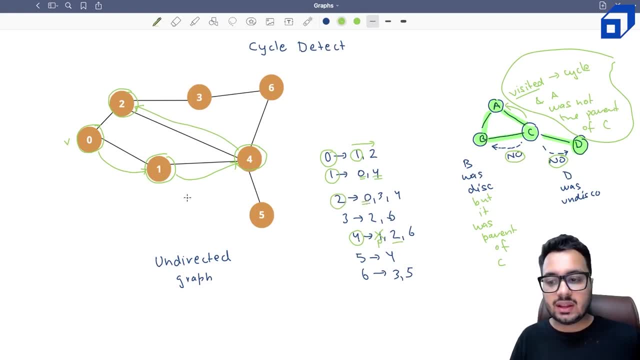 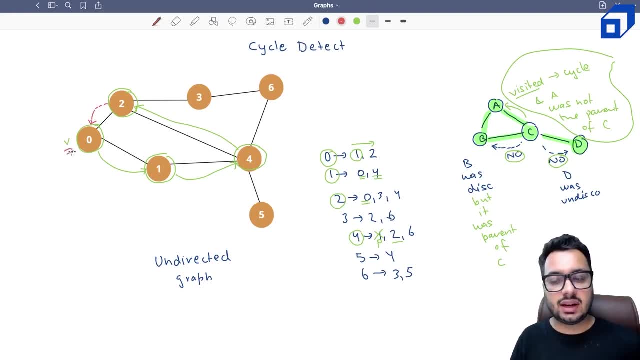 what is the condition at zero? zero is already visited right, and zero is not the parent of two, right. so basically, you're hitting this edge. we will call this edge as a kind of a back edge, right. so it is taking us back in the same path, from where we. 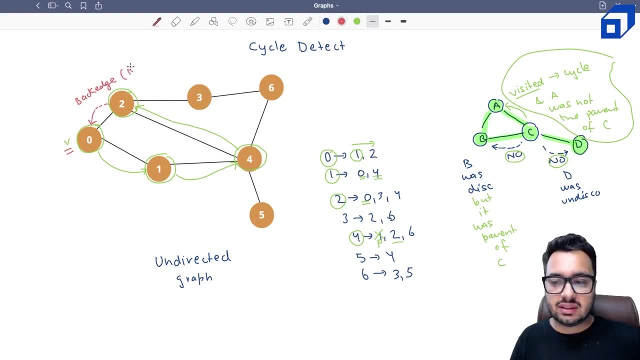 started or to one of the ancestor nodes. okay, so it is an edge from the current node to some ancestor node. why ancestor? because, if you look at, the path that we have traced is zero, one, four, two, and then from two we are going back, we are going at zero. this is like a back edge right as soon as 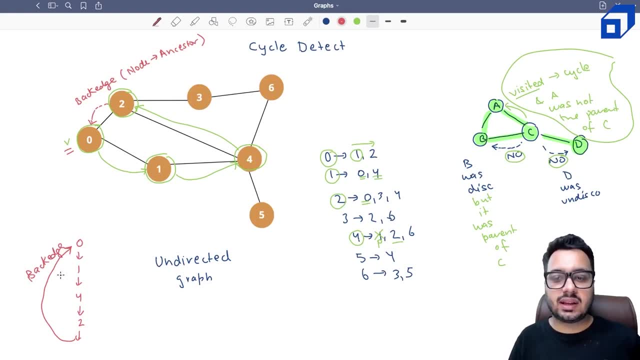 i get this edge, it will be the terminating case right. so at this point i can directly say, without looking at the rest of the graph: yes, there is, there is a cycle, so this is going to return true. okay, so i'm going to say, okay, i'm going to return a true from this node two. so this true. 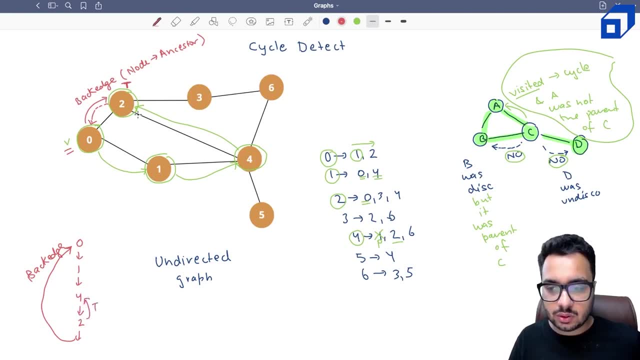 will be told back to four: okay. so two will say, okay, that, yes, i found a cycle. okay, so what? four would have said that, okay, i do not see a cycle in my. i am not seeing the cycle as of now, but let me call a neighbor and check if it can discover a cycle. so two discovered a cycle. so that true is. 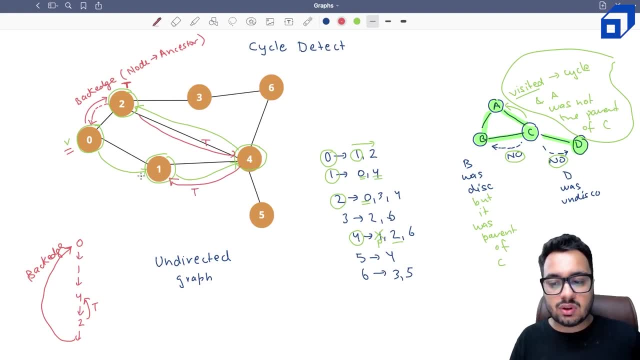 returned to four, four will also return true, one will also return true and zero will also return to right, because it's going to be a stark based algorithm. so this true will be propagated back to the main in this manner, right? so there will be a base case, there will be a recursive case. let us 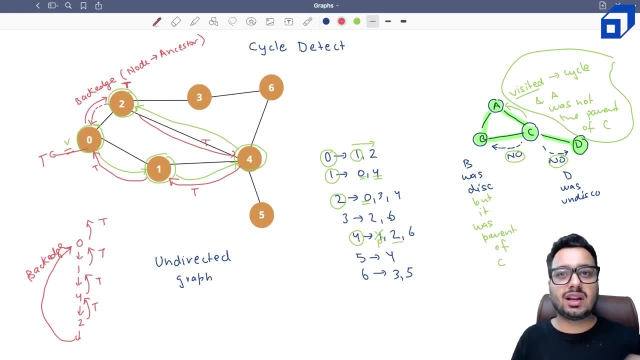 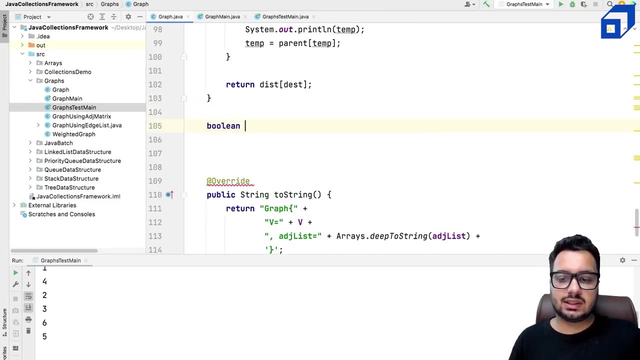 try to write the code and understand this algorithm in little more detail. so let us write the code for our cycle detection. so i'm going to make a boolean method which is, let's say, detect cycle, and here i need to give some source node from where i want to start. right, or you can take zero as well, right? 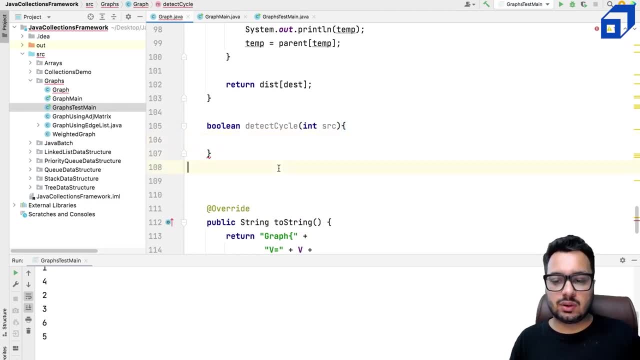 so we are assuming that the nodes are numbered from zero and, uh, we can ignore this source. we can directly give zero as well, right? so now, since it's going to be a recursive function like dfs, right? so one thing we did in dfs was maintained a visited array. so we here, we also need to maintain a visited array that will tell: 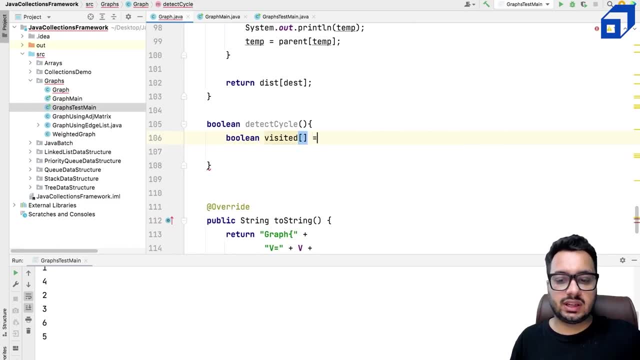 whether a node has been visited or not. so boolean visited, this is equal to new boolean and the size is, let's say, v, right? so by default this visited array is set to false in java, so i'm not explicitly setting it and here i can say: okay, i'm going to create a helper method: detect cycle- helper. 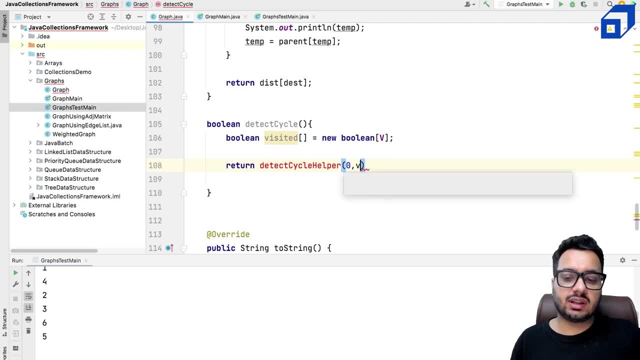 and i'm going to give it a node, let's say zero, and i'm going to give it the visited array, right? so this is. this method is just like a wrapper function, because we need to create the visited array and this needs to be shared across all function calls. so we are going. 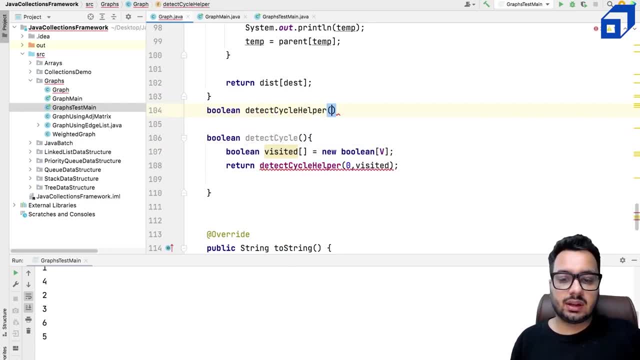 to make a helper method, boolean detect cycle helper. it's going to accept the node and second thing it's going to accept is the boolean visited array. so now here we will return some true or false. let's see how this is going to be. so, first of all, when you are encountering a node for the first, 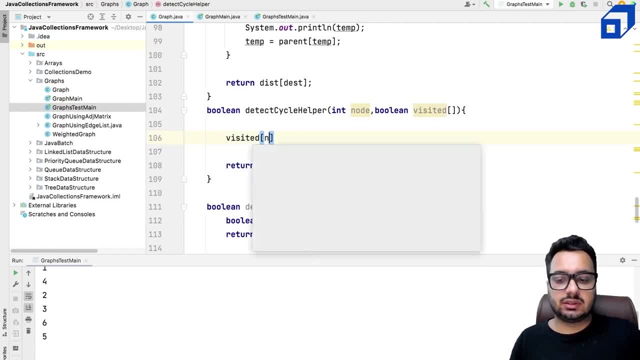 time. so definitely you should mark that node as visited. so visited of node this is equal to true. next thing you will do is you will iterate over the adjacency list of that node and you will make recursive dfs calls. right, so let's see how we can do it. so, just like before we have done here, right. 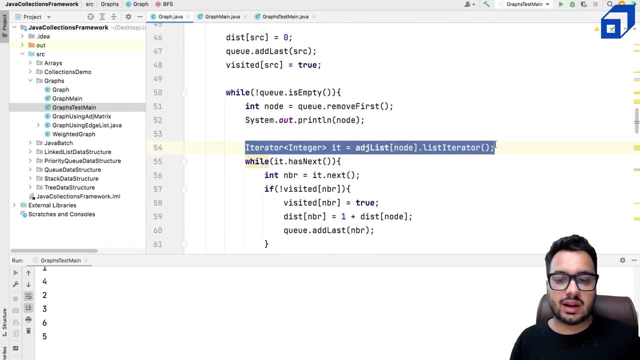 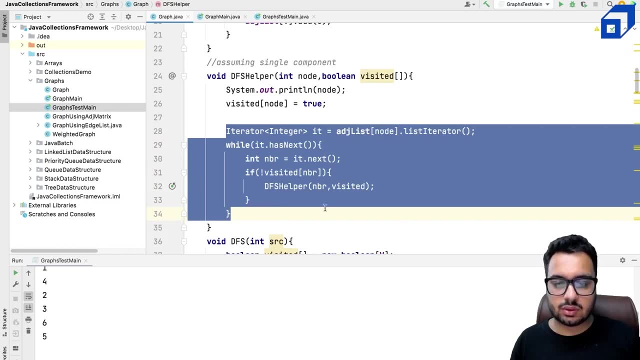 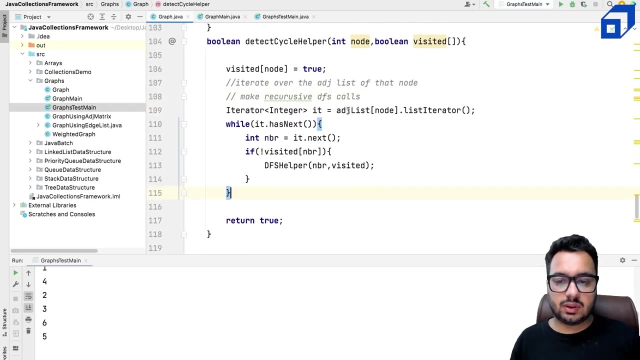 so i'll show you. so you will create a iterator to iterate on that node, right? or like in dfs, right, something similar we will do, right? so i'll just copy this node code and i'll show you what modifications you need to make in the dfs code. right? so here we go. so we have created an iterator. 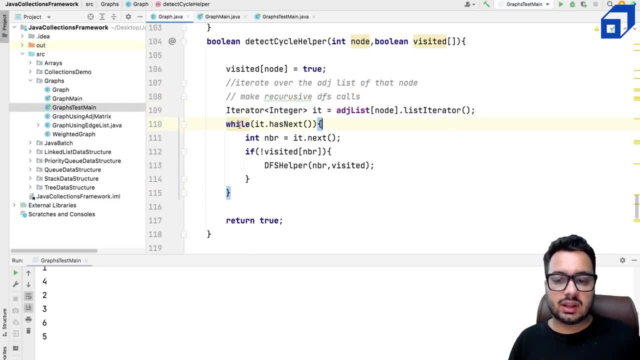 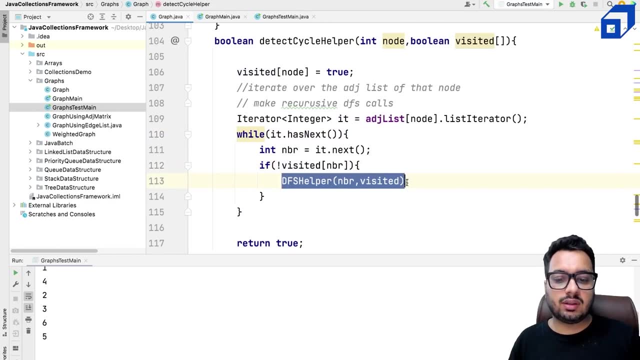 to iterate over the adjacency list of the given node. and then what i'm saying? i'm finding out the neighbor right. so if the neighbor is not visited, let's say. if the neighbor is not visited, let's say that neighbor is not visited. okay, now here the call will be different. okay, so if the neighbor is. 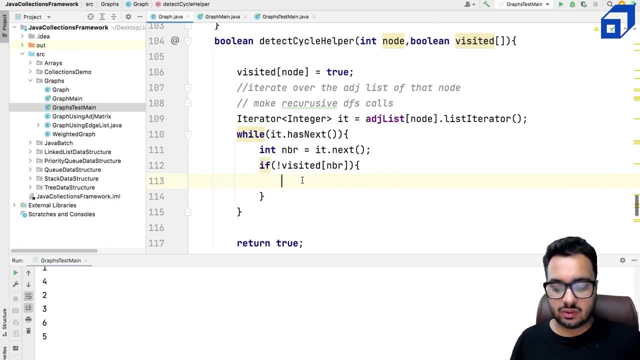 not visited. i will go and visit that neighbor and i will also store the result, what that neighbor is saying. for example, let's say one is connected with 2, 2 is connected with 3, 3 is connected with 4 and 4 is again, let's say, connected with 1. right, so i will make a call at 2. that is the neighbor now. this: 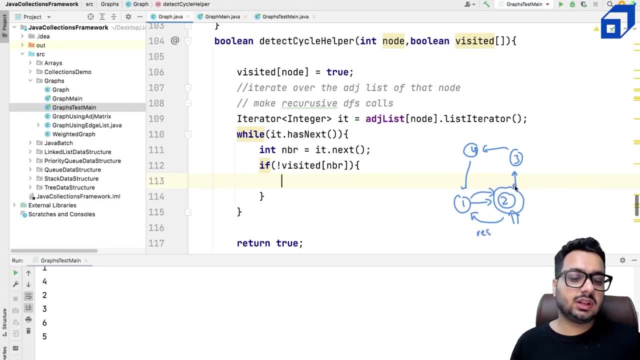 2 is supposed to return some result back to 1. right calls, two might have called three, three might have called four, four might have called one. oh, and here it saw, yes, there is a cycle. so, true, true, true, that will get propagated back right? so if the neighbor is not visited, definitely we have to go and check that. okay, yes, is there a cycle at. 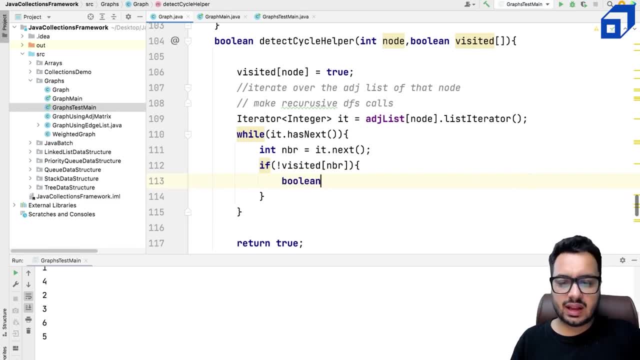 that node or not, i can say okay, boolean, i can say cycle found, it's something like this. so they did find a cycle in in in that part of the graph, right? so here i can make a call to detect cycle helper and here i can give the node which is going to be the neighbor and i'm going to give the. 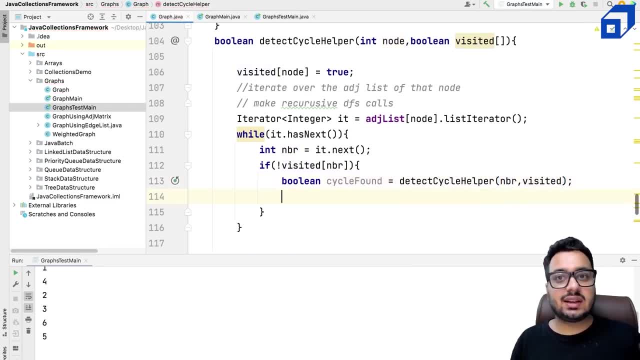 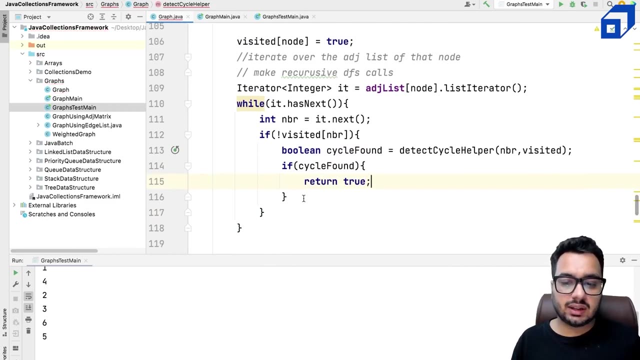 visited array. right now this is like a recursive case. you called some node. that node said: yes, i found the cycle. if the answer is true, if cycle found is true, you can directly return true from this point without iterating on the remaining adjacency list of the current node right. and there is one more scenario that can happen. 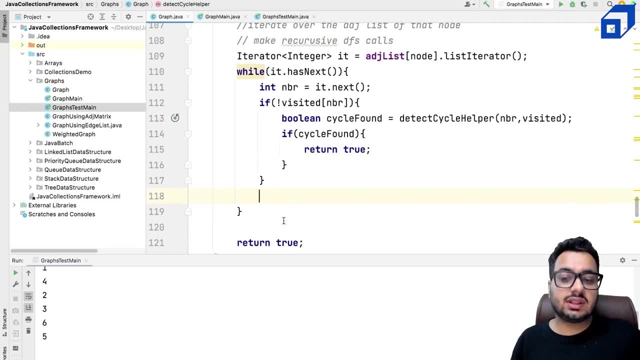 outside this, if right outside this, if so it's, it's like a recursive case. i have written here, so this is like a recursive case. there can also be a base case, right. so base case would be that you are hitting a node which is already visited, right, so i can say else if visited of neighbor, this is true. 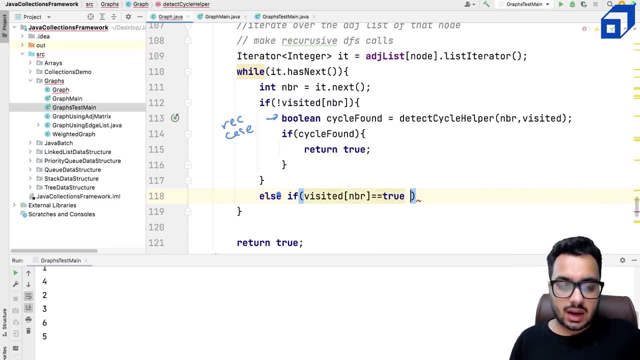 right, this is true, right, and, and there is one more condition, right? so i am basically saying something like this: one is connected with two, two is connected with three, three is connected with four. and now you said, okay, i, i came to this node, i came to this node, i came to this node from four to one. there is an edge. 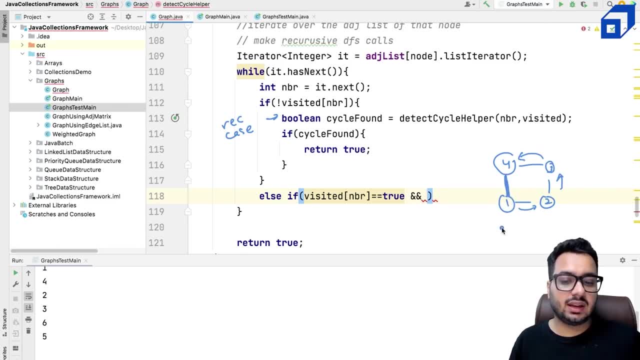 so as soon as you discover this edge, that fine. i am going to a neighbor which is already visited and this one is not the parent of four. okay, so four's neighbor is also three, but three is the parent of four. so you cannot say about cycle at this node. okay, but you can say about cycle because of this edge. 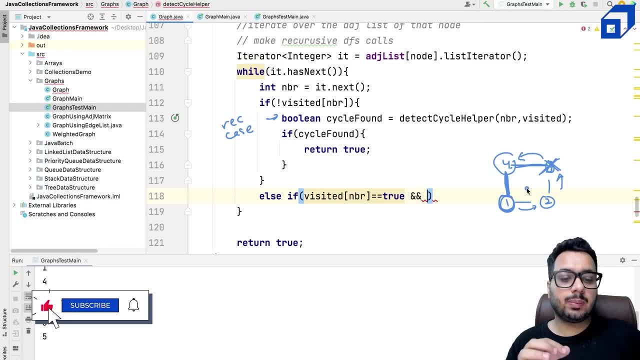 four is taking me to the one, which is the, which is not the parent, right? so you can say: the neighbor that we have discovered is not equal to parent of four. but how do we get parent of four? that is a question. so this is: this is the neighbor, right? so that means: and this is the parent. so we. 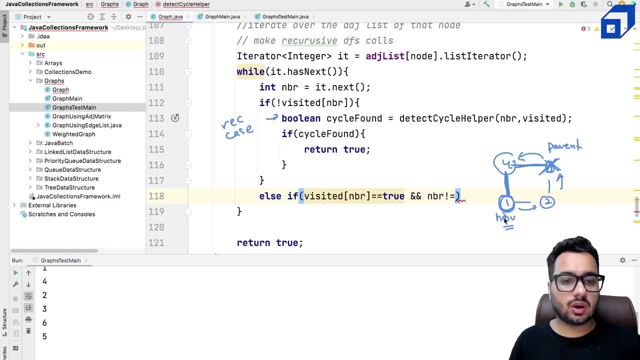 want that this neighbor that we are discovering should not be same as parent, because four's neighbor is also three. right, if it is three, then we cannot say anything. right, we, we have to skip this. but this neighbor, if it is not same as parent, then yes, definitely there is a. 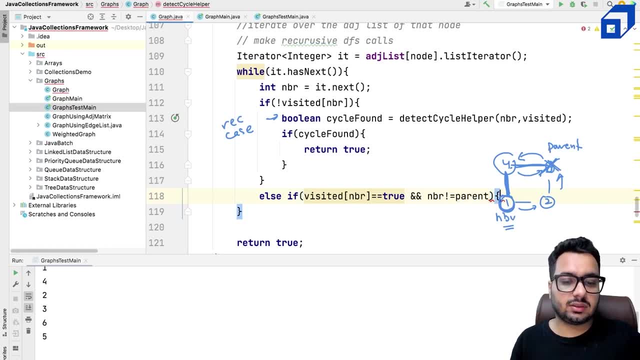 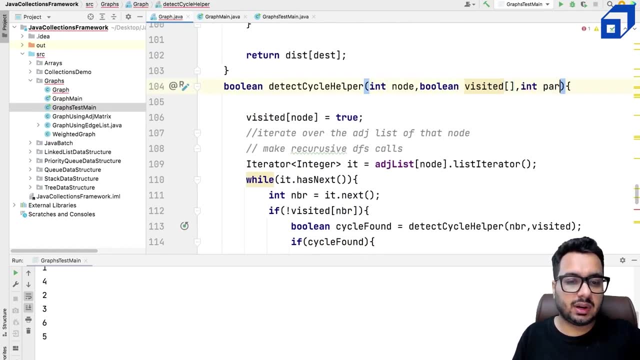 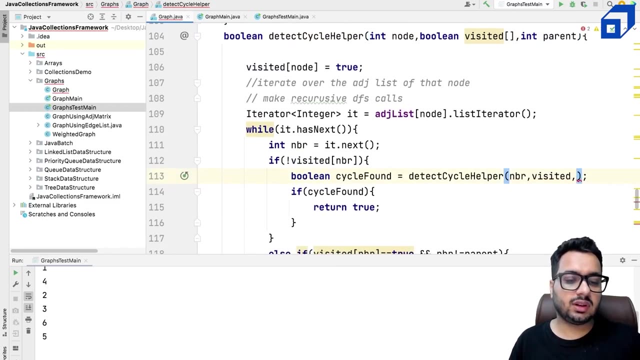 cycle. but how do i find the parent of current node right? so that is a question. this parent we will have to maintain in the function call by passing one more parameter right. so parent, and here we have to. so when you discover this neighbor, right, the parent of this neighbor is going to be the current node right. 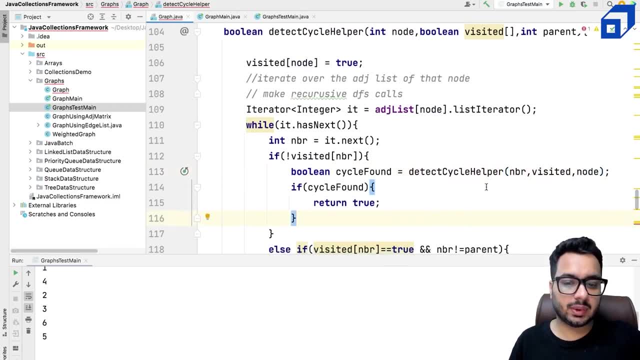 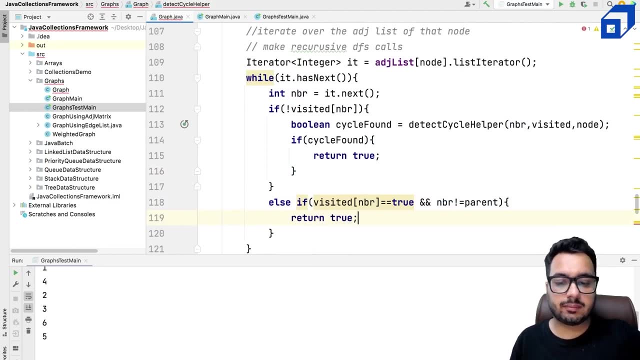 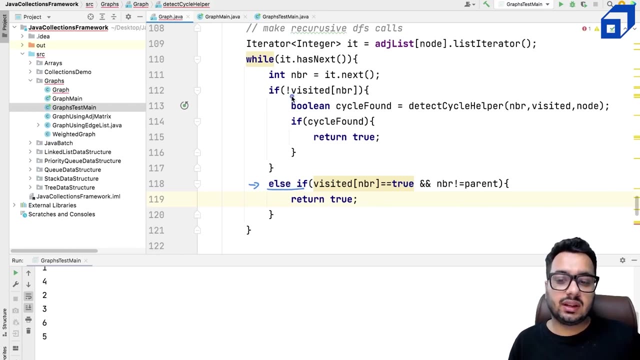 so this will be node, so i'm writing the parent here. if neighbor is not equal to parent, then i can say: return to right, since i'm using the else if condition here. right, this else if will be only executed if the node is already visited, right so? 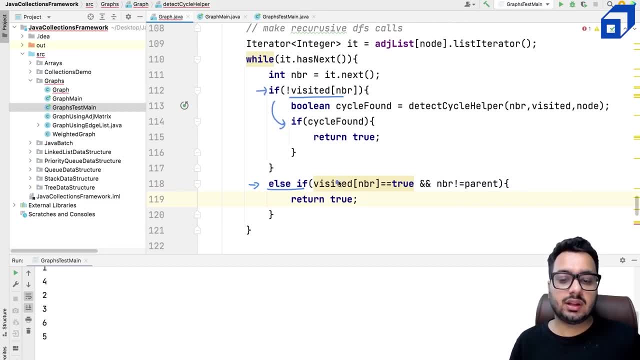 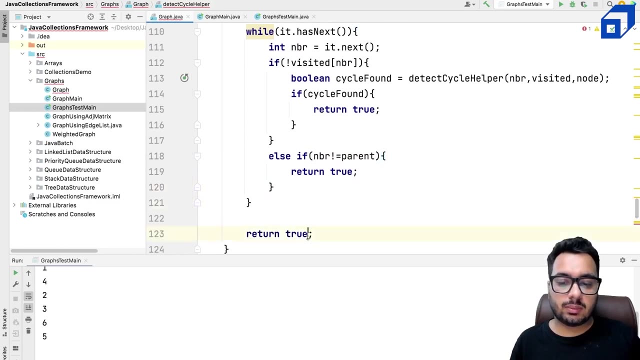 it is not visited, it will go here, but if it is visited, it will come here. that means writing this part is optional, so i can just remove this and i can just simplify. the condition to be only this neighbor is not equal to parent. i'm going to return to, but if i come outside the while loop. 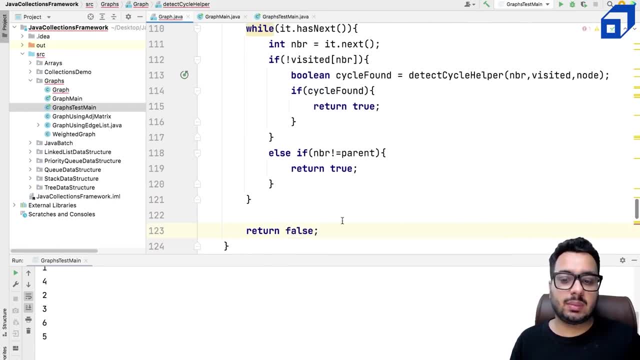 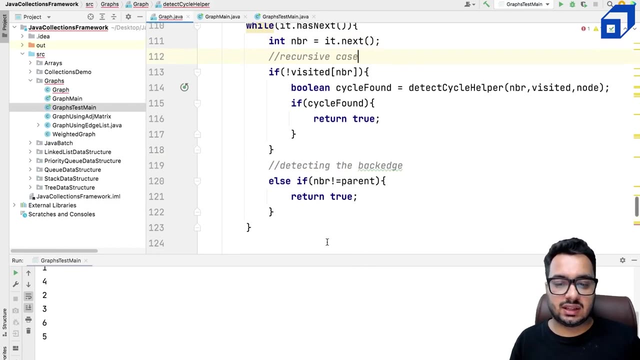 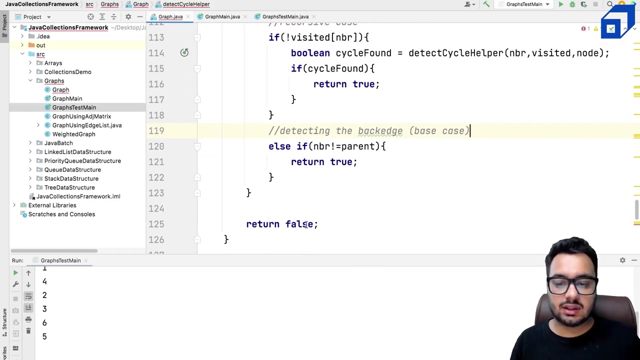 that means i could not detect any back edge right. so this is actually the point where we are detecting the back edge, back edge and this is actually the recursive case. this, if condition is a recursive call, that's it right. this is kind of a base case that we found a back edge right. otherwise, if we could not find 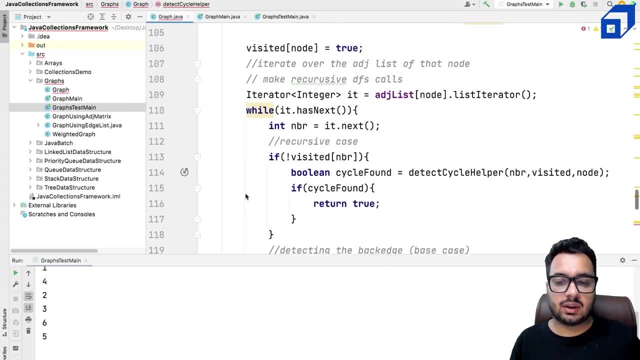 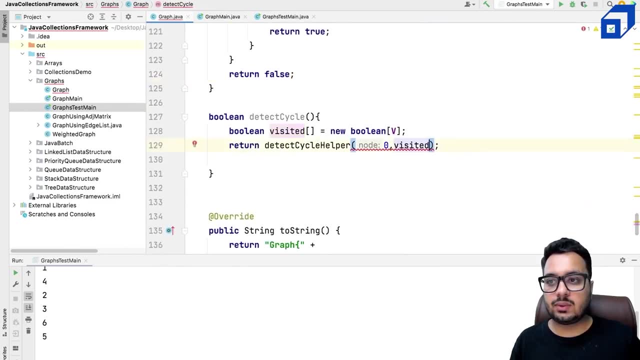 any back edge, we are going to return false from that node. so i think this function looks good to me. now we have to give a parent here as well, so parent of the source node, we can just set it to minus one. no parent right, and let us dry run this code and let us also test. 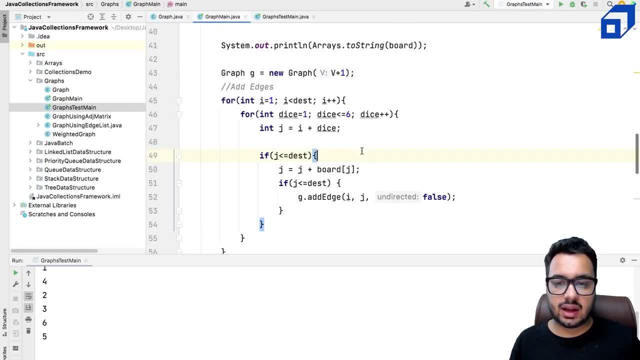 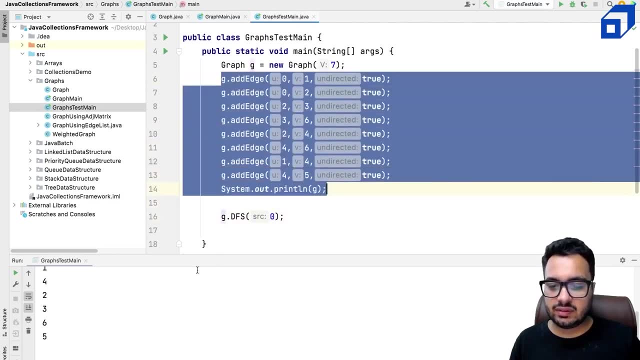 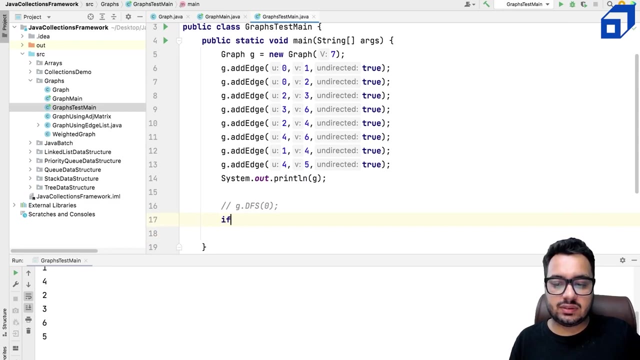 the functionality first. so here in the main, I have this file, so I have created a graph. I have done the DFS, simple DFS works. but now I want to s out about the cycle detection. so if G dot detect cycle, you can just see out s out: yes, there is a cycle, else you can. 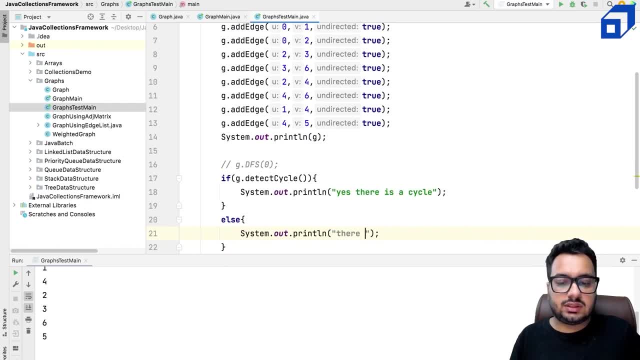 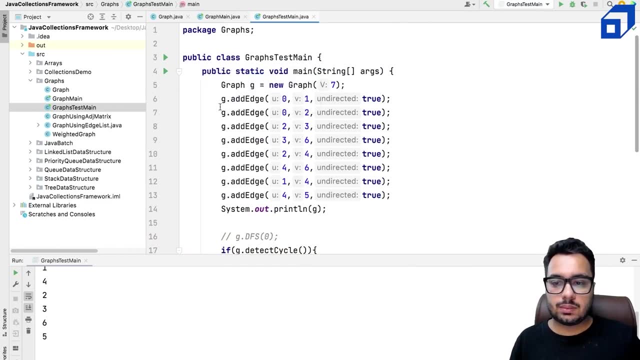 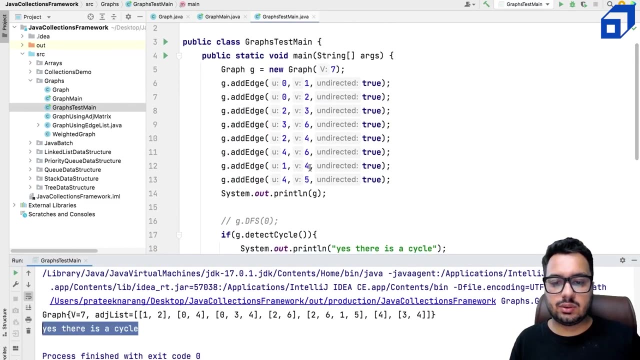 say: s out, there is no cycle. let's go and run this code. so let's see what output do we get? so it says, yes, there is a cycle. I'll show you. this is the same graph that we have in the figure. so yes, it contains a cycle. 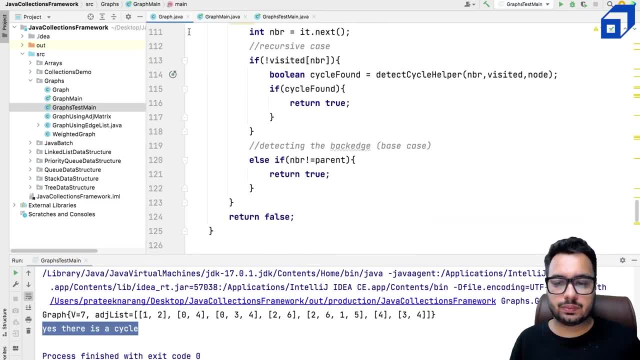 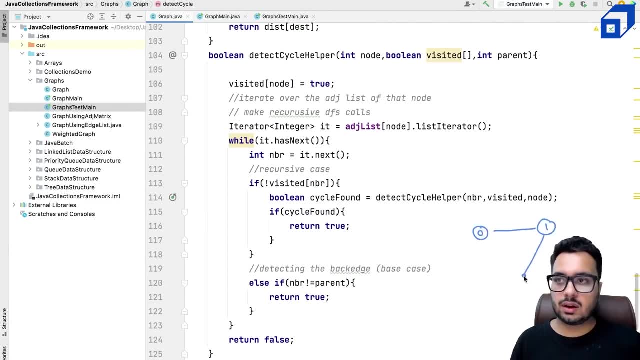 so let me dry run this code for you once again. I'll do it on a smaller graph. let's say the graph looks like this: zero, one, two, three, four. and let's say: this is the edge, right? so you start from zero. so parent is minus one. so you look at neighbors of zero, right? so you said okay. 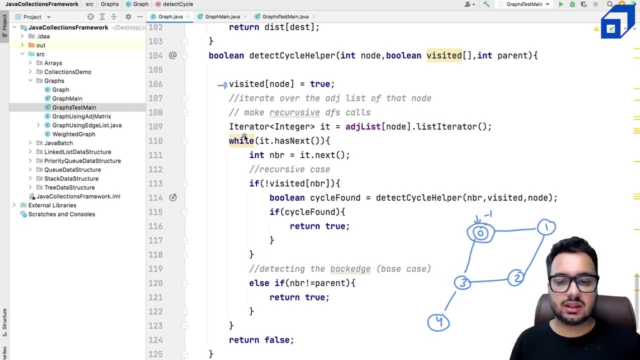 visited of node, this is true. so this is marked as visited. then you iterate over the neighbors. so neighbors of zero are one, two or one and three. first we will go to one. one is not visited, so we may make a recursive call and ask: did you find a cycle? so one is now marked as visited. 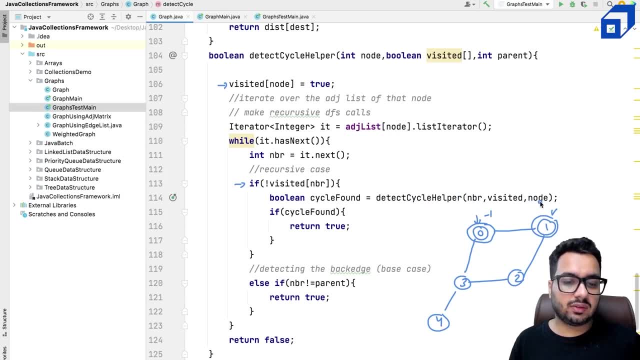 and when I marked one, so I said the parent of one as the node. so this was the node, this was the neighbor. so neighbor's parent is going to be the node. the parent is zero. so once parent is marked as zero, and again same story repeats at one, what do I do? I make a recursive call. so I 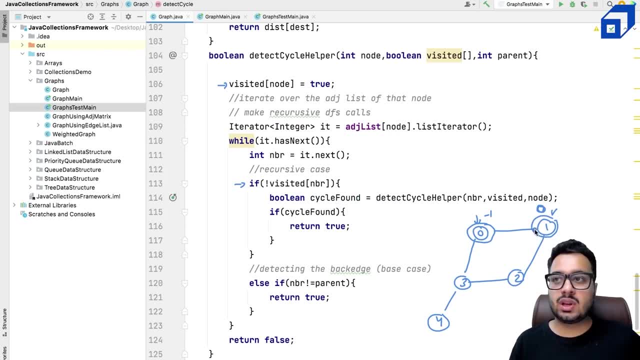 ask: neighbor of one. right now one has two neighbors. one of the neighbor is zero. zero is visited. but what happens here? is this condition true? what is the neighbor? neighbor of one is zero. what is parent of one? that is also zero. so we do not execute this as if block, so we basically ignore this case, okay. 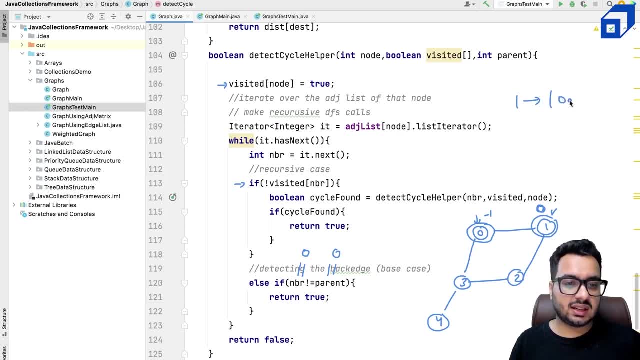 any work here. then we look at the second neighbor. so one has neighbors that are zero and two right, so nothing happens here. what about two? so two is not visited, so we make a recursive call. right, so we go to this node. we make a recursive call. now. two is marked as visited. parent of two is one. 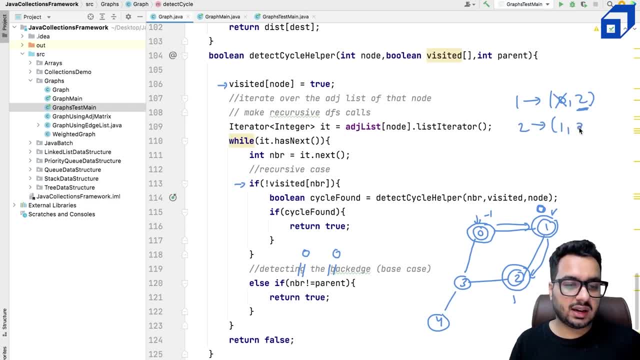 now two also has two neighbors. two has a neighbor that is one and it has a neighbor three. so I do not. if I look at one, one is already visited, right. so I come into this as if, okay, if it is not visited, I go here. so it is visited, I come here. so what is the neighbor of two that is one? what is parent of two? 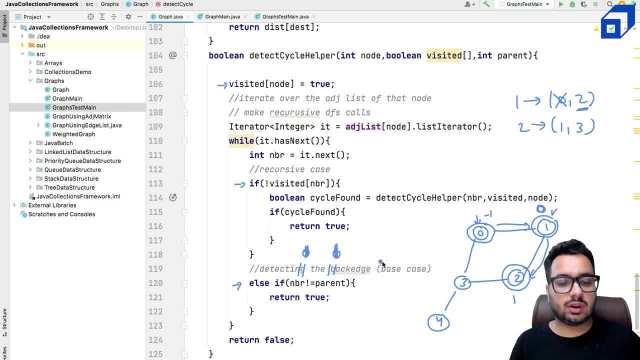 that is also one. so this condition is also not true. so I do not do anything here, so nothing happens. here. we talk about this edge two to three, so I go to three. now, at three, what happens? three has two neighbors, zero and four, so I go to zero. is zero visited? yes, zero is visited, so I do not go into. 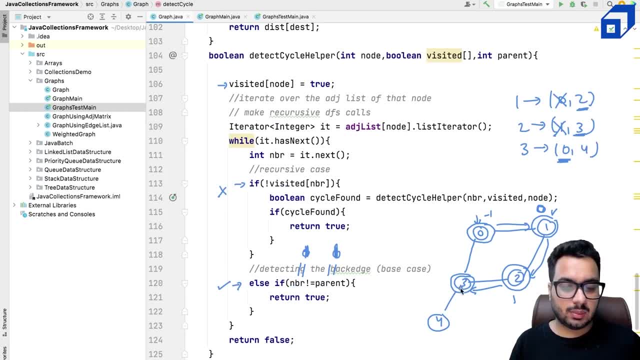 what is the neighbor, right? so what is now the neighbor of three? so the neighbor of three that I'm considering here is because of this edge, that is zero. what is the parent of three? the parent of three is actually two, right? so they are not equal. yes, zero and two, they are not equal, that means yes. 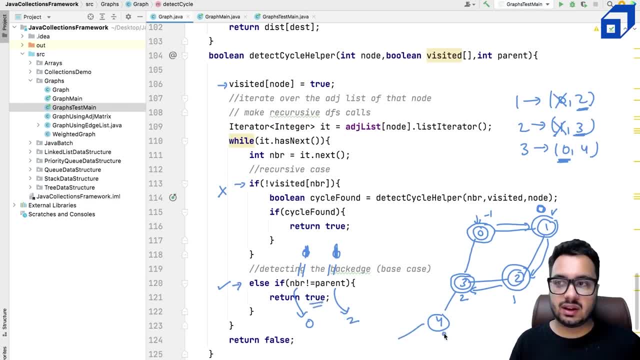 return true. so without looking at this part of the graph, three returns are true right now. two got to know yes, there is a cycle found. so two also returns are true. it goes back. one also gets to know: yes, there is a cycle found. so as soon as it gets a true it. 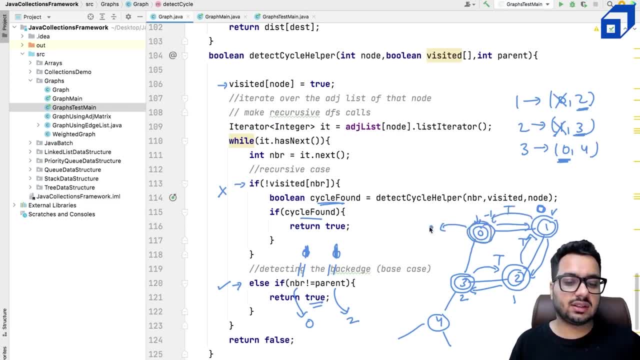 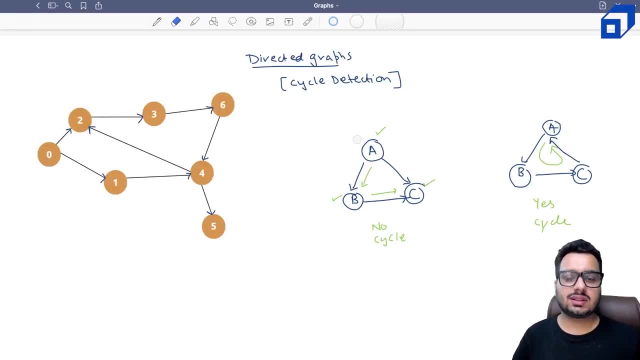 returns a true zero, gets to know: yes, there is a cycle. it returns a true back to the main. so this is how this algorithm is working and I hope you understood it. now we will talk about cycle detection in case of directed graph. so in case of directed graphs, not just the structure of the 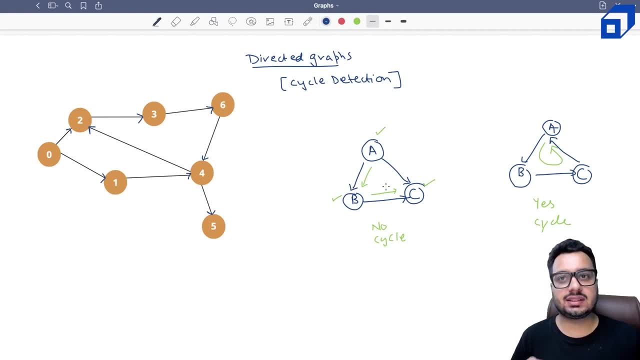 graph, but the direction of edges also decide whether there is a cycle or not. if you look at this example, the edges are like this: and if you start from A, you can go to B, you can go to C, but from C you are not able to go to A right. 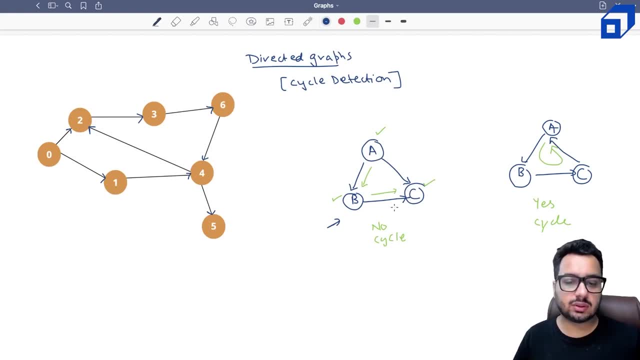 and of course there is no loop present here, right, so hence there is no cycle. but if I change the direction of the just this edge, I reverse it, right, I can go from A to B, B to C and from C I can again go back to a node. I can go in a cycle. so hence, yes, there is a cycle. right now. I will tell you if you. 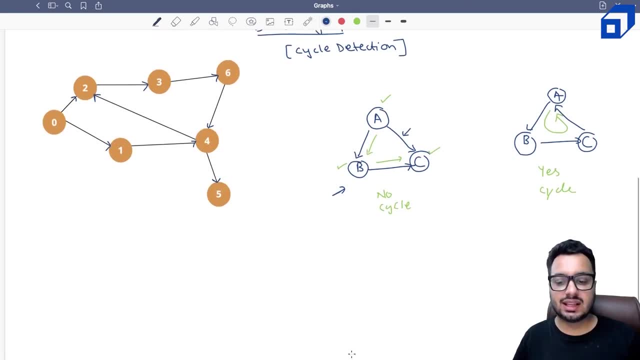 have a problem you are going to face, right, it's not going to work in the same manner. so let me take up one more example. let's say the graph is like this: let's say A, from here we have B. let's say C, D, E, F, and let's say this is connected, like this. and let's say I have G, and it is connected. 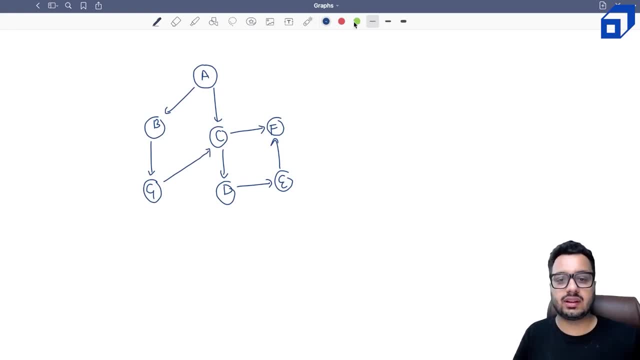 with. let's see right. so suppose you start doing DFS from A and you say, if I hit a node which is already visited, I will say there is a cycle. this, this is the logic we did in the undirected graph. so let's say you started doing DFS, you started from A. you went to C, okay, from C you went to D, from D you went to E. from E. 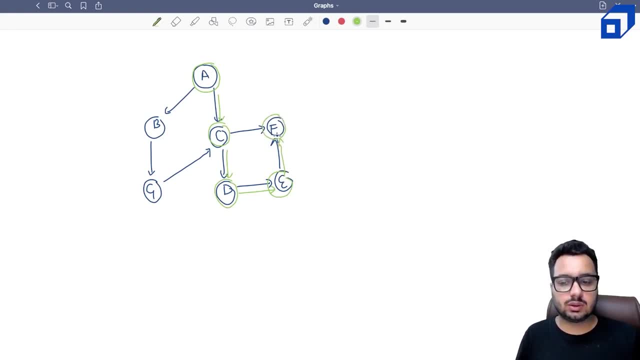 you went to F and from F you cannot go anywhere else. so you come back and you say: okay, no, there is no cycle. so you're, you come back, you return false right, and from E again you come back B, you again come back at C, and again you come back at A, and from A you come. 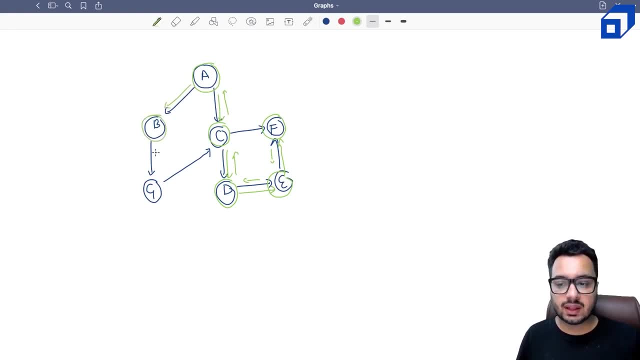 back at B. now you go to V. B is not visited. right from B you go to G, and from G you go to C. and now you see that I am going to a node that is already visited. this edge right and it is C. C is not the. 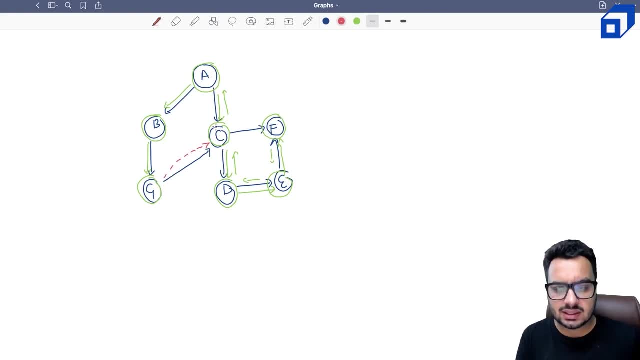 parent of G. that means I am going back in the path, but is it really a cycle? my question to you is: is it really a cycle? the answer is no. if you start traveling from A, you can come to C and you cannot get stuck into cycle. from C you can go to E, right, so this is not a cycle. or you can go to D, right. 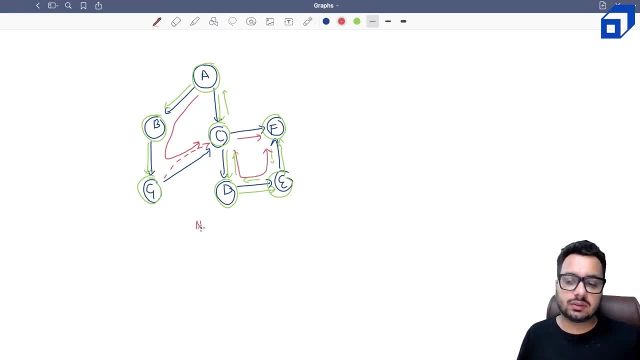 then go this way. so this is again a case of non-cyclic graph, right. but if you run the previous algorithm that we executed on a directed graph, it is going to say, yes, there is a cycle, because from C you discovered a node which is already visited, right. hence we need to fix this algorithm, right. 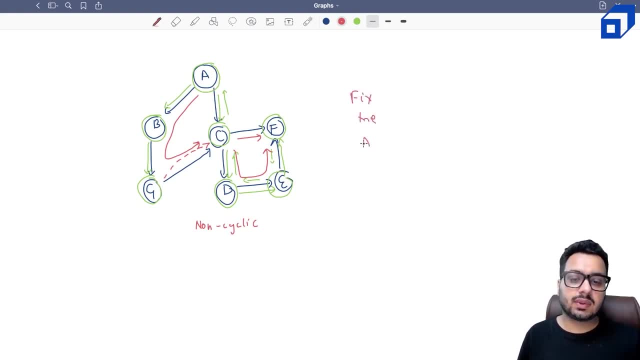 so we need to fix the algorithm for directed graph for directed. other question is: how do we fix it? the thing is, we need to again detect back edges correctly, right? so from G to C, this is not a back edge, right? I will tell you what is a back edge in. 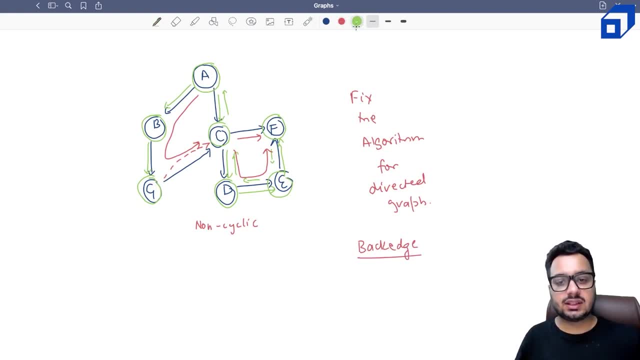 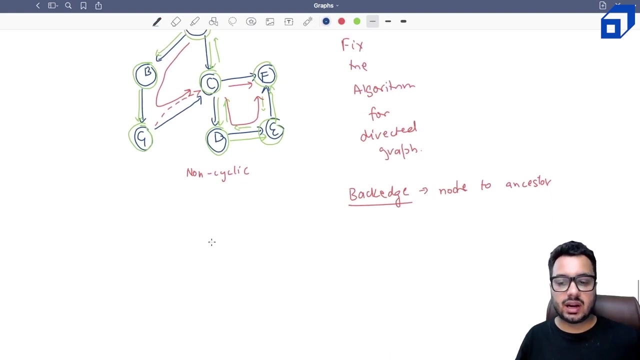 of a directed graph. the back edge is a edge that takes you back to, from one of the node to some of, to some ancestor node in the same path right from the current node to some ancestor right. so let us take, take another example inspired from this graph only. let's say: I have a, I have C. 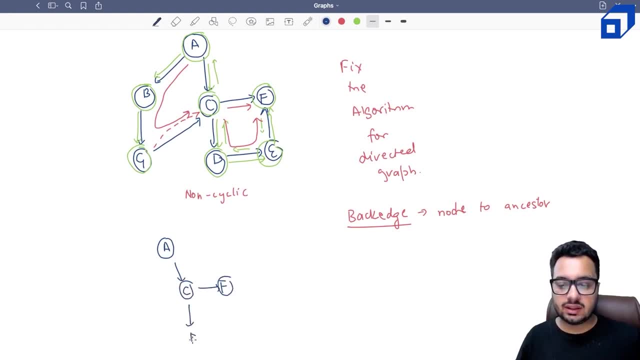 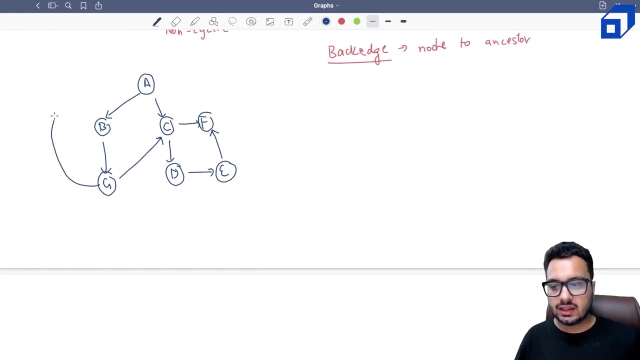 I have F, I have D and I have E and I have F, then I have, let's say, B, then I have, let's say, G, and then I'm pointing to, let's say, C, and let me add one more edge in this graph. so this graph, this edge maybe looks like this. let's say, the edge is like this: do: 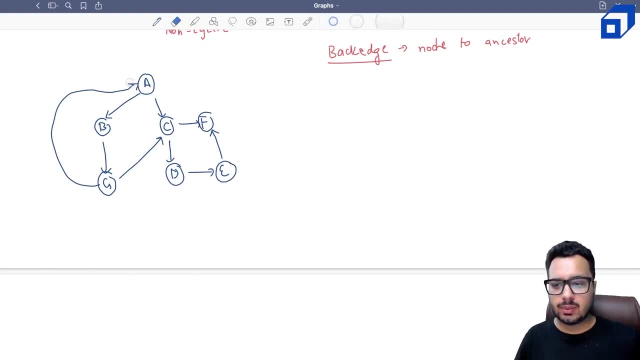 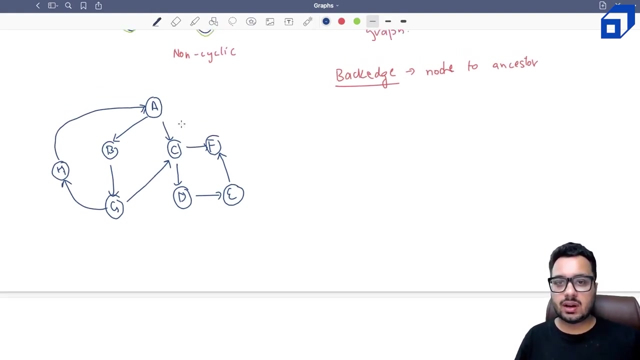 you see a cycle here. the answer is yes, there is a cycle, right? or add two more nodes, right. let me add a node. let's say h and let me add a node. that's it. let's say one more node i have added. now, in this part of the graph there is no cycle, but yes, in this part, 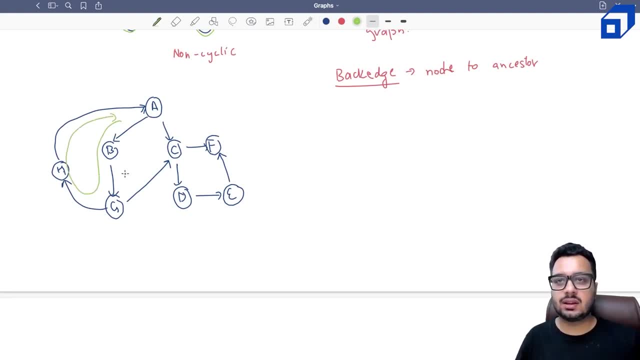 of the graph. there is a cycle, because you can revolve in this path again and again, right? so let us try to see what is a back edge in this scenario. right, let's say we started doing dfs. from a, i went to c, from c, i went to d, i went to e. from e, i went to f. from f, i cannot go anywhere. 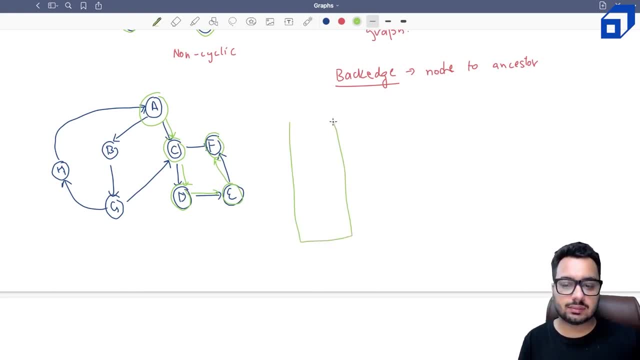 so i will just come back. right, what is the state of the call stack? the call stack has a, it has c, it has d, it has e, it has f. f says i cannot go anywhere, so i'm just going to return false. so false is propagated back. then e says: okay, i cannot go anywhere, else i will come back. 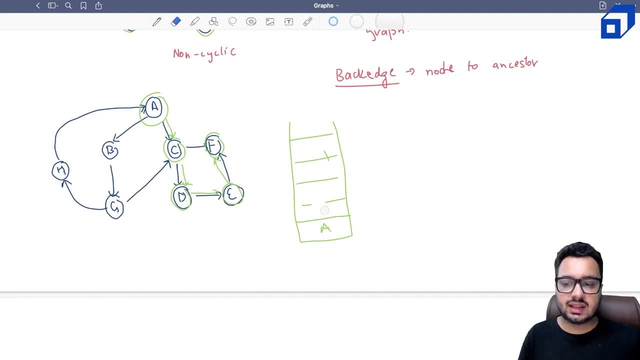 you. he says i cannot go anywhere else, i'll come back. he says i cannot go anywhere else, i come back to a now. a says, okay, let us go to b. b goes into the stack. b says let's go to g. g goes into the stack. now from g, i can go to c. c is already visited, but is it a back edge? the answer is still no right. 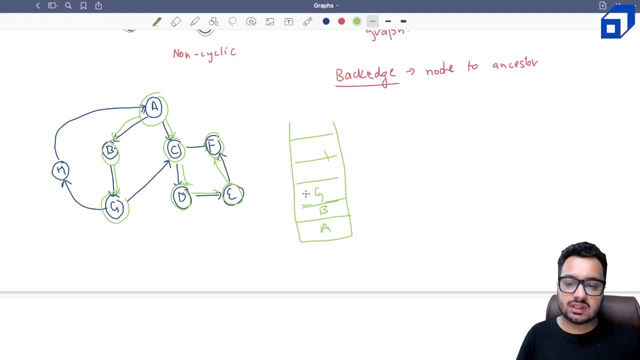 because in the current path, right. so if g is giving giving me a edge that is pointing back to one of the ancestor in this false stack, only then it will form a cycle, right? so the answer still here is no, so i will not take this edge. so can i go anywhere else? okay? so basically, what is? 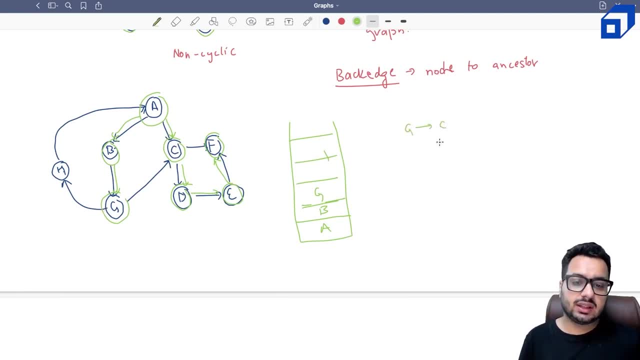 the condition i'm going to check here. so when i'm checking g to c, c is visited, c is visited, but c is not in the stack. c is not in the stack. that means i came to g- g via path which does not include c. okay, it is not in the stack. that is important condition right? 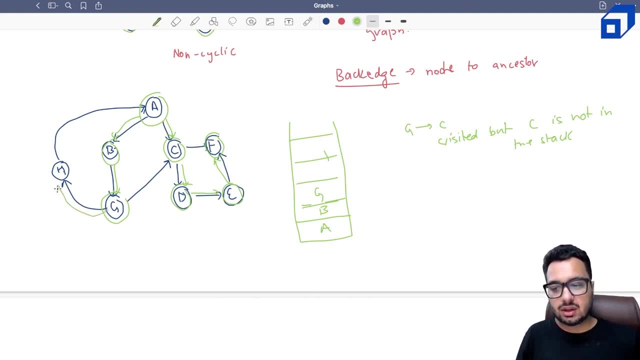 now g can say: okay, let me go to h, h is not visited, fine, h goes into the stack. now h says i can go to a. so what is what happens here? we are going to a node that is visited and that is also in the current path. right, that means from h i can go to a from a, if you. 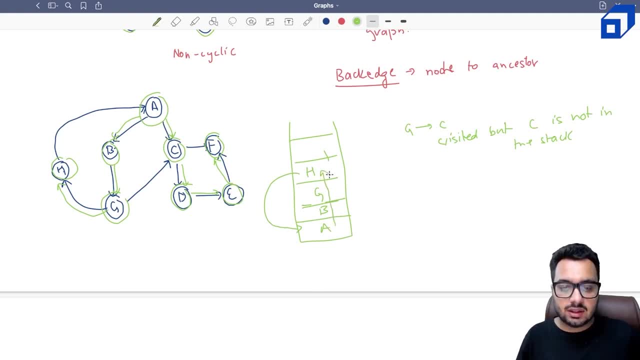 a. again. you can go to h, a, b, g, h. that means these nodes will form a cycle: a, b, g, h. right, what is the condition to detect a back edge? so i will say, okay, in this dfs, reversal this edge from h to a, this is forming a back edge. right, because i'm going back to one of the ancestor.